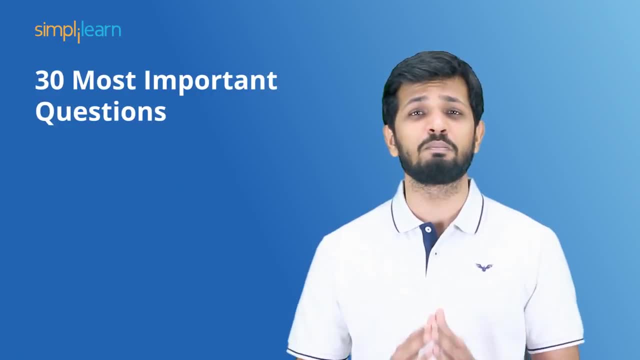 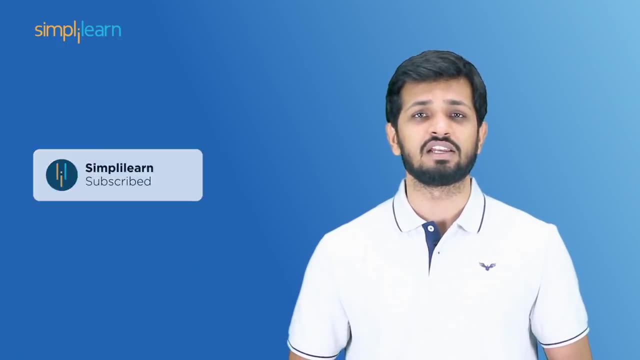 field. Finally, we have selected 30 of the most important questions you need to know to crack a data science interview. Before we begin, make sure to subscribe to our channel and click on the bell icon to never miss an update from Simply Learn With that out of. 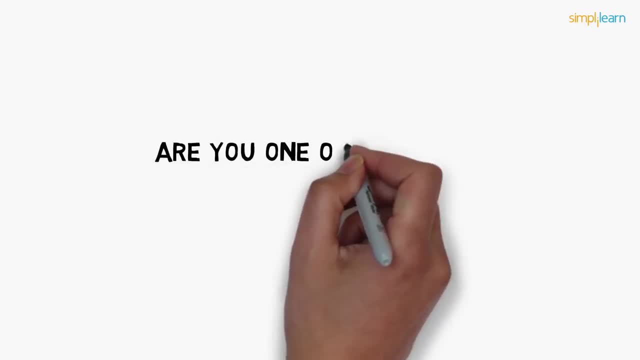 the way, let us have a look at our animated video. Are you one of the many data scientists who are performing well in the data science and data science industry? Do you want to many who dreams of becoming a data scientist keep watching this video? if? 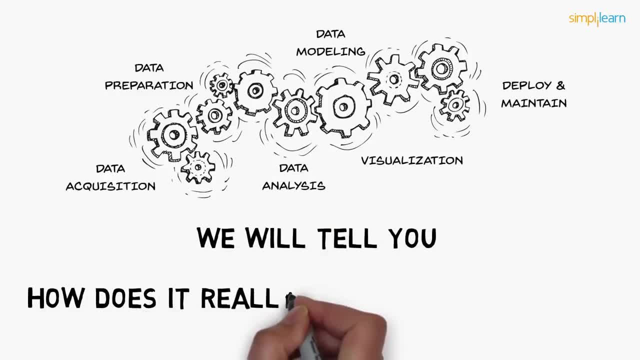 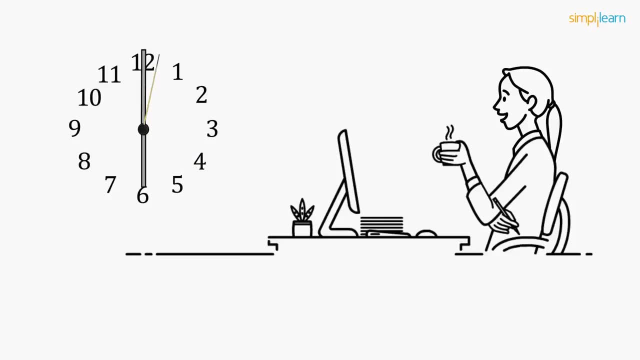 you're passionate about data science, because we will tell you how does it really work. under the hood, Emma is a data scientist. let's see how a day in a life goes while she's working on data science project. well, it is very important to understand the business problem first. in our meeting with the 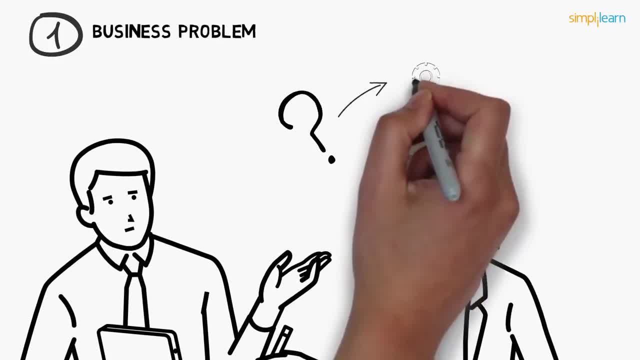 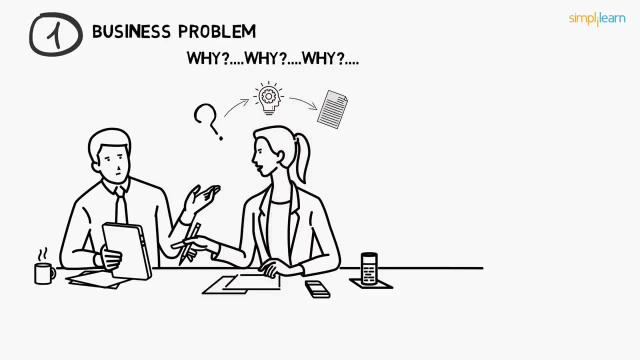 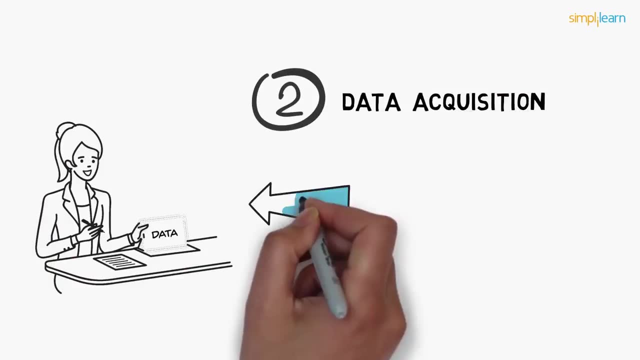 clients. Emma asks relevant questions, understands and defines objectives for the problem that needs to be tackled. she's a curious soul who asks a lot of eyes- one of the many traits of a good data scientist. now she cares up for data acquisition to gather and scrape data from multiple sources like web servers. 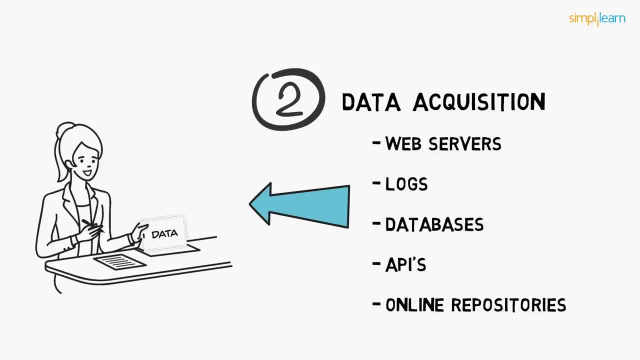 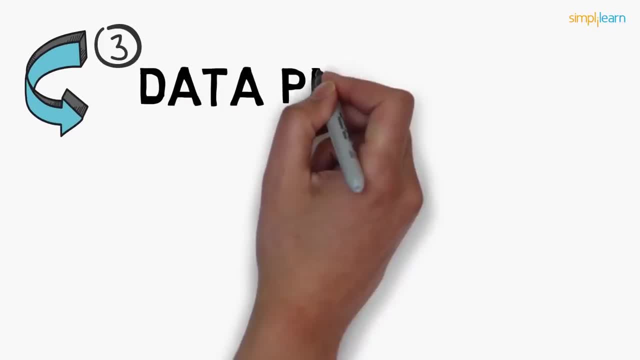 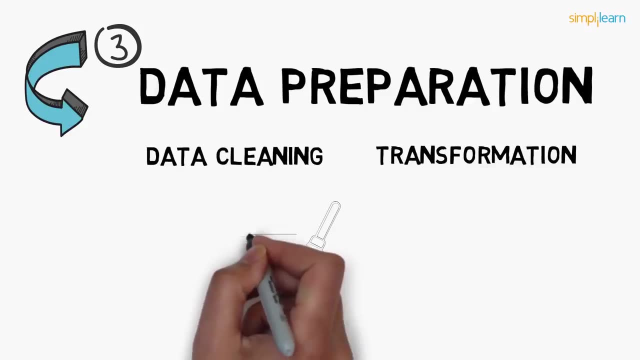 logs, databases, api's and online repositories. oh, it seems like finding the right data takes both time and effort. after the data is gathered comes data preparation. this step involves data cleaning and data transformation. you data cleaning is the most time-consuming process, as it involves handling many complex scenarios. here, Emma deals with inconsistent data types. 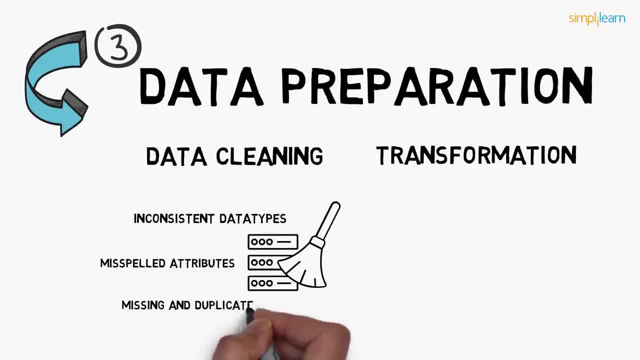 misspelled attributes, missing values, duplicate values and whatnot. then in data transformation she modifies the data based on defined mapping rules. in a project, ETL tools like talent and informatica are used to perform complex transformations. that helps the team to understand the data structure better. 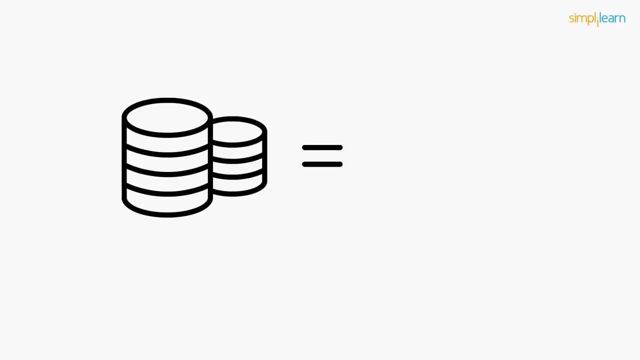 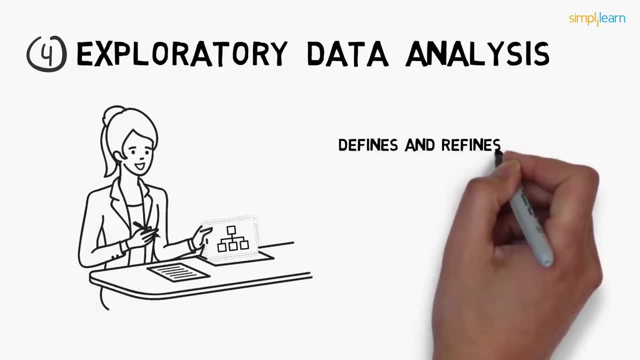 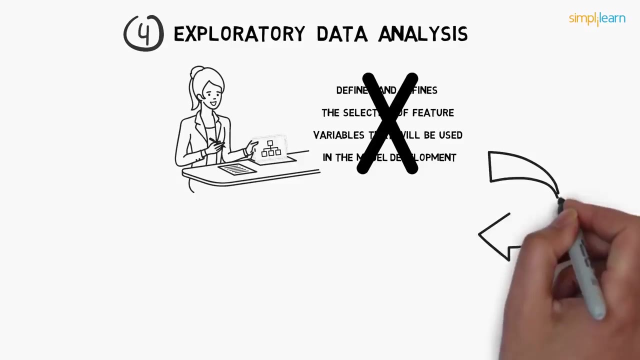 then understanding what you actually can do with your data is very crucial. for that, Emma does exploratory data analysis. with the help of EDA, she defines and defines the selection of feature variables that will be used in the model development. but what if Emma skips this step? she might end up choosing the wrong variables, which will 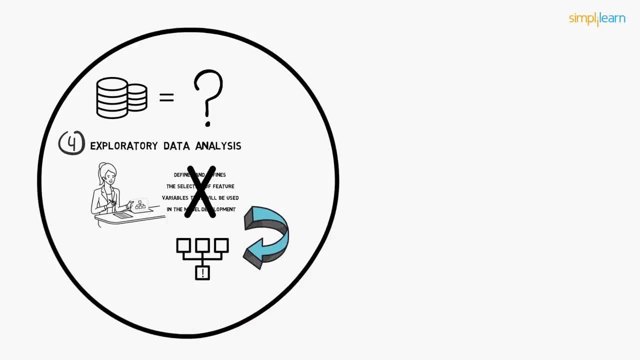 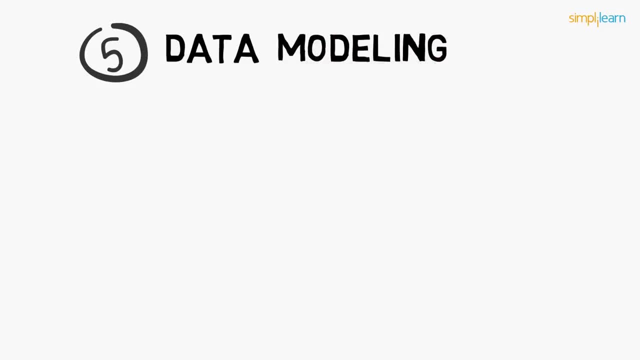 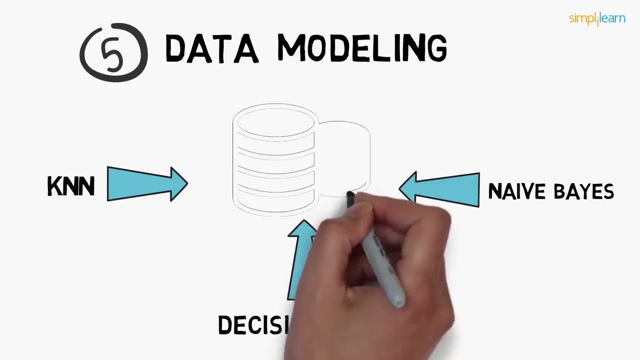 produce an inaccurate model. thus exploratory data analysis becomes the most important step. now she proceeds to the core activity of a data science project, which is data modeling. she repetitively applies diverse machine learning techniques, like KNN decision tree knife base, to the data to identify the model that best fits the business requirement. 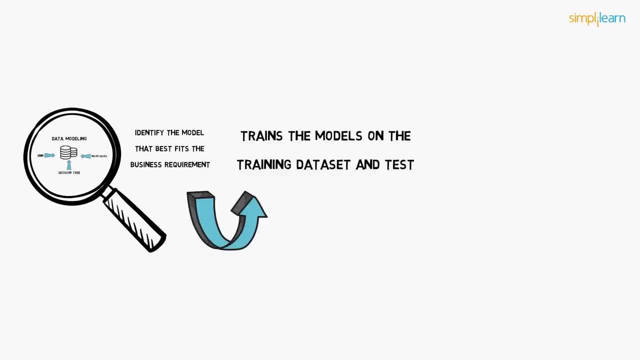 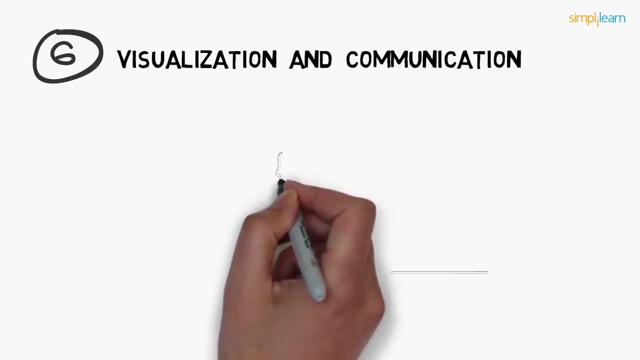 she trains the models on the training data set and tests them to select the best performing model. Emma prefers Python for modeling the data. however, it can also be done using R and SAS. well, the trickiest part is not yet over: visualization and communication. Emma meets the clients again to communicate to the 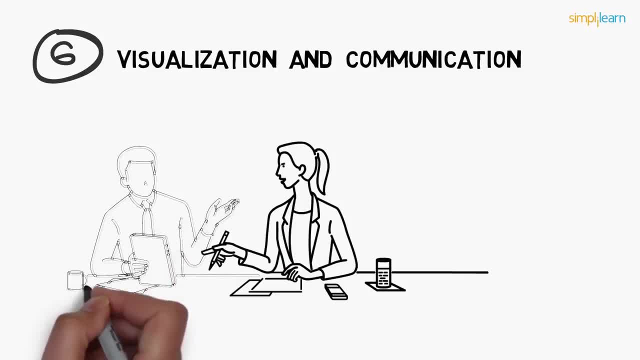 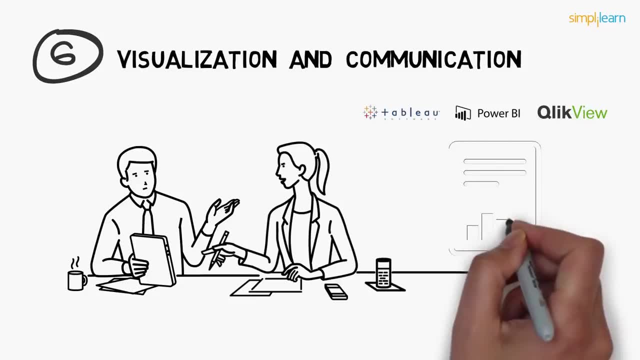 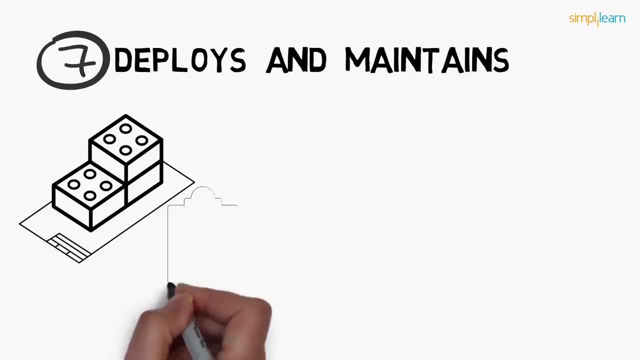 business findings in a simple and effective manner to convince the stakeholders. she uses tools like tableau power, bi and click view that can help her in creating powerful reports and dashboards. and then, finally, she deploys and maintains the model. she tests the selected model in a pre-production. 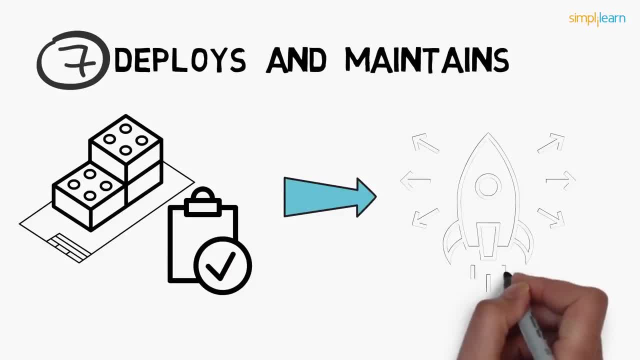 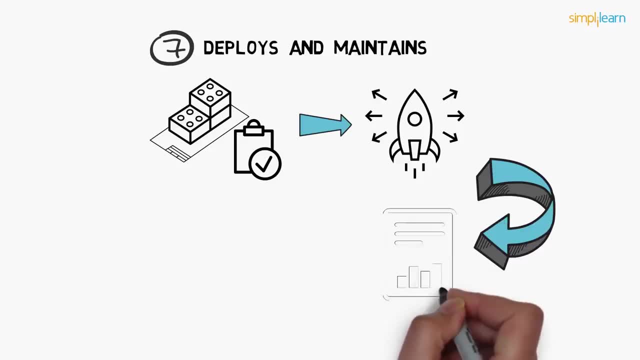 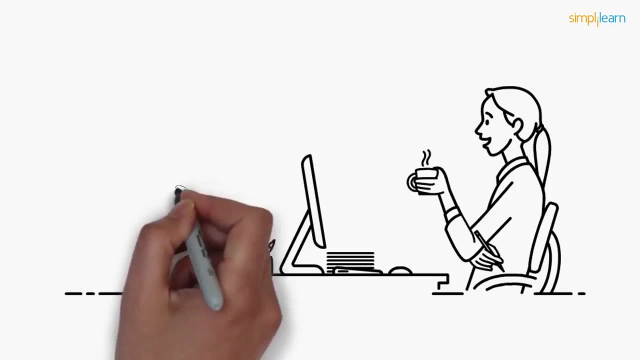 environment before deploying it in the production environment, which is the best practice. right after successfully deploying it, she uses reports and dashboards to get real-time analytics. further, she also monitors and maintains the project's performance. well, that's how Emma completes the data science project. we have seen the daily routine of a data. 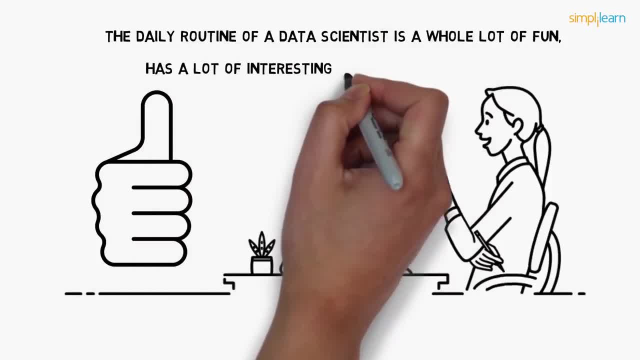 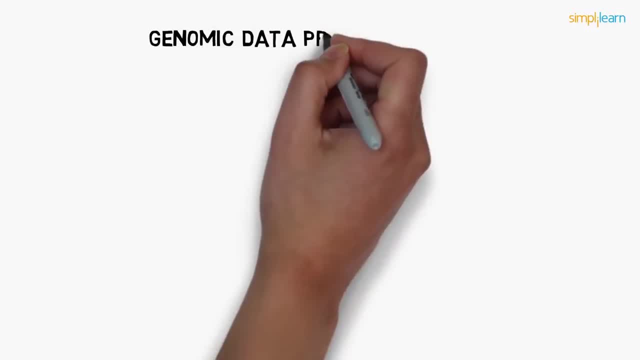 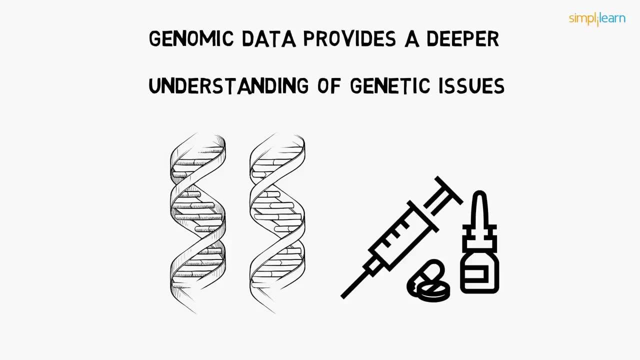 scientist is a whole lot of fun, has a lot of interesting aspects and comes with its own share of challenges. now let's see how data science is changing the world. data science techniques, along with genomic data, provides a deeper understanding of genetic issues in reaction to particular drugs and diseases. logistic companies like DHL. 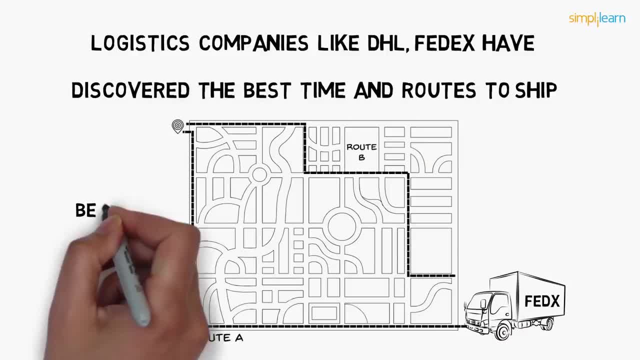 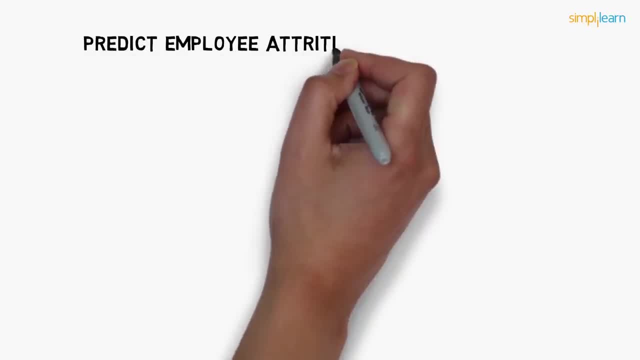 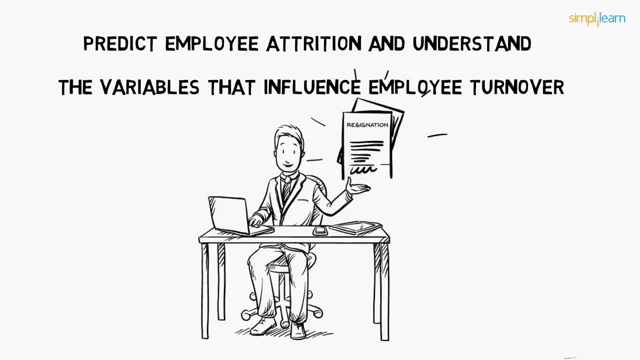 fedex have discovered the best rules to ship, the best suited time to deliver, the best mode of transport to choose, thus leading to cost efficiency. with data science, it is possible to not only predict employee attrition, but to also understand the key variables that influence employ turnover. also, the 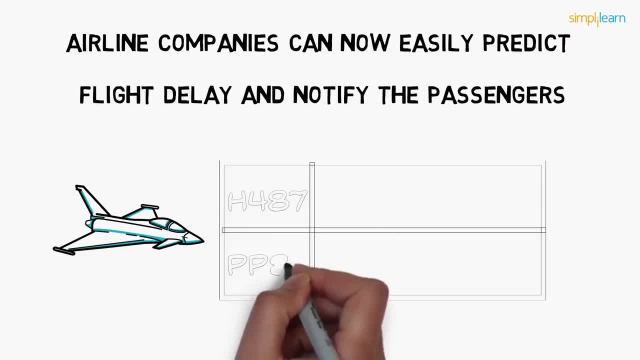 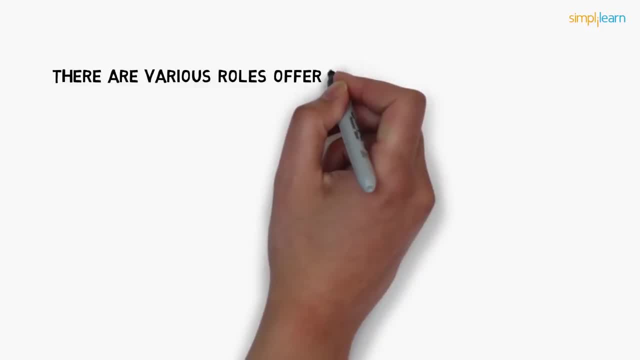 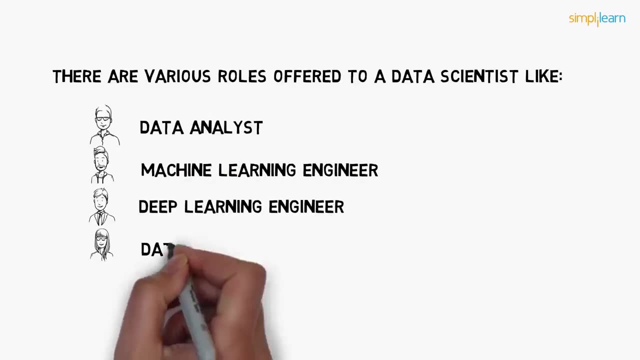 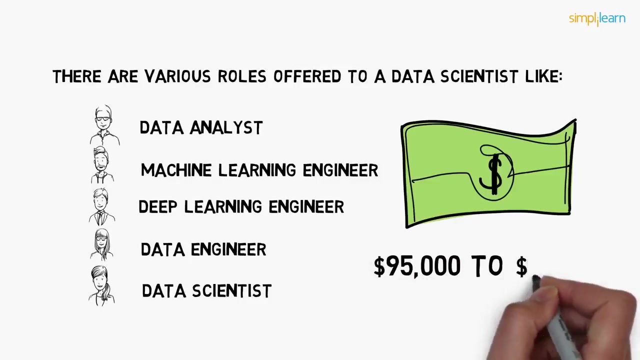 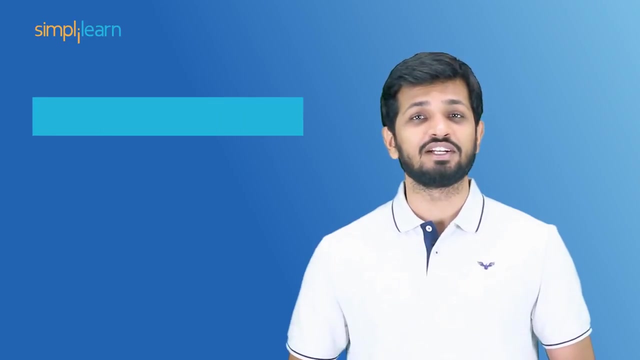 airline companies can now easily predict flight delay and notify the passengers beforehand to enhance their travel experience. well, if you're wondering, the various rules that can be employed by a smart responsibility will unique for each delivery and mobility efficiencies alone. I hope that has got you excited to learn data science. We now have Richard, Mohan and Pete. 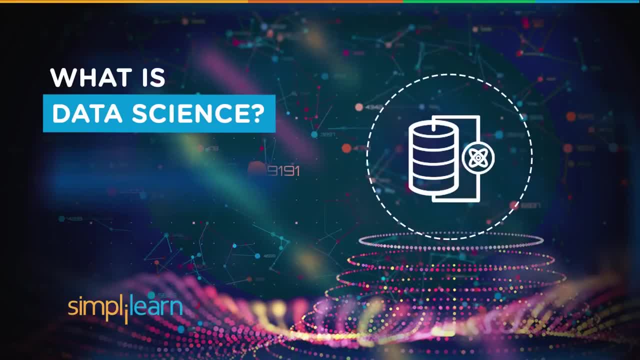 who will explain the various concepts of data science. Hello and welcome to this session on data science. My name is Mohan and today we are going to take a look at what this buzz is all about. So what is the agenda for today? We will talk about what is. 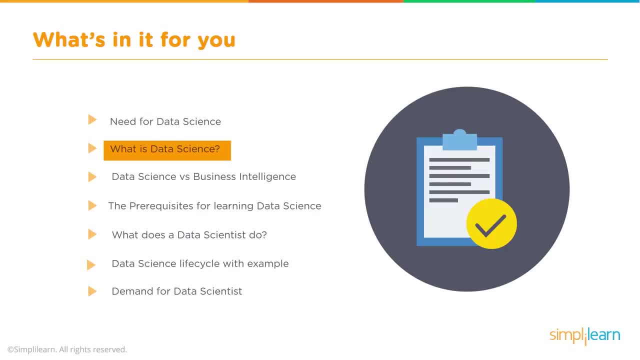 the need for data science. and then, what exactly is data science? some definitions and also understand the differences between data science and business intelligence. Then we'll talk about the prerequisites for learning data science. and then, what does a data scientist do? What are the activities performed by a data scientist as a part of his daily life? And then we will talk. 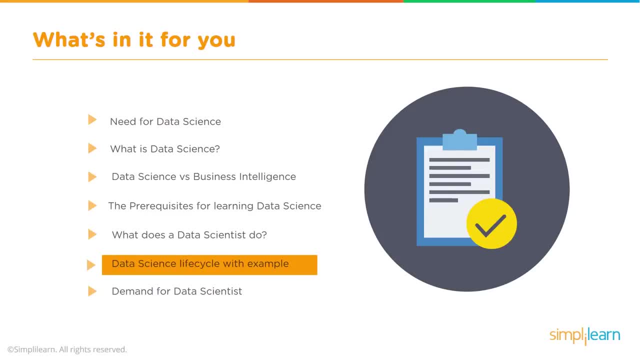 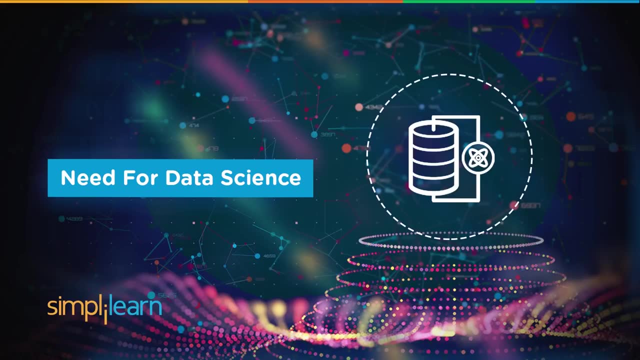 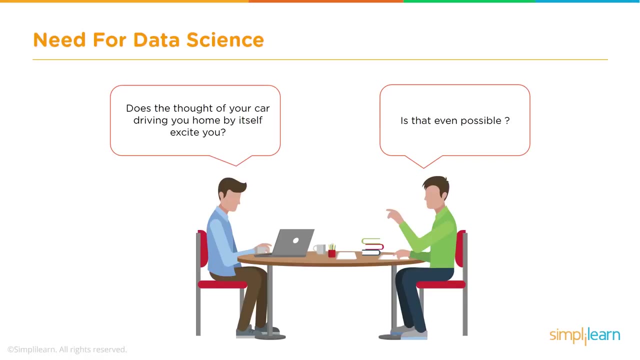 about the data science life cycle with a quick example and briefly touch upon the demand, or ever increasing demand, for data scientists. All right, so let's get started Now. you must have already heard about autonomous cars, So I'm sure you must be excited to have a car driving by itself. 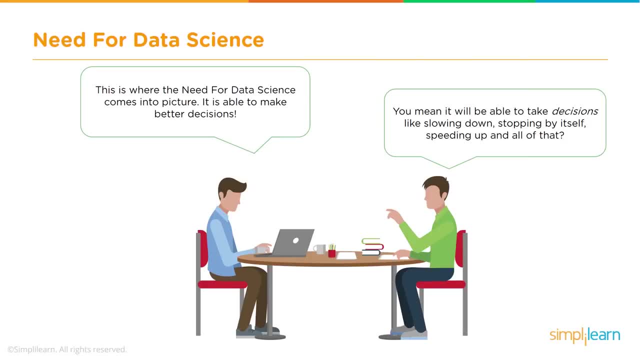 home to office or office to home right, And that's where one of the examples where data science is used. Now the car needs to take a lot of decisions in this whole process: whether to speed up, whether to apply the brake, take a left turn, right turn or slow down. So all these decisions. 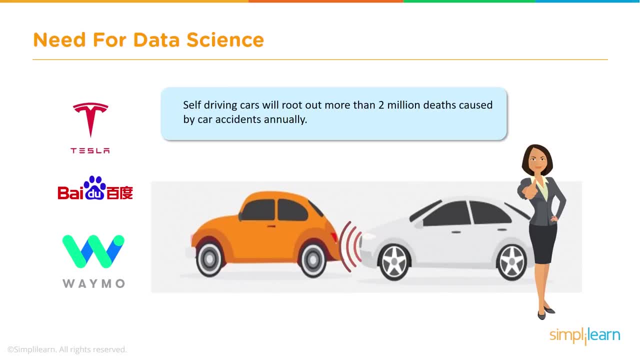 are basically a part of data science, And there is a study that says that self-driving cars will minimize accidents and accidents. So if you have a car driving by itself, you must have a car driving by itself. In fact, it will root out more than 2 million deaths caused by car accidents annually. 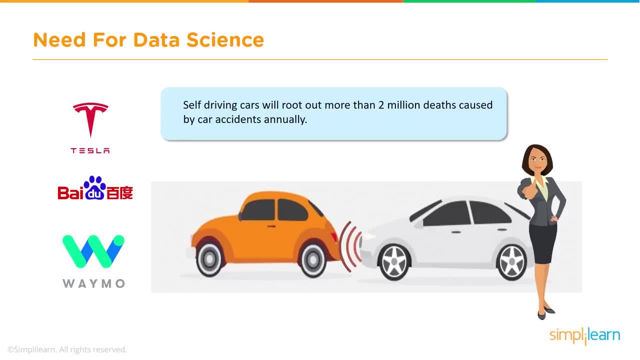 Self-driving cars. right now. there's a lot of research and there is a lot of testing going on. Not a lot of cars are yet in production in terms of usage, but it's going to happen. Every automotive company worth its name is investing in self-driving cars, So in about 10 to 15 years, some of the 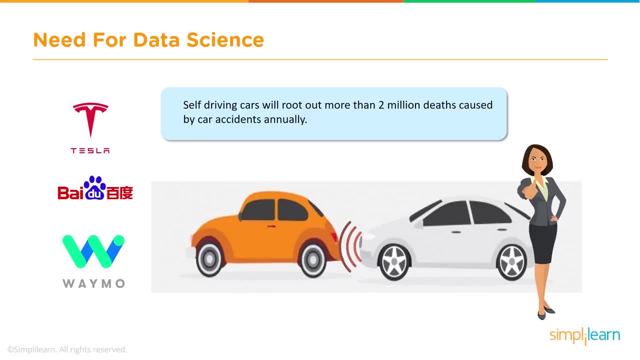 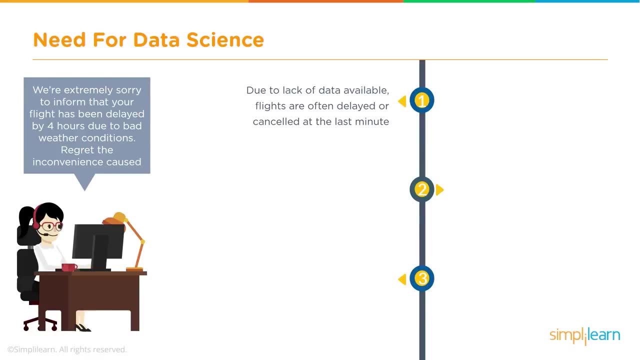 companies say that most of the cars will be autonomous or self-driving cars. Where else there are issues? For example, if we take airlines, this is another area where data science contributes in a major way. Flights get delayed due to weather conditions, because the weather is not predicted. 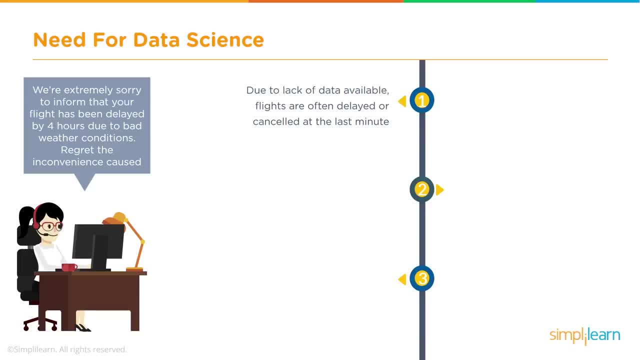 in time and the demand of passengers is not probably seen ahead of time. For all these you need data science. Then this could be improper route planning and some customers might miss some flights. That again needs data science And similarly it could be incorrect decisions in selecting the 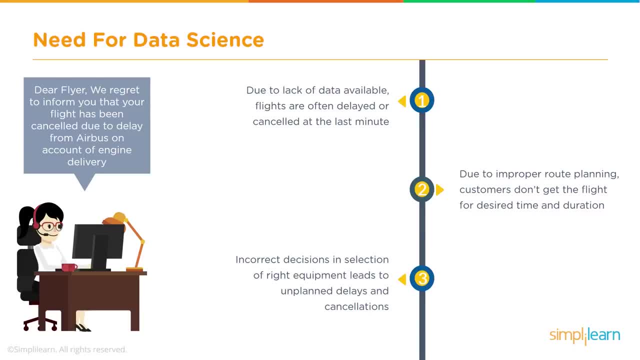 right equipment, So which plane should fly in which route. That's the equipment that's being mentioned here. If that is not planned properly, then you might end up in a situation where the plane is not available, whereas you have planned for a flight in a particular route. 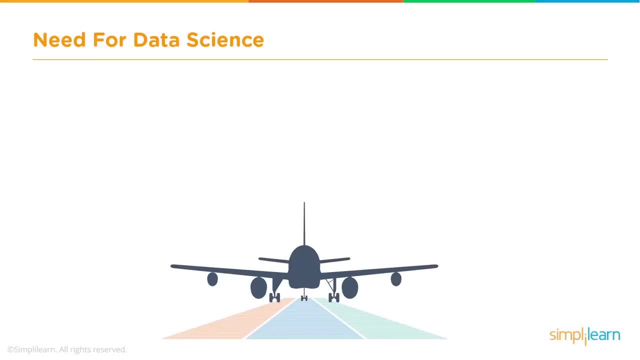 So these are some of the challenges in one of the representative industries we are talking about, which is airlines. So if we use data science properly, all of these, or most of these- problems can be avoided, and that will help in reducing the pain both for the airlines. 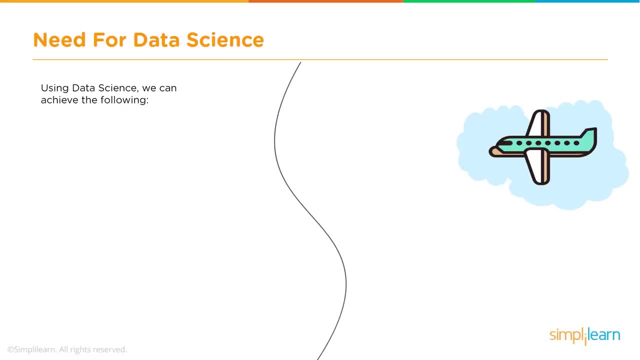 and also for the passengers. A few more examples. What else can we do? Here are some of the other things that we can do, and we will stick to the airline industry: Better route planning, so that there are less cancellations and less frustrated people. We can. 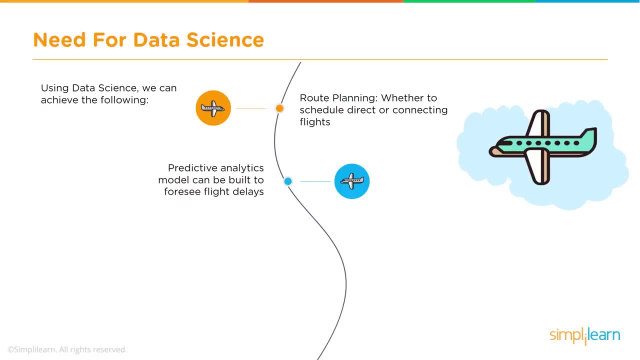 predict, use predictive analytics and predict any delays. that are there so that some flights can be rescheduled ahead of time and there are no last minute changes. Data science can also be used to make promotional offers And the last but not least is what kind of planes should be used, or? 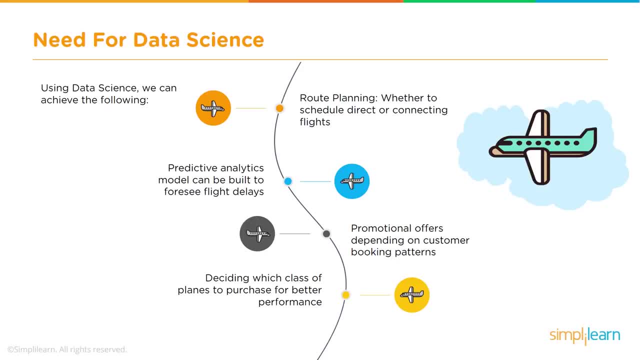 the different classes of planes that should be used to make promotional offers. So this is a good example of how data science should be used in different routes for better performance. So these are some examples of how data science can be used in airlines. And another example: 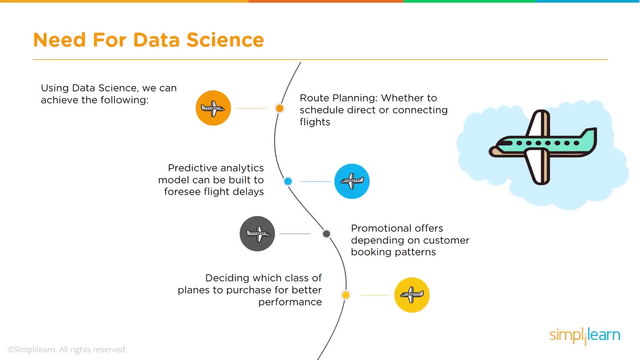 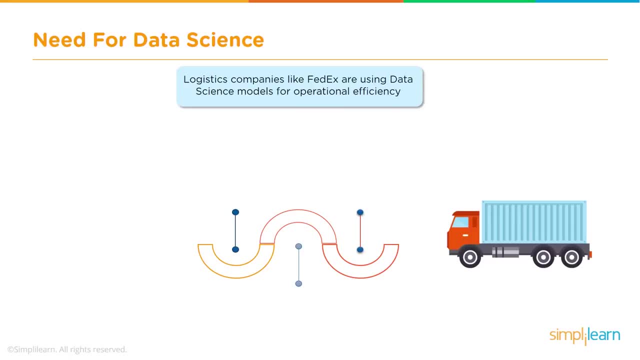 or another industry where data science can be used and benefited would be in logistics. So companies like FedEx. they use data science models to increase their efficiency drastically, to optimize the routes and cut costs and so on. So before their delivery truck actually arrives, they determine which is the best possible route to ship their items to the customers. 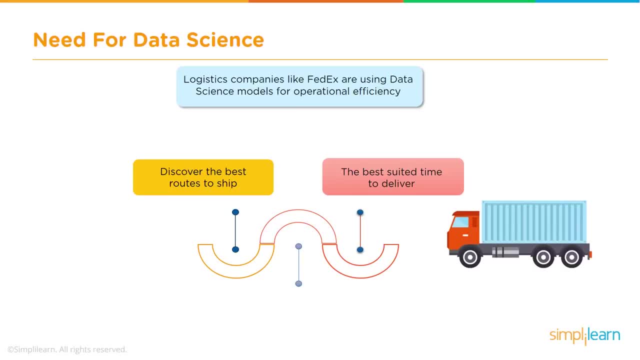 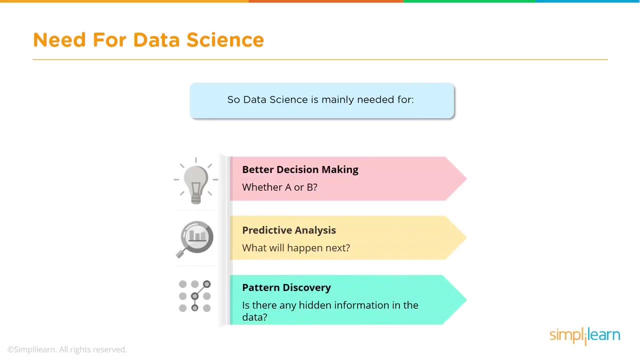 And, based on various inputs, they also predict or come up with the best suited time to deliver And, last but not least, they determine what is the best mode of transport for this delivery as well. So what is data science used for? These are some of the main areas where data science is used for. 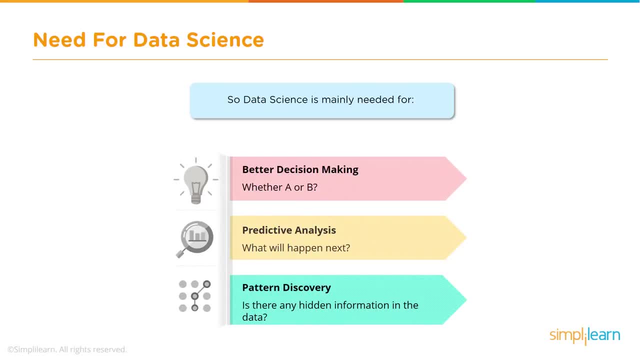 better decision making. There are always tricky decisions to be made. So which is the right decision, Which way to go? So that is one area Then for predicting, for performing predictive analysis like, for example, can we predict delays, like in the case of airlines? Can we predict the demand for certain products, let's say in e-commerce? 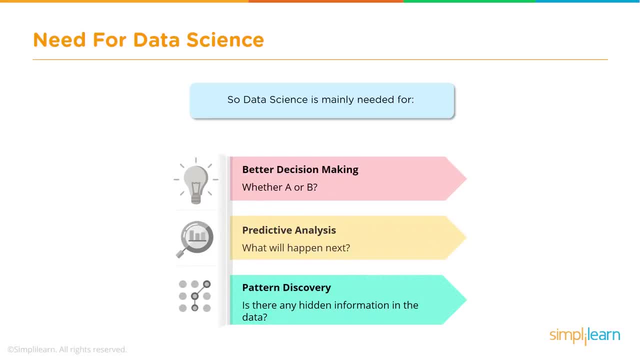 That is the second area. The third area is pattern discovery or pattern recognition. Is there a pattern in which people are buying items? For example, it could be seasonality. If you take the data for multiple years, there may be a pattern in the way people are buying. That's a buying pattern. 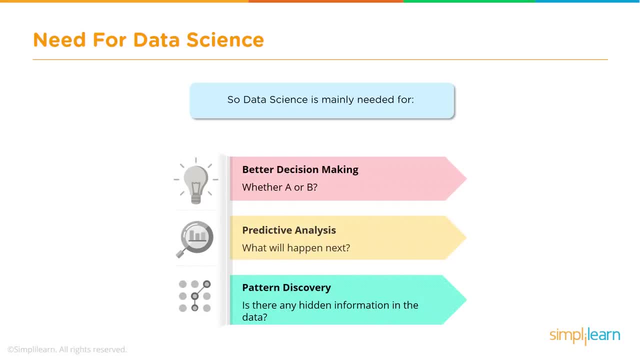 Certain months, probably, the sales will increase. Certain months the sales will come down. Certain quarters. traditionally, the sales will be higher Certain quarters. So that is a pattern And this pattern discovery is another area where data science is applied. So what is data science? 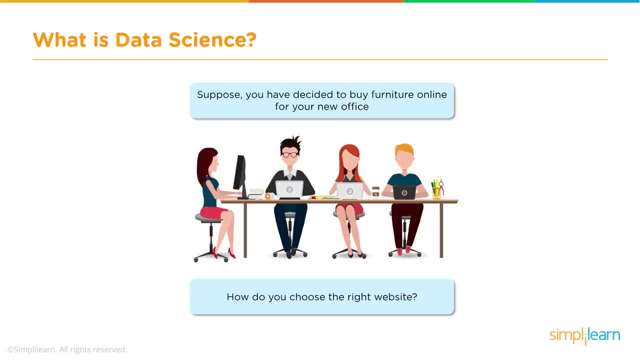 Now let's take an example, a real life example. On a day to day basis, we use, or we try to make some decisions. Let's say we want to buy some furniture online for our new office. So how do you go about doing this? You need to take a bunch of decisions to actually do the purchase. So we 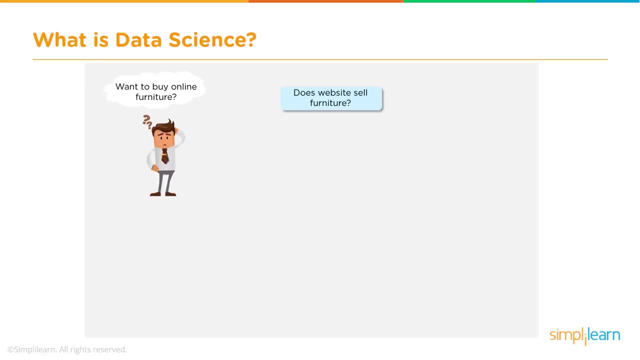 start with which website, which portal or which website you should use. So we try to find out. let's say you want to buy the furniture. Obviously you don't go to an online grocery store because you need furniture, because there are several websites. So that is the first decision you need to take. 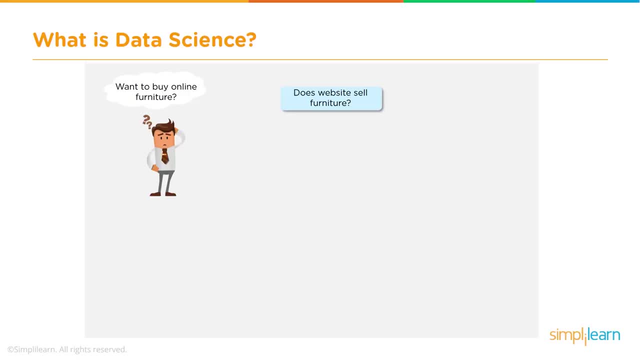 I should use. So, once we have multiple websites, you kind of discard all the websites which don't sell furniture and you stick to those websites which sell furniture. Now, within that, we try to find out what is the ratings of these websites. If the ratings is more, that means they are. 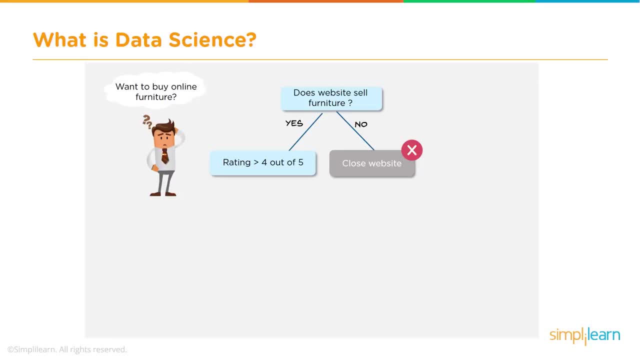 reliable, the quality probably is good, and so on and so forth. So only then you want to buy from that particular website. So anything that doesn't satisfy this criteria, you close all those websites. Close in the sense you close the browser right. So you still are left with. 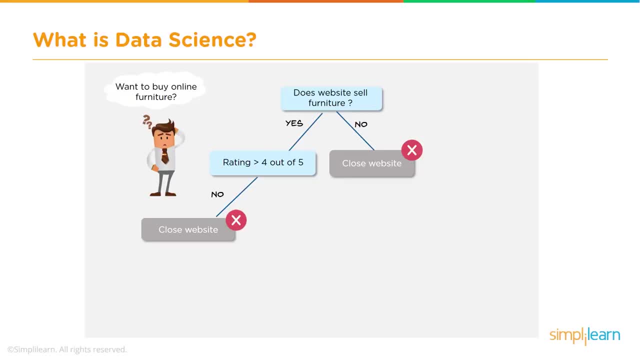 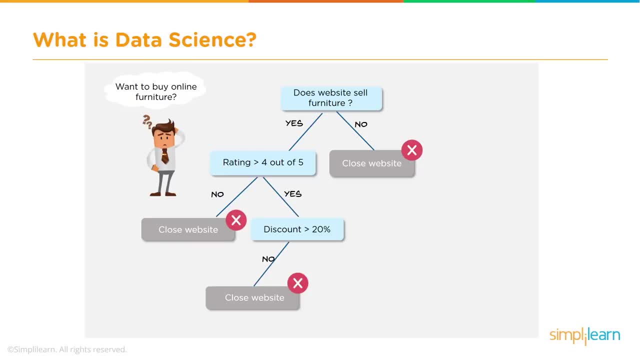 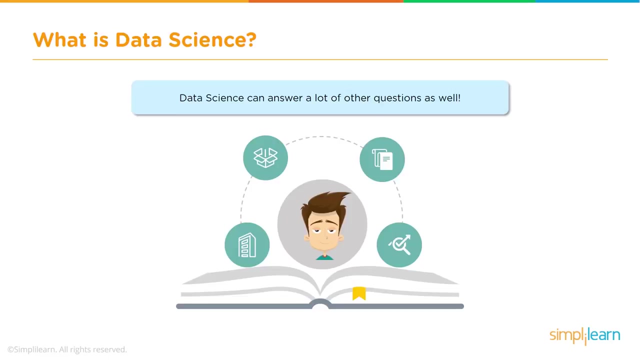 Is somebody providing a discount greater than 20%. Then again you filter out some of them which probably are not providing any discount, and zero down to one or two websites which are probably providing those discounts, and go ahead and select the furniture and purchase it. So this is a very basic example. You probably don't follow this always exactly the same way, but just to illustrate, drive home the point. So we can answer a lot of questions using data science, For example. 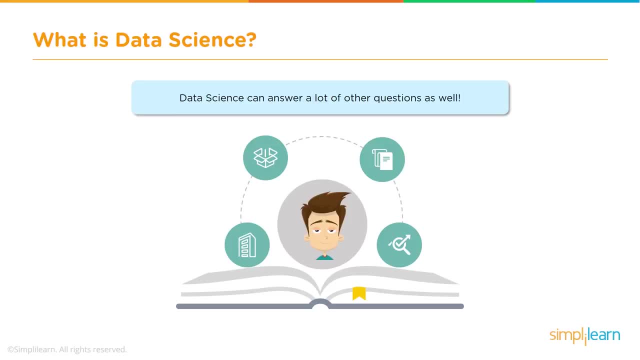 when we take a cab, when we book a cab now to go from location A to location B, what is the best route that the cab can take to reach in the fastest way or in the least amount of time? There could be several factors: There could be traffic, there could be bad road, there could be weather. Now all these come as inputs and a decision needs to be taken as to which is the best route. Another example is TV shows, So Netflix. 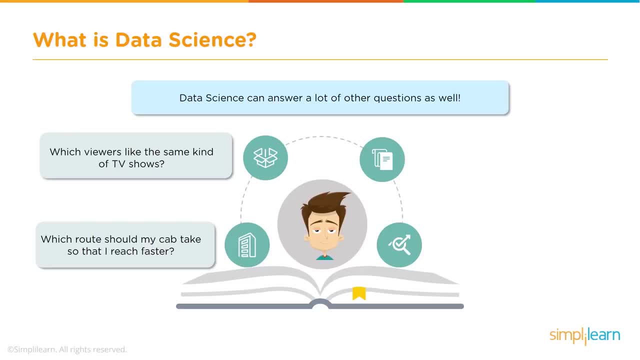 and maybe even other, a lot of other TV channels. they have to perform this analysis to find out what kind of shows people are viewing, what kind of shows people are liking, and so on and so forth, so that they can then sell this information to advertisers, because their main source of revenue is advertising. So this is again major function of data science: Predictive maintenance. We need to find out. we'll. 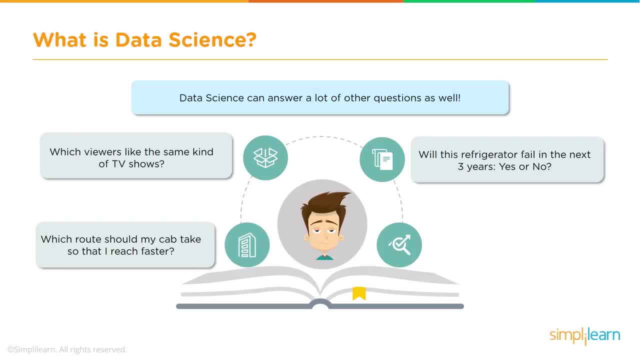 my car break down? will my refrigerator break down in the next year or two years? Should I be prepared to buy a new refrigerator? You can potentially apply data science here as well. And then in politics. a lot of data science is applied in politics. You must have seen on TV about US elections, or in UK or even in India. Nowadays everybody is applying data science in elections and trying to capture the. 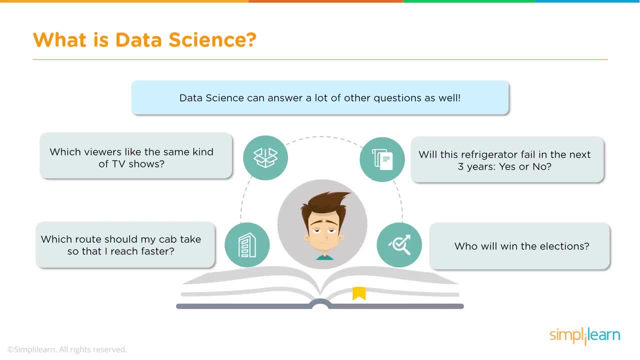 results, or rather, the voters influence the voters, personalized messages, providing personalized messages, and so on and so forth, And that is one Not only that, people use data science to even predict who is going to win the elections. It's a different matter that probably not all predictions come out to be true, But then, yes, this is, they use data science to do this: predictions. So what is the process, Or what are the? 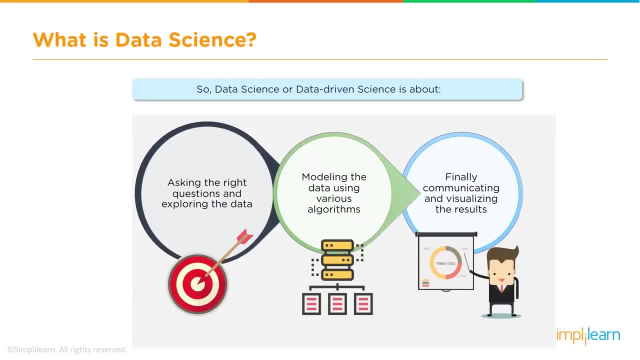 various steps in data science. The first step is asking the right question and exploring the data. Basically, you want to know what exactly is the problem you're trying to solve. So that is asking the right question. So that is the this circle out here. Then the next step is after exploring the data. So, as a first step, you will ask some questions- what exactly is the problem you're trying to solve? And then obviously you will have some data for that, as in 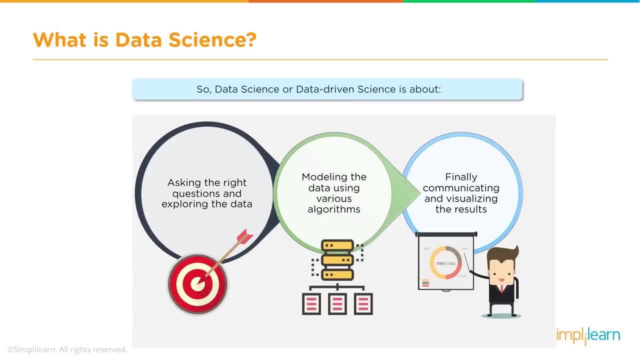 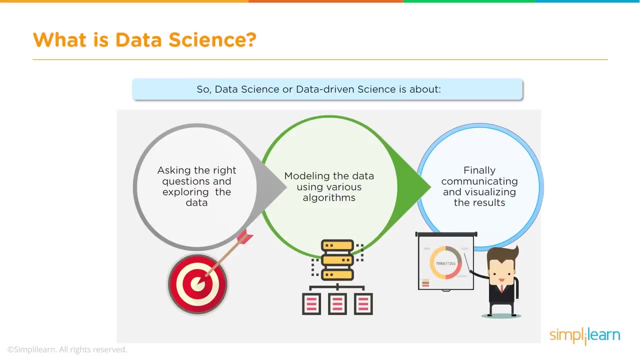 you perform some exploratory analysis on the data. For example, you need to clean the data to make sure everything is fine, and so on and so forth. So all that is a part of exploratory analysis. And then you need to do the modeling. Let's say, if you have to perform machine learning, you need to decide which algorithm to use and which model to use, And then you need to train the model, and so on and so forth. So that's all part of the modeling process And then you run your 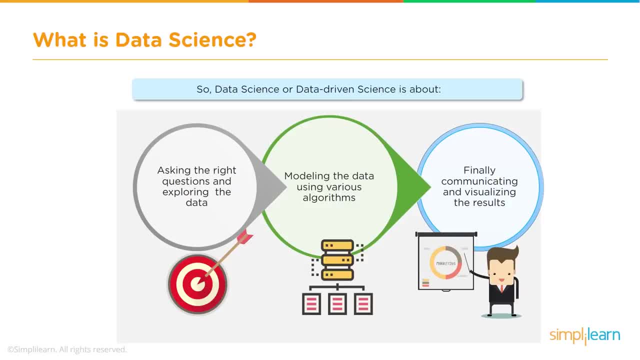 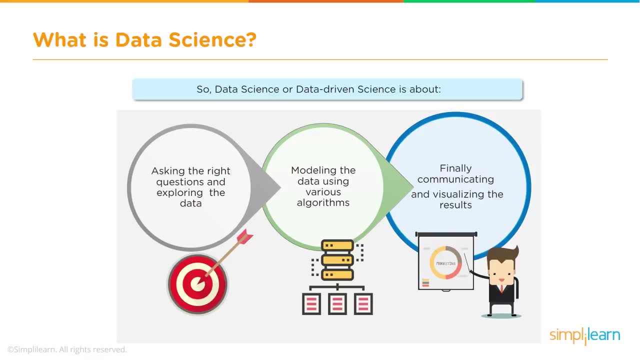 data through this model and then through this process, And then you come out with the final results of this exercise, which includes visualizing the results and preparing a way to communicate the results to the concerned people. So it could be in the form of PowerPoint slides or it could be in the form of a dashboard, which is basically what we call as a visualization, And so all the insights that have been 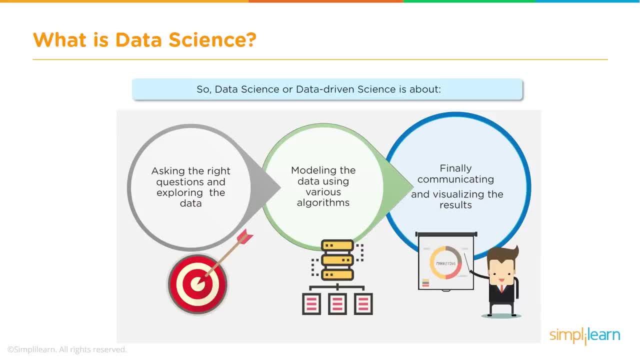 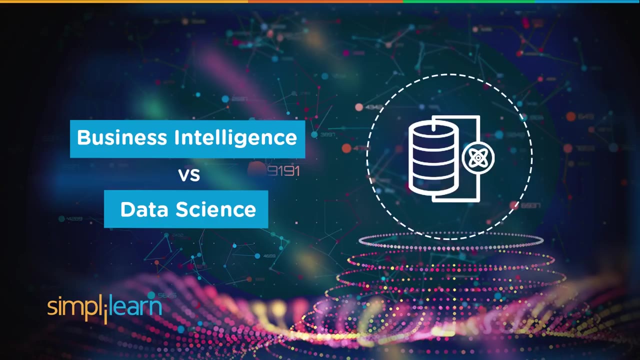 gathered through this exercise. that has to be communicated in a proper way, in an easy to understand way, which is again a key part of this whole exercise: communicating the results. So let's now talk about the difference between business intelligence and data science. Now, business intelligence was one of the initial phases where people started making, or wanted to make, some sense out of data. So, for some of you, 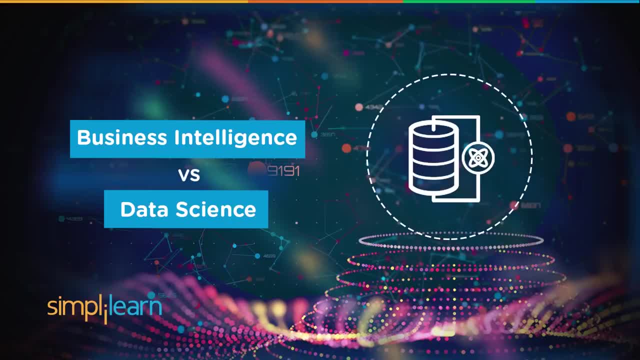 who may not be aware, there were multiple phases of this IT revolution. So initially there was all automations. you had automation of your selling process, manufacturing process. you had your ERP systems, your CRM systems and so on, which are basically enterprise resource planning and customer relationship management, ERP and CRM, And all these enterprise applications were generating a lot of data. So then people started saying that. 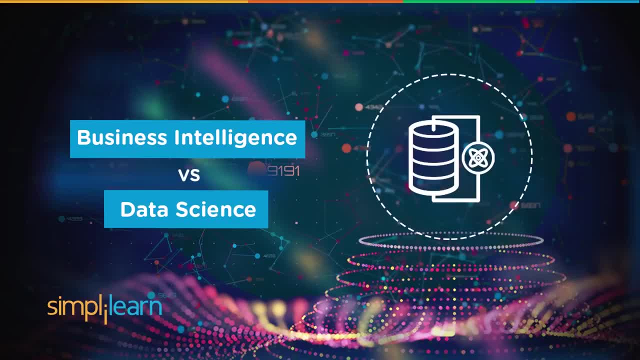 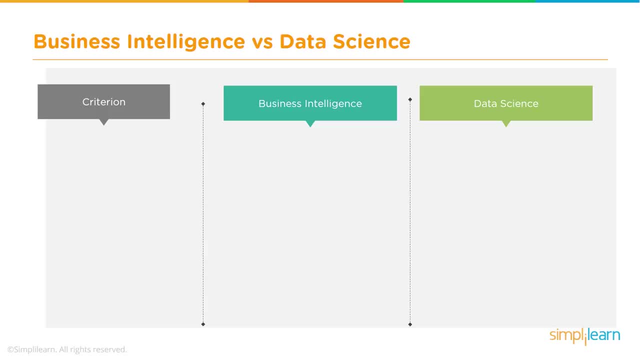 okay. we need to understand or get some information out of this data. So that's how business intelligence started. So if we take from a data source perspective, let's compare these from with each of these criteria. The criteria are: what is the data source, What is the method, What are the skills And what is the focus? If we compare business intelligence with data science, this is how it looks. As far as the data source is concerned, business intelligence was primarily using structured data. 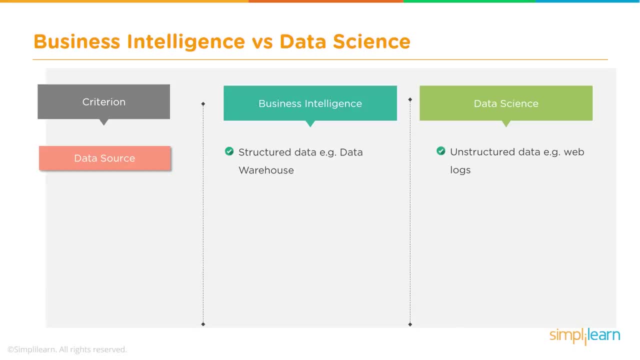 So you had all your enterprise applications like ERP, CRM and so on, And they were working out of pretty much RDBMS, relational database management systems like Oracle, MS SQL, MySQL and so on. So all this data was structured in neat form, form of tables, rows and columns, And then they were all brought into a centralized place because, remember, these were still different applications, So they were working off different data points. 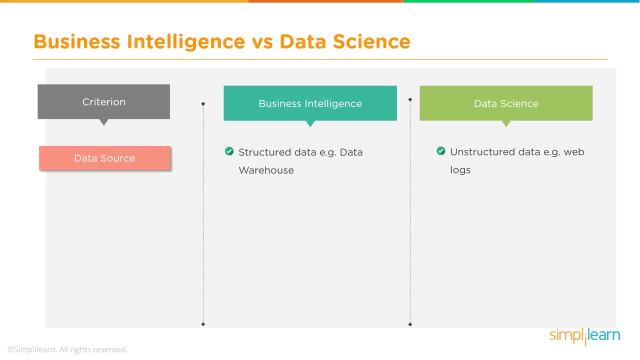 So if you wanted to get a combined view, you needed to create what is known as a data warehouse and bring all this data together and then look at it in a uniform way. So this is what business intelligence was doing. Pretty much it was structured data and it had reports and dashboards. That was pretty much what was there in business intelligence. Now, with data science, in addition to structured data, we also use a lot of data. 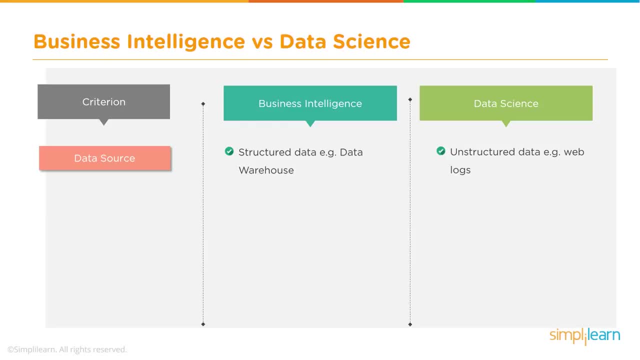 We use a lot of unstructured data, example, web logs or comments, If we are talking about customer feedback. there is a structured part. there is an unstructured part where people write free text. Data science includes that as well and brings everything and then performs analysis. So, data source wise, that is the difference. Now, methods In business intelligence: pretty much it is analytical in the sense that, okay, you have some data. we are just trying to present the truth And mostly what has happened, historical data. 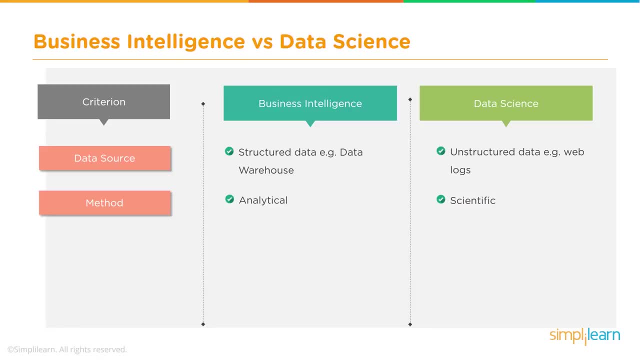 That's it. In case of data science, we go beyond that. We go deeper in terms of finding why a certain behavior has occurred, and also go beyond just providing a report. There is a deeper statistical analysis that is done, That is what is the scientific part, And deeper insights are gathered, not just reporting. So that's from a method perspective, From a skills perspective. business intelligence needs a little bit of statistics but more of 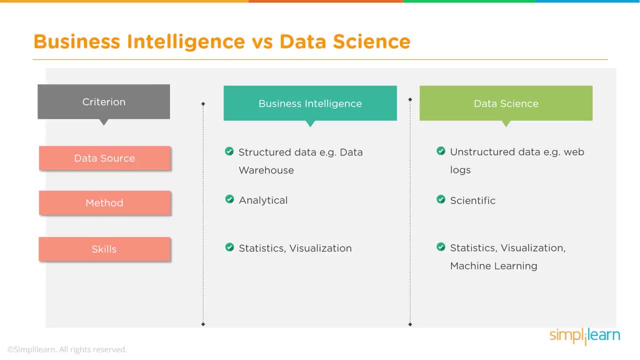 visualization, because they primarily consisted of dashboards, or they primarily consist of dashboards and reports, Whereas in data science the visualization of course is there, But there is a lot more of statistics involved, because we are looking at things like correlation. We are looking, for example, if we perform machine learning, we try to do regression, try to predict what will be the sales maybe in the future, and so on and so forth. So it is much more involved. 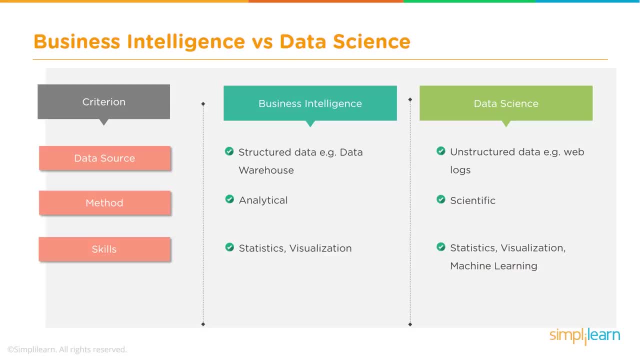 In case of data science compared to business intelligence. the skills are many more compared to business intelligence. And last but not least, what is the focus? Focus of business intelligence is pretty much historical data. So the sales have happened based on the sales. till today, You try to come up with a report: What was my sales? maybe for this whole year, or maybe for the last five years, and so on and so forth. In data science, you take historical data, but you also take historical data. 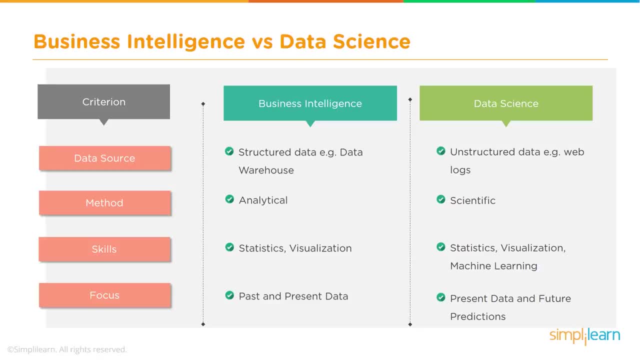 combine that with maybe some other required information and you also try to predict the future. so we try to extrapolate, maybe the sales and say, okay, sales as of now, as of today, this is sales is 5 million and if we, based on the, the historical information, we see that sales increase. 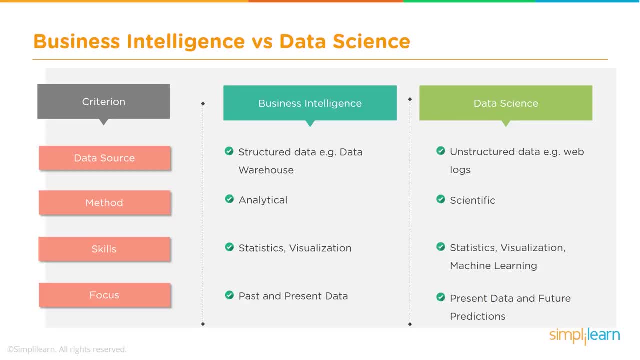 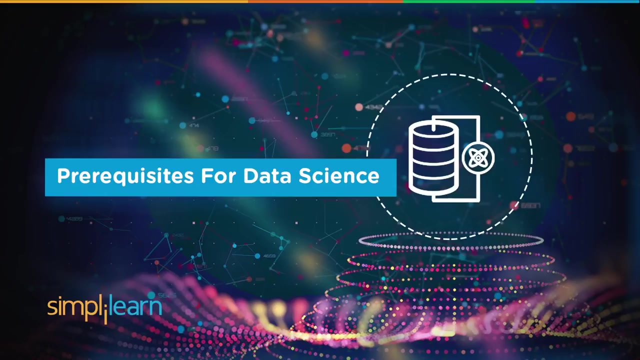 on a- maybe, i don't know- monthly basis- 10 percent, that is what history says. so our sales for next month will be this much right. so that is the focus of data science. it goes beyond just reporting. so what are the prerequisites for data science? there are three essential traits required for to be a 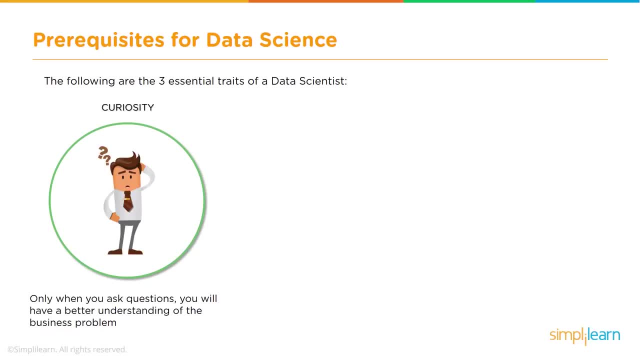 data scientist. one is curiosity. you need to be able to ask questions. the first step in data science is asking question: what is the problem you are trying to solve? if you ask the right question, only then you'll get the right answer. very often, this is a very crucial step where 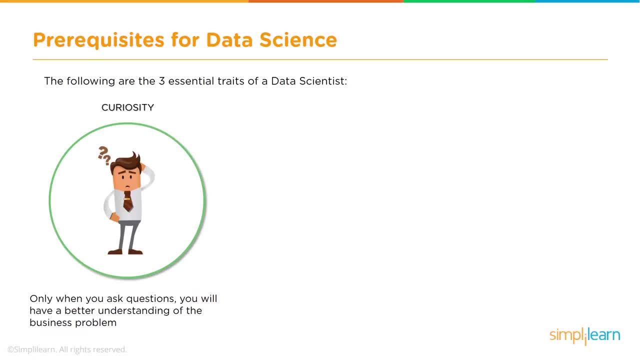 you can't just ask a question. you have to ask a question and you have to ask a question. a lot of data science projects fail because you're you may be asking the wrong question and then, obviously, when you get the answer, that's not the answer you're looking for. so it is very important. 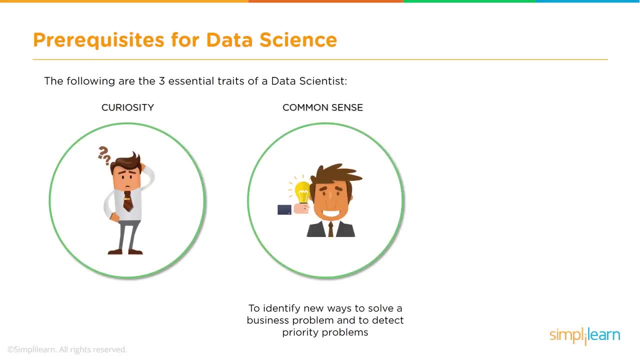 that you ask the right question. needless to say, then, the second part, or the second trait, is common sense. so you need to be creative, you need to come up with ways to use the data that you have and try to solve the business problem on hand. in many cases, you may not have all the data that you need. 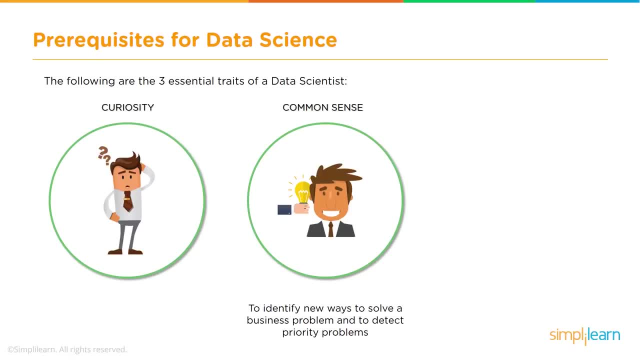 in many cases, the data may be incomplete, so that is where you need to come up with ways. what are the best ways to fill these gaps wherever this is missing? and that's where common sense comes into play. last but not least, after doing all this analysis, if you are unable to communicate the results in the 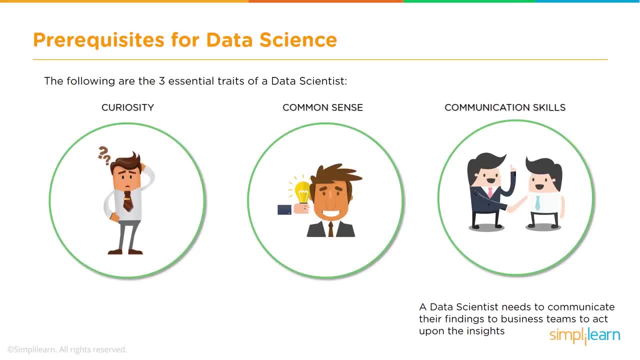 right way, the whole exercise will fail. so communication is a key trait for a data scientist. maybe technically you may be a genius, but then if you are unable to communicate those results in a proper way, once again that will not help. so these are the three main traits: curiosity, common. 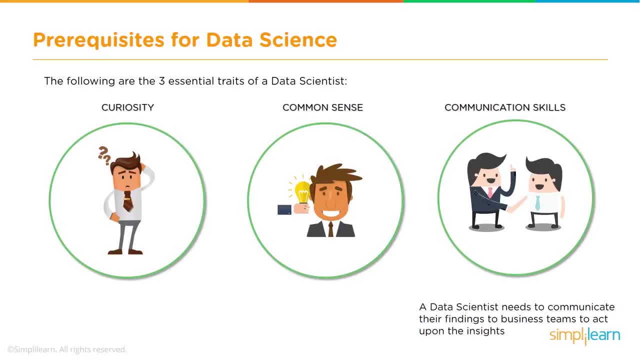 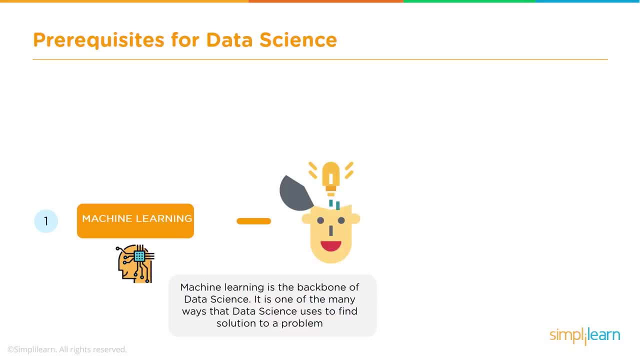 sense and communication skills. in a way, you can say: these are the three, c's okay. so what are the other prerequisites? first one, so machine learning. machine learning is the backbone of data science. data science involves quite a bit of machine learning in addition to the basic statistics. 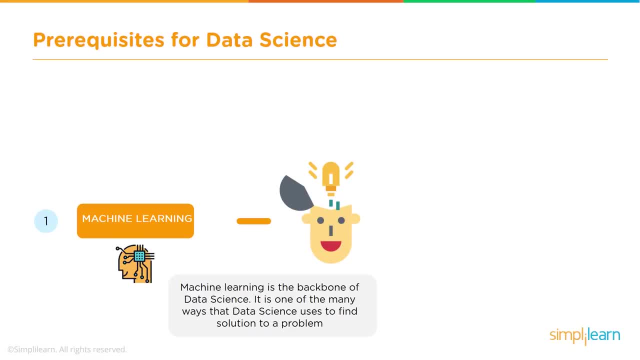 that we do so. a data scientist needs to have a good hang, or need to be very good at doing that- very good at data science. the second part is modeling. so modeling is also a part of machine learning in a way, but you need to be good at identifying what are the algorithms that are. 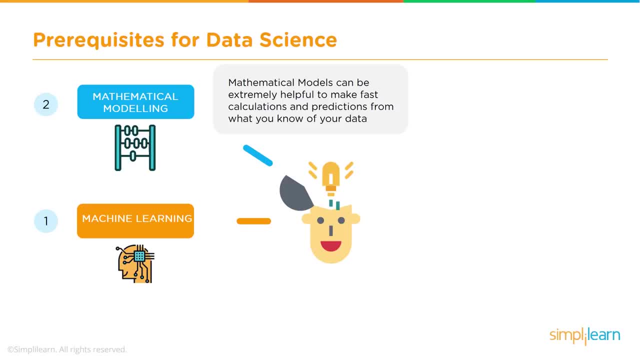 most suitable to solve a given problem, what models can we use and how do we train these models, and so on and so forth. so that is the second component. then statistics: statistics is like the core foundation of data science. so you need to understand statistics and you need to have a good hang of statistics in order to be a good data scientist. 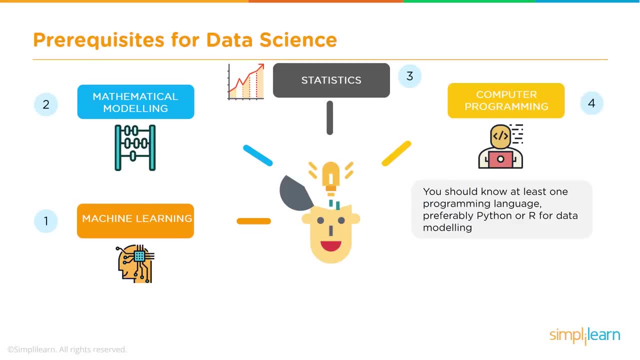 and this will also help in getting good results. programming is to some extent, required. at least some program or the other would be required as a part of executing a data science project. the most common programming languages are python and r. python, especially, is becoming a very popular programming language in data science because of its ease of learning, because of 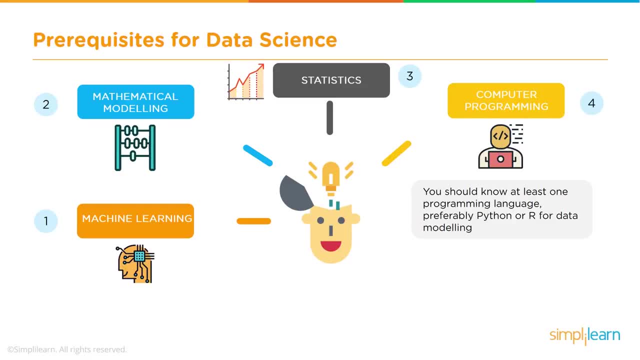 the multiple libraries that it supports for performing data science and machine learning, and so on. so python is by far one of the most popular languages in data science. if any one of you is is wanting to learn a new language, that should be python, and then, of course, you. 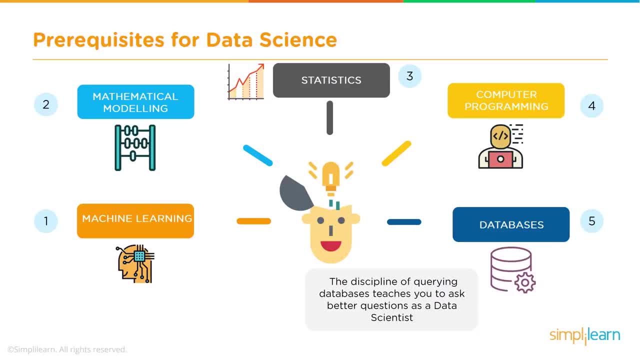 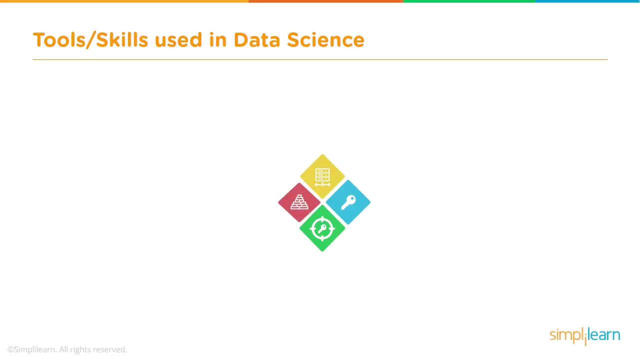 need to understand databases, how databases work and how to handle databases, how to get data out of databases, and so on. so these are some of the key components of data science. now coming to the tools and skills that are used in data science. these are some of the skills. from a language perspective- it is python or r- and from a skills, 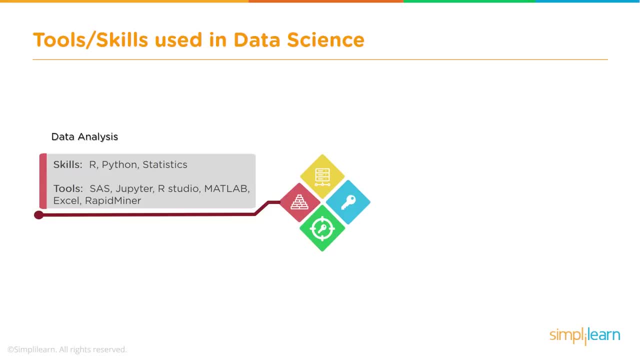 perspective. in addition to some of the programming languages, it would help if you have a good knowledge or good understanding of statistics and what are the tools that are used in data analysis. sas is one of the most popular tools. it's been there for a very long time and that's the reason it is very popular and, however, this is 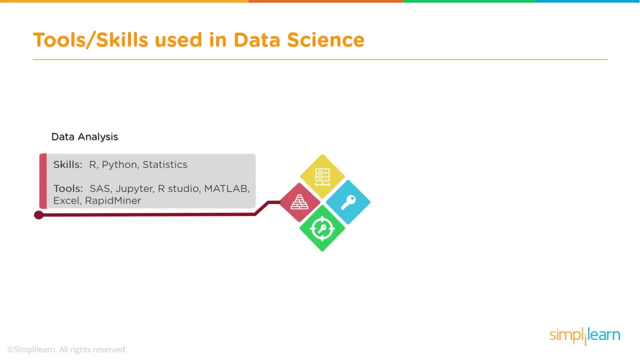 compared to most of the other tools, it is a proprietary software, whereas python and r are mostly open source. the other tools are like jupiter, jupiter notebooks. you have r studio. these are more development environments and development tools. so jupiter notebooks is a interactive development environment. similarly, r studio is for 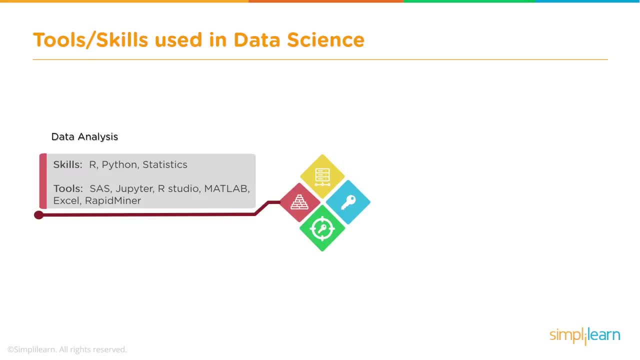 performing or writing r code and performing analytics and performing data analysis and machine learning activities you can perform in r studio. it has a very nice ui and initially r was not so popular, primarily because it did not have user interface. and r studio is a relatively new edition and after the advent of r studio, r became extremely popular and there are other tools like 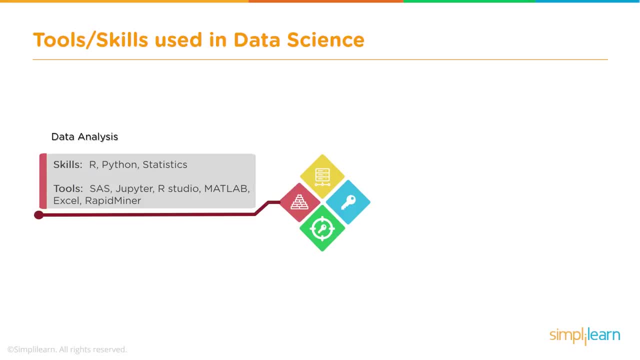 matlab and, of course, some people do with excel as well. as far as data warehousing is concerned, some of the skills that are required are etl. so in order to extract data and transform load, etl stands for extract, transform load, so you have data in the 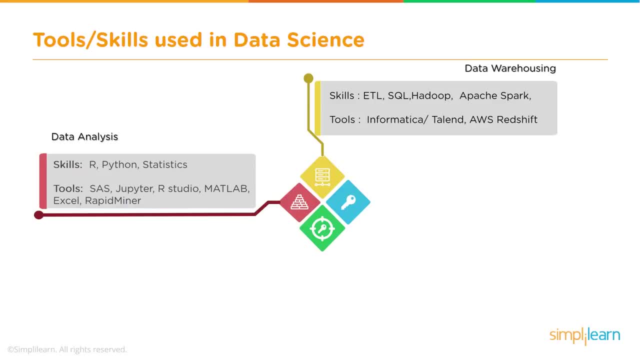 databases like your erp system or a crm system. you need to extract that and then do some transformations and then load it into your warehouse so that all the data from various sources looks uniform. then you need some sql skills, which is basically querying the data, writing SQL queries. Hadoop is another important skill. 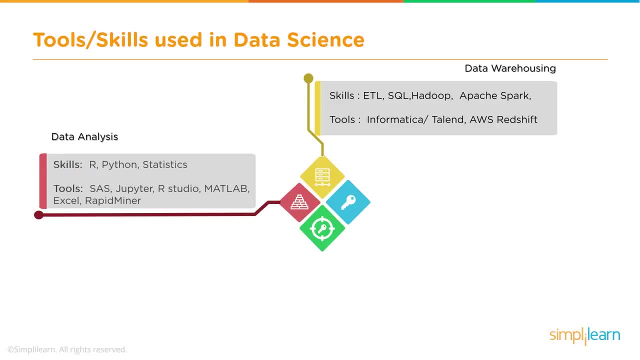 especially if you're handling large amounts of data, And also one of the specialties of Hadoop is it can be used for handling unstructured data as well. So it can be used for large amounts of structured and unstructured data- Then Spark is an excellent computing engine for performing. 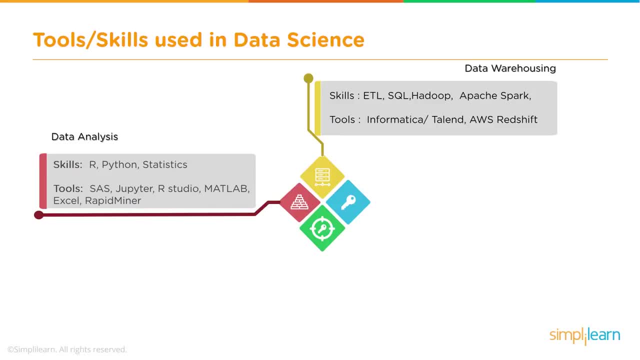 data analysis or machine learning in a distributed mode. So if you have a large amount of data, the combination of Spark and Hadoop can be extremely powerful. So you store your data in Hadoop, HDFS and use Spark as your computation engine. It works in a distributed 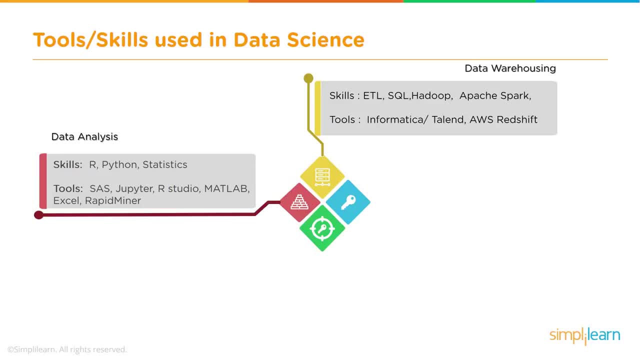 mode similar to Hadoop, like a cluster. So those are excellent skills for data warehousing And there are some standard tools that are available, like Informatica, Data Stage, Talent and also AWS Redshift. If you want to do some on the cloud, I think AWS Redshift is again. 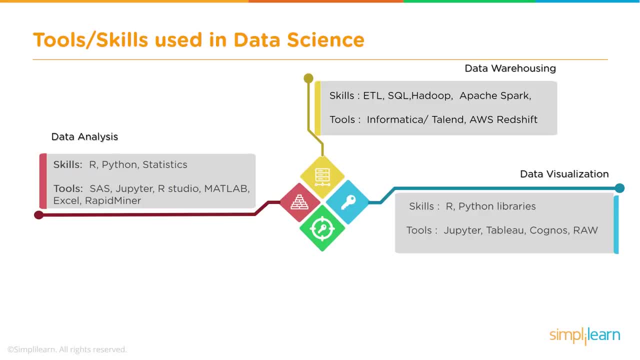 a good tool: Data visualization tools. For data visualization, some of the skills that would be required are, let's say, R. R provides some very good visualization capabilities, especially for developing during development. And then you have Python libraries, Matplotlib and so on. 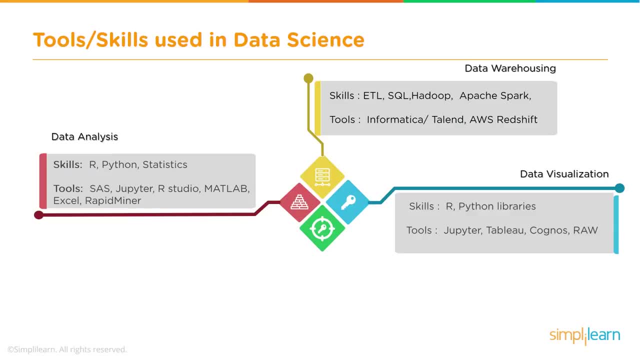 which provides very powerful visualization capabilities, And that is from skill perspective, Whereas tools that can be used are: Tableau is a very, very popular visualization tool. Again, that's a proprietary tool, so it's a little expensive maybe, but excellent capabilities from. 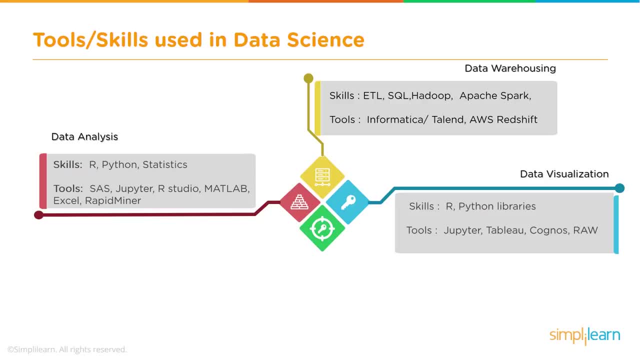 a visualization perspective, Then there are tools like Cognos, which is an IBM product, which provides very good visualization capabilities as well. And then, coming to the machine learning part of it, the skills required there are Python, which is more for the programming part, And then you will. 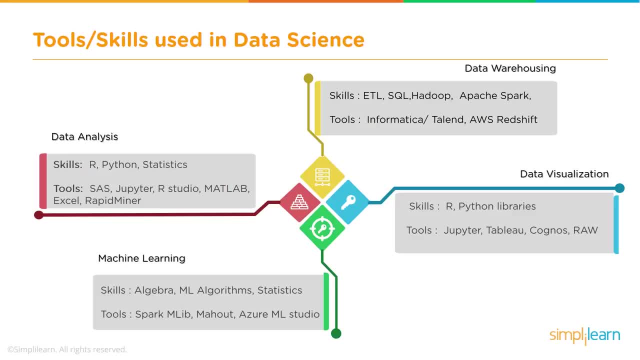 need some Mathematical skills, like algebra, linear algebra especially, and then statistics and maybe a little bit of calculus and so on, And the tools that are used for machine learning are Spark, MLlib and Apache, Mahout And on cloud, if you want to do something, you can use Microsoft Azure ML Studio as well. 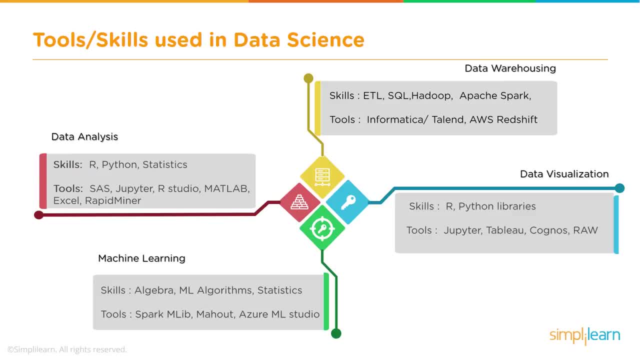 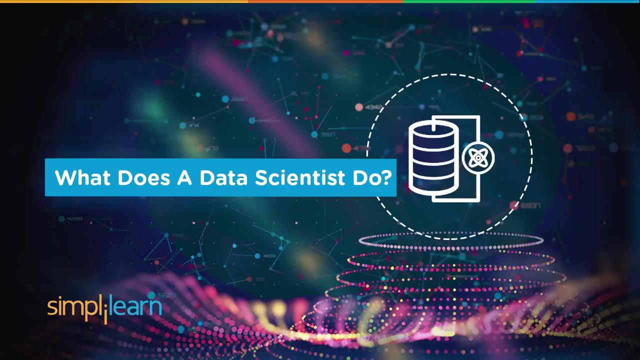 So these are by no means an exhaustive list. There are actually many, many tools and probably a few more skills also also maybe there, but this is this gives a quick overview, like a summarizing of summarization of the tools and skills. Now, moving on to the life of a data scientist: What does a data scientist do? 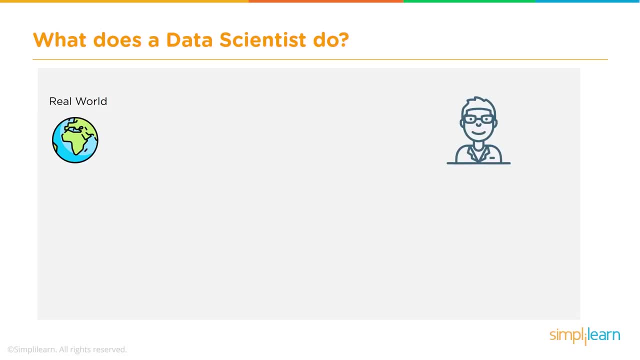 during the course of his work. So let's see. So, typically, a data scientist is given a problem, a business problem that he needs to solve, and in order to do that, if you remember from the previous slide, he basically asks the question as to what is the problem that he needs to solve. So 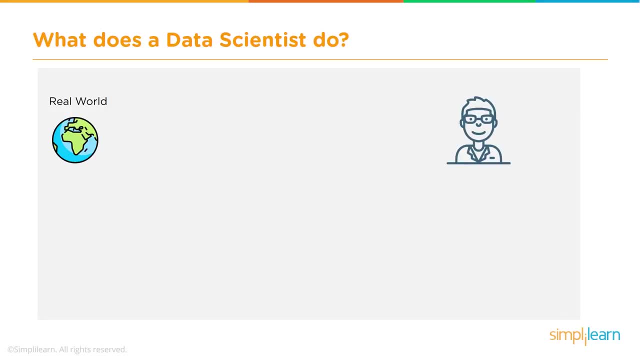 that is the first thing. he has got the problem. then the next thing is to gather the data that is required to solve this problem. So he goes about looking for data from anywhere it could be the enterprise. very often the data is not provided in the nice format that he would like to have it. 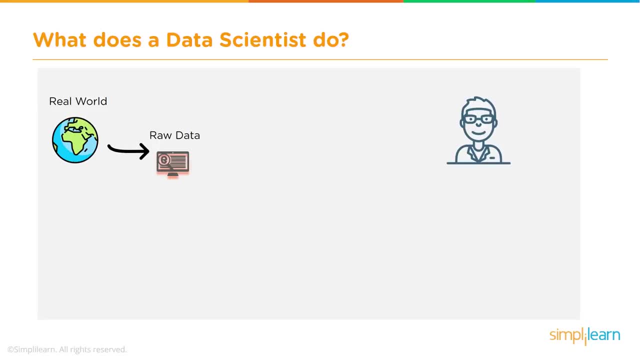 or we would like to have it. So first step is to get whatever data that is possible- what is known as raw data- in whatever format. So it could be enterprise data, it could be. it is a probably a requirement to go and solve the problem. So he goes about looking for data from anywhere it could. 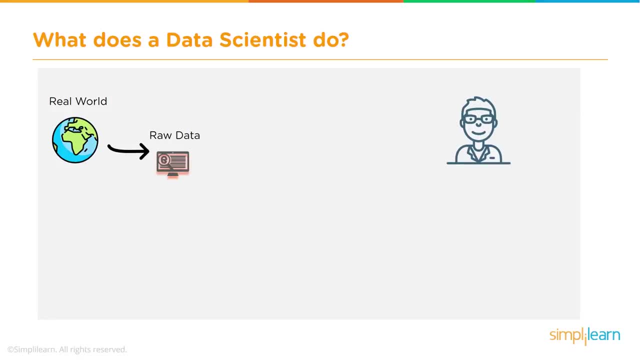 be town hall or for every corner of the city, Then he will go and get some public data in some cases. so all that raw data is collected and then that is processed and analyzed and in prepared into a format in which it can be used, And then it is fed into the analytics system, be it a machine learning algorithm. 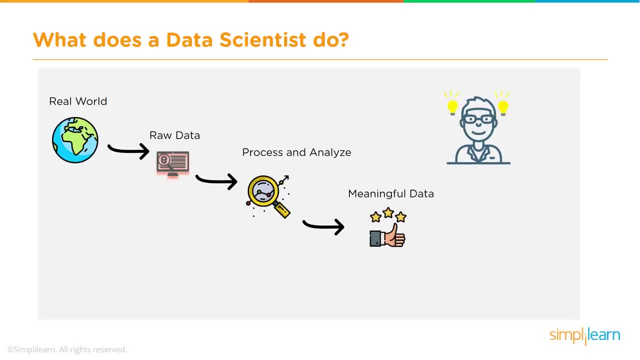 or a statistical model, and we get the output, and then he puts this output in a proper format for presenting it to the stakeholders and communicating insights or the results to the stakeholders. so this is a very high level view of like a day in the life of data scientists: gathering data, raw data. 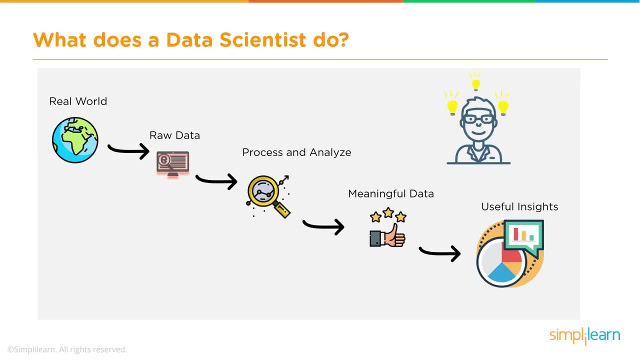 performing some quick analysis on that and maybe processing or manipulating this data to bring it into a certain good format so that it can be used for the analysis, feeding this into that analysis system that has been designed- be it mathematical models, machine learning models- and then get the results. 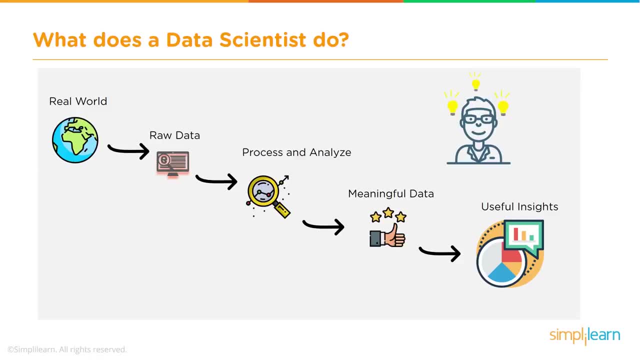 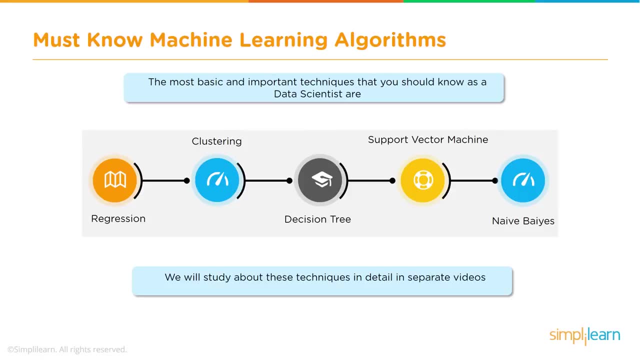 the insights and then present it in a nice way so that the stakeholders can understand how. about machine learning algorithms? so let's see what are the various machine learning algorithms that would be required for a data scientist. so these are a few of the algorithms. again, there's not an exhaustive list. we 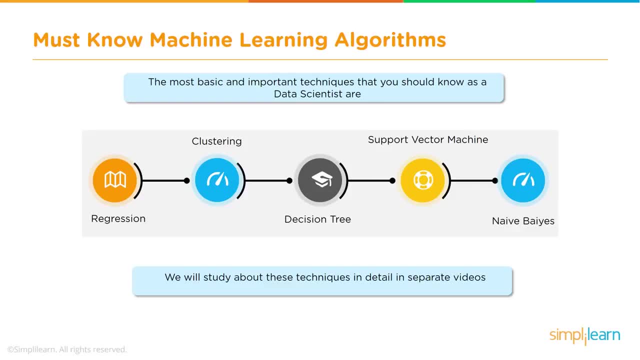 have. regression is one of the the supervised learning models or techniques. so in case of regression you try to, let say, come up with a continuous number. so the difference between regression and, let's say, a classification is that in case of classification those are discrete values, whereas here we are talking about regression, where you, let's: 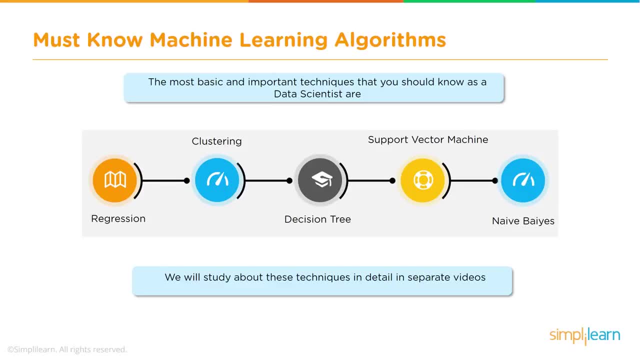 say you are trying to predict the temperature, which is a continuous value, or the share price, which is a continuous value. so that is regression. so you need to know what is regression, how to perform regression and we need to understand clustering. so clustering is one of the unsupervised learning. 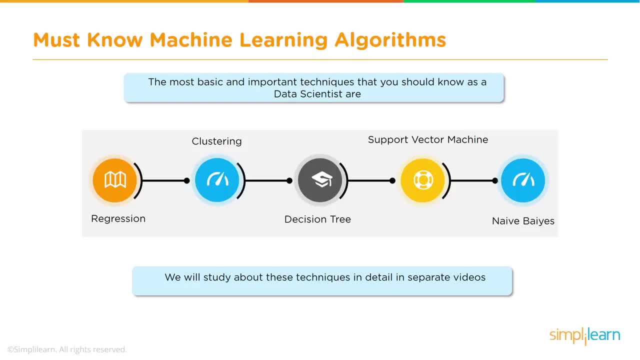 techniques. in this case, there is no label data that is available and you get some data and then you want to put this into some shape so that you can analyze it and you try to make sense out of it. let's say you have one example, is you? 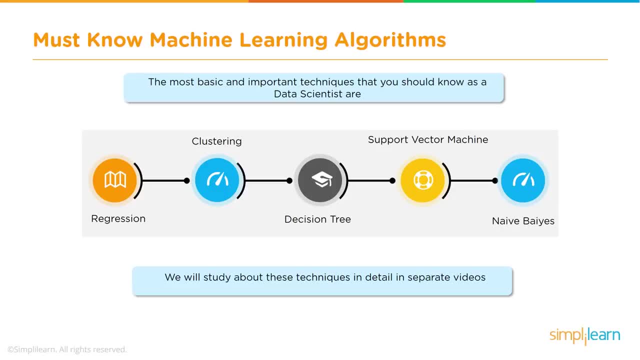 have a list of cricketers and they have not been marked as bowlers and batsmen or all-rounders are whatever. so you just have their names and maybe how many runs they scored, how many wickets they have taken and so on, but there is no readily available information saying that. okay, this. 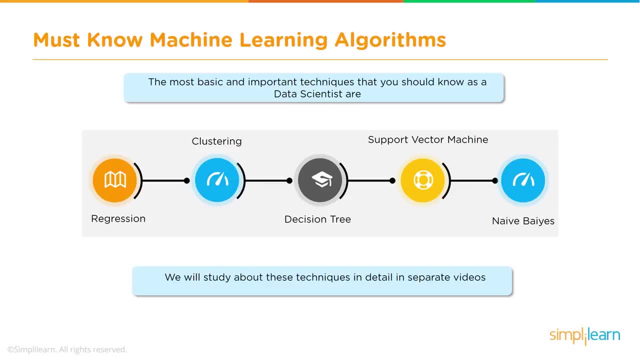 person is a batsman, this person is a bowler, and so on. so I'm talking about cricket- hopefully most of your familiar with the game of cricket. so how do we find out? so then we put this into a clustering mechanism and then the system will say that, okay, these 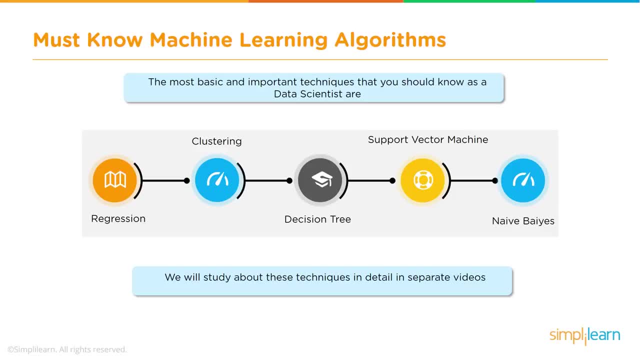 people who are all who have all scored good amount of runs, So they belong to one cluster. These are all the people who have taken good amount of wickets, So they belong to one cluster. And maybe here are some people who have taken good amount of wickets and they have made good. 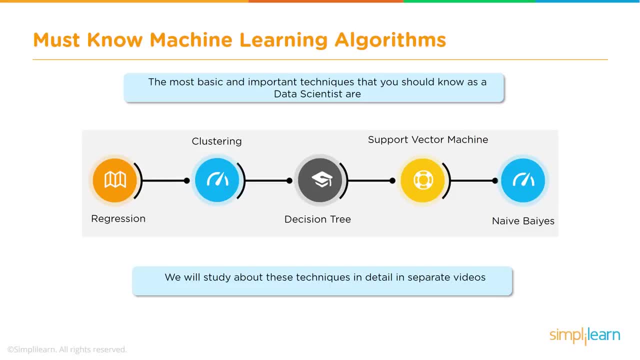 amount of runs, So they may be belonging to one group, And then we take a look at it and then we label them as okay, people who have all together and those who have, you know, scored many runs they are. we label them as batsmen. People who have taken a lot of wickets, we label them as 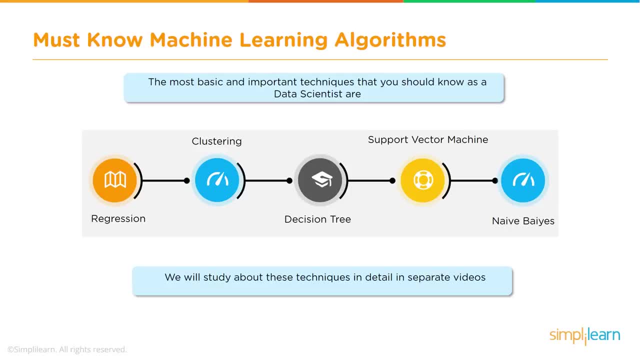 bowlers And people who have taken a good amount of wickets and also made some good runs. we label them as all-rounders. But the system will just say: okay, this is cluster one, cluster two, cluster three, The names we give. we human beings have to give the names. Now decision tree is used. 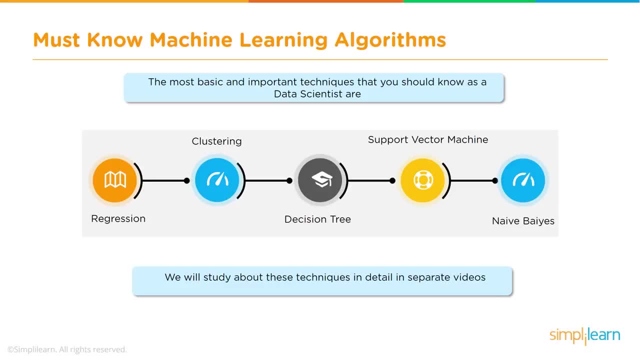 for what is known as classification Primarily. it can also be used for regression, but by and large it is used for classification, And here again it's a very logical way in which the algorithm goes about classifying the various inputs. One of the biggest advantages of decision tree is that 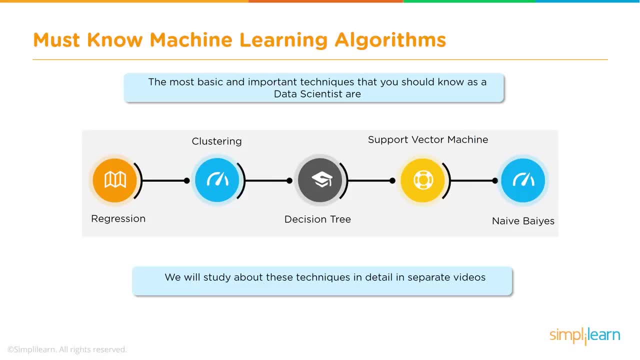 it's very easy to understand and it's very easy to explain why a certain object has been classified in a certain way compared to, maybe, some of the other mechanisms like, say, support vector machines or logistic regression and so on. So that's the question. 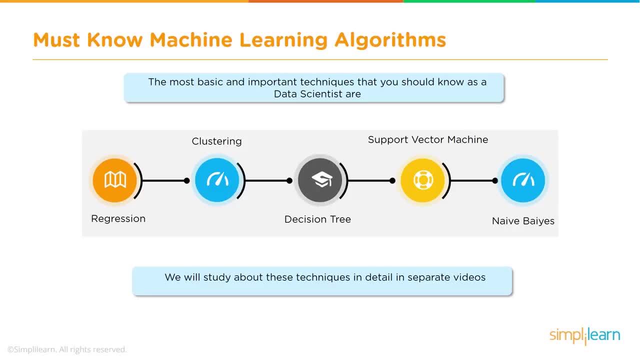 Advantage of decision tree, but that is also a very popular algorithm. Then we have support vector machines, primarily for classification purpose, And then we have naive base. This is a statistical probability-based classification method. So these are a few algorithms. There are a few more that are not listed here, but there are some more algorithms as well. And, by the way, 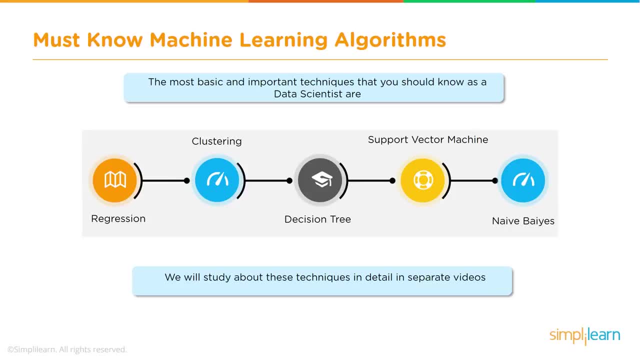 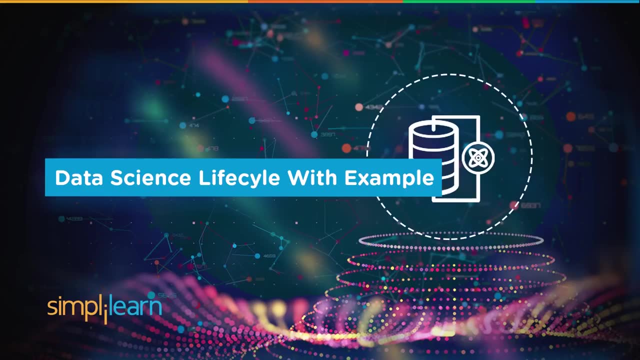 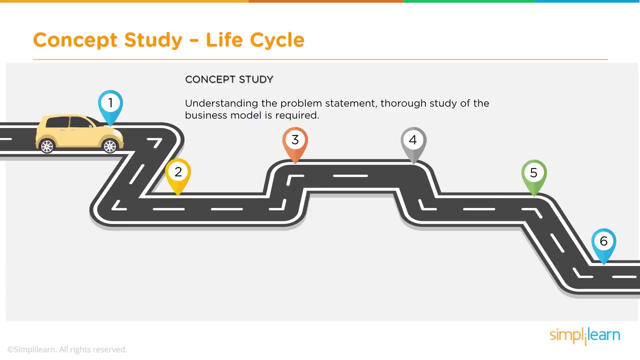 there are more detailed, or there are detailed videos about each of these algorithms Available. you can check in the playlist. So now let's talk about the life cycle of a data science project. Okay, the first step is the concept study. In this step, it involves understanding. 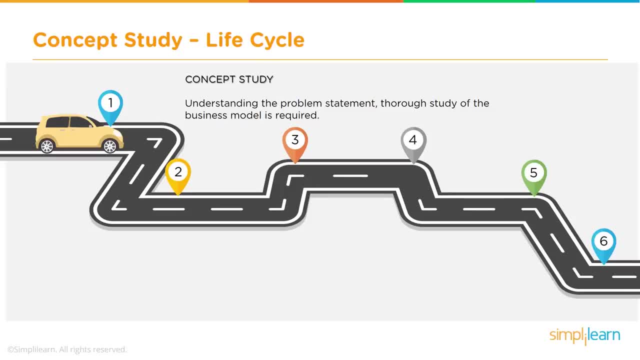 the business problem: asking questions, get a good understanding of the business model, meet up with all the stakeholders, understand what kind of data is available, And all that is a part of the first step. So here are a few examples We want to say. for example, we want to: 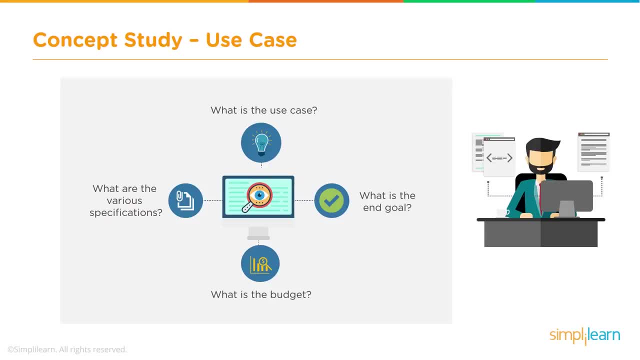 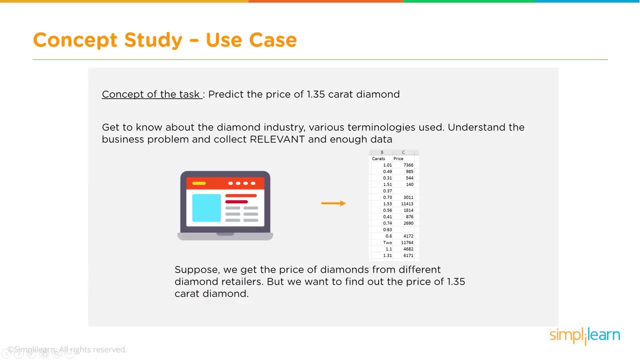 see what are the various specifications, And then what is the end goal, What is the budget? Is there an example of this kind of a problem that has been maybe solved earlier? So all this is a part of the concept study, And another example could be a very specific one: to predict the price of a 1.35. 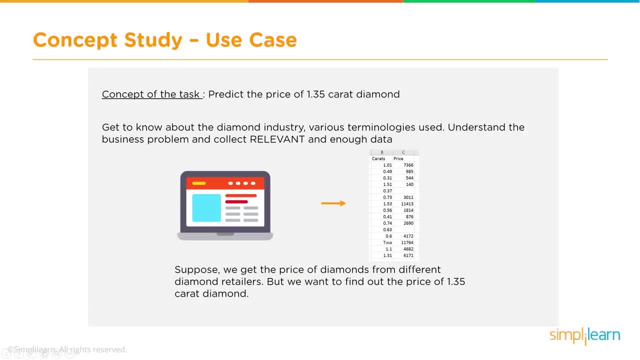 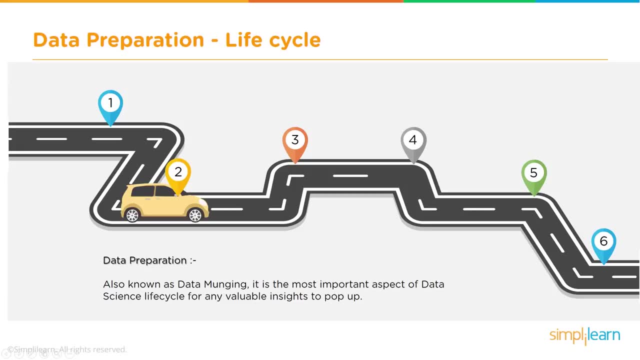 carat diamond And there may be relevant information inputs that are available And we want to predict the price. The next step in this process is data preparation: data gathering and data preparation, also known as data munging, or sometimes it is also known as data manipulation. So what happens here is the raw data that is 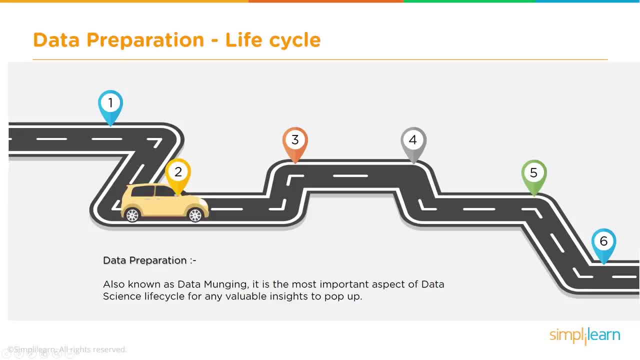 available may not be usable in its current format for various reasons. So that is why, in this step, a data scientist would explore the data. He will take a look at some sample data maybe pick. there are millions of records. pick a few thousand. 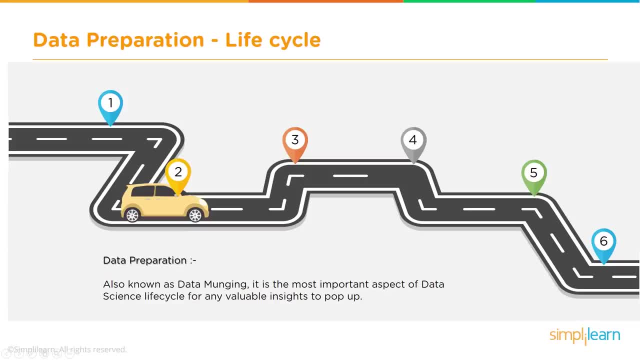 records and see how the data is looking. Are there any gaps? Is the structure appropriate to be fed into the system? Are there some columns which are probably not adding value may not be required for the analysis. Very often these are like names of the customers. They will probably not add any value. 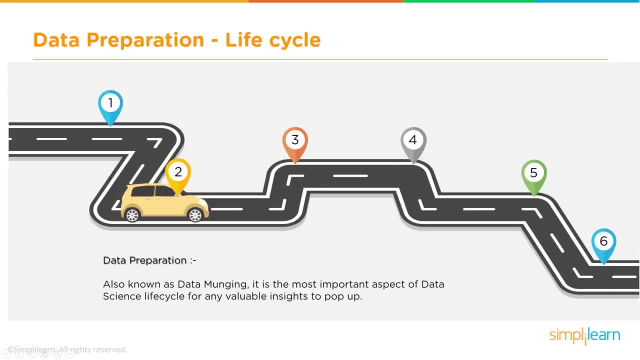 or much value from an analysis perspective. The structure of the data: maybe the data is coming from multiple data sources and the structures may not be matching. What are the other problems? There are gaps in the data, So the data, all the columns, all the cells are not filled. If you're. 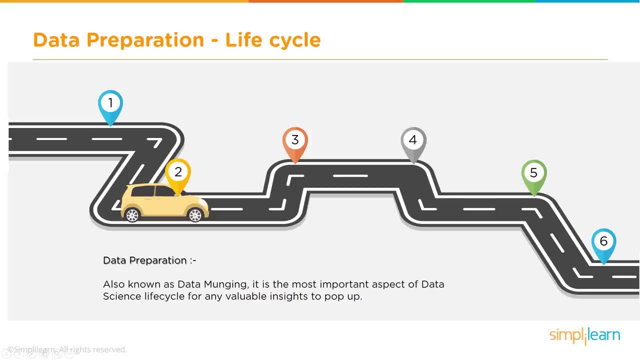 talking about structured data. there are several blank records or blank columns. So if you use that data directly, you'll get errors or you will get inaccurate results. So how do you either get rid of the data or how do you fill those gaps with something meaningful? So all that is a part of 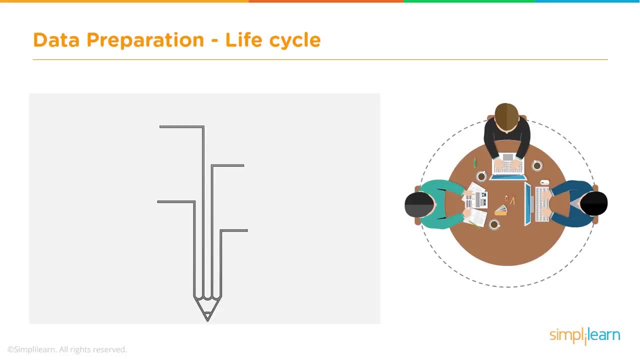 data munging or data manipulation. So these are some additional sub topics within that. So data integration is one of them. If there are any conflicts in the data there may be, data may be redundant. Yeah, data redundancy is another issue. 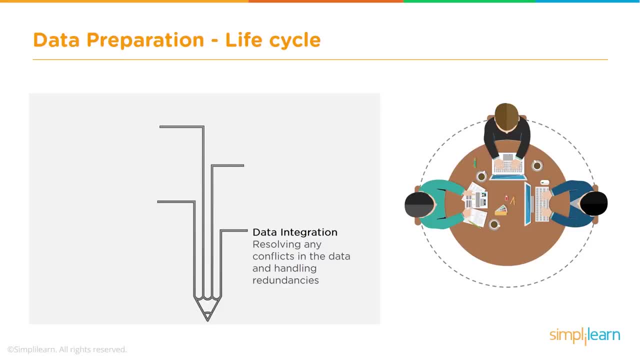 There may be. you have, let's say, data coming from two different systems and both of them have customer table, for example, customer information. So when you merge them, there is a duplication issue. So how do we resolve that? So that is one Data transformation. as I said, there will be. 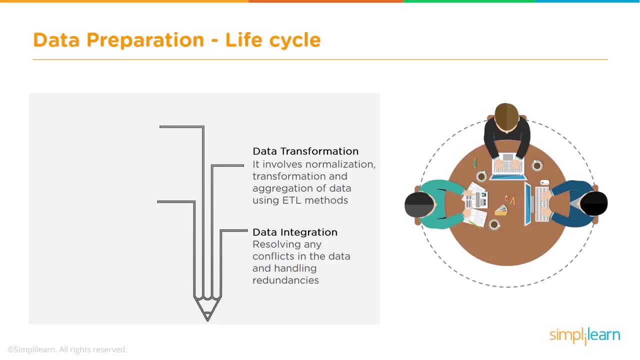 data is coming from multiple sources and then when we merge them together they may not be matching. So we need to do some transformations to make sure everything is similar. We may have to do some data reduction If the data size is too big. you may have to come up with ways to. 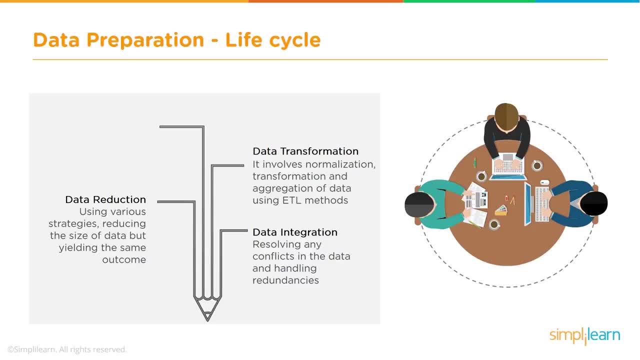 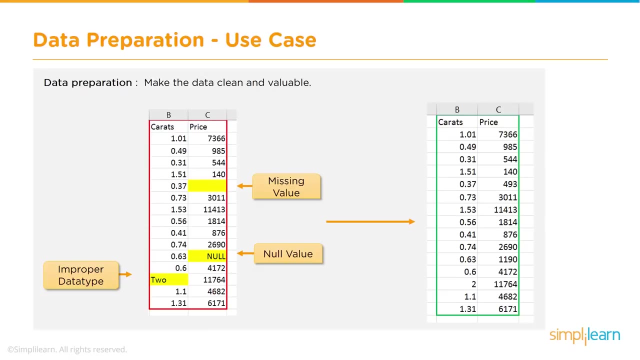 reduce it meaningfully without losing information. Then data cleaning. So there will be either wrong values or null values, or there are missing values. So how do you handle all of that? A few examples of very specific stuff. So there are missing values. How do you handle missing values? 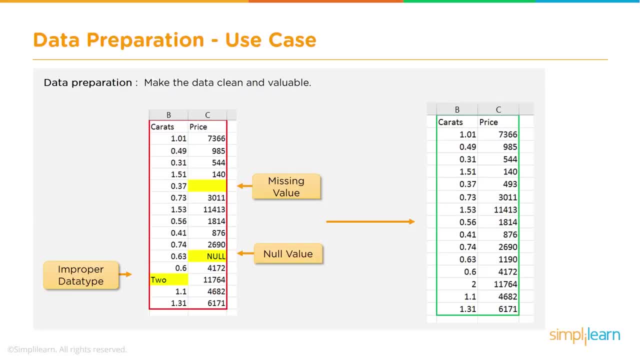 or null values. Here, in this particular slide, we are seeing three types of issues. One is missing value. Then you have null value. You see the difference between the two, right? So in the missing value there is nothing, Blank Null value. it says null. Now the system cannot handle. 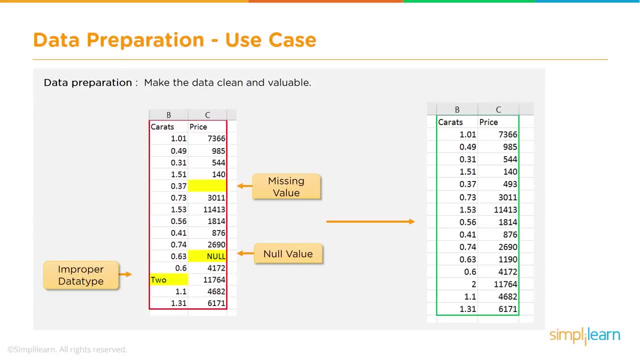 if there are null values. Similarly, there is improper data, So it's supposed to be numeric value, but there is a string or a non-numeric value. So how do we clean And prepare the data so that our system can work flawlessly? So there are multiple ways and there 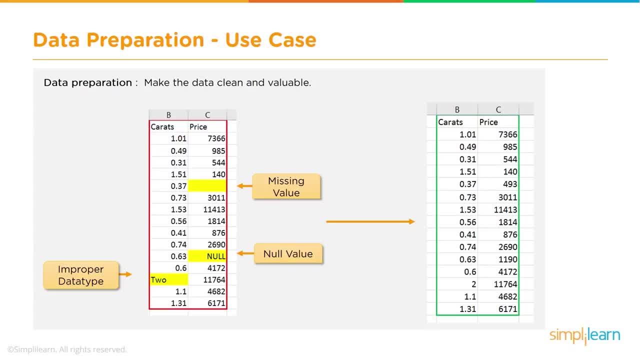 is no one common way of doing this. It can vary from project to project. It can vary from what exactly is the problem we are trying to solve. It can vary from data scientist to data scientist, organization to organization. So these are like some standard practices people come up with And 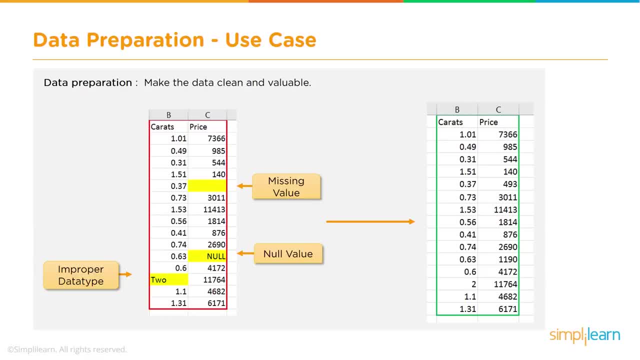 of course, there will be a lot of trial and error. Somebody would have tried out something and it didn't work. So that's how we need to take care of data cleaning. Now, what are the various ways of doing? you know, if values are missing, how do you take care of that? Now, if the data is too? 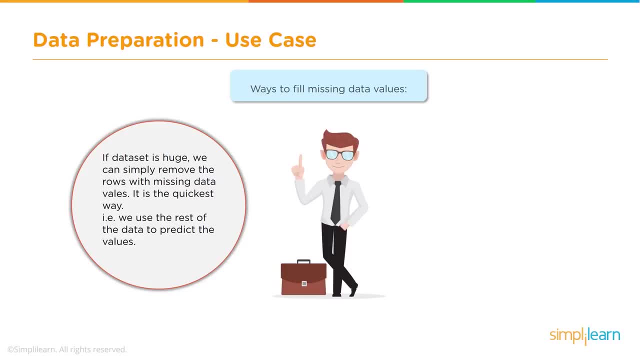 large and only a few records have some missing values, then it is okay to just get rid of those entire rows, for example. So if you have a million records and out of which a hundred records don't have full data, So there are some missing values in about a hundred records, So it's absolutely fine. 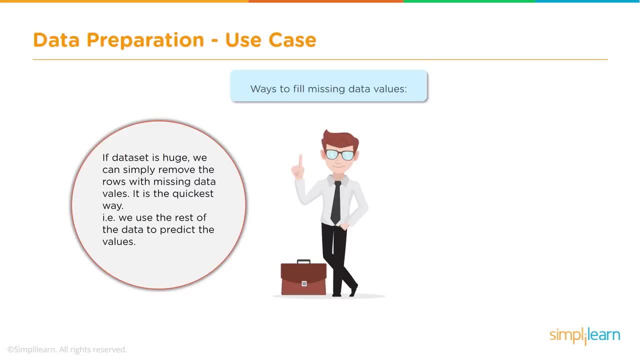 Because it's a small percentage of the data, So you can get rid of the entire records which have missing values. But that's not a very common situation. Very often you will have multiple or at least a large number of a data set. For example, out of a million records, you may have 50,000. 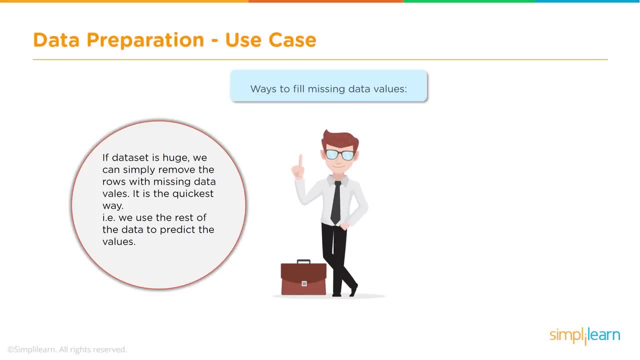 records which are like having missing values. Now that's a significant amount. You cannot get rid of all those records. Your analysis will be inaccurate. So how do you handle such situations? So there are multiple ways of doing it. One is you can probably if a particular values are missing in a particular 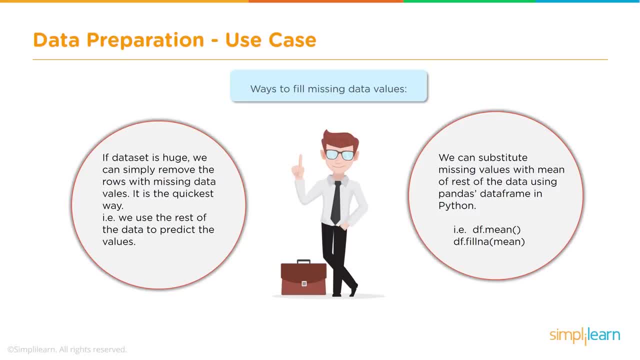 column, you can probably take the mean value for that particular column and fill all the missing values with the mean value, So that, first of all, you don't get errors because of missing values And, second, you don't get results that are way off because these values are completely different from. 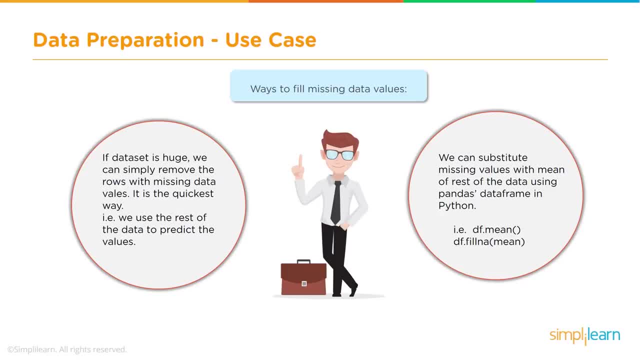 what is there. So that is one way. Then a few other could be either taking the median value or, depending on what kind of data we are talking about, So something meaningful we will have put in there. If we are doing some machine learning activity, then obviously as a part of data preparation. 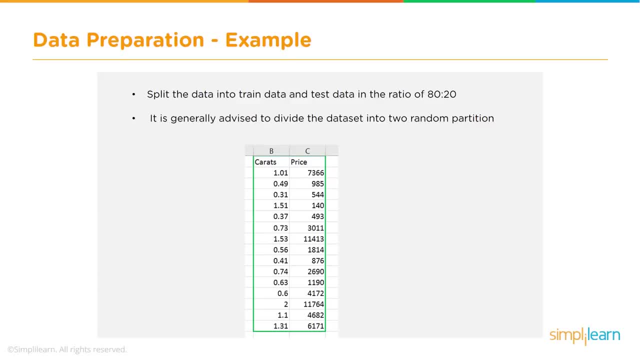 you need to split the data into training and test data set. The reason being, if you try to test with a data set which the system has already seen as a part of training, then it will tend to give reasonably accurate results because it has already seen that data, And that is not a good measure of. 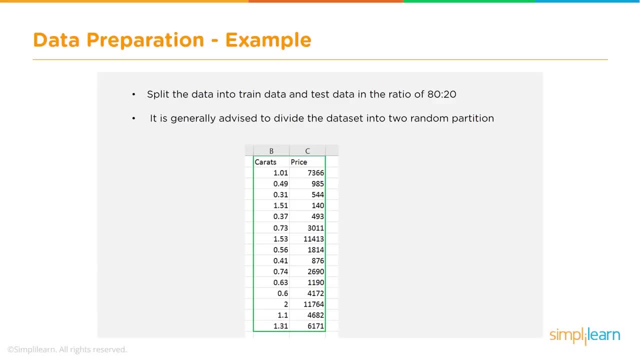 system. So typically you take the entire data set, the input data set, and split it into two parts. And again the ratio can vary from person to person, individual preferences. Some people like to split it into 50- 50.. Some people like it as 63.33 and 33.3 is basically two third and one third. 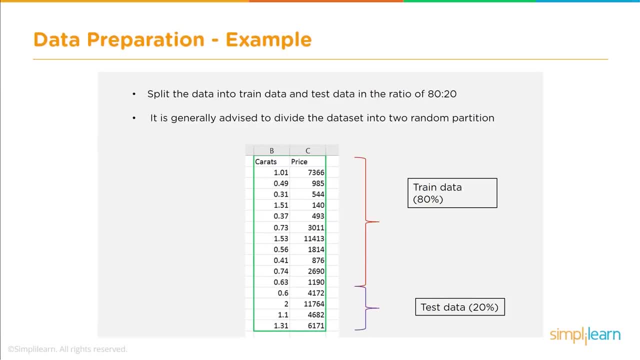 And some people do it as 80: 20,- 80 for training and 20 for testing. So you split the data, perform the training with the 80% and then use the remaining 20% for testing. All right, So that is one more data preparation activity. 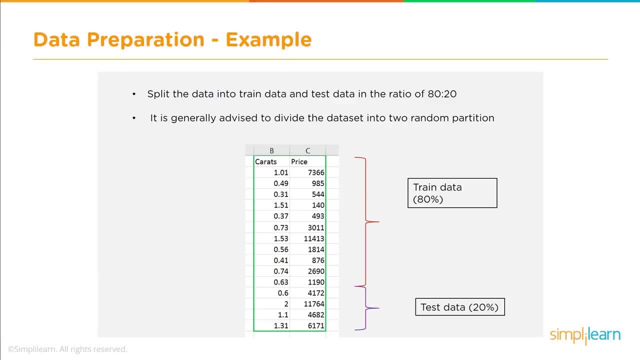 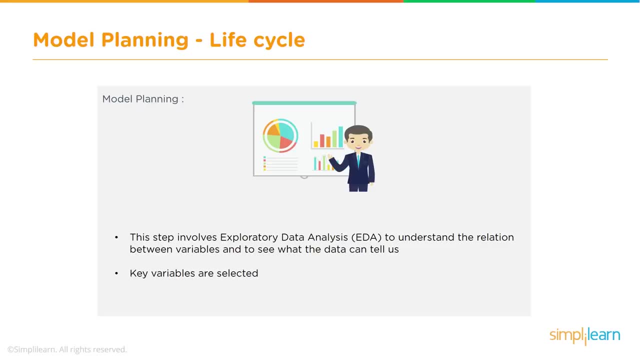 that needs to be done before you start analyzing or applying the data or putting the data through the model. Then the next step is model planning. Now this models can be statistical models. This could be machine learning models. So you need to decide what kind of models you are going to use. 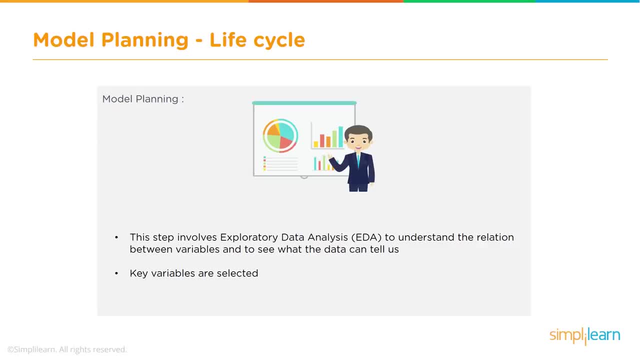 Again, it depends on what is the problem you're trying to solve. If it is a regression problem, you need to think of a regression algorithm and come up with a regression model So it could be linear regression. Or if you're talking about classification, then you need to pick up. 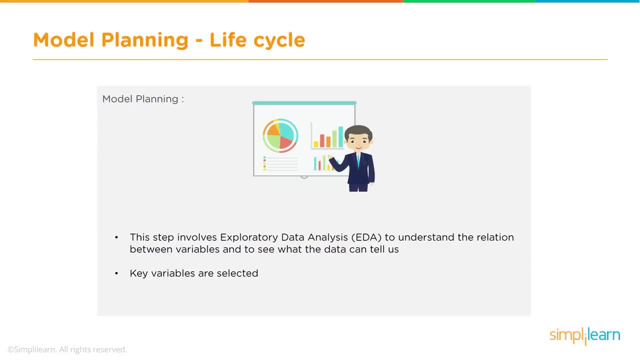 an appropriate classification algorithm like logistic regression or decision tree or SVM, and then you need to train that particular model. So that is the model building or model planning process, And the cleaned up data has to be fed into the model. And, apart from cleaning, 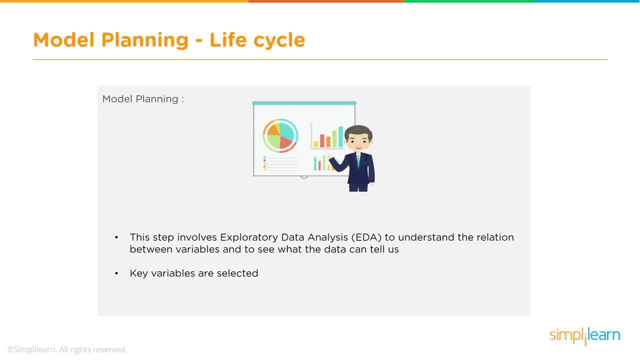 you may also have to. in order to determine what kind of model you will use, you have to perform some exploratory data analysis to understand the relationship between the various variables and see if the data is appropriate, and so on. Right, So that is the additional preparatory step that needs to be done. 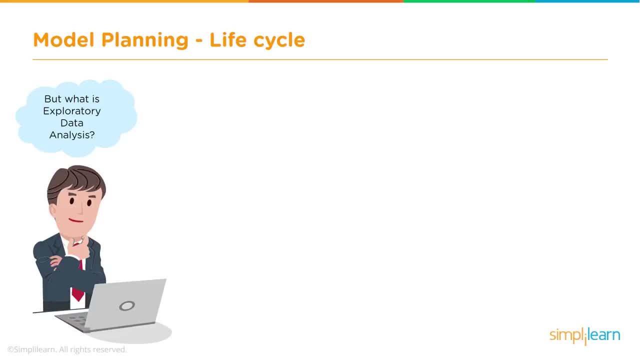 So little bit of details about exploratory data analysis. So what exactly is exploratory data? analysis is basically to, as the name suggests, you're just exploring. you just receive the data and you're trying to explore and find out what are the data types and what is the. is the data clean in each of the columns? 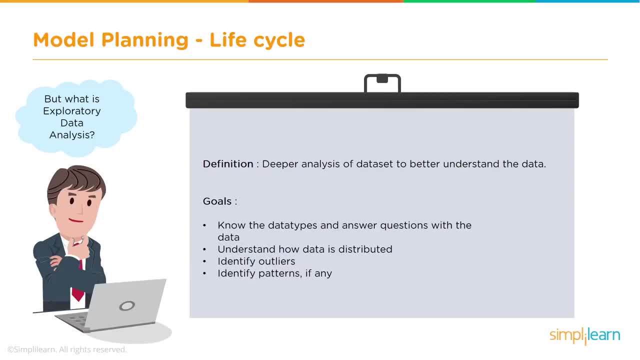 What is the maximum minimum value? So, for example, there are out of the box functionality available in tools like R. If you just ask for a summary of the table, it will tell you for each column, it will give some details as to what is the mean value, what is the maximum value, and so on and so 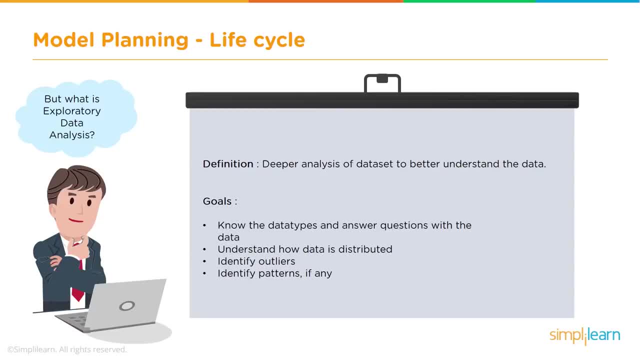 forth. So this exercise, or this exploratory analysis, is to get an understanding of your data. then you can take steps to. during this process you find there are a lot of missing values. you need to take steps to fix those. you will also get an idea about what kind of model. 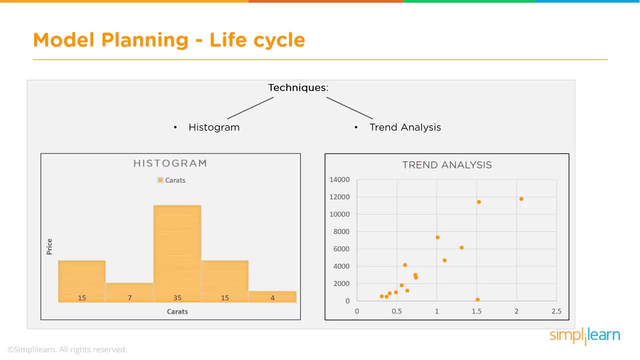 to be used, and so on and so forth. what are the various techniques used for exploratory data analysis? typically, these would be visualization techniques. like you use histograms, you can use box plots, you can use scatter plots, so these are very quick ways of identifying the patterns or a few of the trends of the data, and so on. and then, once your data is ready, 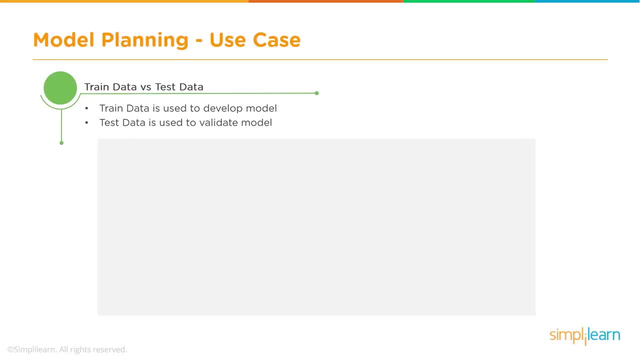 you. you decided on the model, what kind of model, what kind of algorithm you're going to use. if you're trying to do machine learning, you need to pass your 80 percent the training data, or rather, you use that training data to train your model and the training process. 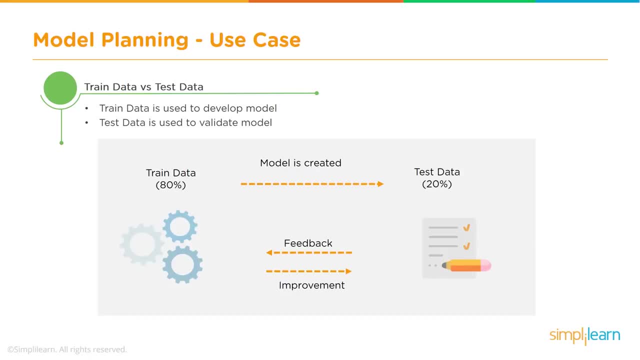 itself is iterative, so the training process you may have to perform multiple times. and once the training is done, Done and you feel it is giving good accuracy, then you move on to test. so you take the remaining 20 percent of the data. remember, we split the data into training and test, so the test data 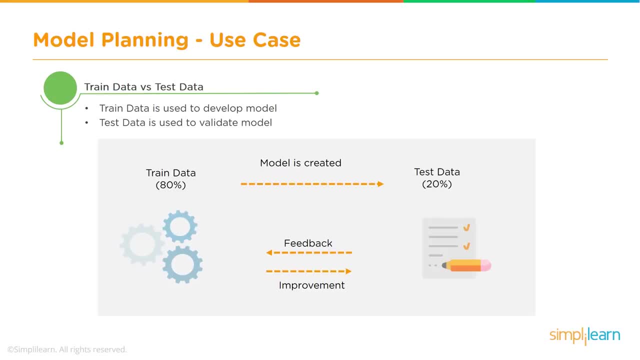 is now used to check the accuracy or how well our model is performing and if there are further issues. let's say, model is still during testing. if the accuracy is not good, then you may want to retrain your model or use a different model. So this is the first step. 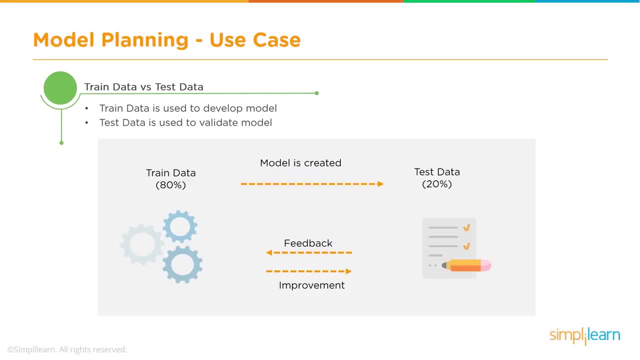 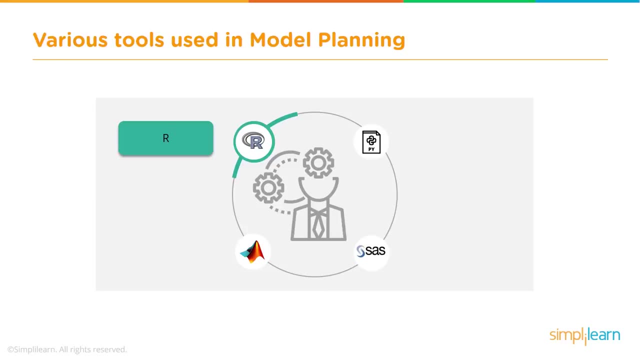 This whole thing again can be iterative, but if the test process is passed, or if the model passes the test, then it can go into production and it will be deployed. all right. so what are the various tools that we use for model planning? R is an excellent tool in a lot of 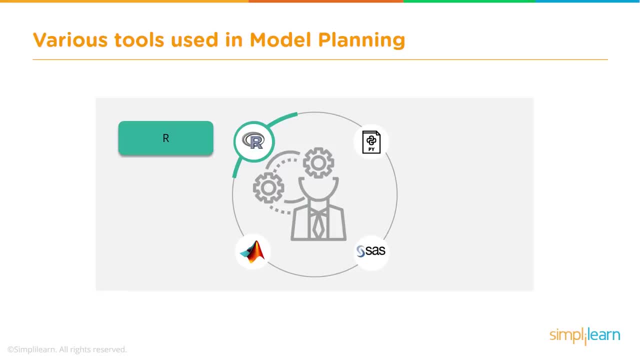 ways, whether you're doing regular statistical analysis or machine learning or any of these activities are in. along with R, studio provides a very powerful environment to do data analysis, including visualization. it has a very good integrated visualization or plot mechanism which can be used for doing exploratory data analysis and then later on to do analysis. 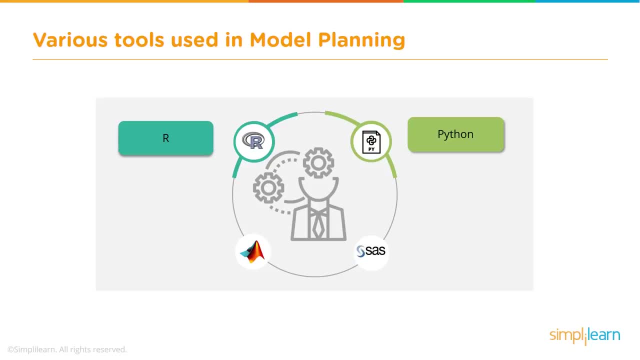 detailed analysis and machine learning, and so on and so forth. then, of course, you can write python programs. python offers a rich library for performing data analysis and machine learning, and so on. MATLAB is a very popular tool as well, especially during education, so this is a very popular tool. 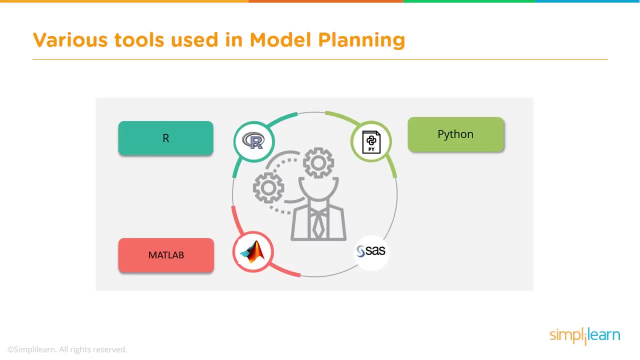 This is a very easy to learn tool, so MATLAB is another tool that can be used. and then, last but not least, SAS. SAS is again very powerful. it is a preparatory tool and it has all the components that are required to perform very good statistical analysis or perform data. 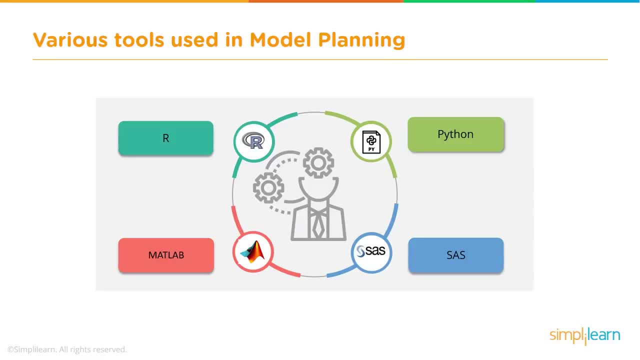 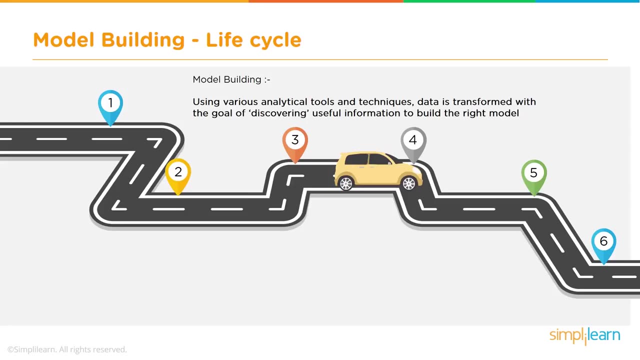 science. so those are the various tools that would be required for, or that that can be used for, model building, and so the next step is model building. So we have done the planning part. we said, okay, what is the algorithm we are going to use, what kind of model we are going to use. now we need to actually train this model, or 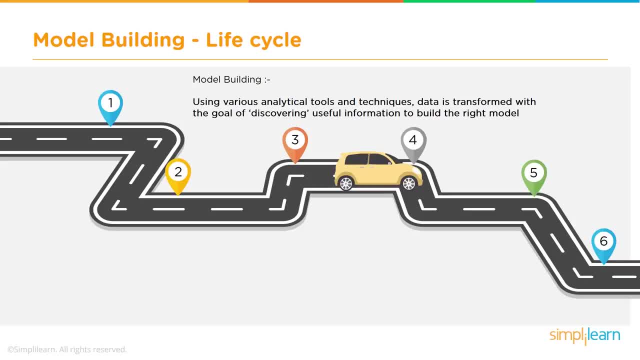 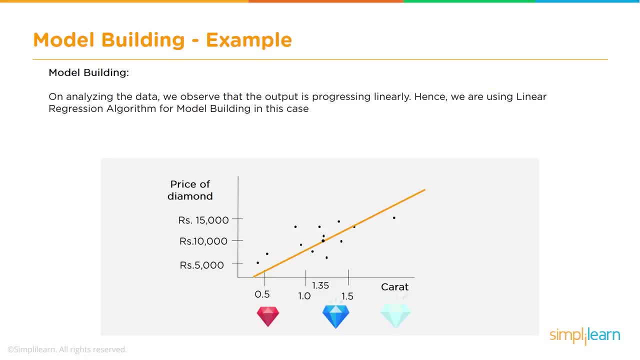 build the model, rather so that it can then be deployed. So what are the various ways, or what are the various types of model building activities? so it could be, let's say, in this particular example that we have taken, you want to find out the price of 1.35 carat diamond. 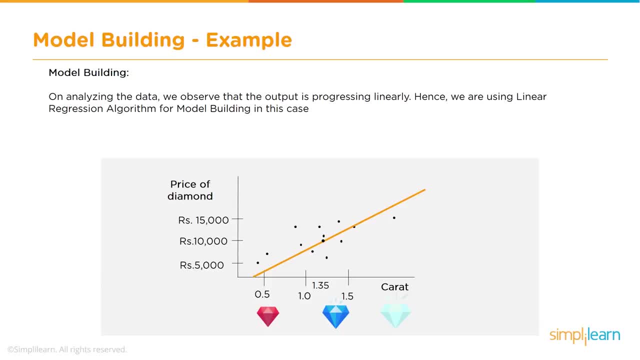 So this is, let's say, a linear regression Regression problem. you have data for various carats of diamond and you use that information, you pass it through a linear regression model or you create a real linear regression model which can then predict your price for 1.35 carat. 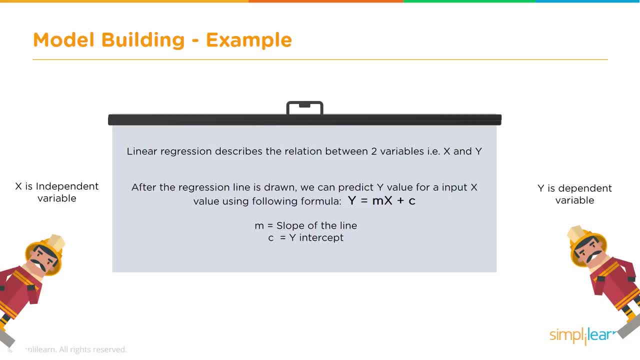 So this is one example of model building and then little bit details of how linear regression works. So linear regression is basically coming up with a relation Relation between an independent variable and a dependent variable. So it is pretty much like coming up with equation of a straight line which is the best fit for. 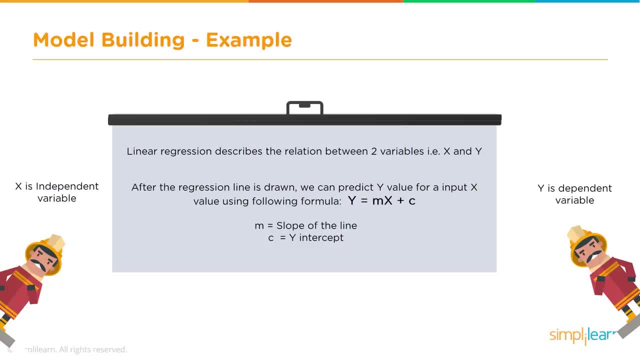 the given data. So like for example here: y is equal to mx plus c, so y is the dependent variable and x is the independent variable. we need to determine the values of m and c for our given data. So that is what the training process of this model does. 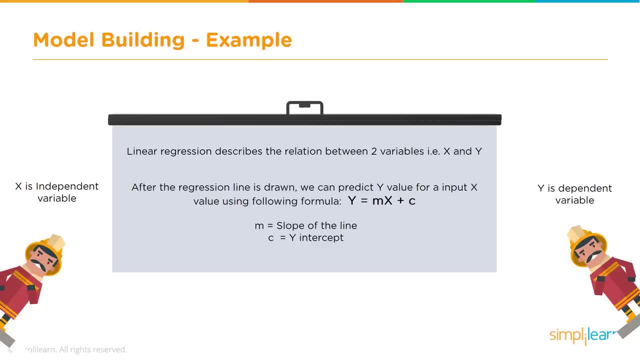 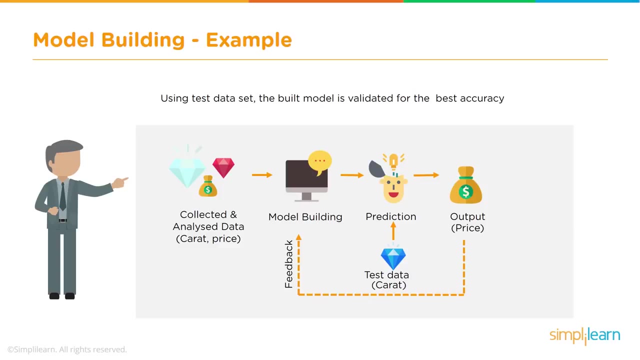 At the end of the training process you have a certain value of m and c and that is used for predicting the values of any new data. that comes Alright. so the way it works is: we use the training and the test data set to train the model and then validate whether the model is working fine or not using test data and 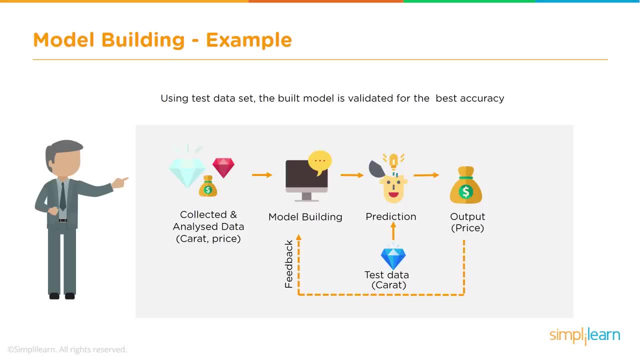 if it is working fine, then it is taken to the next level, which is put in progress In production. if not, the model has to be retrained. if the accuracy is not good enough, then the model is retrained, maybe with more data, or you come up with a newer model or algorithm. 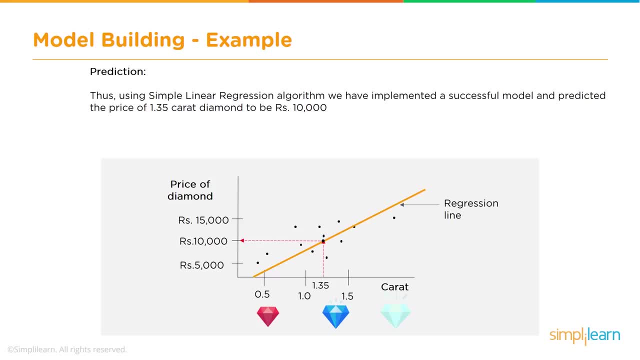 and then repeat the process. So it is an iterative process. Once the training is completed- training and test- then this model is deployed and we can use this particular model to determine what is the price of 1.35 carat diamond. Remember that was our problem statement. 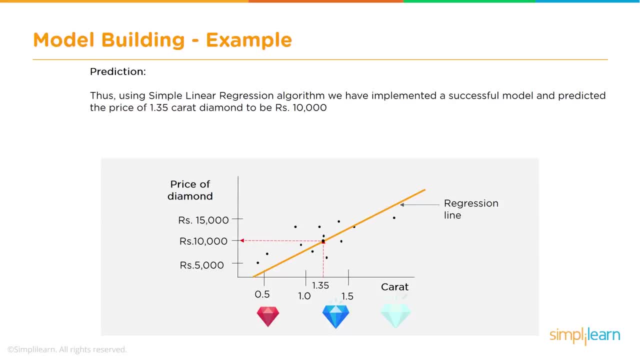 So, now that we have the best fit for this given data, we have the price of 1.35 carat diamond, which is 10,000.. So this is one example of how this whole process works. Now how do we build the model? 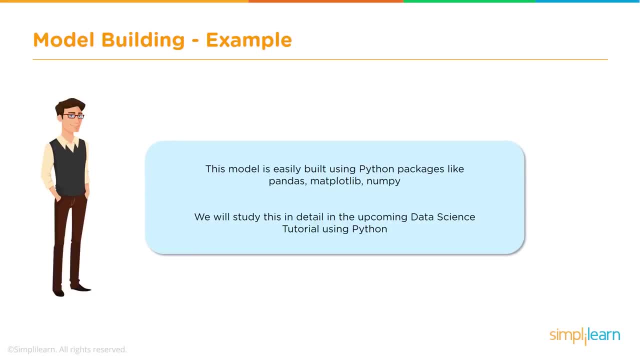 There are multiple ways. You can use Python, for example, and use libraries like pandas or numpy to build the model and implement it. This will be available as a separate tutorial, a separate video in this playlist. Thank you for watching, So stay tuned for that. 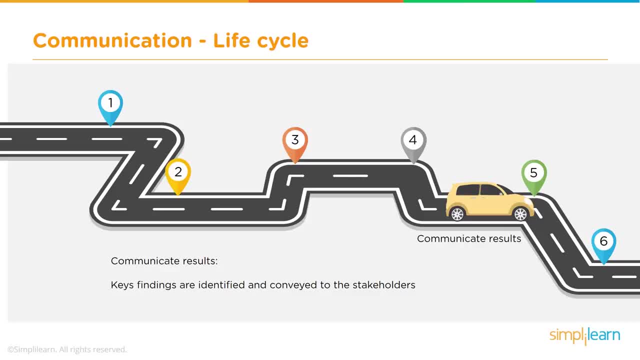 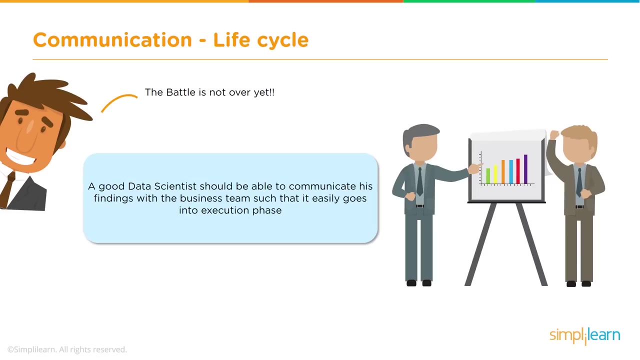 Moving on. once we have the results, the next step is to communicate these results to the appropriate stakeholders. So it is basically taking these results and preparing like a presentation or a dashboard and communicating these results to the concerned people. So finishing or getting the results of the analysis is not the last step, but you need. 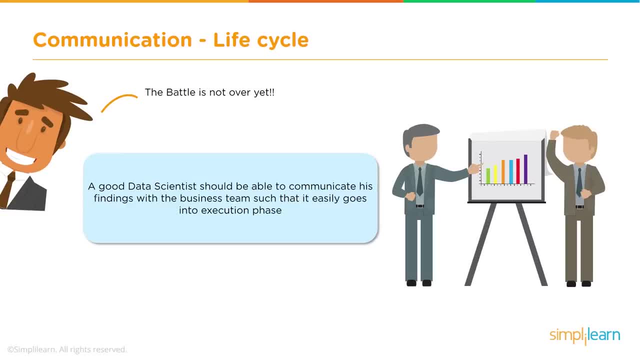 to, as a data scientist, take these results and present them to the appropriate stakeholders, And present it to the team that has given you this problem in the first place and explain your findings, explain the findings of this exercise and recommend, maybe, what steps they need to take in order to overcome this problem or solve this problem. 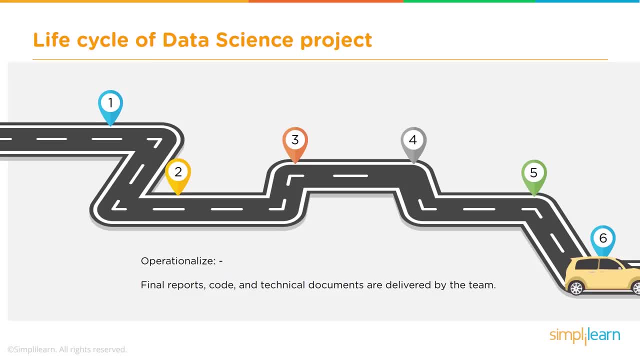 So that is the pretty much once that is accepted, and the last step is to operationalize. So if everything is fine, your data scientist presentations are accepted, then they put it into practice And thereby they will be able to improve or solve the problem that they stated in step. 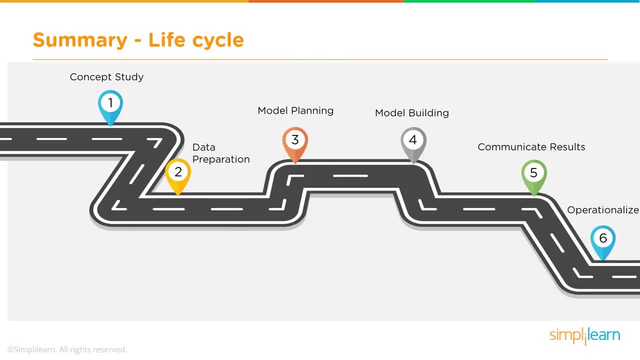 one. Okay, so quick- summary of the lifecycle. you have a concept study which is basically understanding the problem, asking the right questions and trying to see if there is enough data to solve this problem And then even maybe gather the data. then data preparation, the raw data, needs to be. 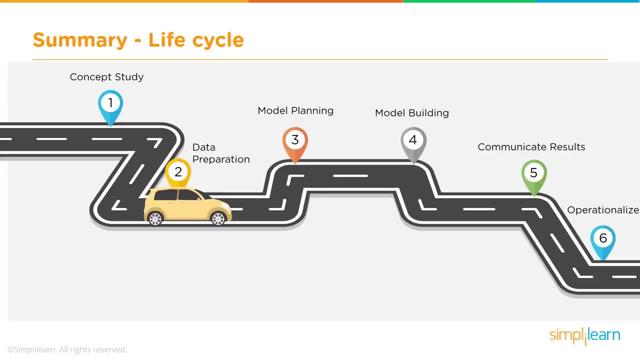 manipulated. you need to do data munging so that you have the data in a certain proper format to be used by the model or our analytics system, And then you need to do the model planning: what kind of a model, what algorithm you will. 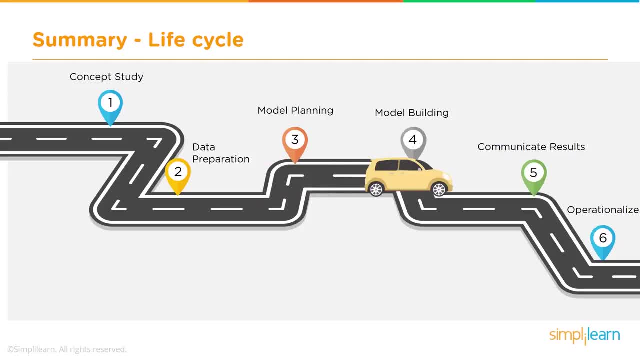 use for a given problem and then the model building. So the exact execution of that model happens in step four and you implement and execute that model and put the data through the analysis in this step And then you get the results. these results are then communicated, packaged and presented. 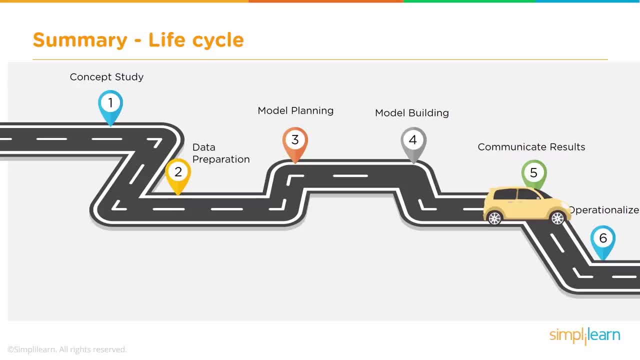 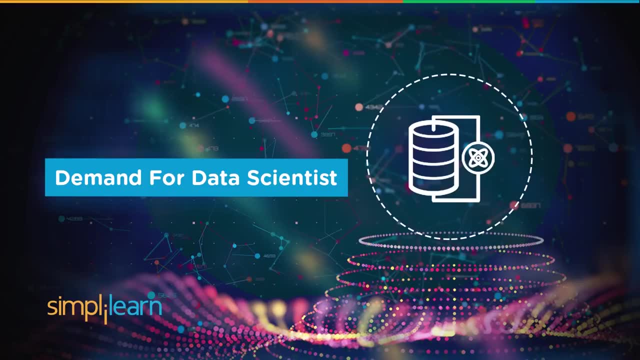 and communicated. Okay, They are communicated to the stakeholders and once that is accepted, that is operationalized. So that is the final step. Now, in the end, let's take a quick look at the demand for data scientists. Data science is an area of great demand. 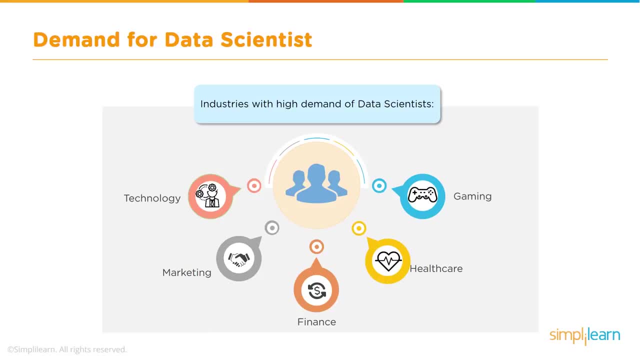 The demand for data scientists is currently huge and the supply is very low, so there is a huge gap. So what are some of the industries with high demand for data scientists? I think gaming is definitely one area Where it's an industry which is consumer facing industry and a lot of people play. 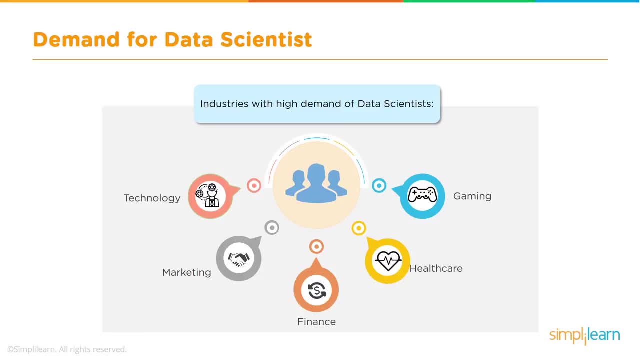 games and growing industry, and it requires a lot of data science, So that is an area where data scientists are in demand. Then we have healthcare, For example. data science is used for diagnosis and several other activities within healthcare, predicting, for example, a disease. 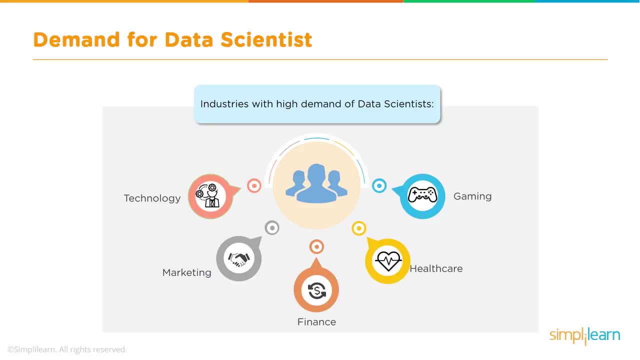 So healthcare is definitely, finance definitely banks, insurance companies- all of these. there is a huge demand. There is a huge demand for data scientists. Marketing is like a horizontal functionality across all industries. There's a demand for data scientists there. Then, of course, in technology area, 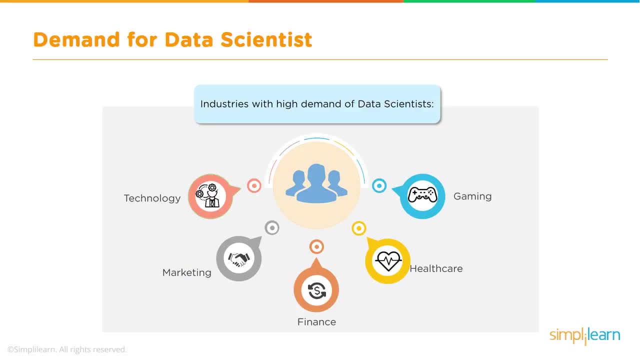 So pretty much all of these areas. there is a lot of demand. globally there is a huge demand, So this is a very, very critical skill that would be required currently as well as in the future. Let's take a look at what are the various techniques that are used for data cleaning. 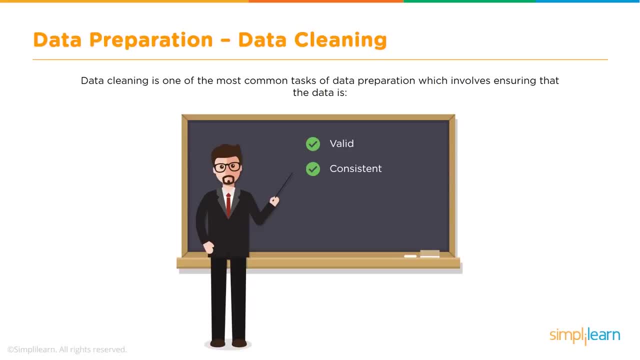 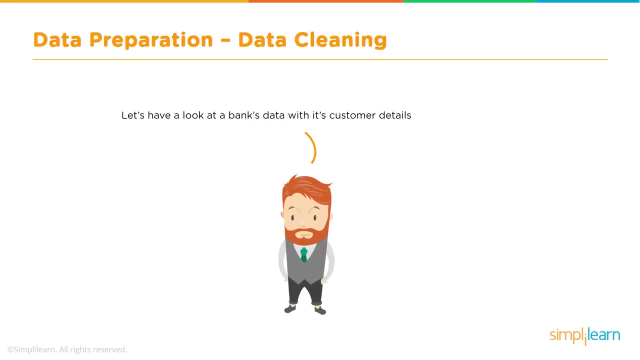 So we need to ensure that the data is valid, Okay, And it is consistent and uniform and accurate. So these are the various parameters that we need to ensure as a part of the data cleaning process. Now, what are the techniques that that are used for data cleaning? or so we will see what. 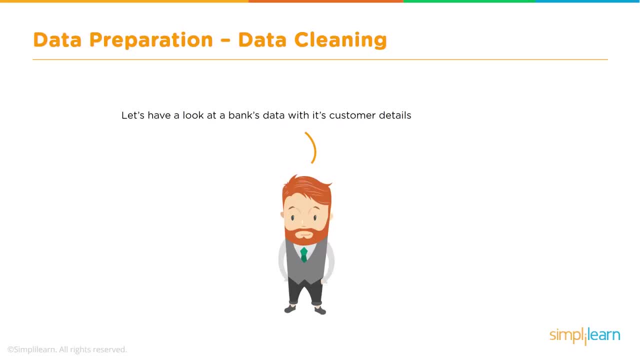 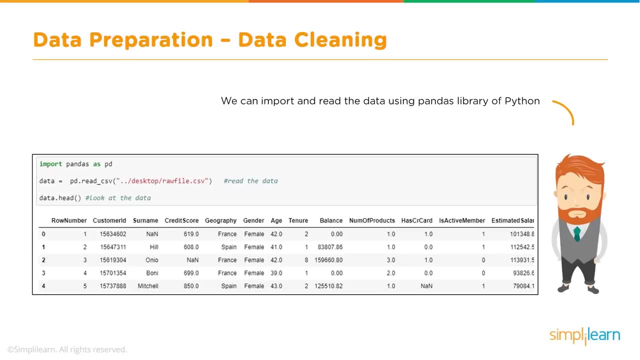 each of these are in this particular case, And so what is the data set that we have? We have data about a bank and its customer details, So let's take an example and see how we go about cleaning the data, And in this particular example, we're assuming we are using Python. 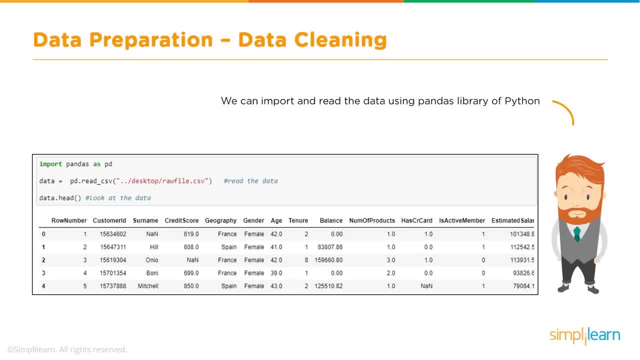 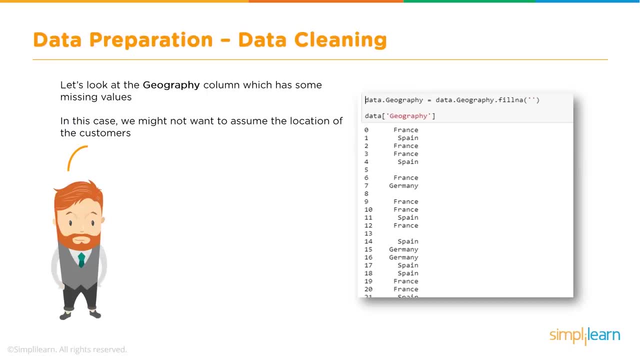 So let's assume we loaded this data, which is the raw file dot CSV. This is how the customer data looks like And we will see. for example, we take a closer look at the geography column, We will see that there are quite a few blank spaces. 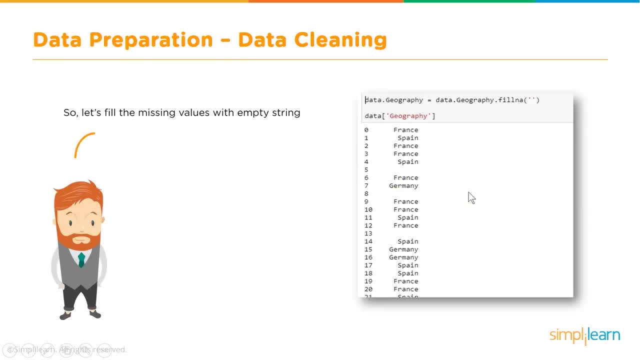 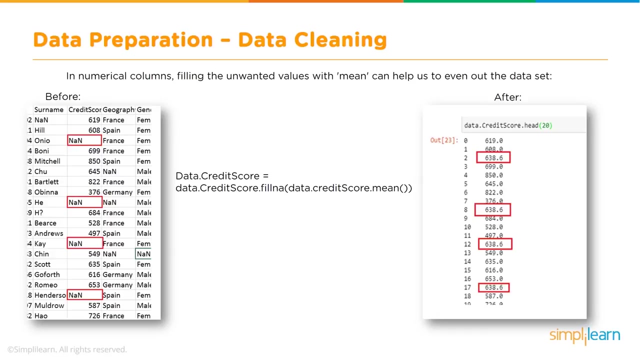 So how do we go about? when we have some blank spaces? or if it is a string value, Then we put a empty string here, or we just use a space or empty string. If they are numerical values, then we need to come up with a strategy. 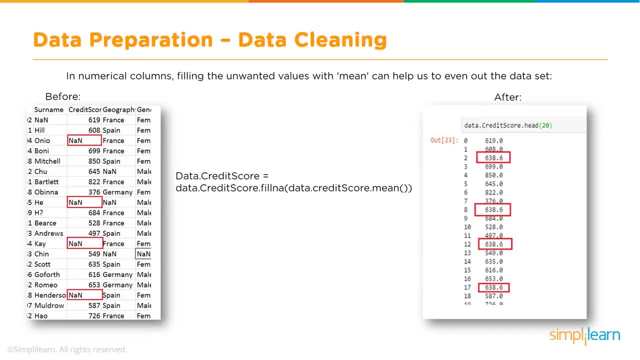 For example, we put the mean value. So wherever it is missing we find the mean for that particular column. So in this case, let's assume we have credit score and we see that quite a few of these values are missing. So what do we do here? 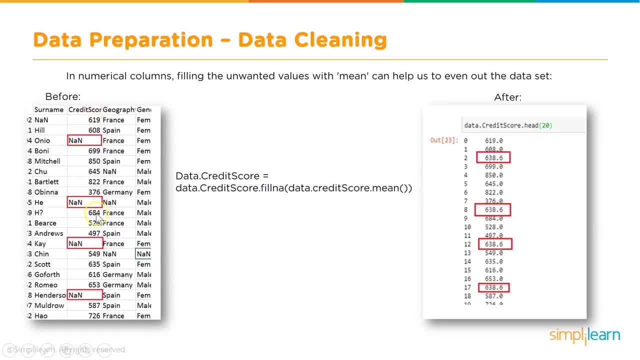 We find the mean. Okay, So this column for all the existing values and we found that the mean is equal to 638.6.. So we kind of write a piece of code to replace wherever there are blank values. NAN is basically like null and we just go ahead and say: fill it with the mean value. 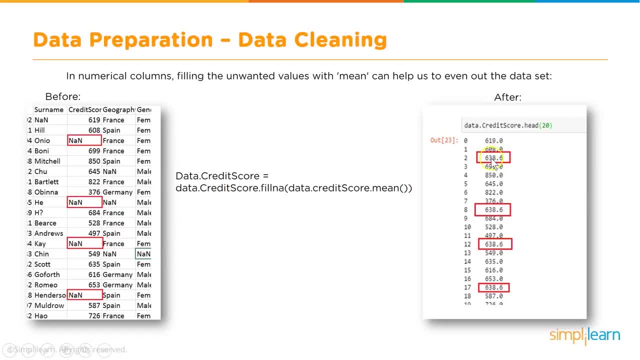 So this is a piece of code we are writing to fill it, So all the blanks or all the null values get replaced with the mean value. Now, one of the reasons for doing this is that very often, if you have some such situation, many of your statistical 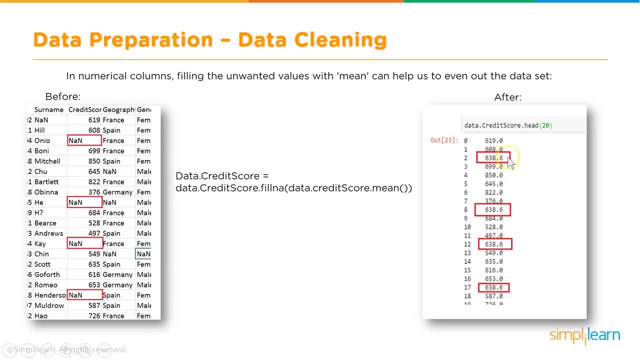 Functions may not even work. So that's the reason you need to fill up these values, or either get rid of these records or fill up these values with something meaningful. So this is one mechanism which is basically using a mean. There are a few others. 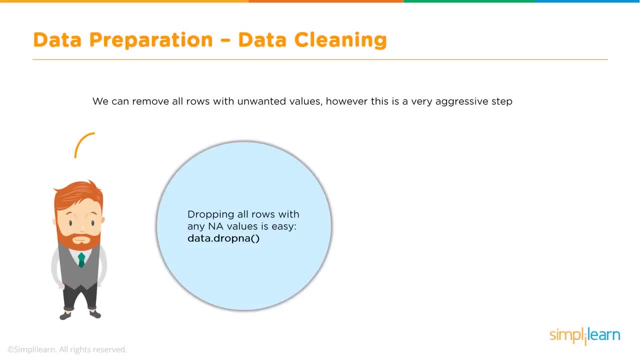 As we move forward we can see what are the other ways. for example, we can also say that any missing value in a particular row, even one column, the value is missing. You just drop that particular row or delete all rows where even a single column has missing. 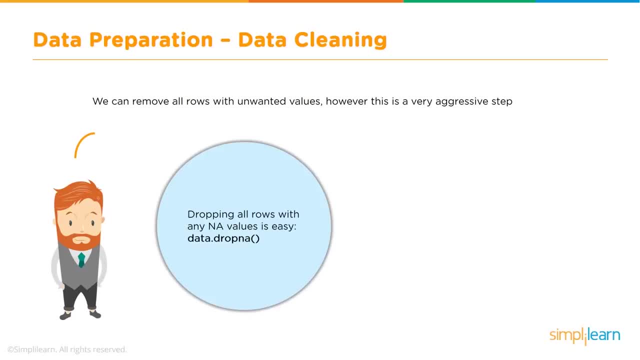 So that is one way of dealing. Now, the problem here can be that if a lot of data has, let's say, one or two columns missing and we drop many such rows, then overall you may lose out on, let's say, 60% of the. 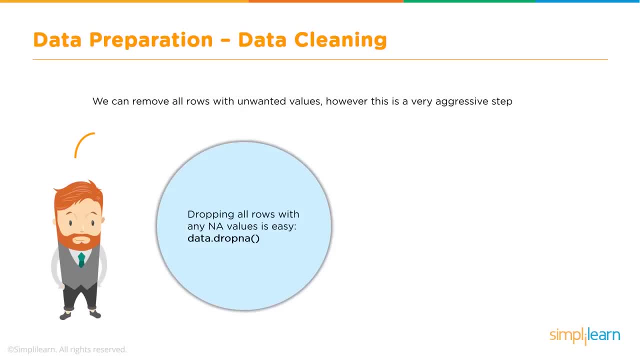 data has some value or the other, missing 60% of the rows, then it may not be a good idea to delete all the rows in that manner, because then you're losing pretty much 60% of your data. Therefore your analysis won't be accurate. 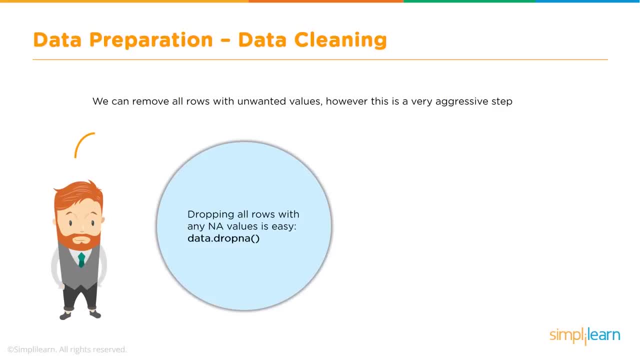 But If it is only 5 or 10%, then this will work. Another way is only to drop values where, or rather drop rows where all the columns are empty, which makes sense, because that means that record is of really no use, because it. 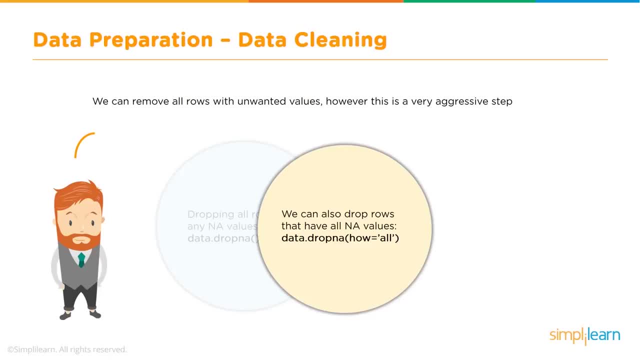 has no information in it. So there can be some situations like that. So we can provide a condition saying that drop the records where all the columns are blank or not applicable. We can also specify some kind of a threshold. Let's say you have 10 or 20 columns. 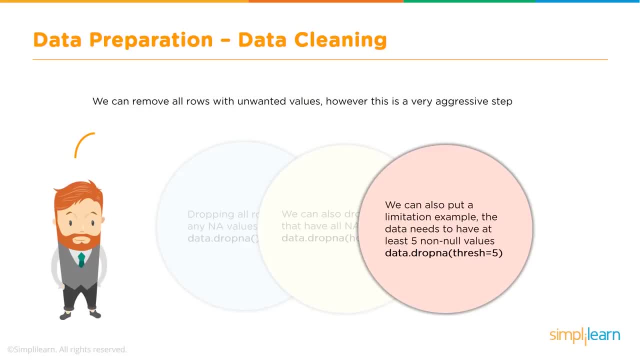 In a row you can specify that maybe five columns are blank or null, Then you drop that record. So again, we need to take care that such a condition, such a situation, the amount of data that has been removed or excluded, is not large. 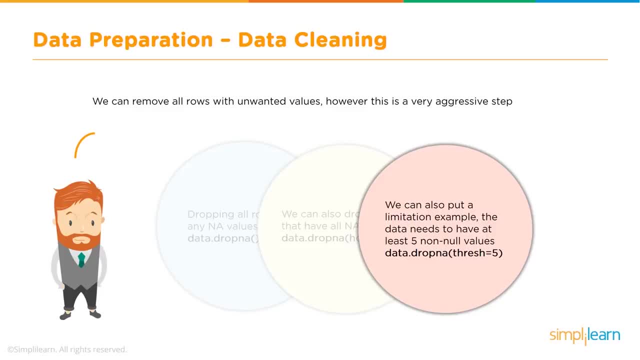 If it is like maybe 5%, maximum 10%, then it's okay. But by doing this, if you're losing out on a large chunk of data, then it may not be a good idea. You need to come up with something better. 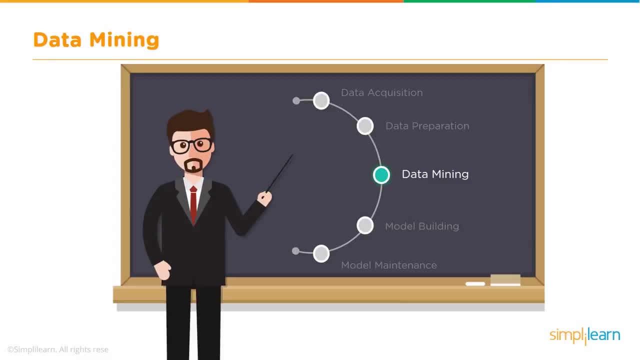 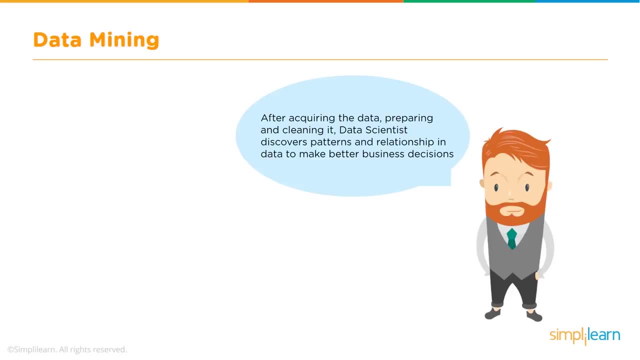 What else we need to do next is the data preparation part is done, So now we get into the data mining part. So what exactly we do in data mining? primarily, we come up with ways to take meaningful decisions. So data mining will give us insights into the data, what is existing there, and then 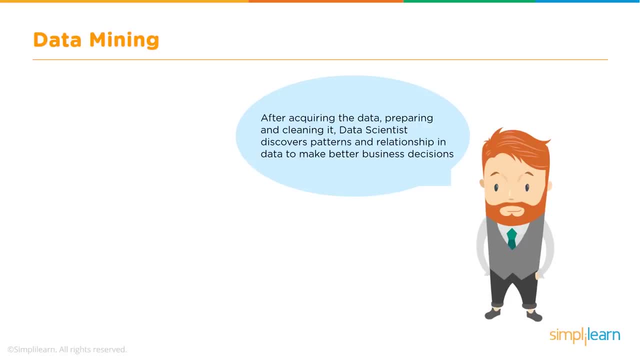 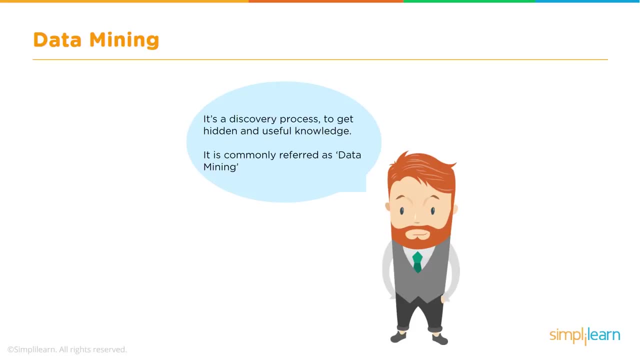 we can do additional stuff, like maybe machine learning and so on, to perform advanced analytics and so on. So one of the first steps we do is what is known as data discovery, which is basically like exploratory analysis. So we can use tools like Tableau for doing some of this. 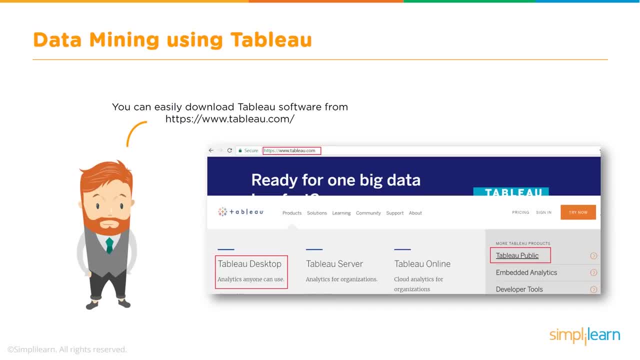 So let's just take a quick look at how we go about that. So Tableau is excellent data mining, or actually more of a reporting or a BI tool, And you can download a trial version of Tableau at tableaucom or there is also Tableau public. 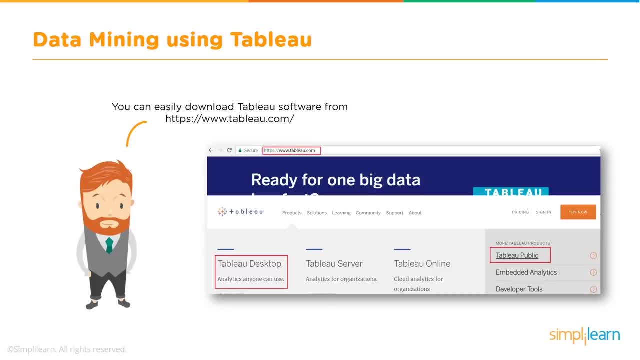 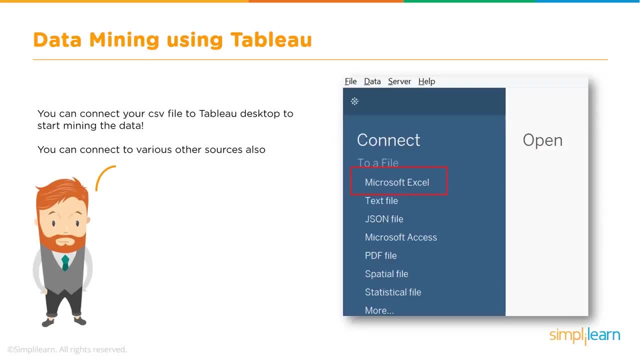 which is free and you can actually use and play around. However, if you want to use it for enterprise purpose, Then it is a commercial software, so you need to purchase license and you can then run some of the data mining activities, Say your data source. your data is in some Excel sheet so you can select the source. 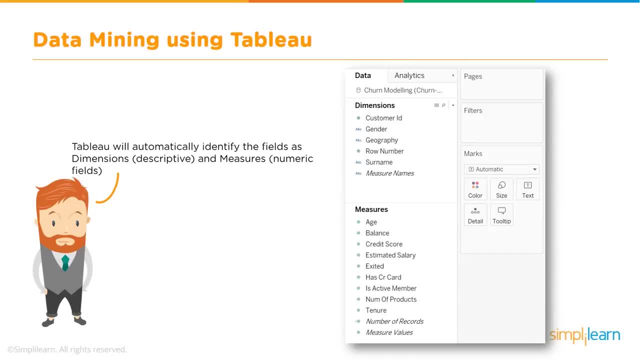 as Microsoft Excel or any other format, and the data will be brought into the Tableau environment and then it will show you what is known as dimensions and measures. So dimensions are all the descriptive columns, So, and Tableau is intelligent enough To actually identify these dimensions and measure. 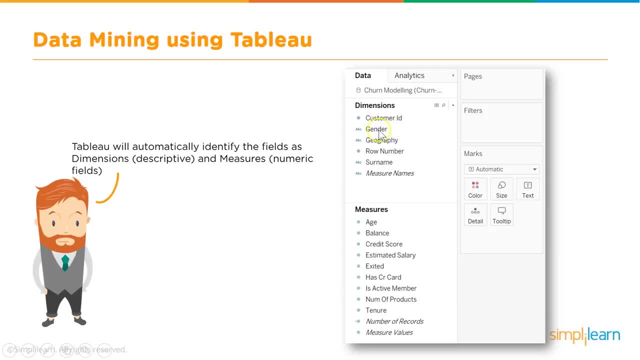 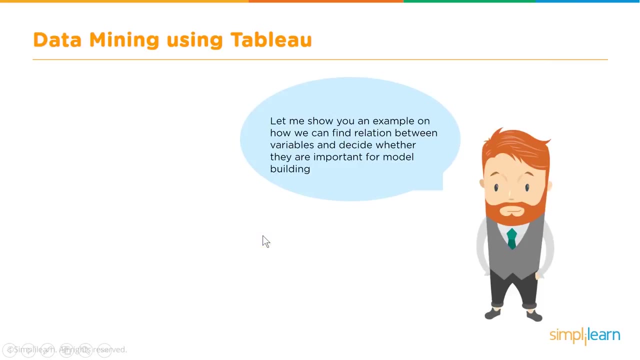 So measures are the numerical values. So, as you can see here, customer ID, gender, geography- these are all dimensions, non numerical values, whereas age, balance, credit score and so on are numeric values, So they come under measures. So you've got your data into Tableau and then you want to, let's say, build a small model. 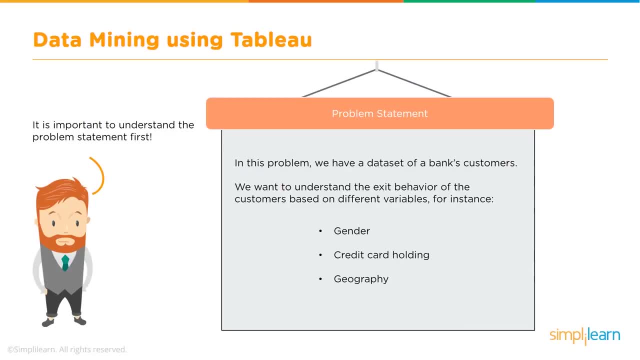 and you want to, let's say, solve a particular problem. So what is the problem statement? All right, Let's say we want to analyze Why customers are leaving the bank, which is known as exit, And we want to analyze and see what are some of the factors for exiting the bank. 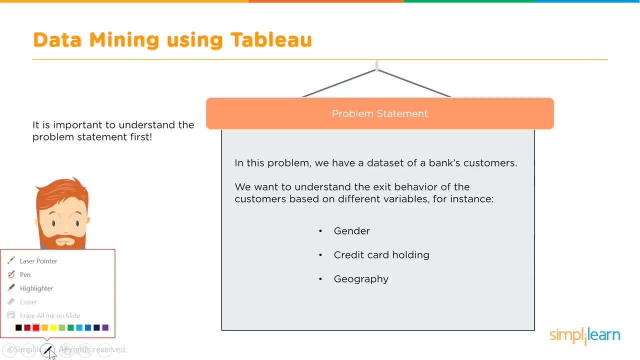 And we want to, let's assume, consider these three of them like, let's say, gender, credit card and geography- these as criteria and analyze if these are in any way impacting or have some bearing on the customer exiting or the customer exit behavior. 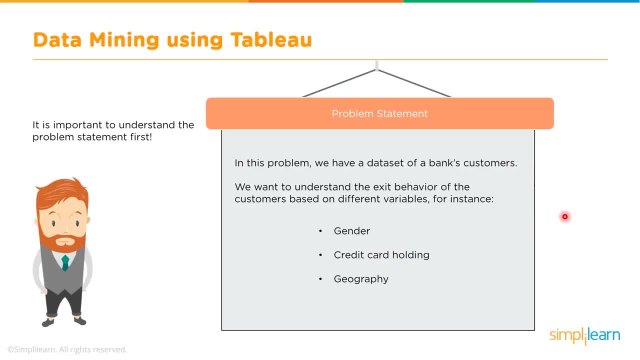 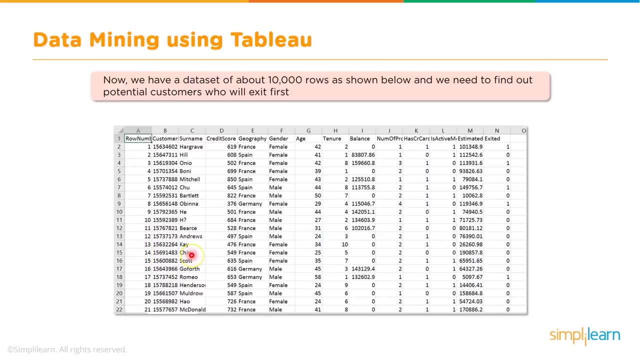 Okay, So we can use Tableau and very quickly we will be able to find out how these parameters are affecting All right, So let's see. So this is our customer data. So from our Excel sheet we have data set about, let's say, 10,000 rows and we want 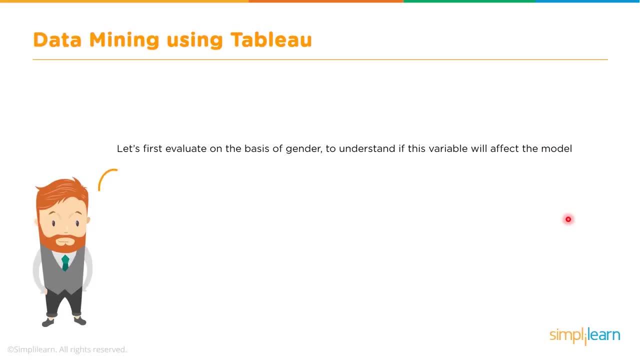 to find out what is the criteria. Let's start with gender. Let's say we want to first use gender as a criteria. So Tableau really offers an easy drag and drop kind of a mechanism. So that makes it really really easy to perform this criteria. 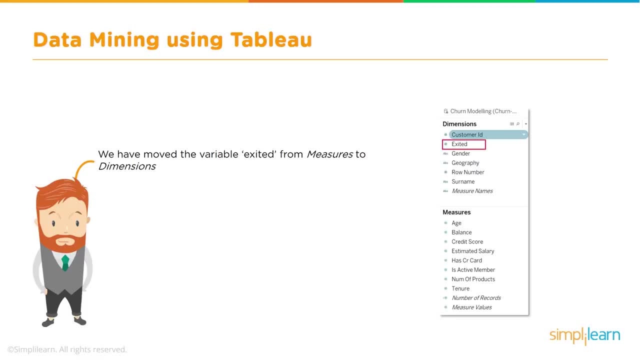 So what we need to do is exit. it says whether the customer has exited or not, So it has a value of zero and one, And then of course you have gender and so on. So we will take these two and simply drag and drop. 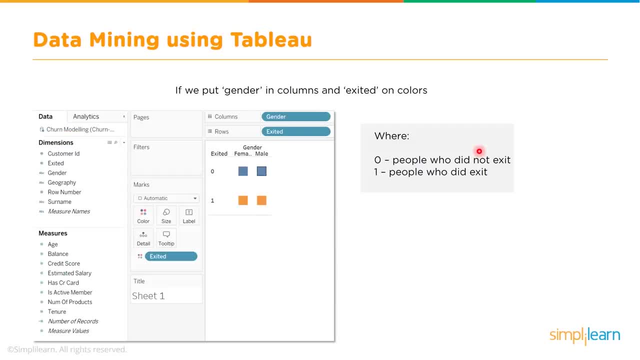 Okay, So exit it And then we will put gender And if we drag and drop into the analysis side of Tableau, all right. So here what we are doing is we are showing male, female as two different columns here and zero for people who did not exit. 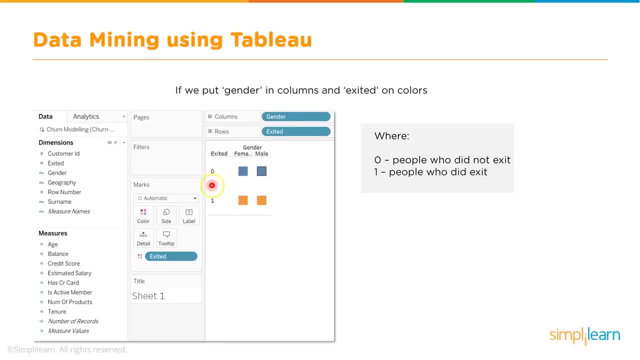 Okay, And one for people who exited, and that is color coded. So the blue color means people who did not exit and this yellow color means people who did exit. All right, So now if we pull the data here, create like bar graphs. this is how it would look. 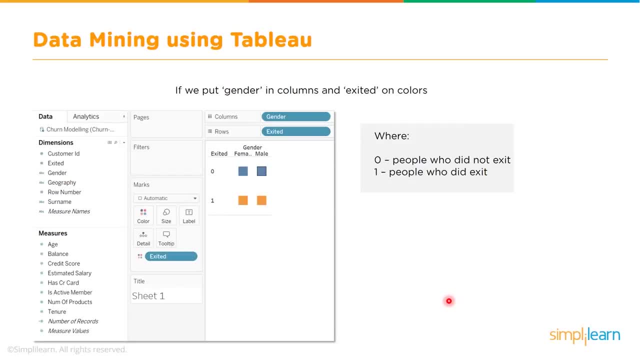 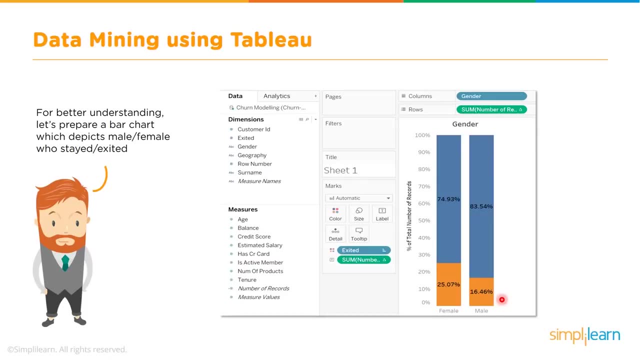 So what is yellow? Let's go back. So yellow is who exited, and for the male, only 16.45% have exited, And we can also draw a reference line that will help us So that you can create the reference line here. 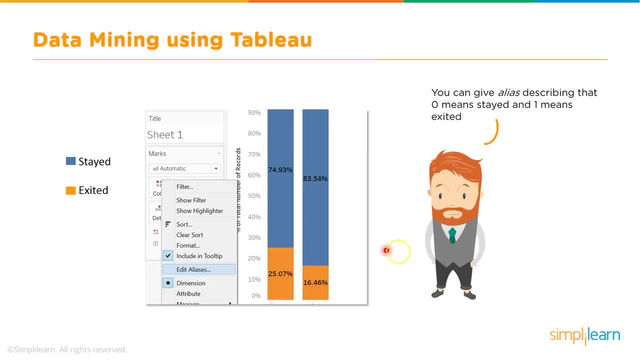 So you can see here: if you want to make reference lines as you go up, you are going to choose a reference line and you list this as the reference line. If you want to add the reference line as you go up, you can easily do so. 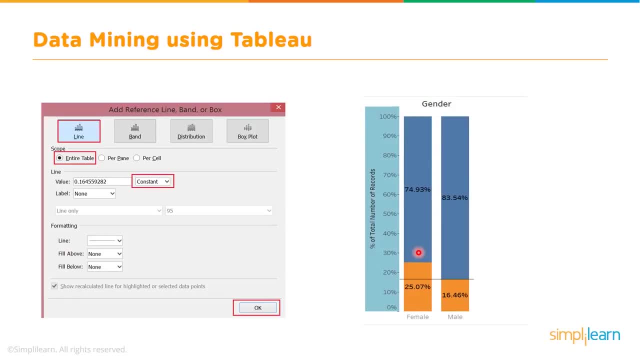 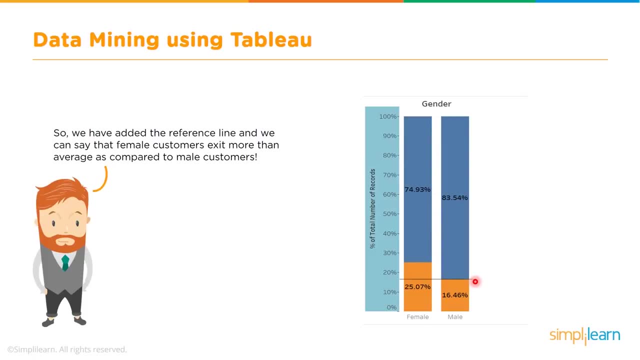 So you can create various reference lines or even provide aliases. So these are a lot of fancy stuff that is provided by Tableau. You can create aliases and so that it looks good rather than basic labels, And you can also add a reference line. 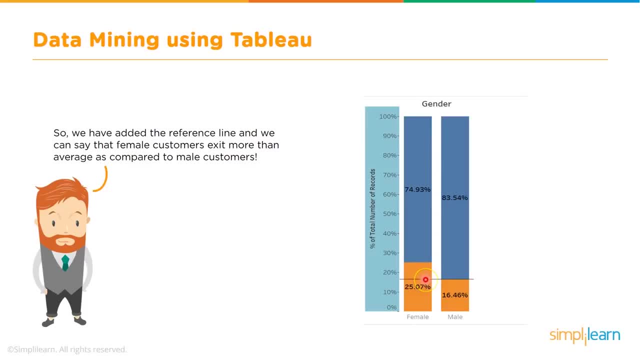 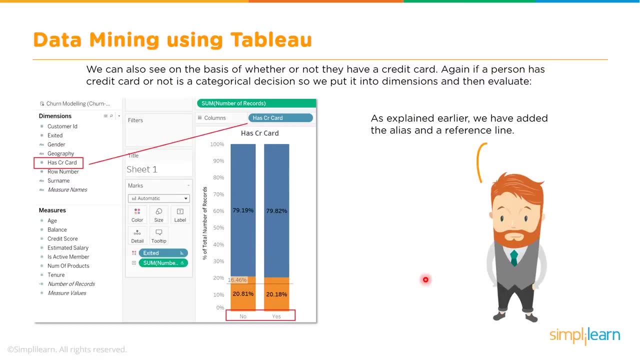 So you add a reference line, something like this: From here we can make out that, on an average, female customers exit more than the male customers. Right, see that there is some difference in the male and female behavior. now let's take the next criteria, which is the credit card. so let's see if having a credit 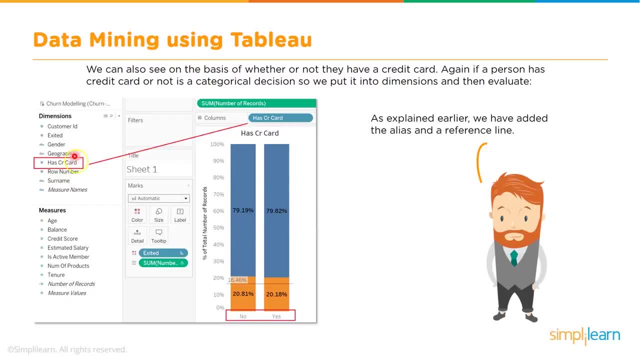 card has any impact on the customer exit behavior. so, just like before we drag and drop the credit card, has credit card a column. if we drag and drop here and then we will see that there is pretty much no difference between people having credit card and not having credit card. twenty point eight, one percent of people who 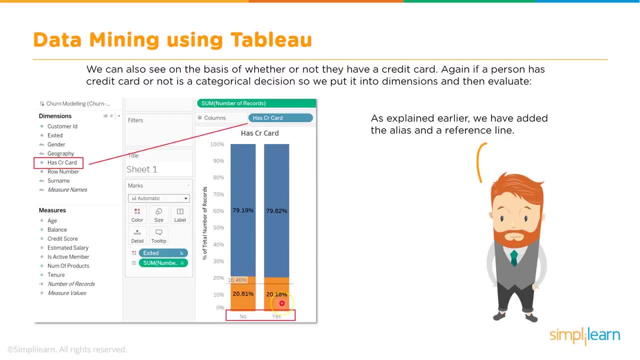 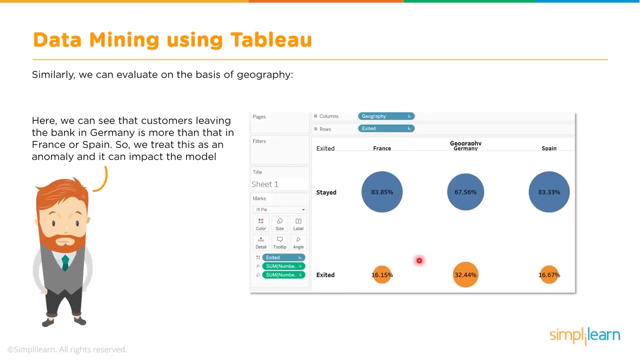 have no credit card have exited, and similarly, twenty point one eight percent of people who have credit card. I have also exited. so the credit card is not having much of an impact. that's what this piece of analysis shows. last. we will basically go and check how the geography is impacting. so once again, we 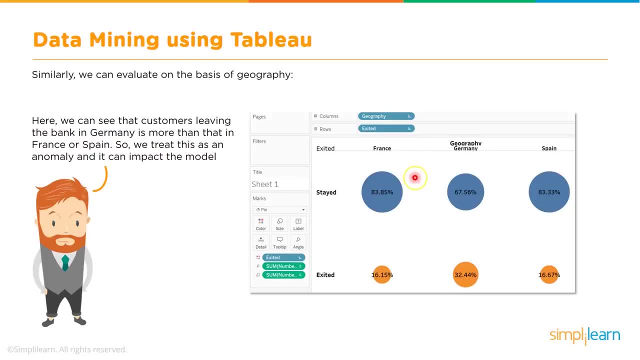 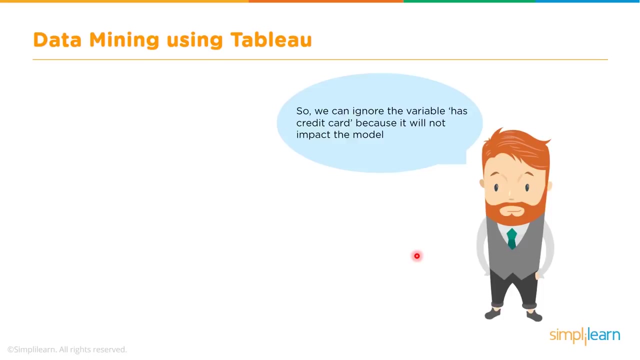 can drag and drop geography column onto this side and if we see here there are geographies like- I think there are about three geographies like france, germany and spain, and we see that there is some kind of impact with the geography as well. okay, so what we derive from this is that the credit card is really. we can ignore the credit. 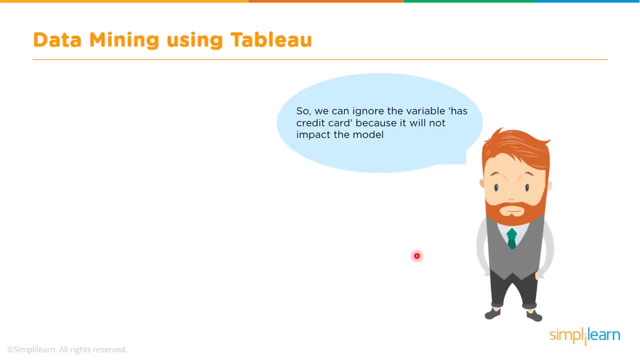 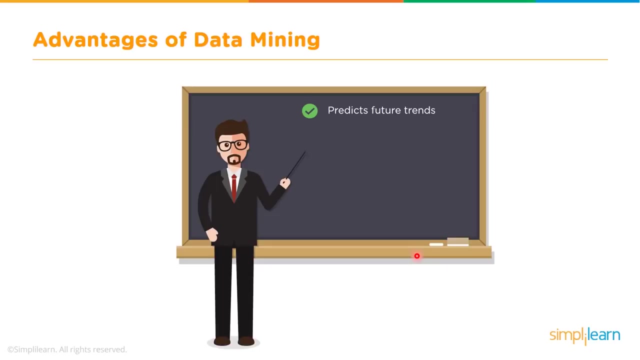 card, variable or feature from our analysis, because that doesn't have any impact but gender and geography. we can keep and do further analysis. okay, all right, so what are some of the advantages of data mining? bit more detailed analysis can help us in predicting the future trends and it also 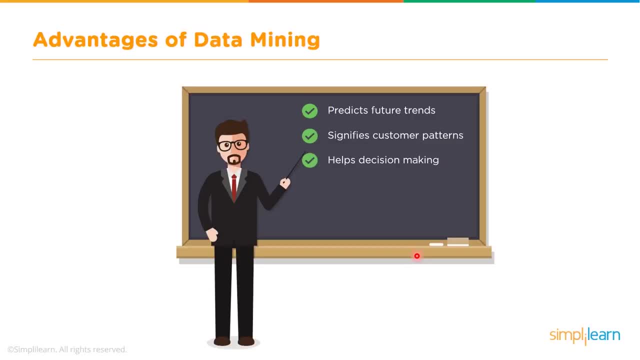 helps in identifying customer behavior patterns. okay, so you can take informed decisions, because the data is telling you or providing you with some insights, and then you take a decision based on that. if there is any fraudulent activity, data mining will help in quickly identifying such a fraud as well, and, of course, it will also help us in identifying the right algorithm. 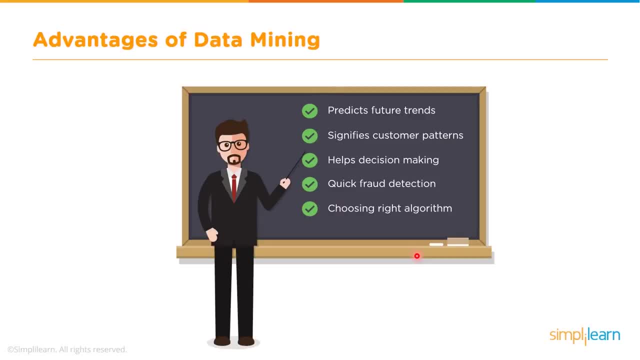 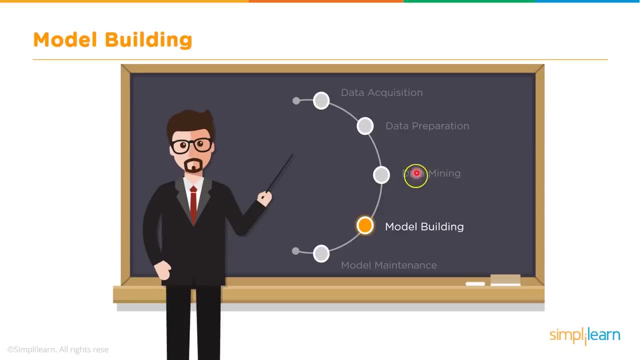 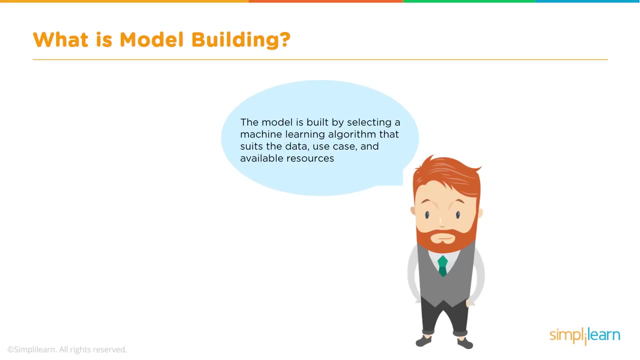 for performing more advanced data mining activities, like machine learning and so on. all right, so the next activity: now that we have the data, we have prepared the data and performed some data mining activity. the next step is model building. let's take a look at model building so. 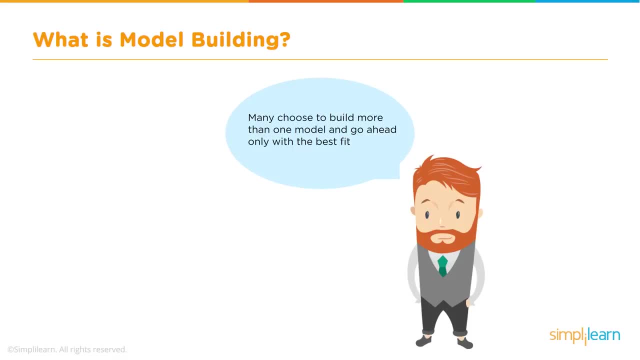 what is a model building? if we want to perform a more detailed data mining activity, like maybe perform some machine learning, then you need to build a model. and how do you build a model? first thing is you need to select which algorithm you want to use to solve the problem on hand, and 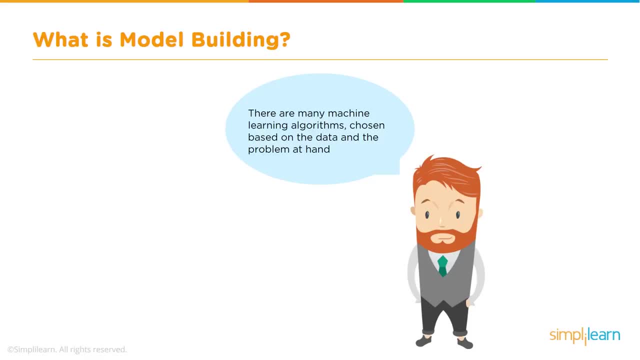 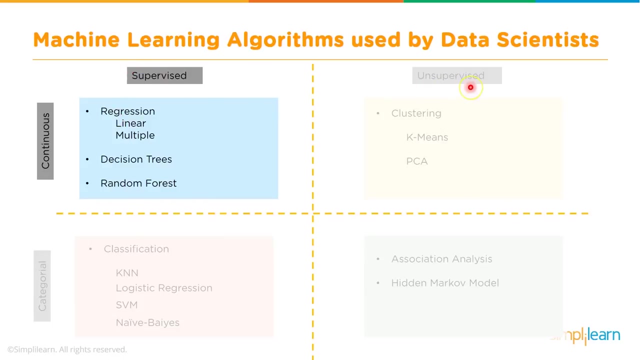 also what kind of data that is available, and so on and so forth. so you need to make a choice of the algorithm and based on that you go ahead and create a model, train the model and so on. now machine learning is kind of at a very high level, classified into supervised and unsupervised. so 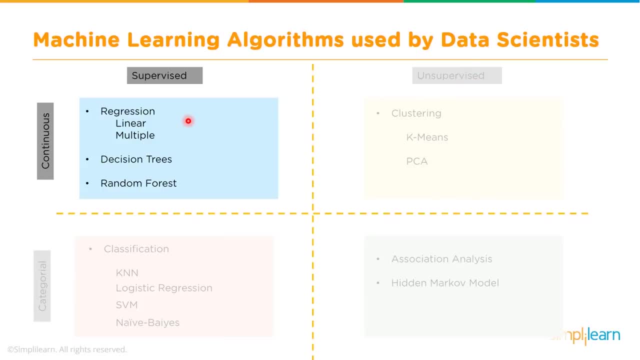 if we want to predict a continuous value, it could be a price or a temperature or or a height or a length or things like that. so those are continuous values, and if you want to find some of those, then you use techniques like regression, linear regression, simple linear regression, multiple linear regression, and so on. so these are the algorithms. 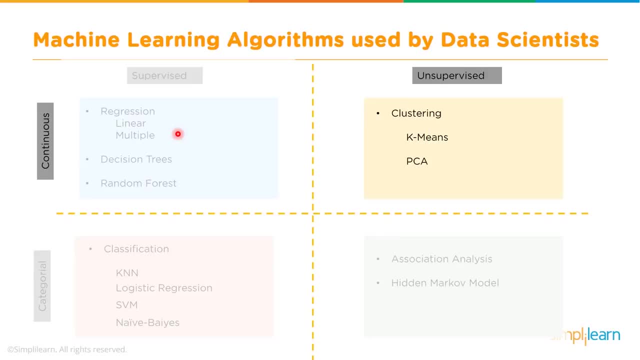 on the other hand, there will be situations, or there may be situations, where you need to perform unsupervised learning. case of unsupervised learning: you don't have any historical labeled data so to learn from. so that is when you use unsupervised learning and some of the algorithms in unsupervised learning are clustering. k-means clustering is 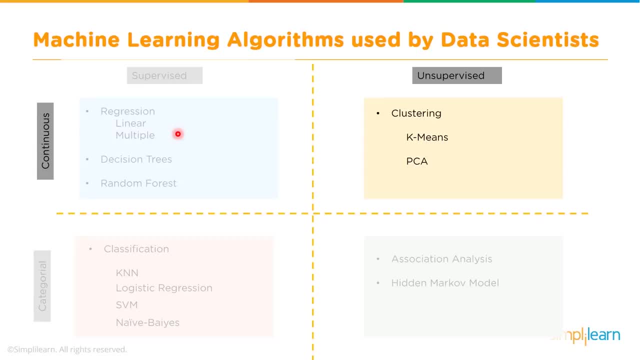 the most common algorithm used in unsupervised learning and similarly in supervised learning, if you want to perform some activity on categorical values like, for example, it is not measured but it is counted, like you want to classify whether this image is a cat or a dog, whether you want to 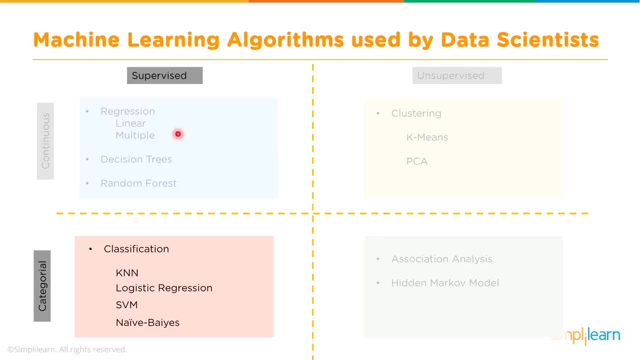 classify whether this customer will buy the product or not, or you want to classify whether this email spam or not spam. so these are examples of categorical values and these are examples of classification. then you have algorithms like logistic regression, k, nearest neighbor or knn and support vector machine. so these are some of the algorithms that are used in this case and similarly. 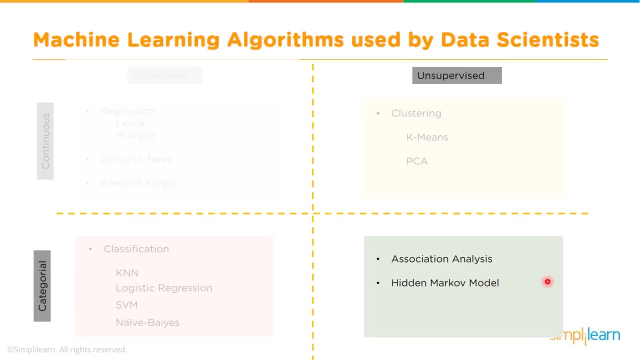 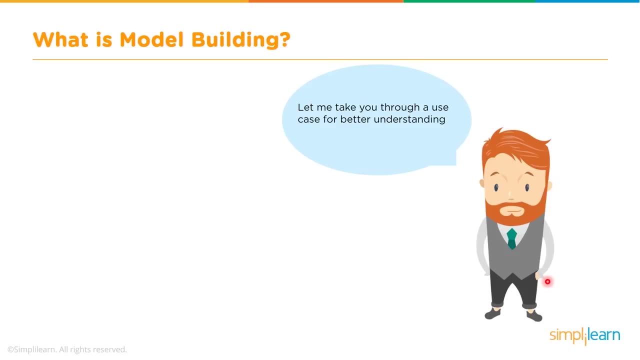 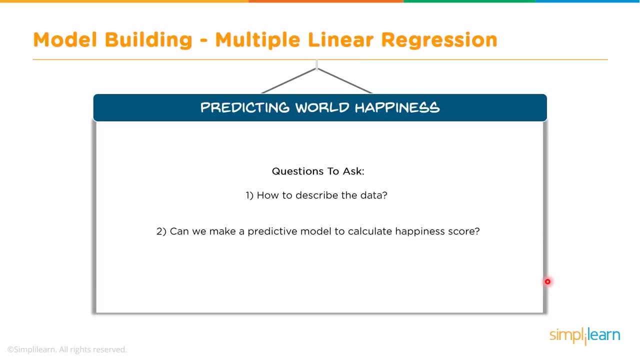 in case of unsupervised learning, if you need to perform on categorical values, you have some algorithms like association analysis and hidden marco model. okay, so in order to understand this better, let's take an example and take you through the whole process, and then we will also see how. 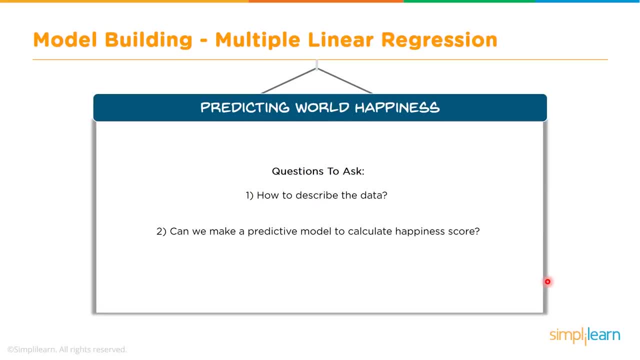 the code can be written to perform this. now let's take our example here, where we want to perform supervised learning, which is basically we want to do a multi-linear regression, which means there are multiple independent variables, and then we want to perform a linear regression to predict. 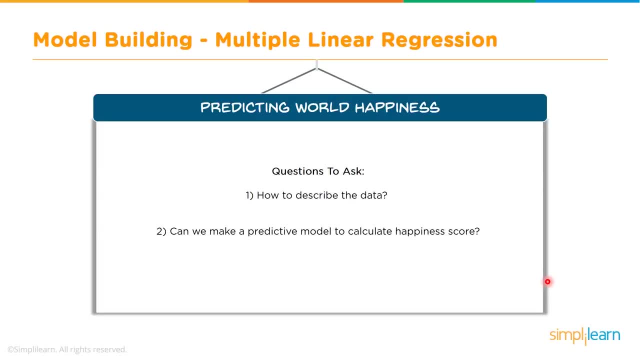 certain value. so in this particular example, we have world happiness data. so this is a data about the happiness quotient of people from various countries, and we are trying to predict and see whether our, how, our model will perform. so what is the question that we need to ask? first of all, how? 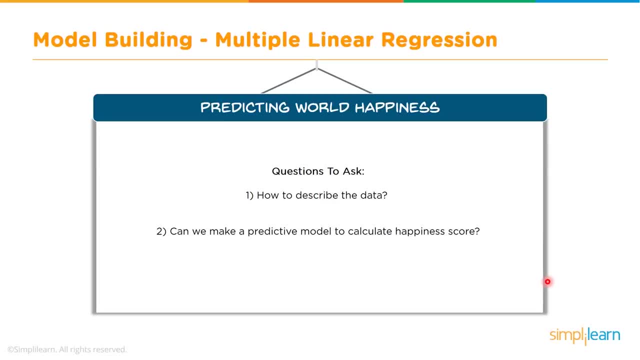 to describe the data and then can we make a predictive model to calculate the happiness score right? so based on this, we can then decide on what algorithm to use and what model to use, and so on. so variables that are available or used in this model: this is a list of variables. 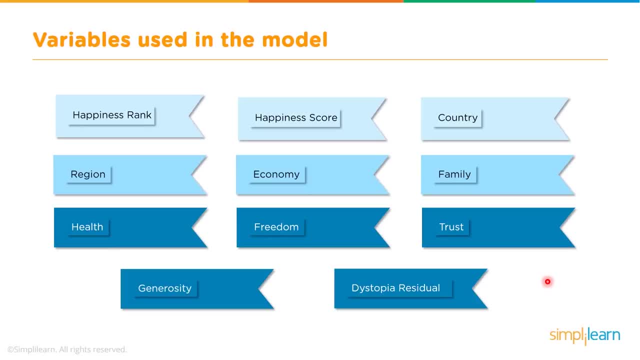 that are available. there is a happiness rank. i'll load the data and or i'll show you the data in a little bit so it becomes clear what are these. so there is what is known as a happiness rank, happiness score, which is happiness score is more like absolute value, whereas rank is: what is the ranking and then which country we are talking? 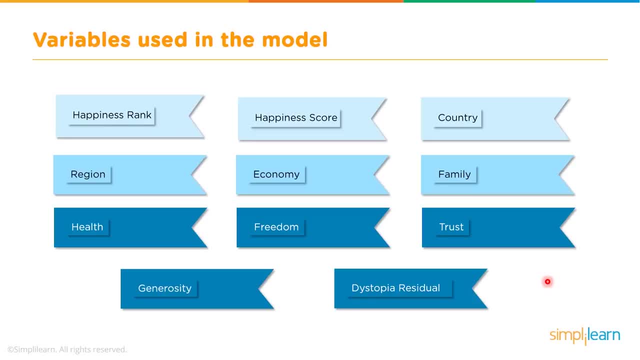 about and within that country, which region and what kind of economy, and whether the family, which family and health details and freedom, trust, generosity and so on and so forth. so there are multiple variables that are available to us and, uh, the specific details probably are not required and there can be um in another example, the 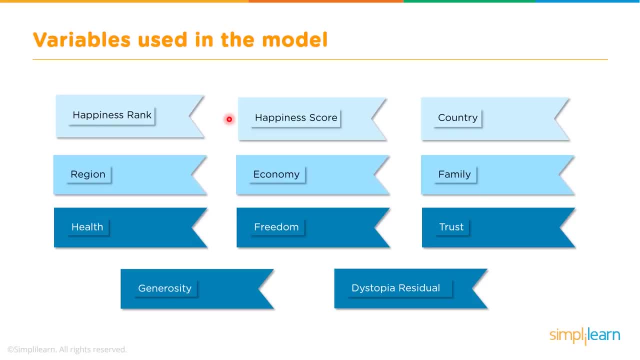 variables can be completely different, so we don't have to go into the details of what exactly these variables are, but just enough to understand that we have a bunch of these variables and now we need to use either all or some of these variables. and then, which we also sometimes refer to as features, 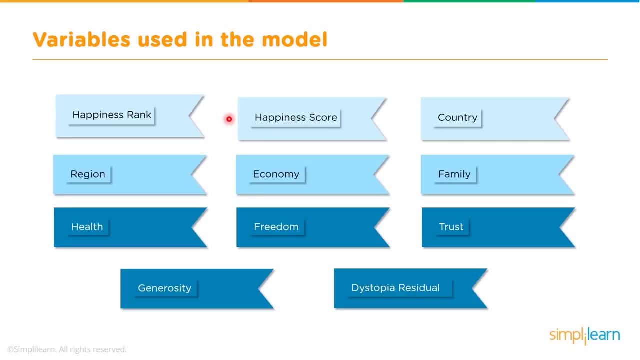 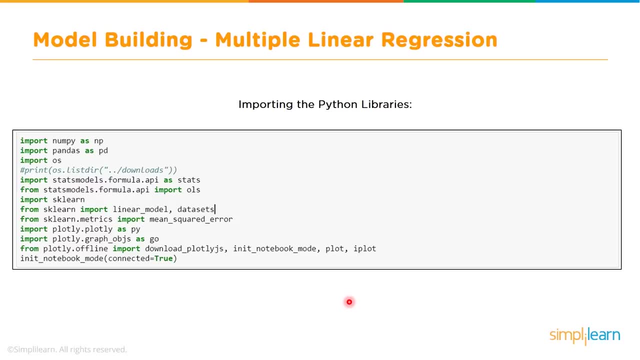 and then we need to build our model and train our model. all right, so let's assume we will use a python in order to perform this analysis or perform this machine learning activity, and i will actually show you in our lab, in a little bit, this whole thing. we will run the live code, but quickly. 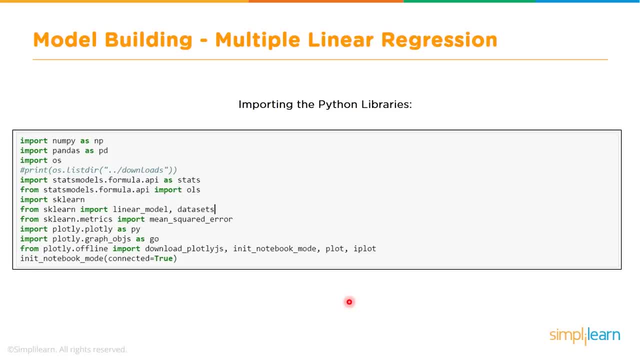 i will run you through the slides and then we will go into the lab. so what are we doing here? first thing we need to do is import a bunch of libraries in python which are required to perform our analysis. most of these are for manipulating the data, preparing the data and then scikit-learn or 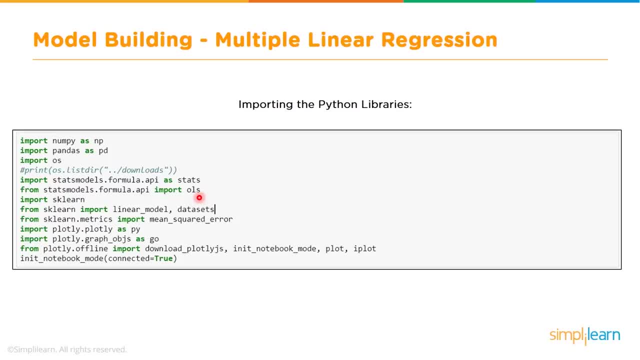 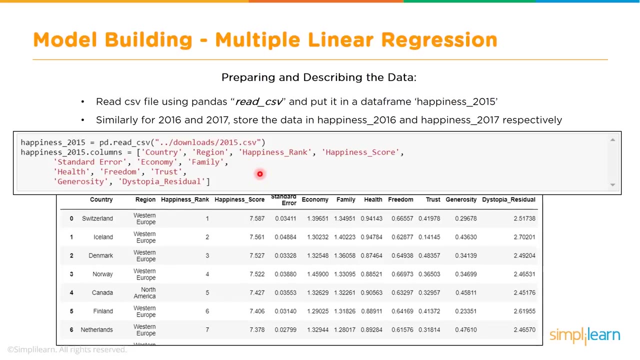 the library which we will use actually for this particular machine learning activity, which is linear regression. so we have numpy, we have pandas and so on and so forth. so all these libraries are imported and then we load our data, and the data is in the form of a csv file and there are different 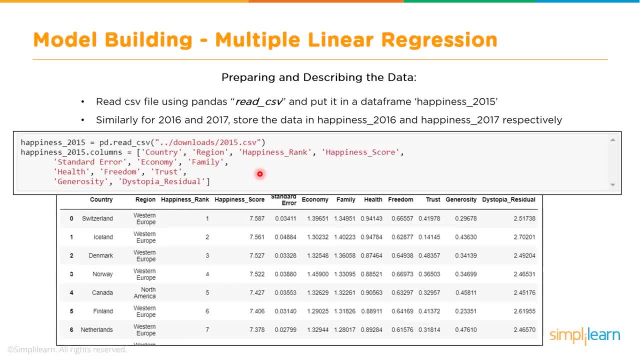 files for each year. so we have data for 2015, 16 and 17, and so we will load this data and then combine them, concatenate them to prepare a single data frame. and here we are making an assumption that you are familiar with python, so it becomes easier. 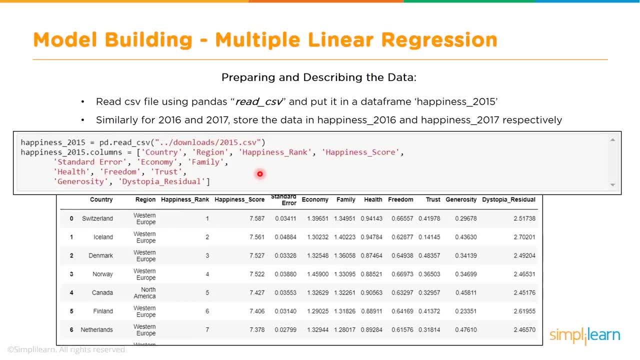 if you are familiar with python programming language, or at least some programming language, so that you can at least understand by looking at the code. so we are reading the file, each of these files for each year, and this is basically. we are creating a list of all the names of the columns. 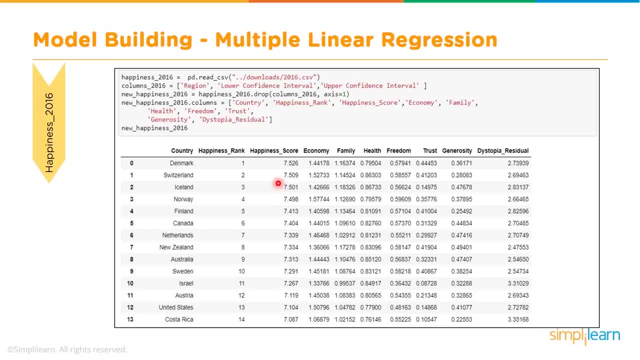 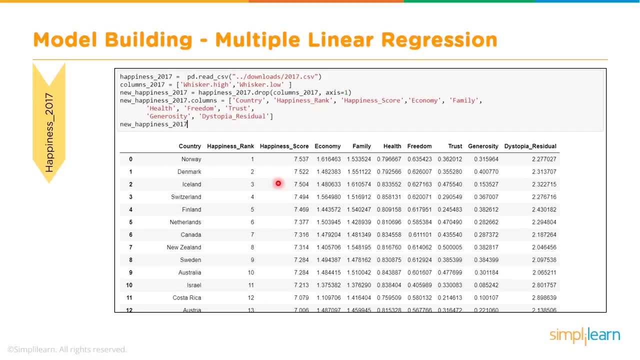 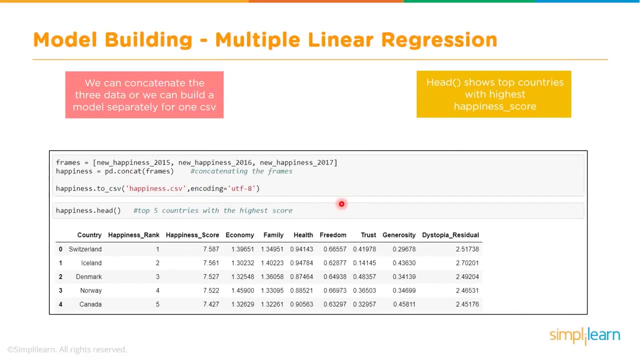 we will be using later on, you will see in the code. so we have loaded 2015, then 2016 and then also 2017. so we have created three data frames and then we concatenate all these three data frames. this is what we are doing here. then we identify which of these columns are required. which, for example? 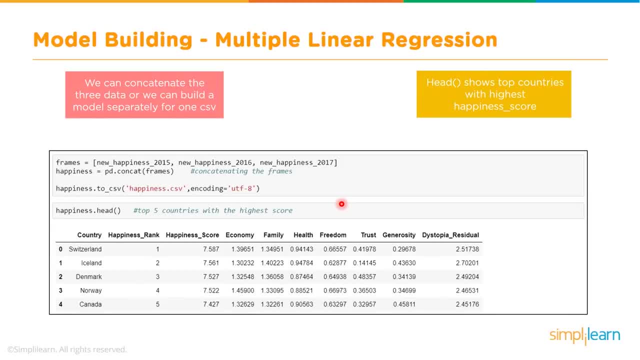 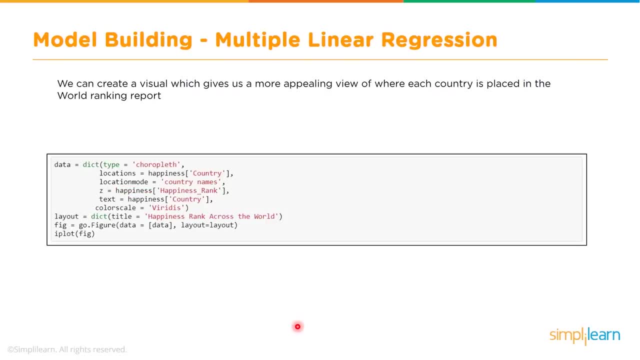 some of the categorical values. do we really need? we probably don't. then we drop those columns so that we don't unnecessarily use all the columns and make the computation complicated. we can then create some plots using plotly library, and it has some powerful features, including creation. 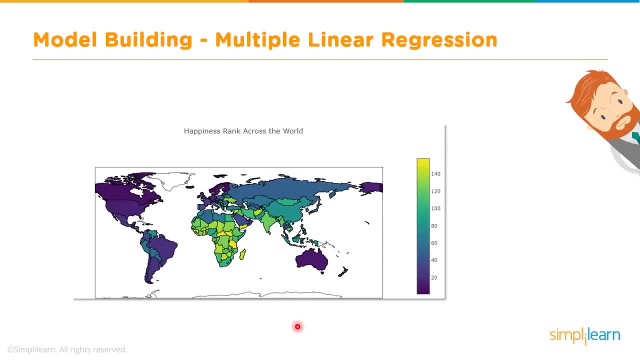 of maps and so on just to understand the pattern, the happiness quotient or how the happiness is across all the countries. so it's a nice visualization. we can see each of these countries how they are in terms of their happiness score. this is the legend here, so the lighter 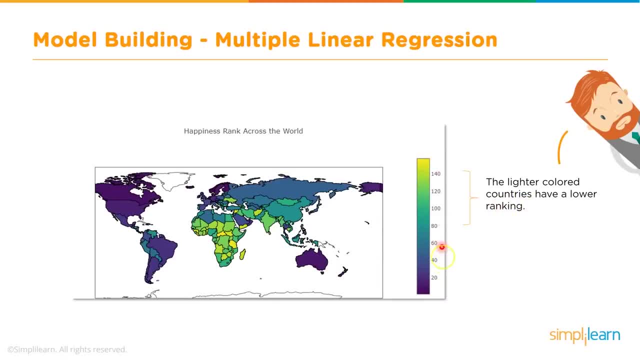 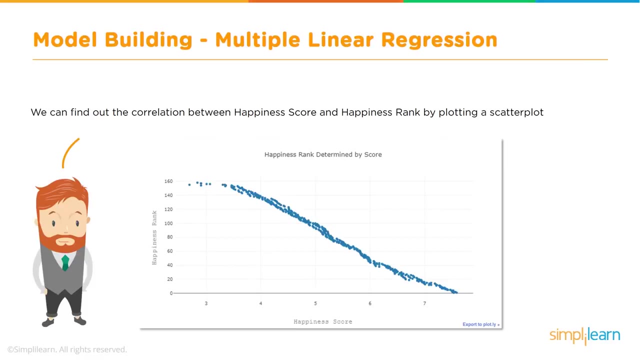 colored countries have lower ranking, and so these are the lower ranking ones and these are higher ranking, which means that the ones with these dark colors are the happiest ones. so, as you can see here, australia and maybe this side- uh, us and so on, are the happiest ones. okay, the other thing that we need to do is the correlation between the 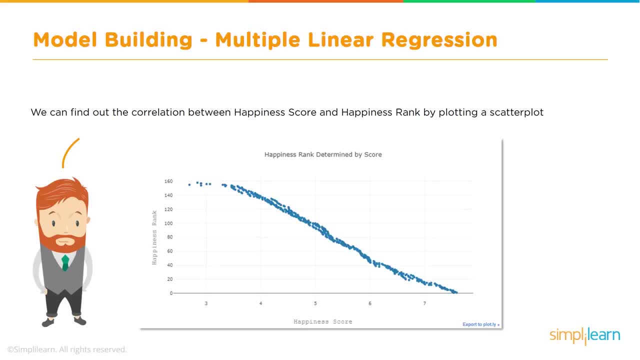 happiness score and happiness rank. we can find a correlation using a scatter plot and we find that, yes, they are kind of inversely proportion, which is obvious. so if the score is high, happiness score is high, then they are ranked number one. for example, highest is scored as number one, so that's. 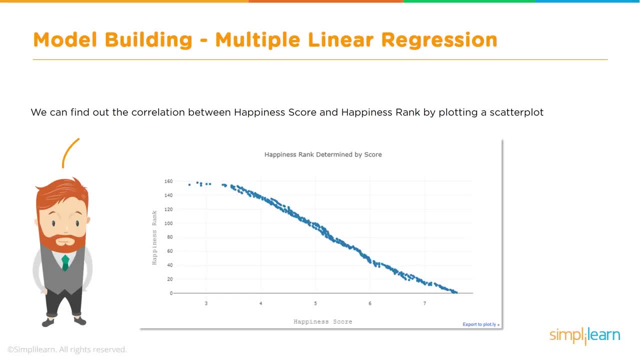 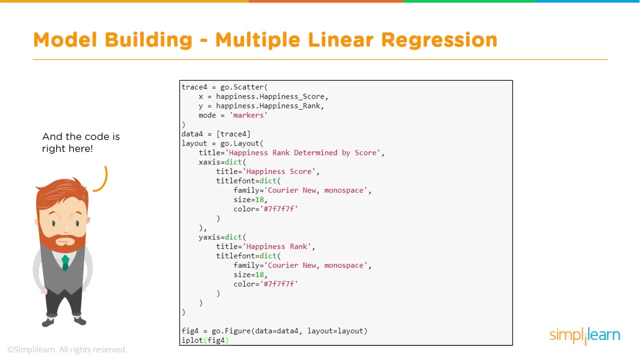 the idea behind this. so the happiness score given here and the happiness rank is actually given here. so they are inversely proportional, because the higher the score, the absolute value of the rank will be lower. right number one has the highest value of the score, and so on. so they are inversely correlated, but there is a strong. what this graph shows is: 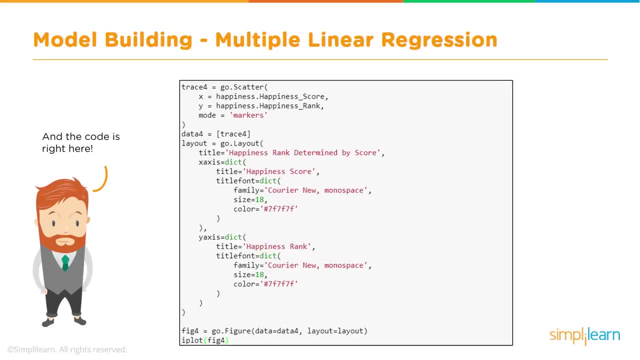 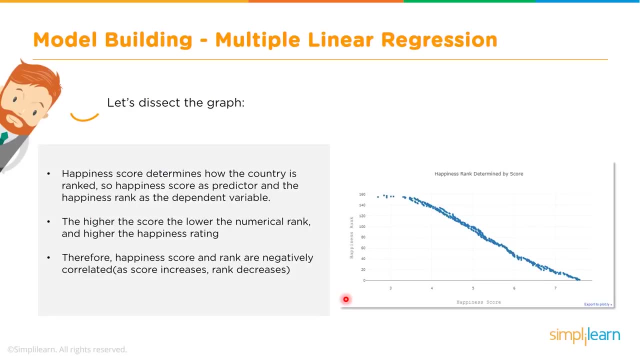 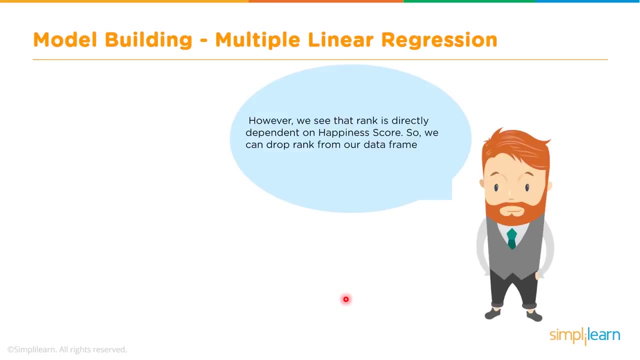 that there is a strong correlation between happiness rank and happiness score. and then we do some more plots to visualize this. we determine that probably rank and score are pretty much conveying the same message, so we don't need both of them. so we will kind of drop one of them, and that is what we are doing here. so we drop the happiness. 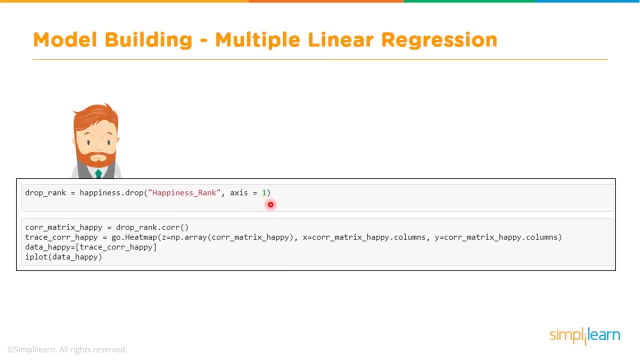 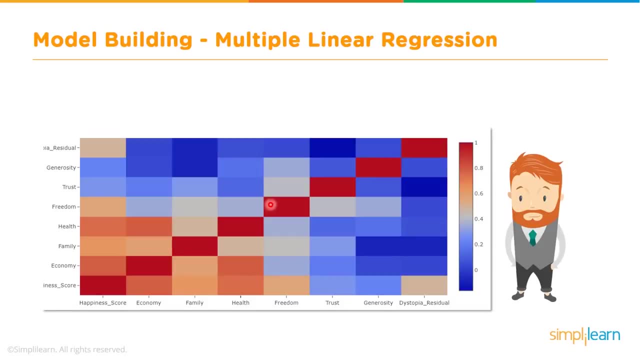 rank and similarly. so this is one example of how we can remove some columns which are not adding value, so we will see in the code as well how that works. moving on, this is a correlation between pretty much each of the columns with the other columns, so this is a correlation you can plot. 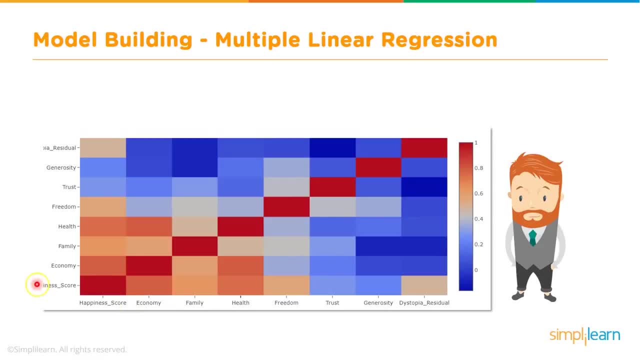 using plot function and we will see here that, for example, happiness score and happiness score are correlated. strongest correlation, right, because every variable will be highly correlated to itself. so that's the reason. so the darker the color is, the higher the correlation, and as so the and correlation in numerical terms goes from 0 to 1.. so 1 is the highest value and it can only 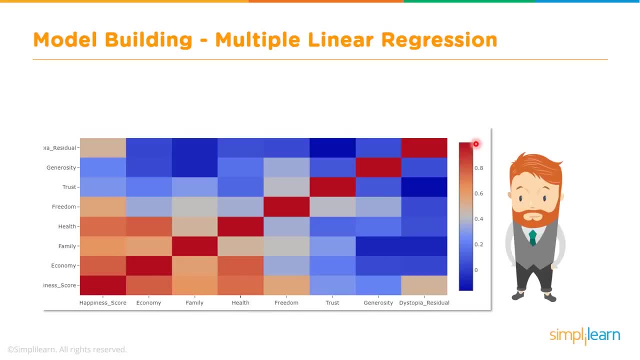 be between 0 and 1.. correlation between two variables can be only have a value between 0 and 1.. so the numerical value can go from 0 to 1, and 1 here is dark color and 0 is a kind of. 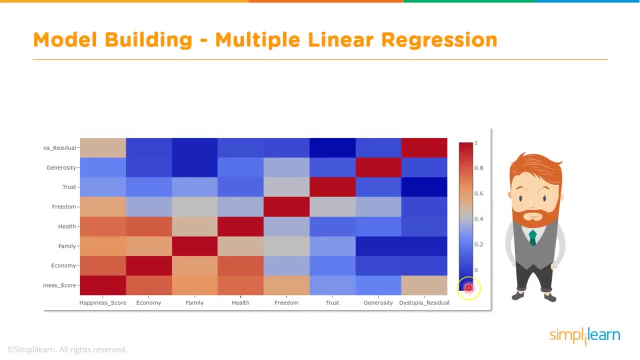 but it is blue colors, from red it goes down. the dark blue color indicates pretty much no correlation. so the from this heat map we see that happiness and economy and family are probably also help, probably are the most correlated. and then it keeps decreasing, after freedom kind of keeps. 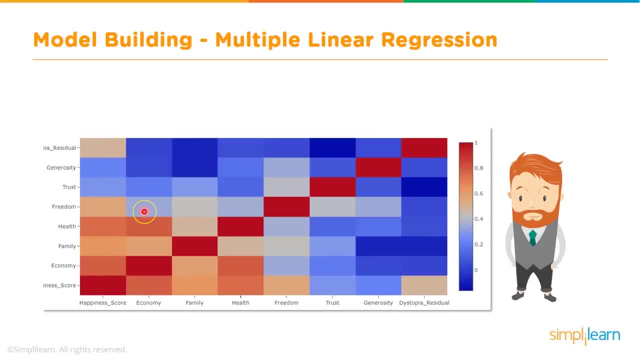 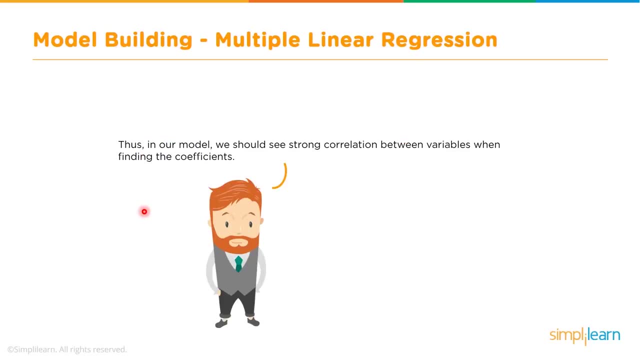 decreasing and coming to pretty much z all right, so that is a correlation graph, and then we can probably use this to find out which are the columns that need to be added to the graph. so first of all we have to see which are the columns that need to be dropped, which do not have. 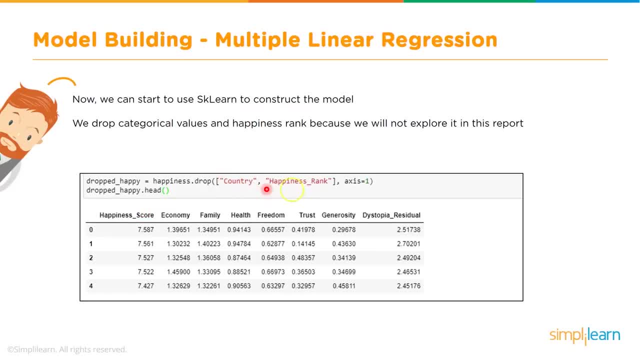 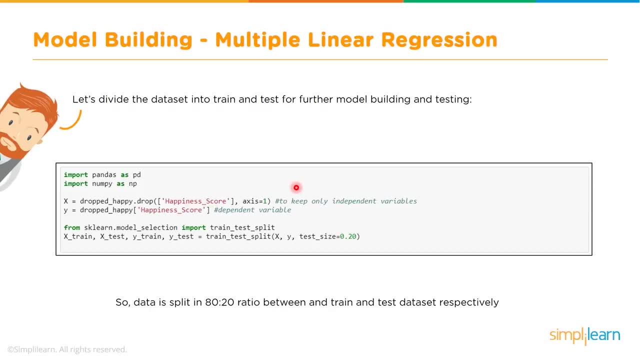 very high correlation and we take only those columns that we will need. so this is the code for dropping some of the columns once we have prepared the data. when we have the required columns, then we use scikit-learn to actually split the data. first of all, this is a normal 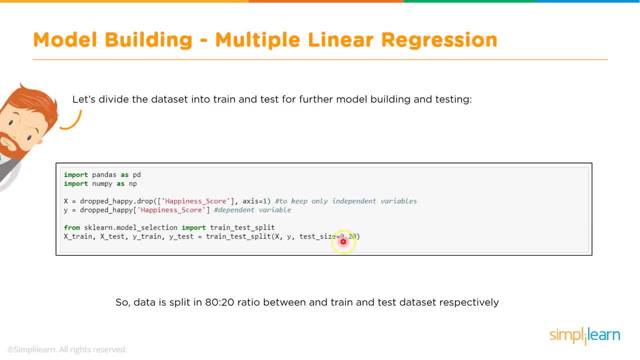 machine learning process, you need to split the data into training and test data set. in this case we are splitting into 80- 20.. 20 is the test data set. so that's what we are doing here. so we use train test split method or function. so you have all your training data in x underscore train, the labels in y underscore train. 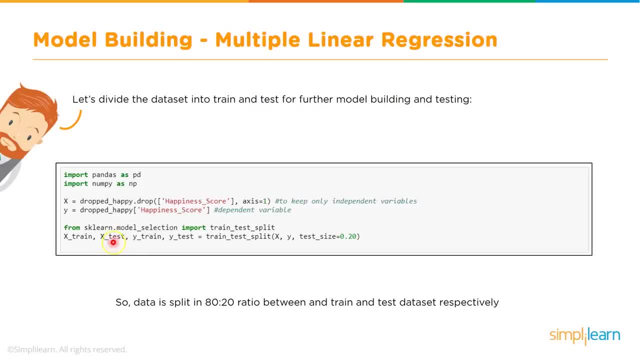 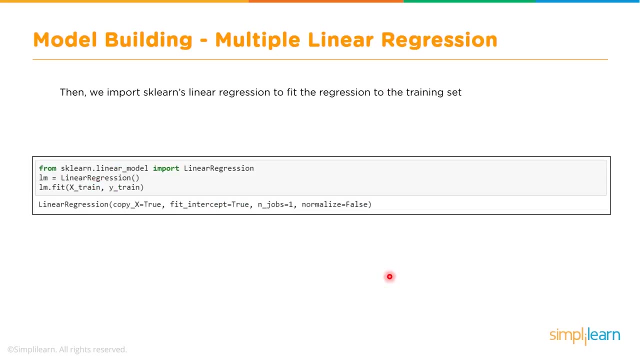 similarly, x underscore test has the test data, the inputs, whereas the labels are in y underscore test. so that's all. and this value, whether it is 80, 20 or 50, 50, that is all individual preference. so in our case we are using 80, 20, all right. and then the next is to create a linear regression. 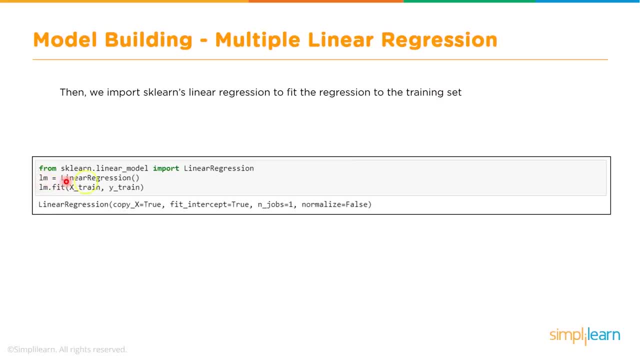 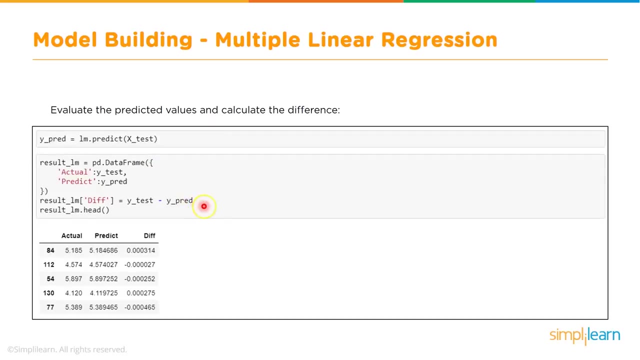 instance. so this is what we are doing: we are creating an instance of linear regression and then we train the model using the fit function and we are passing x and y, which is the x value, and the label data- regular input- and the label data, label information. then we do the test, we run. 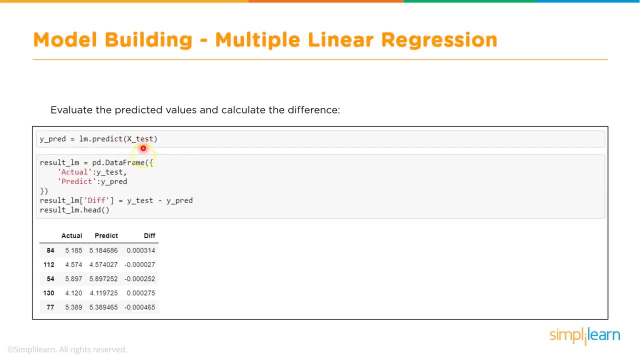 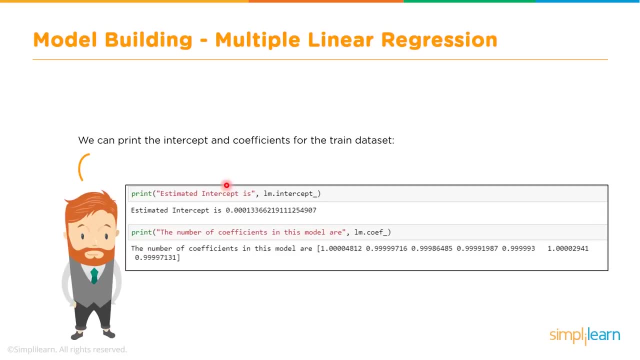 or we perform the evaluation on the test data set. so this is what we are doing with the test data set, and then we will evaluate how accurate the model is, and using the scikit-learn functionality itself, we can also see what are the various parameters and what are the various. 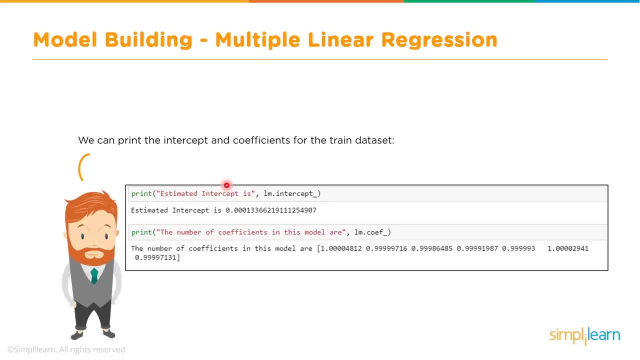 coefficients, because in linear regression you will get like a equation of, like a straight line: y is equal to beta 0 plus beta 1 x 1 plus beta 2 x 2. so those beta 1, beta 2, beta 3 are known as the 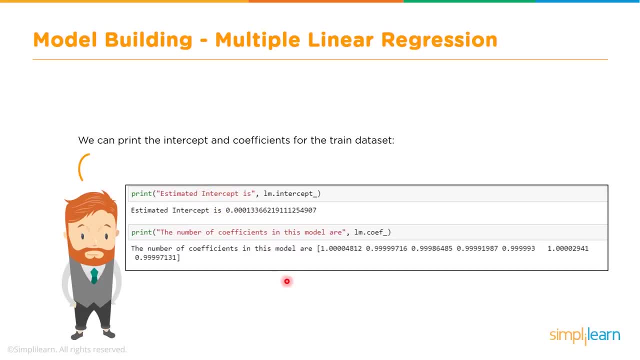 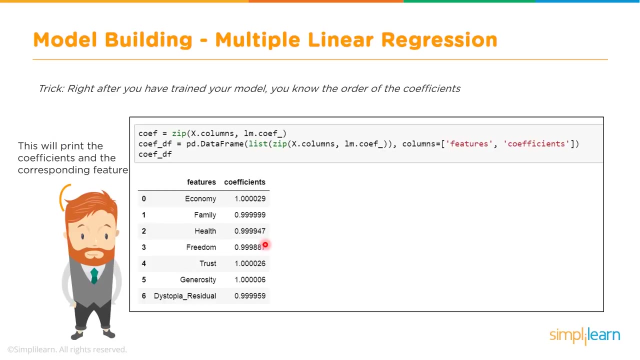 coefficients and beta 0 is the intercept. after the training, you can actually get these information of the model- what is the intercept value, what are the coefficients, and so on- by using these functions. so let's take quickly go into the lab and take a look at our code. okay, so this is my 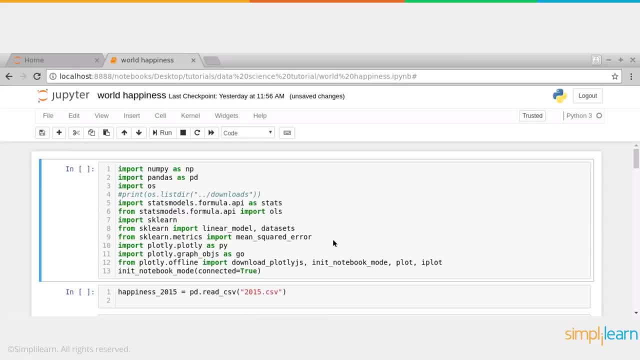 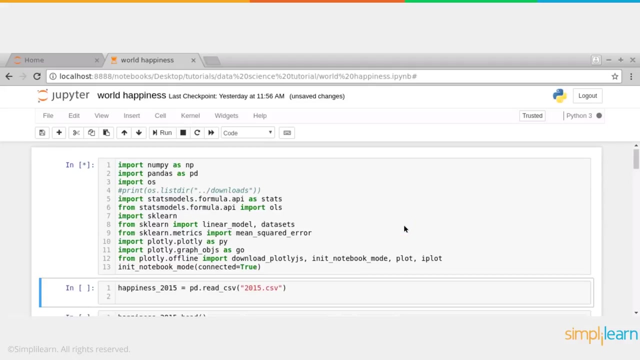 lab. this is my jupyter notebook where the code. i have the actual code and i will take you through this code to run this linear regression on the world happiness data. so we will import a bunch of libraries, numpy, pandas, plot, plotly, and so on. also, yeah, scikit-learn, that's also very important. so that's the first step. then i will 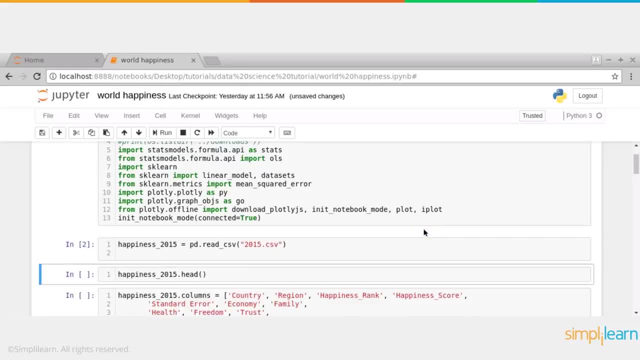 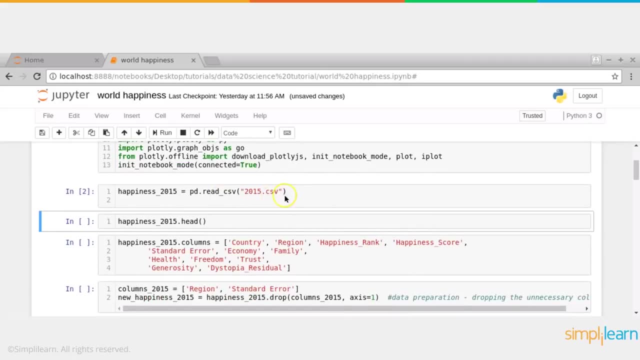 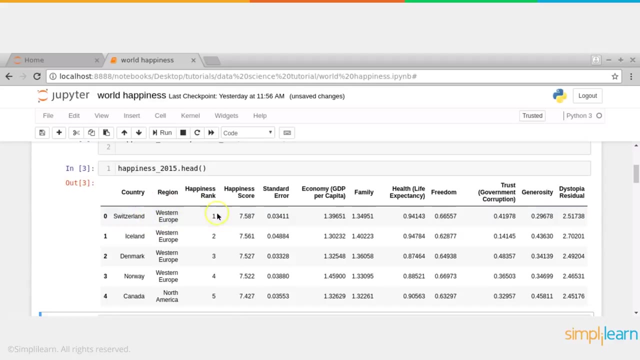 import my data, and the data is in three parts. there are three files, one for each year- 2015, 2016 and 2017- and it is a csv file. so i've imported my data. let's take a look at the data quickly. so this is how it looks: we have the country, region, happiness rank and then happiness score. 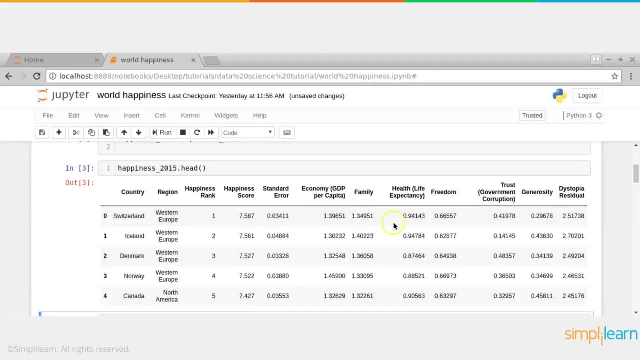 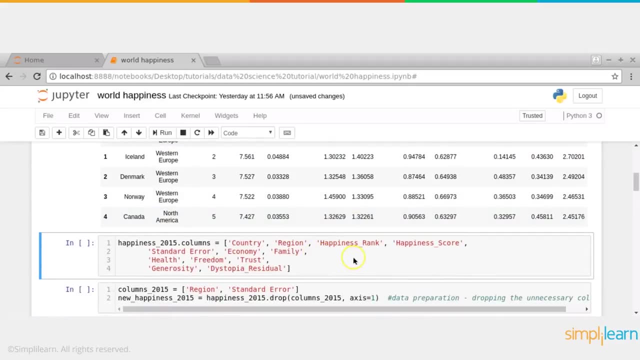 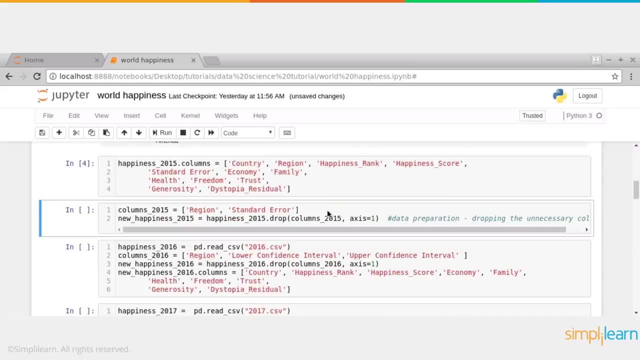 there are some standard errors. and then what is the per capita family, and so on. so, and then we will keep going. we will create a list of all these column names we will be using later. so for now, just i will run this code and no need of major explanation at this point. we know that some of 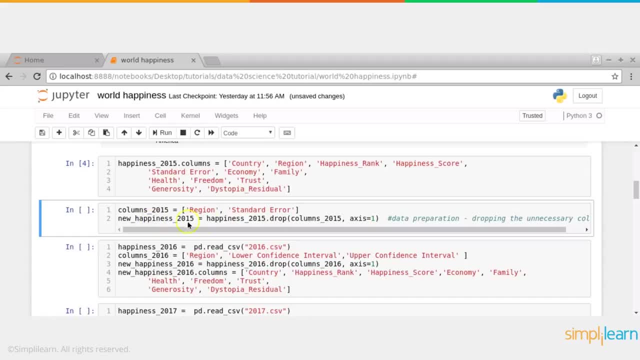 these columns probably are not required, so you can use this drop function to run this code and It'll give you the functionality to remove some of the columns which we don't need, like, for example, Digit diagram, region and standard. error will not be contributing to our model, so we will basically drop those. 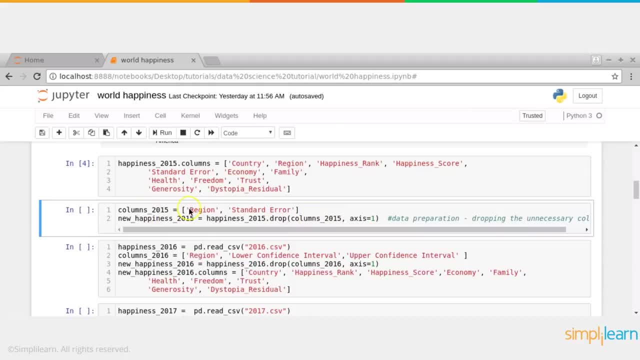 values out here. so we use the drop проис from our data frame. it will remove region and standard error, these two columns. then the next feature we're going to use is greater enough environment if earlier functions as well. this is the first field jump change we can see. so we'll change the position to: either it is some structure selected, but they all work, ferramenta and we你是. 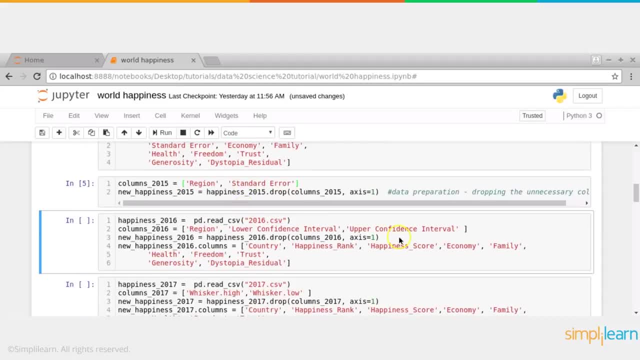 and then same function region and call it column. this is my column- calls a variable, so a rationale we use again to produce form sounds in order for some of the trials already used by the collection named Form license and standard error. these two columns, then the next step. we will read the data for 2016. 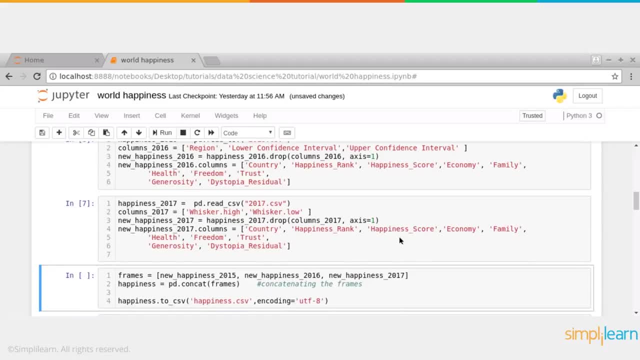 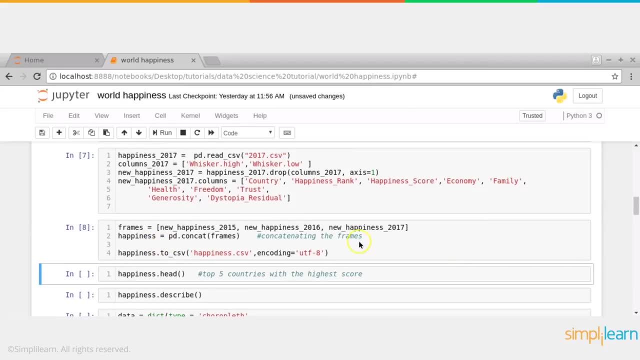 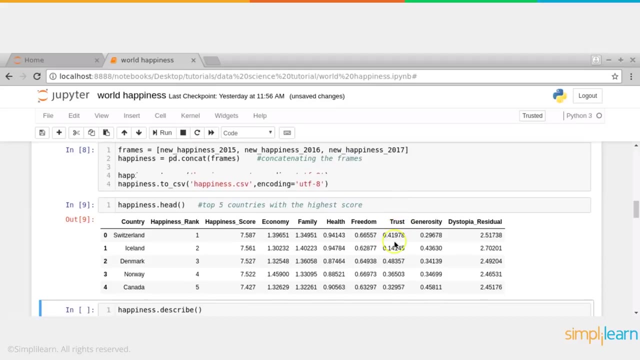 and also 2017, and then we will concatenate this data. so let's do that. so we have now data frame called happiness, which is a concatenation of both all the three files. let's take a quick look at the data now. so most of the unwanted columns have been removed and 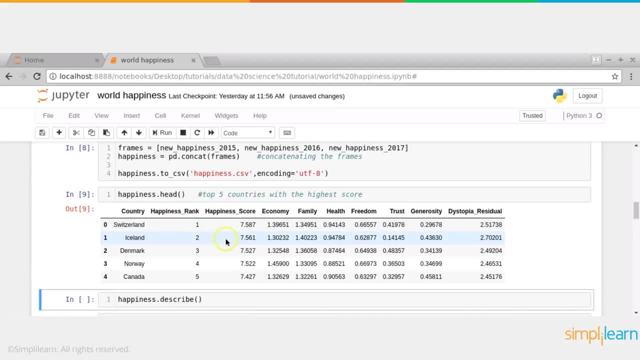 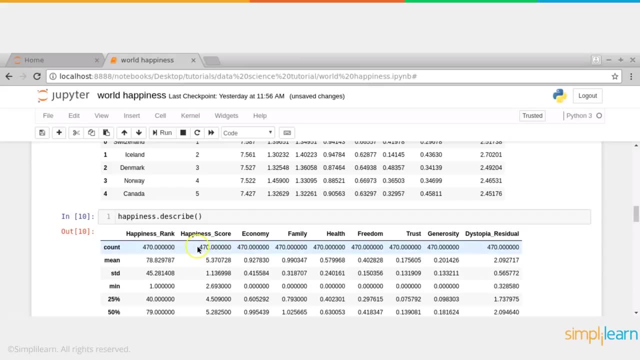 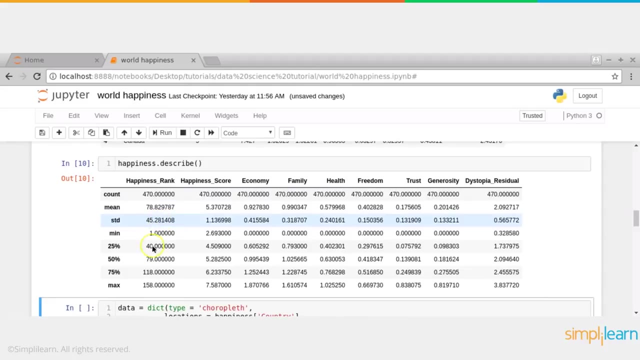 you have all the data in one place for all the three years and this is how the data looks and if you want to take a look at the summary of the columns, you can say describe and you will get this information. for example, for each of the columns: what is the count, what's? what is the mean value? 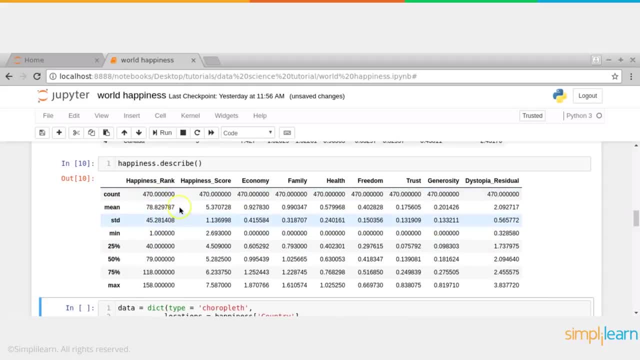 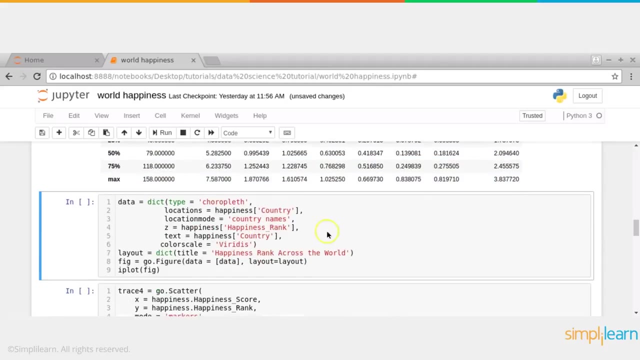 standard deviation, especially the numeric values. okay, not the categorical values. so this is a quick way to see how the data is and initial little bit of exploratory analysis can be done here. so is you can maximum value, what's the minimum value, and so on for each of the columns. all right, so then we go. 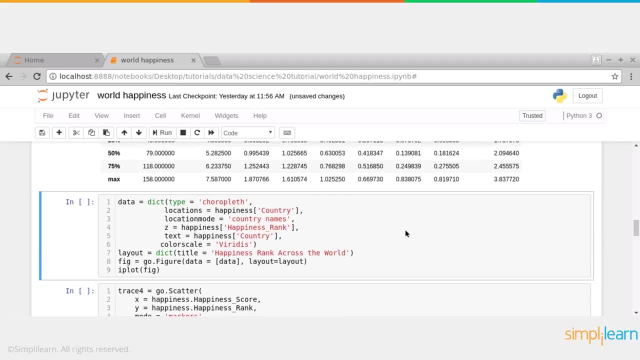 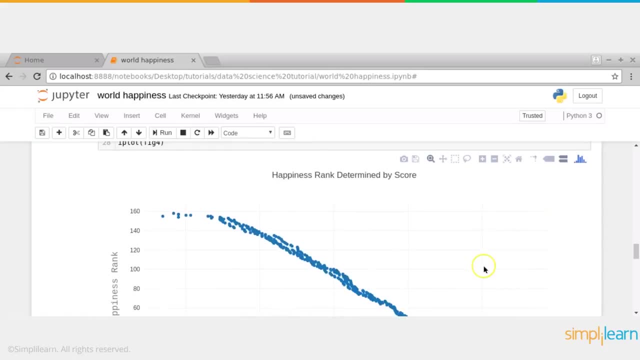 ahead and create some visualizations using plotly. so let us go and build a plot. so if we see here now- this is the relation correlation between happiness rank and happiness score. this is what we have seen in the slides as well- we can see that there is a tight correlation between them. 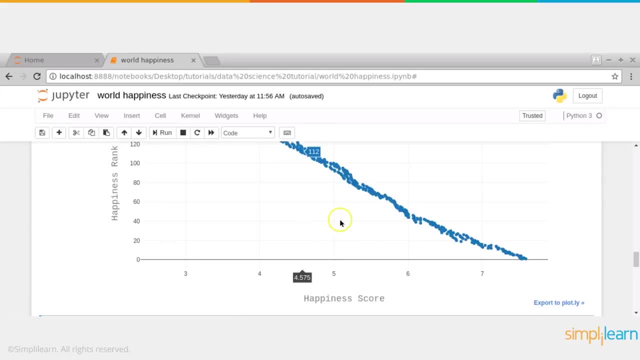 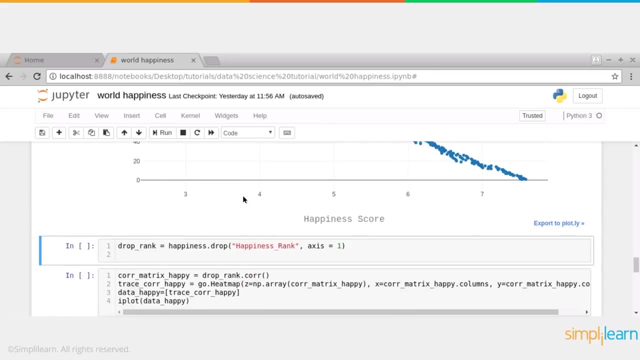 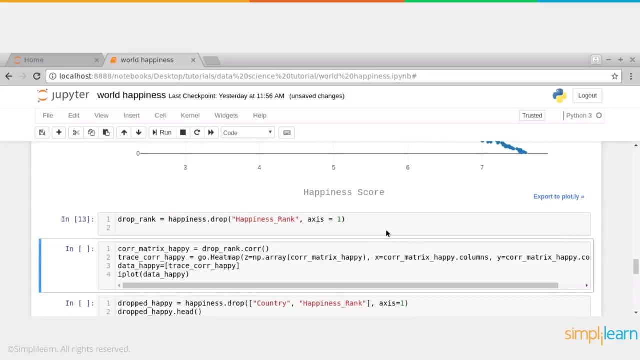 only thing is it is inverse correlation, but otherwise they are very tightly correlated, which also says that they both probably provide the same information. so there is no, not much of value add. so we'll go ahead and drop the happiness rank as well from our columns. so that's what we're. 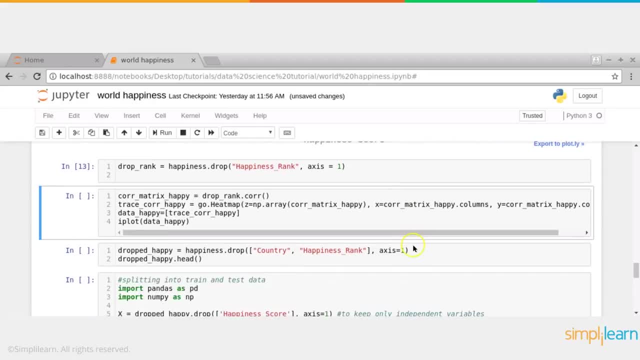 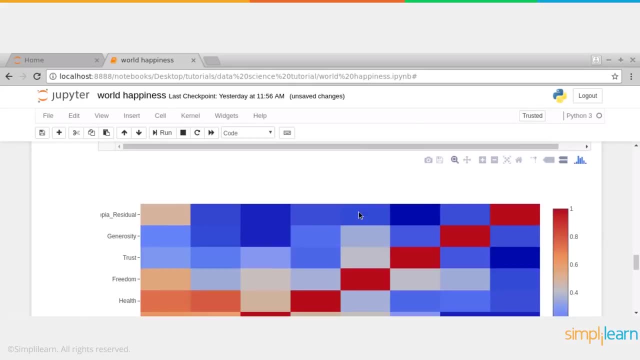 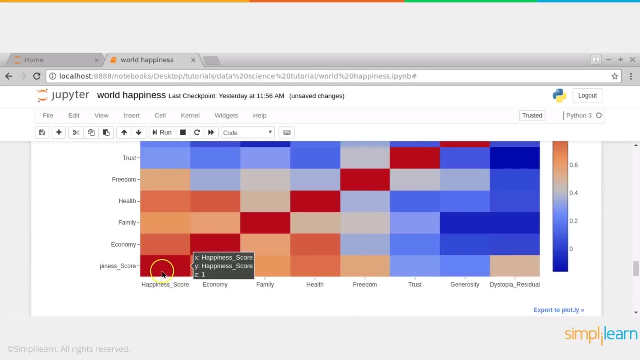 doing, here and now we can do, the creation of the correlation heat map. let us plot the correlation heat map to see how each of these columns is correlated to the other and we, as we have seen in the slides, this is how it looks. so happiness score is very highly. 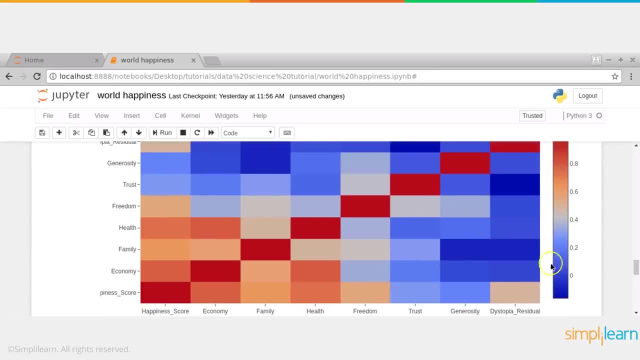 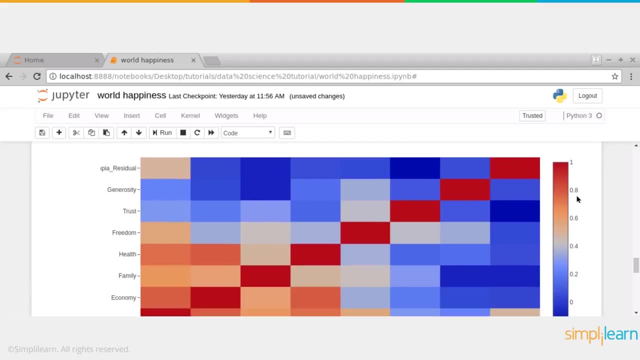 correlated. so this is the legend we have seen in the slide as well. so blue color indicates pretty much zero or very low correlation. deep red color indicates very high correlation and the value correlation is a numeric value and the value goes from zero to one if the two items or two features. 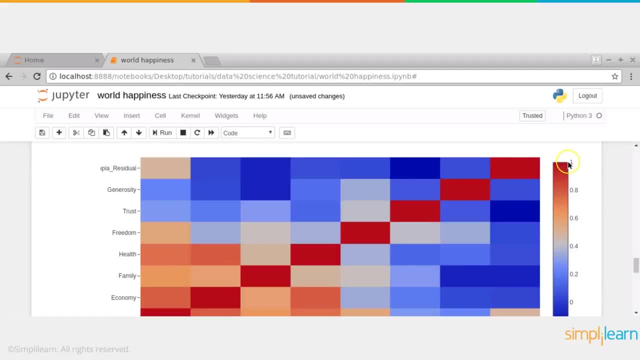 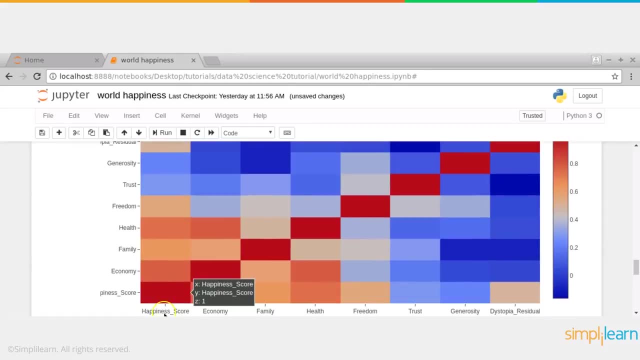 or columns are highly correlated, then they will be as close to one as possible, and two columns that are not at all correlated will be as close to zero as possible. so that's how it is. for example, here: happiness score and happiness score- every column or every feature will be highly. 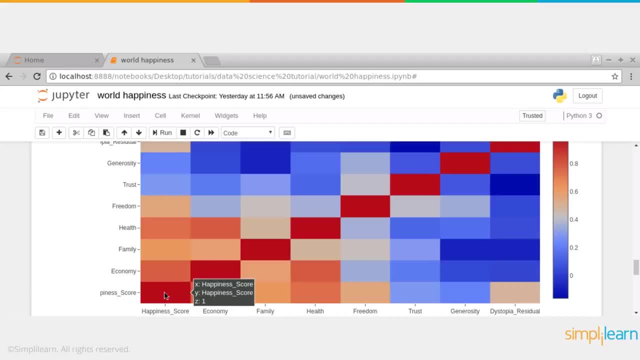 correlated to itself. so it is like between them there will be correlation, value will be one, so that's why we see deep red color, but then others are. for example, with higher values are economy and then health, and then maybe family and freedom. so these are generosity and trust- are not very highly. 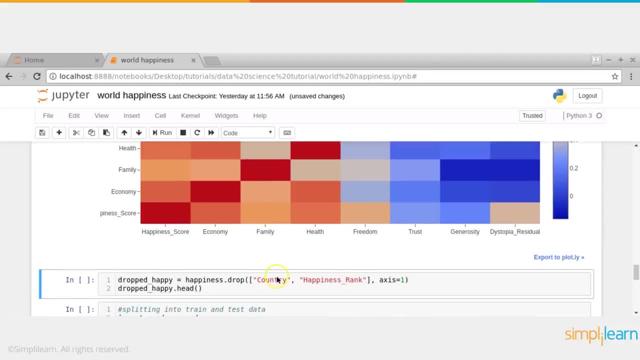 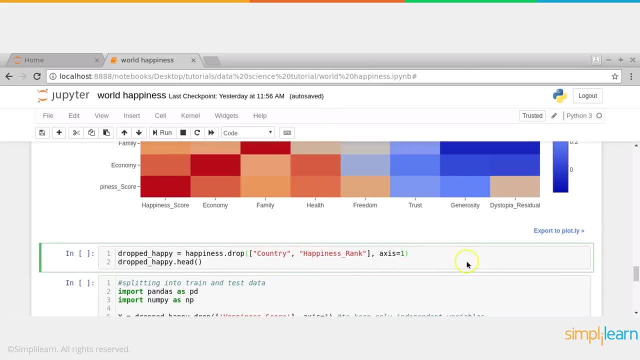 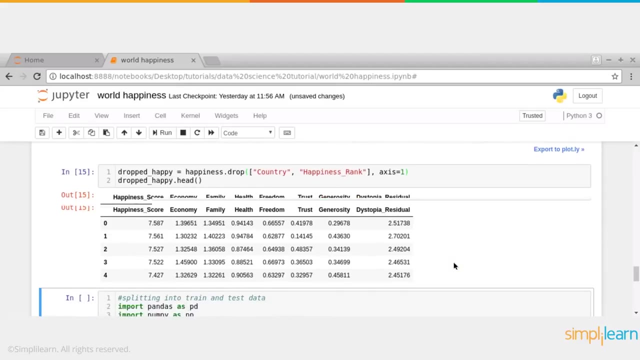 correlated to happiness score. so that is one quick exploratory analysis we can do and therefore we can drop the country and the happiness rank, because they also, again, don't have any major impact on the analysis, on our analysis. so now we have prepared our data, there was no need to clean the data because the data was clean. but 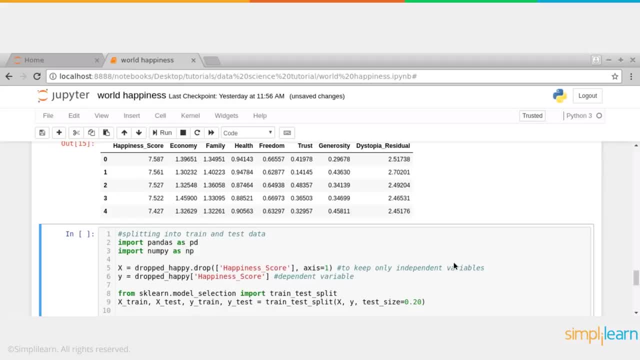 if there were some missing values and so on. as we have discussed in the slides, we would have had to perform some of the data cleaning activities as well, but in this case the data was clean. all we needed to do was just the preparation part. so we removed some unwanted columns and we did some exploratory data analysis. 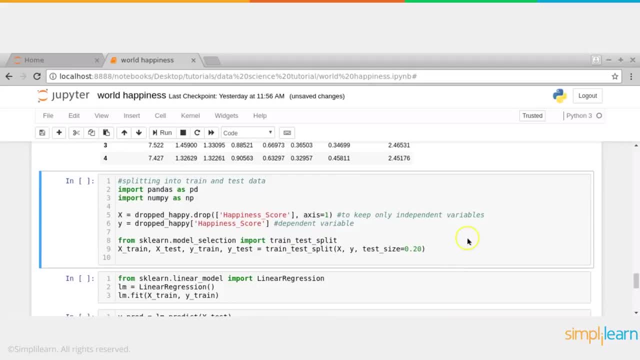 now we are ready to perform the machine learning activity, so we use scikit-learn for doing the machine learning. scikit-learn is python library that is available for performing our machine learning. once again, we will import some of these libraries, like pandas and numpy, and also scikit-learn. 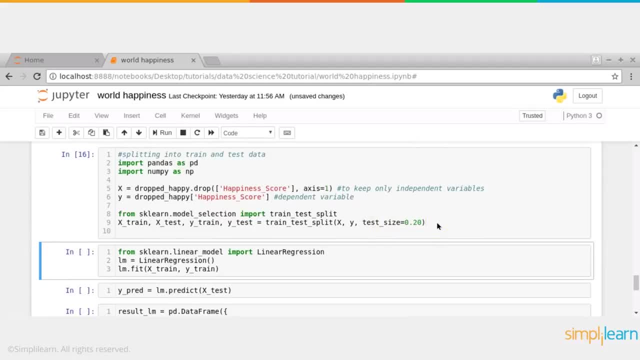 first step we will do is split the data in 2080 format. so all the test data, which is 20 percent of the data, is test data and 80 percent is your training data. so this test size indicates how much of it is the. what is the size of the test data? so the 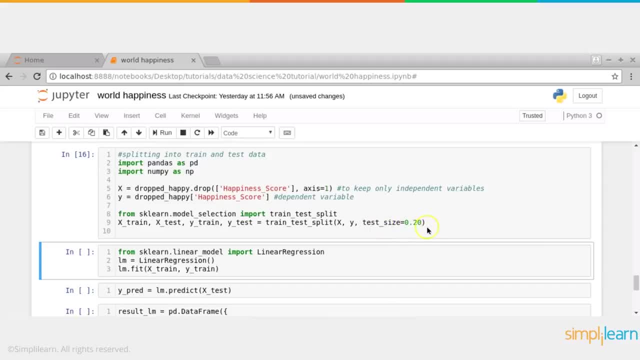 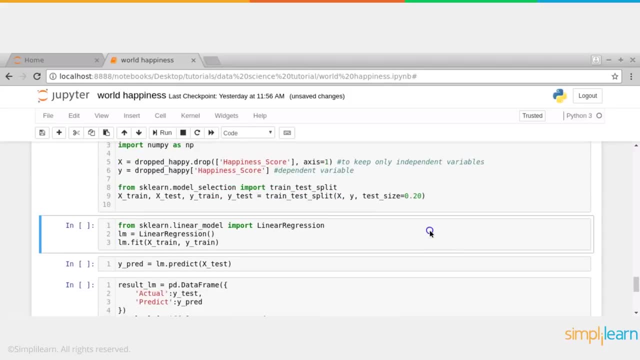 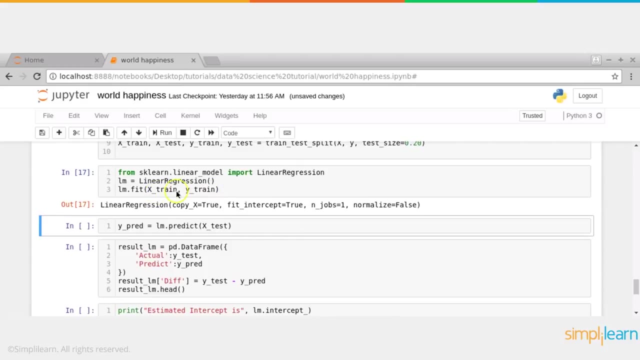 remaining, which is point. here we are saying 0.2. therefore that means training is 0.8, so training data is 80 percent. all right, so we have executed that, split the data and now we create an instance of the linear regression model. so lm is our linear regression model and we pass x and y, the training. 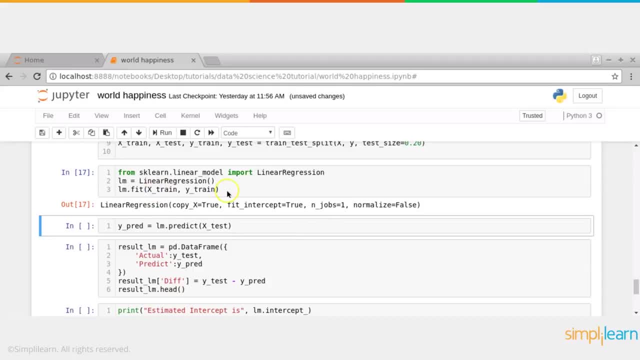 and call the function fit, so that the model gets trained. so now, once that is done, training is done, training is completed, and now what we have to do is we need to predict the values for the test data. so the next step is using. so you see, a fit will basically run the training method, predict will. 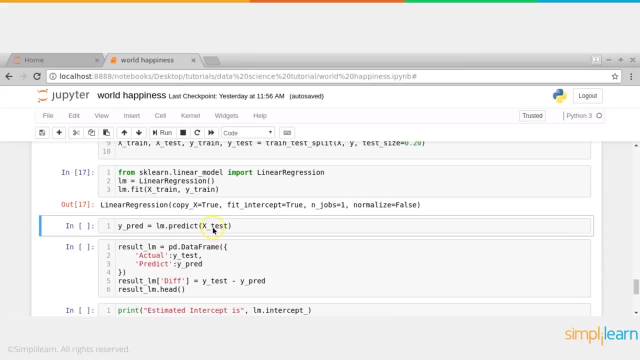 actually predict the values. so we are passing the input values, which is the independent variables, and we are asking for the values of the dependent variable, which is what we are capturing in y underscore track, and we use the predict method here- lm dot predict. so this will give us all the predicted y values and remember we already have y underscore test has the 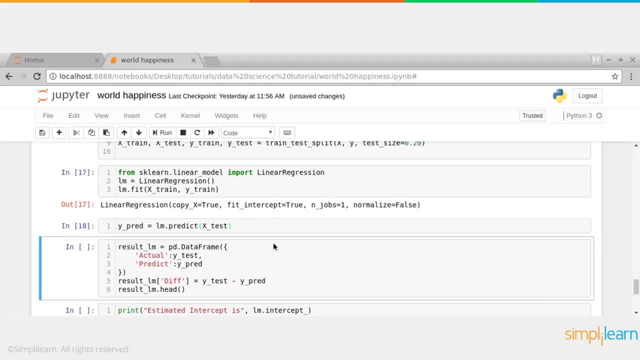 actual values, which are the labels, so that we can use these two to compare and find out how much of it is error. so that's what we are doing here: we are trying to find the difference between the predicted value and the actual value. y underscore test is the actual value for the test data and y. 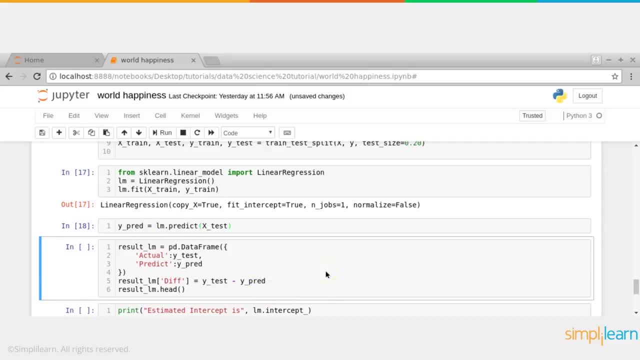 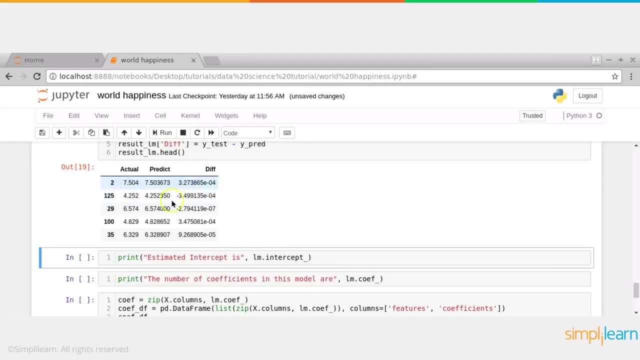 underscore: predict is the predicted value. we just found out the predicted value, so we will run that and we can do a quick check as to how the data looks. how is the difference? so? in some cases it is positive, some cases it is negative, but in most of the cases I think the difference is very small. this is: 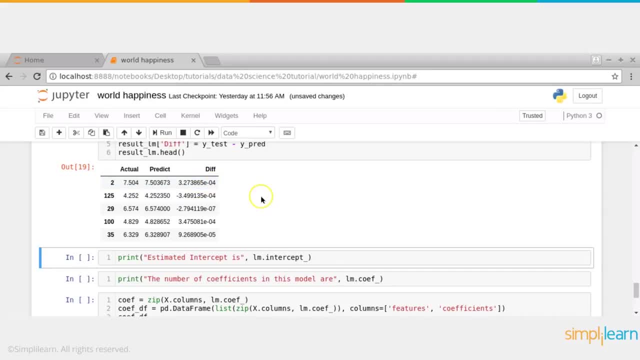 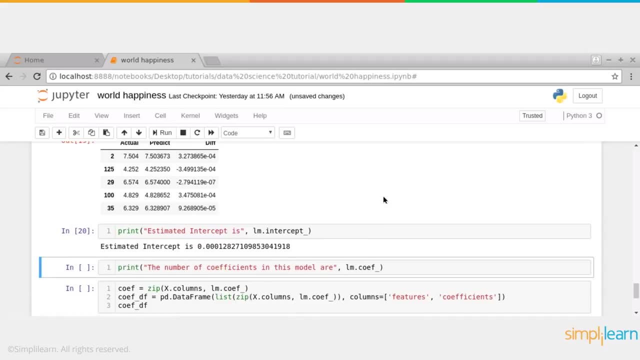 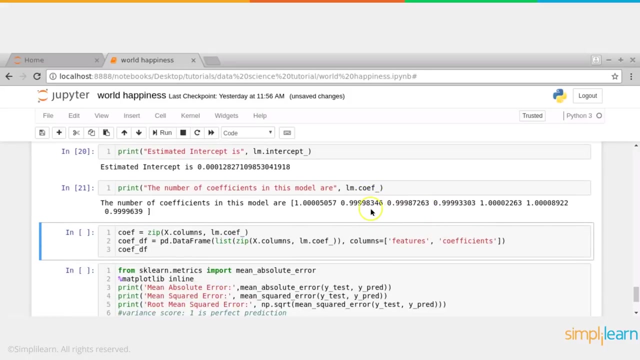 exponential to the power of 0 minus 0, 4 and so on. so looks like our model has performed reasonably well. we can now check some of the parameters of our model, like the intercept and the coefficients. so that's what we are doing here. so these are the coefficients of the various parameters that we are the coefficients of the. 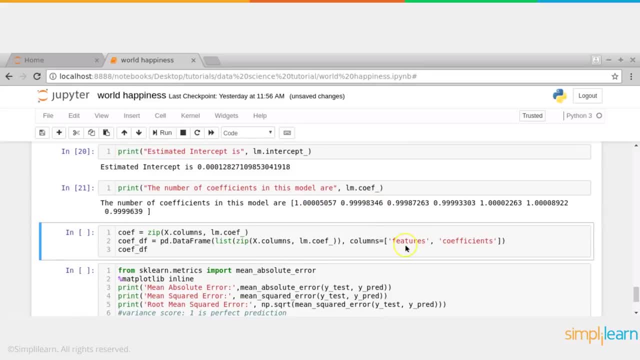 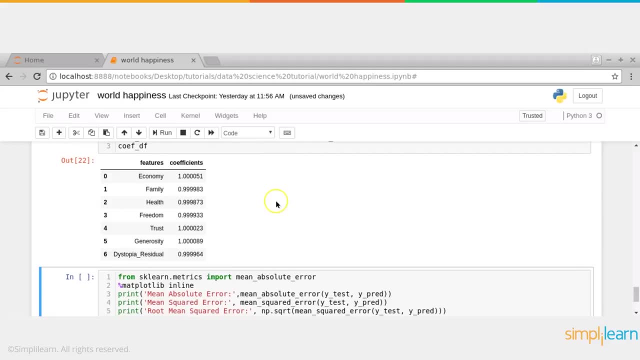 various independent variables. okay, so these are the values. then we can- we can quickly go ahead and list them down as well- against the corresponding independent variable. so the coefficients against the corresponding independent variable. so one point zero, zero, five. one is the coefficient for economy. point 9993 is for family coefficient for family and health, and so on and so forth. so that's. 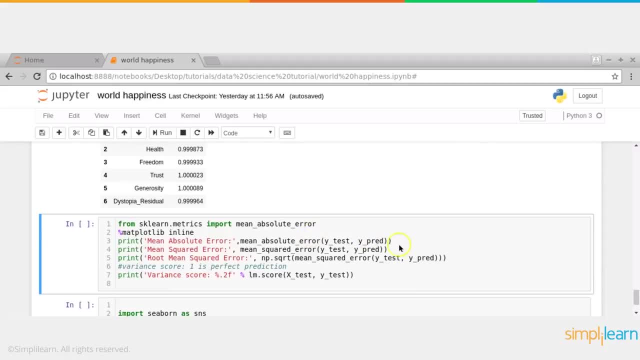 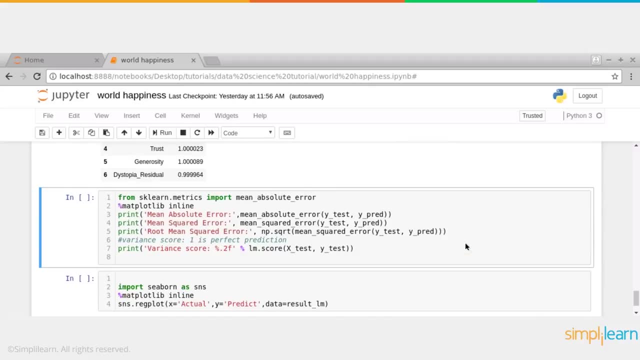 what this is showing. now we use the functionality readily available functionality of scikit-learn and then plot that to find some of the parameters which determine the accuracy of this model, like, for example, what is the mean square error, and so on. so that's what we are doing here, so let's just go. 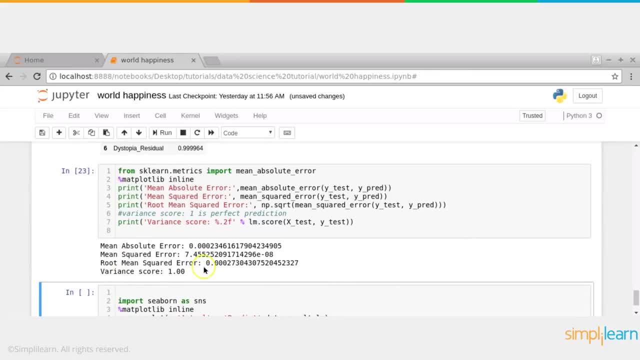 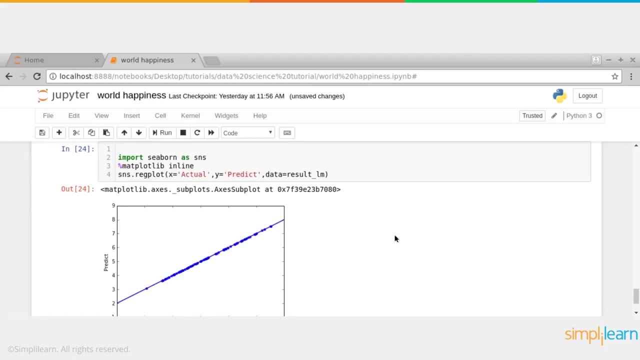 ahead and run this, so you can see here that the root mean square error is pretty low, which is a good sign and which is a one of the measures of how well our model is performing. we can do one more quick plot to just see how the actual values and the predicted values are looking, and once 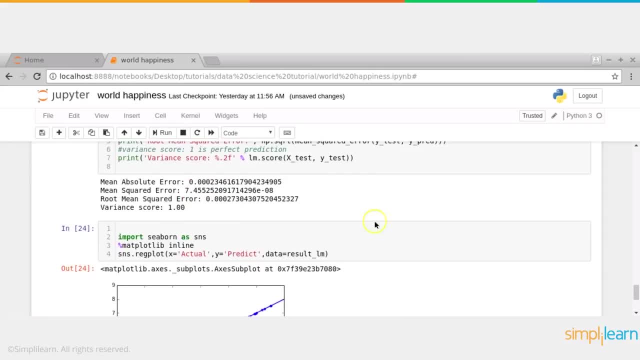 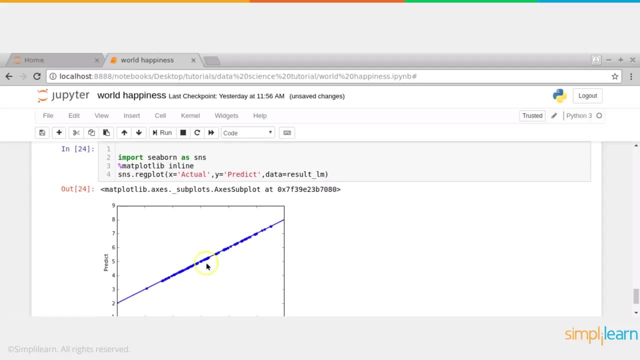 again, you can see that, as we have seen from the root mean square error, root mean square error is very, very low. that means that the actual values and the predicted values are pretty much matching up, almost matching up, and this plot also shows the same. so this line is going through the predicted. 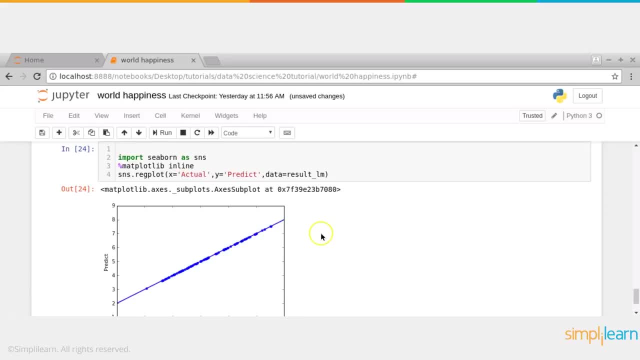 values and the actual values, and the difference is very, very low. so again, this is actual data. this is one example where the accuracy is high and the predicted values are pretty much matching with the actual values. but in real life you may find that these values are slightly more scattered and you may get the error. value can be relatively. 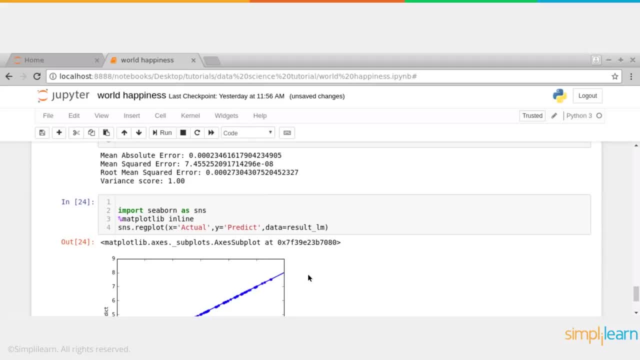 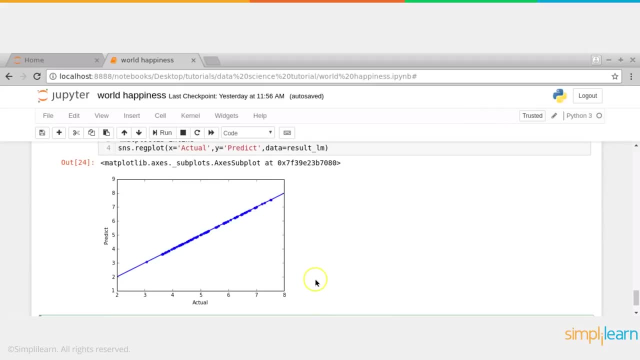 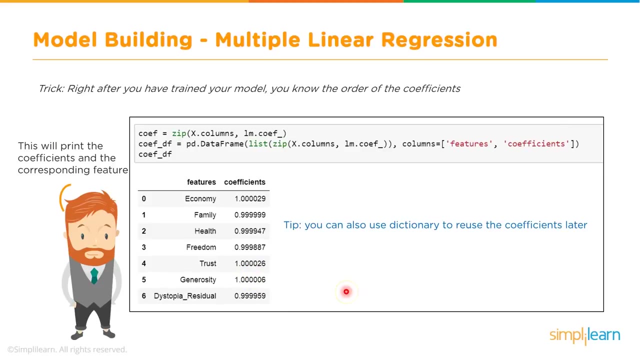 on the higher side, the root mean square. okay, so this was a good, quick example of the code to perform data science activity or machine learning or data mining activity. in this case, we did what is known as linear regression. so let's go back to our slides and see what else is there and 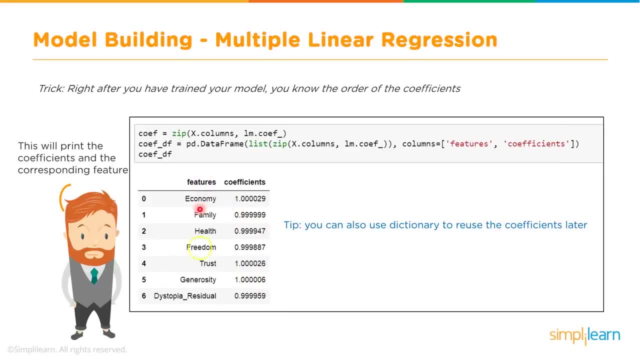 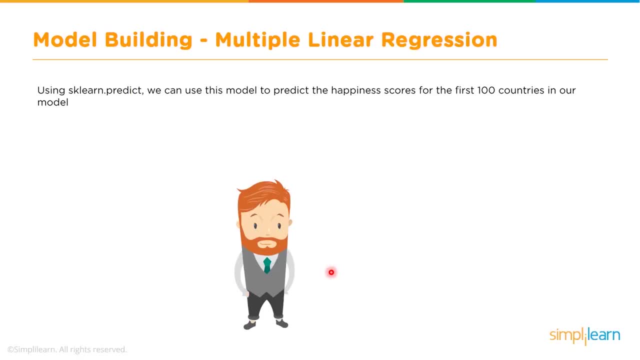 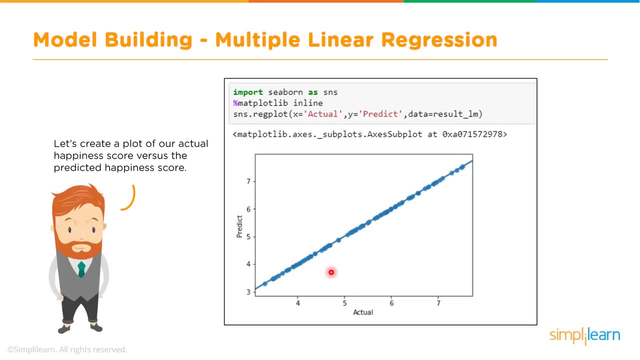 here. so we saw this. these are the coefficients of each of the features in our code and we have seen the root mean square error as well, and we can take a few hundred countries, certain values and actually predict to see if how the model is performing, and I think we have done this as well. 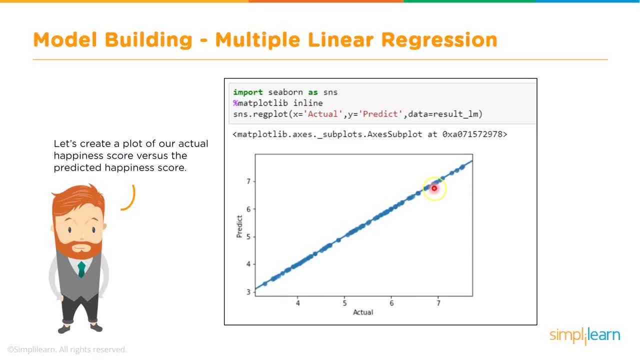 and in this case, as we have seen, the pretty much the predicted values and the actual values are pretty much matching, which means our model is almost hundred percent accurate. as I mentioned, it may not be the case, but in this particular case we have got a pretty good model, which is: 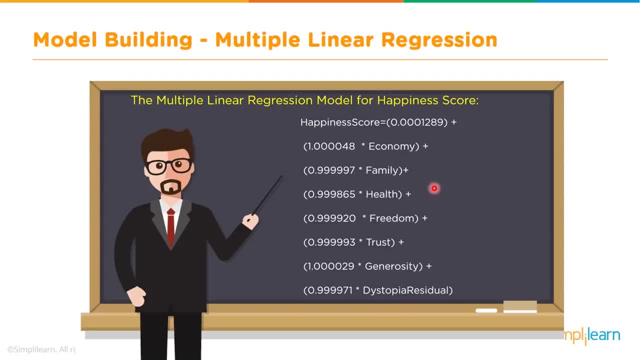 very good. also, subsequently, we can assume that this is how the equation in linear regression- the model is nothing but an equation like y- is equal to beta 0 plus beta 1 x 1 plus beta 2 x 2 plus beta 3 x 3, and so on. so this is what we are showing here, so this is our intercept, which is: 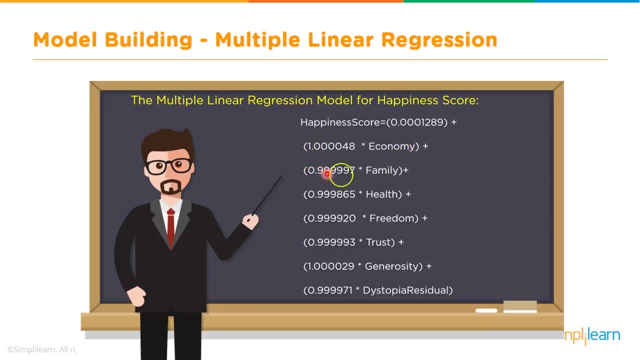 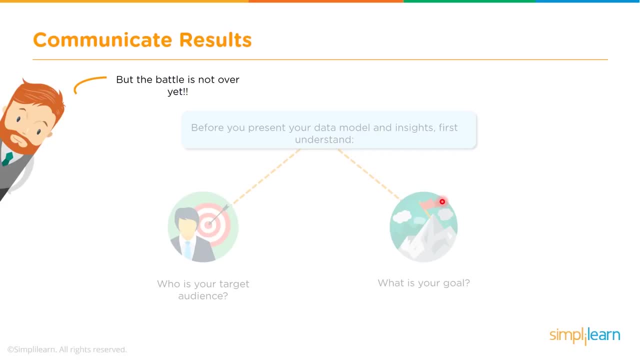 beta 0, and then we have beta 1 into economy value, beta 2 into the family value, beta 3 into health value, and so on. so that is what is shown here, okay. so I think the next step, once we have the results from the data mining or machine learning activity, the next step is to communicate. 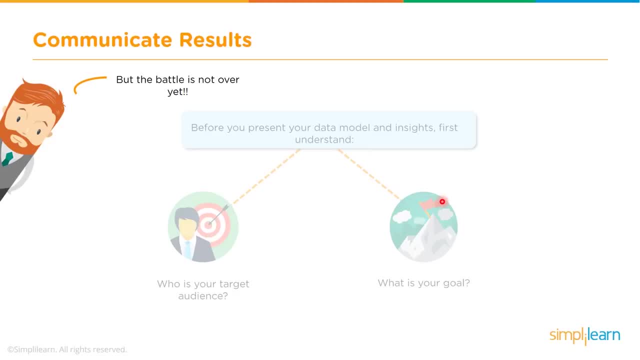 these results to the appropriate stakeholders. so that is what we will see here now. so how do we communicate? usually, you take these results and then either prepare a presentation or put it in a document and then show them these actionable results or actionable insights, and you need to find out who are your target audience and put all the results in context. 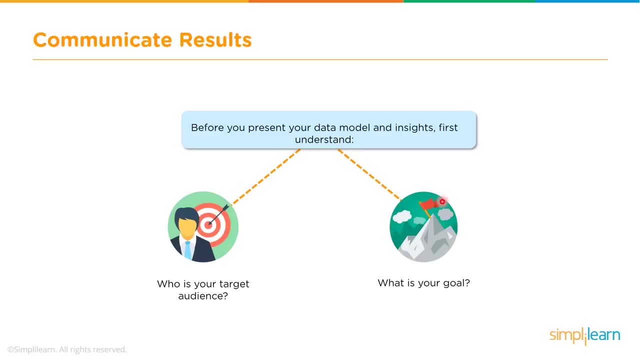 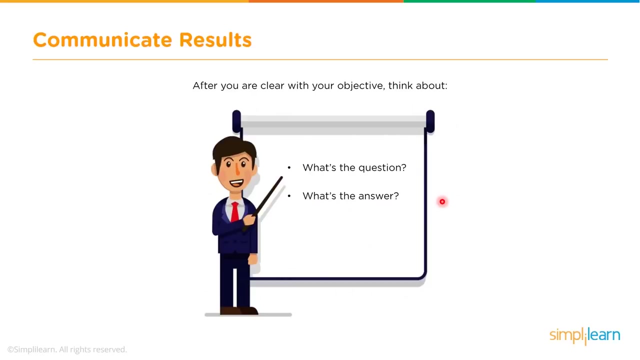 and maybe if there was a problem statement, you need to put this results in the context of the problem statement. what was our initial goal that we wanted to achieve so that we need to communicate here based on? I remember we started off with what is the question and what is the data, and so on, and 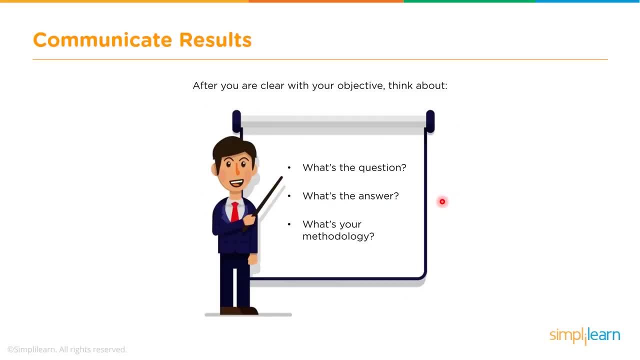 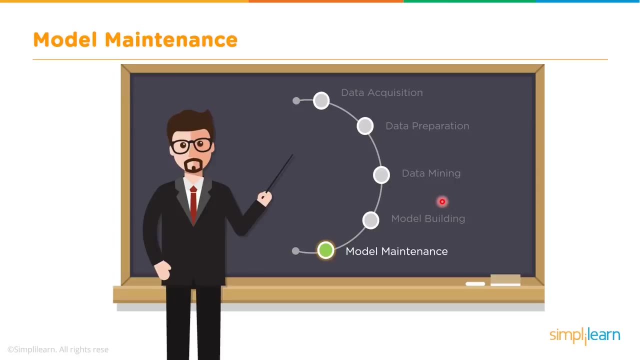 then what is the answer? so we we need to put the results and then is the methodology that we have used. all that has to be put and clearly communicated in business terms so that the people understand very well from a business perspective. so once the model building is done, once the results are published and communicated, the last part is maintenance of 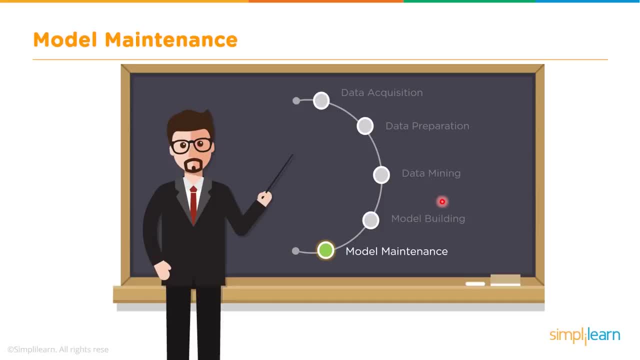 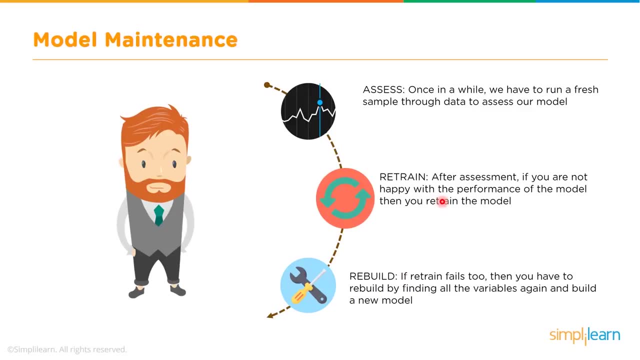 this model. now, very often what can happen is the model may have to be subsequently updated or modified because of multiple reasons. either the the data has changed, the way the data comes has changed, or the process has changed. for whatever reason, the accuracy may keep changing once you. 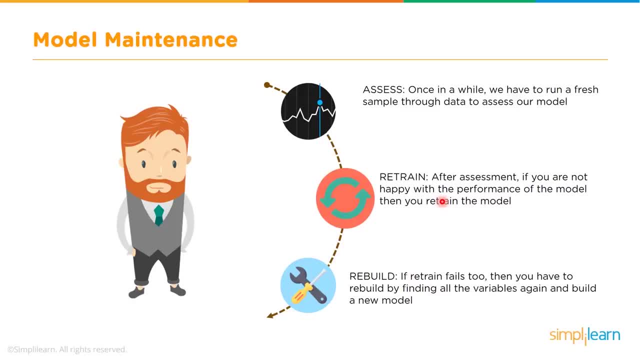 have a trained model- the, for example- we got a very high accuracy, but then, over a period of time, there can be various factors which can cause that. so from time to time, we need to check whether the model is performing well or not. the accuracy needs to be tested once in a while and, if required, 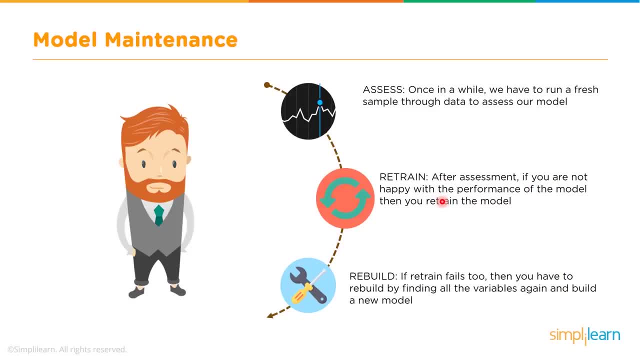 you may have to rebuild or retrain the model. so you do the assessment, you you see if it needs any tweaks or changes and then, if it is required, you need to probably retrain the model with the latest data that you have and then you deploy it. you build the model, train it and then you deploy it. so that is. 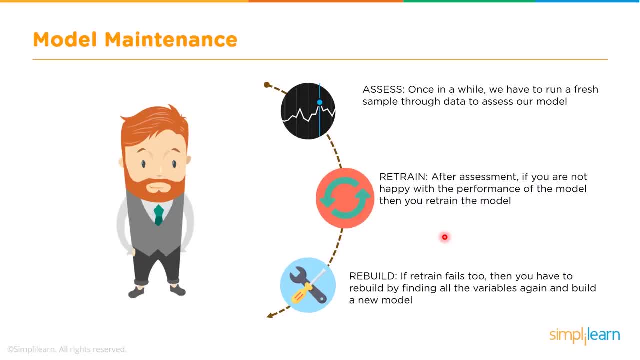 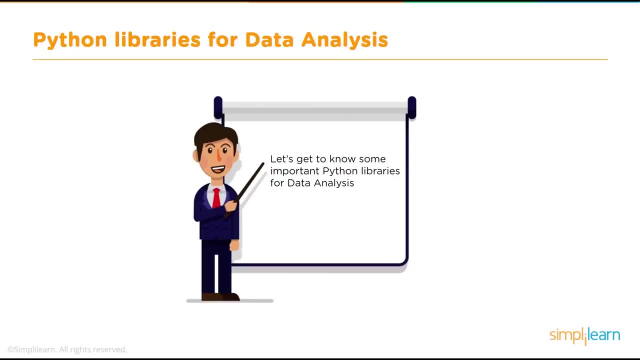 like the maintenance cycle that you may have to take the model through. let's take a look at what are the various libraries that are available. so python is a very easy language to learn and there are some basic stuff that you can do, for example, adding or printing a hello world statement, and. 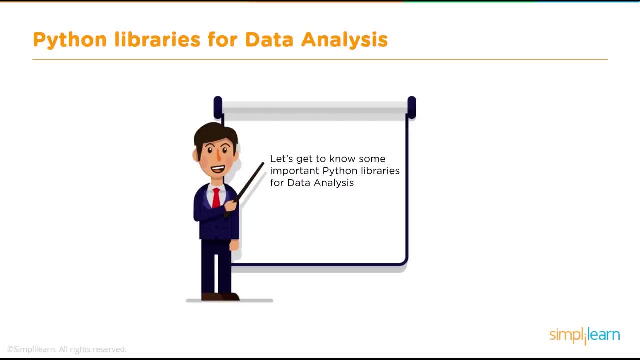 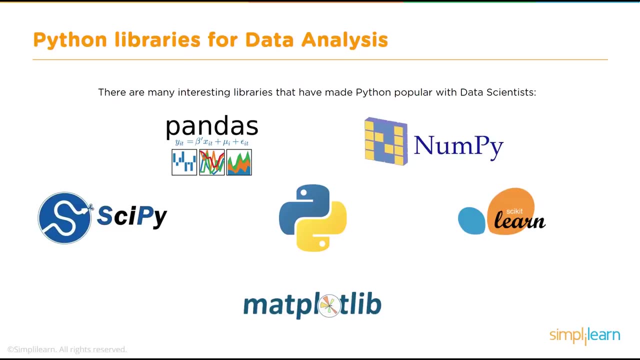 so on, without importing any specific libraries. but if you want to perform data analysis, you need to include or import some specific libraries. so we are going to talk about those as we move forward. so pandas, for example, is used for structured data operations. so if you, let's say, are performing something on a csv file, you import a csv file, create a data frame and then 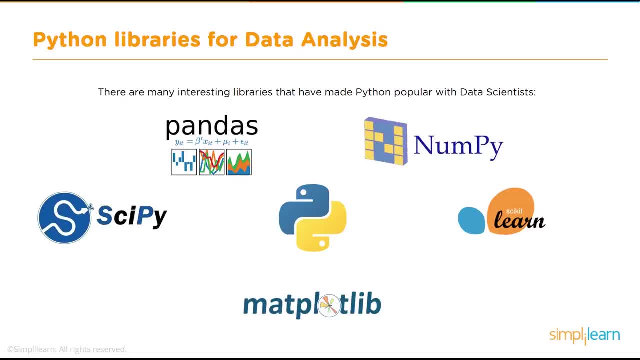 you can do a lot of stuffs like data munging and data preparation before you do any other stuff like, for example, machine learning or so on. so that's pandas scipy, as the name suggests it is kind of. it provides more scientific capabilities, like, for example, it has linear algebra, it has 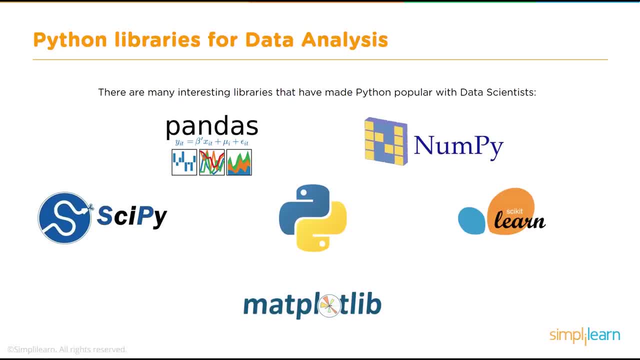 fourier transform, and so on and so forth. then you have numpy, which is a very powerful library for performing n-dimensional or creating n-dimensional arrays, and it also has some of the stuff that is there in sci-fi, like, for example, linear algebra and Fourier transform, and so on and so forth. then you have matplotlib, which 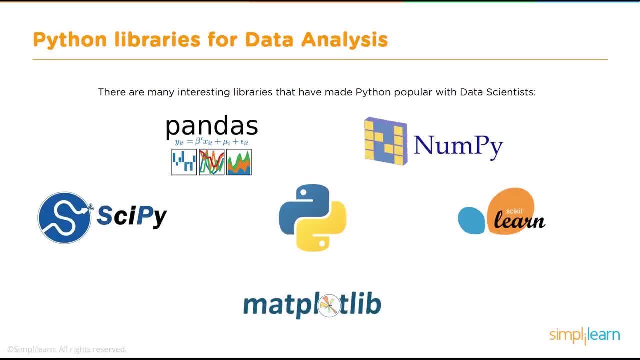 is primarily for visualization purpose. it has, again, very powerful features for visualizing your data, for doing the initial what is known as exploratory data analysis, for doing univariate analysis, bivariate analysis. so this is extremely useful for visualizing the data. and then scikit-learn is used for. 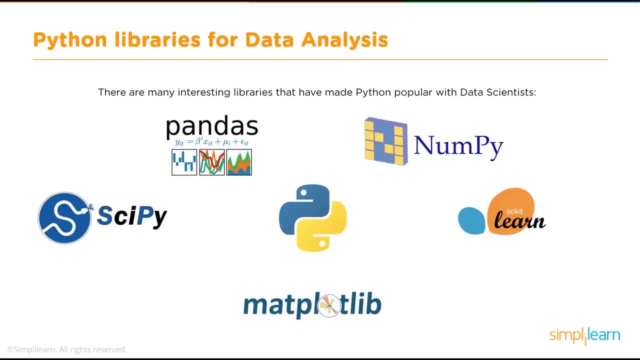 performing all the machine learning activities. if you want to do anything like linear regression, classification or any of this stuff, that the scikit-learn library will be extremely helpful. in addition to that, there are a few other libraries, for example networks and iGraph. then, of course, a very important 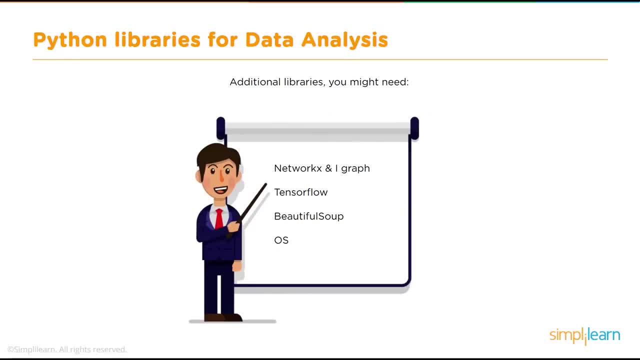 one is tensorflow, so if you are interested in doing some deep learning or AI related stuff, then it would be a good idea to do that, to learn about tensorflow, and tensorflow is one of the libraries. there is a separate video on tensorflow. you can look for that, and this is one of the 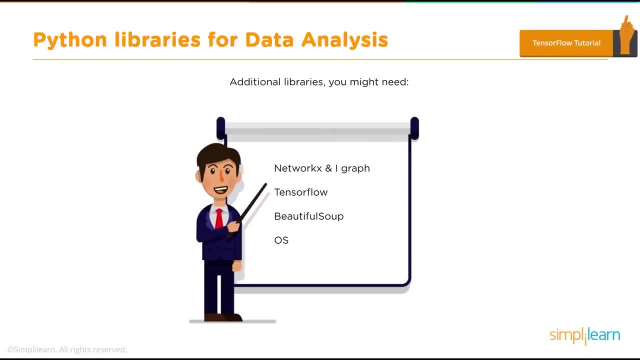 libraries created by Google open source library. so once you are familiar with machine learning, data analysis, machine learning, then that may be the next step to go to deep learning and AI, so that's where tensorflow will be used. then you have beautiful soup which is primarily used for web scraping. and then you take 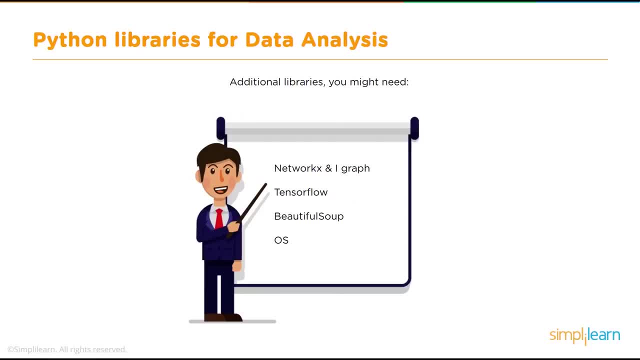 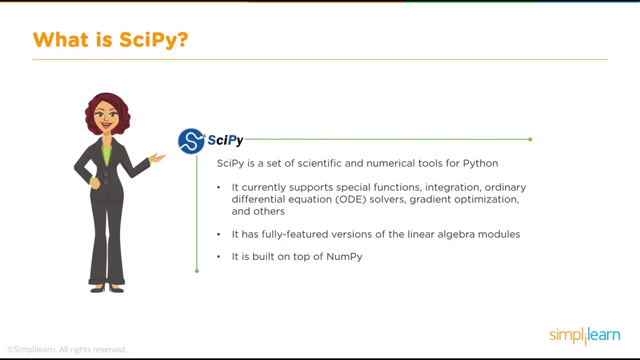 the data and then analyze and so on, then OS library is a very common library as an operating system. so if you want to do something on creating directories or folders and things like that, that's when you would use OS, all right. so, moving on, let's talk in a little bit more detail about each of these libraries. so scipy. 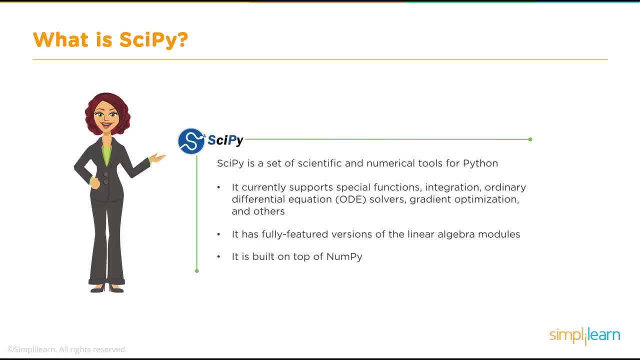 as the name suggests, is a scientific library and it very specifically it has some special functions for integration and for ordinary differential equations. so, as you can see, these are mathematical operations or mathematical functions and so these are readily available in this library. and it has linear algebra modules and it is built on top of numpy, so we will see what is there in numpy. so 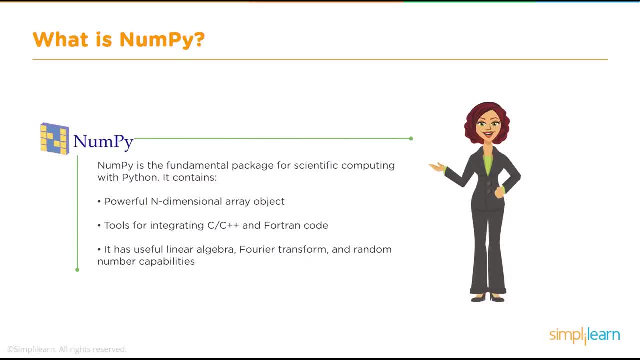 this is a. again, as the name suggests that num comes from numbers, so it is a mathematical library, and one of its key features is availability of an n-dimensional array object. that is a very powerful object and we will see how to use this. and then, of course, you can create other let's objects and so on, and 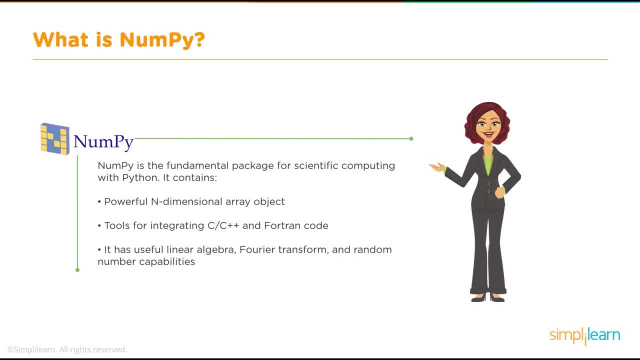 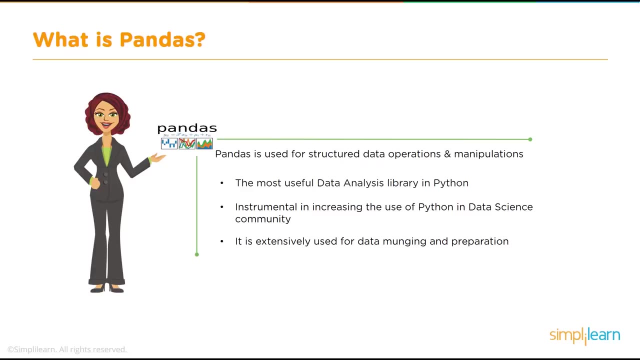 it has tools for integrating with C, C++ and also for trancode, and then it of course also has linear algebra and Fourier transformation and so on. all these scientific capabilities. okay, what else? pandas is another very powerful library, primarily for data manipulation. so if you are importing any files, you 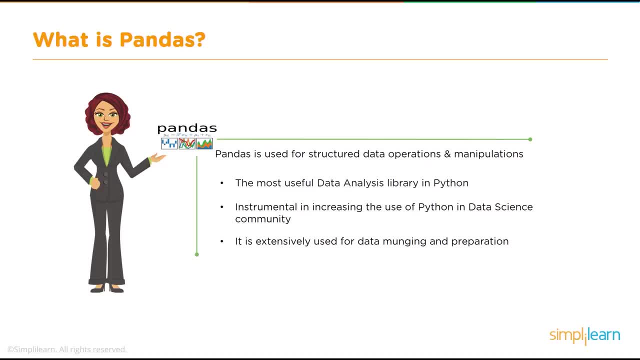 will want to create it like a table, so you will create what is known as data frames. these are very powerful data structures that are used in python, so pandas library provides this capability and once you import a data, input the data into data frame, you can pretty much do whatever you're doing. 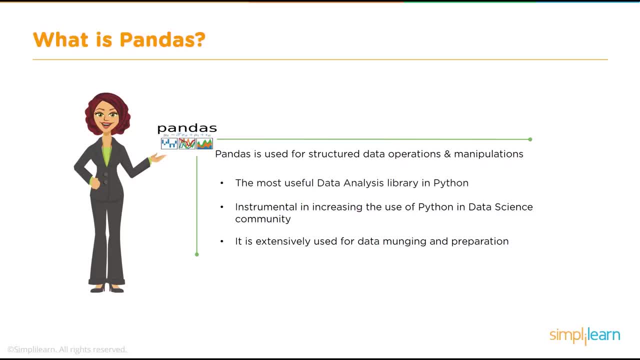 like in a regular database of people who are coming from a database background or SQL background, would really like this because it is very they will feel very much at home because it feels like you're using, you're viewing a table or using a table and you can do a lot of stuff using the pandas library now there. 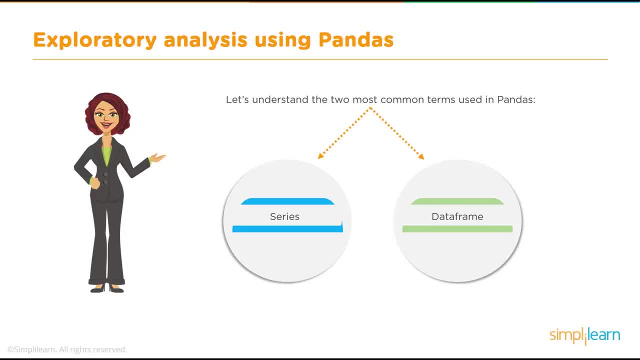 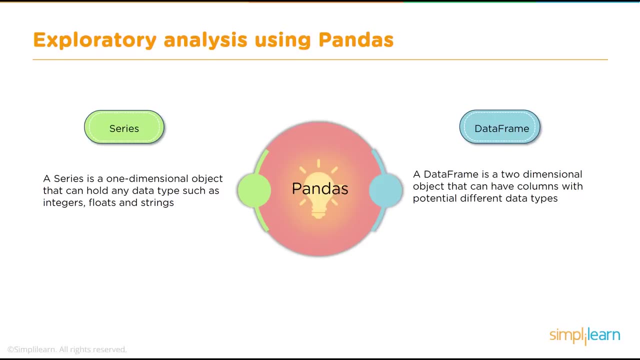 are two important terms or components in pandas: series and the data frame. i was just talking about the data frame, so let's take a look at what are series and what is a data frame. so within pandas, we have series and data frame. so series is primarily- some of you may also be knowing this- as, let's say, an array, so it's a. 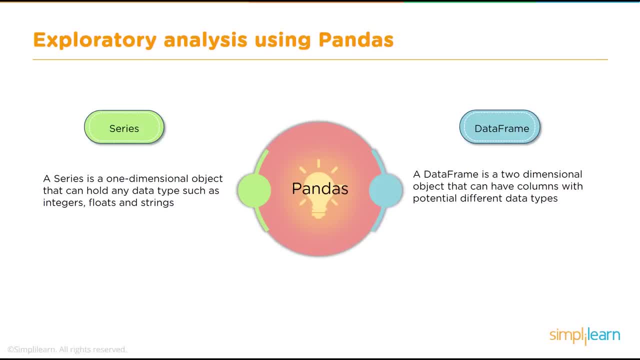 one-dimensional structure, data structure, if you will. so in some other languages we may call it as an array or maybe some others probably an equivalent of a list in r. perhaps i'm not very sure on that aspect, but yes, so this is like a one-dimensional storage of information, so that 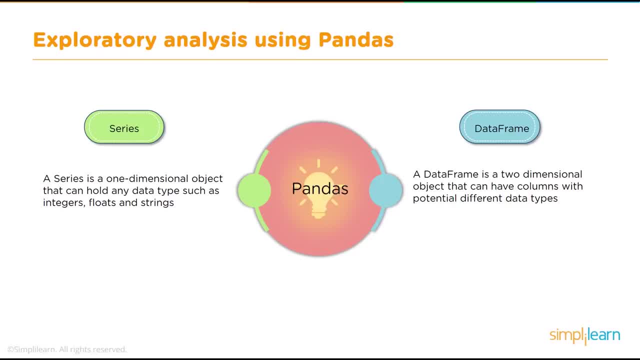 is what is series, whereas data frame is like a table. so you have a two-dimensional structure: you have rows and you have columns, and this is very people, as i said, who are familiar with sql and databases will be able to relate to this very quickly. so you have like a table, you have rows and 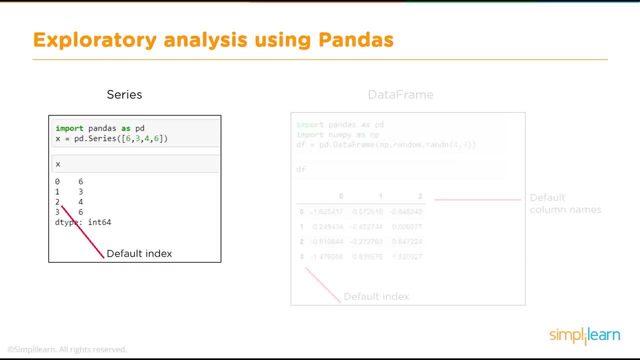 columns and then you can manipulate the data. so, if you want to create a series, this is how you would create a code snippet and, as you can see, the programming in python is very simple. there are no major overheads. you just need to import some libraries, which are essential, and then start. 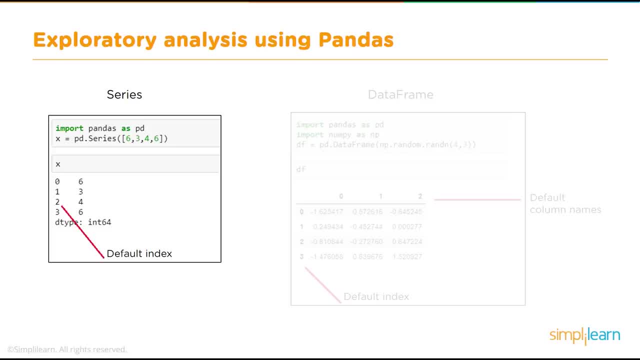 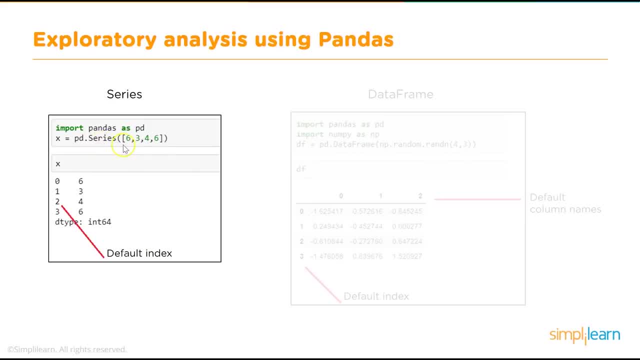 four, five, six, three, four, five, six, three, four, six, and x is my object, consisting of the series. so if you display, if you just say x, it will display the contents of x and you will see here that it creates a default index. then you have data frame. so if you want to create a data frame, as you can see the 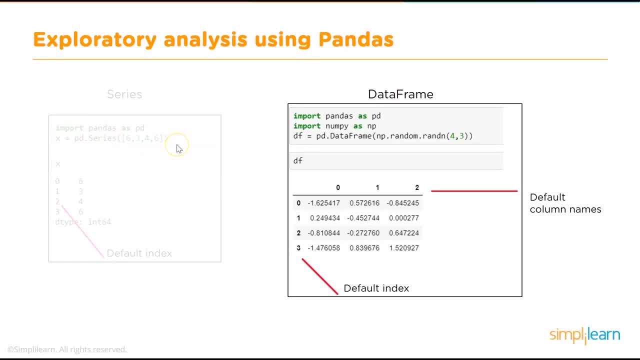 series is like a one-dimensional structure. there is just like a row, one row of items, whereas a data frame looks somewhat like this: it is a two-dimensional structure, so you have columns in one dimension and then you have rows in the other dimension. how do you create a data frame? you can. 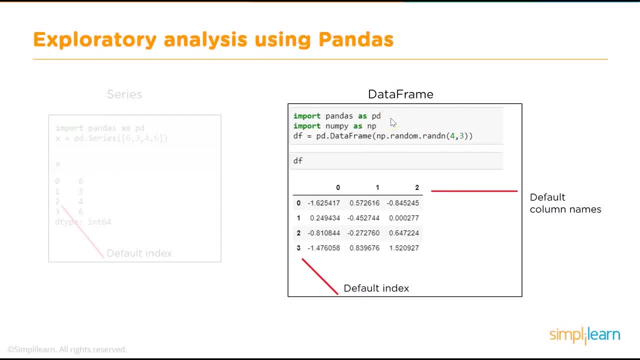 create a data frame. you need to create, you need to rather import pandas and then you import. in this case, we are basically creating our own data. so that's the reason we are importing numpy, which is one of the libraries we just referred to a little bit before. so we are using one of the 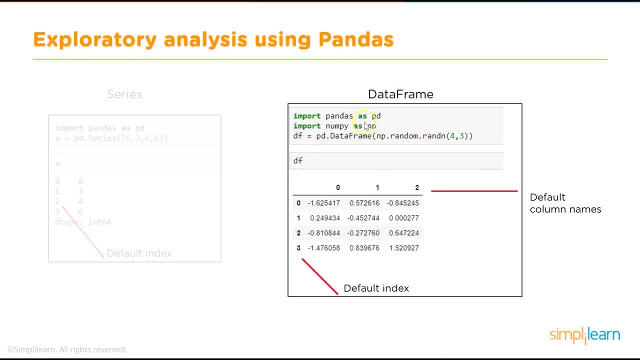 functionalities within numpy to create some random numbers. otherwise this is not really mandatory. you probably will be importing the data from outside- maybe some csv file- and import into the data frame. so that's the reason. we are importing numpy from outside- maybe some csv file- and import into the data frame. so that's. 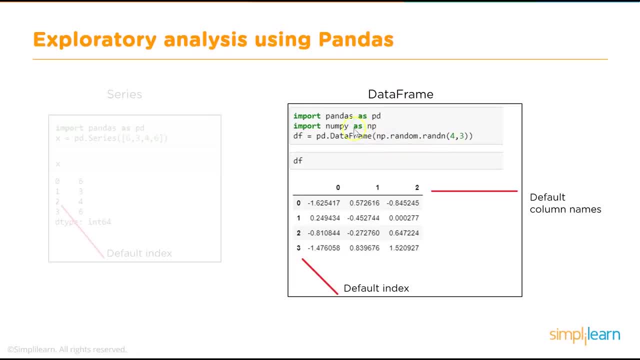 what we are doing here. so in this case we are creating our own test data. that's the reason we are importing numpy as np, and then i create a data frame saying pd dot data frame. so this is the keyword here. similarly, here in this case, while creating series, we said pd dot series and then 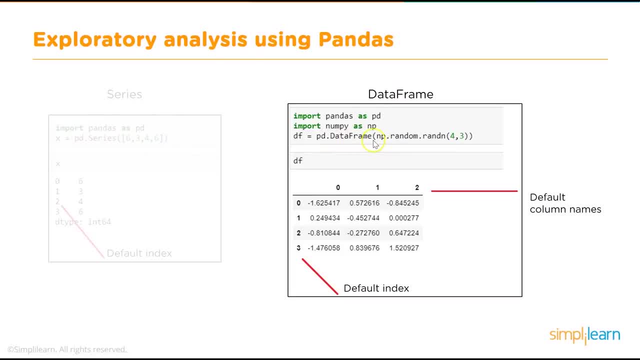 you pass the values. similarly, here you're saying pd, dot data frame. now, in order to create the data frame, it needs the values in each of these cells. what are the values in the rows and what are the values in the column, so that, in our example, we are providing using this random number of values? 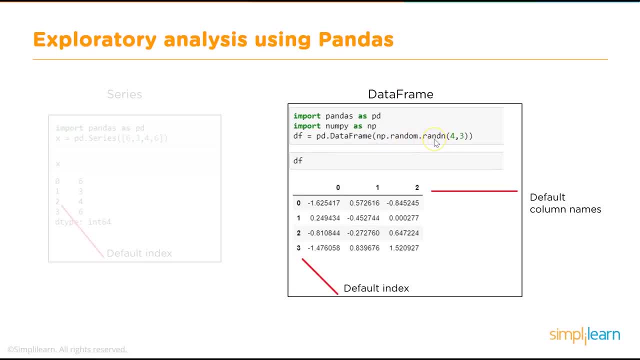 random number generator. so np, dot random is like a class or a method that is available in numpy and then you are saying, okay, generate some random numbers in the form of a 4 by 3 matrix or 4 by 3 data frame. the 4 here indicates the number of rows and the 3 here indicates the 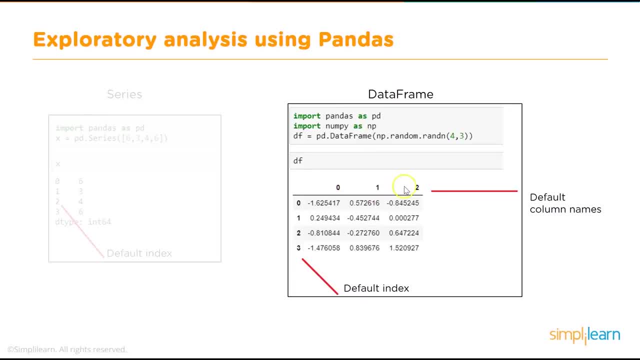 number of columns. so these are the columns: 0, 1, 2 are the columns and these are the rows here: 0, this is 1, this is 2, this is 3. okay, and once again it will. when you display df, it will give us a default index. there are ways to omit that, but 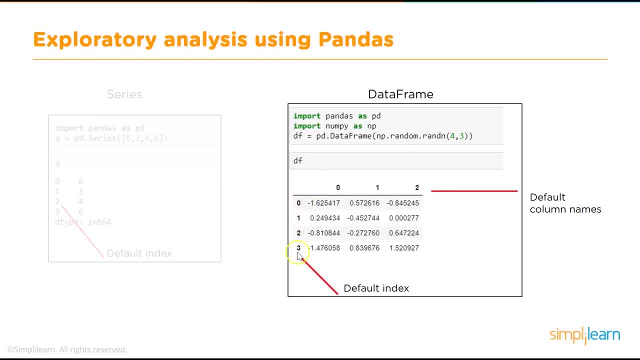 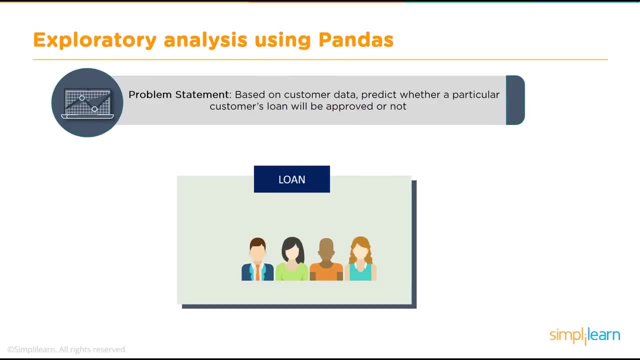 at this point we will just keep it simple. so it will display the default index and then the actual values in each of these rows and columns. so this is the way you create a data frame. so now that we have learned some of the basics of pandas, let's take a quick look at how we use this in real life. 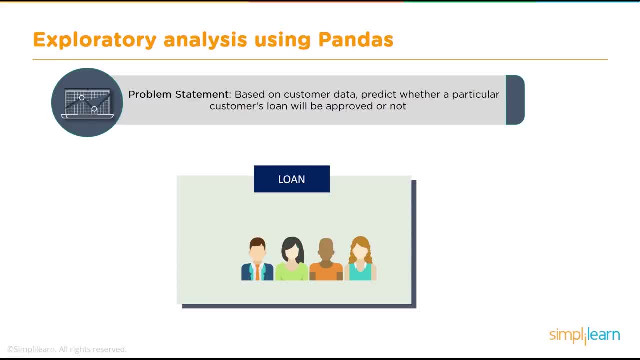 so let's assume we have a situation where we have some customer data and we want to kind of predict whether a customer's loan will be approved or not. so we have some historical data about the loans and about the customers and using that we will try to come up with a way to maybe predict whether 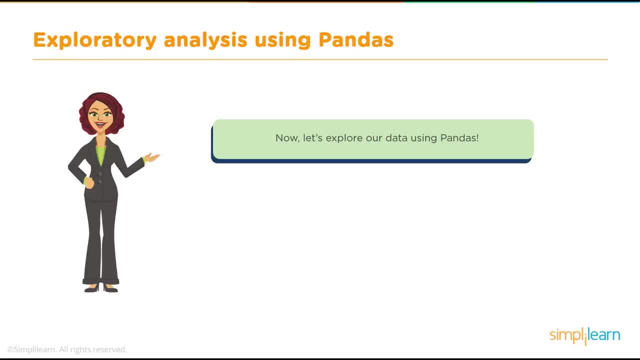 loan will be approved or not. so let's see how we can do that. so this is a part of exploratory analysis. so we will first start with exploratory analysis. we will try to see how the data is looking. so what kind of data? so we will, of course, i'll take you into the jupyter notebook and give you a. 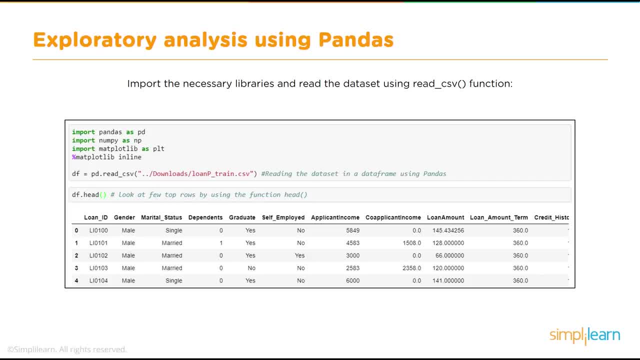 quick live demo, but before we do that, let's take a look at some of the data that we have here. so we will. of course, i'll take you into the jupiter notebook and give you a quick live demo, but before that, let's quickly walk through some of the pieces of this program in slides, and then i will. 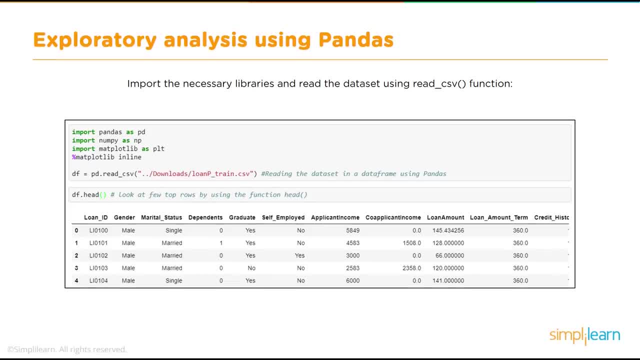 take you actually into the actual code and do a demo of that. so the python program structure looks somewhat like this. the first step is to import your all the required libraries. now, of course it is not necessary that you have to import all your libraries right at the top of the code. 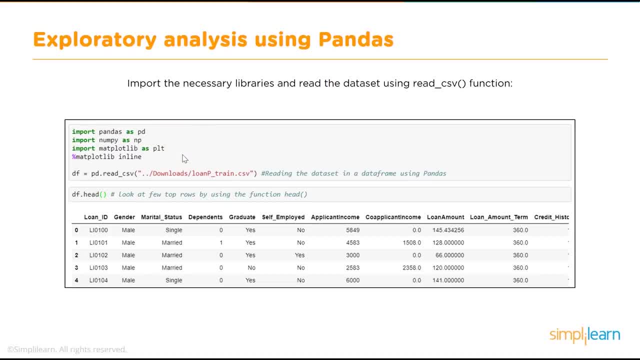 but it is a good practice. so you, if you know you are going to need a certain set of libraries, it may be a good idea to put from a readability perspective. it's a good practice to put all the libraries that you're importing at the beginning of your code. however, it is not mandatory, so in 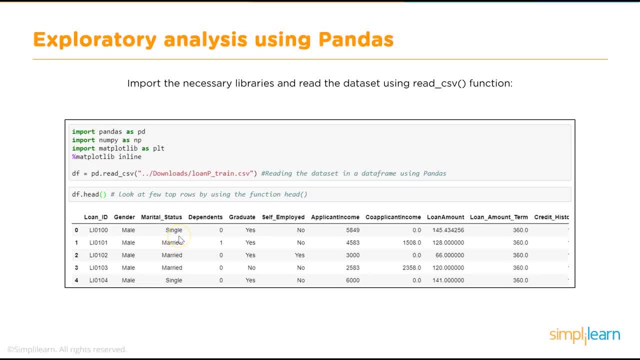 the middle of the code somewhere. if you feel that you need a particular library, you can import that library and then start using it in the middle of the code. so that's also perfectly fine. it will not give any errors or anything. however, as i said, it's not such a good practice, so we will. 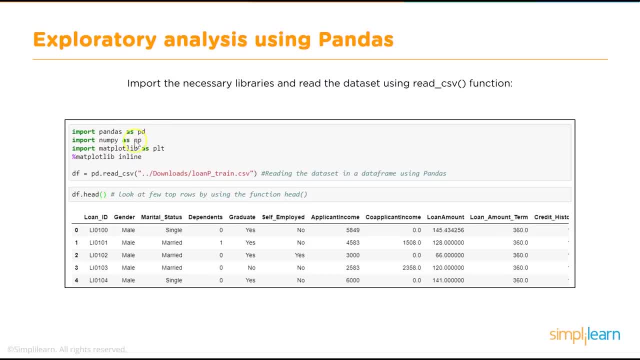 import all the required libraries. in this case we are importing pandas, numpy and other libraries and matplotlib and, in addition, if we include this piece of code- percentage matplotlib- inline, what will happen is all the graphs that we are going to create, the visualizations that we are going to create, will be displayed within the notebook. so if you want to have that kind of a, 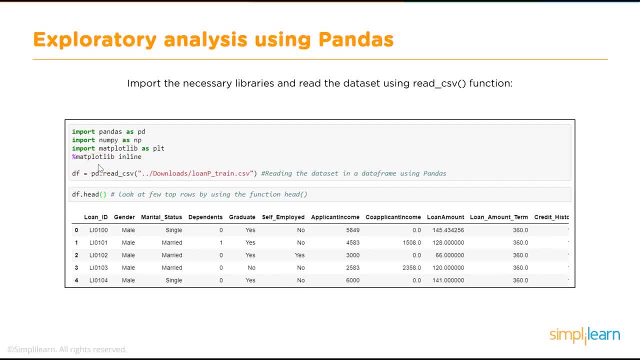 provision. you need to have this line, so it's always a good idea when you're starting off. i think it's a good idea to just include this line so that your graphs are shown in line. okay, so these are the graphics that we are going to use for the program, so that you are going to do that. 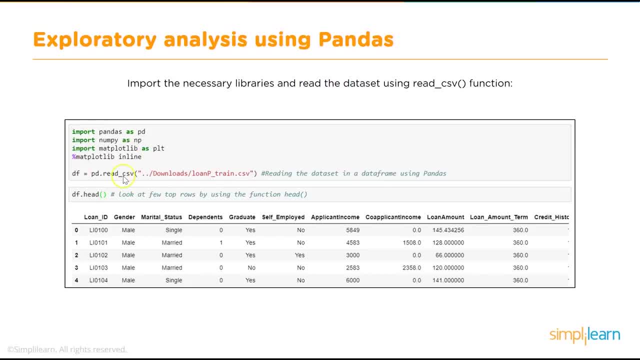 the four. we will start with these four lines of code. then the next step is to import your data. so in our case, there is a training data for loans by the name loan, pe, underscore, train, dot csv, and we are reading this data. so in this case, you see here, unlike the previous example where we created a 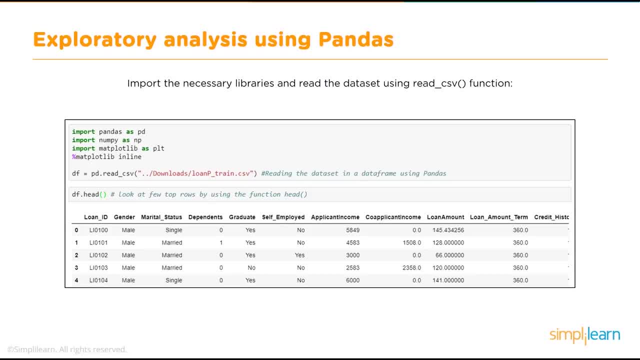 data frame with some data that we created ourselves. here we are actually creating a data frame using some external data, and it's. the method is very, very straightforward. so you use the read underscore csv method and it is a very intuitive function name and you say pd dot. 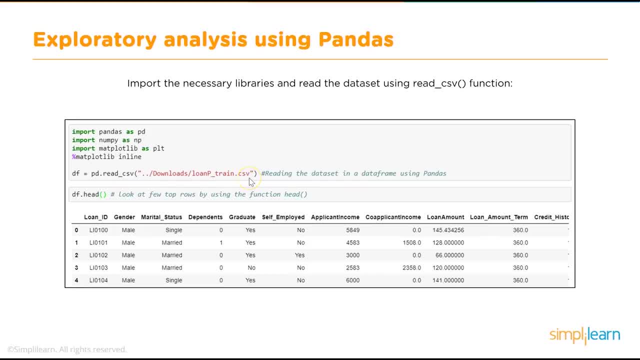 read underscore csv and give the path of the file: csv, file, that's about it and then that is read into the data frame df. this can be any name we are calling it df. you can call xyz anything. there's a name, just name of the object. so head is one of the 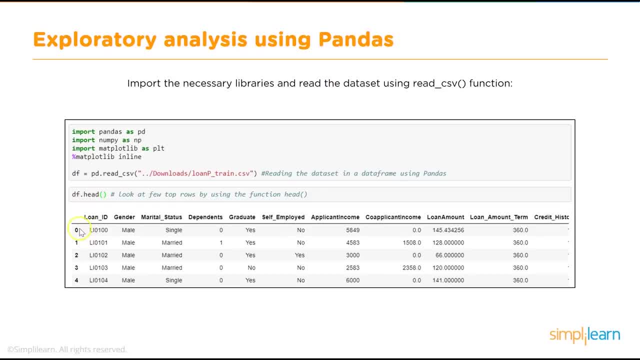 methods that we are going to use to create a data frame. so we are going to create a data frame and so we are going to create a data frame and it will give us the first five. so this is just to take a quick look. now you have imported the data, you want to initially have a quick look. 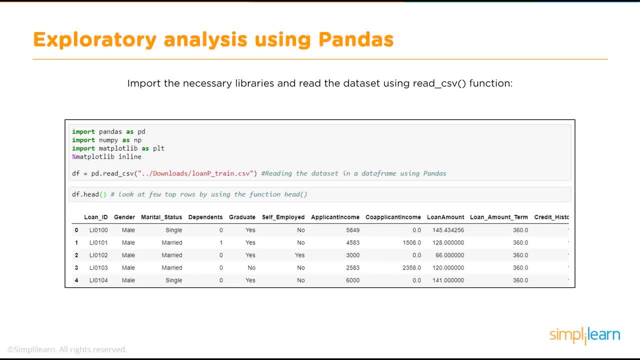 how your data is looking, what are the values in some of the columns and so on and so forth. right, so typically you would do a head df, dot head to get the sample of, let's say, the first few lines of your data. so that's what has happened here, so it displays the first few lines and then 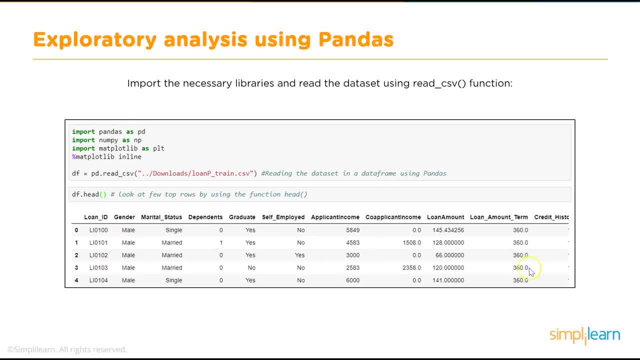 you can see what are the columns within that and what are the values in each of these cells, and so on and so forth. you can also, typically you would like to see if there are any null values, or are there any? is the data, for whatever reason, is invalid or looking dirty for? 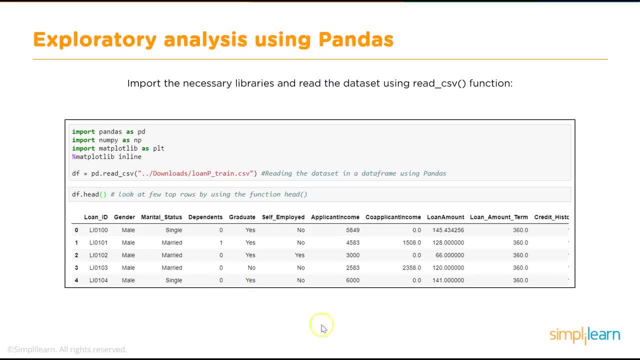 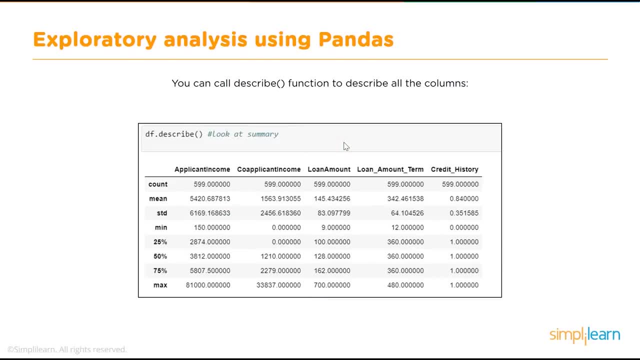 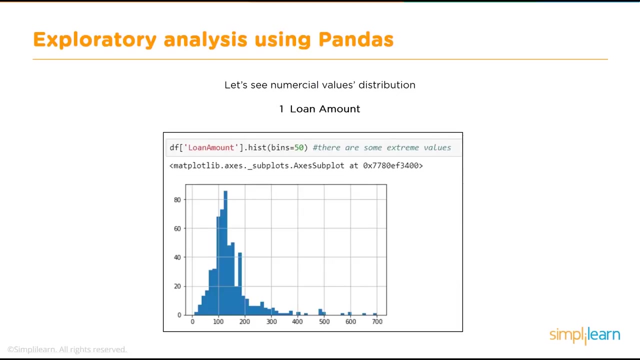 whatever reason, some unnecessary character. so this will give a quick view of that. so in this case, pretty much everything looks okay. then the next step is to understand the data a little bit overall. for each of the columns, what is the information? so the describe function will basically give us a summary of the data. what else can we do? pandas also allows us to visualize. 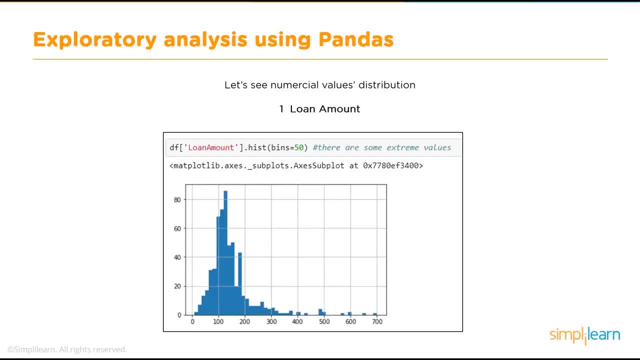 the data and this is more like a part of what we call it as univariate analysis. that means each and every column you can take and do some plots and visualization to understand data in each of the columns. so for example, here the loan amount column we can take and then the hist. 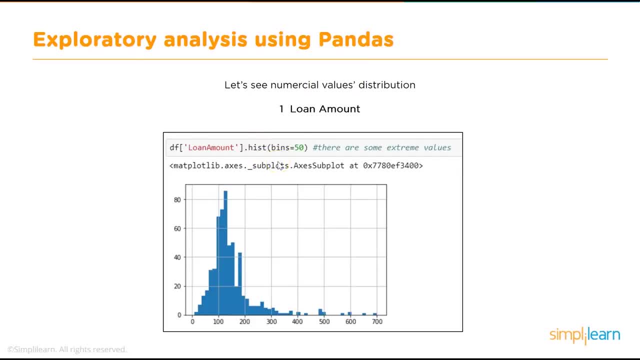 basically, hist method will create a histogram. so you take all the values from one column, which is loan amount, and you create a histogram to see how the data is distributed. right? so that's what is happening here and, as you can see, there are some extreme values. so this is again to identify. 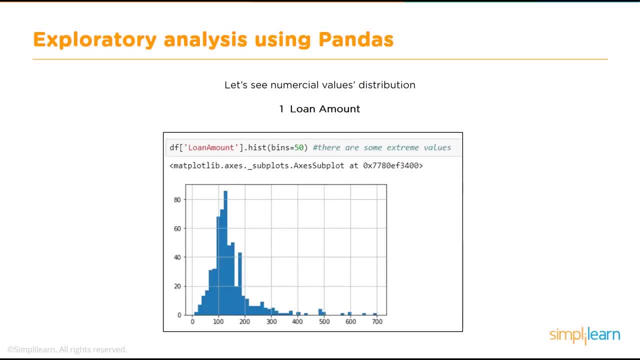 do we have to do some data preparation? because if the data is in a completely haphazard way the analysis may be difficult. so with these are the initial or exploratory data. analysis is primarily done to understand that and see if we need to do some data preparation before we get into the other. 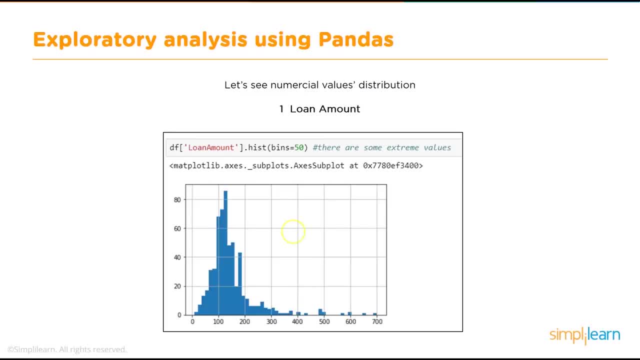 categories. so in this case we will see that here by plotting this histogram we see that there are some extreme values. so there are some values, a lot of it is around 100 range, but there is also something of one or two observations in the 700 range. so it's pretty scattered in that sense, or 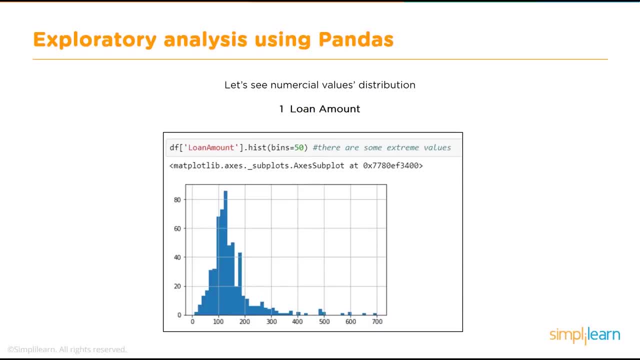 they're not really scattered- distributedly scattered, but it is randomly scattered, so the range is really huge. so what can we do about this? so there are some steps that we need to do- normalization and so on. so we'll see that in a bit. so this is a very simple way to understand that. 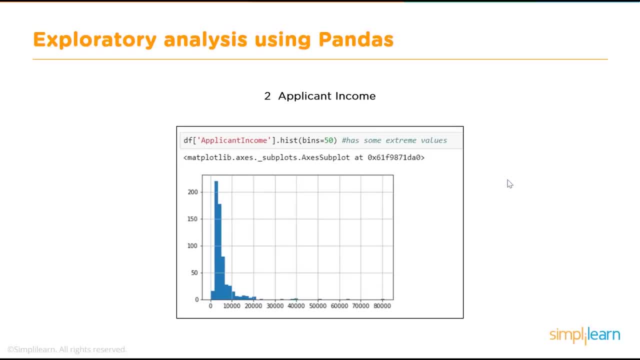 this is for one of the columns. let's take another column, which is applicant income. similar kind of similar situation. you have most of your observations in this range, but there are also some which are far off from where most of the observations are. so this is also pretty, this also. 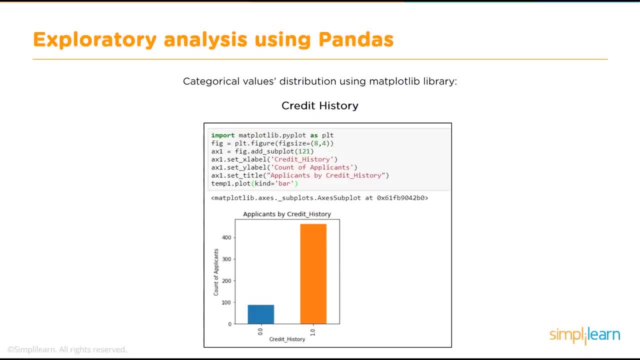 has some extreme values, so we'll have to see what can be done. credit history is the binary value, so some people have a zero value and some will have credit history of one. this is just like a flag, so this basically is telling us how many people have. 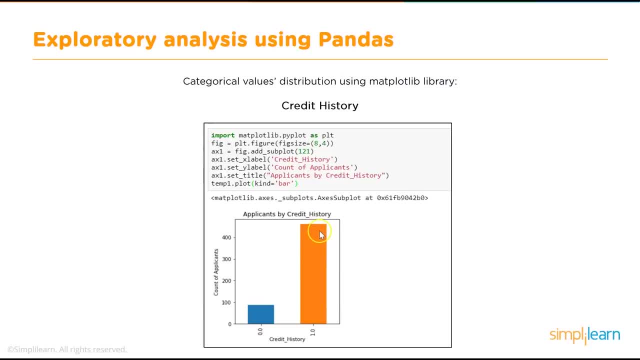 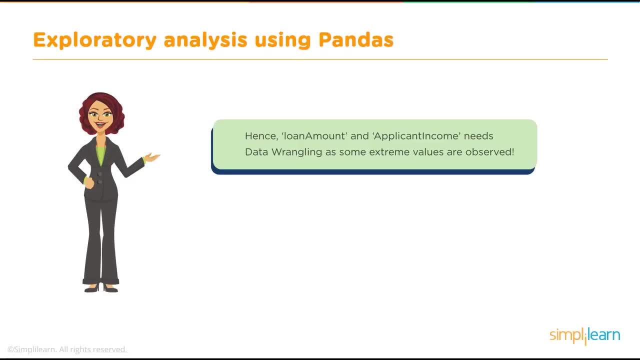 a one, and how many people have zero. so looks like majority of them have a value of one and a few- about hundred of them- have a value of zero. okay, what else can we do? so we now understood a little bit about the data, so we need to do some data wrangling or data munging and see if we can. 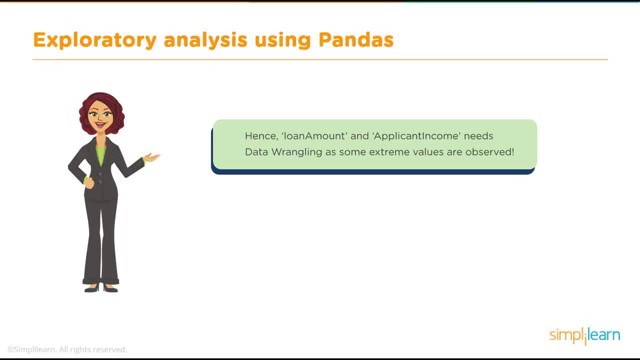 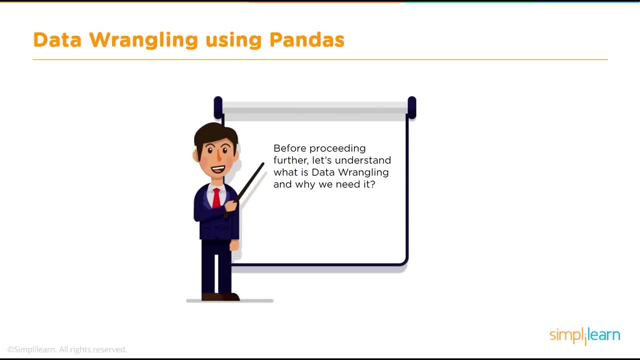 some bring in some kind of normalization of all this data, and we will kind of try to understand what is data wrangling and before we actually go into it. okay, so data wrangling is nothing but a process of cleaning the data, if let's say there are there. 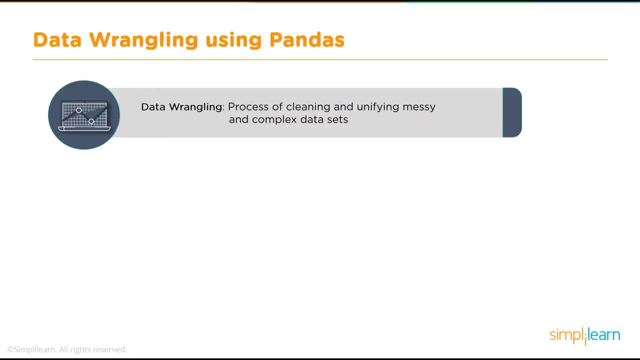 are multiple things that can happen. in this particular example, there were no missing values, but typically when you get some data, very often it will so happen that a lot of values are missing. either they are null values or there are a lot of zeros. now you cannot use such data as it is. 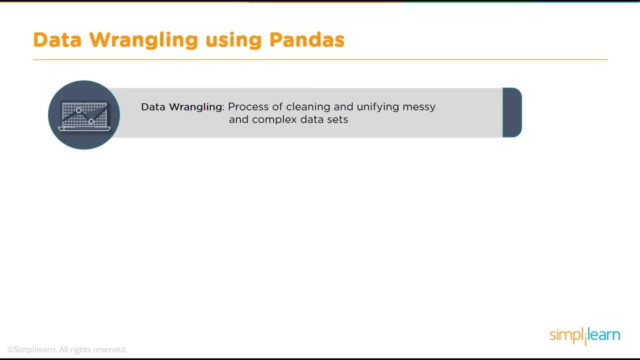 to perform some, let's say, predictive analysis, or perform some machine learning activities and so on. so that is one part of it. so you need to bring in the data. the other is unifying the data. now, if these ranges of this data are very huge, some of them are going from. some columns are going from zero to 100 000 and some columns are just. 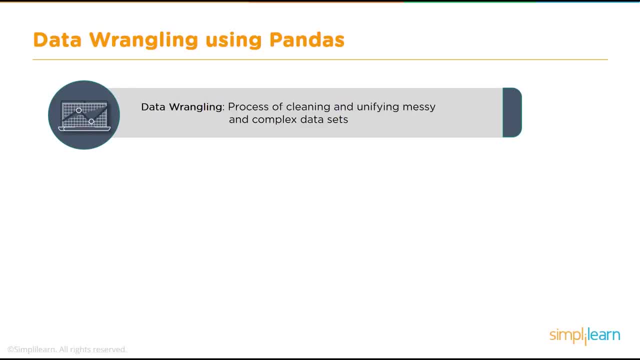 between 10 to 20 and so on. these will affect the accuracy of the analysis. so we need to do some kind of unifying the data and so on. so that is what wrangling data wrangling is all about. so before we actually perform any analysis, we need to. 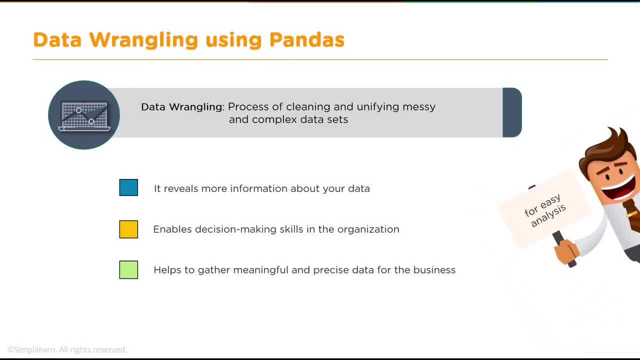 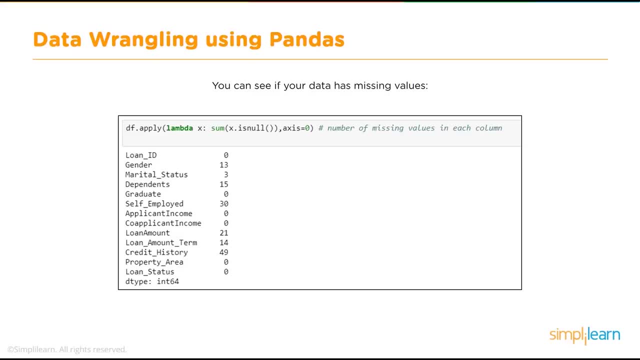 bring in the data so to some kind of a shape so that we can perform additional analysis, actual analysis on this and get some insights. now, how do we deal with missing values is a very common issue when we take data or when we get data from the business, when a data scientist gets the data. 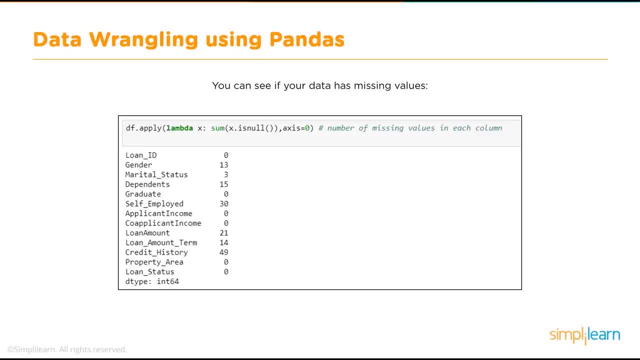 from the business. so we should never assume that all our data will be clean and all the values filled up and so on, because in real life very often there will be the data will be dirty. so data wrangling is the process where you can do that. so now let's talk about data wrangling. 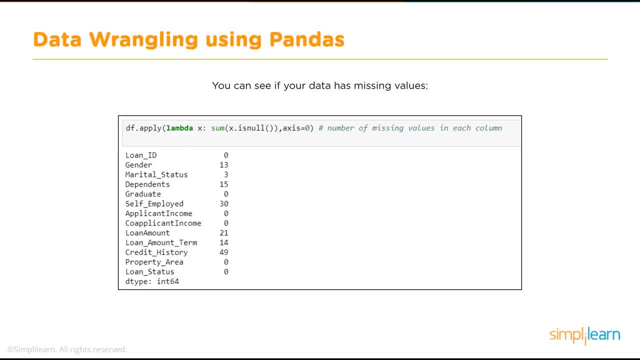 of clean up the data: first of all identify whether the data is dirty and then clean up. so how do we find some data is missing? so there are a few ways. you can write a small piece of code which will identify if, for a given column or for given row, any of the observations are null. 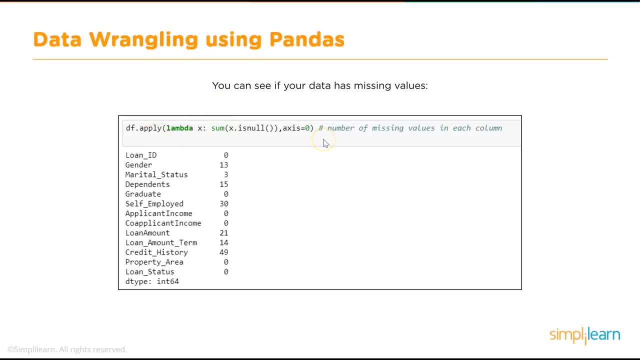 primarily so. this line of code, for example, is doing that. it is trying to identify how many null values or missing values are there for each of the columns. so this is a lambda function, and what we are saying is find out if a value is null, and then 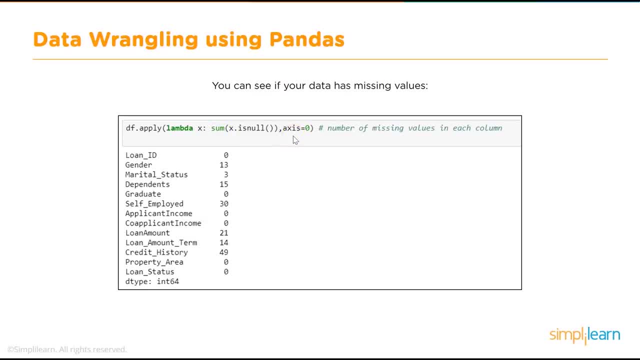 you add all of them, how many observations are there where this particular column is null? so it does that for all the column. so here you will see that for loan id, obviously it's an id, so there are no null values or missing values. gender has about 13 observations where the values are missing. 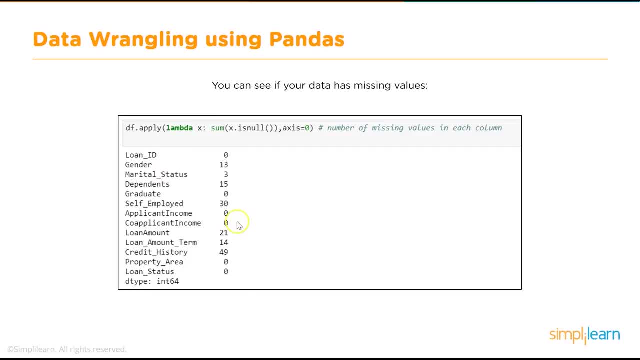 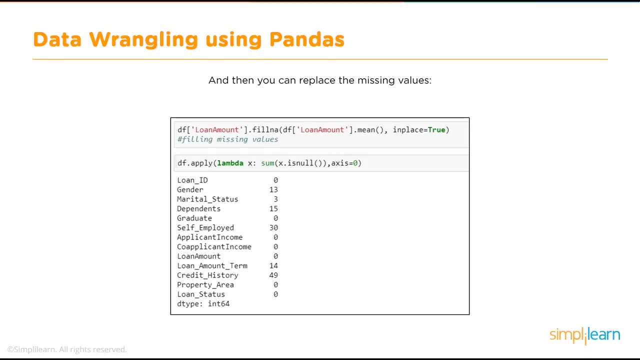 similarly, marital status has 3 and so on and so forth. so we'll see here, for example, loan amount: the values are missing. loan amount term has 14 observations and so on. so we'll see how to handle this. missing values. so there are multiple ways in which you can handle missing values. if the 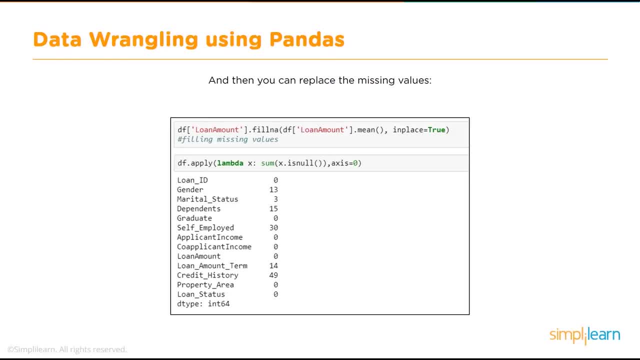 number of observations are very small compared to the total number of observations, then sometimes one of the easy ways is to completely remove that data. so or delete that record, exclude that record, so that is one way of doing it. so if there are, let's say, a million records, and maybe 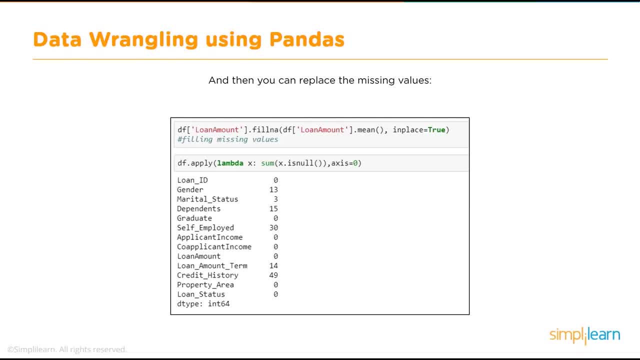 records are having missing values, it may not be worth doing something to fill up those values. it may be better off to get rid of those observations right. so that is, the missing values are proportionately very small. but if there are relatively large number of missing values, if 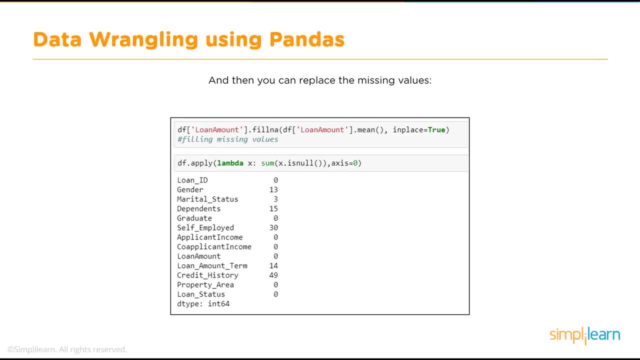 you exclude those observations, then your accuracy may not be that very good. so there, the other way of doing it is we can take a mean value or for a particular column and fill up wherever there are missing values. fill up those observations or cells with the mean value. 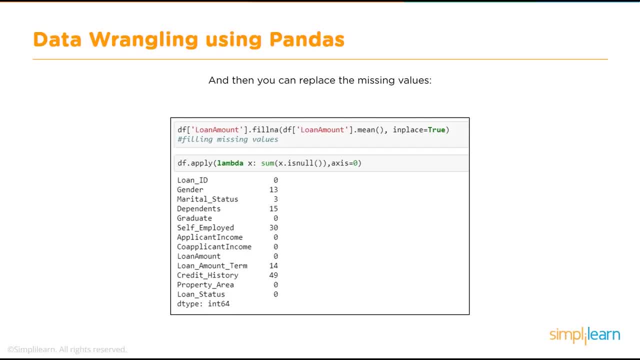 so that way, what happens is you don't give some value which is too high or too low and it somehow fits within the range of the observations that we are seeing. so this is one technique again there are. it can be case to case and you may have to take a call based on your specific situation. 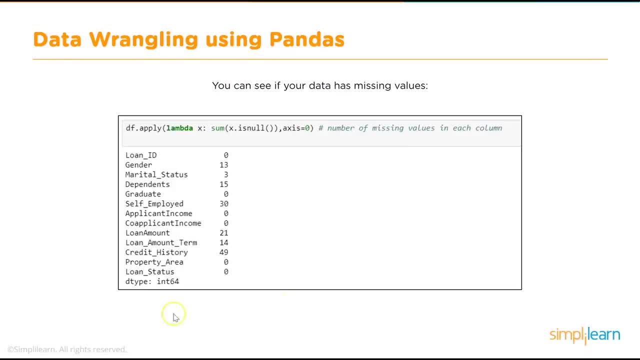 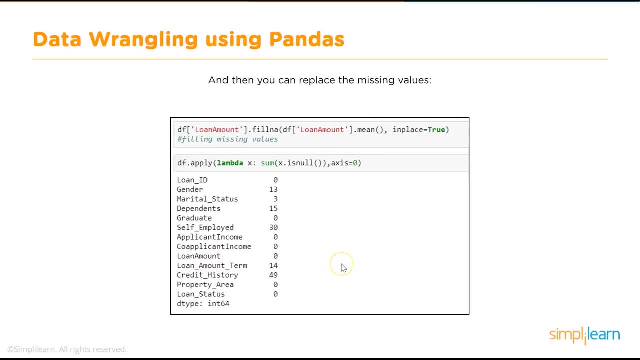 but these are some of the common methods. if you see, in the previous case, loan amount had 21 and we went ahead and filled all of those with the mean value, so now there are zero with missing values. okay, so this is one part of a data wrangling activity. what else you can do, you can also check. 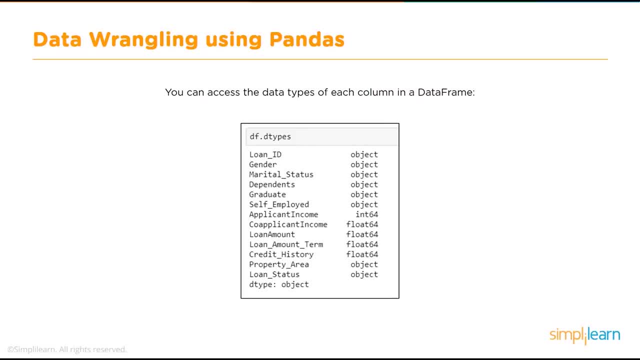 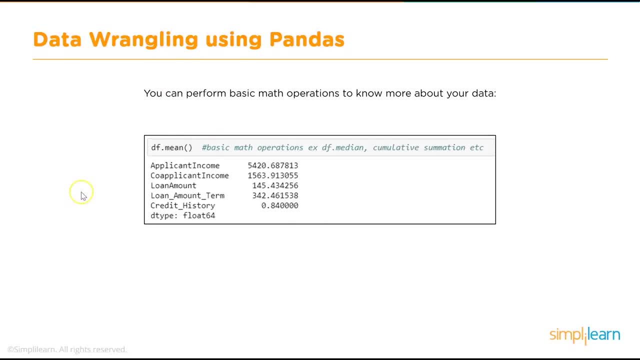 what are the types of the data. so df, dot, d types will give us what are the various data types. so all right, so you can also perform some basic mathematical observations. we have already seen that mean, we found out. so similarly, if you do call the mean method for the data frame object, it will 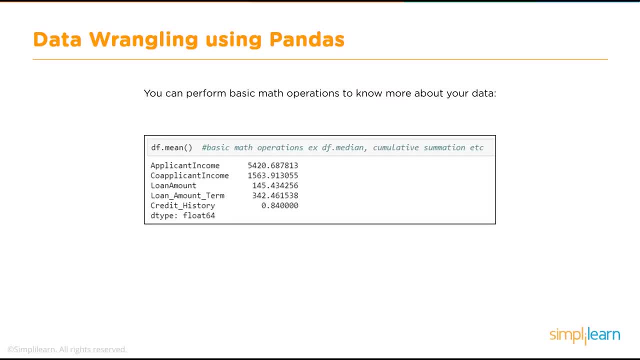 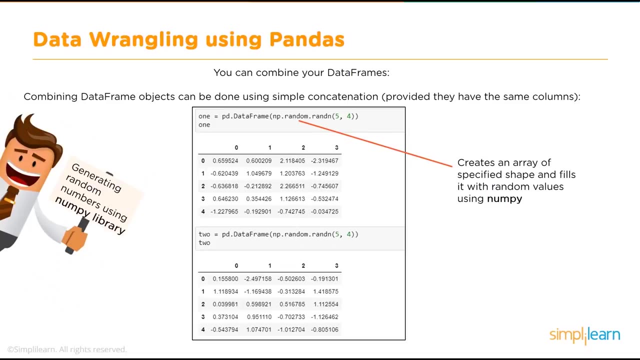 display the experience processing data. now the way data frame is built is to display the mean values on both the data frame and other data a so this will automatically visit and at those eight times it will go wanna look that verse on the data frame. it will consider everything. 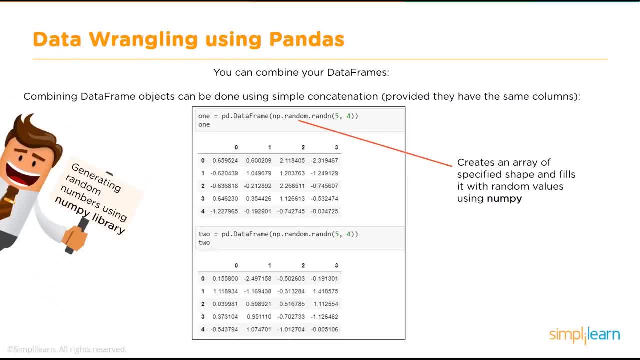 to be the same close. it select the relationship between the data and the numbers on the data frame and see whether it succeeds or it fails, whether it works or it fails, or this is the the empathy grid right here else. Yes, sure, data, okay. one example could be that you have data in the form of csv files, one csv file for each. 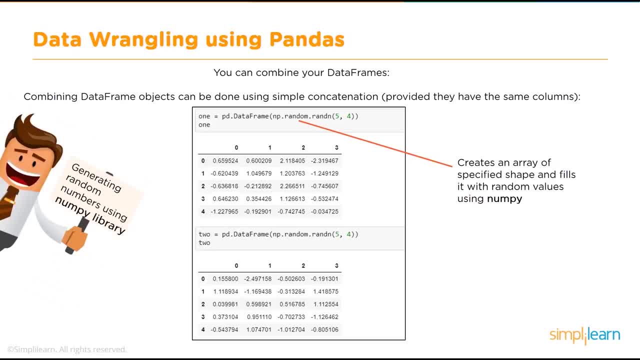 month of the year- january, february, march- each of these are in a different, so you can import them into, let's say, 12 data frames and then you can merge them together as a single data frame and then you perform your analysis on the entire data frame or the entire data for the year. so that is. 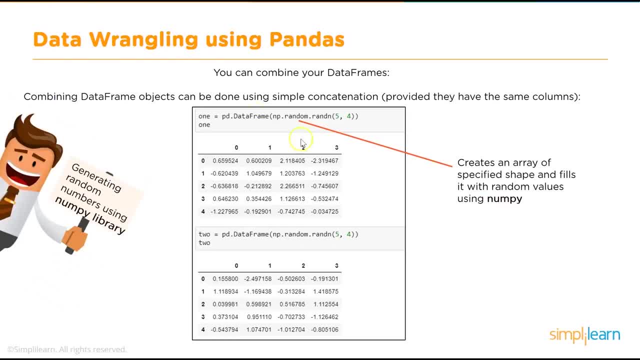 one example. so how do we do that? this is how we do again. in this case we are not importing any data, we are just creating some random values or using some random values. so let's assume i have a data frame which is by the name one and i assign some random values here, which is a five by four format. 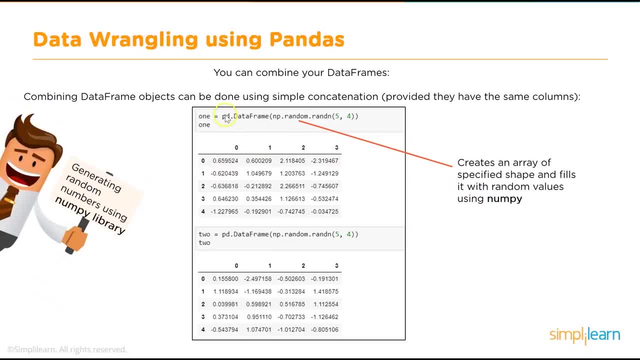 so there are five rows and four columns and this is how my data frame one looks. and then i create another data frame, which is data frame two, again random numbers of the format five by four, and i have something like this. now i want to combine these two. how do i combine these two? 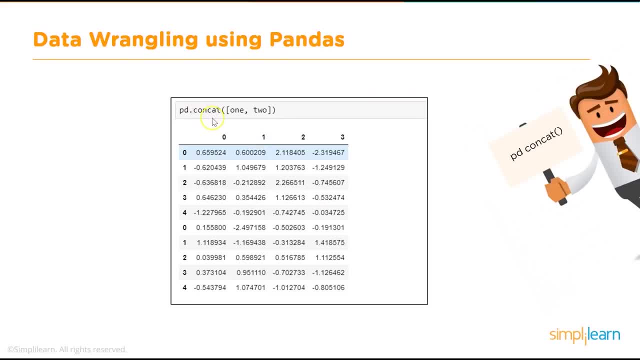 i'm going to do that by using the data frame one and i'm going to do that by using the data frame. i can use the concatenate or concat method and i can combine these two. so pd, dot, concat, and it takes the the data frames one and two. if you have more of them, you can provide them and it will just. 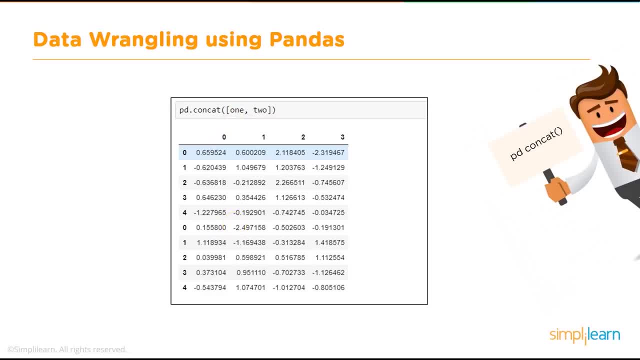 simply add all of them, merge all of them or concatenate whatever you call, whichever term you call, it will. so, of course, we have to make sure that the structure remains the same. like i said, this could be, let's say, sales data coming for 12 different months, but each of the files has the 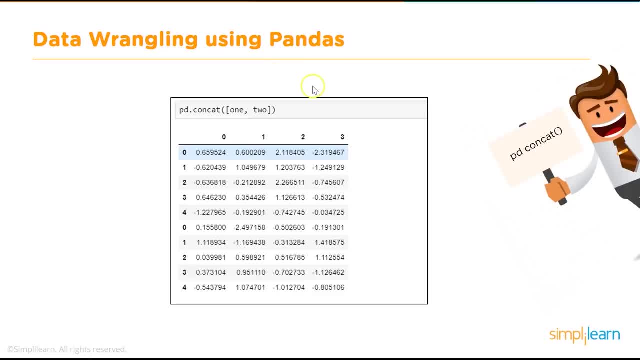 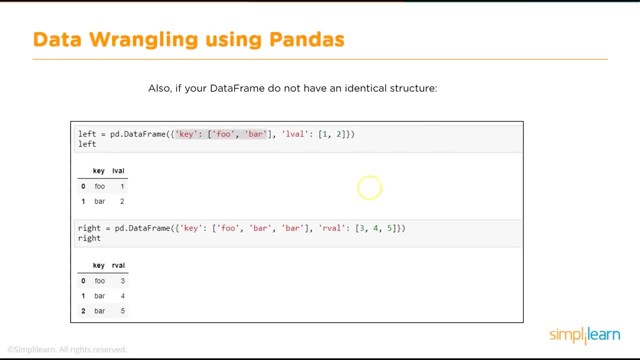 same structure. so now you can combine all of them, merge all of them by using the concat method. if we have, let's say, structure is not identical, then what will happen? let's say we have these two data frames: one has a column by the name key and the second column is lval, and a second data frame. 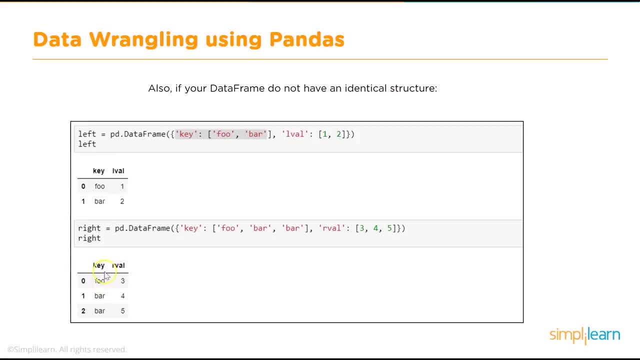 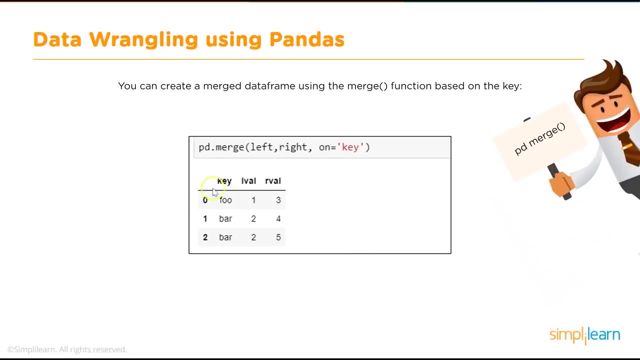 which has a column by the name key but the second column by the name rval, not lval. so you see, here the structure is not identical, so you can still combine them. but then the way they get combined or merged is somewhat like this: so it takes the key as a common parameter between them. some common column has to be there, otherwise this: 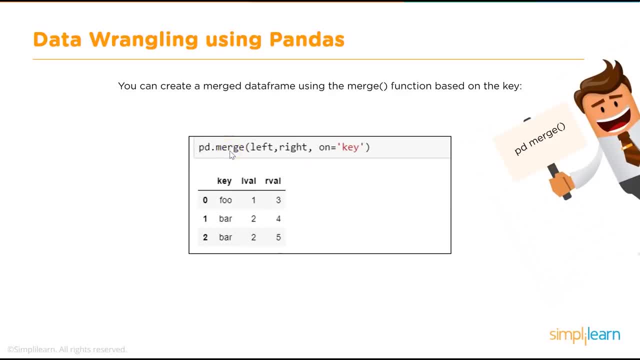 will not work, and then we have to use merge instead of concatenate, and when we do a merge then we get the result will be in this format. what it does is it uses the key as a common thread between them and then it kind of populates the values accordingly. so if you see here, 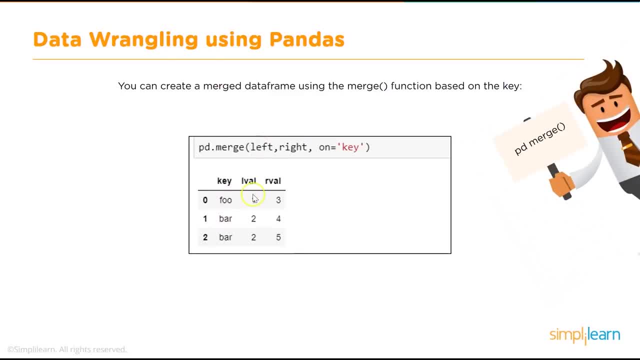 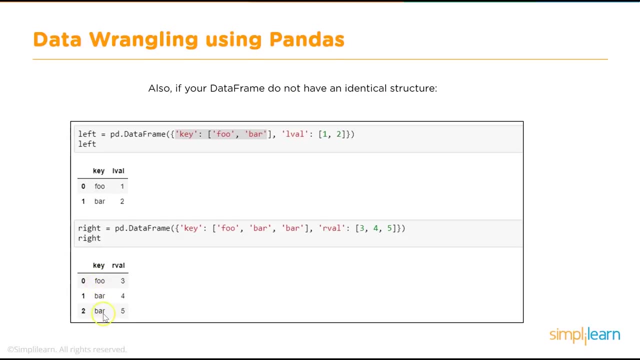 the first one had foo and bar for key and then it had l values of one and two, right. so if we go back, foo and bar had one and two l values. so that's what we see here- one and two, whereas in the right data frame we had foo, bar and bar as a second time, and then r values are three, four and five. so what it? 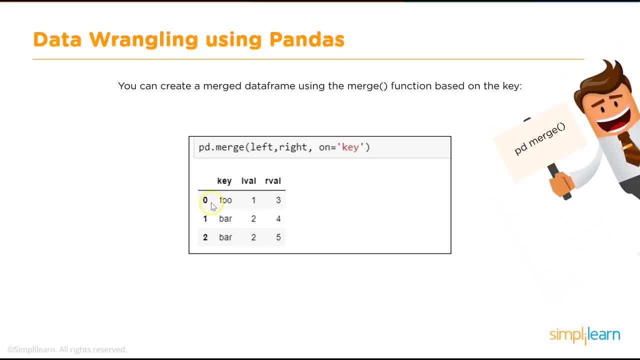 has done for foo. it has put for the existing right, for foo is already existing because it has come from left. so it will just put the value of rval here, which is three. similarly, it will put four here, because for bar, if you go back for bar, it is the value is four and since it has one more value of bar, it will go and add this. 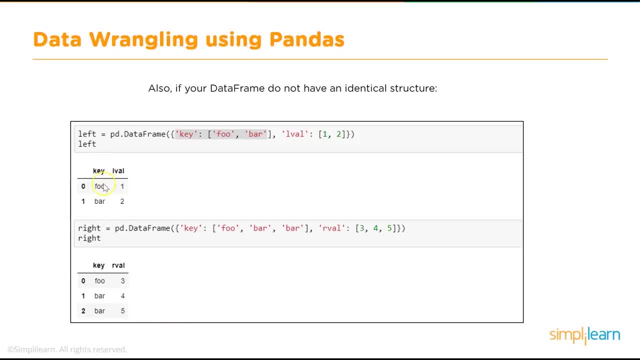 five as well. the only thing here is that this one had, for example, left had only two values and only one value for bar. but since we are appending or merging and there are two key values with the bar, therefore it will kind of repeat the value of lval here. so that's what we are seeing in this case, right? so l value appears. 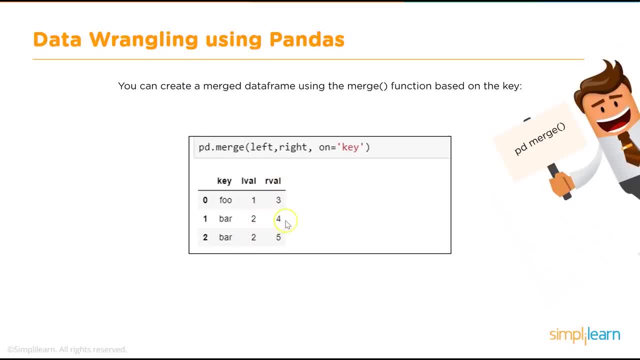 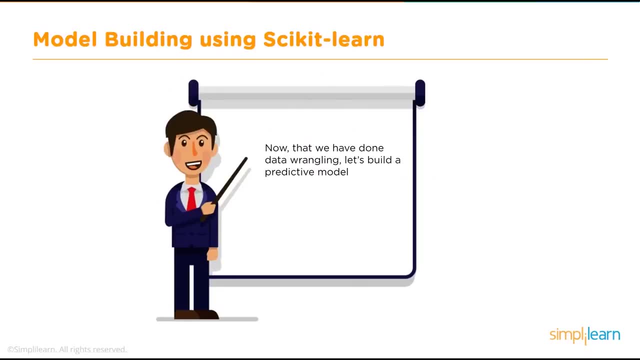 twice. the number two appears twice, but that is because r value. there are two of them. okay, all right. so that is how, when you don't have identical structure, that's how you merge. now we will talk a little bit about scikit-learn. so scikit-learn is a library which is used for doing machine learning. 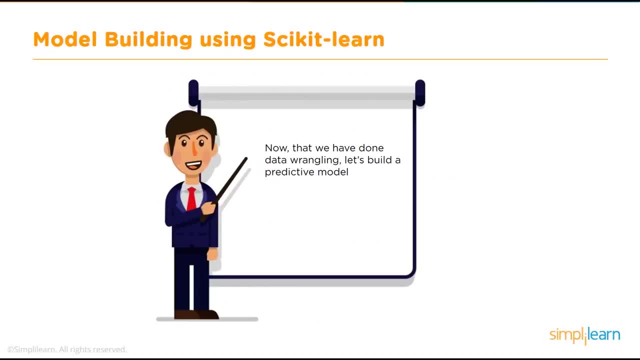 or for performing machine learning activities. so if you want to do linear regression, logistic regression and so on, there are easily usable APIs that you can call. and that's the advantage of scikit-learn, and it provides a bunch of algorithms. so I think that is the good part. 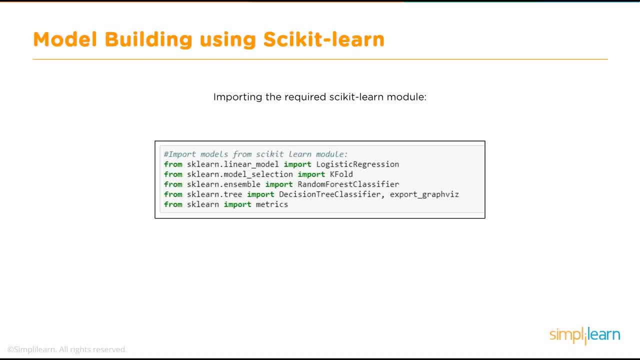 about this library. so if you want to use scikit-learn, obviously you need to import these modules, and also there are some sub modules you may have to import based on what you're trying to use, like, for example, if we know, if we want to use logistic regression again, people who are 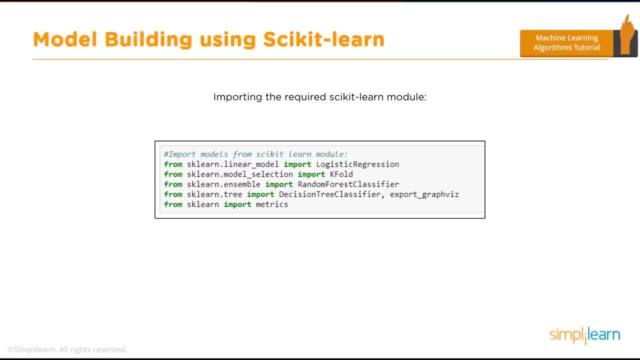 probably not very familiar with machine learning. there is a separate module for machine learning. you may want to take a look at that, but we will just touch upon the basics here. so machine learning has some algorithms like linear regression, logistic regression and random forest classification and so on. so that is what we are talking about here. so those algorithms are available and when, if you? 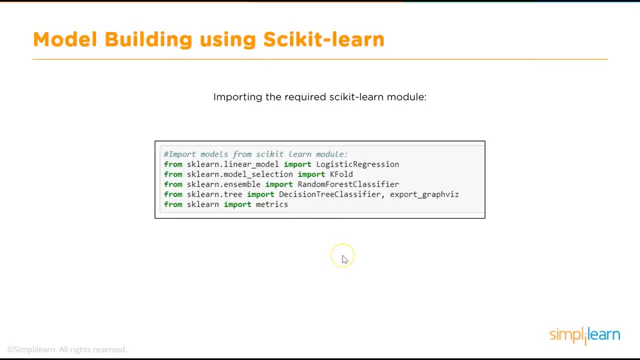 want to use some of them, you need to import them, and from the scikit-learn library. so scikit-learn is the top level library, which is basically sk learn right, and then it has a kind of sub parts in it. you need to import those based. 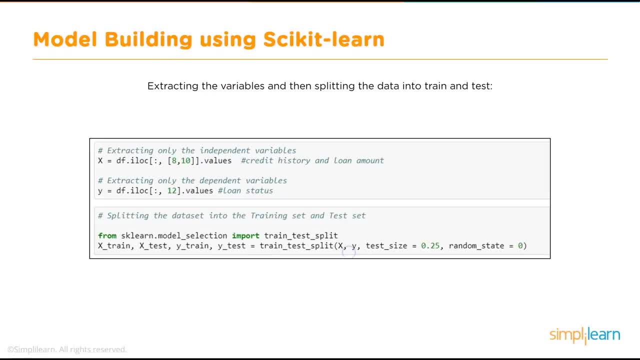 on what exactly you will be or which algorithm you will be using. so let's take an example. as we move, and we will see that whenever we perform some machine learning activity- those of you who are familiar with machine learning will already know this- we split our labeled data into two parts. 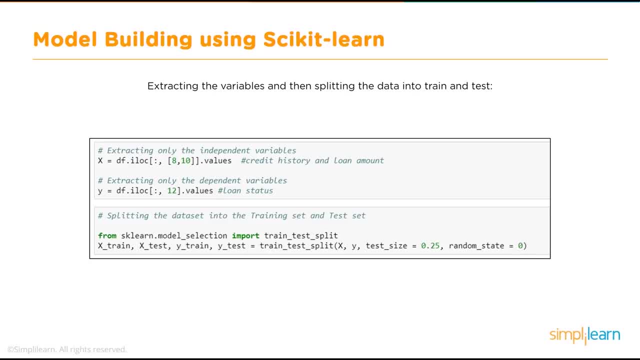 training and test. now there are multiple ways of splitting this data. how do we either? some people like 50, 50, some people do it 80, 20, which is training is 80, and test it is 20 and so on. so it is an individual preference. there are no hard and fast rules. by and large, we have seen that. 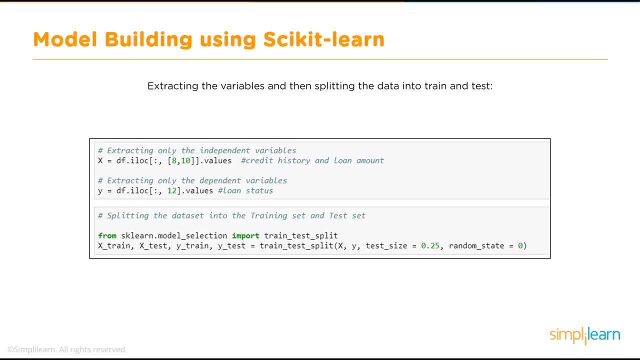 training data set is larger than the test data set and again, we will probably not go into details of why do we do this at this point, but that's one of the steps in machine learning. so scikit-learn offers a readily available method to do this, which is train test split. all right, so in this example, 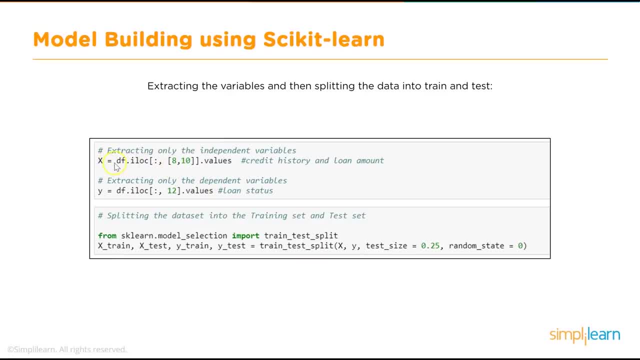 let's say we are taking the values x and y are our values, x is the independent variables and y is our dependent variable. okay, and we are using these two. and then I want to split this into train and test data. so what do we do? we import the train test split sub module from within scikit-learn. 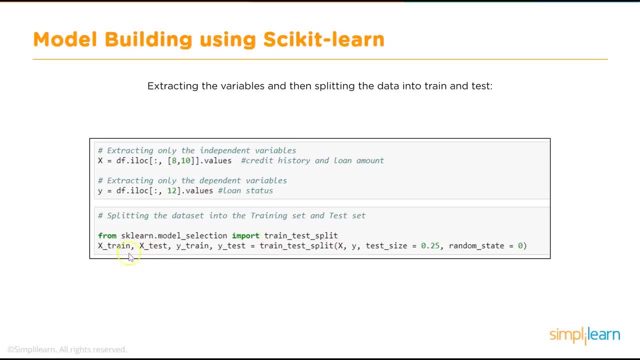 which is sk learn right. so within that we import train test split and then you call this train test data. so x is the- all the values of the independent variables, and y is our labels. so you pass x and y and then you specify what should be your size of the test data. so only one you need to specify. so 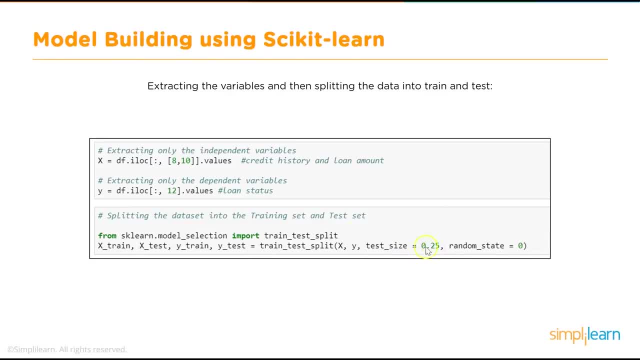 if you say test size is 0.25, it is understood that train size will be 0.75. so you're telling what should be the ratio of the split. so technically it doesn't nothing prevents you from giving whatever you like here, so you can give test as 80 and 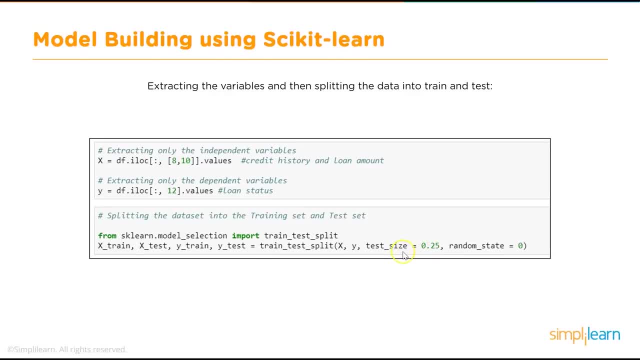 as 20, so whichever way. but then there's normal practices you will have. the training data set would be larger than the test data set, and typically it would be 80, 20, 75, 25 or 65, 35, something like that. right, so that is the second parameter, and this is just to say that you know. 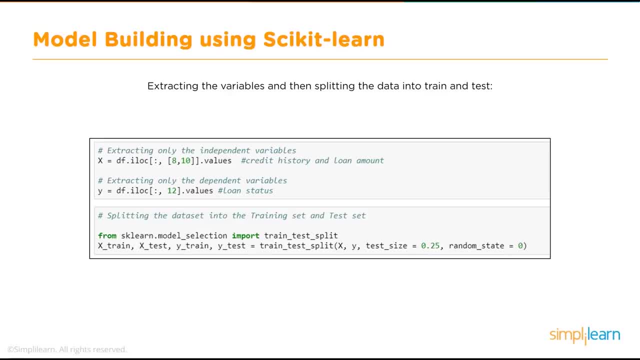 the data has to be randomly split. so it shouldn't be like you take the first 75 percent and put it in training and then the next 25 percent and put it in test, so that. so such a thing shouldn't happen. so we first set the state, random state, so that the the splitting is done in a very random way. so 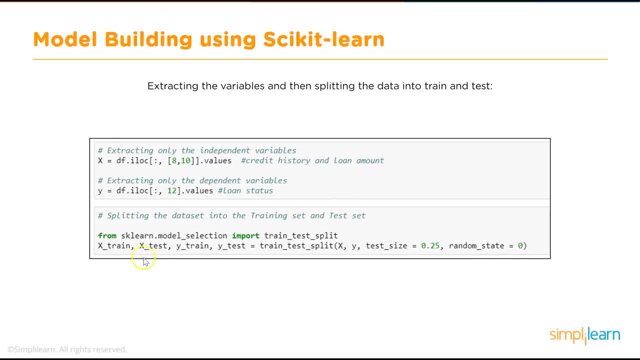 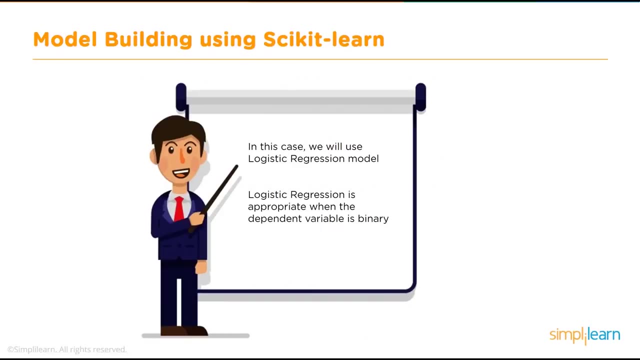 if they are randomly picked up the data and then put it into training and test and then this results in these four data frames. so x- train and x test and y train and y test. okay, so that is basically the result it will. now that the splitting is done, let's see how to implement or execute logistic. 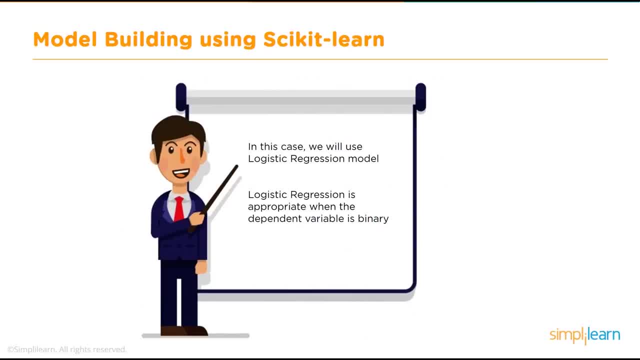 regression. so in logistic regression what we try to do is try to develop a model which will classify the data. logistic regression is an algorithm for supervised learning for performing classification. so logistic regression is for classification and usually it is binary classification. so binary classification means there are two classes. so 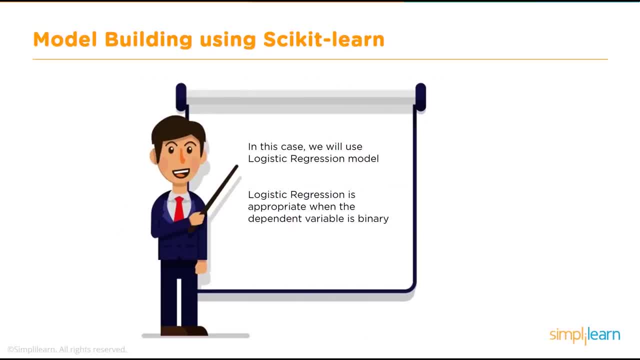 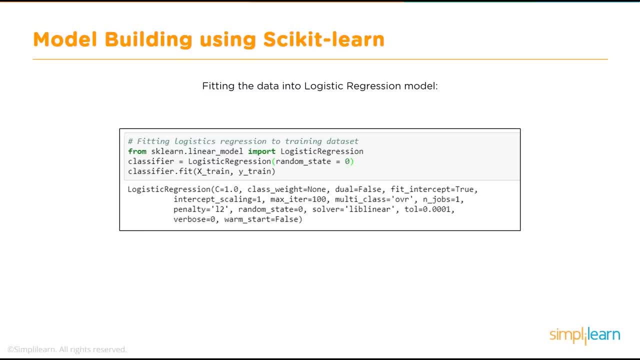 either like a yes, no or, for example, customer will buy or will not buy. so that is a binary classification. so that's where we use logistic regression. so let's take a look at the code: how to implement something like that using scikit-learn. so the first thing is to import this logistic regression submodule or subclass. 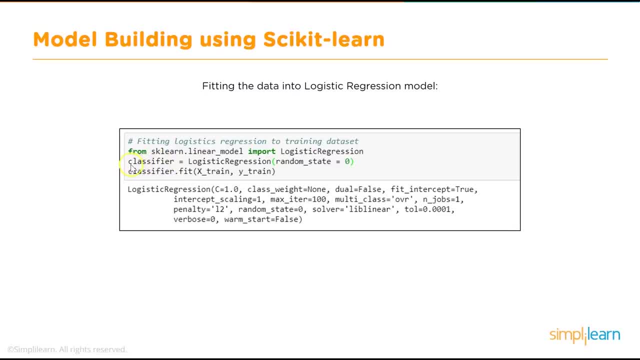 whatever you call it, and then create an instance of that. so our object is classifier. so we are creating an object by the name. this is a name, by the way, you can give any name. in our case, we are saying classifier, we say classifier is equal to logistic regression. so we are creating an instance. 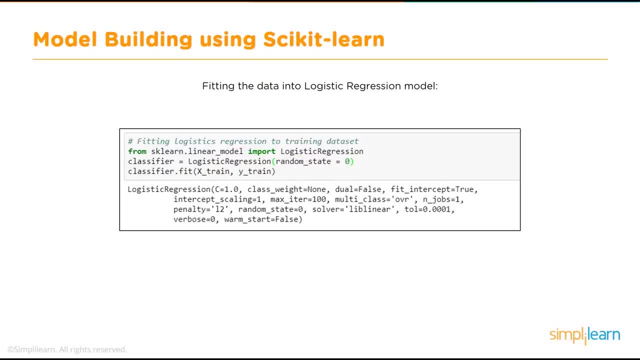 of the logistic regression variable or class or whatever. okay, and you can pass a variable or a parameter rather, which is the random state is equal to zero, and once you create the object, which in our case is named classifier, you can then train the object by calling the method fit. so this is important to note. 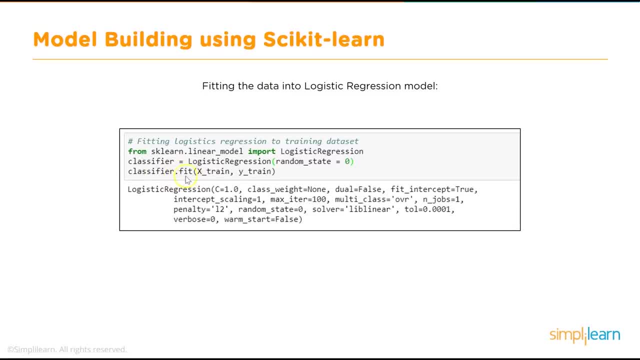 we don't call any. there is no method like train here, but we call what is known, as there is a method called fit. so you are basically, by calling the fit method, you are training this model, and in order to train the model, you need to pass the training data set. so 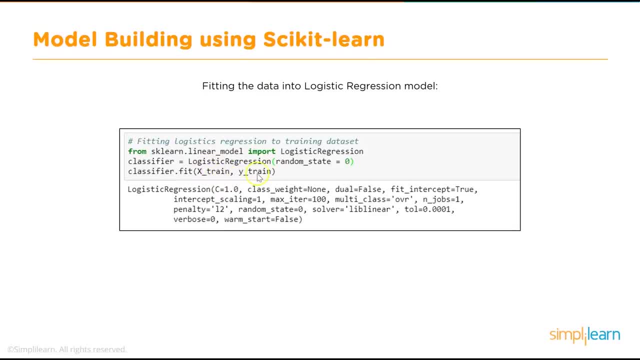 underscore train is your independent variables, the set of independent variables, and y underscore train is your dependent variable or the label. so you pass both of these and call the fit function or fit method, which will actually result in the training of this model classifier. now this is basically showing what are the possible parameters that can be passed or initiated when we are calling. 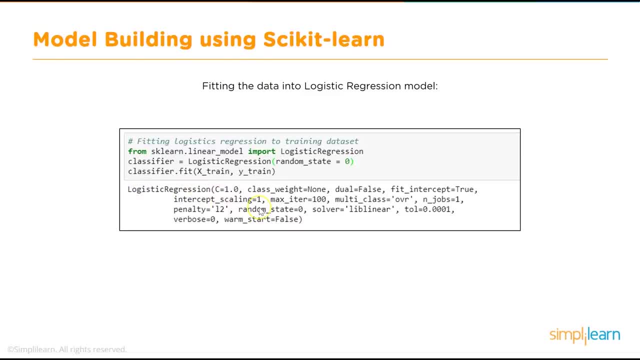 the logistic or the instance of logistic regression. so this is, but you can also look up the help file if you have installed python. so some of these are very intuitive, but some you may want to take a look at the details of what exactly they do. all right, so moving on, once we train the model by calling: 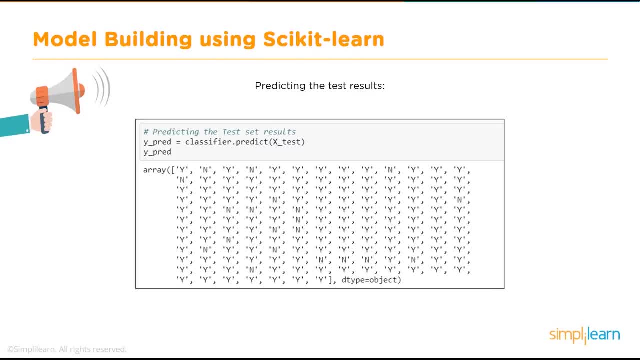 fit. then the next step is to test our model. so this is where we will use the test data. you need to pay attention here. here I am calling. so there are two things. one is, in order to test our data, we have to actually call what is known as the method, known as predict right? so here, this is where 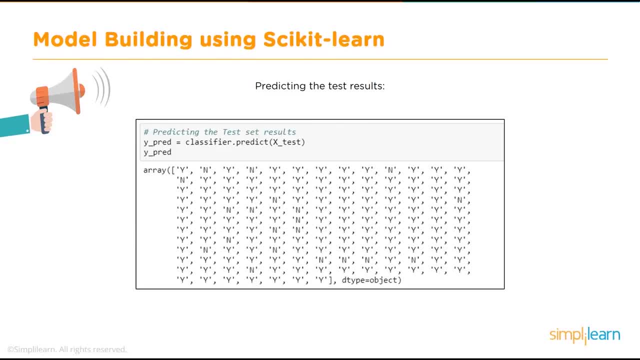 training is done, now is the time for inference, isn't it so? we have the model. now we want to check whether our model is working correctly or not. so what do you do? you have your test data, remember? we split it. 25 of our data was stored here, right? we split it into test and training so that 25? 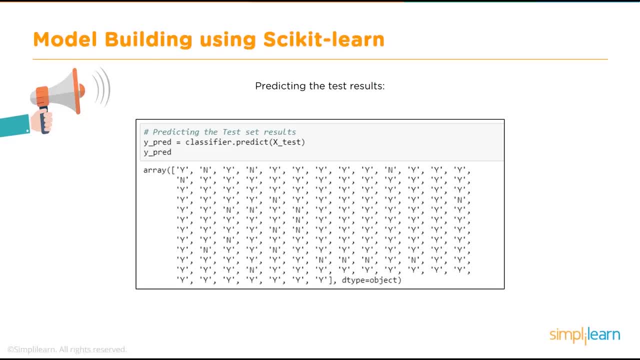 of the data we pass to and call the method predict, so that the model will now predict the values for y right. so that's why here we are calling it as y underscore, predict, and if we display here, as I said, logistic regression, which is basically binary classification, so it gives us the results like 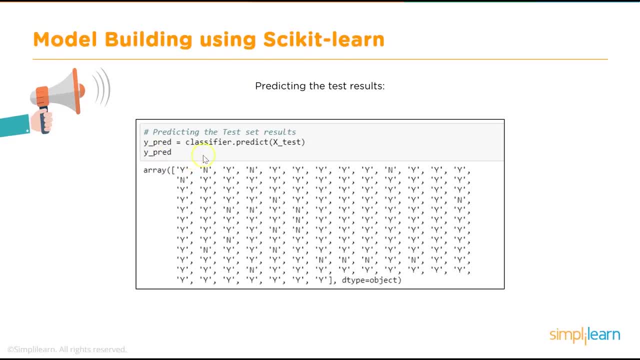 yes or no in this particular case, and then you can. so this is what the model has predicted, our model has classified now, but we also know we already have the labels for this. so we need to compare with the existing labels, with the known labels, whether this classification is correct or not. so 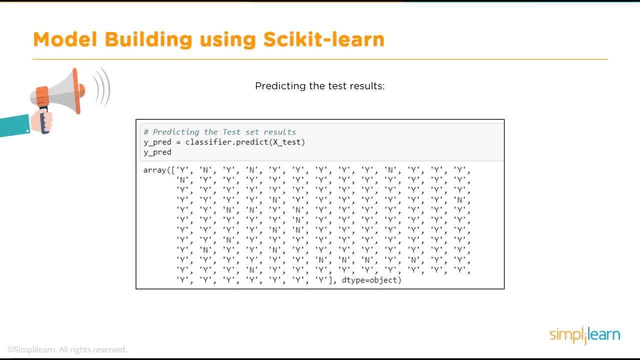 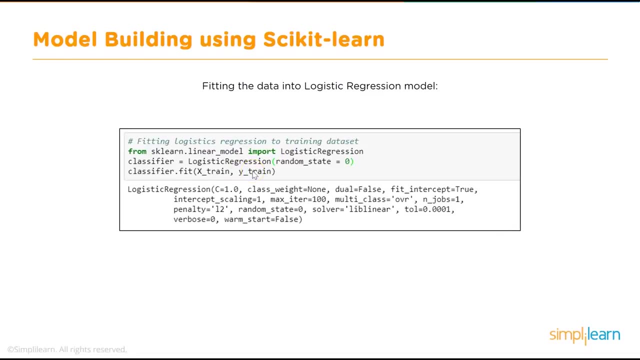 that is, where is the next step, which is basically calculating the accuracy and so on, will come into play. okay, so in this case, the first thing, the most important thing to note, is we do the prediction using predict, and here we are passing x, underscore test and not train right. in this case we did x and y, so again one more point. 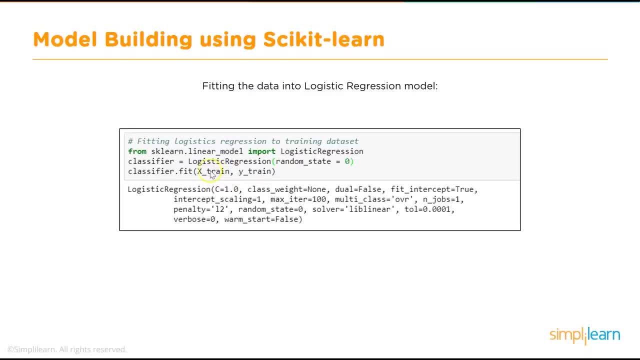 to be noted here: in case of training, we will pass both the independent variables and also the dependent variables, because the system has to internally, it has to verify. that is what is the training process. so what it will do: it will take the x values. it will try to come up with the y. 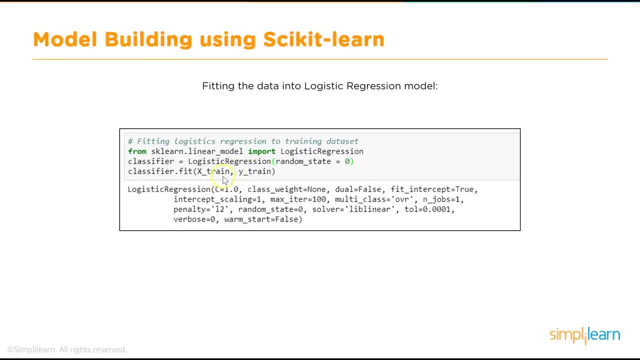 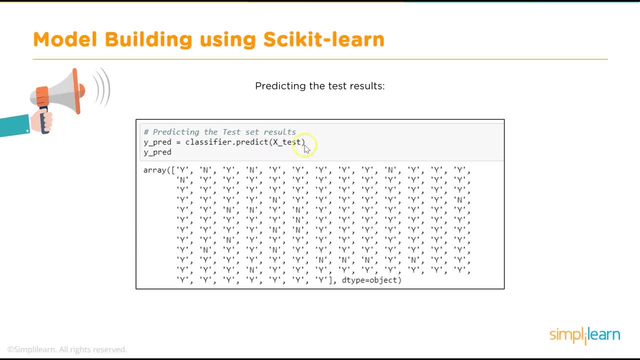 value and compare with the actual y value. right? so that is what is the training method. so that's why we have to pass both, x as well as y, whereas in case of predict, we don't pass both. we only pass because we are pretending, as if this. 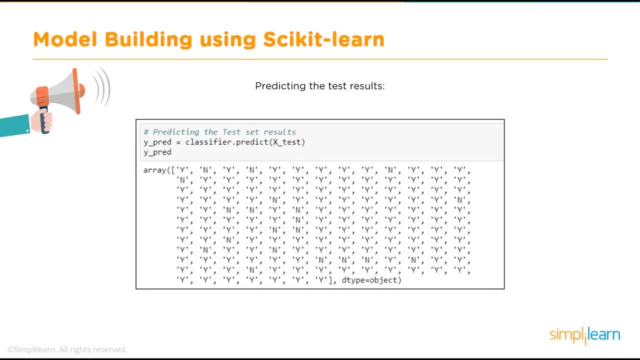 is the actual data. so in actual data you will not have the labels, isn't it? so we are just passing the independent variables and the system will then come up with the y values, which we will then- okay, remember, we also know the actual value. so we will compare this with the actual values and we will 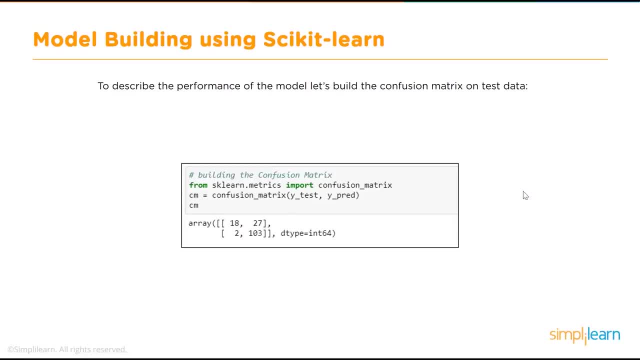 find out whether how accurate the model would be is. so how do we do that? we use what is known as a confusion matrix, so this is also readily available in Python library. so we import this confusion matrix and some of you who already know machine learning will find this familiar. but 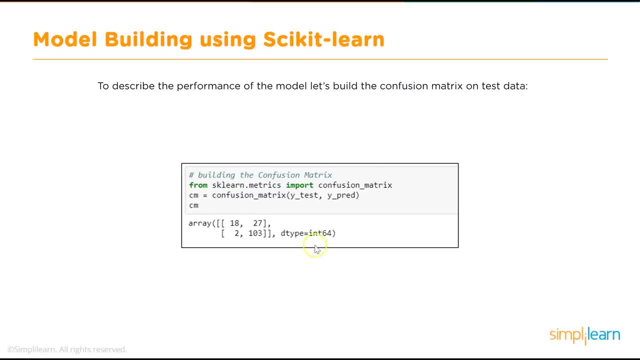 those who are new to machine learning, this confusion, matrix is nothing but this matrix, this kind of a matrix which basically tells how many of them are correctly predicted and how many of them are incorrectly predicted. so though some of the characteristics. let's quickly spend some time on this confusion. 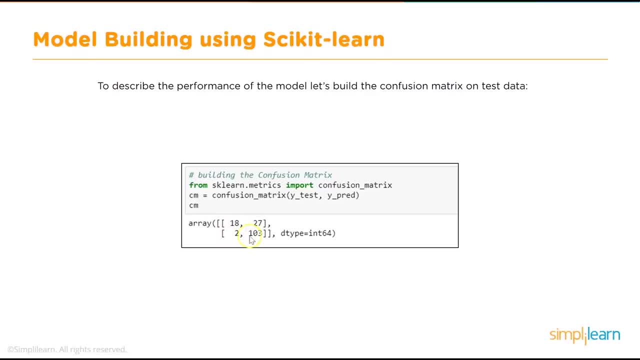 matrix itself. this the total numbers out here. these are just the numbers, these are like number of observations. then the accuracy is considered to be highest when the, the numbers or the sum of the numbers across the diagonals is maximum. okay, and numbers outside of the diagonals should be minimum. so which? 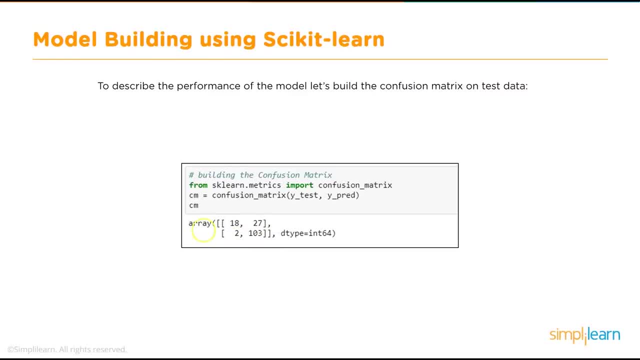 means that if this model was hundred percent accurate, then the sum of these two. there would have been only numbers in these two along the diagonal, this would have been zero and this would have been zero. okay, so that is like a hundred percent accurate model. that is very rare, but just that you are. 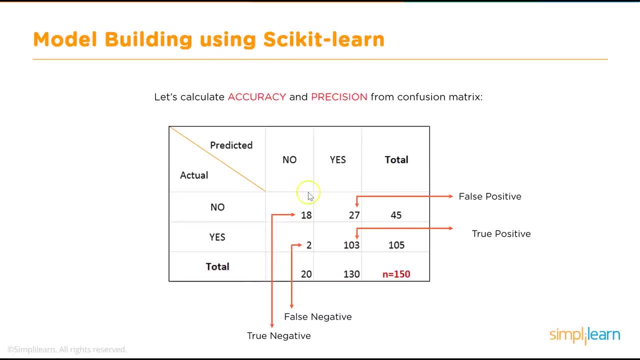 aware. so just to give an idea. okay, all right. so once you have the confusion matrix, you then try to calculate the accuracy, which is in a percentage. so there are two things that we can do from a confusion matrix or that we can calculate from a confusion matrix. one is the accuracy and the other is the 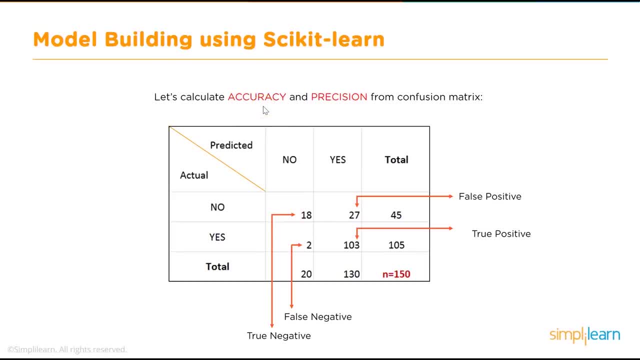 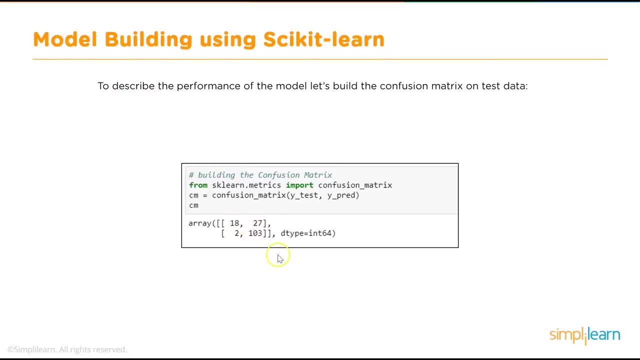 precision. what is the accuracy? accuracy is basically a measure of how many of the observations have been correctly predicted. okay, so let's say this is a little bit more detailed view of the confusion matrix. it looks very similar like as we saw in this case, right? so this is a two by two matrix. that's what we are seeing here. 18. 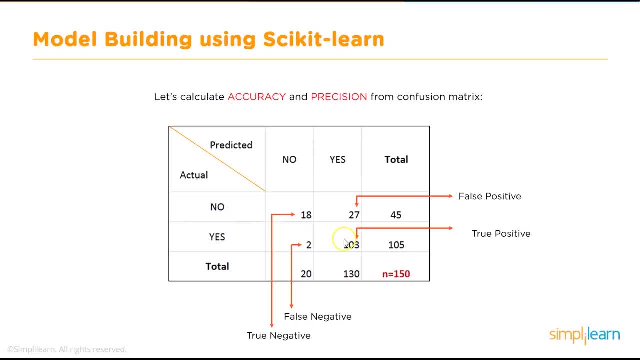 27, 2 1 0 3. so 18, 27, 2 1 0 3. now, but what are these values? that is, what is kind of. the labels are shown here in this. so there are altogether 150 observations. so, as I said, the sum of all these four right. 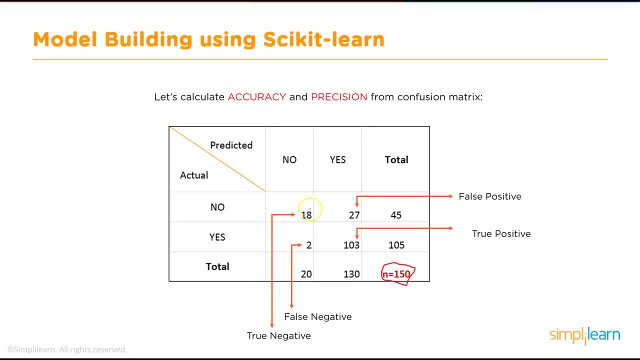 plus 27 plus 1, 0, 3 plus 2 is equal to 150. that is the first thing we have to observe. the sum of all these values will be equal to the sum of test observations. number of test observations: we have 150 test observations because, remember, we 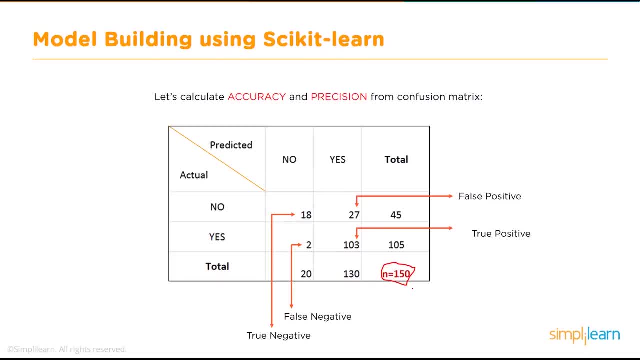 had about 500. we split that into 25, 75, so that is why we have 150 here and, I think, 350 in the training data set. okay, so that we get the numbers correct. so that's the first thing. now this next thing is: let's take a look at the actual values. 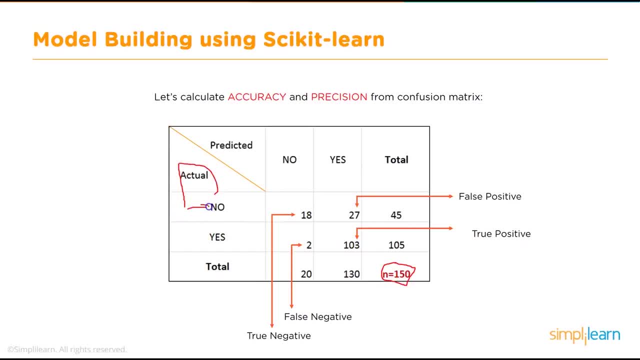 this view is the actual view, so there are actually right. in the actual data we have labels yes and no. so, as per the actual data, there are 45 observations tagged as no and similarly, there are 105 observations that are tagged as yes or labeled as yes. okay, now I know for. 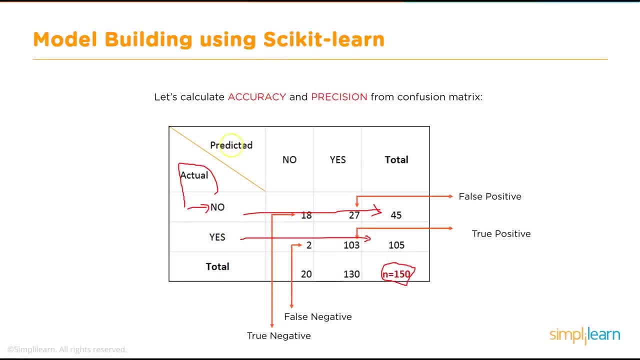 the first time when you're seeing this. it may be a little confusing, but just stay with me, okay. so this side tells us the predicted part of it. so our model has predicted- and it has totally predicted- 20 of them as no right. so that is what this is: totally 20 of them. it. 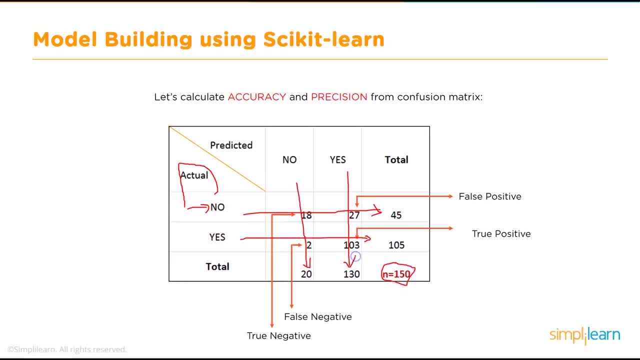 has predicted as no and it has predicted 130 of them as yes. okay, I hope this part is clear. so before we go into the middle part, let us first understand what exactly are these numbers so? actually tagged as no: there are 45 total. actually tagged as yes: there are 105 and predicted no. 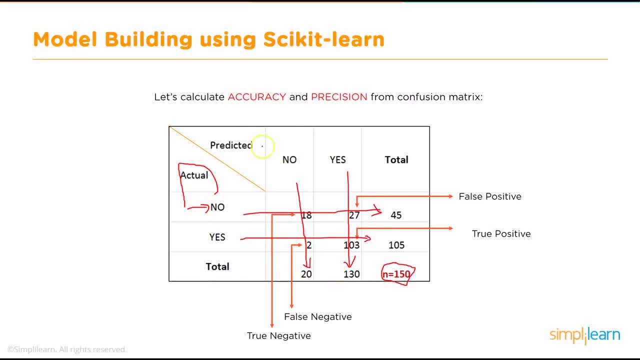 there are 20 predicted as, yes, there are 130.. this is the result from our model. okay, this is the result from our model and this is the actual value, which we already know, because this is our label data. that is the first thing now. now let us take a look at each of these individually. okay, now what? 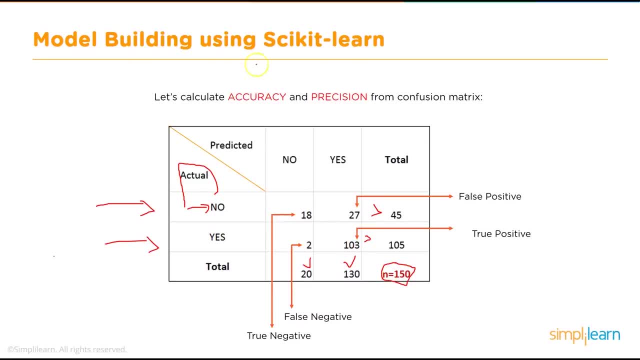 are the options we have once again. okay, so now what is happening here? let us look at these, these values. so this 18 says that these are actually tagged as no and the model is also predicted as no, which means this is what is known as a true positive right or true negative, sorry right, which. 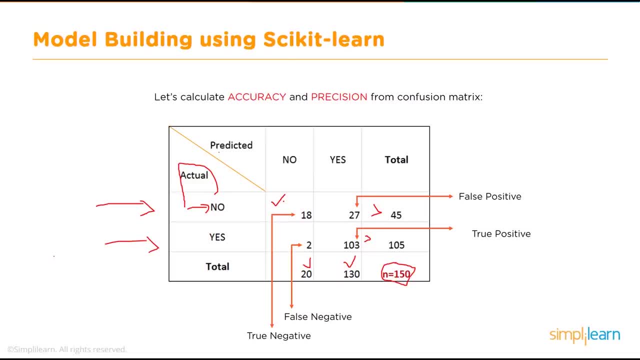 means that our model has predicted- is it correctly? it is negative because it says no, so, and it has also predicted no, so it is known as what is known as true, negative. okay, now let's come to this side of it. that way, we are talking about the diagonal. remember, I said most of the value should be in the 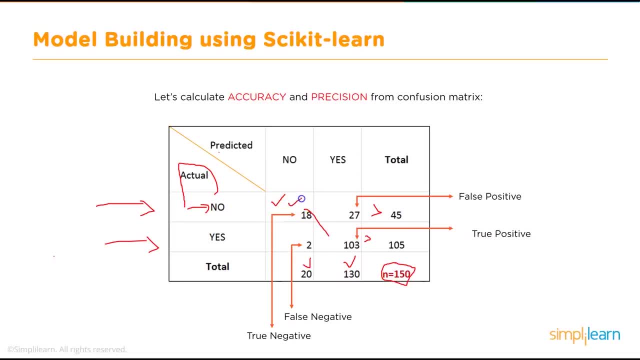 diagonal. okay, so that means these 18 are correctly tagged. they are labeled as no. our model has predicted as no, so these are correctly tagged and these are known as true, negative, okay. similarly, if we come diagonally down, there are 103 observations which are labeled as yes. 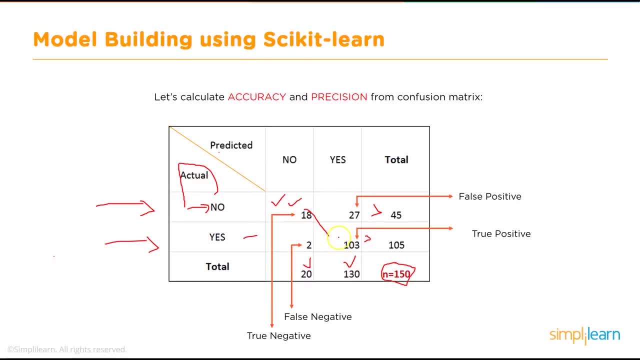 actual value is s, and our model is also predicted as yes, and these are known as true positive values. positive because of this. yes, okay, right. so what is important is: this is true, this is also true, so we have to make sure that the maximum number of values are in the 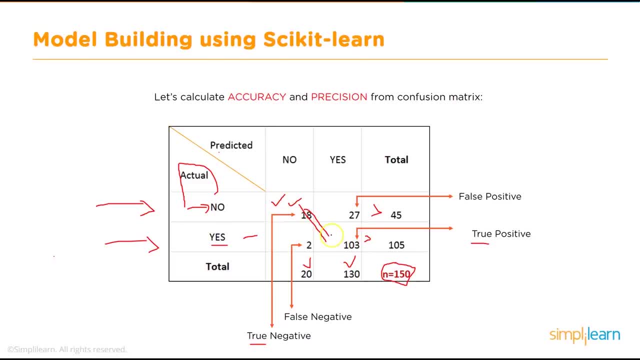 true section. okay, true positive and true negative. that's the reason I said the sum along the diagonal should be maximum. now let's see: if our model was 100 accurate, this sum in this case it is only 103 plus 103 plus 18, which is 121. but if our model was accurate, the sum of these two would: 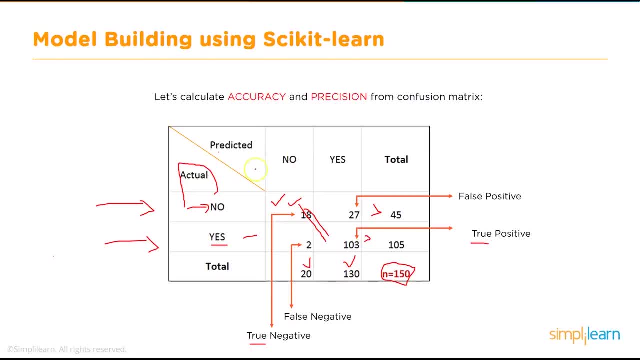 have been 150.. that means it's a perfect model. okay, all right. now what else? since we covered these two, let's also cover these two. so here, this says that 27 of them were actually labeled no, but our model has predicted as yes. that means this is wrong. 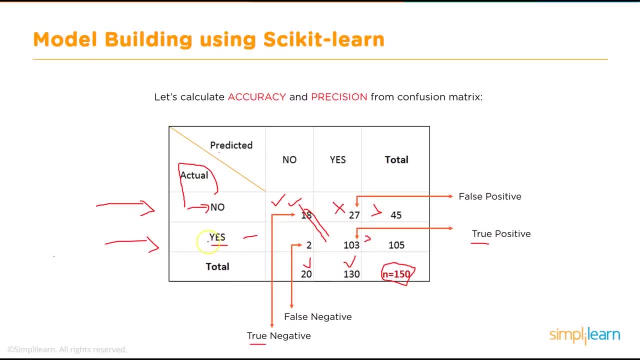 right. similarly, these are two of them where the actual value is yes, but our model has predicted as no. that means it's a wrong prediction, so you get the point. so, therefore, along the diagonals are the correct values, whereas in other places it is all wrong values. so wrong predictions. 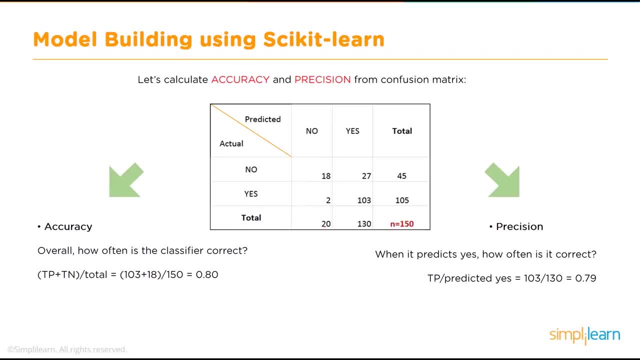 okay, now how do we calculate accuracy from this information? so the way to calculate accuracy is: so we'd say: okay, there are, total observations are 150 and what are the correctly predicted values? these are the correctly predicted values, which is 18 plus 103. so this will. 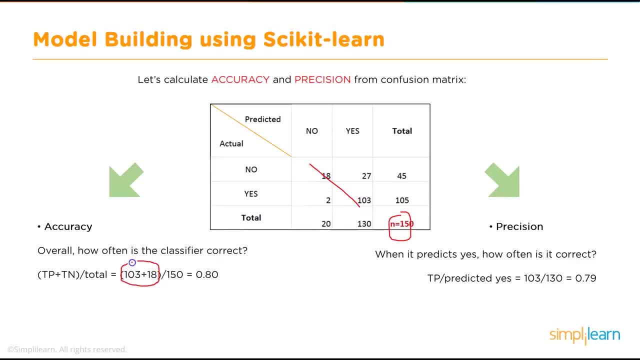 give us our accuracy. so 103 plus 18, which is 121, divided by our total observations, which is 150, is our accuracy, which is 0.8, or we can say it is 80 percent. okay, now there is another concept called precision, so precision is given. 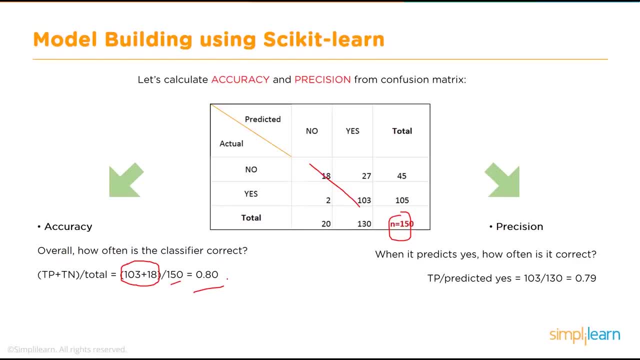 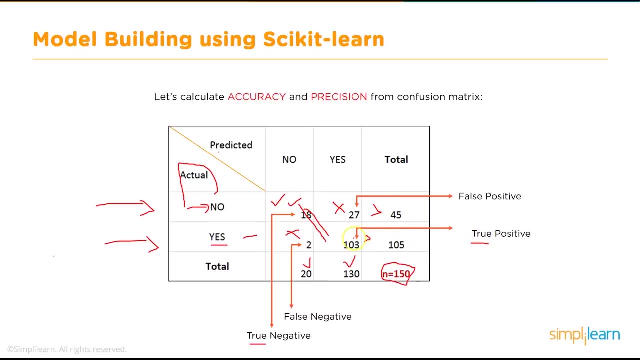 by the formula: true positives divided by the predicted positives, totally predicted positives. okay, what do we mean by that? which are the true positives here? remember which are the true positives. we just recall, we just talked in the previous slide. which are the true positives you see here. so this 103 are the true positives, which means that the value is positive. actual value is. 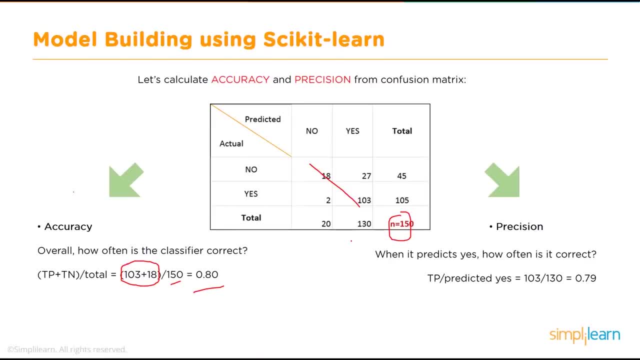 positive. predicted value is also positive, so that's why it's called a true positive. so 103 divided by so that is our true positive: 103 divided by totally predicted as yes. now, what is totally predicted as yes? remember, 130 of them have all together been predicted as yes. not that they are correctly predicted, only 103 have been. 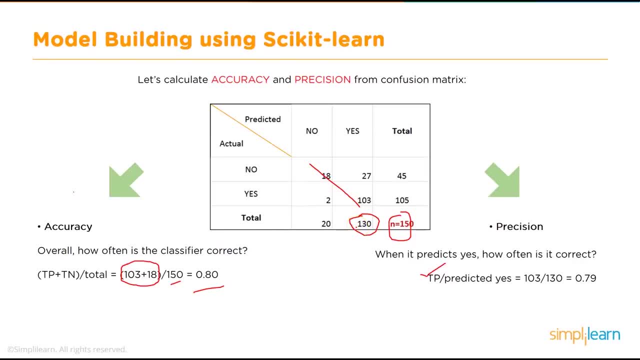 correctly predicted, but 130 of them have been predicted as yes. so precision is basically the ratio of these two out of the totally predicted. how many of them are actually true? that ratio, so 103 by 130, which is again about 80 percent, is the precision. that's how you calculate precision. so this is just a simple formula and the term that 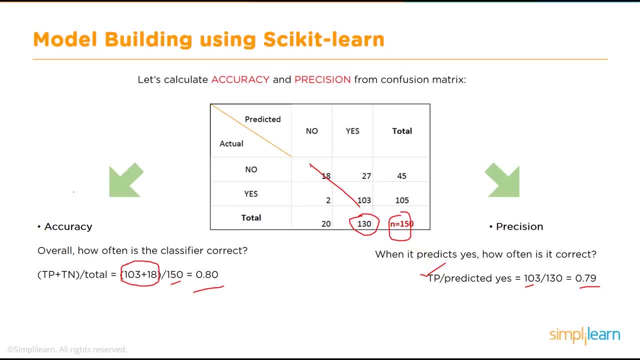 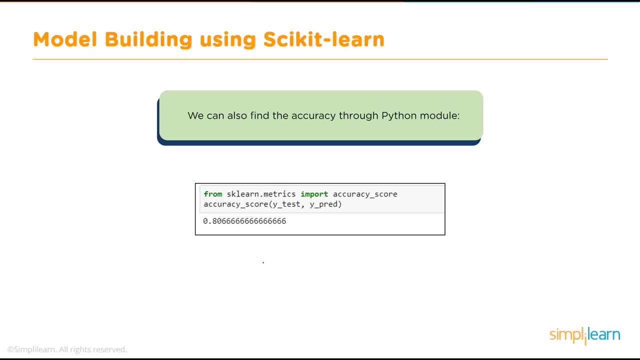 you need to remember. so accuracy is: you need to take total of true positive and true negative divided by the total number of observations, whereas precision is true positives divided by the totally predicted positives. okay, so that is our accuracy and precision. now, what we did, the accuracy calculation was manual, but we can also use some libraries which are: 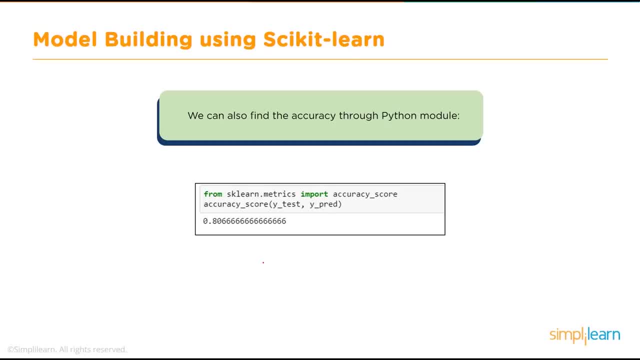 already existing and the functions within that library. so a psychic provides one such method. So, for example, accuracy underscore score is one such method. So if you use that and pass your test and predicted values, only the y you need to pass. 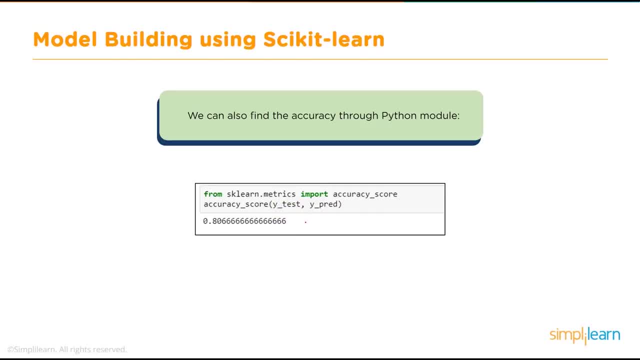 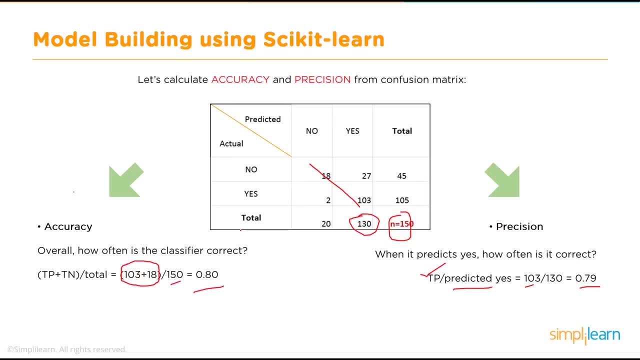 right, the dependent variable values. So if you pass that, it will calculate it for you. So in this case again, as you can see, it still calculates the same, which is 80%, which we have seen here as well. Okay, so this can be done using the method. Great, So that's. 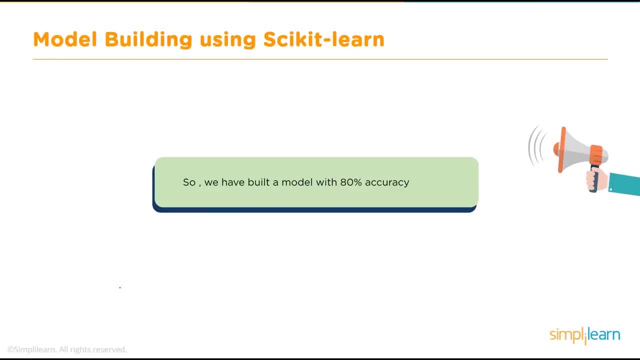 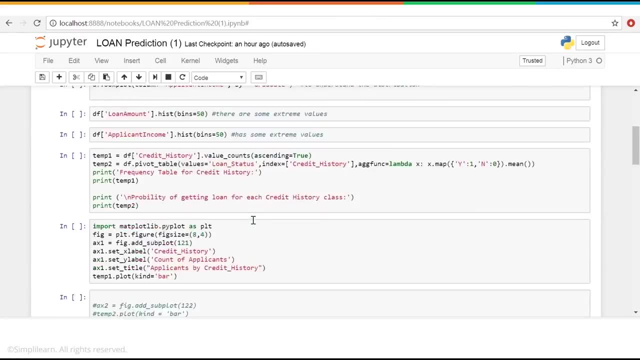 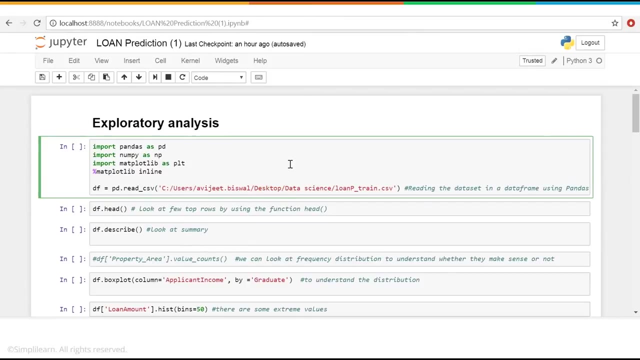 pretty much what we have done here. Before we conclude, let me take you into the code and show you how it actually looks. Okay, so this is our code. Let me run it, Okay, one by one. we have already seen most of the steps and slides, So I will. but I will run this in the actual Jupyter. 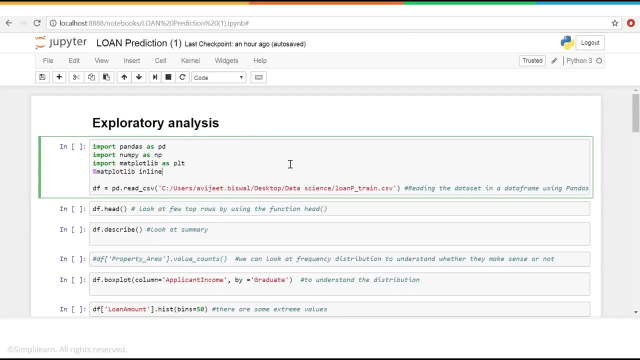 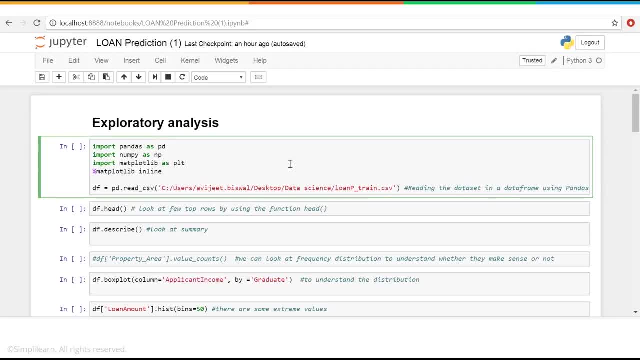 In this tutorial also, we there was one slide on how to install Python and Jupyter notebook. If you have not yet done, please do that, so that then you can actually walk through this code while you're watching this. Okay, So what are we doing here? We are importing the libraries. 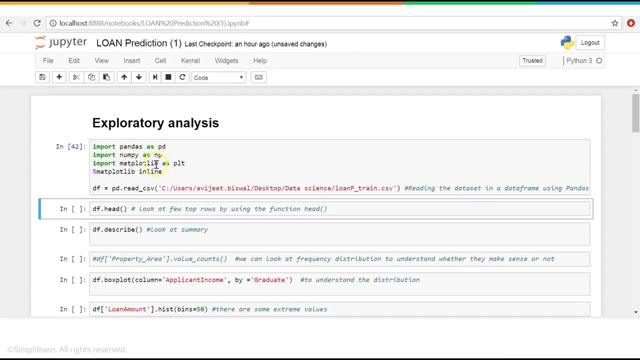 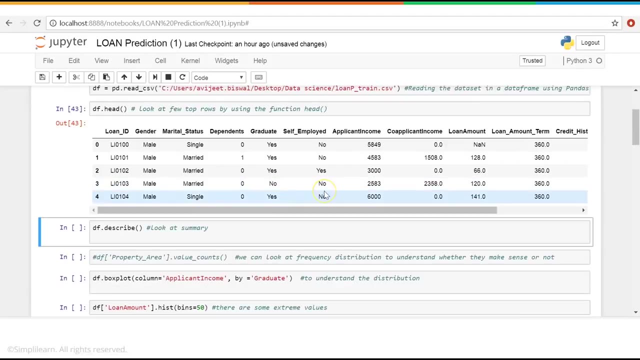 required libraries. Recall: here we have pandas, we have numpy and for visualization we have matplotlib, And this line is basically reading the CSV file. So we have the CSV file locally on our local drive And this is where I'm checking the data, just so that I'm 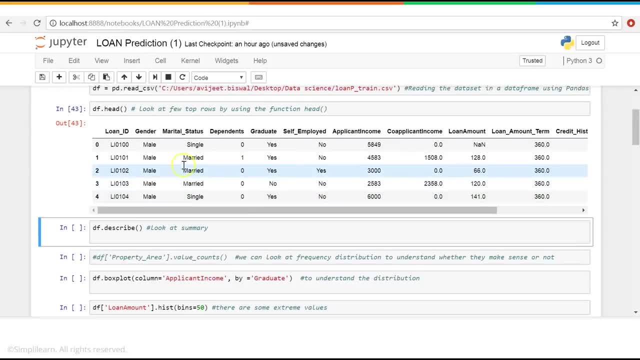 starting with my exploratory analysis, how the data is looking. So it looks good. There are no major missing values or anything like that. So it will display all the columns and it will show me the first five rows when I'm using this head function. And then I want to see a kind of 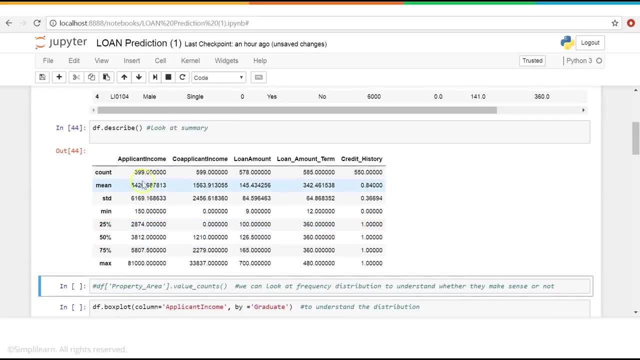 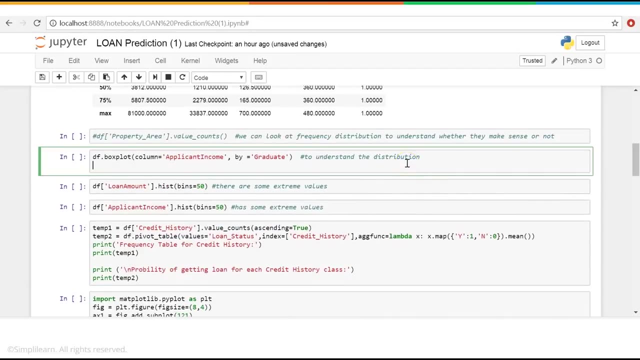 summary of all the each of the numerical columns. So that's what I'm doing here. So these are the numerical columns And it gives a summary like: how many observations are there, what is the mean- standard deviation, minimum, maximum, and so on and so forth for each of them, And then you can do some visualization. 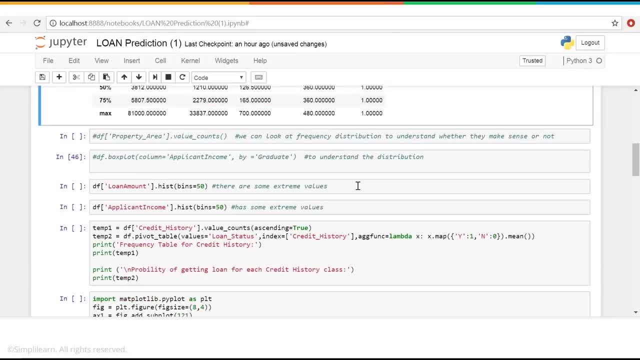 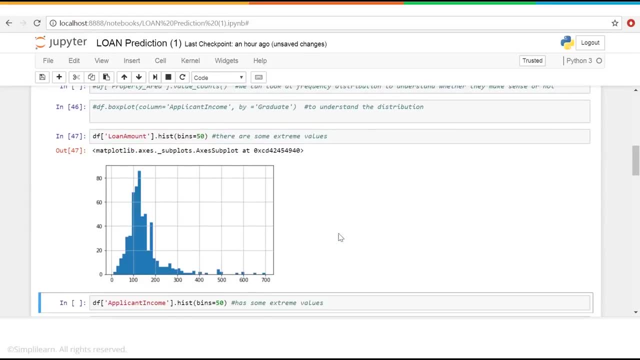 So this is the visualization for this. Okay, The next step is to view the data data visualization And we will do that using a histogram for a couple of these columns. So in this case, I'm taking a look at the loan amount And if I create the histogram, it displays. 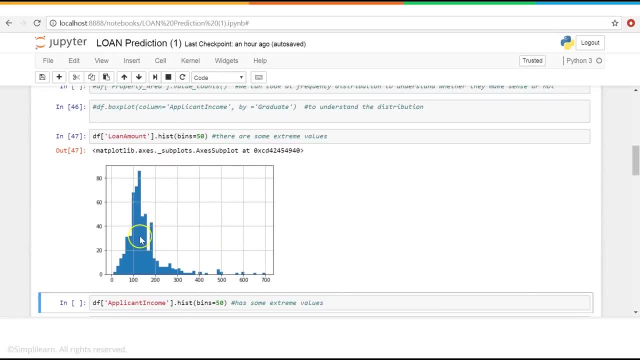 the data here in the form of a histogram, One thing that we gather from this, as I mentioned in the slides, as well as how the data is kind of scattered. So, while most of the values are in this range- 0 to 300 range- there are a few extreme values around the 700 range. So that is. 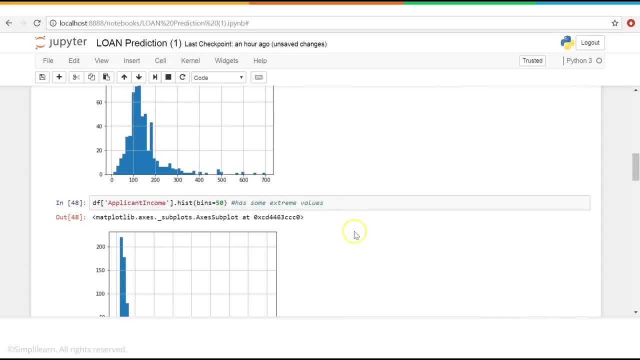 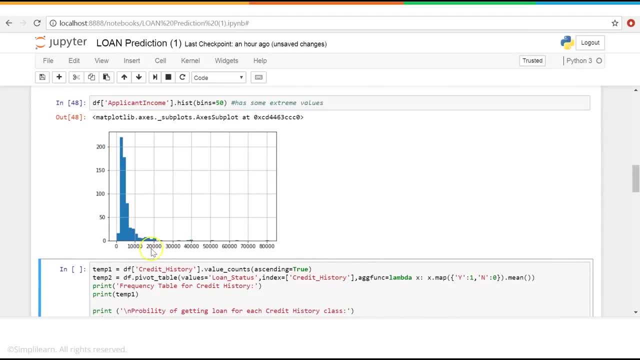 one information we get from this histogram. Similarly for the applicant income, if we draw a histogram, something similar, we can see that while most of the values are in this range, 0 to 20,000 range, there are a few in the range of 80,000 range. So that is one information we get from this. 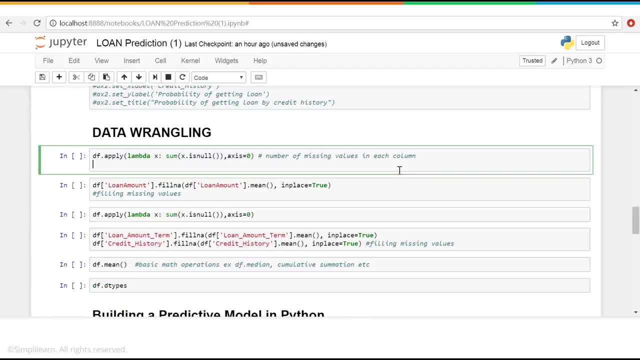 histogram. So we can see that while most of the values are in this range- 0 to 30,000 range- there are a few in the range of 80,000 range. So that is one information we get from this. 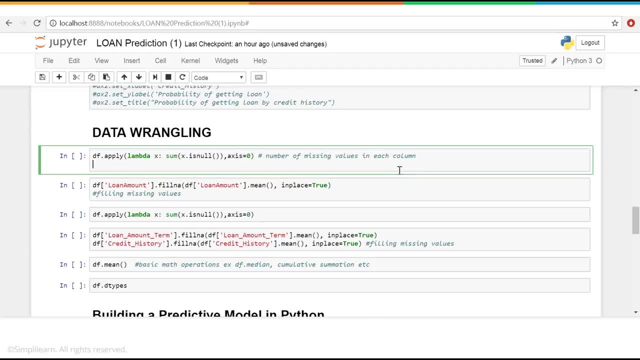 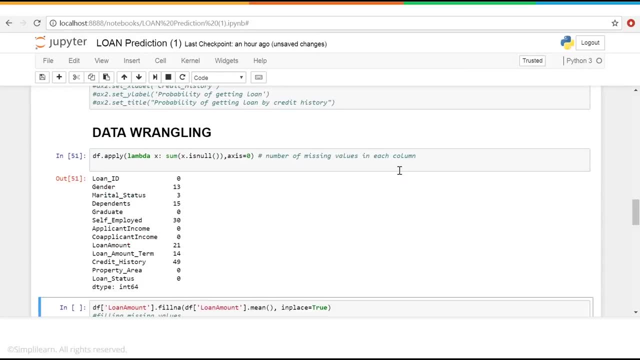 histogram. So that is one information we get from this histogram. So the next step is to perform data wrangling, where we will check if any data is missing and how to fill those missing values and so on. So in this case we will just check for all the columns how many data or how many entries. 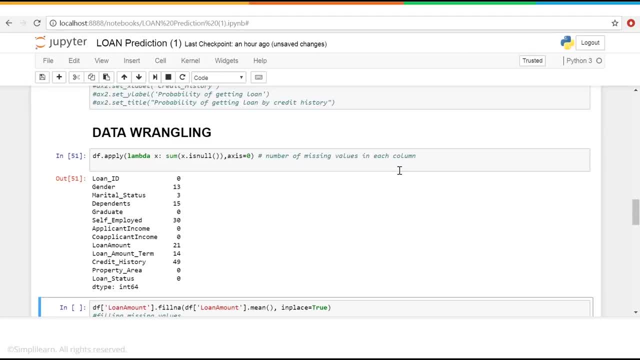 are there with missing values. So this is the result. So loan ID has all the columns or all the cells filled. Gender has 13 missing values. Marital status has three missing values, and so on and so forth. Loan amount: 0 to 300 range: there are a few missing values. So this is the. 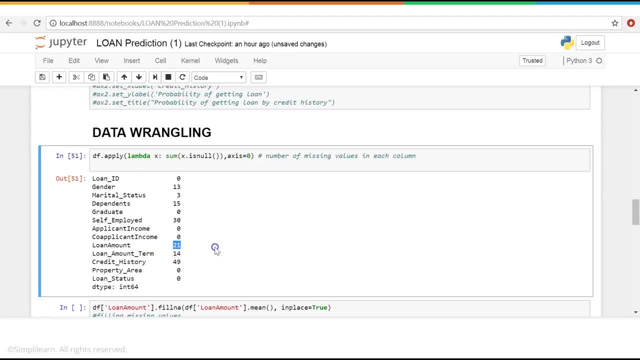 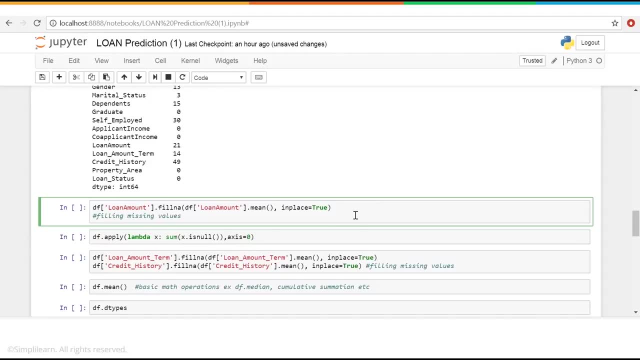 as 21, and this is what we are going to show you: how to remove these missing values. so when you have missing values, as i mentioned in the during the slides, there are a couple of ways of handling that. one is you can completely remove those or you fill in with some meaningful values. so in this, 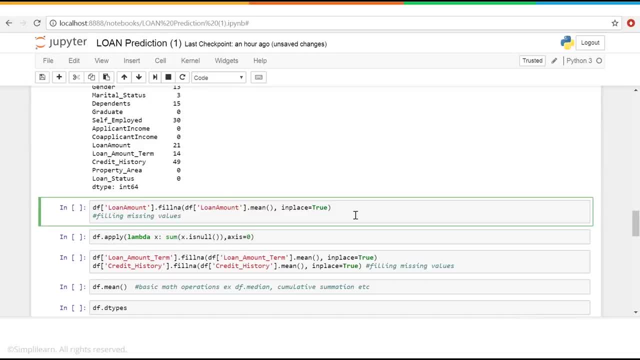 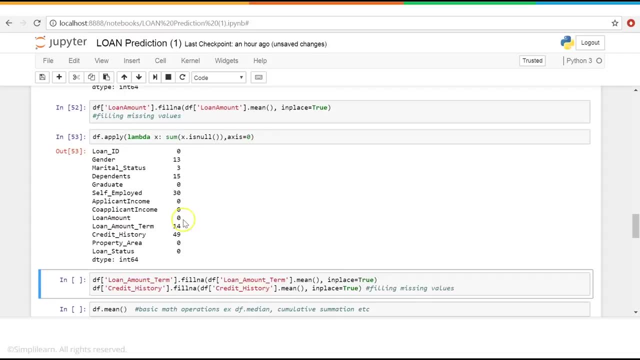 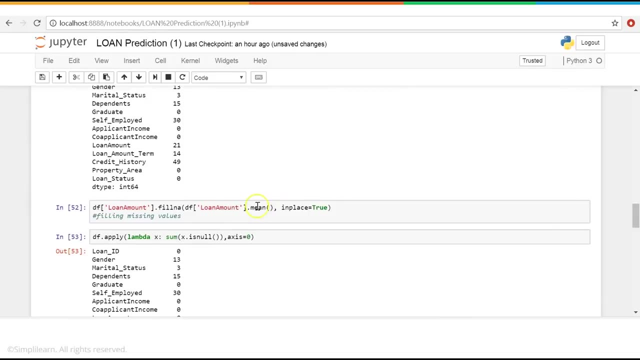 case, we will fill the missing values with the mean value of the loan amount. so let's go ahead and do that. and now, if we check here now, loan amount number of missing values is zero, because what we did was, for all these 21 cells where the values were missing, we filled with the mean value of the 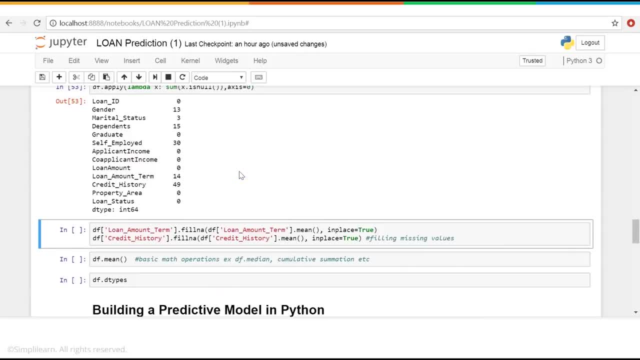 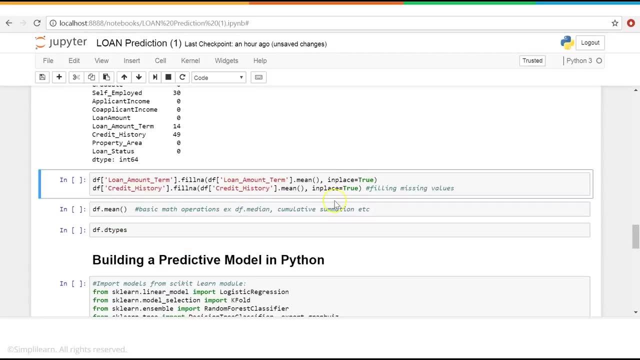 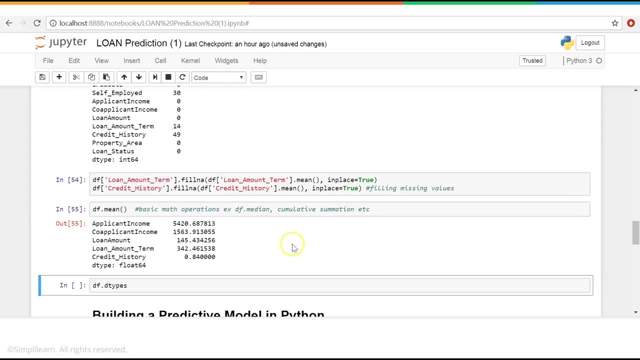 loan amount. so now there are no more missing values for loan amount. we can do this for other columns as well, but this was just one example, so we have shown it here. okay, so we will run this for credit history and loan amount term as well, and then if we calculate the mean of pretty 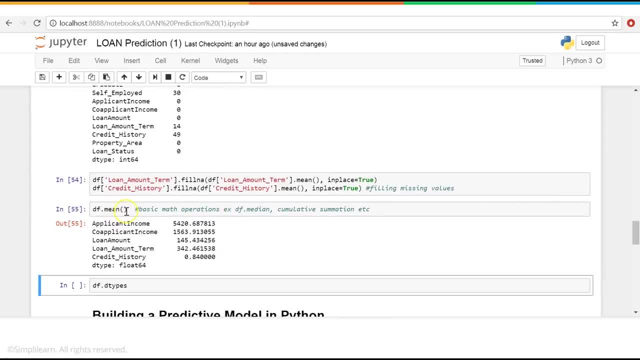 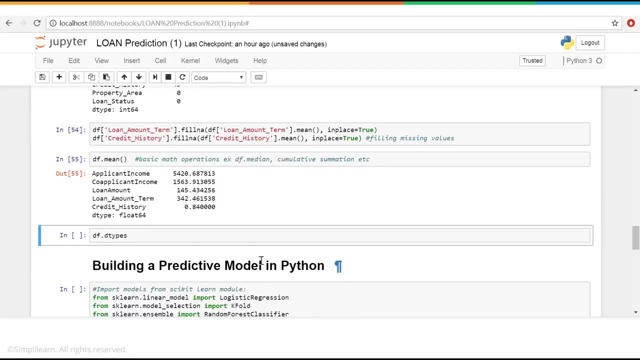 much all the numerical columns. that's the method. call so df, dot, mean will give us the mean value, give us the mean of all the numerical values. and another thing that we can do is we want to find out what are the data types of each of these columns. so you can call df, dot, d types and get. 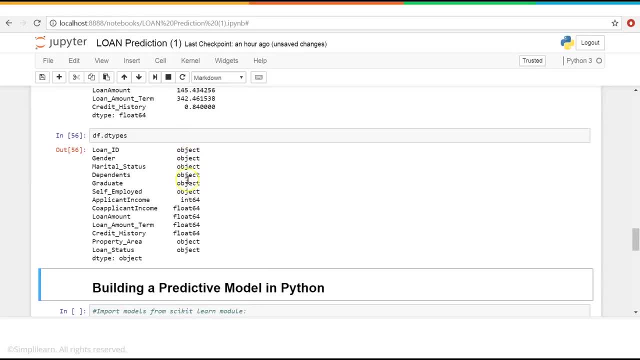 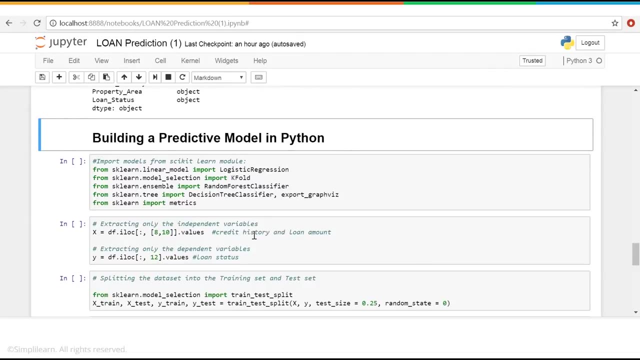 the data types. of course it may not be that very useful. most of the cases is an object, but for example this one: it shows as int 64 and there are float 64 and so on and so forth. now, in addition to doing the exploratory data analysis, we can do some machine learning activity as well. so in this, 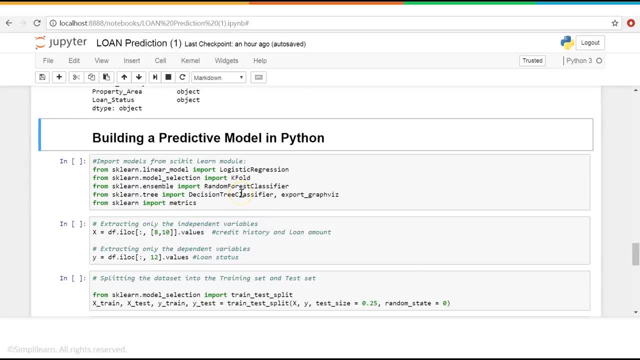 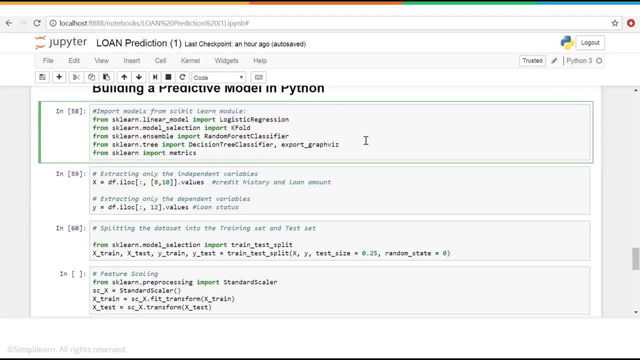 case, we are going to do logistic regression, so this is the example that i have shown you in the slides as well. this is the actual code for that. all right, so the first step here is to import the libraries, and then the next step is to separate the independent variables and the 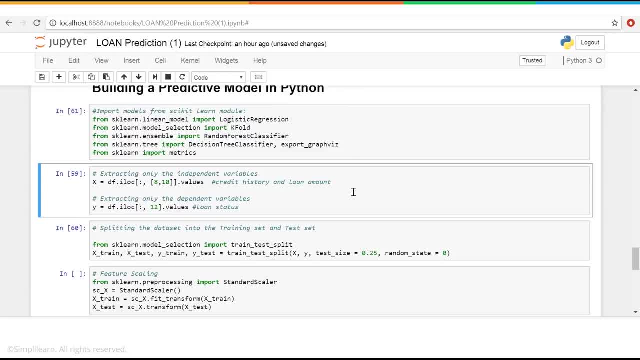 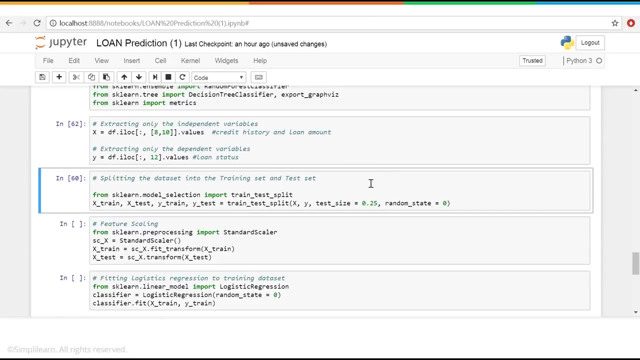 dependent variables. so x is our independent variable and y is our dependent variable. so we separate the data into two parts, and this will be our target as well. right, so that's how we separate it. now we have to split the data into training and test data sets, as i mentioned in the during the 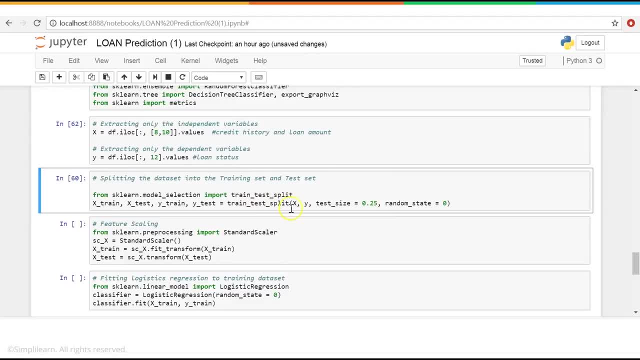 slides. we use the train test split method and when we call this and pass the independent variables and the dependent variables and we specify the test size to be 0.25, which means the training size will be 0.75, which is nothing, but you split the data into training data set, which is 75 percent. 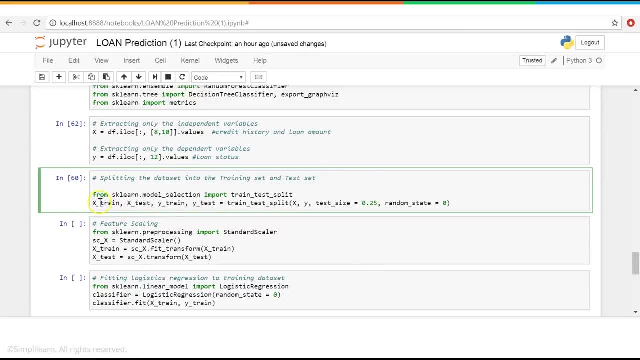 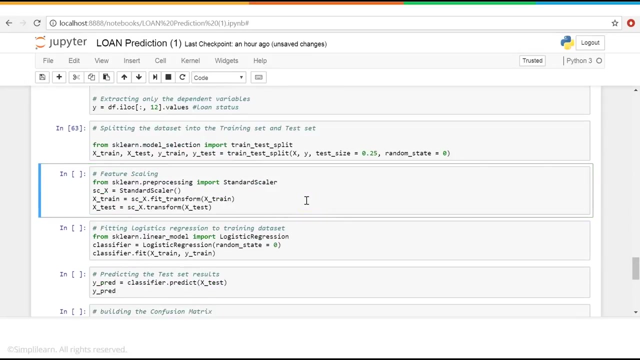 okay, so once you split that, you will have all your independent variables data in x- train, the training data, which is 75 of it. similarly, independent variables for test will be in x- under score test and dependent variables train will be in y- underscore train and dependent variable test will be y- underscore test. once we do this, we have to do a small exercise for scaling. 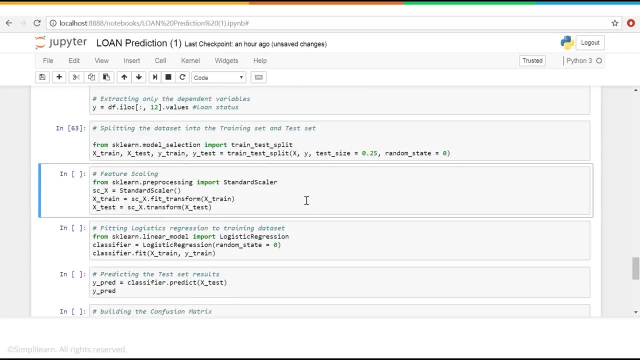 remember we had some data which was kind of very scattered and we didn't want to use the text in the there were some extreme values and so on. So this will take care of that, so that the data is normalized, so that, before we pass to our algorithm, the data is normalized, so that the performance 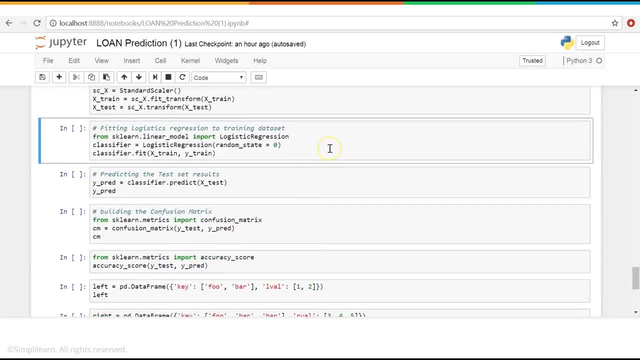 will be much better. The next step is to create the instance of logistic regression object. So that's what we are doing here. So classifier is our logistic regression instance. right, Classifier is equal to logistic regression. we are saying: So one instance of logistic regression is created. 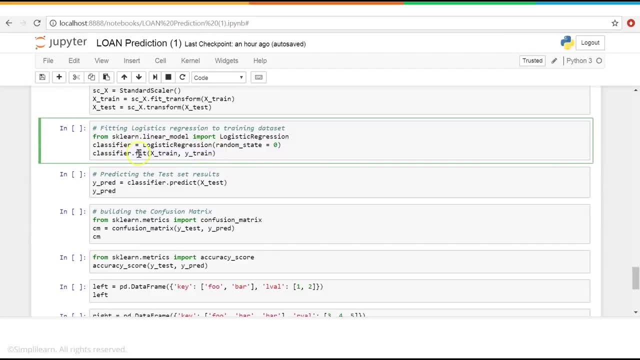 and then we call the training method. The name of the method actually is fit, but what it is doing is it is taking the training data. X is the training data or the independent variables and Y is the dependent variables. So we are taking both of these and the model gets trained. So the 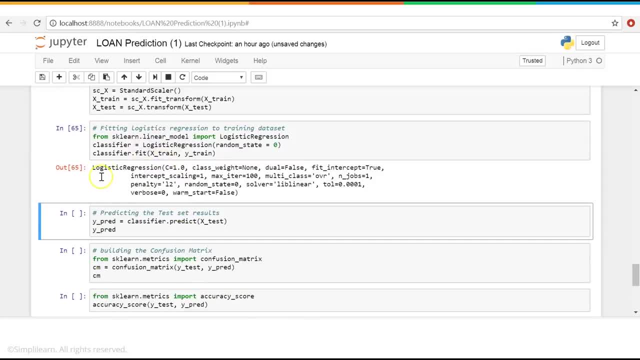 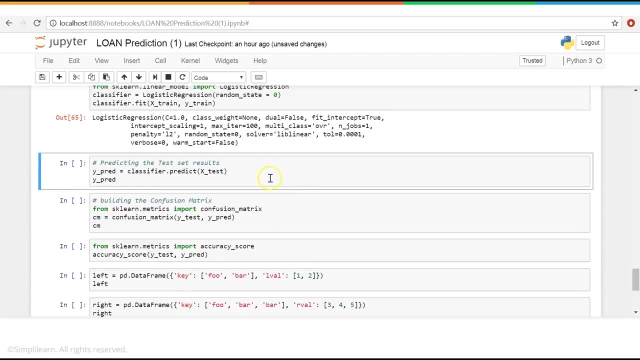 method for calling the training is fit, Okay, so it gives us the output and then, once we are done with the training, we do the testing. And once again, just to recall, in the slides, when I was showing you the slides also, I mentioned: 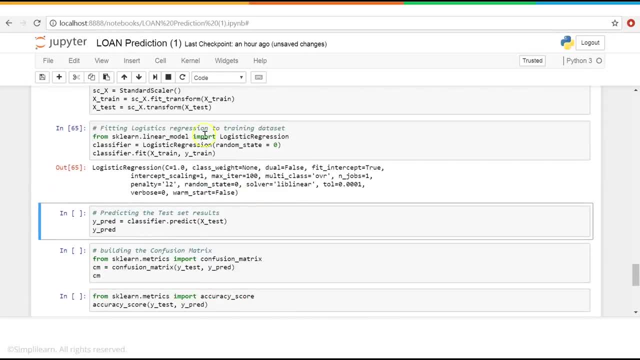 we don't pass Y here, while we are testing, While for training we do pass Y, but right. so for fit, we are passing X and Y, but for test we are only passing X, something you need to observe, because Y will be calculated by the model and we will then compare that with the known value of Y. 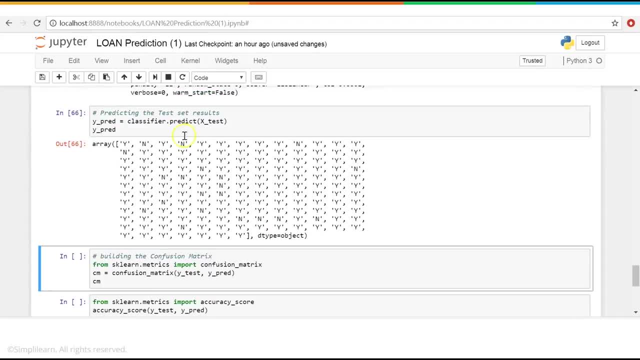 to measure the accuracy. So that's what we will do here, And the method that is called here is predict, So this will basically create or predict the values of Y. Now we have in this case a binary classification, So the outputs are yes or no. Y indicates yes. 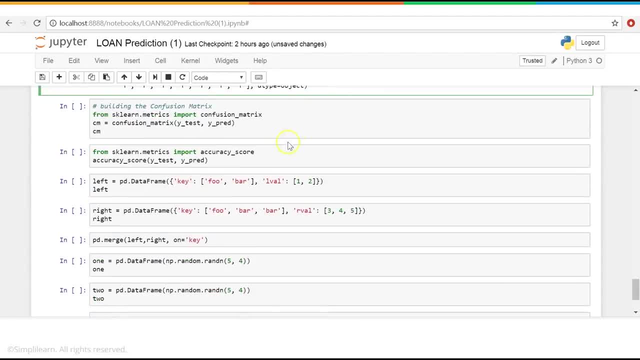 and then indicates no. So Y or N is the output. Now how do we measure the accuracy? As we have seen earlier, I described how confusion matrix works and how we can use confusion matrix for calculating the accuracy. That's what we are seeing here. So this is the confusion matrix. 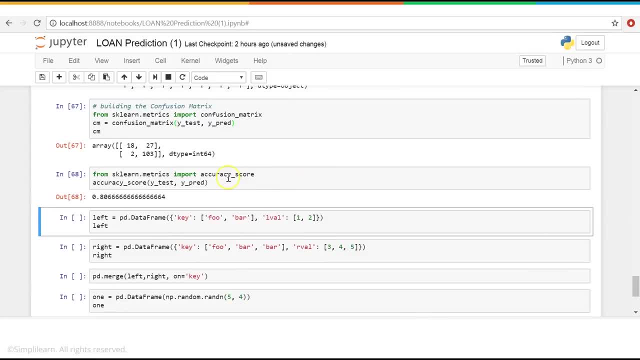 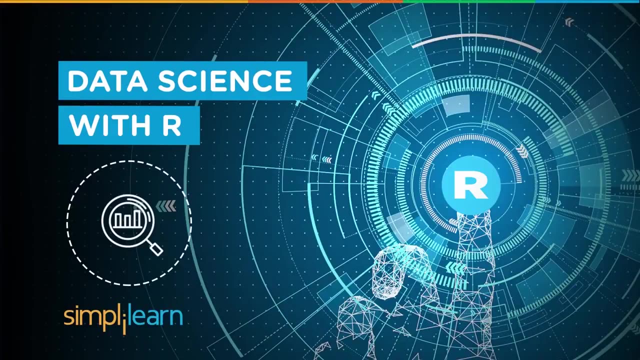 And then you want to do the measure, the accuracy. you can directly use this method and we find that it is 80%. So we in the slides we have seen, when we calculate manually as well, we get an accuracy of 80%. Data science with R, sponsored by SimpliLearn, That's wwwsimplilearncom. Get certified. 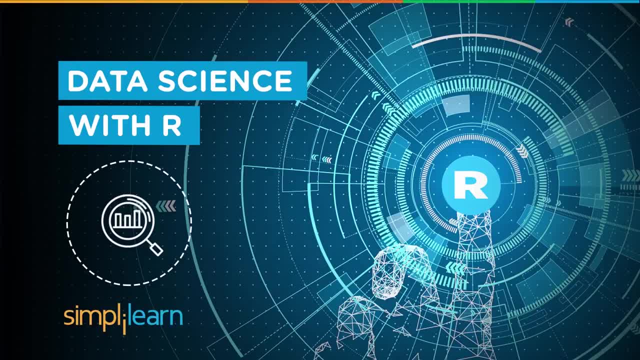 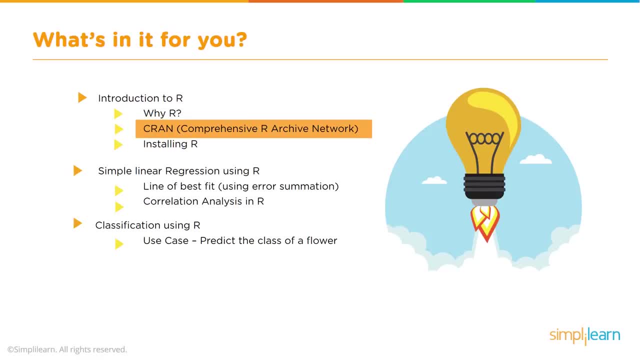 get ahead. My name is Richard Kirshner and I'm with the SimpliLearn team. What's in it for you? We're going to go through an introduction to R, Y-R, CRAN, Comprehensive R Archive Network and cover installing R. Then we'll get into simple linear regression using R. 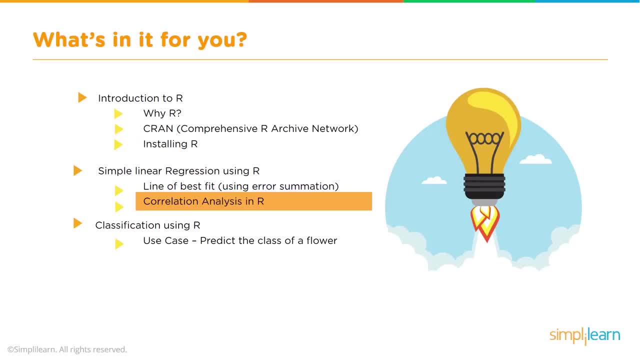 Line of best fit using error summation, Correlation analysis in R, And then we'll get into classification using R. Use case: predict the class of a flower. Let's start with an introduction to R First. it's an open source. 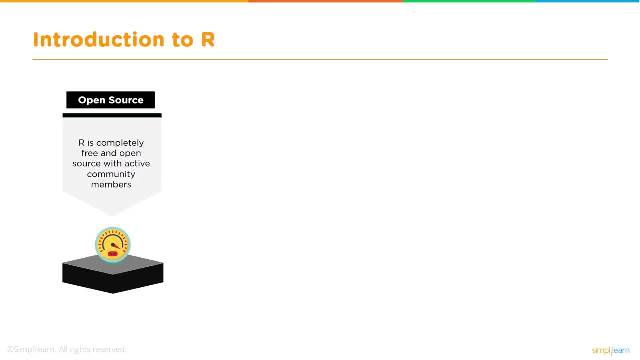 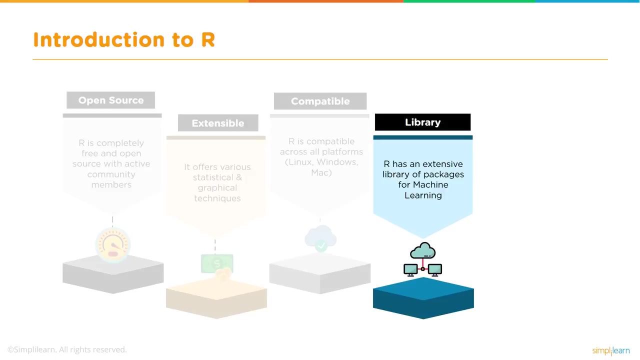 R is completely free and open source, with active community members. Extensible: it offers various statistical and graphical techniques. Compatible: R is compatible across all platforms: Linux, Windows and Mac. Library R has an extensive library of packages for machine learning. 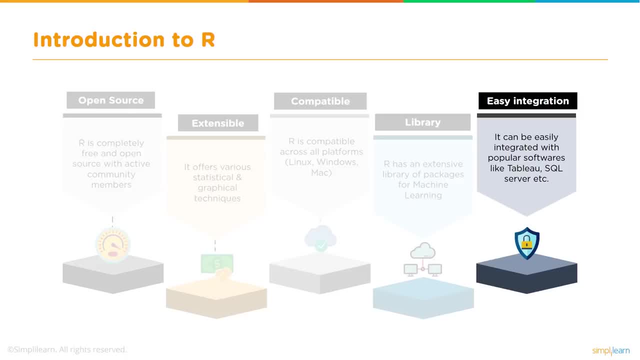 Easy integration. it can be easily integrated with popular softwares like Tableau, SQL Server, etc. This only touches a little bit on these different aspects of R. The fact that it's a free: it's very extensive. It probably has one of the most extensive set of data analysis packages currently out. 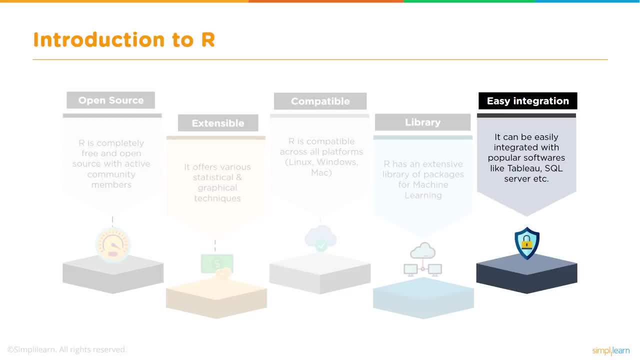 It has a compatibility that is continually growing, So it's integrated with everything from cluster computing to Python integration, which is now coming out, And it's extensive libraries. allows you to import the different libraries to use for whatever your needs are. Makes it a very diverse and easy to use coding source for analyzing data. 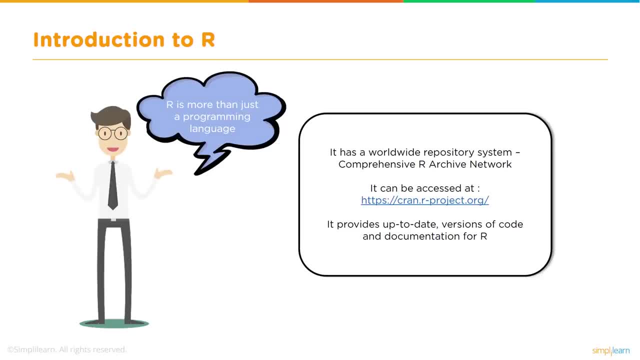 R is more than just a programming language, As I just touched upon it. it has a worldwide repository system Comprehensive R archive network, And it can be accessed at https//cranrprojectorg. It provides up to date versions. It provides up to date versions of code and documentation for R. 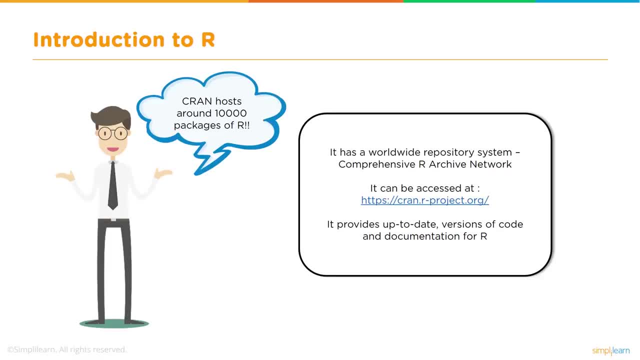 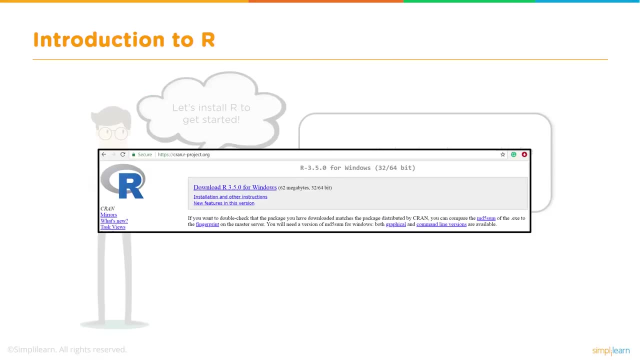 CRAN hosts around 10,000 packages of R. That is a huge repository focused on just data analytics. Let's install R to get started. You can easily download the executable file for R and install it from CRAN website If you go under the downloads. in this case, since I'm on a Windows machine, 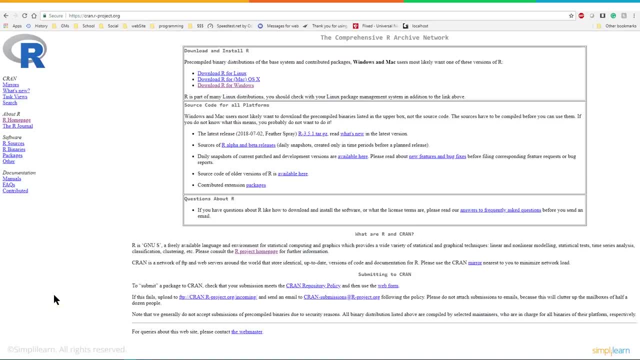 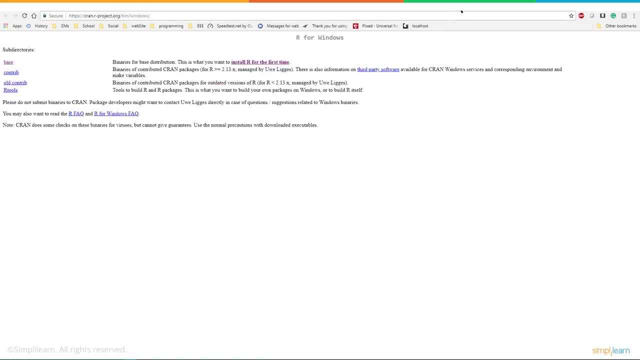 we'll walk through it from the R 3.5 version for Windows. Here we are at https//cranr-projectorg And you can see down here we have the different options for the downloads. If we go under Windows, which is, I'm on a Windows machine. 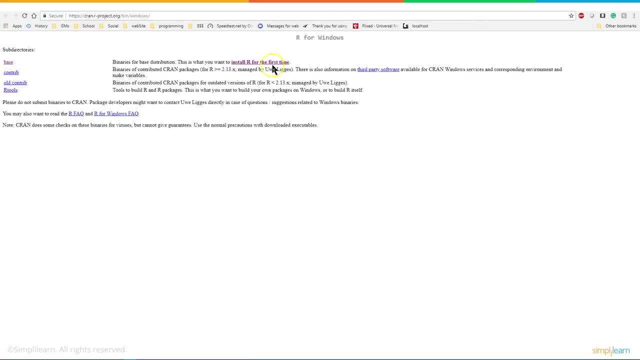 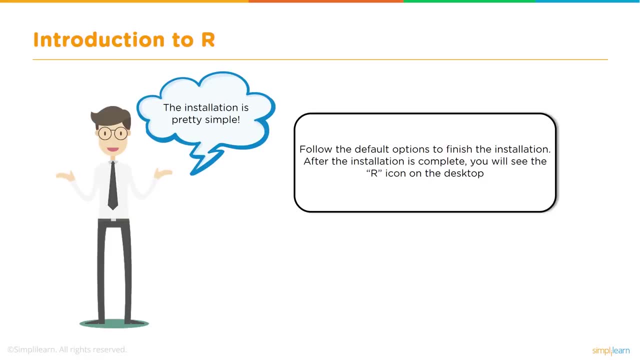 If you're on a Mac machine you can do the Mac or Linux. There's install R for the first time. Just click on that and open and run it. The installation is pretty simple. Follow the default options to finish the installation. After the installation is complete, you'll see the R icon on your desktop. 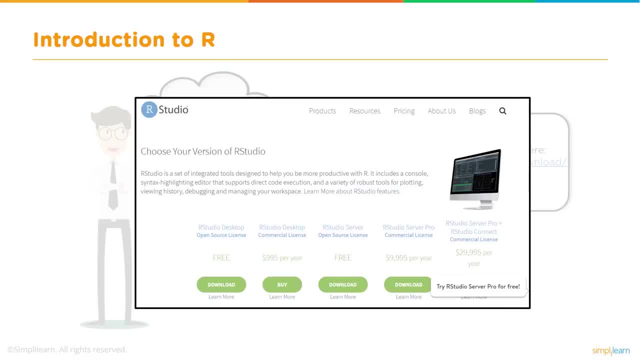 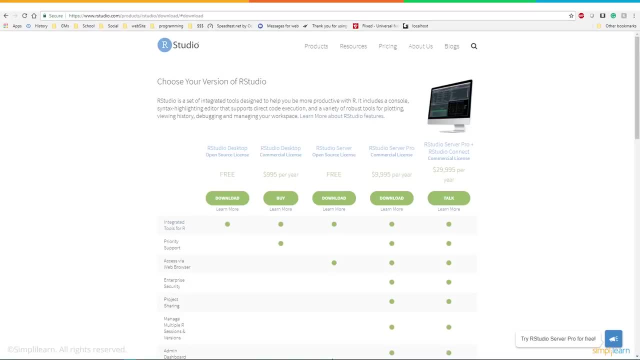 Alternatively, if you want to install R, just click on the R icon. Alternatively, there are mirror sites, and so we can go into RStudio. Let's just take a quick look at that. If you're on the RStudio website, that's wwwrstudiocom. 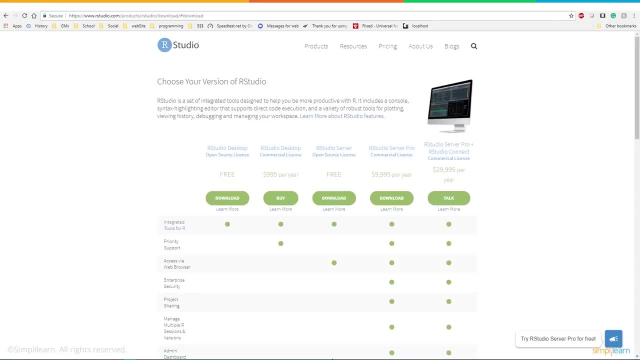 You can go down under products and RStudio download. You'll see a number of options here. The first one is the RStudio desktop open source license. That's the same thing. you just download it. So if you download that, that's what you're getting. 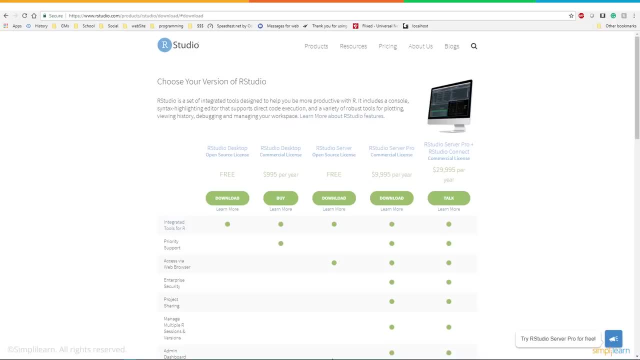 There's also an open source server setup which is also free. You can download from here, And then RStudio offers a number of paid packages which includes all kinds of different supports for company and individual level setup. Whether you go through the CRAN site or the RStudio site, the installation is pretty simple. 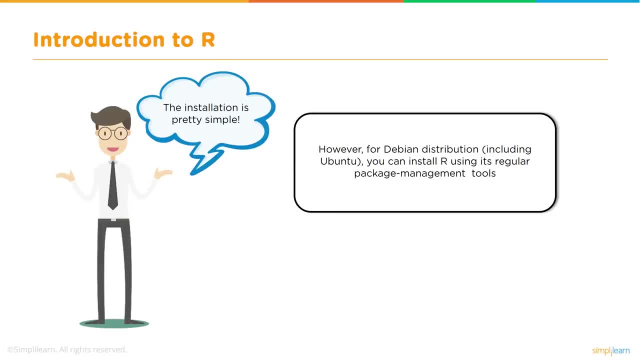 Just a quick note. if you're a Debian distribution, including Ubuntu, you can install R using its regular package management tools, And when you're using a Linux system, that is preferred because then it registers it properly on the setup system. Let's go ahead and open up our RStudio and take a look. 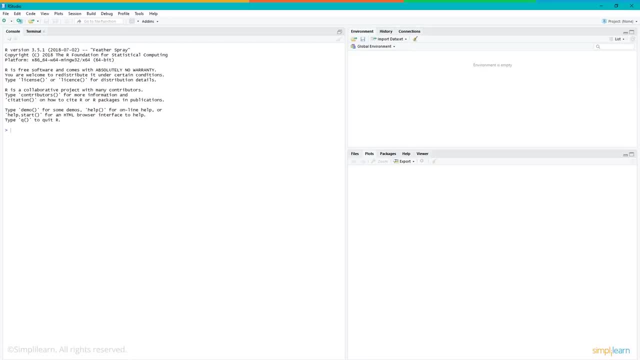 Here we are. We opened this up in the RStudio version, which automatically opens up some extra windows, which is nice. Let's go ahead and take a look at that. We have our console on the left. This is your main workspace. 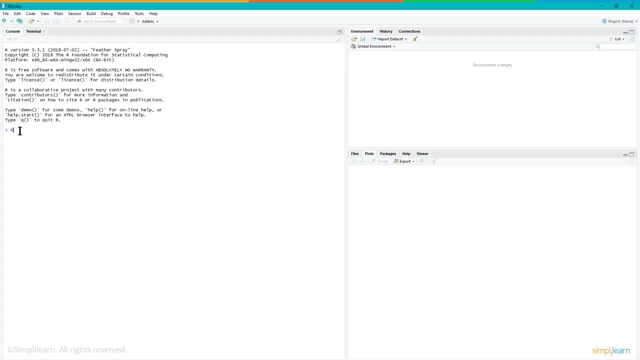 So if I go in here and I click the mouse and I do a 4 plus 4, it'll come up and say the answer is 8. And you have some environmental information And over on the right, you have plots. Usually when you're working in here, let's do a script. 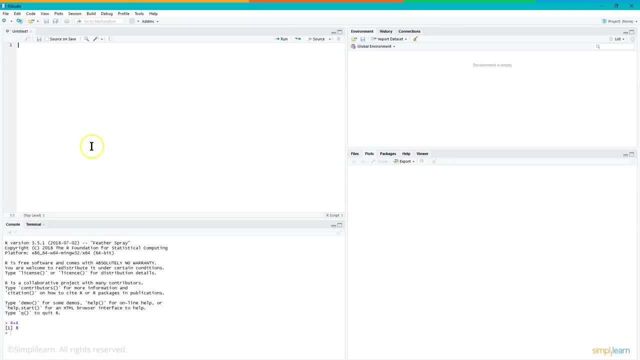 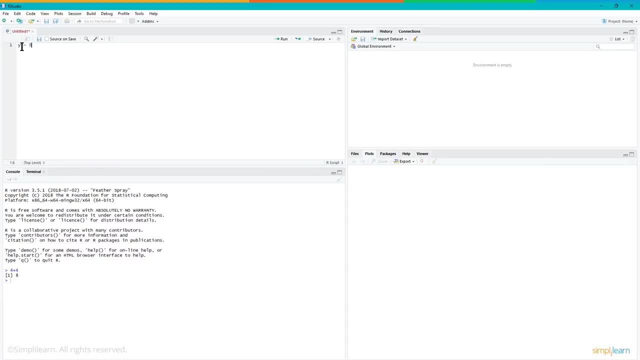 We'll go up here to the plus sign in the upper left-hand corner And just add some scripts. In this case it showed up on the top, but you can move these windows around And let's say I do. y equals 3 plus 4.. 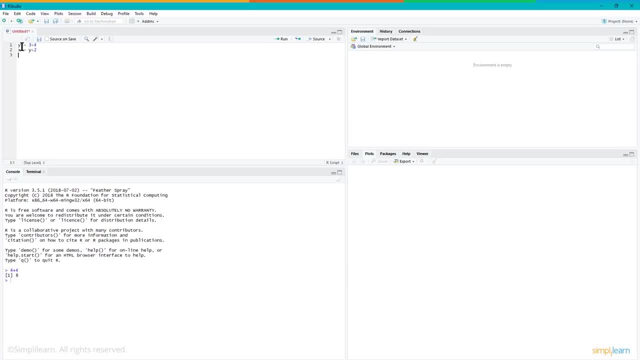 x equals y plus 2.. And then I'm going to do just x, And let's do a plot. We'll throw a plot in there. C- C is a notation that these are going to be Cartesian points. So we got 1 comma, 2 comma 3.. 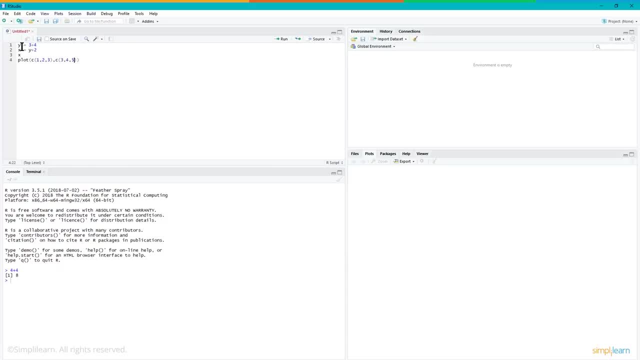 That would be like your x And then y, 3 comma, 4 comma, 5, for just a standard call scatter plot. We don't have to memorize this. We'll go into some of this later on, And then I can take all of this. 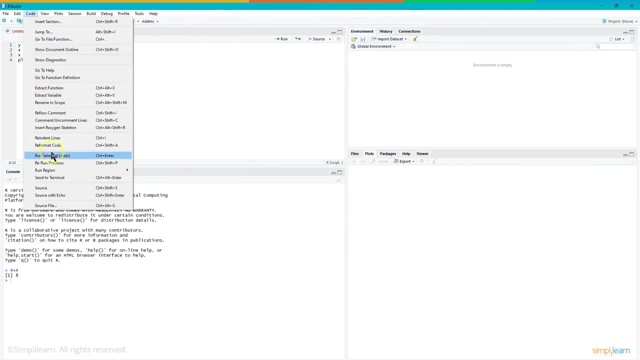 If I go under code, since I'm working in the code console And I go down to run Region and just run all, It takes this code and just runs it through my console And you can see down here it's executed. y equals 3 plus 4.. 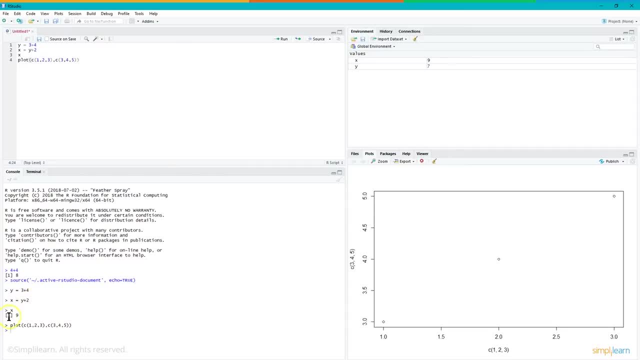 x equals x plus 2.. And if you add 3 plus 4 plus 2, you get 9.. That's what the x does. And then I did a plot. I threw the plot in there. I'm plotting 1,, 2,, 3.. 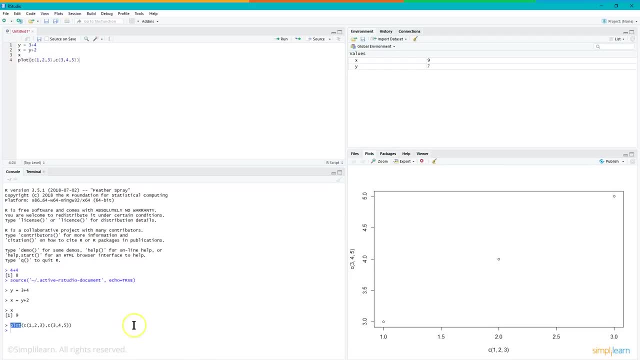 3,, 4,, 5.. And if you use just a straight plot, it's a scatter plot And you can see that this appears on the bottom right where you have your plots coming in. So it's a very quick way to show data. 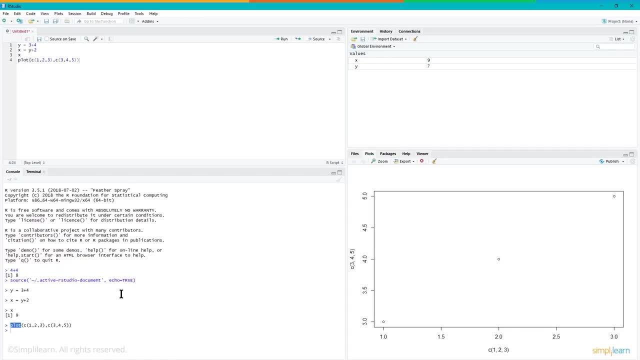 And that's one of the wonderful things about R is it's very easy and quick to go through and do different functions on the data and analyze it, So it's a very popular package. Before you start programming in R, you should install packages and its dependencies. 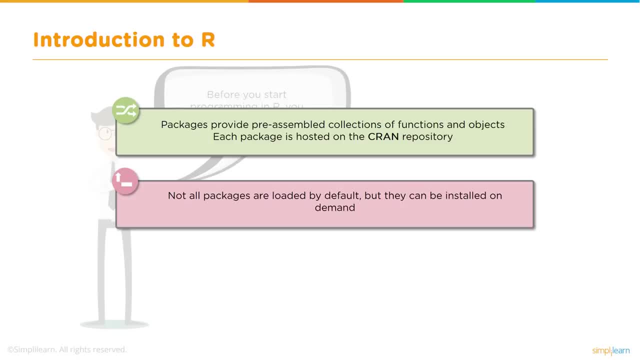 Packages provide preassembled collections of functions and objects. Each package is hosted on the CRAN repository. Not all packages are loaded by default, but they can be installed on demand. Remember earlier we were talking about all the different packages available. You don't want to install everything from R. 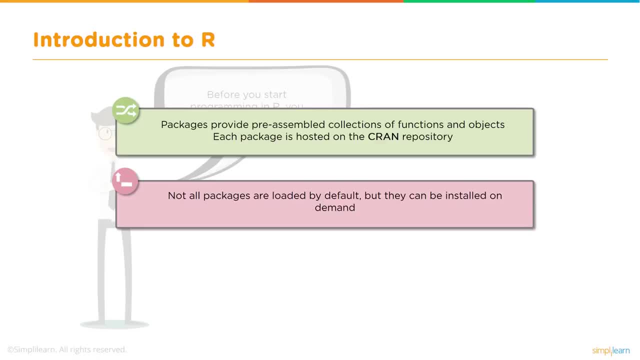 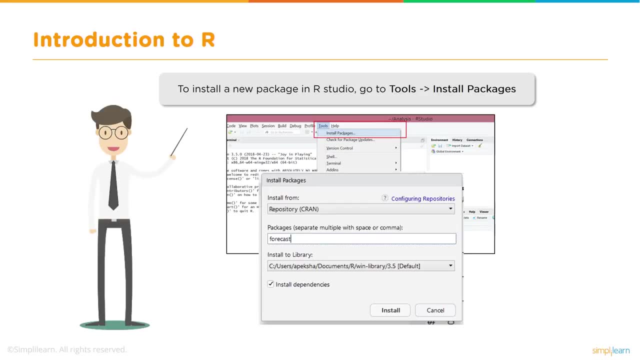 It would just be a huge waste of space. You want to just install those packages you need. So, to install packages in RStudio, you go under Tools and Install Packages. When you click on the Install Packages, you'll get a dialog box. 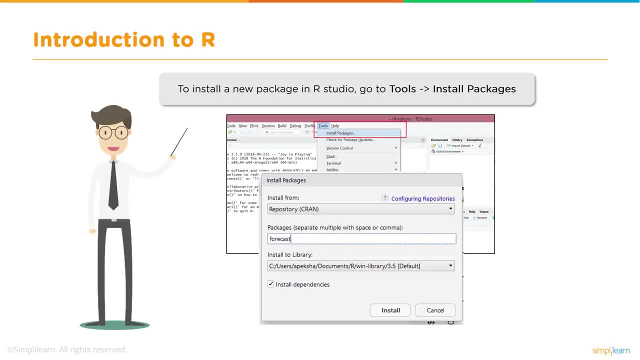 You'll see where it has Repository CRAN, Because there's other repositories and you can even download and install your own packages you can build And then you'll pick out the packages you want and separate multiple with spaces or commas So you can install numerous packages at the same time. 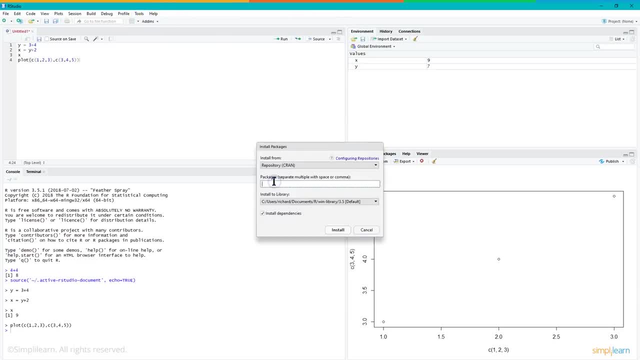 In this case we're installing the Forecast package And you can see down here. I just type in Forecast: Install all the dependencies It uses other packages to build on. It has those. Then just click on Install and it's done. Before we cover the basic linear regression model. 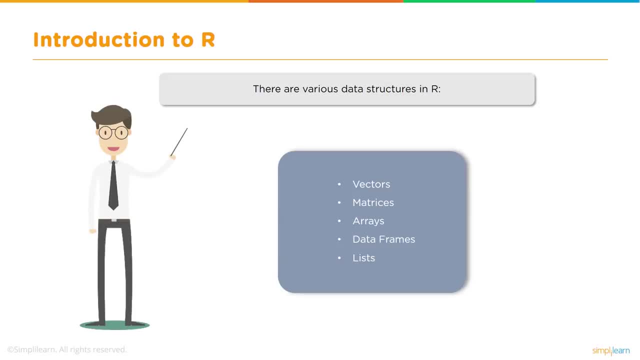 let's just take a quick look at some of the different parts of R or parts of programming you'll need, or scripting. First you need to know there are various data structures in R. We have vectors, we have matrices, we have arrays, data frames and lists. 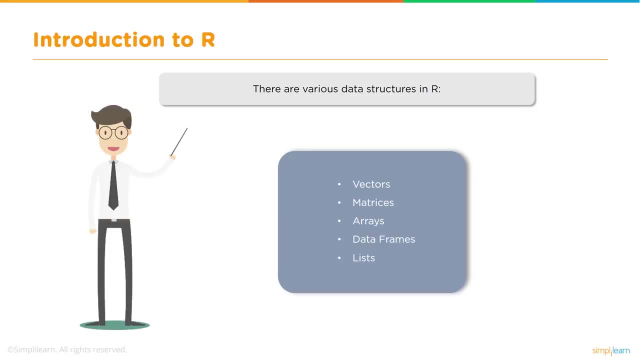 Vectors is the most basic data structure. If you remember, vectors are a location and a direction. That's how they're generally defined, Although vectors, when you're talking about scripting, can contain numerous different values. So you could have vectors with four, five, six, seven, eight different values in it. 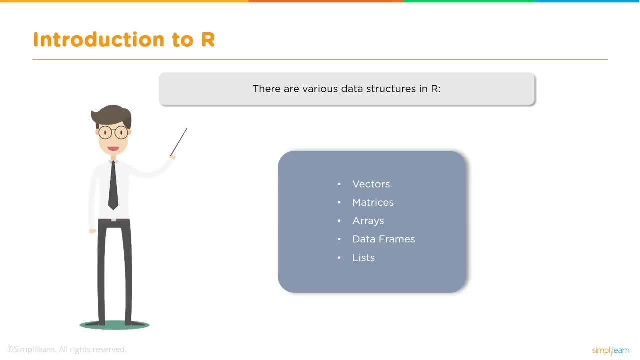 For example, a picture on the computer might have the location of the pixel and the number for the red hue and the green hue and the blue hue. So now you have something with five different numbers in it, consisting of that vector. Matrixes allow you to move stuff around. 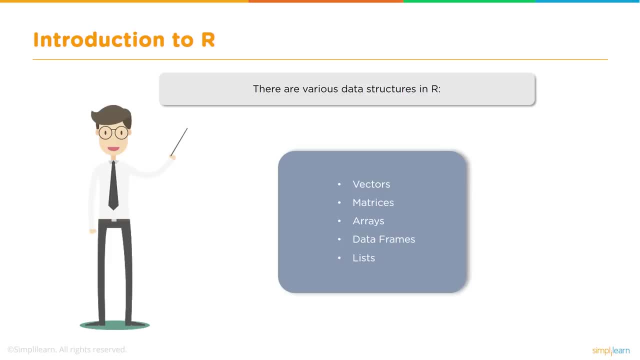 So you might have a two-by-three matrix that you switch to a three-by-two. We looked at an xy plot earlier. It might be that you have everything is you have ten different numbers and each one has two values- xy- and you need to switch that matrix. 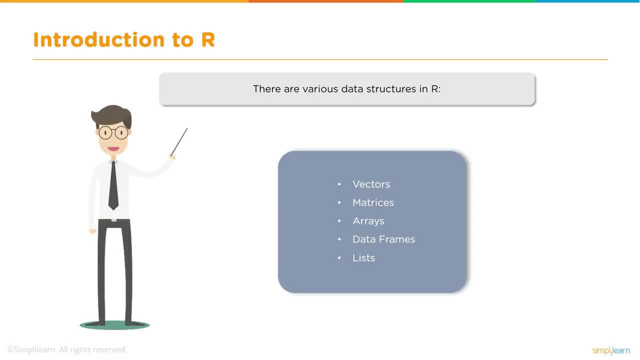 So then you have two arrays of five numbers. Arrays are just that- a collection- and you can have arrays of arrays of arrays. Data frames have labels on them, which makes them easier to use. So usually we use a lot of data frames when we're working with data because they're just easy. 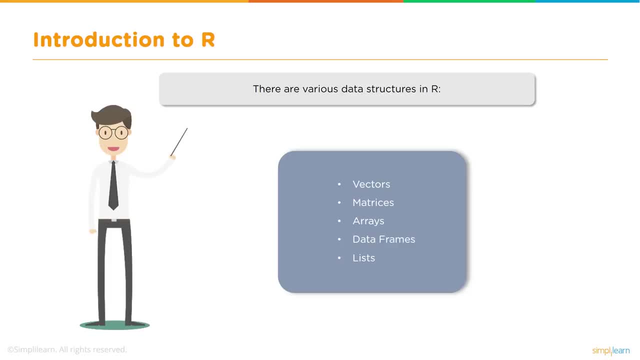 You can have a column and you can have a row. So think of rows and columns when you see the term data frames And then lists are usually homogenous groups. So in R you're listing data. You're usually looking at similar data that's connected in the list. 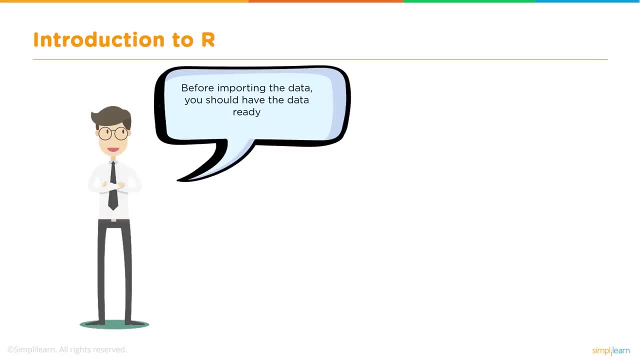 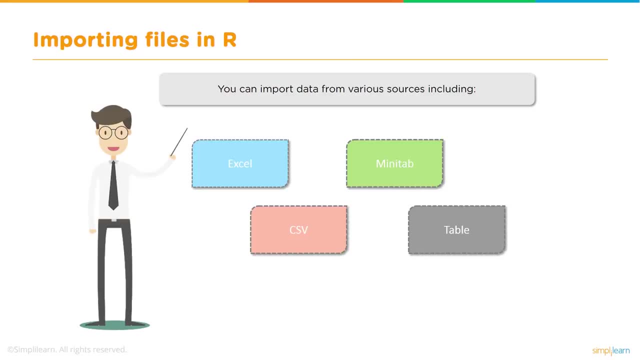 So the first thing we do, before we're even importing the data, you should have the data ready, So we need to look at the data and see what's going on. You can import data from various sources, including Excel, Minitab, CSV, Table, text files. 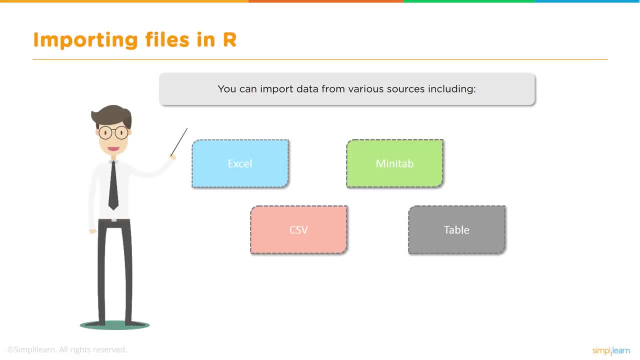 CSV is usually a text file. comma-separated variables, tab-separated variables- There's all kinds of different options here, And importing the table is very simple. We have table read. table file equals data, table Header equals true. And let's just take a closer look at what we're talking about here. 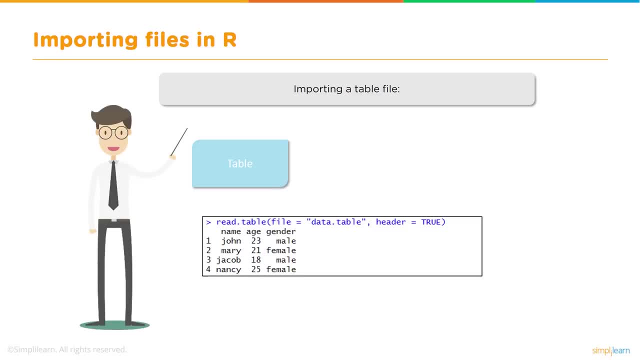 Scratch the closer. look, I didn't realize, it was just, for example. So importing a table file is pretty simple. You readtable file equals datatable. So whatever the name of the file is, Comma header equals true, So if there's a header to it. 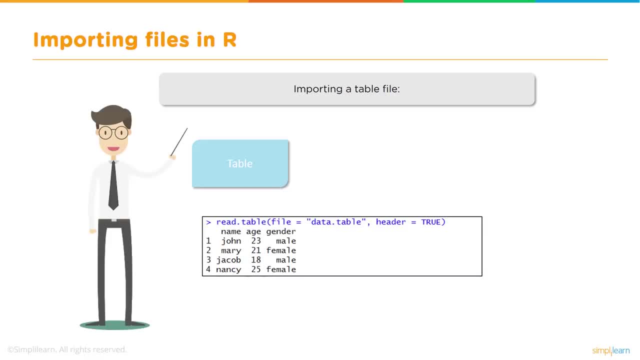 In this quick flash they have name, age, gender. We'll actually do this in R with another data set in just a minute, But you can see it's very easy to read. A lot of people use R, even in other programming languages. 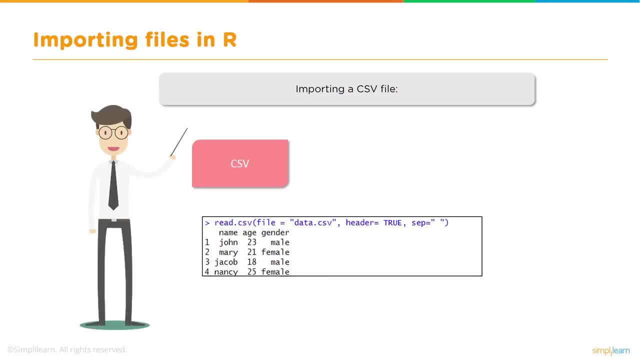 So they can quickly look at the data before they even start analyzing it. CSV file: same thing. Readcsv File equals data. CSV Header equals true Separation equals space. So in this case, even though CSV stands for comma-separated variable, 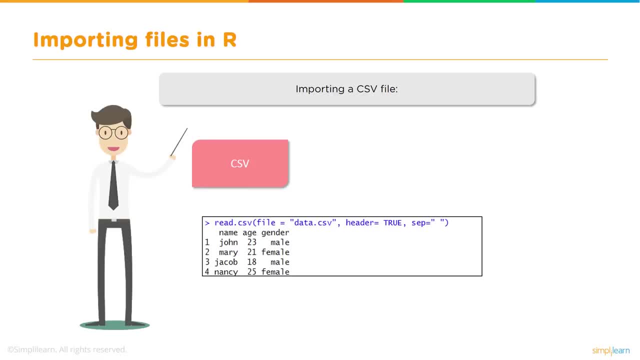 this one is separated by spaces And they have the header name, age, gender, So it's the same file saved as a CSV file. And there's also Excel. Excel has its own issues as far as making sure you know what the tables are. 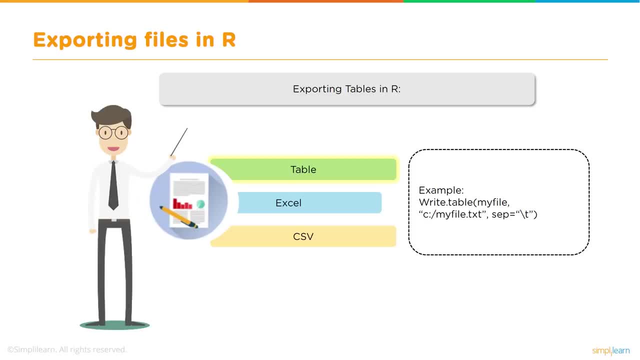 and the headers are, But you can see that each one of these is easy to use. You can also import, And just like it's easy to import the data, you can also export tables in R. So you can see here: writetable myfile c, myfiletext separated. 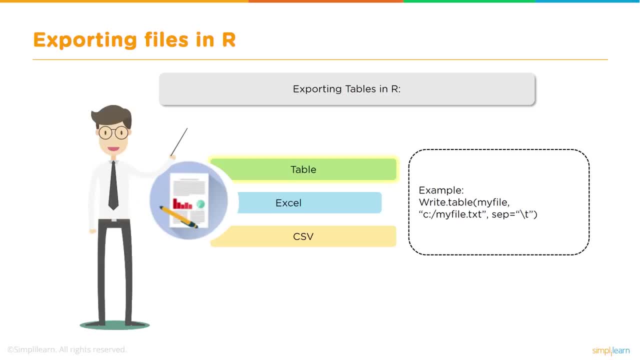 And the scoop t just means it's tab-separated. So if you're using tabbed files on there- Example Excel- So you can write a xls to myfile. In this case they did a text Separation equals scoop t. 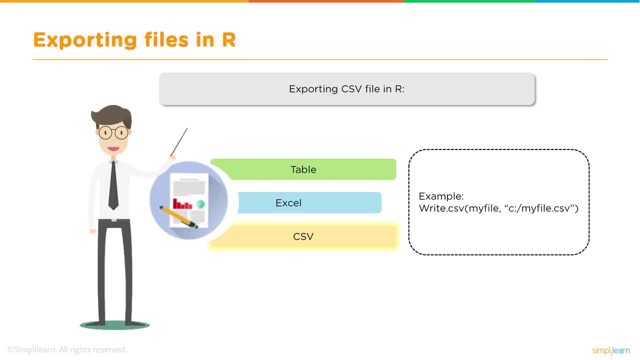 So it's a tab-separated for Excel file, CSV: same thing. Very easy to write a CSV file on there And you can also export it to your computer once you've changed the data or altered it, depending on what you're doing with it. 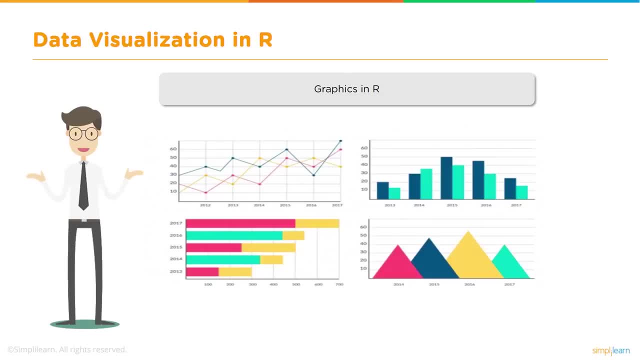 And once we have our data imported and we can save it afterwards and export it. graphing Visualization in R is very powerful and it's quick. I love doing this before even exploring the data. Sometimes you just want to graph it to see what it is there. 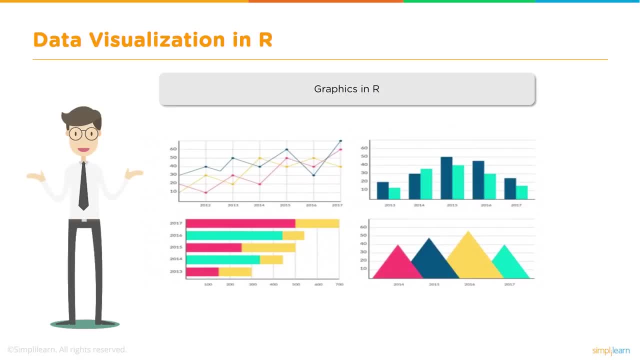 so you have an idea of what you're looking for. So graphics in R cover a huge amount of different things. R includes a powerful package of graphics that help in data visualization. These graphics can be viewed on screen, saved in various formats, including PDF, PNG, JPEG, WMF and PS. 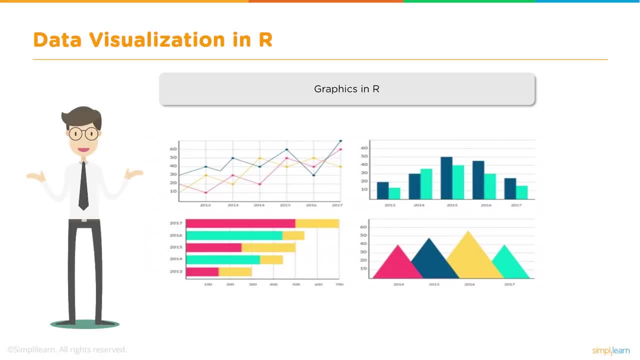 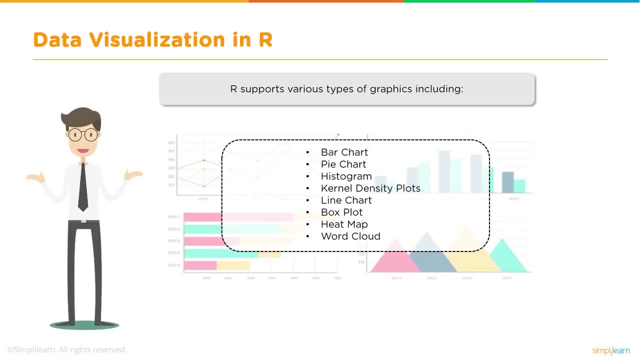 It can be customized according to varied graphic needs. You can copy and paste in Word or PowerPoint files. R supports various types of graphics, including bar chart, pie chart, histogram, kernel density plots, line chart, box plot, heat map, word cloud. 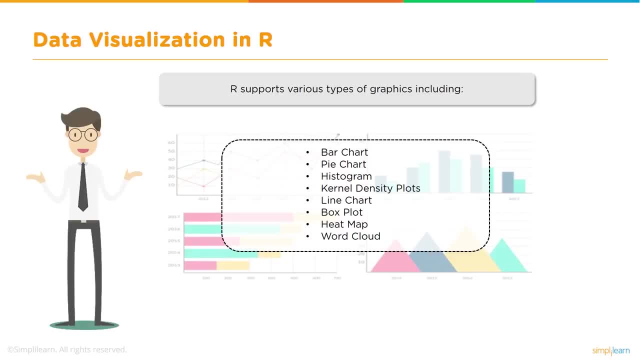 There's even some more obscure ones, But these are the main ones that most people use. I know I use a lot of heat maps, but word clouds are a lot of fun if you're doing websites and word analysis And histogram is very popular. 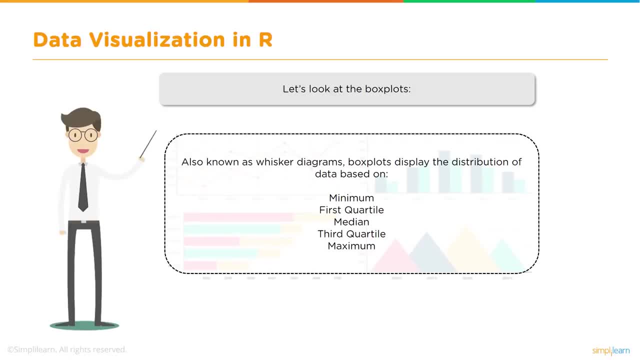 All of these are very widely used. Let's look at the box plots, Also known as whisker diagrams. box plots display the distribution of data based on minimum, first quartile, medium, third quartile and maximum. So right off the bat, we can use a box plot to explore our data with very little work. 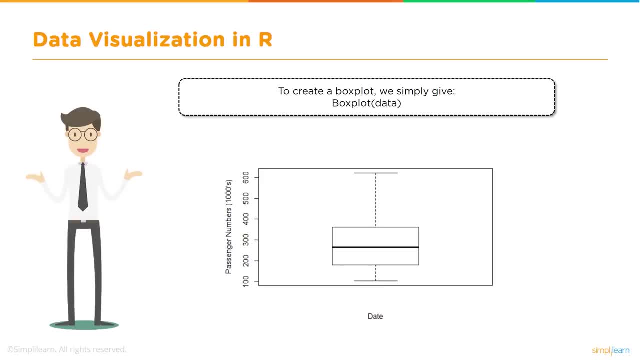 To create a box plot. we simply give a box plot and the data Very straightforward, So we might have passenger numbers in the thousands. I guess this is exploring data dealing with airplanes And you can see here they just have a simple plot. If you break it down, you have your, if we go back one. 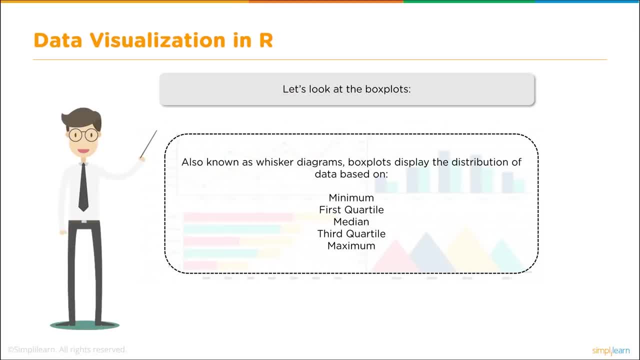 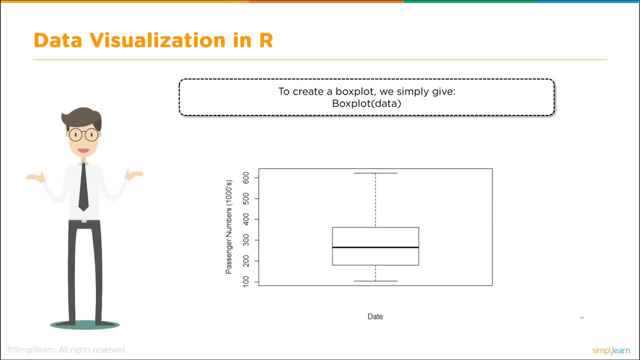 you'll notice, we have like a minimum, a maximum, our medium, first quartile and third quartile. Let's just break that apart. You can see the line on the bottom is your minimum, Your line on the top is the maximum. 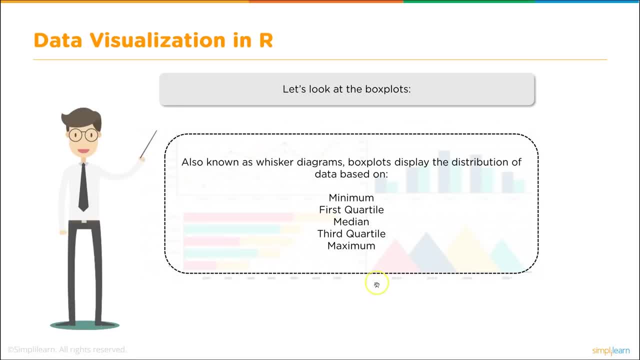 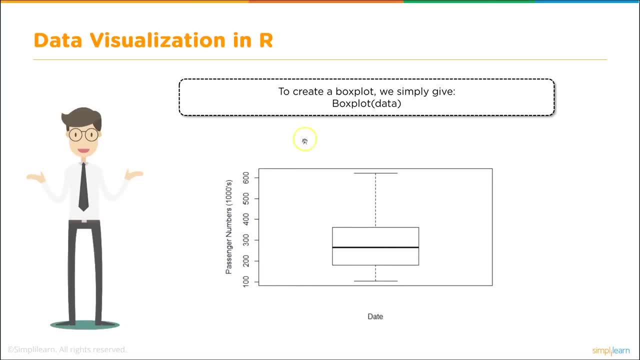 You have your medium and your first quartile right there- First quartile and third quartile- And the way a lot of times you read this is things that are above the box are outliers and things below the box are outliers, And what's in the middle of the box is usually the data you're looking at. 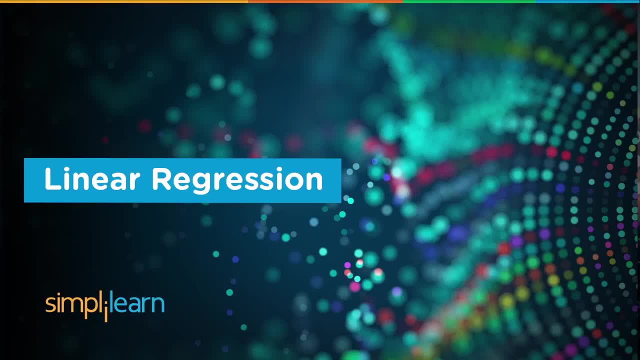 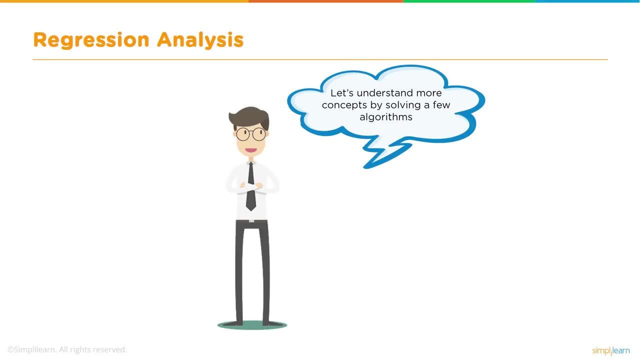 Linear regression. Now that we have a few tools of what R can do, let's look at the theory behind linear regression and how that applies to what we're going to use in R. Let's understand more concepts by solving a few algorithms. Firstly, linear regression, which can be applied in two ways. 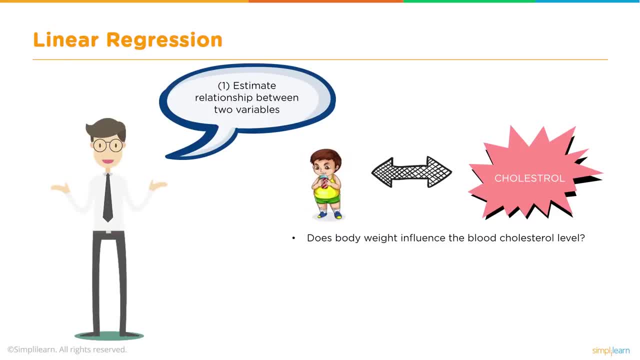 One we can estimate the relationship between two variables. Does body weight influence body weight? Does body weight influence the blood cholesterol level? So we just want to know if it's even a valid connection or not. Will size of the house affect the house price? 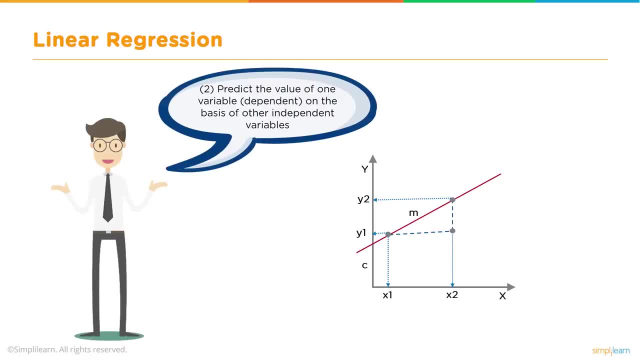 So we can estimate the relationship between two variables also, And then we can predict the value of one variable dependent on the basis of other independent variables. So once we know they're connected, we want to use that to go ahead and predict it. In the cases above, maybe the body weight versus cholesterol. 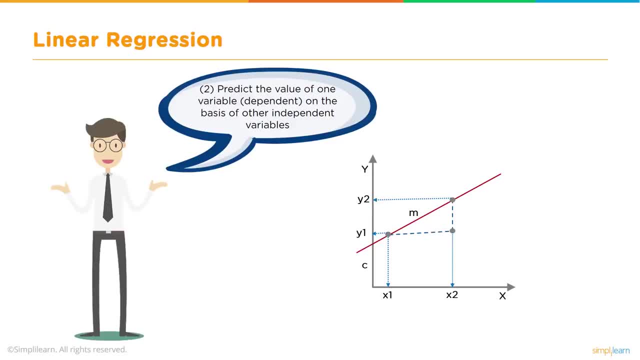 So the more, the higher the body weight is, probably the higher cholesterol. So first we explore: is there a connection? And if there is, can we actually apply that to a linear regression model where we can see those, how they're connected? 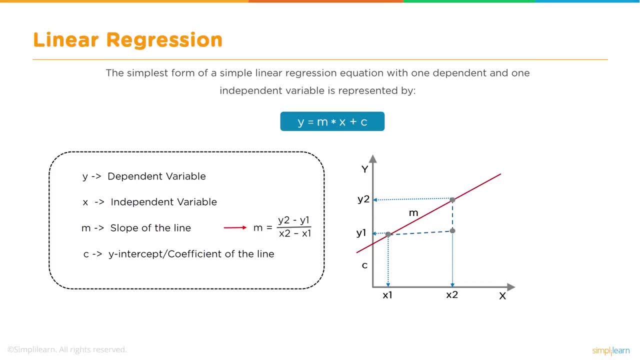 Same thing with house pricing. The simplest form of a simple linear regression equation with one dependent and one independent variable is represented by: y equals m times x plus c, y being the dependent variable, x being the independent variable, m being the slope of the line which you can see over here on our graph. 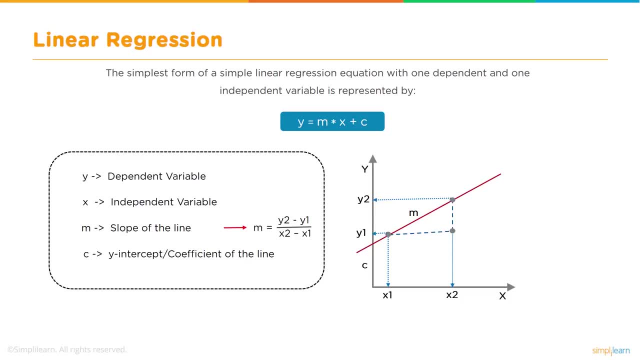 equals y2 minus y1 over x2 minus x1.. And c being the intercept or the coefficient of the line. Now you don't have to memorize all the formulas we're going to go in here, because most of R does this for you. 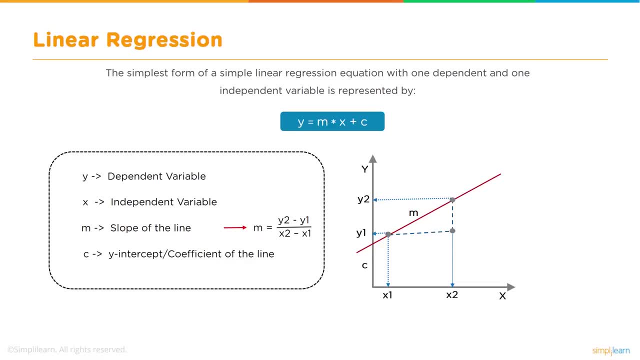 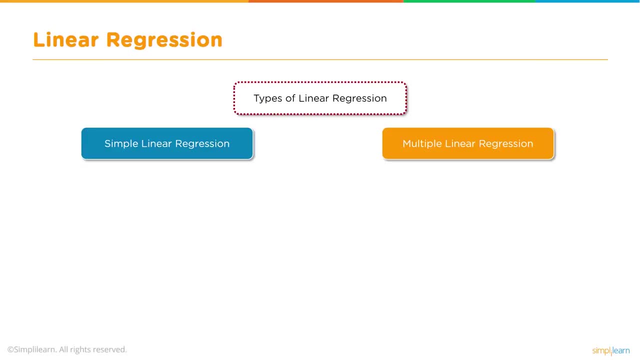 But you do need to know what's going on in the back end so that you can understand if it's working or it's not working where the problem lies. Types of linear regression: There's simple linear regression: considers one quantitative and independent variable. 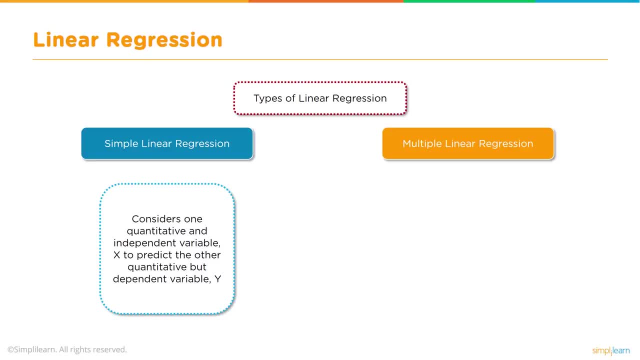 x to predict the other quantitative but dependent variable, y, And that's a formula we just saw: y equals m times x, Y equals m times x plus c. And then we have multiple linear regression: considers more than one quantitative and independent variable. 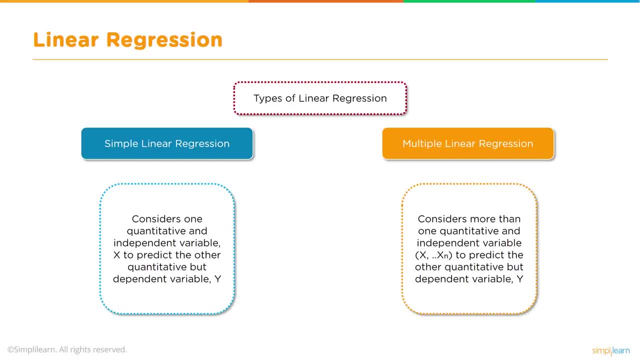 So instead of having just x, you have x of 1,, x of 2,, x of 3, to predict the other quantitative but dependent variable, y. So instead of looking at just body mass, we might also look at height. 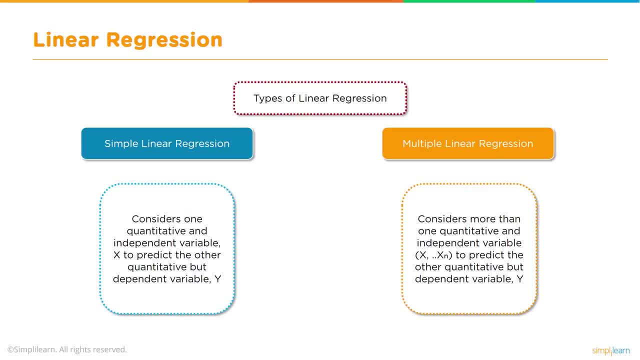 So you have: body mass and height would be two independent variables. Housing prices might have to do with the distance to a certain area, So location might be one of the variables, along with the size of the house. Let's consider a sample data set with five rows. 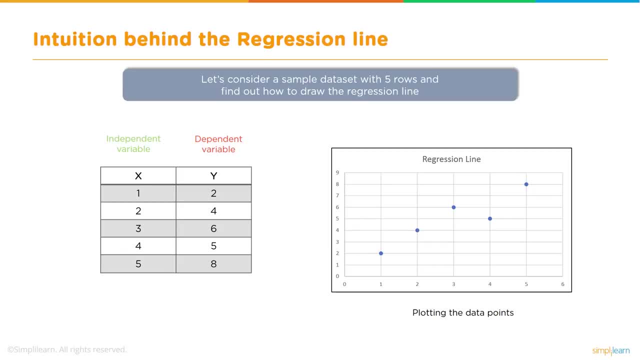 and find out how to draw the regression line. So in here you can see we have independent variable and our dependent variable. We've taken some random data. In this case we have 1,, 2,, 3,, 4, 5 for x. 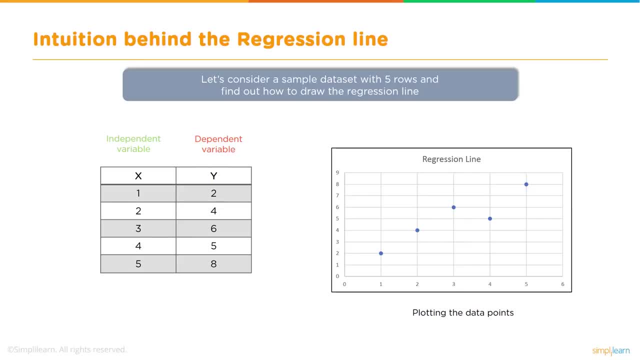 and we have 2,, 4,, 6,, 5,, 8 for y And the first thing we do is we might plot it. If you look at the plot you can see that it has a nice line through it. 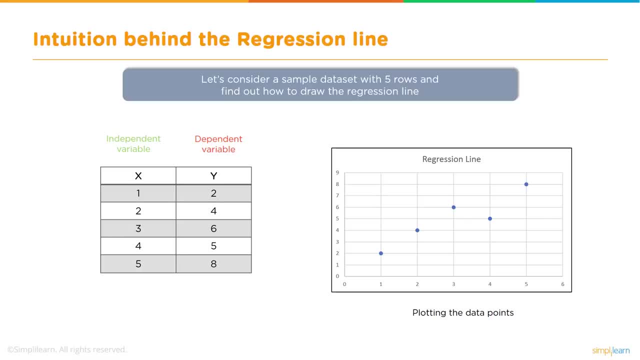 Just eyeballing it, you can guess that there's probably a linear regression model that will fit this data. Then we go ahead and calculate the mean. We count the mean of x and the mean of y And you can see that. we plotted that on there- 3,, 5 for this particular data set. 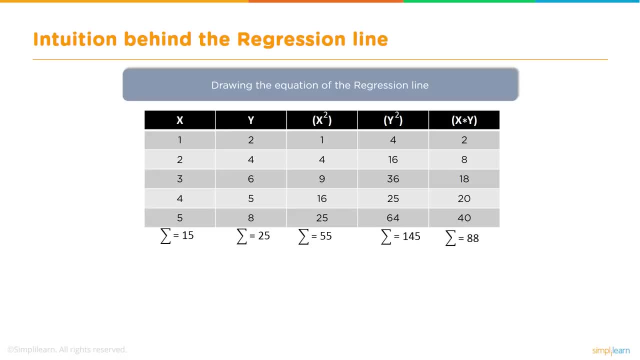 And so, drawing the equation of the regression line, we'll go ahead and take a summation of x, a summation of y, take a summation of x squared and a summation of y squared, and then x times y. This is why it's so nice for the computer to do this work for you. 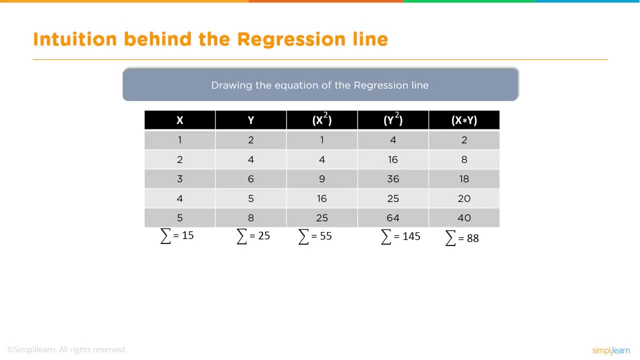 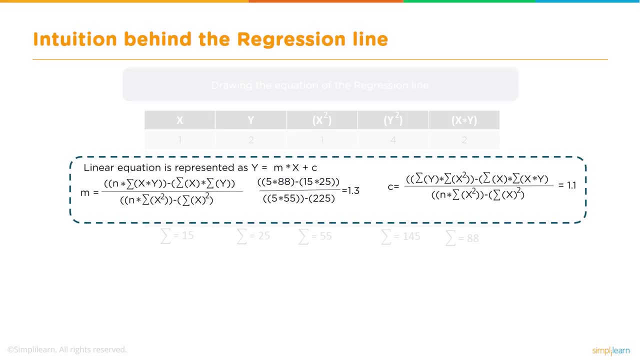 because I don't know about you, but I hate sitting there with a calculator And if you have just five variables that would be very long, not a big deal. But if you're doing hundreds of variables, definitely much easier to let the computer do it all. 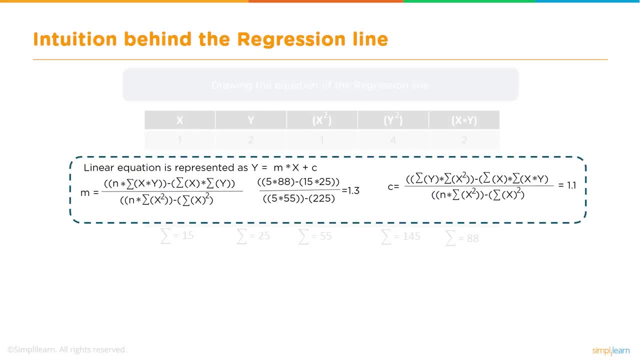 So the intuition behind the regression line breaks down to the linear equation, which is represented as: y equals m times x plus c. In this case, m equals this very lengthy formula where you have your summations. So all the values that we've already computed fit right into this equation. 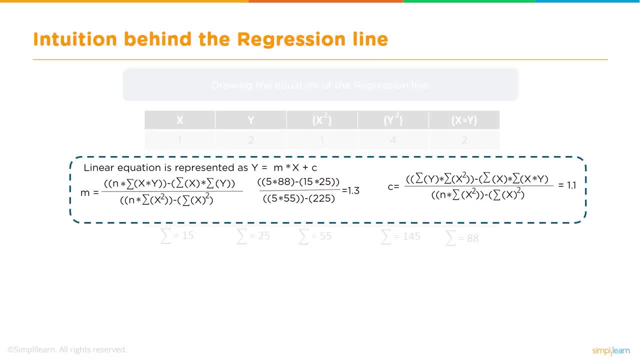 And so you have n being the number of variables. That's what the n stands for: Your x times y. we computed the sum of x sum of y over the number of variables times the sum of x squared, minus the sum of x squared. 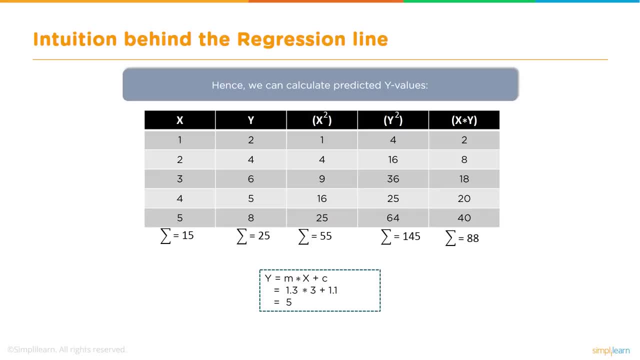 And then, of course, you put the numbers in and you get a value of 1.3, and you find out that your c is equal to 1.1.. Once we have this formula, we can easily compute the y values. 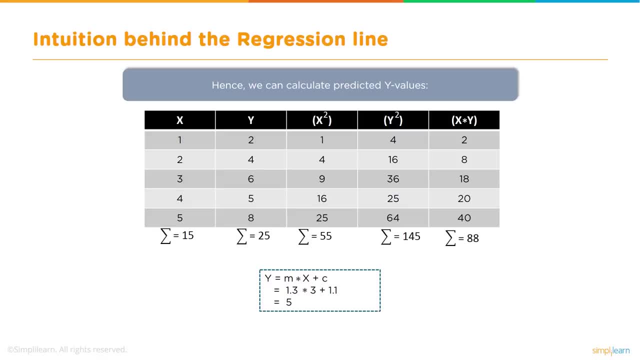 y equals m times x plus c equals 1.3 times 3 plus 1.1 equals 5.. And this would be the example of x equals 3.. You could also put in x equals 6, an unknown value. Let's find out the predicted values of y for corresponding values of x. 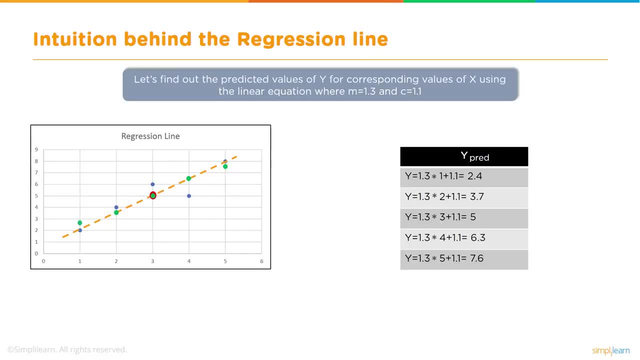 using the linear equation, where m equals 1.3 and c equals 1.1.. So here's our regression line, And then you can see if we put in all the numbers 1,, 2,, 3,, 4,, 5,. 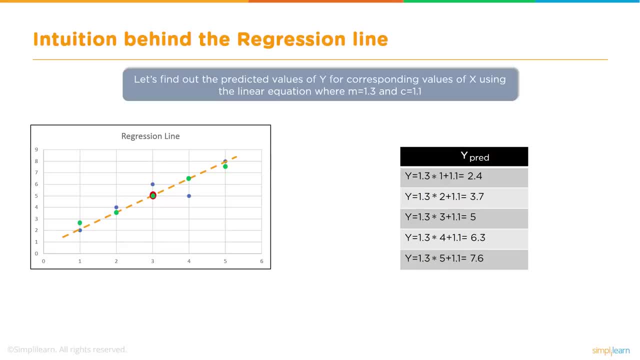 we don't get the exact prediction because it's a line. through the data You'll see that it's ever so slightly off: 2.4, 3.7, 5, 6.3, 7.6.. But it is a good estimate of what the data is going to generate. 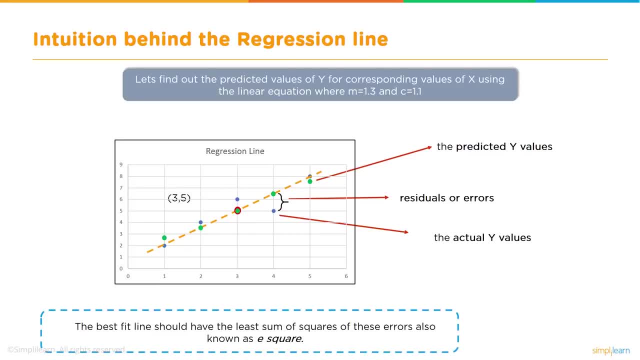 Let's find out the predicted values of y For corresponding values of x using the linear equation. where m equals 1.3 and c equals 1.1,, the best fit line should have the least sum of squares of these errors, also known as e squared. 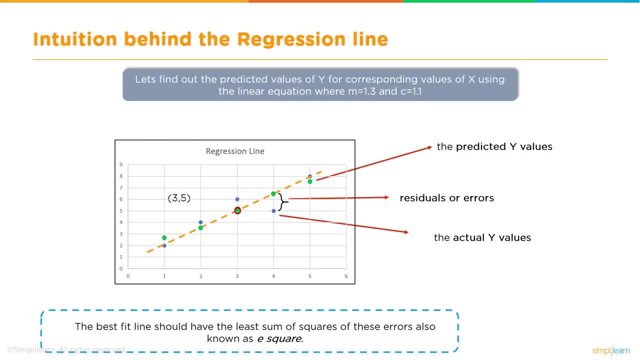 The predicted y value, residuals of errors, the actual y values. So one of the things we're looking at when we put this information together is we want these distances to be minimized So it has the smallest amount of error possible. Let's find out the predicted values of y. 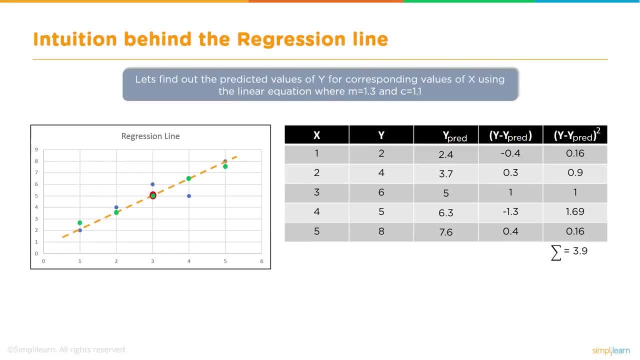 for corresponding values of x, For corresponding values of x, using the linear equation, where m equals 1.3 and c equals 1.1.. And here you can see we've done the same kind of chart. We have our y predicted and then we have the actual y minus the y predicted. 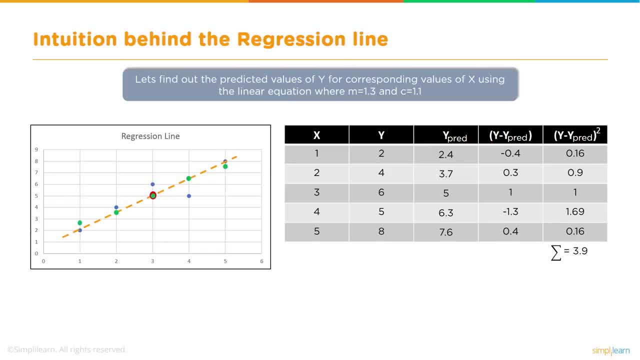 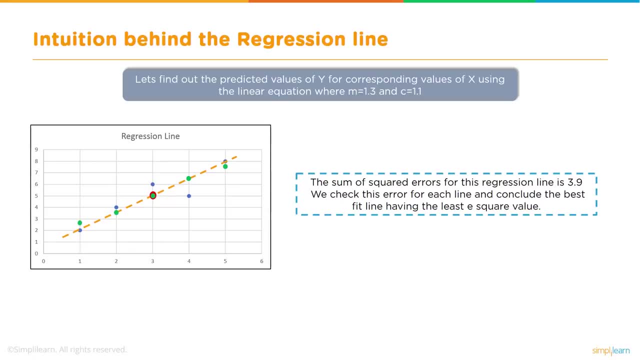 because we are looking for the error squared or the e squared values. The sum of the squared errors for this regression line is 3.9.. We check this error for each line and conclude the best fit line having the least e squared values. Minimizing the distance. 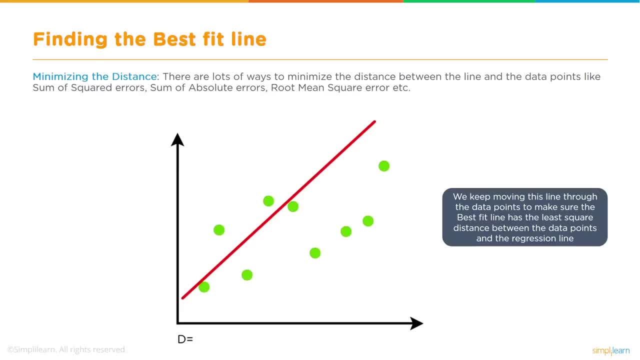 there are lots of ways to minimize the distance between the line and the data points, Like sum of squared errors, sum of absolute errors, root mean, square error, etc. And no matter how you compute the errors you can see here, this is what it's basically going through. 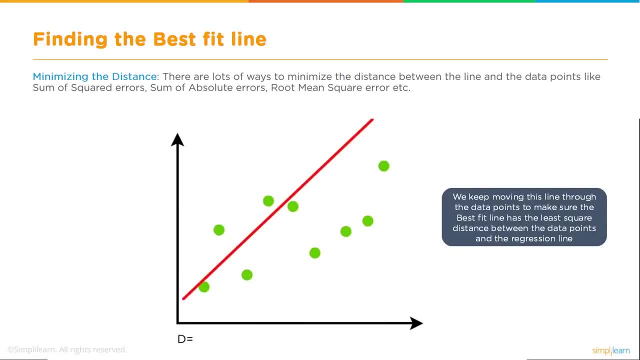 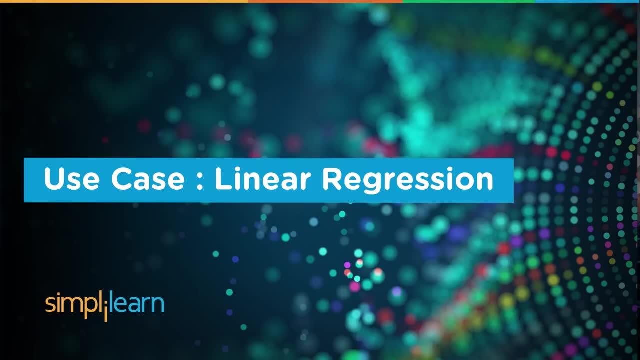 It's taking the line and slowly adjusts it until it has the minimal error available, the minimal distance between the line and the different data points. Use case. We'll start with linear regression and then we'll jump in and also do a decision tree so you can see how they are the same. 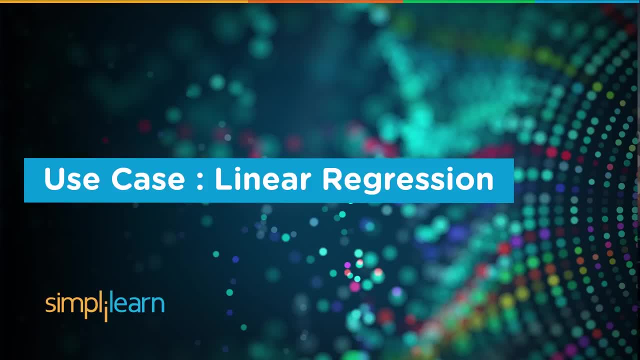 and how they differ in the way they function and what they're used for. And while we're going through the use case, you can start linking the theory behind it connected to the actual use. And as you connect those dots, you can see that by making changes in the model, 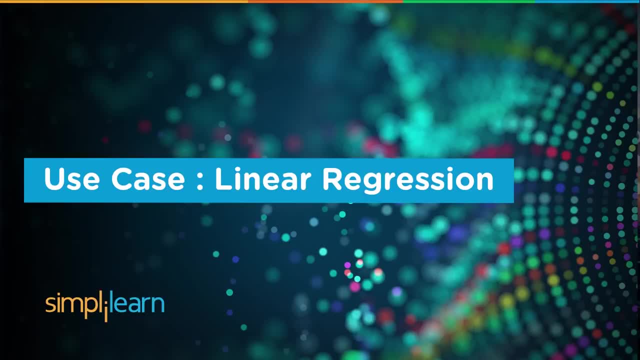 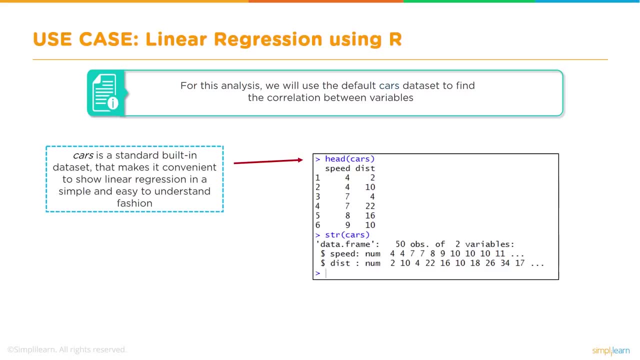 based on the theory. you can also fine tune it. We'll talk about that briefly as we go through this. For this analysis, we'll use the default CARS dataset to find the correlation between variables. CARS is a standard built-in dataset. 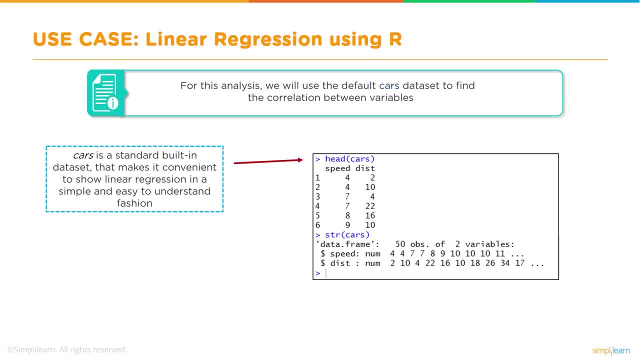 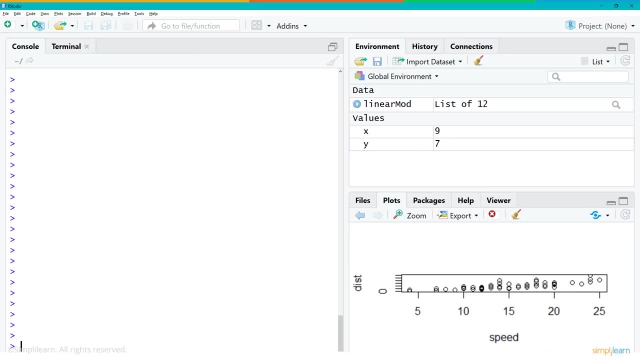 that makes it convenient to show linear regression in a simple and easy to understand fashion, And we'll start with head cars and string cars. Now I've gone ahead and removed the script on here to make this easier to see, And we don't have to do any kind of importing of data. 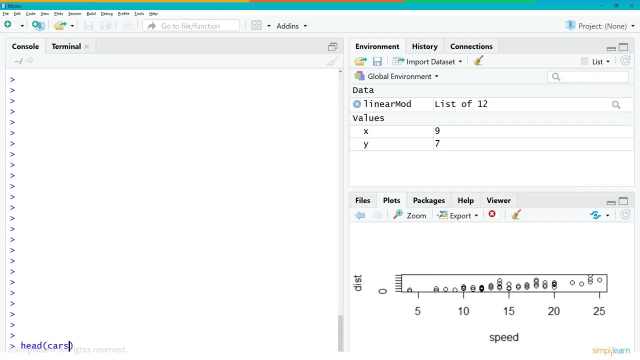 because it's already in there. I'm just going to type in head and cars and hit enter And what you're going to notice is it's going to display the first six rows: one, two, three, four, five, six. 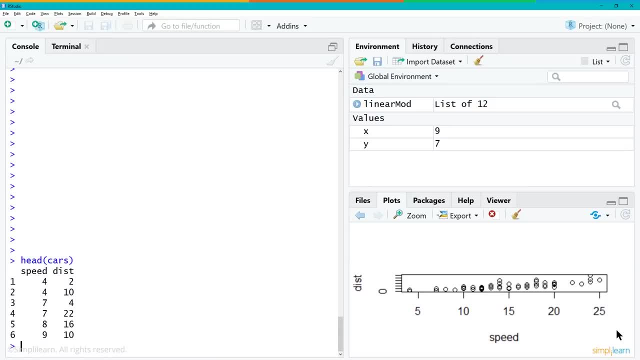 and you'll see speed and distance. Now this is a little bit like a spreadsheet, So if you're using an Excel spreadsheet, it should look the same And this is a standard data frame kind of setup In this case, whenever you say head. 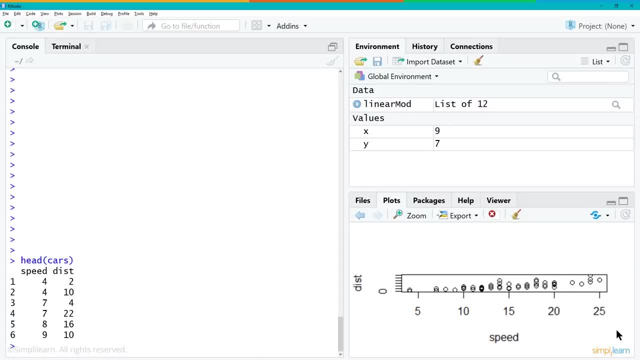 it usually lists the first number of rows, depending on your package. In R it starts with one and then it does the first six rows String. when we do string of cars, it's going to break it down and show us that it's a data frame. 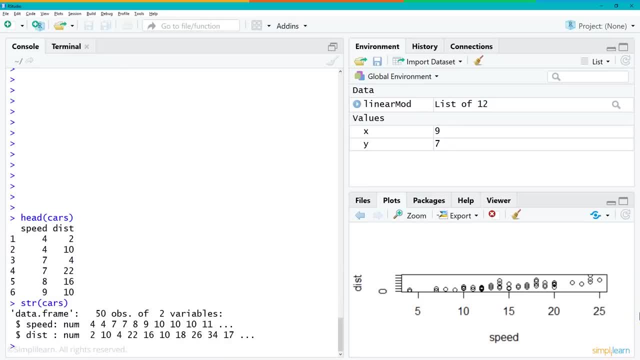 It has 50 objects, that's with the 50 OBS of two variables. And then we have speed. The first variable is going to be a number. that's what NUM stands for: four, four, seven, seven. It just starts listing the data there. 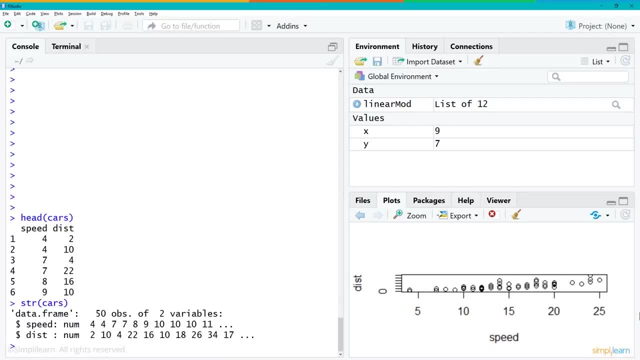 And distance. Now I'm assuming the speed is the speed of the engine. Otherwise, if it's the speed of the car, then the distance should always be the same, And that would just be kind of silly. But this is the speed of the engine. 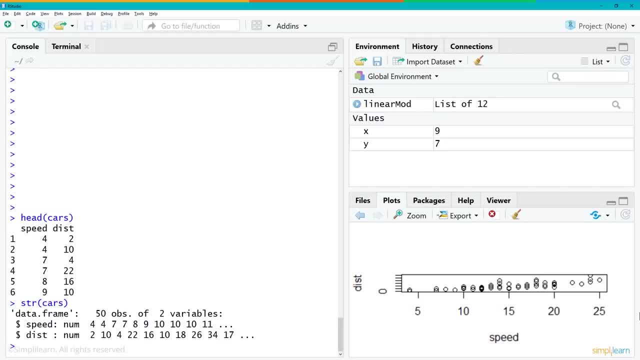 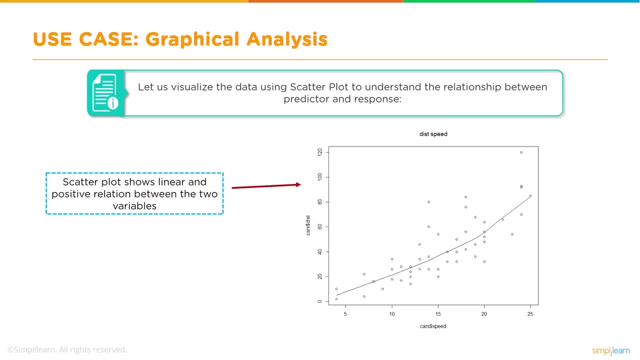 and based on the speed of the engine. can we correlate that to the distance? Let us visualize the data using scatterplot to understand the relationship between predictor and response, And I want you to notice that in this slide a line has been drawn through the data. 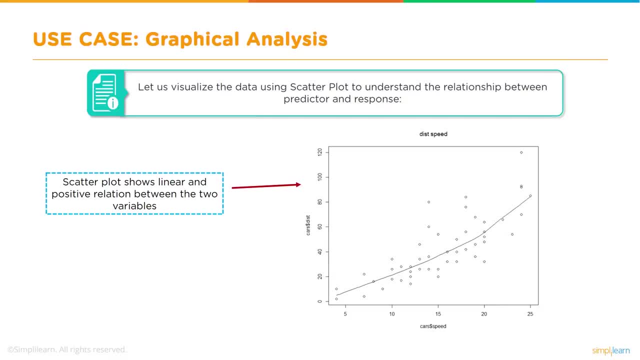 Now, when we first start with data, you don't have that line. So as we plot it, I want you to kind of visualize that line there and just kind of say, hey, does this stuff kind of scatter around a line or not? 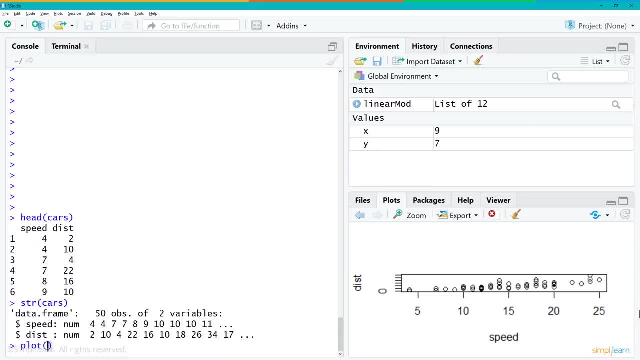 before we actually create the model, And we simply do plot- and I'm going to do a shorthand here- cars and I hit enter and it comes over here to the right and plots our data for us. Now, because there's only two variables, 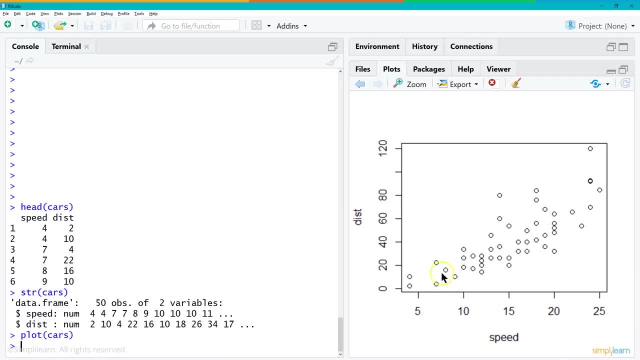 I don't have to do anything special. I'm going to expand this over environment so we can see it And you can see. you can just visualize a line right through the data and it's all clumped into that line, which makes it really nice. 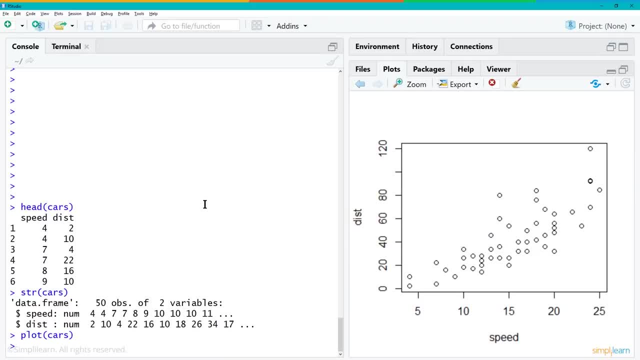 for doing a linear regression model. Now I did something a little tricky here because I'm very lazy. I typed in plot cars A lot of times. you don't want to do that because you don't want to plot all the data We can do plot. 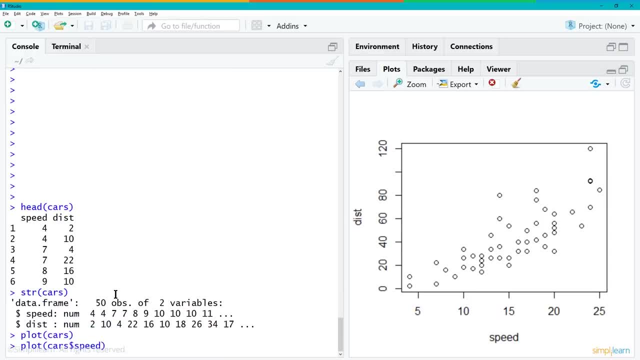 in this case, cars- dollar sign speed. the first variable: cars- dollar sign distance. When I do that, I get the same plot. All I'm doing is telling it to use just these two columns of data, And although the first one is quick and easy, 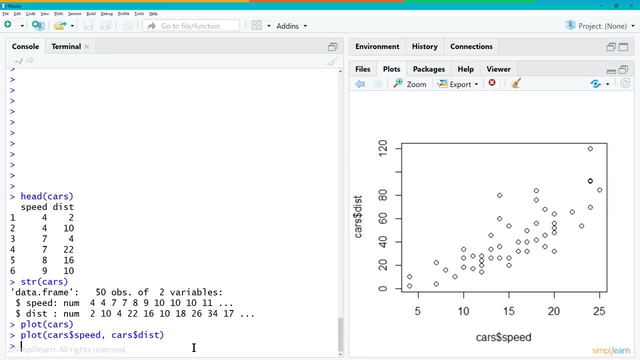 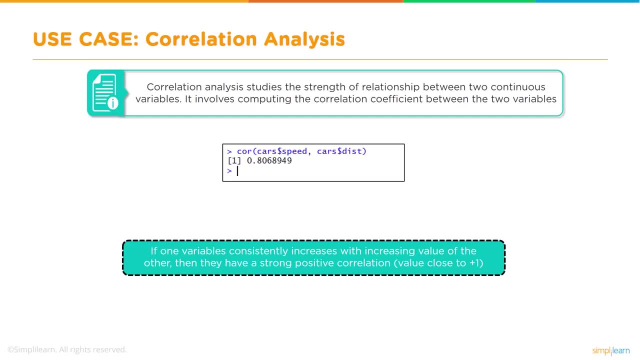 if you only have two columns of data. the second one is what you really want to do when you're plotting data like this. You want to control which columns you're using, And then we want to do a correlation. Correlation analysis studies the strength. 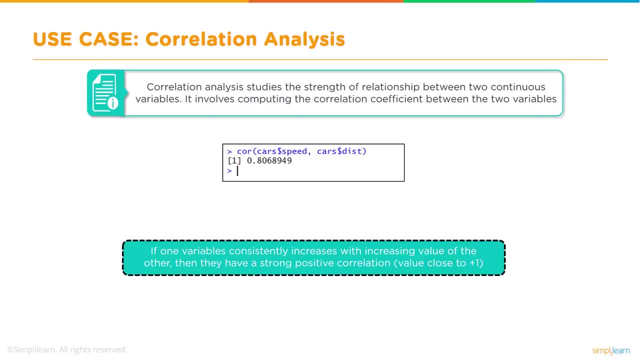 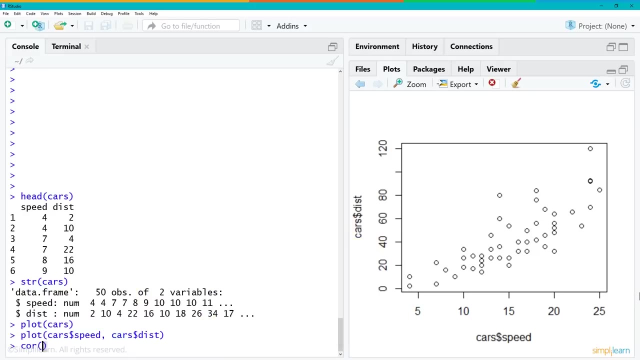 of relationship between two continuous variables. It involves computing the correlation coefficient between the two variables. If one variable consistently increases with increasing value of the other, then they have a strong positive correlation, a value close to one. And again I can just type in correlation cars: 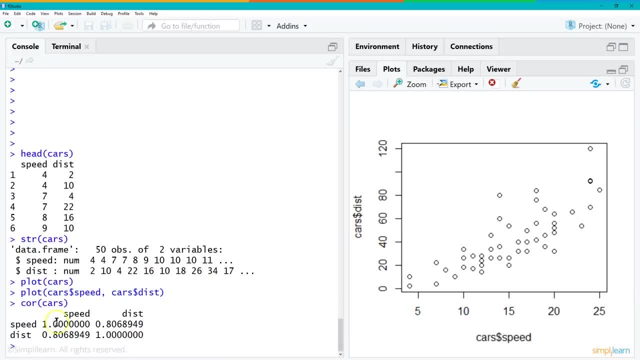 the short form, and we can see we have a nice correlation going on there between the two. What we really want to do, though, is we want to correlate cars, and then we're going to do the speed cars and the distance. 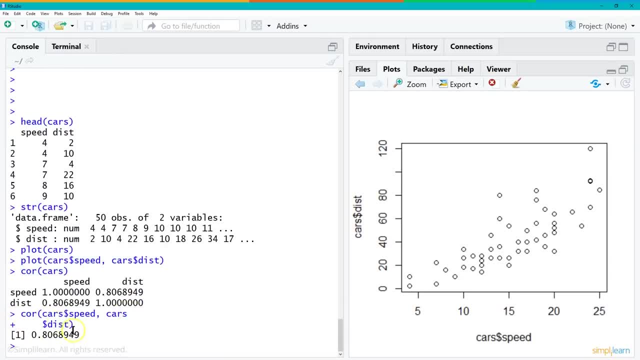 And so, when you look at this, I actually hit the enter key in the middle of that, which is fine. You can, in R, do it line by line. So if you're trying to do a bunch of different columns, you might want to do that to make it easier to read. 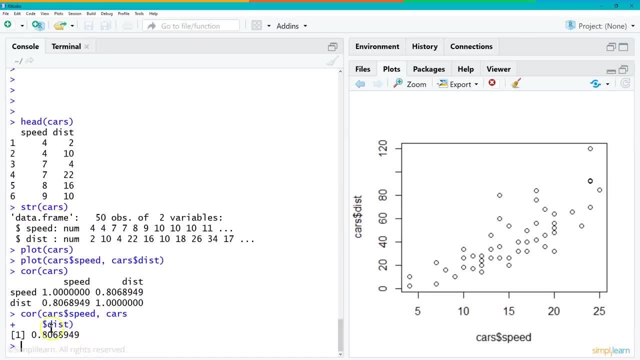 And you can see here I get the point 806894.. The closer this is to one, the more these correlate. So it's saying there's a pretty good correlation, a positive correlation, between the two variables. And if you look at it when I did just cars- 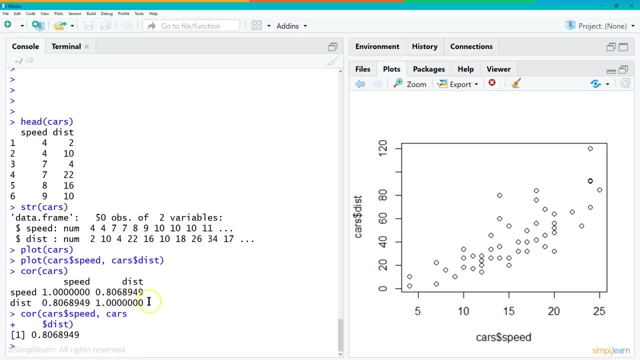 which did the correlation over all the variables, you'll see that speed correlates with speed 100%, because they're the same. That's just the nature of that. But when you look at speed versus distance we get the point 806849.. 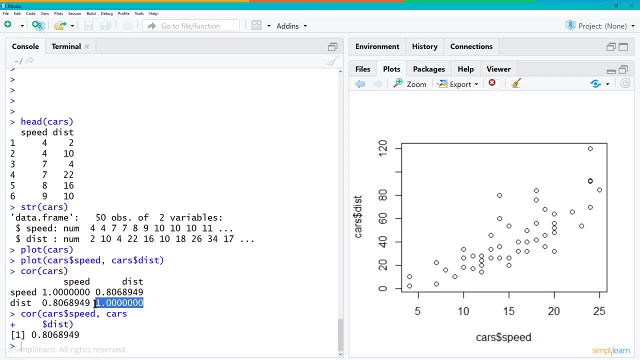 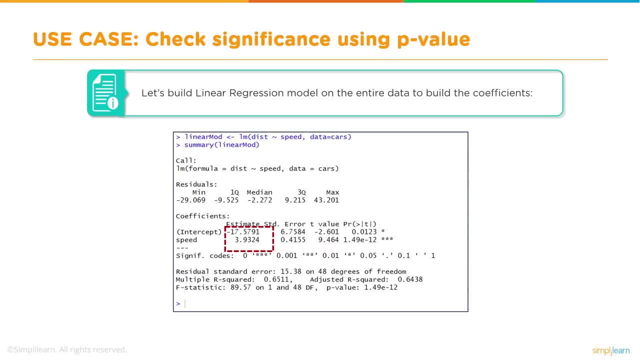 And if you do distance to distance, you get also one, since they're identical variables. So now it's time to build our linear regression model on the entire data set To build the coefficients. Let's just take a look and see what that looks like. 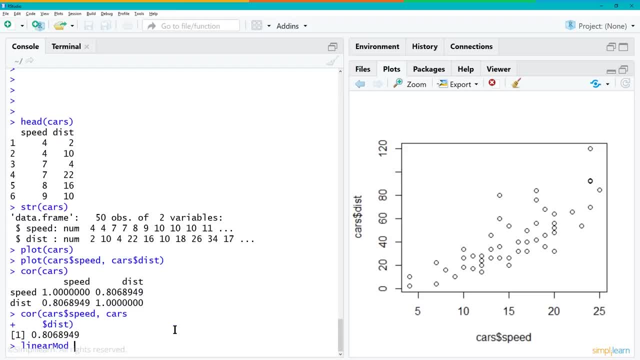 Back in our console. I'm going to type in linear mod And in R we want to do the arrow kind of like an arrow on a line, or, in this case, the less than minus sign. That's the same as assigning whatever we're going to put after it. 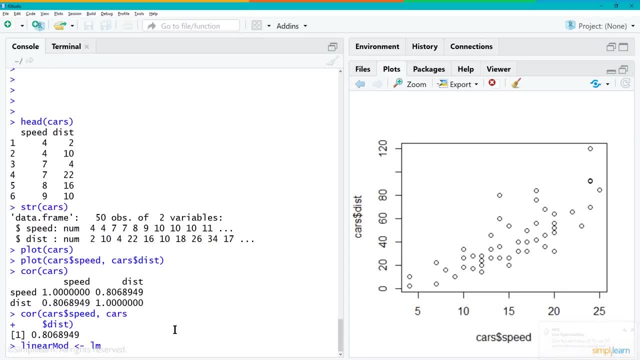 to this variable. So we're creating the linear variable. LM stands for linear module And we're going to look at speed and distance. So we put the little squiggly bracket between them. This lets R know we're going to deal with these two columns. 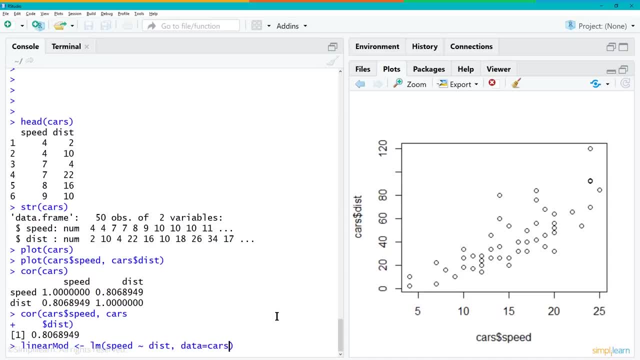 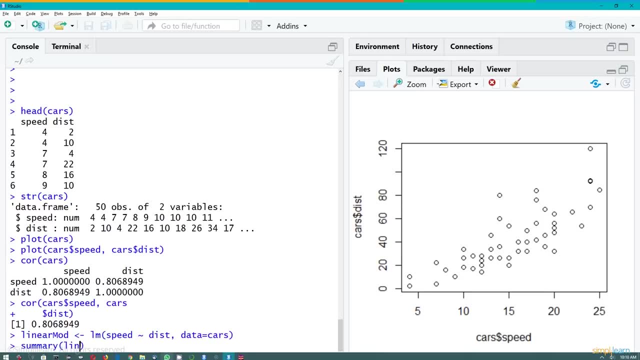 comma data equals cars. And when I hit enter on here, we've generated our linear mod. Now we want to go ahead and summarize it And we simply do a summary and then brackets linear mod and it generates all kinds of information on our model. 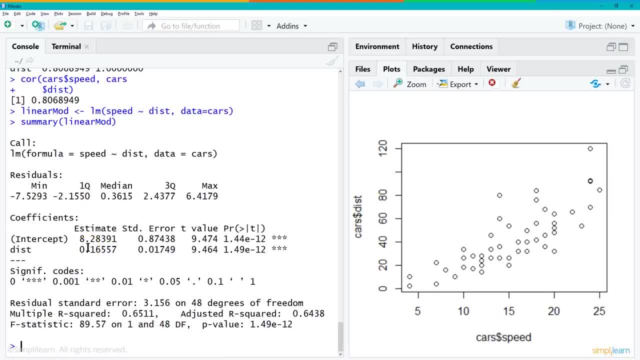 So we can explore just how well this model is fitting the data we have right now. Now, if you've done linear regression in other packages and scripts, you're going to see that this is so easy to explore data in R, So even somebody who's working in. 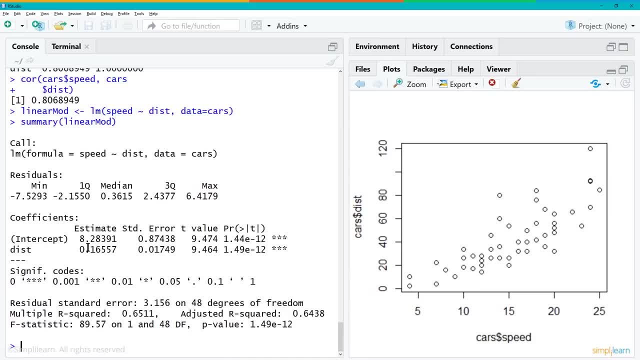 say Python or Spark Hadoop. coming back to the R console to do some basic exploration of the data is very beneficial And if you use just R, R goes into all kinds of different packages and you can even do cluster computations through H2OR. 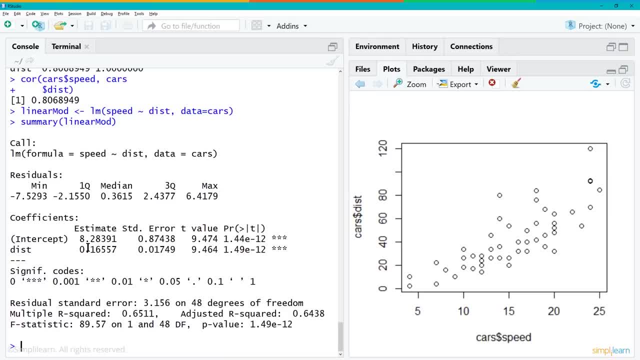 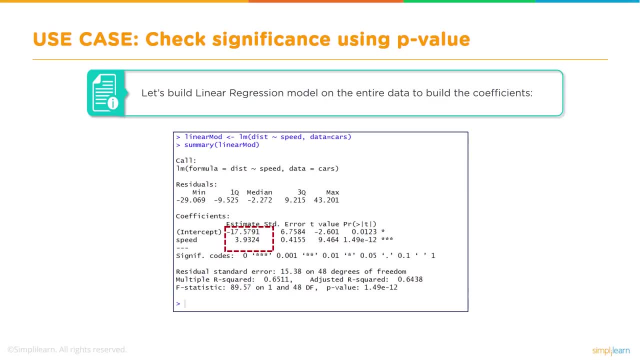 There's a lot of cool things. This is what makes R so wonderful is how easily we can summarize something like a linear model. And to explore this data, let's go back to the slide And we'll see here where it says the residuals. 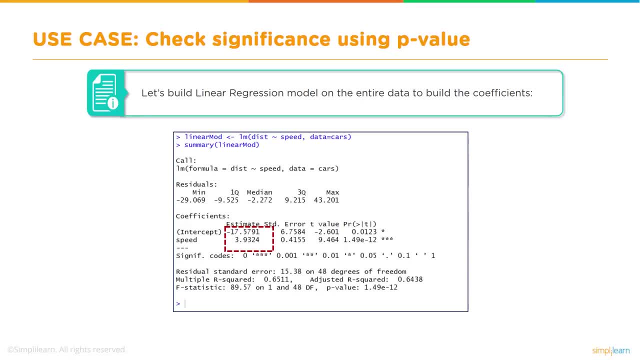 the first one, Q stands for first quadrant median, third quadrant max coefficients, And we first want to do is look at the estimate standard deviation on here And you'll see the intercept is at minus 17.5791 and speed 3.9324.. 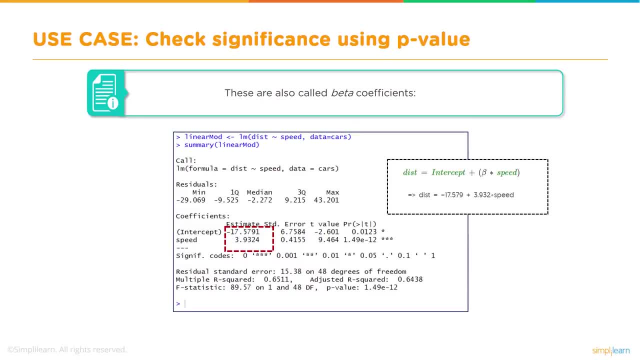 So we can compute: the distance equals to the intercept plus the beta times the speed, which just means that we can assign a distance equal to minus 17.579 plus the 3.932 times the speed. The value of P should be less than 0.05. 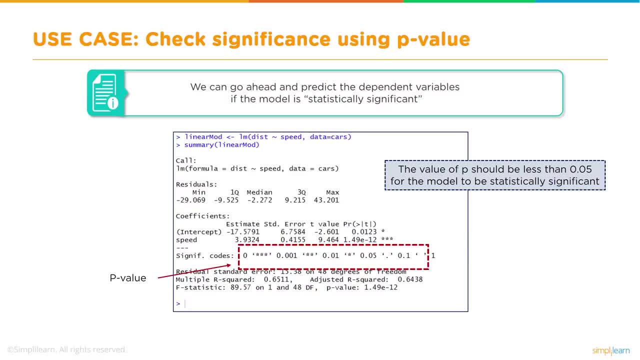 for the model to be statistically significant, And this is one of the things I love about R. You can see right down here we've punched in the numbers and it even tells you the significant codes. So if you're trying to guess or remember, 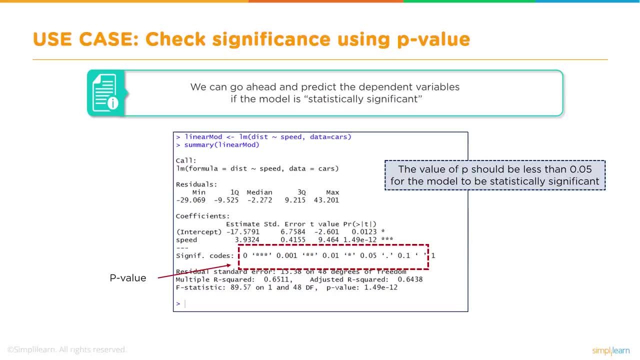 it tells you right away: hey, this 1.49 to the minus 12th is way below 0.001 on there, And it even puts three stars next to it. So you can see that that is a very high correlation. 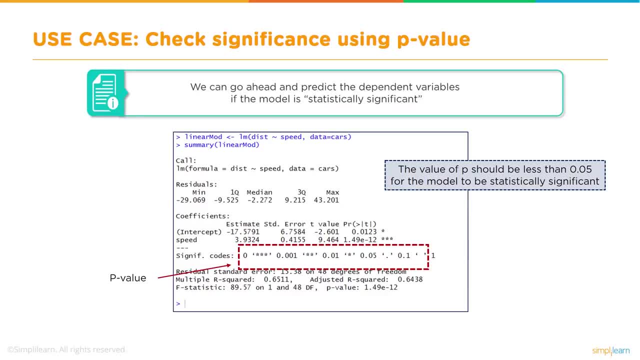 And you can see the 0.0123 gets one star because it is greater than the 0.05 or it's less than the 0.05.. So this shows that there's a very high correlation. Statistically it's very significant. 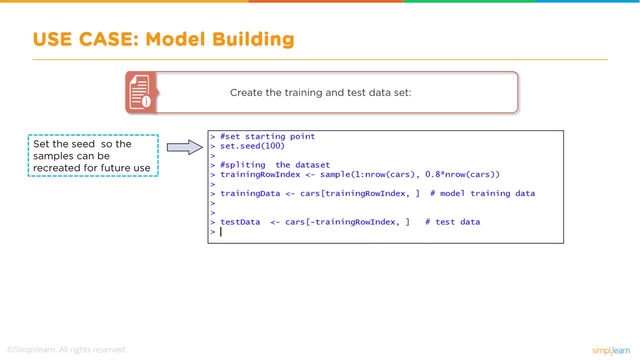 So now we're going to go ahead and create a training and a test data set, And the first thing we want to do is we want to set the seed so the sample can be recreated for future use. Remember, in all these different regression models, 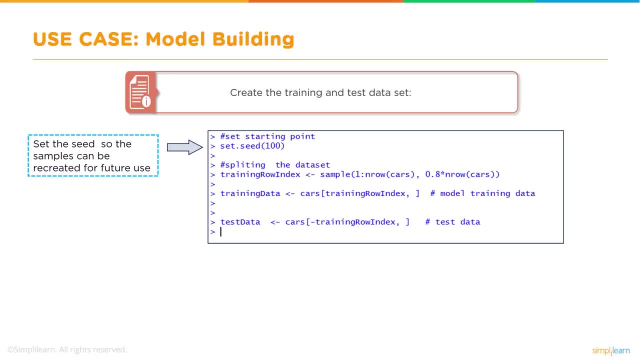 they usually have some randomization going on in the back to kind of fit it and guess where it's going to go. And if you want everything to match you want to start with the same seed in that randomizer. That way it recreates it identical. 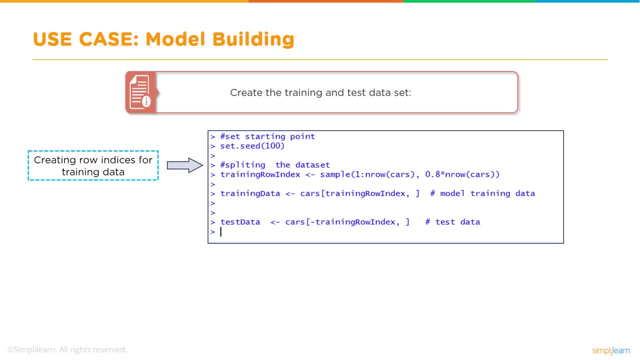 every time you run it on a different computer And just like working with data in any package, we're going to create indices for the training data and we're going to model the training data, and then we're also going to do the test data and build our model on the training data. 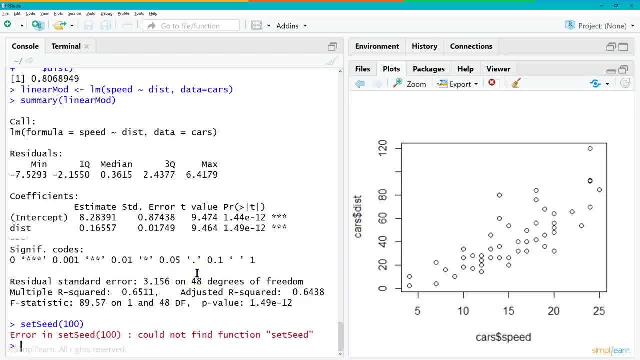 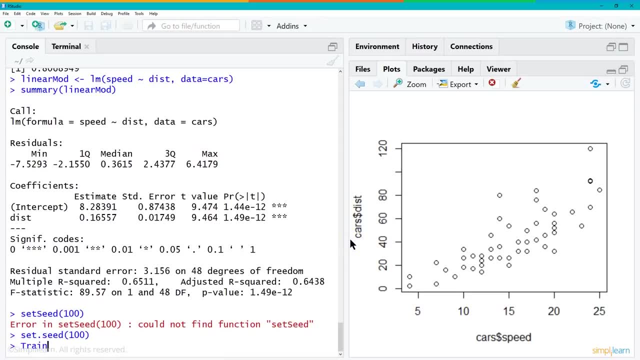 And let's walk through that and see what that looks like in R- And I actually mistyped that one- Let's type in setseed to set our seed for the 100.. Let's go, training row index and that's our name. we're making up for our variable. 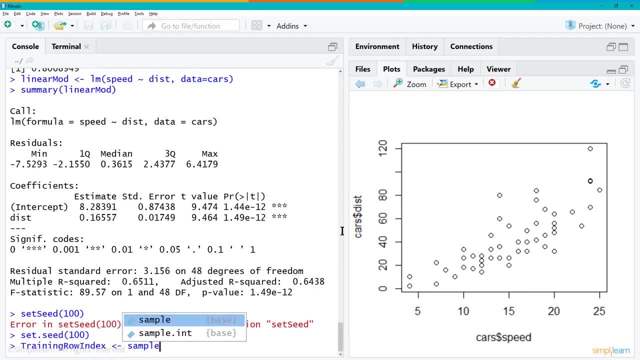 and we're going to set that to sample. Now, sample is a command in R, so we're going to take a random sample of some of the data And then we're going to do 1 colon in rows cars. So this is the number of rows in cars. 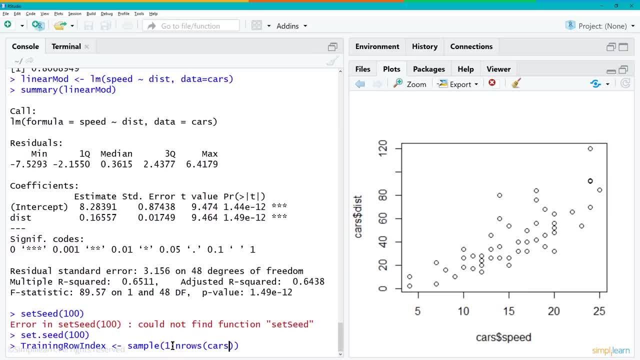 and we're going to start with 1 and sample them. So row 1 of the data, Skipping any of the titles on the top, And then in the sample it has two variables that go in. The first one is the in rows of cars. 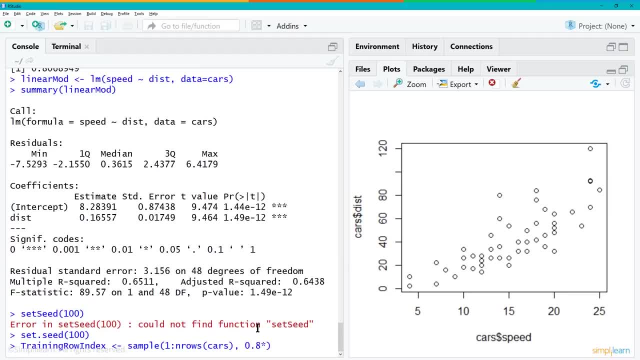 and then we want to do 0.8 times in rows of cars. This basically says that we're going to take 80% of all the rows in the cars sample. We'll hit enter to go ahead and run that. We see here that I had an error. 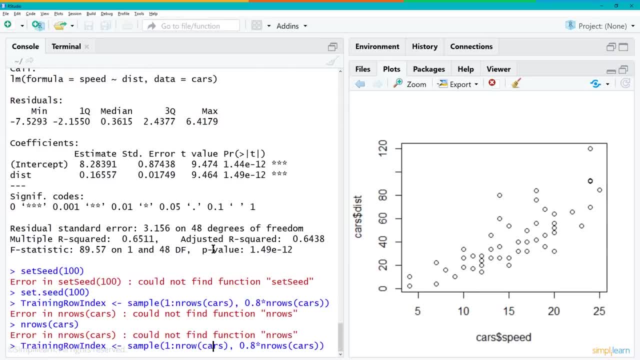 and that is because it's in row. Actually, put an S on there. That's something I do a lot on. We'll just fix that real quick. Brings up a point that if you use your up down arrow, you can quickly paste through the last things you typed in. 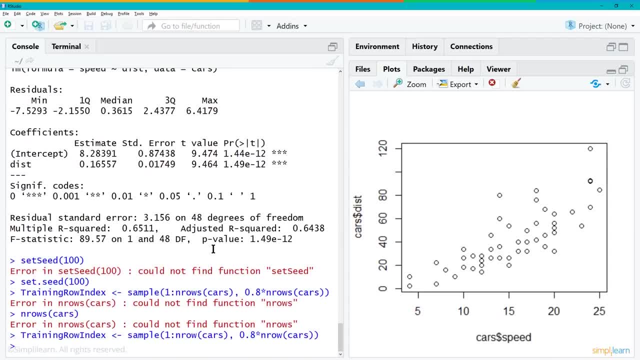 and then you can reuse them. So there we go. Now I have our training row index, which is basically a list of all the rows we're going to use, And now that we have a training row index, we'll go ahead and create our training data variable. 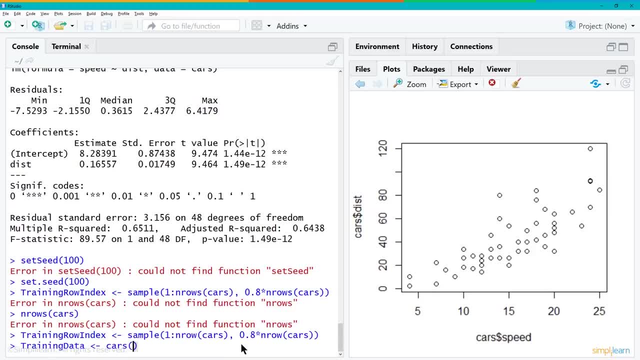 And we'll assign that cars and we'll put that as training row index And this is supposed to be brackets because we're dealing with an array type format. We want to do the training row index comma because we just need the index of the row. 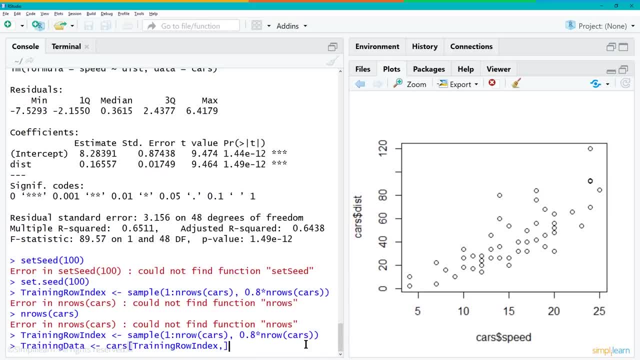 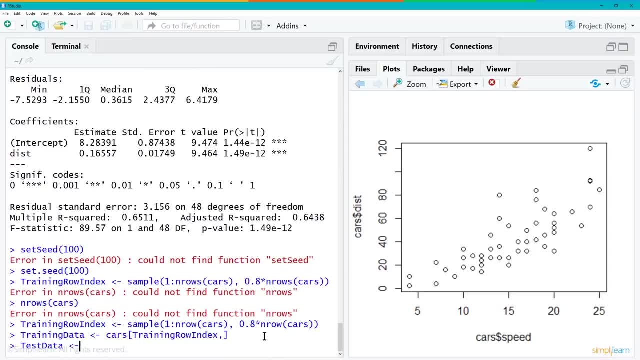 and as far as the columns, we want all the columns. So here we have our training data And now we set up a training data. we also need our test data And with our test data we'll assign that also to cars And because we used the training row index. 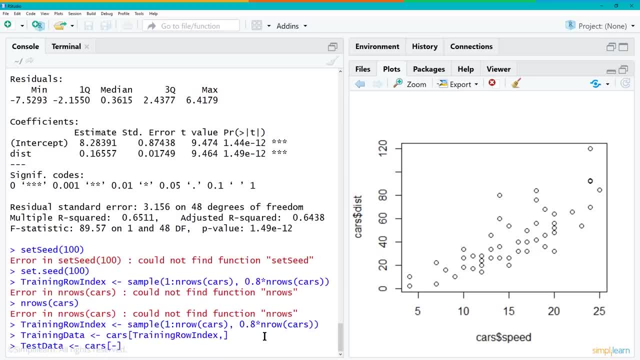 and we used the sample to create it. we can simply do a minus sign, training index comma, So it's identical to the training data, but the test data is going to be the ones the rows that were not included in the random sample of 80%. 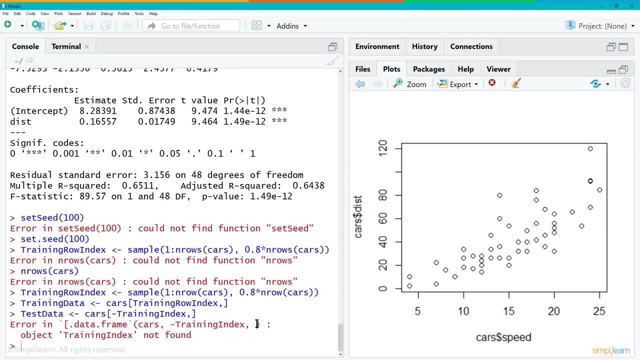 So it's going to be 20% of the data And of course it's very easy to do mistakes on here, so we'll come back into this, bring back up the error and then we have training into training index. training row index. There we go. 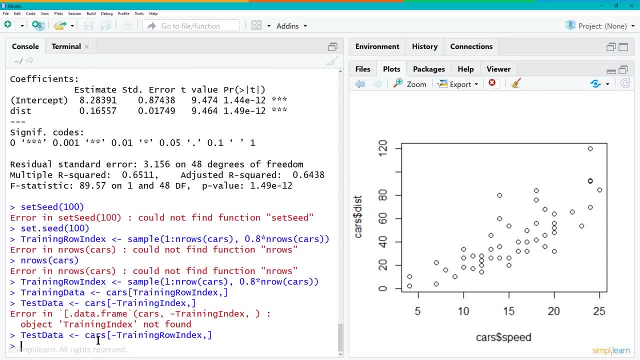 Very easy to correct errors in R. So now we have our training data and our test data. So we have 80% in training data and 20% in test data, And let's go ahead and create our model. We'll call it lmmod. 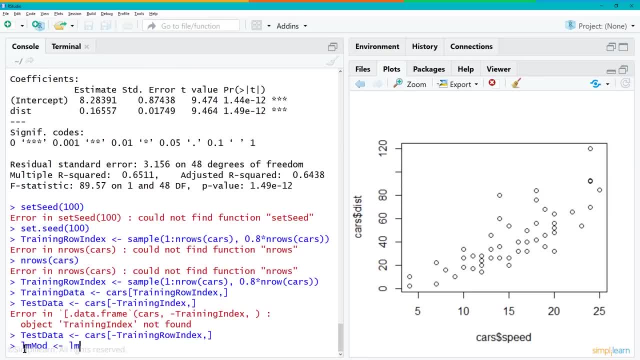 and this is identical to what we did earlier. Here's our linear model. We're going to have our two different columns. If you remember above, we had to tell it which columns we wanted. I'm going to do distance and speed, and then the data. 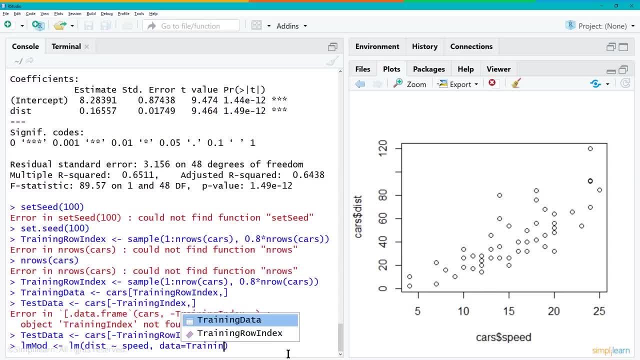 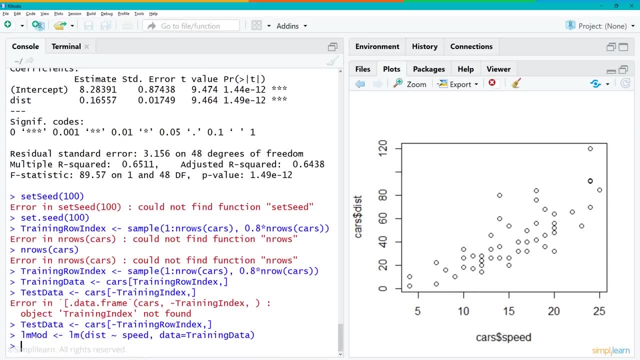 We're going to set equal to training data. So, as opposed to doing all of cars, we want to use just the training data on here, And now that we've created a model off of the training data, we need to go ahead and run our prediction. 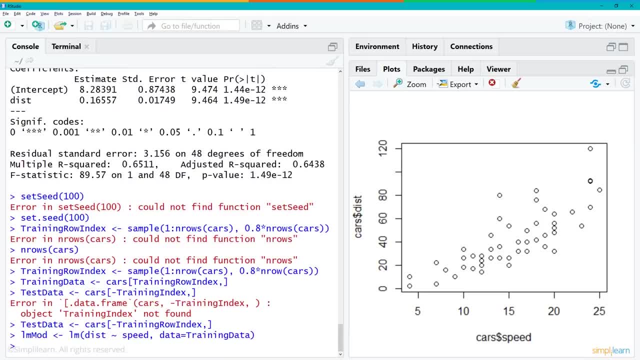 off of our test data. So we're going to see how the test data- which has nothing to do with the model so far, how well it fits, And we'll go ahead and call it distance predict. There's our assignment, So we're going to assign the value to it. 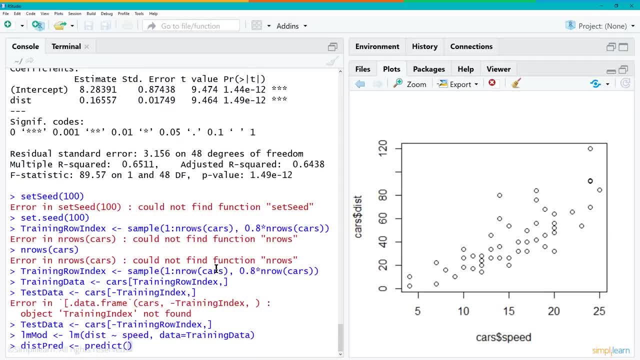 And with R we type in predict, and then we called our model. We go ahead and pull up our model, lmmod, and so we're going to use that model and then we want to put in the test data. Here's our test data. And so now we're creating the distance predict variable. 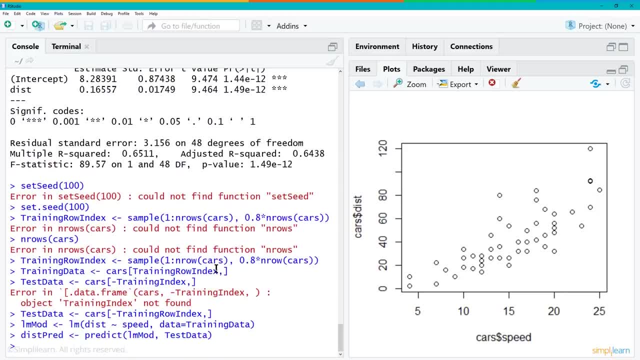 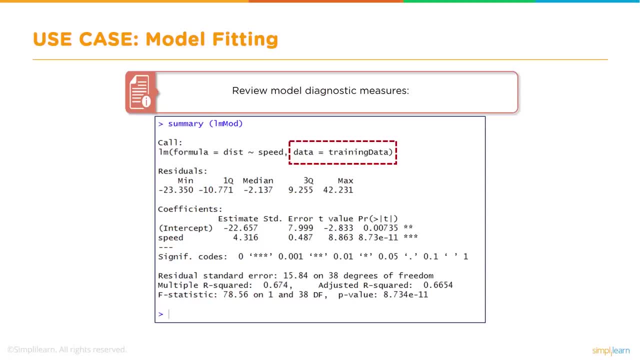 and we're going to put all the information we're predicting on our test data And we'll run that. Just hit the enter key And then, if you remember from before, we want to review the model diagnostic measures And so we're going to go in here and do a summary. 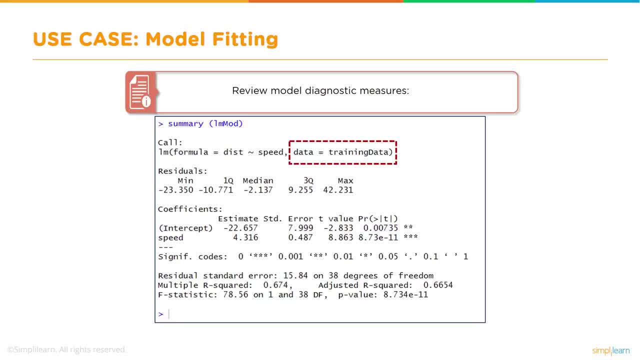 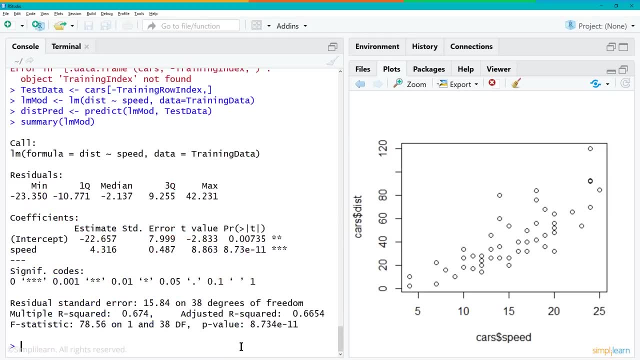 And you'll see in here we have a couple different things going on, But let's go ahead and take a summary of this and just walk through what this means. So summary, and then we call that lmmod and we hit enter and it pulls it up. 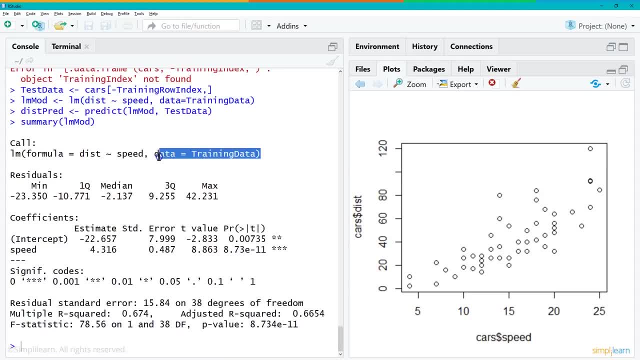 And we have a nice summary of our lmmod, And the first thing we're going to note is that the data that's right now in our lmmod that we're summarizing is our training data, And let's go back to the slide and highlight this. 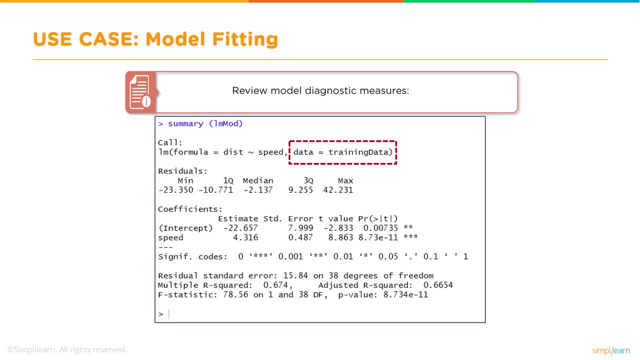 So the data equals the training data. That's where the lmmod comes in. Residuals, we have our minimum, our first quarter, medium, third quarter, and the max, Or quadrant, not quarter. You'd think I was doing business analysis. 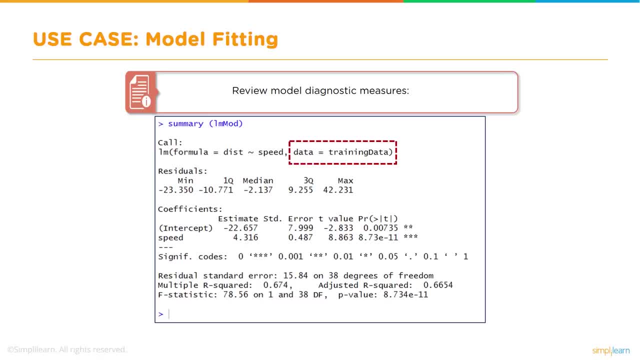 as opposed to end of the year taxes and first quarter versus quadrant. We look at our coefficient, We can see where our intercept is and our speed is, And we note over here our significance codes. So they all match up. So a simple correlation between the actuals. 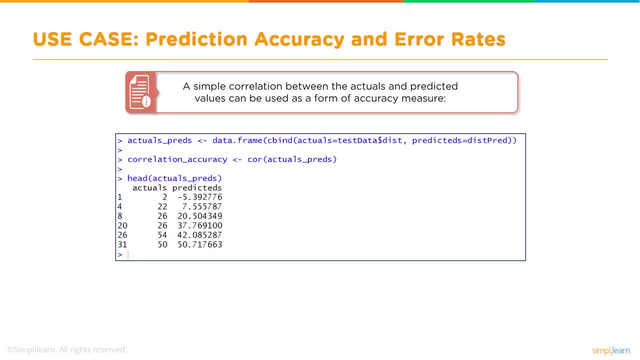 and the predicted values can be used as a form of accuracy measurement. So we took a look at the model we created and now we need to take our predictions and just see how accurate it is on the data that we didn't use to program the linear model. 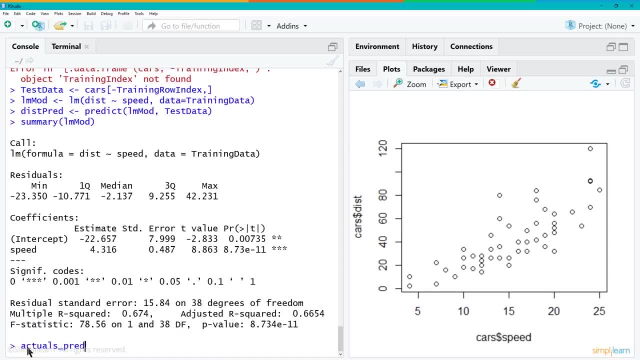 So let's create a variable called actuals- underscore- predicts- and assign it data frame. This is how we create a data frame: is we just assign data dot frame And we'll do a C bind And in our C bind we're going to take our data. 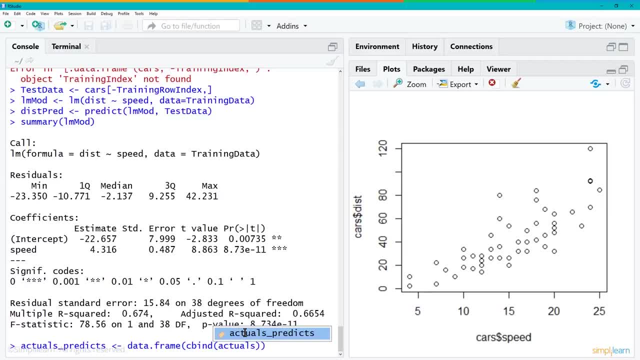 and we're going to create a column called actuals. So this is our choice: the name actuals. This is going to equal test data and we're going to use a dollar sign and distance, And we're running out of a little room there. 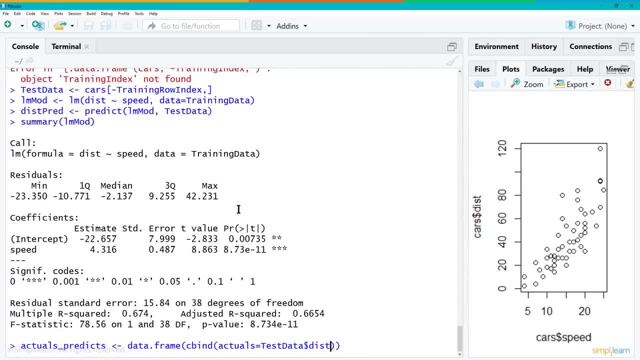 so let me pull this over so we can see it better. There we go, distance, And then we also want to take and compare that to what we predicted for our other data And we'll call this column predicteds And that's going to equal our distance predict. 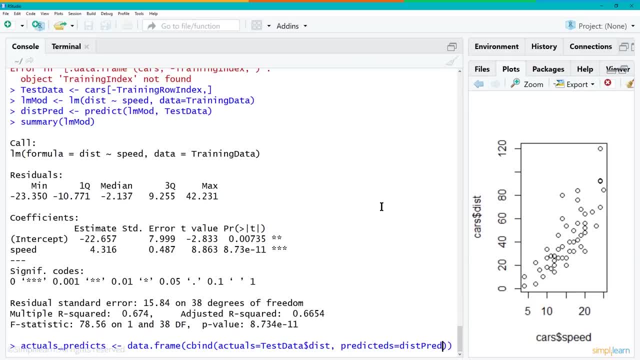 And remember, distance predict is set to the predicted values of our test data. So what this is is we're saying, hey, here's our test data, the actual data and the distance, and then we have what we predicted that distance to be. 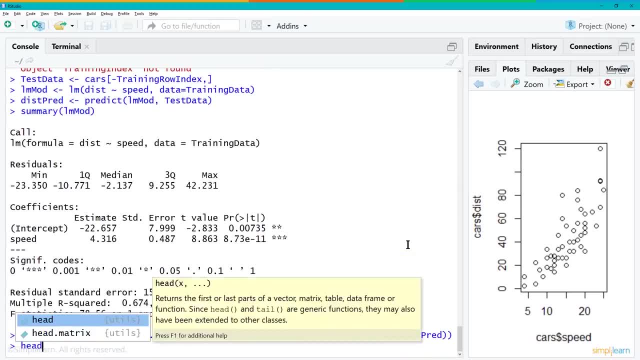 And we'll go ahead and assign that And we can do a quick head actuals predicts. there we go And remember: head shows us it's a data frame, So it's going to show us the labels and the first set of data. 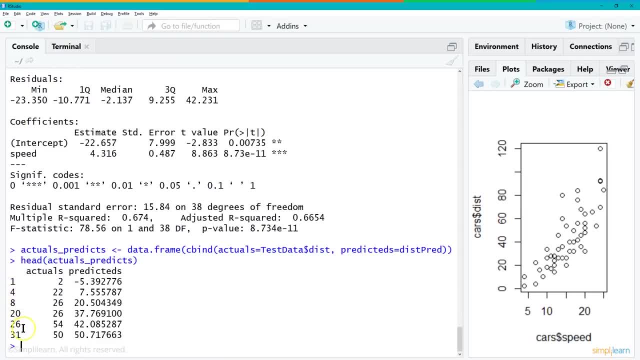 In this case, you'll notice that the rows are a different count. They're not 1, 2, 3, 4, 5, 6.. Well, we randomly picked 20% of the data, So this is the first 6 rows of that random selection. 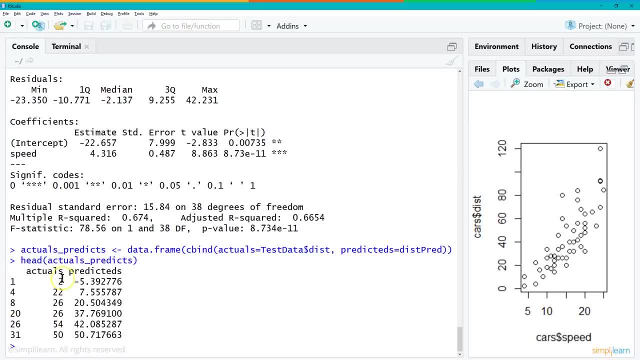 which comes out as 1,, 4,, 8,, 20,, 26,, 31.. And we have the actuals. so the actual value is 2.. And the predicted value on this first one is minus 5, so they're way off. 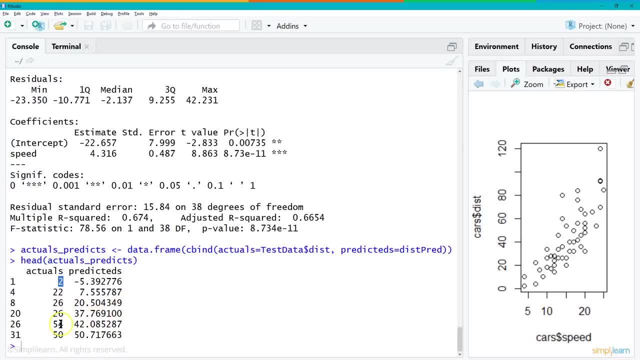 22,, 7,, 26,, 20,, 26,, 37,, 54 to 42,, 50 to 50.. So one of these is actually pretty right on where a lot of them are really off at the beginning. 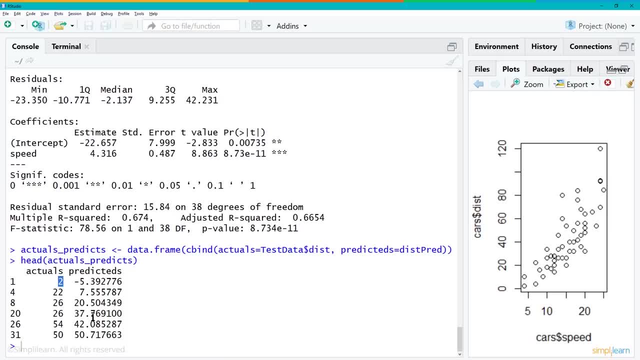 Let's just see what that looks like, though. Well, the first 6 rows does not tell us what's really going on, So let's create another variable, correlation accuracy, And we're going to assign this correlation cor. Remember, we do a cor. 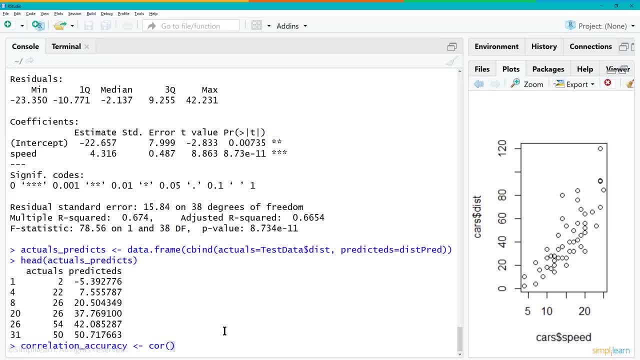 And we have our actual predictions. So let's just see how our actual values versus the prediction correlate with each other. And we assign that one actuals underscore predicts. There we go, Let it auto-finish for me, And we can just go ahead and type in. 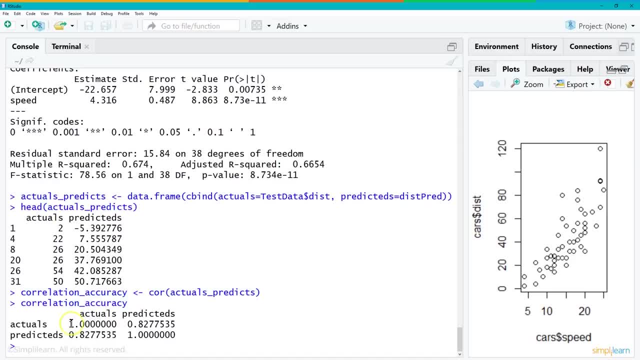 correlation accuracy and see what that looks like. So we have an actuals 1, a predicts 0.8.. And you can see how they kind of correlate. We have the 0.82.. And if you remember from before, we're looking for either 0.001, 0.01, 0.05, 0.1.. 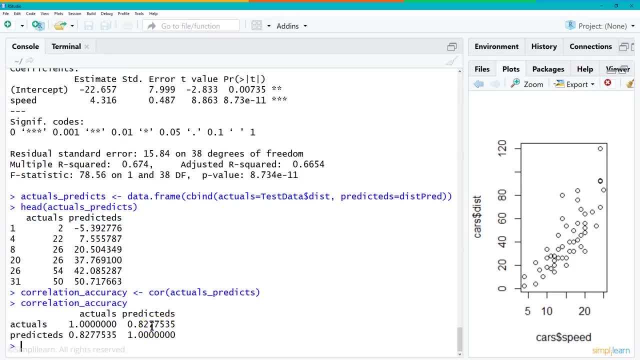 That is the p-value, which we're not looking at here. This is not based on the p-value. This is based on what we looked at earlier with correlation, that the closer to 1,, the closer the values are, And so 0.82 gets upwards of 1,. 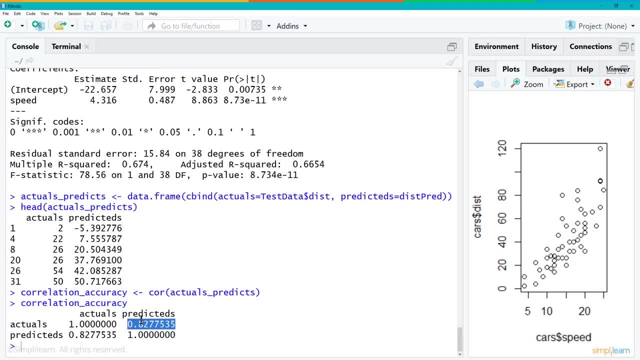 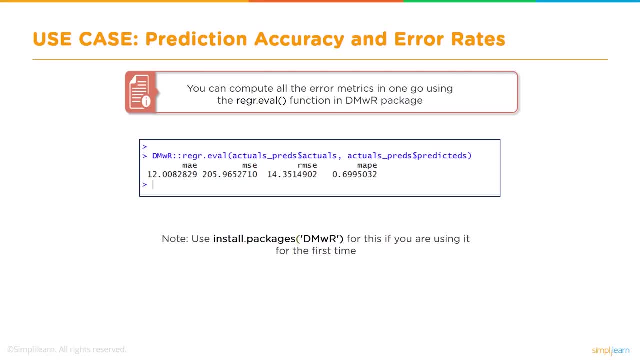 so you see that there's a normal, pretty much a correlation in here. But we want to dig a little deeper, because this doesn't really tell us how accurate it is. For that we're going to use another tool. For that we're going to calculate. 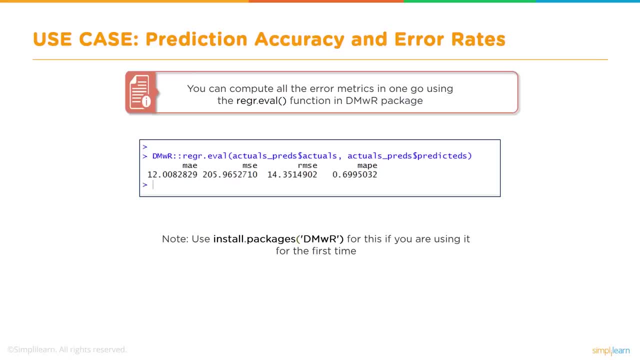 the min-max accuracy and MAPE. And the min-max accuracy equals the mean value of the minimal actuals and predicts over the max value of the actuals and predicts, And then the mean absolute percentage error, or MAPE as it's called. 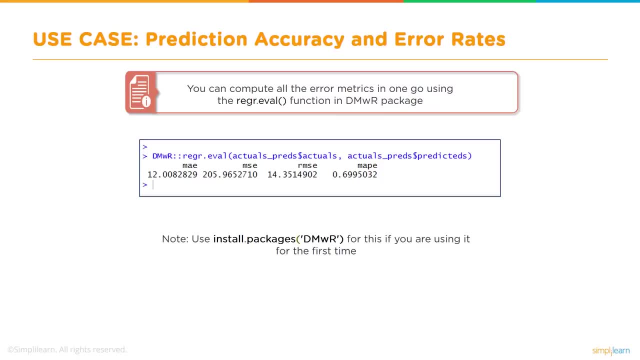 equals the mean of the absolutes minus actuals over the actuals. That's a lot to follow as far as remembering all these different math and theory behind it. Cool thing, though, is it's all done pretty much for you, So you can compute all the error matrices in one go. 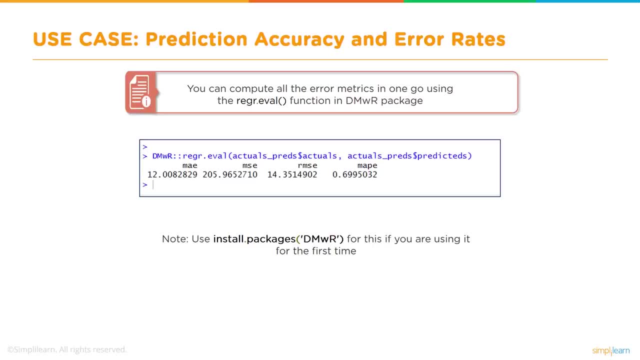 using the regress eval function in dmwrpackage. Since this is the first time I've used this install, I'm going to have to install the dmwrpackage, So we can actually install it two different ways. If you remember, we talked about installing. 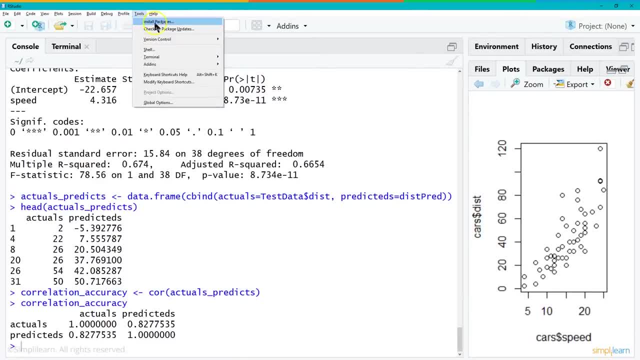 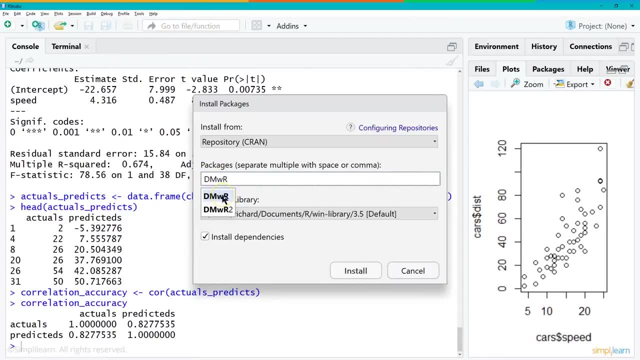 package earlier. We can go under tools and install packages And I certainly could type in dmwr. It even comes up and lets me know that's one of the main packages up there. Well, that's a tool of the RStudio setup. 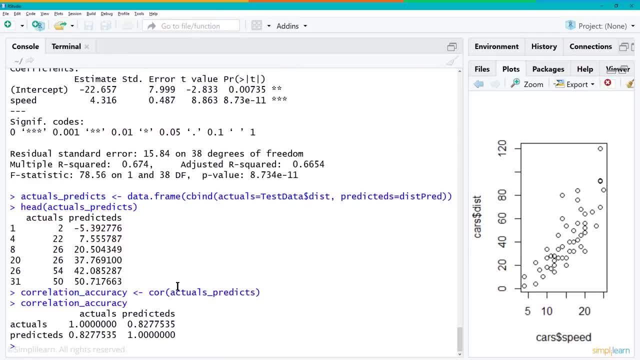 You can also install this using the console. We simply type in install. You can even see here it comes up install packages and then dmwr, And when I hit enter it should do the same thing as the other one does. It goes through and installs the dmwrpackage. 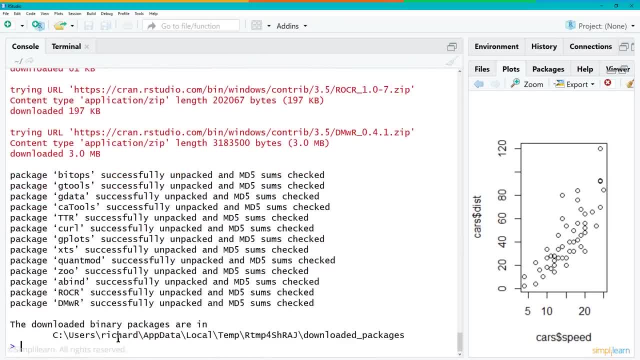 It takes just a moment to zip through all the different package setup And then the format for dmwr is dmwr. We're going to go colon, colon. We are specifically looking at the regressioneval And then we're going to do actuals. underscore predicts. 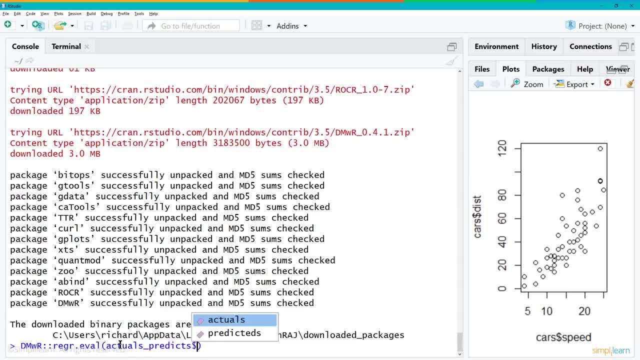 And we'll go ahead and put in the individual columns on this one. So we have actuals- I love the auto typing- And then again actuals, predicts. And this time we want to do it against the predicteds And we'll go ahead and hit enter on here. 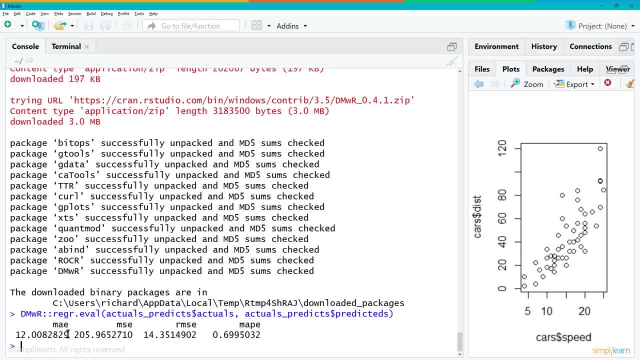 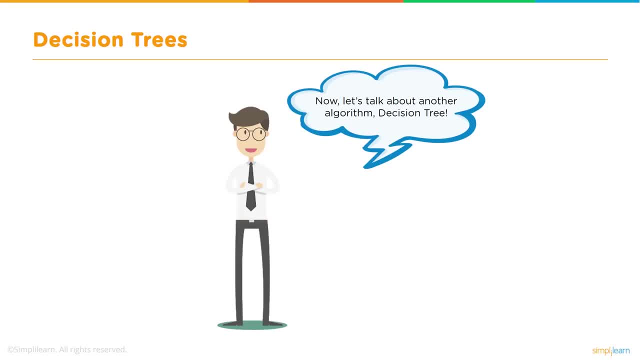 And you'll see in here, it comes up with our mae, mse, rmse and the mape values. So we looked at the linear regression model. Let's go ahead and take a look at the decision trees. So let's go ahead and talk about another algorithm. 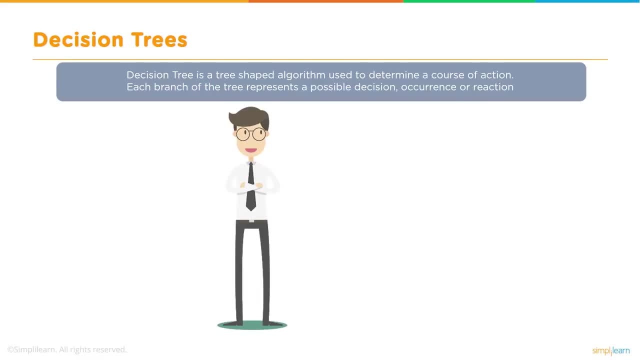 decision tree. Decision tree is a tree-shaped algorithm used to determine a course of action. Each branch of the tree represents a possible decision occurrence or reaction. It's a tree which helps us by assisting us in decision making. Let's look at the basic terminologies to 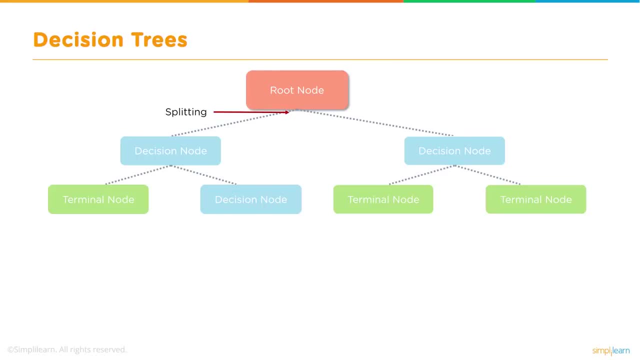 understand decision trees. We have our root node, We have a splitting, We have decision node, decision node and then those split into terminal node, decision node, terminal node, terminal node- And each decision node continues to split until it ends in a terminal node. 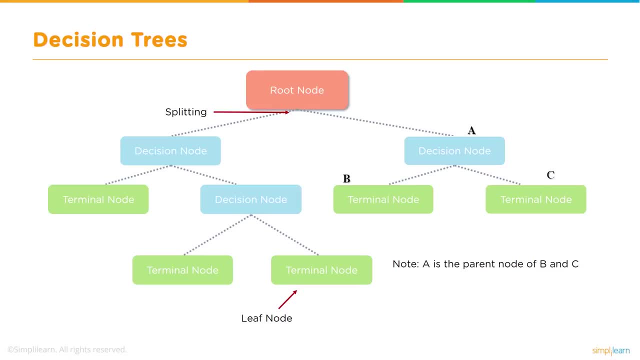 Note A is the parent node of B and C. Also note we call the terminal nodes leaf nodes. You can also see that we have a branch or a subtree. So when you have a split, everything under that split, under one side, is called a split. 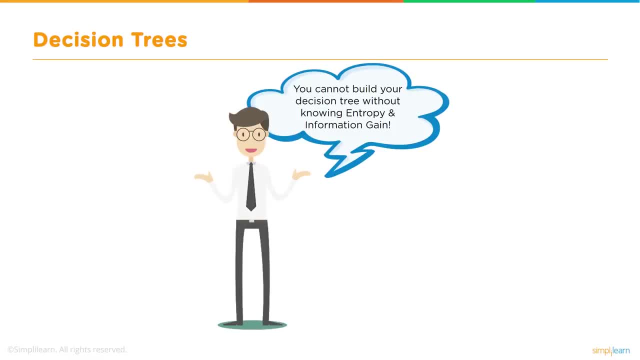 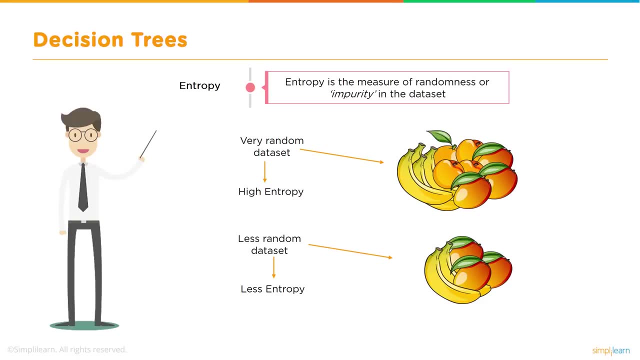 One side is called a subtree. You cannot build your decision tree without knowing entropy and information gain Entropy. Entropy is the measure of randomness, of impurity in the data set. So we have here a bunch of fruit and you can see we have. 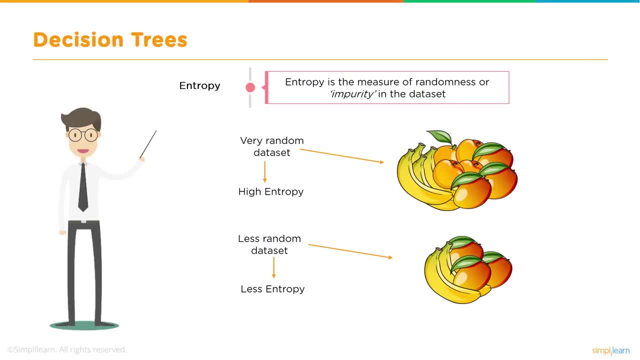 it looks like apples, oranges and bananas. It's very chaotic, So it's a very random data set. It has a very high entropy And if we take out one group- let's say we take out the apples- it's a little less random. 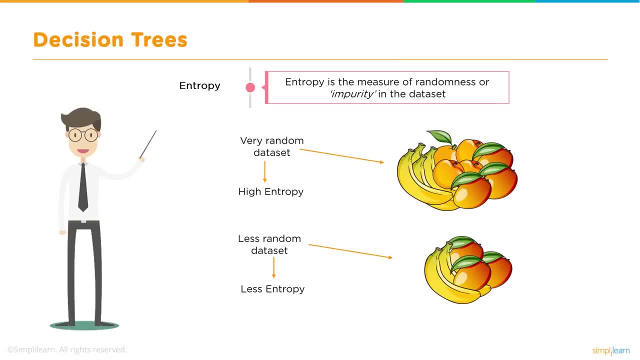 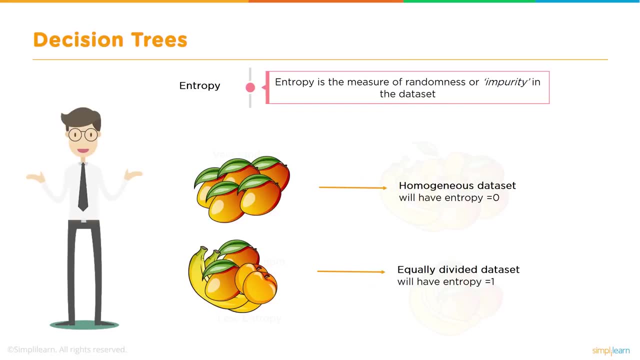 Now we only have bananas and oranges, So it's a less random data set and we have a lower amount of entropy. Entropy is the measure of randomness or impurity in the data set. So when you have a homogenous data set, we will have entropy equals zero. 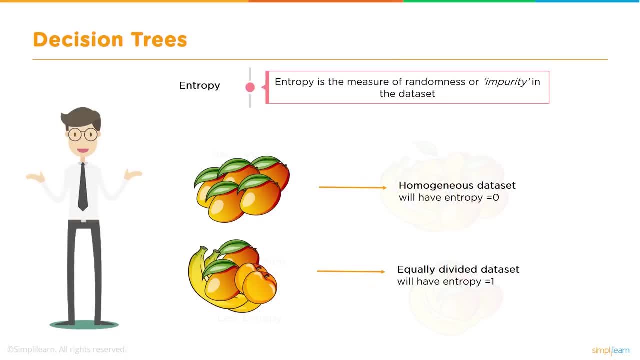 And here you can see it's all oranges. An equal divided data set will have an entropy equal to one. So here we have half, or what is it? It looks like a couple bananas, a couple oranges and a couple apples, So everything is equal. 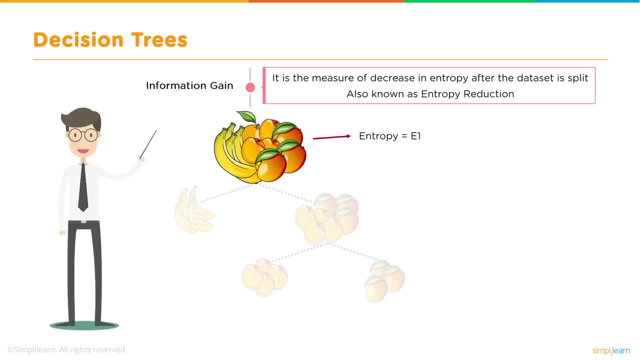 So we have an entropy of one on there, since there's two of everything: Information gain. It is a measure of decrease in entropy after the data set, Also known as entropy reduction. So we look over here and we have an entropy equals E1.. 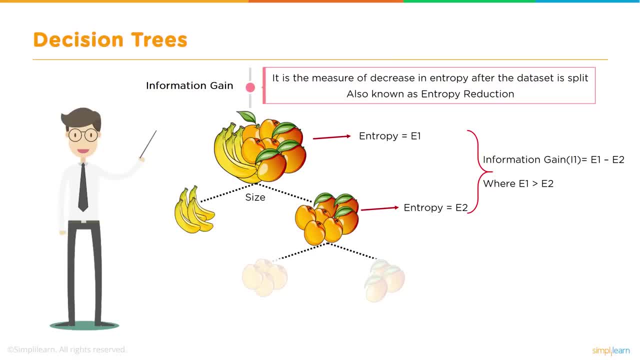 And the information gain. as we split the bananas out, the size becomes smaller and you'll see that E1 is going to be greater than E2.. Or we measure E2 of the apples and oranges. in this case, If you love your fruit, it's probably getting you hungry. 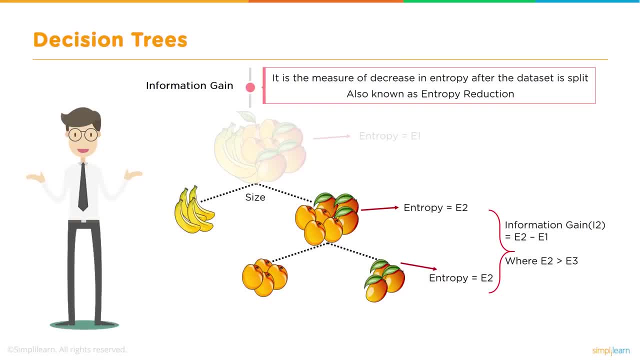 right about now, And then the information gain from our level two equals E2 minus E1, where E2 is greater than E3. And as we come down here, we'll see that the E3 is now the third level where we split the oranges and apples out. 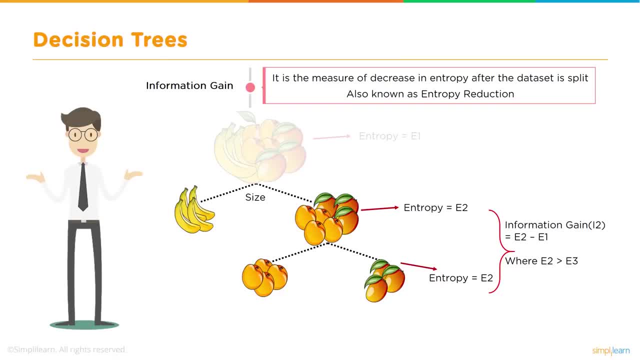 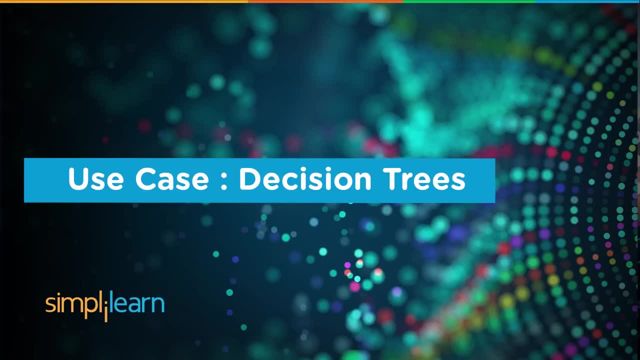 And each time that entropy becomes less and less and less until, in this case, we have an entropy of zero, since they're all homogenous in their order: All oranges, all apples, all bananas. So let's take a look at the use case decision tree. 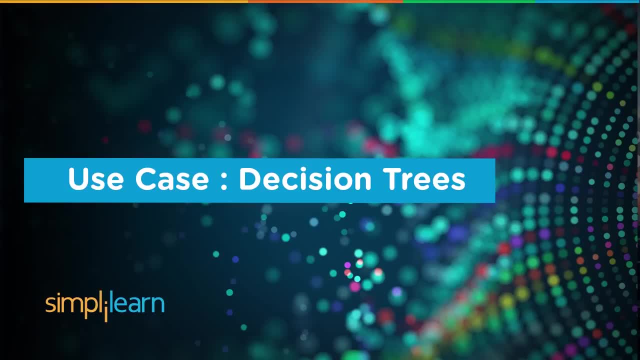 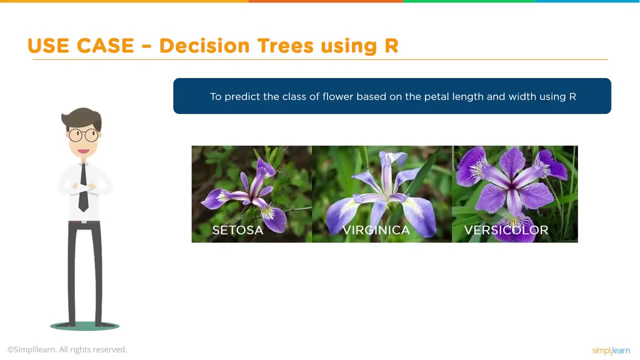 and actually put this into code and see what that looks like as we go from theory to script And to predict the class of flower based on the petal length and width, using R, And you'll see, here we have these beautiful irises, probably the most popular data set. 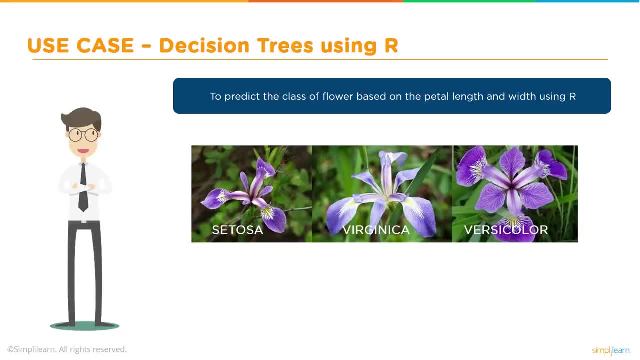 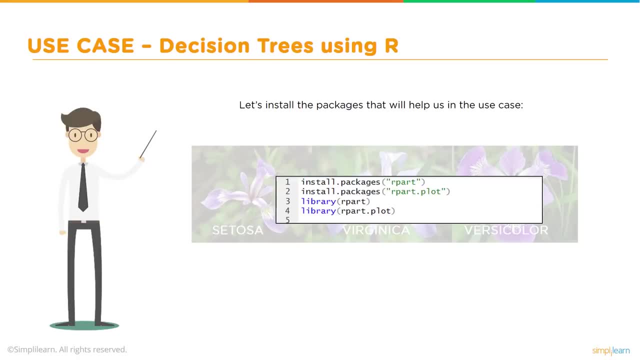 for beginning data analysis and statistics. We have the setosa, the virginica and the versicolor. Let's install the packages that will help us in the use case. So, because we're doing decision tree, we have rpart, rpartplot. 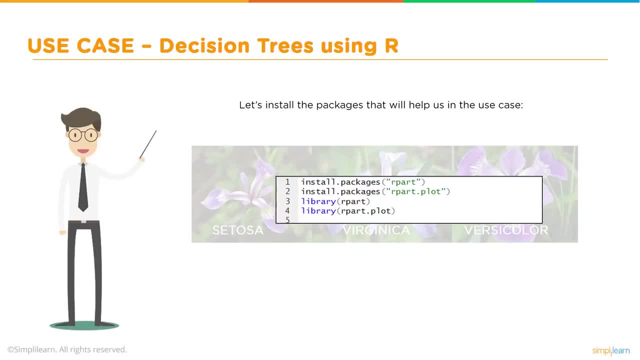 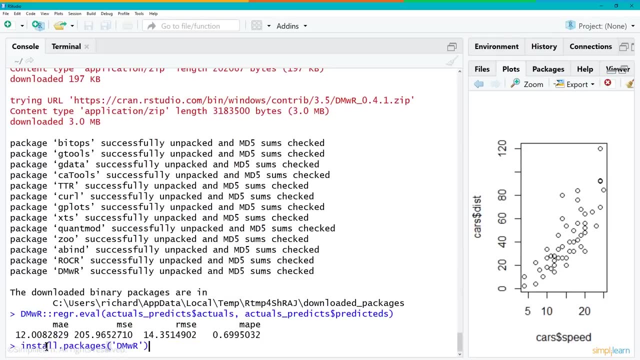 and then we have the library rpart and the library rpartplot. Let's go ahead and take a look at that. If you remember, we have two ways of installing it. We can do the install packages. We did that earlier. Here we go. 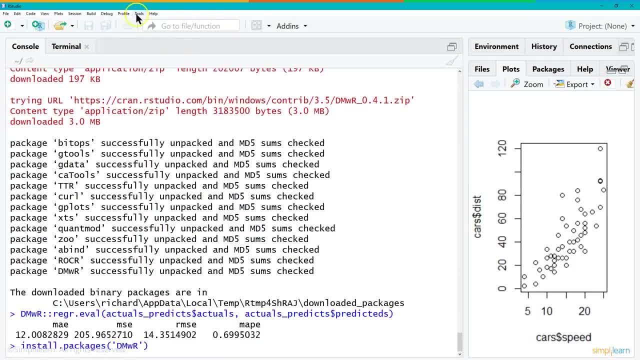 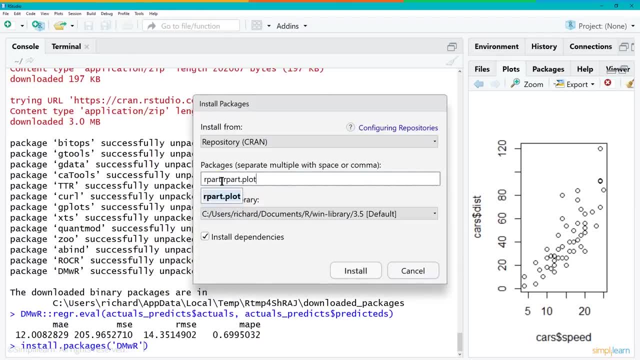 Install packages using my up error to get to it. Or we can go up to tools install packages and I can do rpart and rpartplot and then go ahead and hit the install. It will be updated as they are currently loaded. Oh, it looks like some of them are already loaded. 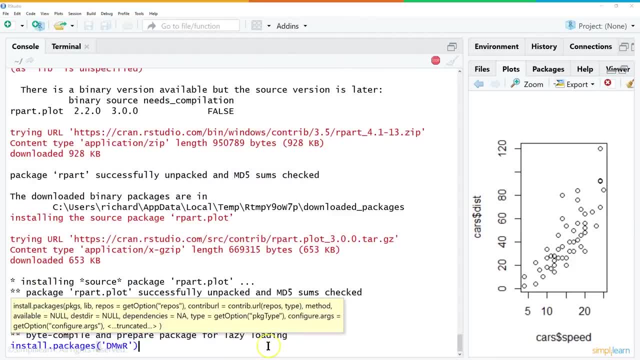 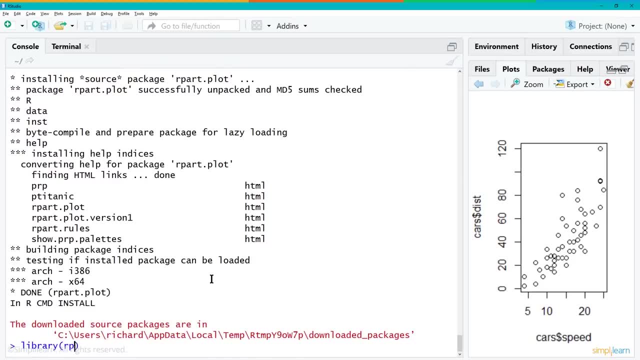 That's fine, We'll just go ahead and update those And once we have those updated, let's take a look and see what we have going on here. Oops, still loading. Let's go ahead and type in library rpart and library rpartplot. 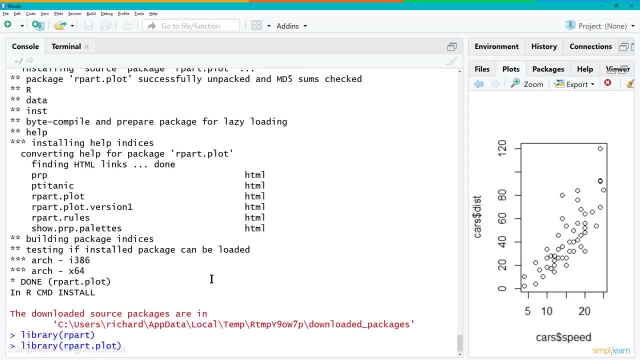 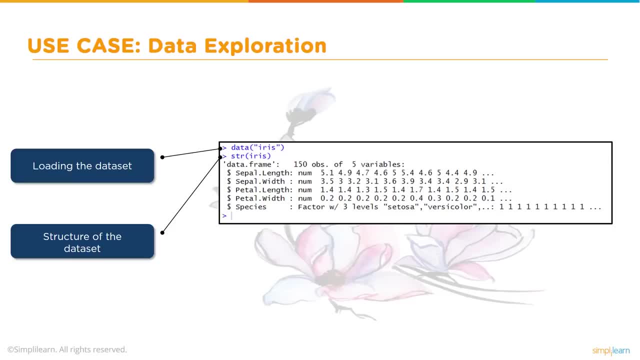 So we want to bring it into our console that we're working in. So up until now we just downloaded the packages and now we want those libraries available to what we're doing. So the iris, although it's built into the rpackage download on the basic download. 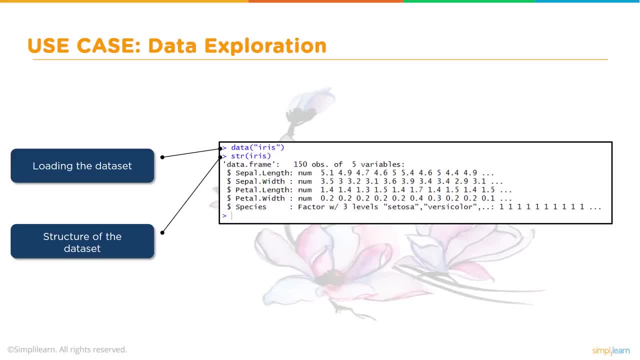 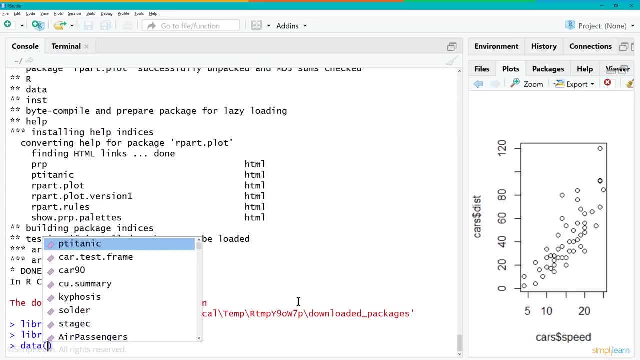 we actually have to install the data or bring the data in. So we're going to do the data iris, and then we're going to do the string iris And let's just flip back on over to our RStudio and set up our data iris. 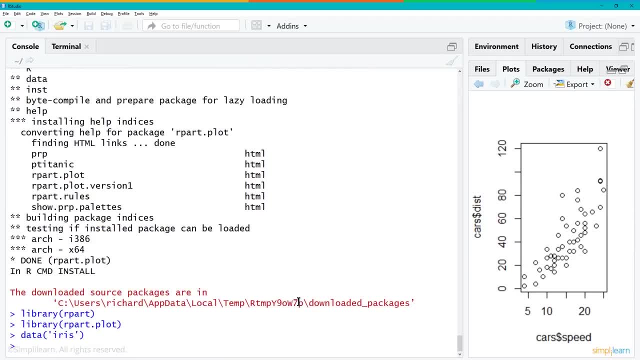 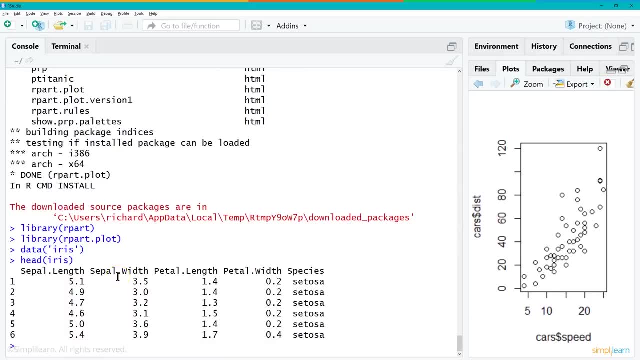 and then we're going to do string. Before we do that, let's do head, Head iris. There we go And you can see the head has sepal length, sepal widths, petal length, petal width, species. In this case, the top part is all setosa. 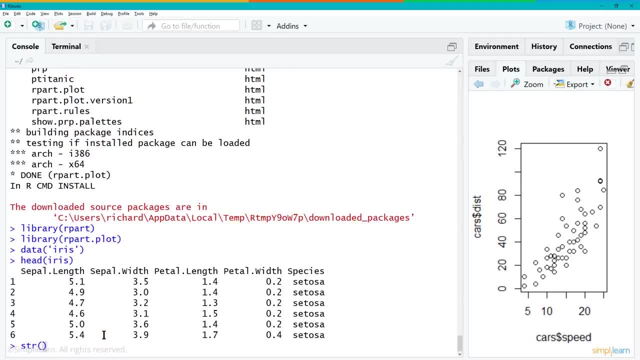 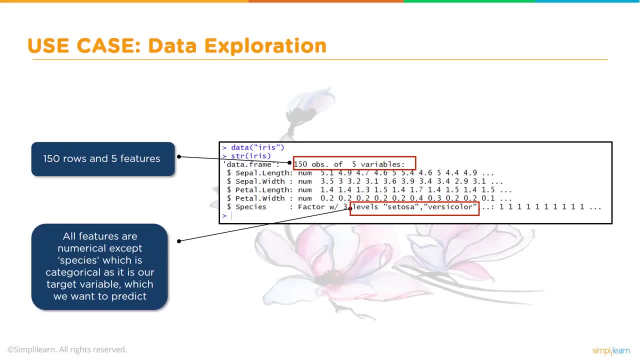 and each row gets a number. And then we did the string iris and that comes up with information. and if we flip back to our slide, you can see here the structure of the database. under string is: it's a data frame. It has 150 objects, 5 variables each. 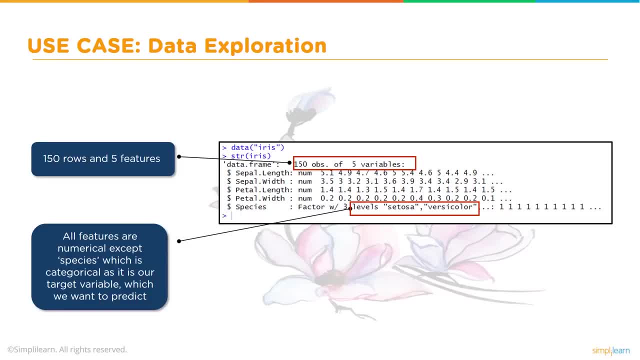 So each one has 5 variables. All features are numerical, except species, which is categorical as it is our target variable which we want to predict. So we want to predict whether it's going to be a varicosa versicolor setosa. 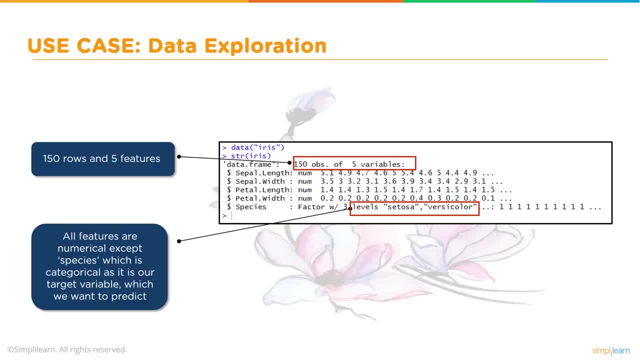 So you can see, here we want to predict all the features are numerical, except species, which is categorical. It is our target variable which we want to predict And you can remember that's a setosa, the versicolor, the virginica, the three different categories. 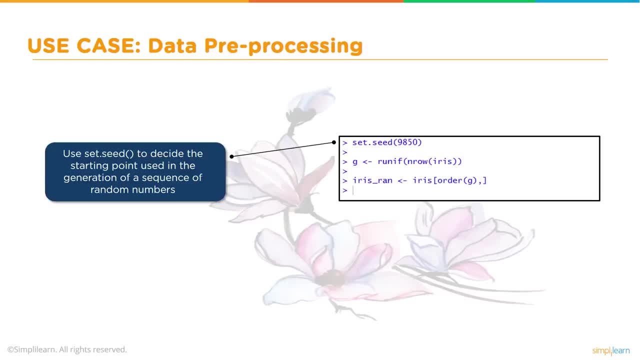 we saw earlier in the beautiful pictures of the flower. And so we're going to go ahead and use the set seed to decide the starting point used in the generation of sequence of random numbers. Remember, we set the seed so that if we ever want to, 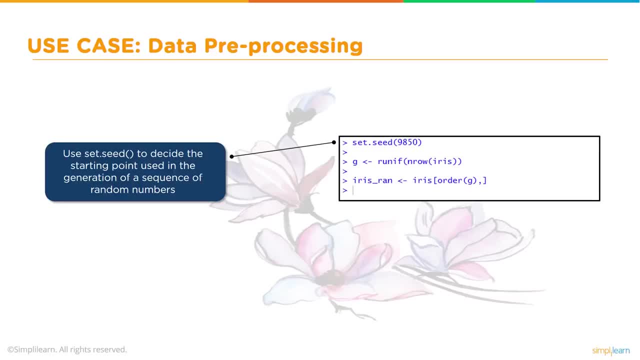 reproduce what we're doing. it will reproduce the same thing each time because it's using the same randomizer seed. It brings slightly different results depending on what you need it for. And then we're going to generate random numbers using runif. And the question is: why do we want to? 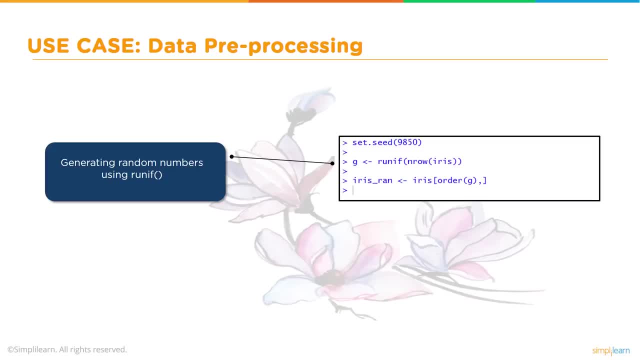 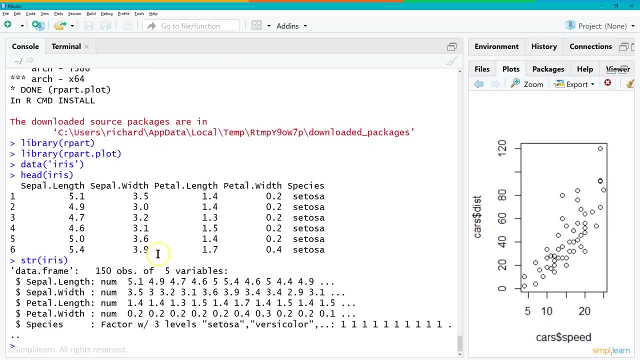 create random numbers on here. It's kind of an unusual thing to do for N-rose iris And let's go back and just take a quick look here. Actually, we want to go back to our R studio And you're going to notice, when I did the head of iris, 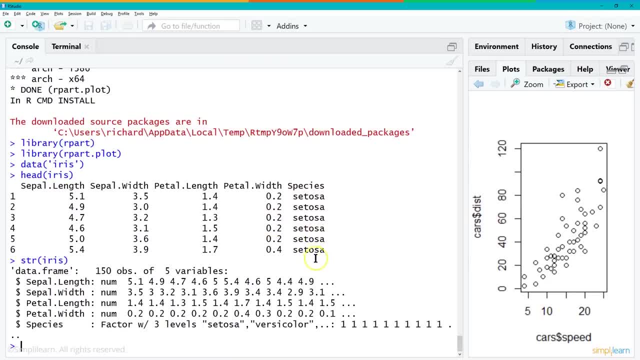 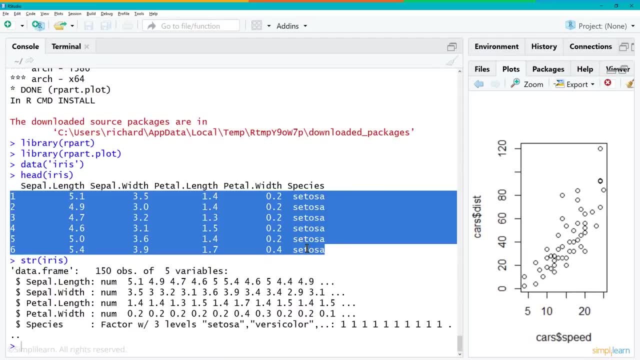 what did I have? I had setosa setosa, setosa, setosa, setosa. So the data is organized by species and it's already grouped them together in the data set. Well, we want to randomize that, so that doesn't affect our output. 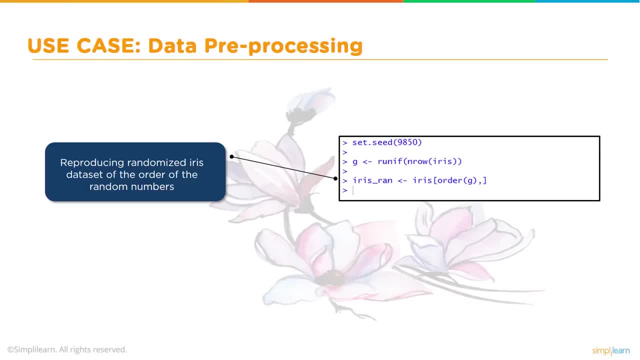 And then we'll go ahead and take and create our iris ran, where we recreate the data frame based on a random order instead of setosa all being grouped together. Let's go ahead and put that into our R studio and setseed and we'll match their number. 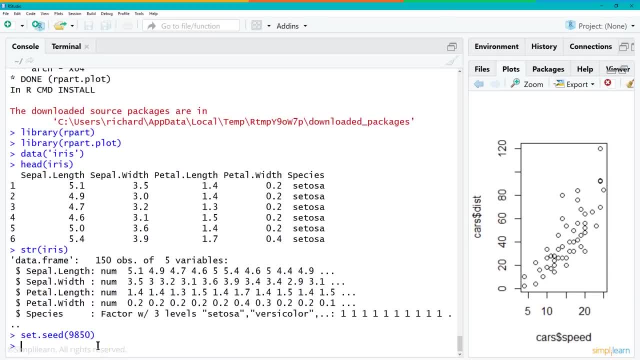 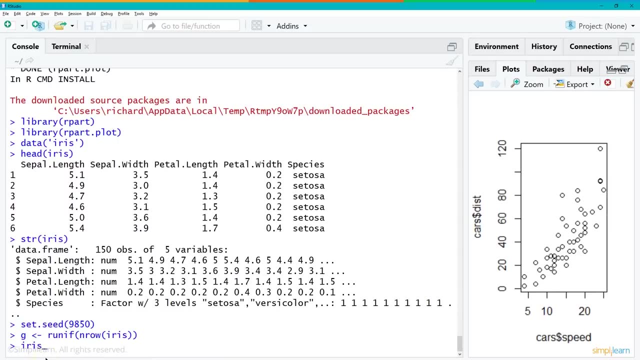 it's 9850. this way we'll have identical results to what they're doing on the slides. Then we're going to set the variable g equal to runif and base this on N-row of iris. and finally we're going to create iris underscore ran. 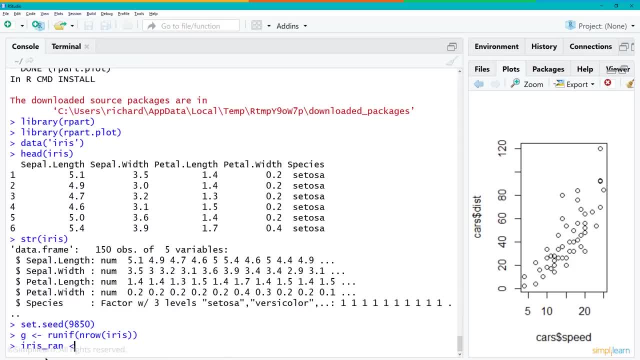 and we're going to assign our variable. we're creating iris underscore ran and we'll set that equal to. we're going to do that to the original database. we're going to set that equal to iris and we need brackets because we're assigning the variables and we want to change the order. 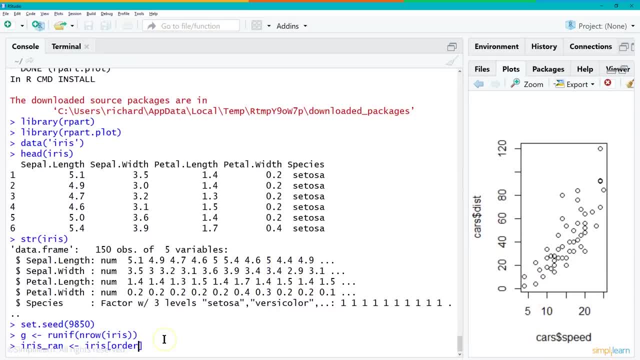 so there's an actual command order we can do, and it's going to be order g, so this means all the rows in the order that g is. so we just randomized all those rows and then we want to keep all the columns, so we'll just put a comma. 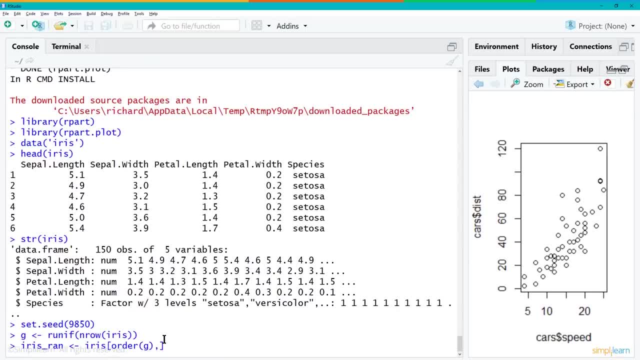 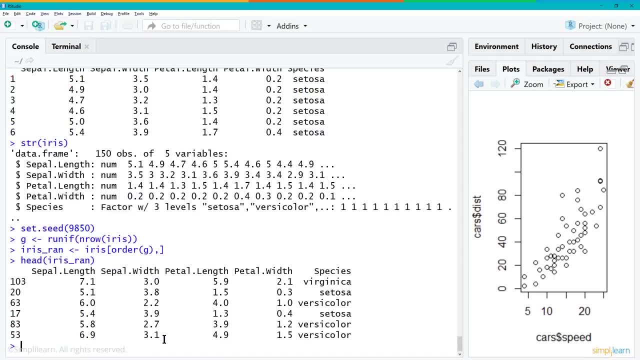 and we'll leave it blank for the columns. So now iris ran will have some randomized rows coming in and if we do head, let's just do this real quick. iris ran, we can see that it's no longer setosa setosa. we now have virginica setosa. 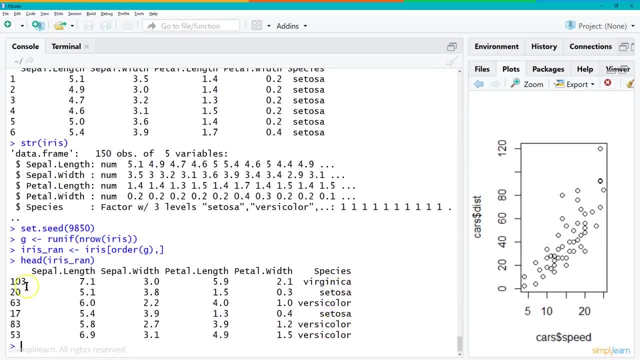 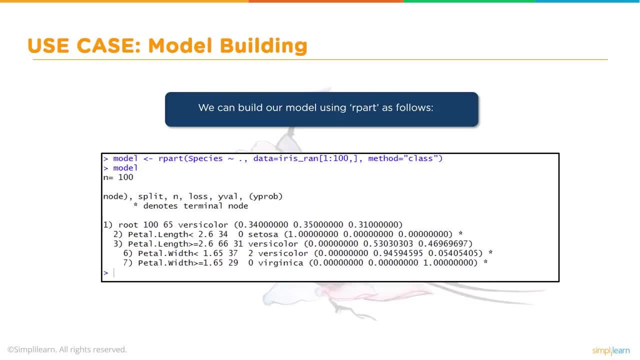 versicolor setosa and you can see the row numbers at the beginning. we have 103,, 20,, 63,, 17, so they're randomized on there pretty well. Now that we've done a little data manipulation, we can go ahead and build our model. 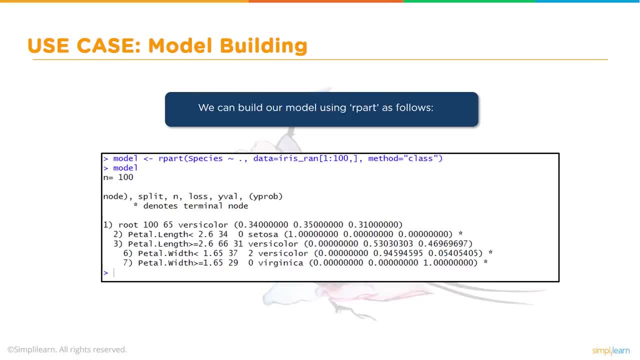 using our part as follows, and one of the things I want you to notice here is we're going to build our model for our r part on the first 100, because our data equals. iris ran 1 to 100. there's 150 objects, so we're keeping a third of them off to the side. 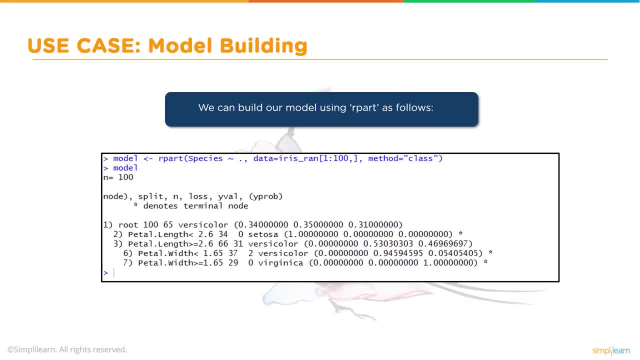 that way, we have our training set and our test set already pre-built, because we randomized the rows going in from the beginning and then, once we've done that, we want to go ahead and print our model out and take a look at it. let's go ahead and put this into our r studio. 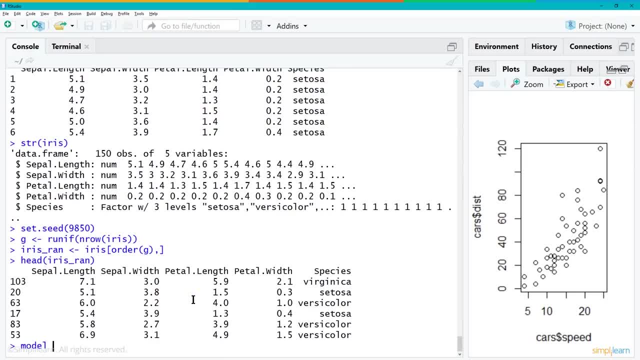 and take a look, and so we have our model. we're going to call it model, that's our variable name that we're giving it. we're going to assign that our part, and in brackets we'll start with species and we want to correlate species to all the other columns. 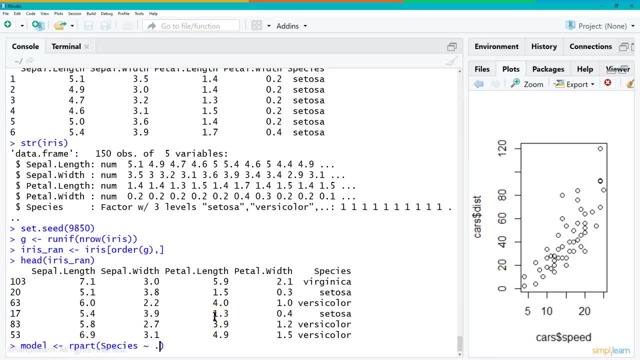 so how do we do that? and the shorthand is just to put a period there and then we're going to put a comma and we want to set our data equal to iris ran. that's the data we put in there. and remember I said we're going to do just the first 100 rows. 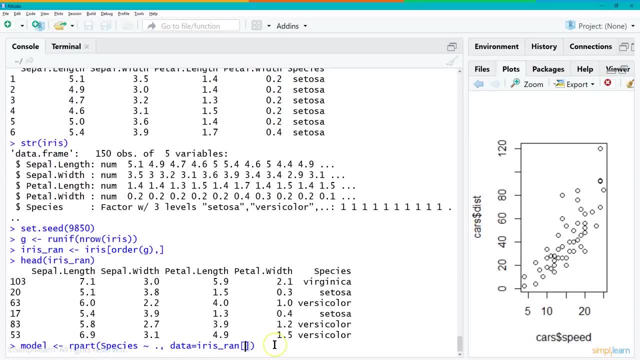 so we can save the last 50 for testing. so we can do that simply by doing row 1 to 100. so in r you start with 1 for your rows and because we want all the columns, we just put a comma and that denotes that we're going to use all the columns in here. 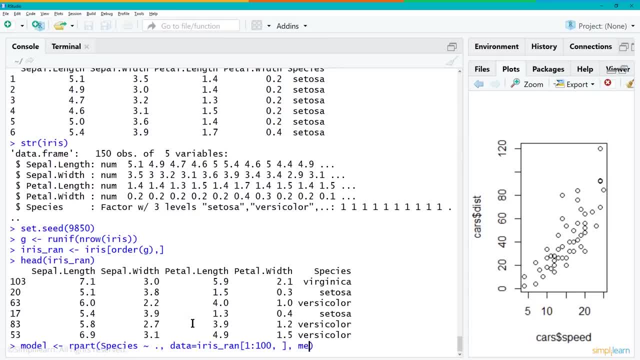 and in the r part there's different methodologies. we're using the method equals class, and you realize that we're doing a classification between the three different types of flowers, and so this is what we want to go ahead and set up our model with, and when we run that, 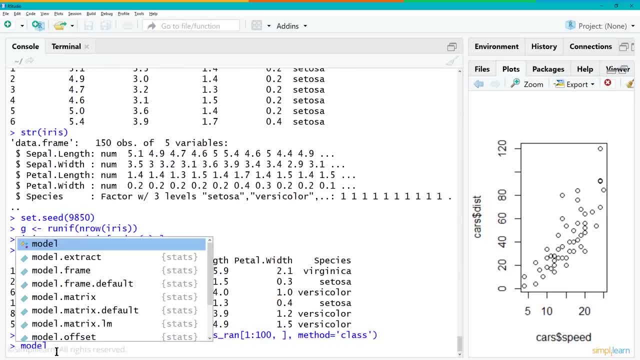 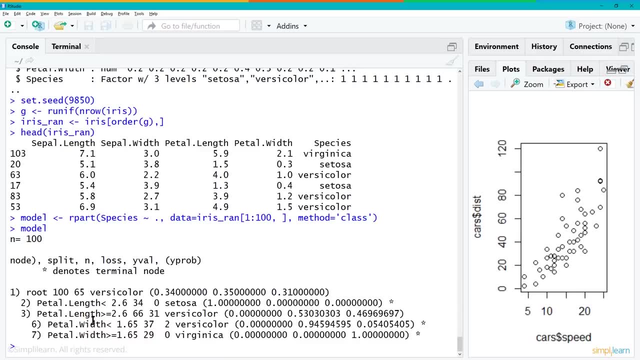 we've now created a nice model for us so we can go ahead and just type in model, hit enter and you'll see it'll print out a bunch of information about our model. so let us know what's going on in there and let's just break that down and see what that looks like. 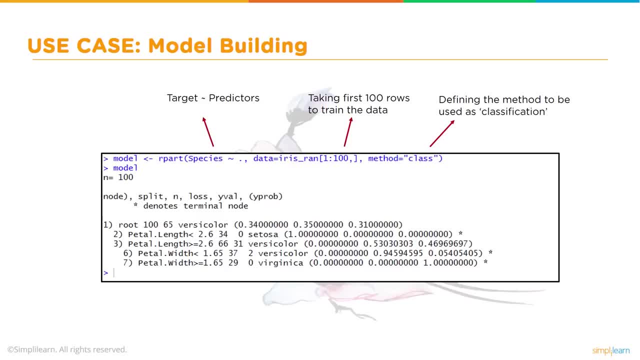 so we have our target, our predictors, that's species and it's going to relate to. we used a period to denote all the columns. we're going to take the first 100 rows to train the data and we have the defining method to be used as classification. 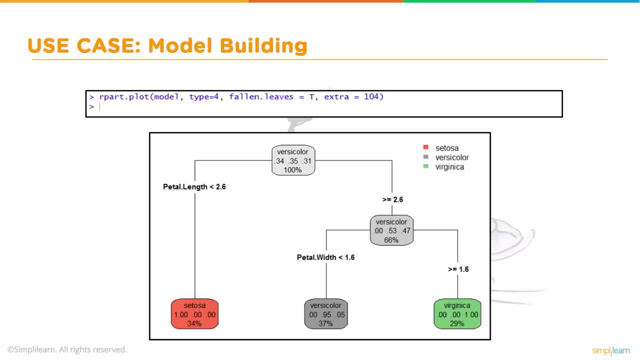 that's what the method equals class is, and what we want to do next is we're going to do a plot and take a look and see what this actually looks like- a little visual here, which is nice. we can simply do that with rplot for the model. 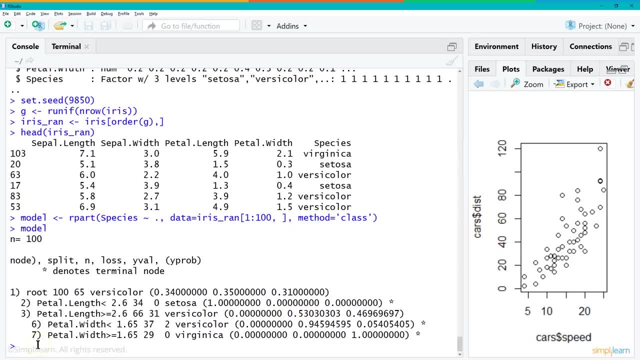 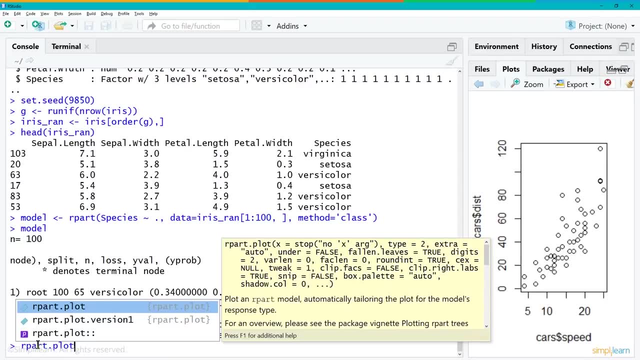 and let's break this down a little bit and see what that looks like in the rsetup. and we do this rpartplot a little bit of a mouthful there. sometimes that's part of the rpart package or module, so when you imported this in, it also included its own plotting format. 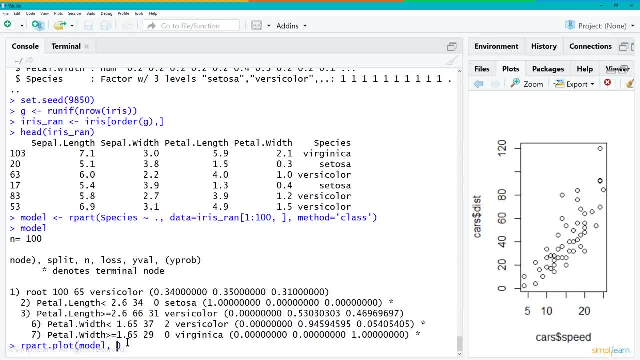 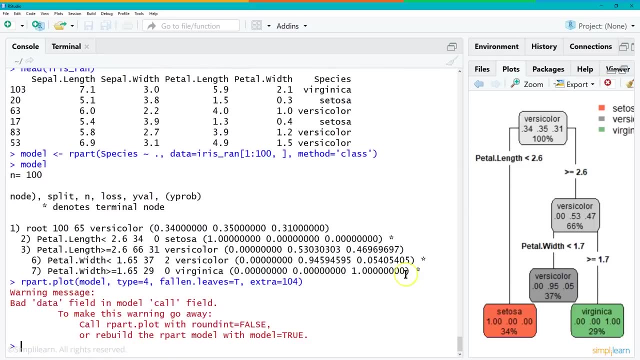 and we're going to send it our variable model. and there are actually a number of types of plots listed for rpart, but we're just going to do: type equals 4, fallenleaves equals t and extra equals 104. let's go ahead and hit enter on there. 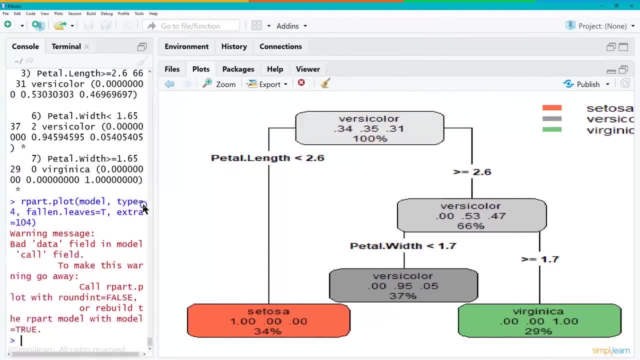 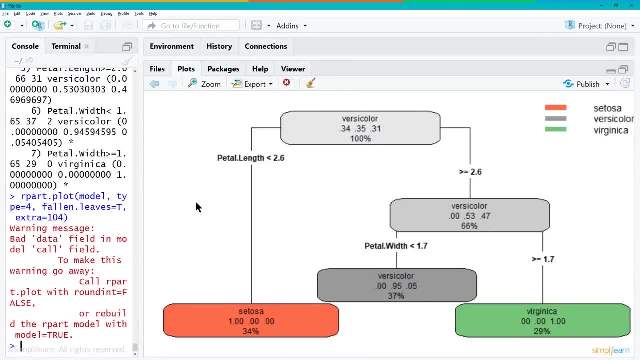 and you'll see, right over here on the right hand side, it goes into our plots. we just enlarge that. we have our versicolor, our setosa versicolor, virginica, and let's go ahead and break that down. as you can see down here, it represents a tree as it splits. 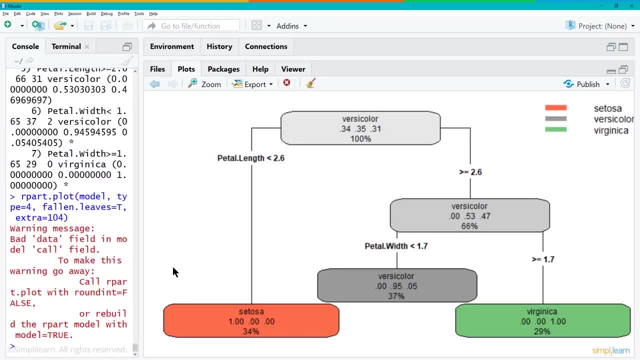 it looks at it and says, hey, if the petallength is less than 2.6, it's going to be a setosa. 34% of them fall into that category. and if the petallength is greater than 2.6, then it looks at that and says, ok, now I have 3 different variables. 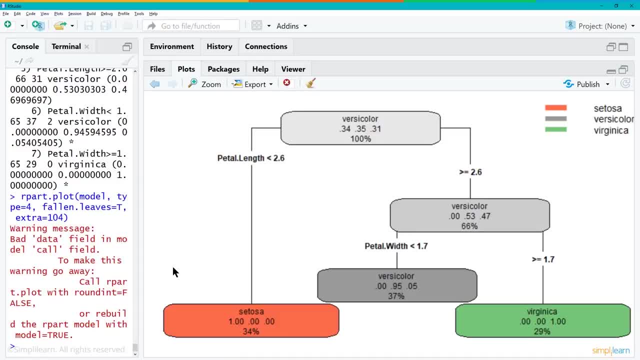 we're going to split it again. petalwidth is less than 1.7, it's going to be a versicolor, and if it's greater than 1.7, it's a virginica. and so you can see here it's a very simple tree. it forms. 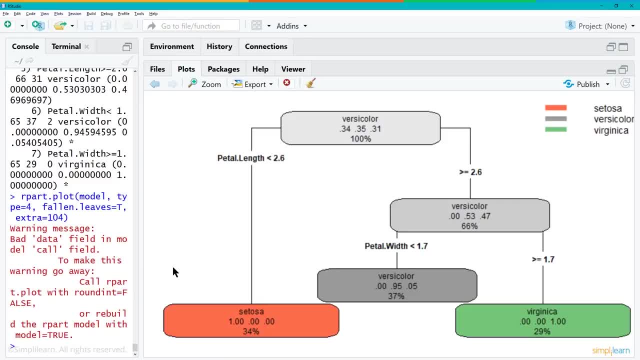 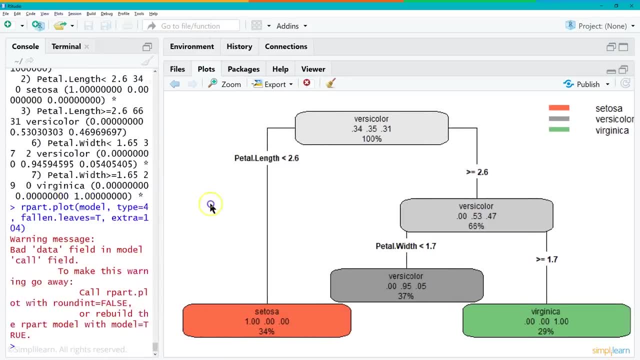 it's only got a couple levels. you can see a branch off to the right. very nice depiction of what's going on as far as the model now that it's created. but once we create the model, we need to figure out: is this model any good? so let me go back over here. 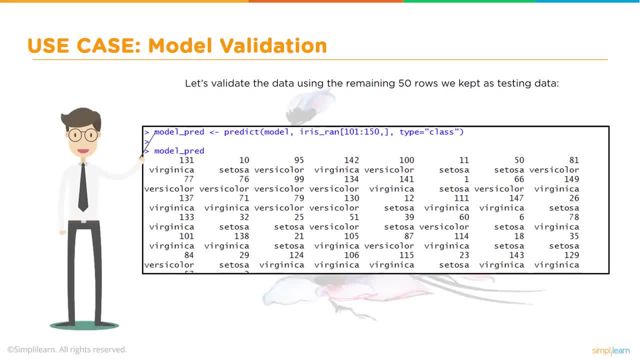 and let's go back to our slides and the first thing we're going to do is we're going to take our test data. remember? we saved 50 rows for the end to go ahead and run a predict on there. so let's go ahead and run that prediction. 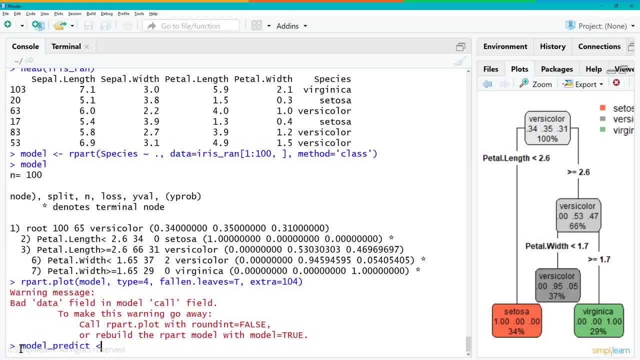 so we'll call it model underscore, predict, and we're going to hit a wrong button there. to predict what are we going to predict? we're going to predict our initial model and we need to send the data. so data equals and we don't actually have to put the data part in. 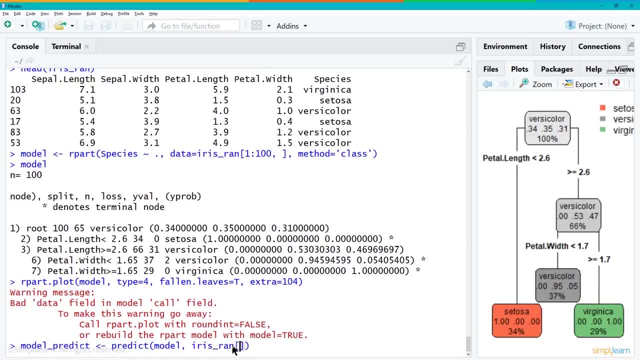 we'll put in iris, underscore ran, and then we want to do just the last 50 rows and we denote that by 101, colon, 150 and then comma, and we'll leave that part blank, since we want all the columns to show up. and then, finally, this is a classification: 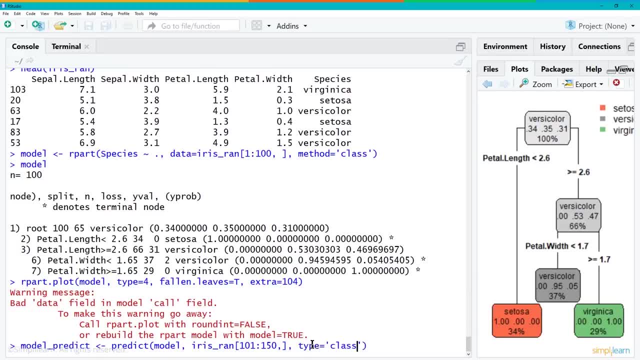 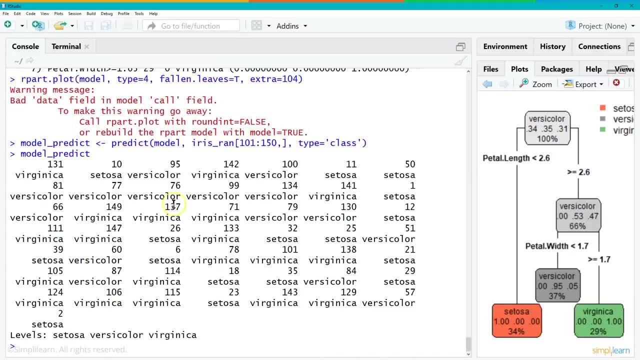 so we need to let it know that type equals class. there we go, and let's just see what that looks like. model predict, and so this is what the data is put out, as it says, whatever this is, 131 is a virginica number, 10 is a setosa. 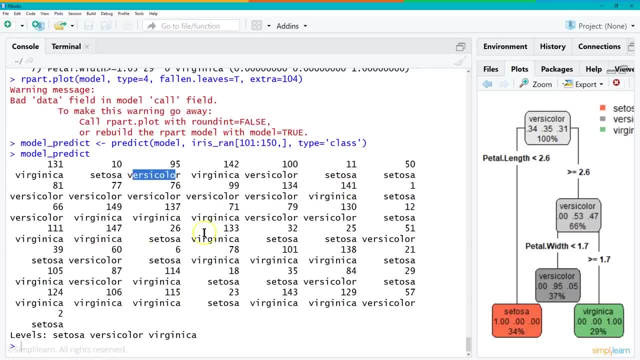 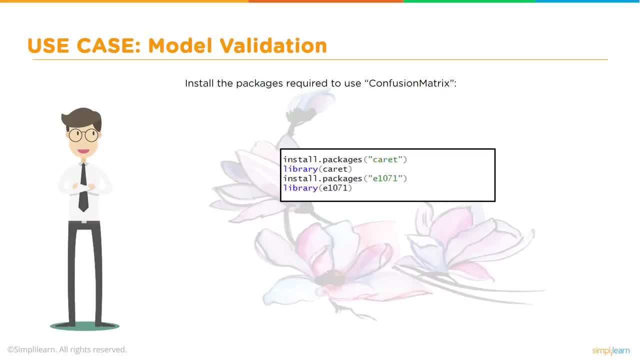 line number 95 is a versicolor, and so on all the way through. what we really want to know is how good our model is, so we're going to go ahead and install a couple more packages. we're going to install the packages required to use the confusion matrix. 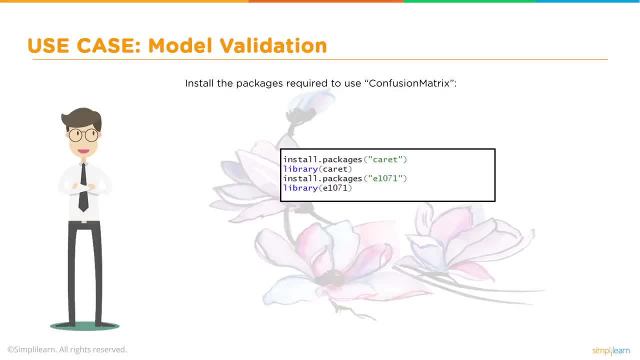 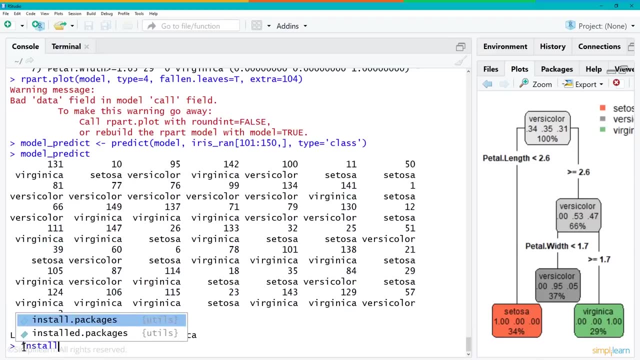 and to do that we're going to install caret and e1071 and then, of course, we want to set them to our project by using the library command, and so we can simply install packages and we want caret, and we'll go ahead and just do that right there. 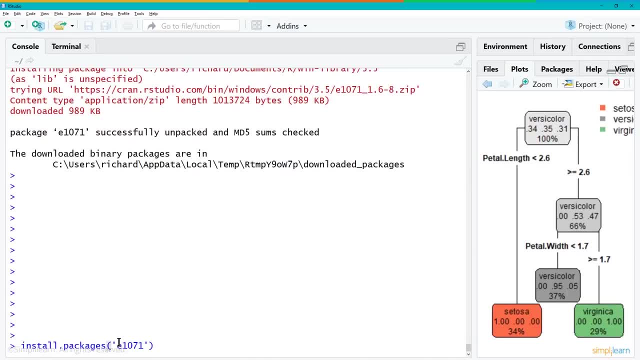 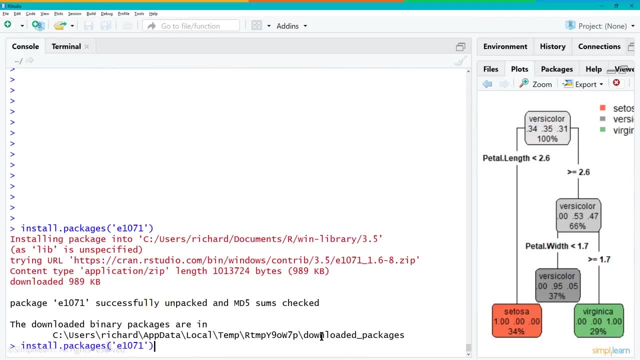 there's caret installed and we went ahead and did the install for packages e1071. see, it goes through there. it's a really quick install compared to the caret. and then, once we've installed the packages, we need to load it into our workspace. so there's our library caret. 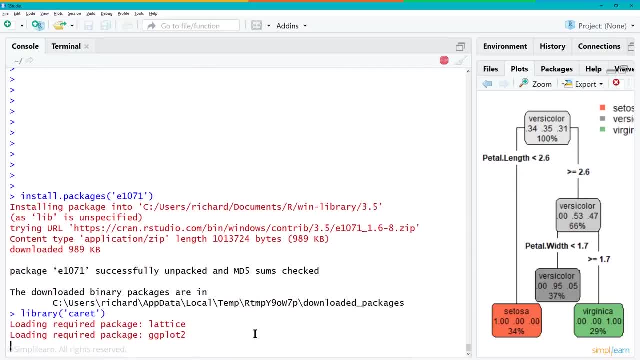 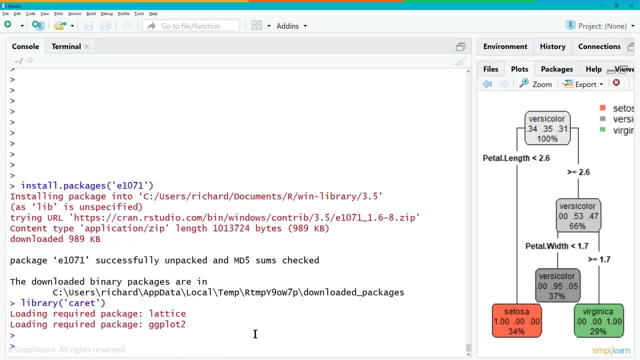 let's just load it in there. there it goes, and once that's loaded, we'll go ahead and also load the or set the library to the e1071, so that we have both those libraries available to us. and here we go, library, and then this one is e1071. 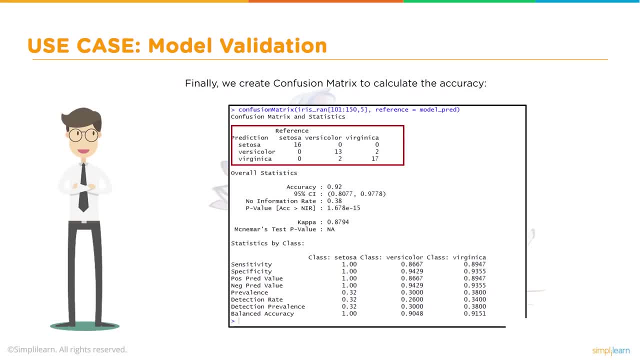 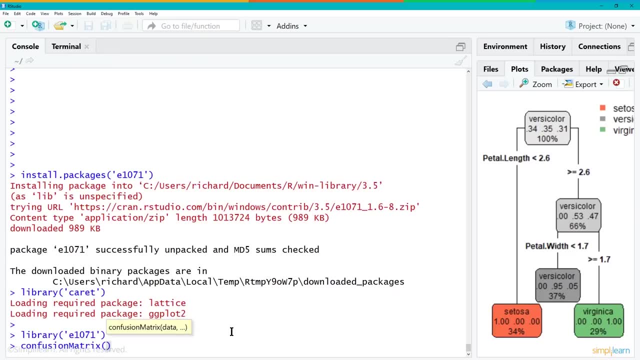 and now these two libraries are fully available to us, and then we're going to use these tools to create the confusion matrix and this one confusion matrix- this is the iris ran- and then we'll go ahead and put the brackets here and we're only going to do 101 to 150. 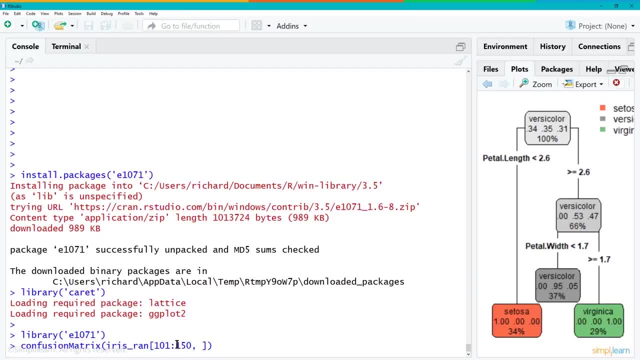 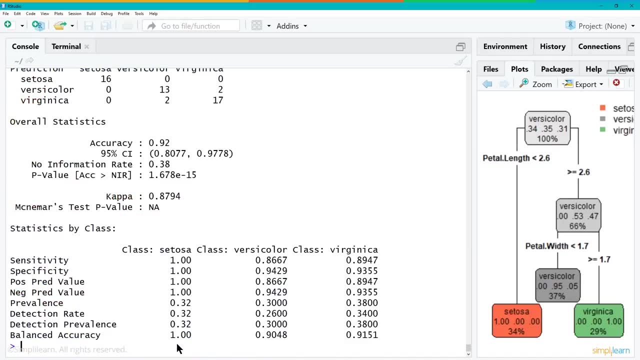 and then we only want the first five columns, not the last five columns. the first five columns, so five in there and we'll set that to our model predict and then when we hit enter, it's going to head and just print out all this information. so right here we're looking at our confusion matrix. 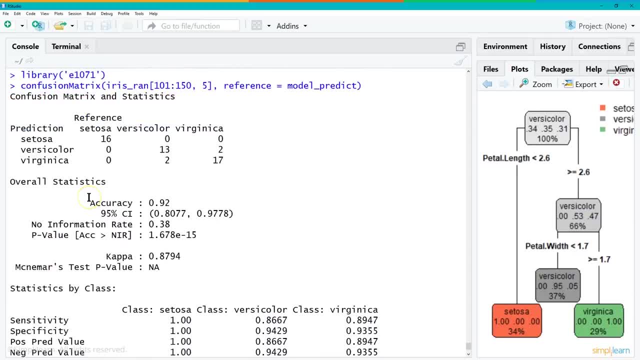 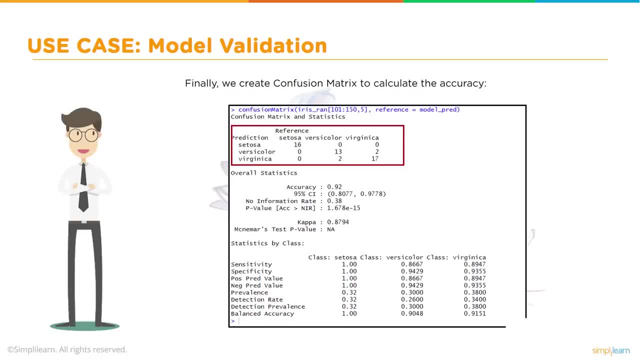 to see how everything kind of balances out. let's go over that and see a little closer what that actually means. so the first part, we see, is a reference, and in here we have our prediction, because that's what we call the column, if you remember correctly, and we have it for setosa versicolor virginica. 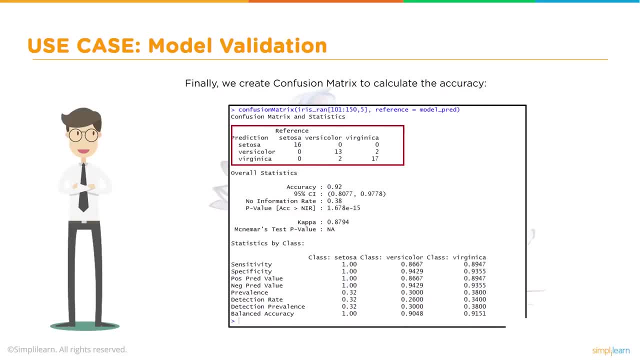 and then we have setosa, versicolor, virginica, going down each side and the way you read this is, if you look at this, we predicted 16 out of 16 setosa and then versicolor. we predicted 13 of the versicolor and then two of those we predicted as virginica. 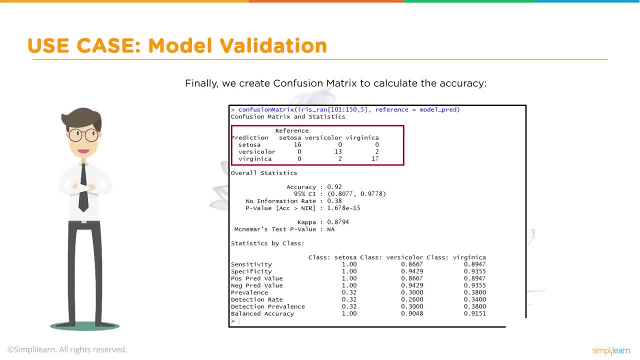 so we were wrong on two of those and with the virginica we predicted 17 correct and we had two wrong that were versicolor. so we look at the overall statistics on here and we have an accuracy of 0.92- 95 percent CI. that's pretty good as we're going through here. 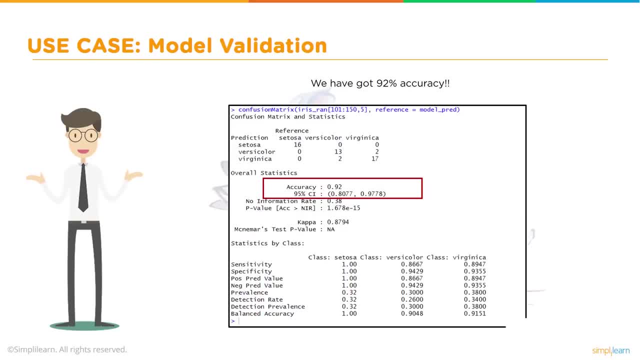 those are good deals on that and there's a lot more information as you go down this. the one thing I want to remind you on this, as we're looking at these predictions- and this is also true for the linear regression model we looked at earlier- when we talk about the accuracy, 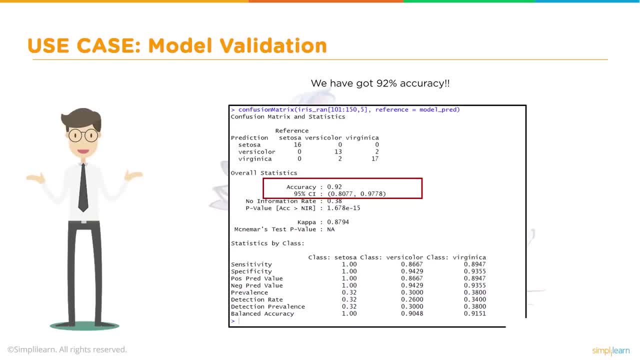 that is the accuracy on this data and we say that as a programmer to make that a very clear distinction, because if you're in data analysis you should cringe if I say this is a 95 percent accurate model without that put in there, because bad data in 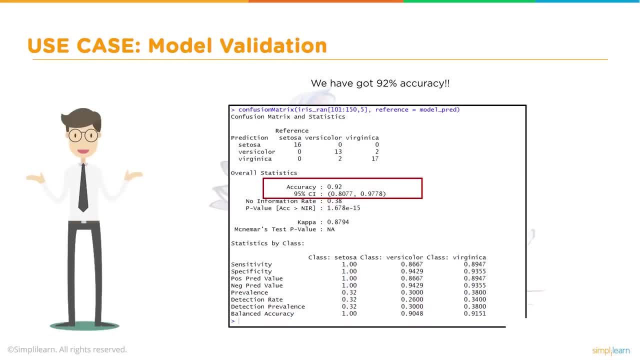 bad data out. we won't go into detail right now on that, but that is very important to note that whenever you quote any of the accuracies on here or you discuss any of these values that come up, hello and welcome to logistic regression in R. my name is Pete Ferrari. 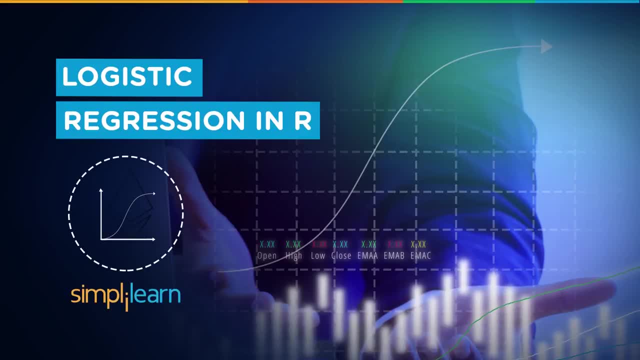 and I am with the Simply Learn team, and today we're going to cover logistic regression in the R programming language. logistic regression is kind of a misnomer in that when most people think of regression, they think of linear regression, which is a machine learning algorithm for continuous variables. 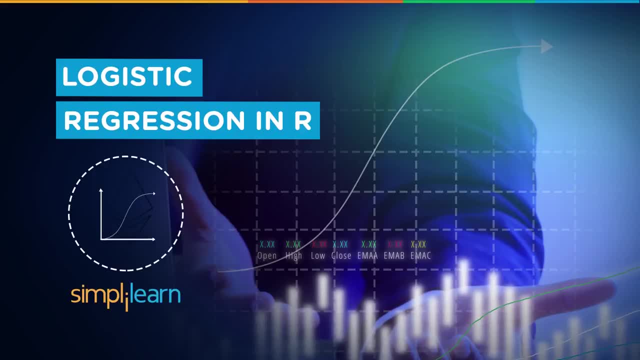 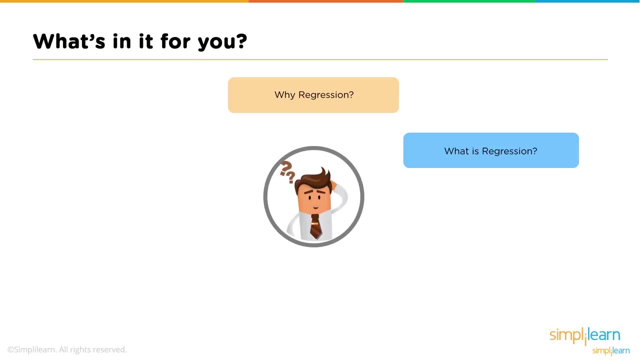 however, logistic regression is a classification algorithm, not a continuous variable prediction algorithm. logistic regression is also sometimes called logic regression. in this video, we are going to learn why we would use regression as a predictive algorithm. what is regression? the different types of regression, as I've already mentioned, 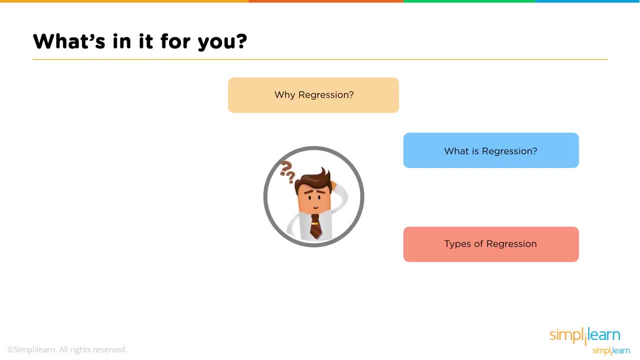 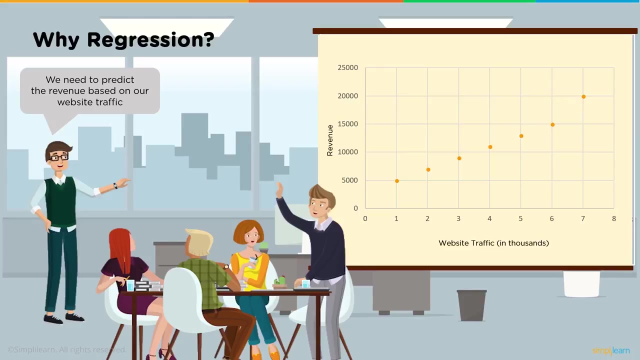 some regression algorithms are classification algorithms and some are continuous variable algorithms. why use logistic regression? what is logistic regression? and then we'll look at a use case: a college admission using logistic regression. so why would we use regression? well, let's say we had a website and our revenue was based on the traffic. 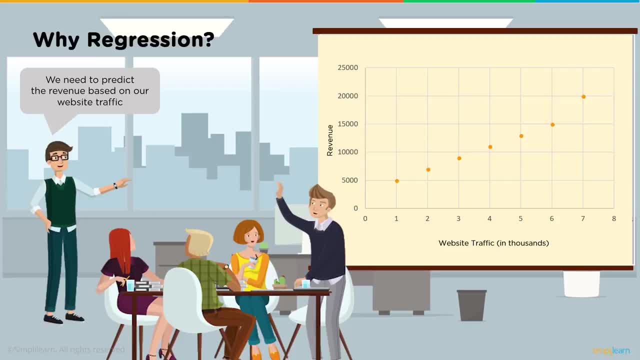 that we could drive to that website, whether through R&D or marketing, and we wanted to predict the revenue based on site traffic. then the website traffic would be related to the revenue we could generate. the more traffic driven to our website then the higher our revenue, or at least that's what we would intuitively assume. 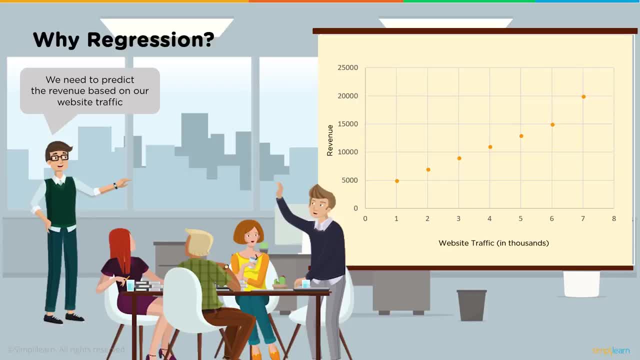 and so we need to predict the revenue based on our website traffic. here we have the plot of revenue versus website traffic. traffic would be considered the independent variable and revenue would be the dependent variable. often the independent variable or variables- if we had more than one- could be called the explanatory variable. 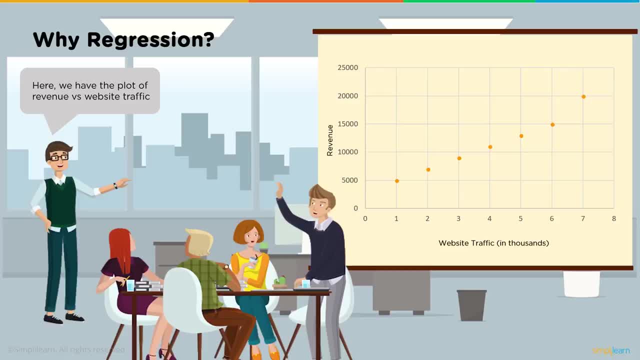 the explanatory variables, and the dependent variable would be called the response variable. however, we typically refer to them as independent and dependent variables. so our intuition tells us that the independent variable drives the dependent variable, and if there is some relationship between the two variables, then we would say that there is a correlation between the two variables. 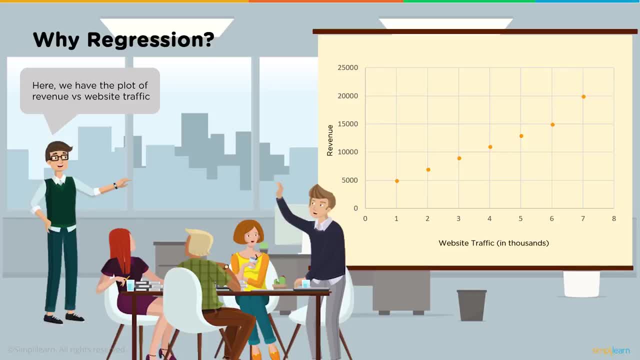 and then we may be able to use the independent variable to make predictions about the dependent variable. if you look at the chart on the right, you'll see there is a clear trend between website traffic and revenue. as website traffic increases, the revenue increases, and we could draw a line to show that relationship. 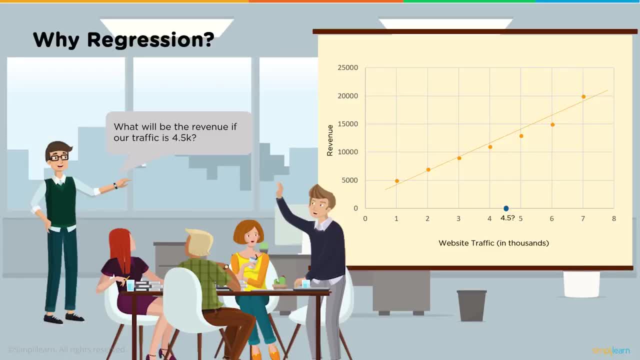 and then we could use that line as a predictor line. so, for example, what will revenue be if our traffic is 4.5k and we see that when the traffic is around 4,500 the revenue is around 13,000? and if we could draw a perpendicular line? 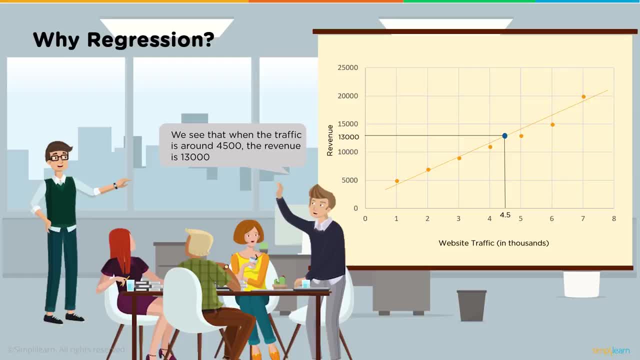 from 4.5k on the axis, on the x-axis, the traffic axis, up to the orange regression line, sometimes called the line of best fit. then we could draw another line over to the y-axis, the revenue axis, and we could see where it lands, and that would be the prediction. 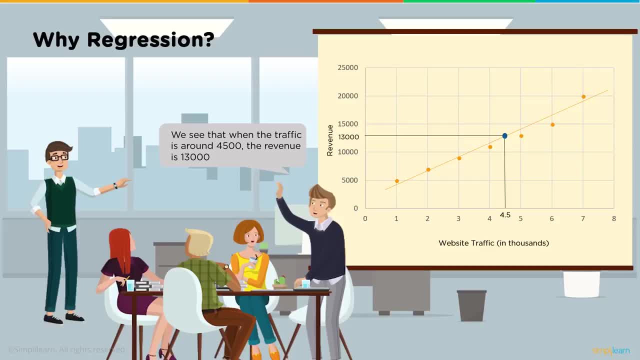 so in this example, when the traffic is around 45,000 hits, the predicted revenue is around 13,000. normally we wouldn't actually draw those lines. we would generate an equation and we would call that equation a model and we could plug the independent variable. 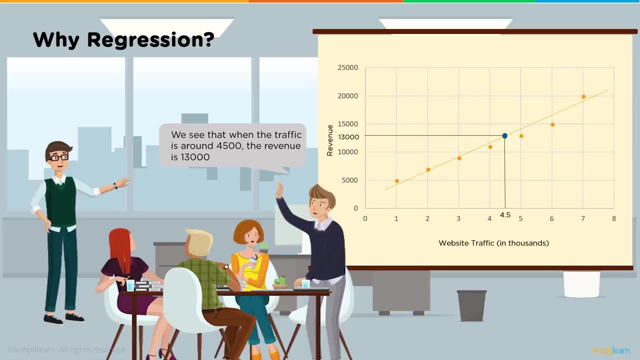 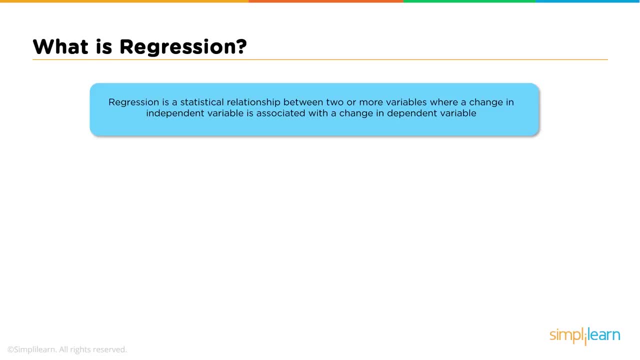 into the equation to generate the dependent variable output which we would call our prediction. so what is regression? regression is a statistical relationship between two or more variables, where a change in the independent variable is associated with a change in the dependent variable. it's important to note that not all variables 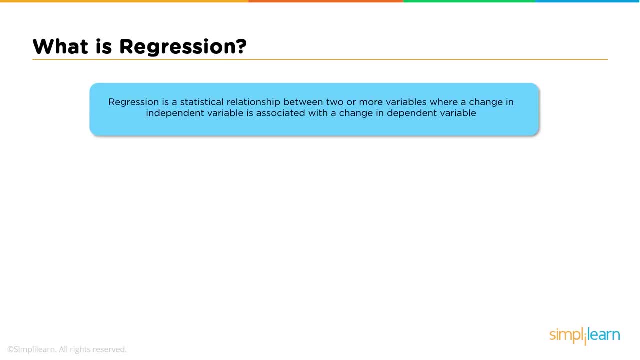 are related to each other. for example, a person's favorite color may not be related to revenue from a website. here the change in one variable height is closely associated with the change in the other variable, age. this makes intuitive sense as you get older from when you're born. 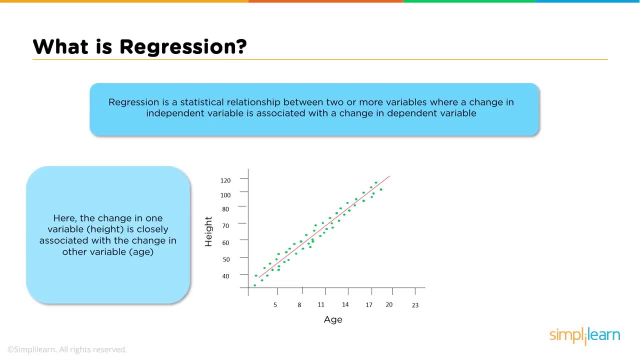 you get taller and it seems to make sense. if we plot that data, we would see those green points on the graph up to some certain age where growth would taper off in the plot. in the middle of the screen we see the clear linear relationship between age and height. 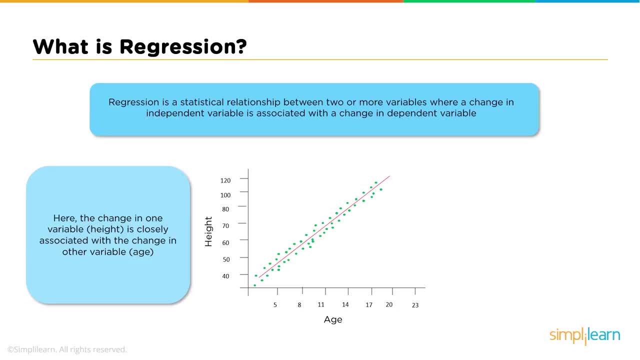 which is indicated by the solid red line. we sometimes call that line a trend line or a regression line or the line of best fit, and we see that the height is the dependent variable and age is the independent variable. of course, you might ask: doesn't height depend on other factors? 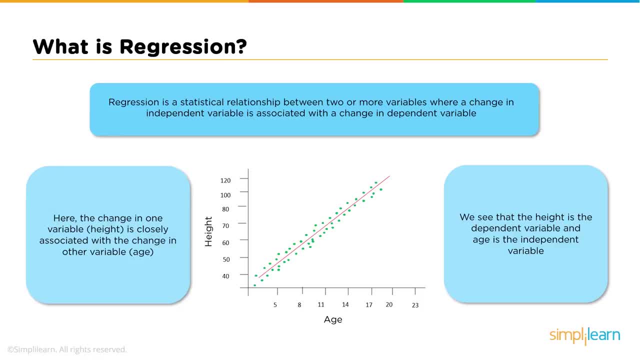 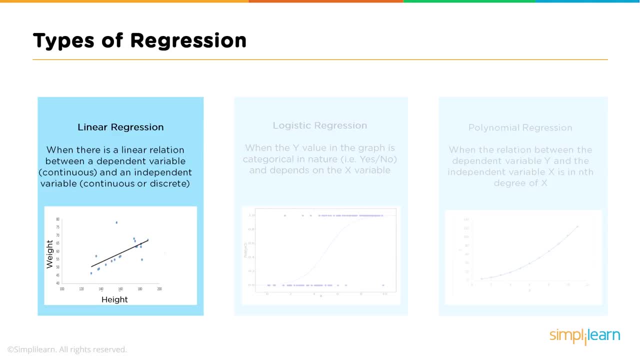 of course it does, but here we're looking at the relationship between two variables, one independent and one dependent: age and height. there are various types of regression: linear regression, logistic regression, multiple linear regression, polynomial regression- and there are others: decision tree regression, random forest regression, but linear regression. 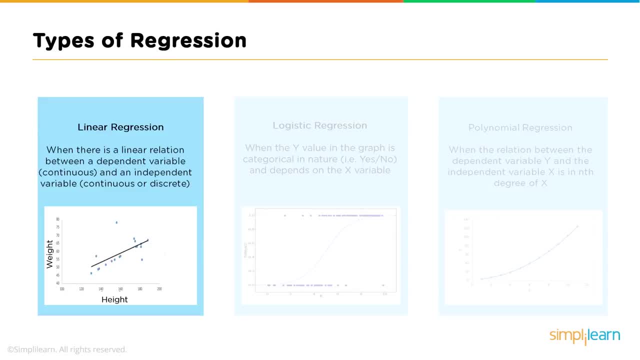 is probably the most well known and by definition. when there is a linear relationship between a dependent variable which is continuous, and an independent variable which is continuous or discrete, we would use linear regression. when the y value in the graph is categorical, such as yes or no, true or false, 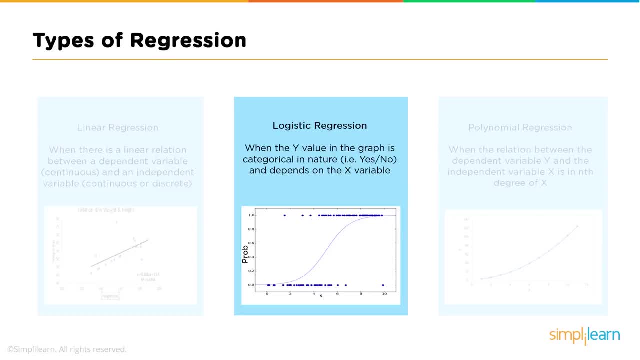 they voted, they did not vote. they purchased something. they did not purchase something. it depends on the x variable. logistic regression is when the y value in the graph is categorical in nature. for example, yes, no, purchased, don't purchase. voted, did not vote. and it depends on the x variable. 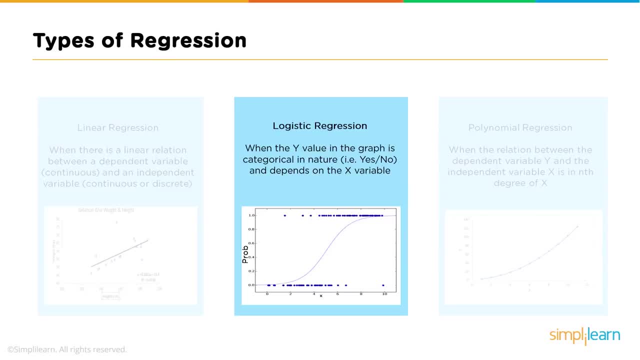 notice the trend line for linear regression and the line for logistic regression. they're different. more on that later. and there's polynomial regression as well, when the relation between the dependent variable y and the independent variable x is in the nth degree of x. sometimes we say an nth degree polynomial of x. 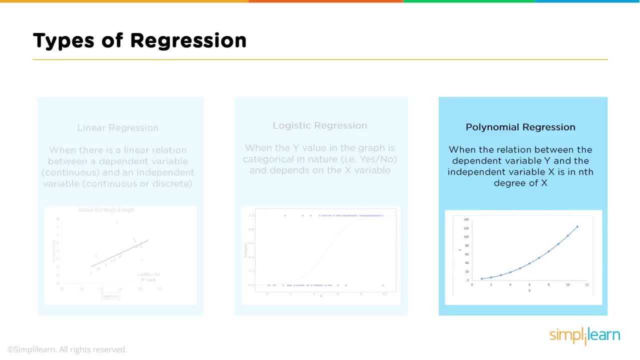 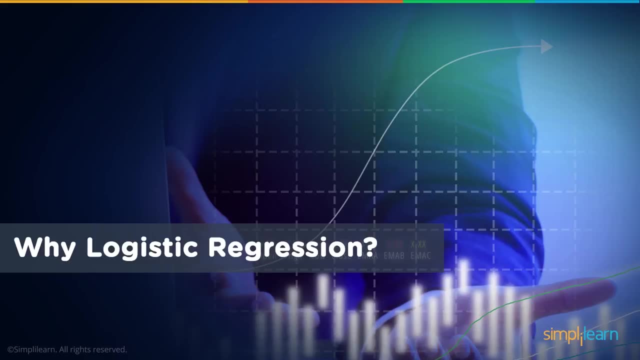 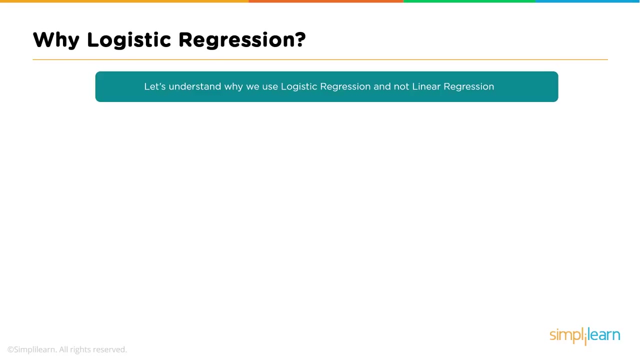 in this picture you can see that the relationship is not linear. there's a curve to that best fit trend line, so why would we use logistic regression? and we need to understand why we would use logistic regression and not linear regression. picking the machine learning algorithm for your problem. 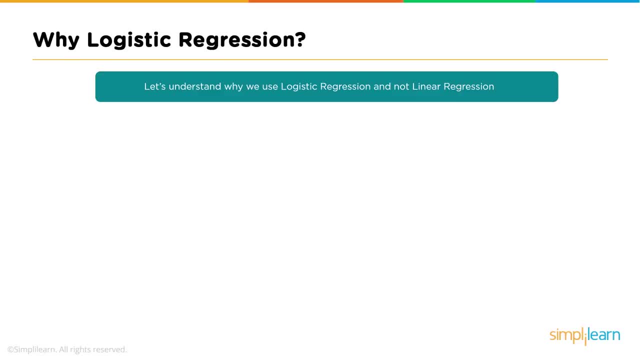 is no small task, and it really behooves us to understand the difference between these machine learning algorithms. linear regression answers the question how much so in our earlier example, if website traffic grows, then how much would revenue grow? whereas logistic regression would answer what will happen or not happen. 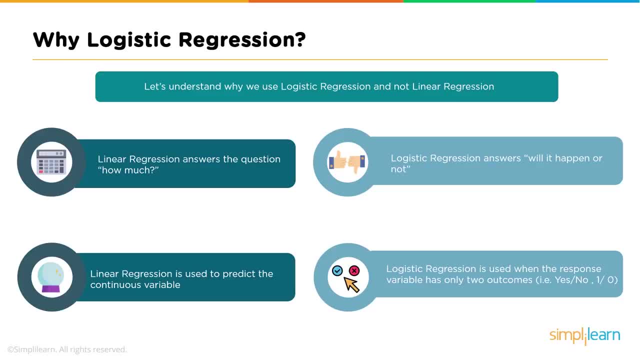 linear regression in general is used to predict a continuous variable like height and weight. logistic regression is used to predict how much revenue will grow, but the response variable only has two outcomes: yes or no, true or false. often we refer to logistic regression as a binary classifier, since there are only 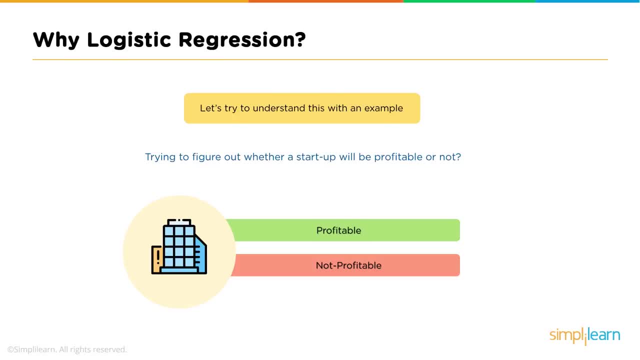 two outcomes. so let's try to understand this with an example. let's say we have a startup company and we are trying to figure out whether the startup will be profitable or not. that's binary, with two possible outcomes- profitable or not profitable- and let's use initial funding. 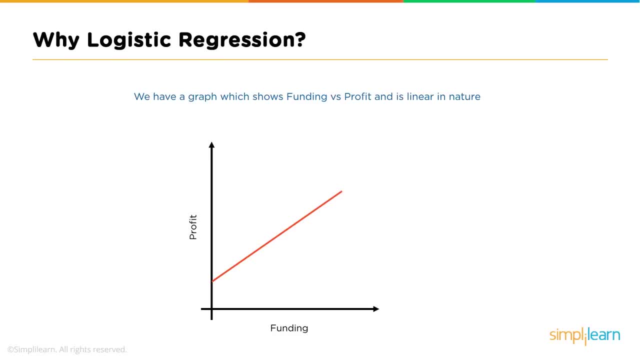 to be the independent variable. here we have a graph that shows funding versus profit appears linear. Once again, our intuition tells us that the more funding a startup has, the more profitable it will be. But of course, data science doesn't depend on intuition, It depends on data. 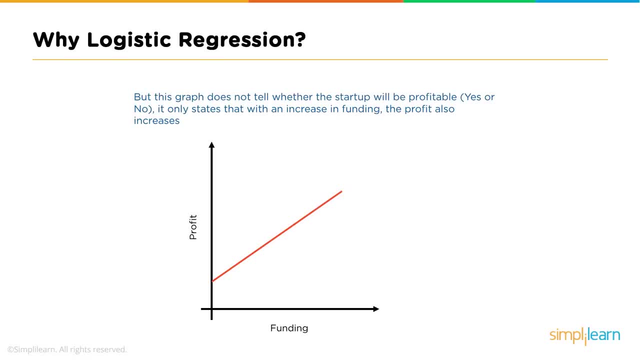 But this graph does not tell whether the startup will be profitable, yes or no. It only states that with an increase in funding, the profit also increases. That's not binary. If we wanted to predict how much profit, then linear regression would be useful. But that's not what we are being. 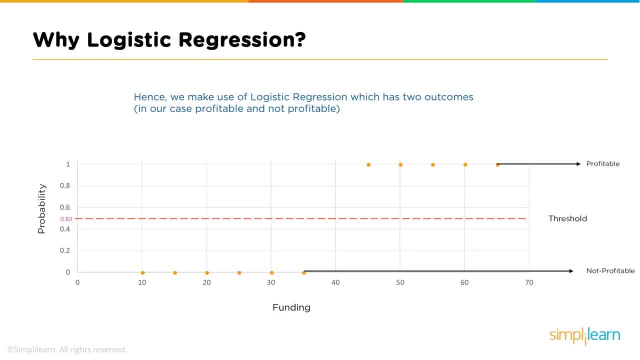 asked. Hence we need to make use of logistic regression, which has two outcomes, in our case: profitable and not profitable. So let's draw a graph again: The x-axis will be our independent variable funding and the y-axis will no longer be the dependent variable profit, but it will be. 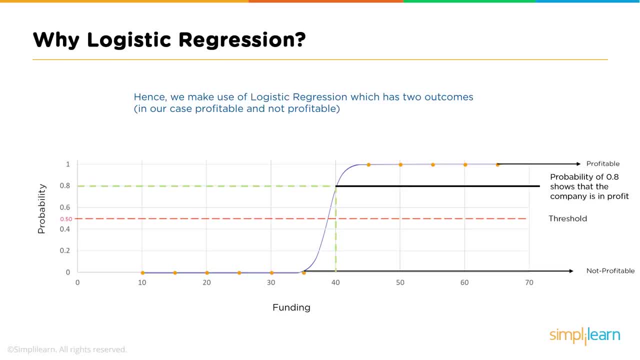 the probability of profit. For example, if you look at a company with a funding of, say, 40, then the probability that that company will be profitable is around 0.8 or 80 percent, based on the probability of profit. So if we look at a company with a funding of, say, 40,, 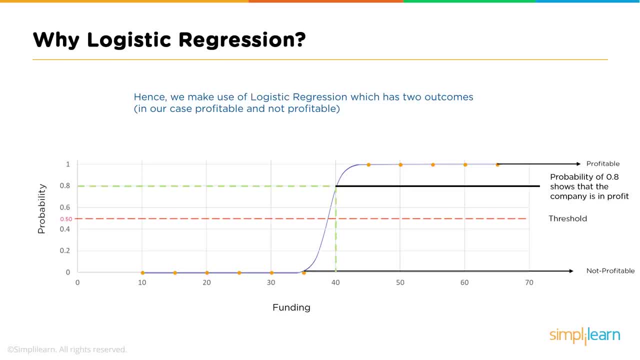 then the probability that that company will be profitable is around 0.8 or 80 percent, based on the best-fit line called a sigmoid curve. In the example we plotted several companies, some with 10,, 15, 20,, some with 50,, 60, or 70, or 65, and we indicated whether they were 0,. 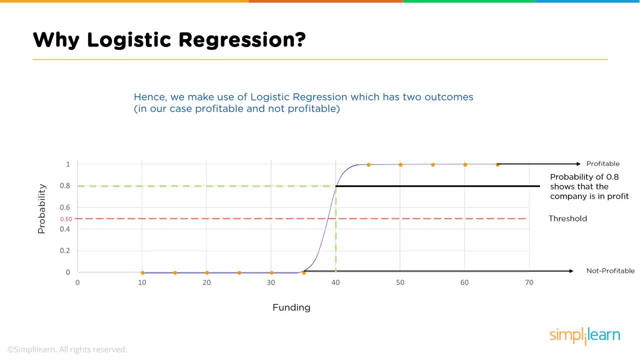 not profitable or a 1, profitable on the graph, And this is how we should think of logistic regression. In this example, given the amount of funding, we calculate the probability that a company will be profitable or not profitable And if we use the threshold line of 50 percent, 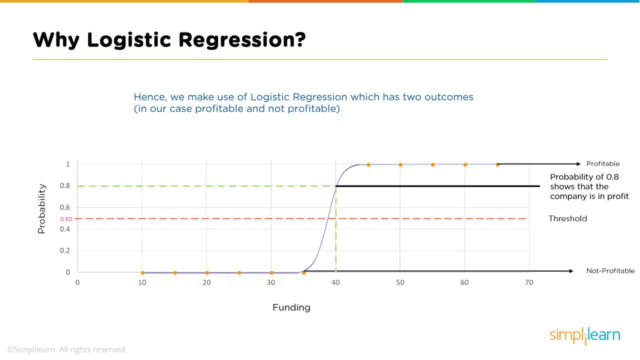 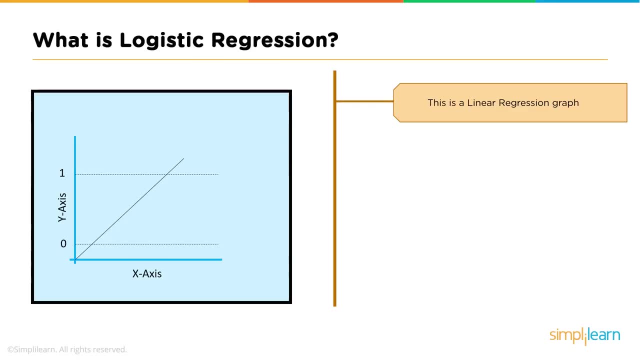 then we have our classifier: If the probability is 50 percent or higher, the company is profitable. If the probability is lower than 50 percent, it's not profitable. So what is logistic regression? This is a linear regression graph, So let's compare linear regression to logistic regression. 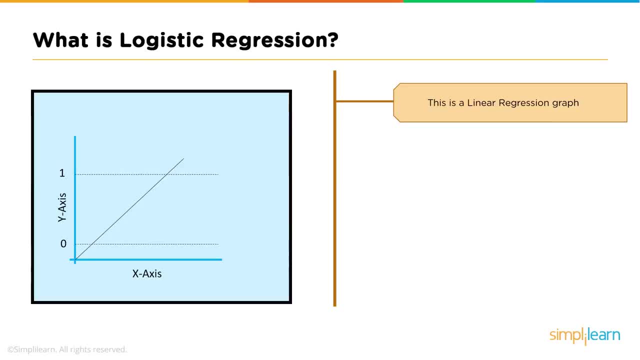 and take a look at the trend line that describes the model. It's a straight line, which is why we call it linear regression. But using linear regression we can't really divide the output into two distinct categories. yes or no To divide our results into two categories? 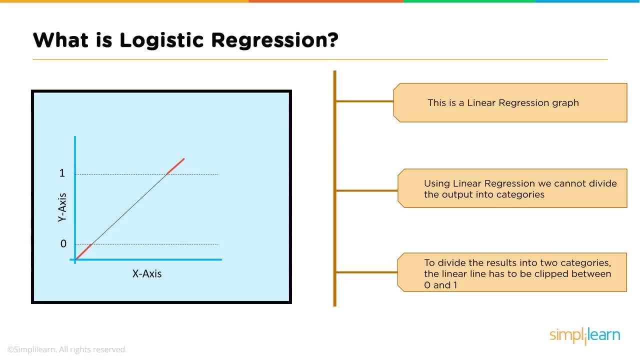 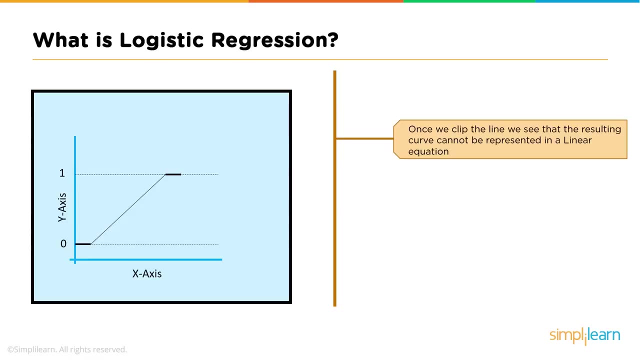 we would have to clip the line between 0 and 1.. If you recall, probabilities can only be between 0 and 1, and if we're going to use probability on the y-axis, then we can't have anything that is below 0 or above 1.. Thus we would have to clip the line, And once we clip the line, we see that 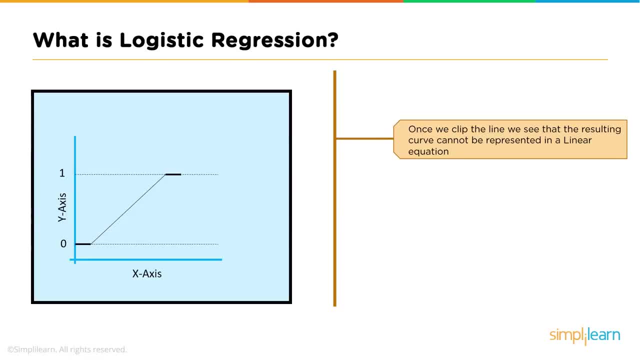 the resulting curve cannot be represented in a linear equation, So for logistic regression we will make use of a sigmoid function, and the sigmoid curve is the line of best fit. Notice that we have a linear regression graph, but it does satisfy our requirement of using a single line. 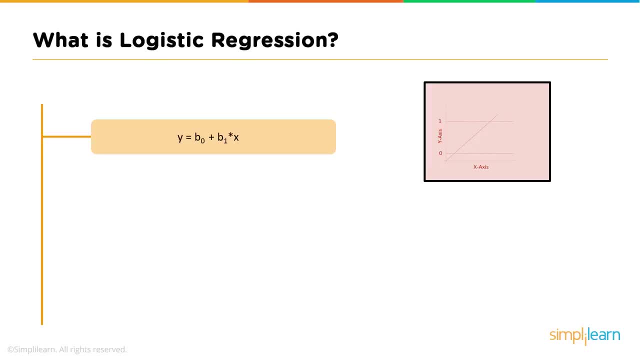 that does not need to be clipped. For linear regression, we would use an equation of a straight line: y equals b sub 0 plus b sub 1 times x, x being the independent variable, y being the dependent variable. But, as we've said, we cannot use a linear equation for binary. 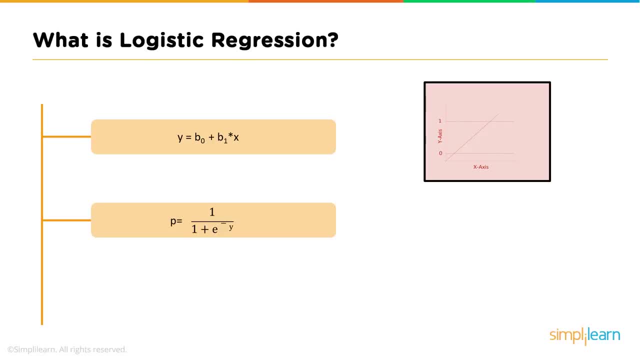 predictions. so we need to use the sigmoid function, which is represented by the equation: p equals 1 divided by the quantity 1 plus 1.. So we have a linear regression graph and we can't use the sigmoid function, So we have to use the sigmoid function, which is represented by the equation. 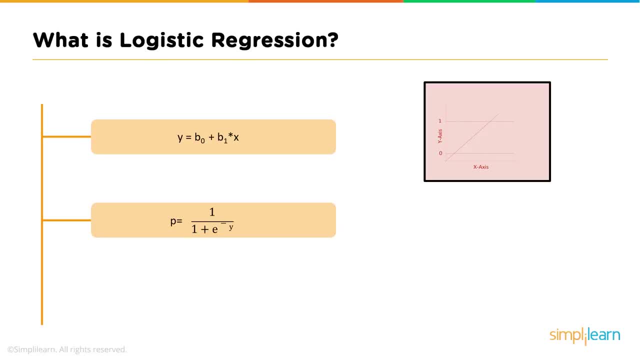 p equals 1 plus 1 plus e to the minus y, e being the base of the natural logs. Then, taking the log of both sides and solving, we get our sigmoid function And graphing it, we get our logistic regression line of best fit. The applications for logistic regression are endless. Here we might. 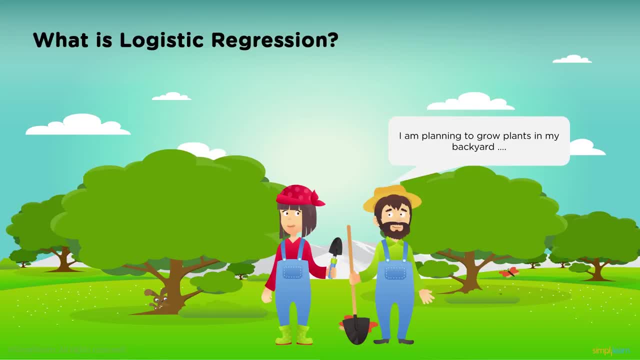 have a couple of gardeners or farmers, and one farmer says: I am planning to grow plants in my backyard and I want to know whether my trees will get infested with bugs, which I'm sure is a huge problem. And these days, the fewer pesticides we use, the better off we are with the plants. So we 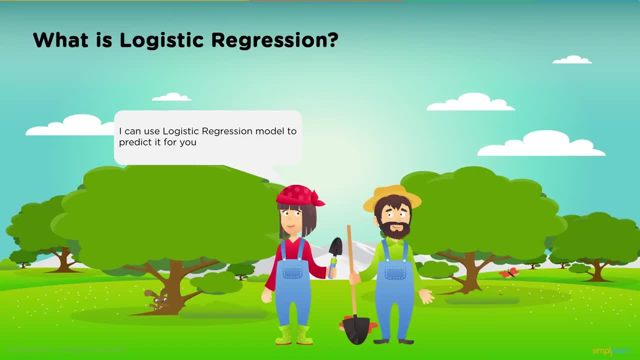 The young lady says: I can use logistic regression in a model to predict it for you. And the other farmer says: well, how is logistic regression going to help? But we know that healthy versus not healthy is a binary classification and we can use a binary classifier like logistic regression. 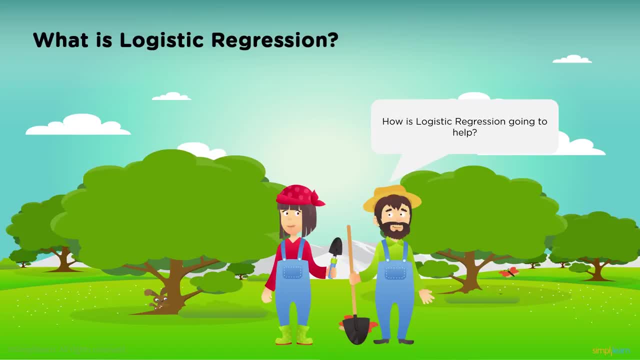 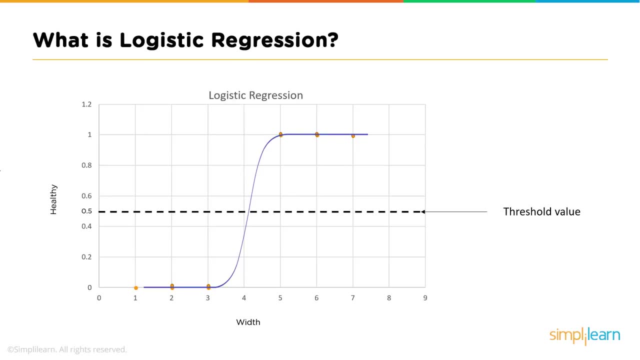 to solve this problem, which is what the young lady has in mind. If we have the data, we can model the data and generate a sigmoid function that best fits our data and then use the probability of the logistic regression to solve the problem. So we have a binary classification and we can. 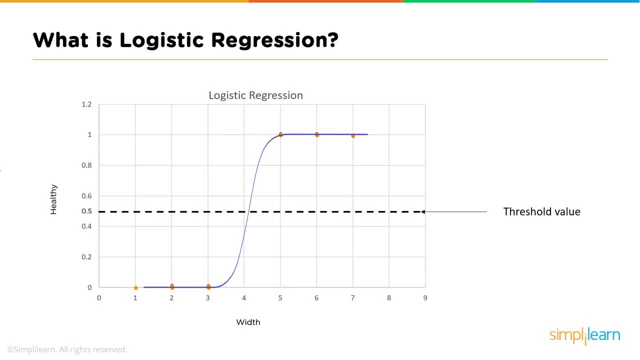 of a healthy tree versus a not healthy tree or an infested tree. Once again we see our sigmoid line of best fit and some points that represent healthy trees and not healthy trees. Once again we plot our sigmoid curve, scratch that And once again, once our sigmoid curve is plotted and our threshold, 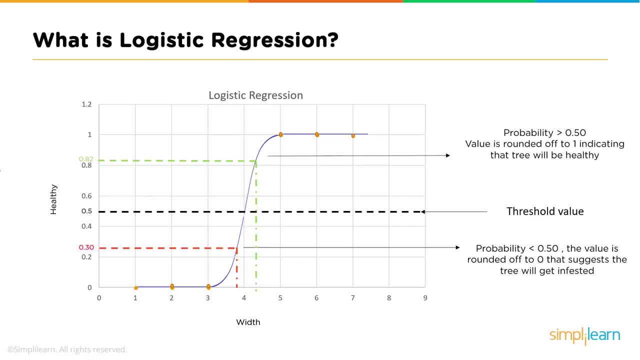 is set almost always at 50%. we can use the sigmoid curve and calculate the probabilities and hear the independent variable of width, which I assume is an application of pesticides or no pesticides, to determine whether or not the probability of healthy is greater than 50% the threshold or less than 50%. 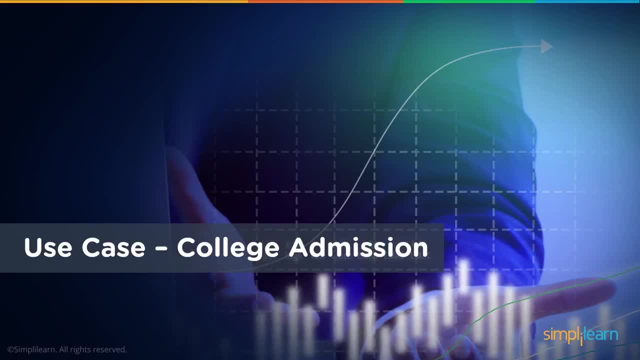 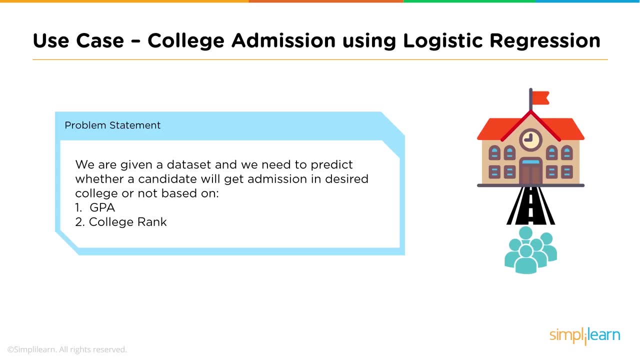 the threshold. And now let's take a use case of a college admission problem. Of course, we can't solve anything using data science if we don't know what the problem is. So we need a problem statement. And here the problem statement is simple: We are given a data set and we need to predict whether a 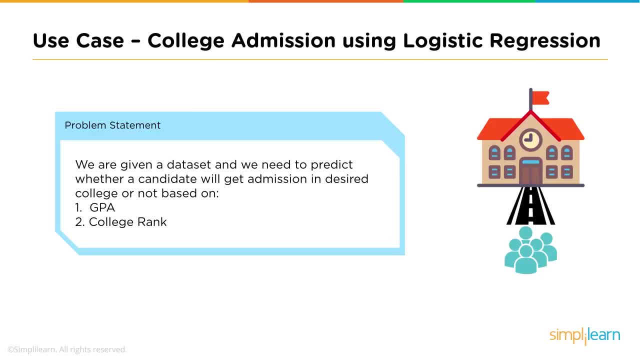 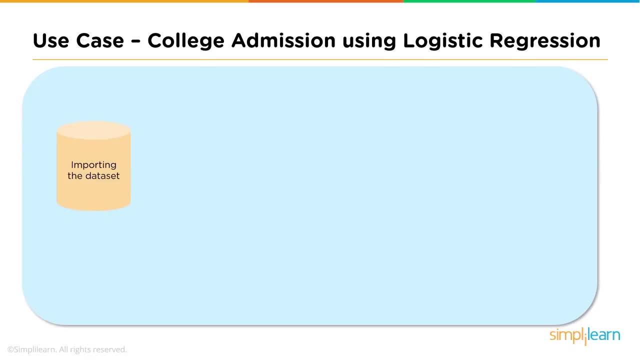 candidate will get admission in a desired college or not, based on their GPA and college rank. So the very first thing we need to do is import the data set, And if it's a small enough data set and it can fit into our computer memory, then we are golden. Otherwise, we have some work to do. The data set that we were given is in. 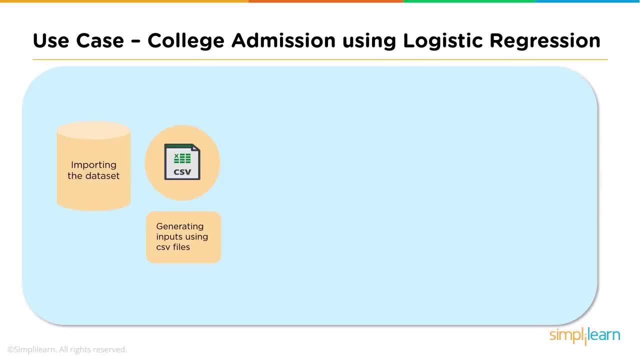 CSV format: comma separated values. CSV files are easily imported into our environment. Once we import the data, we next need to select and import the data set. And we need to select and import the data set And we need to import the libraries that we will need. Although R is a great programming language with a lot of built-in functions, it is easily and. 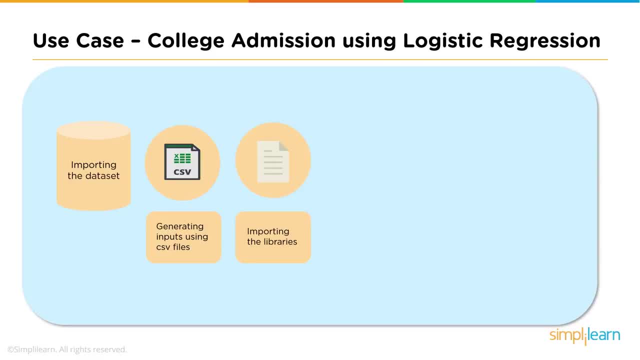 powerfully extended by the use of libraries and packages. Then we need to split the data set into a training set and a test set. It's important to note that the data set that we've imported, that we were given, has the GPAs and college ranks for several. 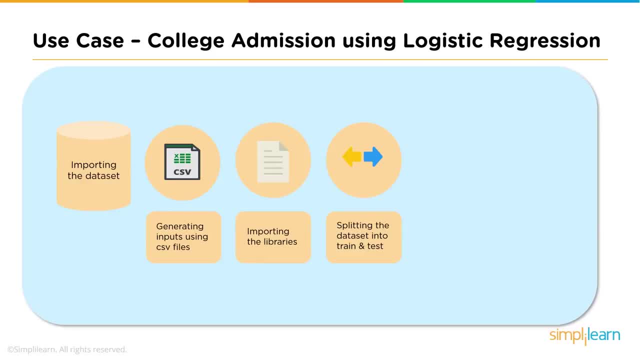 students, But it also has a column that indicates whether those students were admitted or not. So what we're saying is that the data set has the answers, And if you think about it, it must. How could we possibly train a model, have a model, learn, if we 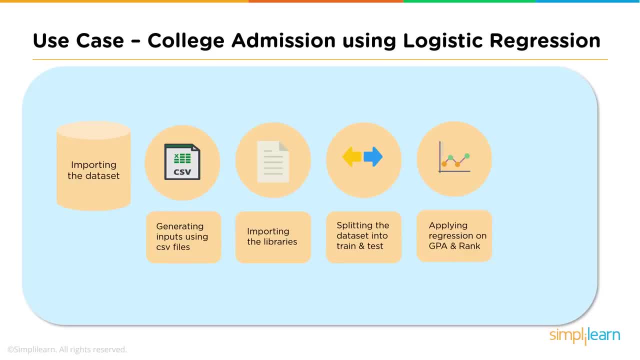 didn't know the answers already. That's why it's called machine learning. So we train the model and then we test the model. Once we split the data into training and test sets, we will apply our regression on the two independent variables, GPA and rank, generate the model and 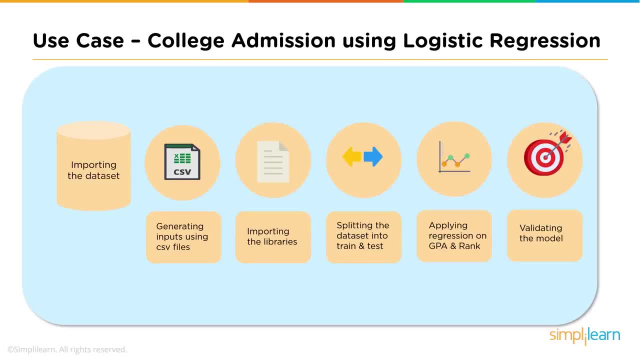 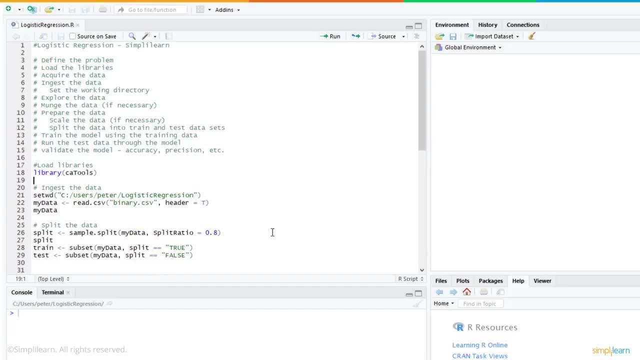 then run the test set through the model. Once that is complete, we will validate the model to see how well it performed. So now it's demo time. So here we have RStudio, my favorite IDE or integrated development environment, And I have a script already composed to run our 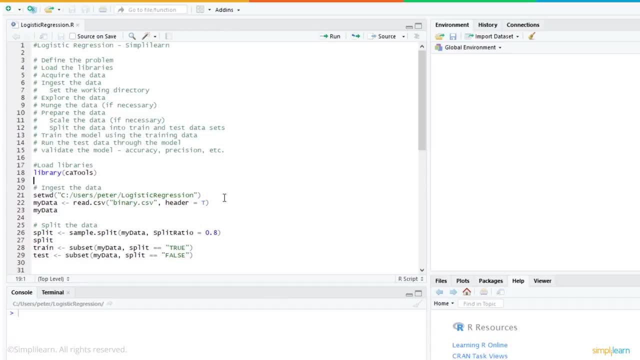 logistic regression on the problem at hand, which is our college admissions problem. So let's just walk down the script before I run it and talk about the various points in the script. So first define the problem. Well, the problem was defined and you really can't do anything in data. 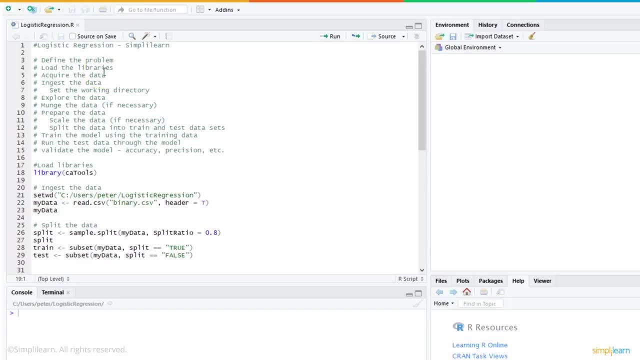 science without a clear problem definition. Once the problem is defined, you can load your libraries, acquire your data, set the working directory- In my case I'm on Windows- Explore the data, munch the data if necessary and then prepare the data, scale the data if necessary, split the data into train and test data sets. then 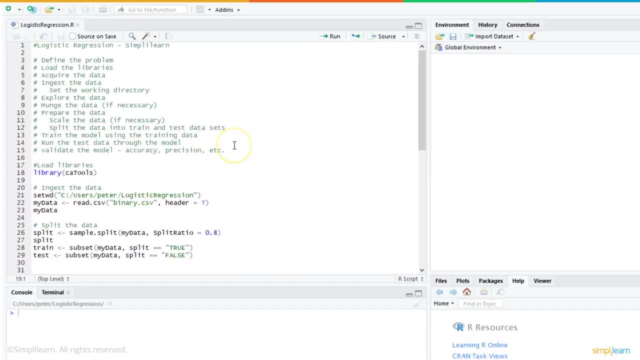 train the model using the training data and run the test data through the model and then validate the model for accuracy and precision, etc. So here we are, going to load our libraries. I'm going to use a package called CA tools And now that the library is loaded, I'm going to set my working directory And if I come over here to the 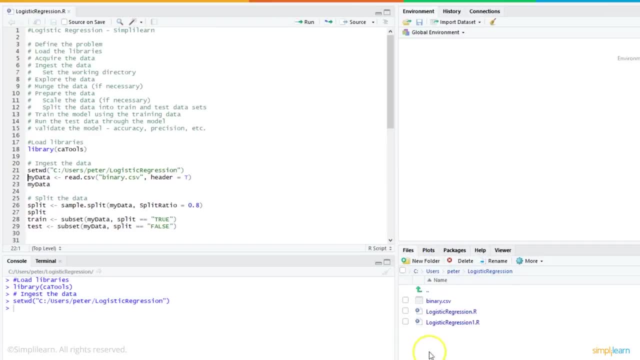 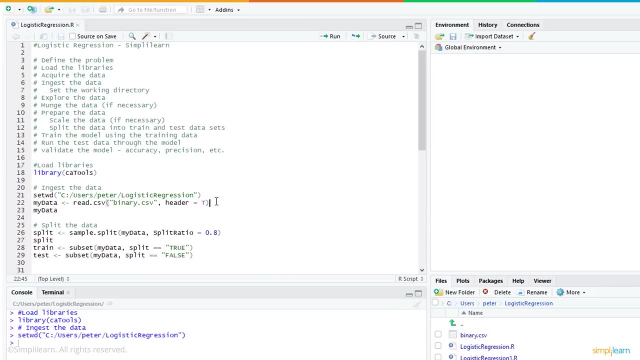 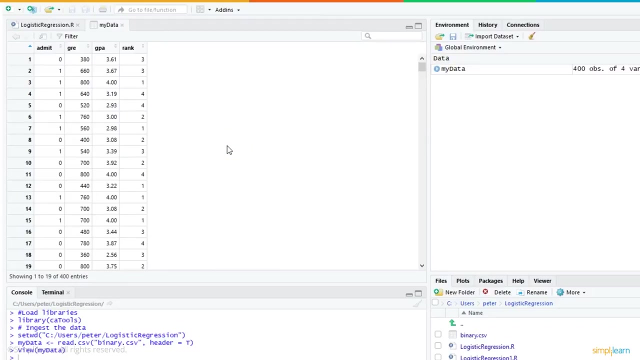 files tab, you'll see that there is my working directory. In that working directory there's a file called binarycsv And that's the CSV, the comma separated value file, that the college gave me. I'm going to adjust and then look at that data And, as you can see, it has four columns: GRE, GPA rank and then the 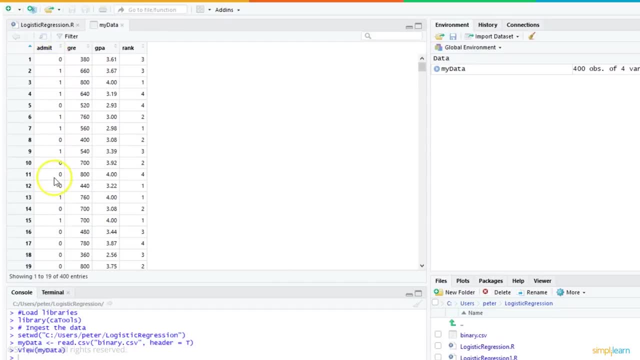 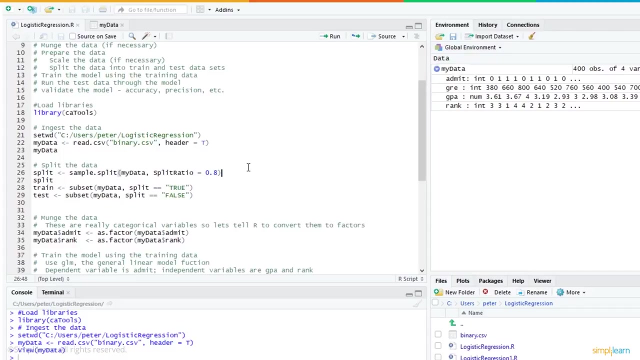 answer column: admit whether or not someone was admitted, which would be a one, or not admitted, which would be a zero. And if we come over to the right and we can look and see some of the first few values of each of those four columns? Now let's split the data. we're going to take this, my data frame, and split it into two a 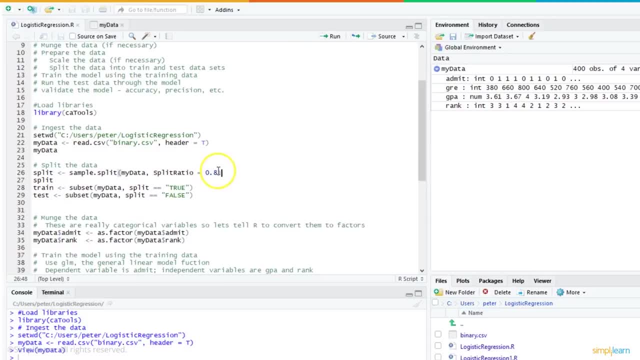 training set and a test set, And the ratio we're going to use is 80: 20.. So 80% of the data will go into the training set and 20% will go into the test set. Now that ratio could be 60-40, it could be 70-30. typically it really depends on the size. 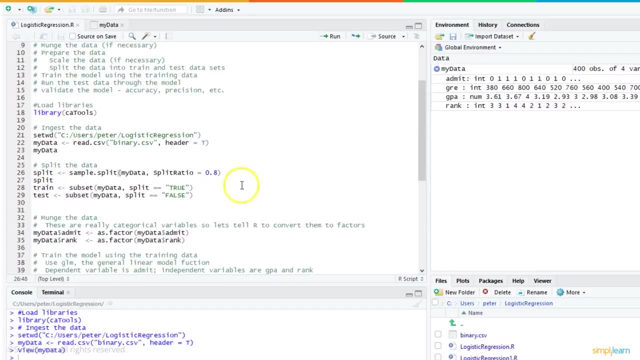 of your data, how much data you have. but this is for our example and for our purposes, 80-20 is perfect. next we'll do a little data munging. in general, you munch the data early on after ingestion and you really have to be careful in. 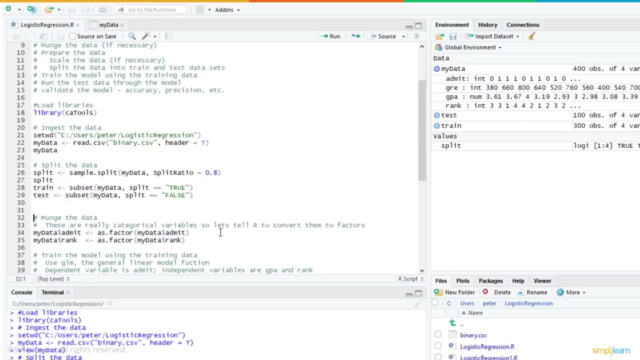 this case we don't have any missing values. we don't have any real outliers. our data was pretty clean when we got it and ingested it. but in general that's not the case and a lot of work and a lot of attention needs to be paid to the 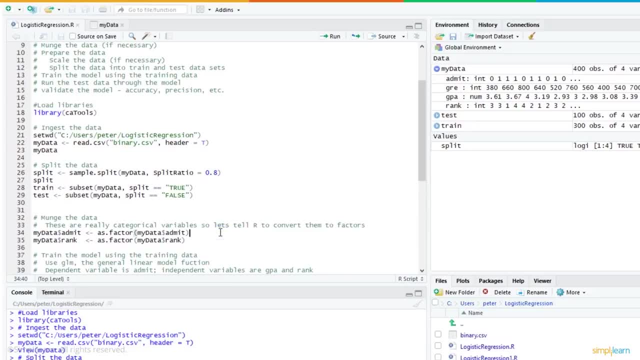 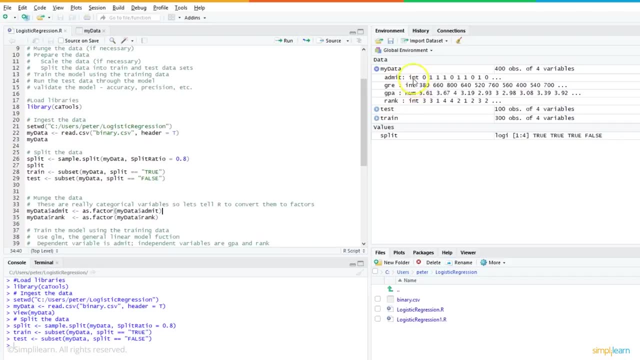 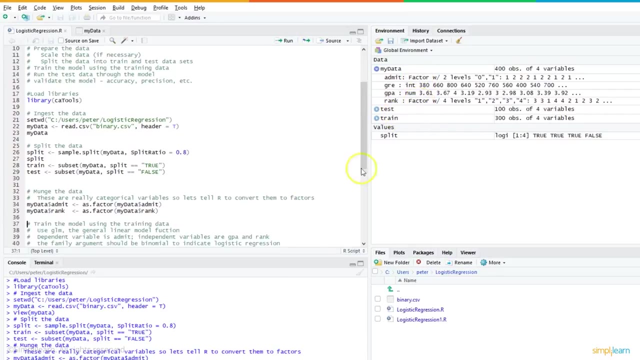 munging process here. we're just going to take our data- the admission column in the rank column- and convert them to categorical variables. right now they're integers, as you can see on the right hand side, and once I run these two lines they will be converted to factors and all the fun stuff we're going to use the 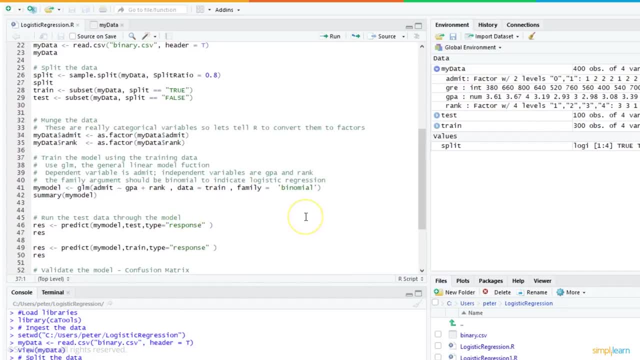 GLM function, the general linear model function, to try to convert the data into the actual data. and we're going to do that by training our logistic regression model. and the dependent variable is admit and the independent variables are GPA and rank. and the little tilde sign here says: 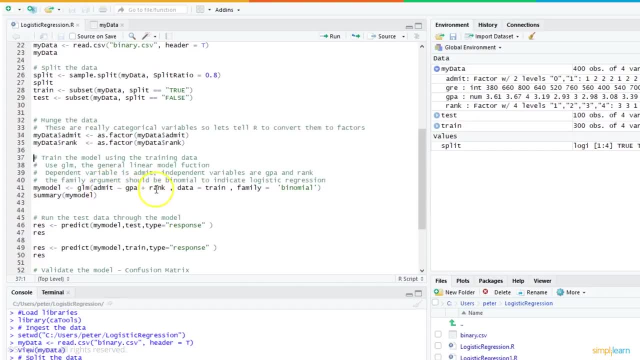 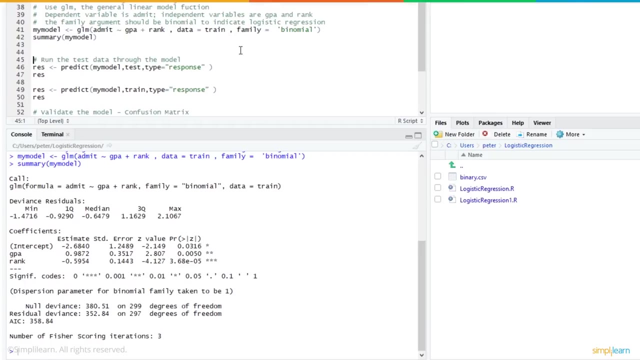 the dependent variable will be a function of GPA and rank the two independent variables. the data will be the training set and the family will be binomial, and binomial indicates that it's a binary classifier. it's a logistic regression problem. there it is. we ran our model and there's a 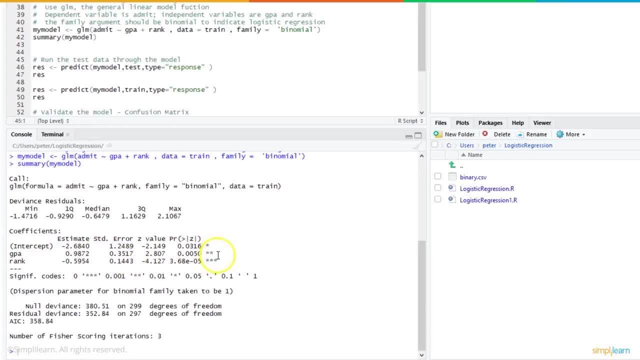 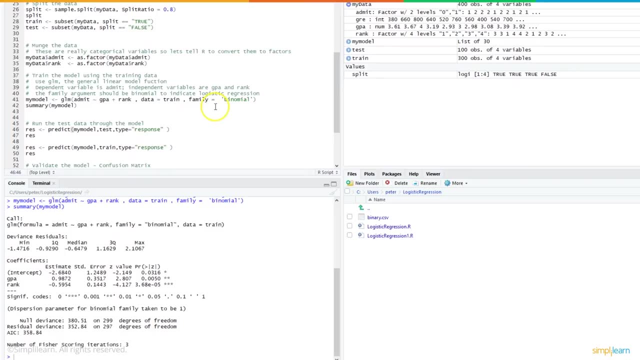 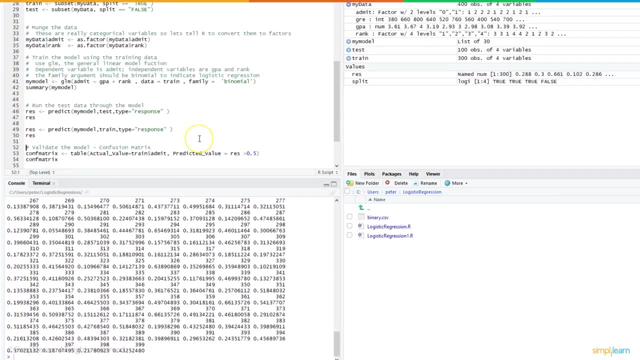 summary of our model. you can see that there is some statistical significance in GPA and in rank by the coefficients and output of the model. so next let's run the test data through the model and once we have done all that, we can now set up a confusion matrix and look. 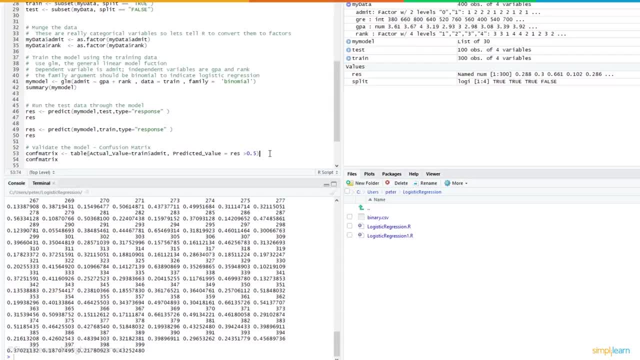 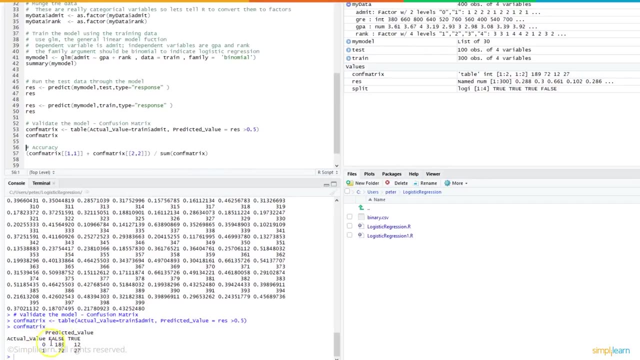 at our predictions versus the actual values. again, this is important: we had the answers and now we took and we predicted some answers, So hopefully our predicted answers match up with the actual answers. We'll run a confusion matrix, As you can see: the predicted values versus the actual values. 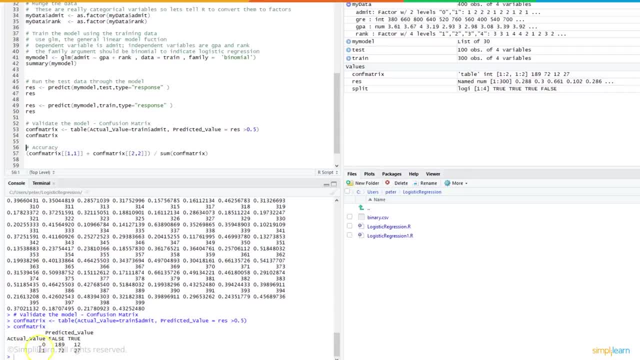 and it's important here to note that if it was predicted false and it was actually false, and we see 189, or if it was predicted true and it was actually true, which is 27, we did well on those. but there are a few that were predicted incorrectly. Some were predicted true but were actually false. 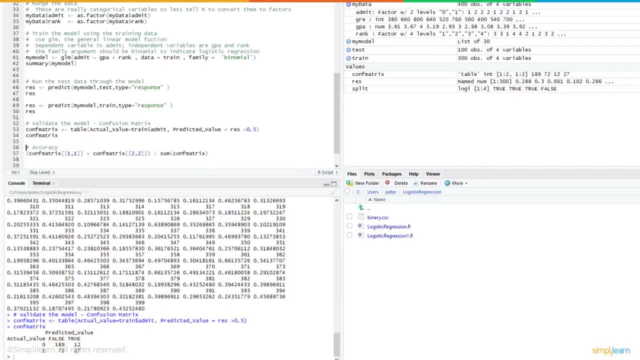 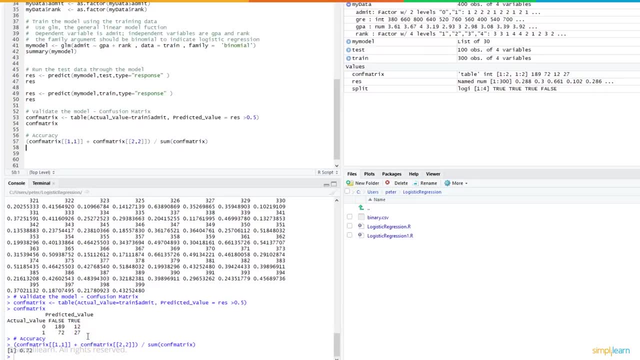 some were predicted false. that were actually true, and now we'll confirm what our percentage accuracy is: 72 percent- Not bad, but we could probably do better. How? We'll leave that to another video. What is a decision tree? And here we have kind of a new looking front panel of a car. 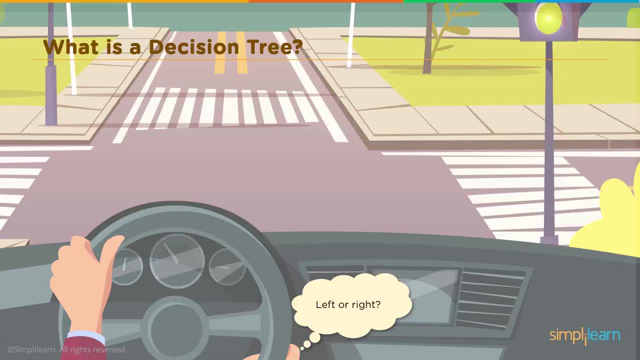 driving down the street and we have left or right, So you come into an intersection. you got to decide which way to go. Are you going to go left or are you going to go right, Wait or go? So do you go right away? We have a green light, so probably want to go right away. after you check for cross traffic. 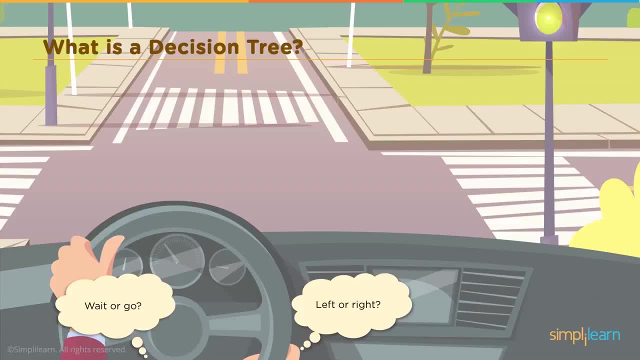 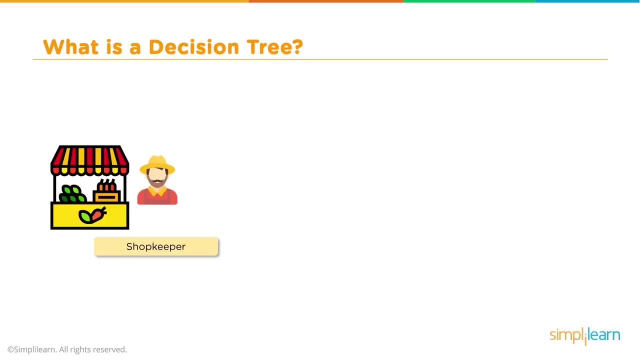 and make sure no one is asleep at the wheel or talking on their cell phone. Decision tree is a tree-shaped algorithm used to determine a course of action. Each branch of the tree represents a possible decision, occurrence or reaction. So another example is we have a shopkeeper very 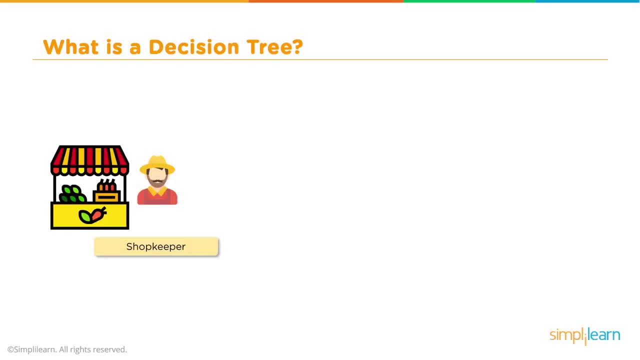 nondescript shopkeeper, kind of a little spooky, without the eyes. So we have a shopkeeper and he wants to organize his stall. So I must organize my stall, just looking around trying to figure out what the best way to stack all his goods are. and he has. 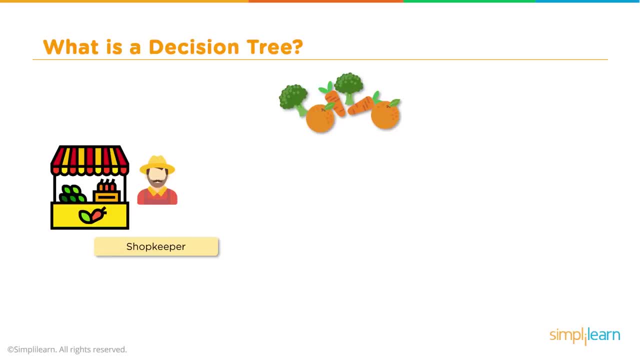 some broccoli, some oranges and some carrots. This is kind of a nice example, because we can see where some of the colors and shapes overlap where others don't, And so you can create a tree out of this very easily and say: is it colored orange? If it's not, well, it goes into one stack. Well, that happens. 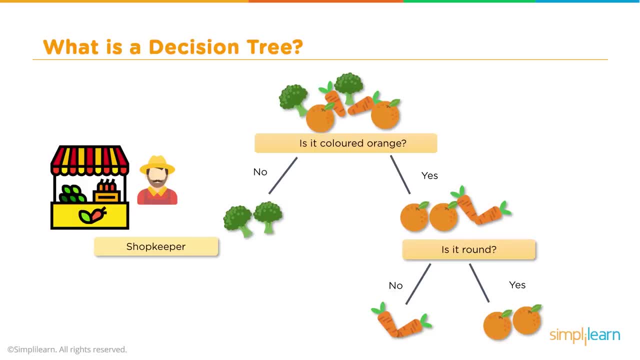 to be all their broccoli, And if it is colored orange, then it goes into another stack and you're like, well, that's still kind of chaotic. You know people are looking at carrots and oranges- a very strange combination to put in a box. So the next question might be: is it round? And if it is, then 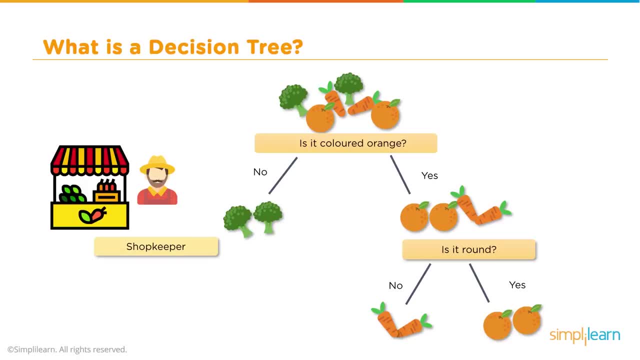 yes, You put the oranges into one box and no, that means it's carrots, We put it in the other box. And you can see that a lot of stuff we do in life easily can fall into like a decision tree. How do you decide something, You know? does it go left, does it go right, Yes or no? And even with this, 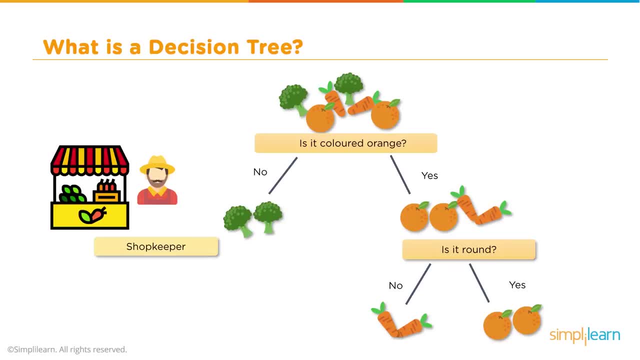 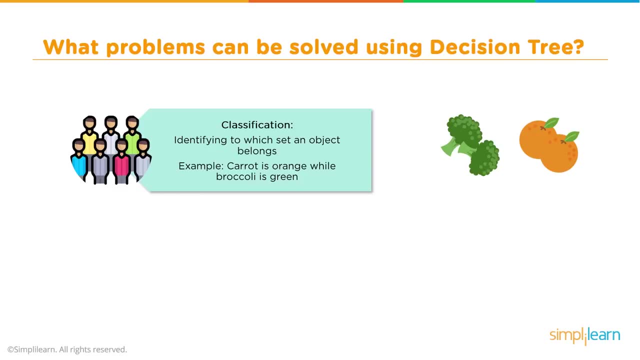 we even have a number of different end choices: Broccoli, carrots and oranges. So what kind of problems does this solve? What problems can be solved by using a decision tree Classification. We're dealing with the classification identifying to which tree the tree is going to be used. So if 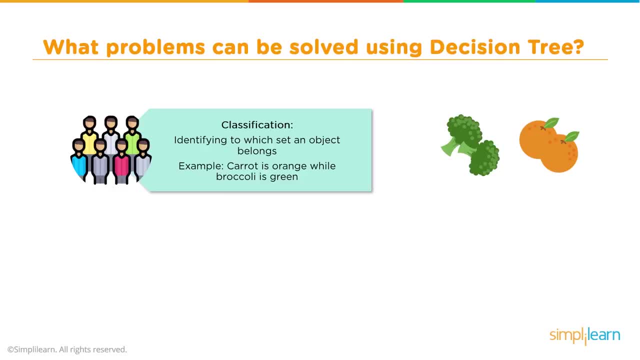 you're looking at a fruit set an object belongs And from our example we just looked at, a carrot is orange while broccoli is green. I guess it's nondescript day. It's kind of without the faces. I love it Because a lot of times you're looking at data you really don't want to know what exactly. 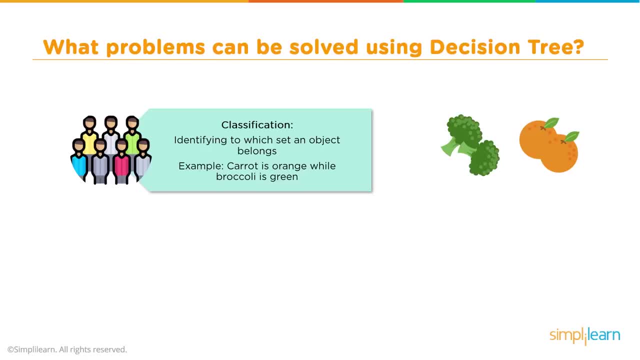 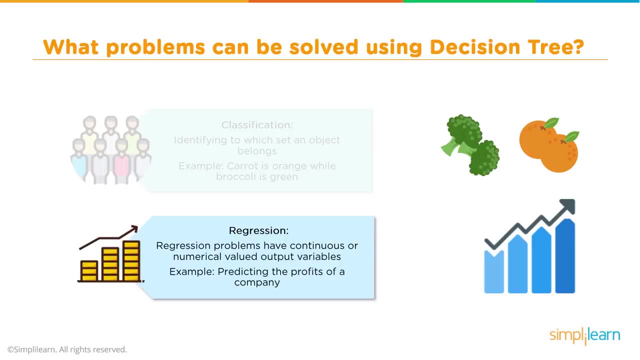 the data is, but you're sorting it. So you know like this kind of represents data that you really don't know exactly where it's coming from. Just kind of a fun thing. Regression: Regression is another problem that can be solved. Regression problems have continuous or numerical valued. 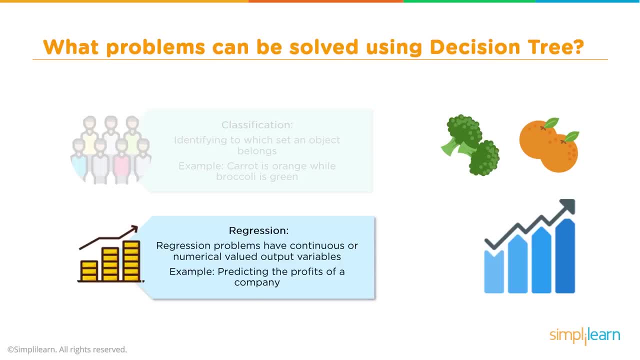 output variables. Example: Predicting the profits of a company. So we have two different primary problems we solve for, We solve for classification- Is it green or is it orange- And we solve for regression, which is a continual number. So you know if you're doing stocks this would be a dollar value that ranges. 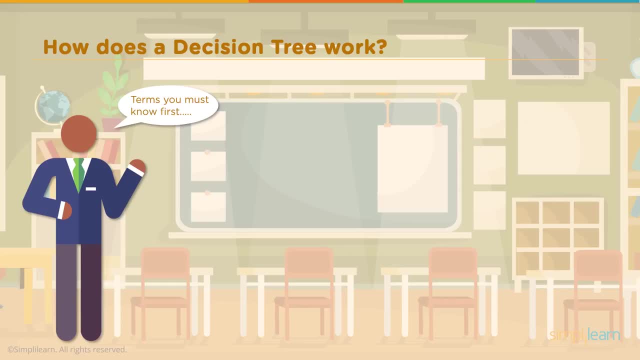 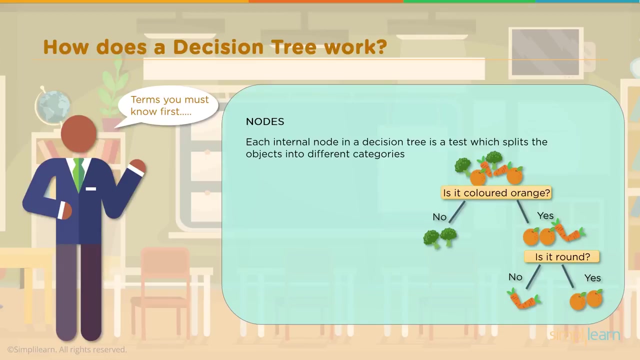 anywhere from zero to thousands of dollars. How does the decision tree work? Terms you must know first. So before we dive into the decision tree, let's look at some of the terminology for the decision tree. We have notes. Each internal node in a decision tree is a test which splits the objects into different categories. 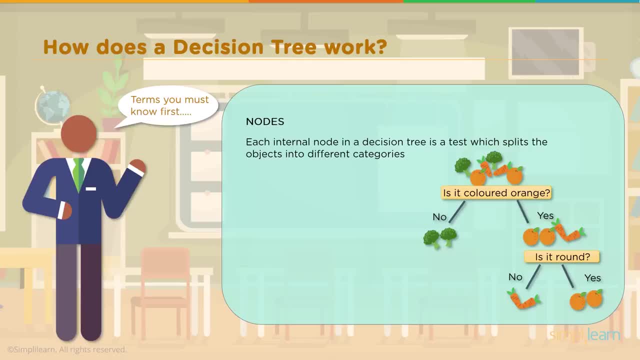 And continuing with our vegetable stand example, we have broccoli- No, it's not orange- And oranges and carrots are, and so on. So you can see right there where it splits. that's a node where the oranges split and the carrots split into each of their own groups, And each one of the splits is a 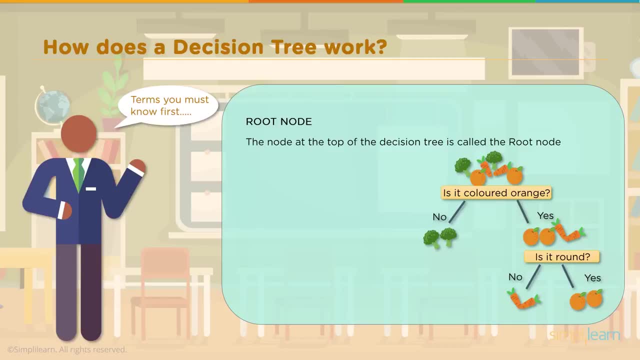 node, The very top node of the decision tree, is called the root node. So the very first one we started off, where we split, it is a colored orange And you can see that pointed out nice and neatly there. this is a root node at the top Each external. 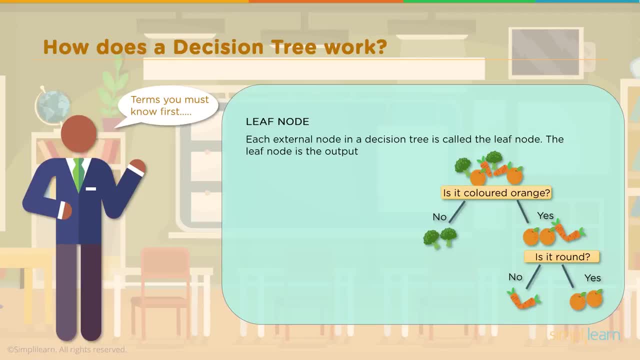 node in the decision tree is called the leaf node. The leaf node is the output And you can see down here we have our broccoli, we have our carrots and our oranges. Each one of those is a leaf node. So, to quickly rehash our terms, we have: anywhere there is a split, that's a node, and if it's at the very top, 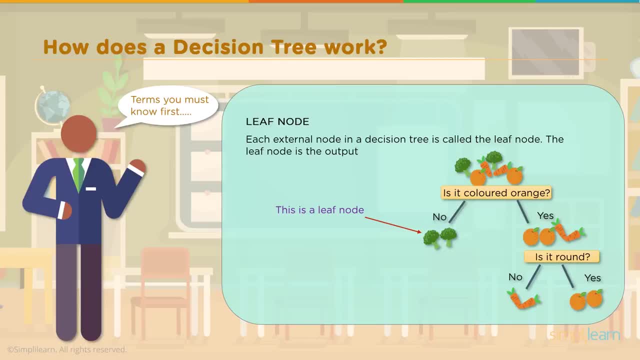 of the tree. that's the root node. And if you're at the very bottom of the tree, we have a final answer: that is the leaf node. so you have a root node, a leaf node and then everything else is just a generic node. so one of the most important terms or concepts that powers 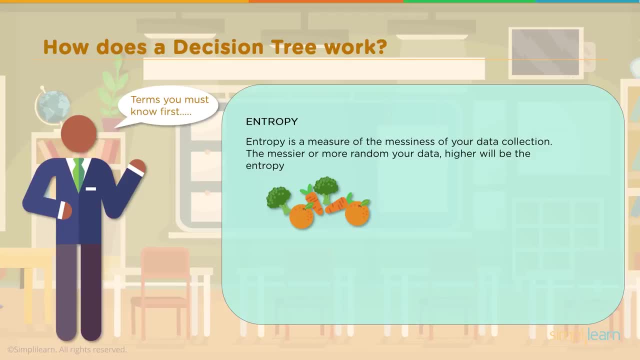 a decision tree is entropy. entropy is a measure of the messiness of your data collection. the messier or more random your data, higher will be the entropy. so we can see: here we have broccoli, oranges and carrots are all mixed together and it's very chaotic and you could say this collection has high entropy. and if we 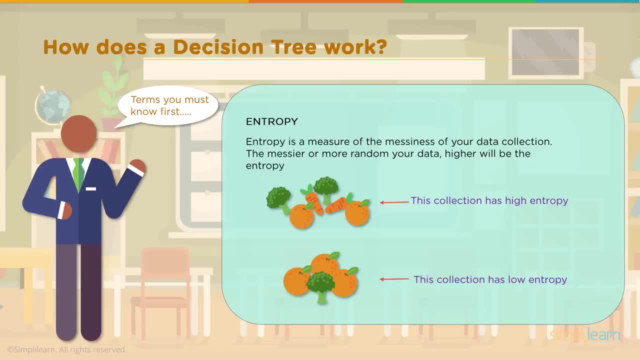 sort out the carrots out of here and I guess just one of the broccoli. I don't know where the other broccoli went. you could save it if you have just the oranges and the broccoli. this is a lower entropy. they say this collection has low entropy, but really it's higher and lower. one is higher or lower than the. 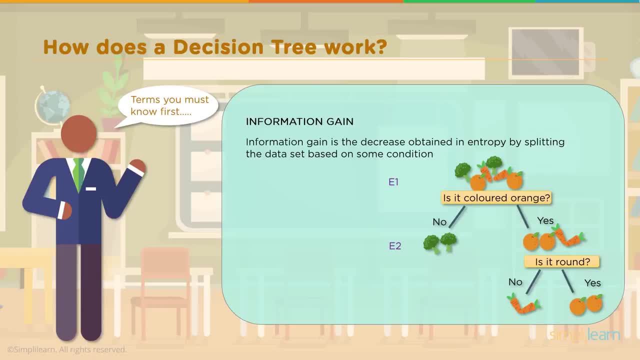 other one, and from entropy we get information, gain information is the decrease obtained in entropy by splitting the data set you based on some conditioning, so we have our information, one which we can actually there's actual computations, and so we have our e1, which is put in there for our entropy. 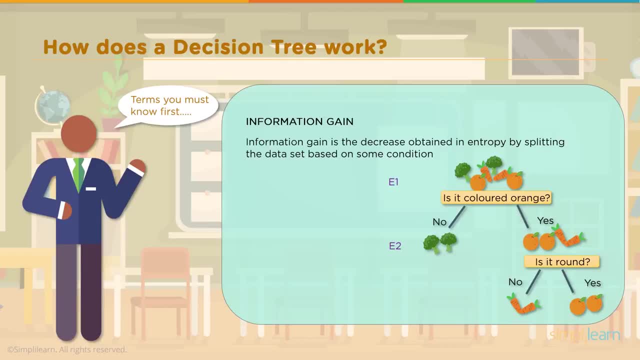 value at the base node, a root node, and we have two, a two which is a leaf node, and so we can actually calculate those calculations for entropy and we actually look at those two values, the entropy and we take that we have e1 is greater than e2. therefore the information gain equals e1 minus e2. so here we have another. 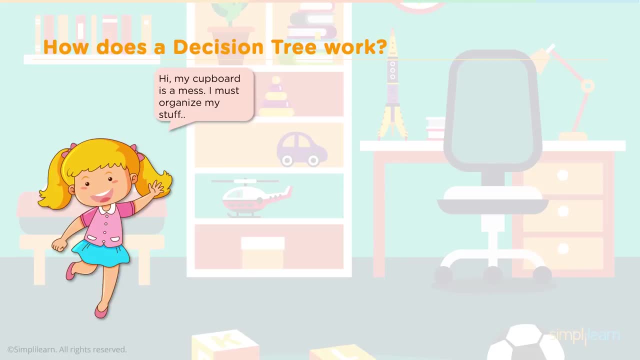 example, we're actually going to attach some values to this one in just a moment. so we're going to add in some value values to this one and we're going to add in some values to this one in just a moment. so we're going to to move away from the fruit and we're going to go to everybody's favorite thing: organizing a. 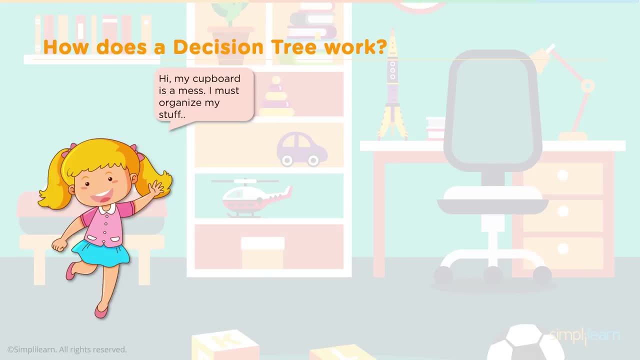 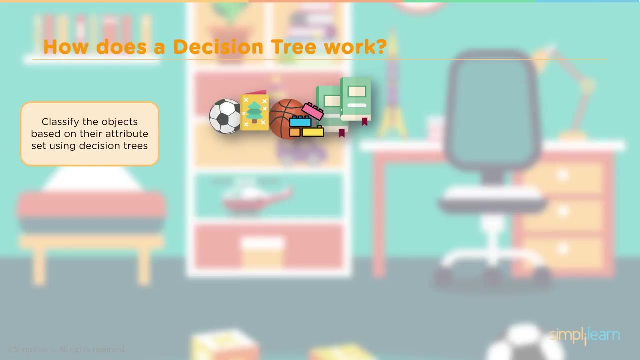 child's closet And here we have a young lady waving at us: hi, my cupboard is a mess. I must organize my stuff And we're going to classify the objects based on their attribute set, using a decision tree. We can look at it. we have a shape, a size and a label and a number, And I'm going to. 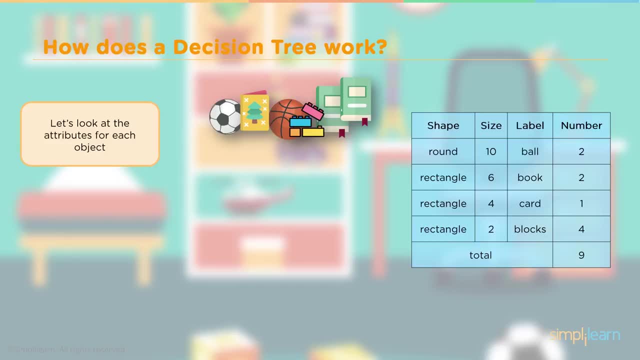 go ahead and look at the labels, because that's really what's key on this one is we have a couple balls in here- some books, cards and blocks- And if you look at that, when you have something that's a ball, it's round, so it's a very different shape. The book card and blocks are all rectangular. 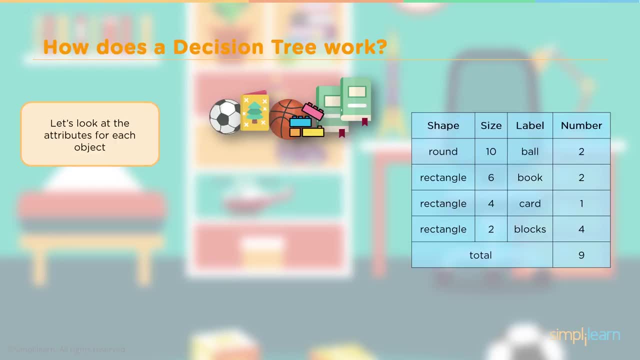 but the books are a different size. So the books have like a size six. I guess you think of them as very large. Cards are size four, so they're not quite as big, And the blocks are little lego blocks. that looks like kind of fun to stack on there And then we can actually quantify this and we can. 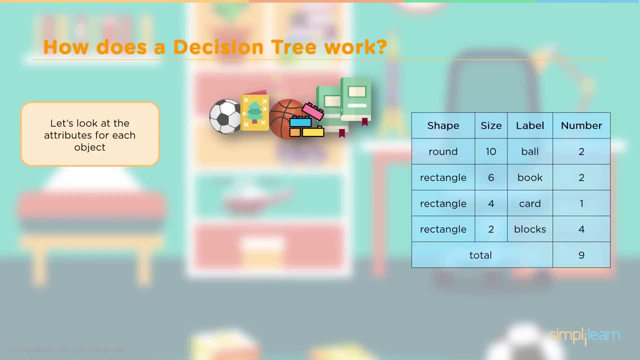 actually say, hey, we got. we have different numbers, We have two balls, two books and we have three books, one card, four blocks, And we split at each level based on certain conditions, on the attributes. So splitting aims at reducing the entropy And we have a formula, our first actual 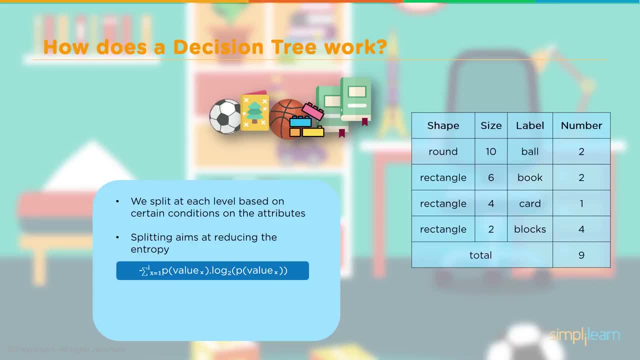 formula that you'll see happens in the background when we're running these different modules in R And it looks a little complicated. but we can break that up and simplify that for you. So we see this formula: the negative sum of i of x equals the probability of one value of x times the log of two. 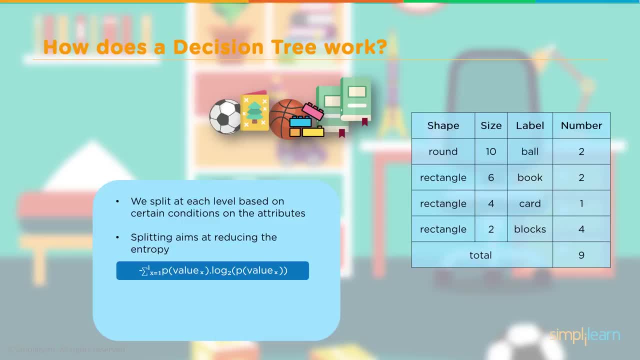 probability, The term probability, value of x. it's probably easiest to understand if we go ahead and put the numbers in there, So you can actually see what we're looking at. And so we plug the numbers in there. We look at the probability of the value of x. Well, if we do, the number of balls there's. 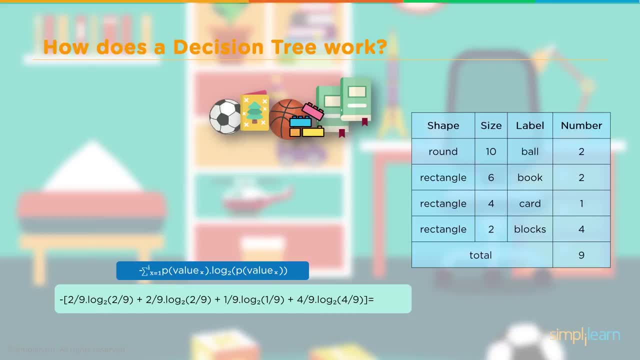 two balls and the total number of items is nine. So we have a probability of any one object being two out of nine. So that's pretty straightforward math. When you look at the numbers, you can actually see that very easily, And so we can calculate our entropy of. 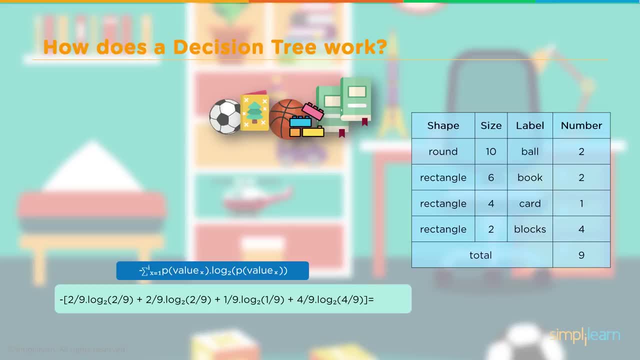 two over nine times the squared log of two over nine plus one. ninth, the log squared of one over nine plus four over nine times the log squared of four over nine. So our whole group is the sum of all the entropies, And so when we look at that, we have the entropy of the balls, which is the two. 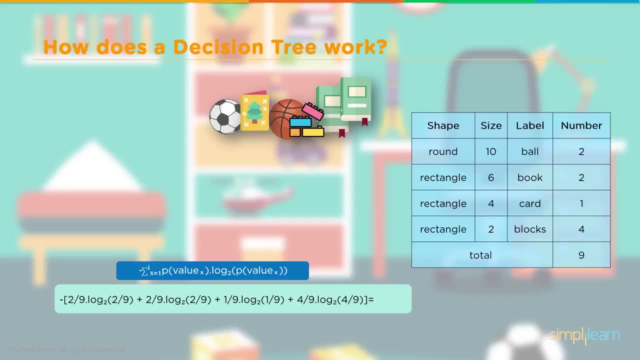 over nine, rectangles two over nine, or I mean books two over nine, cards one over nine and the blocks four over nine, And we can just plug those numbers in there and we get an actual value of 1.8282.. So what the heck does a module do with that number? Well, now we must find the conditions. 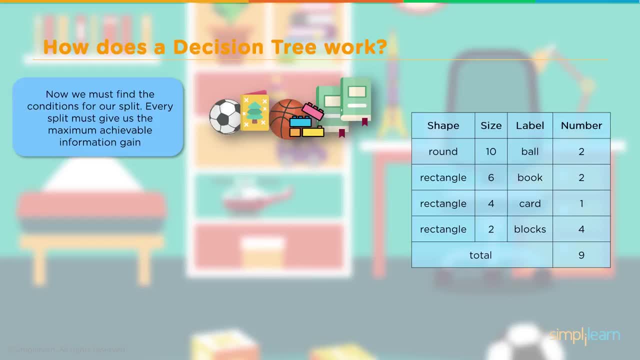 for our split. Every split must give us the maximum achievable information gain, And so we have our first entropy value: 1.8282.. And it turns out: when you compare all the different individual entropy values for the balls, for the books, for the cards, for the blocks, rectangles, you find: 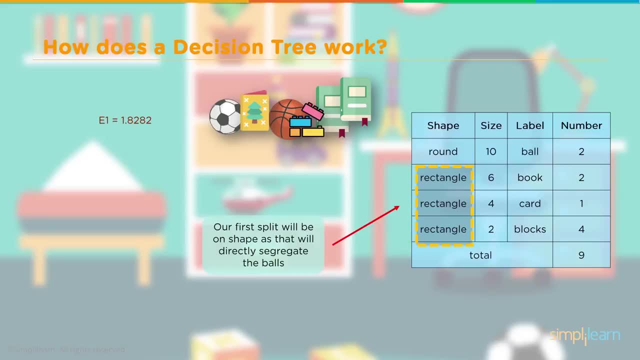 out that the biggest split is going to be in the shape, And it's going to be in the shape of the books, And it's going to be our first split will be on the shape. that will directly segregate the balls out, So they'll split up a huge group from one from the other, And so we compute, that we end. 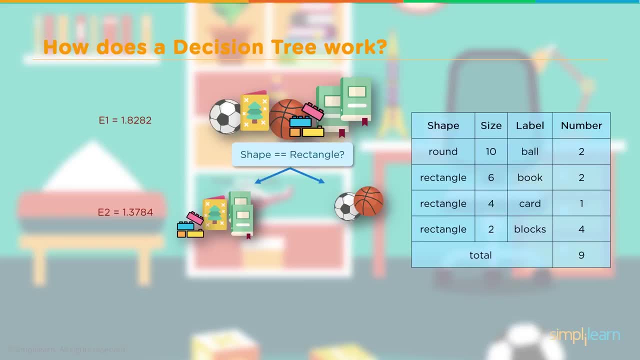 up with E2, which is all of our rectangles, And then we have a leaf node which is the balls, And so with our E2, we see that 1.3784 is much less than the 1.8282.. And so our second split will be: 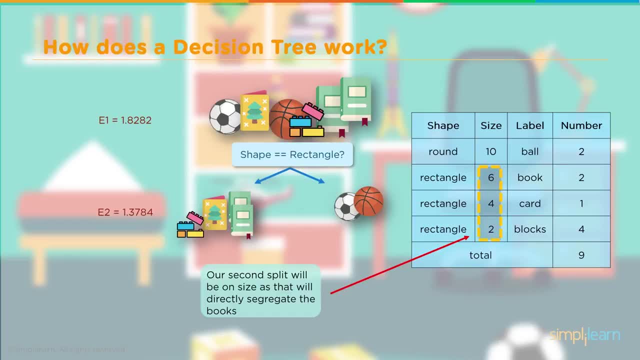 on the size is that will directly segregate the books, And so when we do that, we can see that if the size is greater than five, all the books go to one side, while the cards and the blocks go to the other, And again we have our E3,. 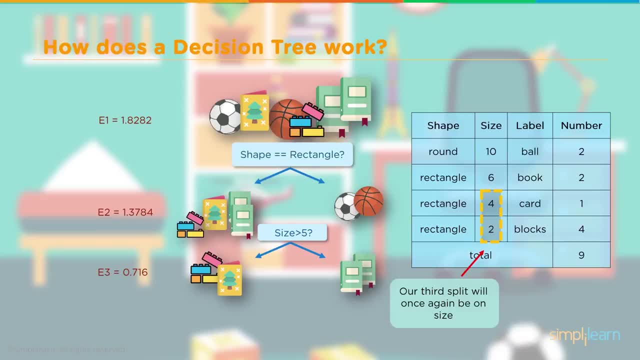 which equals 0.716,, which is considerably less than 1.3784.. So our entropy is dropping each time we do a split. And, of course, our third split we look at and we'll see that we're left with size again And 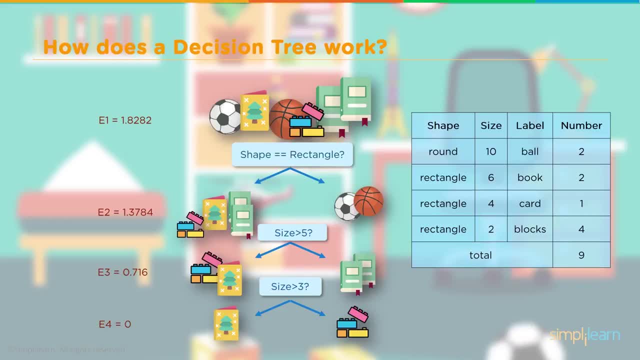 we'd split it with four and two In this case. if it's greater than three, it's going to be a block, If it's less than three, it's going to be a card, And at this point each of our objects is looped. 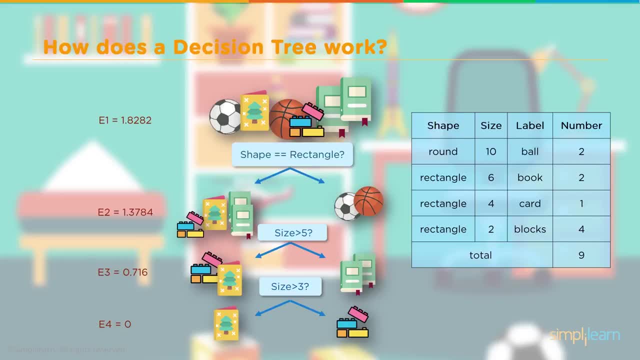 into a single block. And then we have our E3, which equals 0.716,, which is going to be a block, And similarly, so they all look the same and we end up with an entropy of zero. And so you can see, as we go down, the entropy continues to get less, And because it hits zero, 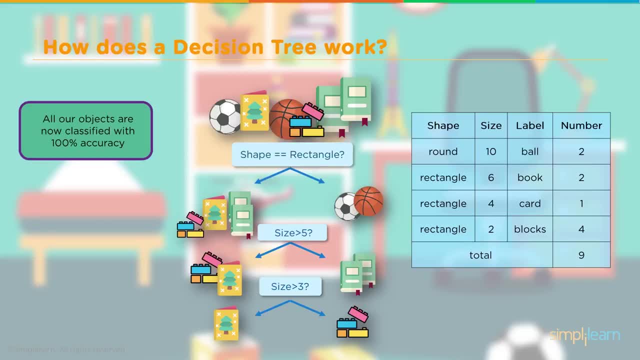 we can see all our objects are now classified with a 100% accuracy. if it was only that easy to clean the kids' closets And you can see, we have a nice drawing that shows you where all the leaf nodes are in this, in which case we have the balls, the books, the blocks. 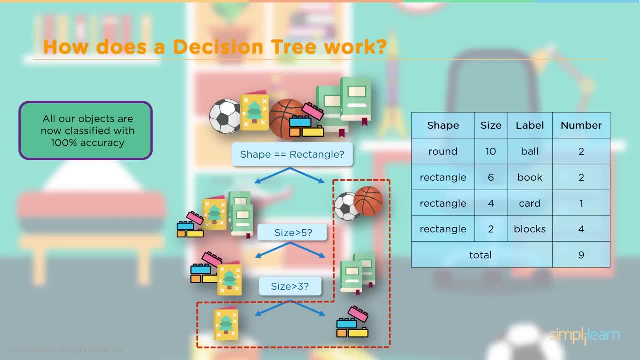 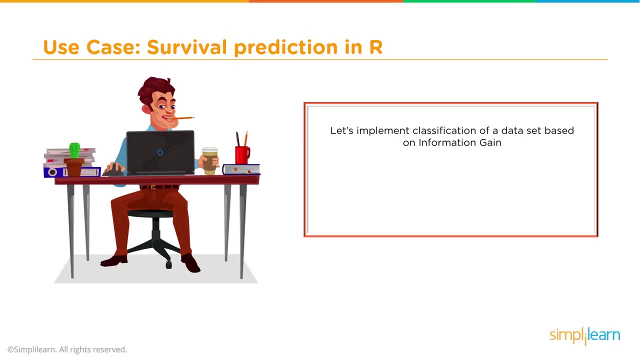 and the cars are part of the leaf node And the root node is our first split and we have all the objects and we're splitting them by a rectangular shape. So we're going to dive into the use case and in this case we're going to get a little morbid. 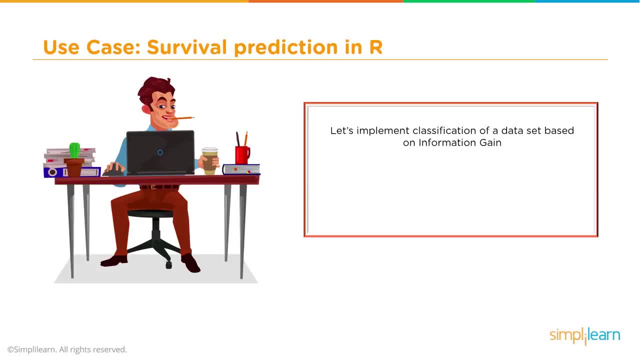 There I am behind my desk. That's definitely not me. I don't have that big of a chin, But I do usually have a cup of coffee and it looks kind of like that. It's sitting next to me on my desk. 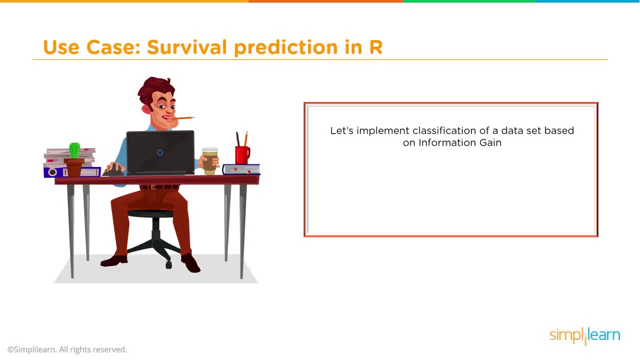 So the use case is going to be survival prediction in R and let's implement a classification of dataset based on information gain. This is going to use the ID3 algorithm. Don't let that scare you. That's the most common algorithm they use to calculate the decision tree. 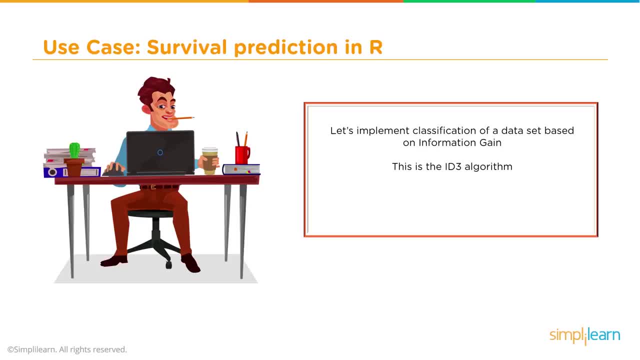 There's a couple different ways they can calculate the entropy, but the formula is all the same behind it. So ID3 is most common in R And then we'll be using the RStudio for our interface, for our IDE. So RStudio is free to download. There's the free version. 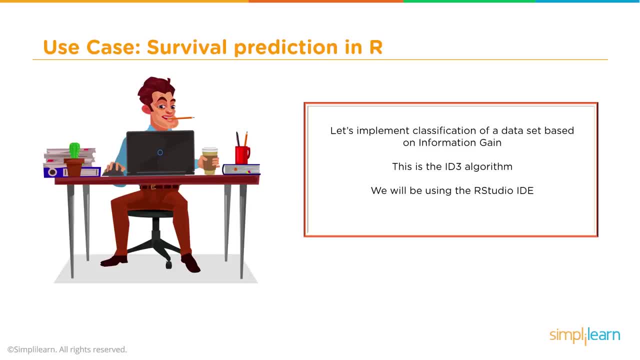 Of course there's an enterprise version and there's all kinds of different choices in there. But one of the wonderful things about R is that it's been an open source for a very long time and it's very well developed. It's also very quick and easy to use on a lot of things. 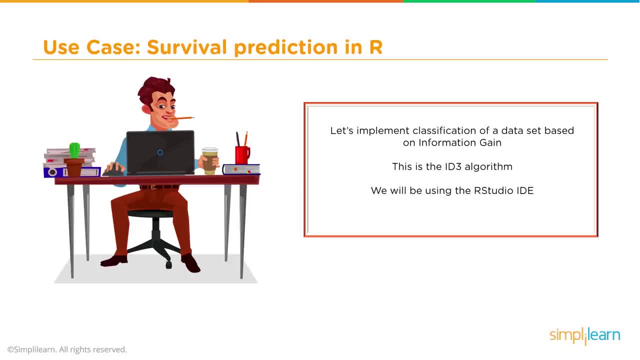 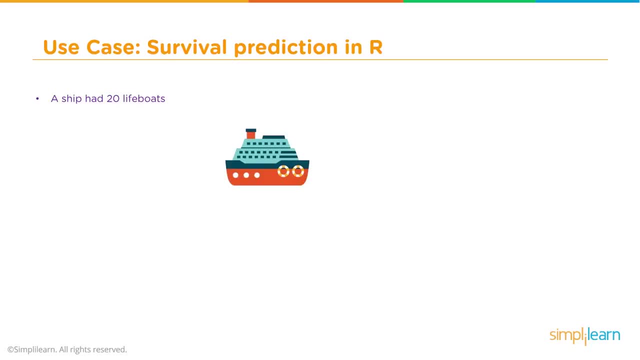 So this is going to be in the RStudio IDE. There's some other interfaces, but this is, I would suggest, using the RStudio. It's the most common one And, if you remember, I said this is going to be a little morbid because we're talking about how many people survived and died on these ships. 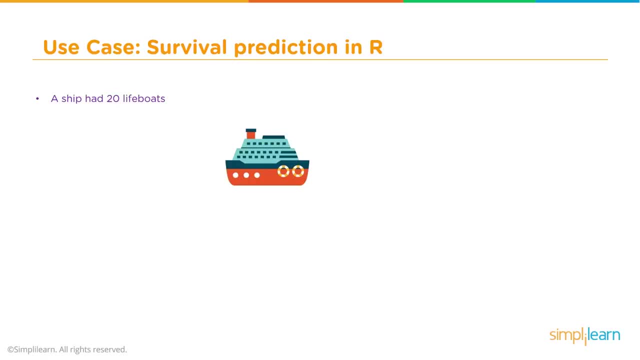 So in this case we have a nice vacation cruise ship going on there, or I'm not sure what that is with the tugboat. So we have a ship and it had 20 lifeboats. The lifeboats were distributed based on the class, gender and age of the passengers. 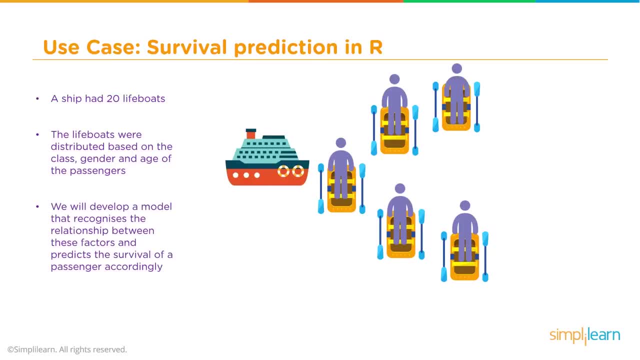 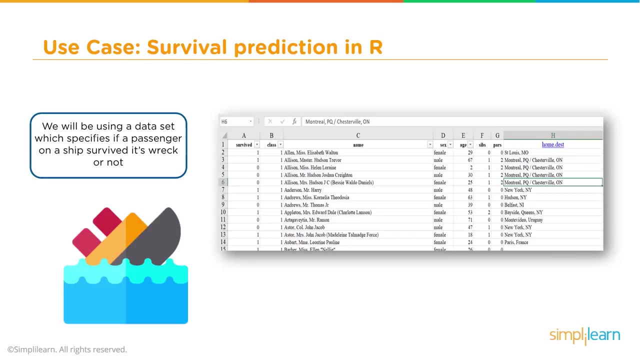 We will develop a model that recognizes the relationship between these factors and predicts the survival of a passenger accordingly. So we want to predict whether the person is going to survive or die in a shipwreck, And we'll be using a data set which specifies if a passenger on a ship survived its wreck or not. 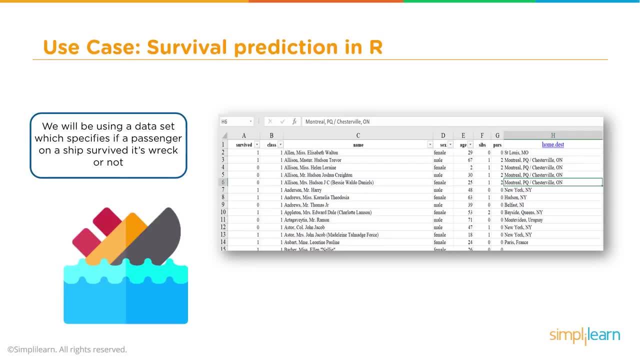 So we're going to look at this data and if you open it up into a spreadsheet- and don't forget- you can always put a note on the YouTube video down below And we will be monitoring that and you can request the data set sent to you. 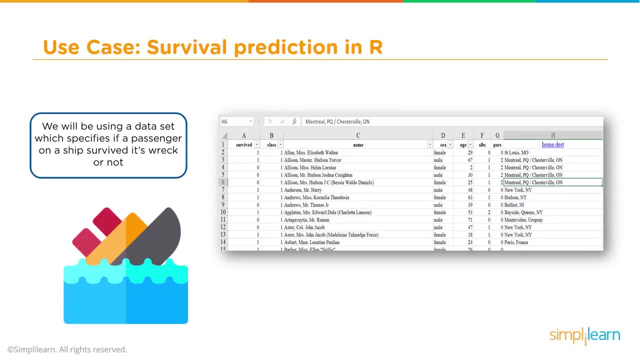 or more correspondence. You can also go to wwwsimplylearncom and request this data set too, And it's just a simple CSV file. we'll send out And you can see right here: we have survived. So one indicates a person survived the wreck. 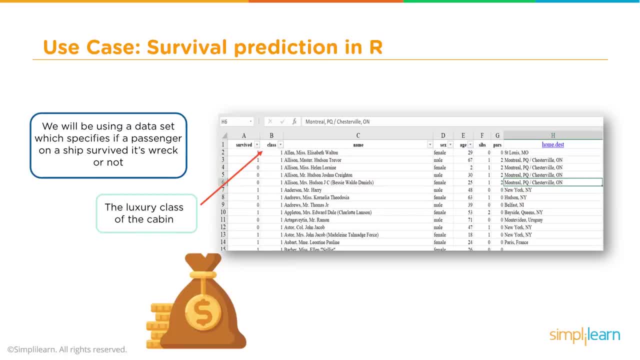 Zero, they didn't make it, They were under the water And the luxury class of the cabin. So if they were in, you know what value is like: one, two, three, depending on what luxury class they were. And then we have- this is kind of interesting- how many siblings they had. 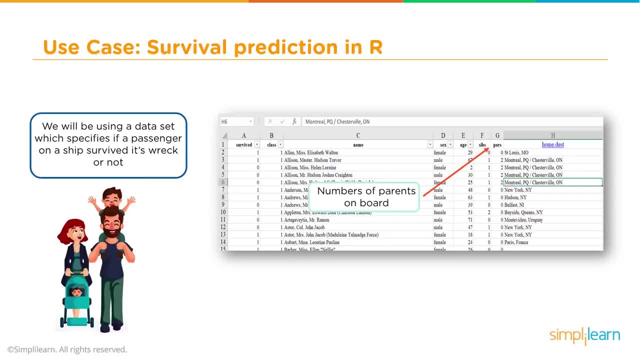 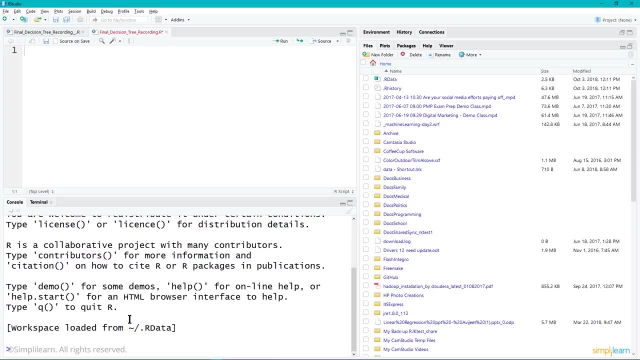 So it's kind of an interesting added statement. It's a statistic in there: Number of parents on board And disembark location, So where the destination is. So here we've opened up RStudio And if this is your first time in RStudio, you'll notice that it opens up standardly in three panes. 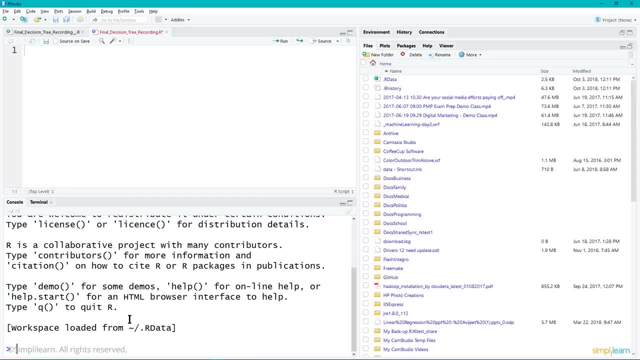 The upper left is for text documents you're bringing in, And then the bottom left is the actual commands as they're processed, And then on the right-hand side you have your environment set up on there. Now I've zoomed in with my font a little oversized. 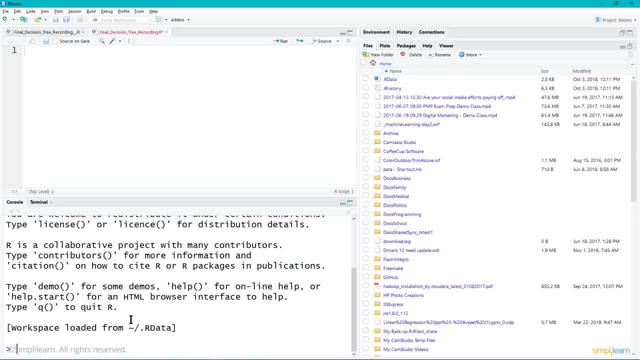 In fact we can even take a look, Take that up one more size and see if we can get a larger setup view. Here we go. So I've set the font for 18.. Probably a lot larger than you need to work on a project. 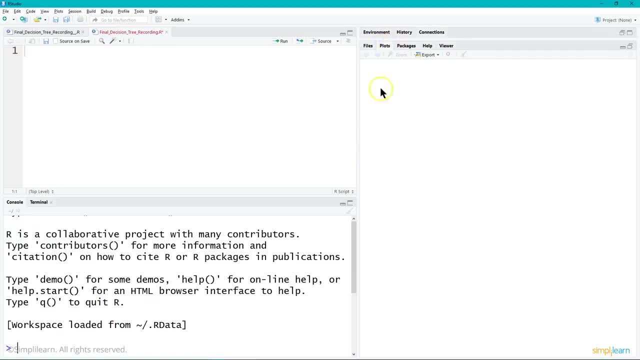 And the first thing I'm going to do is, on the right-hand panel we're going to be working with plots, So I'm going to click on the little plot tab up there And I'm just going to collapse that over to the side for right now. 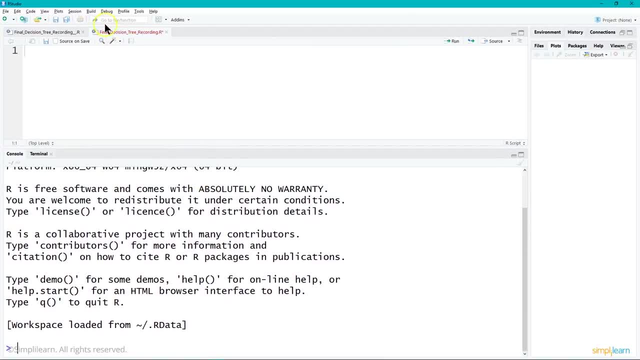 And then I'm going to open up the bottom one And you'll see, on the top I actually have two different tabs. Team in the back was really nice to set up the whole package for what we're working on here And we'll go through this line by line. 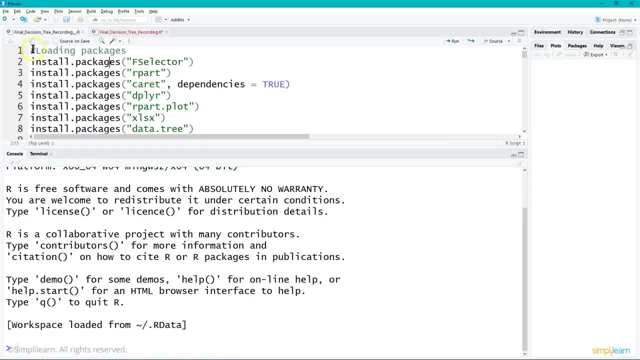 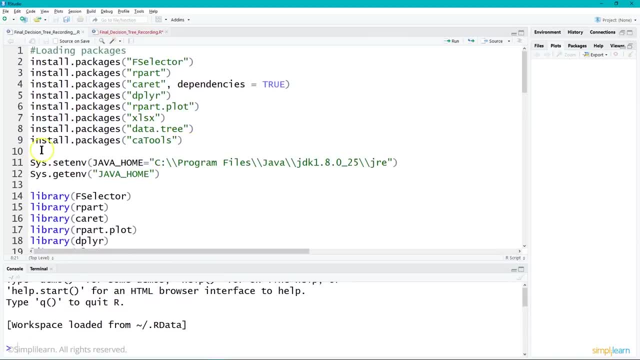 And then you'll see as we execute. the different lines are going to appear down below, So I'll be flipping between these two left panels, And let me go backwards just for a second here. We're going to do this part, So let's take a look at the installs. 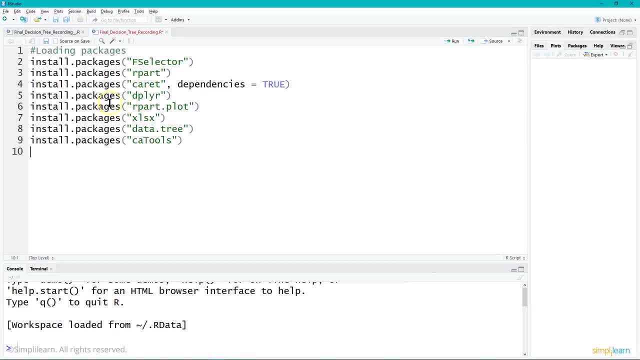 And if you look at the installs- and I'm not going to actually run the installs because I've already run them on my computer, So these are already installed in my R packages and I don't have to rerun them- We have a number of packages we're bringing into R because that's how R functions. 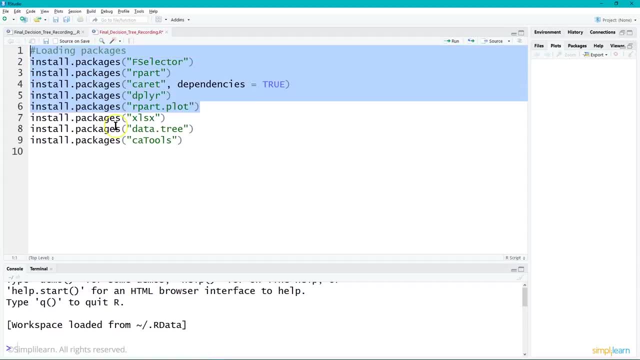 And the first number of packages are all part of our decision tree. So our F selector, our R part, our caret with the dependencies, equal true- and our DPLYR and our R part plot- Ooh, that's a mouthful. 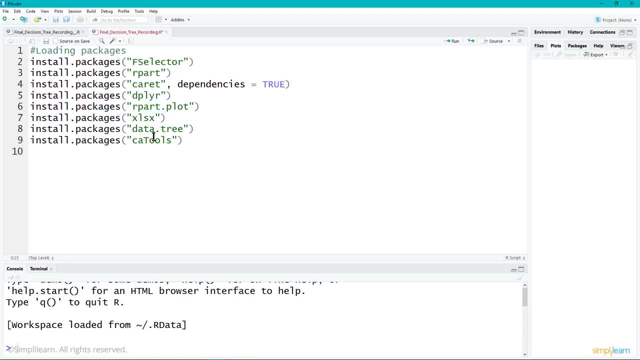 You'll need to import all of these in your setup And the first one, which is your F selector, computes your chi, squared your information, gain your entropy. All of those formulas are a part of the F selector, So when you bring it in, that's what that package is. 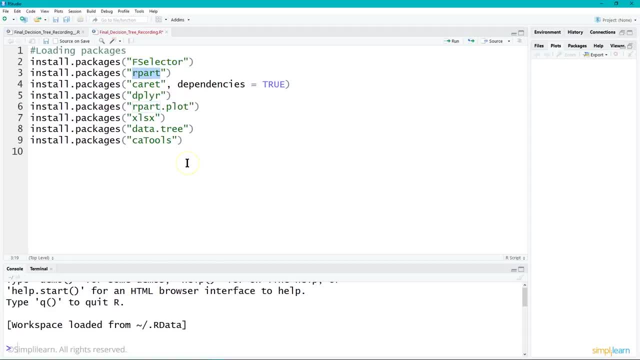 The R part is your partitioning of your decision tree. So these are your primary two decision tree modules that we're bringing in. The caret is a part for actually splitting apart the data, because we always want to do a test set, a train set. 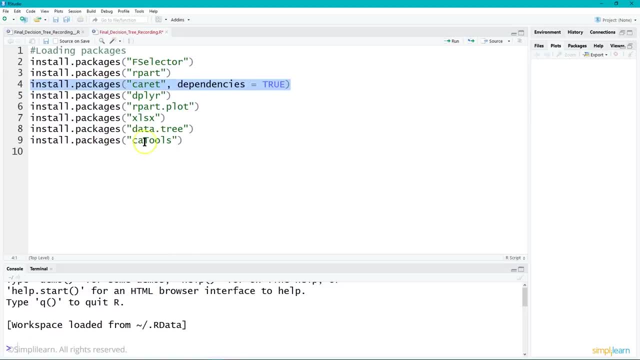 So they built a package, caret, to kind of handle all those. You'll see caret used in a lot of other machine learning packages. when you're doing the R, The DPLYR is for mutating your data, so you can sum it and classify it. 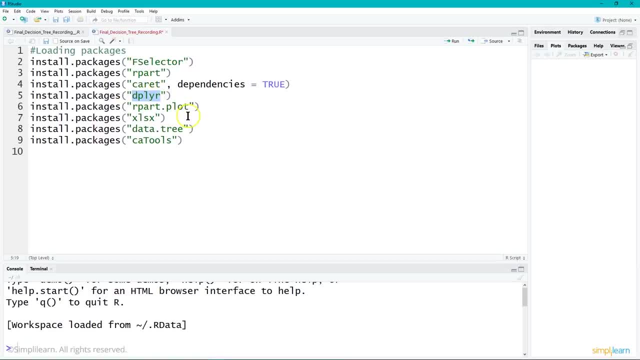 You can filter it. That's all part of the DPLYR And then R part has another piece called plot And that's for helping us plot the data as we sort out the tree, because the R part creates the tree, but you still want to be able to plot it. 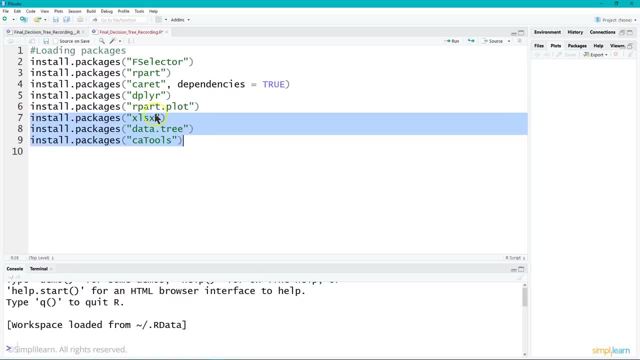 And then we come down here and we have some additional tools. We're going to work with a spreadsheet. This is a Microsoft Access spreadsheet, So we're going to use the XLSX package to import it, And you might think that's a little outdated, because I know when I'm doing any new projects. 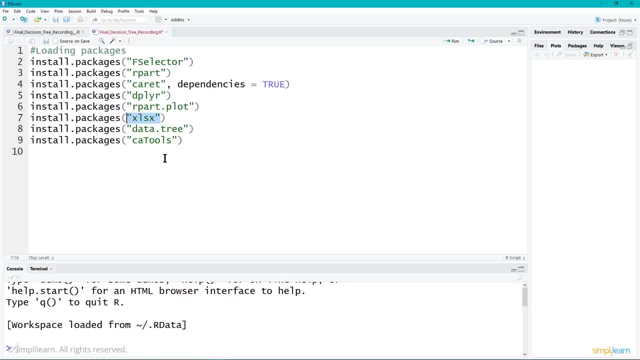 I try to save it. I save my data into a comma-separated variable file or something more standardized. But a lot of times you'll end up with these old databases where they're exporting data and their export comes in an Excel spreadsheet And guess what? 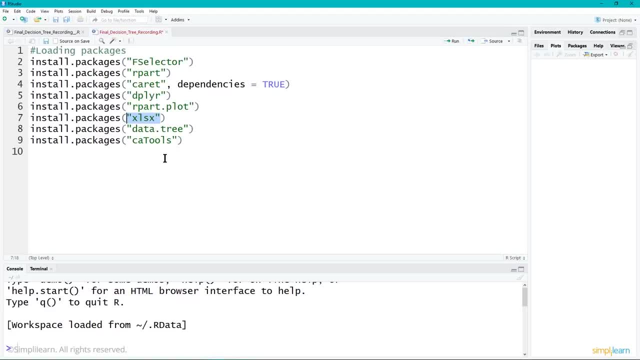 This is a time saver: Instead of opening up the spreadsheet, resaving it as a comma-separated variable file, you can just open it right up in R, which is really nice, And then we have our data tree, which goes right along with displaying the data. 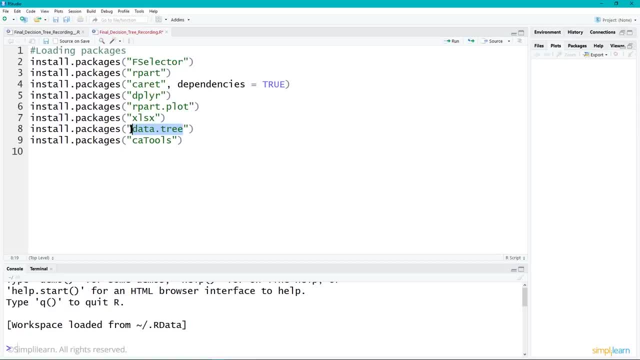 So we have our rpartplot And we're going to put that into the data tree, so we have a nice visual. And finally, you need to install the package caret And we're going to install the package catools. And catools is another package used for general manipulation of your data and your vectors. 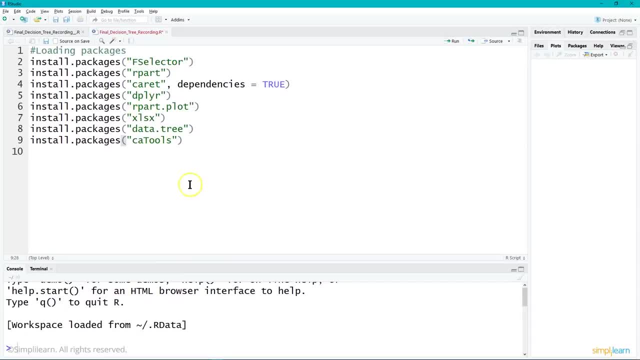 So it also has a split function for training data. I know we have another package for that, but both those packages fit in there as far as working with the data. So a lot of times you'll see these loaded in there together And you'll see in a moment we'll import the elementary statlearn package also, which is 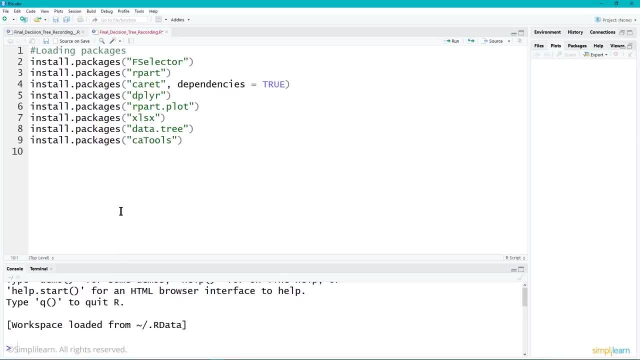 very generic working with data setup as far as statistics and data processing. So, because my Java setup is a little different, because I use a developer package, well, the latest update of the developer package and the R are struggling to see each other, So I need to go ahead and add this in. 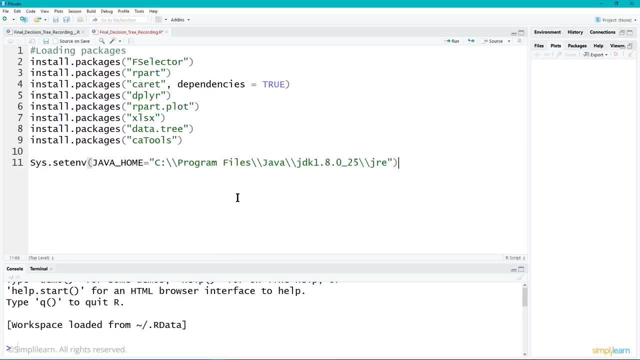 Chances are you don't need to worry about this. But if you do get an R Java error, you'll need to go ahead and add in a line to set your environment And I'm just going to set the Java home. I went ahead and looked up the last solid JRE folder. 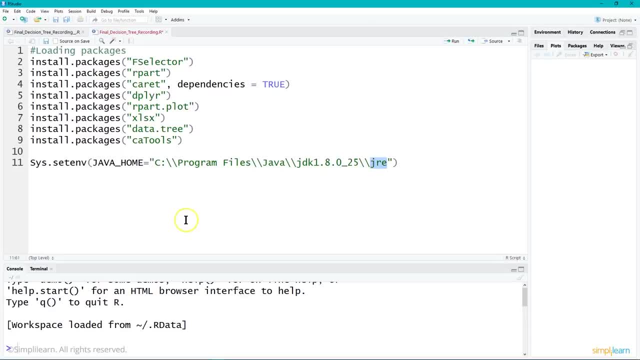 And you'll see under program files Java. You can look them all up To make sure it's the JRE and not the JDK. The difference between those is one is a standard executable. That's a JRE folder. It is a folder, not an actual file. 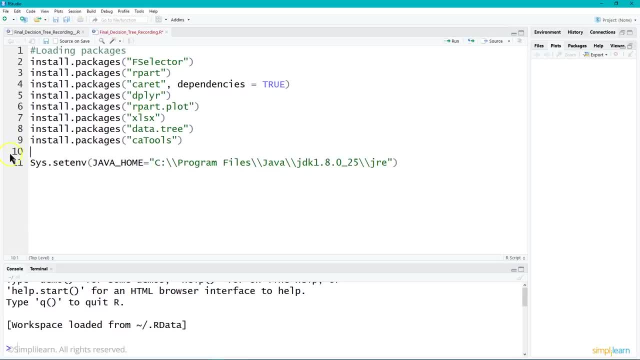 And the JDK deals more with developer side on things. And I'm going to go ahead and run this And if you're in R, you can run these lines individually by holding your control key down and hitting the enter button. So I've now loaded my workspace and set my environment here. 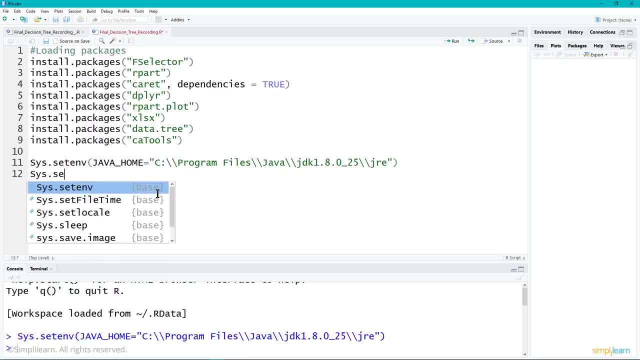 And we can actually look and just make sure System Get environment is the opposite one, And I can just look real quick and say, hey, what's my Java home set to? And if I run that, whoops, I forgot to put brackets around it. 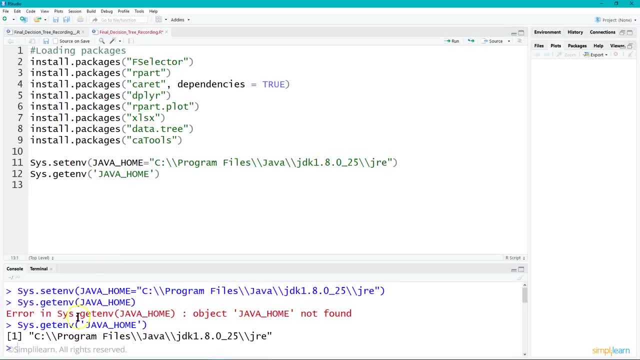 There we go. If I do that, you'll see that it's set to the JDK 18025.. And again we're looking at the split screen And let me just move this up here a little bit And let me hit the enter key. 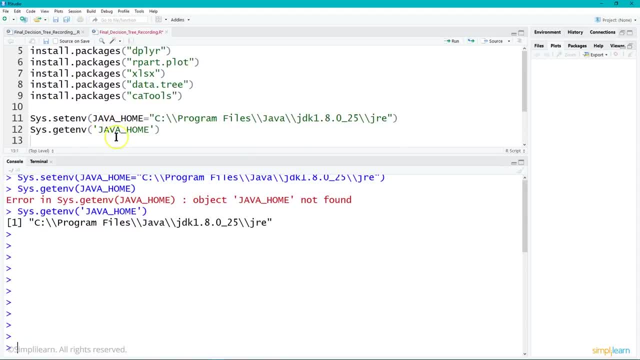 A bunch of times it comes up on the screen When I run it, and I'm running it line by line. the run text then appears down here And this is what's actually being executed. So I could just as easily type it in down here as putting it up here on the top part. 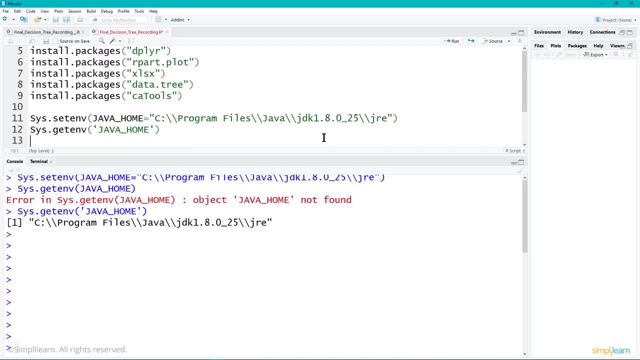 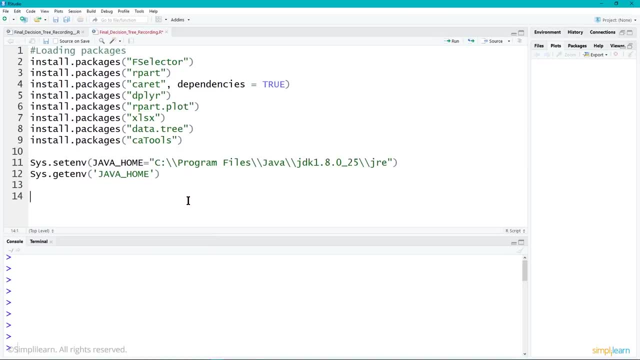 That's just a little bit of RStudio and working with RStudio. So I'm showing you the installs And, again, I've already installed it on my computer, So it takes a minute or two to install it. You need to go ahead and then bring those libraries. 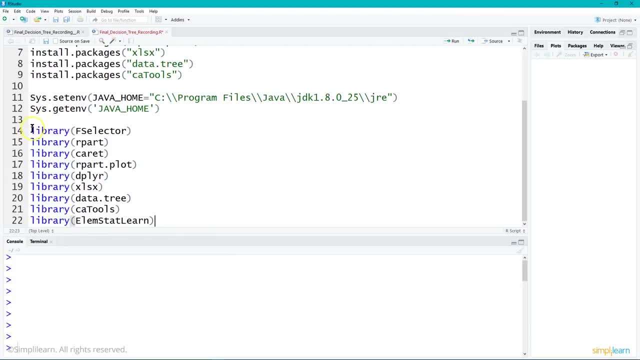 In to work with. So basically we're going through all the different libraries we're using. Elementslearn is a standard R library, So it should already be installed. You don't have to install that one And I can just go right down them. 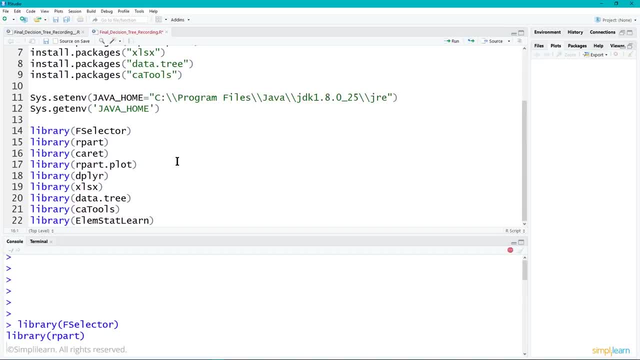 And you'll see, as I install them, that they show up on the bottom And every time you go to run a new setup, you need to go ahead and install these, Pull the libraries in. You got to tell your RStudio these are the libraries you're using. 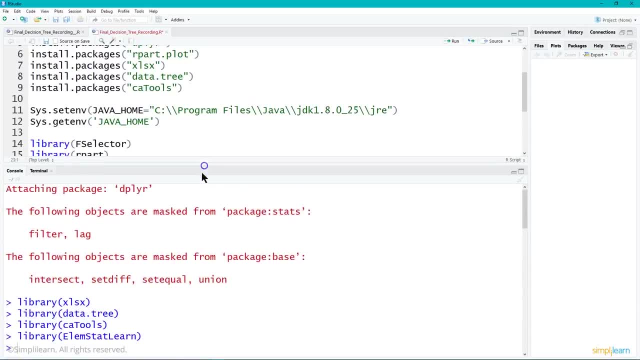 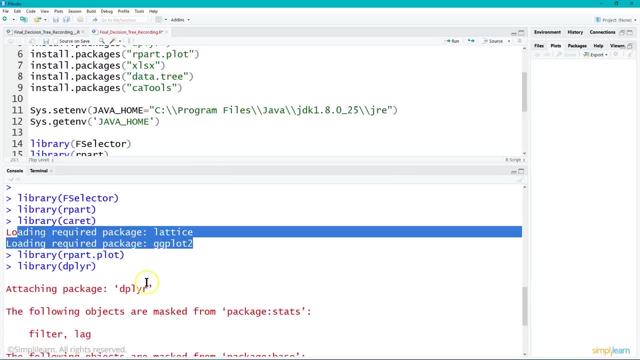 You can see right down here that as it executes them, it has all the different things. One of them had like a couple different parts to it, So it loaded the lattice and the ggplot to really nothing to worry too much, unless you see errors down here. 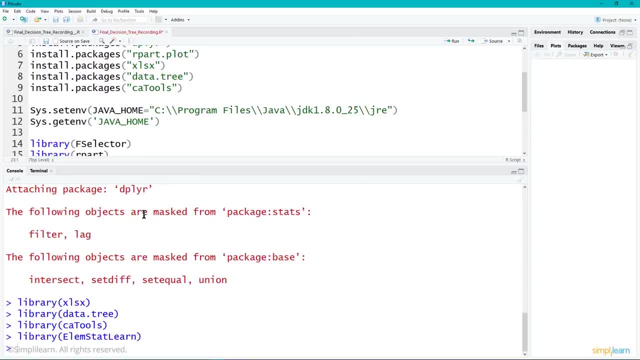 So if you start getting error codes, then you might have to go troubleshoot and find out why it's not installing correctly or did it install correctly. But it's pretty straightforward. We've covered all the libraries And again, if you want a copy of this code, simply let a comment down below on the YouTube video. 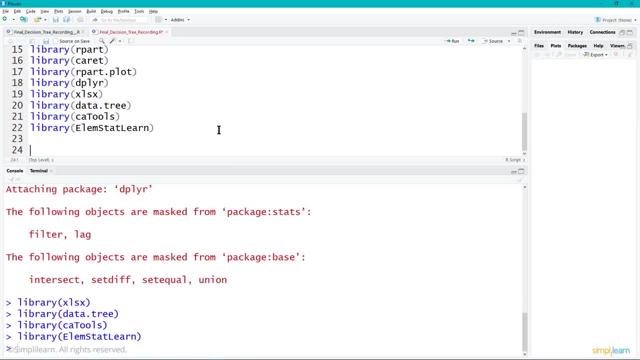 or visit wwwsimplylearncom, and they'll be happy to send you a copy of the base code. The next step is we want to go ahead and load the Excel file after setting the working directory. So let's go ahead and set the working directory. 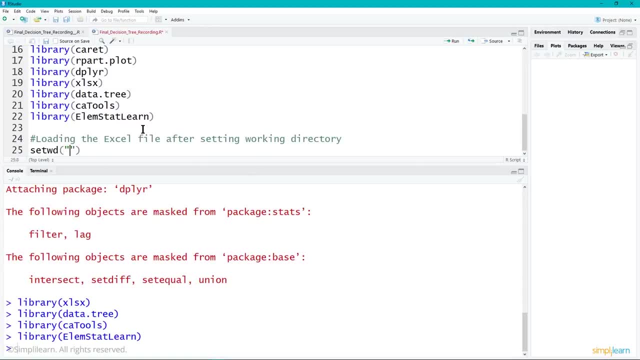 SEWWD is a command for that in R, And then this is wherever you have downloaded your data to and your files to. A lot of times, if you get the zipped framework sent to you, it will unzip all into one location And then you got to look that location up and put that in here. 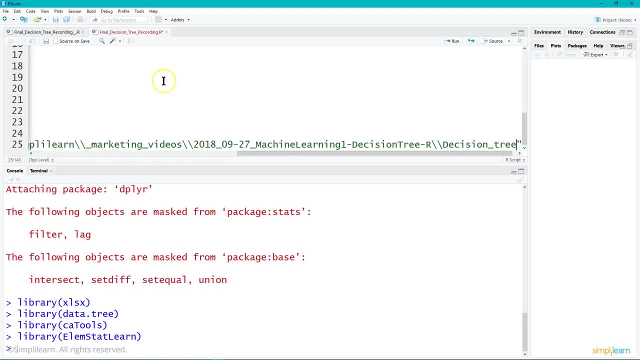 A lot of times it automatically sets up for you if you're working in the same directory. In this case, you can see I've pasted in a very lengthy path because I have this as part of my documents, my business docs and simply learn and marketing videos and so on. 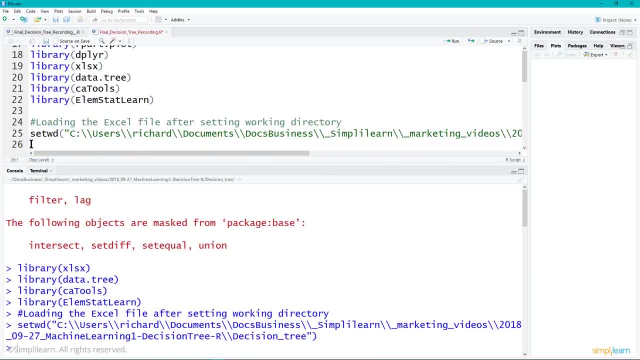 And I'll go ahead and do the control, enter And run that. So now my working directory is set And you can see down below it's executed this on the console down here And if I open up that working directory you can see I have a ship. 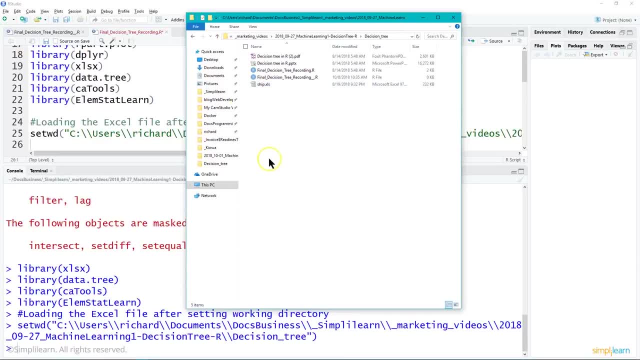 XLS file. That's the data we're going to look at And we looked at that on the slide. You could also open this up, and I want to go ahead and open it up with a notepad. By default, it will open up as a spreadsheet. 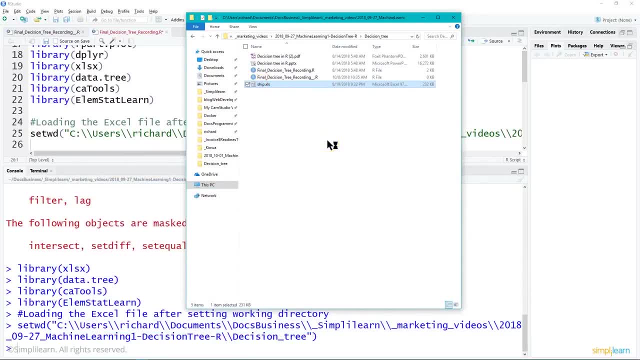 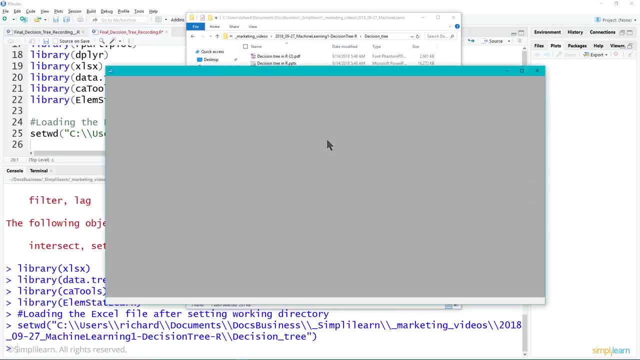 Oh, it is an Excel file, So I would have to do that. I have to open it up as an actual spreadsheet. Wasn't thinking that one through. This is one of the problems with saving stuff as a proprietary ship file, Even something as widely used as Microsoft Excel spreadsheet. 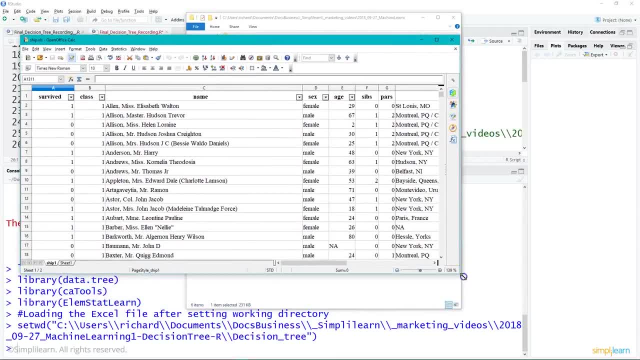 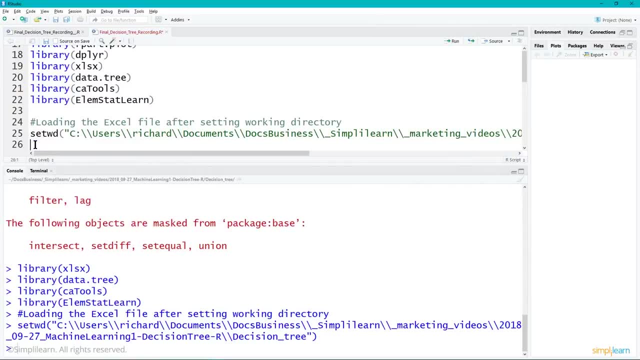 But when we open up the spreadsheet, you can see here the same data we looked at before. This was coming up in this file, And so I take this file. We can go ahead and let's create a variable. We'll call it add. 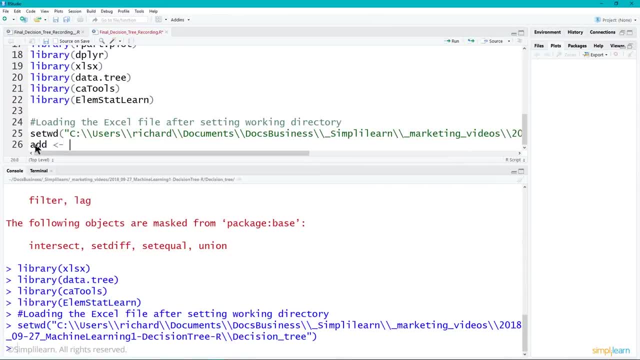 And we're going to assign it. That's what the lesser than dash means. If you've never used R before, we're just going to assign it a ship XLS, And then I'll do my control, enter and you'll see it run down here. 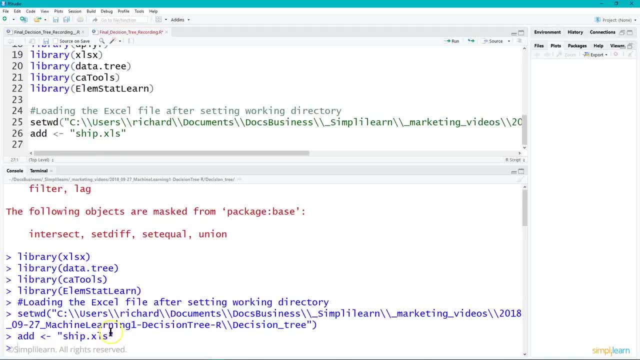 Ship add is assigned ship dot XLS or Excel spreadsheet on there. And then let's have another variable, We'll call it DF for data frame And we're going to assign this read XLSX. And that's from the library SLXX that we just imported. 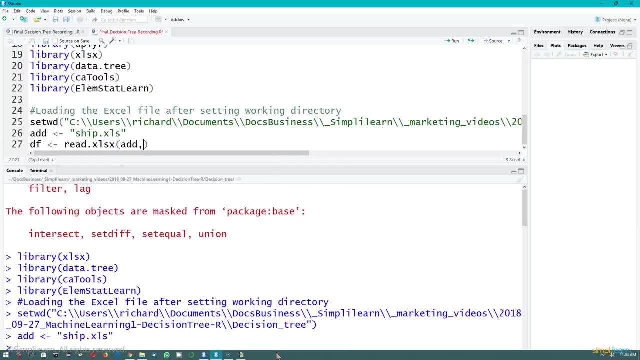 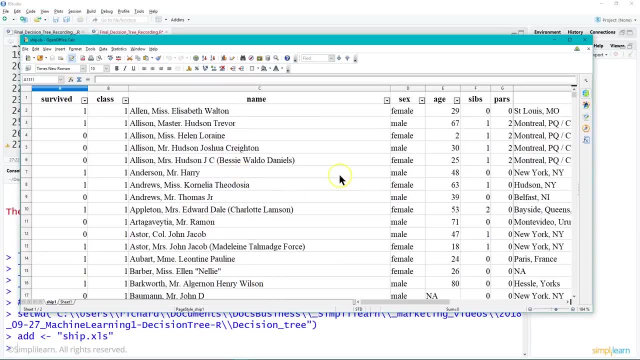 And we want to read the file add, Because we just created that variable with the ship dot XLS And I didn't catch this right away. but you'll see when we open it up in a spreadsheet It might be hard to see in your video screen. 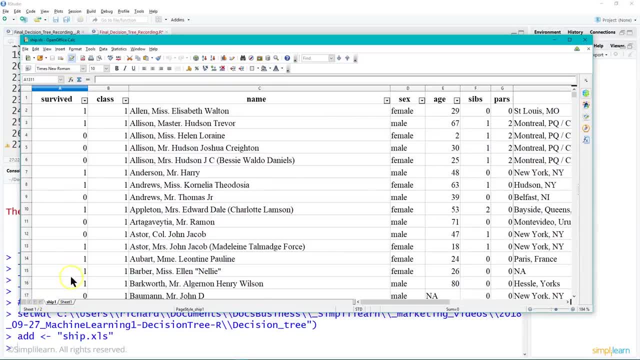 It has. the first sheet is called ship one. So this data is on the page ship one in the Excel spreadsheet And we got to make sure that we tell the reader to look for that, And so we can simply do that in our command line. 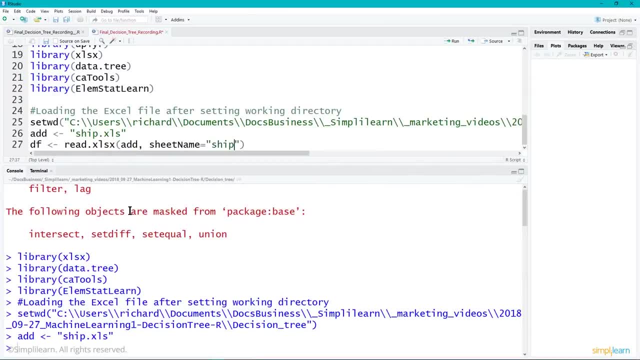 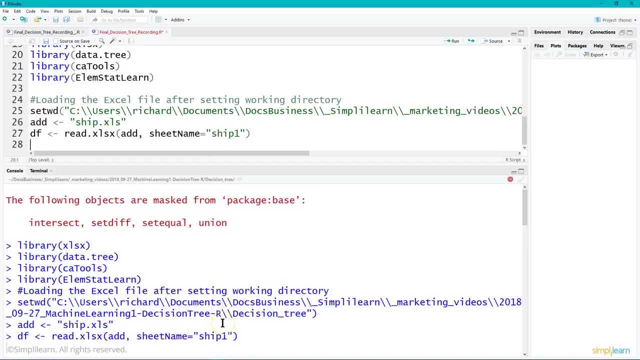 Sheet name equals and it was ship one on there. So we go ahead and hit the control, enter and run this line And it brings it down below and executes it. It's now reading in that data from that spreadsheet. That's what's going on. 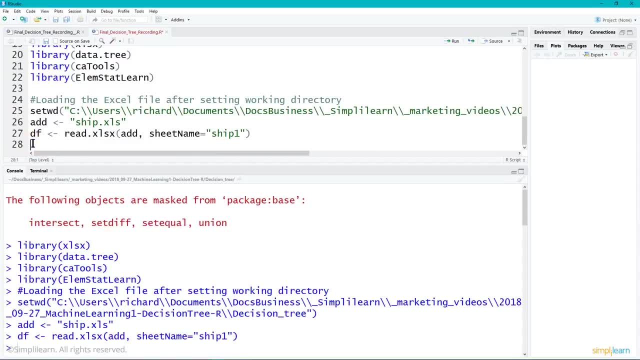 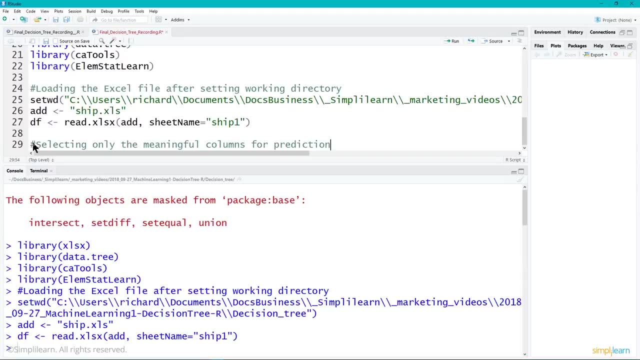 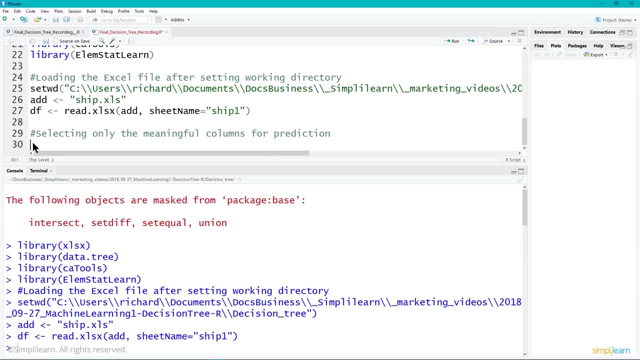 And it takes it just a moment to go ahead and read it in, And then with any data processing, we need to select The meaningful columns for the prediction. So this is important: that we sort through our data and set it correctly So that whatever we're feeding it into can read it correctly. 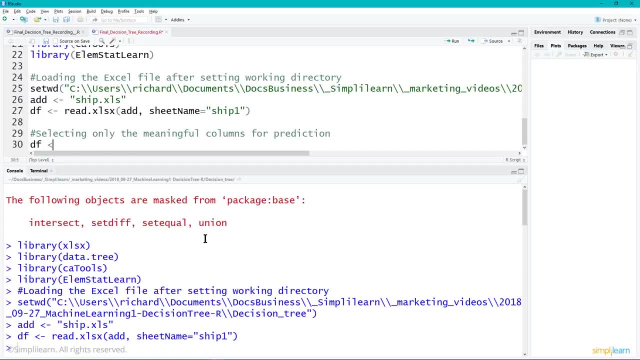 You can do this with DF. We're going to reassign it and we're going to select, And from there we're going to select DF as our main data frame going in And then list the columns that we want. And if we look at the 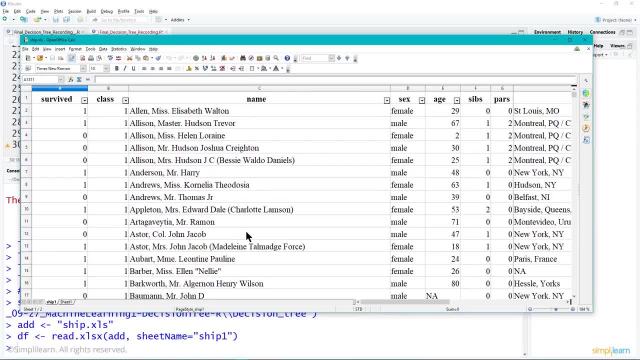 The Data. we have survived. We have a class, We have a name, sex and age, And then there's siblings and parents. We really don't want to know the name, because we don't need the name to run this on here. 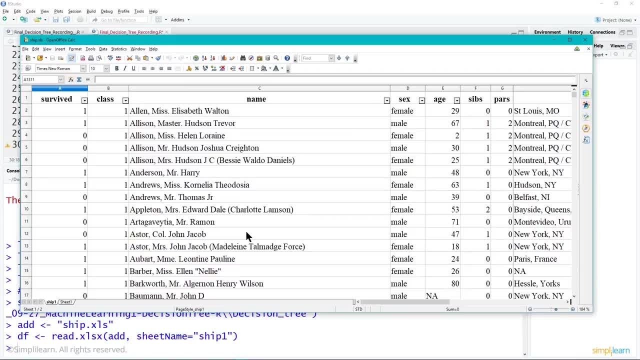 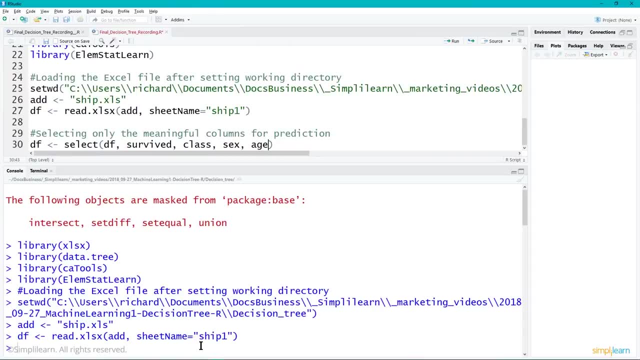 And then we got to decide which one of these we want to work with, And the guys in the back played with the data a little bit And they came up with the following columns Survived, which we need definitely, because that's what we're actually trying to figure. 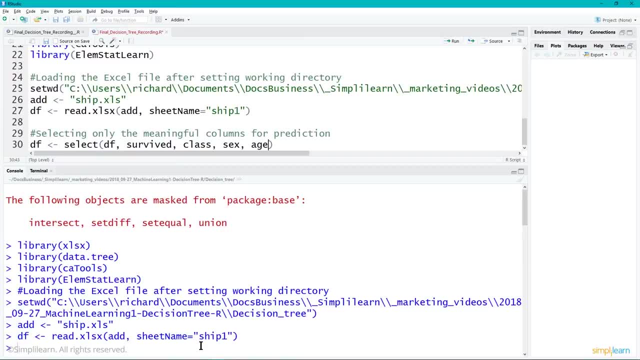 out is whether we're going to survive or not. What class there? Which, Which class of the boat? They're writing in their first class, second class, sex and age, And we went ahead and dropped the rest of them, at least for this example. 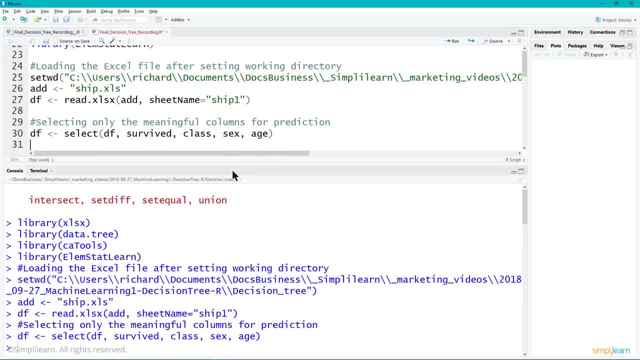 And so I go ahead and do my control: enter and you'll see it execute down below. And now, DF equals these three columns or four columns Plus. our answer is one of those. So I always think of it as three columns plus one, but it is four columns. 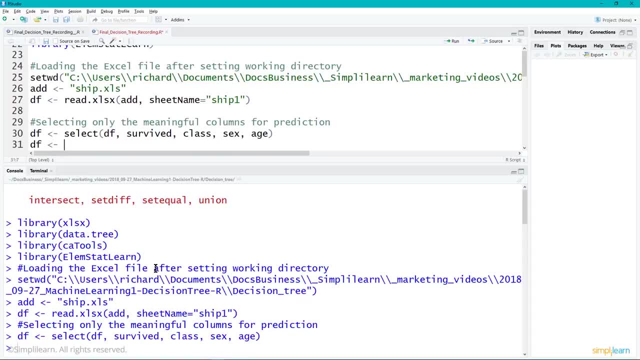 And then for the next step, we want to make sure the data is in the right Format. So again, I'm going to resign the DF and we're going to mutate the data, And that means we're going to take each one of these columns and we're going to let it. 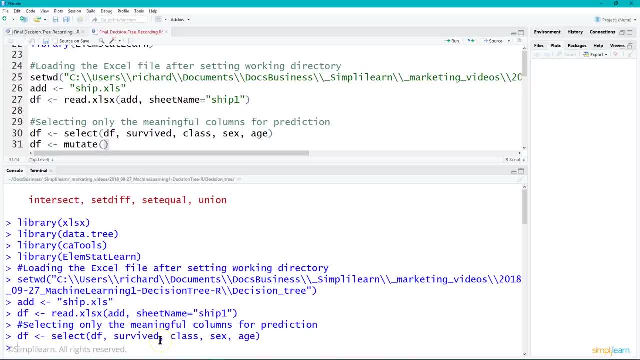 know what kind of data that is. So our first one is: I'm going to put the database in, or the data frame in there, DF, And then we want to go ahead and do. survived equals a factor of survived, So this is a yes- no. 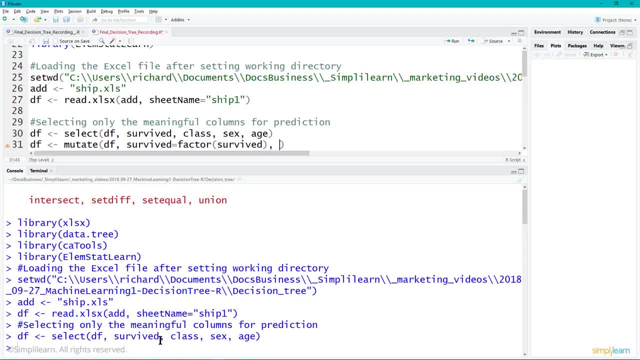 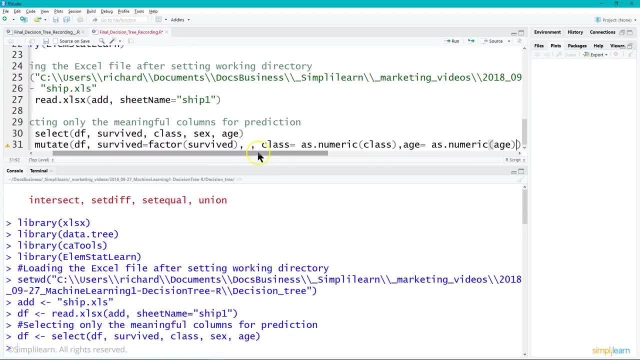 It's letting us know that this is a zero or a one on here, And then for the class and the age, those are as numeric. There's other ways to process class, since it is a very restricted number on there, but for this we're just going to do it as a numeric value. 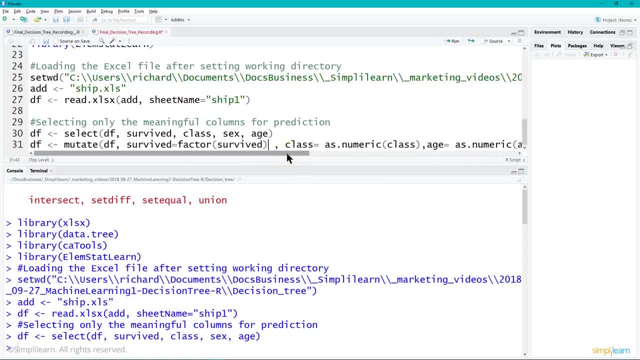 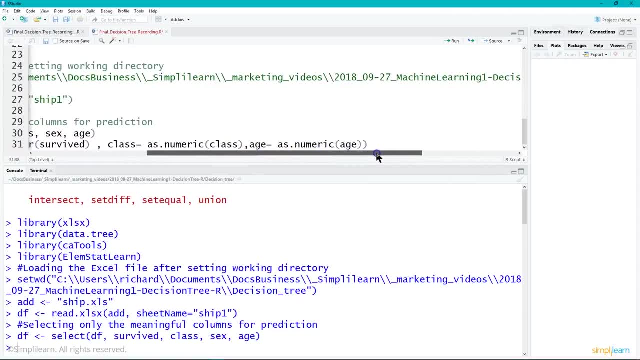 Same thing with age. And you see, we didn't do anything with sex. We're just going to leave that as male or female, And that's fine for this, because it'll pick up on that when we run the decision tree And we'll do our control. enter. 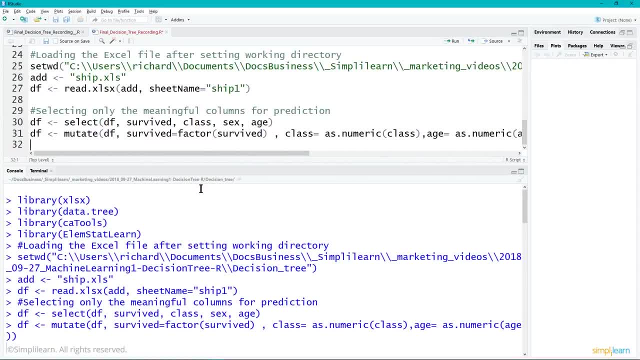 So now I've assigned the new DF and you can see it comes down below. And then we're going to do our control enter. So now I've assigned the new DF And you can see it comes down below As we run it on there. 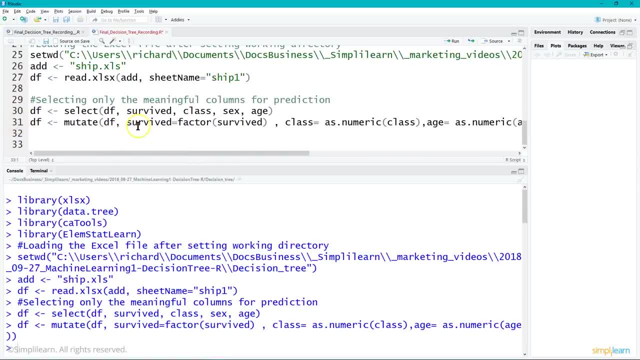 So this is now loaded And DF now is a mutated data frame that we started with And we've set it up with our specific columns we want to work with- In this case survived class, sex and age- And we've formatted three of those columns to a new setup. 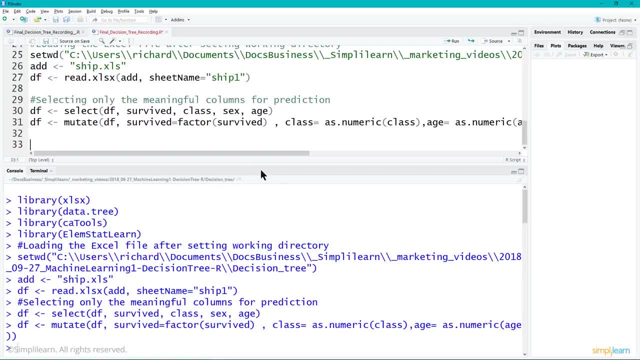 So one of them is factor. That's what we use for survive. So it knows it's a zero and one, And then we switched class and age to make sure that it knows that those are numeric values. Now that we have our data formatted. 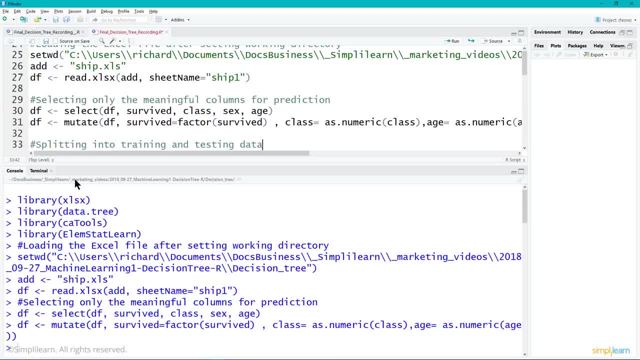 we need to go ahead and split the data into a training and testing data set And by now, if you've done any of our other machine learning tutorials, you know this is standard. You need to have your data that we train it with. 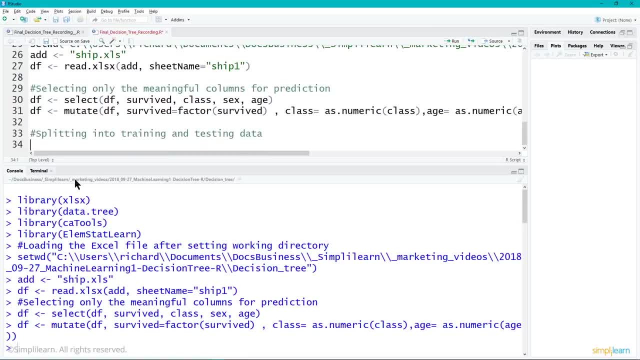 And then you've got to make sure it works on data that it hasn't trained on. So we'll go ahead and do the splitting. Let's take a look and see what that looks like, And when you're dealing with splitting the data, we're doing a little randomness. 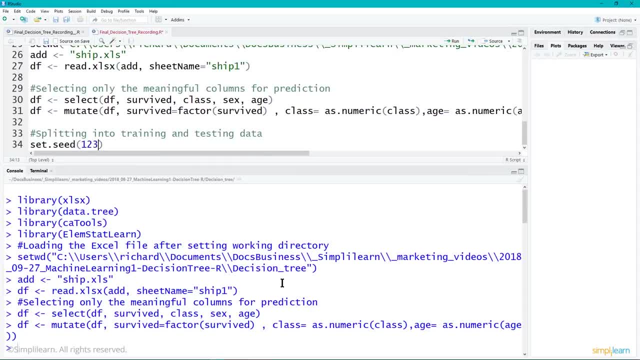 So we'll just go ahead and set the seed to one, two, three. You can set that to whatever number you want. That's just setting the randomness. We're going to variable seed And we'll go ahead and hit enter on there. 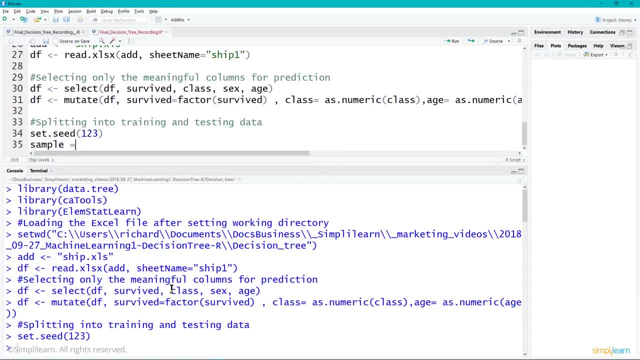 And to do this we're going to create sample And we're going to go equals sample dot split. So we're splitting up the data. This is actually creating a whole new column: Trues and falses. It's all stored in sample. 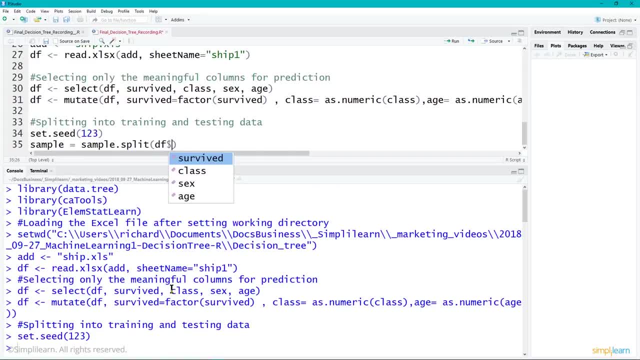 And we want our data frame And we use a dollar sign to denote that we're going to be working with one of the different columns. We have a nice thing you can do in R And it actually shows my survived. So df survived. 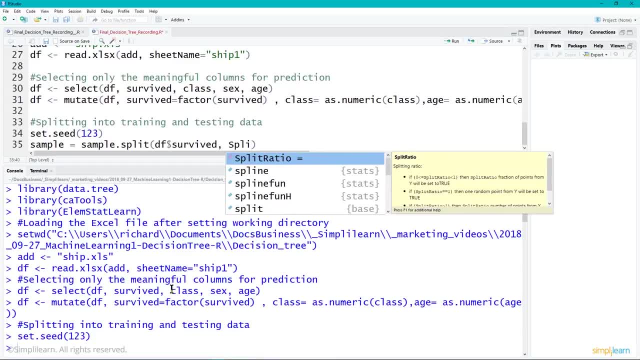 And then our split ratio. Split ratio- I want to add a period in there which it doesn't have. Our split ratio is going to be equal to, And we'll do 0.70.. So we're going to take 70% of the data of those that have survived. 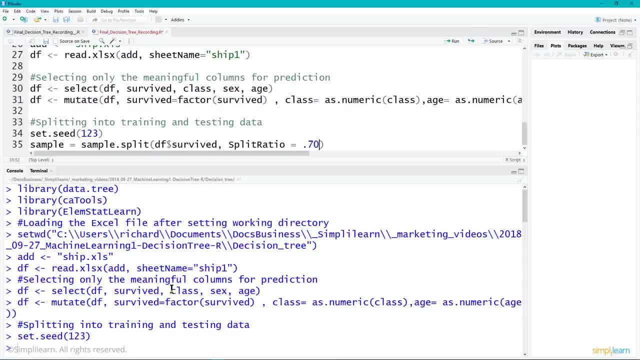 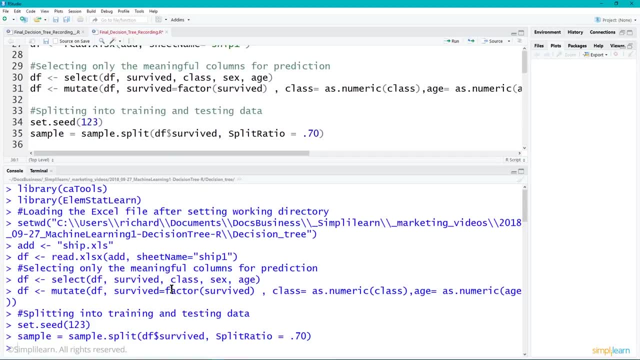 And we're going to just randomly select which one of those we're going to use for training And which one we're going to use For testing it out later, And we'll hit our enter and load that sample in there And then we'll go ahead and create our train and our test data sets. 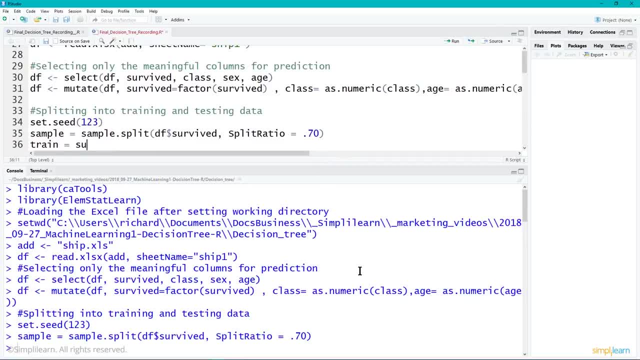 I'm going to set train equal to- And this is where it kind of gets interesting, because we're going to do subset And then we're going to do a subset of our df where sample, And then we're going to use equals, since this is a logic gate. 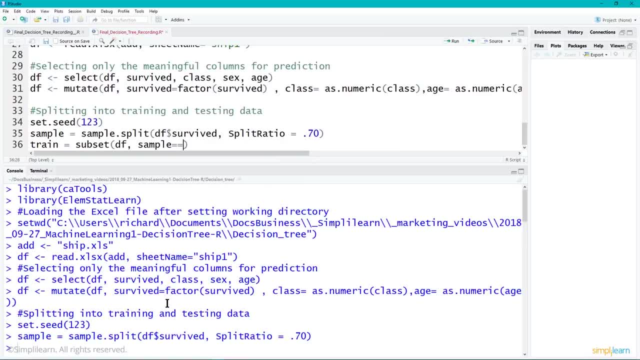 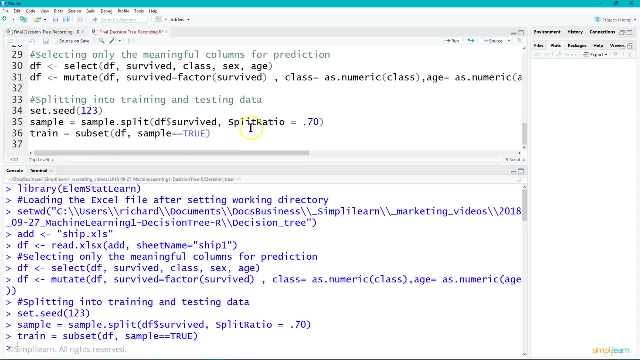 So wherever it says sample equal to true, We're going to use that line in df, And this is of course, r, So it's all capitalized for true. So here's our train data frame we're creating. So when I execute this and it shows up down below, 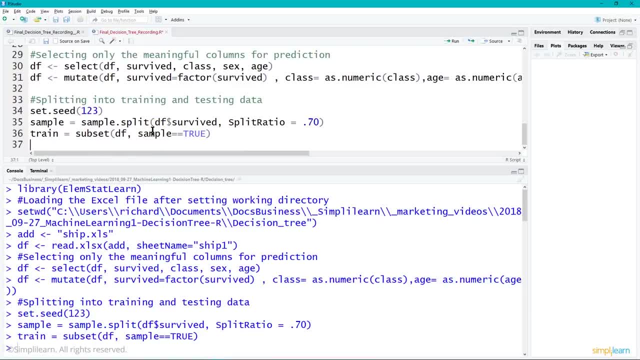 It goes up and says, hey, this sample created a whole bunch of trues and false And we're going to take those trues and falses And, wherever we've created a true, Which is 70% of the data randomly selected, That's what we're going to train the data with. 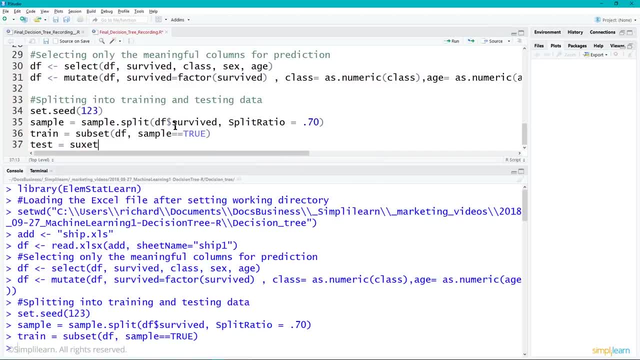 And then we need our test set- And that's a subset, Just the same thing we just did. And we need our data frame And this is where the sample equals false. And again, when I hit control enter, It goes down this line of code: 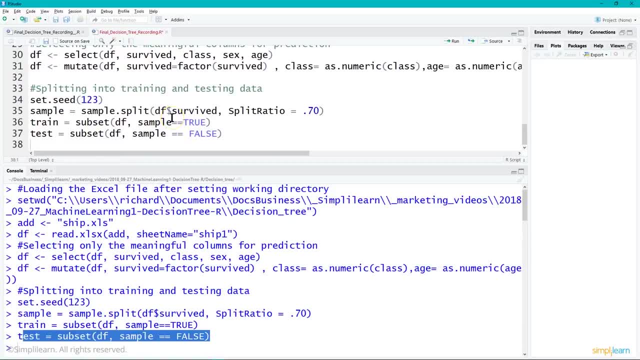 And it runs it down here in our terminal window. So now we've nicely split our data up. We have our training data set and our test data set, And this is, of course, where we get to the point of what we're actually trying to do. 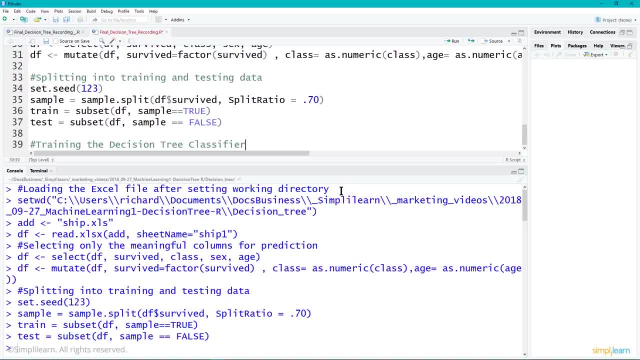 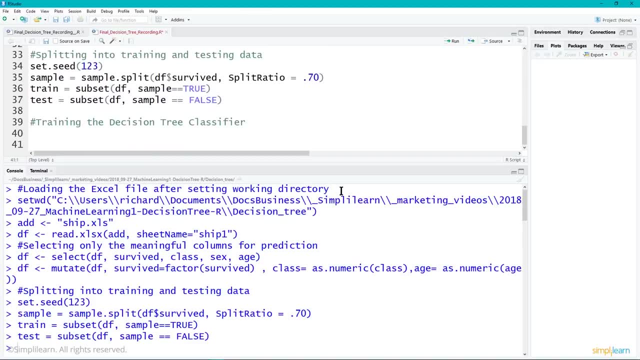 Which is create our decision tree, And we're going to do that by training The decision tree as a classifier. This always gets me. You spend all this work sorting through the data, Reformatting it- In this case, mutating it- And filtering it. 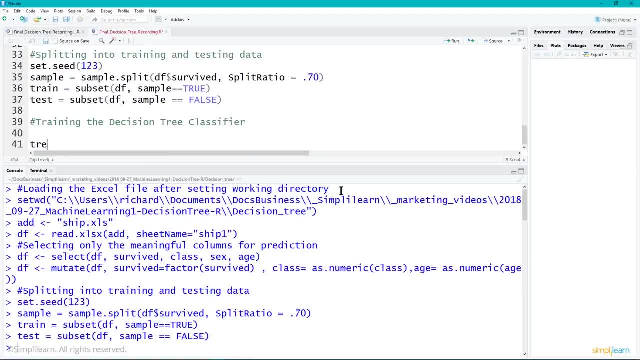 And creating a train set and a test set. So we're going to go ahead and create our tree, We're going to assign to it The R part- That's the module we imported- And for the R part, We need to go ahead and 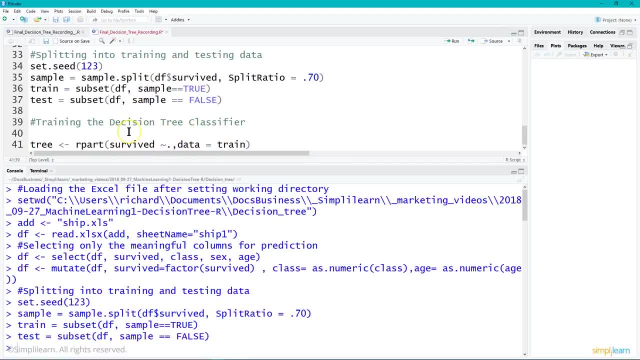 Do what's called a survived, And this is kind of a little complicated to look at. So let's just take a quick look at this. I'm going to go backward on it. The first part is we're importing the data, So data equals train. 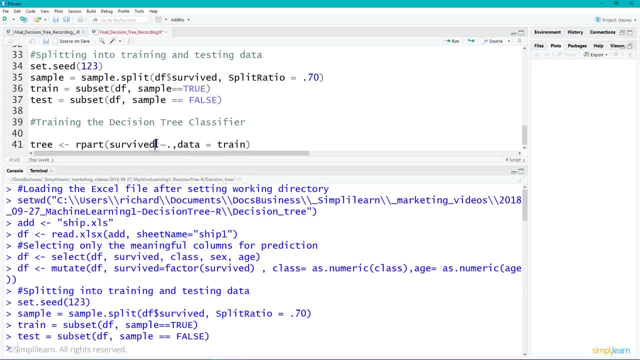 And then what we want to know is who survived. So the first part we put in here is the column we're looking for is survived, And you'll see that we have added the squiggly mark in the period Because we're looking just for this prediction. 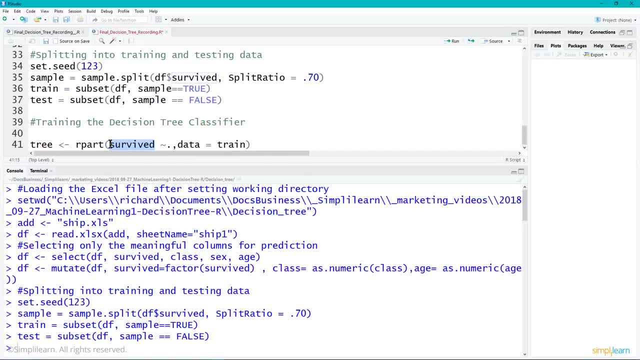 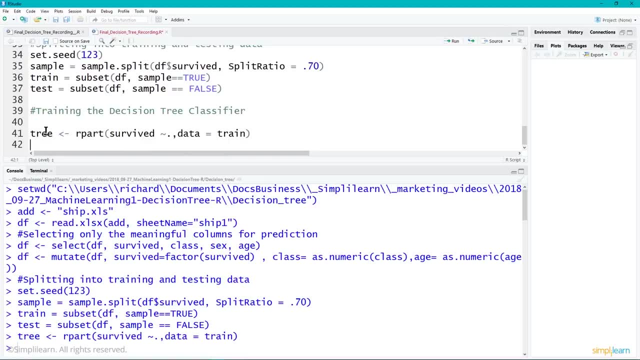 We just want to know who survived on these boats For programming our decision tree. And I'll go ahead and hit control- enter. And we've now created the tree. That tree with all those values is now in there, And if you remember from before, 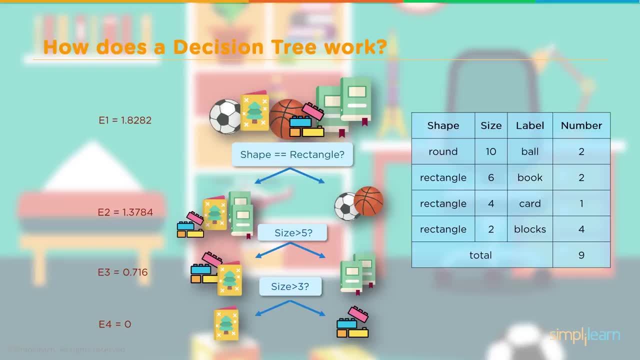 We've taken from when we did the closet full of clutter. We've done the same thing where we have our entropy, And that one line computes the entropy And the increase in information And it brings the entropy down to zero. So it's the same thing. 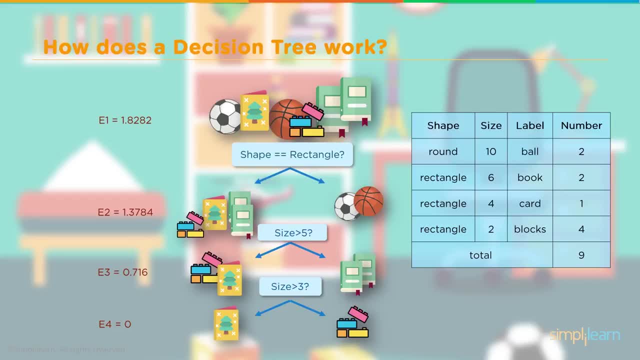 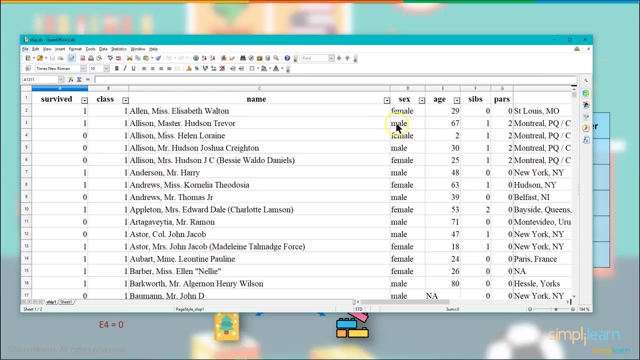 But instead of applying it here, as we did visually to the Closet, It's now applied it to the data on the ship. It's now looked at the survival of zero or one, Based on female, male, What age they are, Where the best split of the age is. 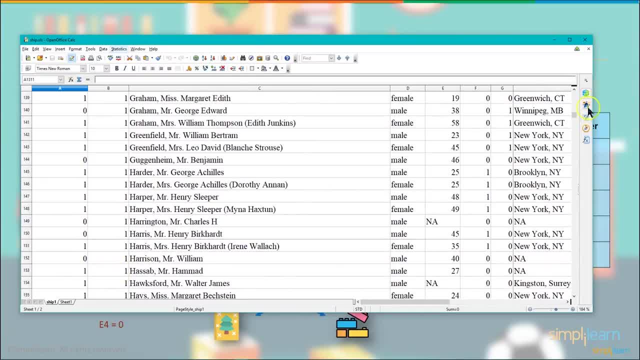 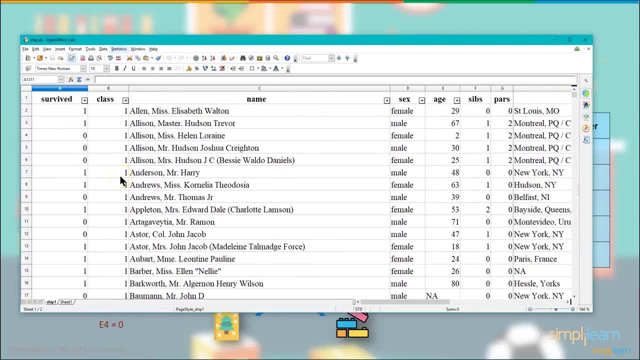 And what class they were in. You can see we have first class If we go down there. I think there's third. yeah, third, second. So I guess it's class one, two and three. But you can see, that's how we split it up. 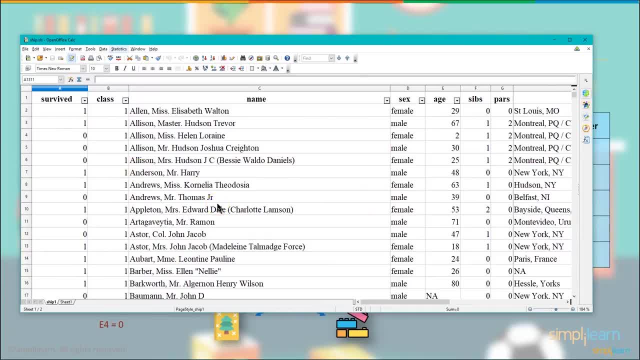 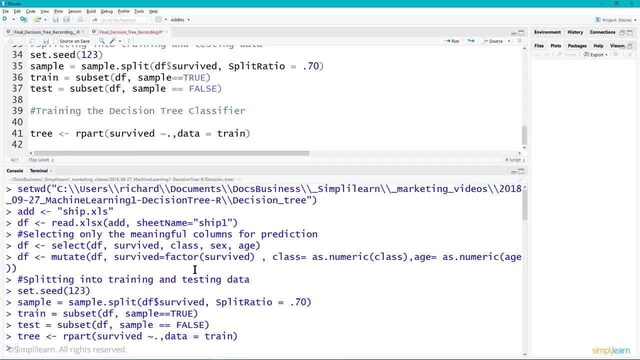 So it's used, these different variables, to minimize the entropy And maximize the information gain, And that's all done in that one line of code. Boy, we worked on all that theory And computer does it for you, in one line of code. It's important to understand the theory behind it. 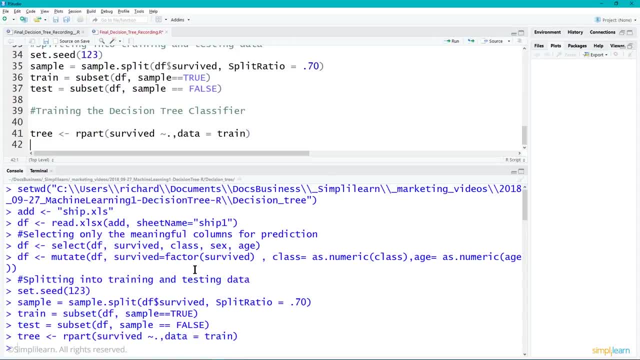 So you know what's happening, Because as they make changes to these Or if you add special settings on it, You have to know what they're doing. But in this case you can see that we, once we get it formatted, The computer does all the heavy lifting for us. 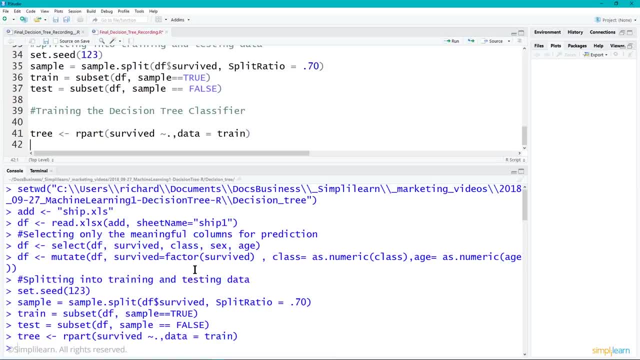 And it never ceases to amaze me Just how advanced machine learning has become these days And how easy it is for people to get into it And learn The basic setups And be able to compute your different machine learning models Once we've computed our decision tree. 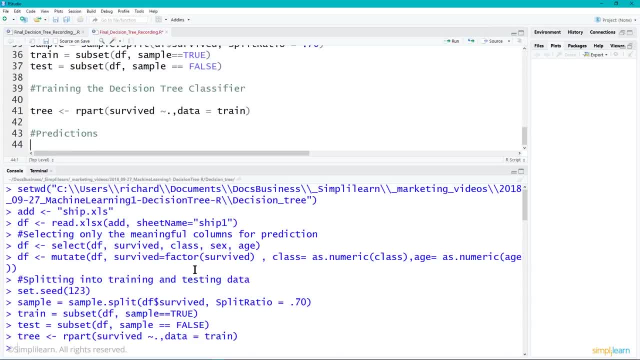 And we built it on there. We want to go ahead and start doing predictions with it. And what are we going to predict? Well, you remember that we created our data with the train and test, So we have our training data, which we program the tree for. 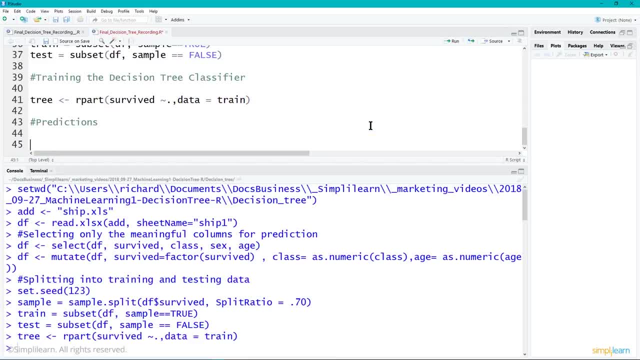 Now we want to see what it does with the test data. So let's see what that looks like And we can wrap that into a tree: dot survived, Dot predicted. We'll assign that to our prediction And this is nice because we have the command predict from one of the modules. 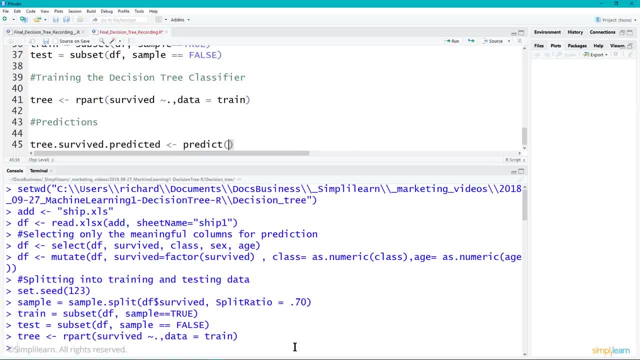 The rpart module that we brought in. I can simply put in here that we're going to use the tree. We have our test data And type. This happens to be classification or class, And this would also be if you were to distribute this tree. 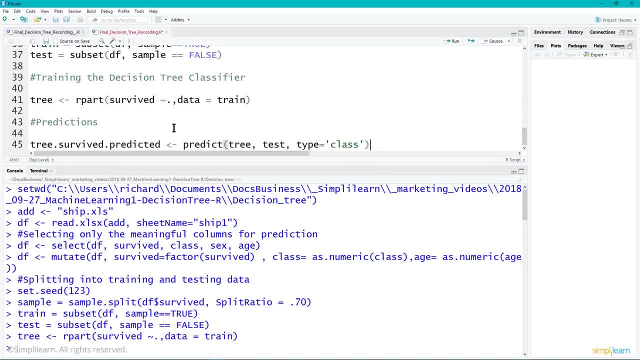 You could save the tree And send it someplace else to be used on new data. This would be the command line you would use to predict on here. Predict you have your tree saved, You have whatever data you're putting through And you let it know. it's doing a classification on the tree. 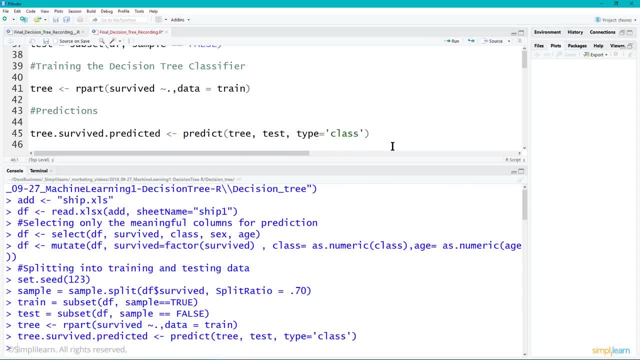 And we'll go ahead and run that. So now that's loaded up And now that we've gone through, We've trained our tree, We run a prediction on our test data. Remember, the tree had never seen the test data until now. 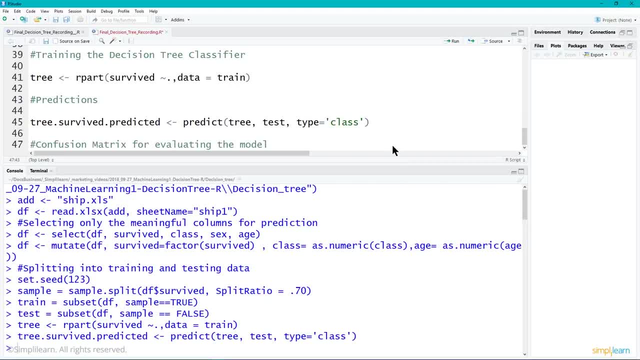 So we've already built the tree, We're just testing it out And to do that, we're going to use a confusion matrix for evaluating the model And let's see what that looks like. And that is simply confusion matrix. So once we have the confusion matrix, 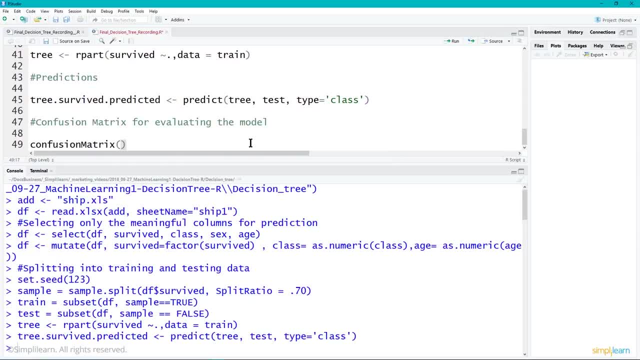 Which came in from our carrot. We need to compare the two different pieces of data, And the first one's going to be the value we generated. up here We have tree dot- survived, dot, predicted, So I'm just going to copy that and paste it down here. 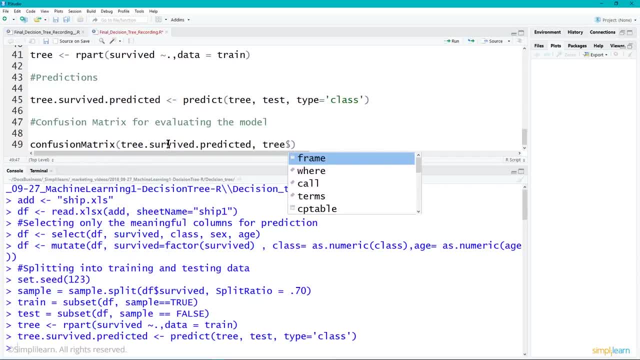 And then the second one is The tree. We're comparing that to let's see survived, But it's not the tree. It's easy to get confused sometimes when you're moving these things around. We're going to compare it to test. 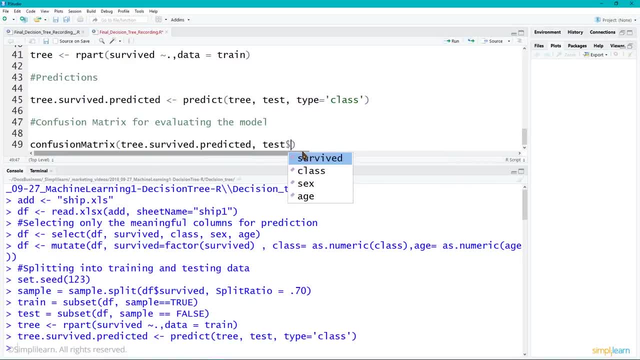 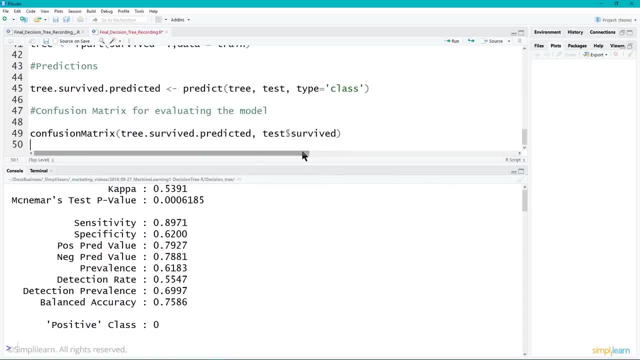 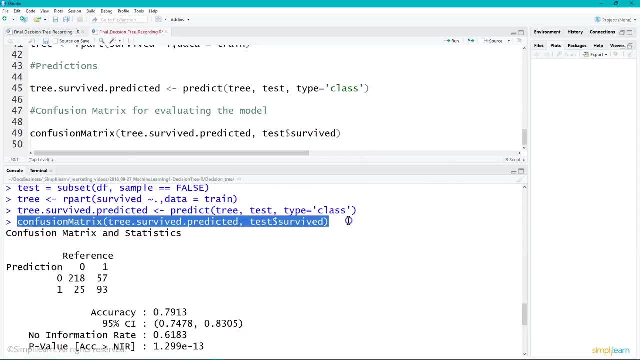 The test group of data, Specifically the survived column, And let's go ahead and run this and see what that looks like. And so let's go ahead and scroll up a little bit here To where it first executed The confusion matrix And the most important part of this. 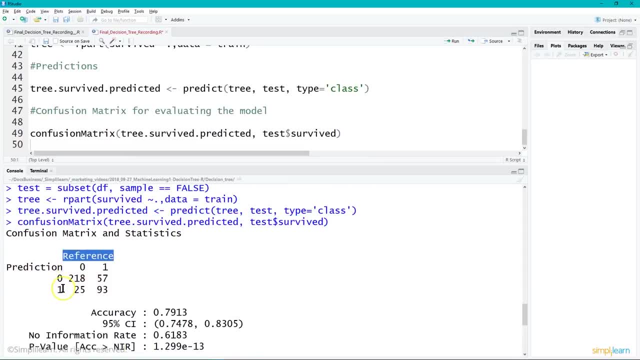 Is that we have our prediction And our reference, And so zero means they didn't survive, One means they survived. We had our prediction on here Versus the actual, And that's what these two columns mean. And so when you read this little chart, 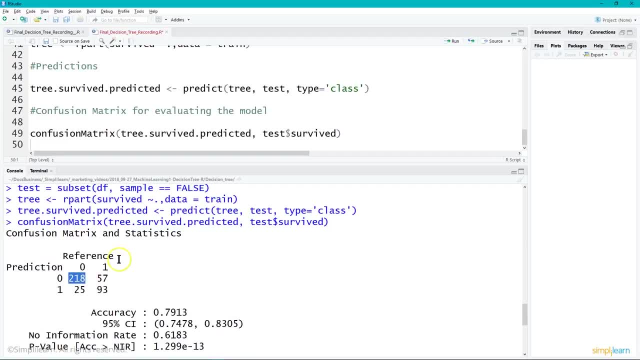 We have zero, zero. So both the prediction and the actual reference said We agreed on 218 values for people who did Not survive. A little grim there for data. Remember I'm talking, this is morbid data, Talking about death rates of people on boats. 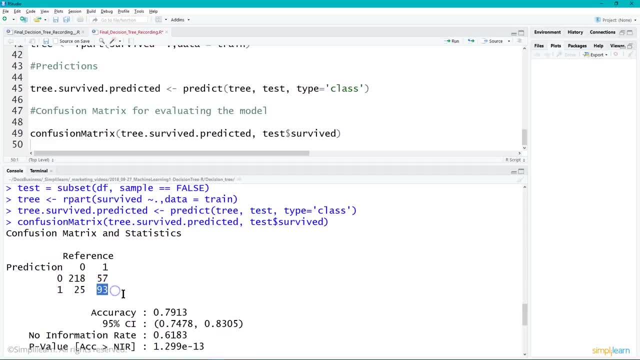 It says that they both agreed on 93.. So 93 of them where we predicted the value that they would survive And the reference came up the same. Likewise The predicted where predicted one, And the reference said no, these people didn't survive. 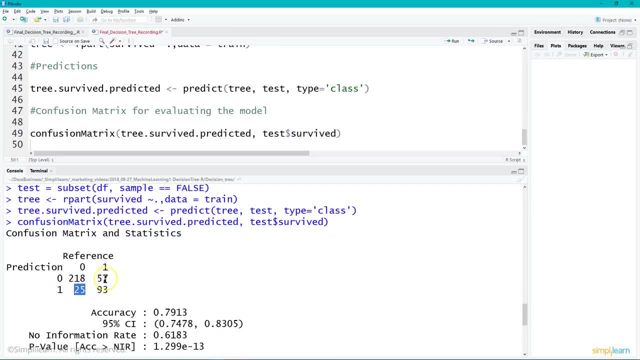 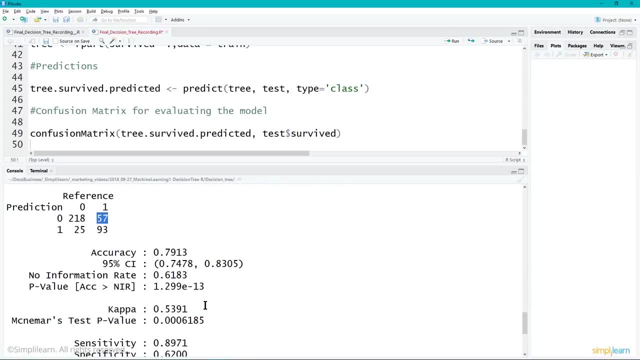 Well, our prediction got 25 wrong And where it says they didn't survive And they actually did- It got 57 wrong And we can come on down with the confusion matrix And we can look at the accuracy It comes up with the 0.7913 or 95 percent CI. 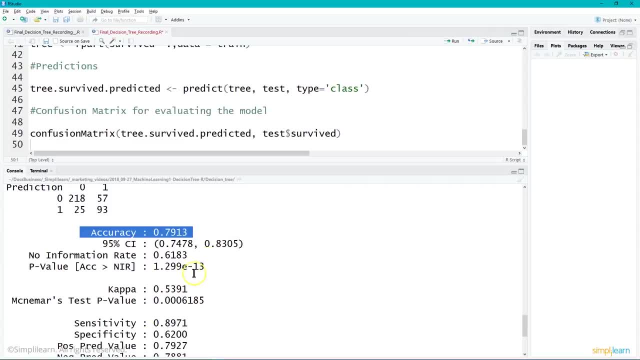 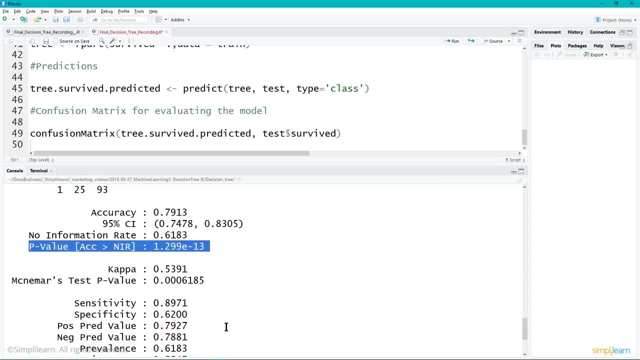 So yeah, you're looking at pretty high accuracy Information ratio P-value. When you're in statistics, the p-value is one of the things we look at. Remember that there are certain values. if it's over 0.95, it's considered highly valuable. 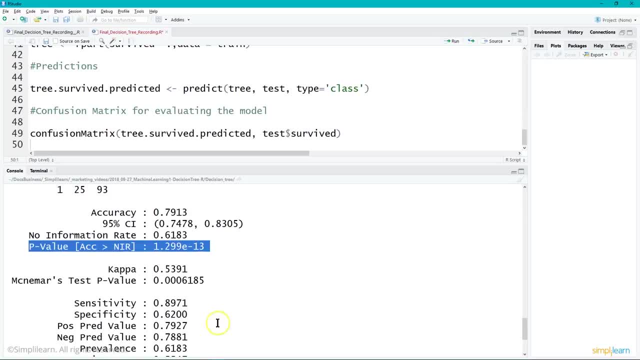 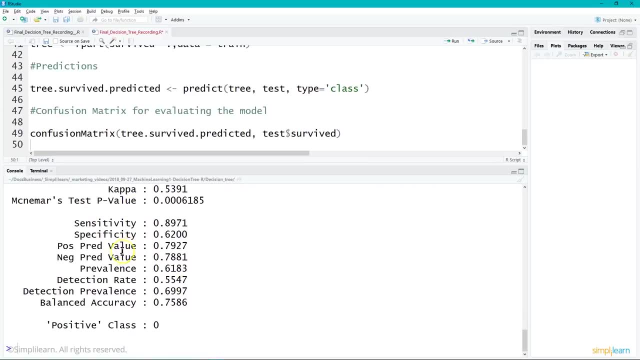 Variable 0.5 means maybe Anything less than that means it's probably not connected. You have to look up the p-value a little bit more on that. And then they just have more information down here Which you can go through, Which you can go through. 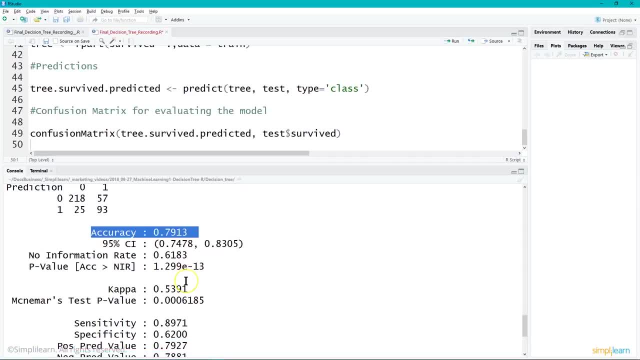 But the important part is that we have a very high accuracy. That's what we're looking at. This is a very accurate model And, again, always remember the domain you're working with. Certainly. This is an example And this is a good little piece of data you can play with. 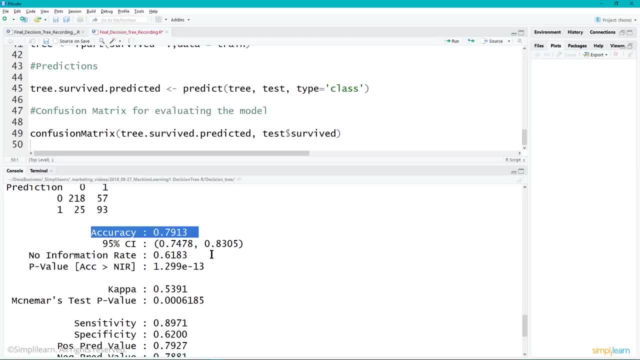 But if I was, say, betting money And my accuracy came up as 79 percent or over 95 percent CI, I'd be like, yes, let's bet on that, That's a good bet. But if I was betting on a life or death situation, 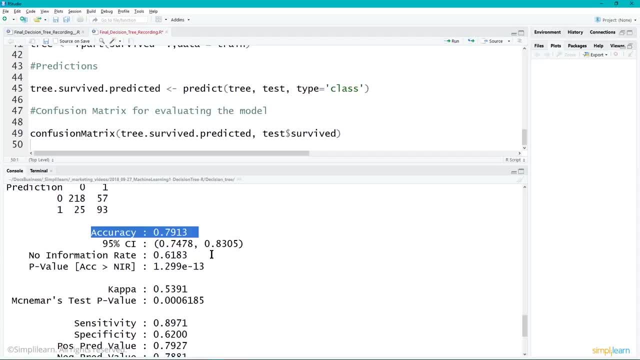 I might kind of rethink that a little bit, If that is, if it's going to affect my life. that way, You can also look at this as if you're trying to figure out where the boats go In this particular example And where to put the lifeboats. 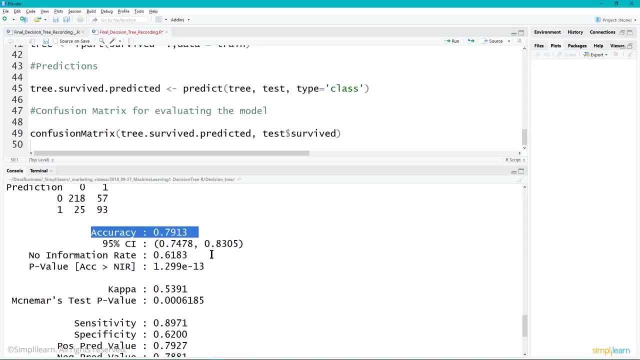 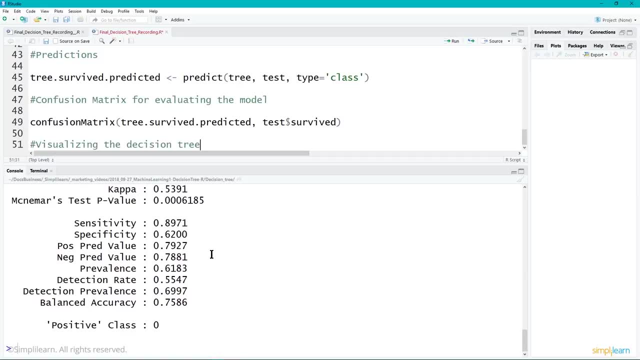 That's actually pretty good. You'll be able to say, Hey, we can increase the chances of people surviving this accident By putting the lifeboats in the appropriate places, And then this is always fun. Let's visualize the decision tree, One of the cool things you can do inside of R real easily. 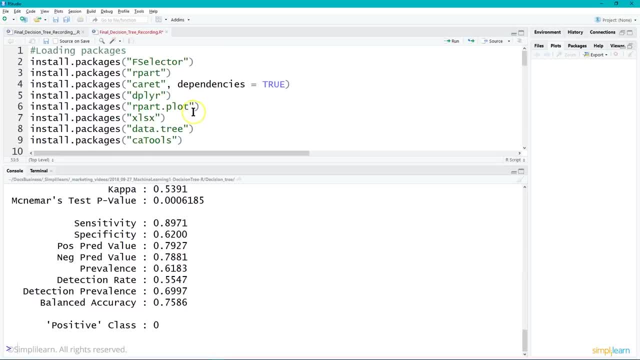 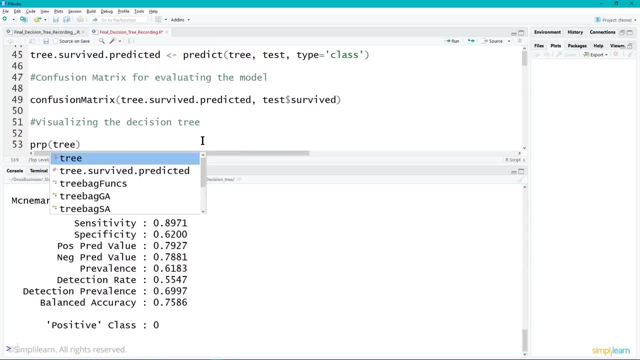 And, if you remember, one of the modules we brought in has a rpartplot. We're going to take that And we're going to dump that into the PRP for the tree And let's go ahead and hit enter. And this is fun. 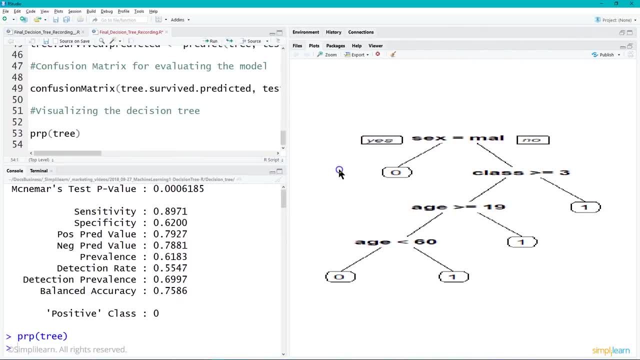 Let me move this over So you can get a nice view. You can see how it actually split it up, And let me just rerun that again. Now they expanded the right. You'll see right here where one of the biggest splits was whether the person was male or female. 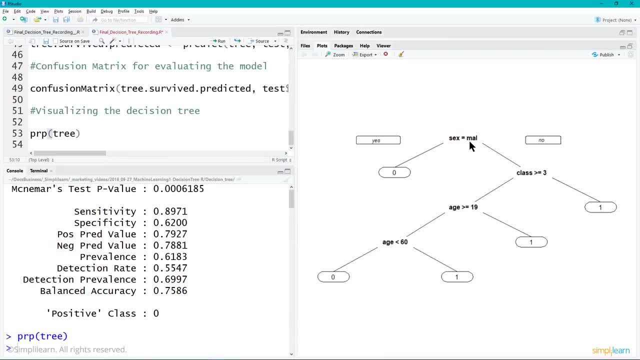 Didn't know. that was probably one of the biggest breaks as far as lowering the entropy and increasing the information gain. And then, once you know sex is male, It came down here and it said: you're not going to survive. I guess the men were throwing themselves overboard on the boat. 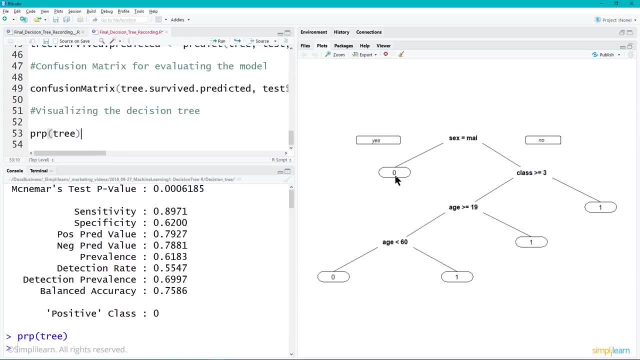 I don't know, Maybe they're being very gallant and letting the women and children Survive, which is what I hope that means. So once you know that it's not a male and it's a female passenger, if you were in class three or above, you had a high chance of surviving. 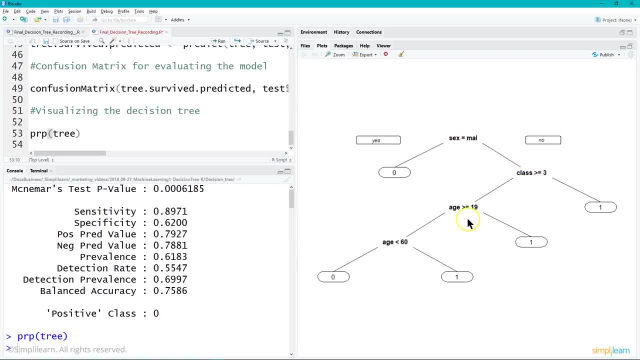 If you're less in class three, class one or two, then it was based on age And so you can see where age was greater than 19.. So anybody over 19 had a high chance of surviving And then if they were, or less than 19,. I'm sorry if the age was a little confusing on that one. 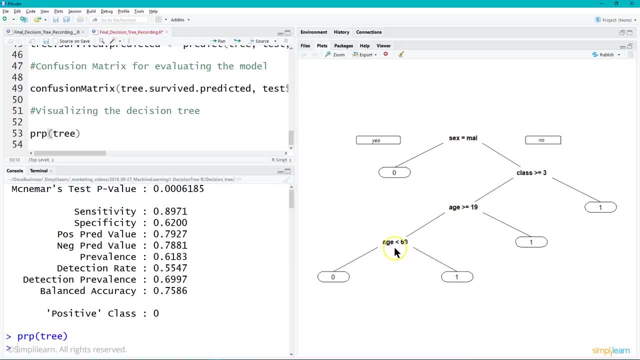 But if the age was one side of 19,, they probably survived. If not, then it said, hey, if your age is less than 60, you probably survived, And if not, people who are older probably didn't make it out of the boat in time. 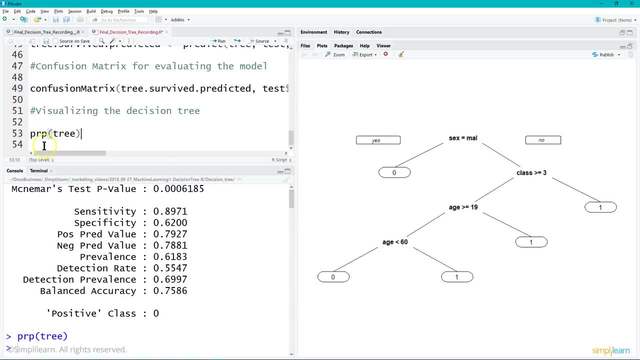 So elderly have a much higher risk, which you would expect. You'd expect that to be the case, That elderly would have a hard time getting off into the lifeboats And they would probably step aside for the younger generation. I know I would. 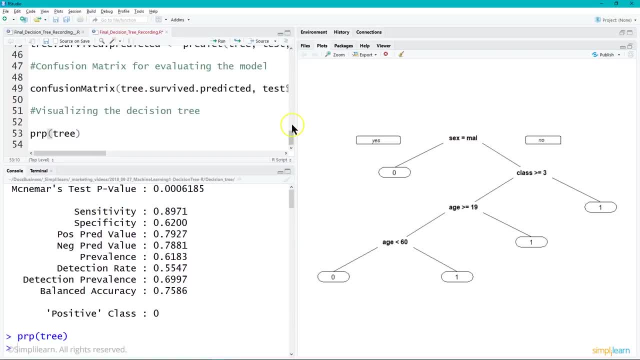 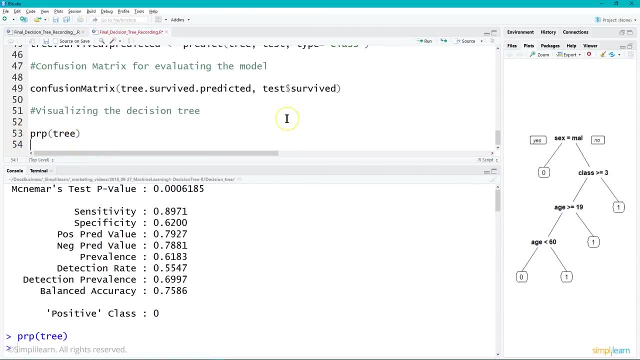 You know. so that might be more of a social norm statistic as opposed to survival rate. Let's go and put this back on over here. If you're working with the shareholders, it's good to have a lot of tools as far as how to display. 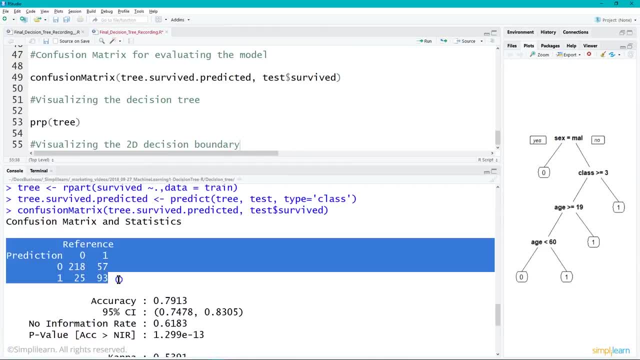 You know they'll want to see this number here, where you say, hey, this is what the confusion matrix looks like And we got a 0.79 accuracy. That would be like the number one thing you talk to the shareholders about. 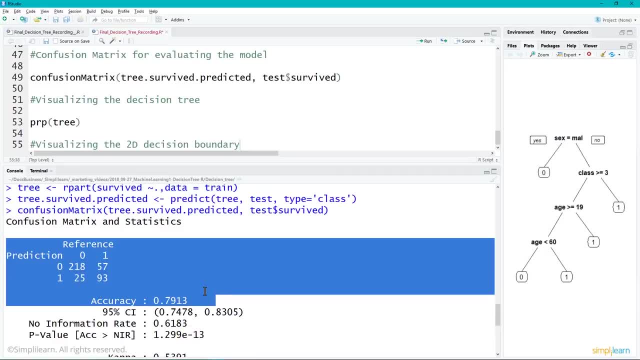 Other data scientists care about the p-value and the information rate and information like that, But this is really the core right here. This is how much data and this also shows them how much data was looked at. So you have a. You can actually. 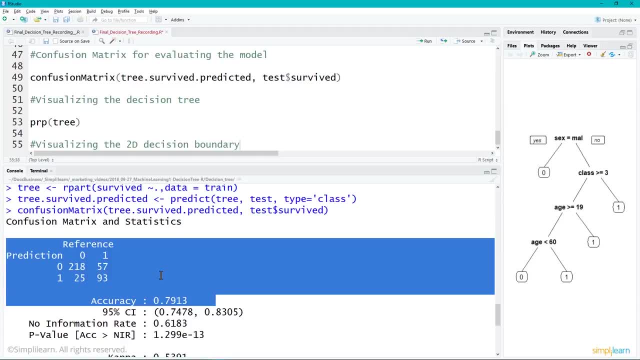 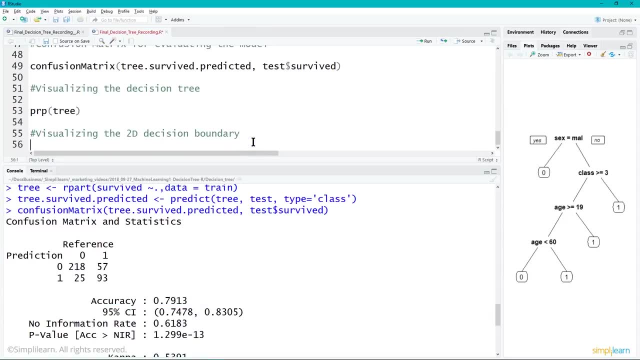 Just add these numbers together and you can see how many different people were in this particular data set, how many lines in the data set. But we go ahead and visualize the 2D decision boundaries. Let's take a look at that. That's kind of fun. 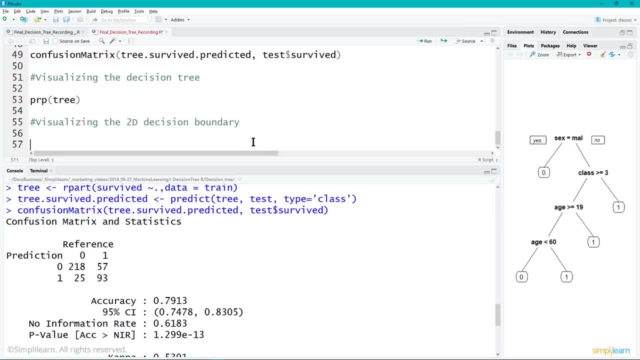 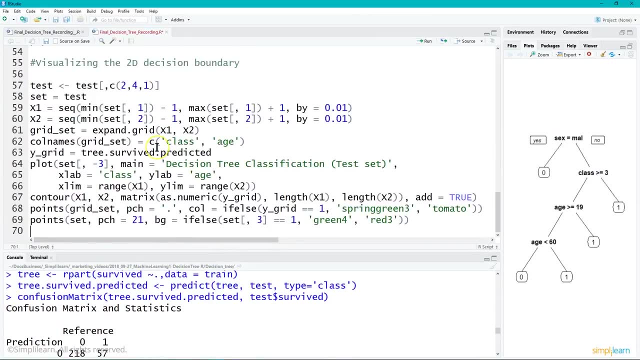 It's a little bit more complicated, so I'm not going to go into it in too much detail today. Now the guys in the back put this code together for me, which is great, So I'm just going to pay settings. Like I said, we're not going to go into it in too much detail. 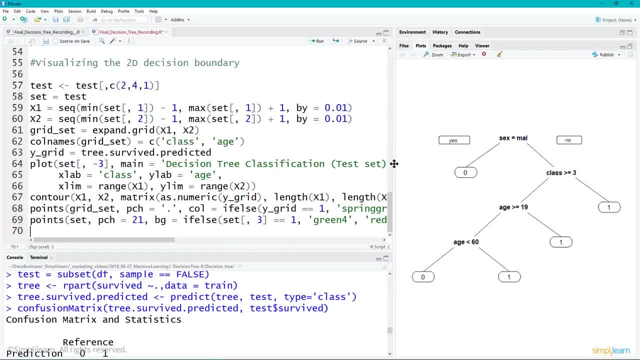 I want to just show you that there's some other ways to display the data. That is not just this nice little tree Over here which gives us a little bit more, maybe, view of what's going on As you dig deeper into data. that becomes very important. 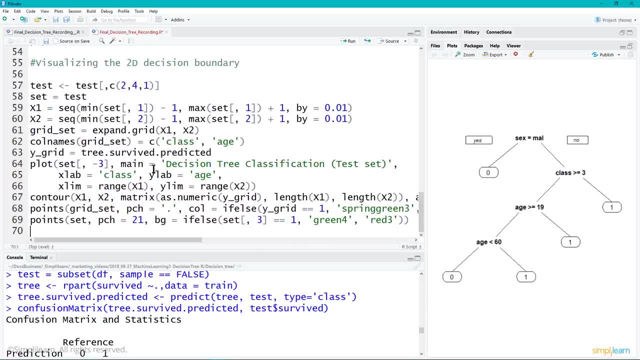 It might not be something so simple where you can look at, in this case, one, two, three, four nodes. So they have four major nodes that they split the data in. So we're looking at this, We're going to go ahead and create a set test equal to test comma C, two, four, one. 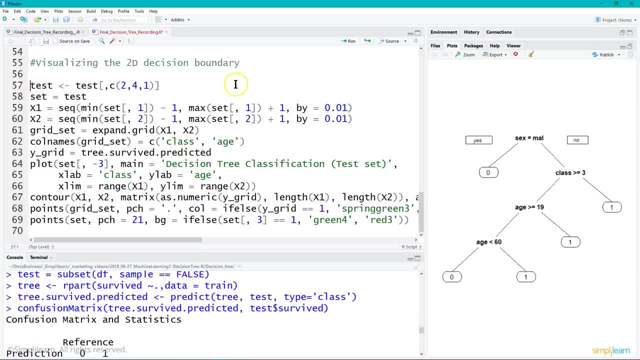 We're just assigning color column to go with the data. Okay, that's what that is. And then we're going to take set and have it equal to test And we'll do X one And we're going to set that equal to minimum set of one minus one, max set of one plus one. 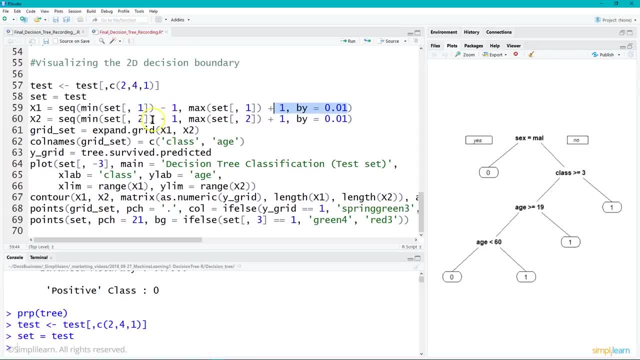 by equals point zero one. They had to play with these numbers a little bit to get this to look right. So we're creating a sequence on here from our the set we created, So our test set, And then X two Is also creating a sequence based on different values. 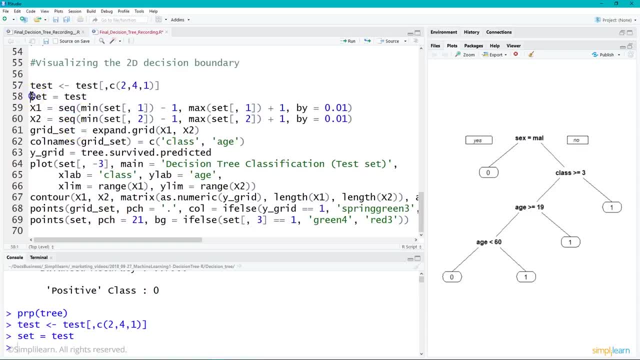 And then we're going to put that all into a grid. So let's go ahead and run that through all the way down to the grid, And they'll make a little more sense when we add the column names to the grid. Okay, so we'll set our test. 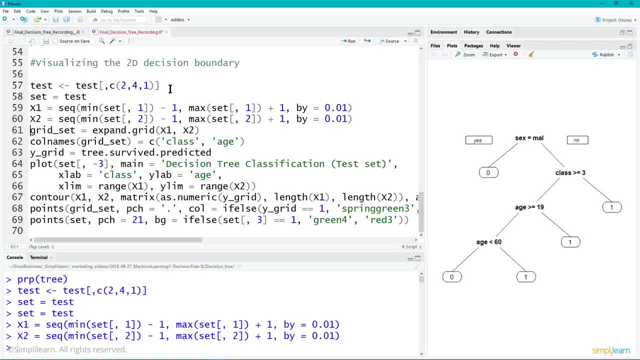 We'll create our X one sequence and our X two sequence. Remember, a sequence is just like in this case, starting with point one. It's like point oh one, point oh two, point oh three, point oh four. So we're going to create a grid with all these values. 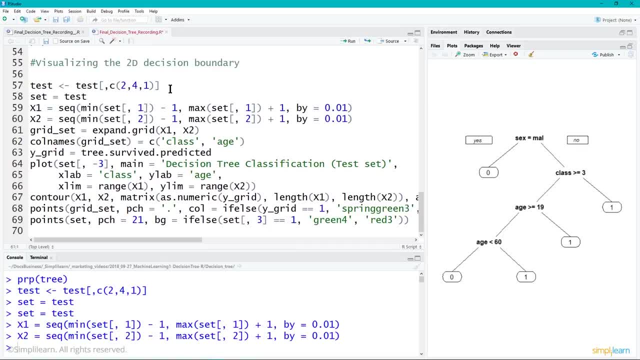 Separated by point. oh one. So that's all we're doing right now And let's go ahead and set that up. There's our grid. And then we want to go ahead and create some column names And for our grid set, we're going to have our C class and age. 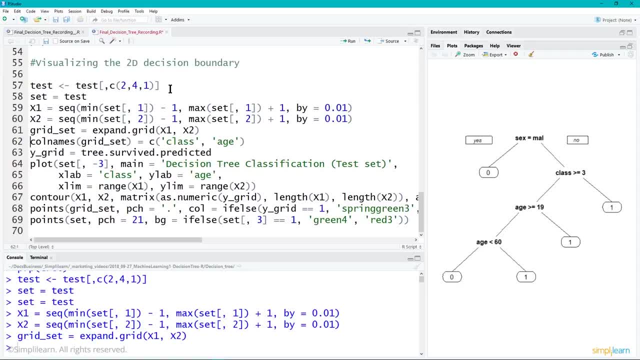 So we're just doing the class and the age on here. Remember we did sex also before. So it's just class and age on this chart that we're pulling out And we're going to create a Y grid And the Y grid is going to equal. tree survived, predicted. 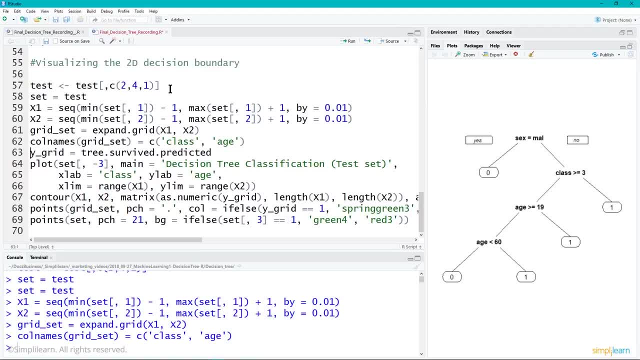 Okay, so here's our Y grid and our predicted values on there. Now we're actually going to do something. We're going to plot, and we're going to plot the Y grid. Oops, hold on, Let me see what's in here. 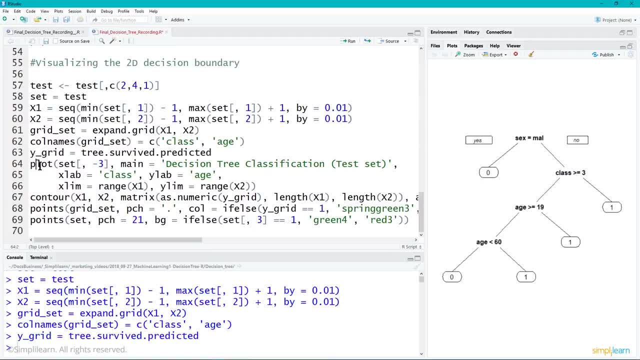 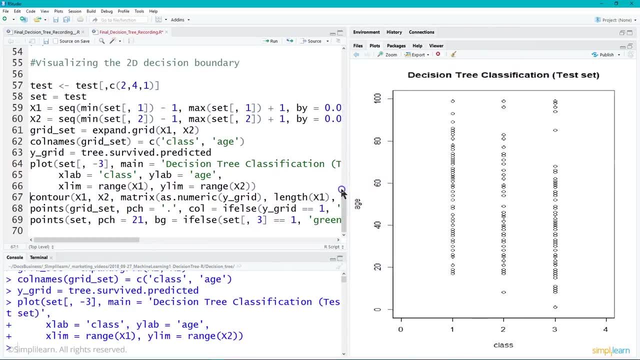 And let me go ahead and just run the plot. It's got to be the. There we go. So let's take a look at this and see if we can make a little sense of this code and what's going on here, because a couple of things going on. 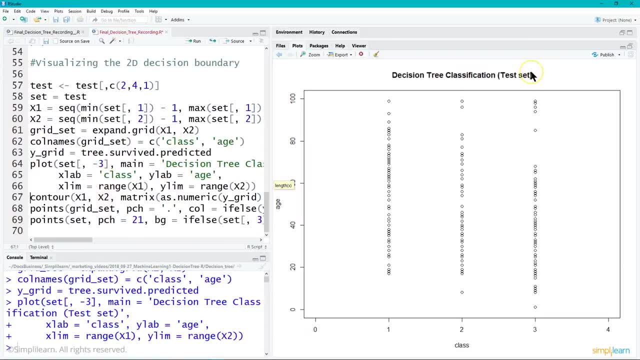 What we've done is we've plotted a decision tree classification Data set. We've done our plot and we have our set. So our set is equal to our test data. And then we have our main. We went ahead and give it a name: decision tree. 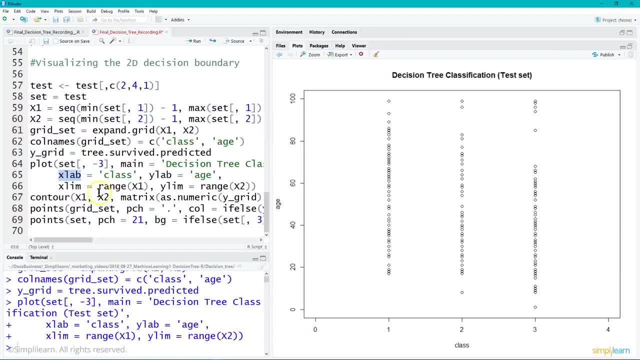 And then we have our X lab And our X limit And we've set those up as class with our Y lab equals age and our X limit equals range X1 comma. Y limit equals range of X2.. And when you look over here you can see that we have age on the left. 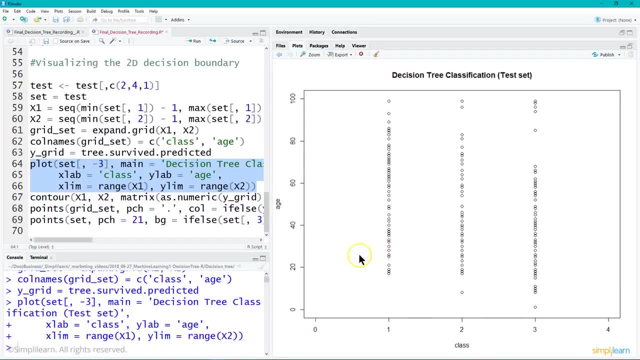 And then And class on the bottom, And so based on age and class. And so once we put in this nice graph here, we want to go ahead and add our contours and our points. So let's go ahead and run that And I'm going to run all three of these so we can see all the colors come in on the graph. 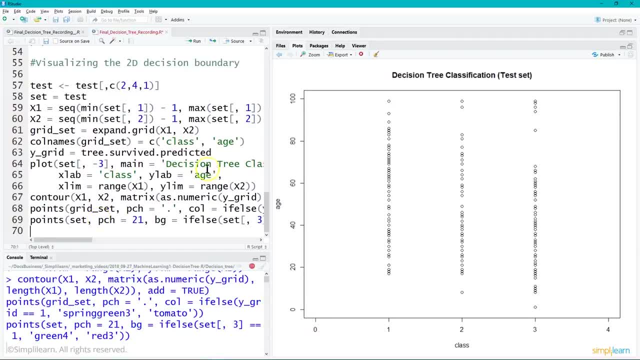 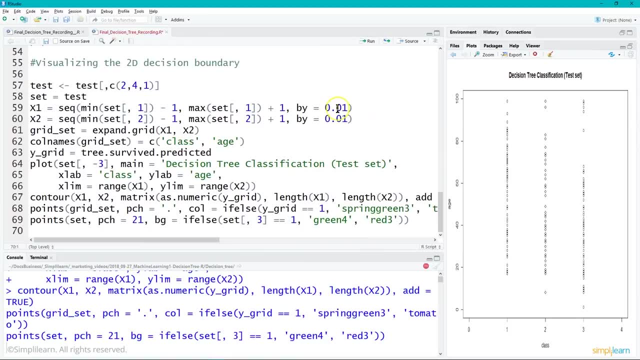 And this is actually going to take a little bit Because, remember, you can make it go a little faster by changing a couple of the notes up here. Well, we did 0.01 from the min to max. By changing that to 0.01 or other values, you can actually run a little quicker. 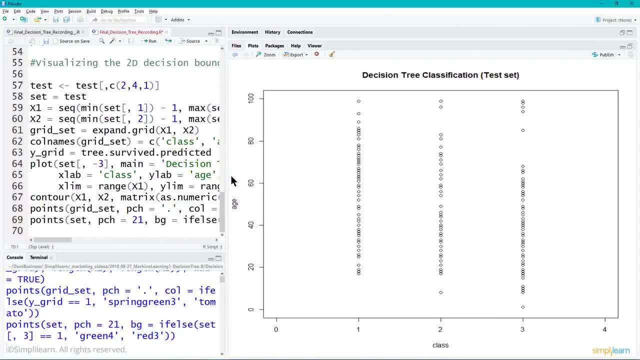 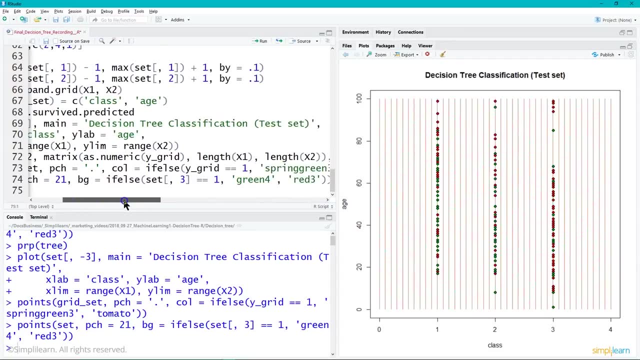 And we're going to create a nice little decision tree classification test set Just to see what that looks like and how that data displays. Now that was taking so long to run with 0.01.. I went ahead and just did a 0.01.. 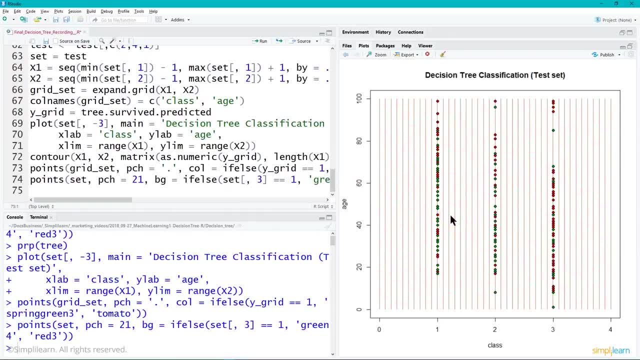 So, instead of filling the whole page with different colors for a really pretty view, Now I just have these different colored lines coming across, And it gives us another Model that we can show for whoever you're working with, in this case Your shareholders of the company. 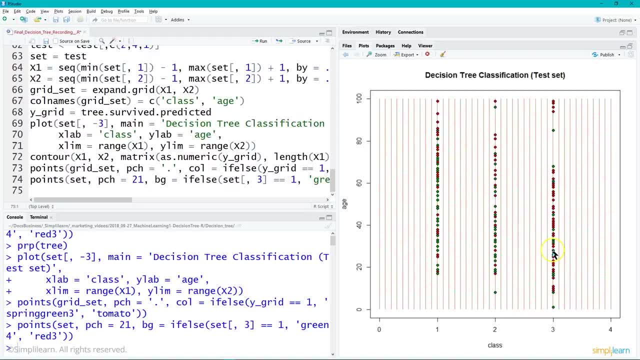 Or the individuals who you're posting to the web for, And you can see where we have the green and the red, And we've set those up to identify from the decision who's going to make it and who's not, Based on age and class. 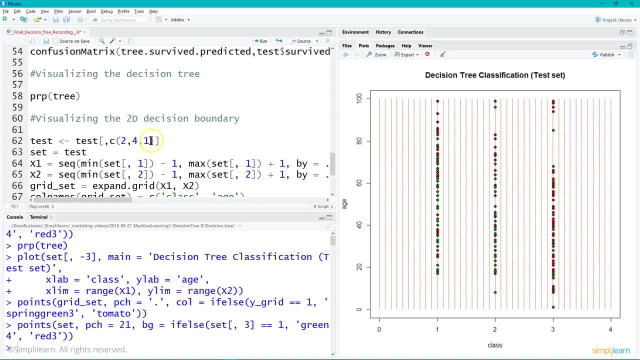 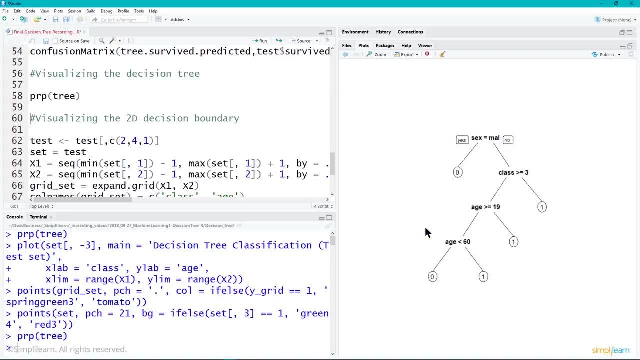 Now, my favorite one on this- And I'm going to go back and just highlight this really quick- Was- let me just rerun that: Go back to PRP tree where we display the tree And that's where we split it in part. 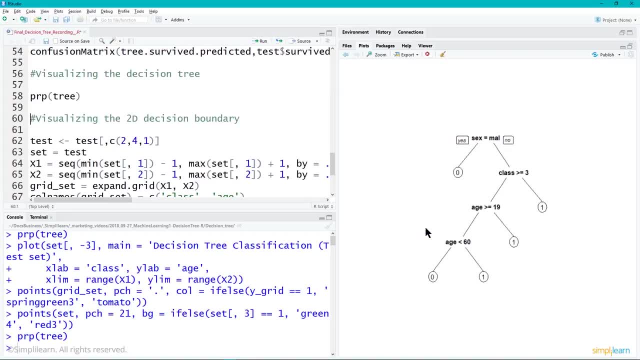 Because this information Gives us some keys that we can then use in other models. So it's good to know that sometimes what you're taking comes out And maybe you create a bucket for people under 19.. Between 19 and 60 and over 60.. 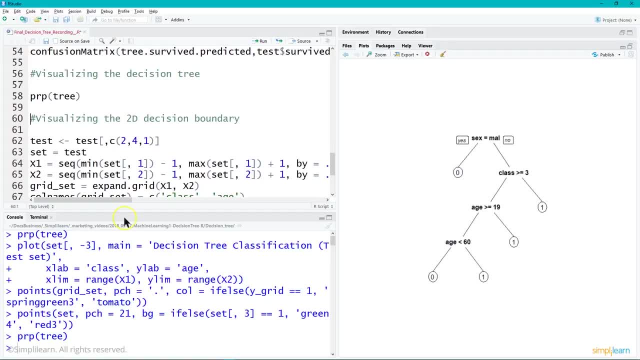 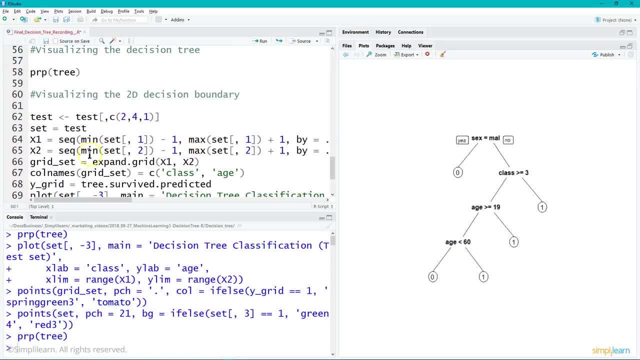 And different things like that, So you can actually put people in buckets In a class age split. Just a quick note on there. Again, you know lots of different things from which you can display the data And you can see how we use the decision tree to figure out. 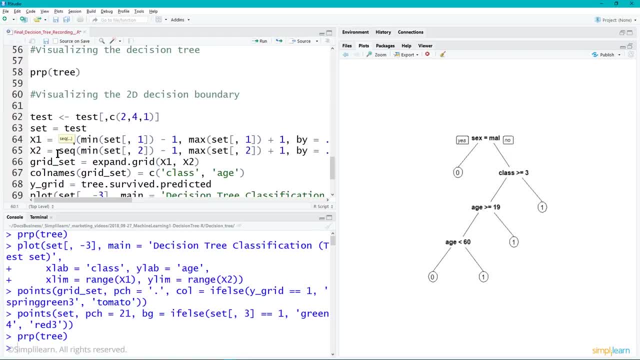 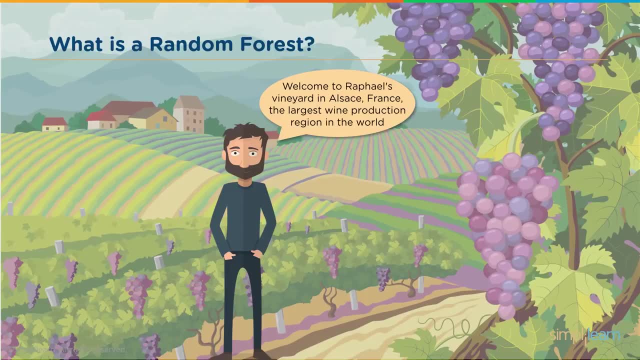 Chances of somebody surviving based on their class and their age. What is a random forest? And welcome to Raphael's Vineyard- And I don't even know how to pronounce that- In Alsace, France, The largest wine production region in the world. 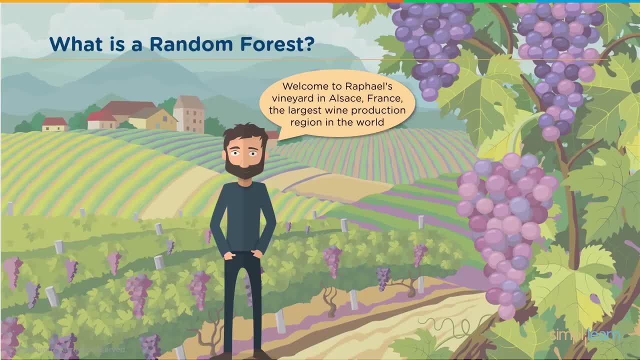 So they have centuries of wine production And data they've collected on how to make the best, How to make their grapes and grow them, And how to properly get the right grapes and ferment them. Like Raphael, Wine makers around the world are facing a grave problem. 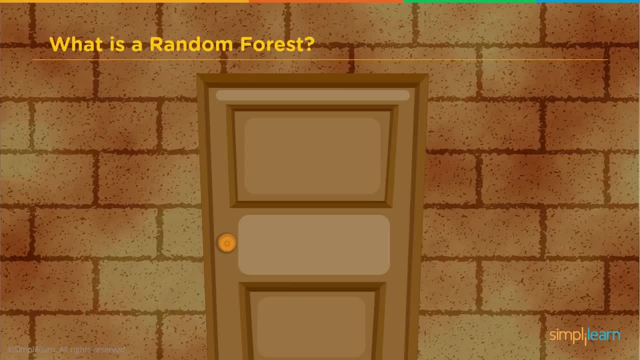 So let's meet the man himself and try helping him out. What is a random forest? And we're going to come back to the vineyard, But we're going to look at some other examples along the way too. Open up the door. 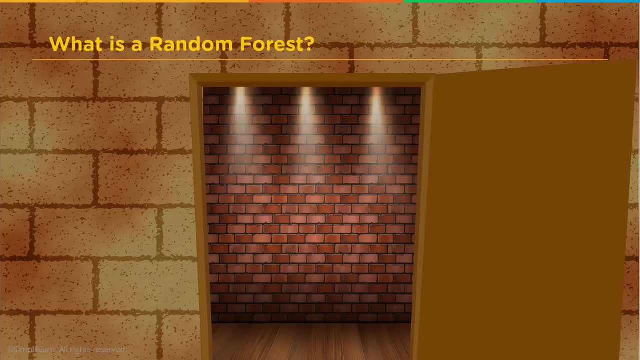 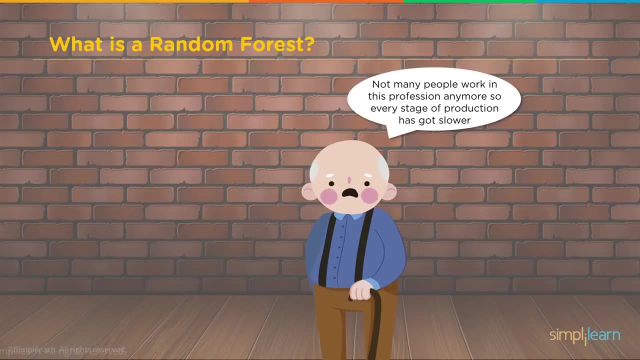 And of course, here comes Raphael. Probably, I'd probably look closer to Raphael than I do to the young lad with the beard. Hey, Raphael, So tell us how it's going. Not as good as before. Not many people work in this profession anymore. 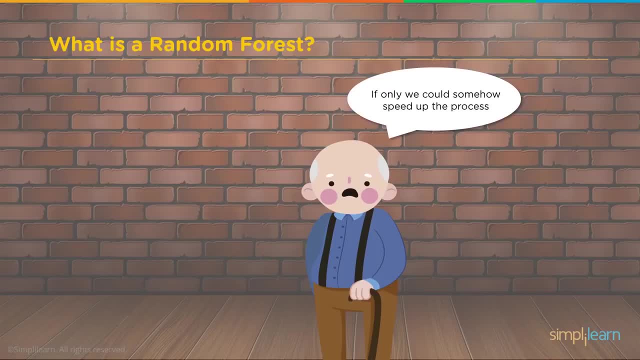 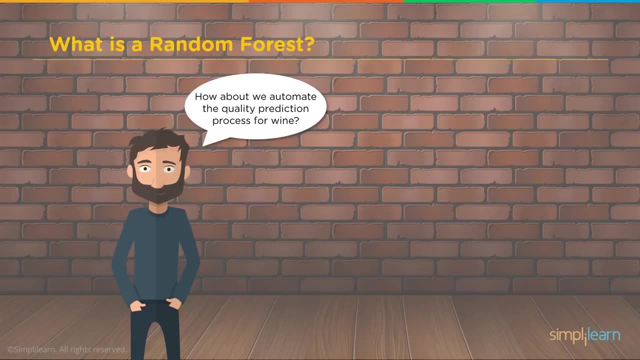 So every stage of production has gone slower. If only we could somehow speed up the process. Well, lucky for you, I'm a machine learning engineer. How about we automate the quality prediction process for wine? Let me begin by telling you what machine learning and random forest is. 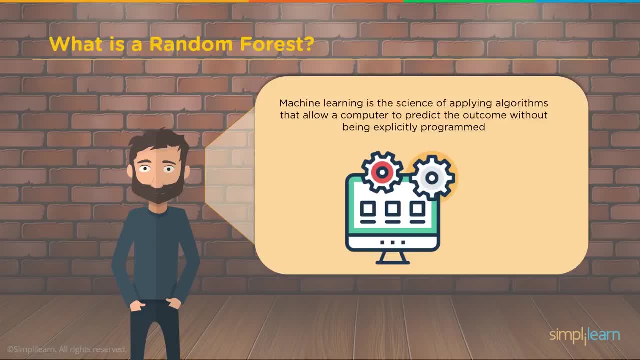 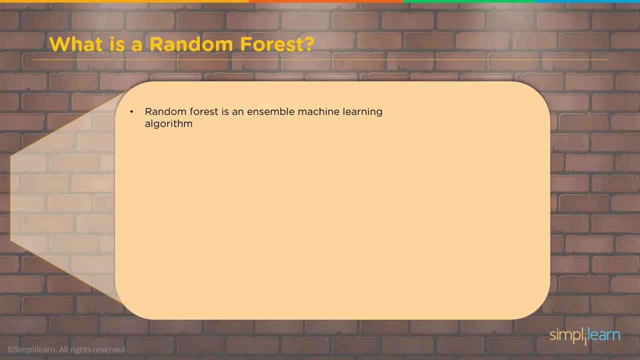 Machine learning is the science of applying algorithms that allow a computer to predict the outcome without being explicitly programmed. Random forest is an ensemble machine learning algorithm, So we're bringing in different pieces and then putting those pieces together. It operates by building multiple decision trees. 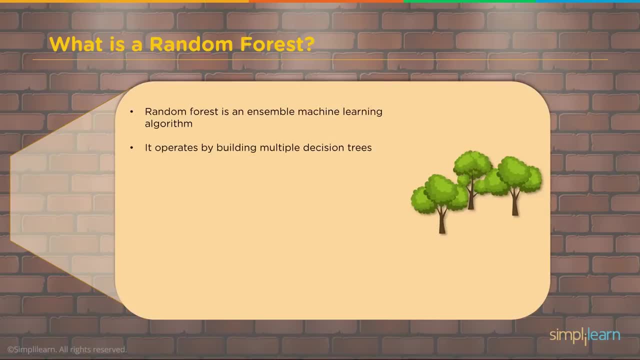 Remember I told you we don't want just a lone tree out there and we want a forest. They work for both Classification. If you remember from part one, We had our vendor With his broccoli and oranges. I think he also had carrots. 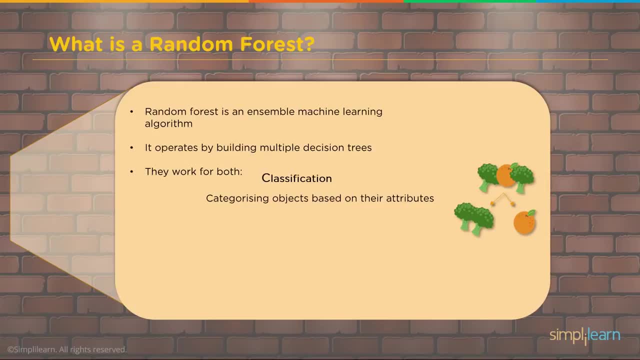 And it also the output given by the majority of his decision trees is the forest final output. So if you have a number of decision trees- You have five decision trees and four of them say it's broccoli, Then it's probably broccoli And you can also use it as a regression model. 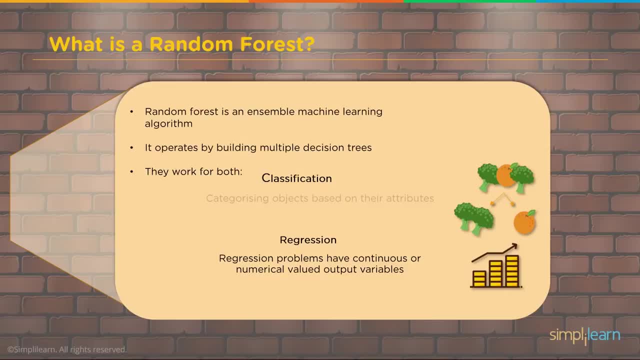 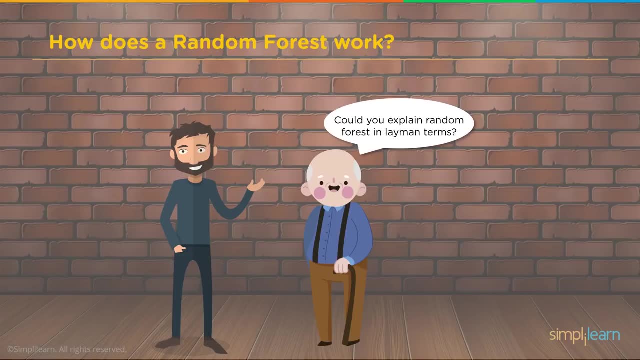 The output given by the majority of decision trees is a forest final output. Just like you do in classification, You can also come up with actual values and numbers as a regression model. Could you explain how a random forest works In layman terms? 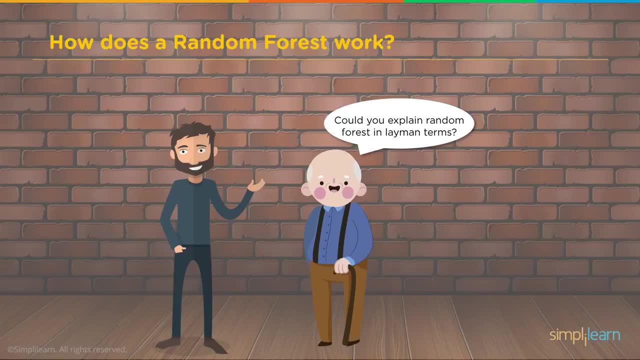 It's always a good thing to explore the information On something a little bit easier to understand and see. Sure, let's consider the case of Sam, a high school student. This so reminds me of my own high school student who's just started his first year in college. 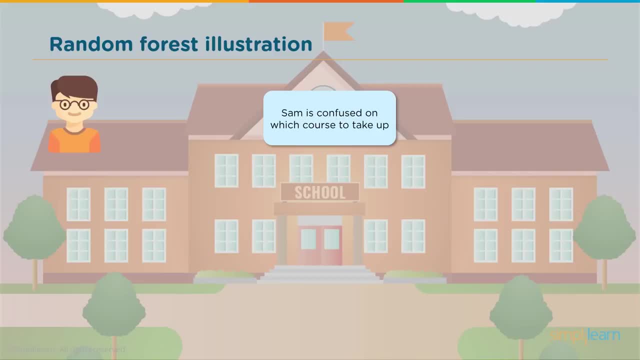 Asking all his friends. So Sam is confused on which course to take up. So he's trying to figure out what his next class is going to be at school. Should he take music lessons, dance lessons, math science, maybe social studies? 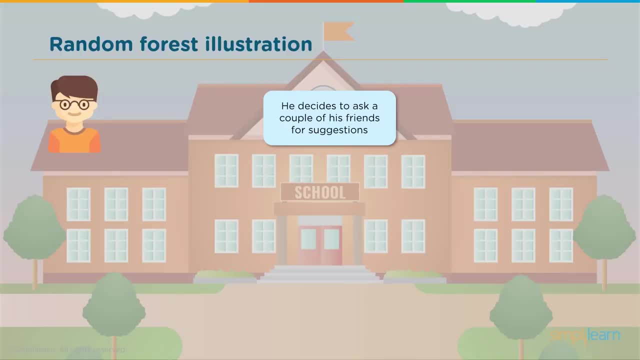 So he decides To ask a couple of his friends for suggestions, And Sam approaches Jane first. So he comes up to Jane and says: hey, which of these classes should I take? And Jane asks Sam a few questions based on which she can suggest. 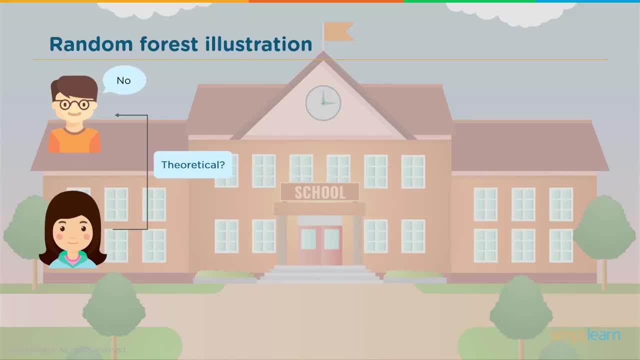 Theoretical. Do you like theory? No, He doesn't like the theory part Calculative: Do you like calculative? He goes. yes, I like doing calculations. And so Jane, based on a couple questions, goes. She has her little decision tree there going. 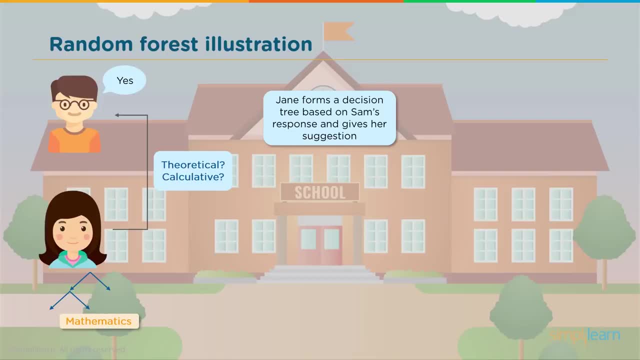 She goes: mathematics sounds good. So Jane's formed a decision tree based on Sam's response And gives her suggestion, And of course, this is based on Jane's views and her history And the data that she's collected over her years in high school. 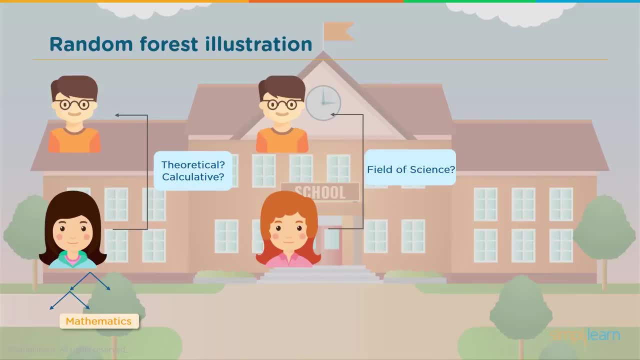 Next, Sam approaches Bella. Bella asks him: hey, do you like the field of science? And Sam goes yes, And then Bella goes: do you like new in industry? He likes new things coming up in industry And Sam goes yes And Bella goes. you know you should similar to Jane. 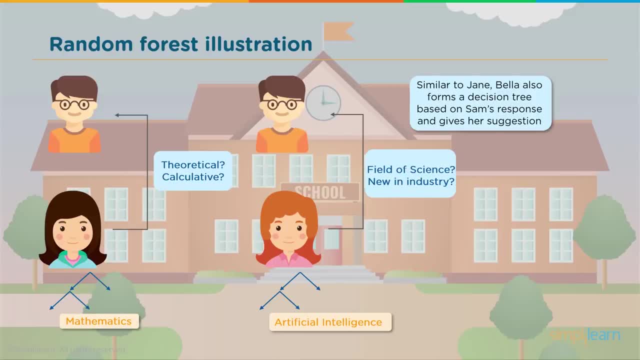 Bella also forms a decision tree based on Sam's response And gives her suggestion And says: hey, how about artificial intelligence? Sam's like: oh, artificial intelligence. So Sam next asks Terry for his suggestion And Sam goes: do you like scoring things? And he goes: yes, 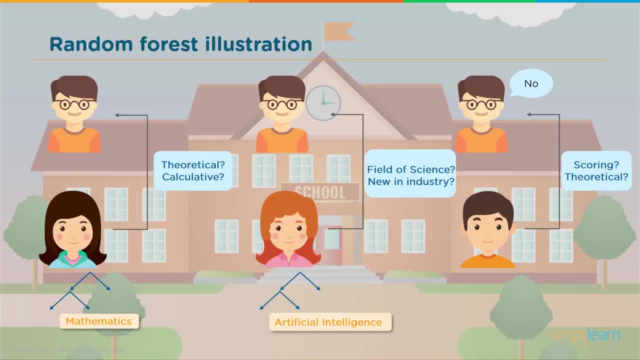 And he goes: do you like theoretical? And he goes no. And he comes up and says mathematics. So you have two people saying mathematics And one person suggesting artificial intelligence. Since two out of three friends suggested math, Sam decides to take mathematics. 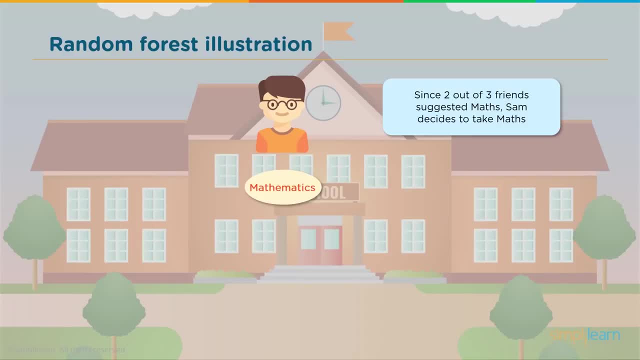 And there's a lot of subtleties in this example. It's actually a really good example. Some of the things we run into in data science Is when we collect data And we collect from different sources. We might have data from one source that measures one thing. 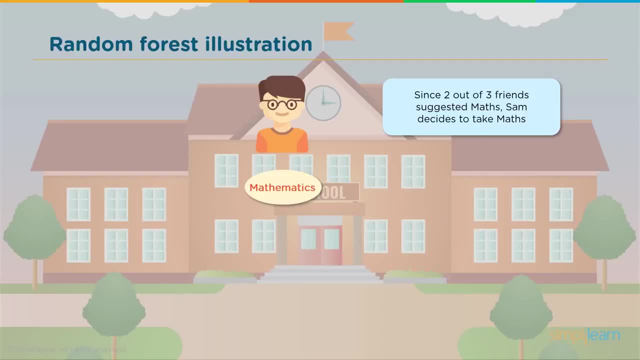 Or one set of instruments, And we might have data from another source that measures something else. We saw that with each of his friends are measuring different things And asking different questions. That's a little bit beyond the scope of this particular tutorial, So let's go back to our wine cellar. 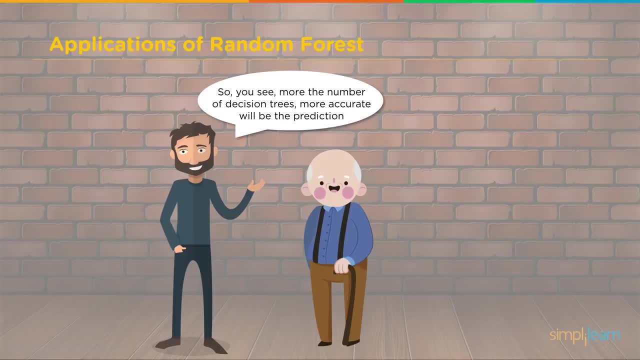 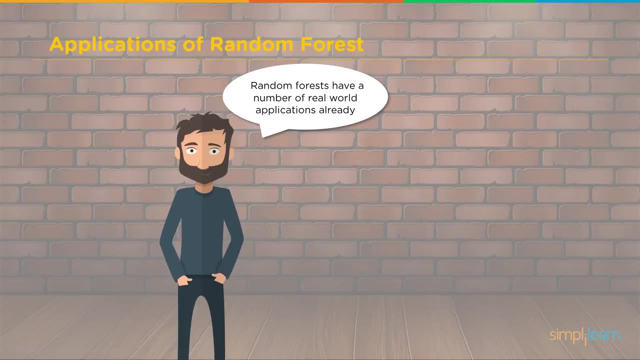 So you see more the number of decision trees, More accurate will be the prediction. Random forests have a number of applications in market already. If you've been watching any of our other tutorials, You'll see that these are very common We have in banking. 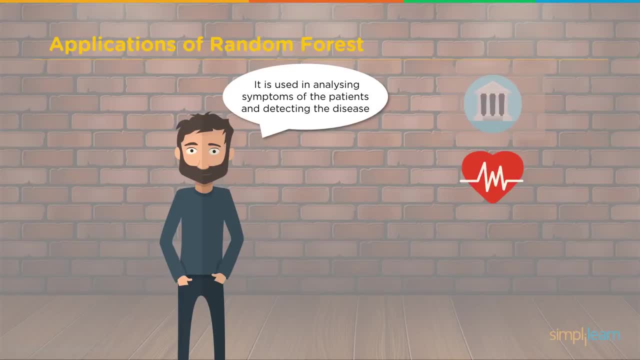 It can be used to predict fraudulent customers. It is used to analyze symptoms of patients and detecting the disease In e-commerce. the recommendations are predicted based on customers activity. Stock market trends can be analyzed to predict profit or loss. Most recently, I was watching a review. 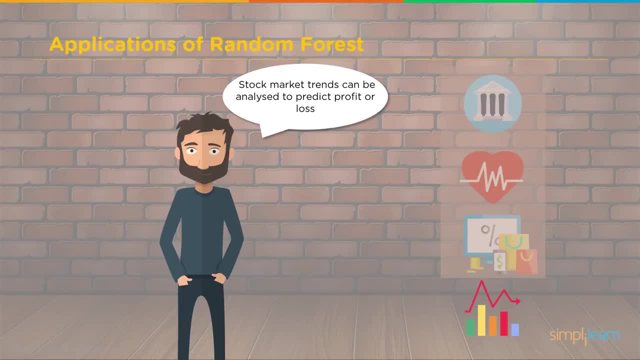 And I realized that there was a lot of information on weather here in the United States And the data they pull in for that, And one of the top weather places actually uses five different models. Random forest was one of them, I believe They use five different models to predict the weather. 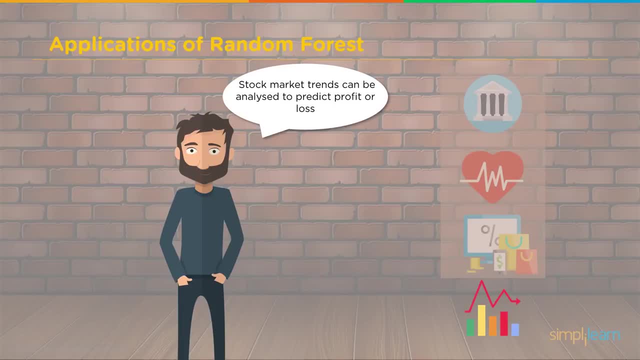 And, depending on what the models come up with And what's going on, Some of the models do better than others. I thought that was really interesting. It's important to note So when you see us repeat the same things over and over. 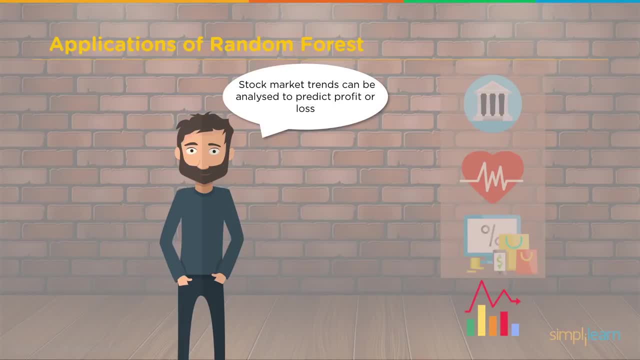 And you're looking at the different machine learning tools. So we can use multiple tools to solve the same problem And we can find the best one that fits for that particular situation. So let's see how that fits back in our wine production To help speed up the process of wine production. 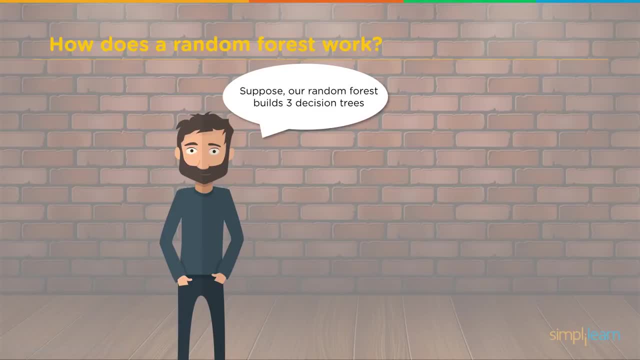 We will automate the prediction of wine quality. Suppose our random forest builds three decision trees. We have the first decision tree, Which is going to divide everything by chlorides Less than 0.08.. And it's either yes or no. And then it's going to look at alcohol greater than six. 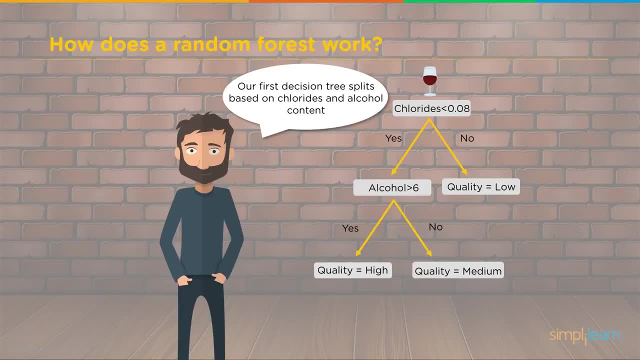 Yes or no, Quality equals high, quality not so good. And if the chlorides were greater than 0.08, quality equals low. So there's our first tree, And then our second tree is going to split it on sulfates less than 0.6 and pH. 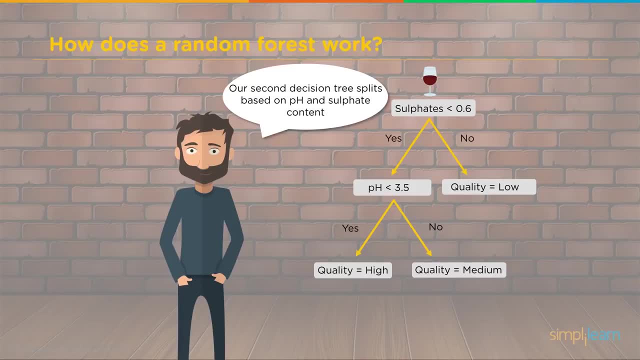 pH less than 3.5.. And again we have it coming down here that if the pH is low and the sulfites are low, the quality equals high. If the pH is a little higher but the sulfides are low, it's. 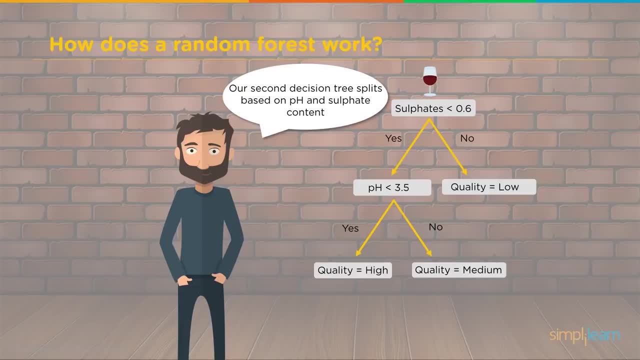 not so good. And if the sulfides are greater than 0.6, we have a quality equal low. And then we'll do a third decision tree. We'll split it based on pH And we can see below how that tree looks like. 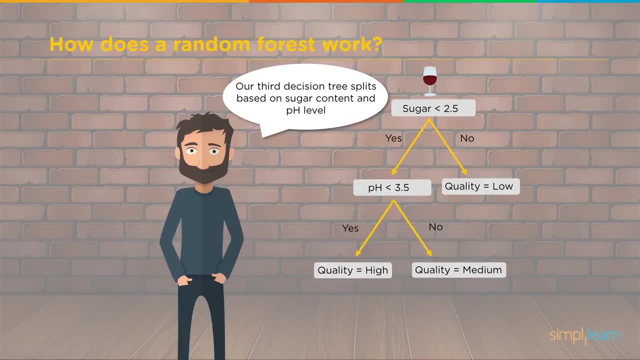 with our sugar less than 2.5. If not, it's a quality equals low, It's a real low quality. And if it is less than 2.5, then the pH decide whether it's going to be a quality high or not. so good. And if 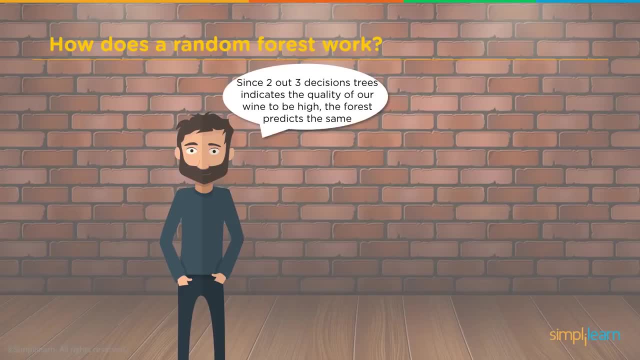 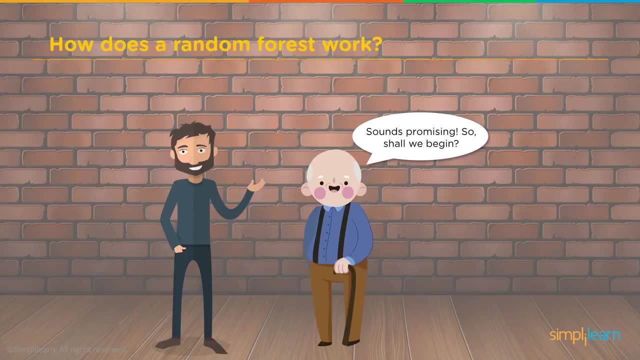 we track one of our wines down the list. we'll look at it. We'll say, oh, two out of three decision trees indicate the quality of our wine to be high. The forest predicts the same, So this sounds promising. So let's go ahead and dive in. 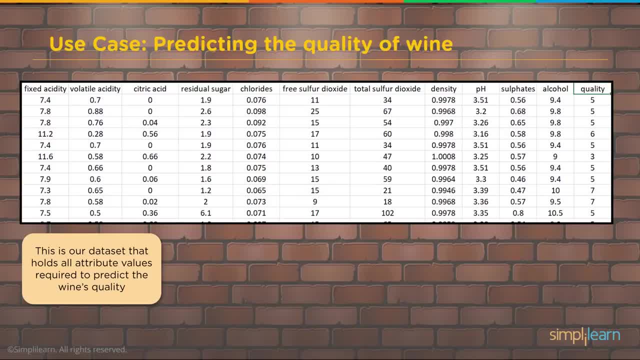 And see what that actually looks like. So this is the data set that holds all the attribute values required to predict the wine's quality, And I'll pull this up in a spreadsheet in just a moment. But you can see, here we have fixed acidity, volatile acidity, citric acid, all the way to. 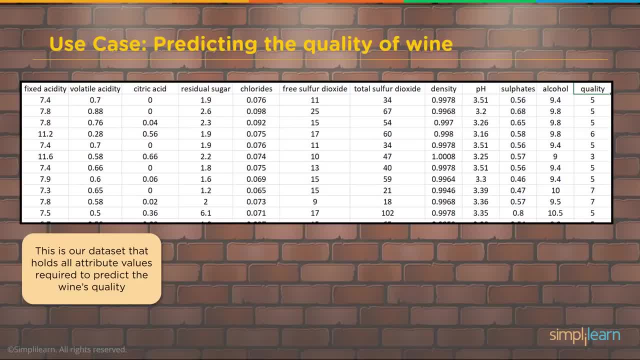 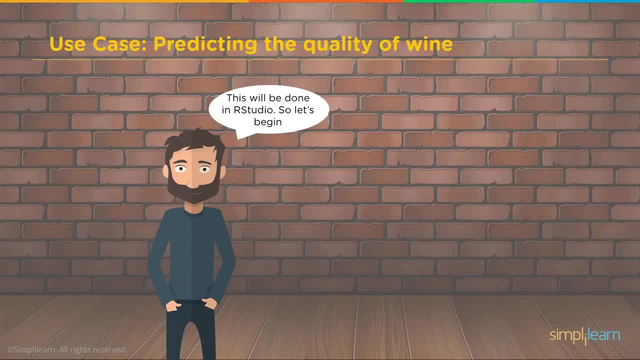 quality, And then quality is like a 4,, 5,, 6, or 7,, I believe, And this will be done in R, So let's go ahead and get started in our coding. We'll be using RStudio Before we dive into RStudio. 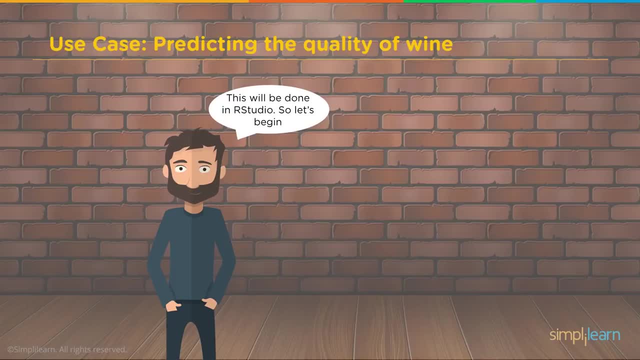 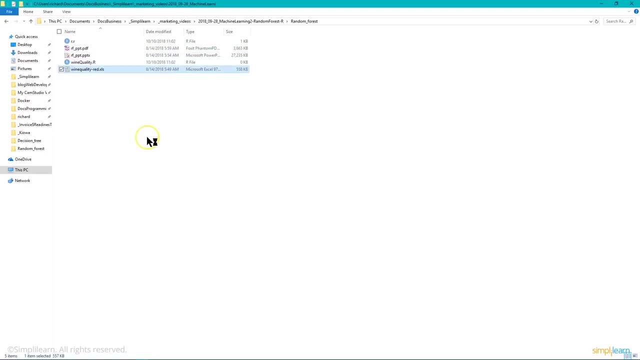 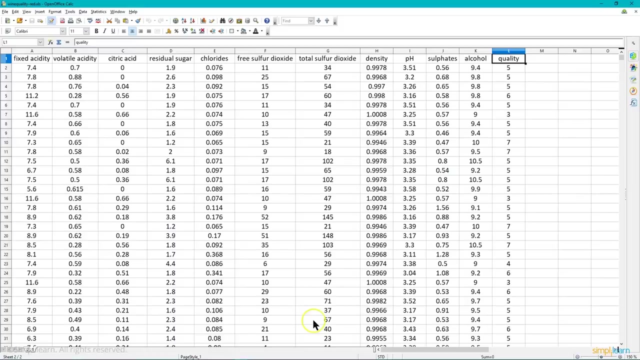 I always like to open up the data in the spreadsheet and look at the actual data that I have, And they've called it winequality-redxls. So it's a spreadsheet, a Microsoft spreadsheet, And when we open it up we'll see that it matches what we had before. 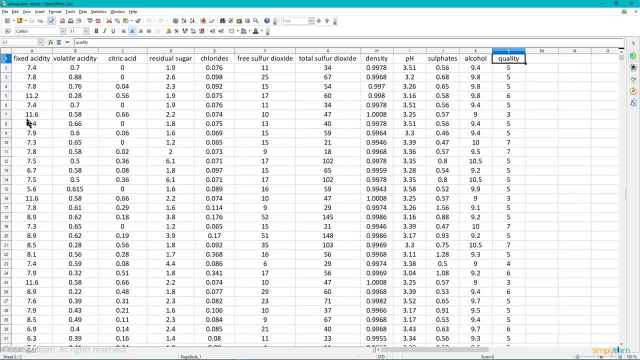 As far as the slide was showing us, we have 12 different columns. The first 11 are our features: our fixed acidity, volatile acid, citric acid- things you always want to look at when you're looking at your data. And we've done this before in the part one, But just a reminder. 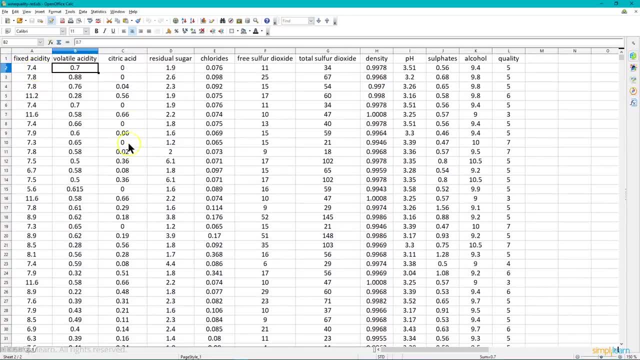 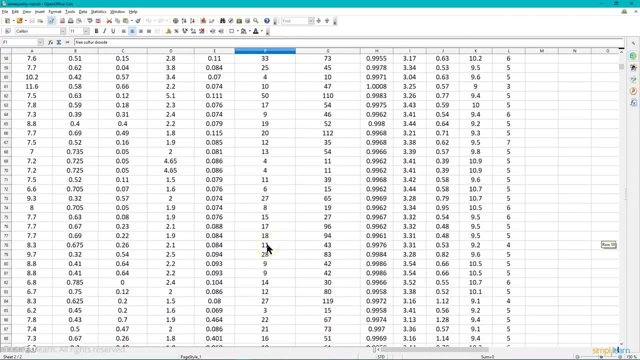 we want to note that we have decimal places here, float values in a lot of these things, especially the first number of columns. Our free sulfur dioxide looks to be an integer, but it varies a lot. So we have, you know, I see some values all the way up to 51,, 7,, 4.. So we'd 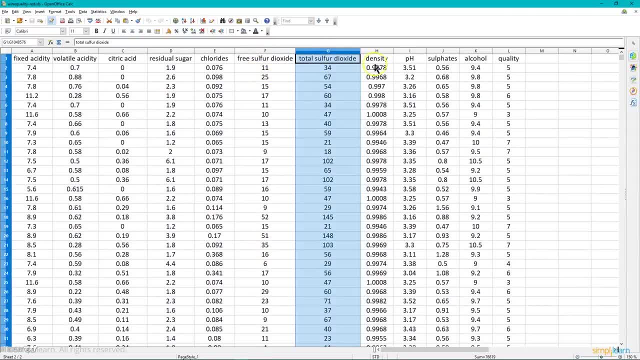 probably keep this as a linear model kind of thing. Same thing with the sulfur dioxides densities- again decimal places. sulfides alcohol Quality: I want you to note in the quality that we only have a few qualities here. This isn't like a spread. 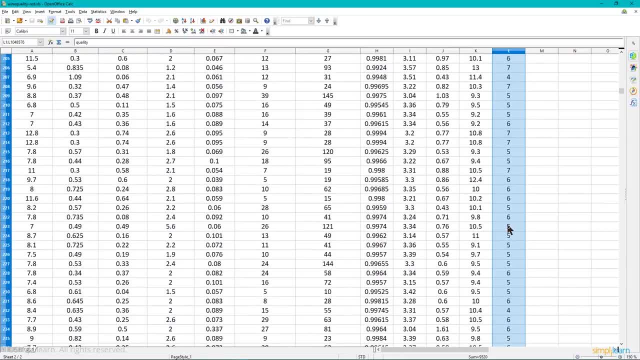 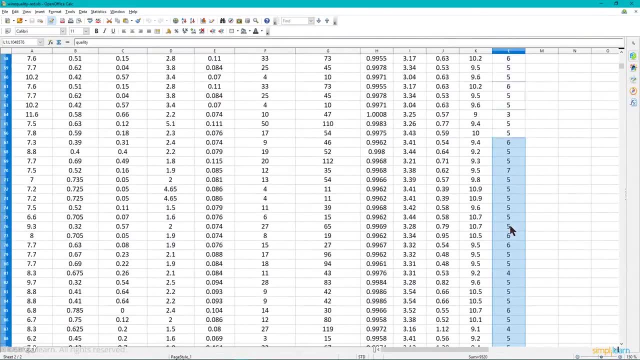 between 0 and 100.. It looks to be 3,, 4,, 5,, 6, and 7.. And so, when we start looking at the processes, we can have the option of either doing this as a series of integers or float values going from 3. 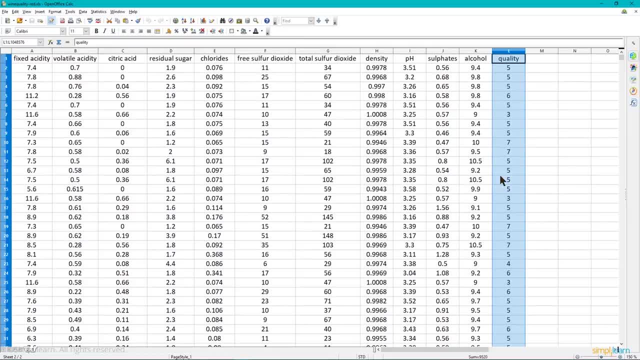 to 7, or we can convert that to a categorical, 3,, 4,, 5,, 6, and 7 being the categories, But we'll look at that in a little bit later. So let's go ahead and take a look at some of these categories. 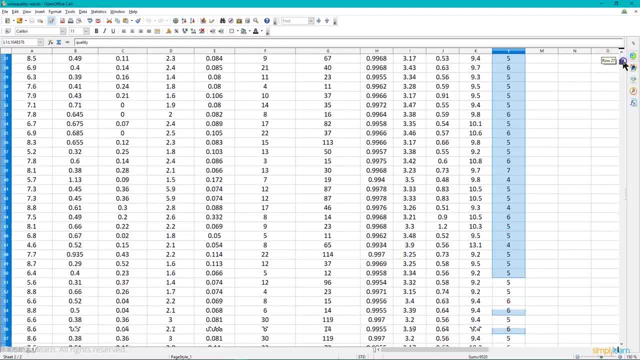 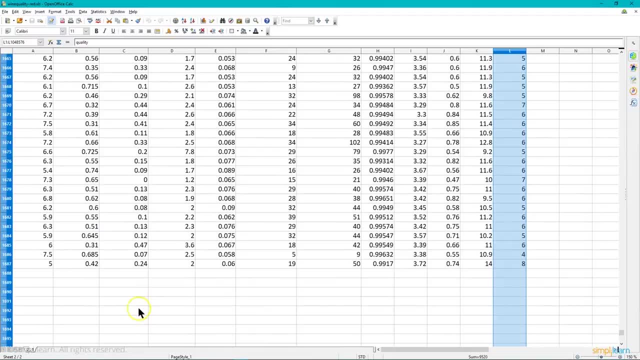 at that in the coding here in just a minute. And finally, you'd want to go ahead and scroll down through the data and just look for missing data or anything weird. Obviously, working with big data, you wouldn't be able to do that if this was spread across numerous computers and you had 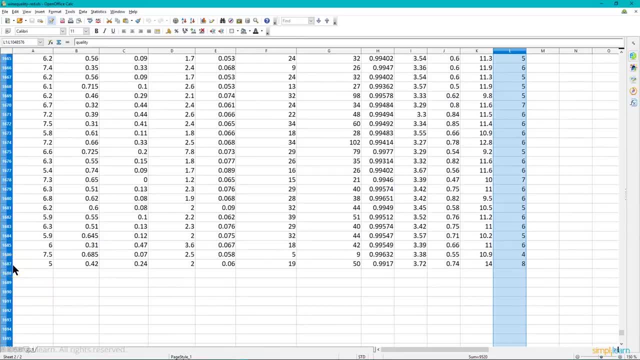 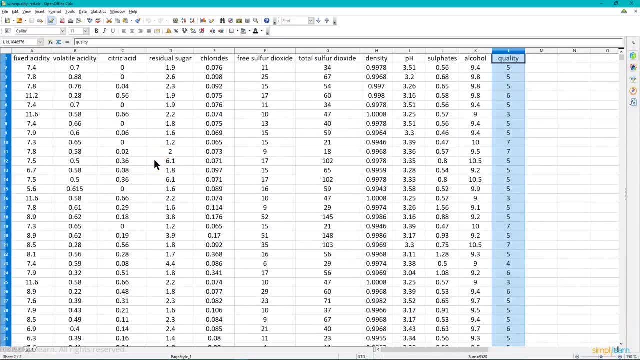 millions of rows. We have what? 1,687 rows here, So it's a nice size spreadsheet, still considered a small data set. Let's go ahead and switch over and let's take a look at this in the R. So here we are in our R studio And, if you remember, we had a little bit of a problem with 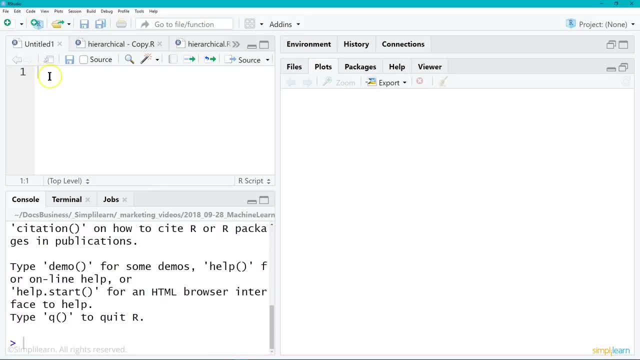 this. So, if you remember, it comes up automatically in three panels. I have my font on fairly large to help out. The upper left panel is a file that's open. You can have multiple files and tabs open, as you can see on mine. right now. I'll probably close most of those in just a minute And this is 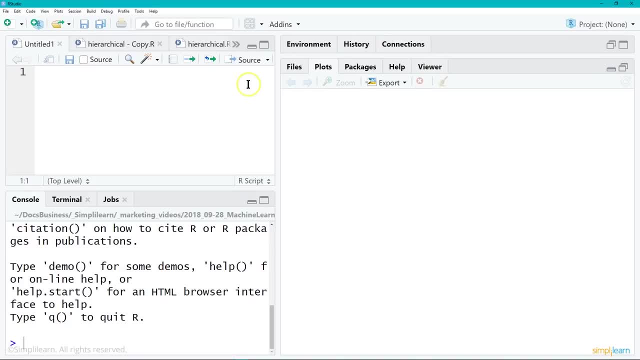 where you can put in your commands. Then you can execute these commands by either clicking on the run box or control enter is the hotkeys for that- And all that does is then puts that down in the console and executes that line of command. You could just paste these directly in the console. 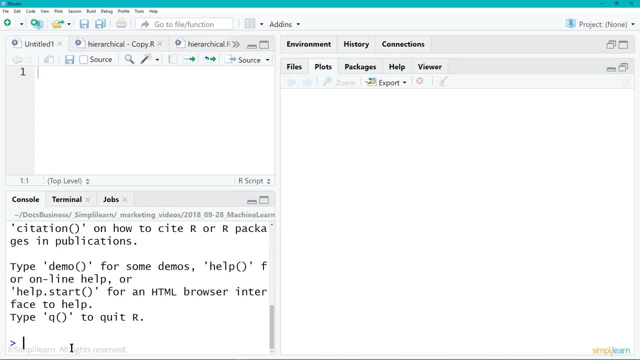 I've certainly been known to do that. if I'm loading up some data and I just want to take a quick look at it in R, because I'm doing the coding in something else, Or if I just want to do a quick explore before I dive in and figure out what needs to be done, that's one of the tricks you can do. 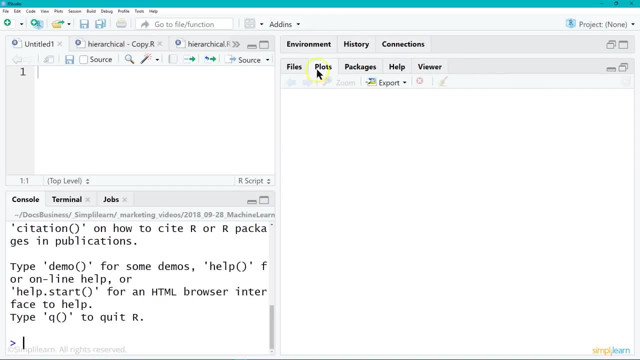 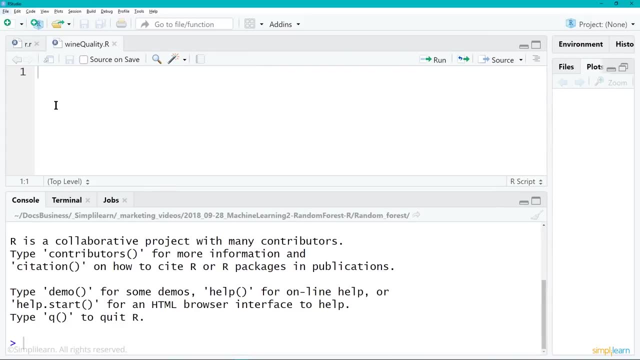 And then, on the right-hand side, we have our environment and history connections. We, mainly, are going to just be sitting on plots, and I'm just going to minimize this for right now, out of the way, while we dive in. If you haven't yet, I'm going to show you how to do that, So I'm going to. 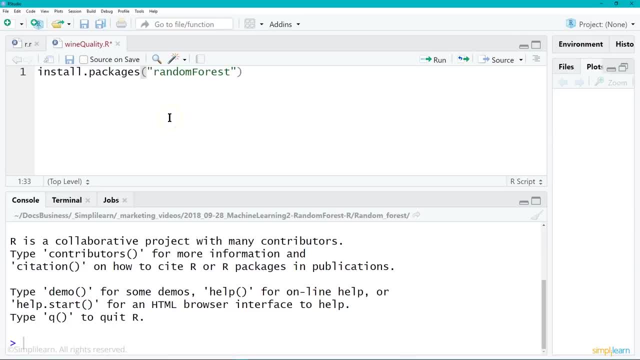 go ahead and install the package random forest. I'm not actually going to do that because I've already run that. We don't need to rerun that- But I am going to go ahead and import it into our project with the library and then random forest. We'll do the control. enter. You can always hit the. 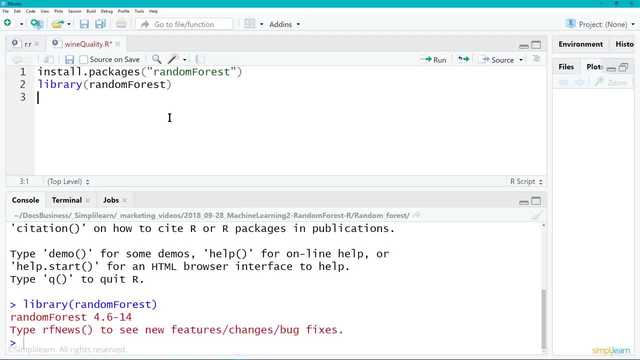 run button up there too, And then now the library has been uploaded in there And you can see down below- it takes this and just copies it and pastes it down below and runs it in our console. And then just a quick troubleshooting. 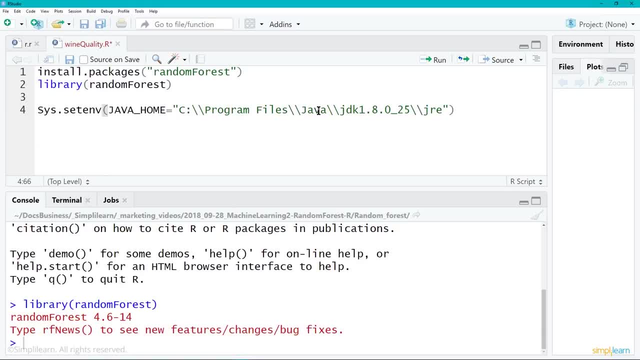 Same thing. My Java happens to be the developer's Java. The latest release of the developer's Java from last week is clashing with my R and rerouting my Java files. So your chances are you don't need to look this up or find out where your Java is, But there's a JRE folder. If you do have an error. 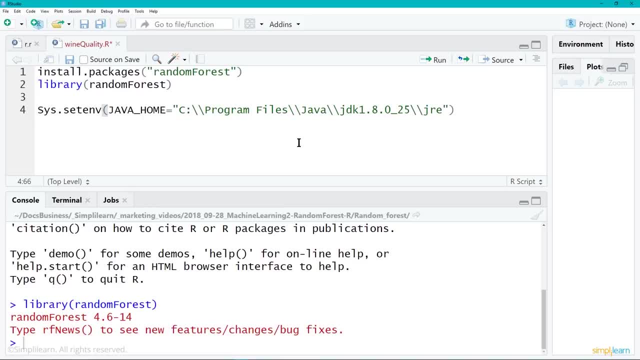 that comes up in the next library. you look that up, It's usually under program files, Java, and you'll see JDK, depending on what version you have on there- And then find that JRE folder And I'm just going to set the environment on there. 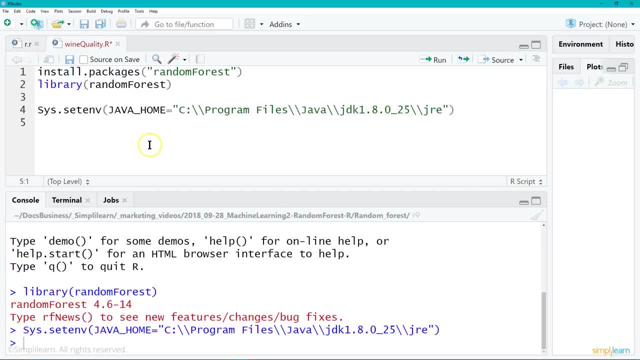 You have to do that every time you run the script. So with R there is a place in R where you can set it permanently, But generally it's set to whatever your system variables are set to. So you don't want to mess with that. So you just want to put this in your code if you're having problems, And you can always. 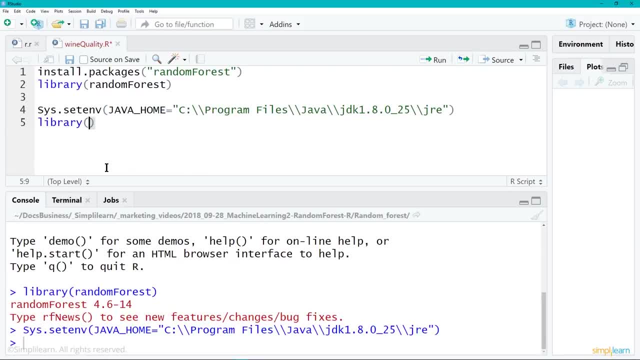 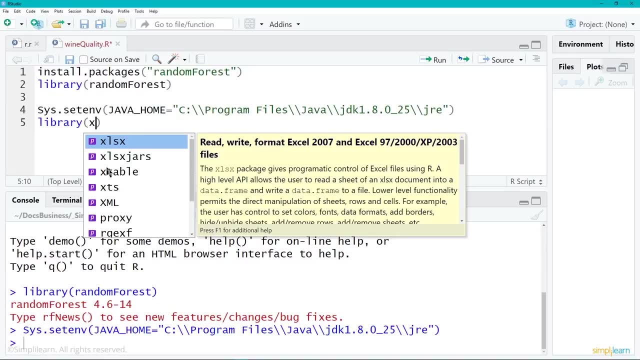 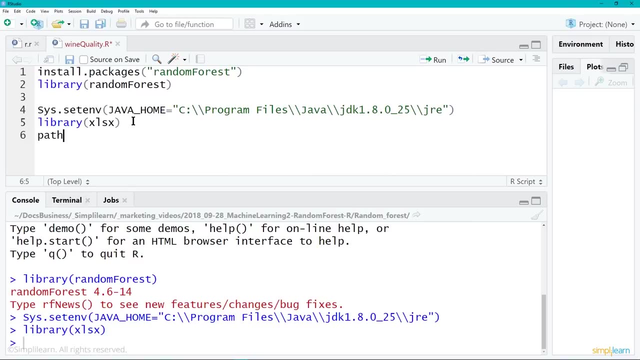 take it out. And then we need to go ahead and bring in another library And we're going to be importing the spreadsheet. So it's the xlsx, since it's a Microsoft spreadsheet, And I'll go ahead and run that. So I'm going to go ahead and add a variable path And let's go ahead and create a variable path. 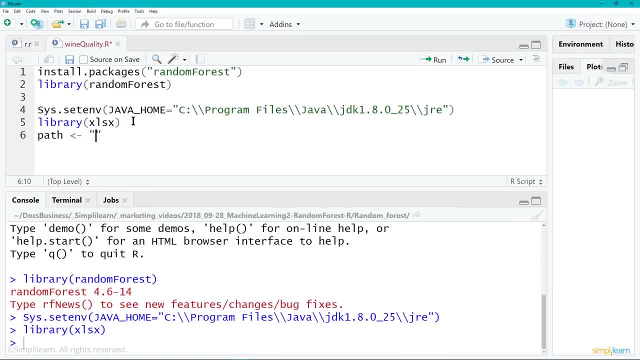 We're gonna assign to variable path the location of our folder, So this is a very lengthy one. You'll have to copy and paste it off your computer. My name is Richard and you can see under it's, under C, column users, Richard's documents, Docs, Business, Simply Learn, Marketing, Random Forest and then. 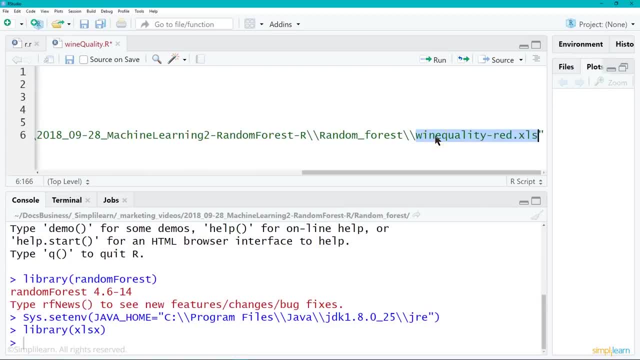 the actual file, which is wine quality dash READ dot xls. So I put in the whole path in here. You could also set up a specific path. You can also set a very simple path up here and here, and you could also set up a new path up here. You can also set it up a little bit less than a few things and you could. 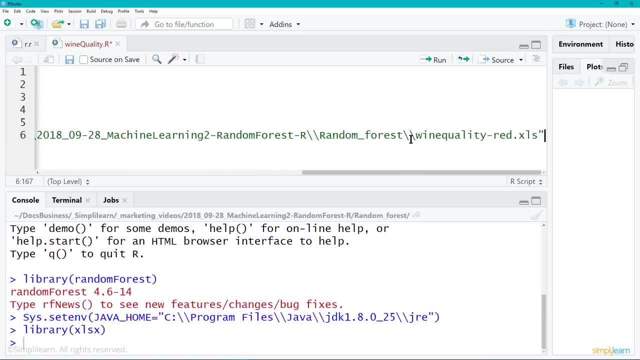 also set a very simple path. You could also set a very simple path up here and you could the computer path to whatever folder you have it in and then just use just the name of the file. but I went ahead and did this because it a lot of times it's. 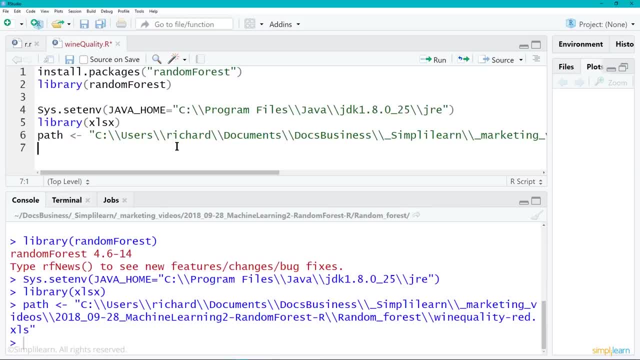 good to be aware where your paths are going, where you're pulling your data from. and again I went the ctrl enter so I could. you'll see that. that pushed the line down below and ran that line. so our path is now set and then let's create a variable called data. 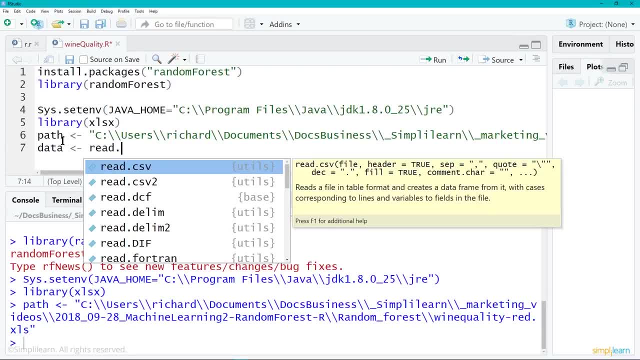 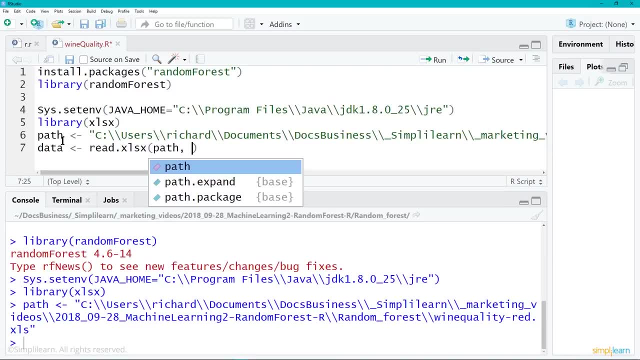 and we'll assign that to a read and we're gonna be reading: see where is it? there it is and spreadsheet. and before I put in, we need the path. but we also need one more thing on the spreadsheet: because it is an Excel spreadsheet, we need to know which page we're on. so let's go look that up and in the 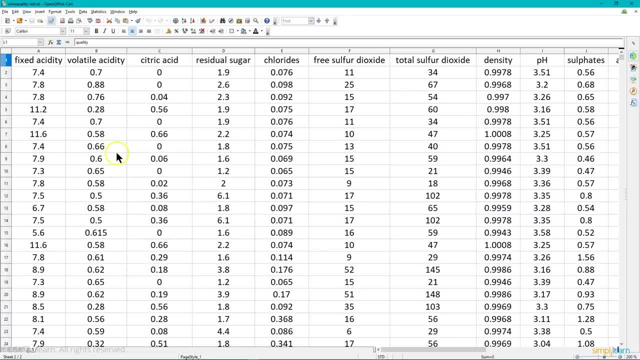 spreadsheets. this might be a little hard to see. it's it's a very tiny font down there, but you'll see the page tabs on the bottom. this actually has two different pages and we want page one for this project, so let's flip back over and put that in our. 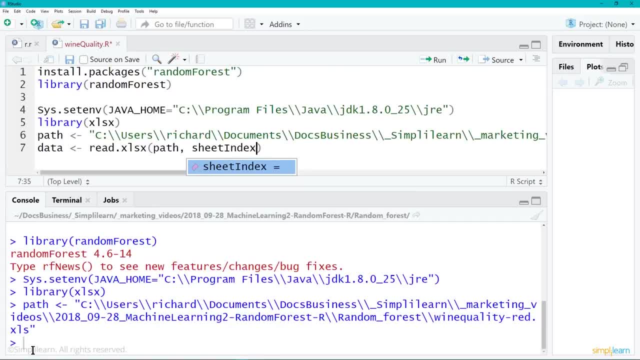 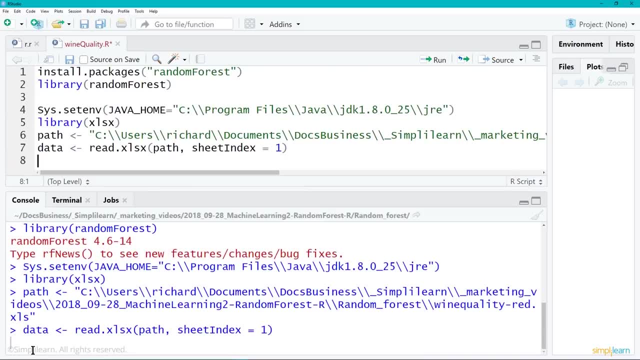 code and the term they use is sheet index. I always have to look that stuff up and it was sheet index of one. we'll go ahead and execute this so at this point. we've now loaded the data into the variable data and it's reading those and 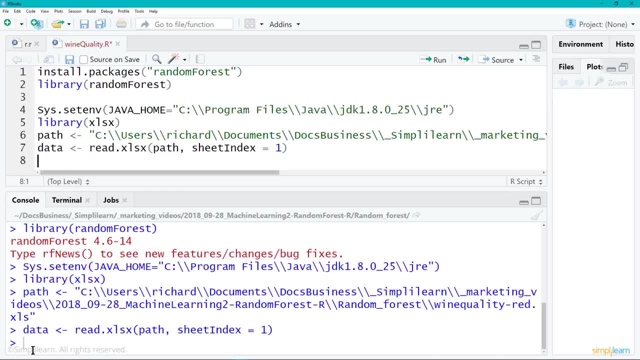 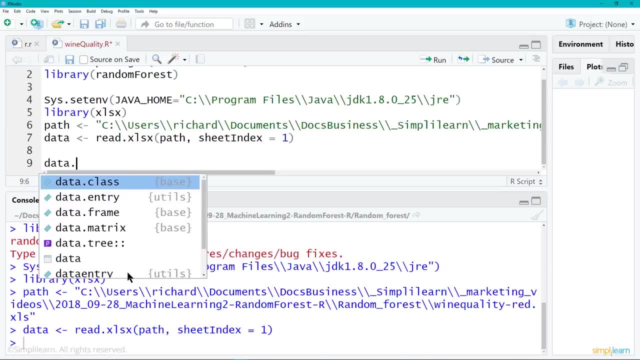 I think there was, like you know, a couple thousand rows of data in there, so it takes it just a moment to pull it in once I have my data in there. I always like to do something like this data and in I always forget. in R it's. 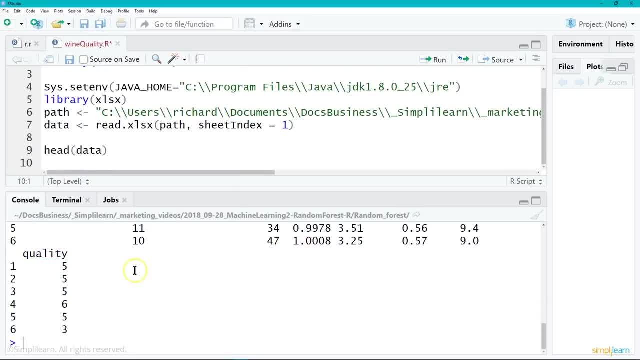 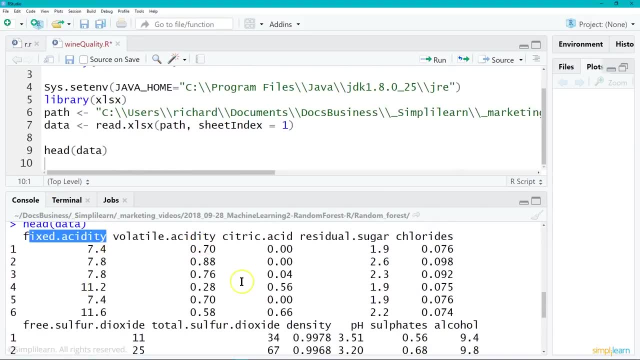 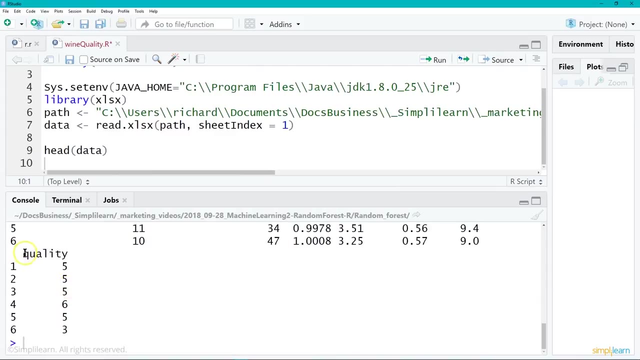 head data and we can run that and you'll see it prints out that what we looked at in the spreadsheet. so we have our fixed acidity, volatile acidity, citric acid, residual sugar, chlorides, free sulfur, all the different things. we're actually looking for quality, so you want to keep that in mind, that quality is the final. 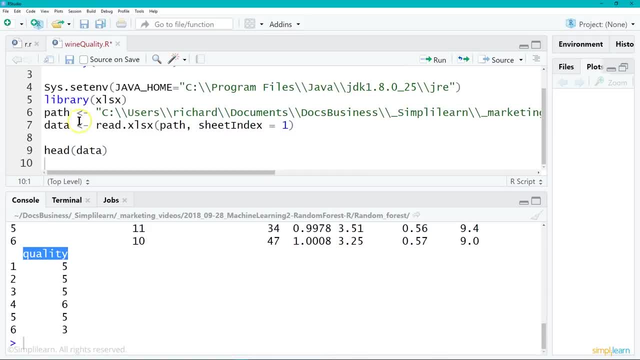 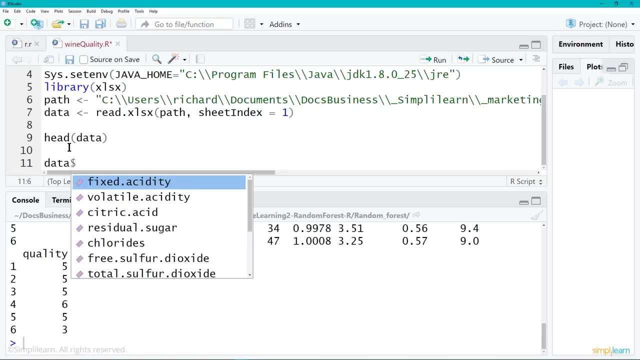 setting. is it a three, four, five, six? what is the quality on there? and the first thing we do is we're actually going to take the data quality and let me see quality. there it is in R. the dollar sign means that you're looking at one of the columns in. 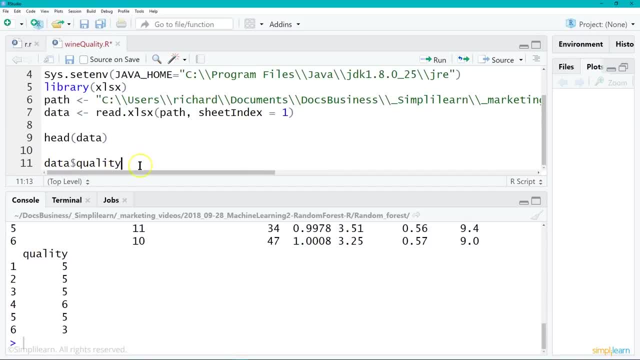 here, or features as it is. so we see data dollar sign quality in R. that means that's what we're going to be editing, and what we want to do is we want to change the quality just a little bit, and so we're going to set it equal to. 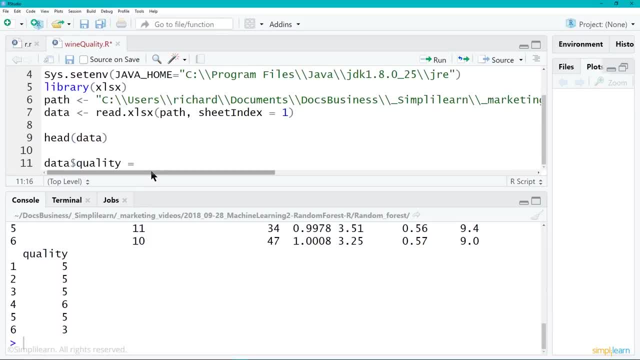 now we're not assigning a variable, we're altering it. so data dollar sign quality equals and we want to do as is one of the functions in R, we're going to do as a factor, and then data quality, because that's what we're actually editing on there and this stuff. 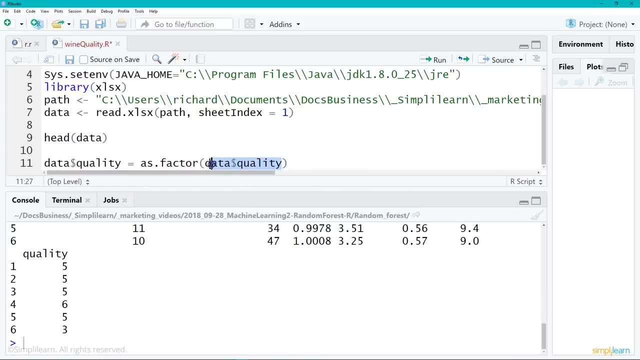 just for a second to look at this factor takes this and looks at the data as a categorically so. instead of it being on a continual scale of, you know, zero to a hundred or something like that, it actually looks at it as category of five, category of six, category of a category of cat, category of dog. there 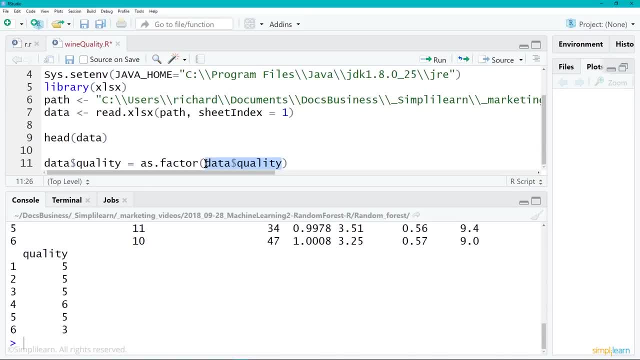 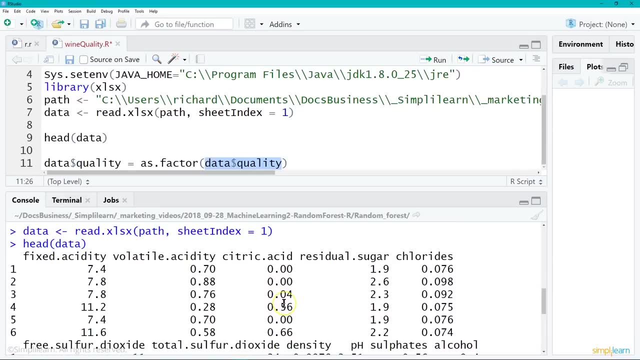 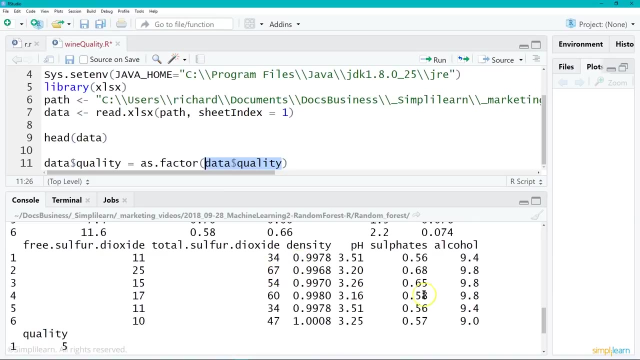 yes-or-no categories versus a continual. now, there's a lot of different things in here that we could do the same thing with, but all of these really are linear numbers. seven point four point seven, oh, sulfur dioxide: 3467. so we really don't we need to mess with any of the other. 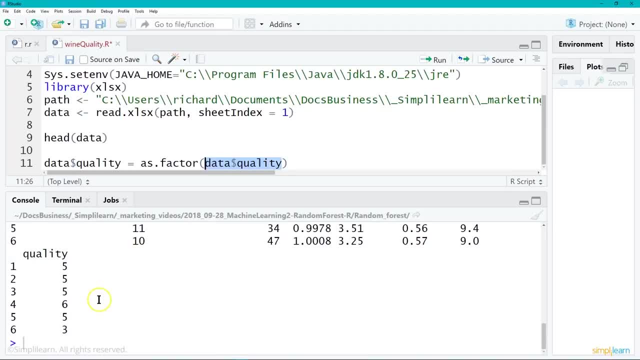 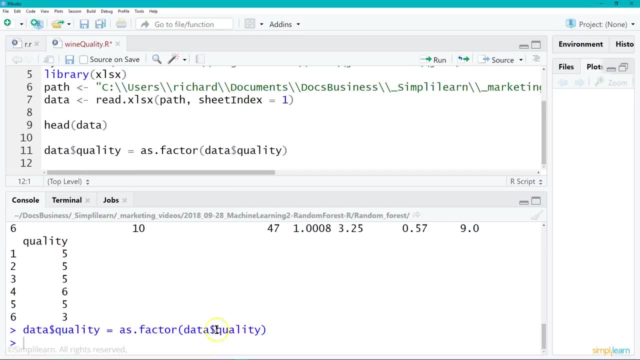 variables in there. but we do want to go ahead and set this up and we'll come up here, we'll do our control, enter and we'll run it down below and you'll see data quality equals as factor data quality. so we've now turned that into a. 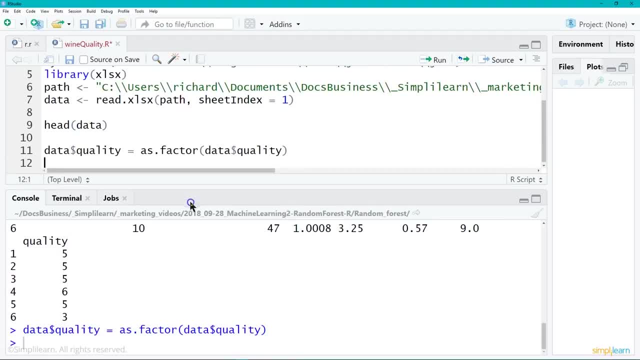 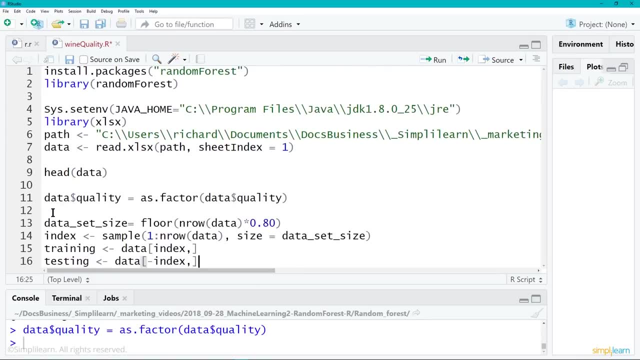 factor or into a categorical data, and so let me just bring this down a little bit: the guys in the back to the rest of this next piece of code. there are so many different ways and if you have been looking at any of our tutorials, this should look kind of familiar. this is one way to do it. 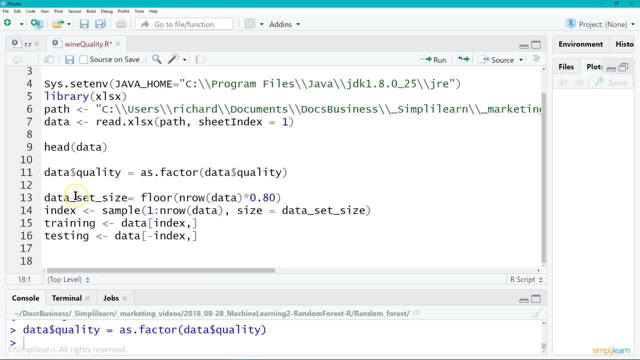 you'll see, we have our training data and our testing data, and so we've done. here is we've got it. we have a data set, size equals, and we're just going to do by the row, and so we want point eight or eighty percent of the data is going to. 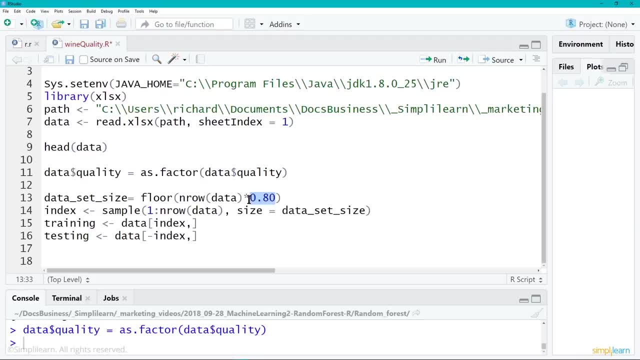 be our training set to train our forest and if you train it forest or any machine learning model, of course want to test it. so we're going to save 20% of the data for testing and when you look at this, we have the index which we set. 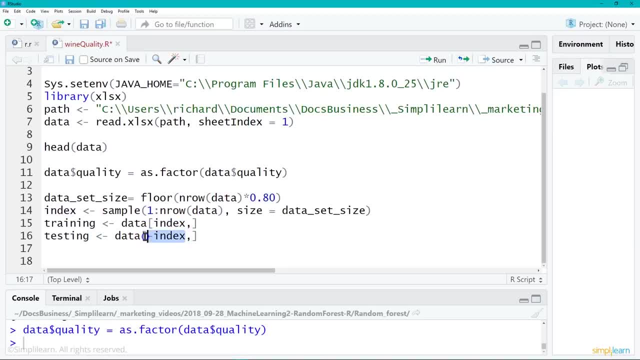 at 80% comma and then a negative index. so that's the remaining setup. so it goes from that index on- this is our notation for sorting out that data. and then we create the index and we use a term sample. and this is just going to go in. 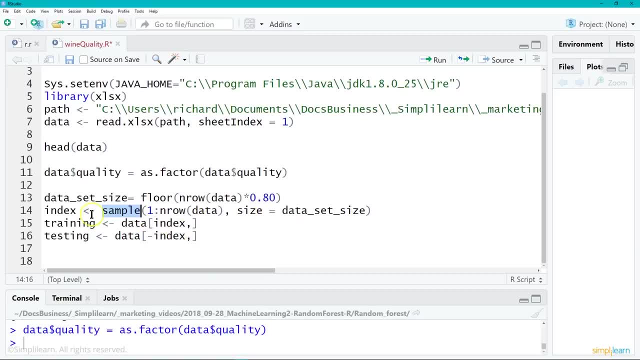 there and set our different samples for in row size, data set, size and everything. so we have an index now. so the data is indexed and we're just going to pull off the first set of index and the end of the index for our data and we can run all of this in one shot. 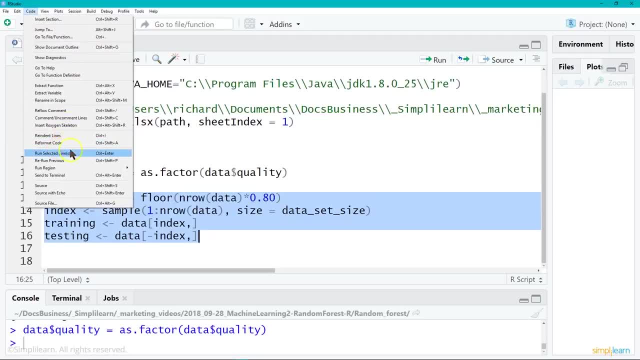 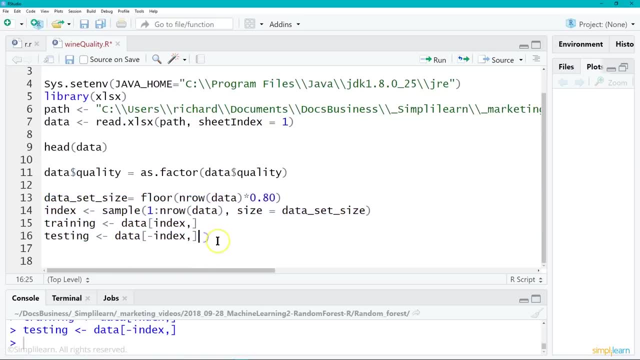 we'll go under code and we'll run selected lines, and so now we have our data in here, we have our training set and our testing set. that's what we wanted to get to. so once we've formatted all the data, then we get to the next. 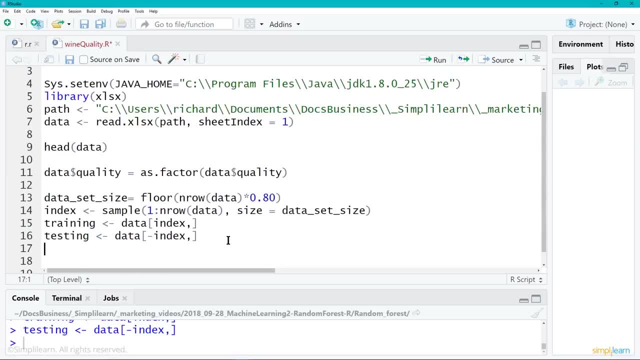 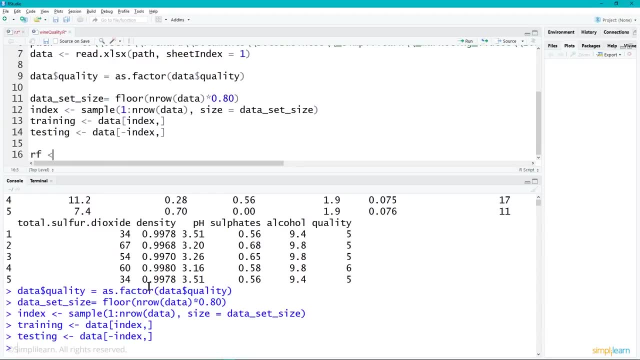 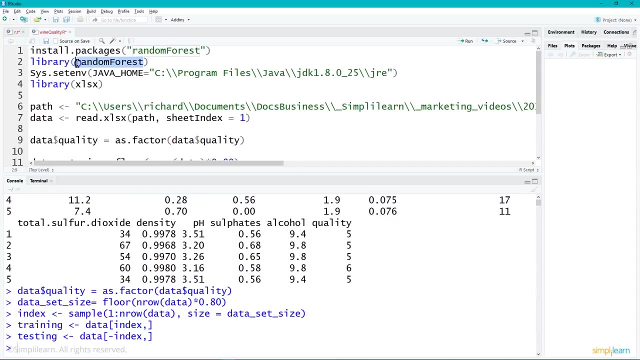 real easy step, which is a single line to bring in our random forest. so let's go ahead and we'll use a variable RF standing for random forest and we're going to assign. if you remember, we brought in our library random. if you wonder why I go up here all the time is, 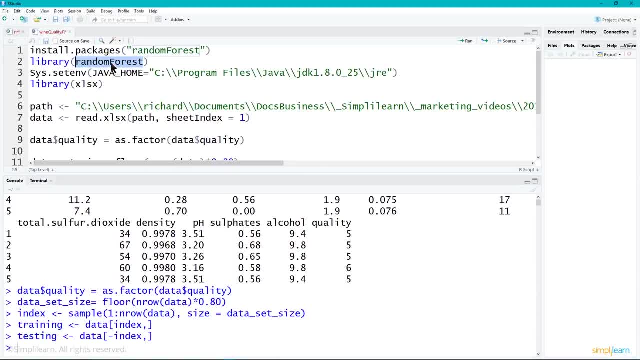 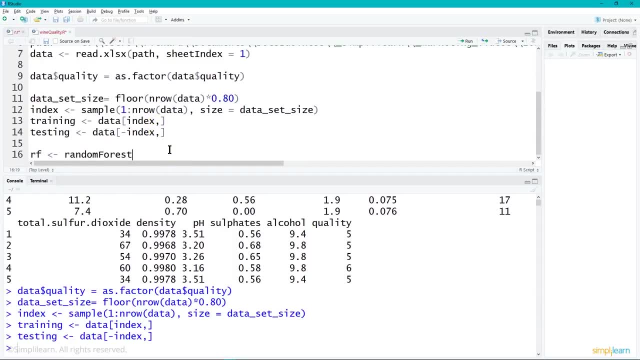 because I'll forget which letters are capitalized in some of these because I switch between packages so much. but it's random with a capital F for forest, random forest. so the RF is going to equal random forest and of course the we start by telling it which column we're trying to predict. and of course you can. 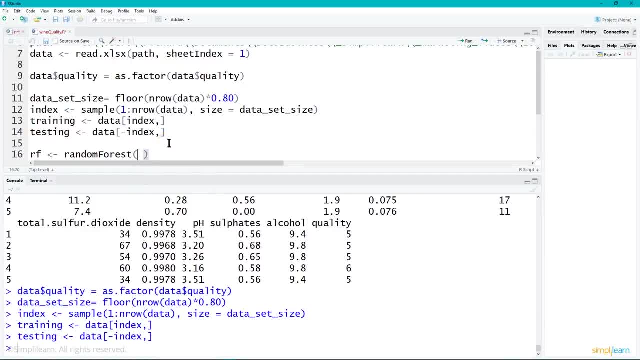 always go down here and double-check. we're running this on the quality. there we go quality and we're using just that column all the way to the end. and then we've added. our team in the back has gone in and played with this a little bit and we'll go a little bit over what they did, but I'm gonna put in. 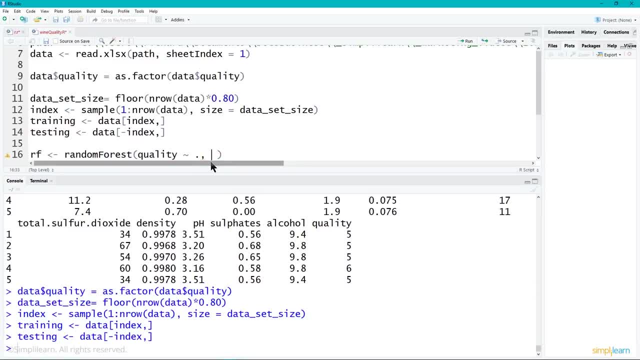 the values that they have set for the different options in the random forest. before I do that, it would help if I tell it what data to use. data is going to equal our training set. and then we have the variables that they put together and let's just talk a little bit about what these different variables mean. 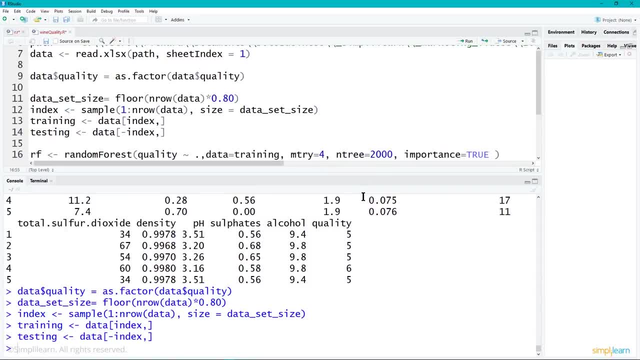 so ha em try an entry. these are some of the variables you play with with the random. for us, the M try not so much when they first put it out, I think I'm try was very common. four is a good value. I can't remember what the default is, but 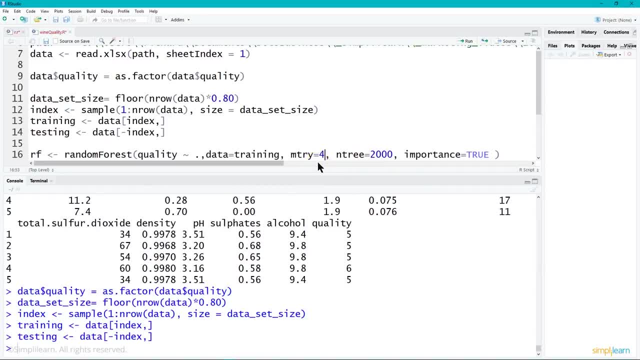 it's probably three, four, five or something like that, depending. I think it depends on how many features you have going in there, so you can even just leave this as a default without too much troubles in tree. this is where it gets important, and i'm going to make this 2001 one of the suggestions. 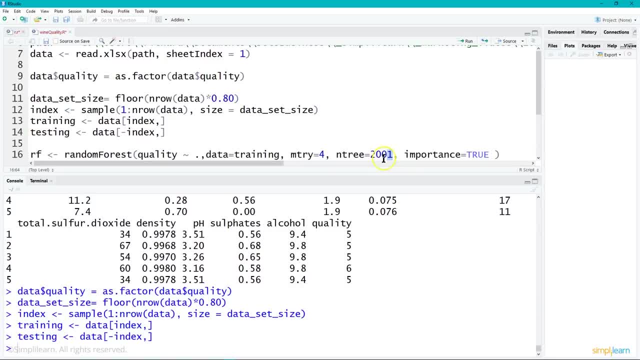 is to always make this odd, like a tie breaker, just in case the default is like 500 or 501. and then, finally, we have importance equals- true. i can't remember what it defaults to, but generally you want to set the importance equals to, true? it actually looks at the correlation between the 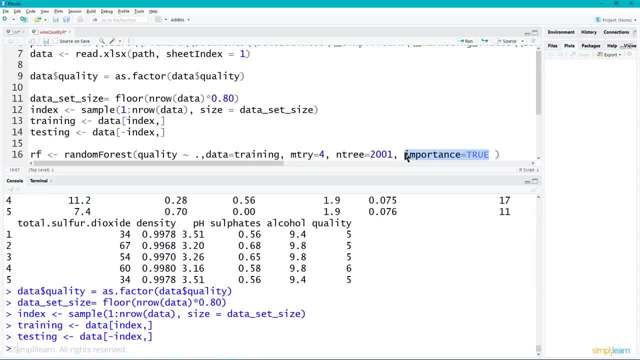 different features to make sure that there is some kind of correlation as it's doing its calculations. so our one line of code is going to assign a random forest and go ahead and train a random for us all in one execution. so this whole thing has been centered around getting to rf set to the 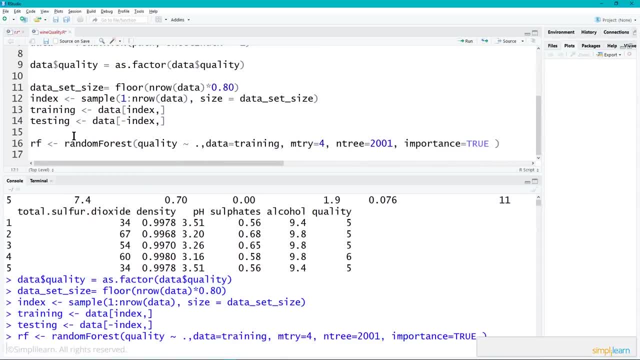 random forest and let's go ahead and execute this variable or this line of code and you'll see it takes a little bit down here to execute as it goes through and sets it up, and you'll see it probably takes a little bit down here to execute as it goes through and sets it up, and you'll see it probably. 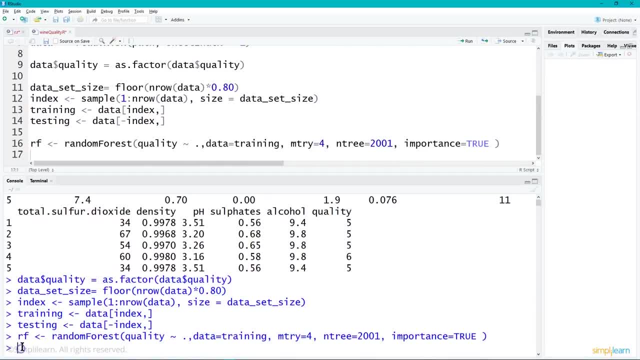 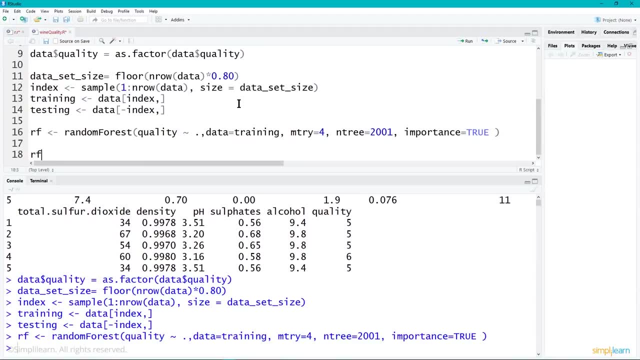 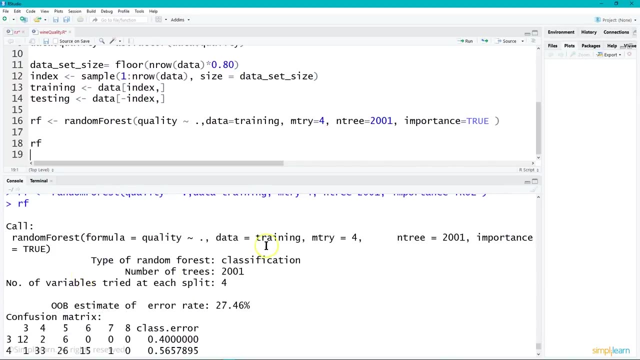 takes a minute or so to execute the code, depending on the size of the data and how good your machine is, and then, with all of our data, we can start looking at the answers. we'll just do rf, we'll execute that and you'll see that the random forest does a nice job. you can see right here it has our 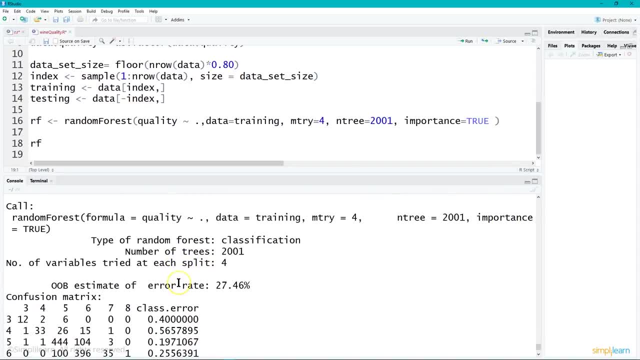 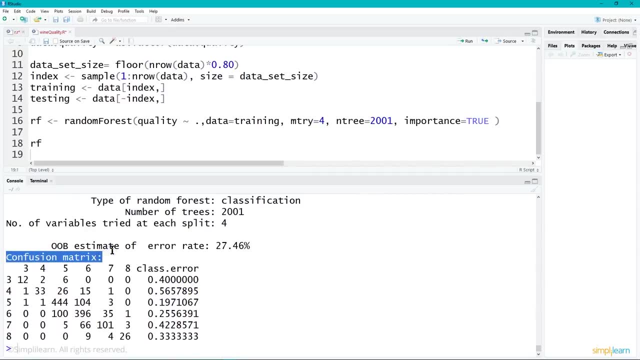 data equals training. it basically goes over everything we talked about and you come down here and it has a confusion matrix, which is nice. we always like our confusion matrix when we're talking to our shareholders and explaining what the data comes out with and how it trains, and we can go ahead and plot our rf. let's see what. 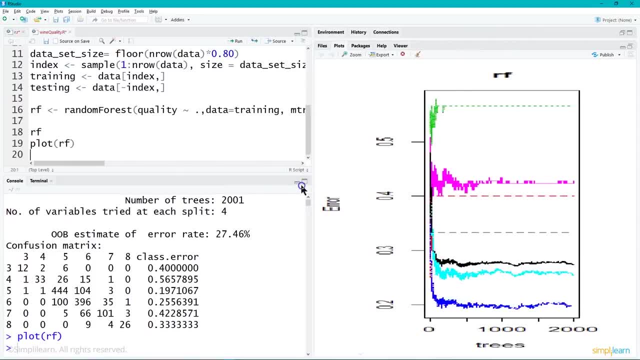 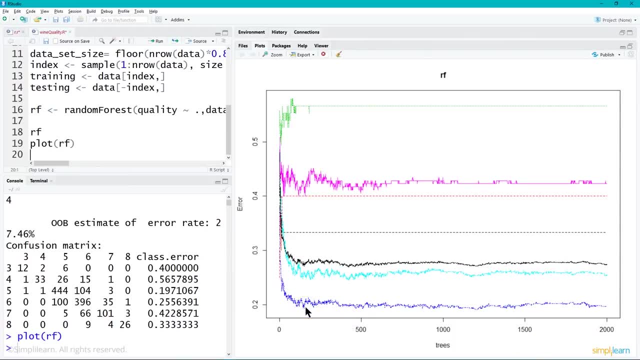 that looks like and as the number of forest grows- remember we set it to 2001 forest- you can also see how the error comes in, how the different error on the different variables. this is kind of a nice graph that gives you an idea. it might help you adjust whether you really want to do 2 000. 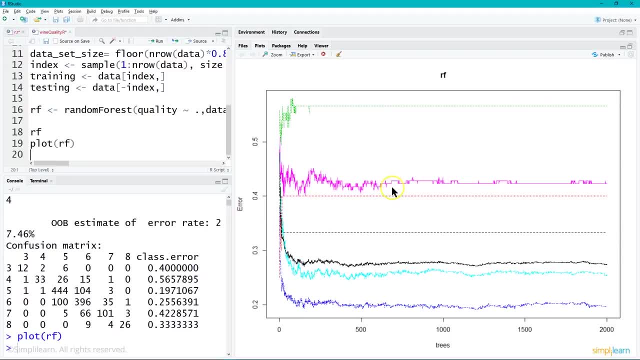 different forests. you might actually want to do 2 000 different forest. you might actually want to do 2 000 different forests. you might actually want to do 2 000 different forest. you might actually truncate this off at around maybe 800, because you notice the lines kind of continue on again. 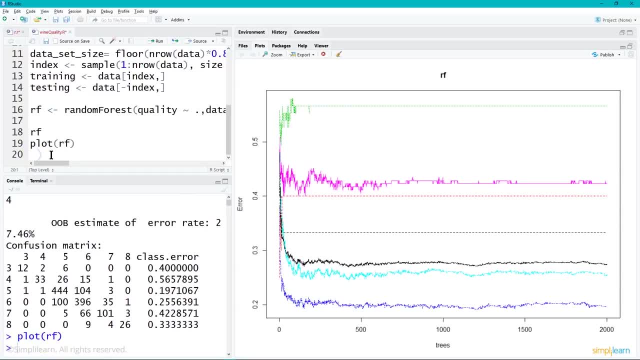 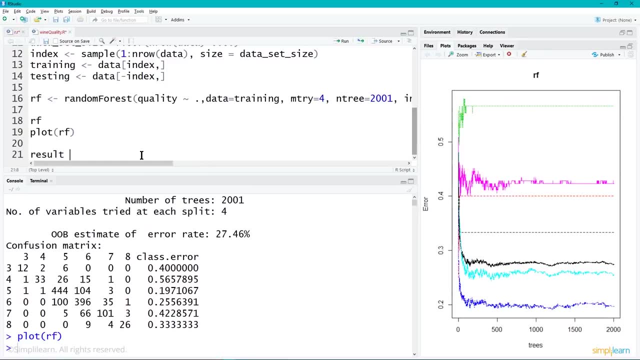 this is just still on the plot and, of course, the next step is we need to go ahead and predict. remember, we split our data into two groups. so let's go ahead and get a result. we'll call it result and we'll assign this one. there we go, we'll set this to a data frame. there we 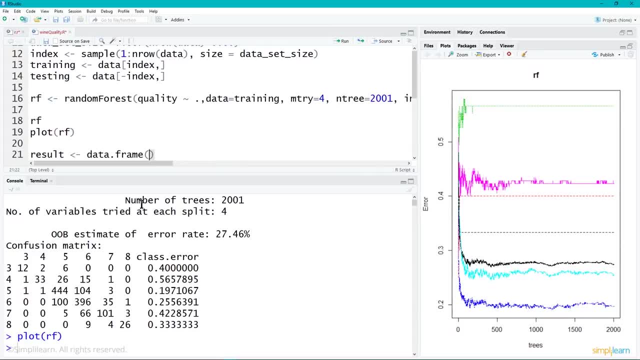 go, there's our data frame and then, oh, let's call this, we have our test, our test quality, because that's what we're setting up on our test group with the quality on there. Then we want to have a predict, a nice little keyword there, to go ahead and run our random forest. 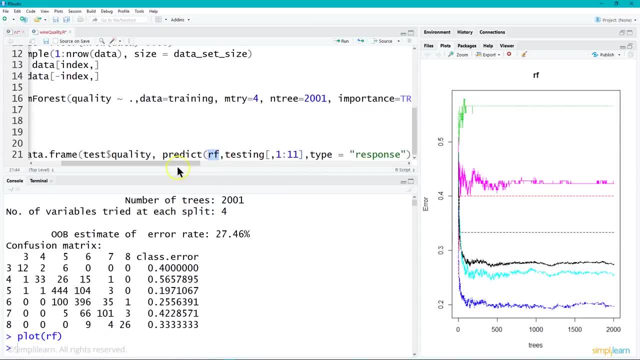 And then we tell it that we're going to predict using our RF, our random forest, our testing group. 1 to 11 is what we're using. Type equals response, So let's go ahead and execute it. That's a mouthful on there. 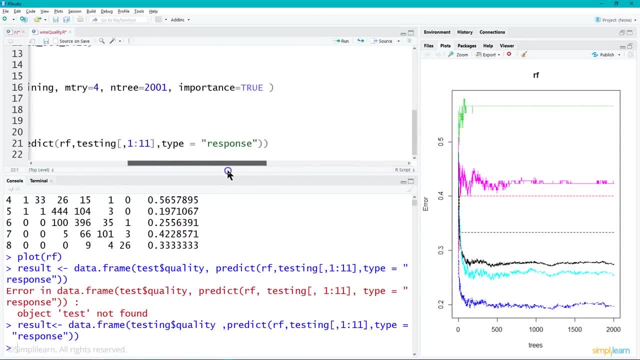 Somewhere I left out a comma in there so it gave me an error. But you can see, right here we've set it in there and now we have a result And just real quick we could do the head of the result result, comma 5, and just take a look at the first five lines. 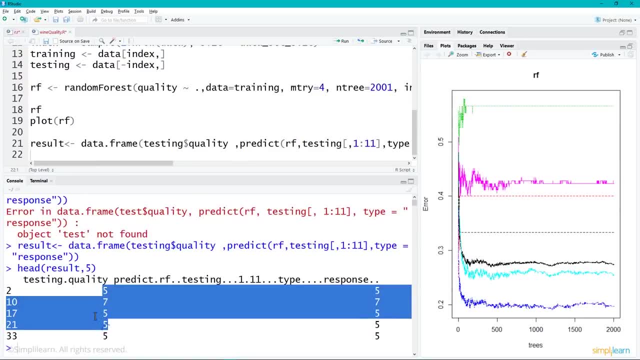 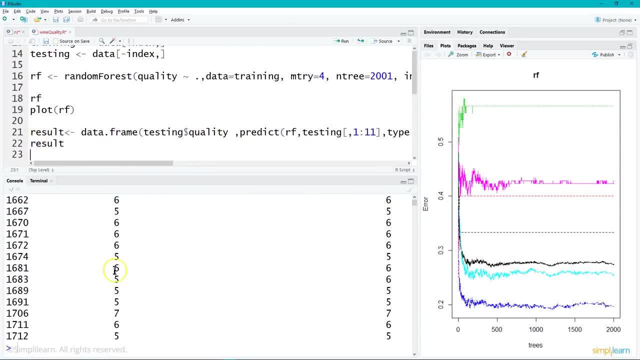 And you'll see. we have the actual value and what we predicted over here. And we could also just do all of the result and just see what that looks like, Oops, And print that out, And so it has all the different data we're going through. 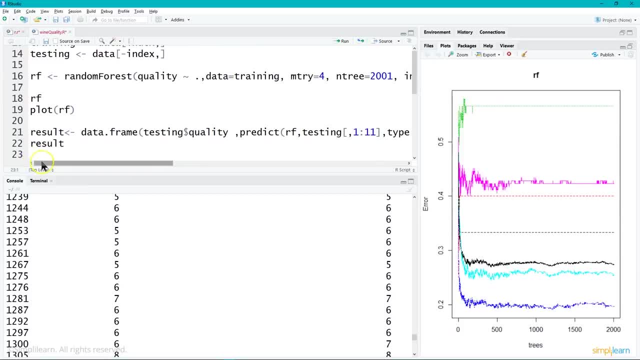 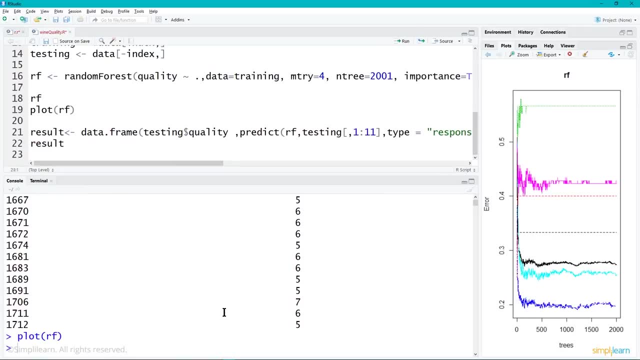 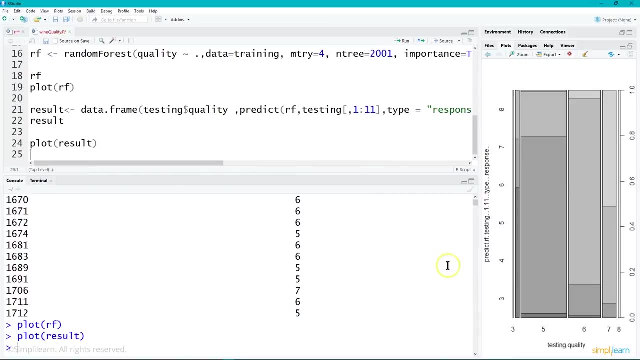 And finally, let's just go ahead and plot. There we go, We'll put plot up here, Plot And let's plot the result and just see what that looks like. Maybe not the best one to show to the shareholders, but it does give you an idea. 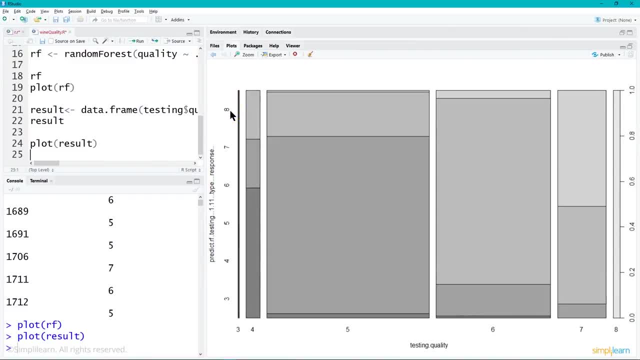 On the left, on the y-axis, you'll see that it predicted 8.. And this tells you that a lot of the 8 and the 8 scale data are predicted 8.. So it was pretty probably gave us about 50%, came up there at 8.. 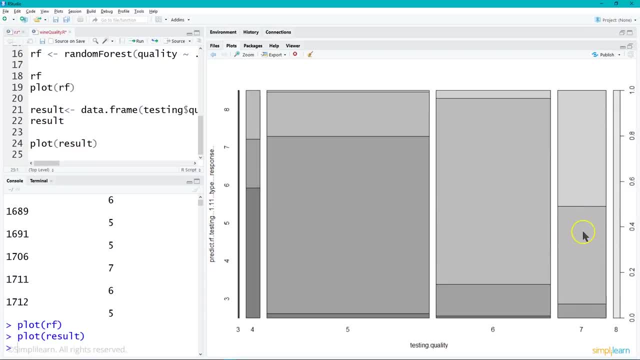 Really maybe 50%. it didn't guess right, but it did come up there and say that it was at least a 4,, 5, or 6,, even where it was considered an 8, and so on. You can see these different blocks coming in. 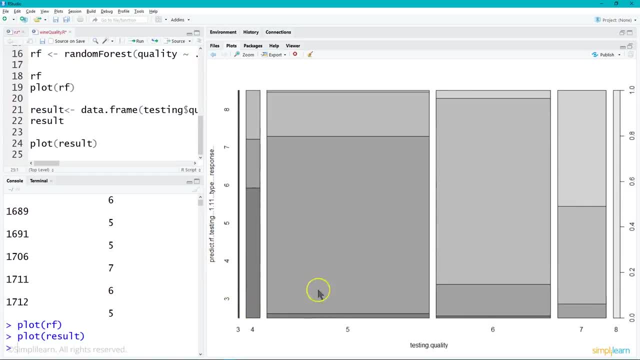 So that if you line up the 3 with the 3,, 4 with the 4, and you kind of cross-index them. a heat map would probably do better, But for this example we'll just do a quick plot of the data. 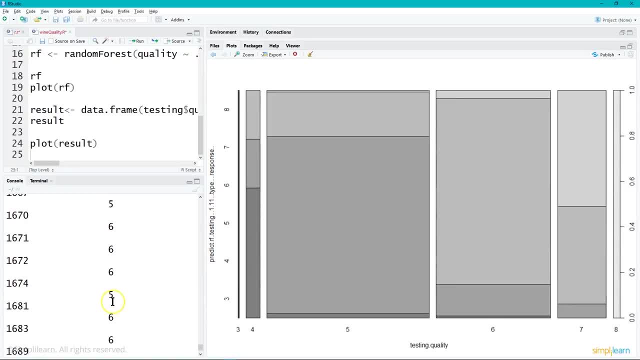 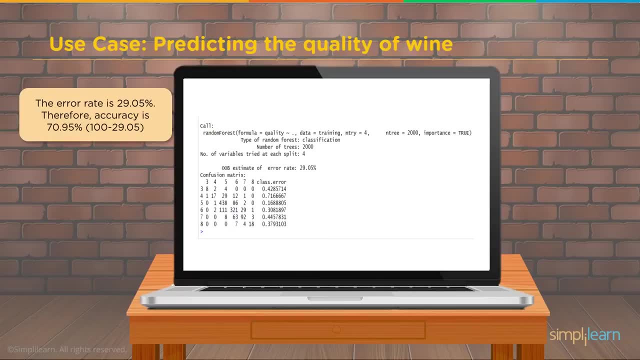 As far as This is how it works and you can again see the results that we predicted over here, and you can look those over, Of course, back in the wine cellar we're talking to our vineyard owner And, if you remember from before, we looked at this chart right here. 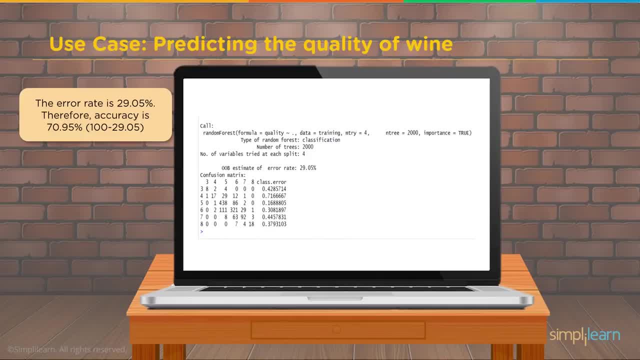 The error rate is 29.05%. Therefore, our accuracy is 70.95%. If you're doing a vineyard, that's probably pretty good accuracy. And always check your domain when you're sharing this stuff, because if you're doing something, that's life or death. 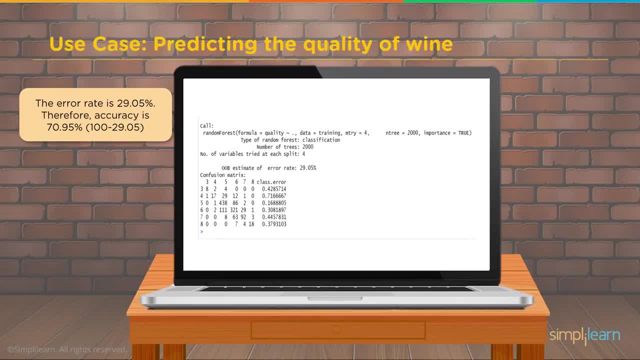 maybe 70.95% is pretty good. 70% accuracy might not be so good, But if you're looking at where you're going to distribute the bottles to for the wine and who's going to drink it, you know 70% accuracy is pretty good for that. 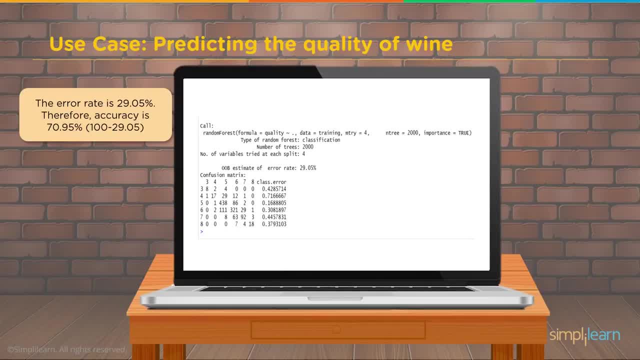 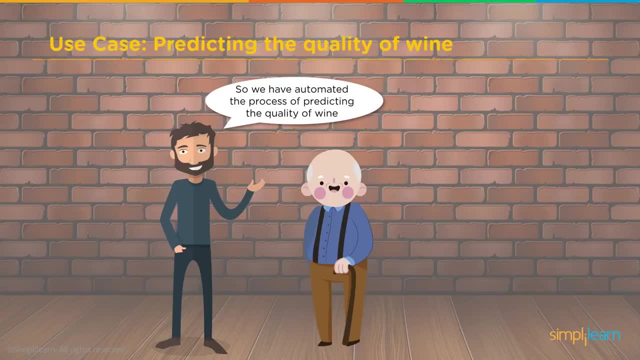 That's probably a lot better than having no accuracy whatsoever and not even knowing what wine's going out to who. So we have automated the process of predicting the quality of wine. I myself prefer to predict it by sampling it. That's great. 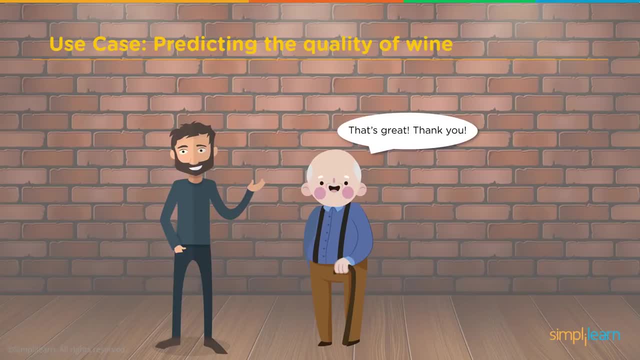 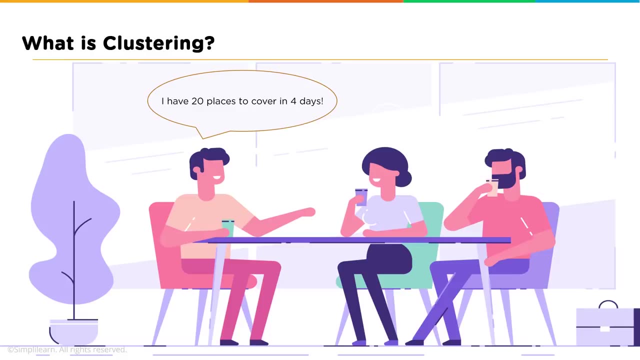 Thank you. I'd like to visit this guy and sample his wine and find out just how good his different vineyards are. What is clustering? Well, we'll have a group of people here hanging out at a table or local coffee shop- I'm guessing coffee shops, since they all have the same mugs. 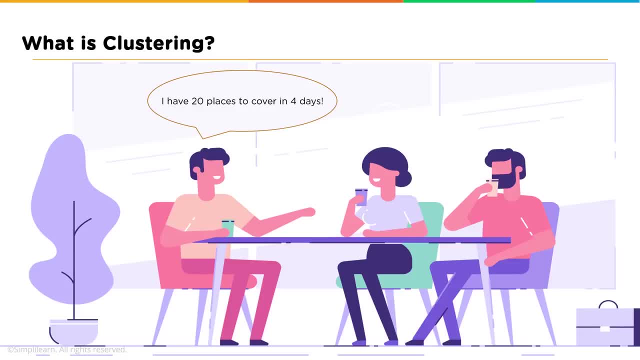 And one of them is trying to figure out what they're going to do. I have 20 places to cover in four days. I guess he's going. traveling- That sounds fun. One of those breeze through Costa Rica or visiting the US or going to Europe to go visit all the highlights. 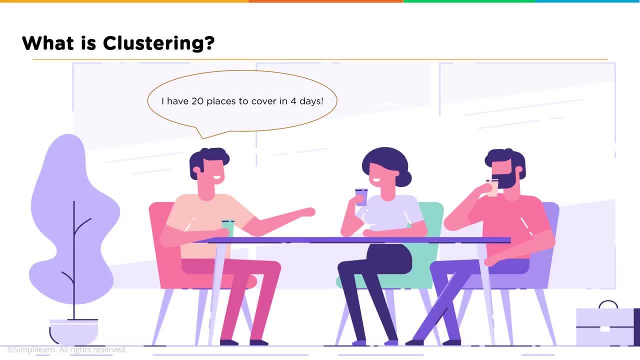 So he's got 20 places he wants to go and he wants to hit them in four days. Very ambitious, And how will I manage to cover all of them? That's the question that he's coming up with. How am I going to get to all these different places in the short time I have? 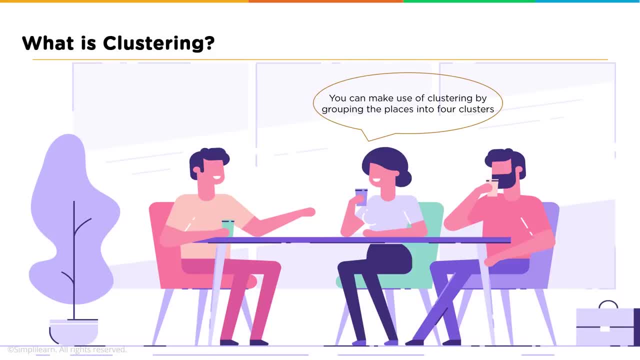 Maybe he's a sales team so he has 20 places he's got to do demos for. You can make use of clustering by grouping the places into four clusters. Each of these clusters will have places which are close by, So we're going to cluster them together by what is closest to the other one. 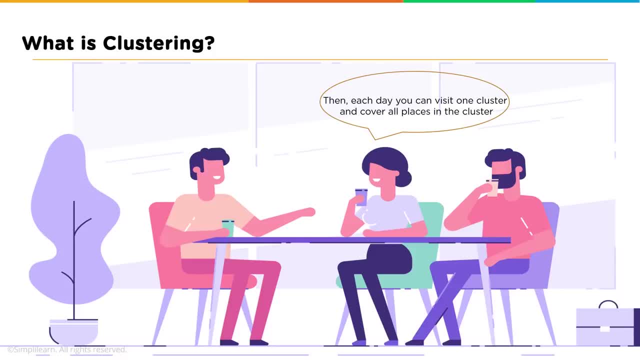 Then each day you can visit one cluster and cover all the places in the cluster. Great, That's a great idea. If you're going to hit four different places, maybe you're going to cluster whatever streets are closest together, so you don't have to travel. spend all your time traveling. 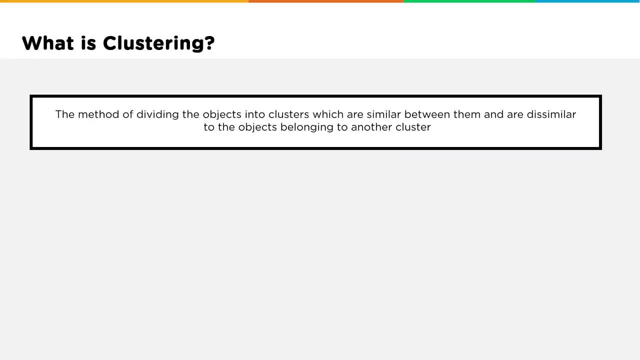 The method of dividing the objects into clusters which are similar between them and are dissimilar to the objects belonging to another cluster. So this is a formal definition of clustering, And we have here what we call hierarchical clustering and partial clustering, And we're going to go more into detail on hierarchical clustering. 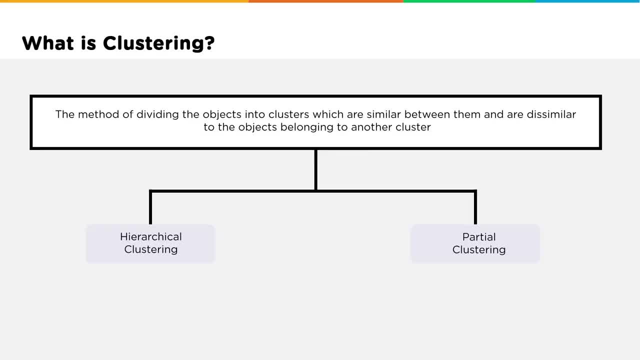 And you'll see the difference between the two, where partial clustering doesn't have the descending graph, it just has groups of things, And under hierarchical clustering we're going to go over agglomerative and divisive. And you can think of agglomerative, of bringing things together, and divisive. 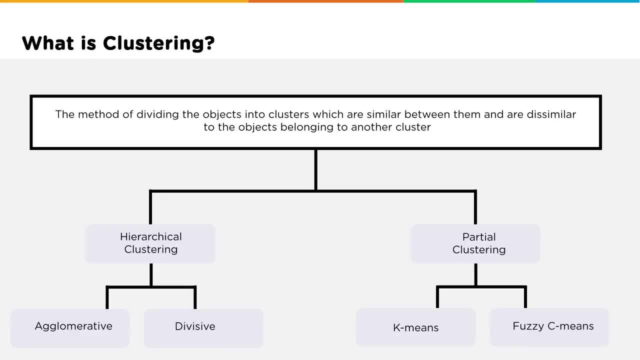 as dividing them apart and then partial clustering. The two most common ones are K-means- That's probably the most common use for partial clustering. There's also fuzzy C-means And there's other ways of clustering and other algorithms out there. 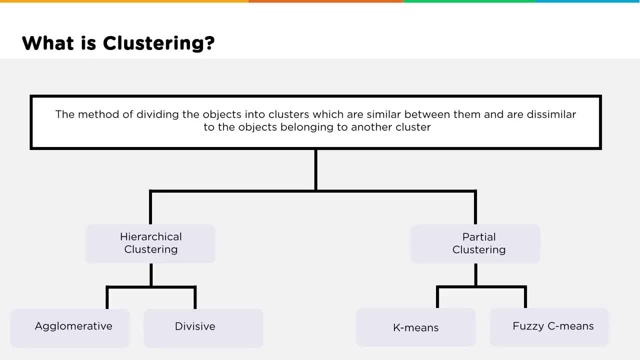 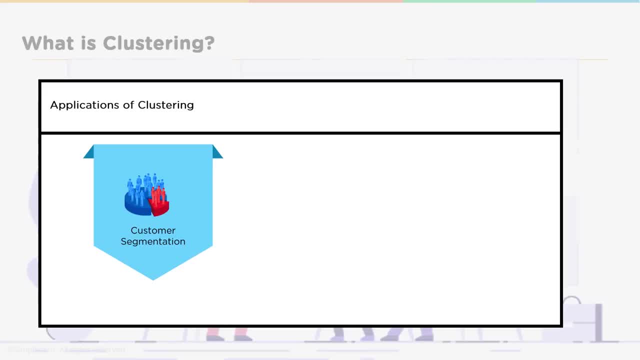 But these are the two big ones, K-means really being the most common one used. But we're not going to dig too deep into partial clustering because we're studying clustering today. So what is clustering? Well, the applications of clustering are pretty numerous. 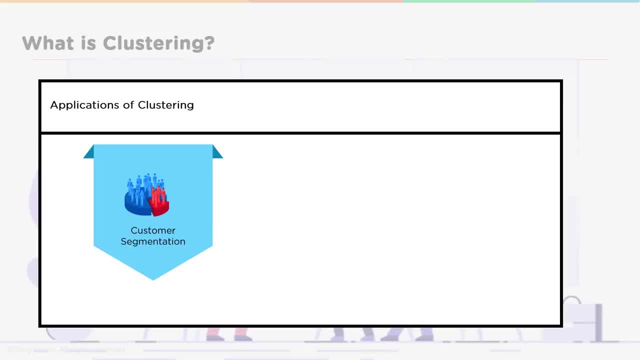 We have things like customer segmentation: what people kind of belong together, How do we group them together? We have social network analysis. So social networks, we might look at sentiments: What group of people like something, What group of people don't like something. 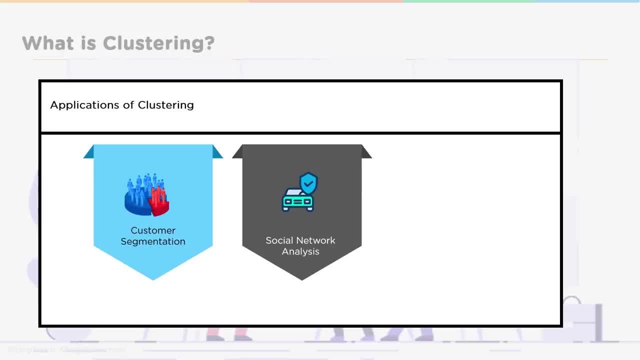 And then we can use that sentiments to suggest new sales for them. You know this whole group is into Harley Davidson motorcycles so we cater to them to sell them. So it's in motorcycle parts And we find out that people in that group also like leather jackets. 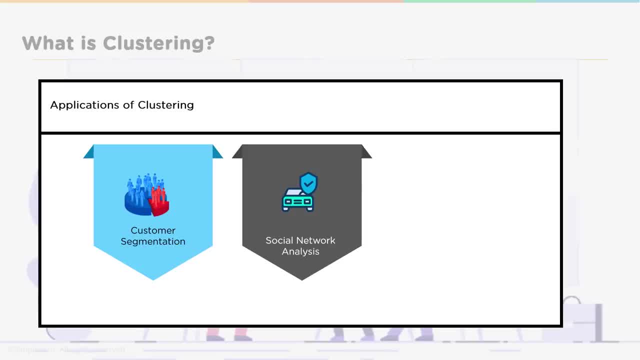 They also like motorcycle boots and they like bandanas, My brother's into Harley Davidson. So that's why I picked that kind of funny example. But you can kind of see, we look for similarities between these people and then we group them together accordingly. 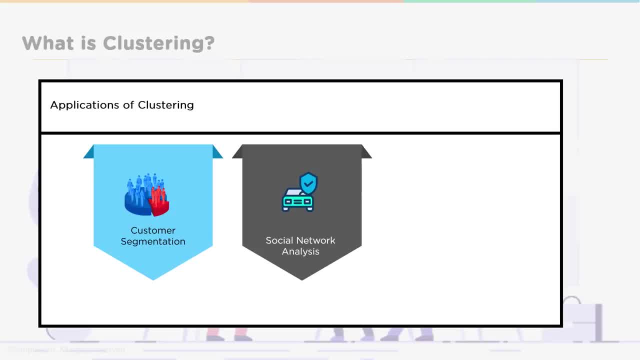 And that's a good. sentimental clustering is very common in so many things today. We want to know the sentiments on stocks. Who is interested in stocks, Who's not? Sentimental analysis: We talked about customer segmentation and sales. Well, we want to know what kind of sentimental view people have on different. 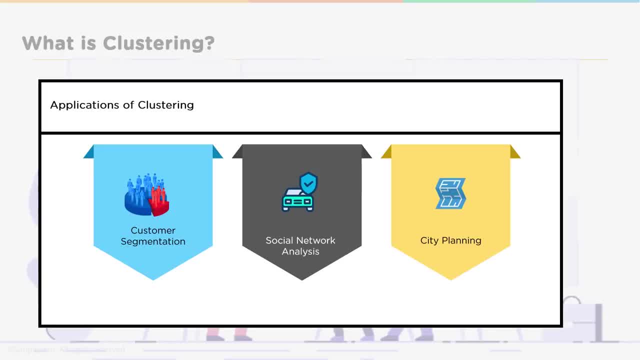 restaurants, if we're going to open up a new restaurant or a new putting stores in- And, of course, city planning- A lot of this I just kind of aimed at the city planning side. City planning is big with clustering. We want to cluster things together so that they work. 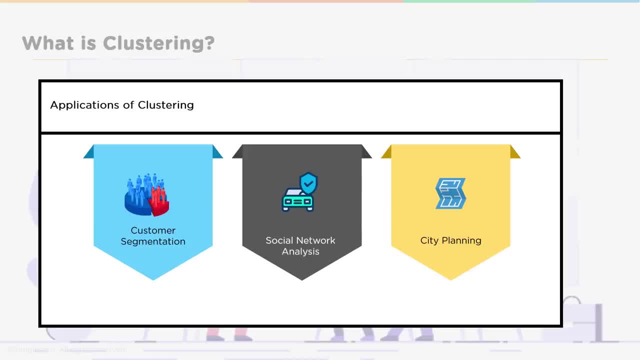 We don't want to put a industrial zone in the middle of somebody's neighborhood where they're not going to enjoy it, or have a commercial zone right in the middle of the industrial zone where no one's going to want to go next to a factory to go eat a high end meal or dinner. 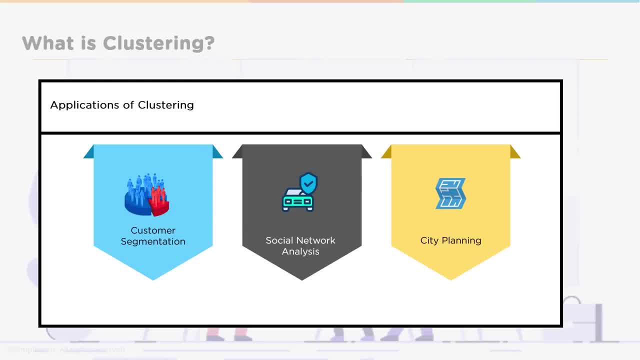 So it's very big in city planning. It's also very big in just preprocessing data into other models. So when we're exploring data, being able to cluster things together, reveal things in the data we never thought about And then, once we have it clustered, we can put that into another model to help. 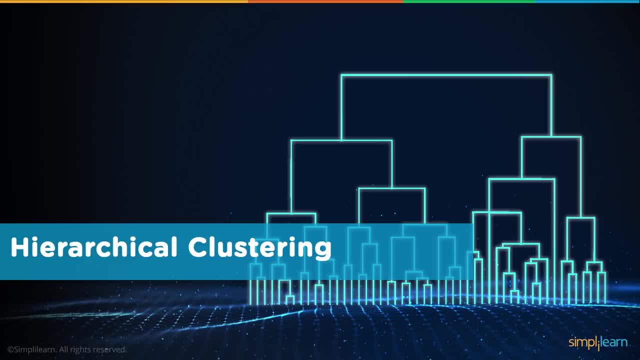 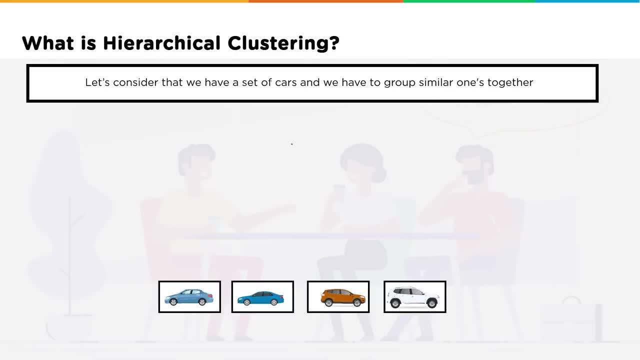 us figure out what it is we want for our solution. So let's go a little deeper into hierarchical clustering. Let's consider: we have a set of cars and we have a group similar. We want to group similar ones. We want to put the sedans together. 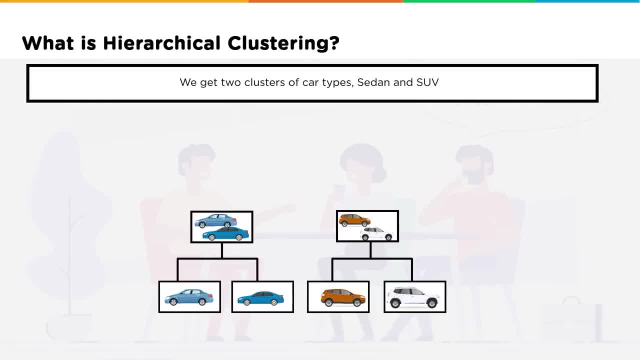 So below we have- you'll see four different cars down there and we get two clusters of car types: sedan and SUV. So if you're just looking at it, you can probably think: oh yeah, we'll put the sedans together and the SUVs together. 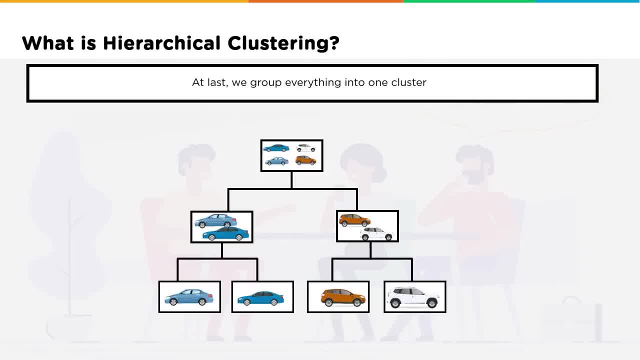 And then at last we can group everything into one cluster. So we just have just cars. So you can see, as we have this, we make a nice little tree. This is very common. We see anybody talks about hierarchical clustering. This is usually what you see and what comes out of it. 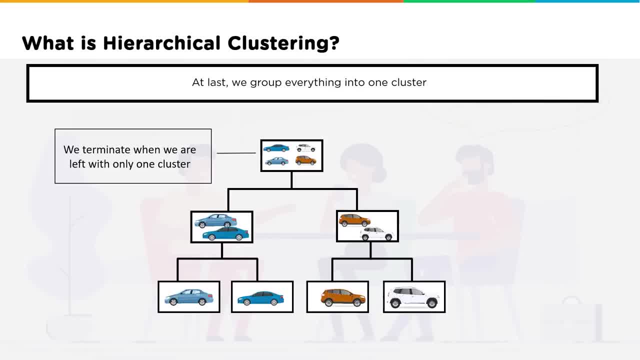 We terminate When we are left with only one Cluster. So we have, as you can see, we bring them all together. We have one cluster. We can't bring it together anymore because they're all together. Hierarchical clustering is separating data. 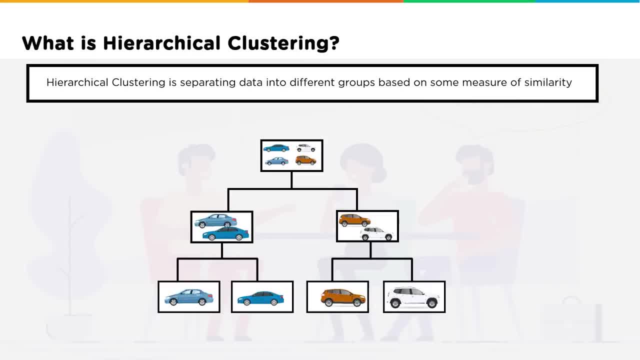 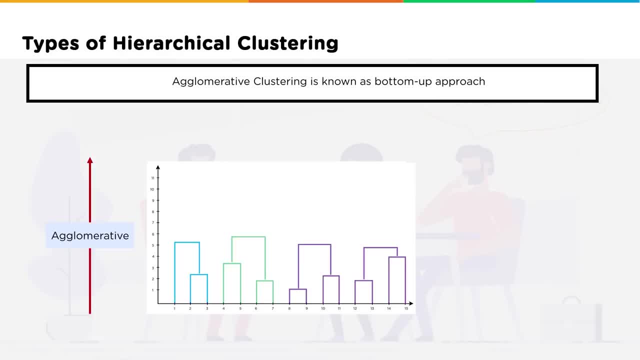 into different groups based on some measure of similarity. So we have to find a way to measure what makes them alike and what makes them different. Agglomerative clustering is known as a bottom up approach, And I said: think of that as bringing things together. 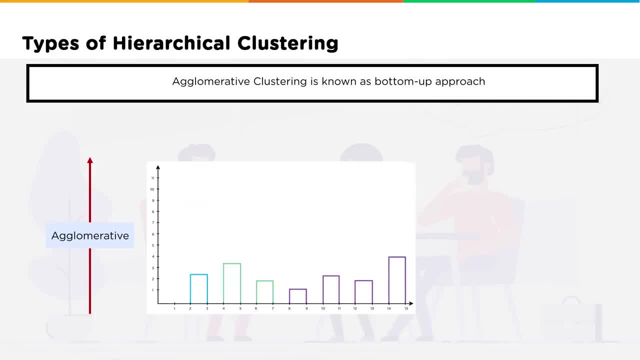 Do you see? I think the Latin term agglomerate is together, because you have your agglomerate rocks, where all the different pieces of rocks are. They're in there. So we want to bring everything together. That's a bottom up, And then divisive is. we're going to go from the top down. 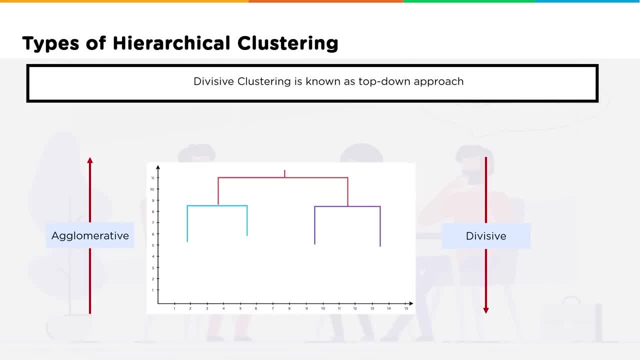 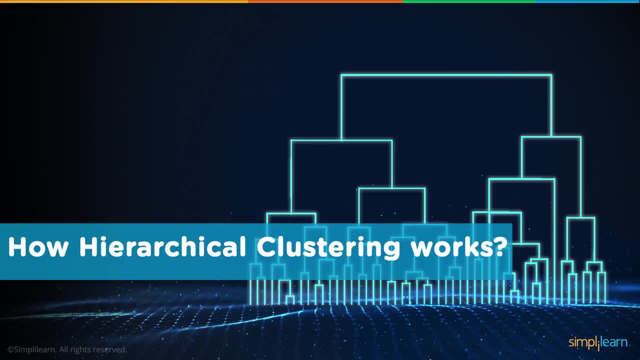 So we take one huge cluster and we start dividing it up into two clusters, into three, four, five and so on. Digging even deeper into how hierarchical clustering works, Let's consider we have a few points on a plane, So this plane is 2D. 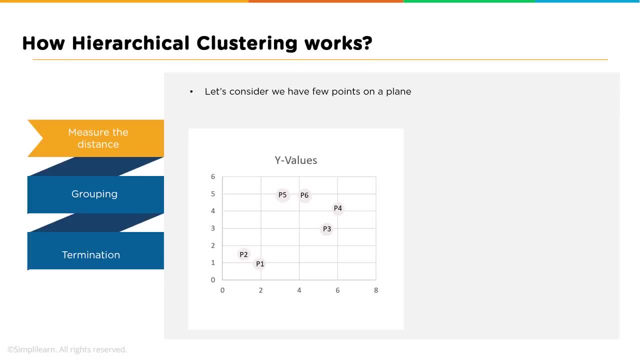 So we have an X- Y coordinates, kind of makes it easy. We're going to start with measure the distance, So we want to figure a way to compute the distance between each point. Each data point is a cluster of its own, Remember, if we're going from the bottom up. 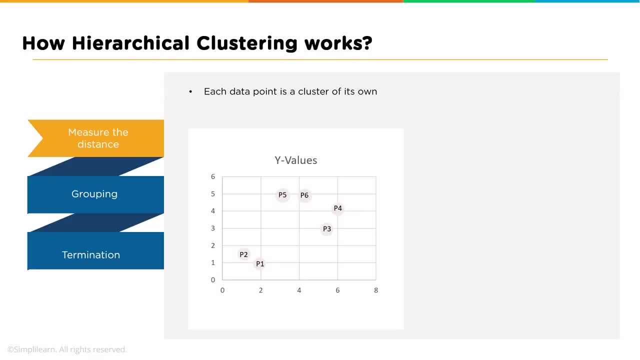 agglomerative, then we have each point being its own cluster. We try to find the least distance between two data points to form a cluster And then, once we find those with the least distance between them, we start grouping them together, So we start forming clusters of multiple points. 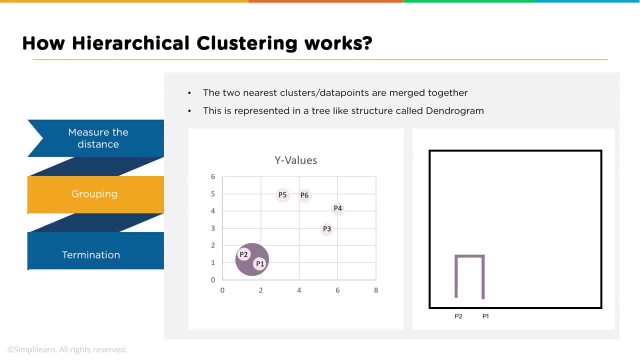 This is represented in a tree like structure called dendogram. So there's another key word, dendogram, And you can see it is. it's just a branch that we've looked at before and we do the second group the same, So it gets its own dendogram and the third gets its own dendogram. 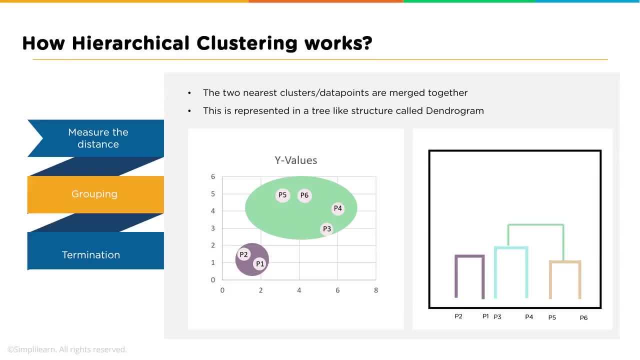 And then we might group two groups together. So now those two groups are all under one dendogram because they're closer together than the P1 and P2. And then we terminate when we are left with one cluster, So we finally bring it all together. 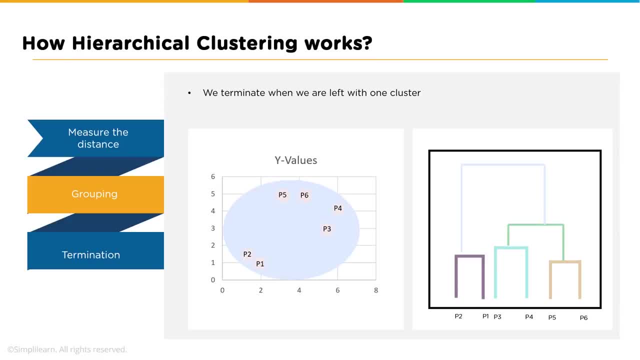 You can see on the right how we've come up all the way up to the top Whoops, And we have the gray hierarchical box coming in there and connecting them. So we have just one cluster and that's a good place to terminate, because there is no way we can bring them together any further. 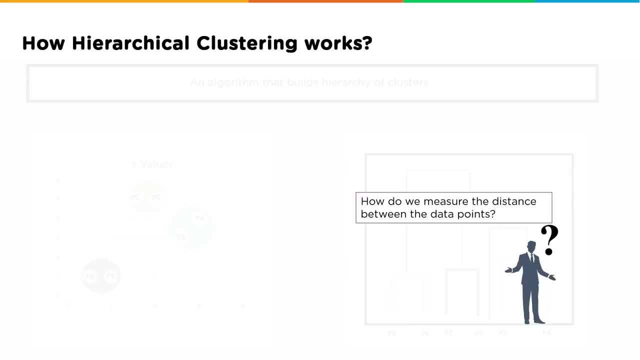 So how do we measure the distance between the data points? I mean, this is really where it starts getting interesting. Up until now, you can kind of eyeball and say, hey, these look together. But when you have thousands of data points, how are we going to measure those? 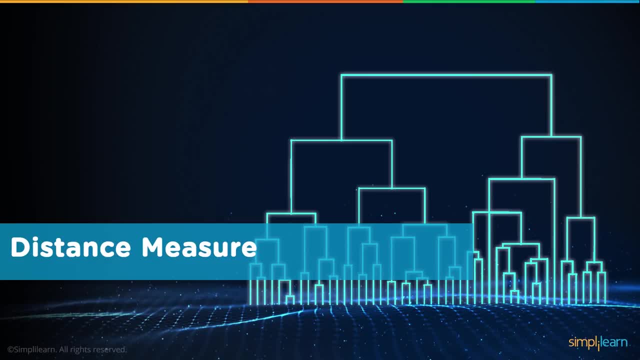 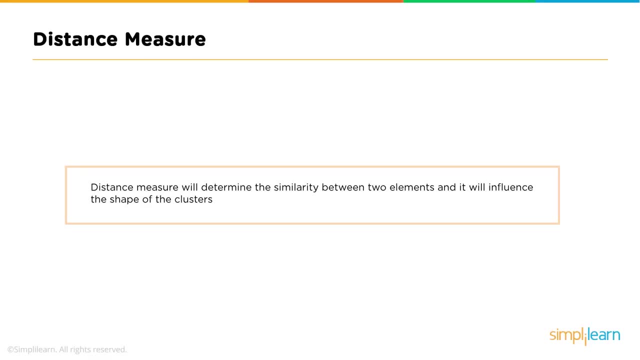 distances And there is a lot of ways to get the distance measure, So let's go and take a look at that. Distance measures will determine the similarity between two elements and it will influence the shape of the clusters, And we have Euclidean distance measure. 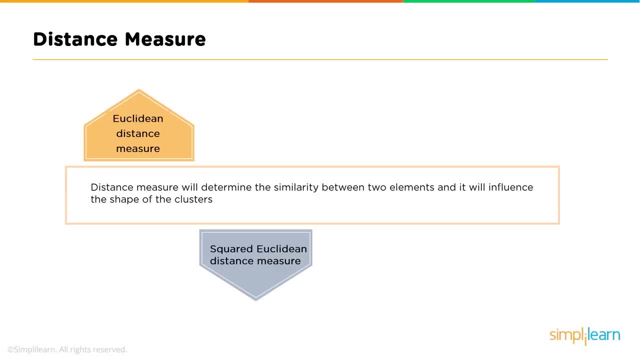 We have squared Euclidean distance measure, which is almost the same thing but with less computations, And we have the Manhattan distance measure, which will give you slightly different results, And we have the cosine distance measure, which again is very similar to the Euclidean. playing with triangles. 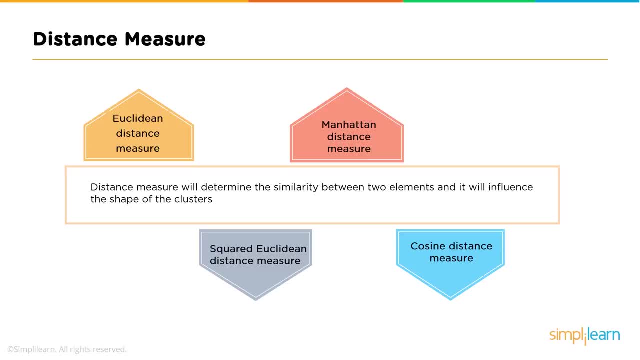 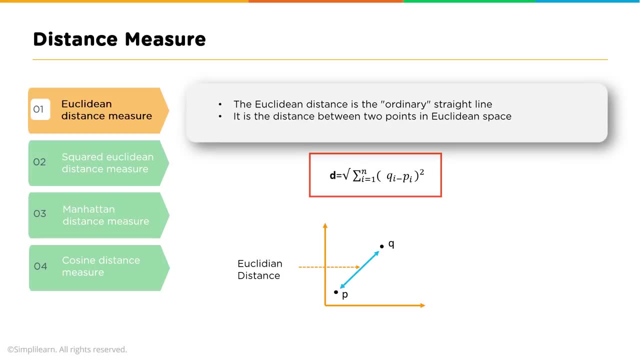 And sometimes it can compute faster depending on what kind of data you're looking at. So let's start with Euclidean distance measure. The most common is we want to know the distance between the two points. So if we have point P and point Q, the Euclidean distance is the ordinary straight. 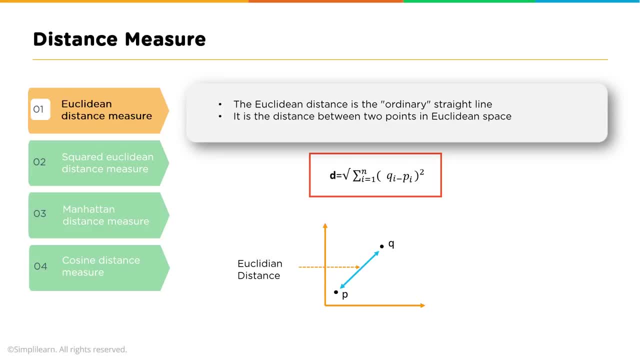 It is the distance between the two points in Euclidean space, And you should recognize D equals in this case. we're going to sum all the points, So if there was more than one point, we could figure out the distance to the not more than one point. 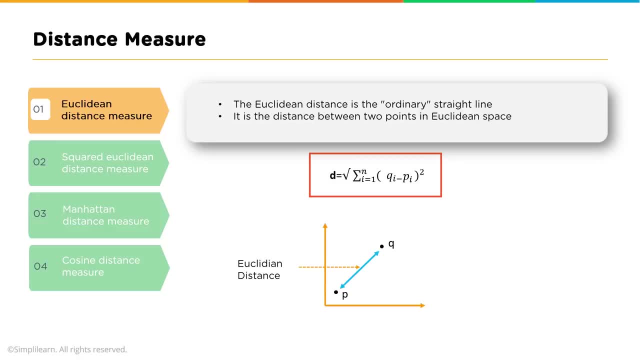 This is the sum of more than two dimensions, So we can have the distance between each of the different dimensions squared And that will give us- and then take- the square root of that And that gives us the actual distance between them, And they should look familiar from Euclidean geometry. 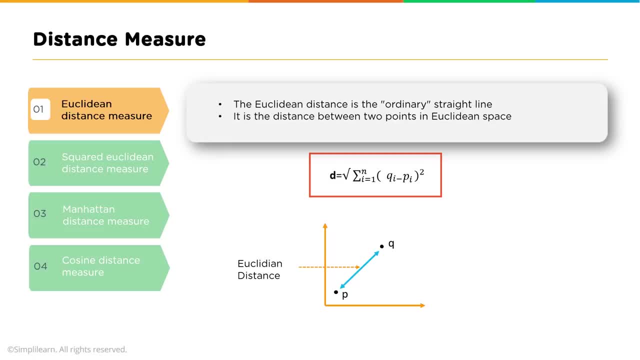 Maybe you haven't played too much with multiple dimensions so the summation symbol might not look familiar to you, But it's pretty straightforward as you add the distance between each of the two different points squared. So if your y difference was two minus one, squared would be two. 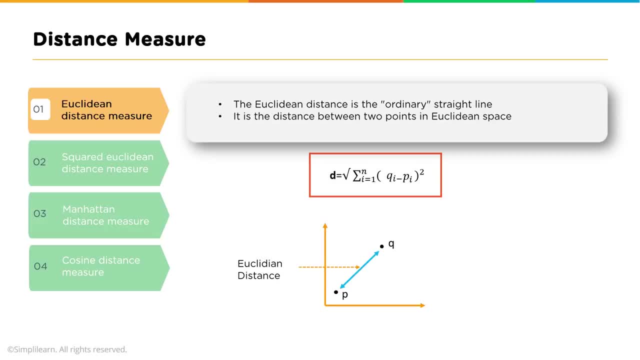 And then you take the difference between the x again squared, And if there was a z coordinates it would be z one minus z two squared, And then take the square root of that and sum it all together and then take the square root of it, So to make it compute faster. 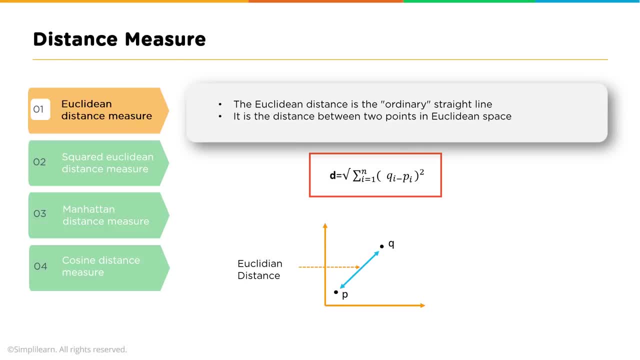 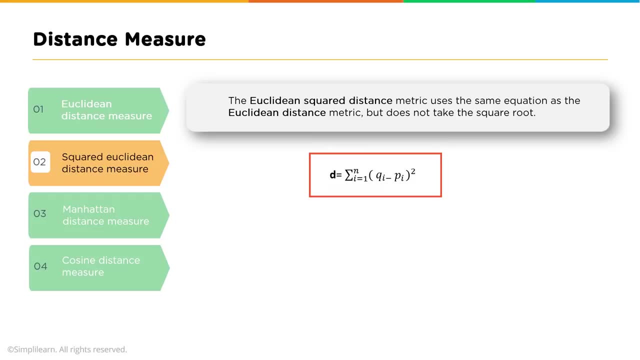 since the difference in distances, whether one is farther apart or closer together than the other, we can do what's called the squared Euclidean distance measurement. This is identical to the Euclidean measurement, but we don't take the square root at the end. 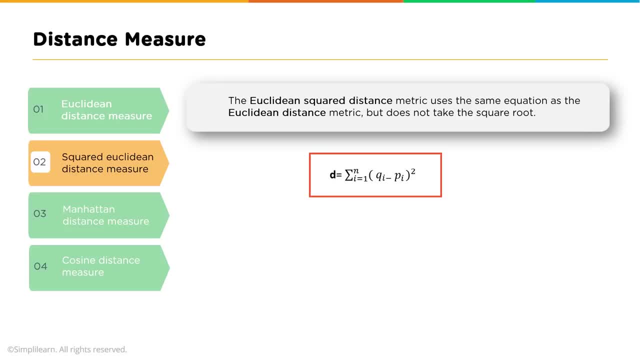 There's no reason to. It certainly gives us the exact distance, But as far as doing calculations as to which one's bigger or smaller than the other one, it won't make a difference, So we'll just go with it. So we just get rid of that final square root. 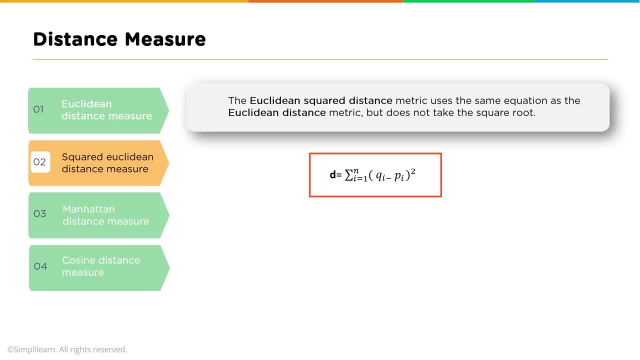 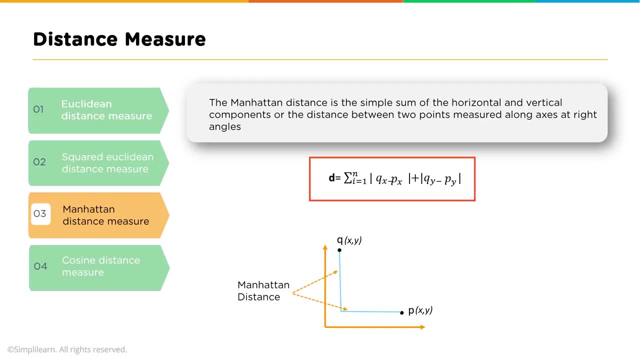 computes faster and it gives us the pretty much the Euclidean squared distance on there. Now the Manhattan distance measurement is a simple sum of horizontal and vertical components, or the distance between two points measured along axes at right angles. Now this is different because you're not looking at the direct line between them. 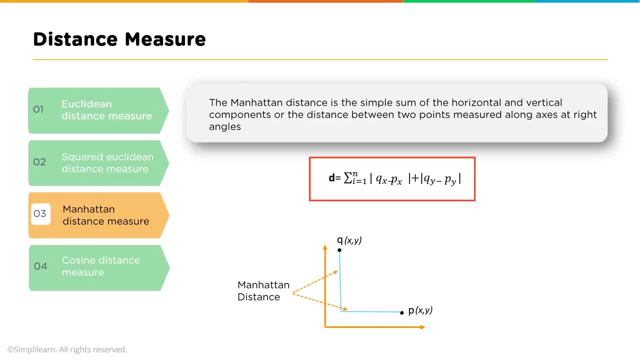 And in certain cases the individual distances measured will give you a better result. Now, generally that's not true. Most times you go with Euclidean squared method because that's very fast and easy to see. But the Manhattan distance is, you measure just the y value and you 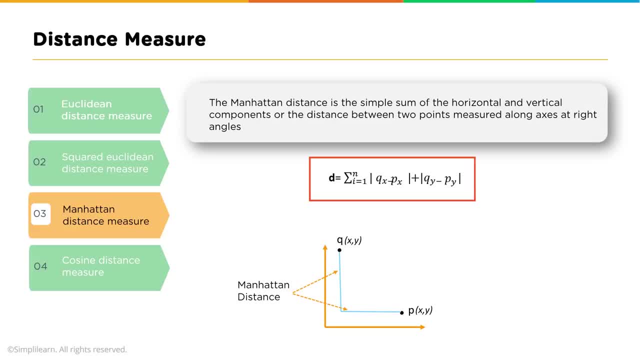 take the absolute value of it and you measure just the x difference. You take the absolute value of it and just the z. And if you had more different dimensions in there- A, B, C, D, E, F, however many dimensions- you would just take the absolute value of the difference of those dimensions. 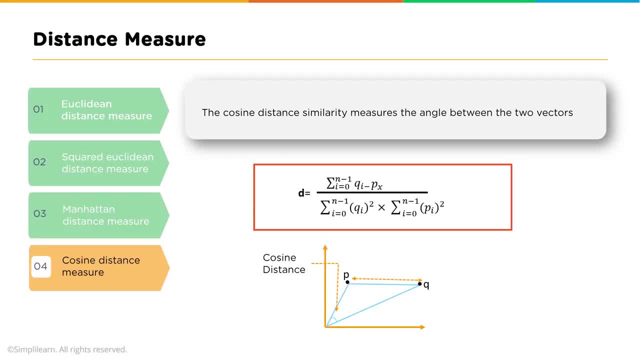 And then we have the cosine distance. Similarity measures the angle between the two vectors And, as you can see, as the two vectors get further and further apart, the cosine distance gets larger. So it's another way to measure the distance, Very similar to the Euclidean. so you're still looking at the same kind of measurement. 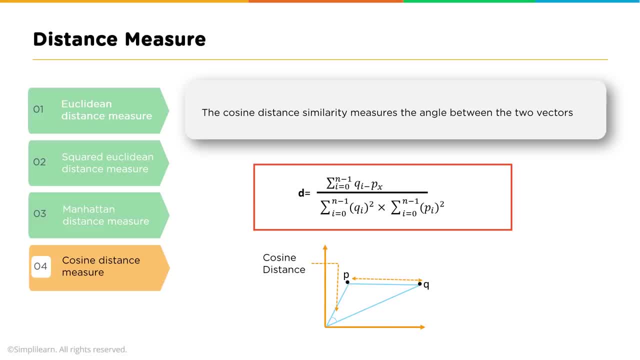 So it should have a similar result as the first two, But keep in mind the Manhattan will have a very different result And you can end up with a bias with the Manhattan. if your data is very skewed, If one set of values is very large and another set of values is very small. 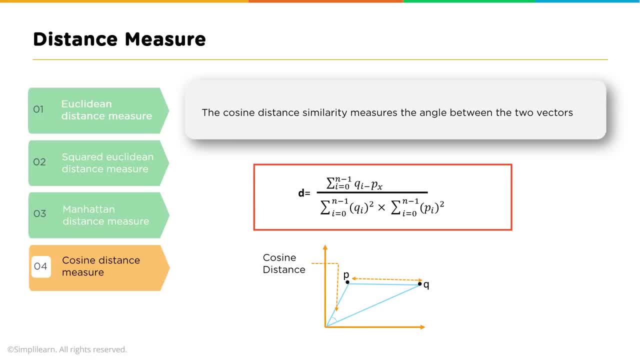 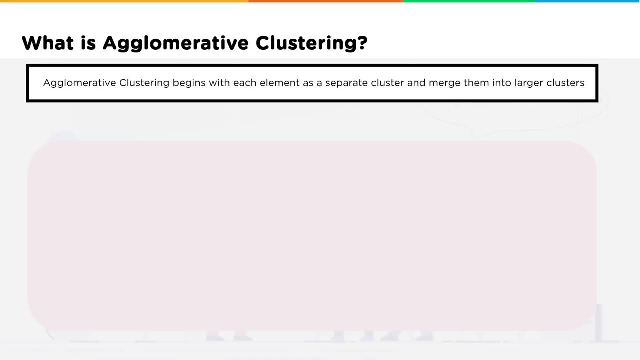 But that's a little bit beyond the scope of this. It's just important to know that about the Manhattan distance. So let's dig into the agglomerative clustering. And agglomerative clustering begins with each element of a cluster and then we merge them into a larger cluster. 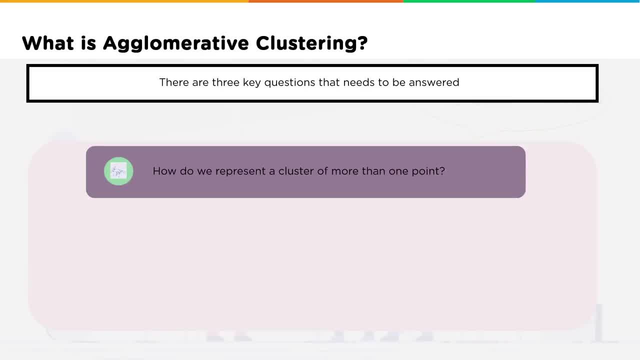 How do we represent a cluster of more than one point? So we're going to kind of mix the distance together with the actual agglomerative and see what that looks like. We're actually going to have three key questions that are going to be answered here. 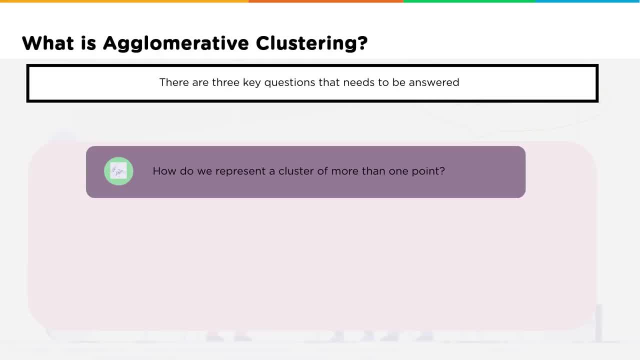 So how do we represent a cluster of more than one point? So we'll look at the math, what it looks like mathematically and geometrically. How do we determine the nearness of clusters? When to stop combining clusters? Always important to have your computer script or your whatever you're working. 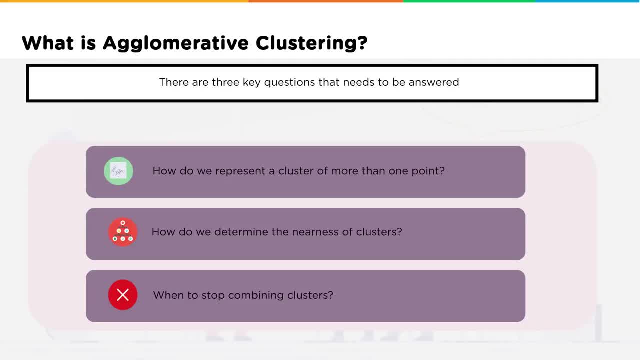 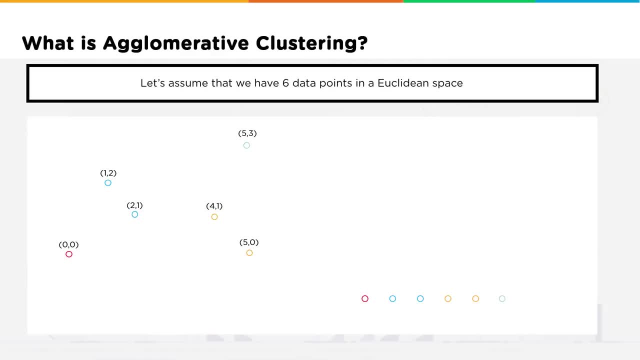 on, have a termination point, so it's not going on eternally. We've all done that, if you do any kind of computer programming or writing a script. Let's assume that we have six data points in a Euclidean space. So again we're dueling with X, Y and Z. in this case just X and Y. 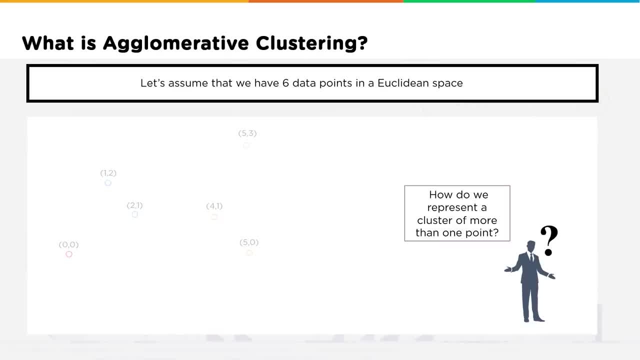 So how do we represent a cluster of more than one point? Let's take a look at that First. we're going to make use of centroids, very common terminology in a lot of machine learning languages, when we're grouping things together. So we're going to make use of centroids, which is the average of its points. 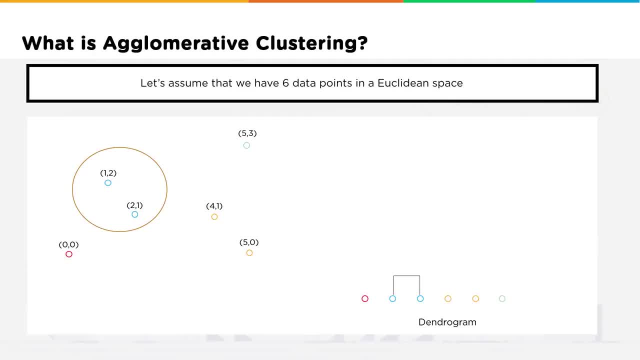 And you can see, here we're going to take the 1, 2 and the 2, 1, and we're going to group them together because they're close And if we were looking at all the points, we'd look for those that are closest. 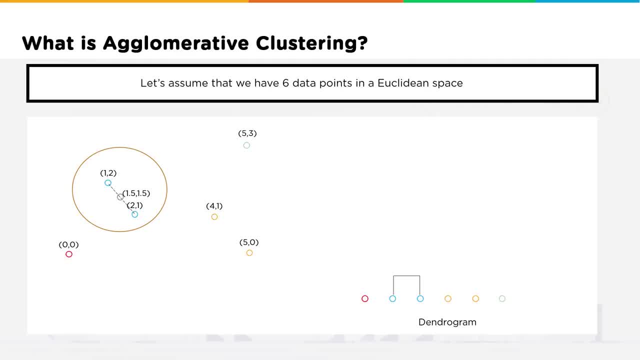 and start with those, and we're going to take those two. We're going to compute a point in the middle and we'll give that point 1.5,, 1.5,, 1.5.. And that's going to be the centroid of those two points. 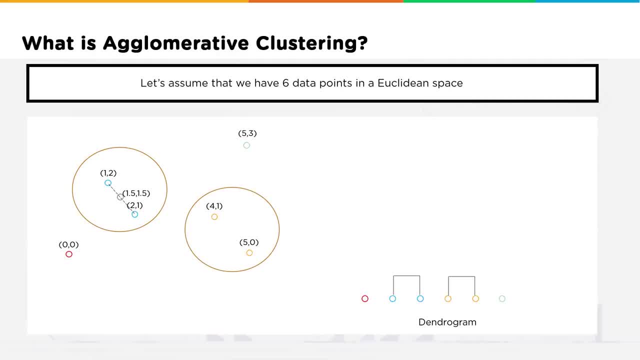 And next we start measuring like another group of points. we got 4, 1,, 5, 0, when they're pretty close together. So we'll go ahead and set up a centroid of those two points. In this case it would be the 4.5 and 0.5 would be the measurements on those two points. 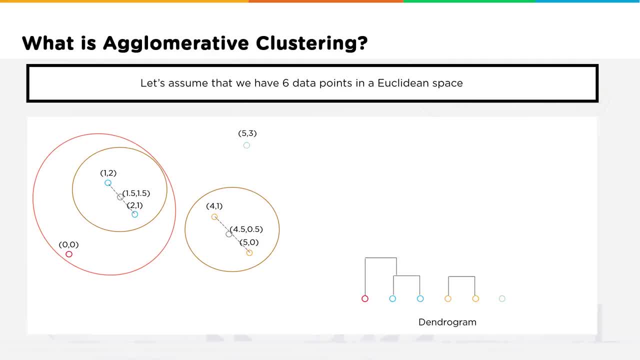 And once we have the centroid of the two groups, we find out that the next closest point to a centroid is over on the left. and so we're going to take this and say, oh, 0, 0 is closest to the 1.5, 1.5 centroid. 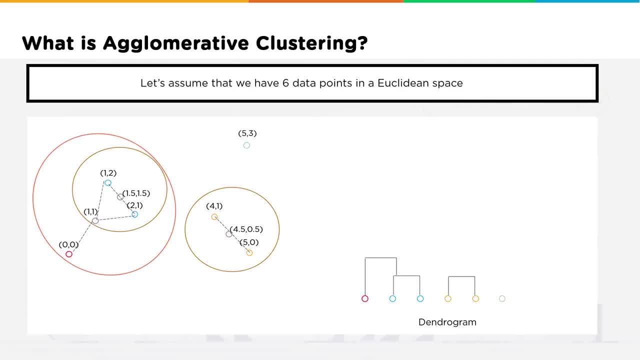 So let's go ahead and group that together And we compute a new centroid based on those three points. So now we have a centroid of 1.1 or 1,, 1.. And then we also do this again with the last point, the 5,, 3,. 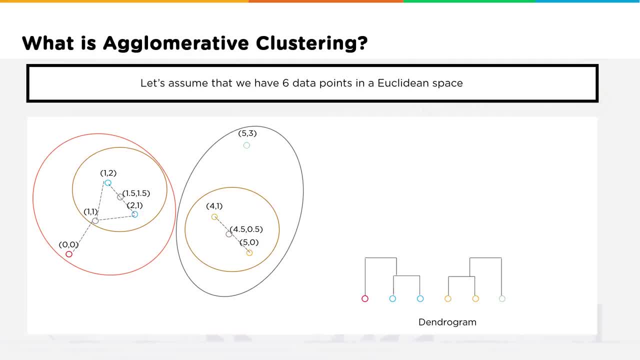 and it computes into the first group And you can see our dendogram on the right is growing. So we have each of these points are become connected and we start grouping them together And finally we get a centroid of that group too. 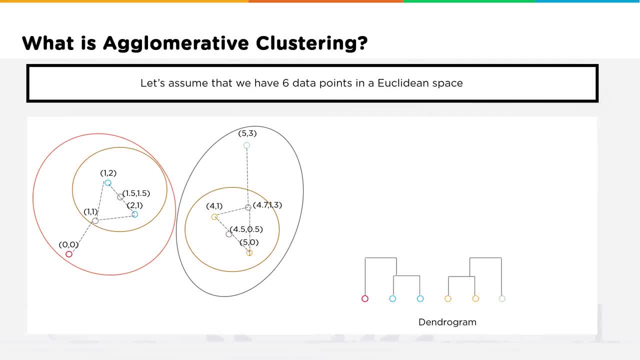 And then, finally, the last thing we want to do is combine the two groups by their centroids, And you can see here we end up with one large group and it'll have its own centroid, although usually they don't compute the last centroid, We just put them all together. 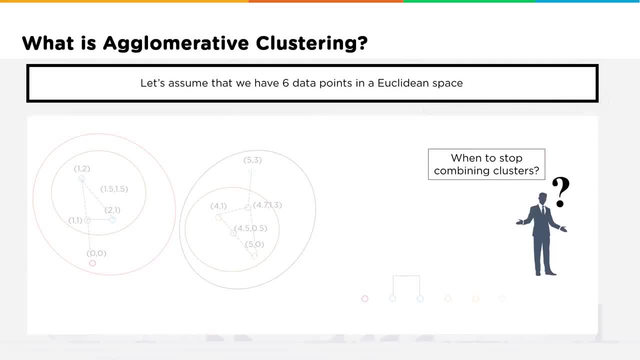 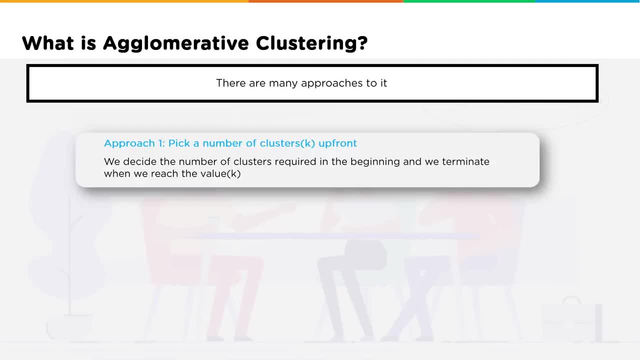 So when do we stop combining clusters? Well, hopefully it's pretty obvious to you In this case when they all got to be one, But there are actually many approaches to it. So first pick a number of clusters K up front. 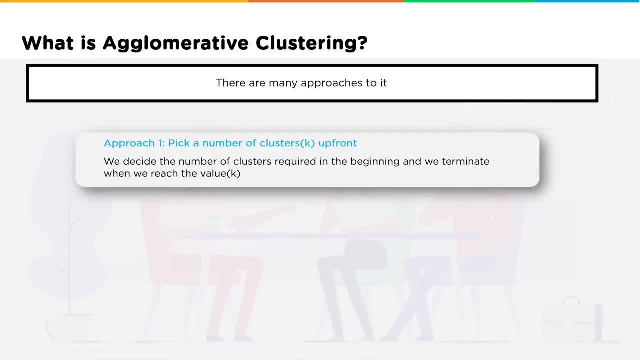 And this is done in the fact that we don't want to look at 200 in clusters. We only want to look at the top five clusters, or something like that. So we decide the number of clusters required in the beginning and we terminate when we reach the value K. 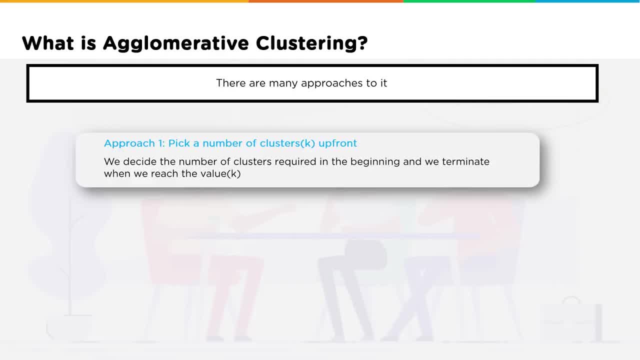 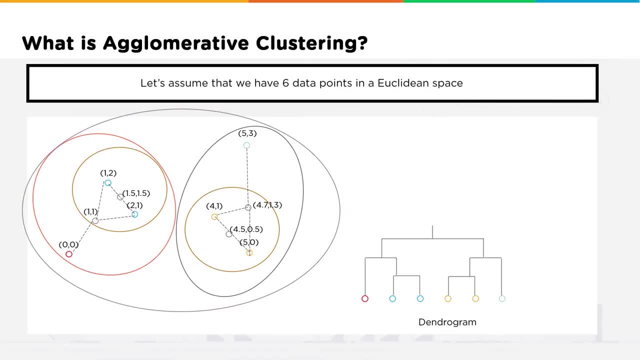 So if you looked back on our clustering- let me just go back a couple of screens- You'll see how we clustered these all together, And we might want just the two clusters, And so we look at just the top two, Or maybe we only want three clusters. 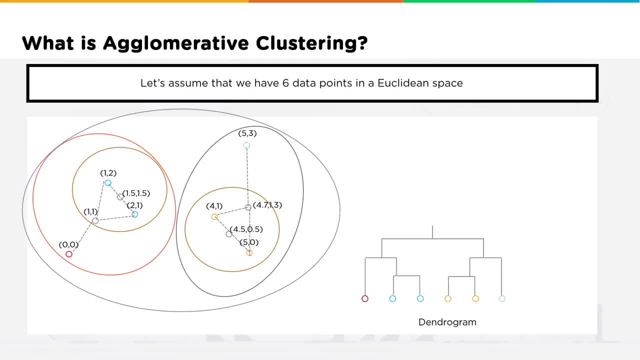 And so we would compute which one of these has a wider spread to it, or something like that. There's other computations to know how to connect them And we'll look at that in just a minute. But to note that when we pick the K value, 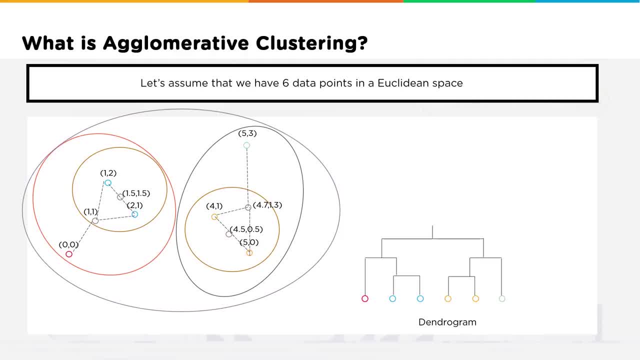 we want to limit the information that's coming in. So that can be very important, especially if you're feeding it into another algorithm that requires three values, or you set it to four values And you need to know that value coming in. So we might take the clustering and say, OK, only three clusters. 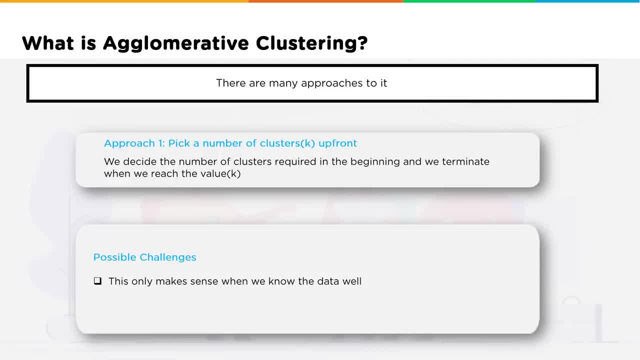 That's all we want for K. So the possible challenges: This only makes sense when we know the data well. So when you're clustering with K clusters, you might already know that domain and know that that makes sense. But if you're exploring brand new data, 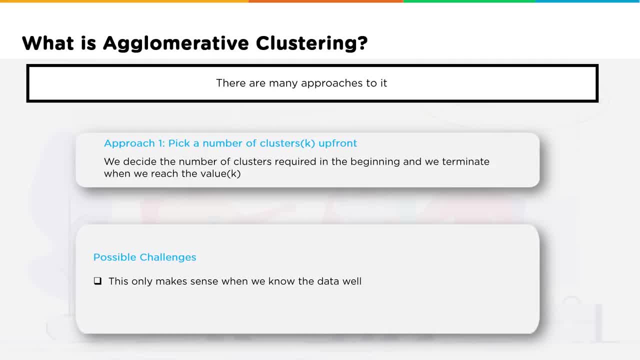 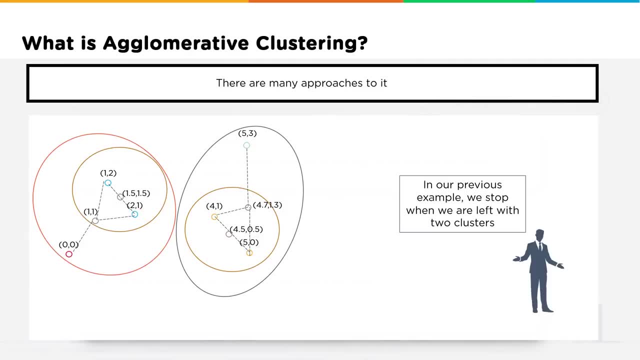 you might have no idea how many clusters you really need to explore that data with. Let's consider the value of K to be two. So in this case, in our previous example, we stop when we are left with two clusters, And you can see here that this is where. 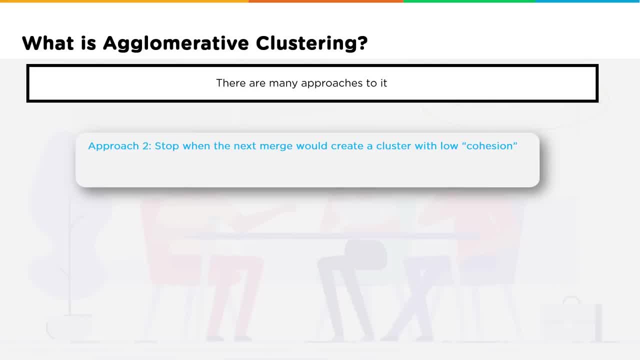 they came together the best while still keeping separate the data. The second approach is: stop when the next merge would create a cluster with low cohesion. So we keep clustering till the next merge of clusters creates a bad cluster, low cohesion set up on there. That means the point is so close to being. 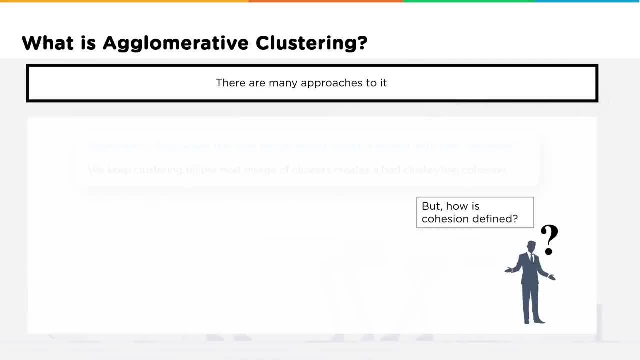 between two clusters. it doesn't make sense to bring them together. But how is cohesion defined? Oh, let's dig a little deeper into cohesion: The diameter of a cluster. So we're looking at the actual diameter of our cluster and the diameter is: 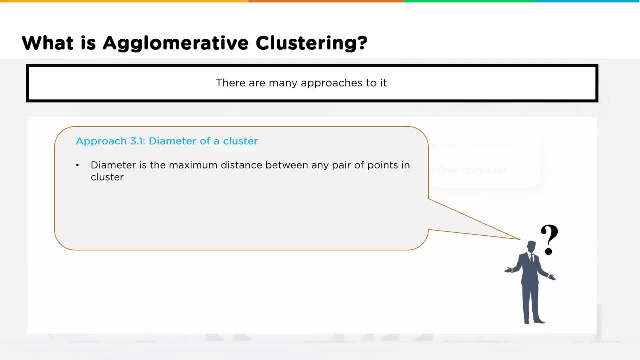 the maximum distance between any pair of points in the cluster. We terminate when the diameter of a new cluster exceeds the threshold, So as that diameter gets bigger and bigger. we don't want the two circles or clusters to overlap. We have radius of a cluster. 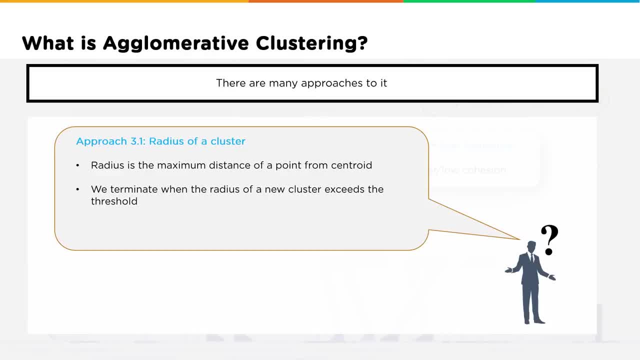 Radius is the maximum distance of a point from centroid. We terminate when the radius of a new cluster exceeds the threshold. Again, we're not. We want things to overlap. So when it crosses that threshold and is overlapping with other data, we stop. 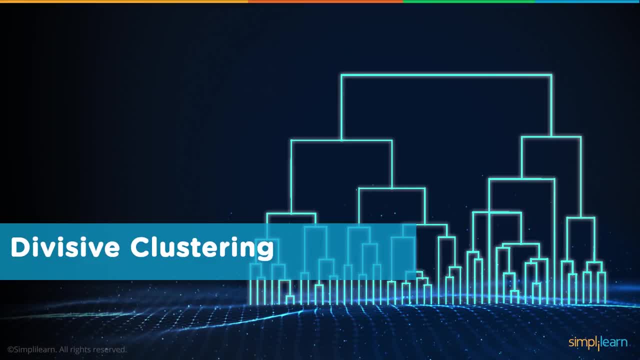 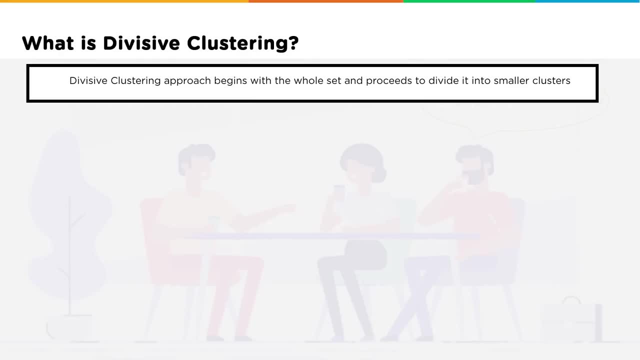 So let's look at divisive clustering. Remember, we went from the bottom up. Now we want to go from the top down. Divisive clustering approach begins with a whole set and proceeds to divide it into smaller clusters. So we start with a single cluster composed of all the data points. 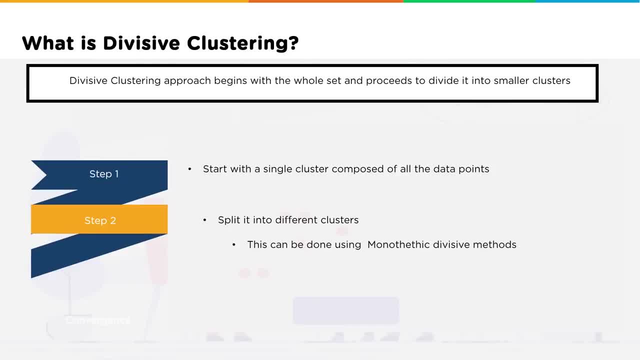 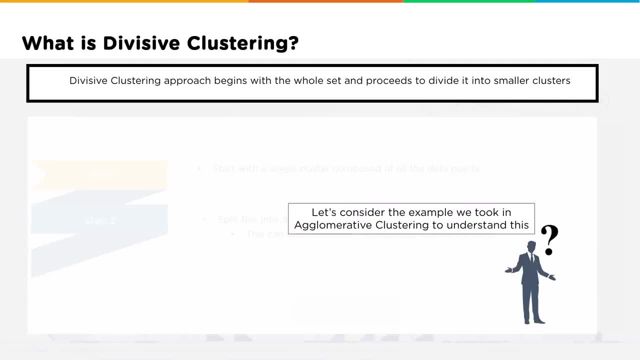 We split it into different clusters. This can be done using monothetic divisive methods. What is monothetic divisive method? And we'll go backwards And let's consider the example we took in the agglomerative clustering to understand this. So we consider a space with six points in it, just like we did before. 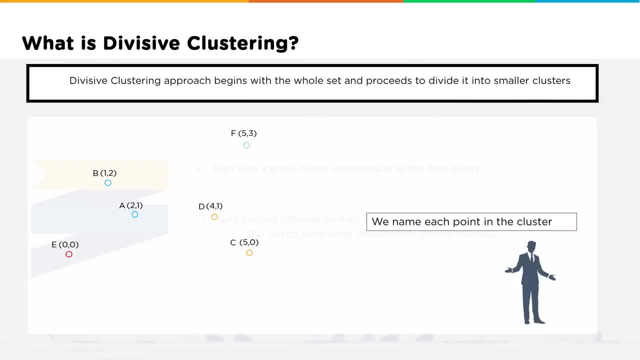 Same points we had before And we name each point in the cluster, So we have in this case. we just gave it a letter value- A, B, C, D, E, F, Since we follow top down approach and divisive clustering. 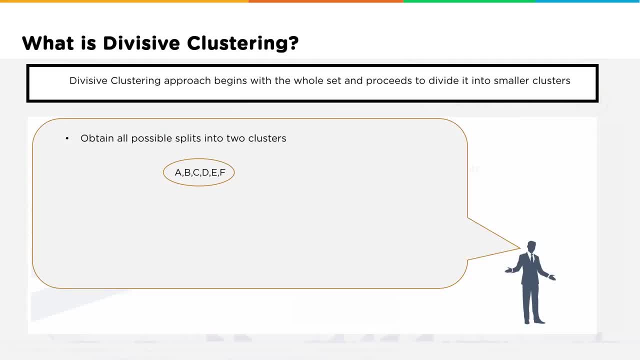 obtain all possible splits into two columns. So we want to know where you could split it here And we could do like a A B split and a, C, D, E, F split. We could do B, C, E, A, D F. 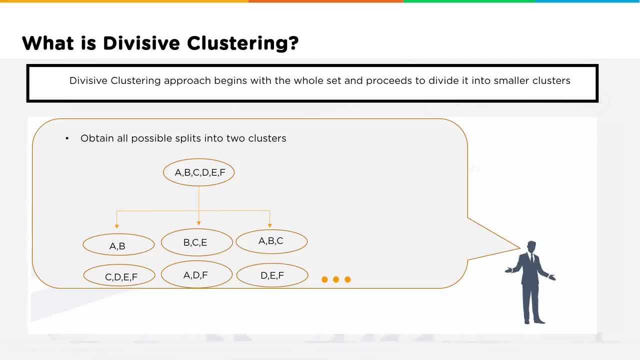 And you can see, this starts generating a huge amount of data: A, B, C, D, E, F, And so for each split we can compute cluster sum of squares And we can see here the actually have the formula out for us. 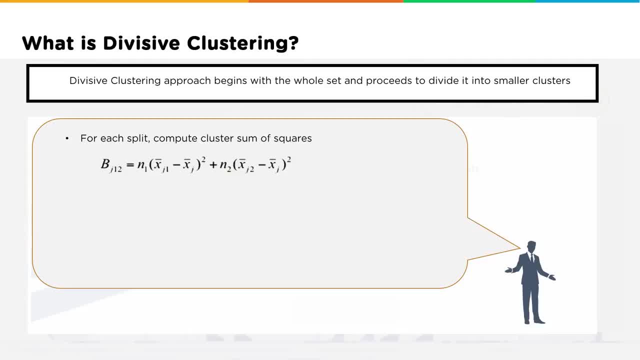 B J 12 equals N1 of absolute value of X minus absolute value of X squared. So again we're computing all the different distances in there, squared back to your kind of Euclidean distances on that, And so we can actually compute B at J. 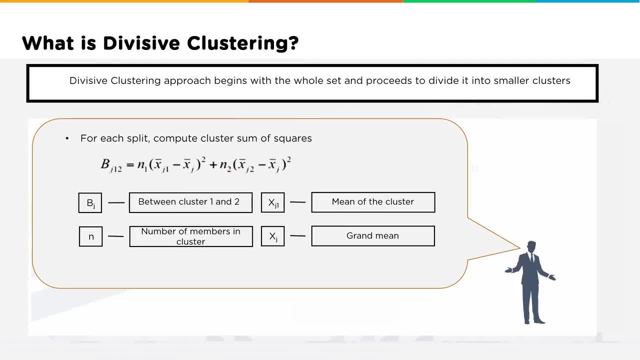 between clusters one and two. We have the mean of the cluster and the grand mean depending on the number of members in the cluster, And we select the cluster with the largest sum of squares. Let's assume that the sum of squared distance is largest for the third split we had up above. 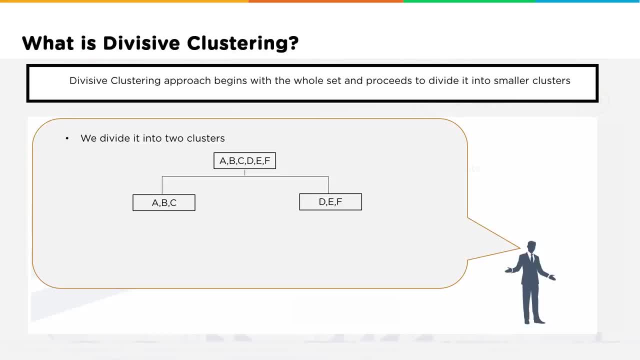 And that's where we split the A, B C out. And if we split the A B C out, we're left with the D E, F. on the other side We again find the sum of squared distances and split it into clusters. 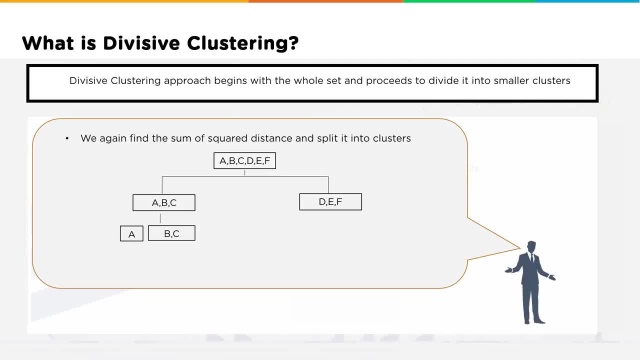 So we go from A, B, C, We might find that the A splits into B, C And D into E, F, And again you start to see that hierarchical dendogram coming down as we start splitting everything apart And finally we might have A splits in B and C and then each one gets their own D, E, F. 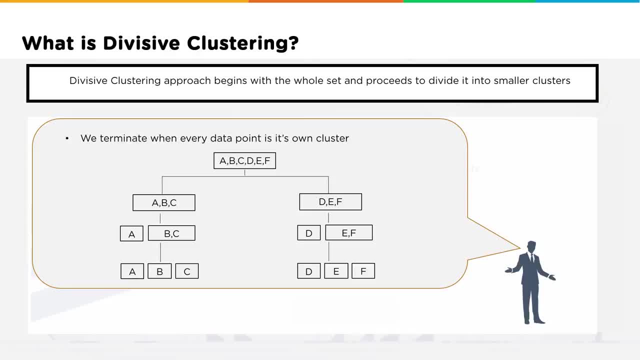 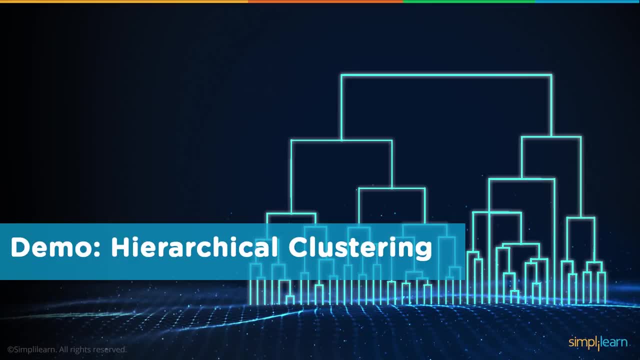 And it continues to divide until we get little nodes at the end and every data has its own point, Or until we get to K if we have set a K value. So we've kind of learned a little bit about the background and some of the math in hierarchical clustering. 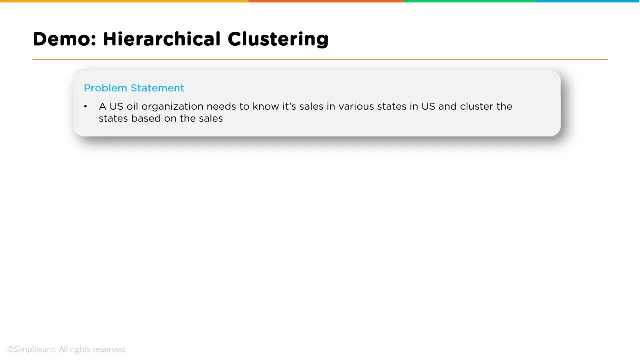 Let's go ahead and dive into a demo, And our demo today is going to be for the problem statement. We're going to look at US oil, So a US oil organization needs to know its cells in various states in US and cluster the states based on the cells. 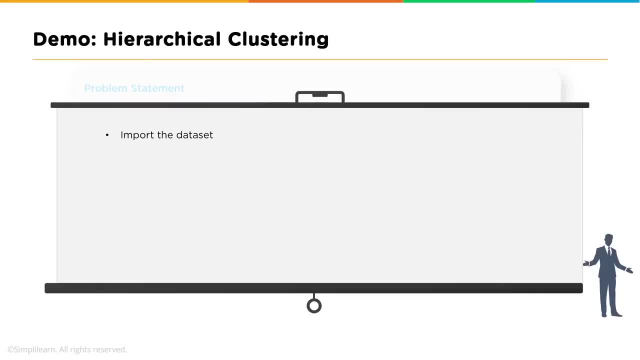 So what are the steps involved in setting this problem up? So the steps we're going to look at- and this is really useful for just about any processing of data, although I believe we're going to be doing this in R today- We're going to import the data set. 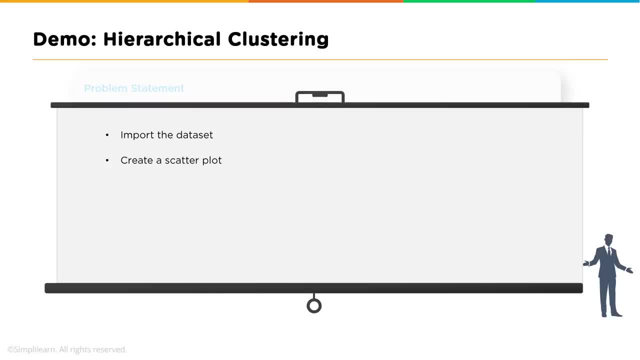 So we'll explore our data a little bit there. Create a scatter plot. It's always good to have a visual, if you can. Once you have a visual, you can know if you're really far off in the model you choose to cluster the data in or how many splits you need. 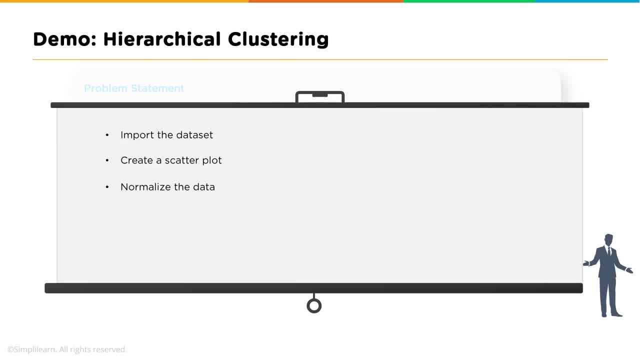 And then we're going to normalize the data. So we're going to fix the data so it processes correctly- And we'll talk more detail about normalization when we get there- And then calculate the Euclidean distance And finally we'll create our dendogram so it looks nice and pretty. 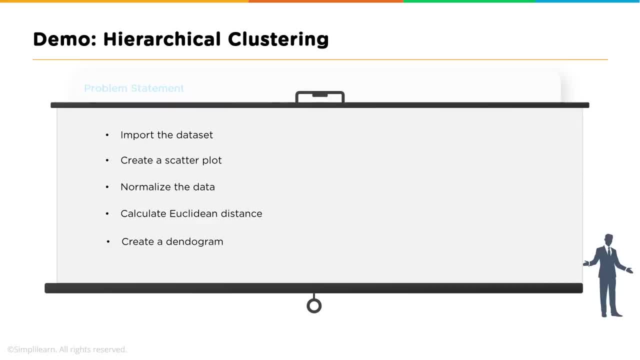 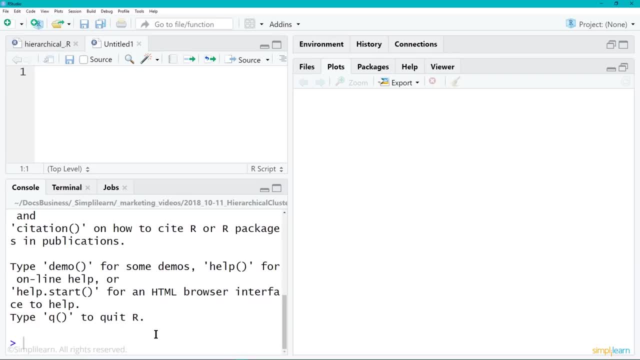 And we have something we can show to our shareholders so that they have something to go on and know why they gave us all that money in salary for the year. So we go ahead and open up R And we're actually using RStudio, which really has some nice features in it. 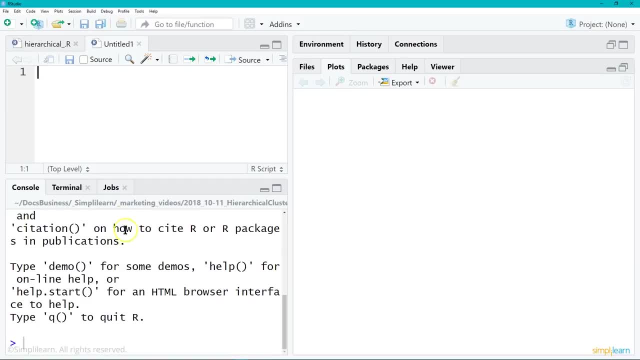 It automatically sets up the three windows where we have our script file on the upper left And then we can execute that script And it'll come down and put it into the console bottom left and execute it And then we have our plots off to the right. 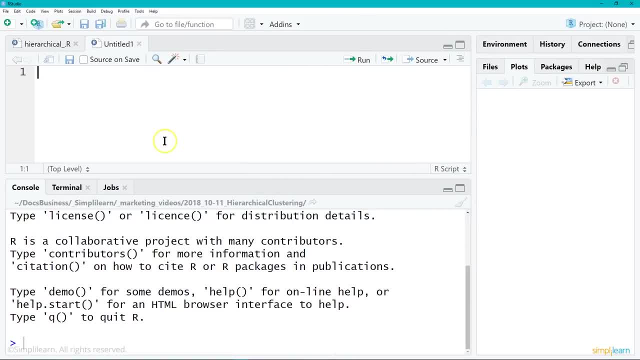 And I've got it zoomed in, Hopefully not too large a font, but large enough that you can see it. And let's just go ahead and take a look at some of the script going in here. It's clustering analysis and we're going to work. 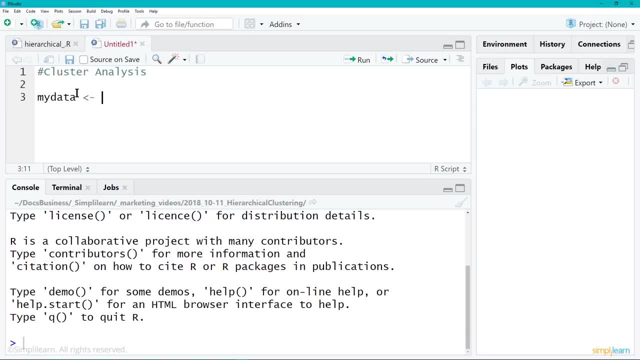 We'll call it my data and we're going to assign it in R. This is a symbol for assigning- And we're going to go read CSV, Read CSV file and put that in brackets And let's. before we go any further, let's just look at the data outside of R. 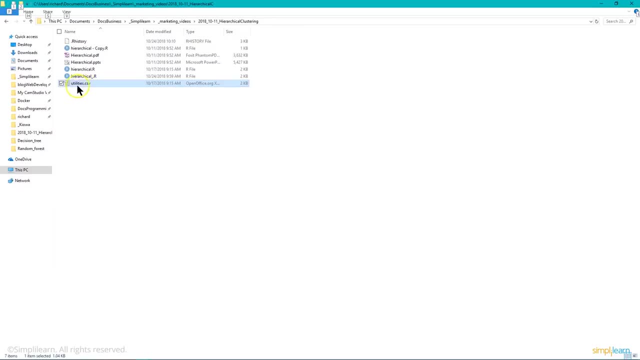 It's always nice to do if you can. The file is going to be called Utilitiescsv. This would also be the time to get the full path, So you have the right path to your file, And remember that you can always post in the comments down below. 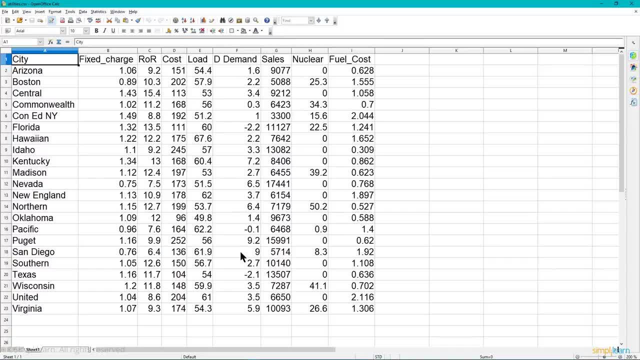 And when you post down there, just let us know you want to connect up with Simply Learn so that they can get you this file, so you can get the same file we're working on and you can repeat it and see how this works. This is Utilitiescsv. 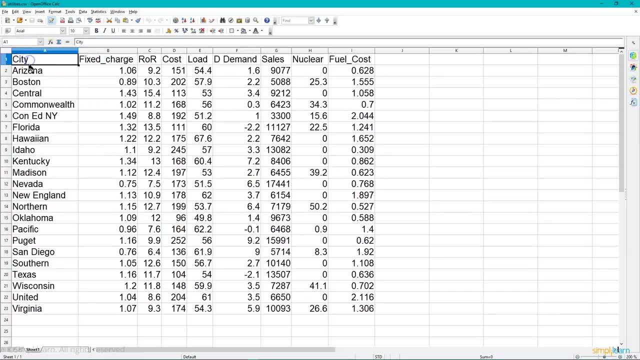 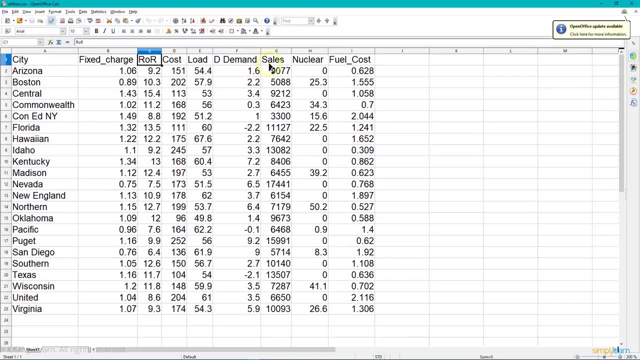 It's a comma separated variable file, so it's pretty straightforward And you can see here they have the city fixed charge and a number of different features to the data, And so we have our ROR cost load demand cells, nuclear fuel cost on here. 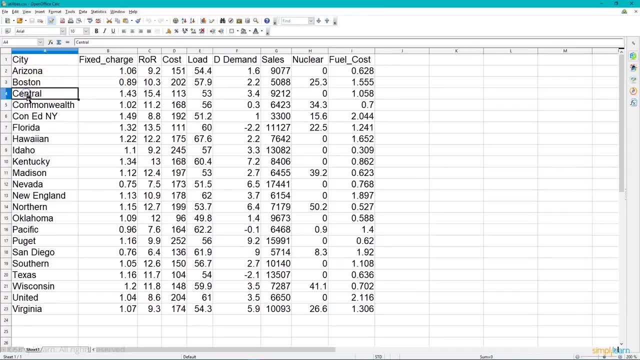 And then going down the other side, we have US cities: Arizona, Boston, They have central US. I guess they're grouping a number of areas together: The Commonwealth area- you can see down here, Nevada, New England, northern US, Oklahoma, the Pacific region and so on. 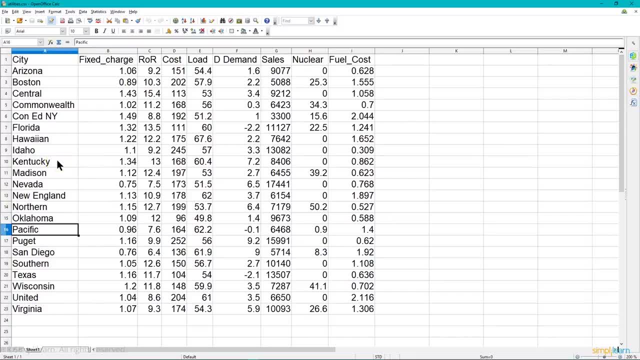 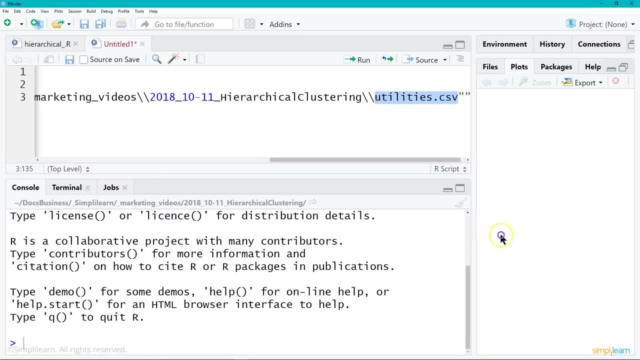 So we have a nice little chart of different data they brought in, And so I'm going to take that complete path that ends in the Utilitiescsv, and we're going to import that file. Let me just enlarge this all the way. I hope I have an extra set of brackets here somehow. 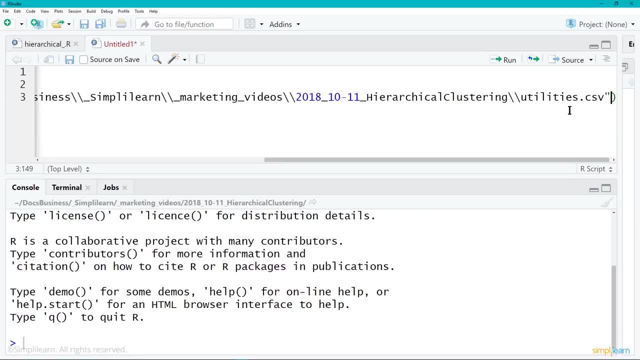 Maybe I missed a set of brackets. This can happen. if you're not careful, you can get brackets on one side and not the other, Or, in this case, I got double brackets on each side. There we go, And then the magic hotkeys in this case are your. 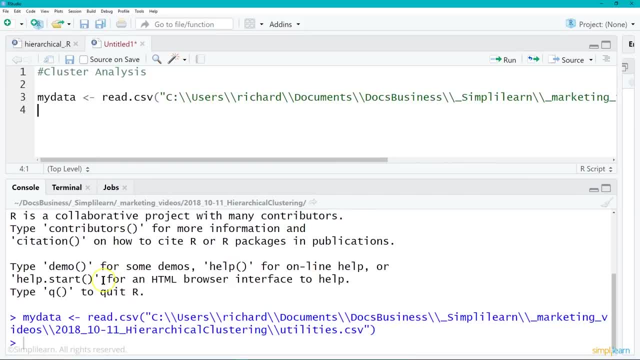 control enter, which will let me go ahead and run the script, And so I've now loaded the data And, as you can see, I went ahead and shrunk the plot, since we're going to be looking at the window down below And we can simply convert the data to a string. 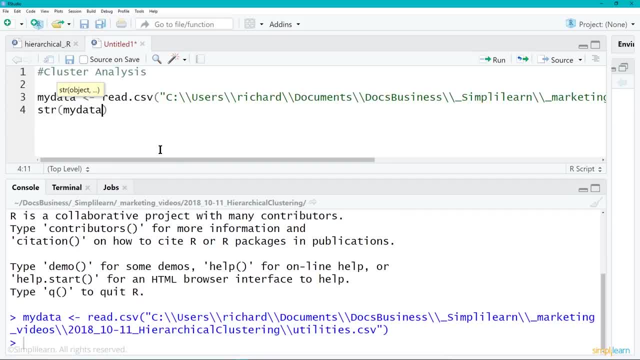 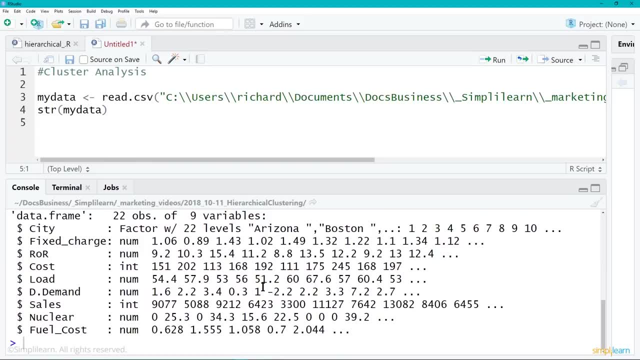 Now, all of us do this automatically the first time. we say, hey, just print it all out as a string, and then we get this huge mess of stuff that doesn't make a whole lot of sense. So when you can see here they have, you can probably kind. 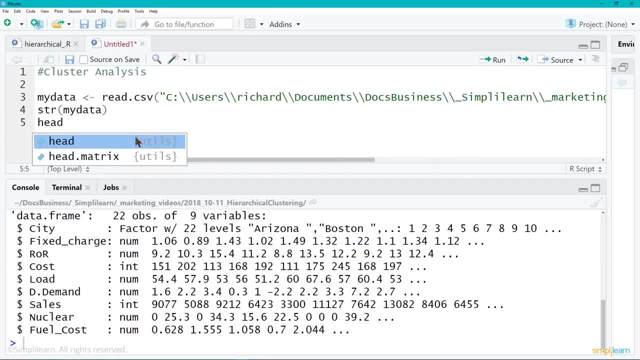 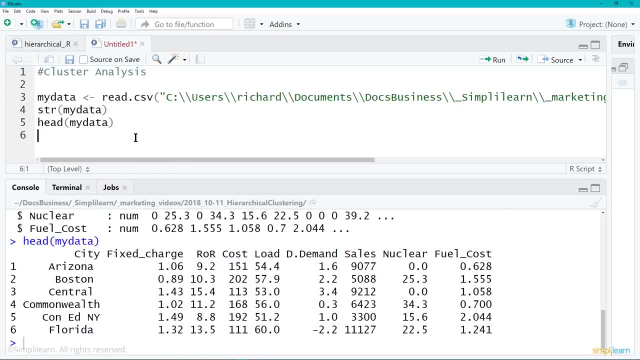 of pull it together as looking at it, But let's go ahead and just do the head. I will do the head of my data. There. we go And control, enter on that And the head shows the first five rows. You'll see this in a lot of different scripts. 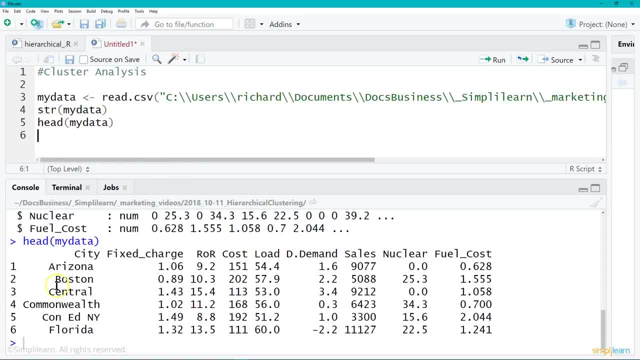 In R it's you type in head and then in brackets, you put your data and it comes through and lists the first five rows, as you can see below, And it shows Arizona, Boston, Central and it has the same columns we just looked at. 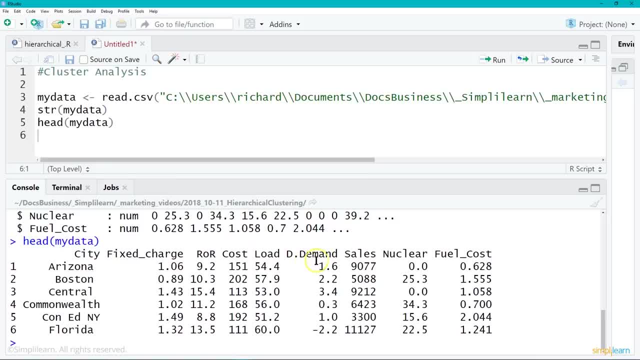 So we have the fixed charge, the ROR, the cost, the load, the D demand. I'm not an expert in oil, so I'm not even sure what D demand is. Cells, I'm guessing nuclear. how much of it's supplied by nuclear? 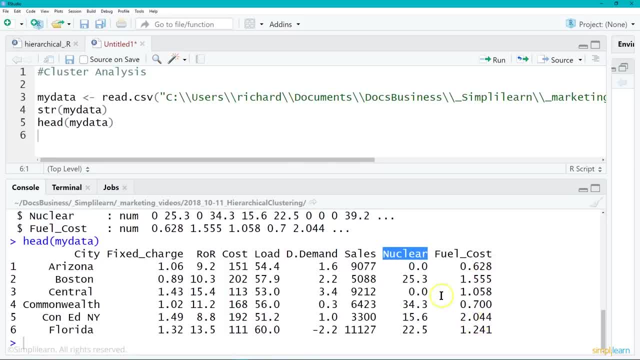 and the actual fuel cost, And then the different states that it's in are different areas, And one of the wonders of R is all these cool, easy to use tools that are so quick. So we'll do pairs, And pairs creates a nice graph. 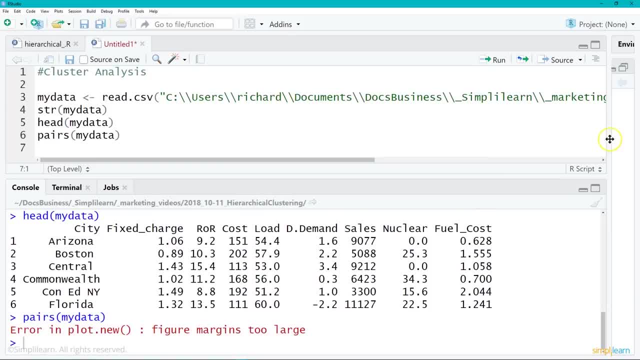 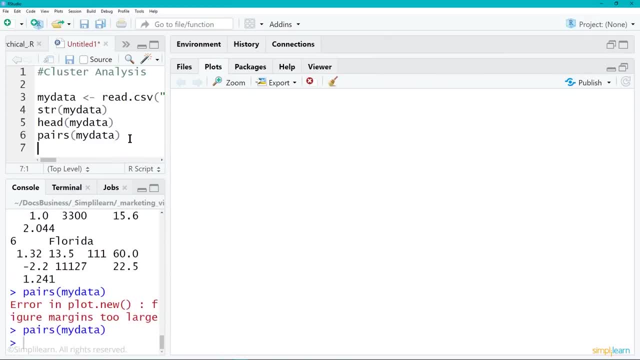 So let me go ahead And run this. Whoops. The reason it gave me an error is because I forgot to resize it, So let me bring my plot way out so we can see it. And let's run that again, And you'll see here that we have a nice graph of the different data and how. 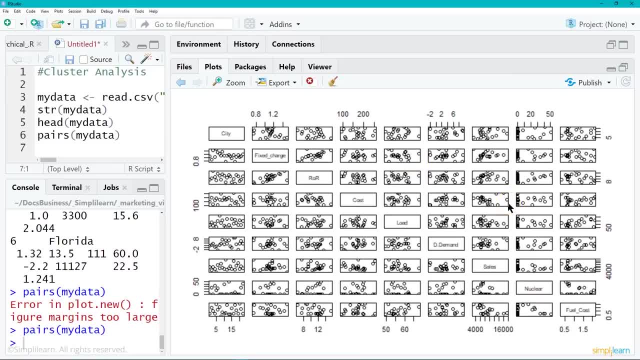 it plots together how the different points kind of come together. This is neat because if you look at this, I would look at this and say, hey, this is a great candidate for some kind of clustering. And the reason is is when I look at any two pairs, 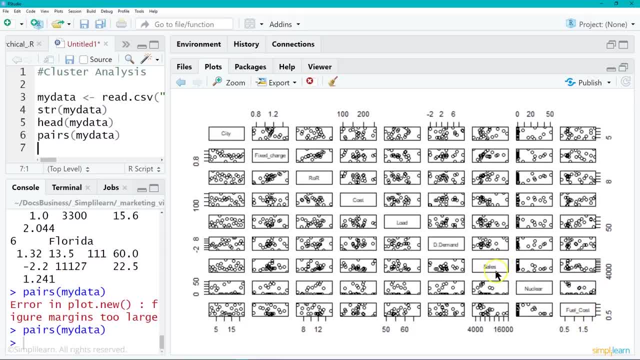 let's go down to say cells and fuel cost towards the bottom right And when you look at them where they cross over, you sort of see things how they group together, but it's a little confusing. You can't really pinpoint how they group together. 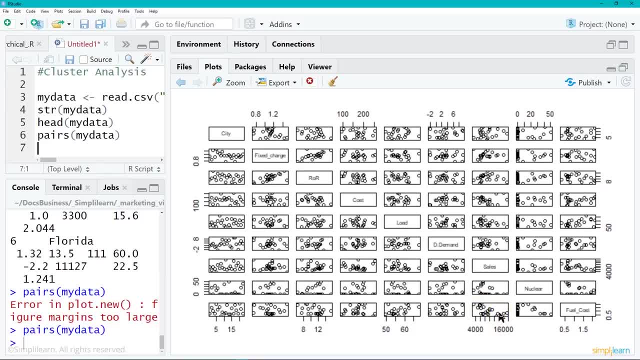 You could probably look at these two and say, yeah, there's pretty good commonalities there, And if you look at any of the other pairs, you'll start seeing some patterns there also, And so we really want to know what are the patterns on all of them put together? 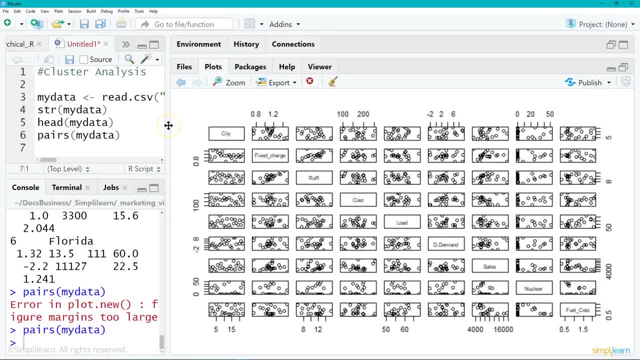 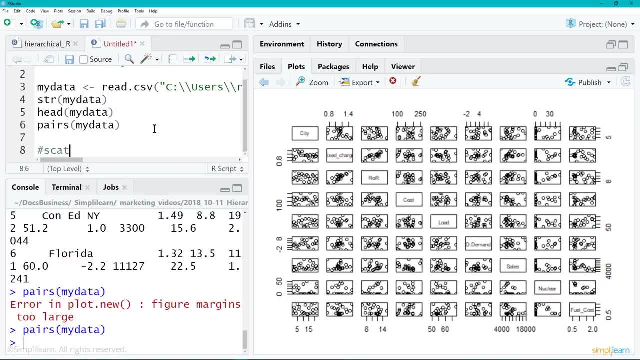 not just any two of them, but the whole setup. Let me go ahead and shrink my this down for just a second, just a notch here, And let's create a scatter plot, And this is simply just use the term plot in brackets. and then, which values do we want to plot? 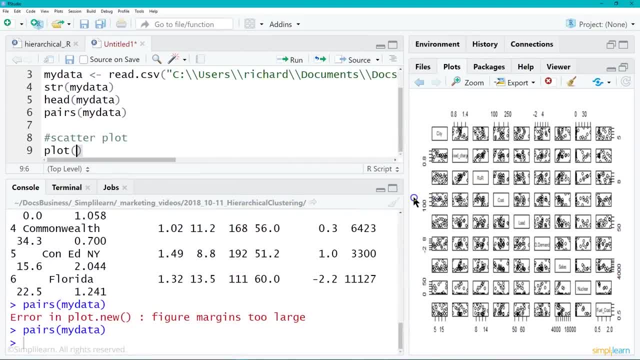 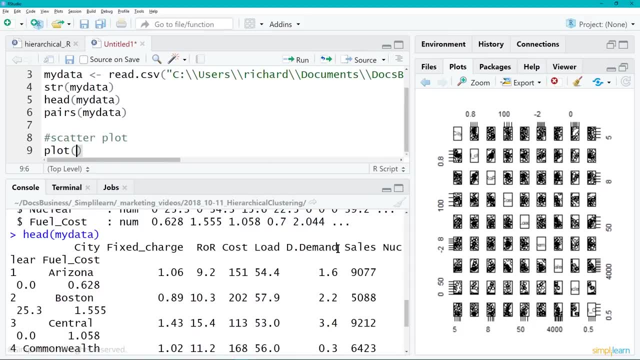 And if we remember when we looked at the data earlier, we just go back this way. In this case, let's go ahead and compare to just two values to see how they look, And we'll do fuel cost and cells, and it's in my data. 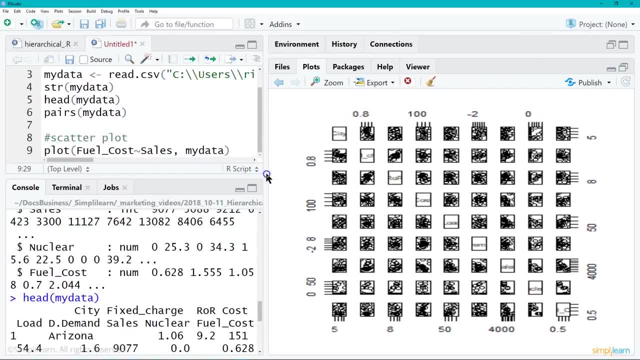 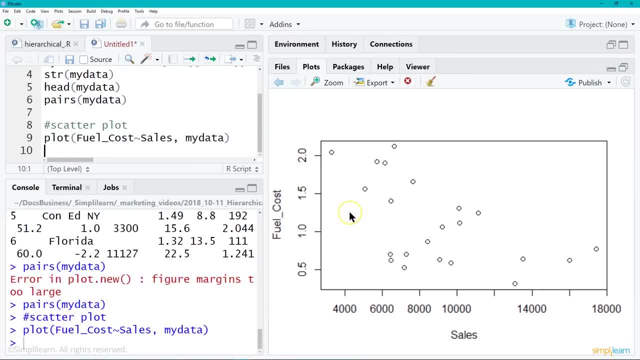 So we got to let her know which two columns we're looking at next to each other And it will open up our plot thing and then go ahead and execute that And we can see on those close up of what we were just looking at in the pairs. 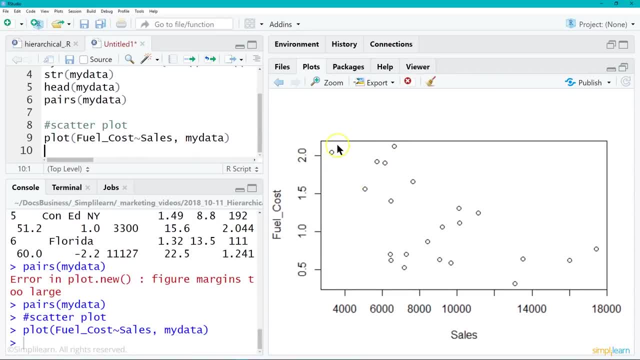 And if I was eyeballing this I would say: oh look, there's a kind of a cluster up here of five items, and this one is hard to tell which cluster it would be with, but maybe it's six, to go in the top one. 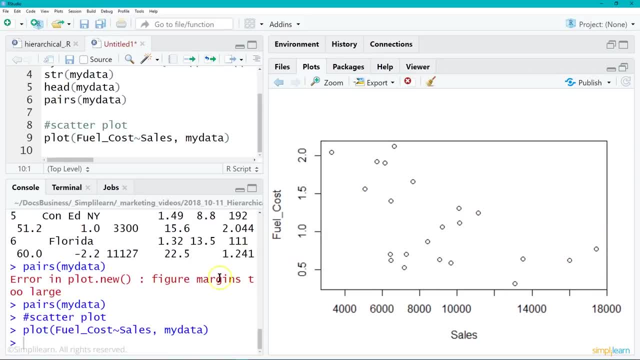 And you have a middle cluster and a bottom cluster, maybe two different clusters, So you can sort of group them together- fuel cost and the cells- and see how they connect with each other. And again, that's only two different values we're looking at. 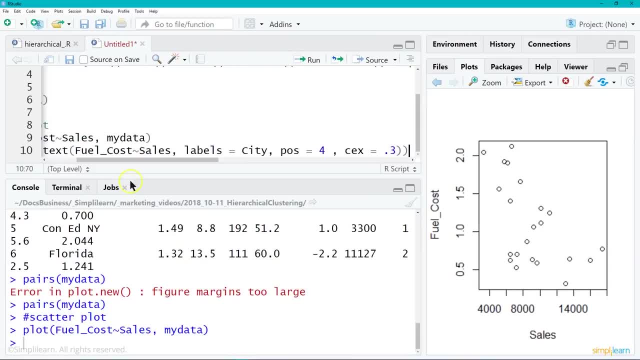 So in the long run we want to look at all of them. And then the people in the back. they sent me the script so we can go ahead and add labels. So with my data text, fuel cost cells, the labels equals city position four. 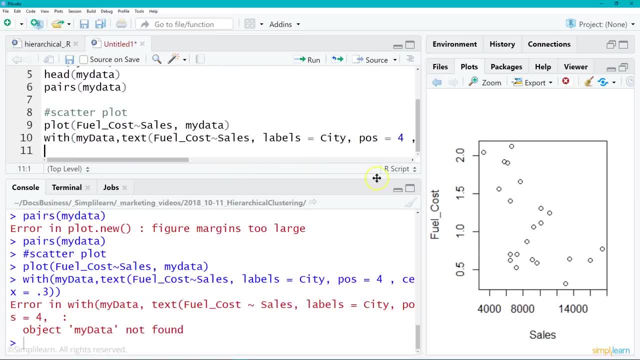 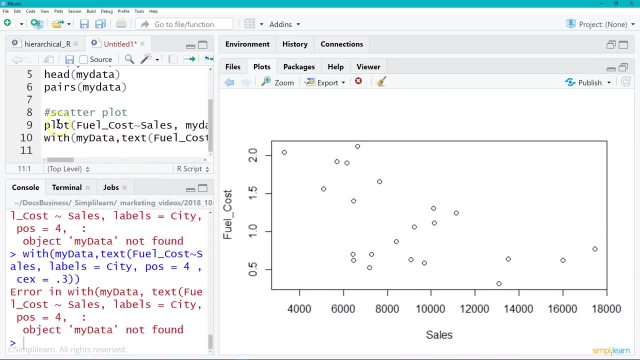 These are numbers you can kind of play with till they look nice. And oops again, I forgot to resize my plot. It doesn't like having it too small And we'll run that. I mistyped something in here. Oh, I did a lowercase D and they did a capital D. 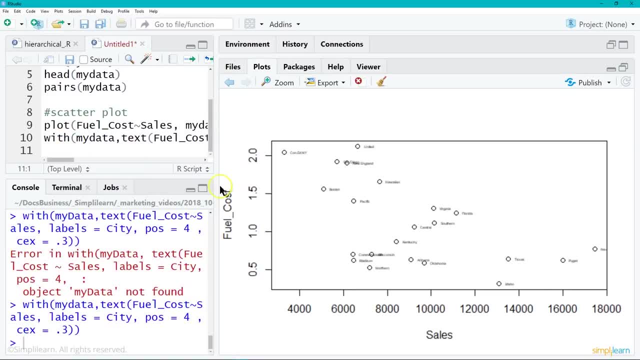 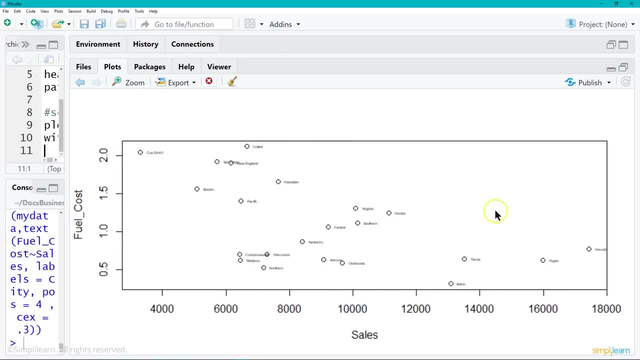 There we go. So now we can go in here and do this with my data And you can see a little hard to see on my screen with all the different things in there. It plots the actual cities. so we can now see where all the cities are in. 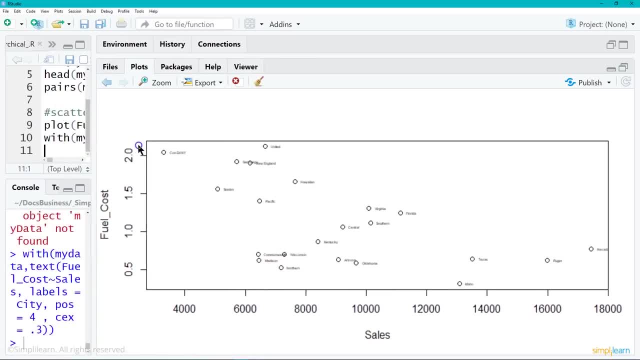 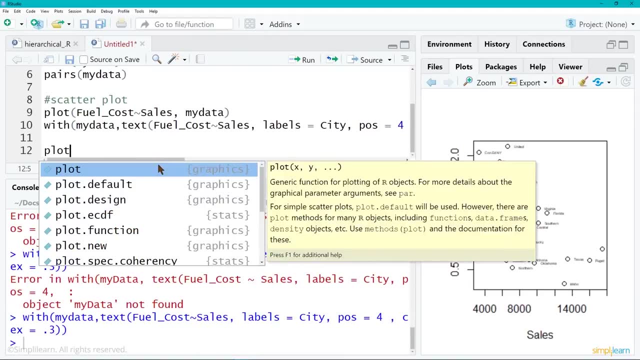 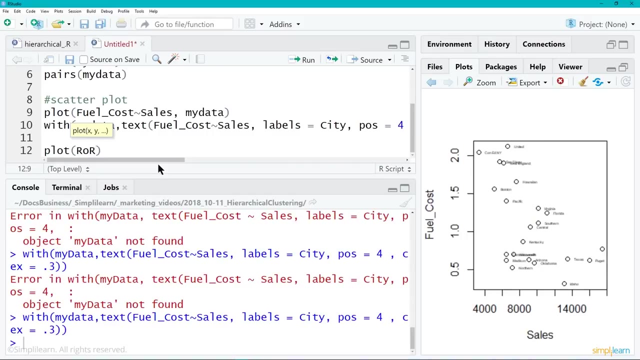 connection with, in this case, fuel cost and cells. So you have a nice label to go with the graph And then we can also go ahead and plot. in this case, let's do oh, the ROR, Oops, And we'll do that. 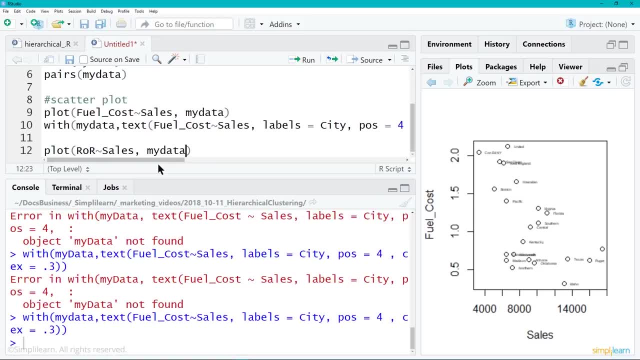 Also with the cells and do my data. remember to leave it lowercase this time. So we plot those two. We'll come over here and it's going to- I'm surprised it didn't give me an error- And then we'll also add in the with statement. 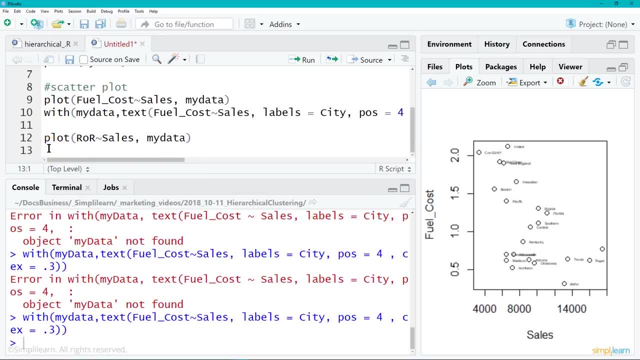 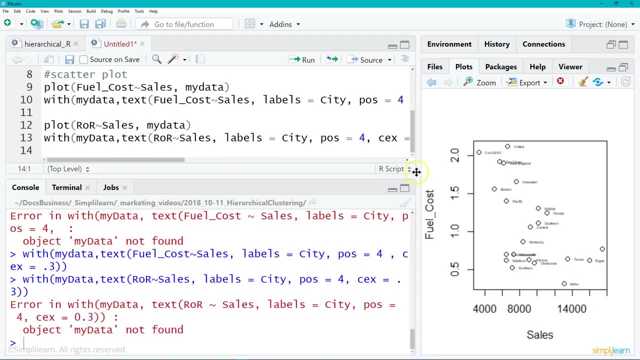 So we put some nice labels in there And it's going to be the same as before, except instead of doing the fuel cost cells, we want the R cells. We'll execute that. Oops, and of course it gives me an error because I shrunk it down. 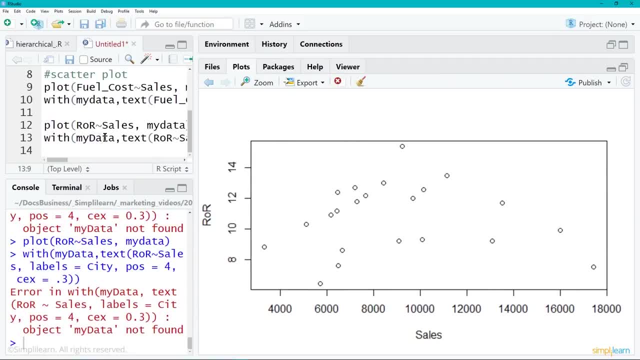 So let's redo those two again. There we go, So we can see. now we have the ROR with cells and we'd probably get a slightly different clustering here. if I was looking at these cities, They're probably different than what we had before. 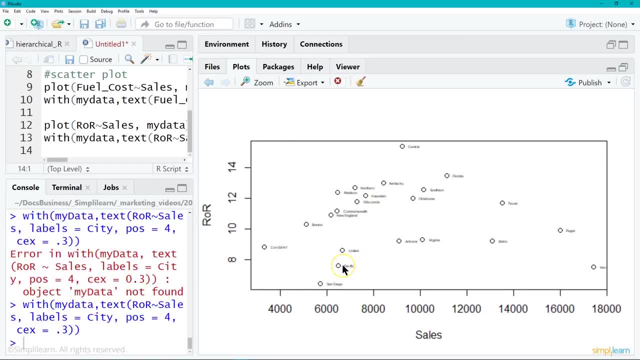 But you could probably look at this and say, oh, these kind of go together and those kind of go together, but again, we're going to be looking at all of them instead of just one or two, And so at this point we want to dive into the next step. 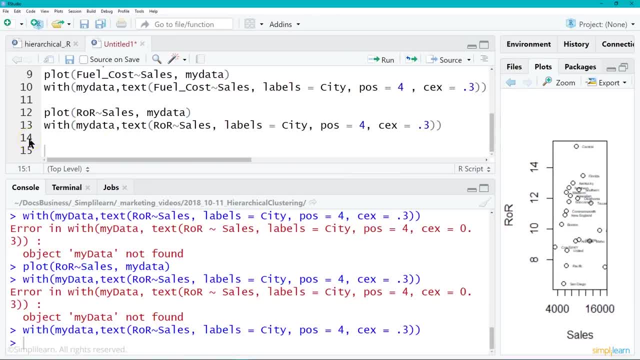 We're going to start looking at a little bit of coding or scripting here. This is very important because we're going to be looking at normalization. We put that in there: normalization, and if you've done any of the other machine learning skills and set up. 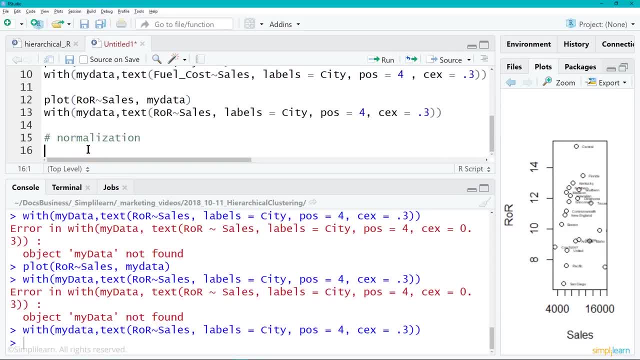 this should start to look very normal in your preprocessing of data, whether you're in R or Python or any of these scripts. We really want to make sure you normalize your data so it's not biased. Remember we're dealing with distances And if I have, let's say, the ROR is even. look at this graph here on the right. 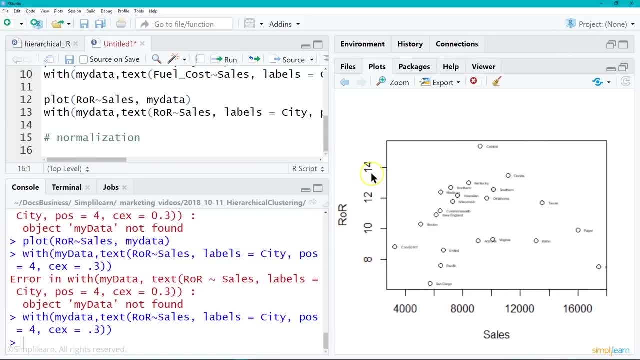 You can see where my ROR varies between 8 and 14.. That's a very small variable, And our cells varies between 4,000 and 16,000.. So you can imagine the distance between 4,000 and 8,000, which is a distance. 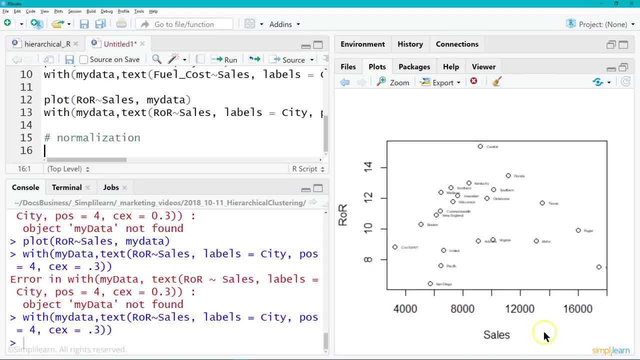 of 4,000 versus 8, to 10 versus 2, the cells is going to dominate. So if we do any kind of special work on this, it's going to look at cells and it's going to cluster them just by the cells alone. 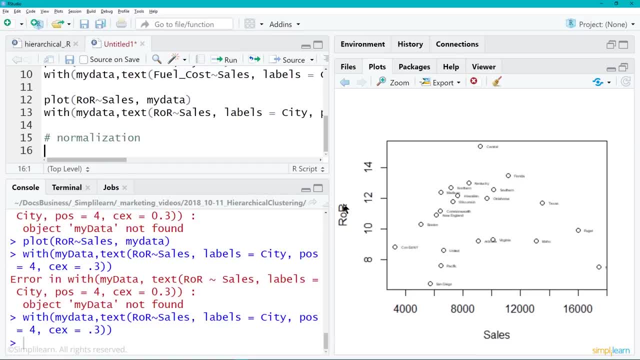 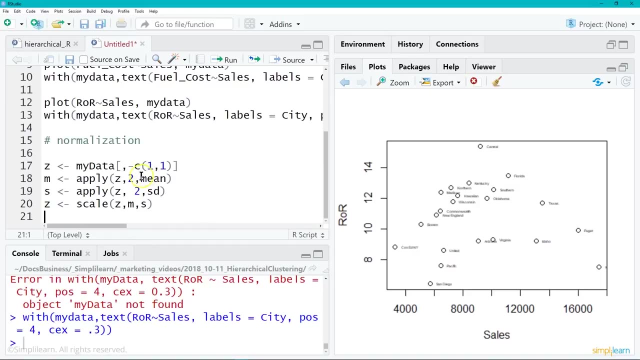 And then ROR might have a little tiny effect of two versus 4,000.. We want to level the playing field. Turns out there's actually a number of ways in script to normalize, so I'm just going to put in the code that they put together in the back for me. 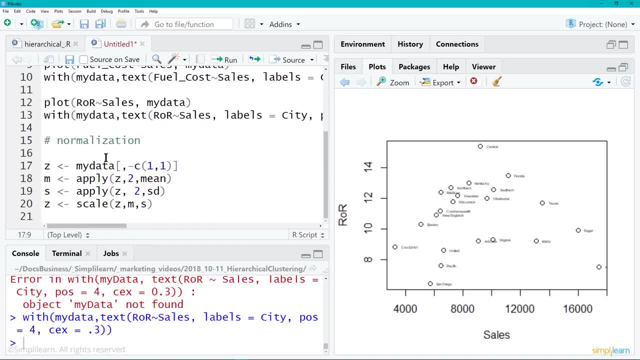 And let's talk about it a little bit. So we have Z, We're going to assign it to my data And it's go ahead, and We're going to do a little reshaping across all rows, or across all columns, each of the rows. a little reshaping there. 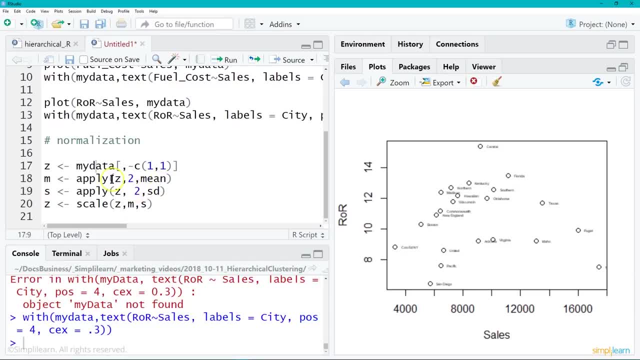 And then we're going to get M, which stands for means, And we're going to apply it to my data. So again, we want to go ahead and create a, the most common variable in there, And then S is going to be. SD stands for standard deviation. 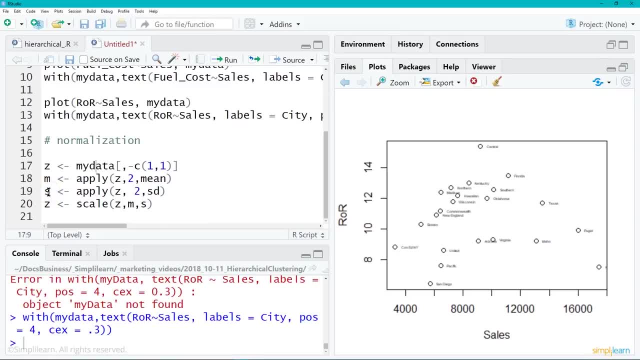 So, instead of just doing a lot of times, what they do with normalization of data is we just reshape the data, everything between zero and one, so that if the lower end is eight, that now becomes zero, and the upper end is 14, that now becomes one. 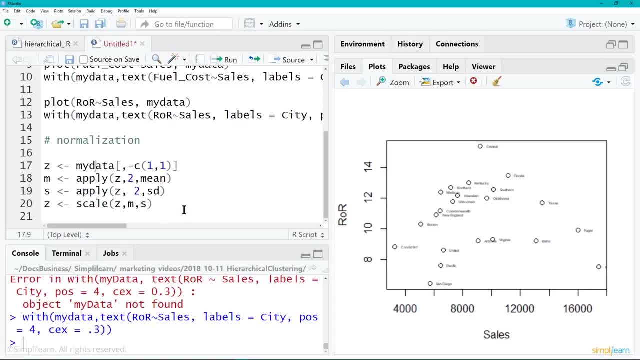 That doesn't help if it is not a linear set of data. So with this we're going to look for the means and the standard deviation for reshaping the data, and that way the most common values now become kind of like the center point and then the standard deviation is how big the spread. 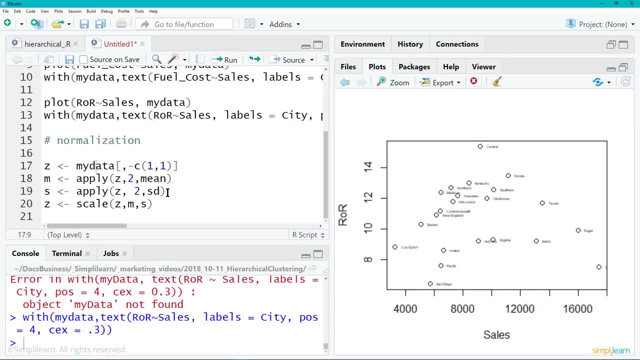 So we want the standard deviation To be equal amongst all of them. And then, finally, we go ahead and take Z And with the Z, we're going to reassigned it and we're going to scale the original, my data, which we reshaped based on M and based on the standard deviation. 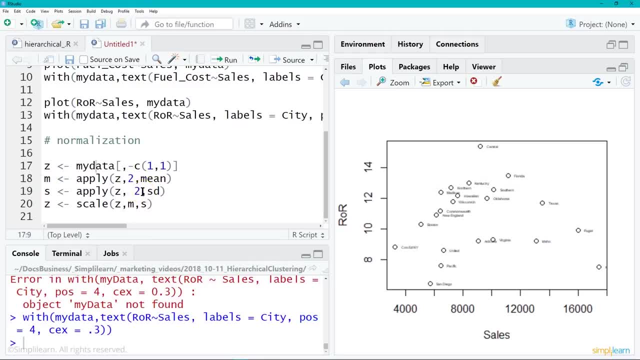 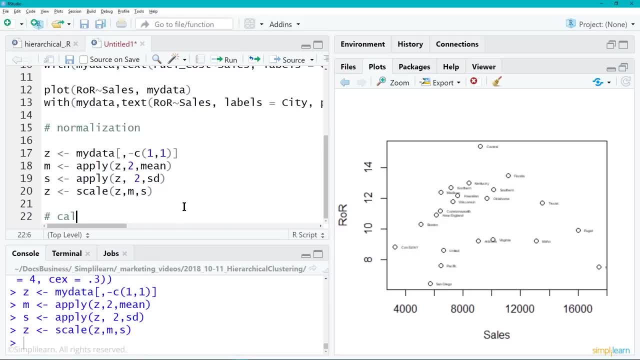 And now we can go ahead and calculate the Euclidean distance. Oops, calcu, There we go, And in R. this is so easy. Once you've gotten to here, we've done all that pre data processing. We'll call it distance. 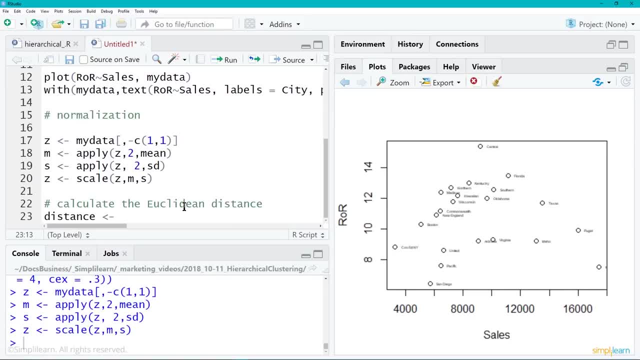 And we'll assign this to dist. so dist is the computation for getting the Euclidean distance, And we can just put Z in there. because we've already reformatted and scaled Z to fit what we want, Let me go ahead and just hit enter on that. 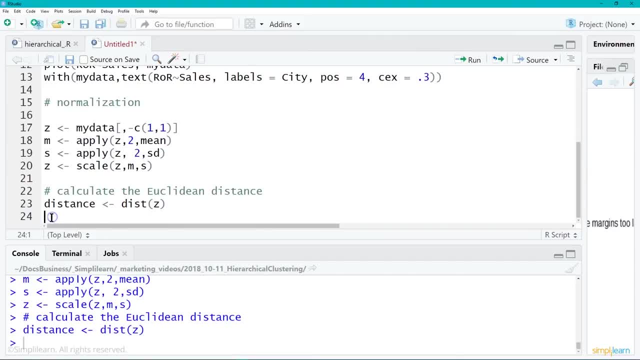 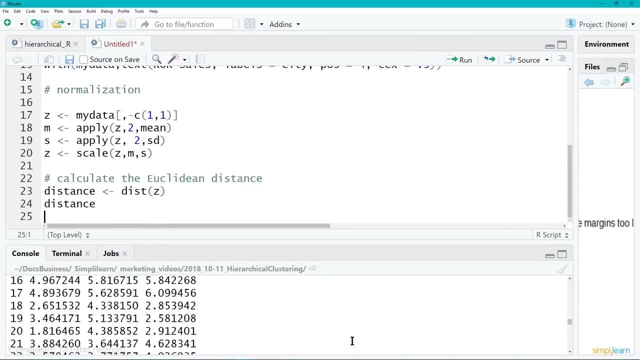 And I'm going to widen my left hand side again. I'm always curious: what does this data look like? So let's just type in distance, which will print the variable down below. Oops, I have to hit control enter And this prints out a huge amount of information. 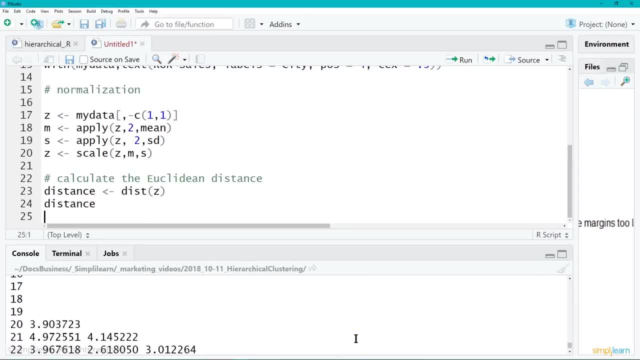 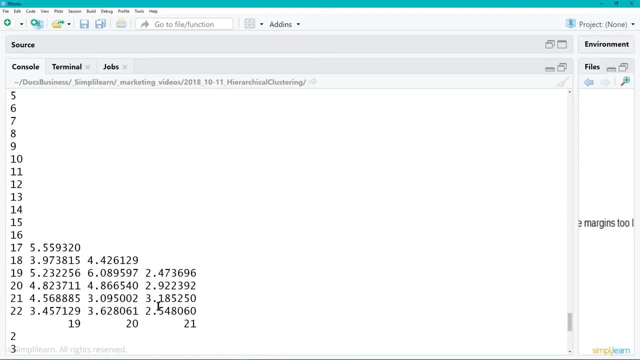 as you can see just kind of streams down there And let's go ahead and enlarge this. And I don't know about you, but when I look at something like this it doesn't mean a whole lot to me, other than I see two, three, four, five, six. 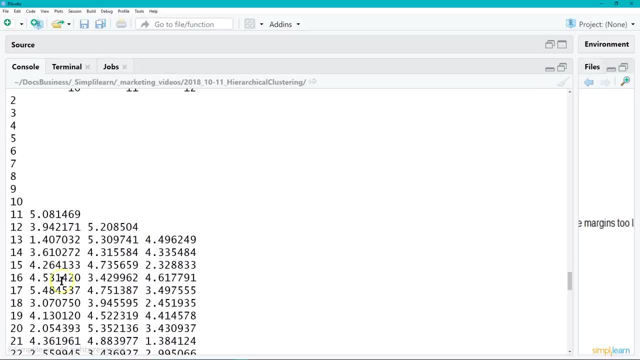 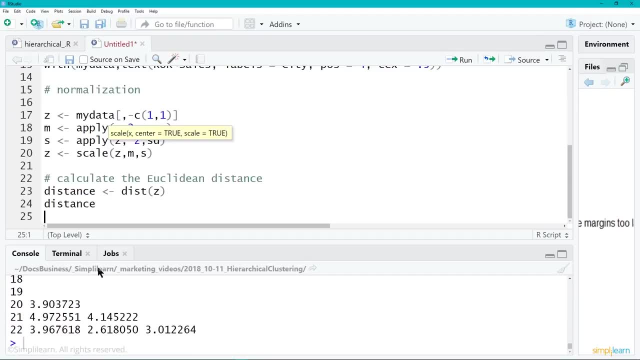 And then you kind of have the top part- six, seventeen, eighteen. So imagine this is like a huge chart. It's what we're looking at And we can go ahead and use print. Oh, distance Digits Equal three. 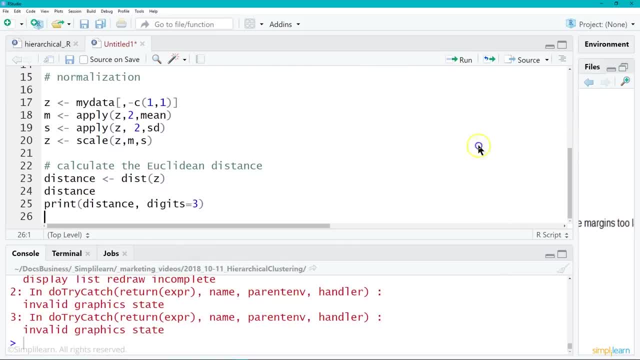 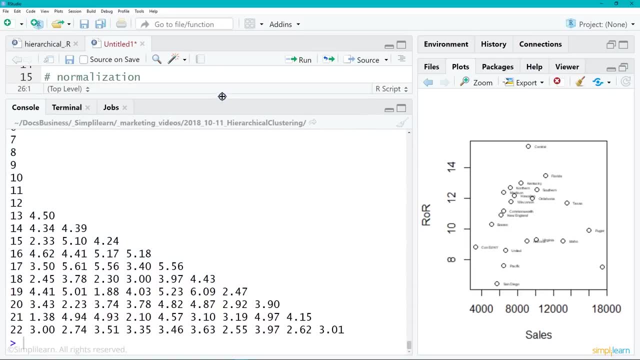 And let's run that. Oops, I keep forgetting that it has to go through the graph on the right And we see a different, slightly different output in here. Let me just open this up so we can see what we're looking at. 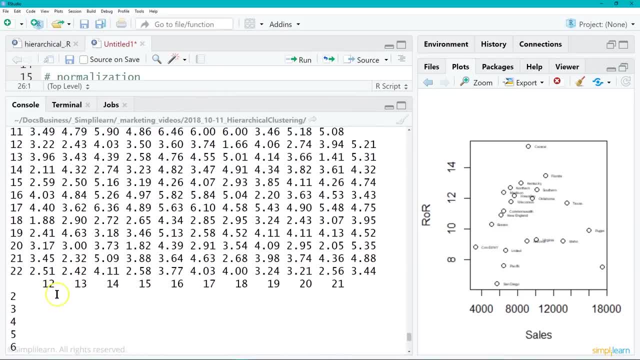 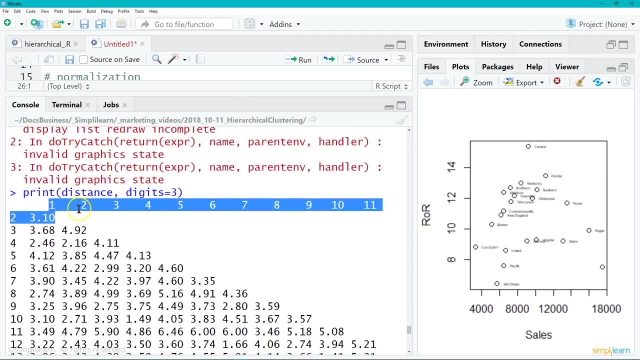 And by cutting down the distance you can start to see the pattern. You can see the patterns here if it's looking at the different distances. So if I go to the top, we have the distance between one and two, one and three, one and four, one and five, one and six, and then two and three and so on. 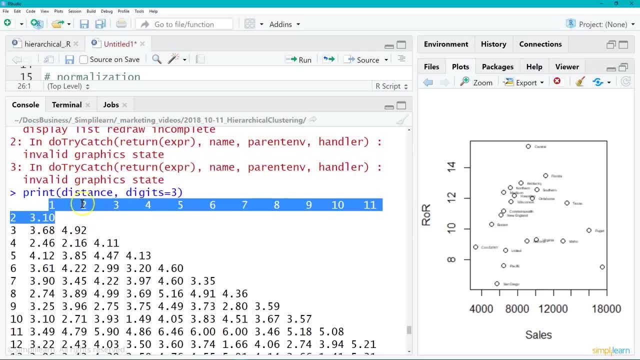 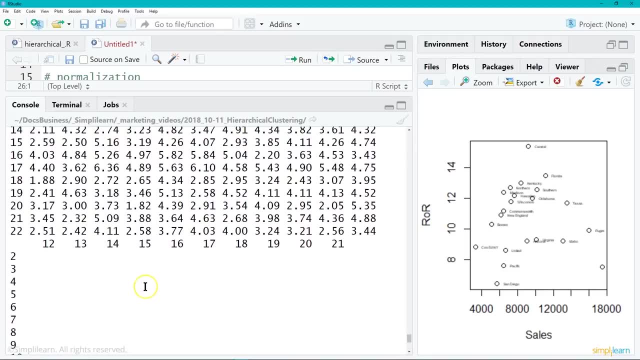 Obviously the distance between itself is zero and it doesn't repeat the data, So we don't care to see two versus one again. We already know the distance between one and two, And so we have a nice view of all the distances in the chart. 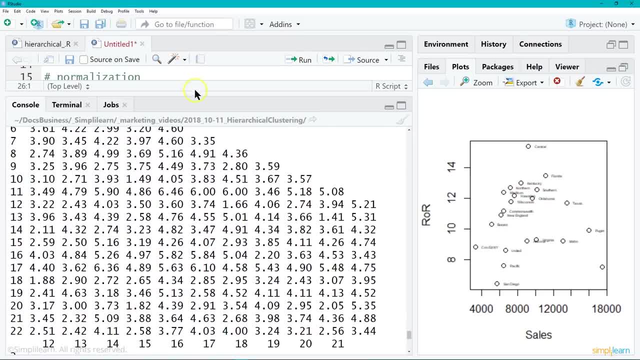 And that's what we're looking at right here And it's a little easier to read. That's why we did the print statement up here. To do: digits equals three make it a little bit smaller. We could even just do digits. 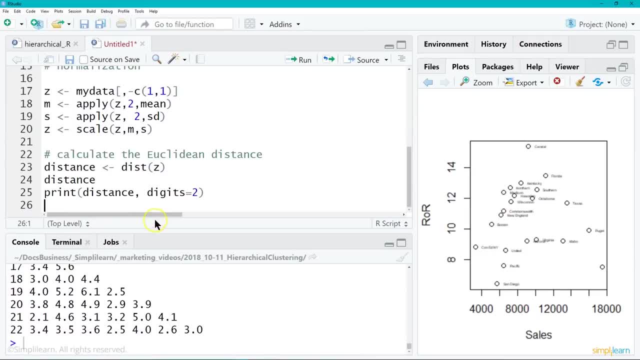 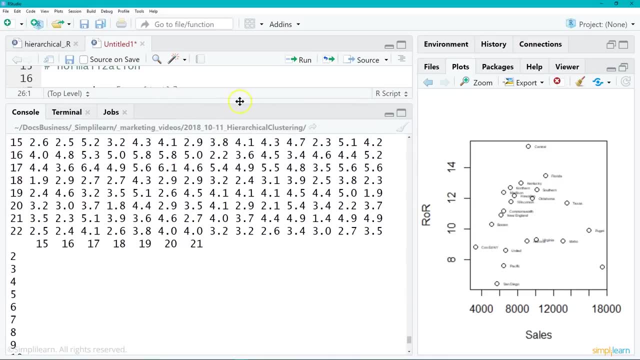 Well, let's just do two see what that looks like. We might lose some data on this one if it's if something's way off, But we have a nice setup and we can see the different distances, And that's what we have computed here between each of the points. 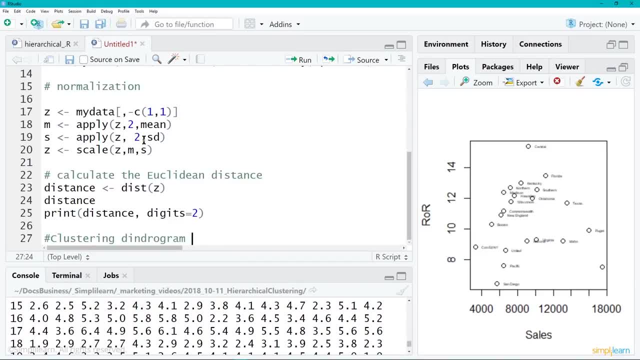 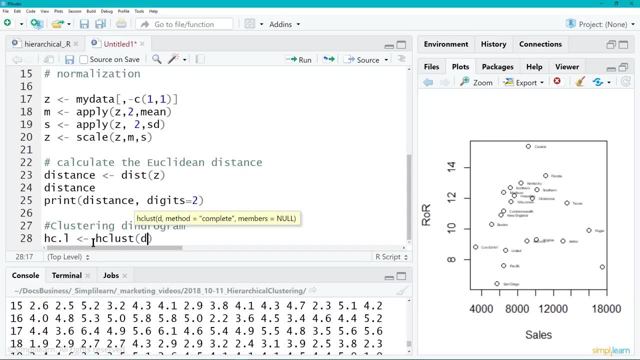 And then the whole reason we're doing this is to get ourselves a nice dendogram going, a nice clustering dendogram. We'll do a couple of these, looking at different things. So we have a variable hcl and we're going to assign it h, cluster and then distance. 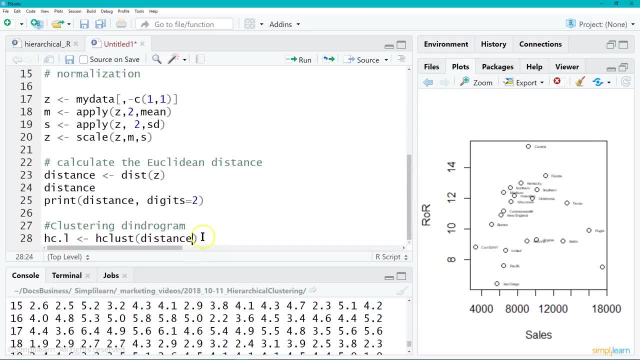 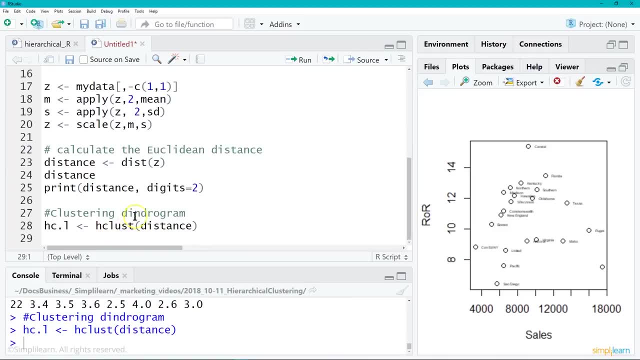 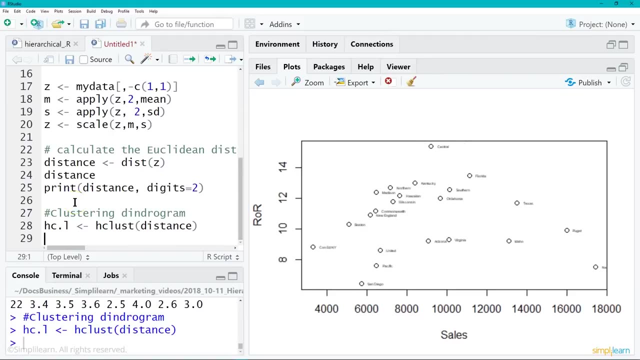 That easy. We've already computed the distances, so the h clustering does all the work for us, And let me hit enter on there. So now we have our hcl, which is assign, the h clustering, computation based on distances and apart. And then I'm going to expand my graph because we would like to go ahead and see what this looks like. 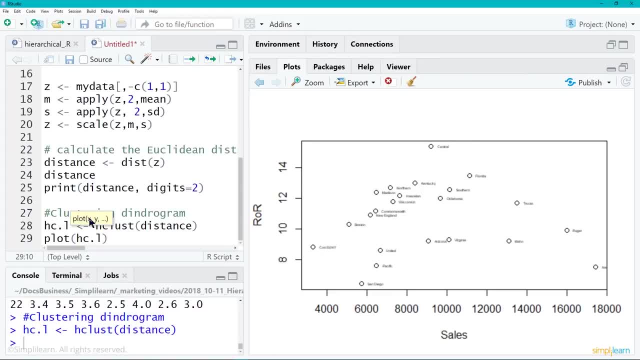 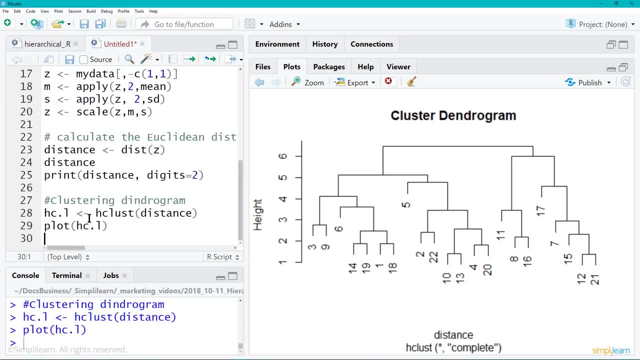 And we can simply plot that And hit the control, enter so it runs And look at that. we have a really nice clustering dendogram. Except when I look at it, the first thing I notice is it really shows like numbers down below. 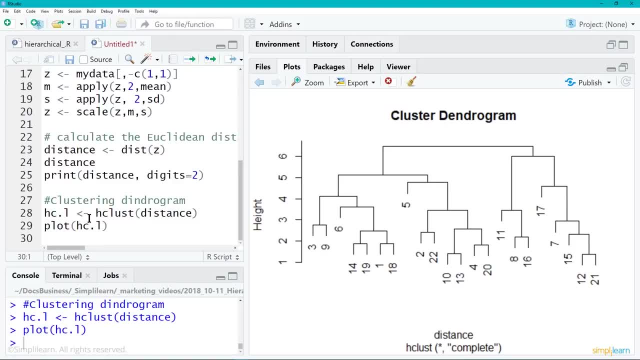 Now, if you were a shareholder and some data scientist came up to you and said: look at this, this is what it means. you'd be looking at that, going what the heck does 3,, 9,, 14,, 19,, 1, 18 mean? 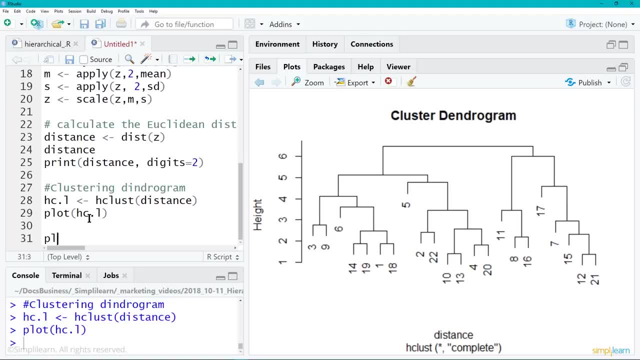 So let's give it some words there. So let's do the same plot with our hcl, Hc. There we go, And let's add in labels. And this is just one of the commands and plots. So we have labels. equals my data. 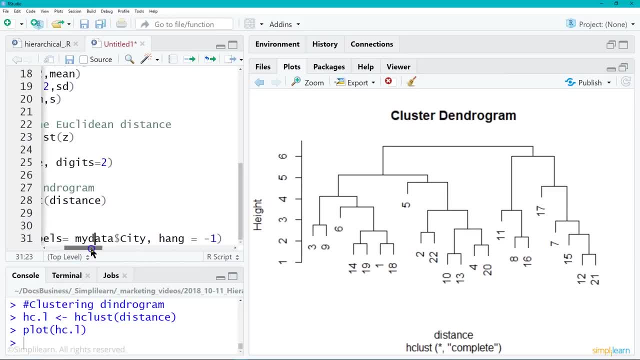 And then, under my data, we want to know the city And we'll have it hang minus one. That's just the instructions to make it pretty, So we'll run that. Okay, Oops, I accidentally ran. just hang my one. Let me try that again. 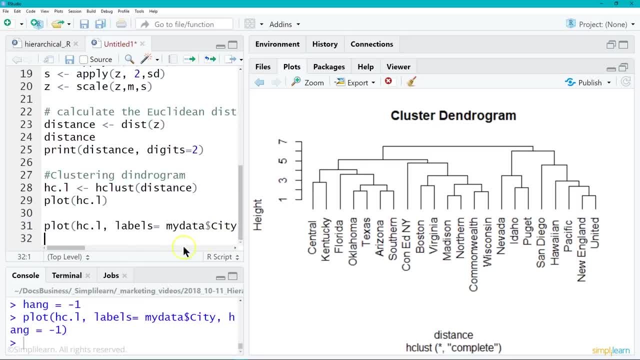 There we go, Okay, So now you can see what it's done And the hang. my one turns it sideways. That way we can see Central, which is Central US, and Kentucky, And we start to actually get some information off our clustering setup. 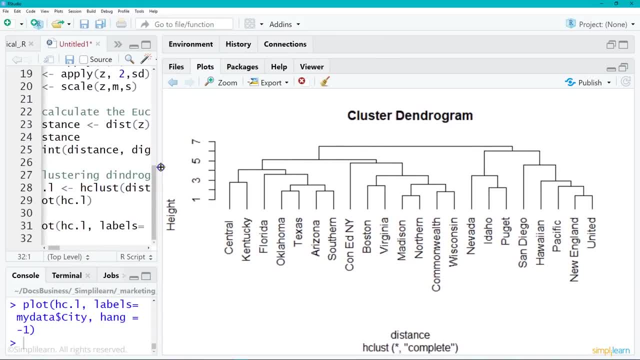 And the information you start looking at is that, when we put all the information together, you probably want to look at Central America and Kentucky together. Oklahoma and Texas has a lot of commonality, as does Arizona and Southern US, And you can even group all five of those. 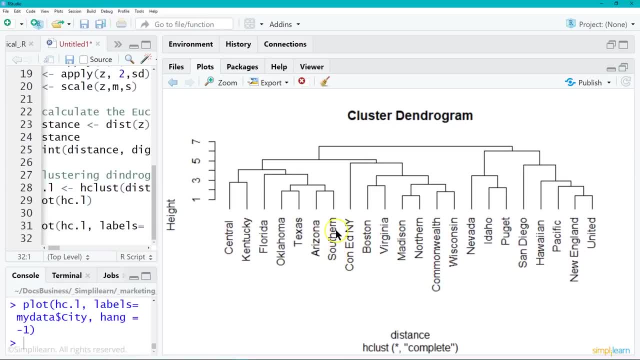 Florida, Oklahoma, Texas, Arizona and Southern US. These regions for some reason share a lot of similarities, And so we want to start asking what those similarities are. But this gives us a place to look. It says, hey, these things really go together. 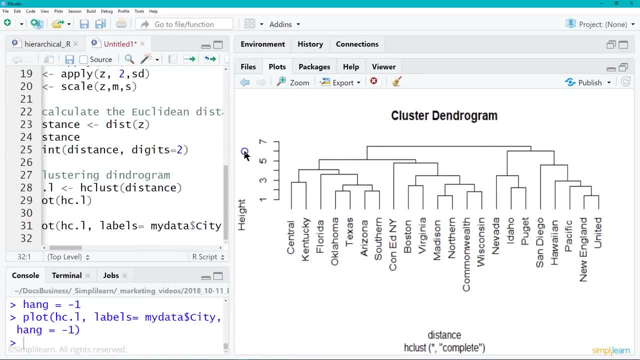 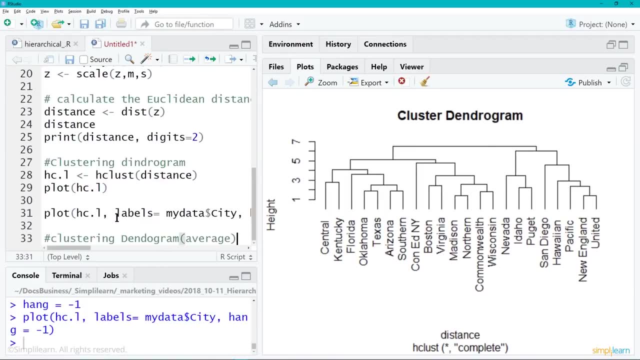 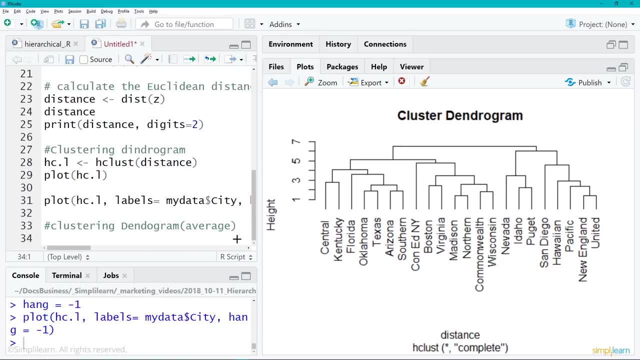 You should be grouping these together as far as your cells and what you're doing, And then one of the things you might want to do is there's also we can do the dendrogram average. This changes how we do the clustering, So it looks very similar like we had before. 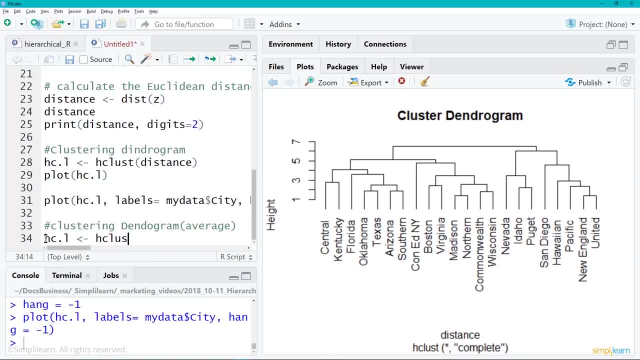 Those are HCL. We're going to assign it, We're going to do an H cluster. We're still doing it on distance distance And this time we're going to set the method to average so we can change the methodology in which it computes the values. 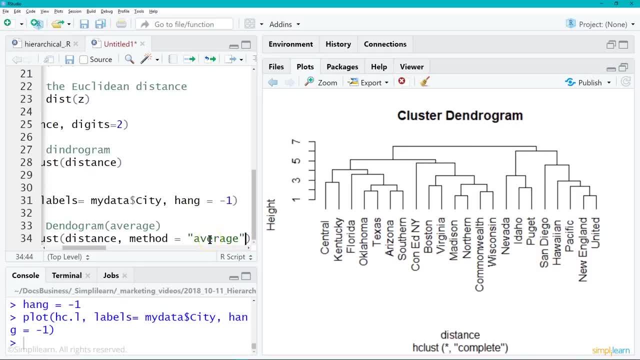 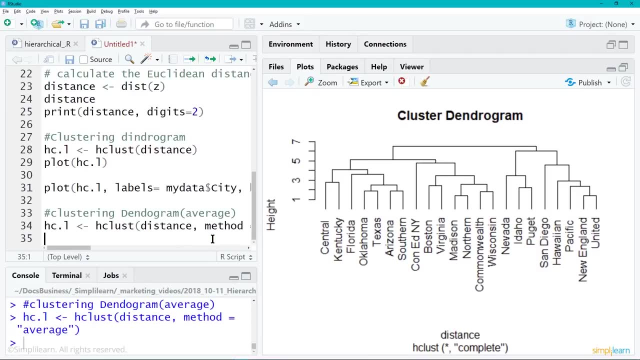 And before, if you remember correctly, we did median. Median is a little bit different than means. We did the most common one. and then we want the average of the median And let's go ahead and run that, And then we can plot. 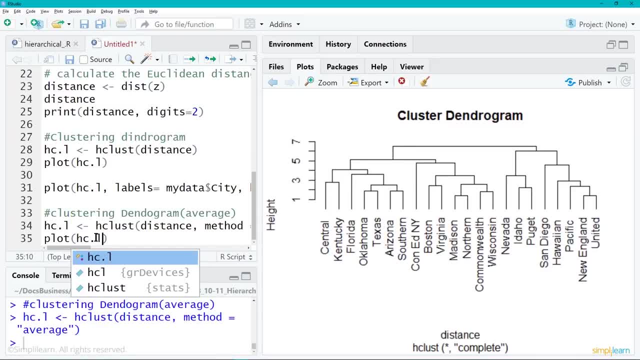 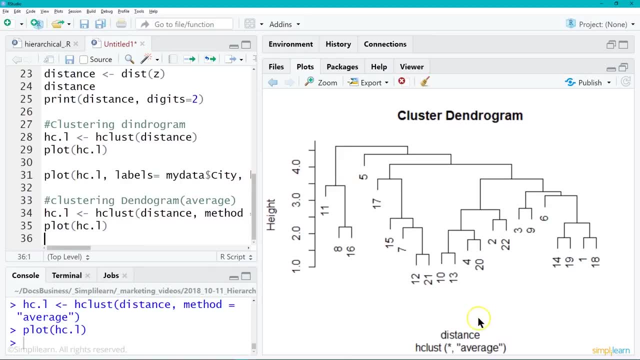 And here's our HCL. There we go, Here's our HCL And I can run that plot And you can see this changed a little bit. So our way it computes and groups things looks a little bit different. It's a little different than it did before. 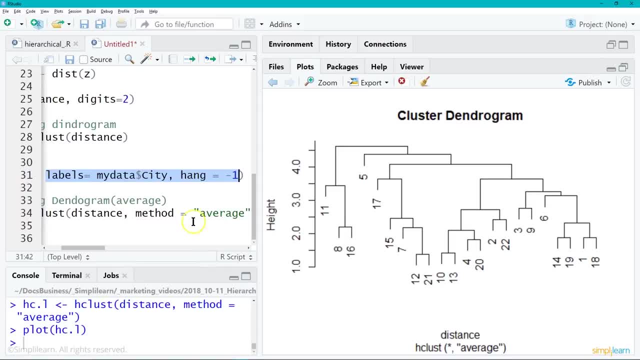 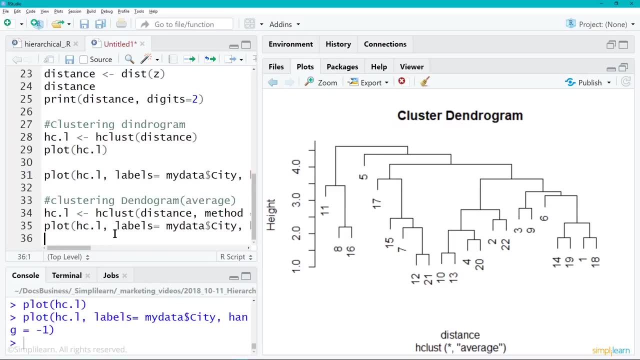 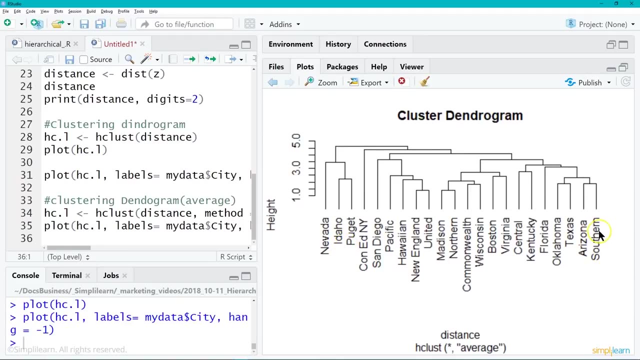 And let's go and put the cities back in there and do the hang Control copy. Let me just really quickly copy that down here Because we want the same labels. And again you can see Nevada, Idaho, Puget. I remember we were looking at southern US. 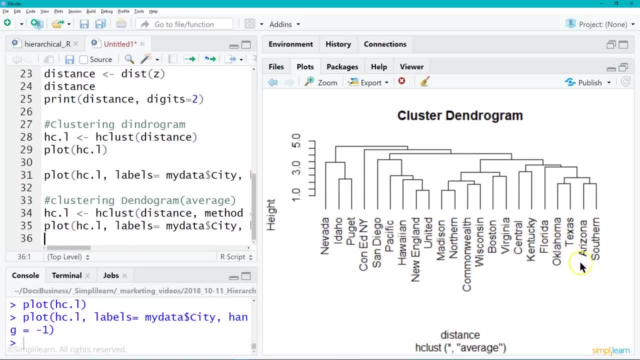 and Arizona, Texas and Oklahoma, Florida, So the grouping really hasn't changed too much. So we still have a very similar grouping. It's almost kind of flipped, But we're going to keep it as far as the distance based on average has. 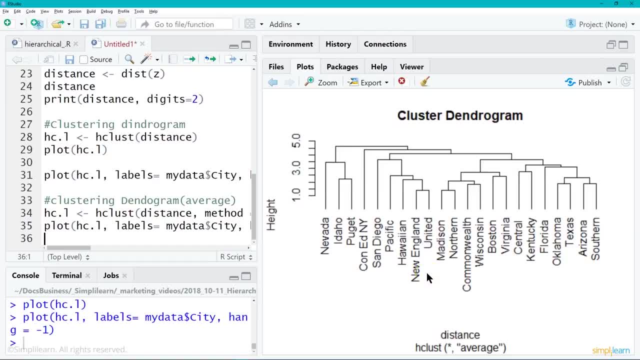 But this is something you could actually take to the shareholders and say, hey look, these things are connected, And at which point you want to explore a little deeper as to why they're connected, because they're going to ask you: OK, how are they connected and why do we care? 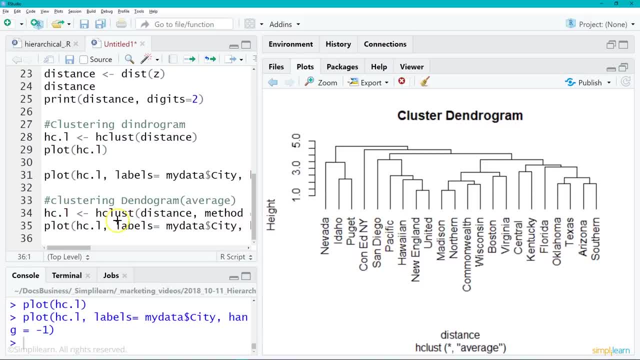 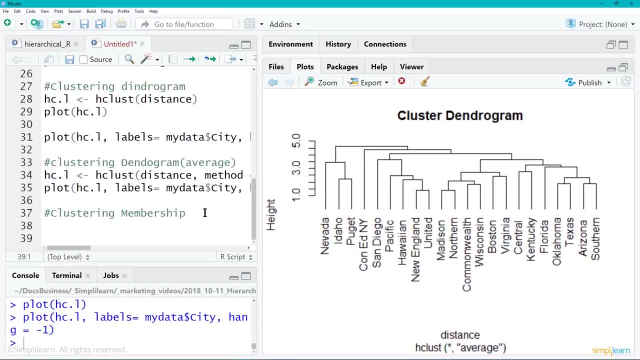 But that's a little bit beyond the actual scope of what we're working on today. But we are going to cover membership- What's called clustering membership- on there And let's create a member. we'll just call it member one. Oops, there, member one. 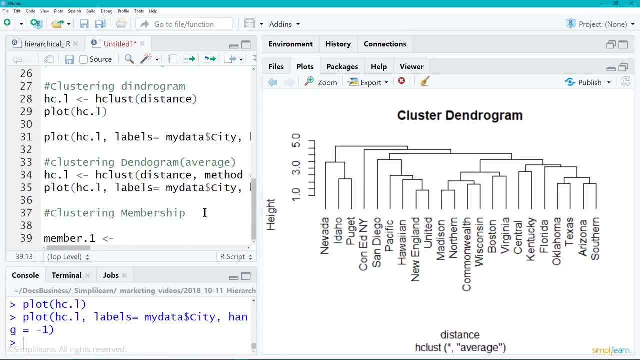 And we're going to assign to this. We're going to do cut tree and cut tree, It limits it. So what that means is I take my hc dot L in here. Oops, there we go, dot L, And so I'm taking the cluster I just built. 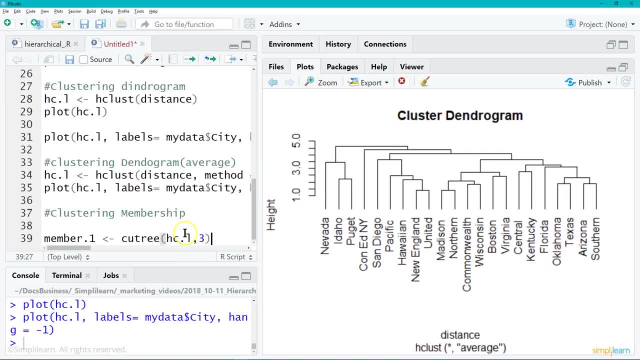 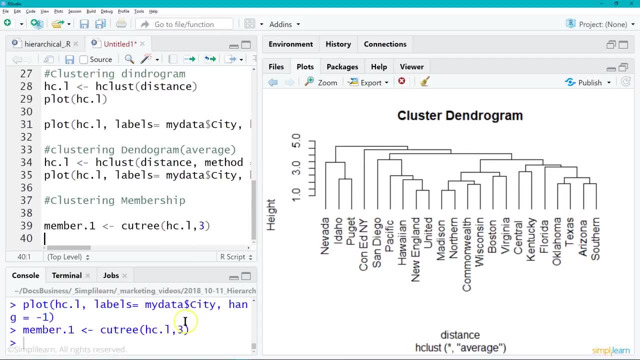 And we want to take that cluster and we want to limit it to just a depth of three. So we go ahead and do that and run that one. Oops, we go, run There we go. So now I've created my member one. 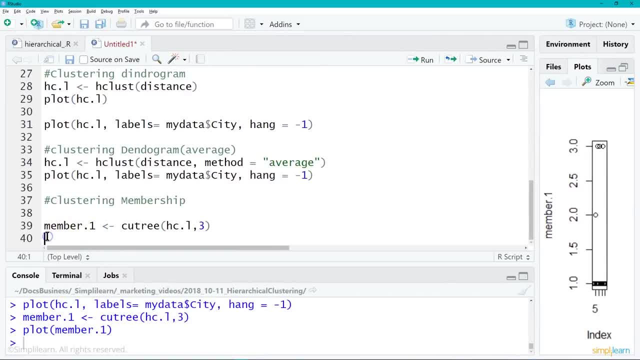 And then- whoops, let me just move this out of the way- We're going to do an aggregate and we're going to use Z from above And we're going to turn member one into a list And then we're going to aggregate that together, based on the mean. 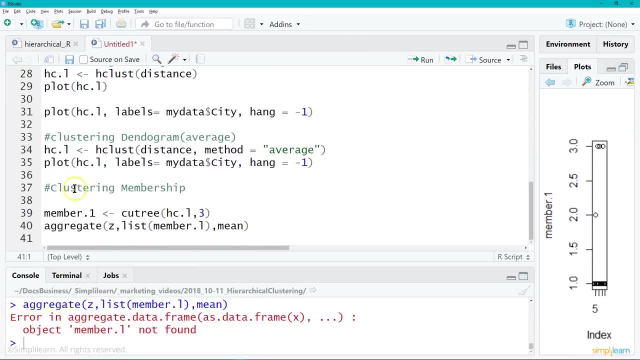 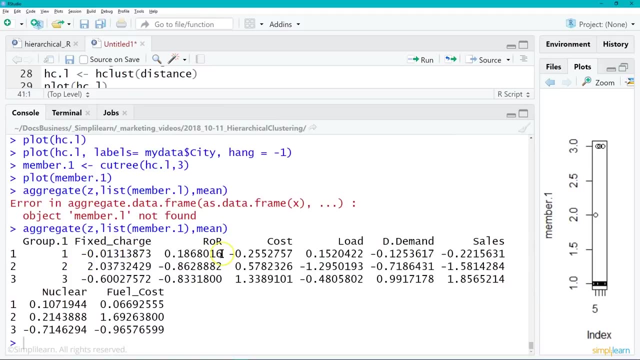 Let me go ahead and enter, And we're going to run that, So I did. member L- it's actually member one. There we go, And if we take a look at this, we now have our group, one fixed charge and then all your different columns listed there. 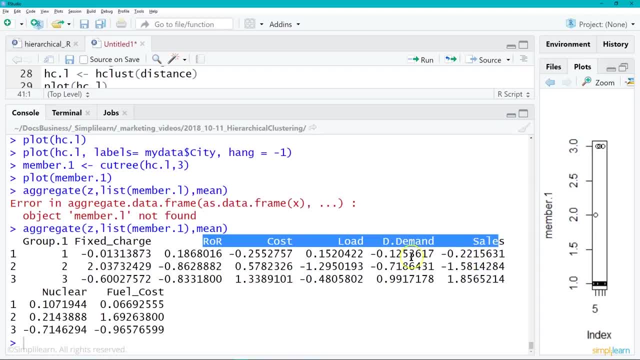 And most of them should come up kind of looking between zero and one. But you'll see a lot of variation because we're varying it based on the means. So it's a means, a standard deviation, not just forcing it in between zero and one. 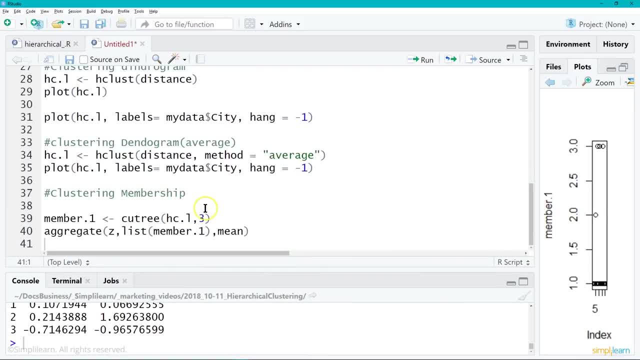 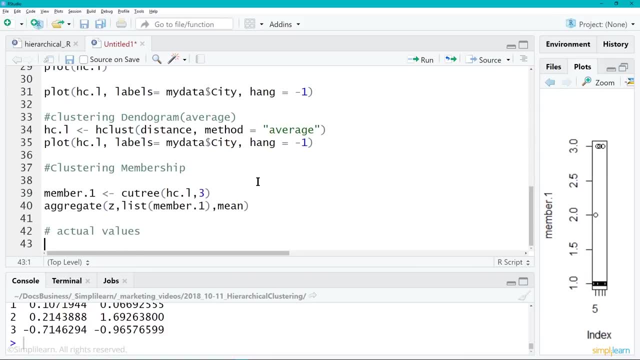 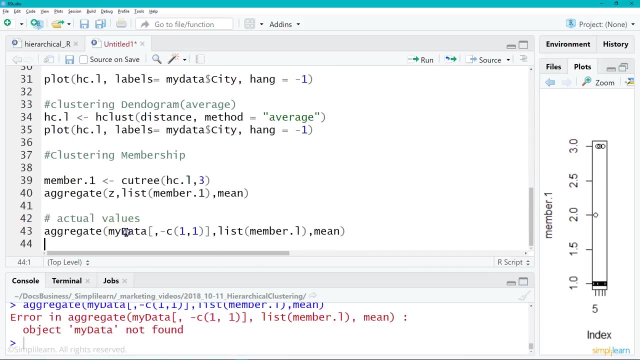 Which is a much better way usually to normalize your data than just doing the zero one set up. And finally, we can actually look at the actual values And the same chart we just did. Oops, I made a mistake on there with my data. 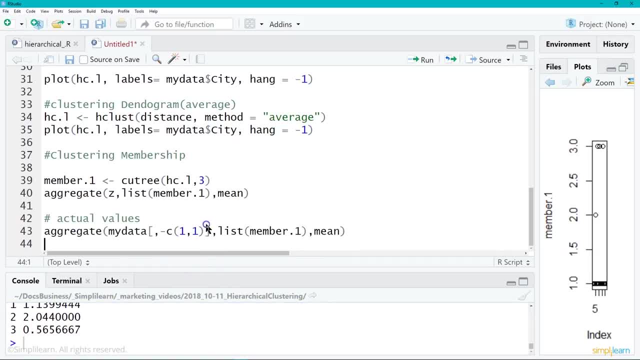 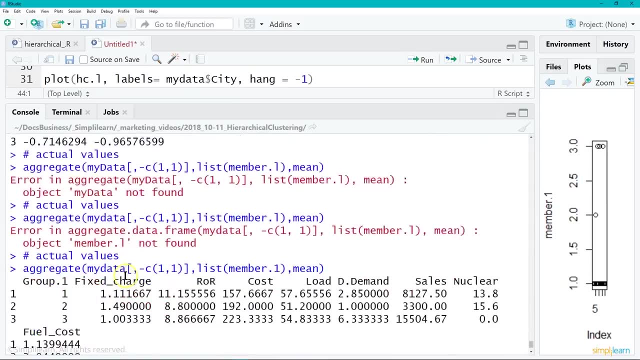 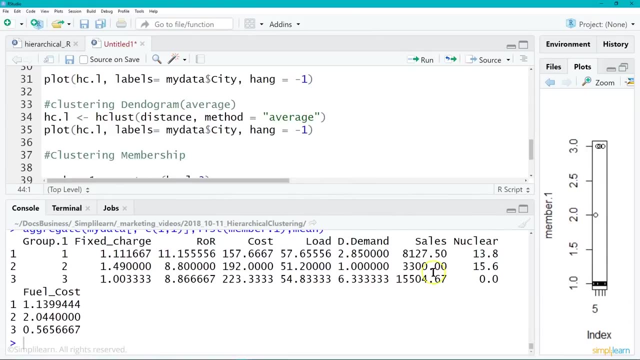 There we go, OK, And again we now have our actual data, instead of looking at just the. if you looked up here, it's all between zero and one, And when we look down here we now have some actual connections and how far distance this different data is. 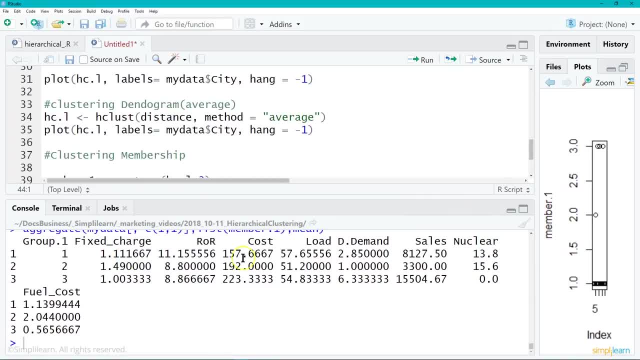 Again, because more of a domain issue and understanding the oil company and what these different values means, And you can look at these as being the distances between different items. So a little bit different view and you have to really dig deep into this data. 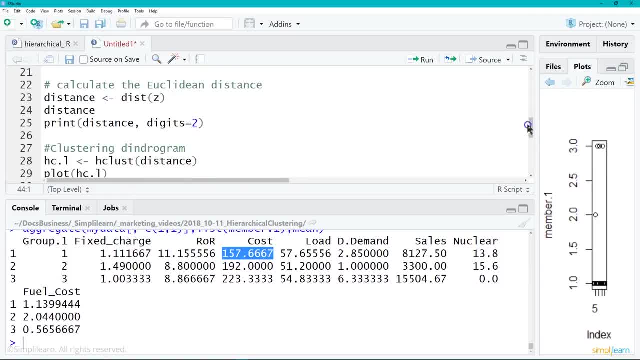 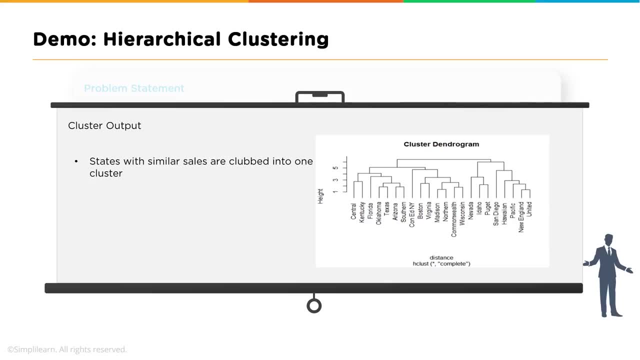 What we really want you to take away from this is the dendogram and the charts that we did earlier, And that is the cluster output and our nice dendogram. So this would be stage one in data analysis of the cells. Again, you'd have to have a lot more domain experience to find out what all 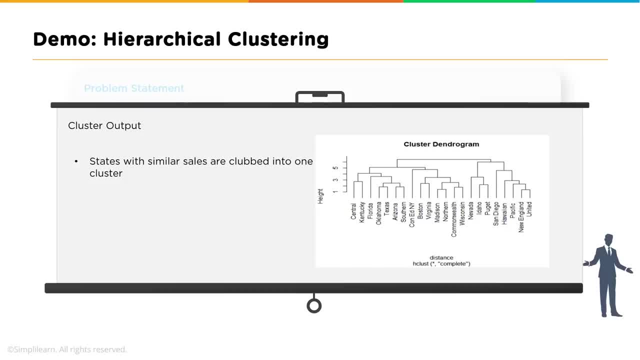 the individual numbers we looked at mean and what the distance is and what's difference between Central America and Kentucky and why they're similar and why they're similar. And then you'd have to go back and look at all of the data that groups, all of Central Kentucky, Florida, Oklahoma, Texas, Arizona. 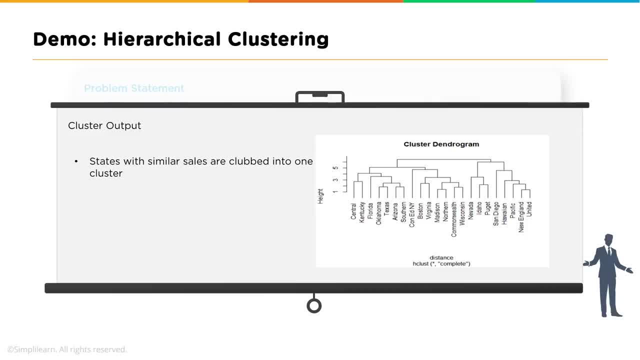 and Southern US together into one larger group. So I'd be way beyond the scope of this, But you can see how we start to explore data and we start to see things in here where things are grouped together in ways we might not have seen before. 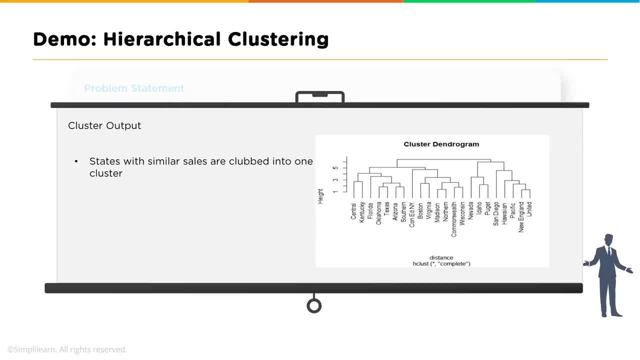 And this is a good start for understanding and giving advice for sales and marketing. maybe logistics, city development, There's all kinds of things that kind of need to explore data And we just want to point out that we get three clusters of regions with the highest 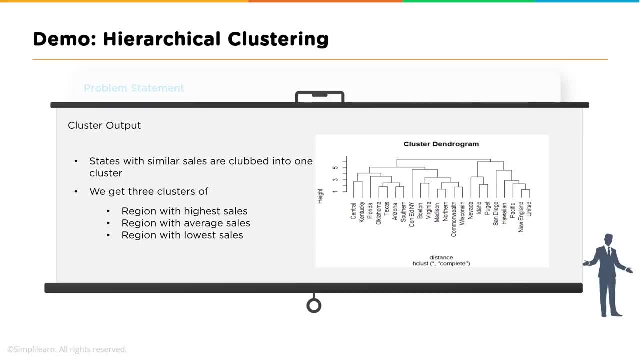 cells. region with average cells. region with the lowest cells. Again, those are some of the things that they clustered it around and you could actually see where things are going on or lacking. You know, in this case, if you're the lowest cells. 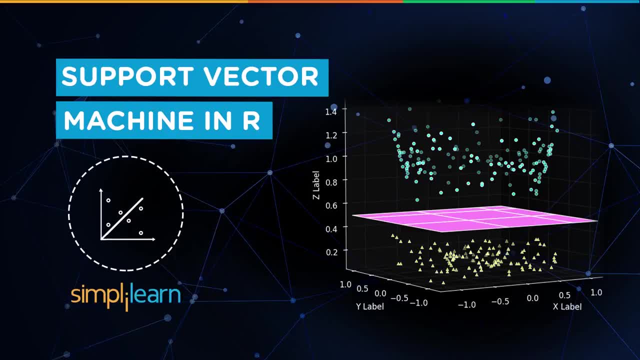 no one wants to be in the region of the lowest cells Support Vector. Machine is a binary classifier, a supervised machine learning algorithm, And in this video we will learn what all that means. Machine learning algorithms come in three major flavors: supervised learning algorithms, unsupervised learning. 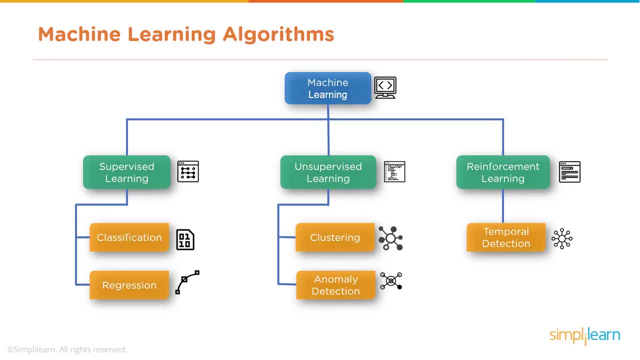 algorithms and reinforcement learning, And today we'll cover classification under supervised learning. Supervised meaning the data set has known outcomes. If it were unsupervised, it would not have known outcomes and we wouldn't have the categories or classes necessary for the machine to learn. 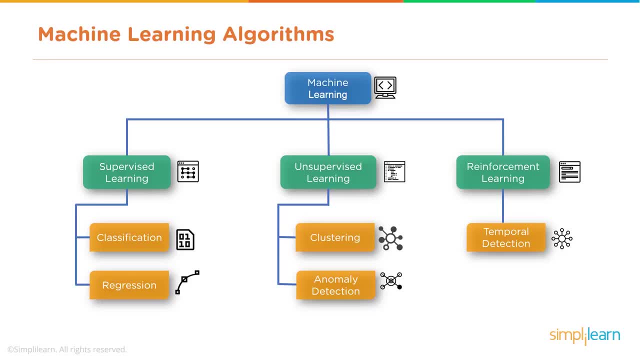 But under supervised learning we do have the known outcomes in the data set. And under supervised learning there are two major types of machine learning algorithms: classification, which we'll cover today, Support Vector Machine and regression Classification: you predict categories and in regression you generally predict values. 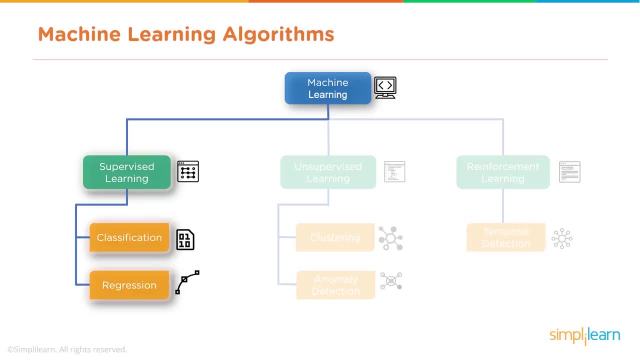 So, while we look at supervised learning, keep in mind that classification can really be considered multidimensional, in the sense that sometimes you only have two classes- yes or no, true or false- and sometimes you have more than two classes. Sometimes you have, say, under risk management or risk modeling, low risk. 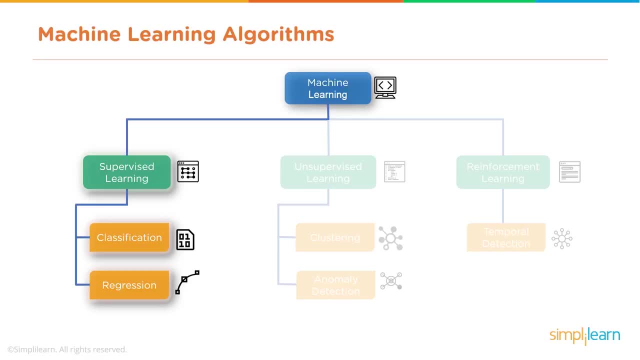 medium risk or high risk, and SVM is a binary classifier. It is a classifier used for those true, false, yes, no types of classification problems, and in supervised learning, features are important. If there are a lot of features, SVM may be the better classification algorithm choice, as. 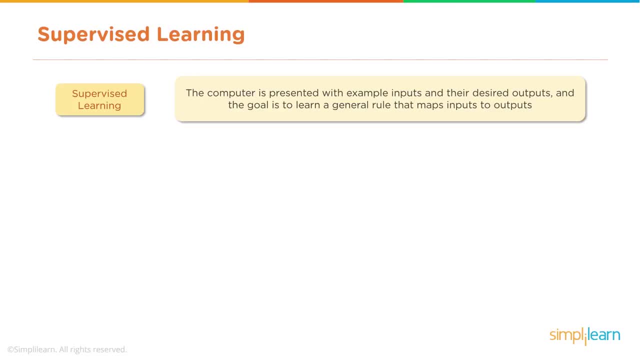 opposed to say logistic regression. So, with supervised learning, the computer is presented with example inputs and their desired outputs, those known outcomes, And the goal is to learn a general rule that maps inputs to those outputs, For example, bug detection or customer churn or stock price prediction. 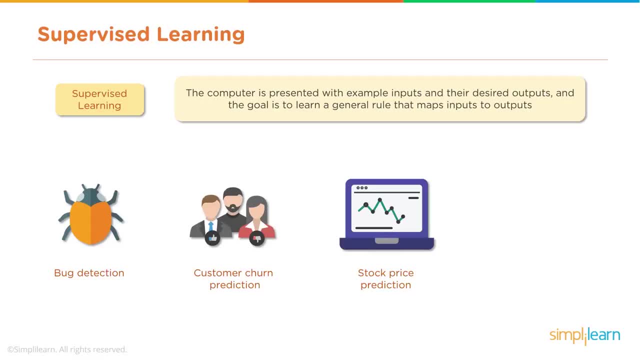 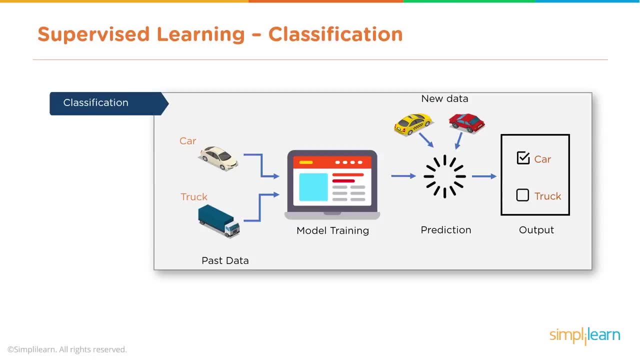 not the value of the stock price, but whether or not it will rise or fall. And weather prediction: sunny, not sunny, rain, no rain. The classification algorithms generally take past data, data that we have. those known outcomes train the model. 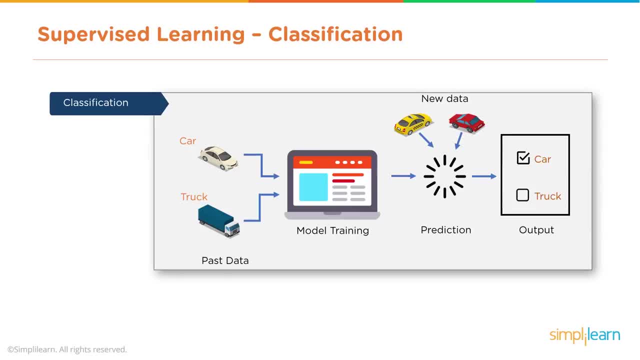 take new data once the model is trained, ingest it into the model and create predictions. Is it a truck or is it a car? And keep in mind that I said, features are important and the number of features, whether or not those features are applicable to your problem, is a whole different discussion. 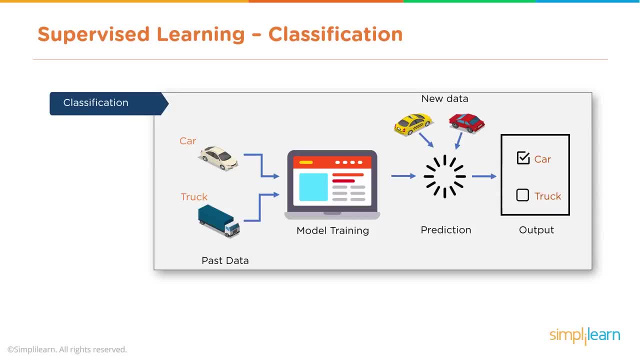 But in some sense you know, probably intuitively, that the color of a car really isn't indicative of whether or not it's a car or a truck, but the length of the vehicle or the number of axles or the weight or the amount of seating may be more applicable. 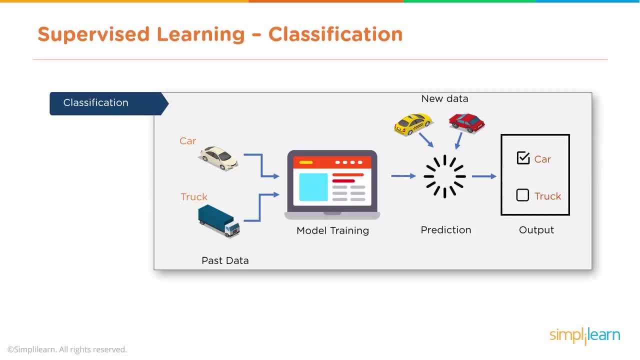 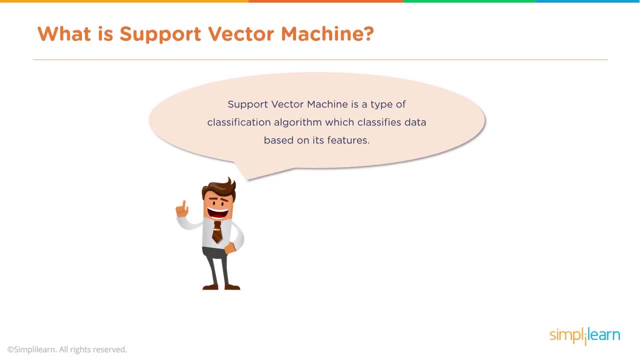 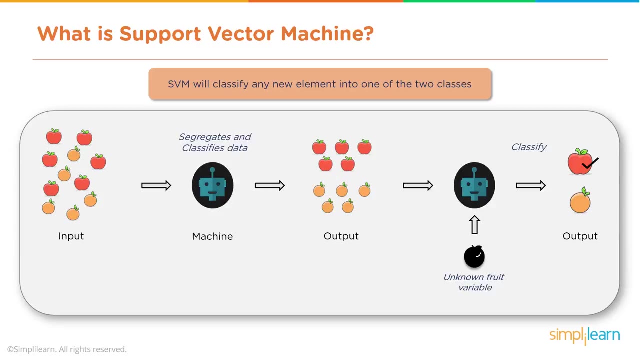 to the algorithm and to training of the model. So what is support vector machine? Support vector machine, or SVM, is a type of classification algorithm which classifies data based on its features, And SVM will classify any new element into one of those two classes. 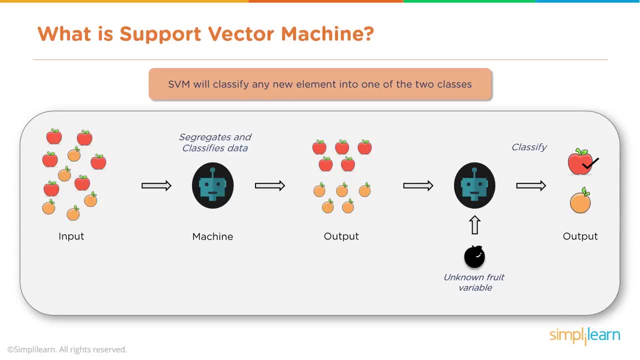 So we'll give it some inputs. The algorithm will segregate and classify the data and then create the outputs. And next, when we ingest new data- an unknown fruit variable in this example- the algorithm will correctly classify the fruit Apple versus Orange. 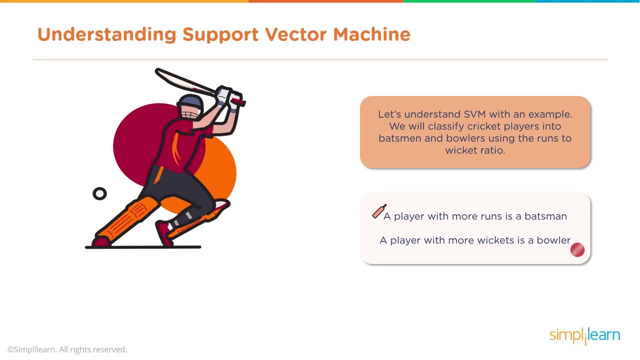 So now let's understand what an SVM is. If you want to understand support vector machine, you really need a good example, And I know that cricket is a wonderful game. I don't know a lot about it, but I know it's very popular around the world. 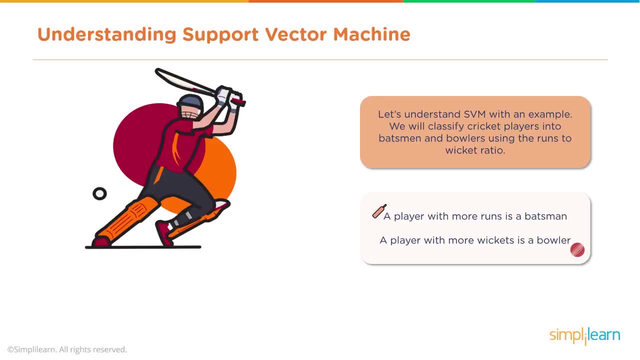 And we're going to use cricket as an example of SVM. So we'll classify cricket players into batsmen or bowlers using the runs to wicket ratio. So a player with more runs would be considered a batsman and a player with more wickets would be considered a bowler. 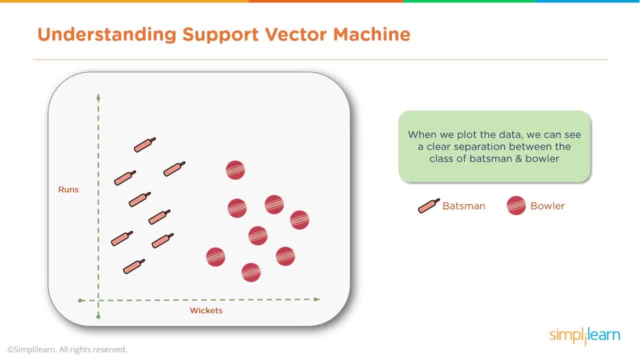 And if we could take a data set, say, of people, cricket players, with runs and wickets in columns next to their names, we could create a plot, a two dimensional plot In this example, clear separation between cricket players considered bowlers and those cricket. 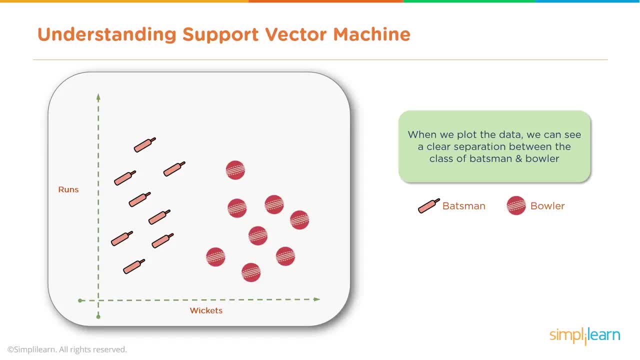 players considered batsmen And you don't always have a data set this clean where there is a clear segregation of data: bowlers versus batsmen. But for the sake of understanding SVM, this example does well. So before we do any separation, before we apply any high level mathematics, 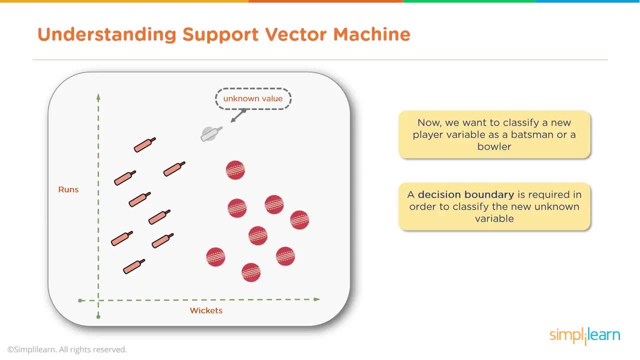 let's just take a look at an unknown value, a new data coming into our data set And that datum- we don't know what class it belongs to. That datum is a bowler or a batsman. We know that much, but we don't know. 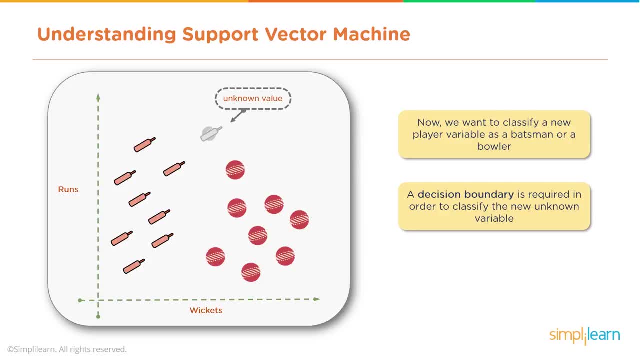 Should we consider that cricket player a batsman or a bowler? And so we want to draw a decision boundary, some type of line separating the two classes, so that we can use that decision boundary to classify the new data point. Of course we could draw lines. 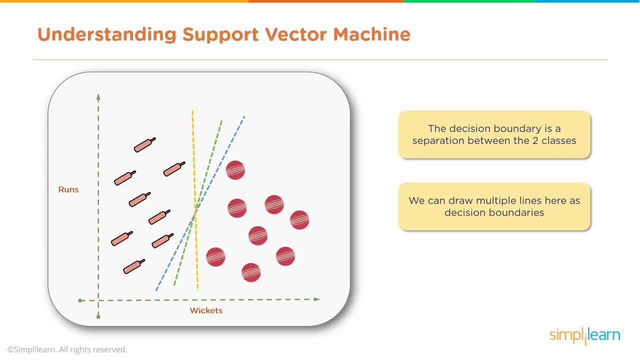 There's a yellow line, a green line, a blue line. There's actually not just three lines, but an infinite number of lines that we could draw between those two classes. So which one do we pick? And this is kind of reminiscent of simple. 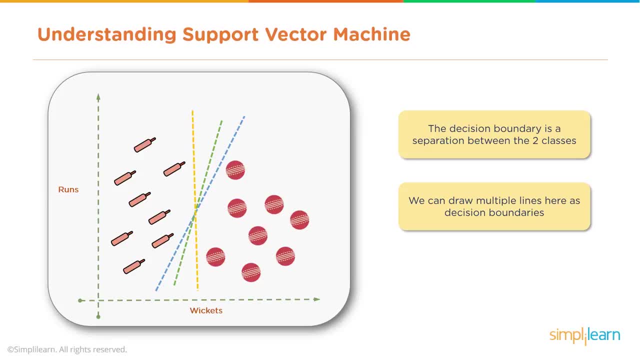 linear regression where we find the line of best fit. We want the line of best separation. We want a line that clearly separates those two groups as much as possible. Once we have the correct line, we would be able to classify the new data point. 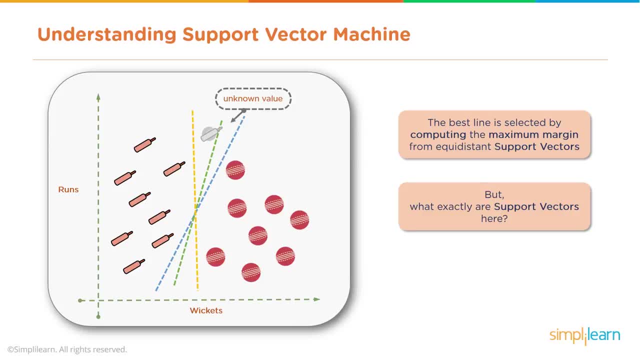 But in this example you can see: if we pick yellow, the new data point would be a bowler. If we picked green or blue, the new data point would be a batsman. So we need the one that best separates the data. 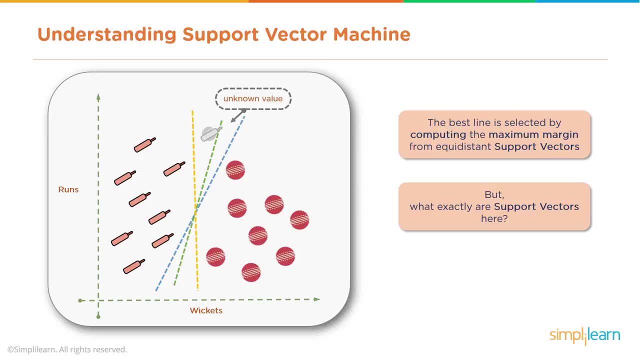 What line best separates the data. We'll find the best line by computing the maximum margin from equidistant support vectors. Now, support vectors in this context simply means the two points, one from each class- that are closest together but that maximize the distance between them, or the margin. 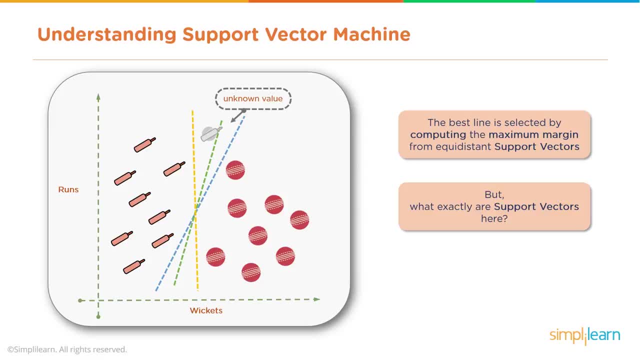 So the word vector here you may think, well, he really means points, data points. Well, in two dimensional space, yes, and maybe even in three dimensional space. But once you get into higher dimensional spaces, when you get more and more features in your data set, 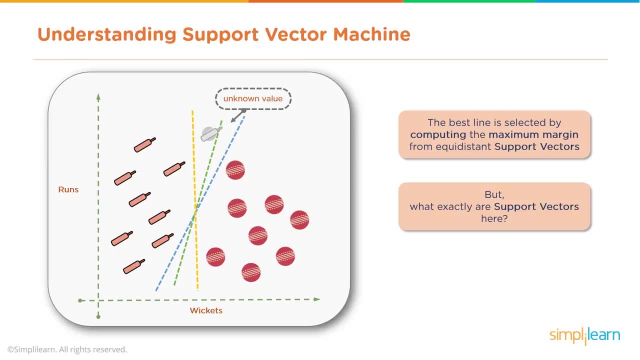 you have to consider these as vectors. You can no longer really describe them as points, So we call them vectors, And the reason they're support vectors is because the two vectors that are closest together, that maximize the distance between the two groups, support the algorithm. 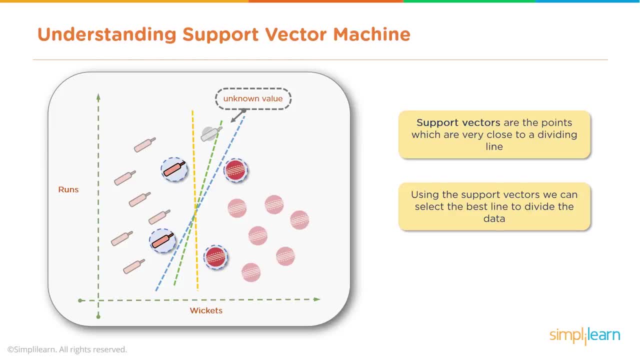 So that's why we call them support vectors. So if you look at our example, there are a couple of points at the top that are pretty close to one another and a couple of points at the bottom of that graph that are pretty close to each other. 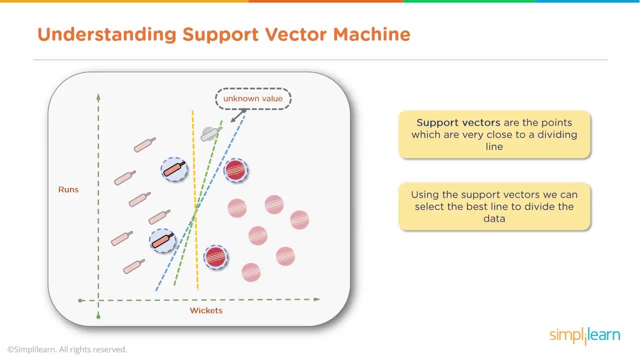 And we're not really sure, looking at the graph, which two are closest. But clearly those points are the ones we need to consider. The rest of the other points are too far away from the rest of the other points. In other words, the bowler points are far. 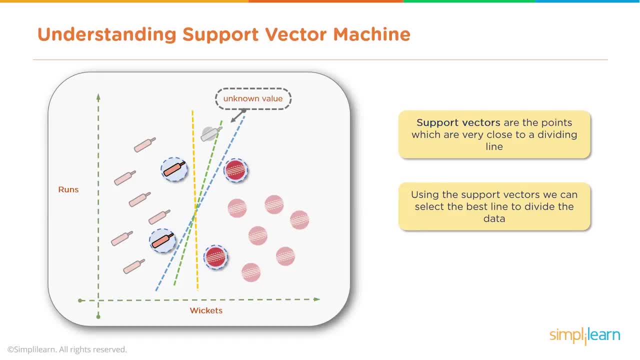 to the right and the batsman data points are far to the left. So we'll look at these four points to begin with. Mathematically, we would calculate the distance among all of these points and we would minimize that distance Once we pick the support vectors. we'll draw a dividing line and then measure. 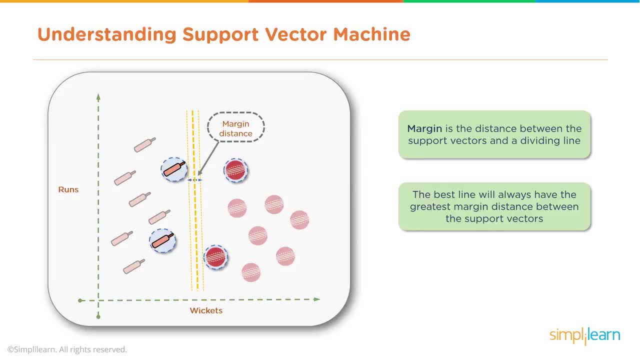 the distance from each support vector to the line. The best line will always have the greatest margin Distance between the support vectors. If we consider the yellow line as a decision boundary, the player with the new data point would be considered a bowler. 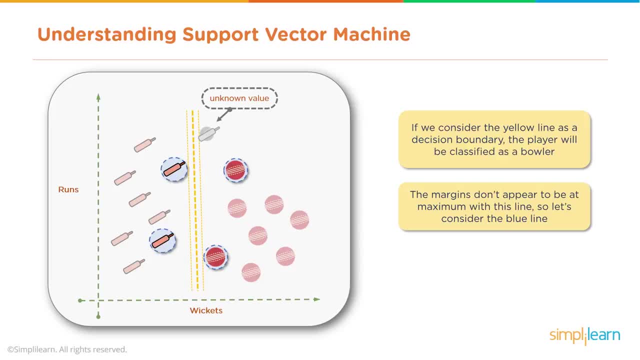 The margins don't appear to be maximum, though, So maybe we can come up with a better line. So let's take two other support vectors and we'll draw the decision boundary between those, and then we will calculate the margin And notice now that the unknown data point 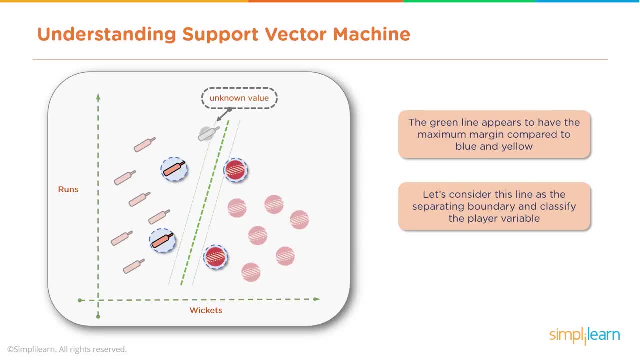 the new value would be considered a batsman. We would continue doing this- And obviously a computer does it much quicker than a human being- over and, over and over again, until we found the correct decision boundary with the greatest margin, And in this case, if you look at the green decision boundary, 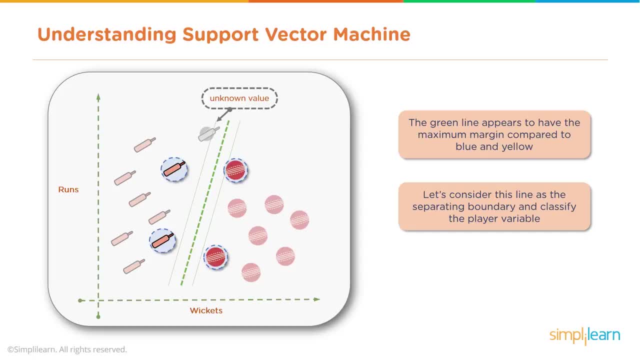 the green line appears to have the maximum margin compared to the other two, And so let's consider this the boundary of greatest margin. and now classifier unknown data value. and now, clearly, it belongs in the batsman's class. The green line divides the data. 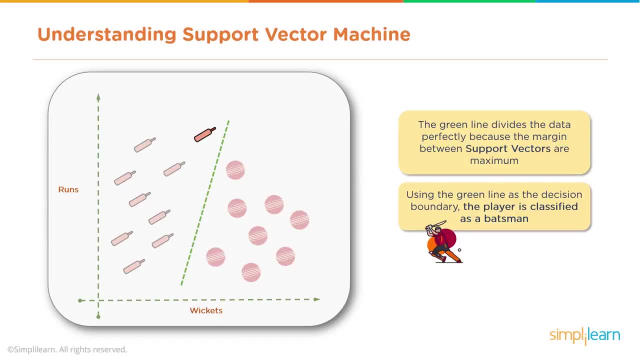 because it has the greatest margin, or the maximum margin between the support vectors, and now we can have confidence in our classification that the new data point is indeed a batsman. Technically this dividing line is called a hyperplane, And the reason it's called a hyperplane will become a little bit more evident. 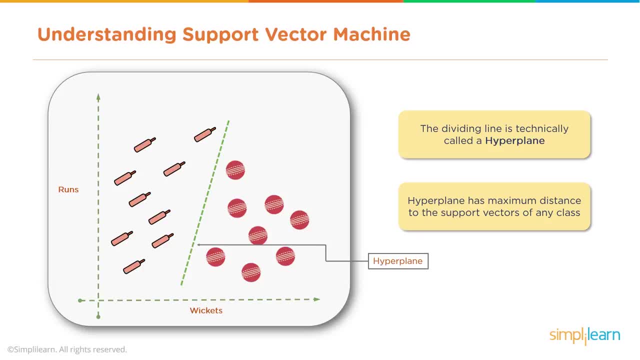 in a few minutes. Generally in two dimensional space we consider those lines, But in three dimensional space and higher dimensional spaces they're considered planes or hyperplanes, So we always tend to refer to them as hyperplanes, and the hyperplane that has 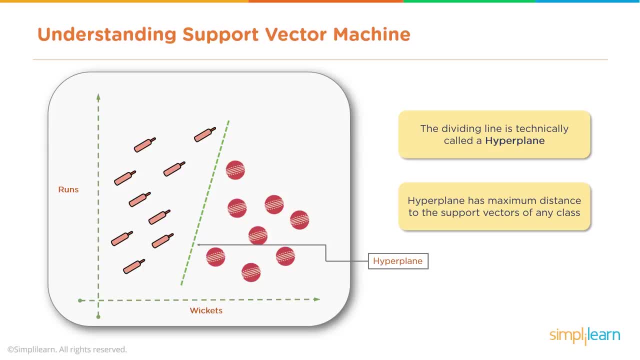 the maximum distance from the support vectors is the one we want, So, sometimes called the positive hyperplane, D plus is the shortest distance to the closest positive point and D minus, sometimes called the negative hyperplane, is the closest shortest distance to the closest negative point. 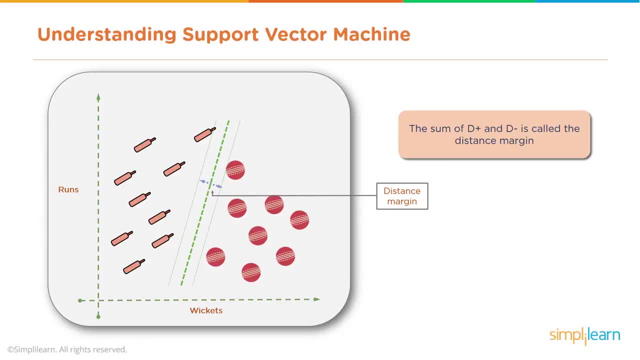 And the sum of D positive and D negative is called the distance margin. So if you calculate those two distances and add them up, that's the distance margin And we always want to maximize that. If we don't maximize it we can have a misclassification. 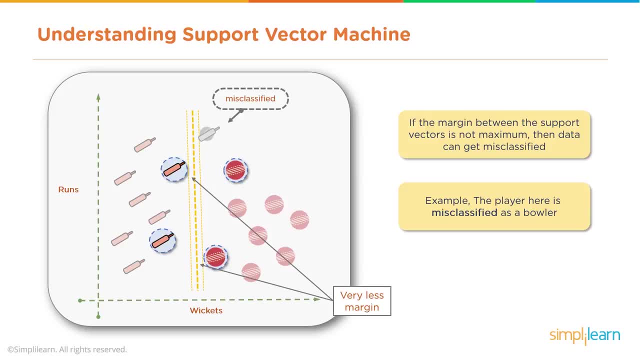 And you can see the yellow margin is much smaller than the green margin. So this problem set is two dimensional, because the classification is only between two classes, And so we would call this a linear SVM. Now we're going to take a look at kernel SVM. 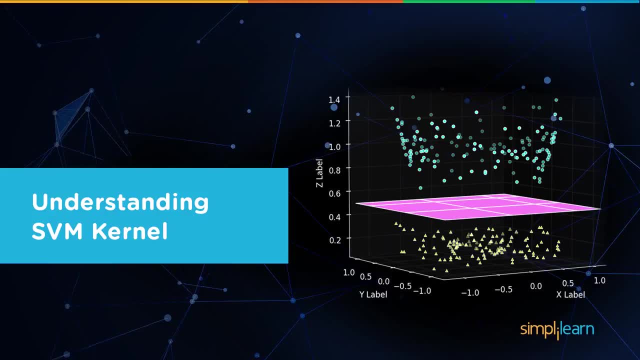 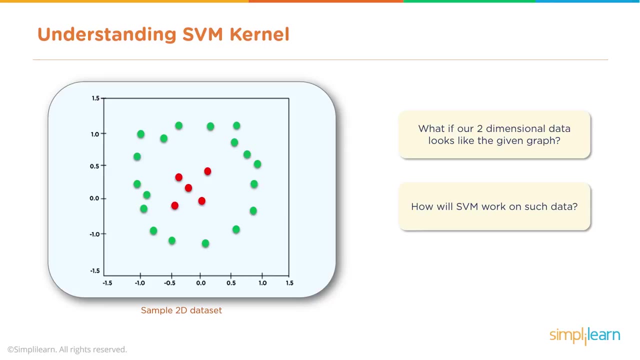 And if you notice in this picture, this is a great depiction of a plane, not a line. This is three dimensional space, so that's the plane that separates those two classes. So what if our two dimensional data looks like this? What if there's no clear linear separation between the two classes and machine learning parlance? 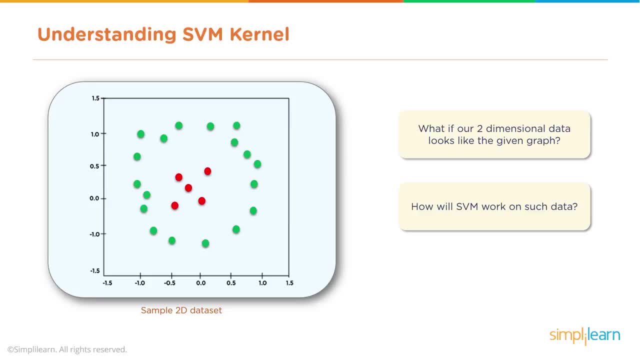 We would say that these are not linearly separable. How could we get support vector machine to work on data that looks like this, Since we can't separate it into two classes using a line? what we're going to do, and clearly there's no line. 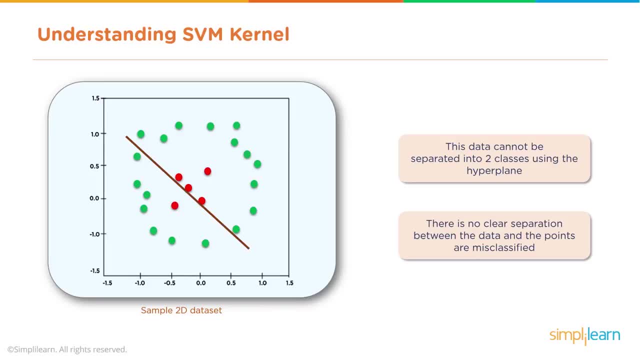 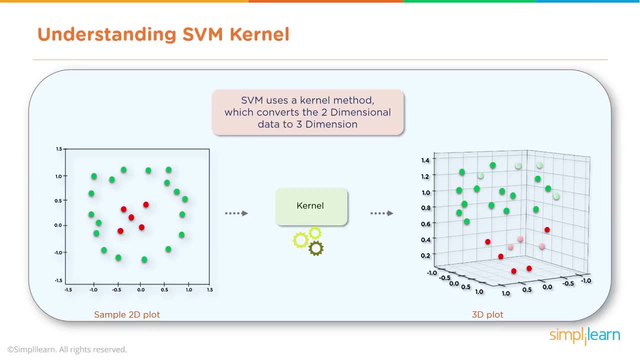 I mean convince yourself. there's no line that goes and separates those two classes. So what we would do is we would apply some type of transformation to a higher dimension. We would apply a function called a kernel function to the data set, such that the data set would be: 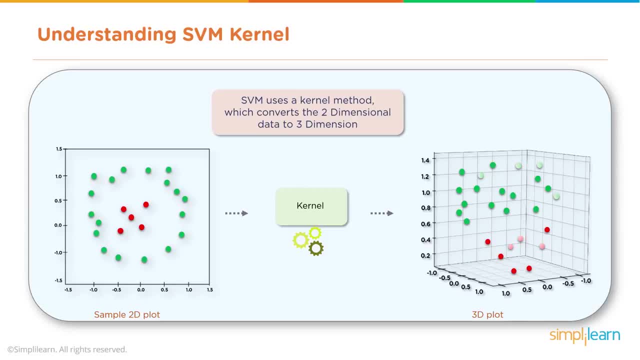 transformed into a higher dimension, a dimension high enough where we could clearly separate the two groups, the two classes, in this case with a plane. much the same way. you saw the picture a few slides ago, where the plane was separating the two classes. 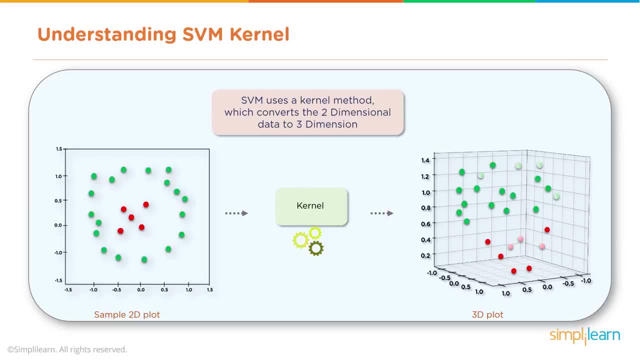 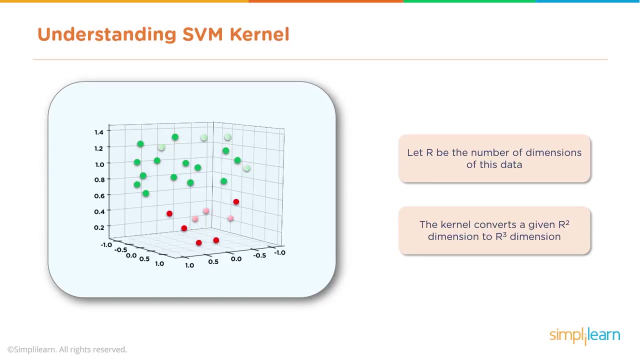 Here we clearly could draw some planes between the green dots and the red dots And of course we could draw an infinite number of planes separating those two classes, but we would draw the one that would maximize the margin. So if we let R be the number of dimensions, then the kernel function would convert a given 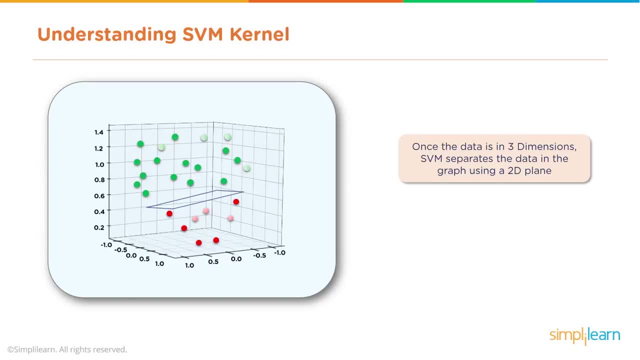 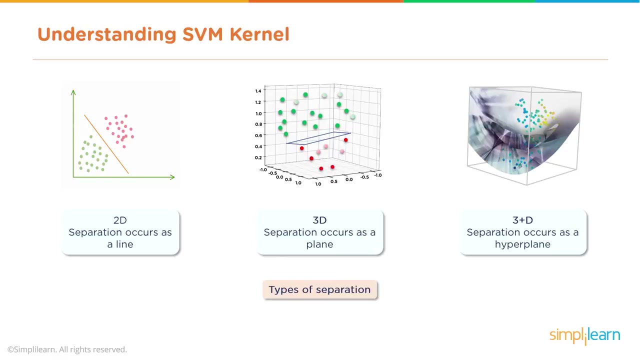 two dimensional space to a three dimensional space And, as I said, once the data is separated in three dimensions, we can apply SVM and separate the two groups using a two dimensional plane, And this is analogous in the higher dimensions. And that last picture on the right hand side would be some type. 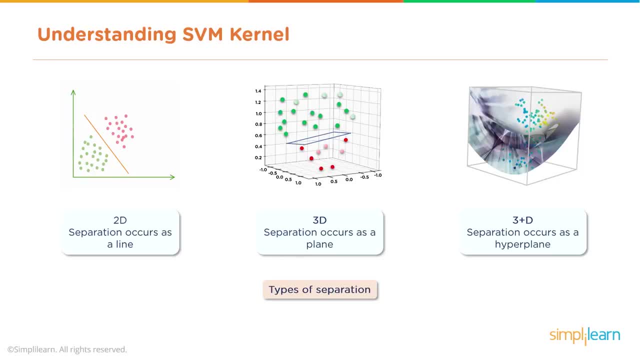 of depiction of a higher dimension hyperplane, And there are more than one type of kernel function. There's Gaussian, RBF kernel, sigmoid kernel, polynomial kernel, depending on the dimension and how you want to transform the data. There are more than one choice for kernel functions. 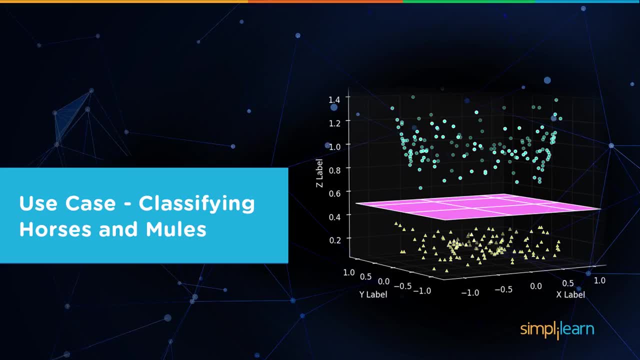 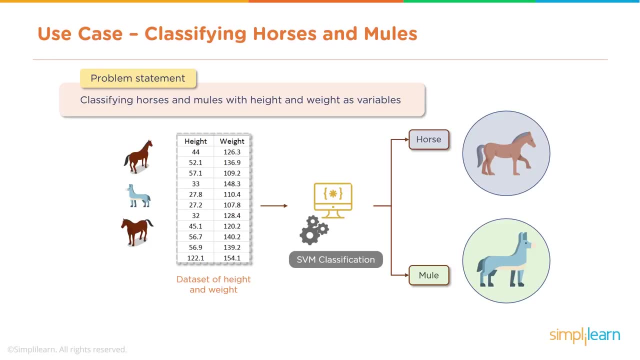 So now let's go through a use case. Let's take a look at horses and mules and see if we can use SVM to classify some new data. So the problem statement is classifying horses and mules And we're going to use height and weight as the two features. 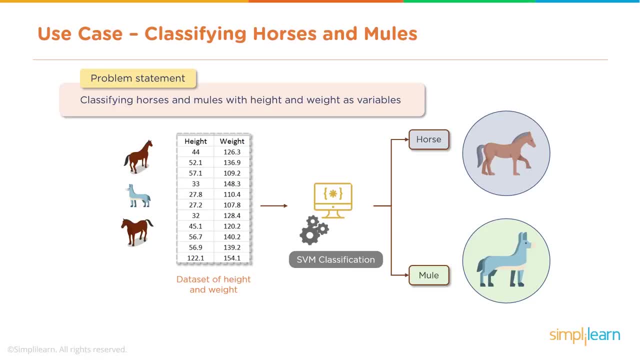 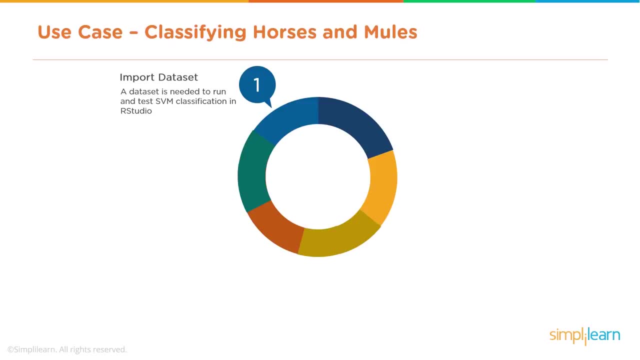 And obviously horses and mules typically in general tend to weigh differently and tend to stand taller. So we'll take a data set, we'll import the data set, We'll make sure we have our libraries- the E1071 library as support vector machine algorithms built in. 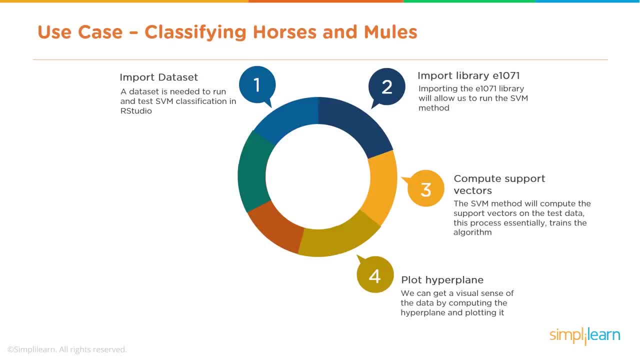 We'll compute the support vectors using the library. Once the data is used to train the algorithm, we'll plot the hyperplane, get a visual sense of how the data is separated, And if it's two dimensional or three dimensional, that's great. 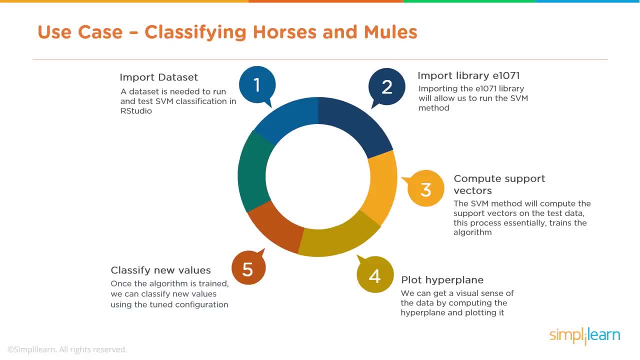 Remember, if it's higher dimensional, it's tough to plot those, And then we'll use the new model, the trained model, to classify new values In general, we would have a training set, a test set And then ingest the new data. 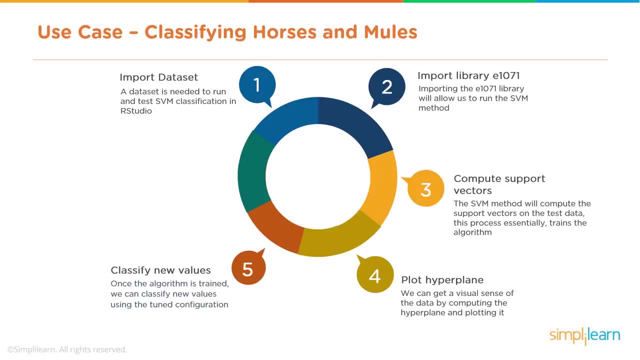 But for our example, we're just going to use the whole data set to train the algorithm and then see how it performs. And once we see how it performs, we'll see: did we get a horse? Did we predict a horse when we had a horse? 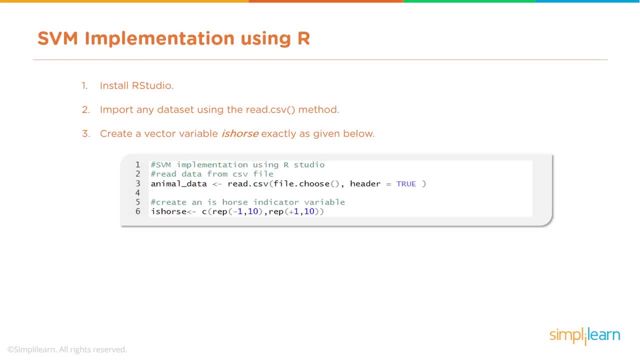 Did we predict a mule when we had a mule? So here's the R code. Of course, if you want to run this R code, you'll have to install R and then RStudio, Then you'll have to ingest the data and then you'll have to create. 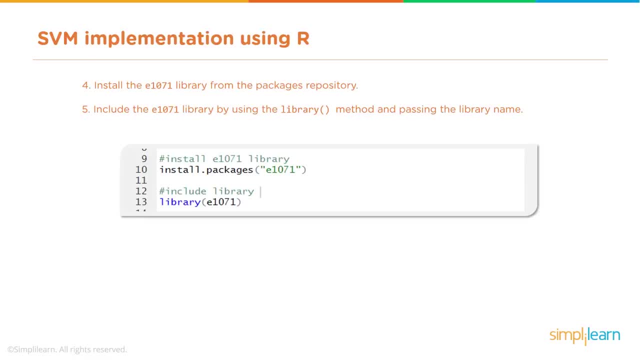 an indicator variable to help us with our plots. We'll install our libraries. I'll call the package- if you don't already have it installed- I do- And then call the library up into the R session that you're working. We'll create the data frame from the data that was ingested. 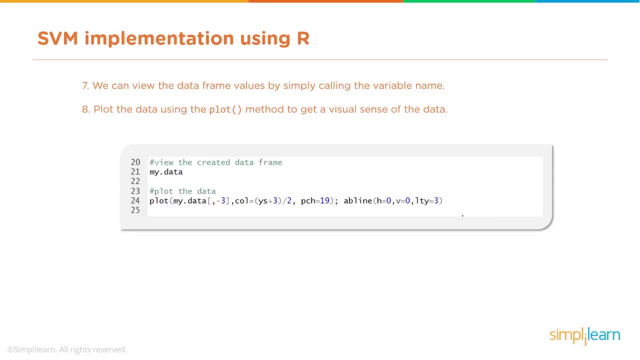 We will then view the data frame And, of course, we have to explore the data frame, hoping that we don't have missing values or we don't have outliers. If we do have missing values or outliers, we'll have to either impute those values or delete those values. 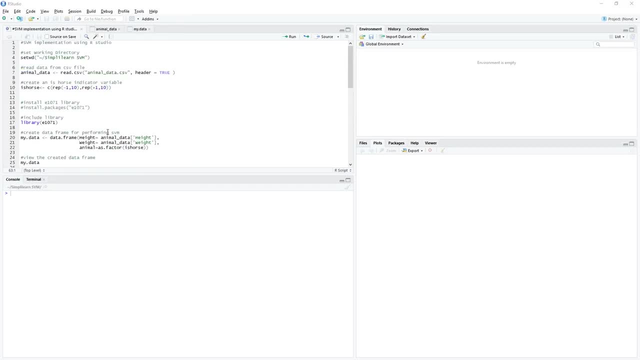 But in this case let's hope we don't have any. And now for a quick demo on support vector machines. so we have a working directory where my data is stored and I'm going to set the working directory to that data source and read the data file into R. 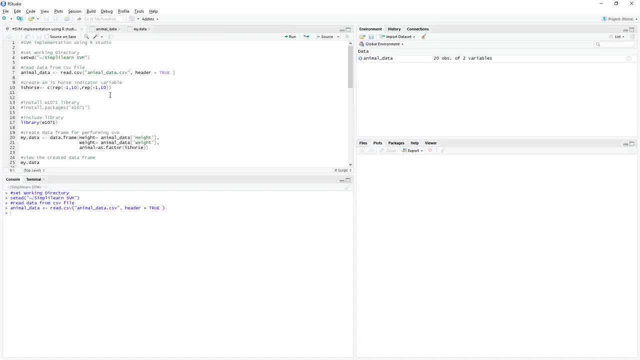 And now I'm going to create a vector that really is just an indicator variable. It's the negative ones and the ones that indicate whether it's a mule or a horse- Negative one for mule, positive one for a horse. So I'll create that vector and SVM. 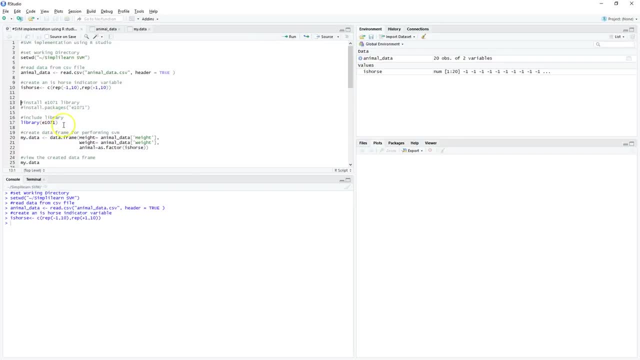 There's a great package- E1071.. Great library that has the support vector machine functions that we're going to use. And now I'm going to create the data frame. I'm going to take my data and I'm going to add to it the is horse vector. 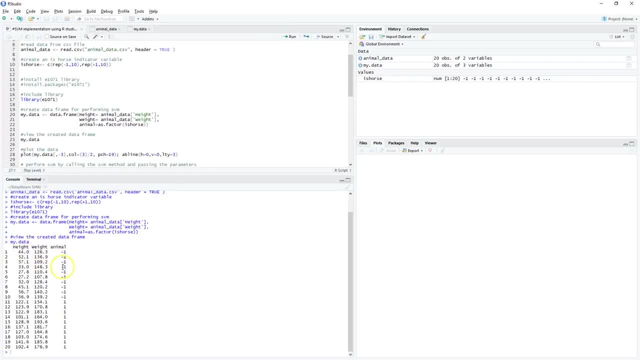 And now let's just take a peek and, as you can see, there's the height, weight and whether or not the animal was a mule or a horse. So remember machine learning: we take a data source with known outcomes and we apply our algorithm to that data source. 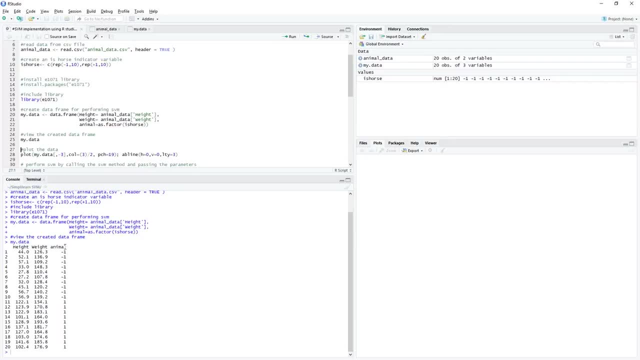 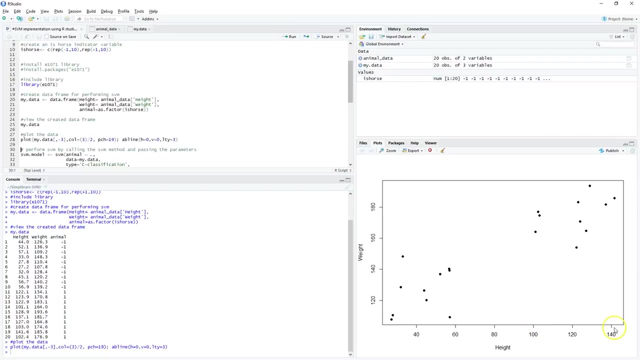 In this case a data frame of heights, weights and the indicator variable, And then we use the machine learning algorithm to learn from that data with those known results. So now let's plot the data, the height versus weight- And as you can see, the horses tend to be. 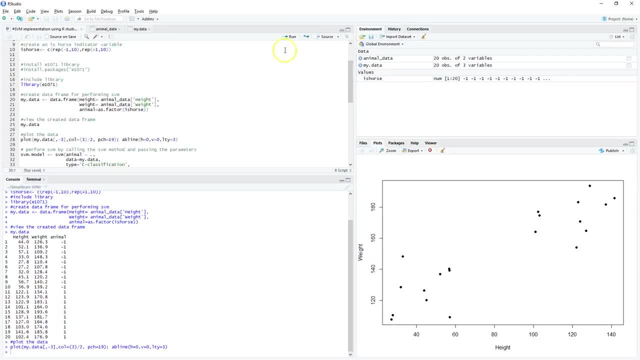 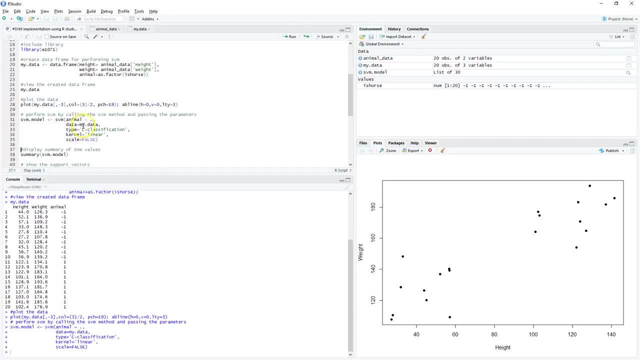 a lot taller and weigh a lot more than the mules. So now let's run our algorithm, our SVM model, against the data, And the key here is that it's a linear model and we've run it and great, Now we have a model. 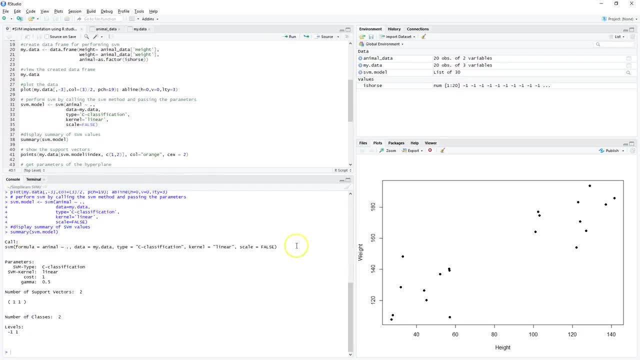 Let's look at the summary of the model And, as you can see, there's the formula that it ran and some of the information about the vectors in the classes And there are two support vectors. So now let's find those two support vectors on our graph. 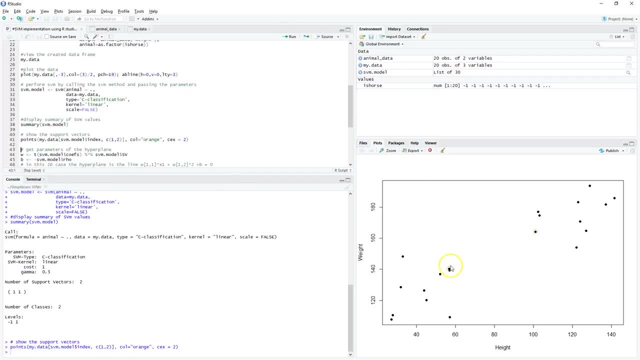 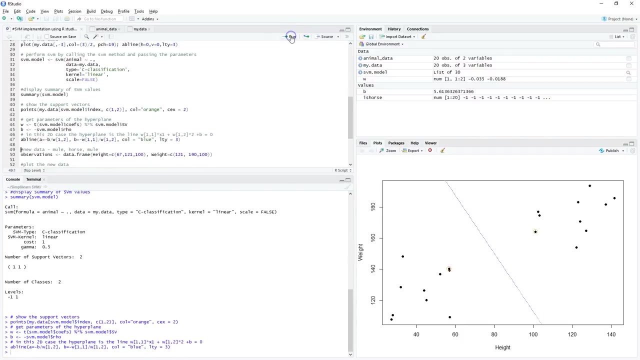 And this might be a little hard to see. the orange outline around this point And this point indicate that those are the two vectors that will support this model, And thus we call them the support vectors. Now let's get the parameters of the hyperplane from the model and let's plot a line that will be our hyperplane. 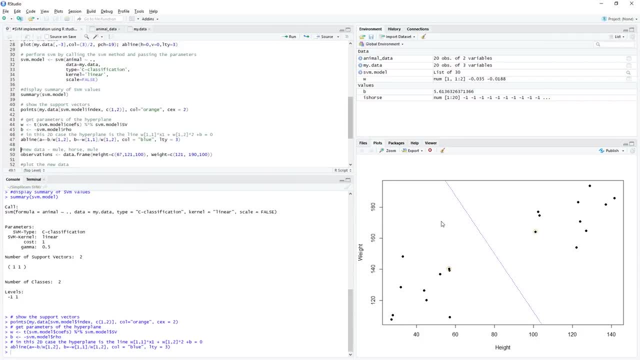 There's our hyperplane line And therefore to the left and below our mules and to the right and above our horses, above that line. Let's take a few new observations And I've encoded these so that it would be illustrative. We'll take these new observations and we'll plot them. 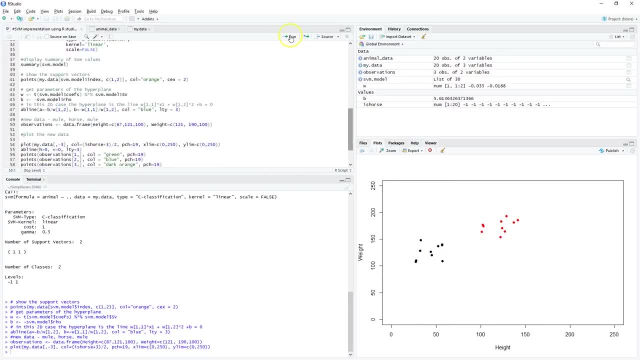 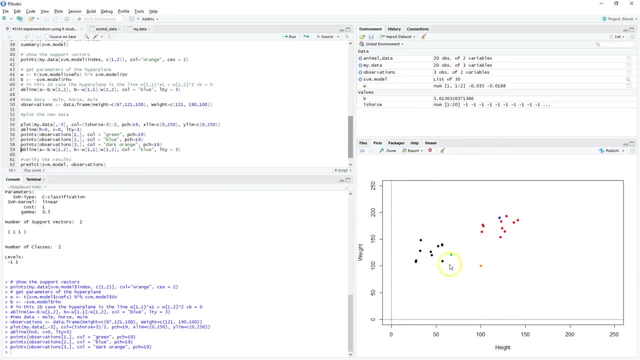 And I'm going to generate a new plot, Red being the horses, black dots being the mules. I'll create an X and Y axis. I'm going to plot three dots and you can see one of them, the green dot. The first one kind of falls near the mules. 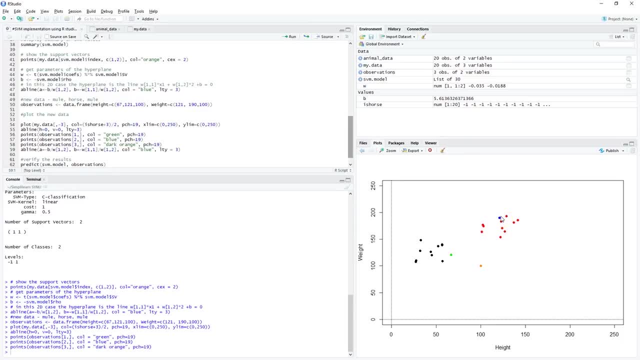 The blue one kind of falls near the horses And visually we might conclude: hey, one's a mule, one's a horse. But what about the orange dot? Well, for the orange dot we really need our hyperplane. 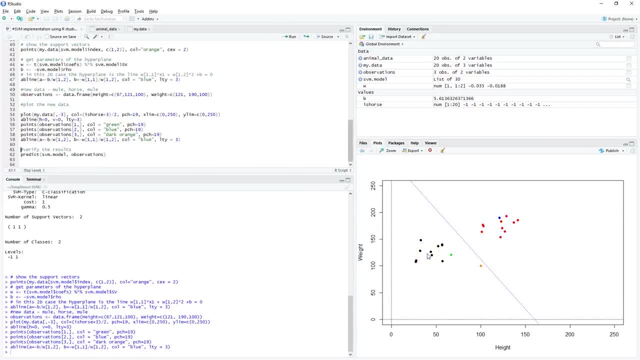 We really need something to clearly indicate which side it's on. And, of course, by looking at this data visualization we can tell that the orange dot is probably a mule. And let's verify those results by sticking those observations into our model and predict some outcomes. 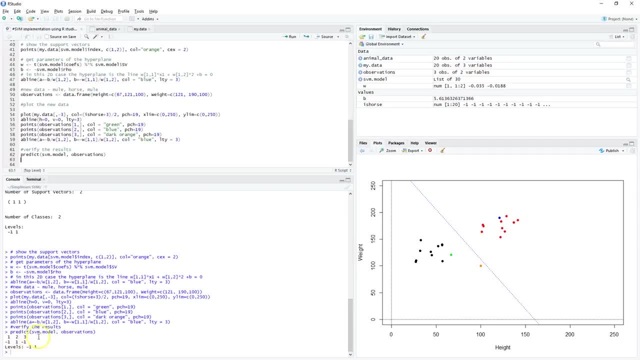 And down below you can see that for the three data points- one, two and three, the first one, the green one, was negative one, That's a mule. The second one was a positive one, That's blue. That's the blue point which was a horse. 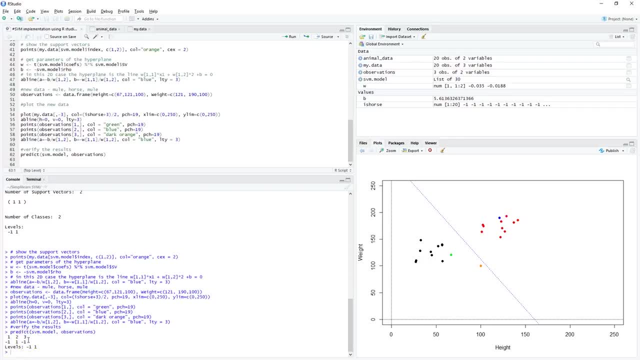 And the third one, which we weren't sure about, but clearly the SVM model correctly predicted that that third point would be a mule and we can visually see that by the hyperplane on the graph. So that's a quick example of SVM. 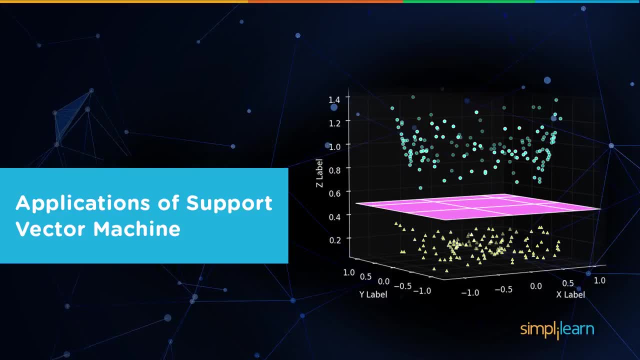 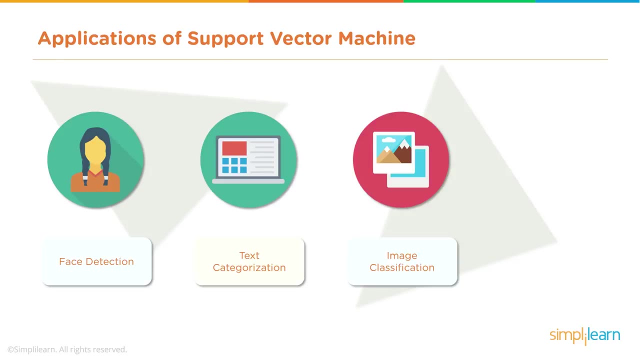 In general, support vector machines are binary classifiers. We don't use them for higher level classification. If you had three or more classes, you might want to use something like Random Forest. What applications You can use it for? face detection, text categorization, image classification and bioinformatics. 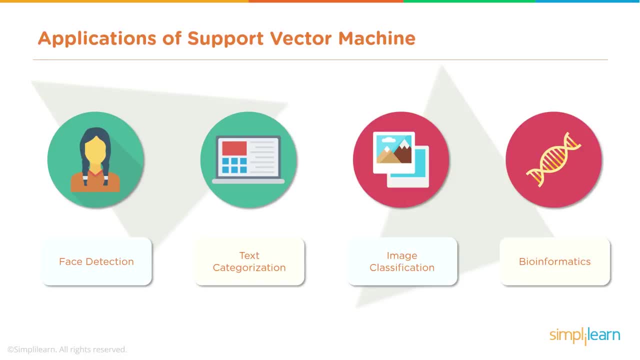 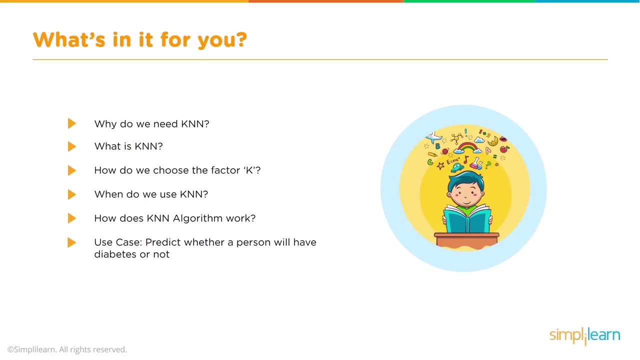 Really anywhere that you have the need to classify things into two groups. Today we're going to cover the K nearest neighbors, a lot referred to as K-N-N, And K-N-N is really a fundamental place to start in the machine learning. It's a basis of a lot of other things. 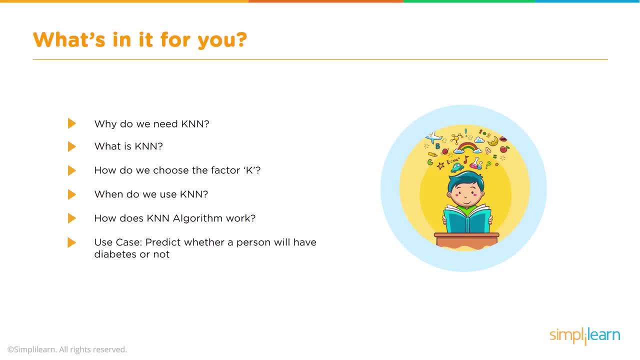 And just the logic behind it is easy to understand and incorporated in other forms of machine learning. So, today, what's in it for you? Why do we need K-N-N? What is K-N-N? How do we choose the factor K? 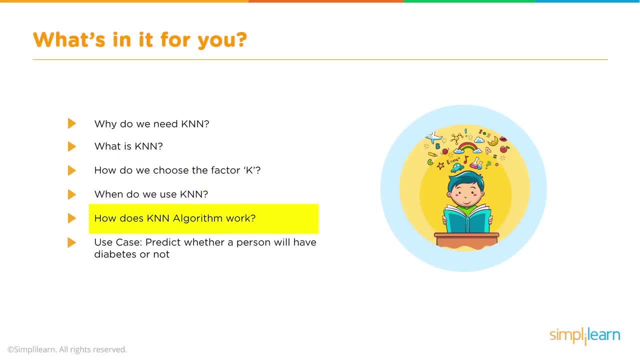 When do we use K-N-N? How does K-N-N algorithm work? And then we'll dive in to my favorite part: the use case Predict whether a person will have diabetes or not. That is a very common and popular used data set. as far as testing out models, 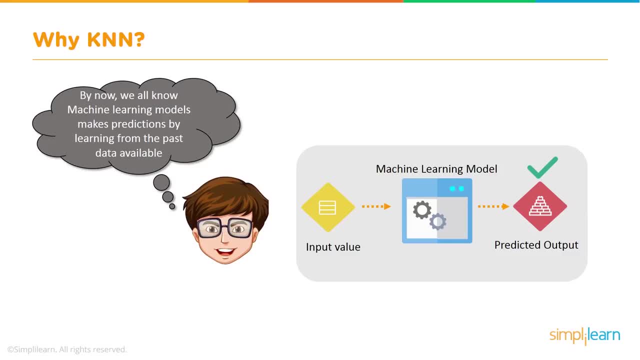 and learning how to use the different models in machine learning. By now we all know machine learning models make predictions by learning from the past data available. So we have our input values. our machine learning model builds on those inputs. We have what we already know. 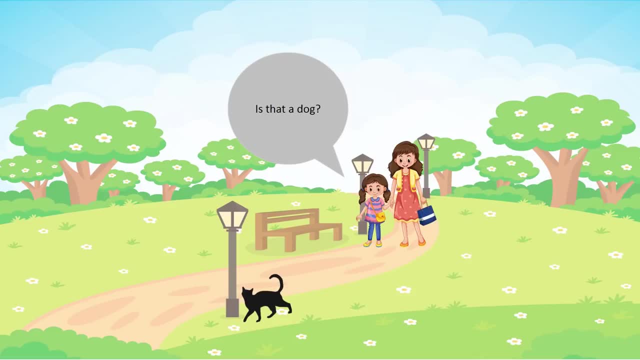 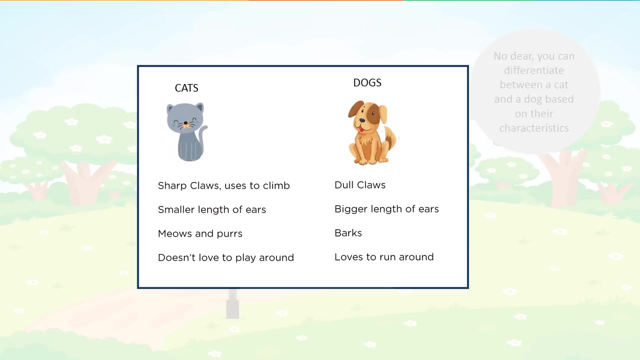 And then we use that to create a predicted output. Is that a dog? Little kid looking over there and watching the black cat cross their path? No dear, You can differentiate between a cat and a dog based on their characteristics: Cats- Cats have sharp claws. uses to climb. 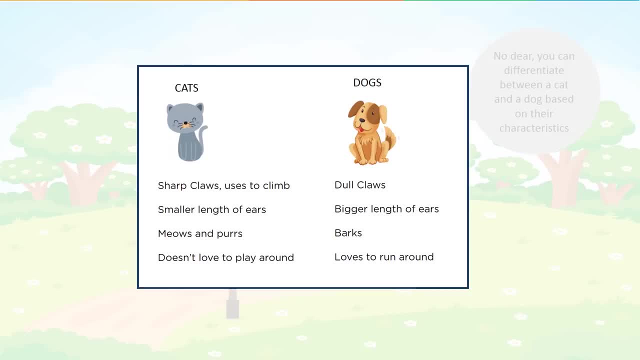 smaller length of ears, meows and purrs. doesn't love to play around. Dogs have dull claws. bigger length of ears. barks. loves to run around. Usually don't see a cat Running around people, Although I do have a cat that does that where dogs do. 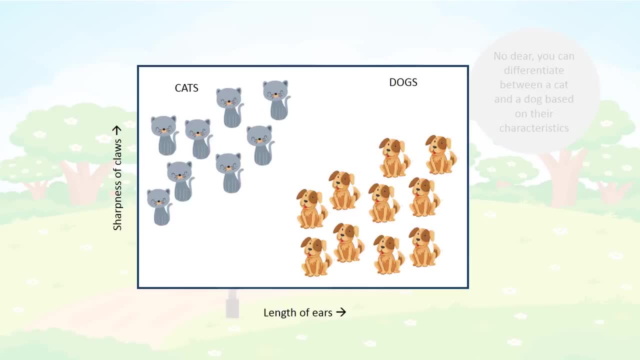 And we can look at these. We can say we can evaluate the sharpness of the claws- how sharp are their claws? and we can evaluate the length of the ears And we can usually sort out cats from dogs based on even those two characteristics. 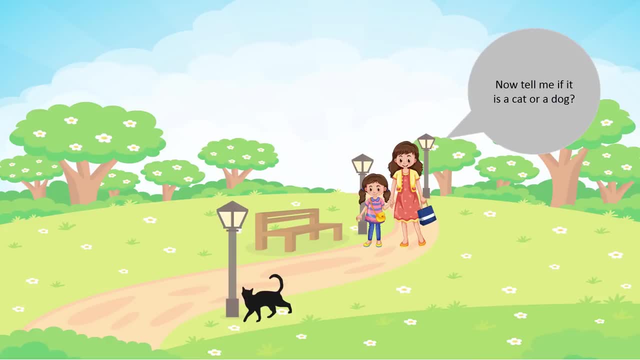 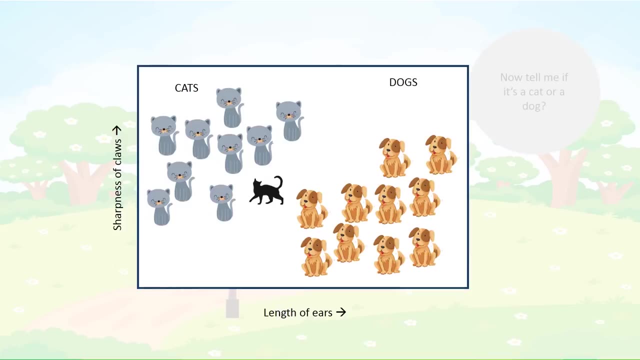 Now tell me if it is a cat or a dog, Not a question. Usually little kids know cats and dogs by now, Unless they live a place where there's not many cats or dogs. So if we look at the sharpness of the claws, the length of the ears, and we can 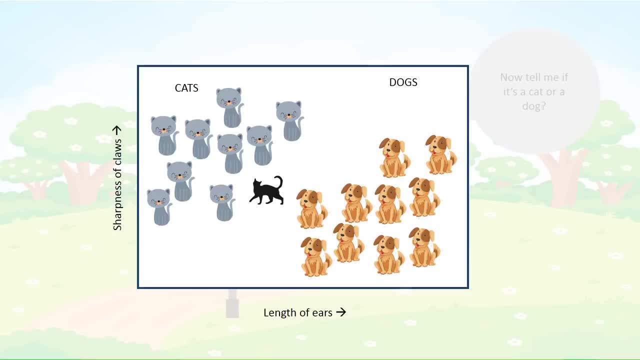 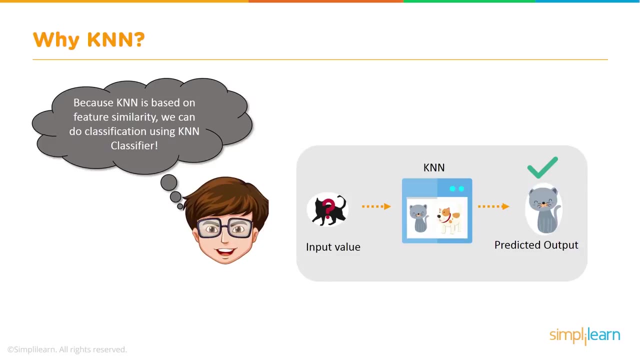 see that the cat has smaller ears and sharper claws than the other animals. Its features are more like cats. It must be a cat- Sharp claws, length of ears- And it goes in the cat group. Because KNN is based on feature similarity, we can do classification using KNN classifier. 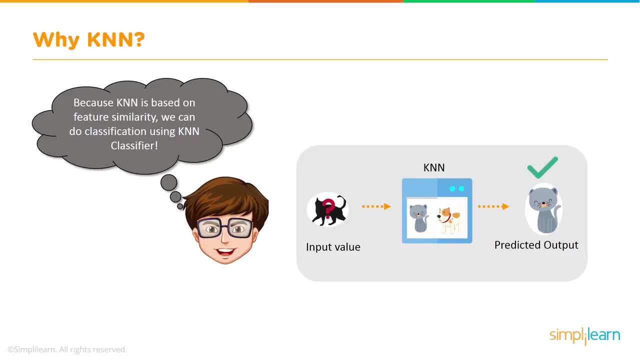 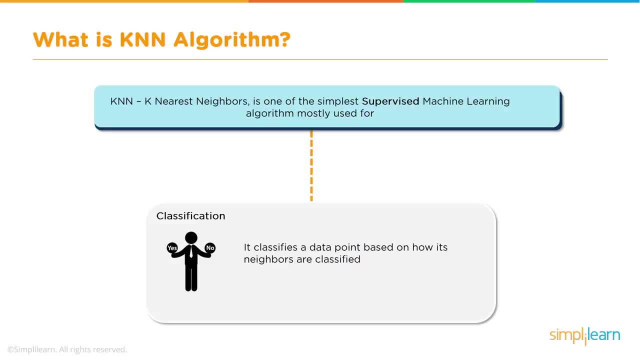 So we have our input value, the picture of the black cat. It goes into our trained model and it predicts that this is a cat coming out. So what is KNN? What is the KNN algorithm? KNN is the K nearest neighbors is what that stands for. 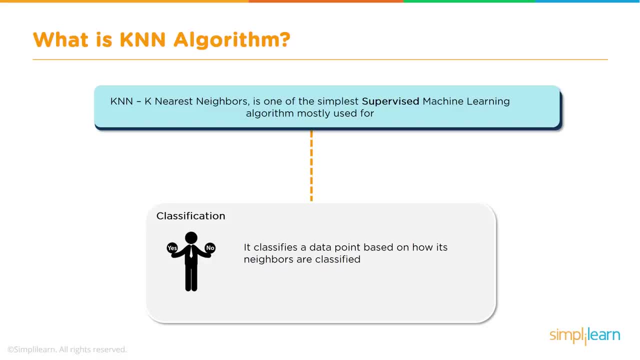 It's one of the simplest supervised machine learning algorithms mostly used for classification. So we want to know: is this a dog or it's not a dog? Is it a cat or not a cat? It classifies a data point based on how its neighbors are classified. 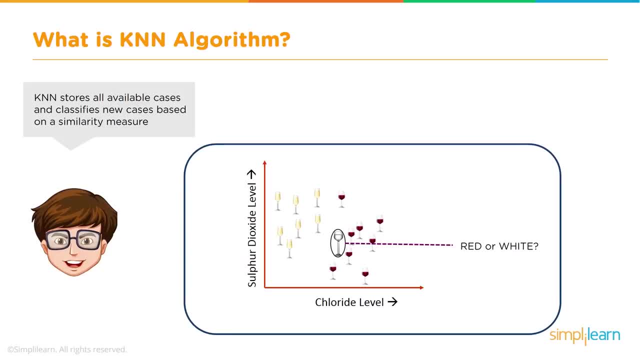 KNN stores all available cases and classifies new cases based on a similarity measure. And here we've gone from cats and dogs right into wine. another favorite of mine: KNN stores all available cases and classifies new cases based on a similarity measure. And here we've gone from cats and dogs right into wine- another favorite of mine. 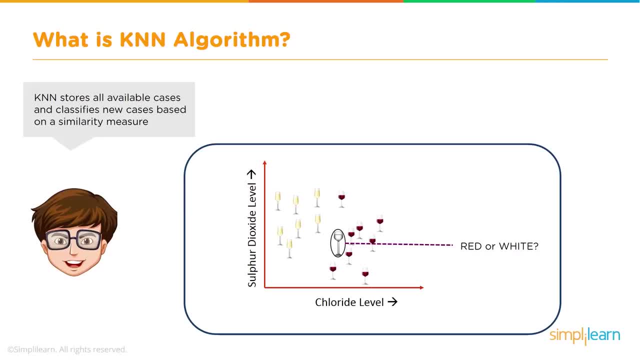 KNN stores all available cases and classifies new cases based on a similarity measure. And here you see, we have a measurement of sulfur dioxide versus the chloride level And then the different wines they've tested and where they fall on that graph, based on how much sulfur dioxide and how much chloride. 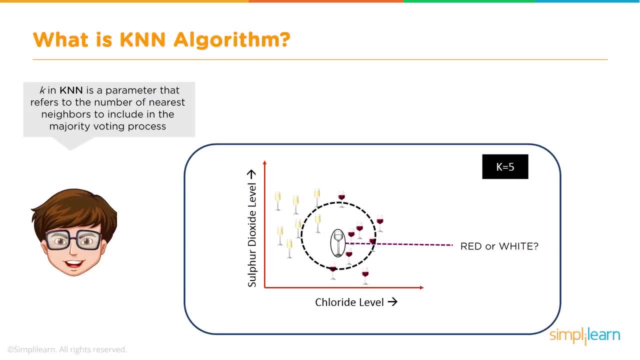 KNN is a perimeter that refers to the number of nearest neighbors to include in the majority of the voting process, And so if we had a new glass of wine there- red or white- we want to know what the neighbors are. In this case, we're going to put K equals five. 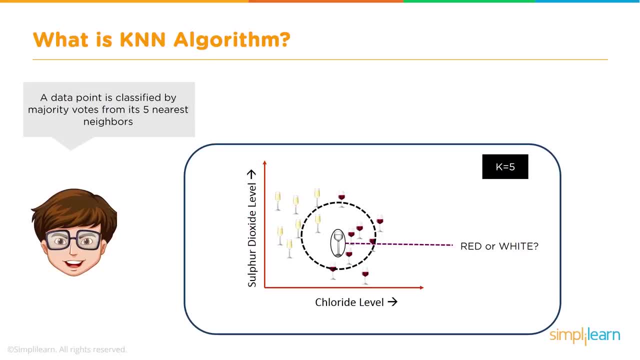 We'll talk about K in just a minute. A data point is classified by the majority of votes from its five nearest neighbors. Here, the unknown point would be classified as red, since four out of five neighbors are red. So how do we choose K? 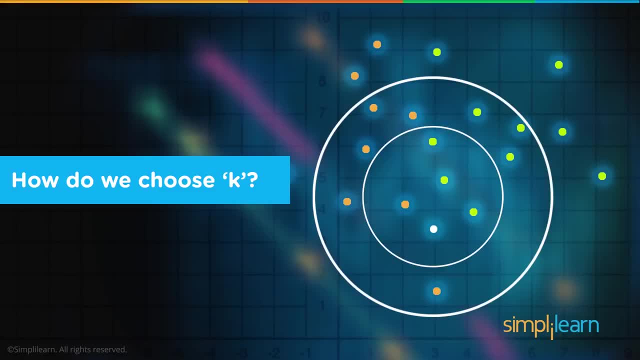 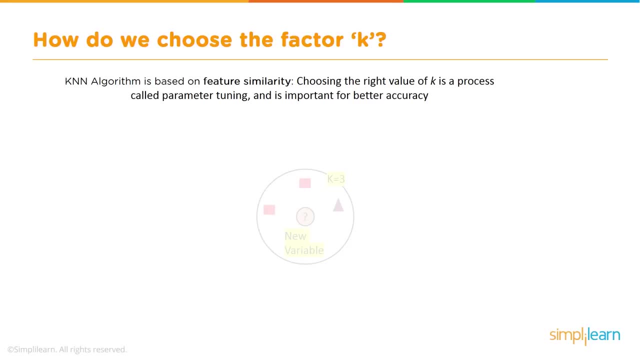 How do we know K equals five? I mean, that was the value we put in there, so we're going to talk about it. How do we choose the factor K? KNN algorithm is based on feature similarity. Choosing the right value of K is a process called parameter tuning and is important for better accuracy. 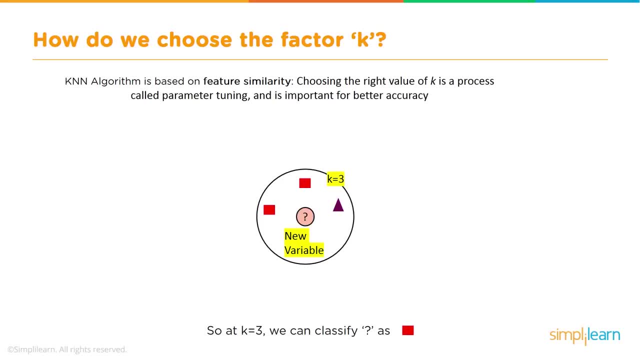 So, at K equals three, we can classify- We have a question mark in the middle- as either a, as a square or not. Is it a square or is it, in this case, a triangle? And so if we set K equals to three, we're going to look at the three nearest neighbors. 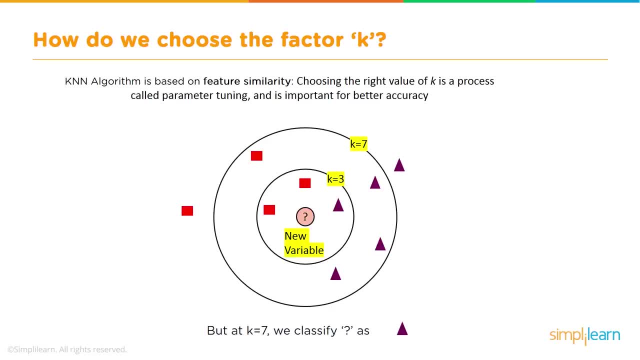 We're going to say this is a square And if we put K equals to seven, we classify as a triangle depending on what the other data is around, And you can see as the K changes depending on where that point is. that drastically changes your answer. 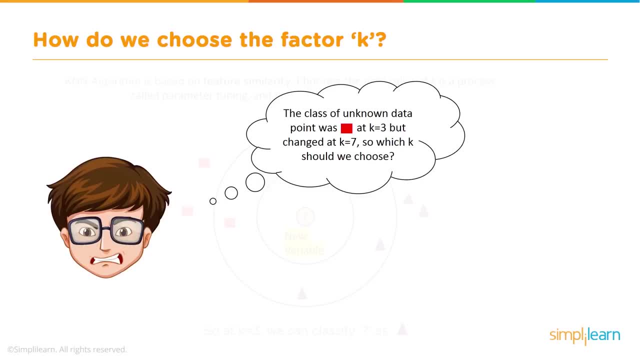 And we jump. here We go. how do we choose the factor of K? You'll find this in all machine learning: choosing these factors, That's the face you get. It's like: oh my gosh, I choose the right K. 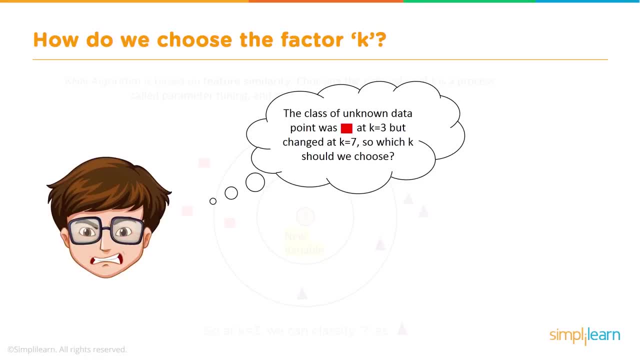 Did I set it right My values in whatever machine learning tool you're looking at, so that you don't have a huge bias in one direction or the other. And in terms of KNN, the number of K, if you choose it too low, the bias is based on- it's just too noisy. 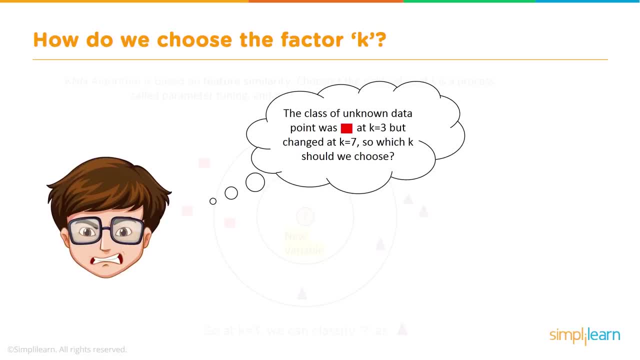 It's right next to a couple of things and it's going to pick those things and you might get a skewed answer And if your K is too big then it's going to take forever to process. So you're going to run into processing issues and resource issues. 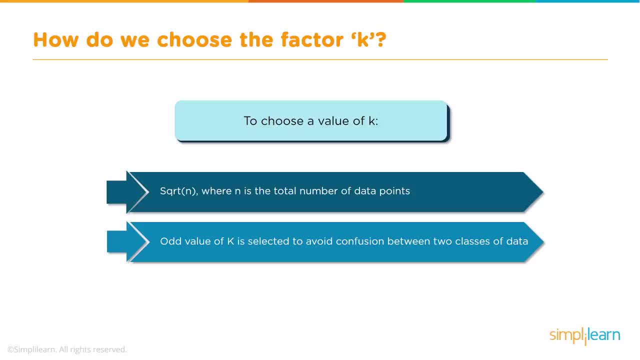 So we do. the most common use- and there's other options for choosing K- is to use the square root of N. So it is a total number of values you have. You take the square root of it. In most cases you also if it's an even number. 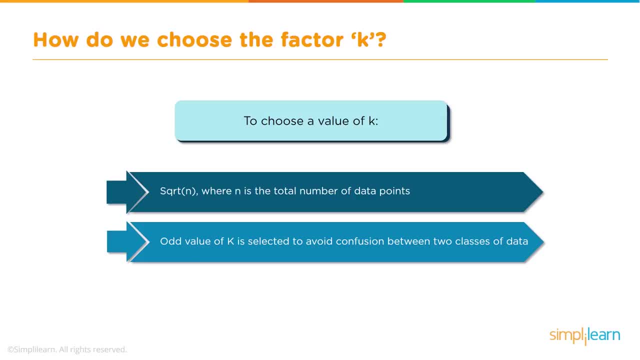 So if you're using, like this case, squares and triangles, if it's even, you want to make your K value odd, That helps it select better. So, in other words, you're not going to have a balance between two different factors that are equal. 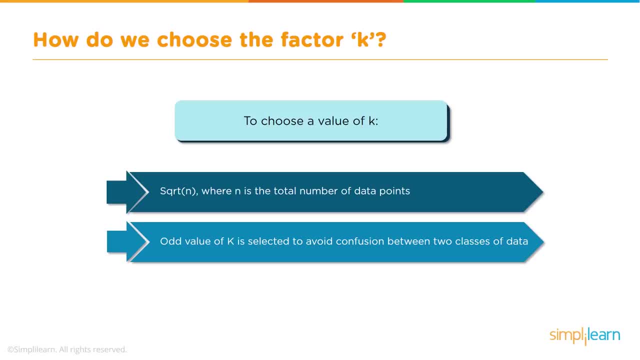 So usually take the square root of N and, if it's even you, add one to it or subtract one from it, And that's where you get the K value from. That is the most common use and it's pretty solid. It works very well. 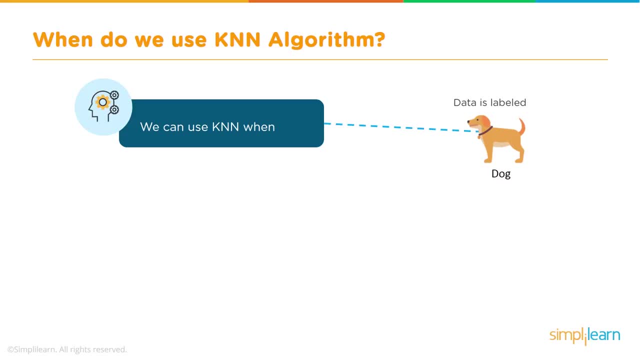 When do we use KNN? We can use KNN when data is labeled, So you need a label on it. We know we have a group of pictures with dogs, dogs, cats, cats. Data is noise free And so you can see here when we have a class and we have like underweight 140, 23.. 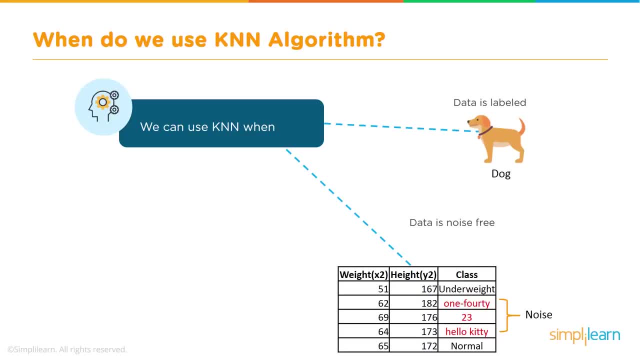 Hello Kitty normal. That's pretty confusing. We have a high variety of data coming in So it's very noisy and that would cause an issue. Data set is small, So we're usually working with smaller data sets where you might get into a gig of data. 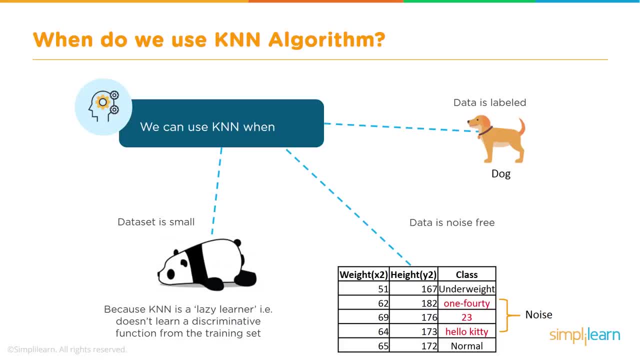 If it's really clean, doesn't have a lot of noise, because KNN is a lazy learner IE it doesn't learn a discriminative function from the training set, So it's very lazy. So if you have very complicated data and you have a large amount of it, 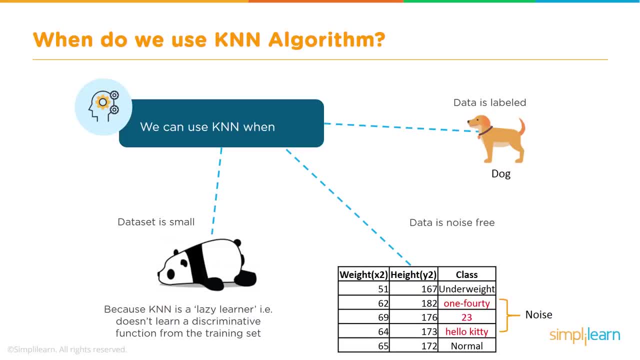 you're not going to use the KNN, but it's really great to get a place to start, Even with large data. you can sort out a small sample and get an idea of what that looks like Using the KNN and also just using for smaller data sets. 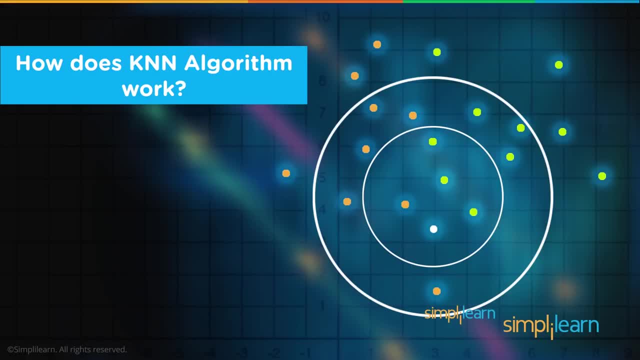 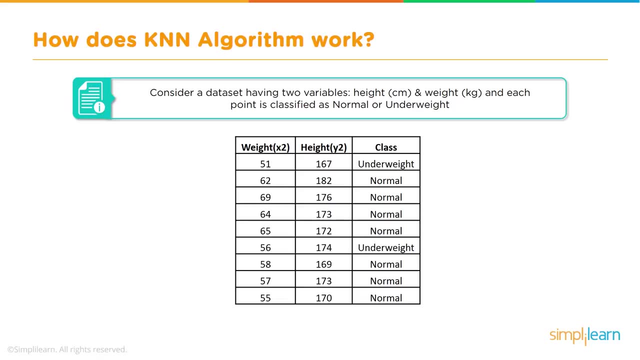 KNN works really good. How does a KNN algorithm work? Consider a data set having two variables- height in centimeters and weight in kilograms, And each point is classified as normal or underweight. So we can see right here we have two variables. 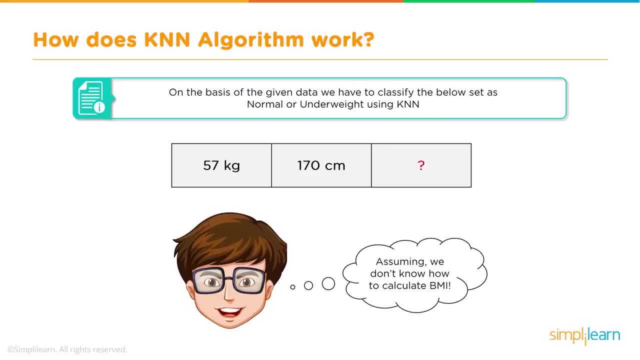 You know true, false, or either normal or they're not. They're underweight. on the basis of the given data, We have to classify the below set as normal or underweight using KNN. So if we have new data coming in that says 57 kilograms and 177 centimeters, 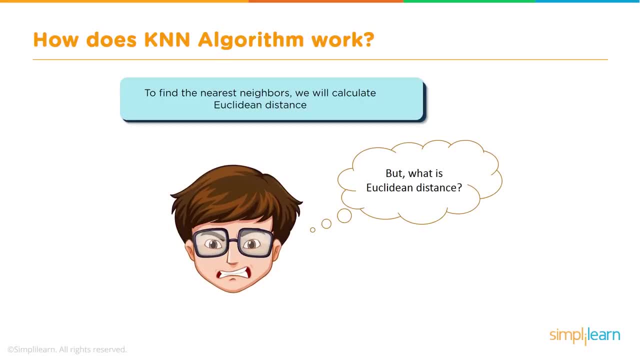 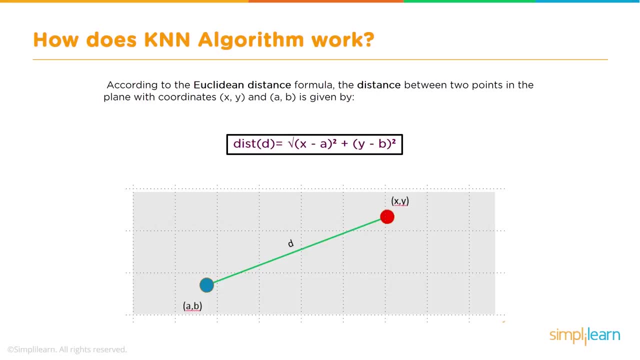 is that going to be normal or underweight To find the nearest neighbors? we'll calculate the Euclidean distance According to the Euclidean distance formula. the distance between two points in the plane with the coordinates XY and AB is given by distance. D equals the square root of X minus A squared plus Y. 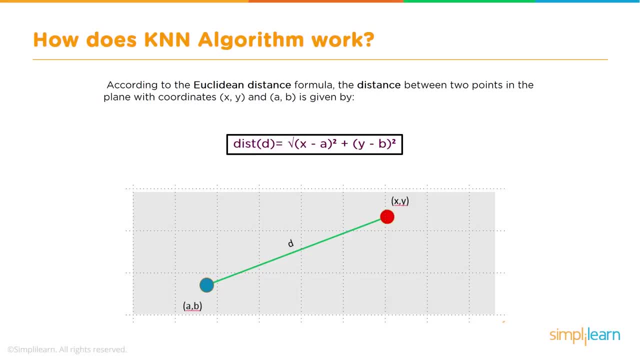 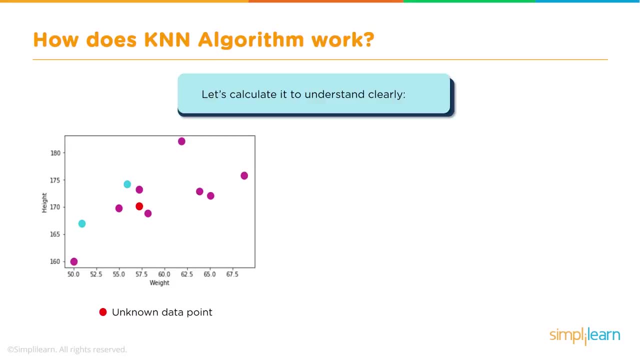 minus B squared, And you can remember that from the two edges of a triangle, We're computing the third edge. since we know the X side and the Y side, Let's calculate it to understand clearly. So we have our unknown point and we placed it there in red. 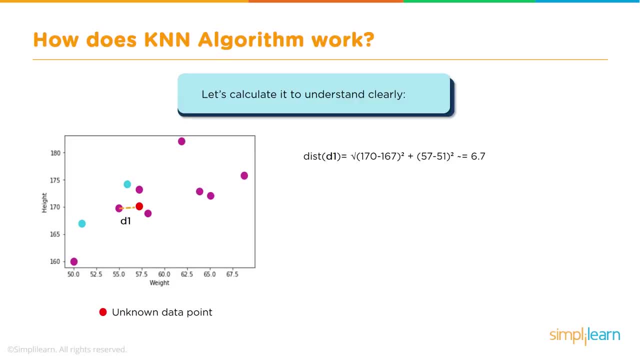 And we have our other points where the data is scattered around. The distance D1 is the square root of 170 minus 167 squared, plus 57 minus 51 squared, which is about 6.7.. And distance 2 is about 13 and distance 3 is about 13.4.. 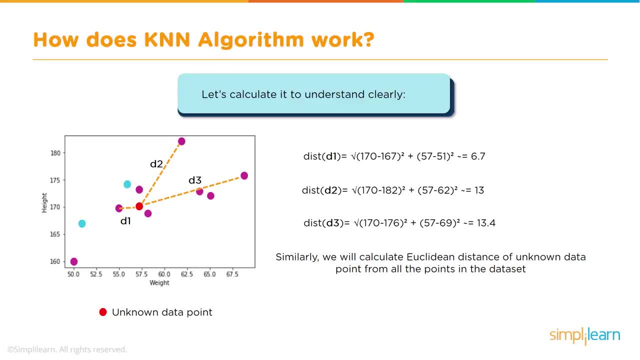 Similarly, we will calculate the Euclidean distance of unknown data point from all the points in the data set And because we're dealing with small amount of data, that's not that hard to do. It's actually pretty quick for a computer and it's not a really complicated math. 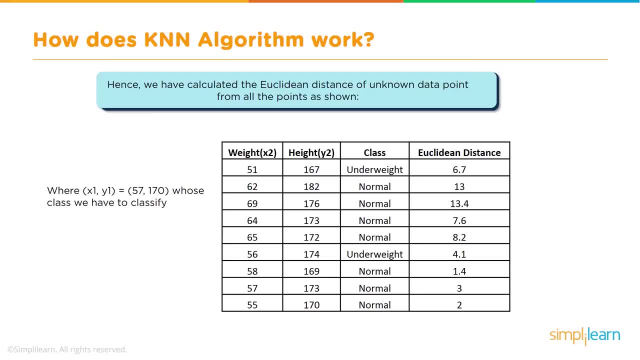 You can just see how close is the data based on the Euclidean distance. Hence, we have calculated the Euclidean distance of unknown data point from all the points as shown, where X1 and Y1 equal 57 and 170.. So whose class we have to classify? 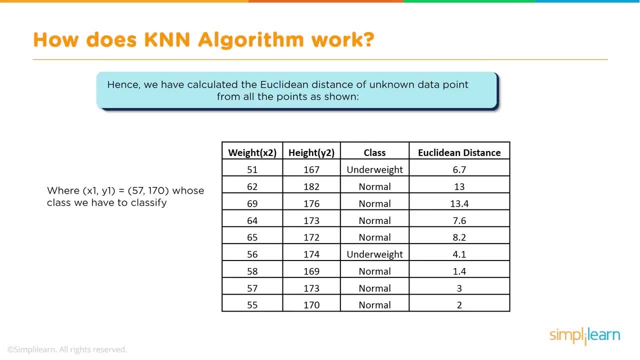 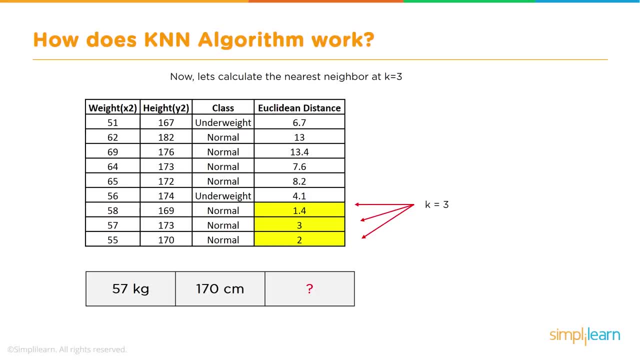 So now we're looking at that, we're saying, well, here's the Euclidean distance, Who's going to be the closest neighbors? Now let's calculate the nearest neighbor at K equals three And we can see the three closest neighbors. puts them at normal. 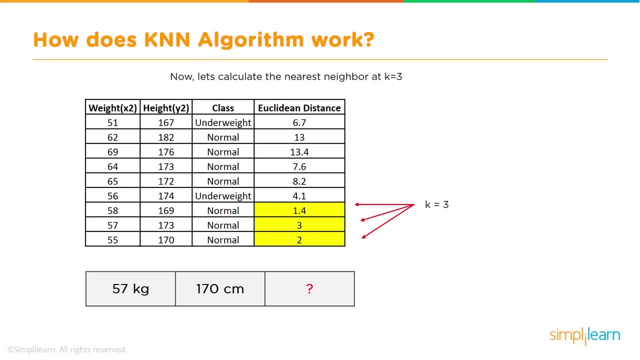 And that's pretty self-evident. When you look at this graph, it's pretty easy to say: OK, what We're just voting, normal, normal, normal. three votes for normal. This is going to be a normal weight. 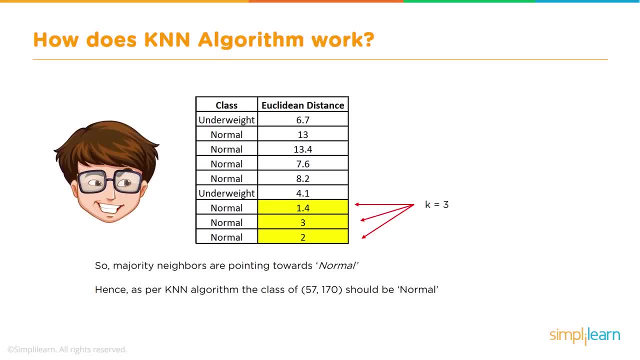 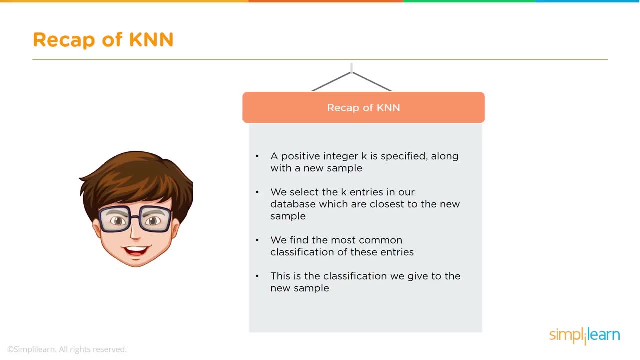 So majority of neighbors are pointing towards normal. Hence, as per K and N algorithm, the class of 57, 170 should be normal. So a recap of K and N Positive integer K is specified along with a new sample. We select the K entries in our database which are closest to the new sample. 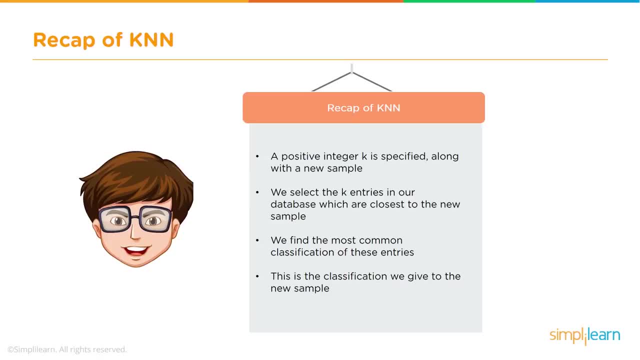 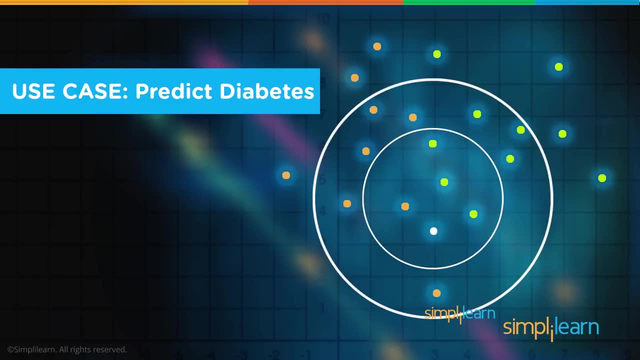 We find the most common classification of these entries. This is the classification we give to the new sample. So, as you can see, it's pretty straightforward. We're just looking for the closest things that match what we got. So let's take a look and see what that looks like in a use case in Python. 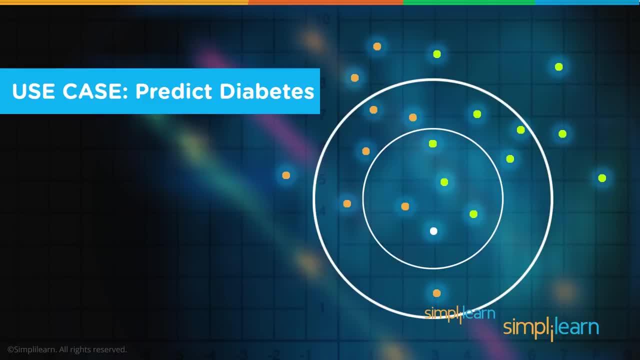 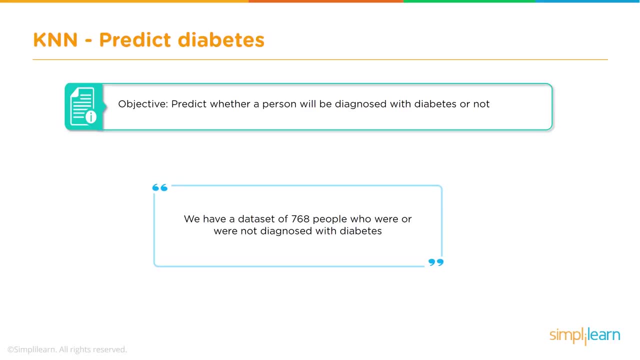 So let's dive into the predict diabetes use case. So use case: Predict diabetes. The objective: predict whether a person will be diagnosed with diabetes or not. We have a data set of 768 people who were or were not diagnosed with diabetes And let's go ahead and open that file and just take a look at that data. 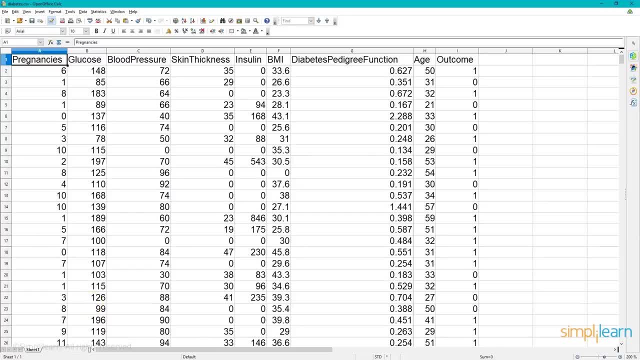 And this is in a simple spreadsheet format. The data itself is comma separated, very common set of data And it's also a very common way to get the data And you can see here we have columns A through I. That's what one, two, three, four. 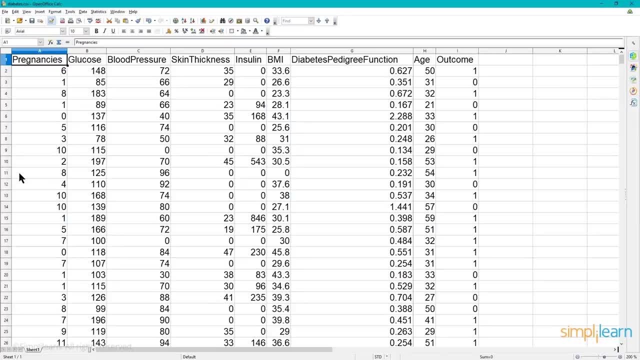 five, six, seven, eight, eight columns with a particular attribute, And then the ninth column, which is the outcome is whether they have diabetes. As a data scientist, the first thing you should be looking at is insulin. Well, you know, if someone has insulin, 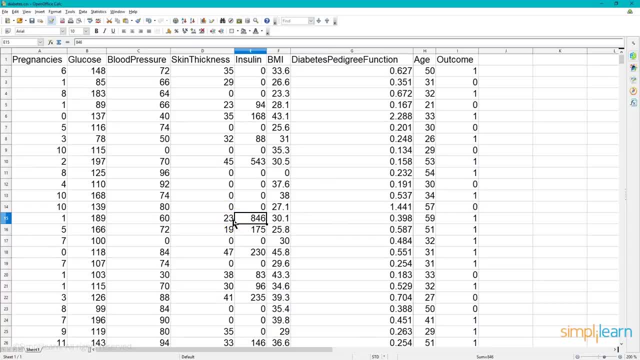 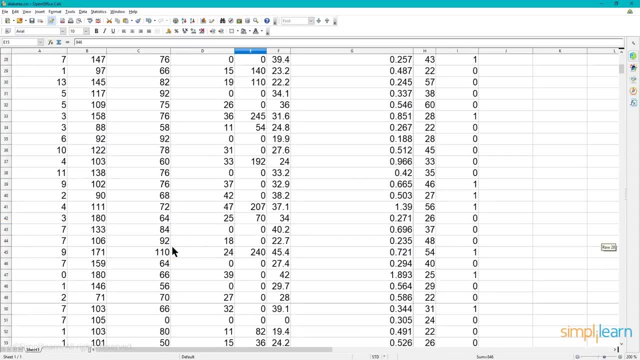 they have diabetes because that's why they're taking it, And that could cause issue in some of the machine learning packages. But for a very basic setup this works fine for doing the KNN And the next thing you notice is it didn't take very much to open it up. 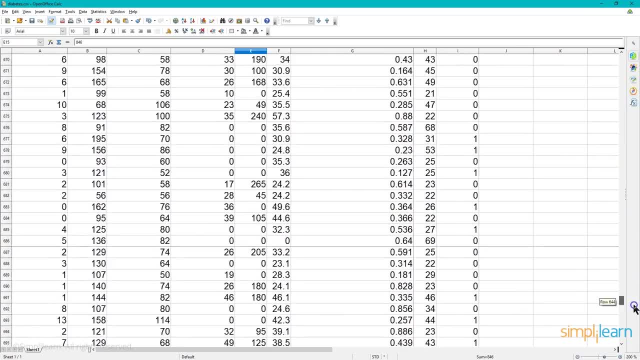 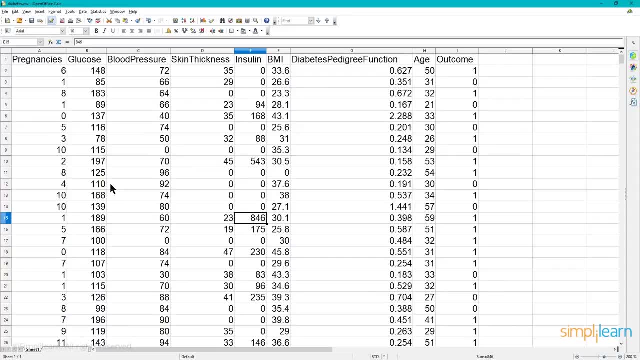 I can scroll down to the bottom of the data. There's seven hundred and sixty eight. It's pretty much a small data set. You know it's seven hundred sixty nine. I can easily fit this into my RAM on my computer. I can look at it. I can manipulate it. 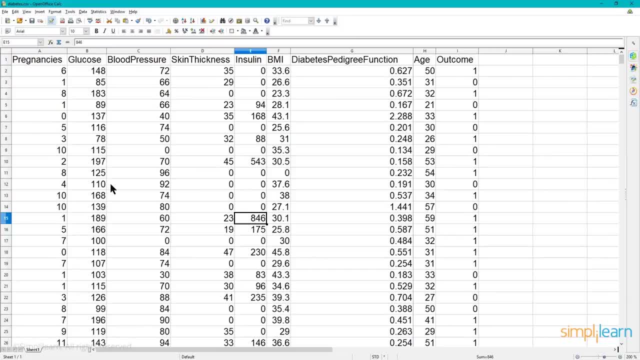 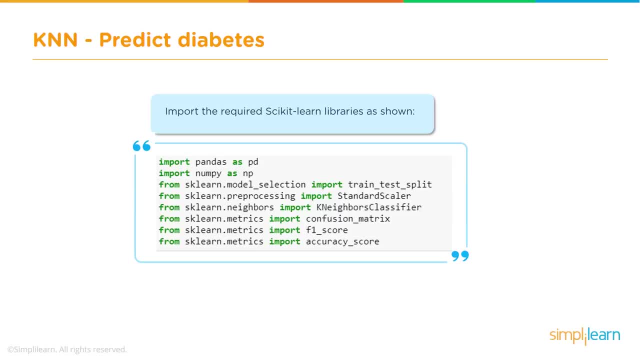 and it's not going to really tax- just a regular desktop computer. You don't even need an enterprise version to run a lot of this. So let's start with importing all the tools we need, And before that, of course, we need to discuss what IDE I'm using. 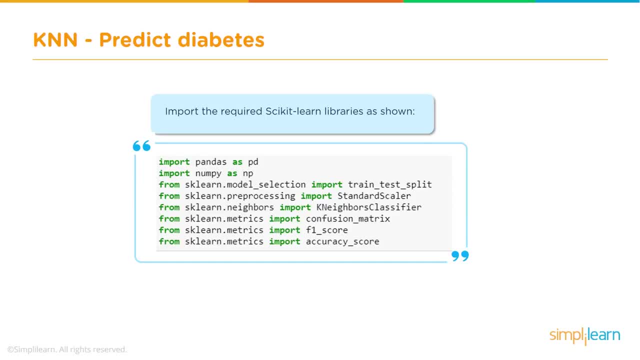 Certainly can use any particular editor for Python, But I like to use, for doing very basic visual stuff, the Anaconda, which is great for doing demos with the Jupyter Notebook. And just a quick view of the Anaconda Navigator, which is the new release out there, which is really nice. 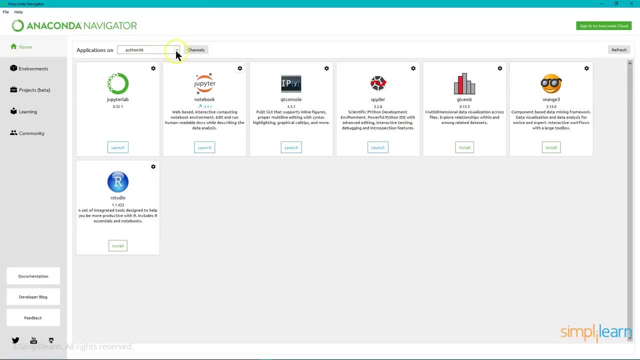 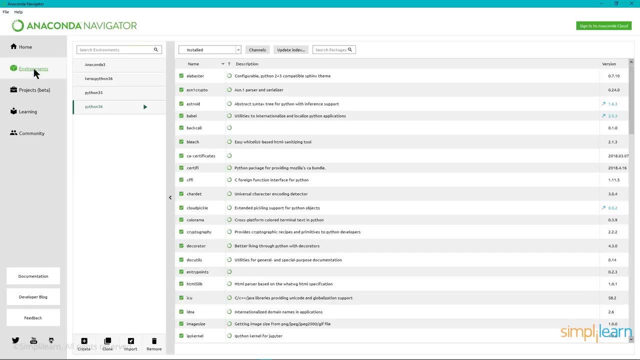 You can see under home, I can choose my application. We're going to be using Python 3.6.. I have a couple of different versions on this particular machine. If I go under environments, I can create a unique environment for each one, which is nice. 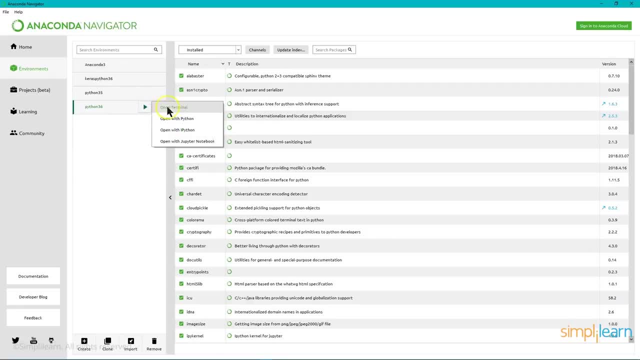 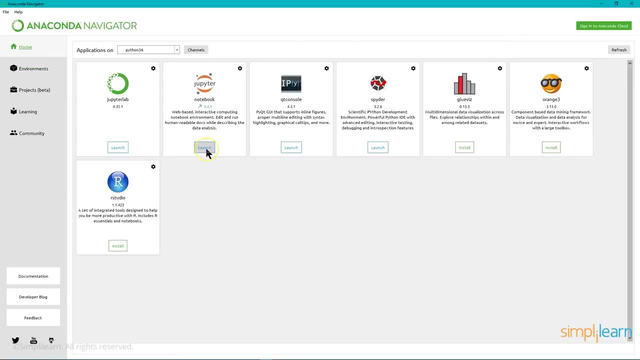 And there's even a little button there where I can install different packages. If I click on that button and open the terminal, I can then use a simple zip install to install different packages I'm working with. Let's go ahead and go back under home and we're going to launch our notebook. 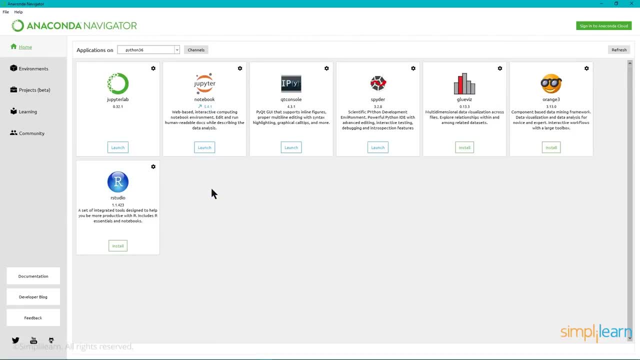 And I've already- you know, kind of like the old cooking shows- I've already prepared a lot of my stuff, so we don't have to wait for it to launch, because it takes a few minutes for it to open up a browser window. 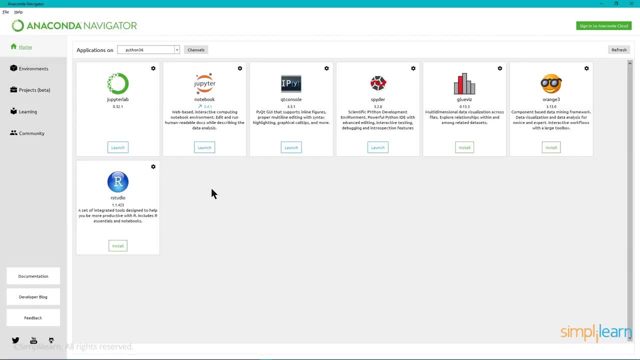 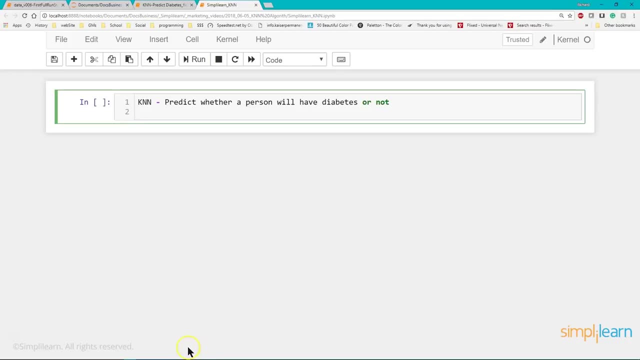 In this case, I'm going to open up Chrome, because that's my default that I use, And since the script is pre-done, you'll see I have a number of windows open up at the top, The one we're working in. And since we're working on, the KNN predict whether a person will have diabetes or not. 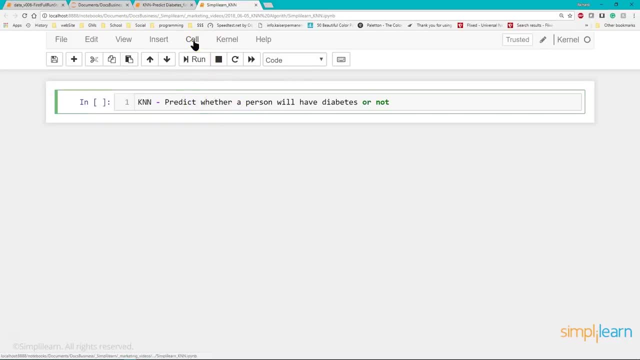 You can put that title in there And I'm also going to go up here and click on cell. Actually, we want to go ahead and first insert a cell below And then I'm going to go back up to the top cell and I'm going to change the cell type to markdown. 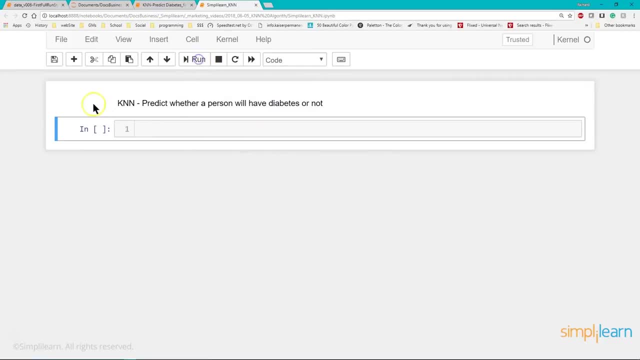 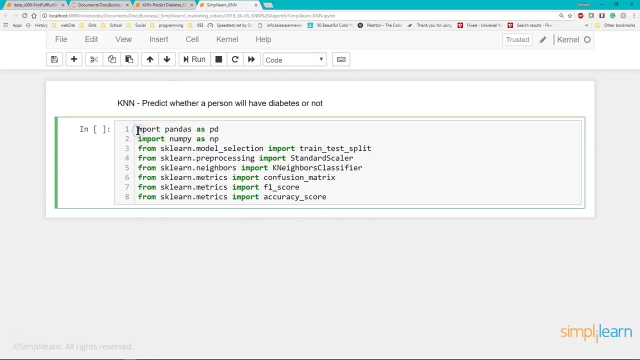 That means this is not going to run as Python It's a markdown language, So if I run this first one it comes up in nice big letters, which is kind of nice, Remind us what we're working on, And by now you should be familiar with doing all of our imports. 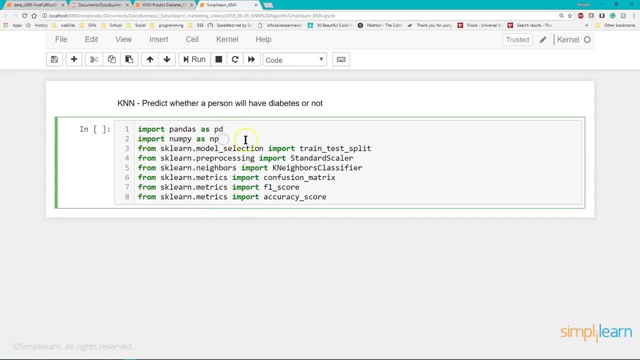 We're going to import the pandas as PD Import, numpy as NP. Pandas is the pandas data frame and numpy is a number array- Very powerful tools to use in here. So we have our imports. So we've brought in our pandas, our numpy, our two general Python tools. 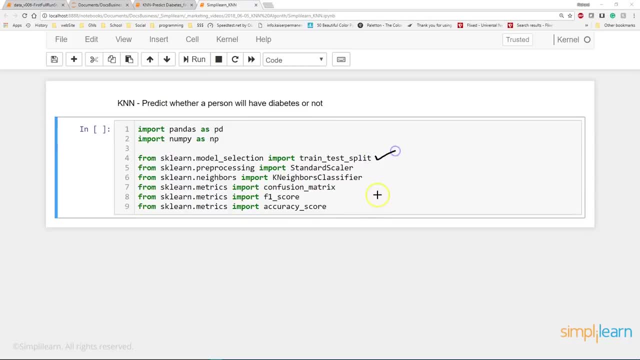 And then you can see over here we have our train test split By now. you should be familiar with splitting the data. We want to split part of it for training our thing and then training our particular model, And then we want to go ahead and test the remaining data to see how good it is. 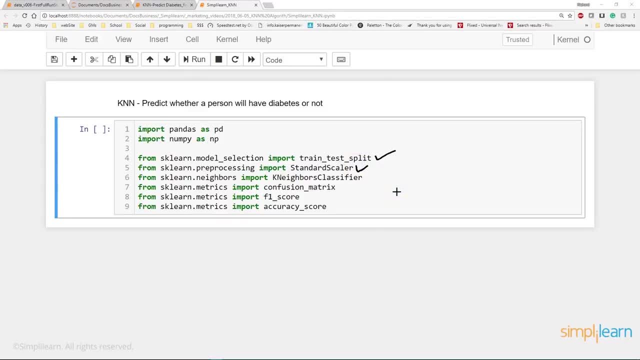 Pre-processing, A standard scalar preprocessor, So we don't have a bias of really large numbers. Remember, in the data we had, like number of pregnancies isn't going to get very large, Where the amount of insulin they take can get up to 256.. 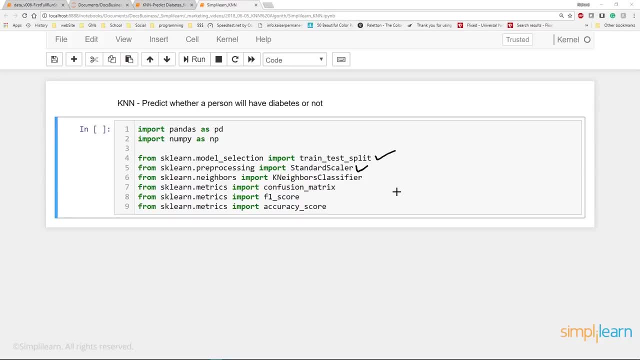 So 256 versus 6, that will skew results. So we want to go ahead and change that so that they're all uniform between minus 1 and 1.. And then the actual tool. This is the k-neighbors classifier we're going to use. 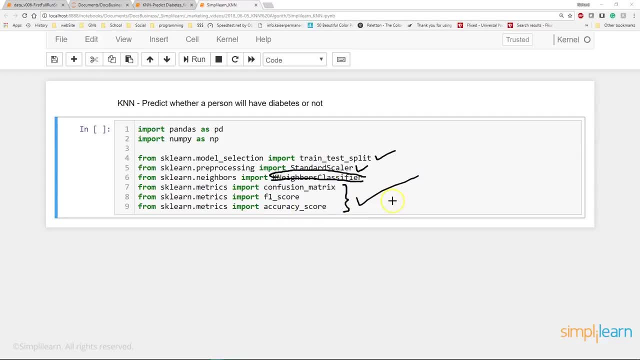 And finally the last three are three tools to test. All about testing our model. How good is it? Let me just put down test on there. And we have our confusion matrix, our F1 score and our accuracy. So we have our two general Python modules we're importing. 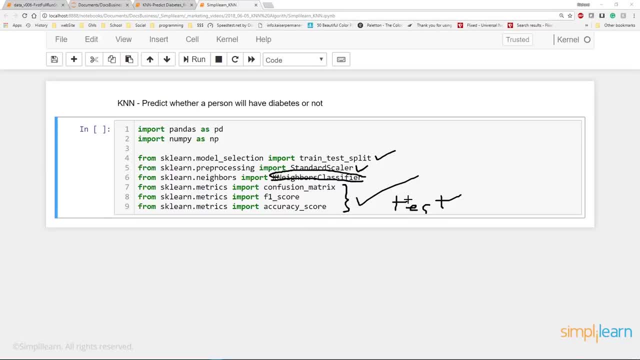 And then we have our six modules specific from the sklearn setup, And then we do need to go ahead and run this, So these are actually imported. There we go And then move on to the next step, And so in this set we're going to go ahead and load the database. 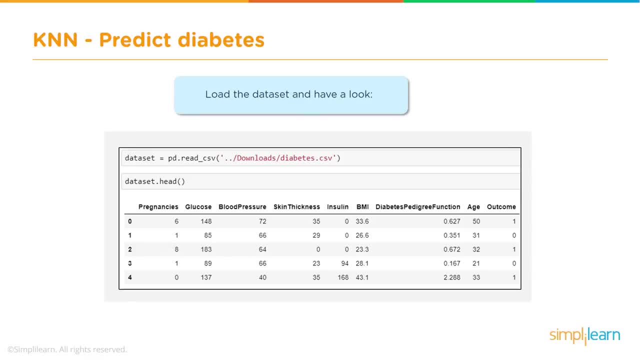 We're going to use pandas- Remember, pandas is PD- And we'll take a look at the data in Python. We looked at it in a simple spreadsheet, But usually I like to also pull it up so that we can see what we're doing. 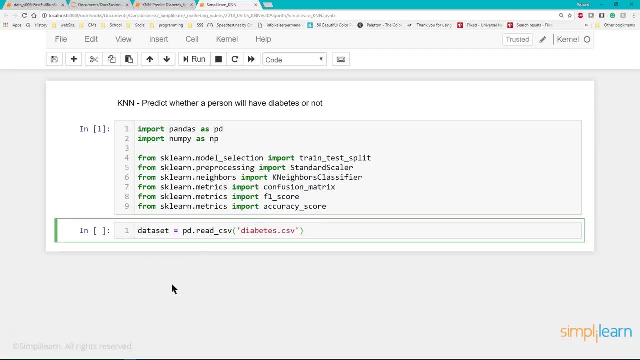 So here's our data set equals pdreadcsv. That's a pandas command, And the diabetes folder I just put in the same folder where my IPython script is. If you put in a different folder you'd need the full length on there. 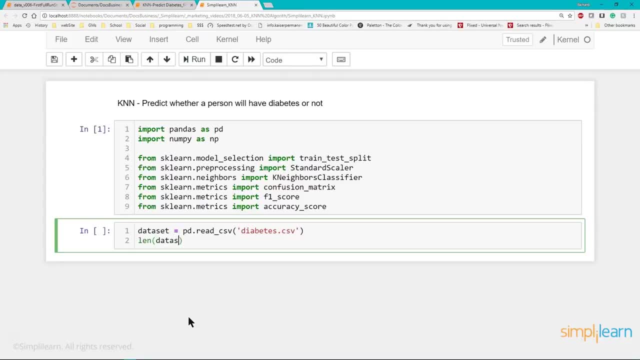 We can also do a quick length of the data set. That is a simple Python command: len for length. We might even let's go ahead and print that. We'll go print If you do it on its own line. lengthdataset in the Jupyter Notebook. 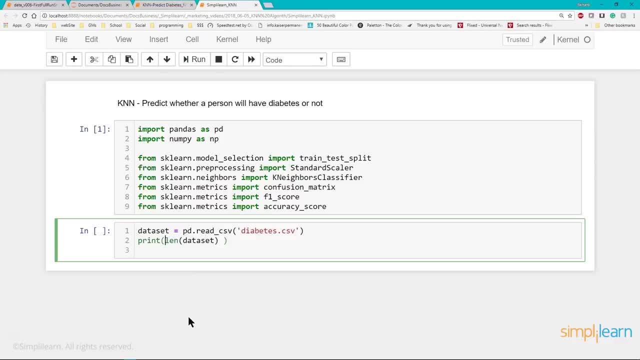 it'll automatically print it, But when you're in most of your different setups, you want to do the print in front of there, And then we want to take a look at the actual data set And since we're in pandas, we can simply do data set head. 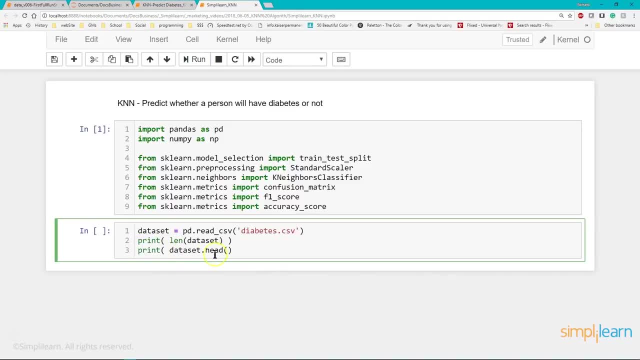 And again, let's go ahead and add the print in there. If you put a bunch of these in a row, you know the data set one head, data set two head. it only prints out the last one. So I always like to keep the print statement in there. 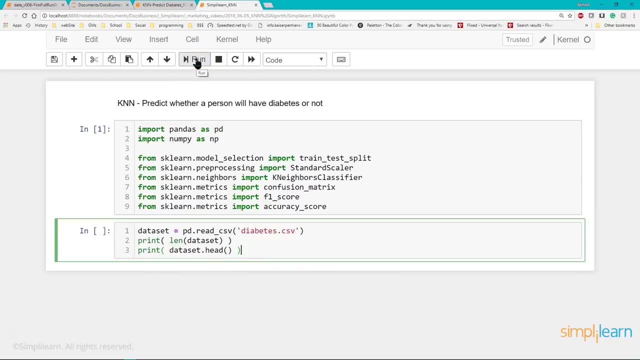 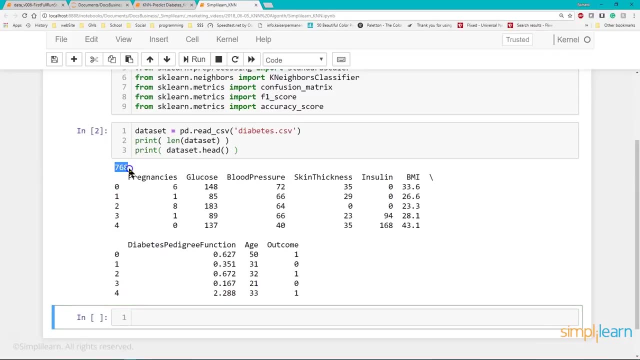 But because most projects only use one data frame- pandas data frame- doing it this way doesn't really matter. The other way works just fine And you can see when we hit the run button we have the 768 lines which we knew. 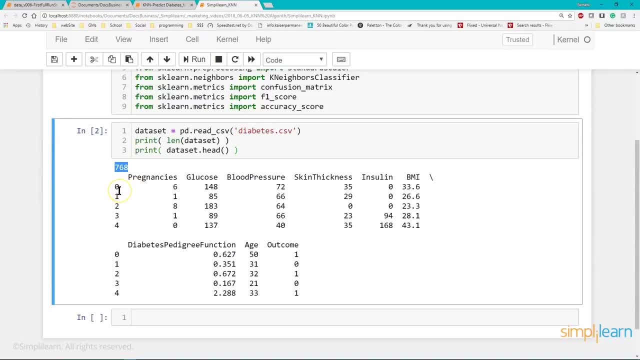 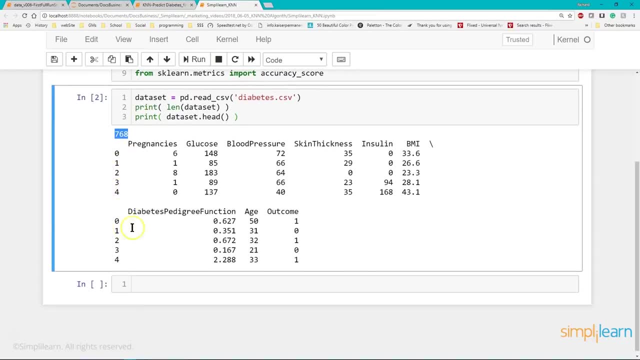 And we have our pregnancies, It's automatically given a label on the left, Remember, the head only shows the first five lines, So we have zero through four And just a quick look at the data You can see it matches what we looked at before. 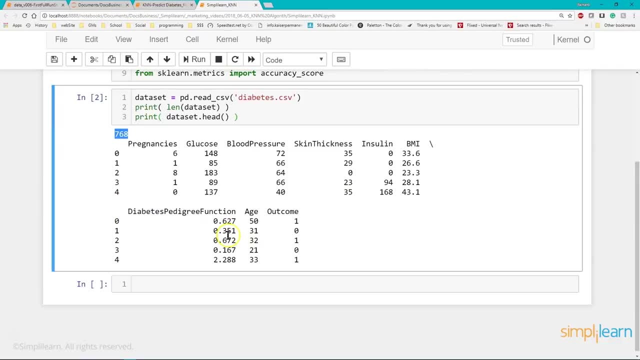 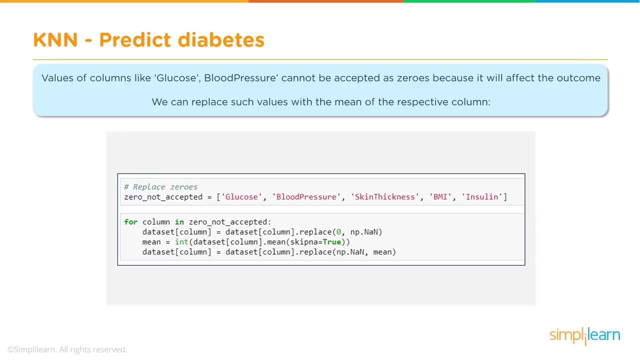 We have pregnancy, glucose blood pressure all the way to age, and then the outcome on the end, And we're going to do a couple of things in this next step. We're going to create a list of columns where we can't have zero. 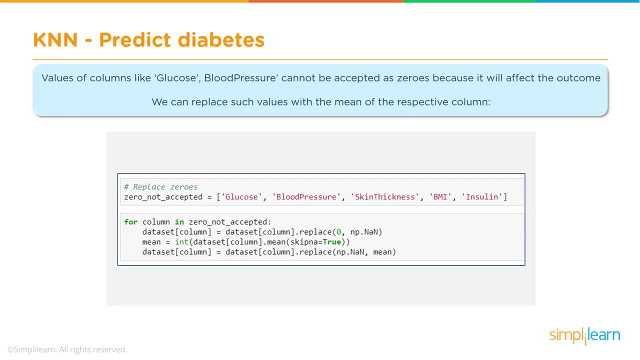 There's no such thing as zero skin thickness or zero blood pressure, zero glucose- Any of those, you'd be dead. So not a really good factor if they don't, if they have a zero in there because they didn't have the data. 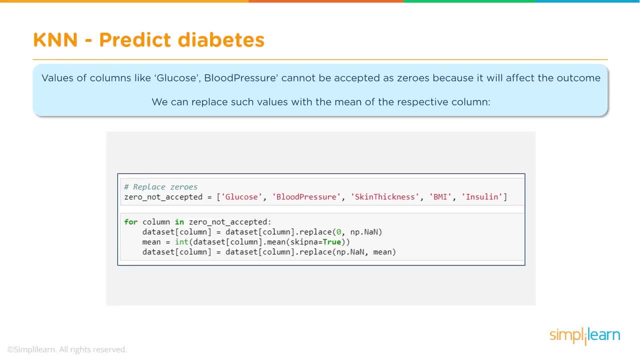 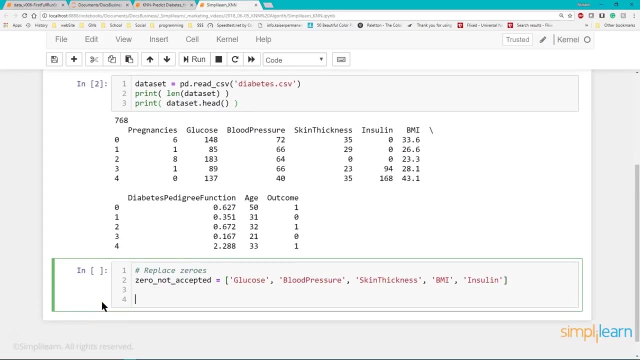 And we'll take a look at that, because we're going to start replacing that information with a couple of different things And let's see what that looks like. So first we create a nice list. As you can see, we have the values we talked. 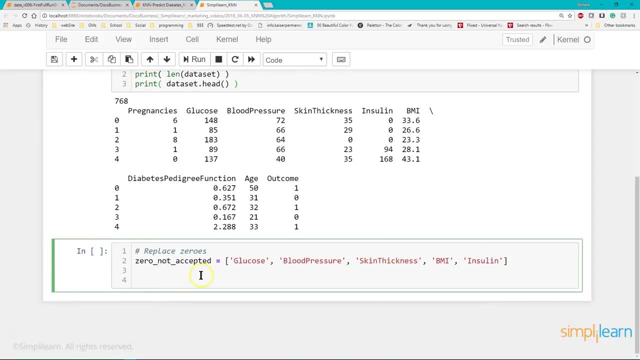 about glucose, blood pressure, skin thickness- And this is a nice way when you're working with columns- is to list the columns. you need to do some kind of transformation on a very common thing to do, And then for this particular setup, we certainly could use the there's some. 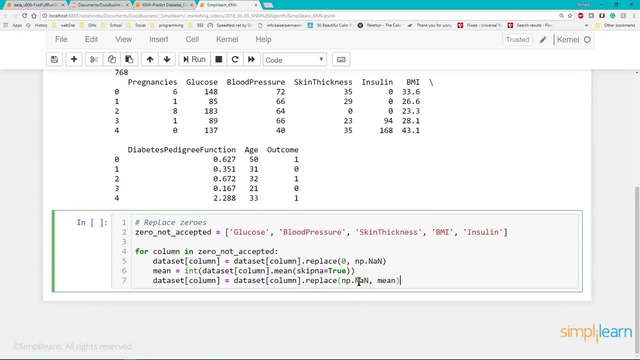 panda tools that will do a lot of this, where we can replace the NA, But we're going to go ahead and do it as a dataset column equals dataset column. dot replace this is still pandas. you can do a direct. There's also one that you look for your NAN. a lot of different options in here. 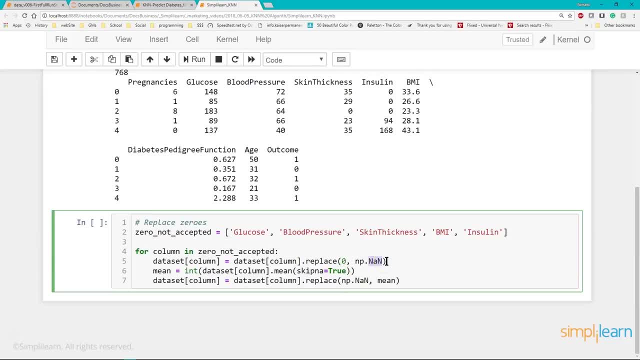 But the NAN- numpy NAN is what that stands for- is none. it doesn't exist. So the first thing we're doing here is we're replacing the zero with a numpy none. There's no data there. That's what that says. 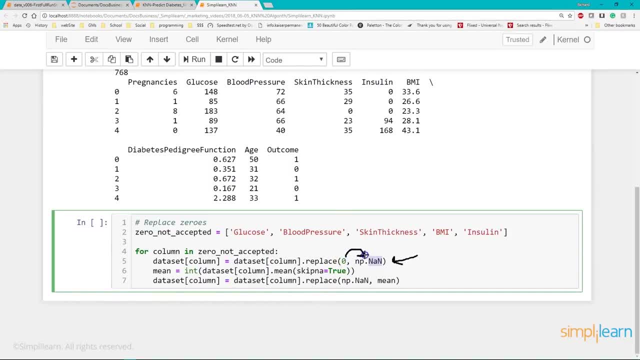 That's what this is saying right here. So put the zero in and we're going to replace zeros with no data. So if it's a zero, that means a person's well, hopefully not dead. Hopefully they just didn't get the data. 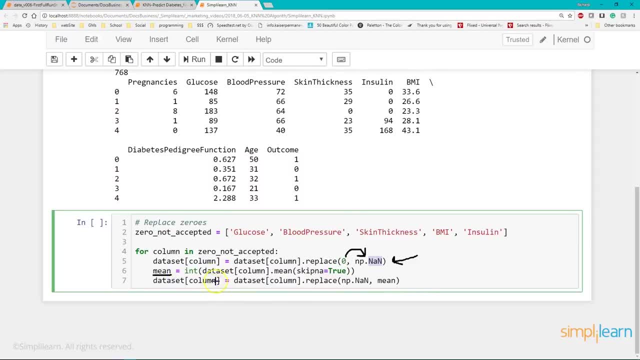 The next thing we want to do is we're going to create the mean, which is the integer from the data set, from the column Dot mean where we skip NAs. we can do that. That is a pandas command. there, the skip NA. 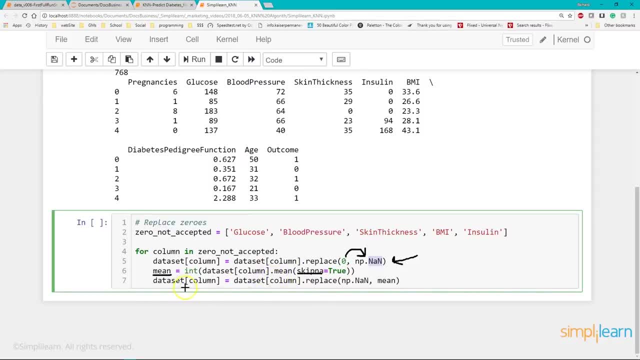 So we're going to figure out the mean of that data set And then we're going to take that data set column and we're going to replace all the NPNAN with the means. Why did we do that? We could have actually just taken this step and gone right down here and just 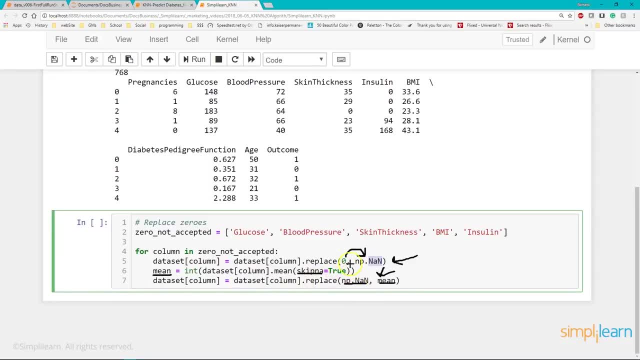 replace zero and skip anything. where except you could. actually, there's a way to skip zeros and then just replace all the zeros, But in this case we want to go ahead and do it this way, so you could see that we're switching this. 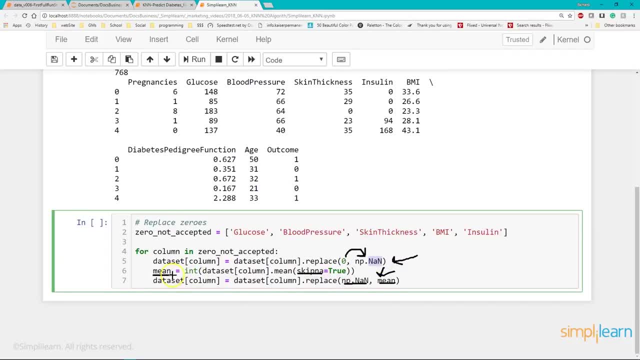 To a non-existent value, then we're going to create the mean. Well, this is the average person. So if we don't know what it is, if they did not get the data, the data is missing. One of the tricks is you replace it with the average. 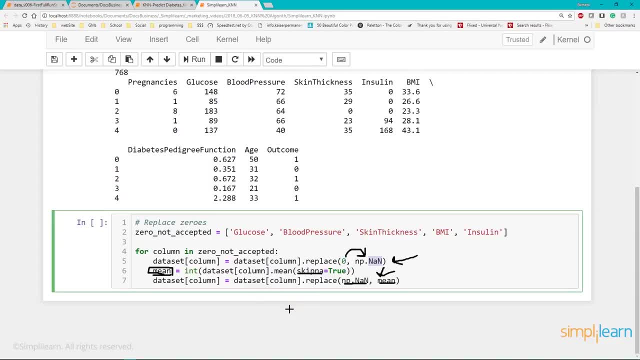 What is the most common data for that? This way you can still use the rest of those values to do your computation And it kind of just brings that particular value of those missing values out of the equation. Let's go ahead and take this and we'll go ahead and run it. 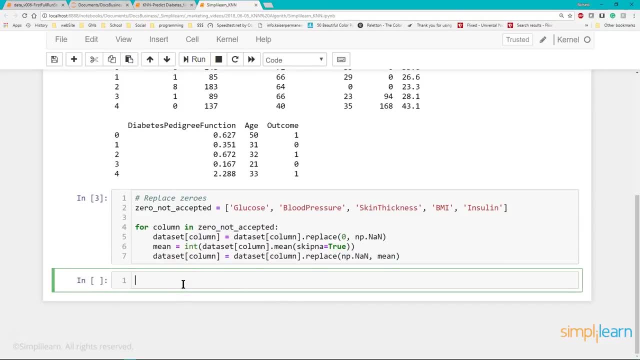 Doesn't actually do anything. We're still preparing our data. If you want to see what that looks like, we don't have anything in the first few lines, so it's not going to show up, but we certainly could look at a row. 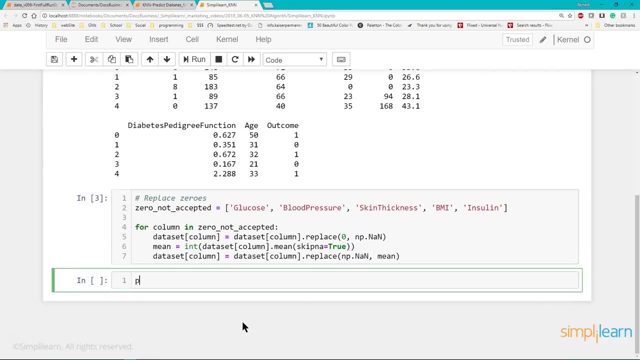 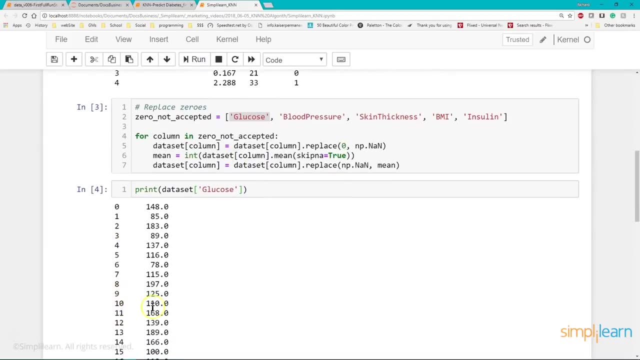 Let's do that. Let's go into our data set, Let's print a data set and let's pick- in this case, let's just do glucose- And if I run this, this is going to print all the different glucose levels going. 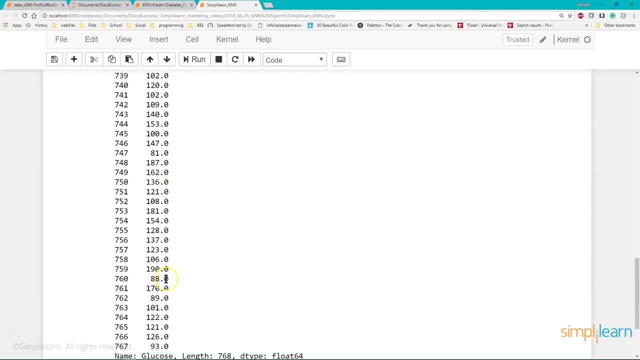 down and we thankfully don't see anything in here that looks like missing data. at least on the ones it shows You can see it skipped a bunch in the middle. That's what it does If we have too many lines in Jupyter Notebook. 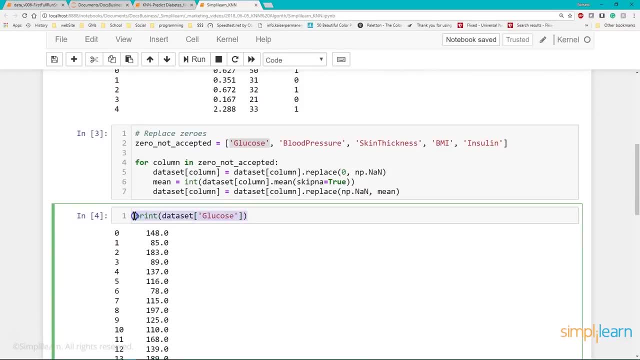 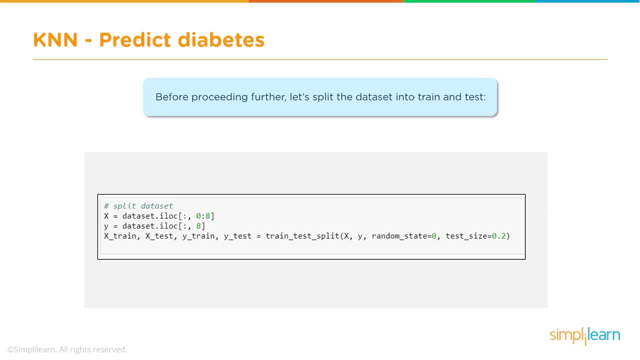 it'll skip a few and go on to the next in a data set. Let me go and remove this and we'll just zero out that. And, of course, before we do any processing, before proceeding any further, we need to split the data set into our train and testing data. 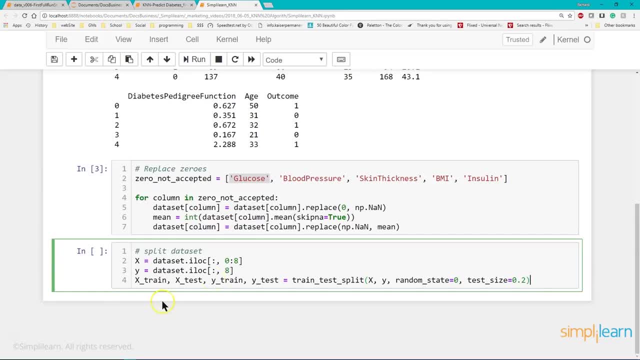 That way we have something to train it with and something to test it on. And you're going to notice, we did a little something here with the Pandas database code. There we go, my drawing tool. We've added in this right here, off the data set. 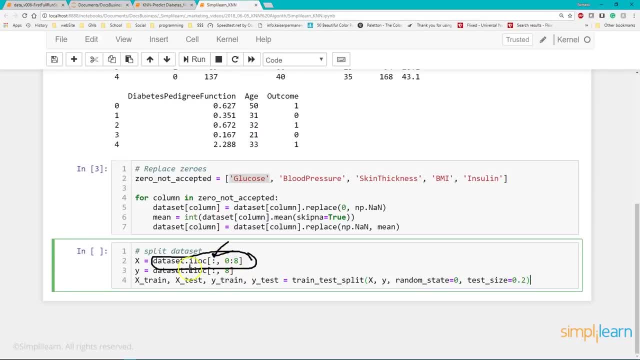 And what this says is that the first one in Pandas- this is from the PD Pandas- It's going to say, within the data set, we want to look at the eye location and it is all rows. That's what that says. 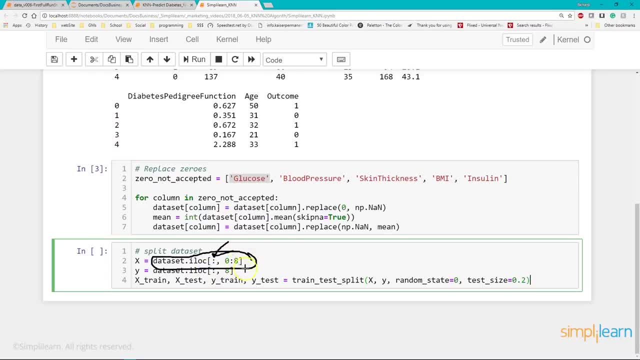 So we're going to keep all the rows, but we're only looking at zero, column zero to eight. Remember column nine? Here? it is right up here. We put it in here as outcome. Well, that's not part of the training data. 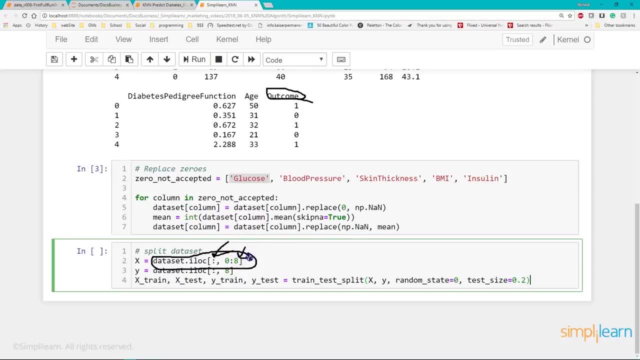 That's part of the answer. Yes, column nine, but it's listed as eight number eight. So zero to eight is nine columns. So eight is the value And when you see it in here, zero. this is actually zero to seven. 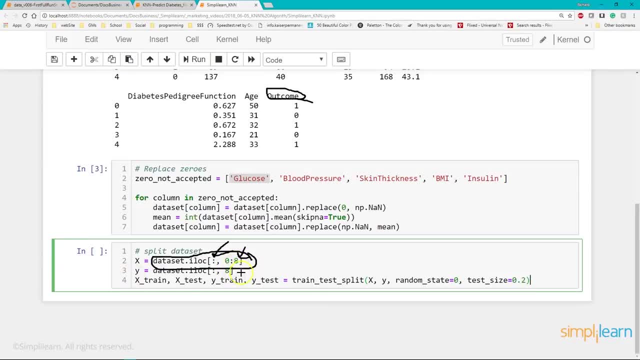 It doesn't include the last one. And then we go down here to Y, which is our answer, and we want just the last one, just column eight, And you can do it this way with this particular notation. And then, if you remember, we imported the train test split. 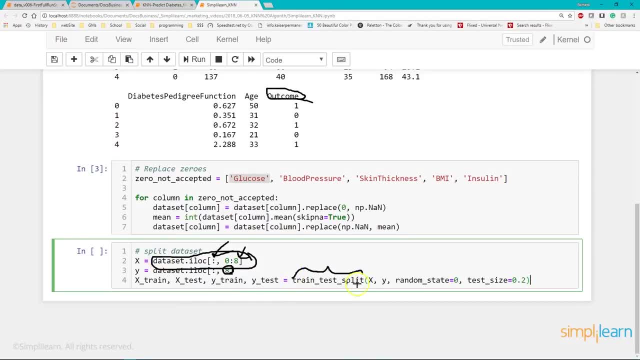 That's part of the SK. learn right there. And we simply put in our X and our Y. We're going to do random state equals zero. You don't have to necessarily seed it. That's a seed number. I think the default is one when you seed it. 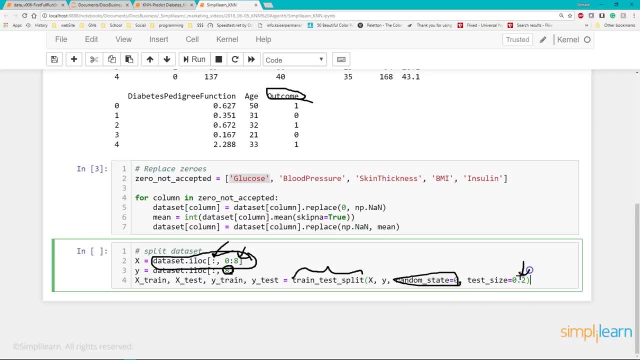 I have to look that up. And then the test size. test size is point two. That simply means we're going to take 20% of the data and put it aside so that we can test it later. That's all that is. 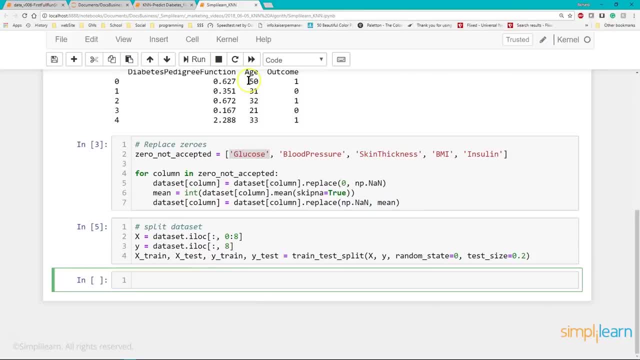 And again, we're going to run it. Not very exciting. So far we haven't had any printout other than to look at the data. But that is a lot of. this is prepping this data. Once you prep it, the actual lines of code are quick and easy. 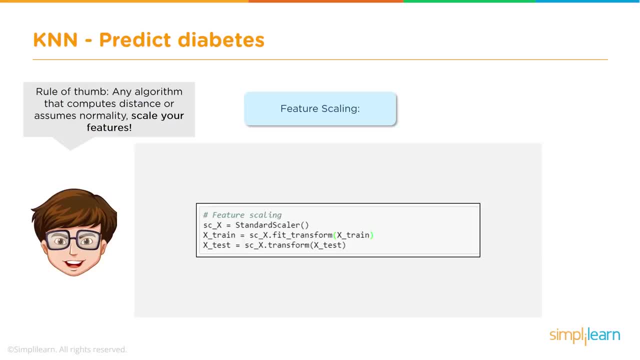 And we're almost there, But the actual running of our KNN. we need to go ahead and do a scale the data. If you remember correctly, we're fitting the data in a standard scalar, which means instead of the data being from five to three hundred and three in one column. 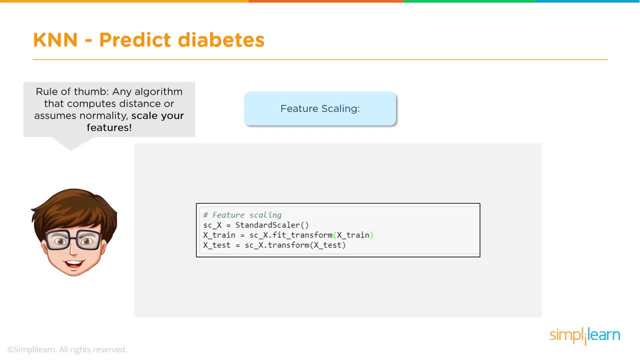 and the next column is one to six. we're going to set that all so that all the data is between minus one and one. That's what that standard scalar does, Keeps it standardized, And we only want to fit the scalar with the training set. 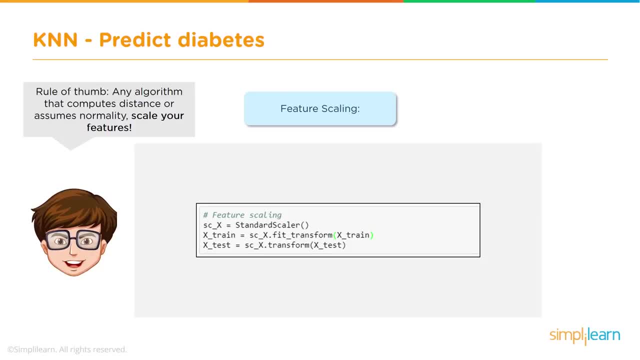 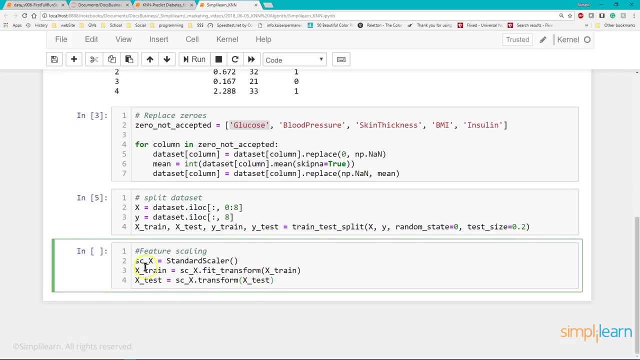 But we want to make sure the testing set is the X test going in is also transformed, So it's processing it the same. So here we go with our standard scalar. We're going to call it SC underscore X for the scalar And we're going to import the standard scalar into this variable. 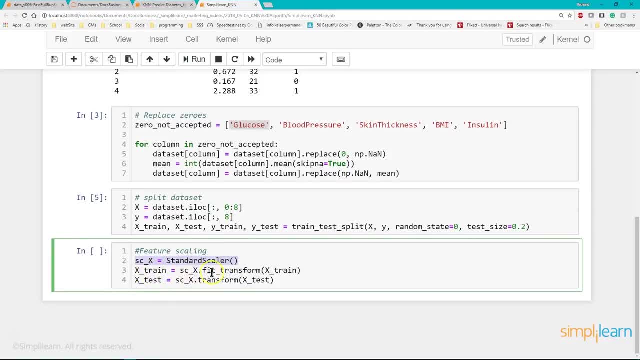 And then our X train equals SC, underscore X, dot, fit, transform. So we're creating the scalar on the X train variable And then our X test. we're also going to transform it. So we've trained and transformed the X train And then the X test isn't part of that training. 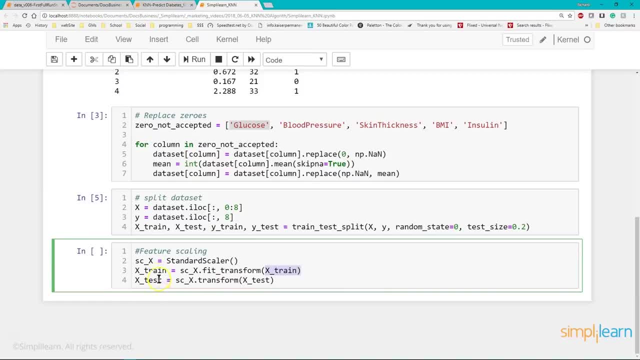 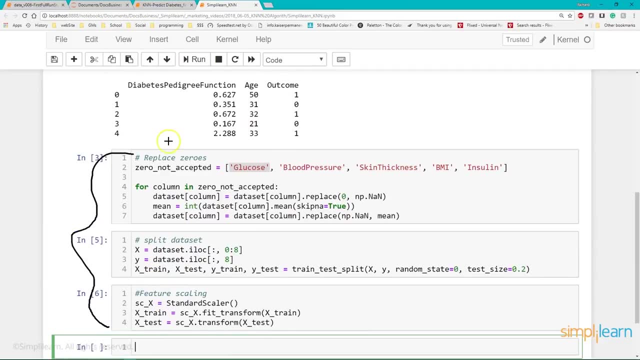 It isn't part of that training the transformer. It just gets transformed, That's all it does. And again, we're going to go and run this And if you look at this, we've now gone through these steps. all three of them, we've taken care of replacing our zeros. 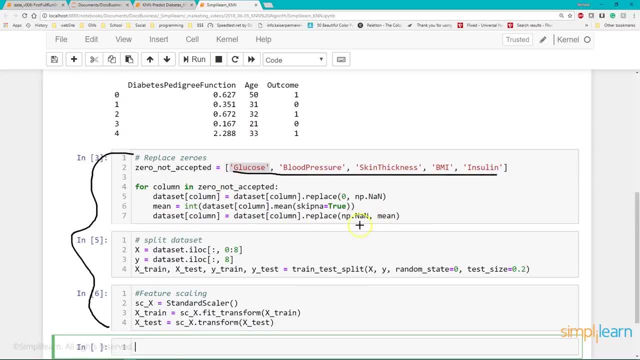 for key columns that shouldn't be zero and we replace that with the means of those columns, that way that they fit right in with our data models. We've come down here and we split the data, So now we have our test data and our training data. 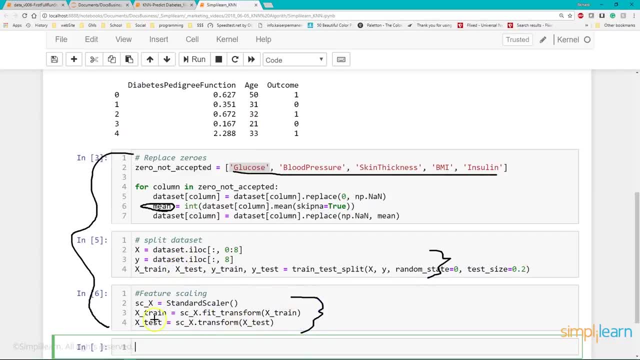 And then we've taken and we scaled the data. So all of our data going in. No, we don't. We don't train the Y part, the Y train and Y test. That never has to be trained, It's only the data going in. 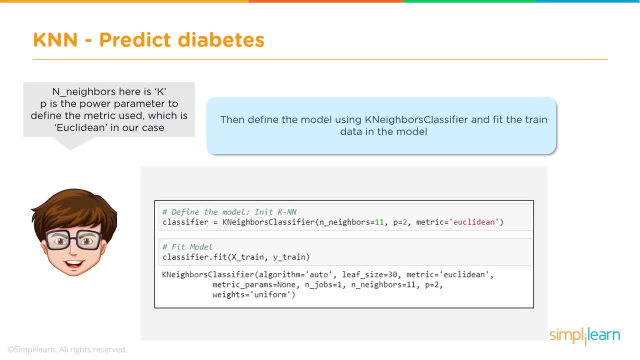 That's what we want to train in there. Then define the model using KNeighbors classifier and fit the train data in the model. So we do all that data prep and you can see down here we're only going to have a couple of lines of code where we're actually building our model and training it. 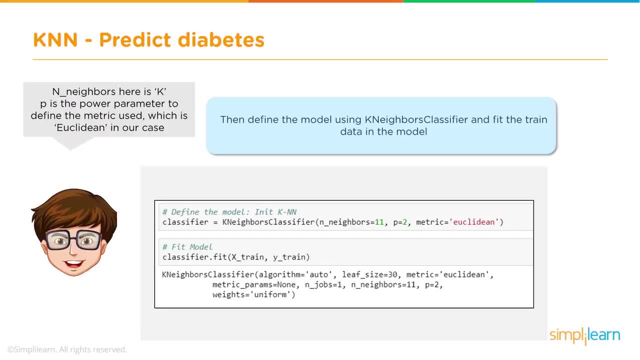 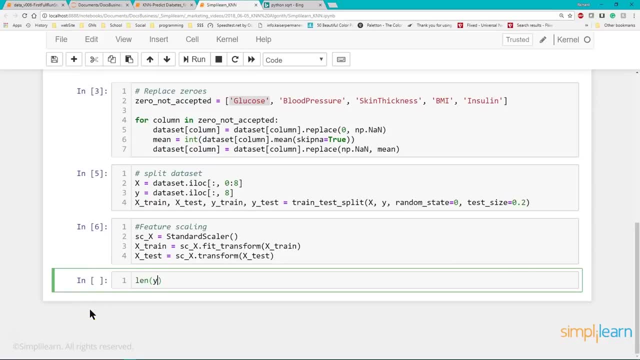 That's one of the cool things about Python and how far we've come. It's such an exciting time to be in machine learning because there's so many automated tools. Let's see before we do this. let's do a quick length of and let's do. 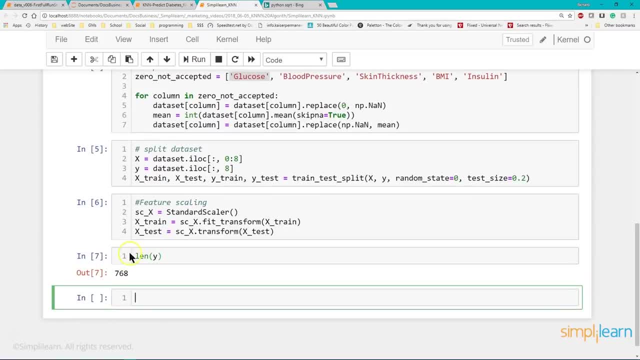 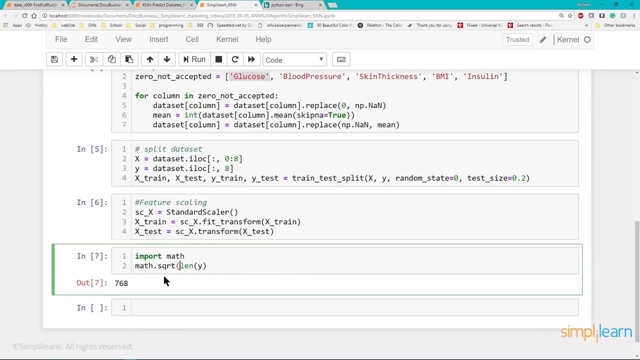 Y we want. let's just do length of Y and we get 768.. And if we import math, we do math, dot square root. Let's do Y train. There we go. It's actually supposed to be X train Before we do this, let's go ahead and do import math and do math square root length. 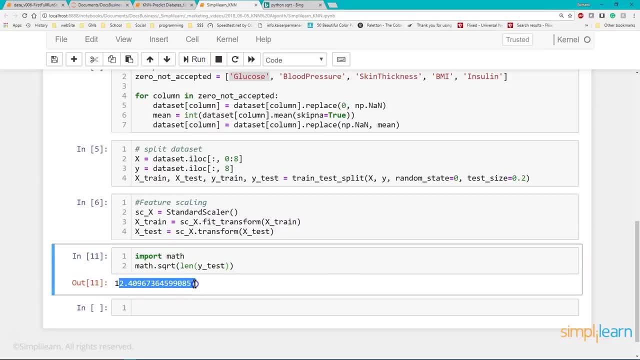 of Y test And when I run that, we get 12.409.. I want to show you where this number comes from. We're about to use. 12 is an even number. So if you know, if you're ever voting on things, remember the neighbors. 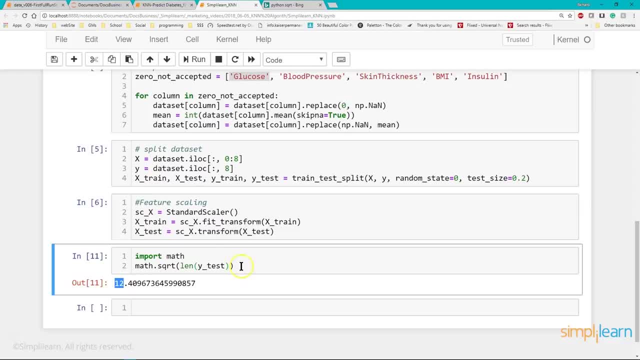 all vote. don't want to have an even number of neighbors voting, So we want to do something odd and let's just take one away. We'll make it 11.. Let me delete this out of here. That's one of the reasons I love Jupyter. 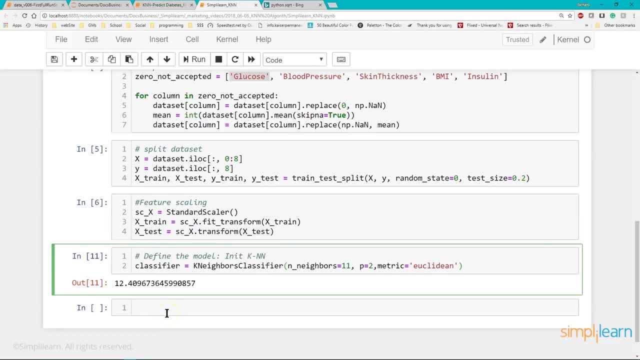 Notebook because you can flip around and do all kinds of things on the fly. So we'll go ahead and put in our classifier. We're creating our classifier now and it's going to be the K neighbors classifier N neighbors equal 11.. 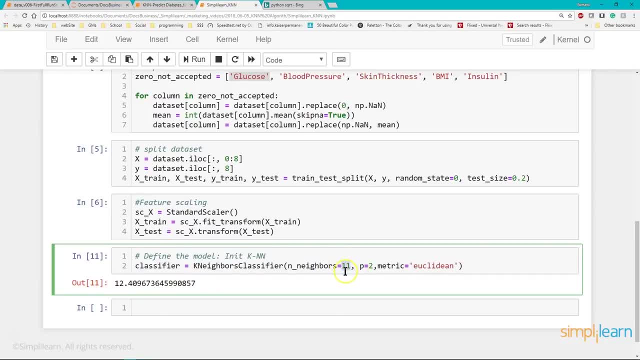 Remember we did 12 minus one for 11.. We have an odd number of neighbors. P equals two, because we're looking for is it are diabetic or not and we're using the Euclidean metric. There are other means of measuring the distance. 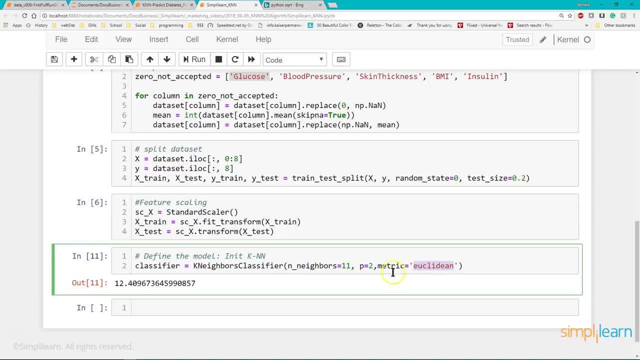 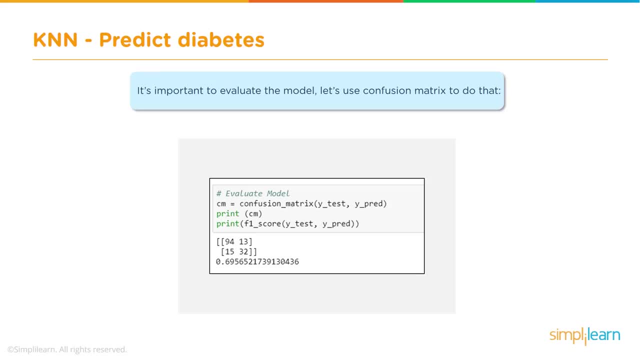 You could do like square. square means values, all kinds of measure this- But the Euclidean is the most common one and it works quite well. It's important to evaluate the model. Let's use the confusion matrix to do that, And we're going to use the confusion matrix. 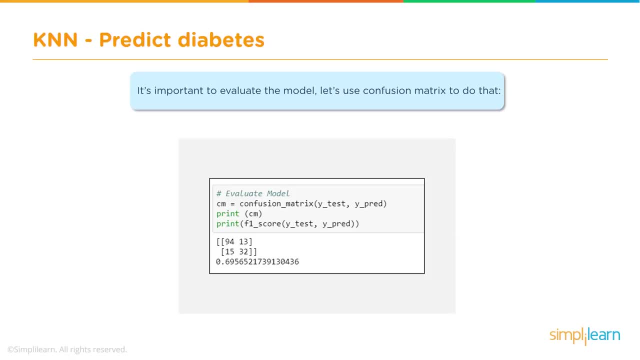 Wonderful tool. And then we'll jump into the F1 score and finally, accuracy score, which is probably the most commonly used quoted number when you go into a meeting or something like that. So let's go ahead and paste that in there And we'll set the CM equal to confusion matrix. 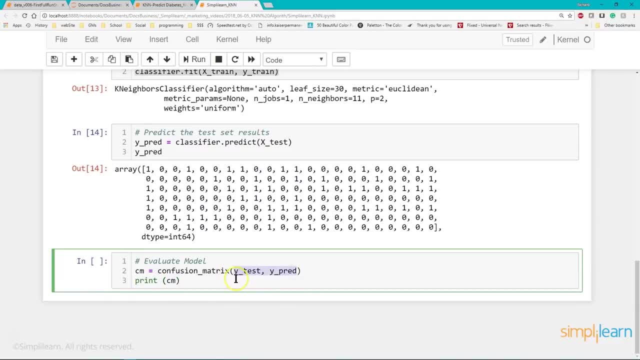 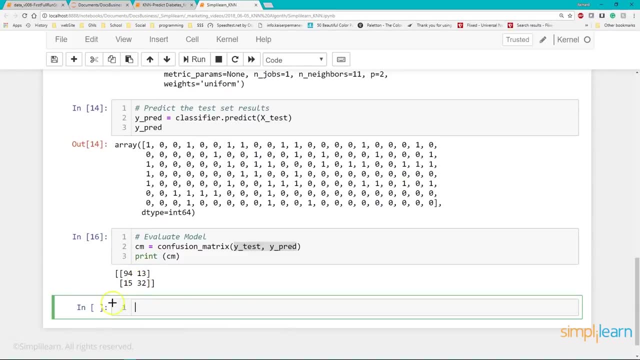 Why test? Why predict? So those are the two values we're going to put in there, And let me go and run that and print it out. And the way you interpret this is: you have the Y predicted, which would be your title up here. 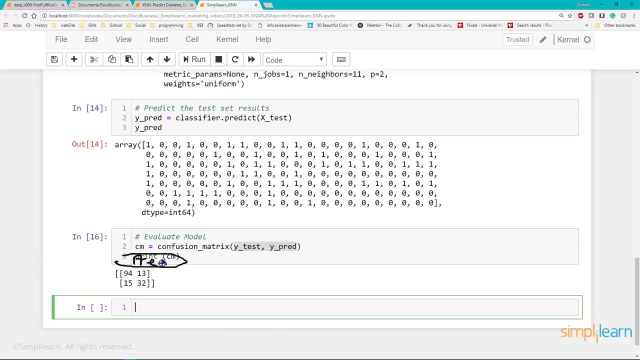 We could do this is to PRED predicted across the top and actual going down. Actual- It's always hard to write in here: Actual. That means that this column here down the middle, that's the important column and it means that our prediction said ninety four. 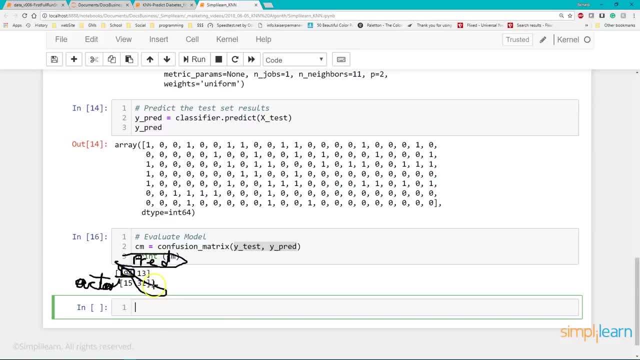 and prediction in the actual agreed on ninety four and thirty two. This number here the thirteen and the fifteen. Those are what was wrong. So you could have like three different, if you're looking at this, across three different variables instead of just two. you'd end up with a third row down here. 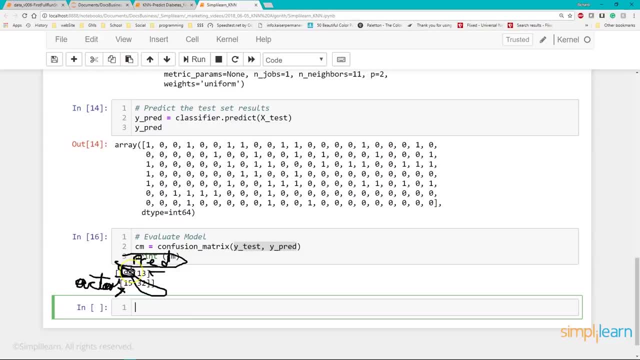 and that column going down the middle. So in the first case we have the, the and I believe the zero is a ninety four people who don't have diabetes. the prediction said that 13 of those people did have diabetes and were at high risk and the 32 that had diabetes that had correct. 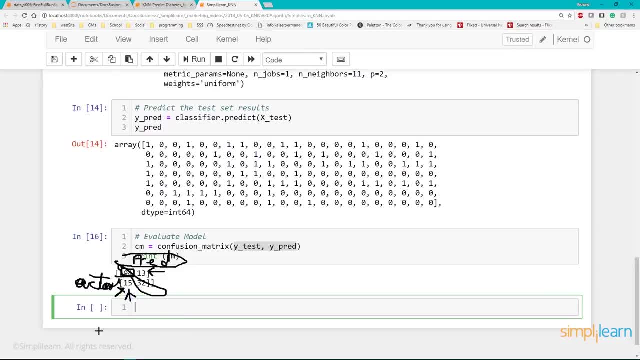 But our prediction said another 15 out of that 15.. It classified as incorrect, So you can see where that classification comes in and how that works on the confusion matrix. And then we're going to go ahead and print the F1 score. 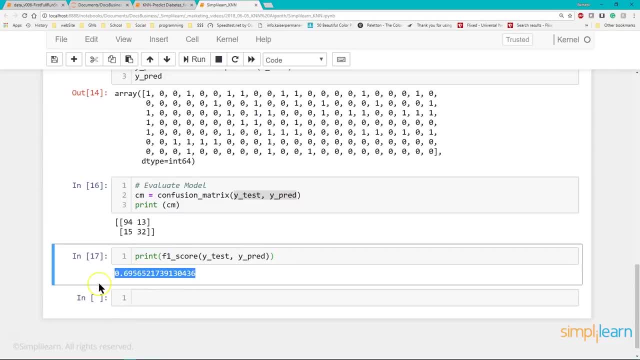 You just run that And you see we get a point six nine in our F1 score. The F1 takes into account both sides of the balance of false positives where, if we go ahead just to the accuracy account- and that's what most people think- 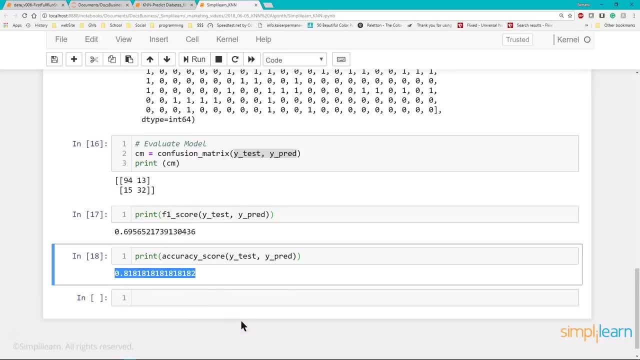 of is. it looks at just how many we got right out of how many we got wrong. So a lot of people, when you're a data scientist and you're talking to other data scientists, they're going to ask you what the F1 score, the F score, is. 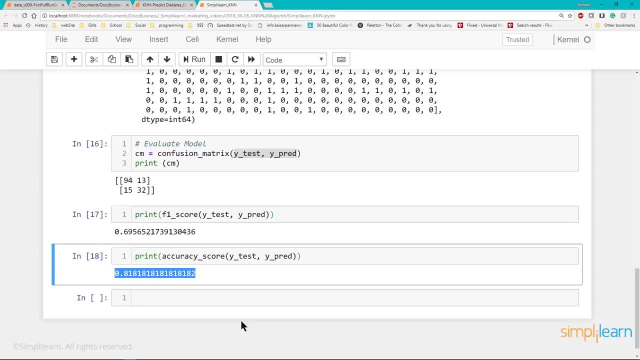 If you're talking to the general public or the decision makers in the business, they're going to ask what the accuracy is. And the accuracy is always better than the F1 score. But the F1 score is more telling. It lets us know that there's more false positives than we would like on here. 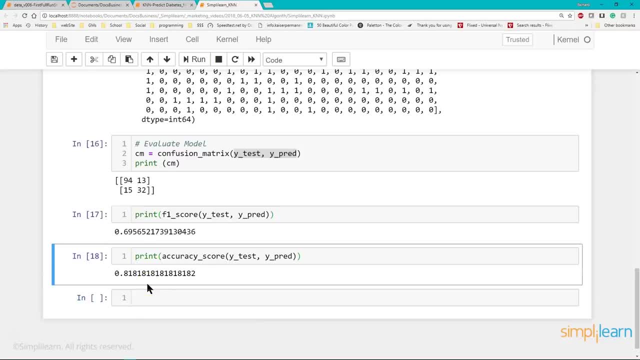 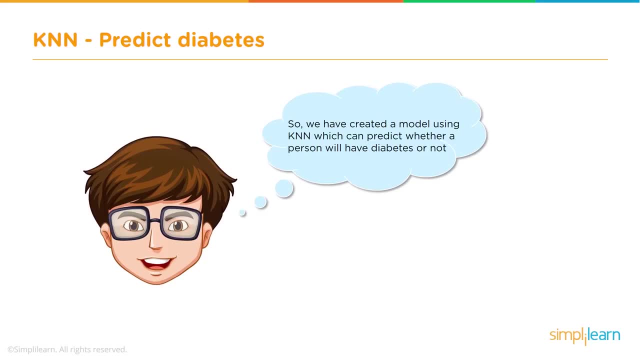 But 82 percent, not too bad for a quick flash. look at people's different statistics and running an SK Learn and running the KNN, the K nearest neighbor on it. So we have created a model using KNN which can predict whether a person will have diabetes or not. 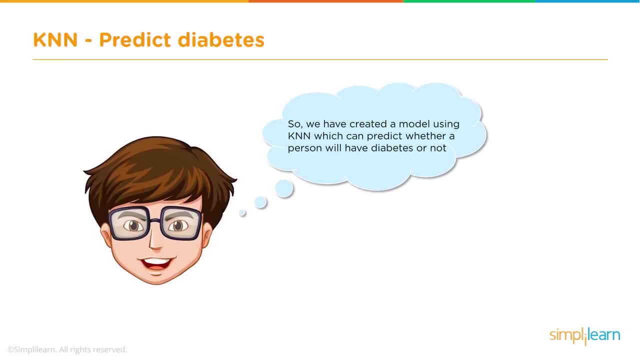 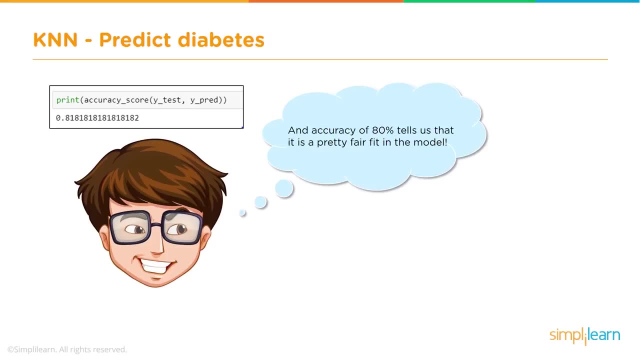 Or at the very least whether they should go get a checkup and have their glucose checked regularly or not. The print accuracy score: we got the point eight. one eight was pretty close to what we got and we can pretty much round that off and just say we have an accuracy of 80. 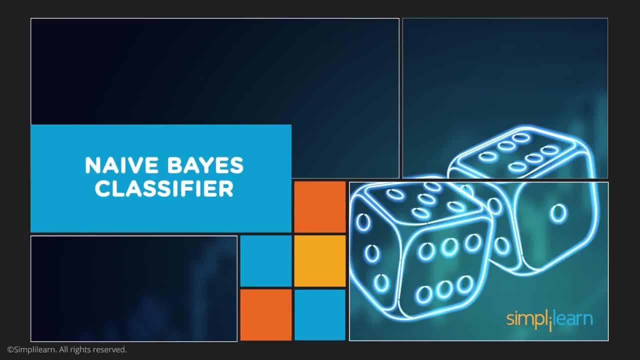 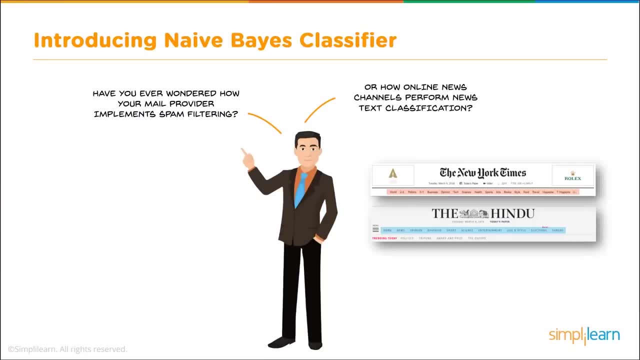 percent tells us it is a pretty fair fit in the model Introducing Naive Bayes Classifier. Have you ever wondered how your mail provider implements spam filtering, or how online news channels perform news text classification? or how companies perform sentimental analysis of their audience on social media? All of this and more is done through a 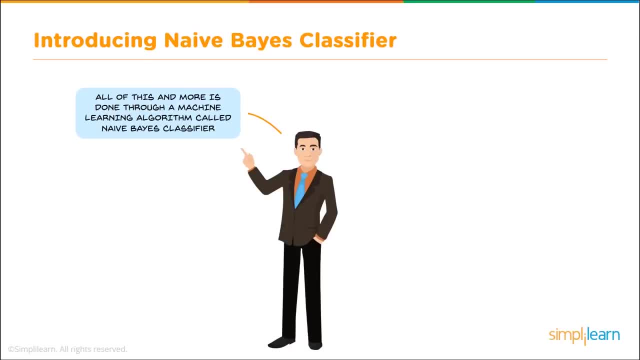 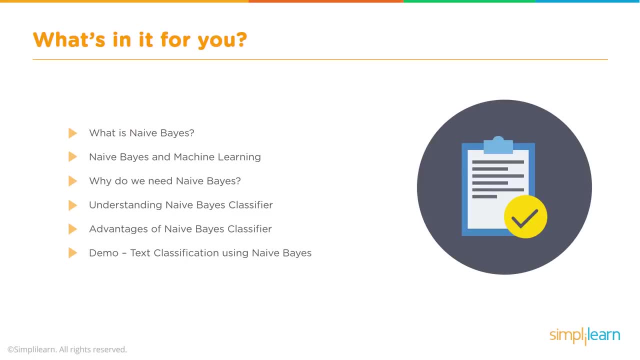 machine learning algorithm called Naive Bayes Classifier. We'll start with what is Naive Bayes, a basic overview of how it works. We'll get into Naive Bayes and machine learning, where it fits in with our other machine learning tools. Why do we need Naive Bayes? 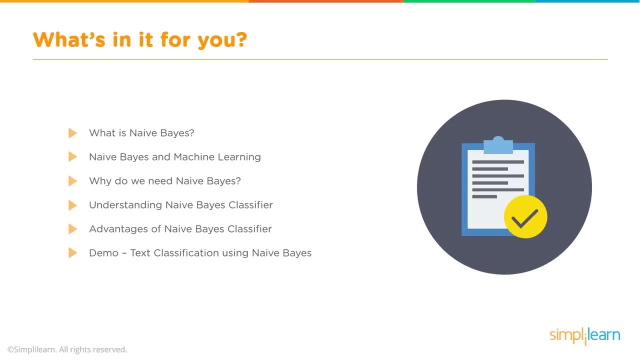 And understanding Naive Bayes Classifier a much more in-depth of how the math works in the background. Finally, we'll get into the advantages of the Naive Bayes Classifier in the machine learning setup, and then we'll roll up our sleeves and do my favorite part. We'll actually do some Python coding. 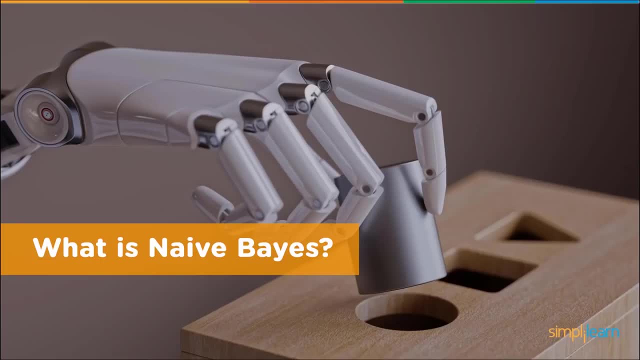 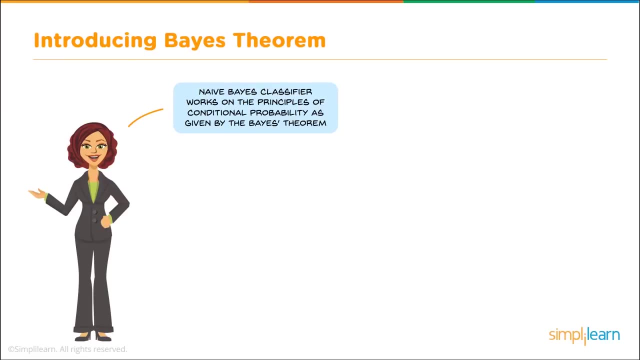 and do some text classification using the Naive Bayes. What is Naive Bayes? Let's start with a basic introduction to the Bayes theorem named after Thomas Bayes from the 1700s, who first coined this in the Western literature. 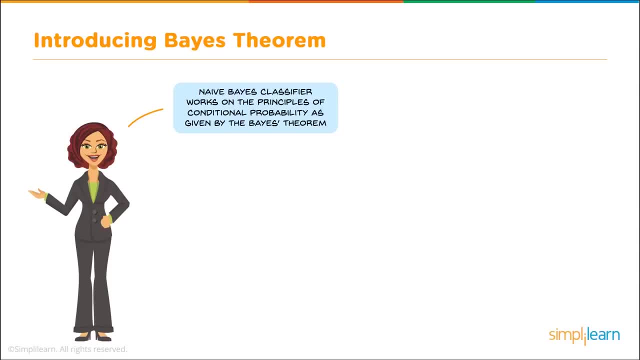 Naive Bayes Classifier works on the principle of conditional probability as given by the Bayes theorem. Before we move ahead, let us go through some of the simple concepts and the probability that we will be using. Let us consider the following example of tossing two coins. 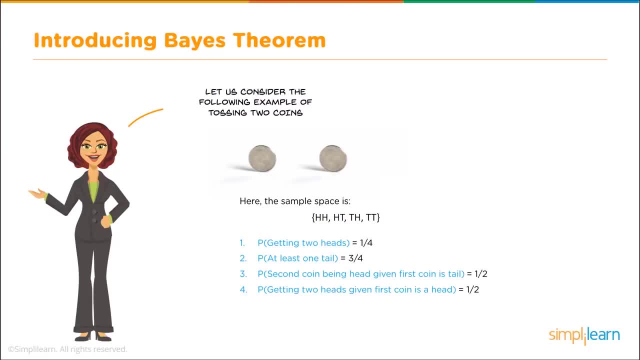 Here we have two quarters and if we look at all the different possibilities of what they can come up as, we get that they can come up as head-heads, come up as head-tell, tell-head and tell-tell. When doing the math on probability, we usually denote probability as a P. 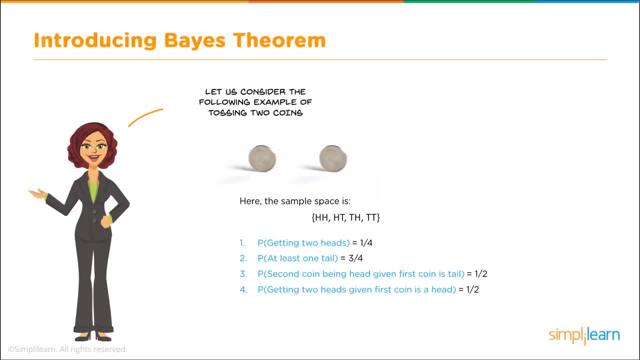 a capital P. So the probability of getting two heads equals one fourth. You can see on our data set we have two heads and this occurs once out of the four possibilities. And then the probability of at least one tell occurs three quarters of the time. You'll see on three of the coin tosses. 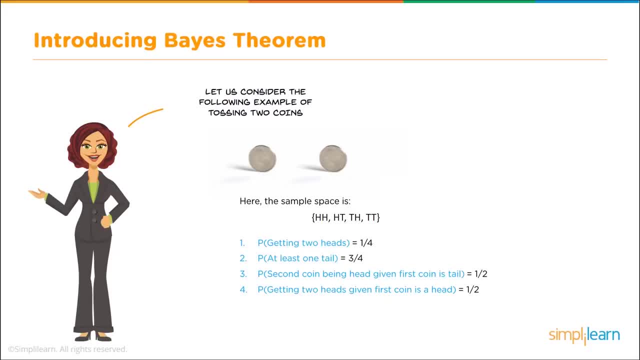 we have tells in them And out of four that's three fourths. And then the probability of the second coin being head, given the first coin is tell, is one half. And the probability of getting two heads, given the first coin is a head, is one half. 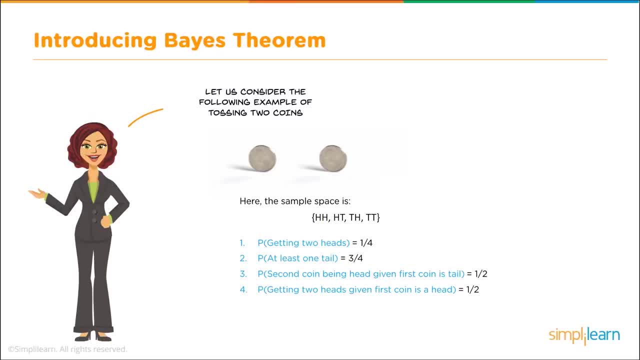 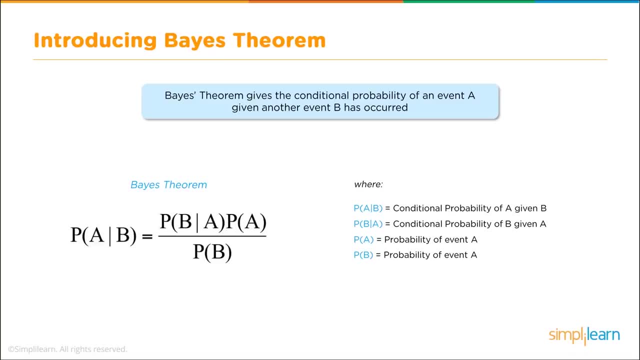 We'll demonstrate that in just a minute and show you how that math works Now. when we're doing it with two coins, it's easy to see, but when you have something more complex, you can see where these formulas really come in and work. 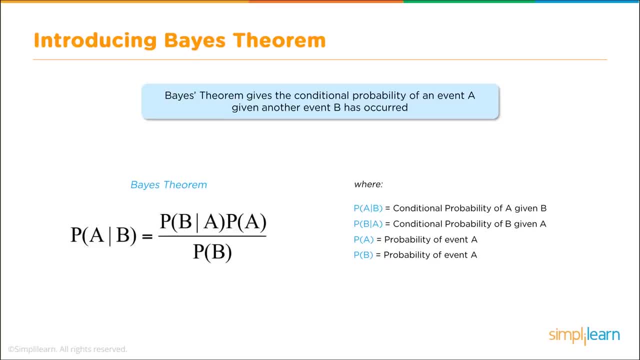 So the Bayes theorem gives us the conditional probability of an event A given another event B has occurred. In this case, the first coin toss will be B and the second coin toss A. This could be confusing, because we've actually reversed the order of them and go from B to A instead of A to B. 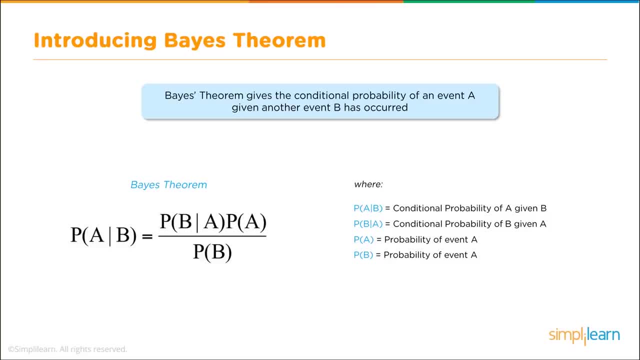 You'll see this a lot when you work in probabilities. The reason is: we're looking for event A, We want to know what that is, So we're going to label that A, since that's our focus, And then, given another event B has occurred In the Bayes theorem. 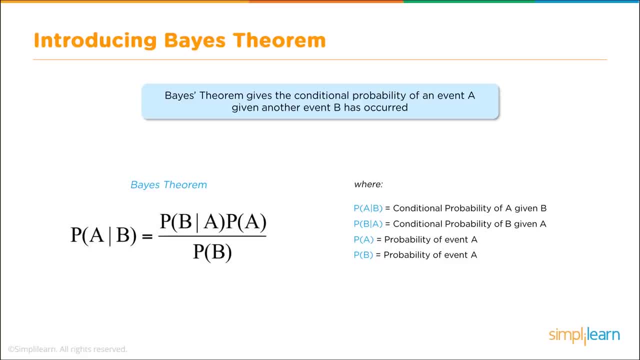 as you can see on the left, the probability of A occurring, given B has occurred equals the probability of B occurring, given A has occurred, times the probability of A over the probability of B. This simple formula can be moved around just like any algebra formula. 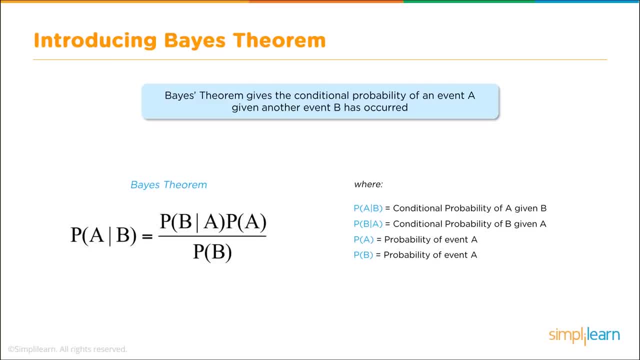 And we could do: the probability of A after a given B times probability of B equals the probability of B given A times probability of A. You can easily move that around and multiply it and divide it out. Let us apply Bayes theorem to our example. 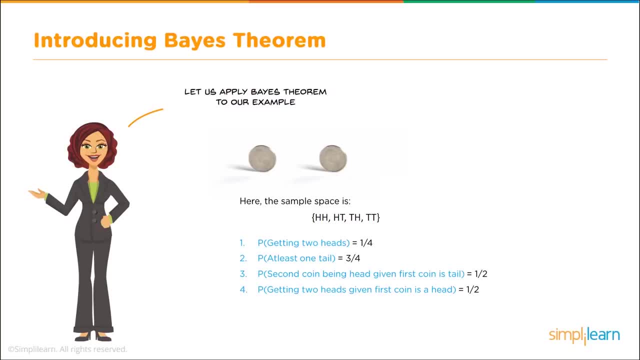 Here we have our two quarters and we'll notice that the first two probabilities of getting two heads and at least one tail we compute directly off the data. So you can easily see that we have one example HH out of four, one fourth. 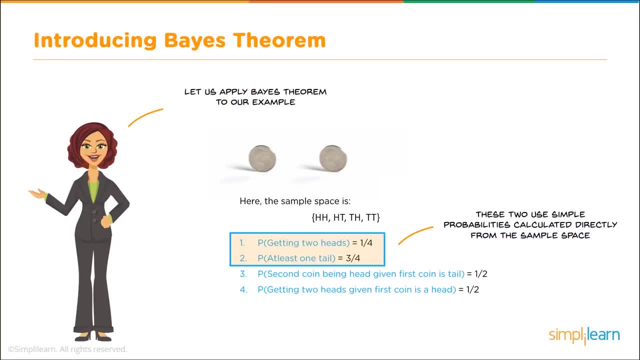 And we have three with tails in them, giving us three quarters or three fourths, 75 percent. The second condition, the second set, three and four. We're going to explore a little bit more in detail Now. we stick to a simple example with two coins because you can easily understand the math. 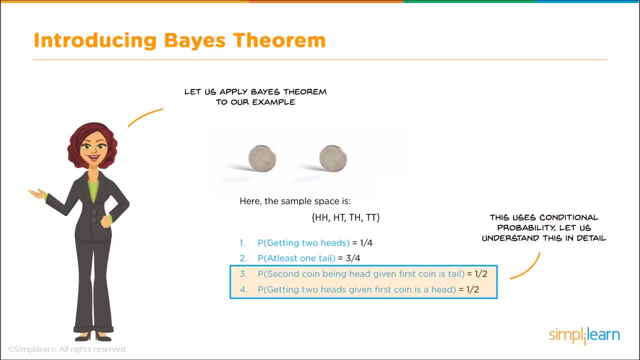 The probability of throwing a tail doesn't matter what comes before it, And the same with the heads. It's going to be 50 percent or one half. But when that probability gets more complicated- let's say you have a D6 dice or some other instance- then this formula really comes in handy. 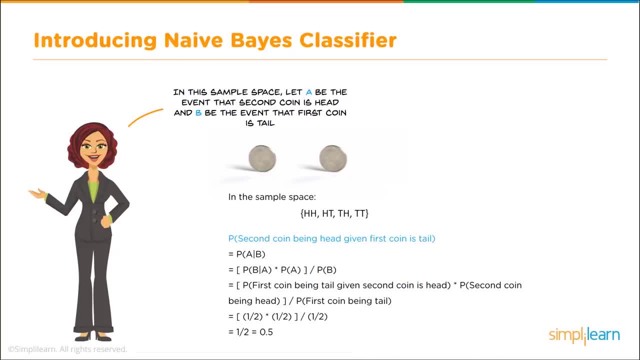 But let's stick to the simple example for now, In this sample space, let A be the event that the second coin is head and B be the event that the first coin is tails. Again, we reversed it because we want to know what the second event is going to be. 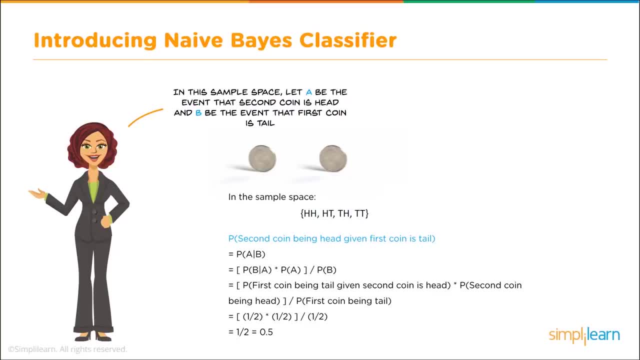 So we're going to be focusing on A And we write that out as the probability of A given B And we know this from our formula, that that equals the probability of B given A times the probability of A over the probability of B. And when we plug that in, we plug in the probability of the first coin being tails. 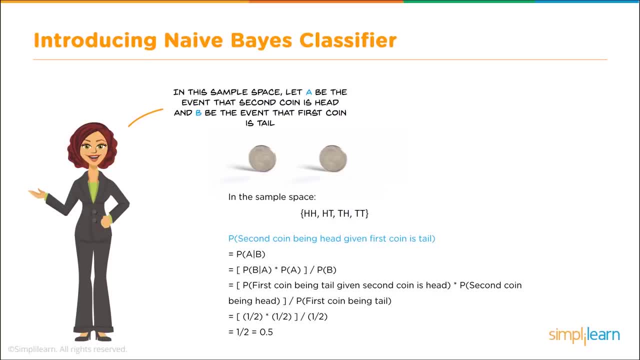 given the second coin is heads, and the probability of the second coin being heads, given the first coin being over the probability of the first coin being tails. When we plug that data in and we have the probability of the first coin being tails, given the second coin is heads, times the probability of the second coin being heads. 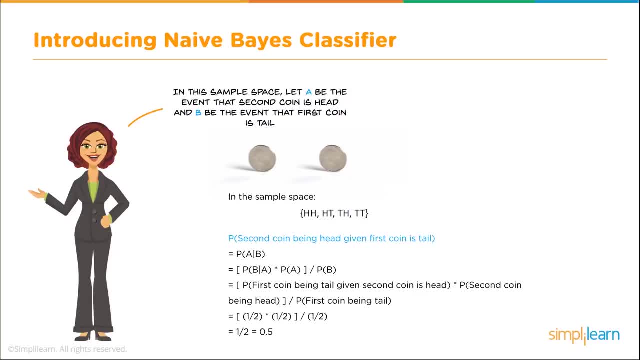 over the probability of the first coin being tails. You can see it's a simple formula to calculate: Half times one, half over one half, or one half equals point five or one fourth. So the Bayes theorem basically calculates the conditional probability of the occurrence. 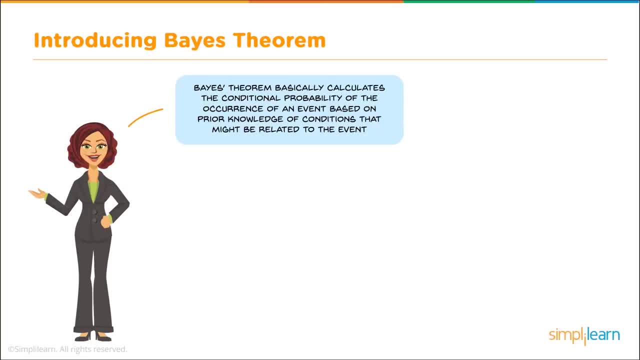 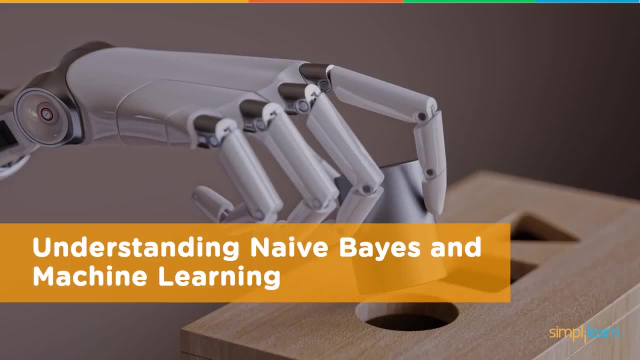 of an event based on prior knowledge of conditions that might be related to the event. We will explore this in detail when we take up an example of online shopping further in this tutorial, Understanding naive Bayes and machine learning Like with any of our other machine learning. 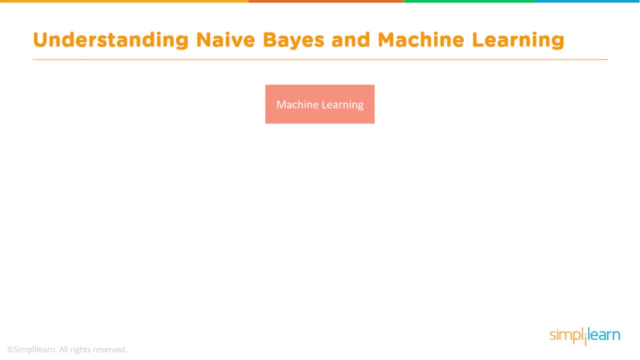 tools. it's important to understand where the naive Bayes fits in the hierarchy. So under the machine Learning we have supervised learning and there is other things like unsupervised learning is also reward system. This falls under the supervised learning and then under the supervised learning. 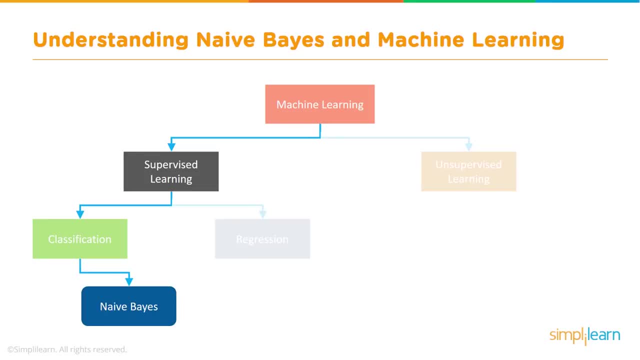 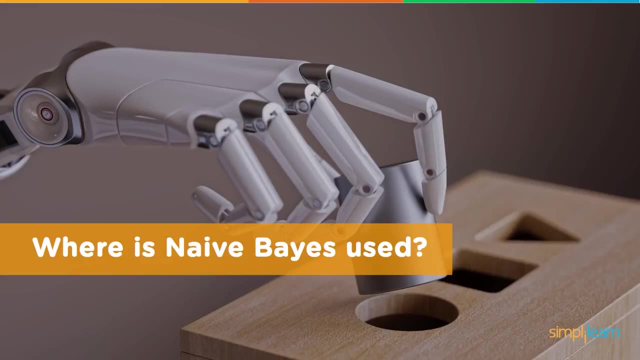 There's classification, There's also regression, but we're going to be in the classification side. And then under classification is your naive Bayes. Let's go ahead and glance into where is naive Bayes used? Let's look at some of the use scenarios for it as a classifier. 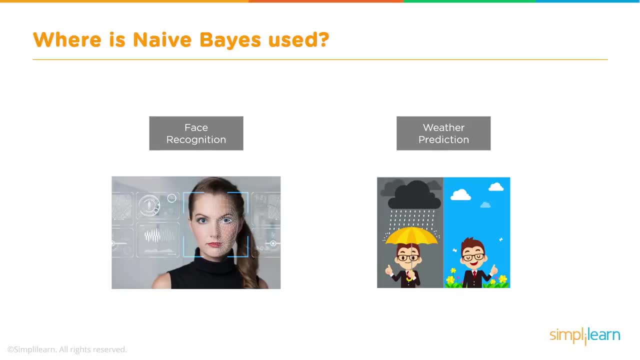 We use it in face recognition: Is this Cindy, or is it not Cindy, or whoever? Or it might be used to identify parts of the face that they then feed into another part of the face recognition program. This is the eye, This is the nose, This is the mouth. 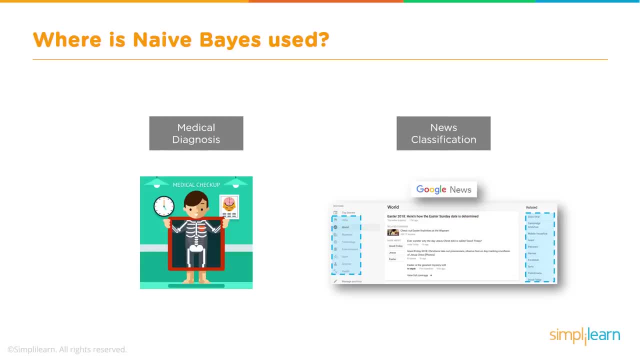 Weather prediction- Is it going to be rainy or sunny? Medical recognition News prediction. It's also used in medical diagnosis. We might diagnose somebody as either as high risk or not as high risk for cancer or heart disease or other ailments, and news classification. 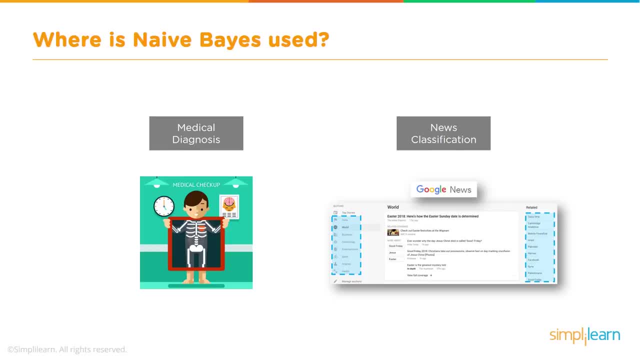 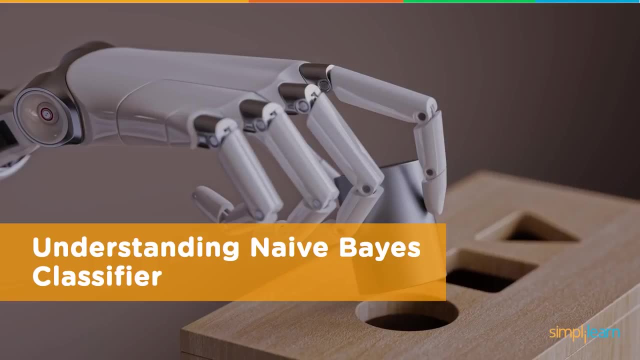 You look at the Google News and it says: well, is this political or is this world news, Or A lot of that's all done with a naive Bayes Understanding naive Bayes classifier. Now, we already went through a basic understanding with the coins and the two. 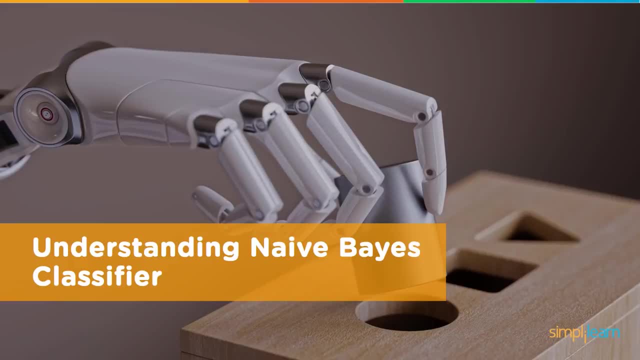 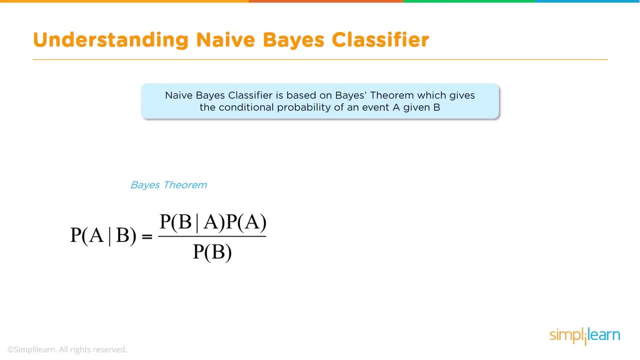 heads and two tails, and head, tail, tail heads, et cetera. We're going to do just a quick review on that and remind you that the naive Bayes classifier is based on the Bayes theorem, which gives a conditional probability of event A given event B, And that's where the probability of A given B equals. 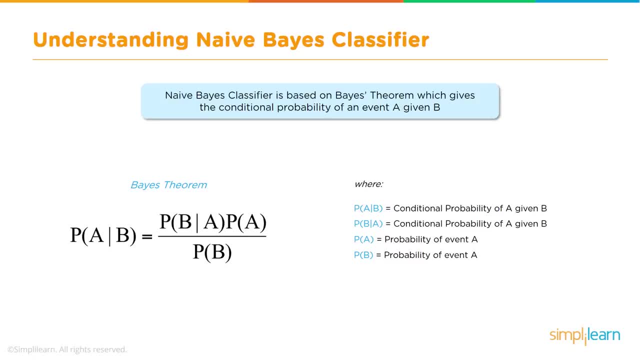 the probability of B, given A times probability of A Over probability of B. Remember, this is an algebraic function so we can move these different entities around. We can multiply by the probability of B, So it goes to the left hand side, and then we could divide by the probability of A. 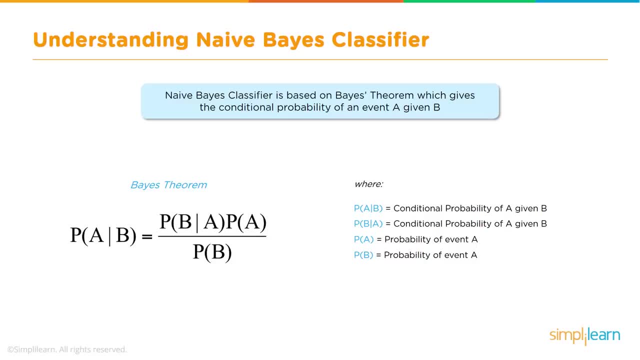 given B and just as easily come up with a new formula for the probability of B. To me, staring at these algebraic functions kind of gives me a slight headache. It's a lot better to see if we can actually understand how this data fits. 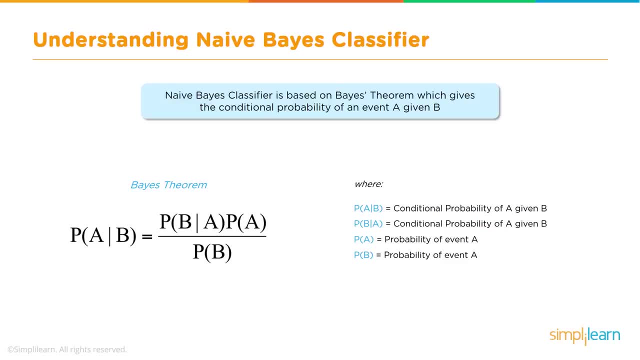 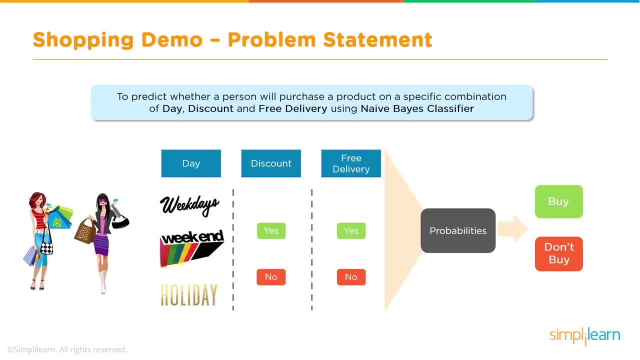 together in a table and let's go ahead and start applying it to some actual data so you can see what that looks like. So we're going to start with The shopping demo problem statement and remember we're going to solve this first in table form so you can see what the math looks like, and then we're going to solve. 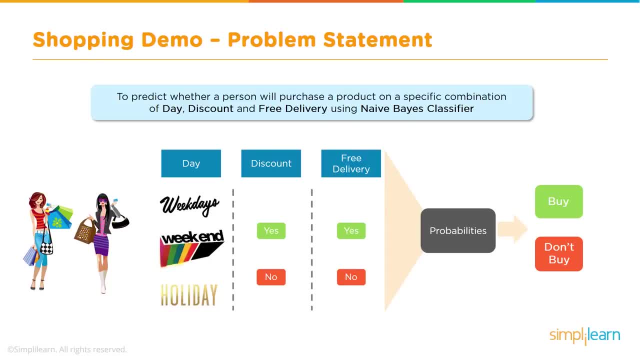 it in Python And in here we want to predict whether the person will purchase a product. Are they going to buy or don't buy? Very important: if you're running a business, you want to know how to maximize your profits or at least maximize the purchase of the people coming into your 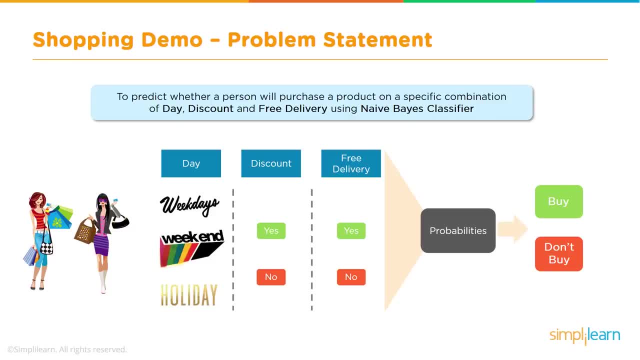 store And we're going to look at a specific combination of different variables. In this case we're going to look at the day, the discount and the free delivery And you can see here under the day. we want to know whether it's on the weekday, you know somebody is working. 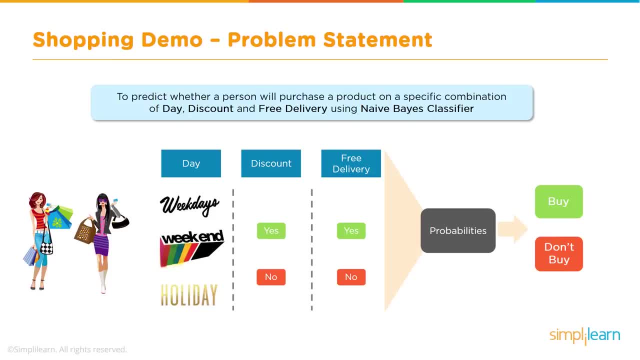 They come in after work, or maybe they don't work Weekend. you can see the bright colors coming down there celebrating not being in work or holiday. And did we offer a discount that day, Yes or no? Did we offer free delivery that day? Yes or no? 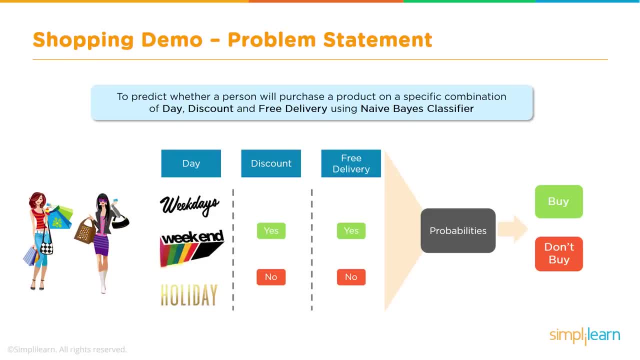 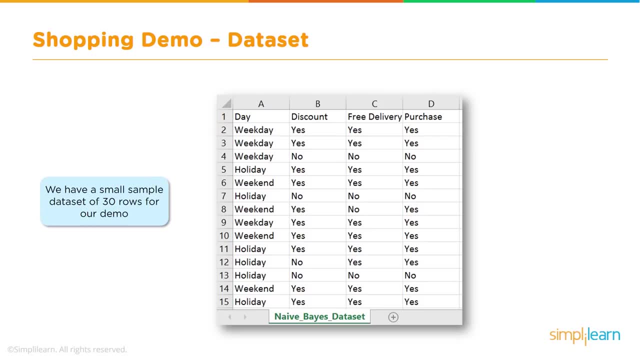 And from this we want to know whether the person is going to buy based on these traits, so we can maximize them and find out the best system for getting somebody to come in and purchase our goods and products from our store. Now, having a nice visual is great, but we do need to dig into the data. 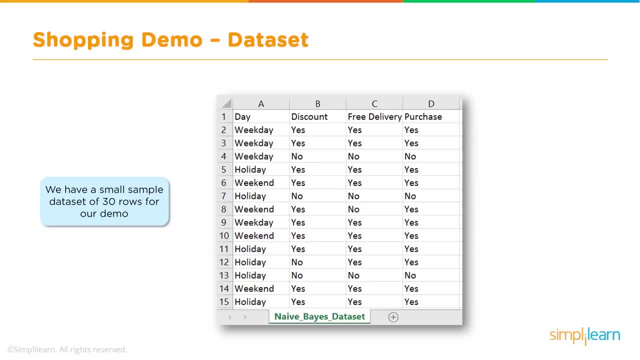 So let's go ahead. Take a look at the data set. We have a small sample data set of 30 rows. We're showing you the first 15 of those rows for this demo. Now the actual data file you can request. 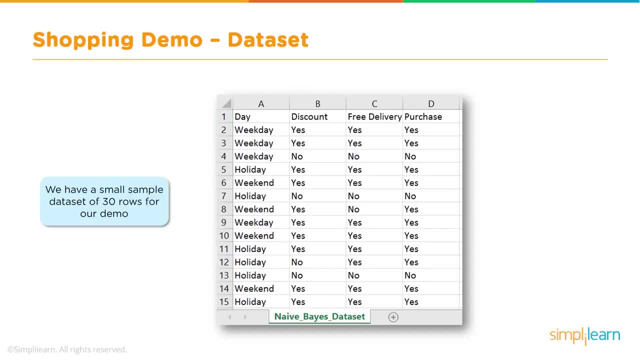 Just type in below under the comments on the YouTube video and we'll send you some more information and send you that file. As you can see here, the file is very simple: columns and rows. We have the day, the discount, the free delivery, and did the person purchase or not? 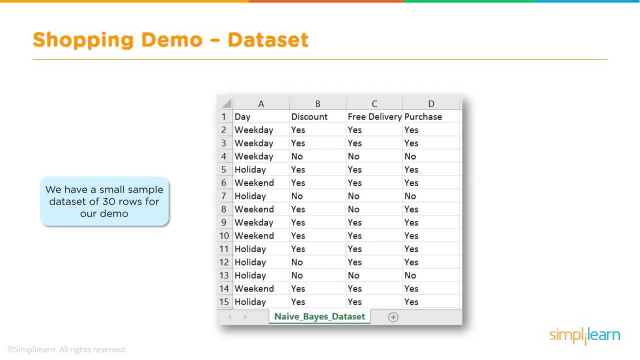 And then we have under the day whether it was a weekday, a holiday, was it the weekend? This is a pretty simple set of data And long before computers, people used to look at this data and calculate this all by hand. So let's go ahead and walk through this. 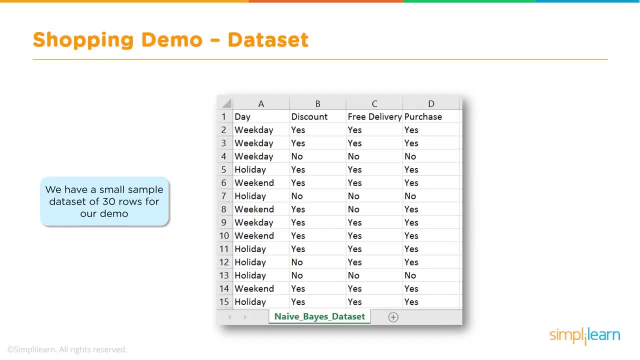 and see what that looks like when we put that into tables. Also note: in today's world we're not usually looking at three different variables in 30 rows. nowadays, because we're able to collect data so much, We're usually looking at twenty, seven, thirty variables across hundreds of rows. 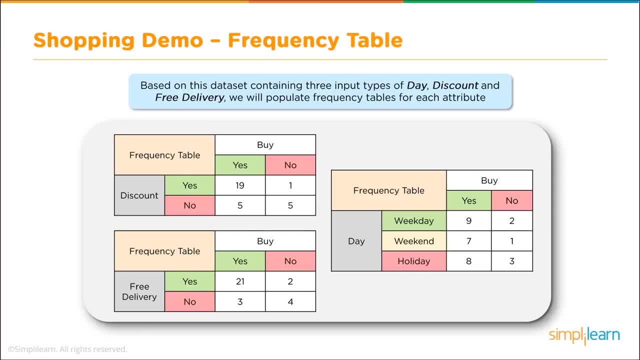 The first thing we want to do is we're going to take this data and, based on the data set containing our three inputs- day, discount and free delivery- we're going to go ahead and populate that to frequency tables for each attribute. So we want to know if they had a discount. 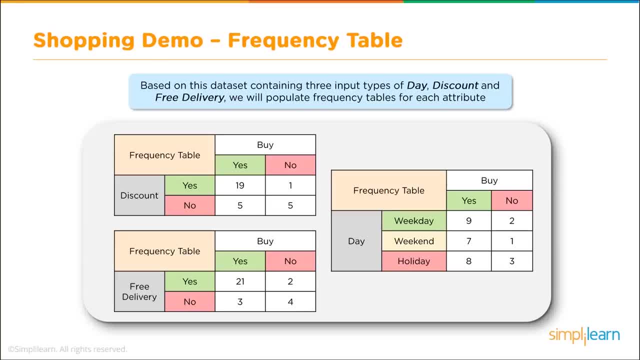 How many people buy and did not buy? Did they have a discount, Yes or no? Do we have a free delivery, Yes or no? On those days, how many people made a purchase, How many people didn't? And the same with the three days of the week. 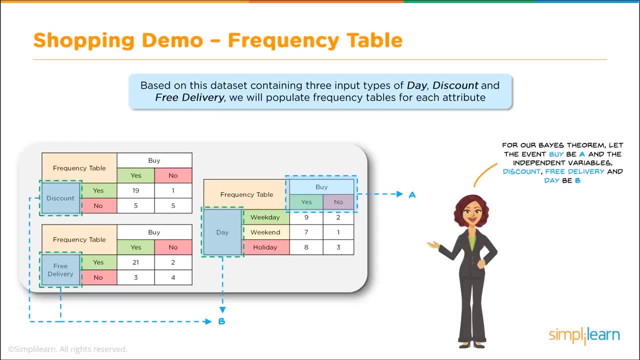 Was it a weekday, a weekend, a holiday? And did they buy, Yes or no? As we dig in deeper to this table for our Bayes theorem, let the event buy be A Remember. we looked at the coins. I said we really want to know what the outcome is. 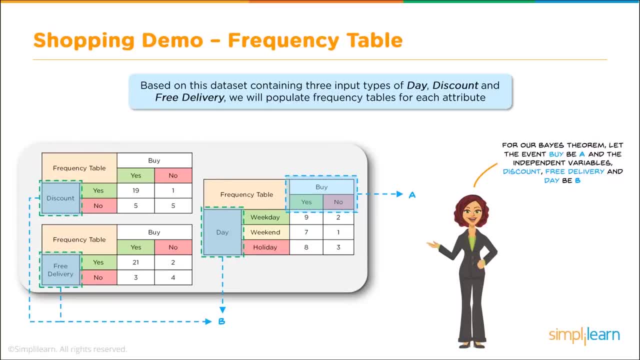 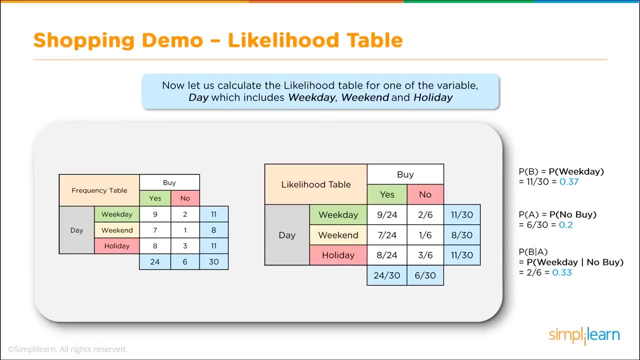 Did the person buy or not, And that's usually event. A is what you're looking for, And the independent variables- discount, free delivery and day be B, So we'll call that probability of B. Now let us calculate the likelihood table for one of the variables. 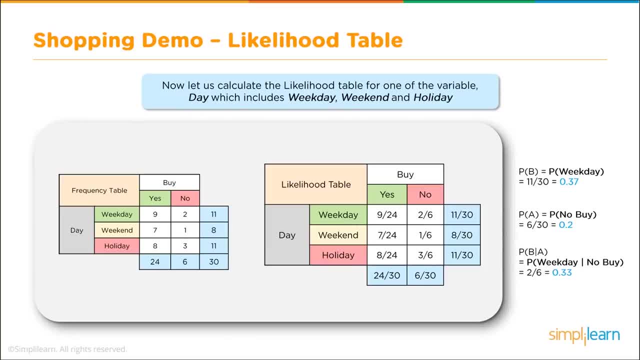 Let's start with day, which includes weekday, weekend and holiday, And let us start by summing all of our rows. So we have the weekday row and out of the weekdays there's nine plus two, So it's eleven weekdays. There's eight weekend days and eleven holidays. 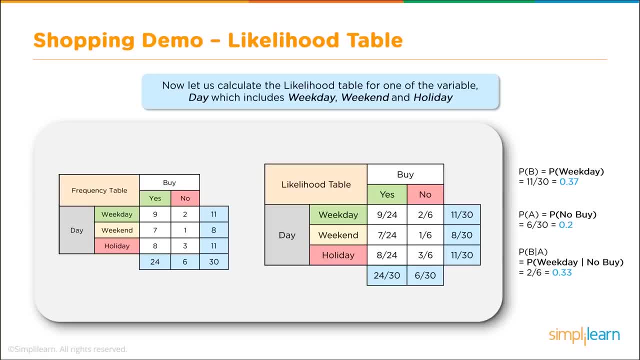 That's a lot of holidays, And then we want to sum up the total number of days, So we're looking at a total of 30 days. Let's start pulling some information from our chart and see where that takes us And when we fill in the chart on the right. 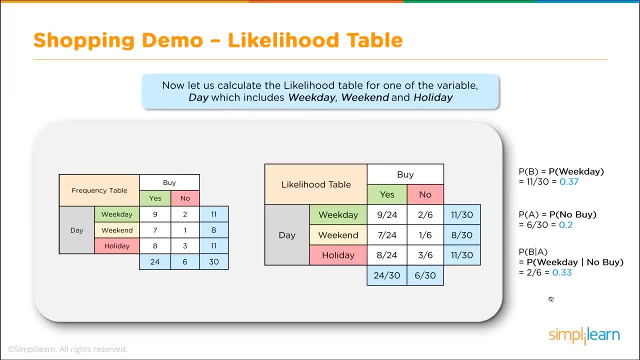 you can see that nine out of 24 purchases are made on the weekday, seven out of 24 purchases on the weekend and eight out of 24 purchases on a holiday. And, out of all the people who come in, 24 out of 30 purchase. 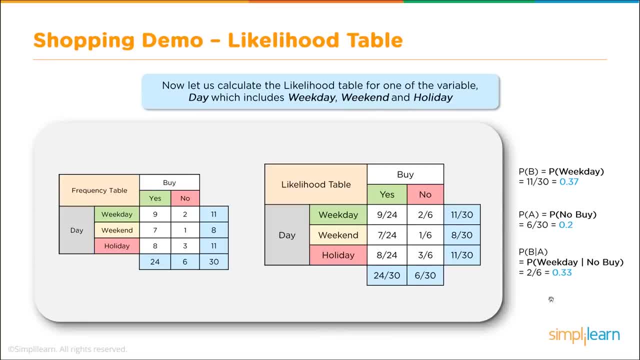 You can also see how many people do not purchase on the weekday. It's two out of six didn't purchase, and so on and so on. We can also look at the totals and you'll see. on the right, We put together some of the formulas. 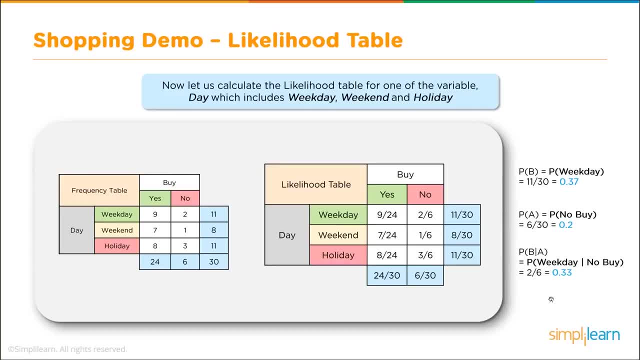 The probability of making a purchase on the weekend comes out 11 out of 30. So out of the 30 people who came into the store throughout the weekend, weekday and holiday, 11 of those purchases were made on the weekday. And then you can also see the probability of them not making a purchase. 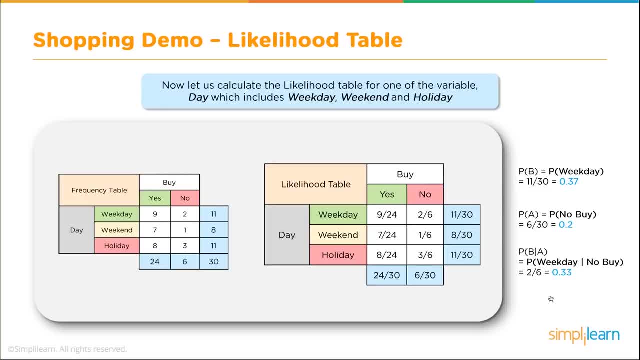 And this is done for doesn't matter which day of the week. So we call that probability: no buy would be six over 30, or point two. So there's a 20 percent chance that they're not going to make a purchase, no matter what day of the week it is. 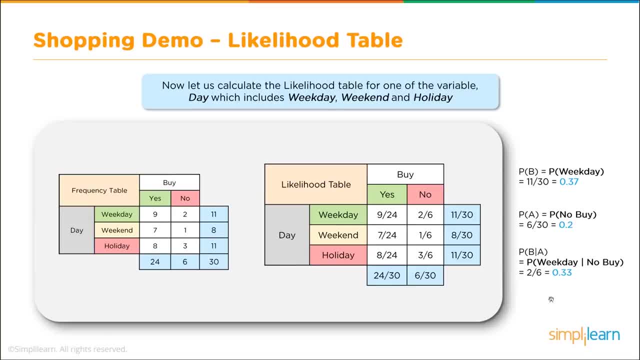 And finally we look at the probability of BFA. In this case we're going to look at the probability of the weekday and not buying. Two of the no buys were done out of the weekend, out of the six people who did not make purchases. So when we look at that probability of the 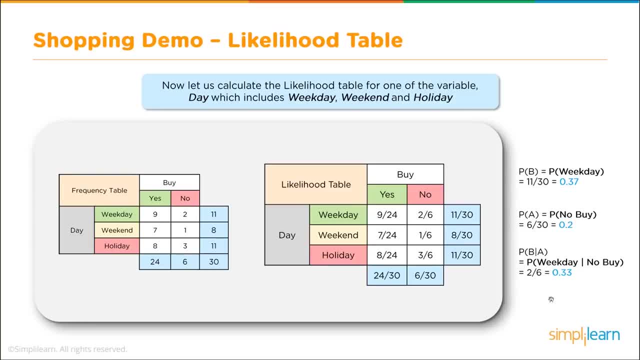 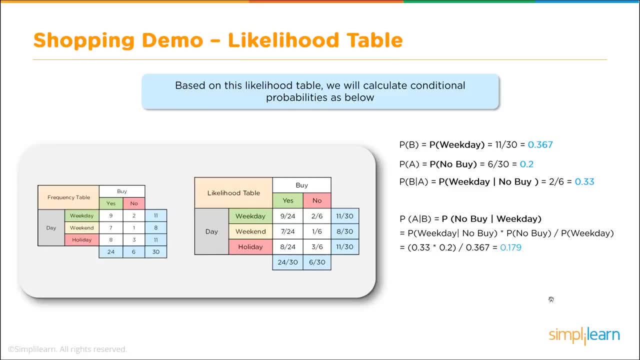 weekday without a purchase is going to be point three, three or thirty three percent. Let's take a look at this, at different probabilities And, based on this likelihood table, let's go ahead and calculate conditional probabilities as below the first three we just did, the probability of making a purchase. 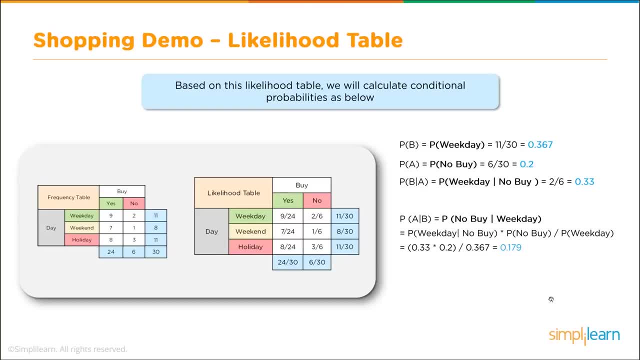 on the weekday is 11 out of 30, or roughly 36 or 37 percent. point three, six, seven. The probability of not making a purchase at all, doesn't matter what day of the week, is roughly point two or 20 percent, And the probability of a weekday no purchase is roughly two out of six. 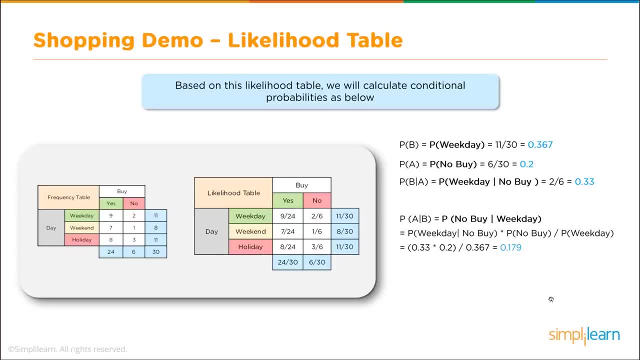 So two out of six of our no purchases were made on the weekday. And then, finally, we take our P of AB. If you look, we've kept the symbols up there. We got P of probability of B, probability of a. probability of B. 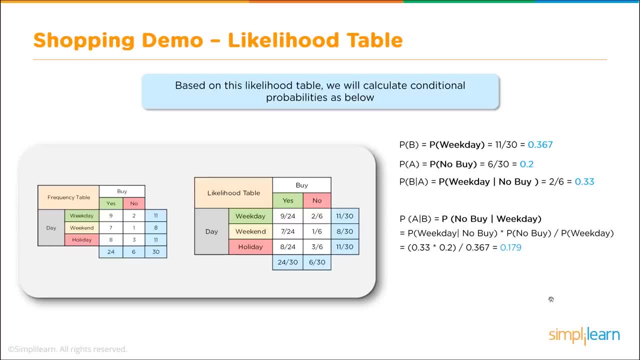 If a. we should remember that the probability of a if B is equal to the first, one times the probability of no buys over the probability of the weekday. So we could calculate it both off the table we created. We can also calculate this by the formula and we get the point three, six, seven. 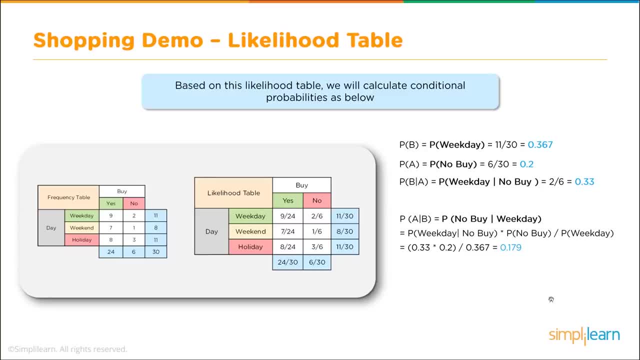 which equals, or point three, three times point two over point three, six, seven, which equals point one, seven, nine, or roughly 17 to 18 percent And that'd be the probability of no purchase done on the weekday. And this is important because we can look at this and say as the probability of 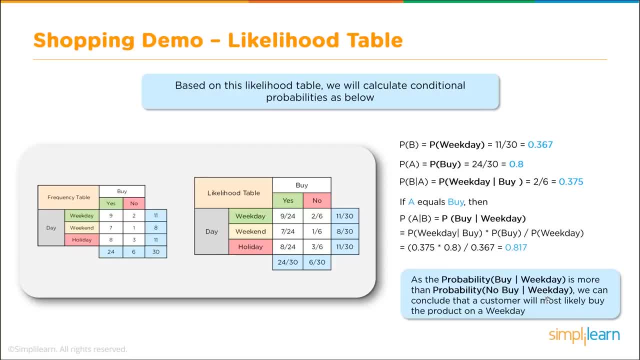 buying on the weekday is more than the probability of not buying on the weekday, we can conclude that customers will most likely buy the product on a weekday. Now we've kept our chart simple and we're only looking at one aspect, So you should be able to look at the table. 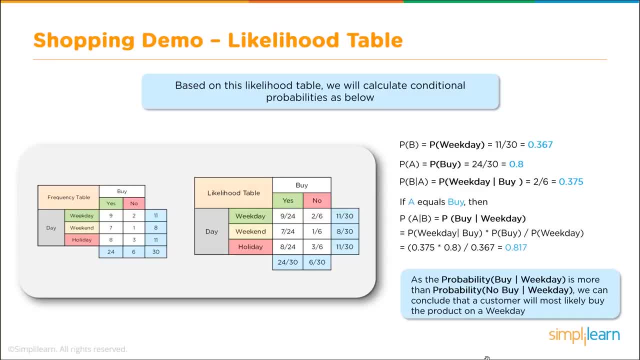 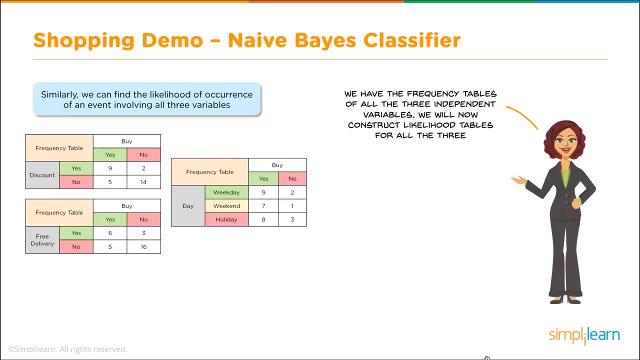 and come up with the same information or the same conclusion. That should be kind of intuitive at this point. Next, we can take the same setup. We have the frequency tables of all three independent variables. Now we can construct the likelihood tables for all three of the variables. we're 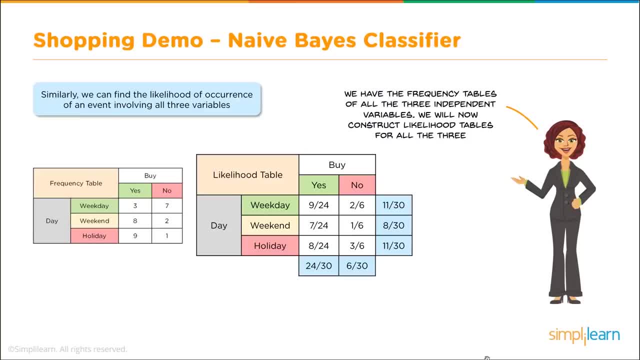 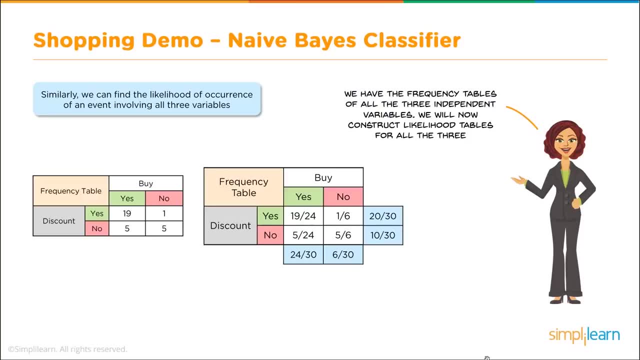 working with. We can take our day like we did before. We have weekday, weekend and holiday. We filled in this table and then we can come in and also do that. for the discount- Yes or no? Did they buy, Yes or no? And we fill in that full table. 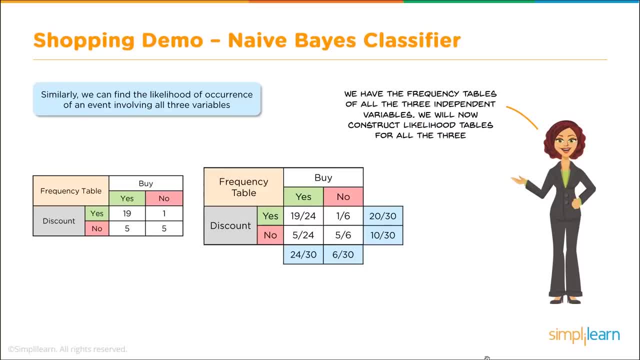 So now we have our probabilities for a discount and whether the discount leads to a purchase or not, and the probability for free delivery. Does that lead to a purchase or not? And this is where it starts getting really exciting. Let us use these three likelihood tables to calculate whether a customer will. 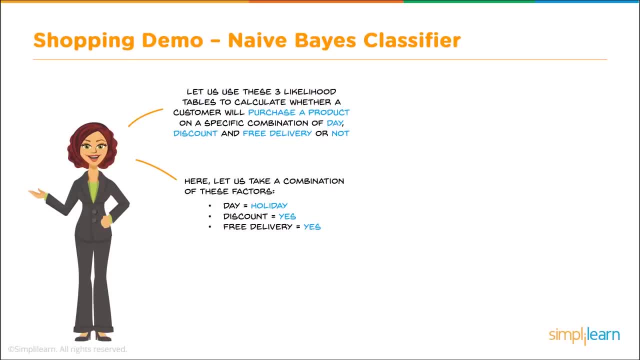 purchase a product on a specific combination of day discount and free delivery or not purchase. Here let us take a combination of these factors: Day equals. holiday Discount equals yes. Free delivery equals- yes. Let's dig deeper into the math to see what this looks like. 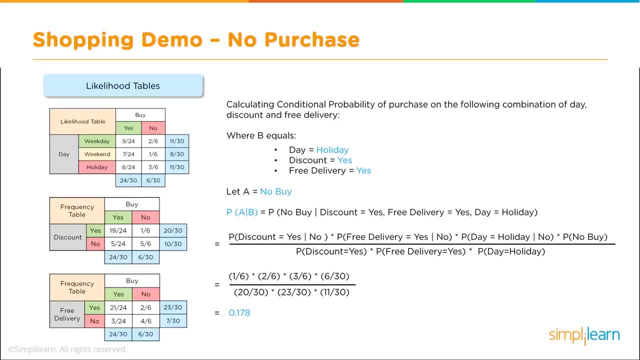 And we're going to start with looking for the probability of them not purchasing on the following combinations of days. We are actually looking for the probability of A equal, no buy, no purchase, And our probability of B we're going to set equal to: is it a holiday? Did they get a discount? Yes, 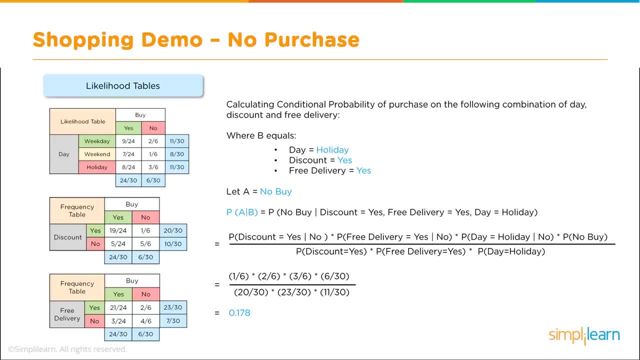 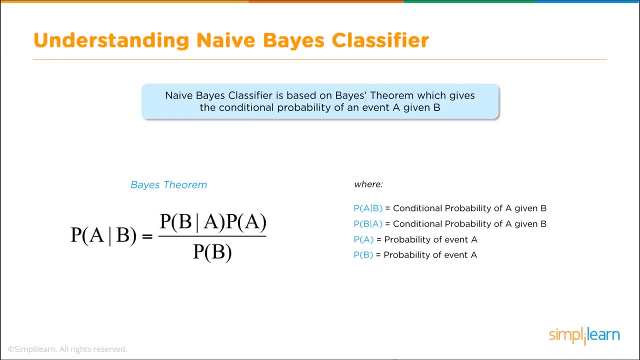 And was it a free delivery? Yes, Before we go further, let's look at the original equation. The probability of A if B equals the probability of B, given the condition A and the probability times. probability of A over the probability of B occurring. 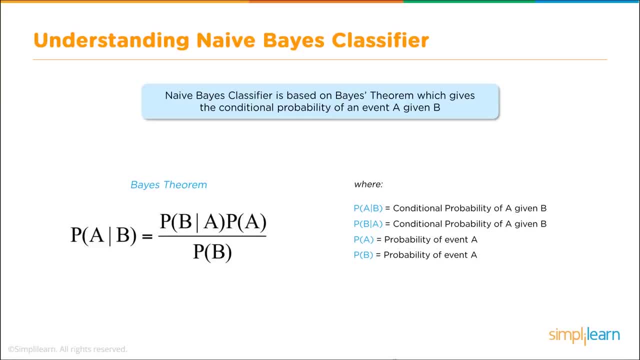 Now, this is basic algebra so we can multiply this information together. So when you see the probability of A given B, in this case the condition is B, C and D, or the three different variables we're looking at, And when you see the probability of B, that would be the conditions. 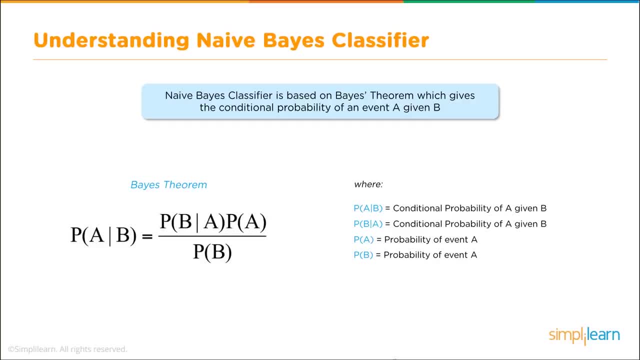 We're actually going to multiply those three separate conditions out: Probability of. you'll see that just second in the formula times the full probability of A over the full probability of B. So here we are back to this and we're going to have let A equal no purchase. 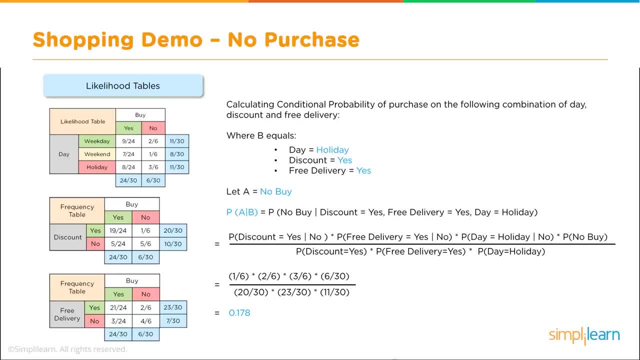 And we're looking for the probability of B on the condition A, where A sets for three different things. Remember that equals the probability of A given the condition B, And in this case we just multiply those three different variables together, So we have the probability of the discount times, the probability. 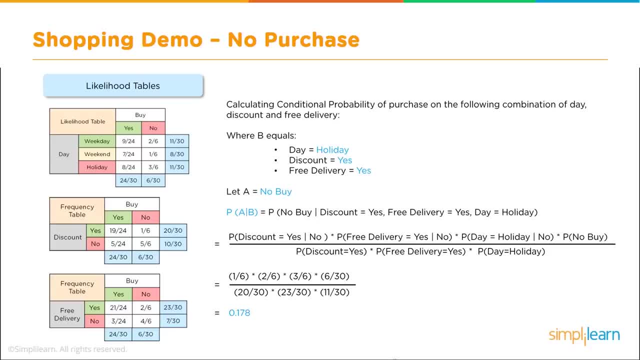 of free delivery times. the probability is a day equal a holiday. Those are three variables of the probability of A, if B, And then that is going to be multiplied by the probability of them not making a purchase, And then we want to divide that by the total probabilities and they're. 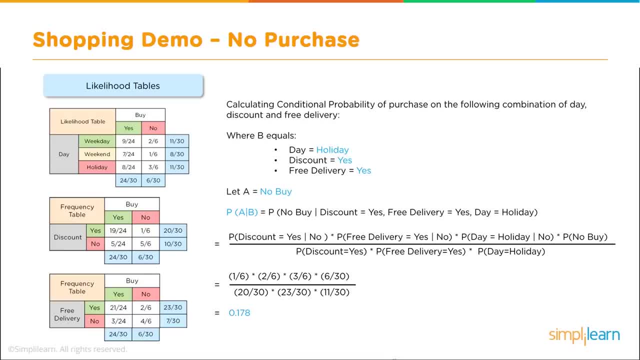 multiplied together So we have the probability of a discount, the probability of a free delivery and the probability of it being on a holiday. When we plug those numbers in, we see that one out of six were no purchase on a discounted day. Two out of six were a no purchase. 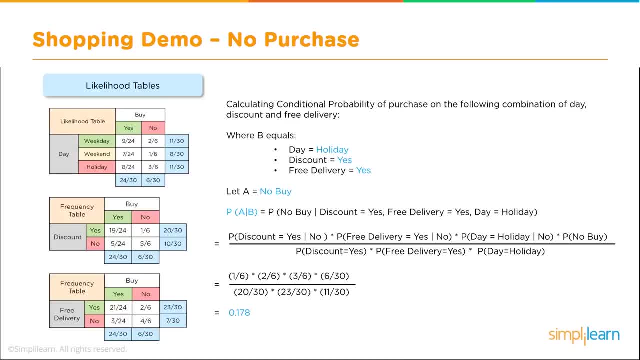 on a free day And three out of six were a no purchase on a holiday. Those are our three probabilities of A if B multiplied out, And then that has to be multiplied by the probability of a no purchase. And remember the probability of a no buy is across all the data. 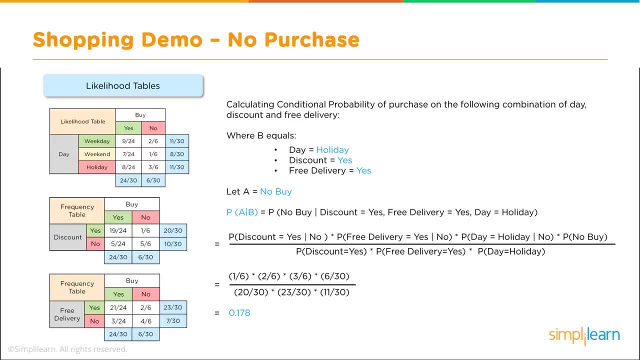 So that's where we get the six out of 30. We divide that out by the probability of each category over the total number, So we get the 20 out of 30 had a discount. 23 out of 30 had a yes for free delivery. 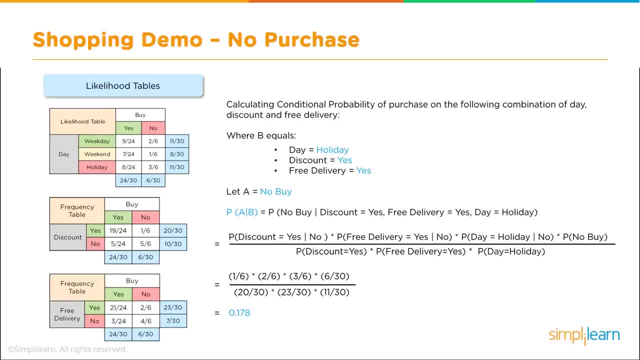 and 11 out of 30 were on a holiday. We plug all those numbers in, we get 0.178.. So in our probability math we have a 0.178 if it's a no buy for a holiday, a discount and a free delivery. Let's turn that around and see what that looks like. 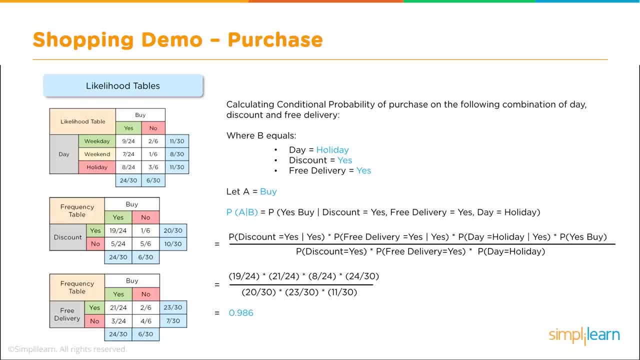 if we have a purchase. I promise this is the last page of math before we dig into the Python script. So here we're, calculating the probability of the purchase using the same math. we did to find out if they didn't buy. Now we want to know if they did buy And again we're going to go by. 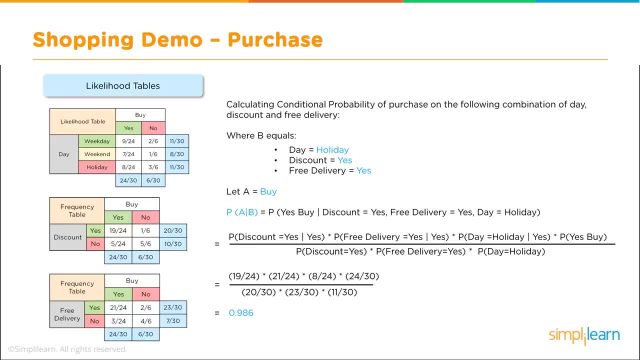 a day equals a holiday discount equals yes. free delivery equals yes. and let A equal buy. Now, right about now, you might be asking: why are we doing both calculations? Why would we want to know the no buys and buys for the same data going in? Well, we're going to show you that in just 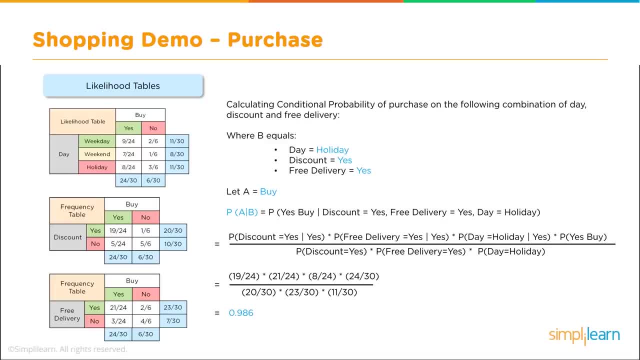 a moment. but we have to have both of those pieces of information so that we can figure it out as a percentage as opposed to a probability equation, And we'll get to that normalization here in just a moment. Let's go ahead and walk through this calculation. 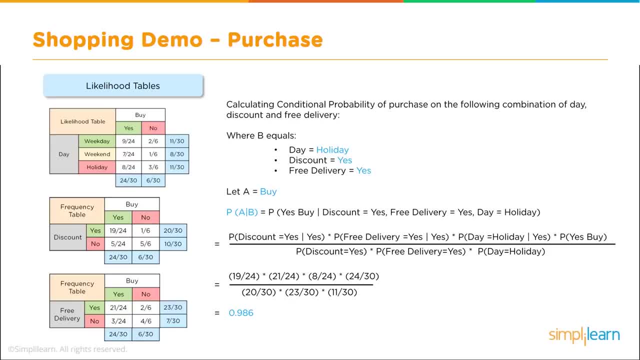 And, as you can see here, the probability of A on the condition of B, B being all three categories. Did we have a discount with a purchase? Do we have a free delivery with a purchase? And is a day equal to holiday? And when we plug this all into that formula and multiply it all out, 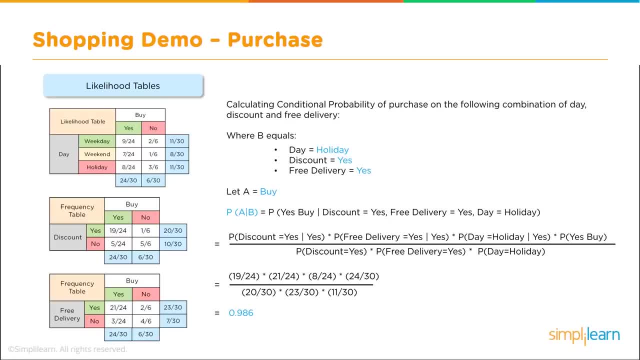 we get our probability of a discount, probability of a free delivery, probability of the day being a holiday times, the overall probability of it being a purchase divided by, again multiplying the three variables out, the full probability of there being a discount, the full probability of being a free delivery. 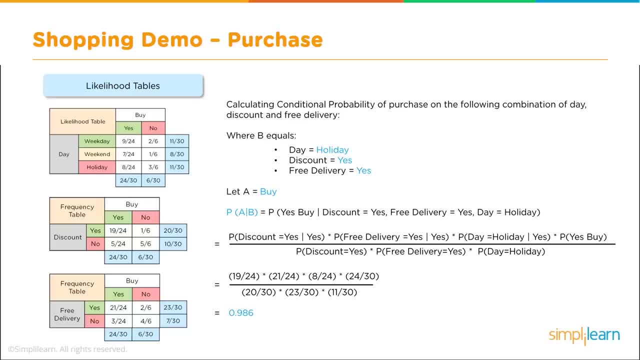 and the full probability of there being a day equal holiday. And that's where we get this: 19 over 24 times 21 over 24 times 8 over 24 times the P of A 24 over 30, divided by the probability of the discount. 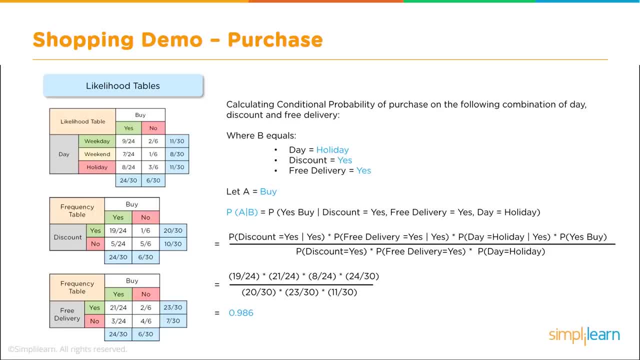 the free delivery times the day, or 20 over 30,, 23 over 30 times 11 over 30. And that gives us our .986.. So what are we going to do with these two pieces of data? We just generate it. 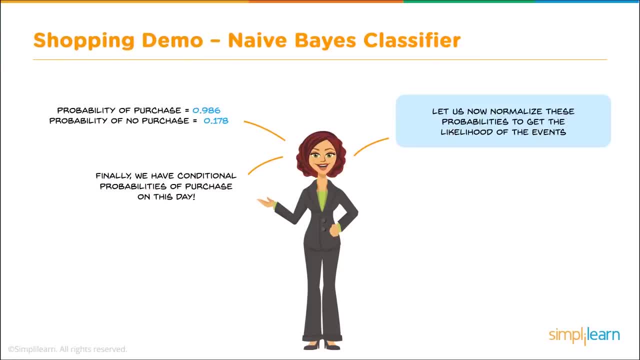 Well, let's go ahead and go over them. We have a probability of purchase equals .986.. We have a probability of no purchase equals .178.. So, finally, we have a conditional probabilities of purchase on this day. Let us take that. 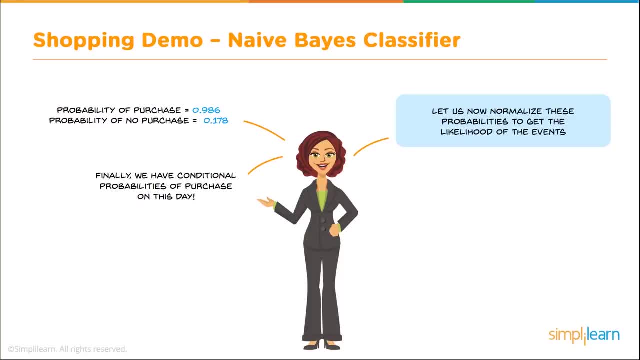 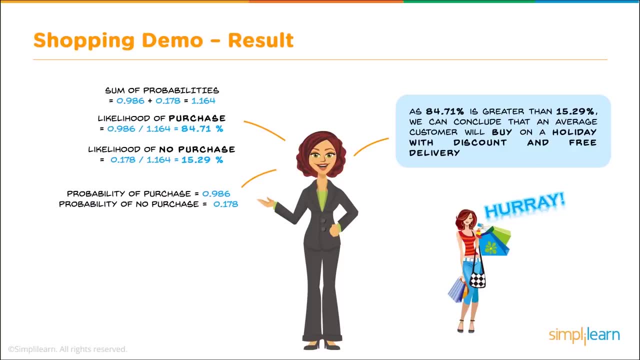 We're going to normalize it and we're going to take these probabilities and turn them into percentages. This is simply done by taking the sum of probabilities, which equals .986 plus .178, and that equals the 1.164.. So if we divide each probability by the sum, we get the percentage. 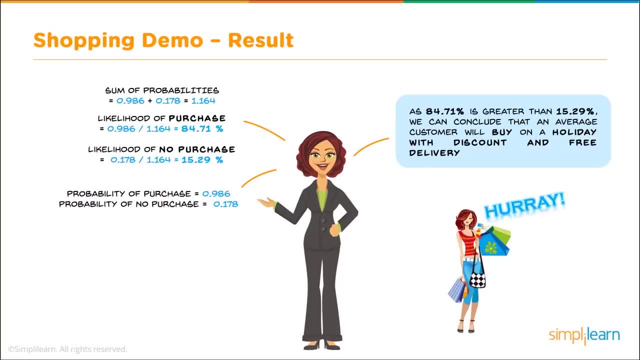 And so the likelihood of a purchase is 84.71% and the likelihood of no purchase is 15.29%, given these three different variables. So if it's on a holiday, if it's with a discount and has free delivery, then there's an 84.71% chance that the customer is going to come in and make. 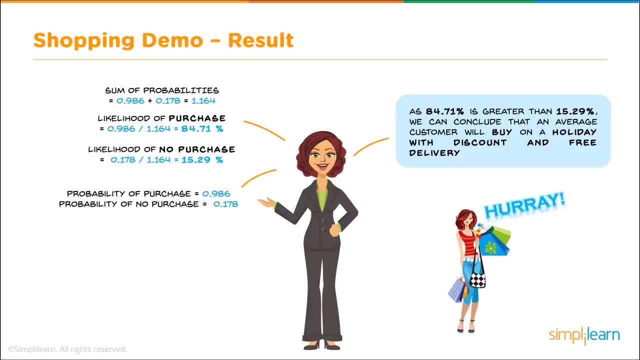 a purchase. Hooray, They purchased our stuff. We're making money. If you're owning a shop, that's like is the bottom line is you want to make some money so that you keep your shop open and have a living. Now, I promised you that we were going. 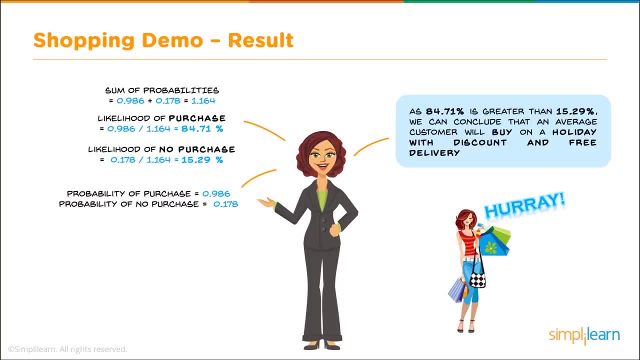 to be finishing up the math here with a few pages. So we're going to move on and we're going to do two steps. The first step is: I want you to understand why you want to, why you want to use the naive Bayes. What are the advantages of naive Bayes? 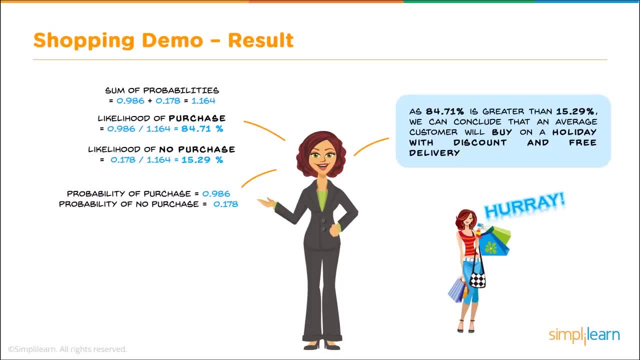 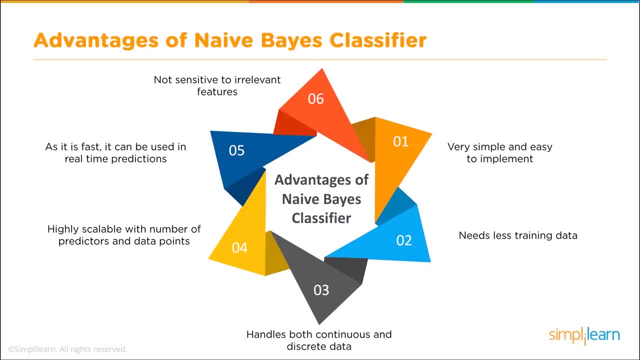 And then, once we understand those advantages, we'll just look at that briefly. Then we're going to dove in and do some Python coding. Advantages of naive Bayes classifier. So let's take a look at the six advantages of the naive Bayes classifier and we're going to walk around this. 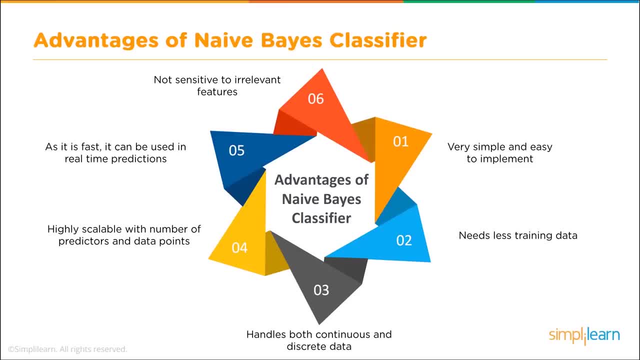 lovely wheel looks like an origami folded paper. The first one is very simple and easy to implement. Certainly you could walk through the tables and do this by hand. You got to be a little careful because the notations can get confusing. You have all these different probabilities. 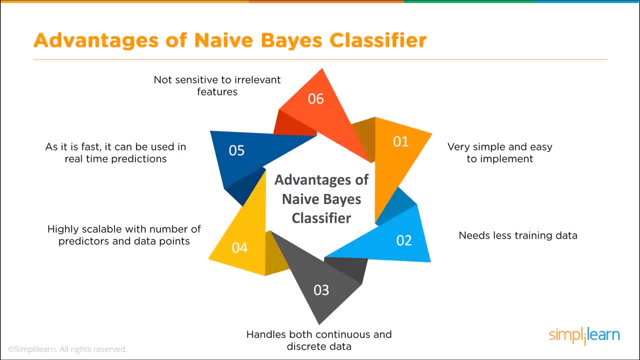 And I certainly mess those up as I put them on. You know, is it on the top of the bottom? Got to really pay close attention to that. when you put it into Python, It's really nice because you don't have to worry about any of that. 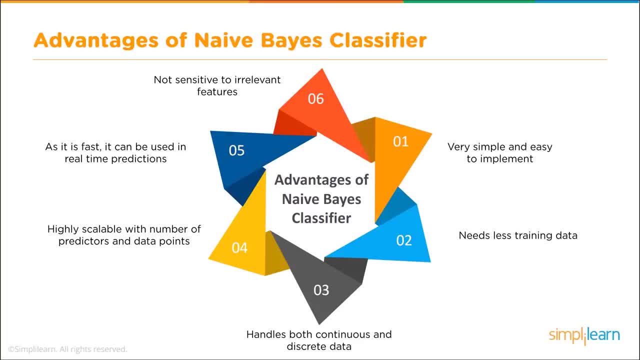 You let the Python handle that, the Python module. But understanding it, You can put it on a table and you can easily see how it works. And it's a simple algebraic function. It needs less training data. So if you have smaller amounts of data, this is great. 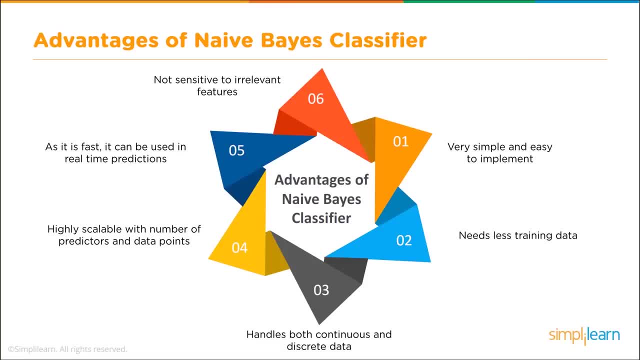 Powerful tool for that handles both continuous and discrete data. It's highly scalable with number of predictors and data points. So, as you can see, you just keep multiplying different probabilities in there and you can cover not just three different variables or sets. You can now expand this to even more categories. 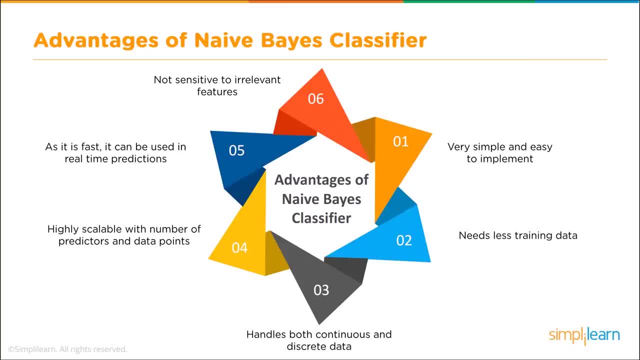 Number five: it's fast. It can be used in real time predictions. This is so important. This is why it's used in a lot of our predictions on online shopping carts, referrals, spam filters is because there's no time delay as it has to go. 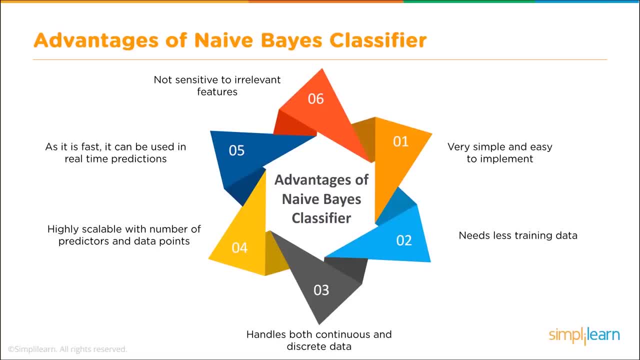 through and figure out a neural network or one of the other mini setups where you're doing classification. And certainly there's a lot of other tools out there in the machine learning that can handle these, but most of them are not as fast as the Naive Bayes. 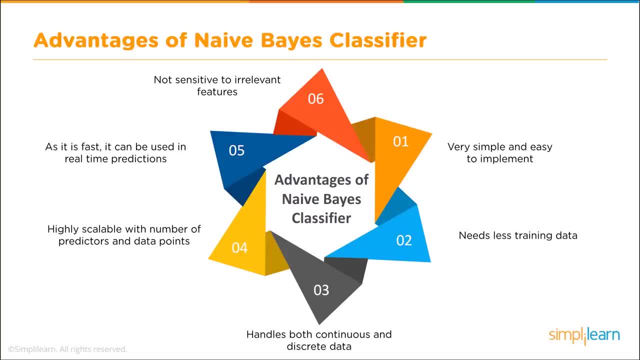 And then, finally, it's not sensitive to irrelevant features. So it picks up on your different probabilities, and if you're short on data on one probability, you can kind of it automatically adjust for that. Those formulas are very automatic, and so you can still get a very solid. 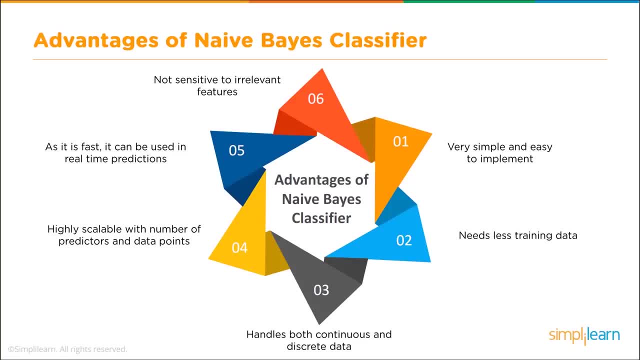 predictability, even if you're missing data or you have overlapping data for two completely different areas. We see that a lot in doing census and studying of people and habits, where they might have one study that covers one aspect, another one that overlaps, And because of two overlap they can then predict the unknowns for the group. 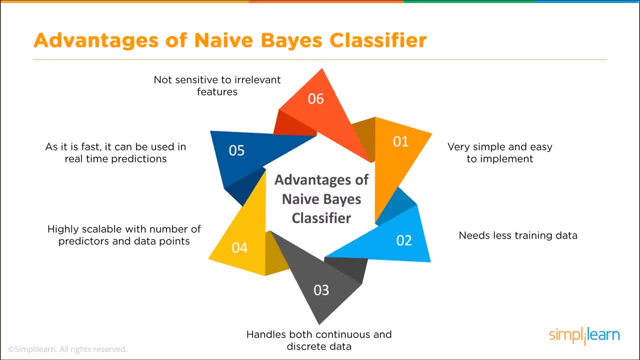 that they haven't done the second study on, or vice versa. So it's very powerful And that it is not sensitive to the irrelevant features, and in fact, you can use it to help predict features that aren't even in there. So now we're down to my favorite part. 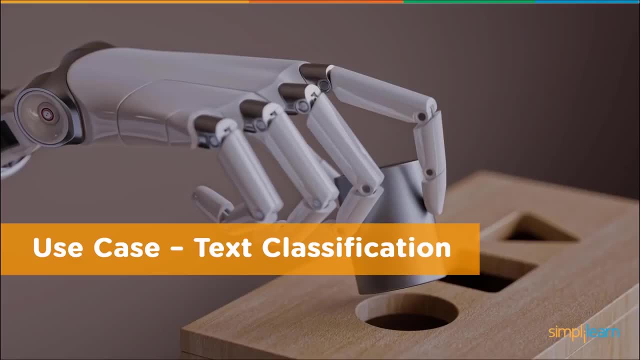 We're going to roll up our sleeves and do some actual programming. We're going to do the use case text classification. Now I would challenge you to go back and send us a note on the notes below underneath the video and request the data for the shopping cart. 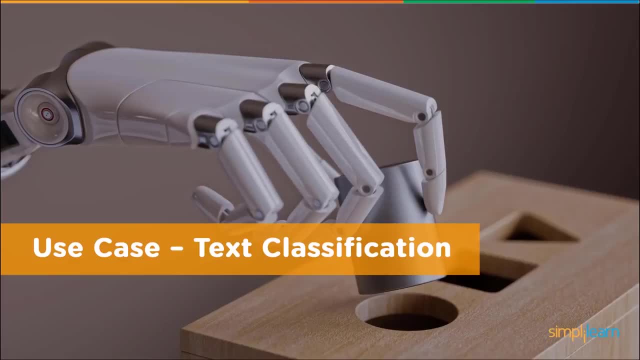 So you can plug that into Python code and do that on your own time. So you can walk through it, Since we walked through all the information on it. But we're going to do a Python code doing text classification- very popular for doing the naive bays. 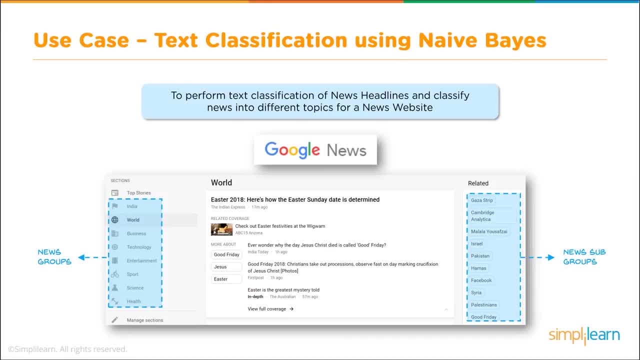 So we're going to use our new tool to perform a text classification of news headlines and classify news into different topics for a news website. As you can see here we have a nice image of the Google News and then related on the right subgroups. 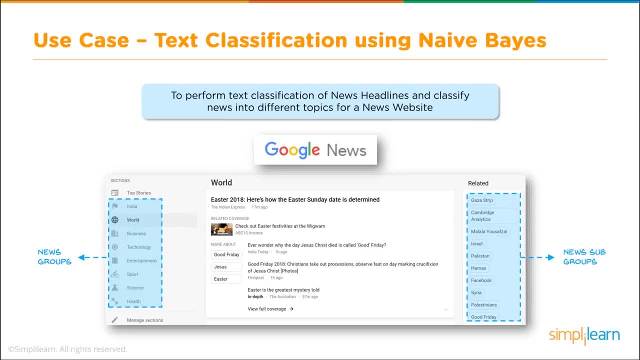 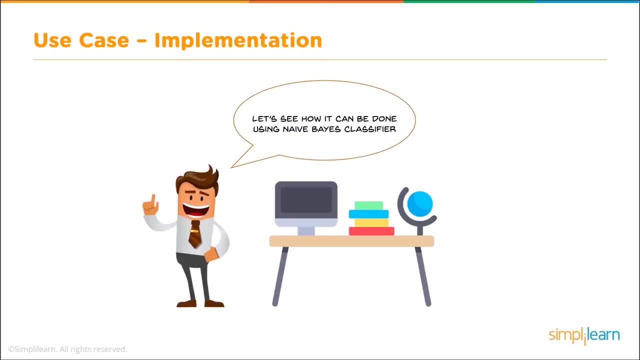 I'm not sure where they actually pulled the actual data we're going to use from. It's one of the standard sets, But certainly this can be used on any of our news headlines, Headlines and classification. So let's see how it can be done using the naive bays classifier. 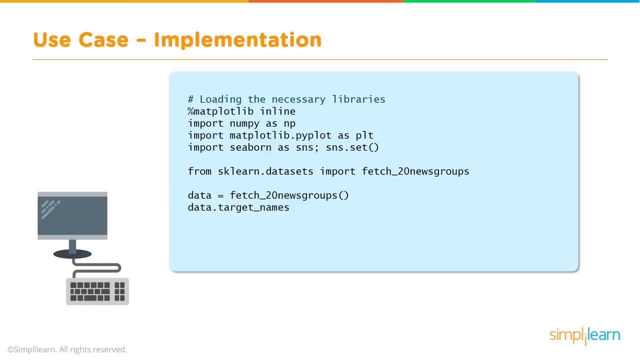 Now we're at my favorite part. We're actually going to write some Python script. Roll up our sleeves And we're going to start by doing our imports. These are very basic imports, including our news group, And we'll take a quick glance at the target names. 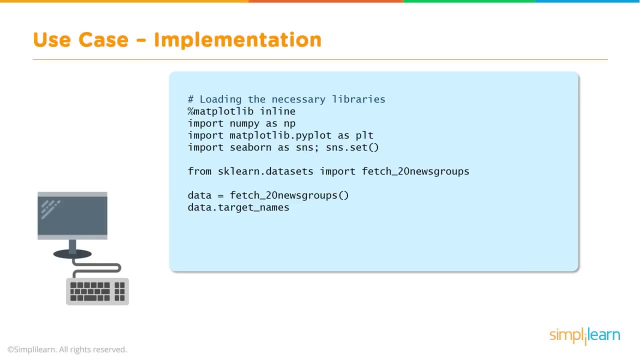 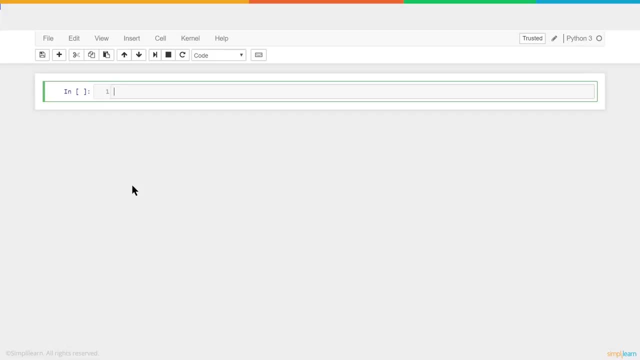 Now I'm going to open up my favorite editor or inline editor for Python. You don't have to use this. You can use whatever your editor that you like, whatever interface IDE you want. This just happens to be the Anaconda Jupyter notebook. 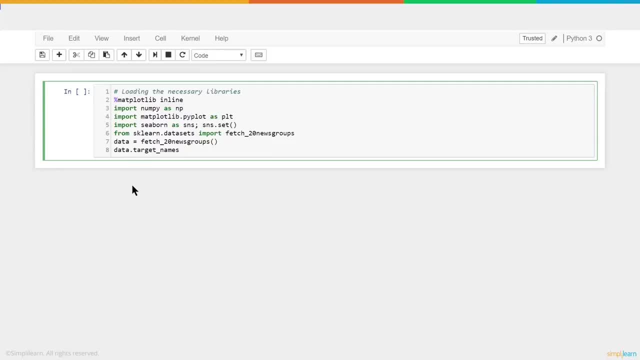 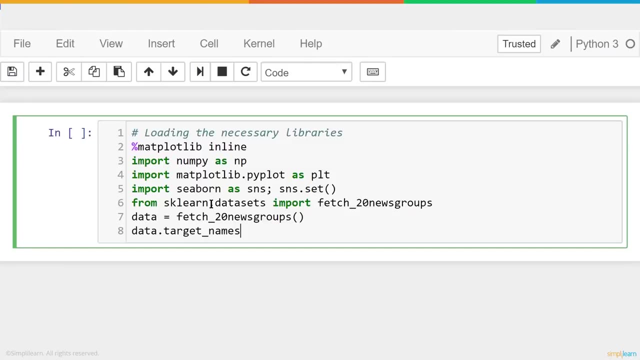 And I'm going to paste that first piece of code in here so we can walk through it. Let's make it a little bigger on the screen so you have a nice view of what's going on. And we're using Python 3,, in this case 3.5.. 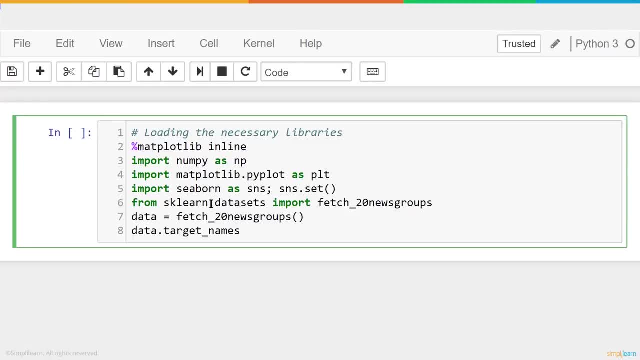 So this would work in any of your 3x. If you have it set up correctly, it should also work in a lot of the 2x. You just have to make sure all of the versions of the modules match your Python version. 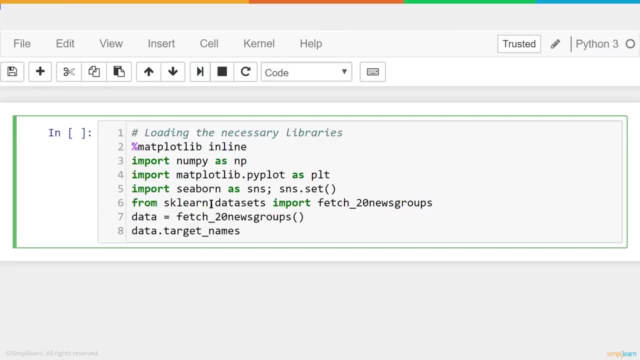 And in here you'll notice. the first line is your percentage matplotlibrary inline. Now, three of these lines of code are all about plotting the graph. This one lets the notebook know, since this is an inline setup, that we want the graphs to show up on this page. 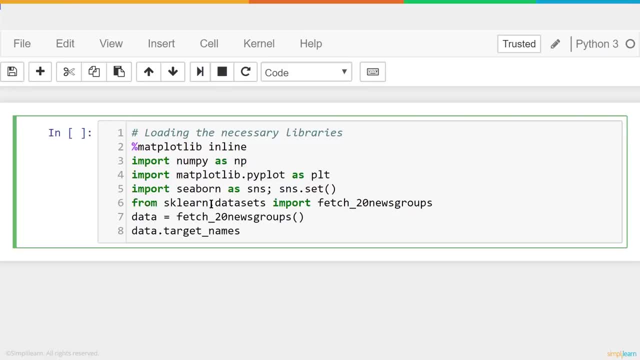 Without it in a notebook like this, which is an explorer interface, it won't show up. Now, a lot of IDEs don't require that. A lot of them like if I'm working on one of my other setups, it just has a popup and the graph pops up on there. 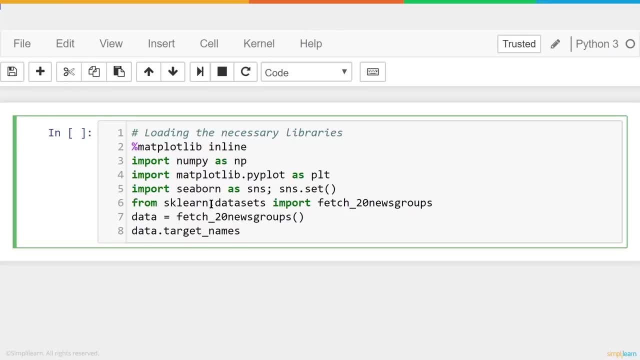 So you have that setup also, But for this we want the matplotlibrary inline, And then we're going to import numpy as np, that's number Python, which has a lot of different formulas in it that we use for both of our sklearn module. 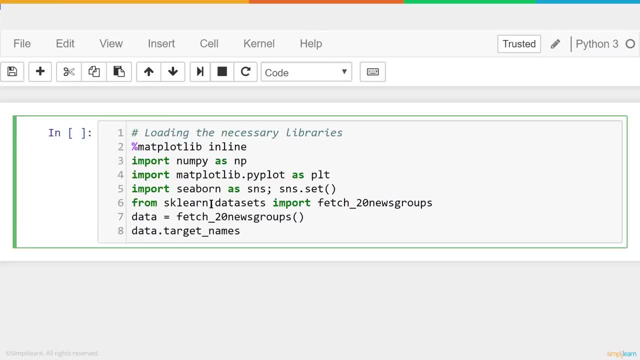 And we also use it for any of the upper math functions in Python and it's very common to see that as np, numpy as np. The next two lines are all about our graphing. Remember I said three of these were about graphing. 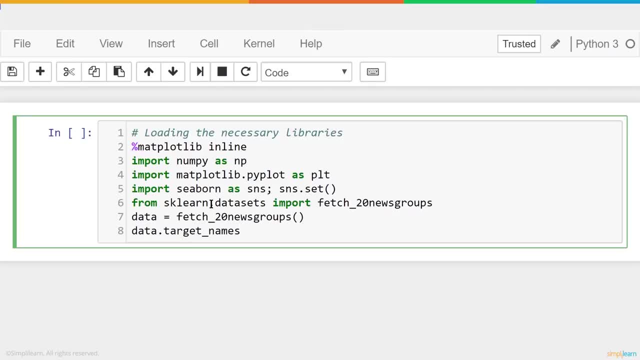 Well, we need our matplotlibrarypyplot as plt, and you'll see that plt is a very common setup, as is the sns and just like the np, And we're going to import sklearn as sns and we're going to do the snsset. 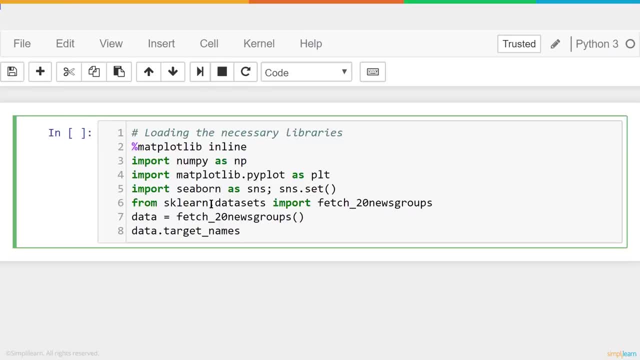 Now sklearn sits on top of pyplot and it just makes a really nice heatmap. It's really good for heatmaps And if you're not familiar with heatmaps, that's a good way to do it. Heatmaps, that just means we give it a color scale. 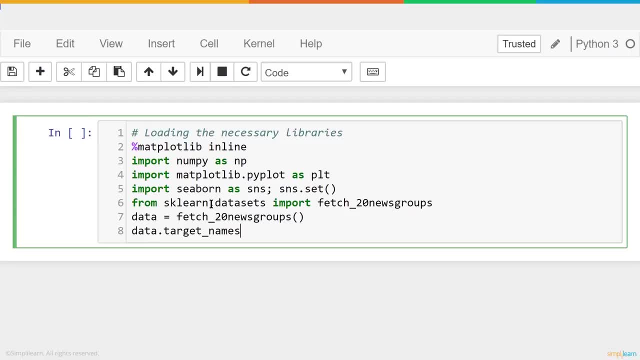 The term comes from the brighter red, it is the hotter. it is in some form of data And you can set it to whatever you want And we'll see that later on. So you'll see that those three lines of code here are just importing the graph function. 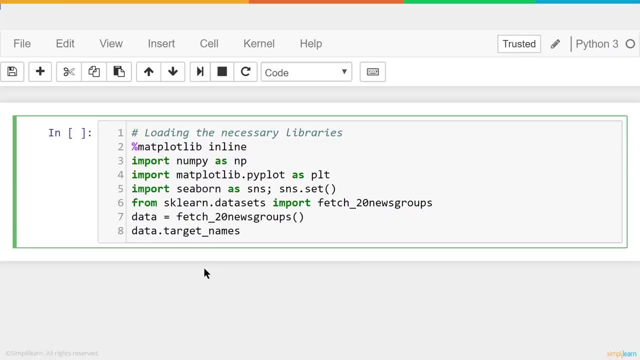 so we can graph it And as a data scientist, you always want to graph your data and have some kind of visual. It's really hard just to shove numbers in front of people and they look at it and it doesn't mean anything. 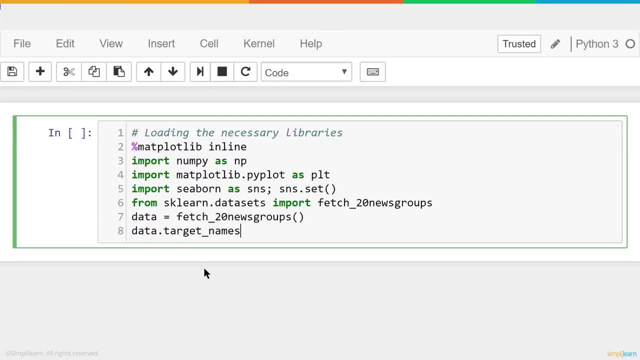 And then from the sklearndatasets we're going to import the fetch20 newsgroups, A very common one for analyzing, tokenizing words and setting them up and exploring how the words work. and how do you categorize different things when you're dealing with documents. 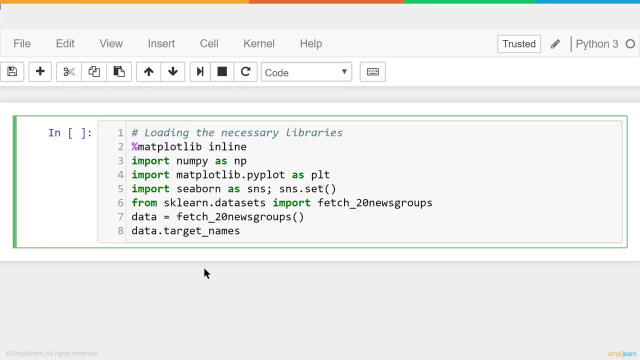 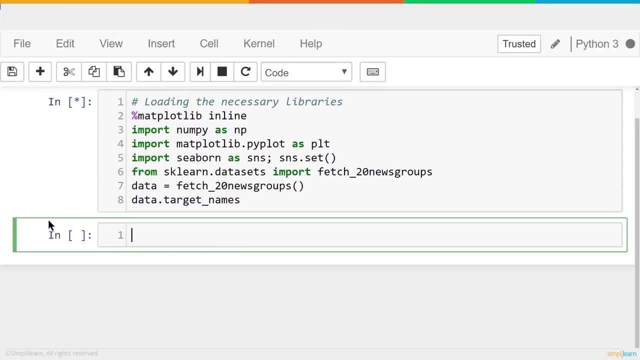 And then we set our data equal to fetch20 newsgroups, So our data variable will have the data in it And we're going to go ahead and just print the target names- datatargetnames- And let's see what that looks like. 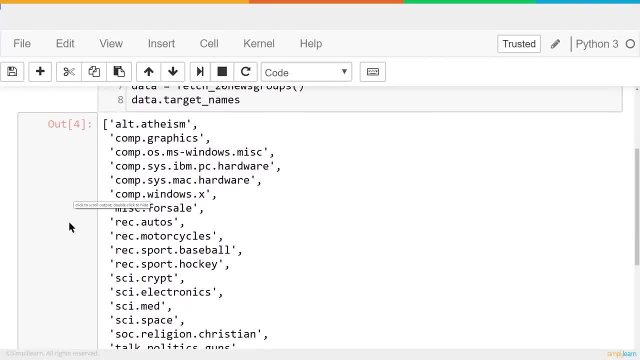 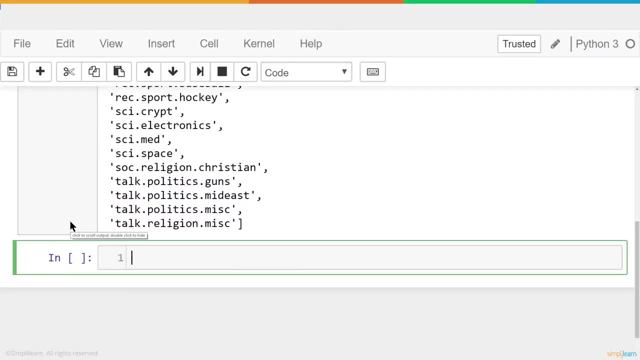 And you'll see here we have alt atheism, comp graphics, comp os, ms windowsmiscellaneous, And it goes all the way down to talkpolls, Talkpoliticsmiscellaneous, talkreligionmiscellaneous. These are the categories they've already assigned to this newsgroup. 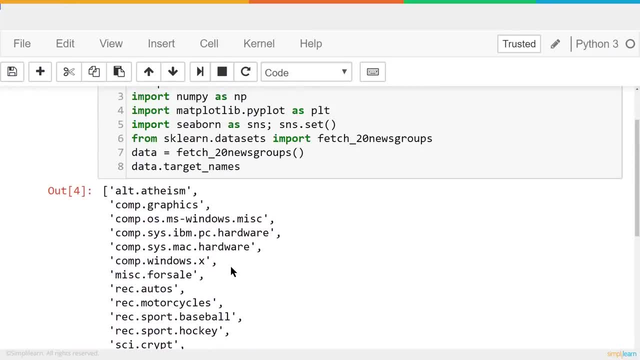 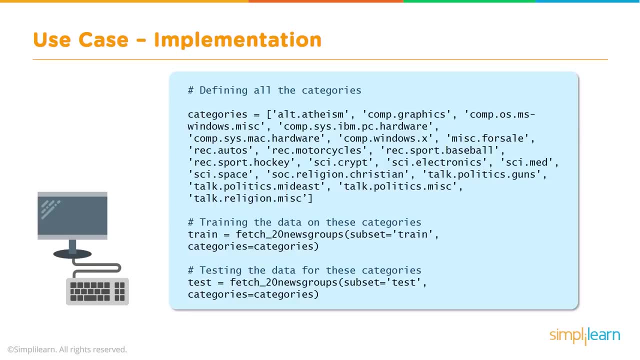 And it's called fetch20 because you'll see, there's- I believe there's- 20 different topics in here, or 20 different categories as we scroll down. Now we've gone through the 20 different categories and we're going to go ahead and start defining. 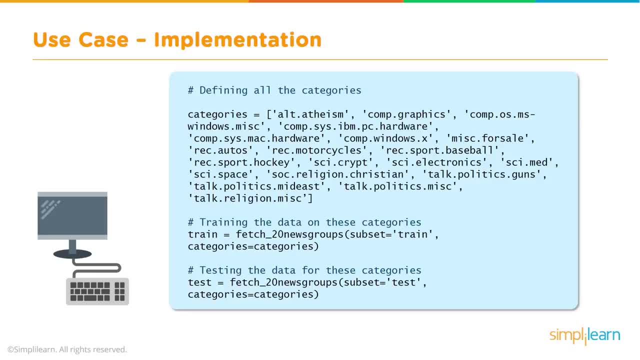 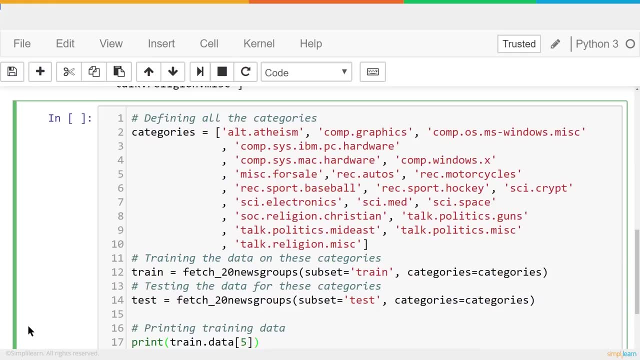 all the categories and set up our data. So we're actually in here going to go ahead and get the data all set up and take a look at our data And let's move this over to our Jupyter notebook And let's see what this code does. 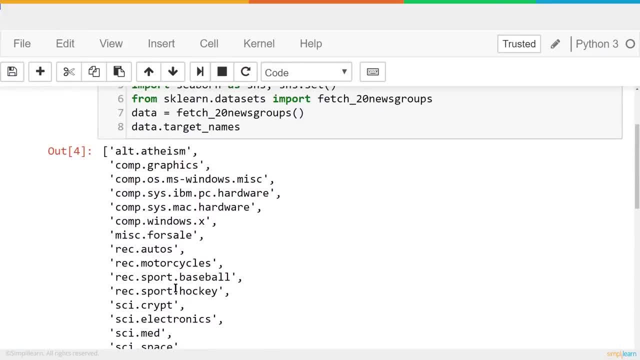 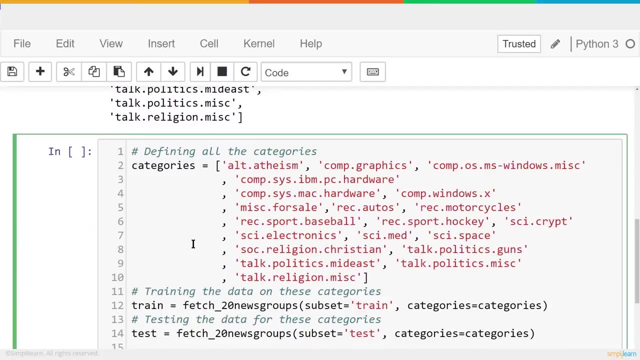 First we're going to set our categories. Now, if you noticed up here, I could have just as easily set this equal to datatarget underscore names, because it's the same thing. But we want to kind of spell it out for you so you can see the different categories. 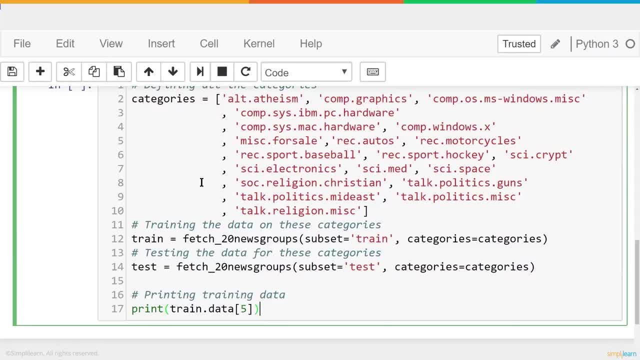 It kind of makes it more visual so you can see what your data's looking like in the background. Once we've created the categories, we're going to open up a train set. So this training set of data is going to go into fetch20 newsgroups and it's a subset. 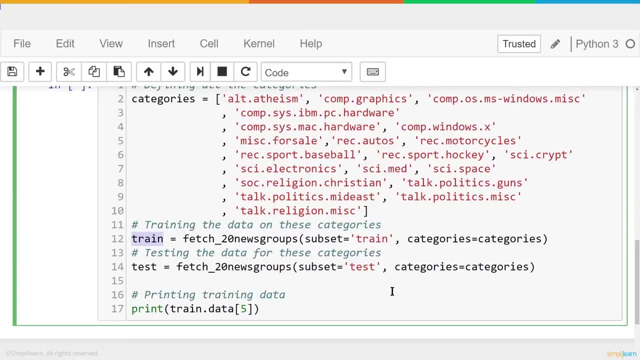 in there called train And categories equals categories. so we're pulling out those categories that match And then if you have a train set, you should also have the testing set. We have test equals fetch20, newsgroups. subset equals test and categories equals categories. 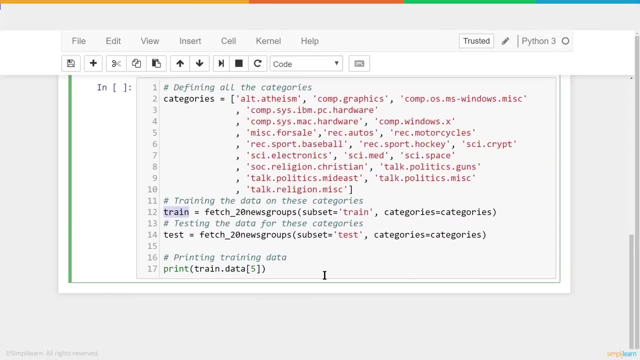 Let's go down one size so it all fits on my screen. There we go, And just so we can really see what's going on. let's see what happens when we print out one part of that data. So it creates train and under train it creates train dot data. and we're just going to look. 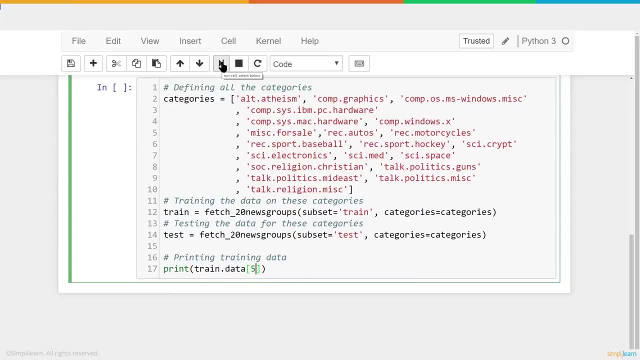 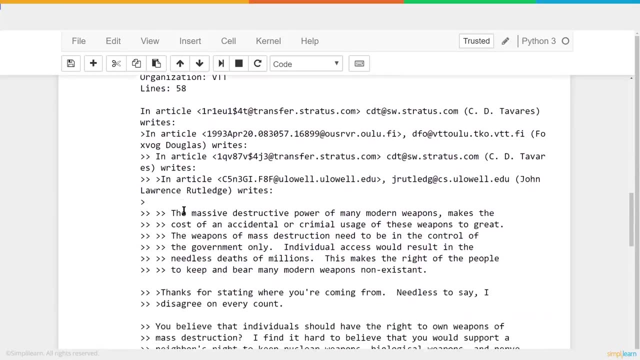 at data piece number And let's go ahead and run that and see what that looks like. And you can see when I print train dot data number five under train it prints out one of the articles. This is article number five. You can go through and read it on there. 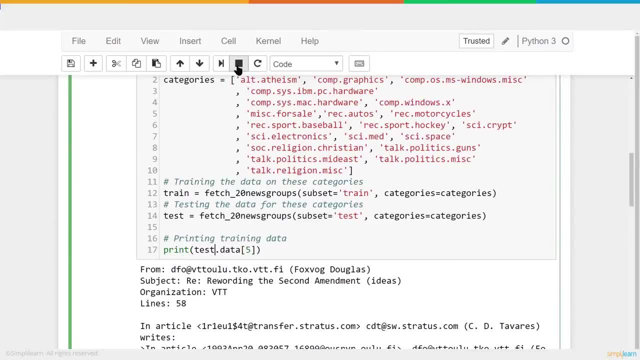 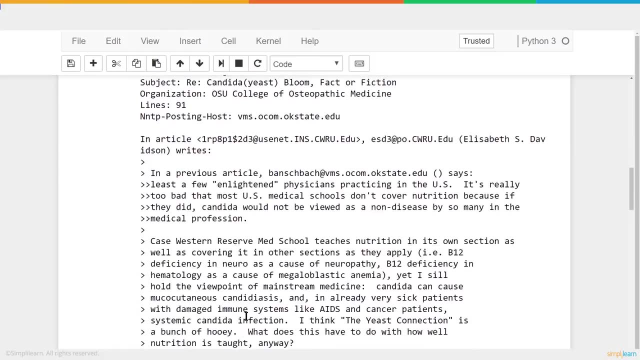 And we can also go in here and change this to test, which should look identical because it's splitting the data up into different groups. train and test And we'll see test. number five is a different article, but it's another article in here And maybe you're curious and you want to see just how many articles are in here. 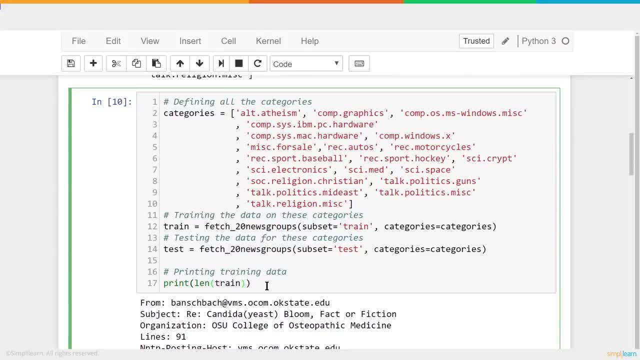 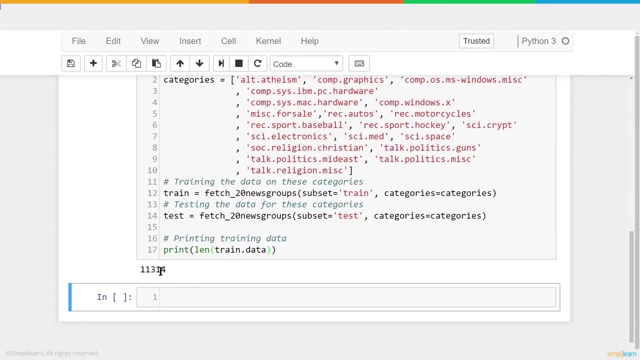 We could do length of train dot data and if we run that you'll see that the training data has 11,314 articles. So we're not going to go through all those articles. That's a lot of articles, But we can look at one of them just so you can see what kind of information is coming. 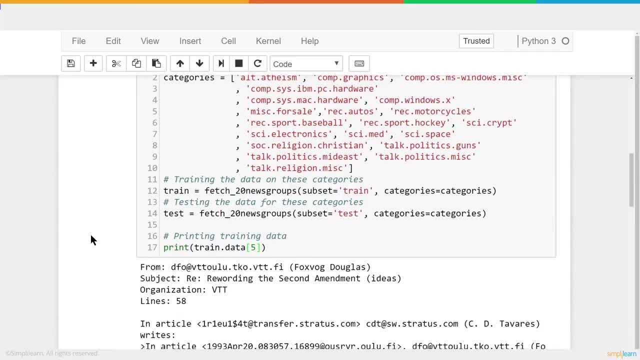 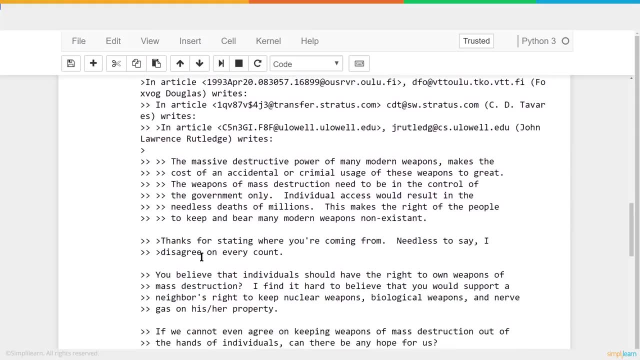 out of it and what we're looking at. And we'll just look at number five for today. And here we have it, rewording the second amendment: IDs VTT, line 58, lines 58 in article, etc. All the way down and see all the different parts to there. 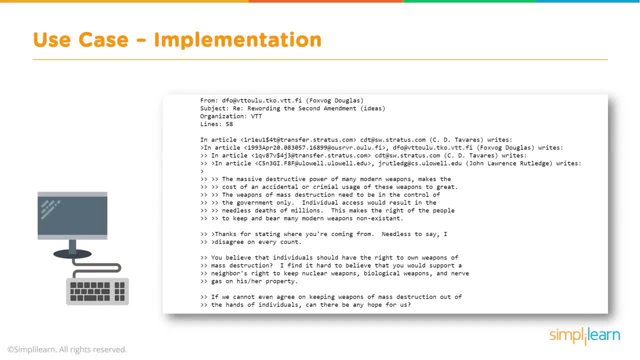 Now, we've looked at it and that's pretty complicated when you look at one of these articles to try to figure out. how do you weight this? If you look down here, we have different words and maybe the word from, Well from- is probably in all the articles, so it's not going to have a lot of meaning. 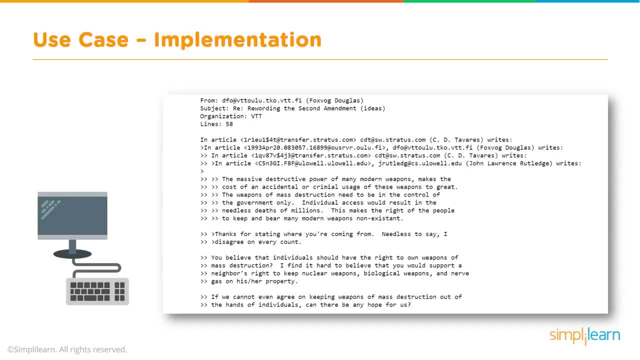 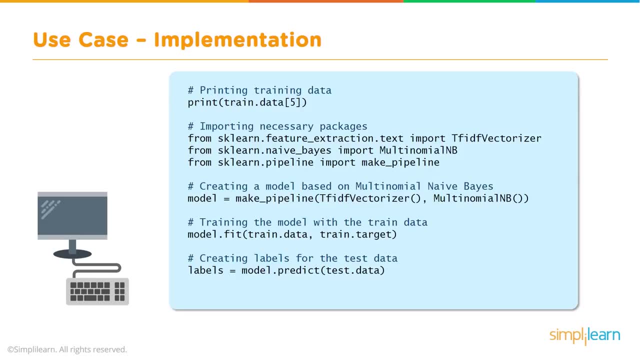 as far as trying to figure out whether this article fits one of the categories or not. So trying to figure out what category it fits in based on these words is where the challenge comes in. Now that we've viewed our data, we're going to dive in and do the actual predictions. 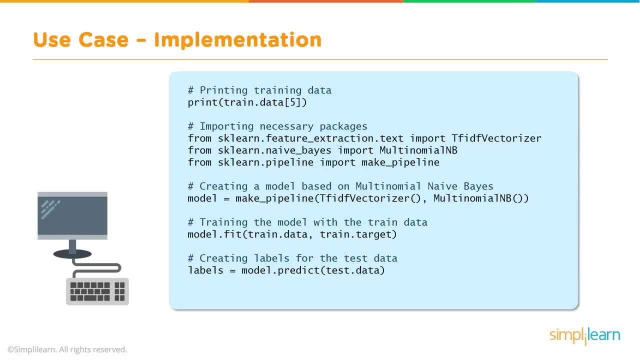 This is the actual naive base and we're going to throw another model at you or another module at you here in just a second. We can't go into too much detail, but it deals specifically working with words and text and what they call tokenizing those words. 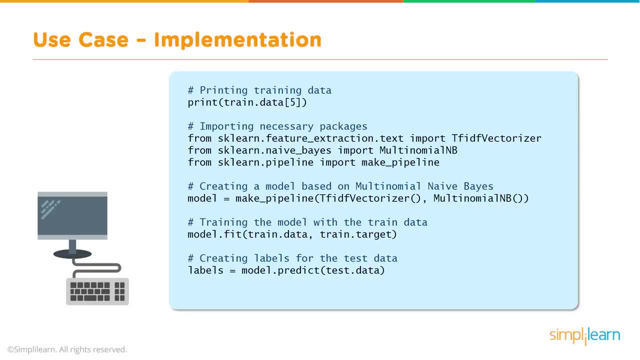 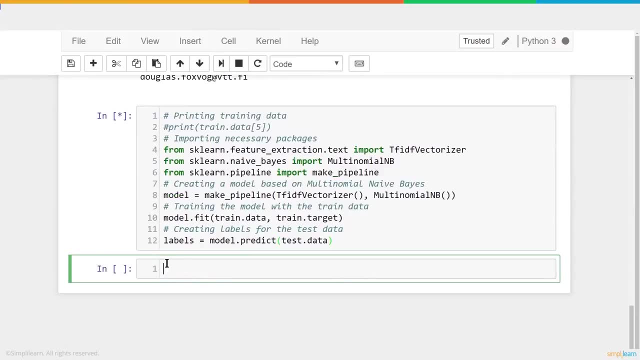 So let's take this code and let's skip on over to our Jupyter notebook and walk through it And here we are in our Jupyter notebook. Let's paste that in there and I can run this code right off the bat. It's not actually going to display anything yet, but it has a lot going on in here. 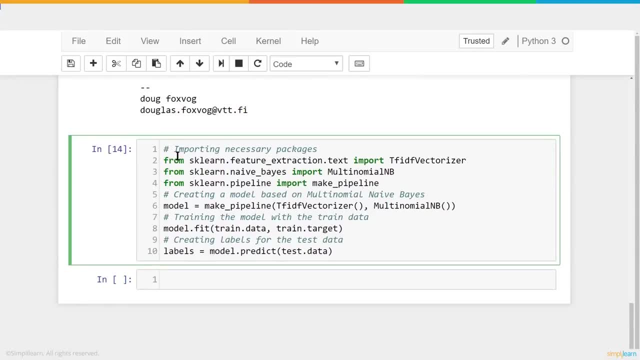 So the top, We have the print module from the earlier one. I didn't know why that was in there. So we're going to start by importing our necessary packages And from the sklearnfeaturesextractiontxt we're going to import tfidfvectorizer. 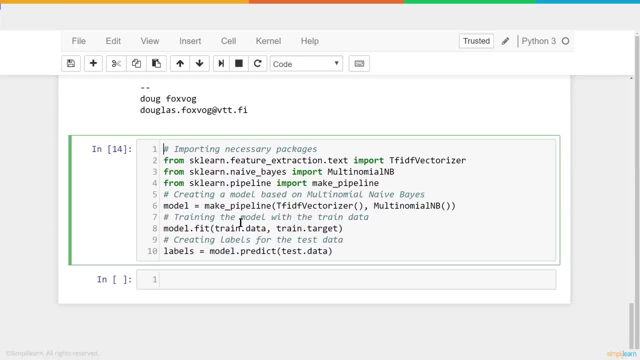 I told you we're going to throw a module at you. We can't go too much into the math behind this or how it works. You can look it up. The notation for the math is usually tfidf And that's just a way of weighing the words and it weighs the words based on how many. 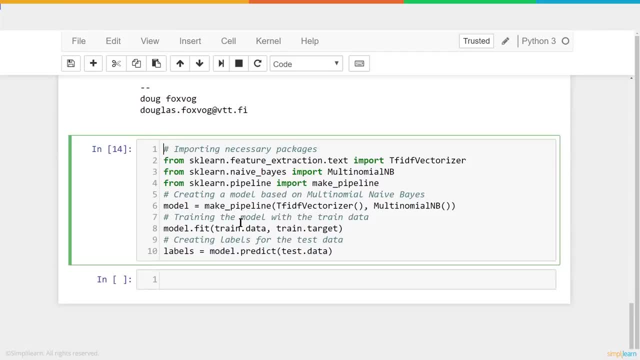 times they're used In a document, how many times or how many documents are used in, And it's a well-used formula that's been around for a while. It's a little confusing to put this in here, but let's let her know that it just goes in. 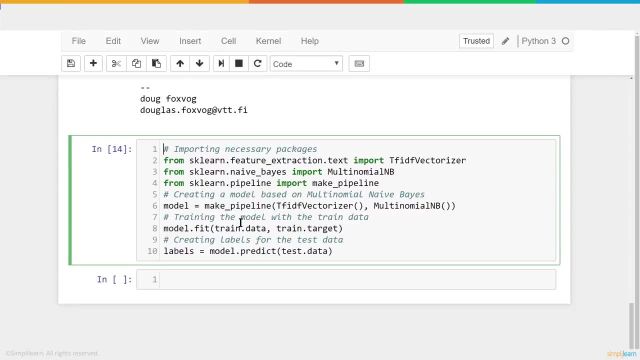 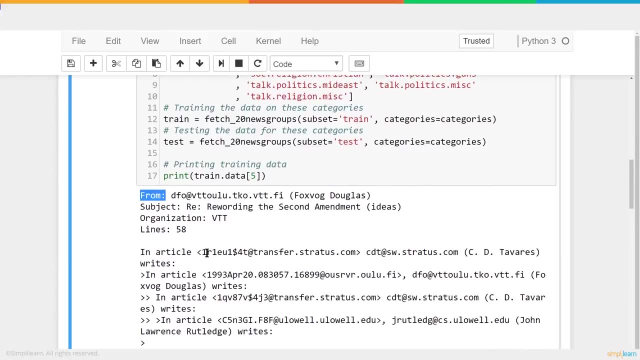 there and weights the different words in the document for us. That way we don't have to wait And if you put a weight on it- if you remember I was talking about that up here earlier- if these are all emails, they probably all have the word from in them. 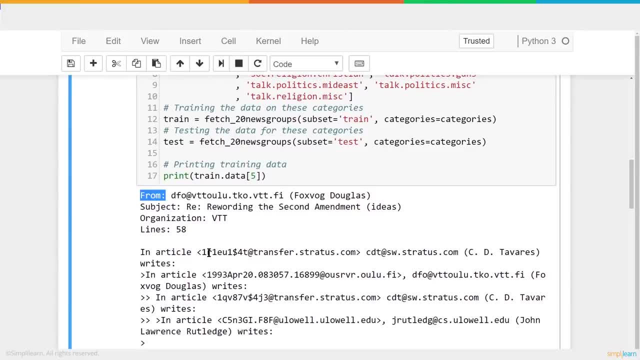 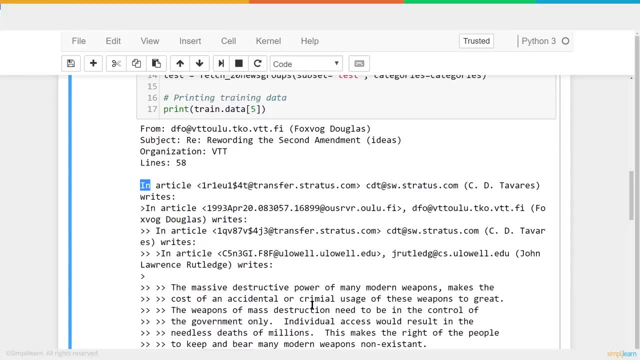 From probably has a very low weight. It has very little value in telling you what this document's about. Same with words like in Article, In articles In Cost of, On, Maybe, cost, might, Or Where words like criminal weapons destruction. 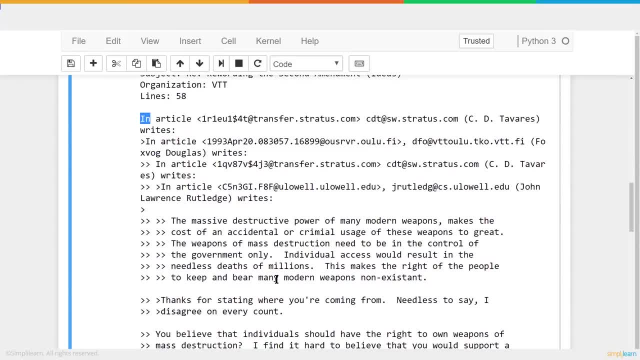 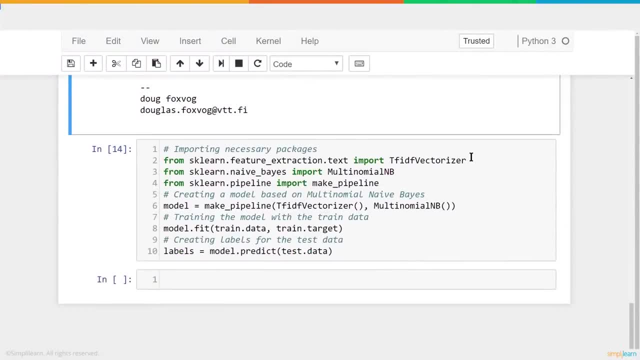 These might have a heavier weight because they describe a little bit more what the article's doing. Well, how do you figure out all those weights in the different articles? That's what this module does. That's what the tfidf vectorizer is going to do for us. 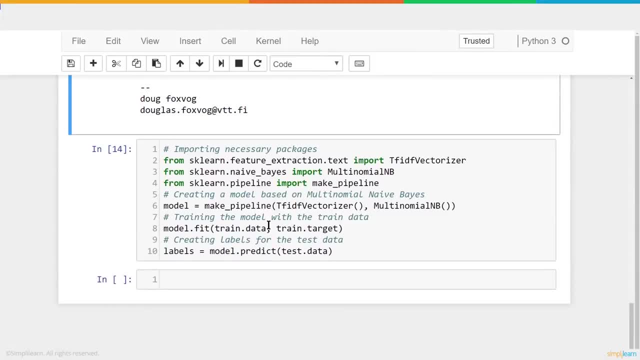 And then we're going to import our sklearnnaivebase And that's our multinomial NB, Multinomial naive base. Pretty easy to understand, Understand that, Where that comes from. And then finally, we have the sklearn pipeline: import, make pipeline. 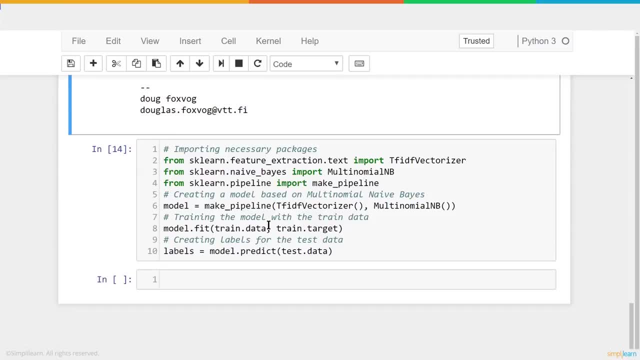 Now the make pipeline is just a cool piece of code because we're going to take the information we get from the tfidf vectorizer and we're going to pump that into the multinomial NB. So a pipeline is just a way of organizing how things flow. 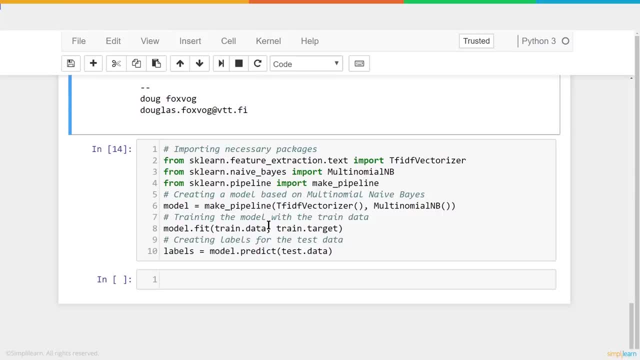 It's used commonly. You probably already guessed what it is. If you've done any businesses, they talk about the sales pipeline. If you're on a work crew or a project manager, you have your pipeline of information that's going through, or your projects and what has to be done, in what order. 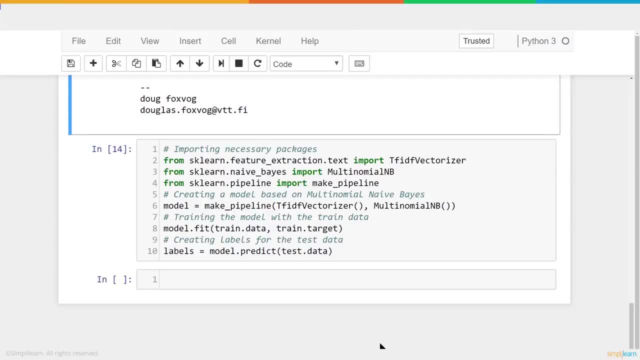 That's all this pipeline is. We're going to take the tfidf vectorizer and then we're going to push that into the multinomial NB. Now we've designated that as the variable model. We have our pipeline model and we're going to take that model, and this is just so elegant. 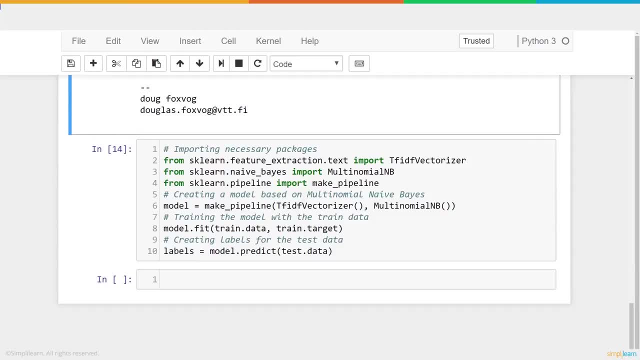 This is done in just a couple lines of code. Modelfit: We're going to fit the data, and first the train data and then the train target. Now the train data has the different articles in it. You can see the one we were just looking at and the traintarget is what category they. 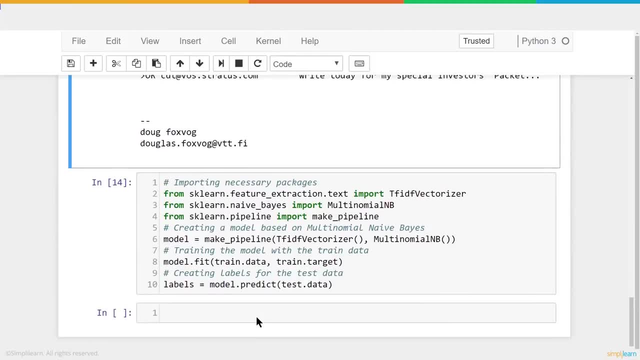 already categorized that particular article as: And what's happening here is the train data is going into the tfid vectorizer. So when you have one of these articles, it goes in there. it weights all the words in there. So there's thousands of words with different weights on them. 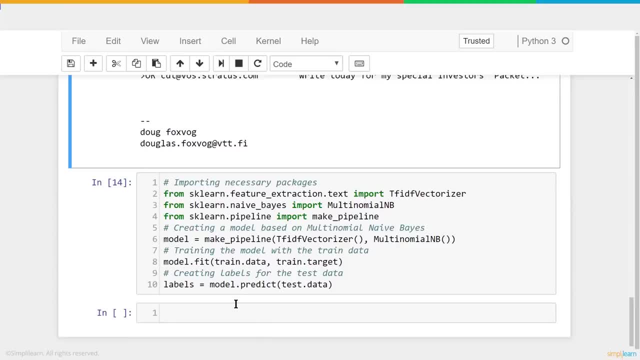 That's what we're going to do. I remember once running a model on this and I literally had 2.4 million tokens go into this. So when you're doing like large document bases, you can have a huge number of different words. 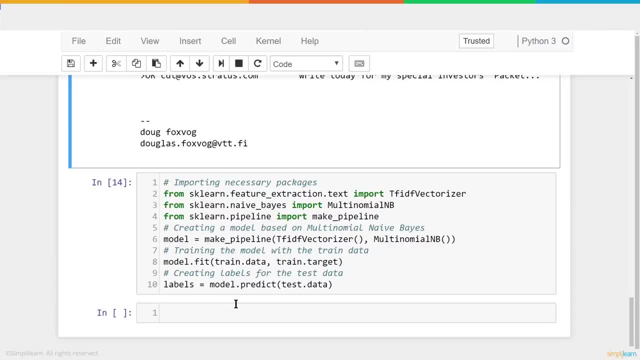 It then takes those words, gives them a weight and then, based on that weight, based on the words and the weights, it then puts that into the multinomial NB And once we go into our naive bays we want to put the train target in there. 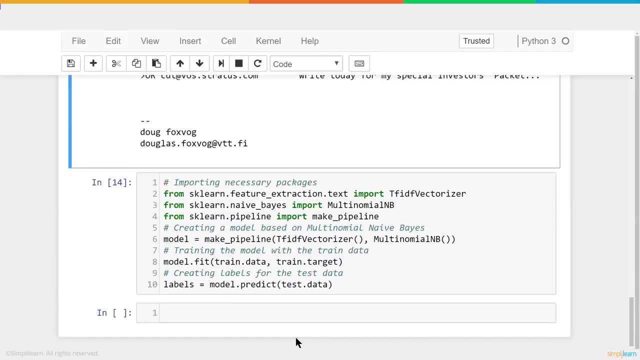 So the train data that's been mapped to the tfid vectorizer Is now going through the multinomial NB, and then we're telling it: well, these are the answers. These are the answers to the different documents. So this document that has all these words, with these different weights, from the first 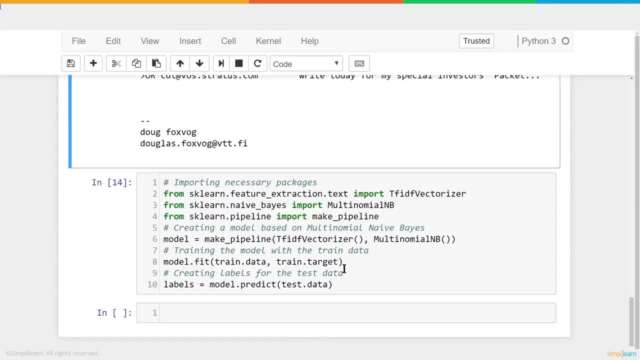 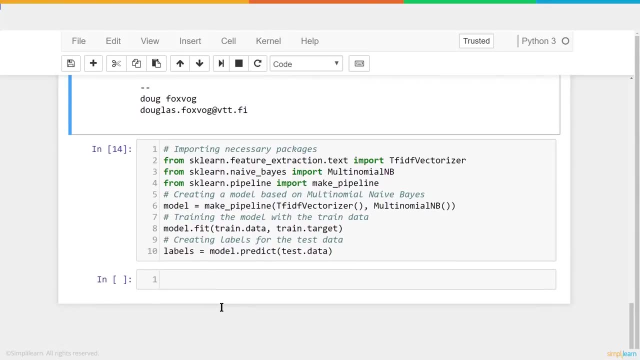 part is going to be, whatever category it comes out of- Maybe it's the talk show or the article on religion- miscellaneous. Once we fit that model, we can then take labels and we're going to set that equal to modelpredict. Most of the sklearn use the term predict. 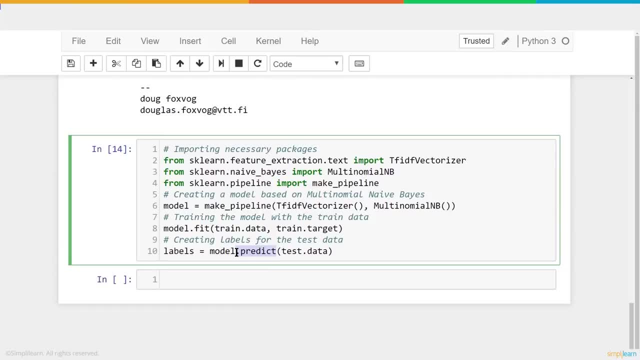 To let us know that we've now trained the model and now we want to get some answers And we're going to put our test data in there, because our test data is the stuff we held off to the side. We didn't train it on there and we don't know what's going to come up out of it and we just 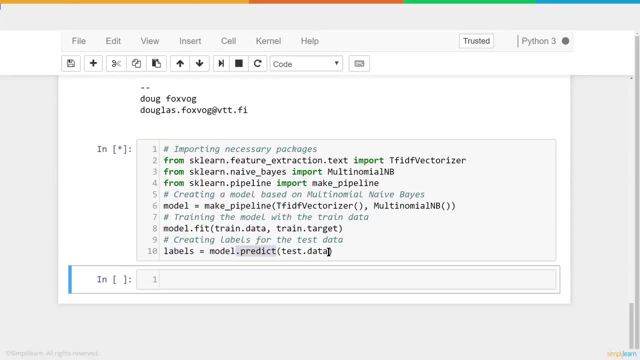 want to find out how good our labels are. Do they match what they should be? Now, I've already run this through. There's no actual output to it to show. This is just setting it all up. This is just training our model, creating the labels, so we can see how good it is and 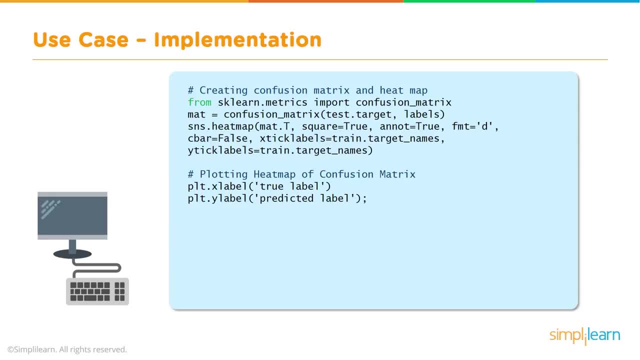 then we move on to the next step: to find out what happened. To do this, we're going to go ahead and create a confusion matrix and a heat map. So the confusion matrix, which is confusing just by its very name, is basically going: 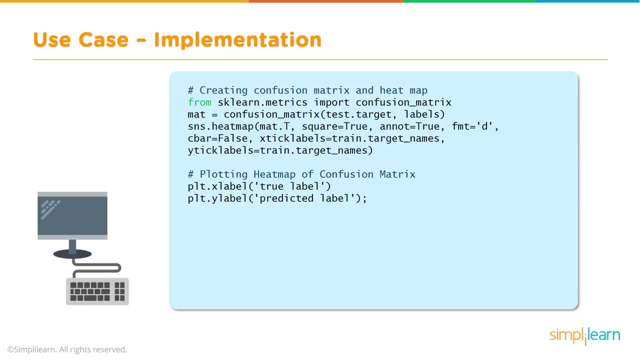 to ask: how confused is our answer? Did it get it correct or did it miss some things in there or have some missed labels? And then we're going to put that on a heat map, so we'll have some nice colors to look at to see how that plots out. 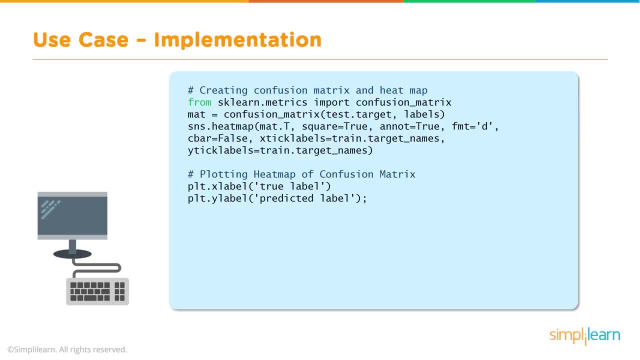 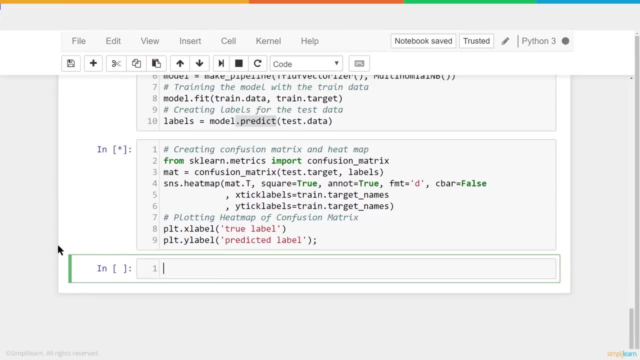 Let's go ahead and take this code and see how that, take a walk through it and see what that looks like. So back to our Jupyter notebook. I'm going to put the code in there and let's go ahead and run that code. 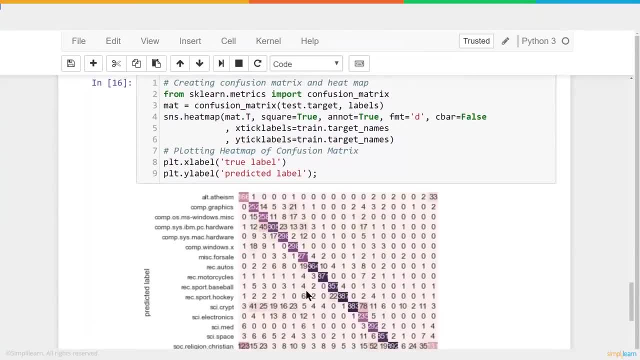 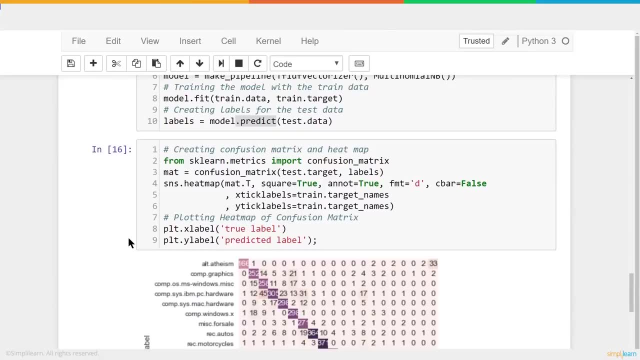 Take it just a moment and remember we had the end line. that way my graph shows up on the end line here And let's walk through the code and then we'll look at this and see what that means. So let me get a little bit bigger. there we go. 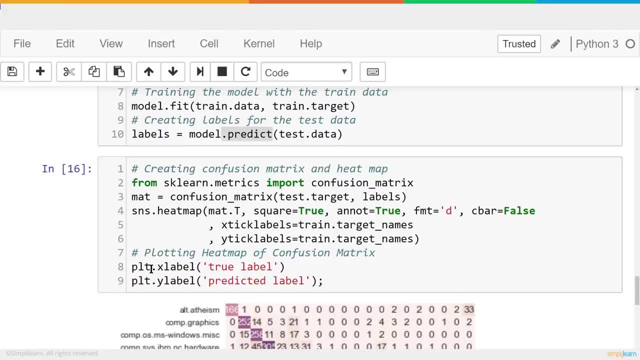 No reason not to use the whole screen too big. So we have here from sklearnmetrics import confusion matrix and that's just going to generate a set of data that says the prediction was such. The actual truth was either agreed with it or it was something different, and it's going. 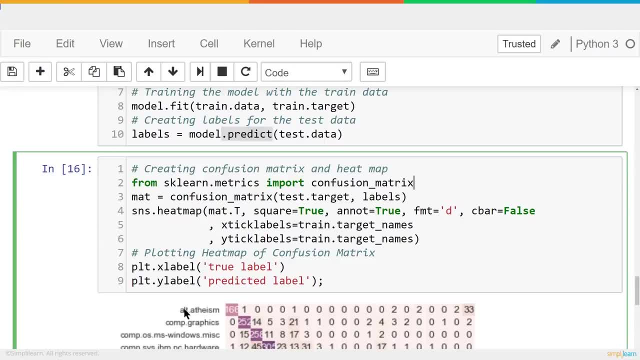 to add up those numbers so we can take a look and just see how well it worked. And we're going to set a variable mat equal to confusion: matrix. We have our test target, our test data. that was not part of the training- Very important in data science. we always keep our test data separate. 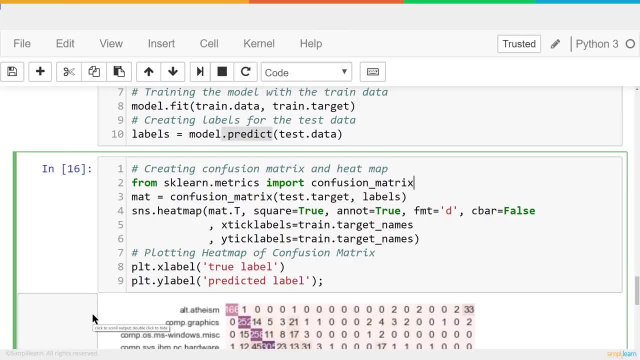 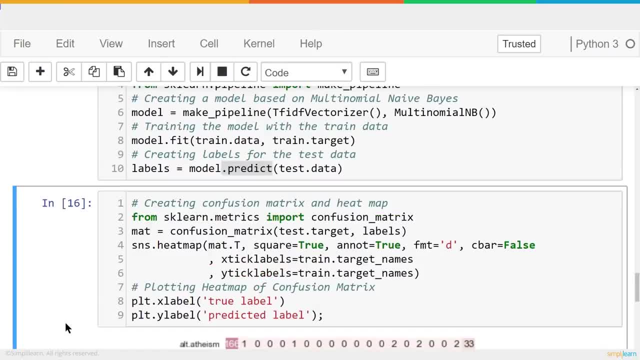 And we're going to go ahead and run that. So we go in and we create our SNHeatMap. The SNS is our seaborne, which sits on top of the pi plot. So we create a SNSheatMap. 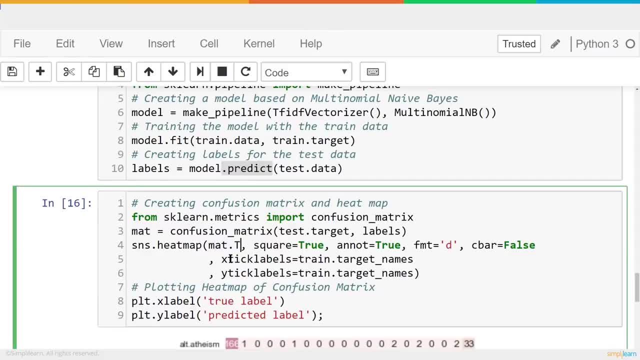 We take our confusion matrix, and it's going to be matt. And do we have other variables that go into the SNSheatMap? We're not going to go into detail what all the variables mean. The annotation equals true. That's what tells it to put the numbers here. 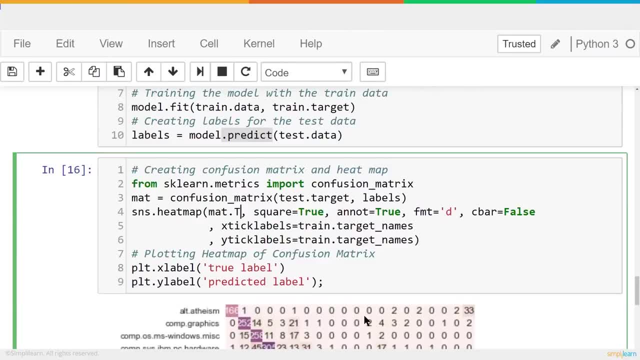 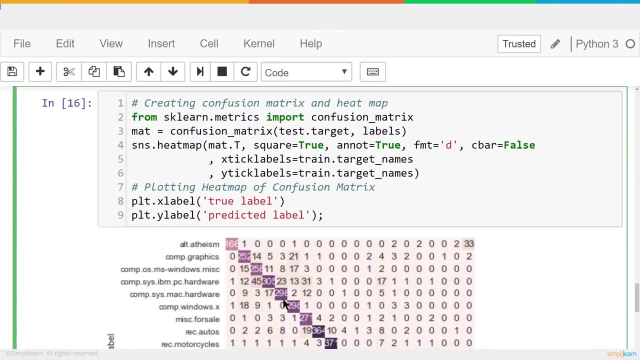 So you have the 166, the 1, the 0001.. Format: Matd and cbar equals false. have to do with the format. If you take those out, you'll see that some things disappear. And then the xtick labels and the ytick labels. those are our target names. 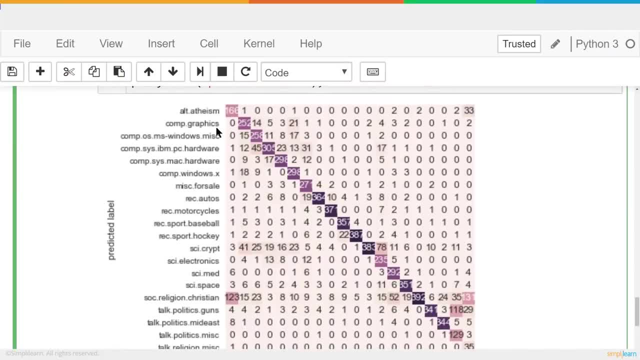 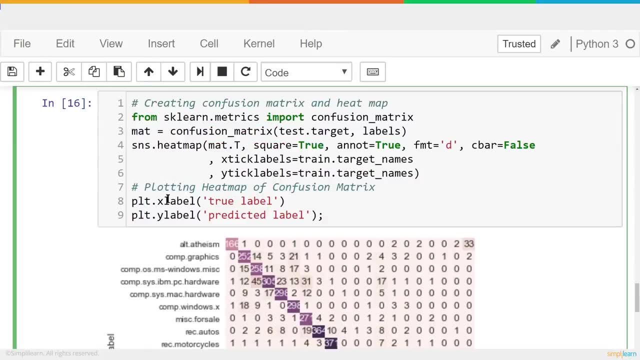 And you can see right here: that's the alt atheism, comp, graphics, comp, osms, windowsmiscellaneous. And then, finally, we have our pltxlabel. Remember the SNS or the seaborne sits on top of our matplotlibrary. our plt. 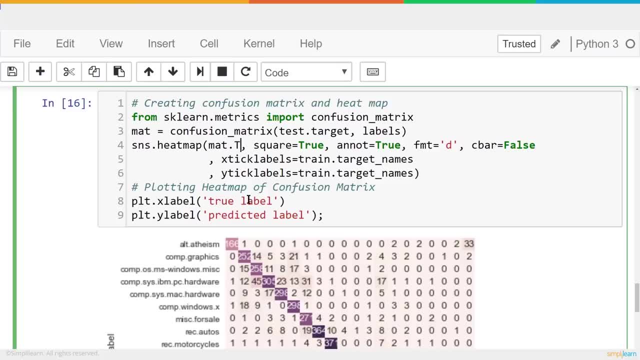 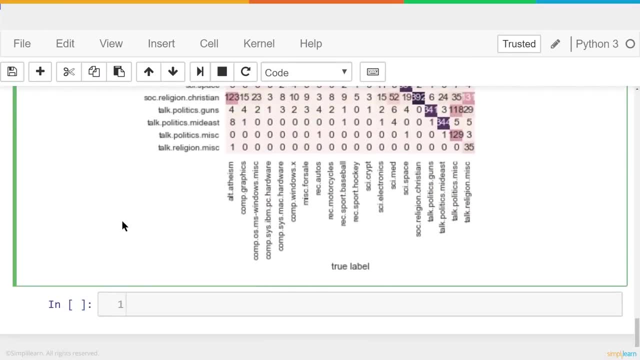 And so we want to just tell it: xlabel equals a true is true, The labels are true. And then the ylabel is prediction label. So when we say a true, this is what it actually is And the prediction is what we predicted. And let's look at this graph, because that's probably a little confusing the way we rattled through it. 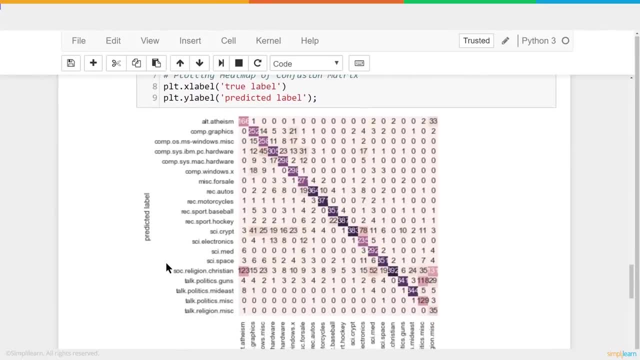 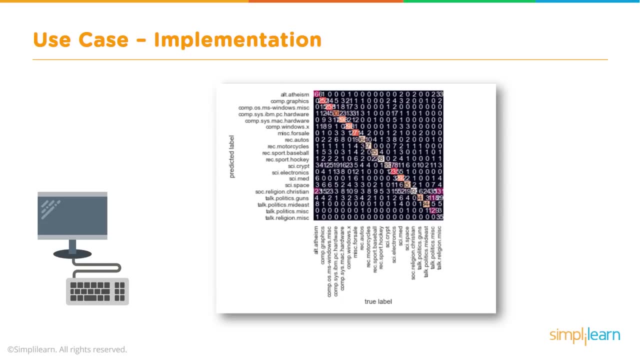 And what I'm going to do is I'm going to go ahead and flip back to the slides, because they have a black background they put in there. that helps it shine a little bit better so you can see the graph a little bit easier. So in reading this graph, what we want to look at is how the color scheme has come out. 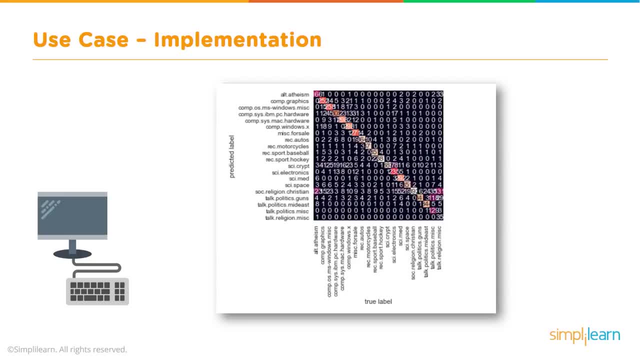 And you'll see a line Right down the middle diagonally from upper left to bottom right. What that is is, if you look at the labels, we have our predicted label on the left and our true label on the right. Those are the numbers where the prediction and the true come together. 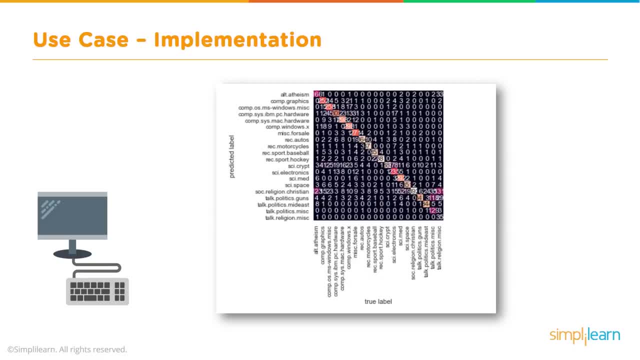 And this is what we want to see- is we want to see those lit up. That's what that heat map does is. you can see that it did a good job of finding those data And you'll notice that there's a couple of red spots on there where it missed. 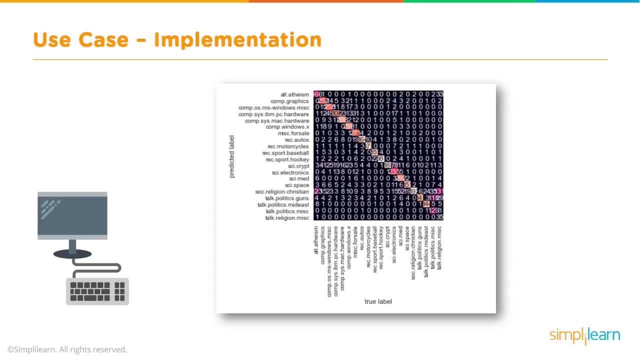 You know it's a little confused. We talk about talk religion- miscellaneous- And then we talk about what's missing, And then we talk about what's missing, And then we talk about what's missing Versus talk politics- miscellaneous. 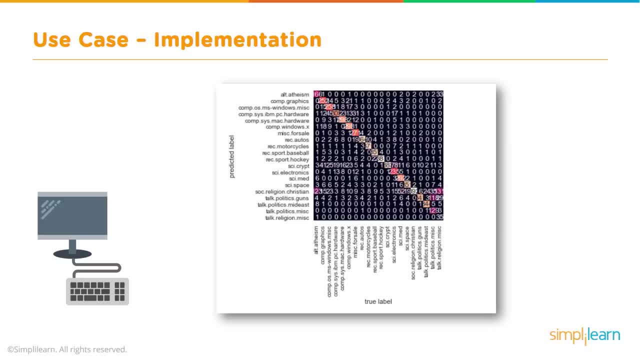 Social religion, Christian versus alt-atheism. It mislabeled some of those, And those are very similar topics, So you could understand why it might mislabel them, But overall, it did a pretty good job. If we're going to create these models, we want to go ahead and be able to use them. 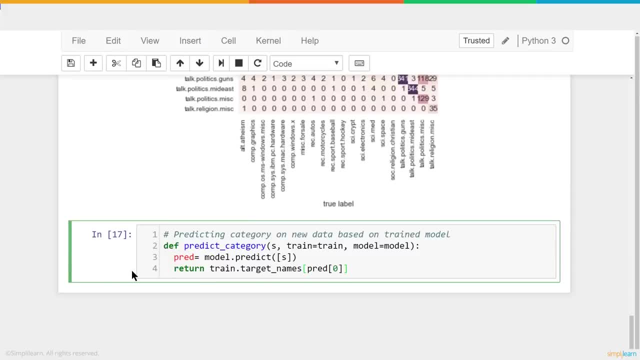 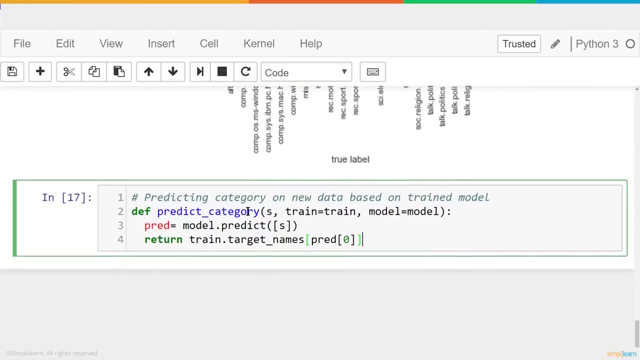 So let's see what that looks like. To do this, let's go ahead and create a definition, a function to run, And we're going to call this function. Let me just expand that just a notch here. There we go. I like mine in big letters. 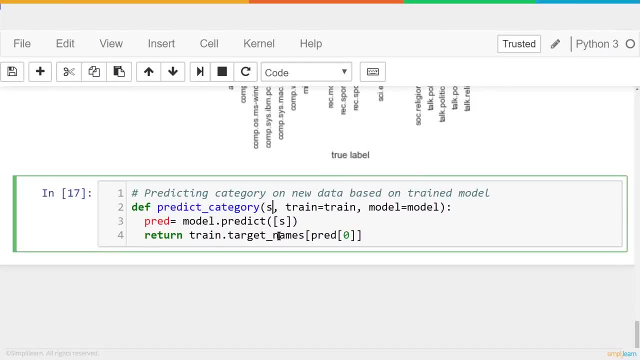 Predict categories. We want to predict the category. We're going to send it s a string And then we're sending it train equals train. We have our training model And then we had our pipeline model equals model. This way, we don't have to resend these variables each time. 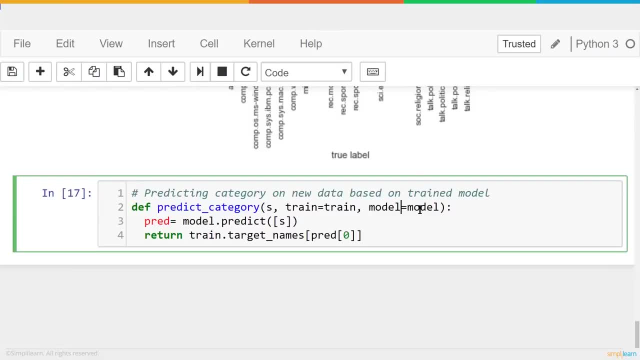 The definition knows that because I said train equals train And I put the equal for model And then we're going to set the prediction equal to the modelpredict s. So it's going to send whatever string we send to it. It's going to push that string through the pipeline. 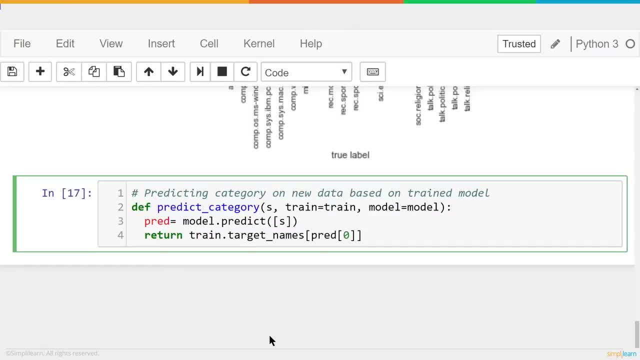 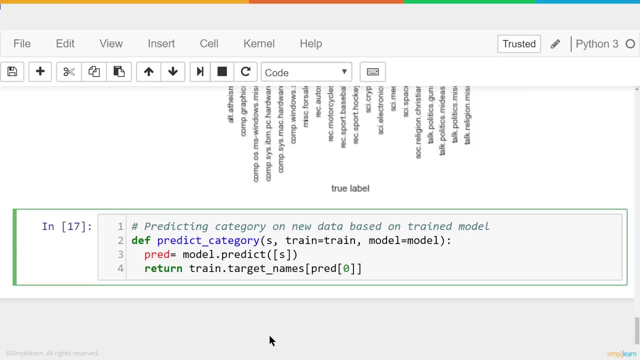 in the model pipeline. It's going to go through and tokenize it and put it through the tf, idf, convert that into numbers and weights for all the different documents and words, And then it'll put that through our naive bays And from it we'll go ahead and get our prediction. 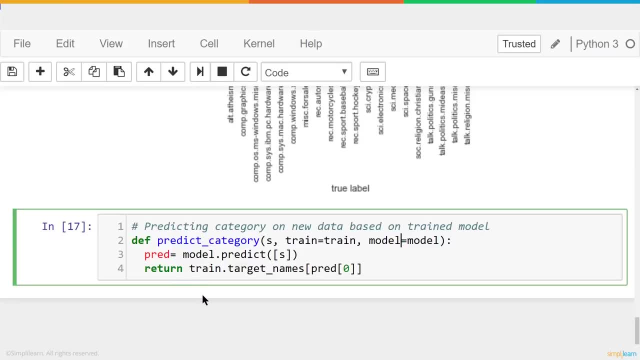 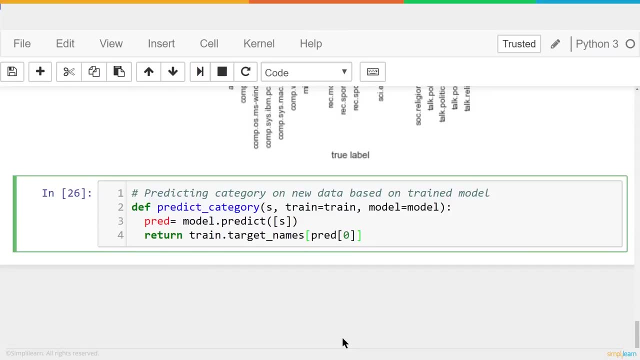 We're going to predict what value it is, And so we're going to return traintargetNamesPredict of zero. And remember that the traintargetNames, that's just categories. I could have just as easily put categories. I could have just as easily put categories in there. predict of zero. 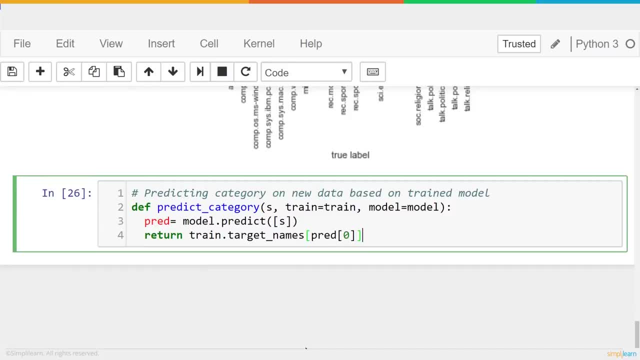 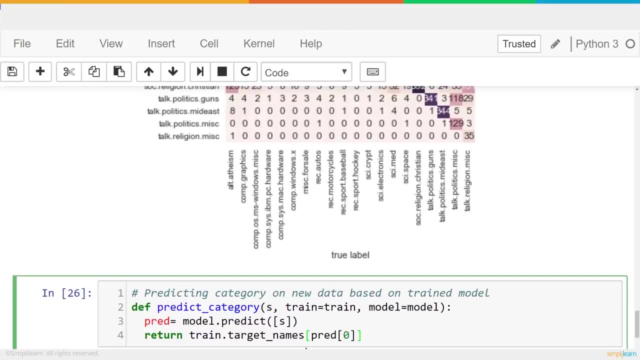 So we're taking the prediction, which is a number, and we're converting it to an actual category. We're converting it from. I don't know what the actual numbers are, But let's say, zero equals alt atheism. So we're going to convert that zero to the word. 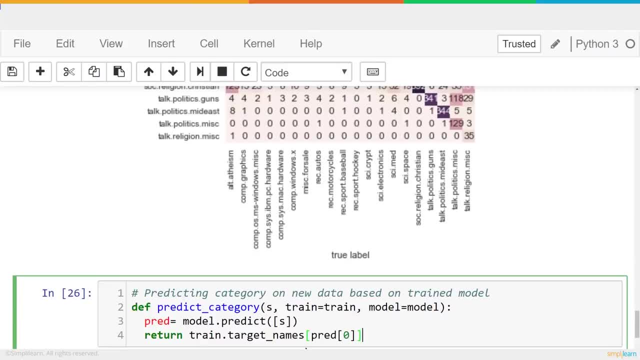 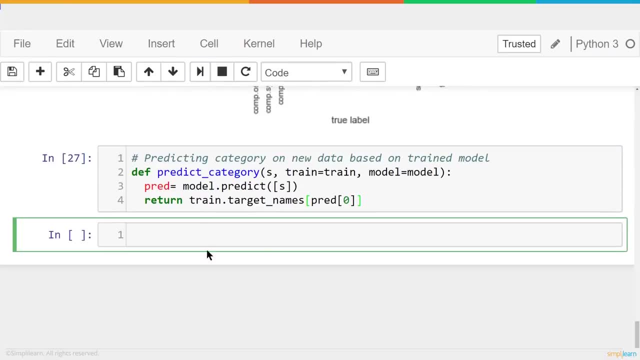 Or one. maybe it equals comp graphics. So we're going to convert number one into comp graphics. That's all that is. And then we got to go ahead, and and then we need to go ahead and run this, So I load that up. 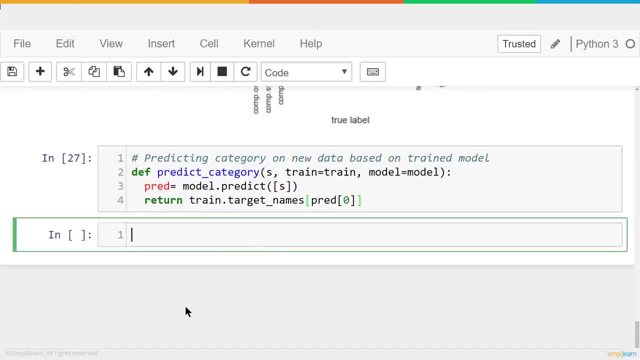 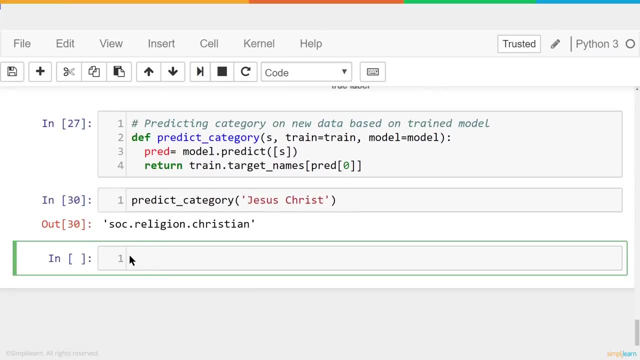 And then once I run that, we can start doing some things. I'm going to go ahead and type in predict category And let's just do predict category Jesus Christ And it comes back and says it's social religion, Christian. 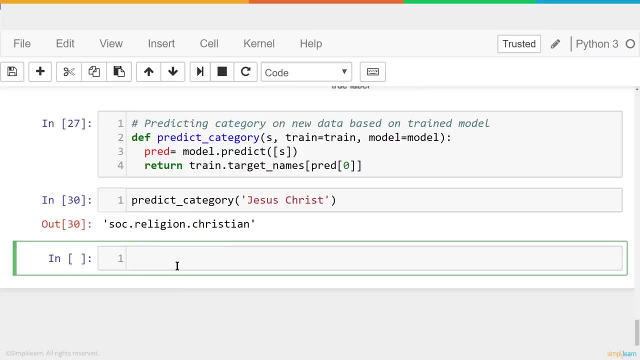 That's pretty good. Now note I didn't put print on this. One of the nice things about the Jupyter Notebook editor and a lot of inline editors is if you just put the name of the variable out, it's returning the variable traintarget, underscore names. 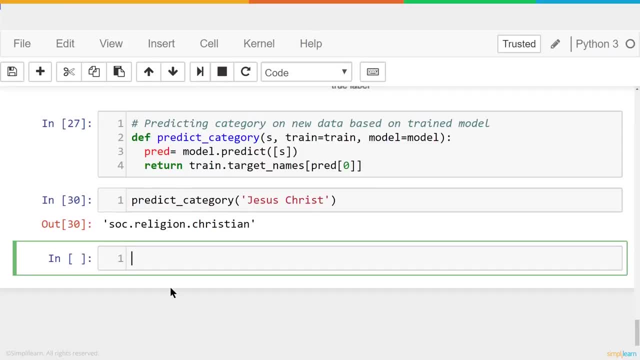 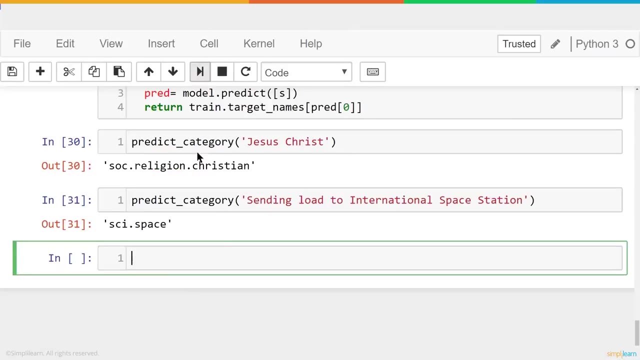 it'll automatically print that for you In your own ID. you might have to put in print. Let's see where else we can take this. And maybe you're a space science buff. So how about sending load to international space station? And if we run that, we get science space. or maybe you're a automobile buff. 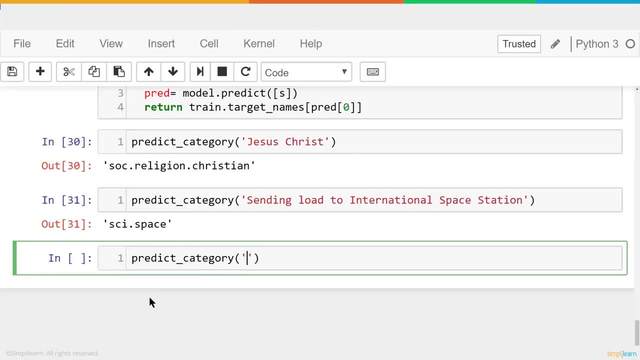 And let's do. they're going to tell me Audi is better than BMW. but I'm going to do BMW is better than an Audi. So maybe you're a car buff And we run that And you'll see. it says recreational. 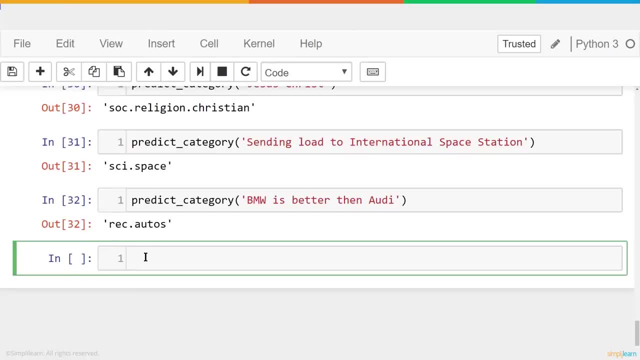 I'm assuming that's what REC stands for- Autos, So I did a pretty good job labeling that one. How about if we have something like a caption running through there, President of India- And if we run that it comes up and says: talk politics, miscellaneous. 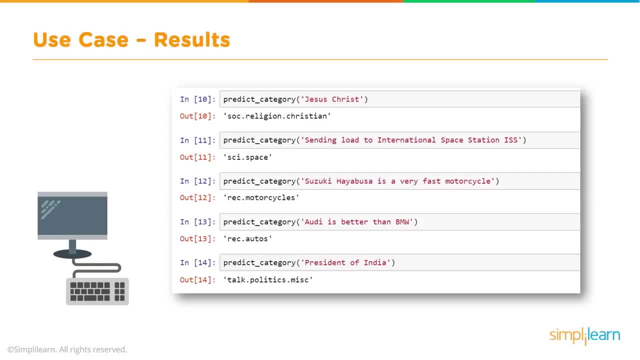 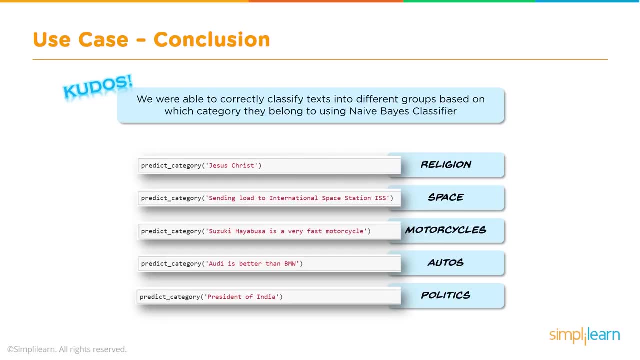 So when we take our definition, our function and we run all these things through kudos, we made it We were able to correctly classify texts into different groups, based on which category they belong to, using the Naive Bayes classifier. 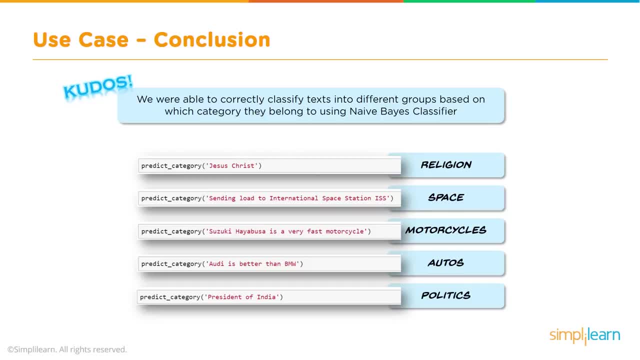 Now we did throw in the pipeline the TF-IDF vectorizer, We threw in the graphs. Those are all things that you don't necessarily have to know to understand the Naive Bayes setup or classifier, But they're important to know. 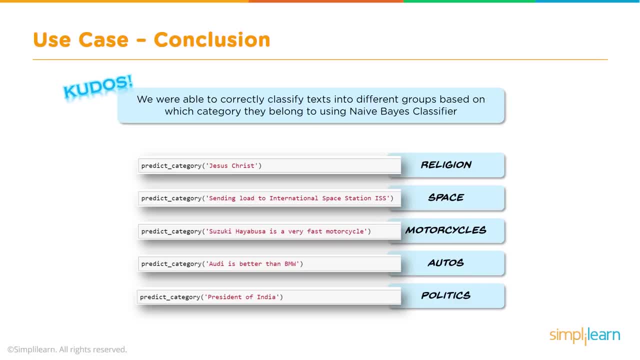 One of the main uses for the Naive Bayes is with the TF-IDF tokenizer or vectorizer, where it tokenizes a word and has labels, And we use the pipeline because you need to push all that data through and it makes it really easy. 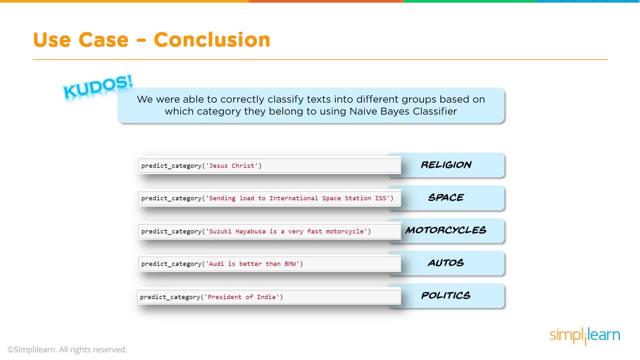 And fast. You don't have to know those to understand Naive Bayes, but they certainly help for understanding the industry and data science. And we can see our categorizer, our Naive Bayes classifier. We were able to predict the category- religion, space, motorcycles, autos, politics- and properly classify all these different things. we pushed into our prediction and our trained model. 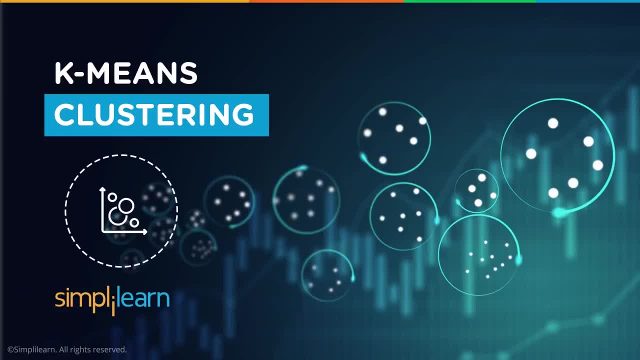 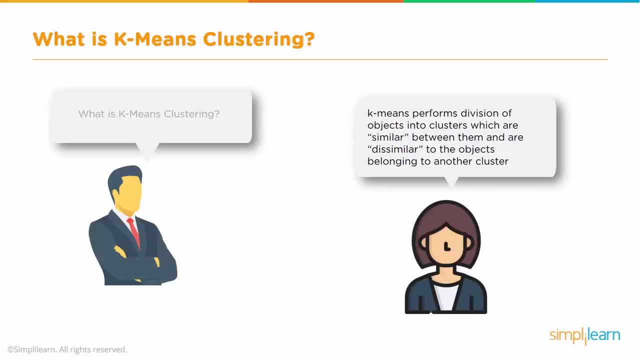 Hello and welcome to the session on k-means clustering. I'm Mohan Kumar from Simply Learn. So what is k-means clustering? K-means clustering is an unsupervised learning algorithm. In this case you don't have labeled data, unlike in supervised learning. 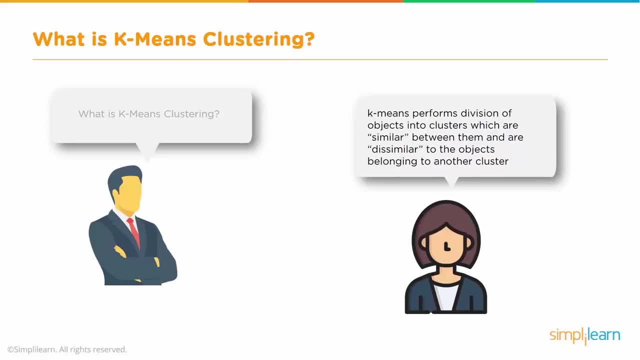 So you have a set of data and you want to group them And, as the name suggests, you want to put them into clusters, which means objects that are similar in nature, similar in characteristics, need to be put together. So that's what k-means clustering is all about. 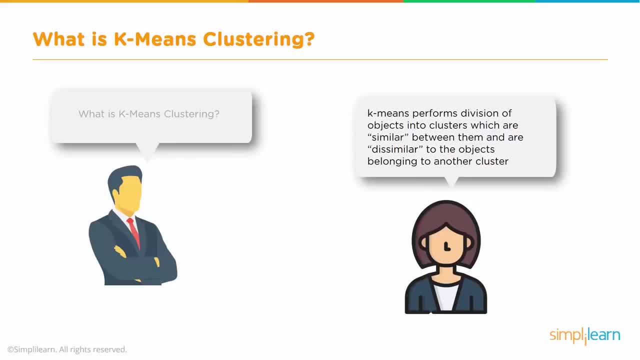 The term k is a term that is used to describe the structure of an object. This, basically, is a number, So we need to tell the system how many clusters we need to perform. So if k is equal to two, there will be two clusters. 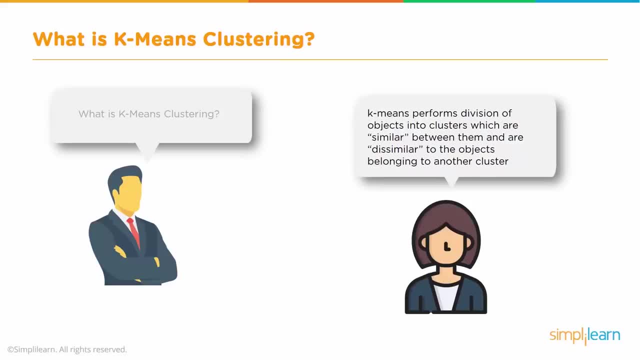 If k is equal to three, three clusters and so on and so forth. That's what the k stands for And of course there is a way of finding out what is the best or optimum value of k for a given data. We will look at that. 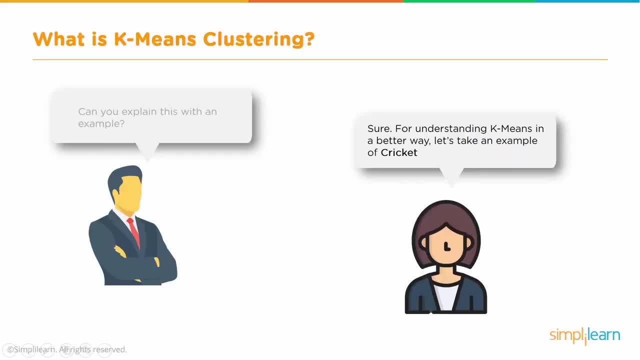 So that is k-means clustering. So let's take an example. K-means clustering is used in many, many scenarios. But let's take an example, An example of cricket, the game of cricket. Let's say you received data of a lot of players from maybe all over the country or all over the world. 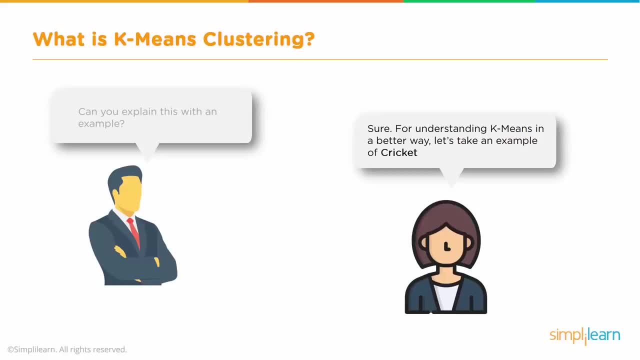 And this data has information about the runs scored by the people or by the player and the wickets taken by the player, And, based on this information, we need to cluster this data into two clusters: batsmen and bowlers. So this is an interesting example. 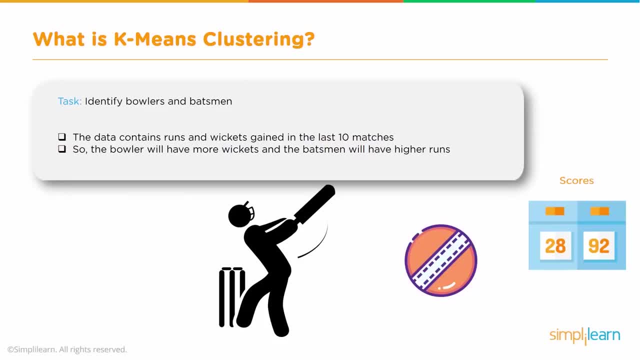 Let's see how we can perform this. So we have the data, which consists of primarily two characteristics, which is the runs and the wickets. So the bowlers basically take wickets and the batsmen score runs. There will be, of course, a few bowlers who can score some runs. 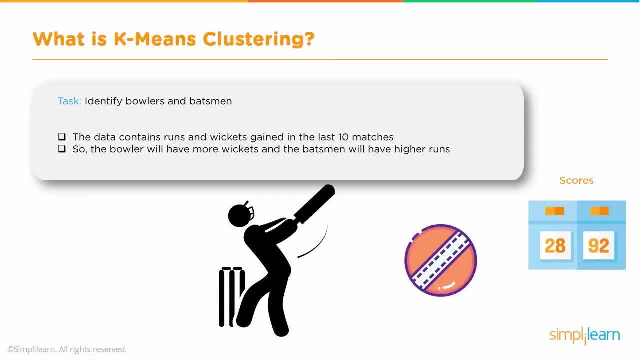 And similarly, there will be some batsmen who would have taken a few wickets, But with this information, we want to cluster those players into batsmen and bowlers. So how does this work? Let's say: this is how the data is. 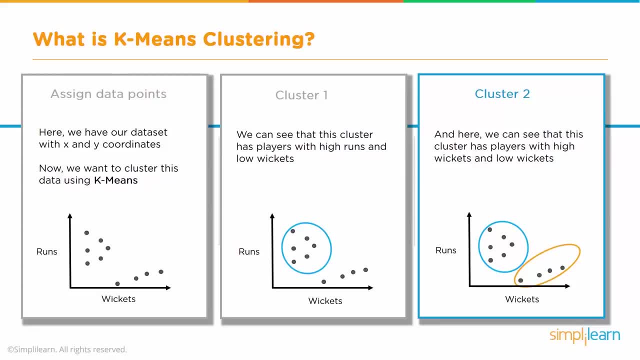 So there are information. There is information on the y-axis about the runs scored and on the x-axis about the wickets taken by the players. So if we do a quick plot, this is how it would look And when we do the clustering, we need to have the clusters, like shown in the third diagram, out here. 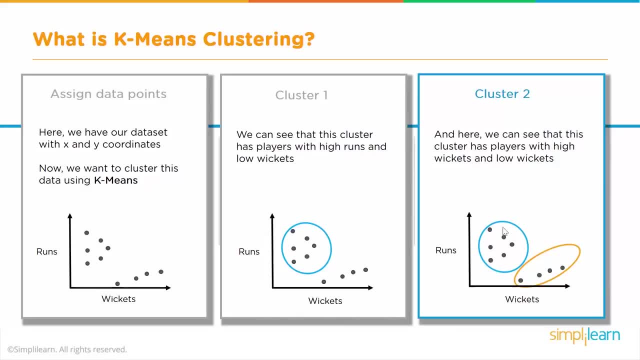 So we need to have a cluster which consists of people who have scored high runs, which is batsmen, And then we need a cluster with people who have taken a lot of wickets, which is typically the bowlers. There may be a certain amount of overlap, but we will not talk about it right now. 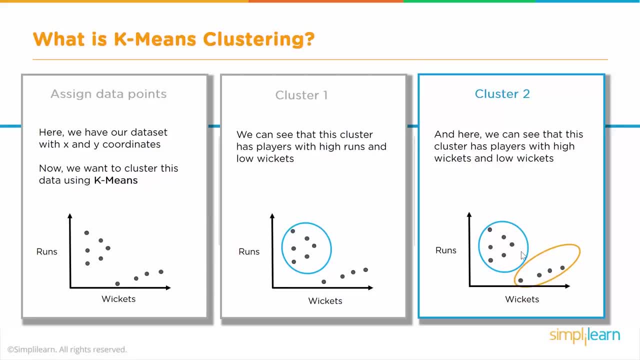 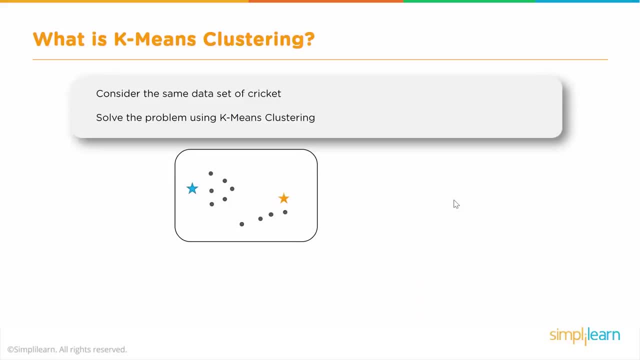 So with k-means clustering we will have here That means k is equal to two and we will have two clusters, which is batsmen and bowlers. So how does this work? The way it works is: the first step in k-means clustering is the allocation of two centroids randomly. 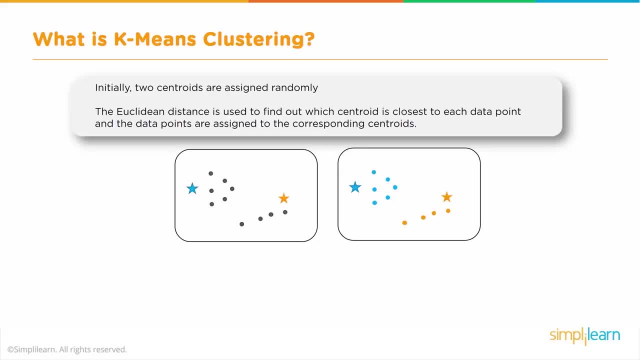 So two points are assigned as so-called centroids. So in this case we want two clusters, which means k is equal to two. So two points have been randomly assigned as centroids. Keep in mind: these points can be anywhere. There are random points. 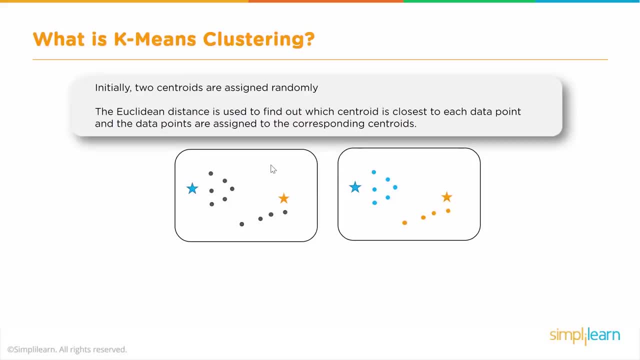 They are not initially. They are not really the centroids. Centroid means it's a central point of a given data set, But in this case It starts off. It's not really the centroid. OK, so these points, though in our presentation here we have shown them one point closer to these data points and another closer to these data points. 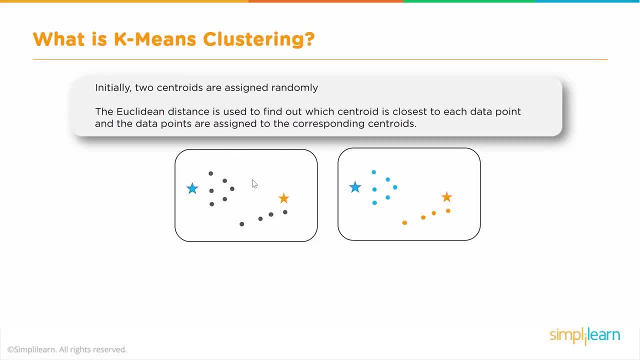 They can be assigned randomly anywhere. OK, so that's the first step. The next step is to determine the distance of each of the data points from each of the randomly assigned centroids. So, for example, we take this point and find the distance. 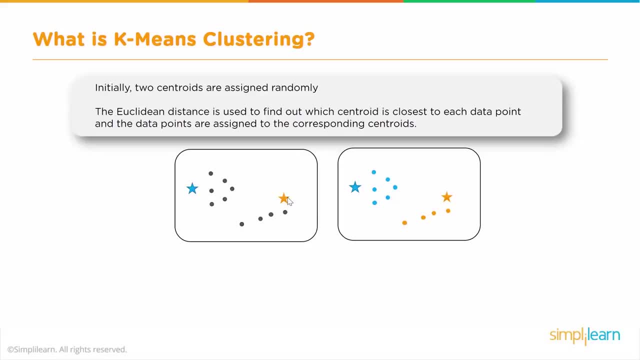 From this centroid and the distance from this centroid This point is taken and the distance is from from this centroid, and second, and so on and so forth. So for every point the distance is measured from both the centroids and then whichever distance is less, that point is assigned to that centroid. 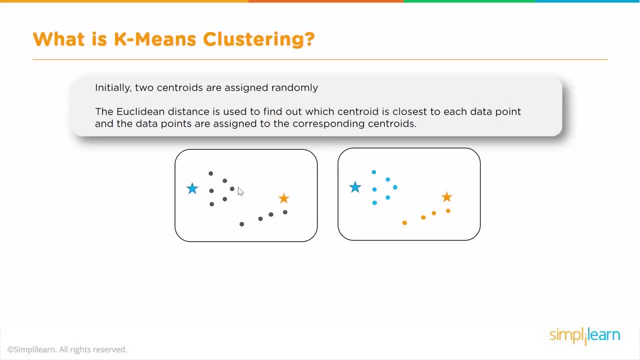 So, for example, in this case, visually, it is very obvious that all these data points are assigned to the centroid and all these data points assigned to this centroid, And that's what is represented here in blue color and in this yellow color. The next step is to actually determine the central point or the actual centroid for these two. 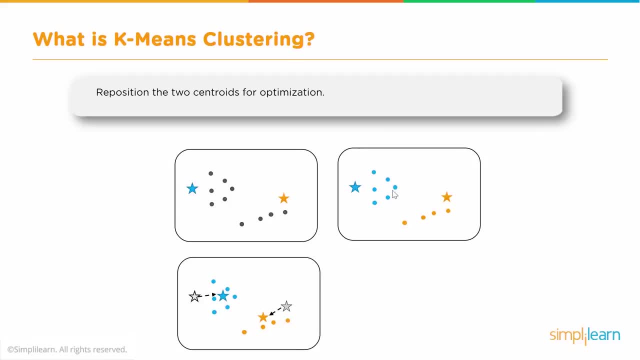 clusters. So we have this one initial cluster, this one initial cluster, But, as you can see, these points are not really the centroid. Centroid means it should be the central position of this data set, central position of this data set. So that is what needs to be determined as the next. 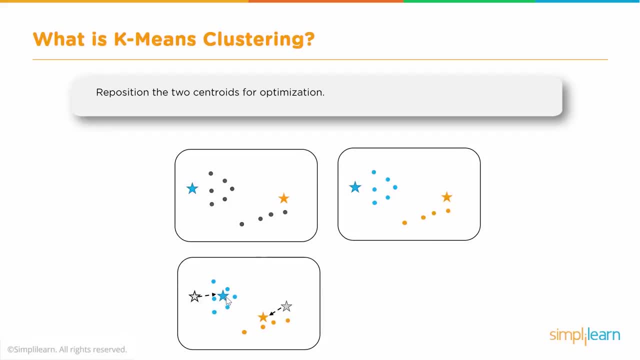 step. So the central point or the actual centroid is determined and the original randomly allocated centroid is repositioned to the actual centroid of these new clusters And this process is actually repeated. Now what might happen is some of these points may get reallocated. In our example that 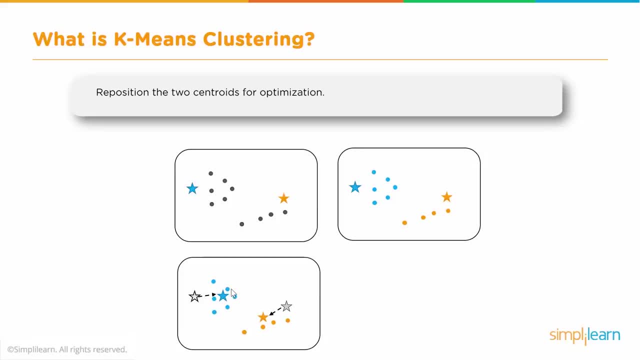 is not happening, probably, but it may so happen That the distance is found between each of these data points, once again, with these centroids, And if there is, if it is required, some points may be reallocated. We will see that in a later example. 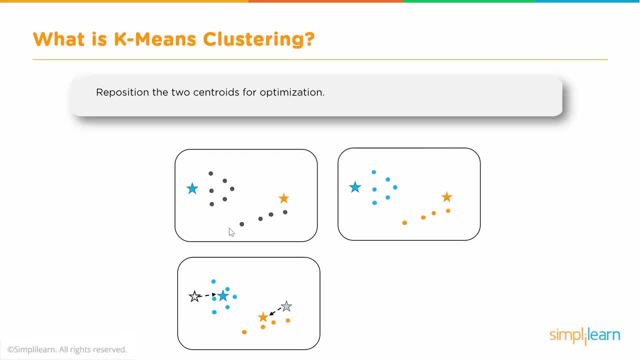 but for now we will keep it simple. So this process is continued till the centroid repositioning stops And that is our final cluster. So this is our. so, after iteration, we come to this position, this situation where the centroid doesn't need. 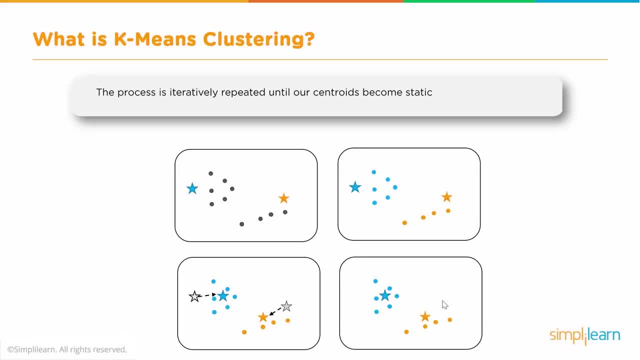 any more repositioning And that means our algorithm has converged, Convergence has occurred and we have the cluster, two clusters, We have the clusters with a centroid. So this process is repeated. The process of calculating the distance and repositioning the centroid is repeated till 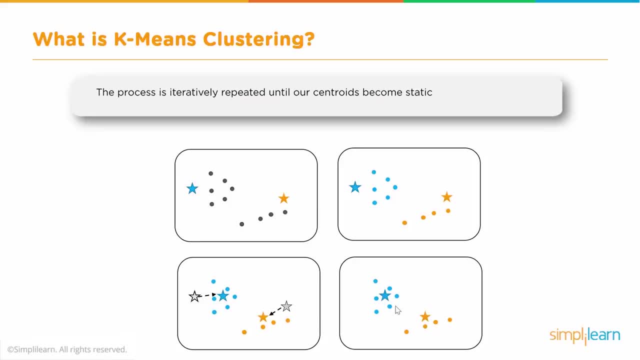 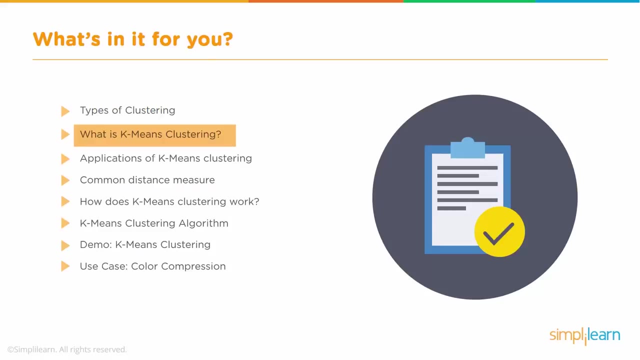 the repositioning stops, which means that the algorithm has converged And we have the final cluster with the data points and the centroids. So this is what you're going to learn from this session. We will talk about the types of clustering. What is k-means? clustering, Application of k-means. 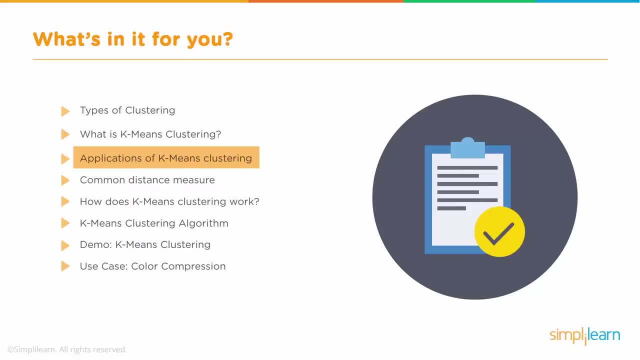 clustering. K-means clustering is done using distance measure, So we will talk about the common distance measures And then we will talk about how k-means clustering works and go into the details of k-means clustering algorithm, And then we will end with a demo and a use case for 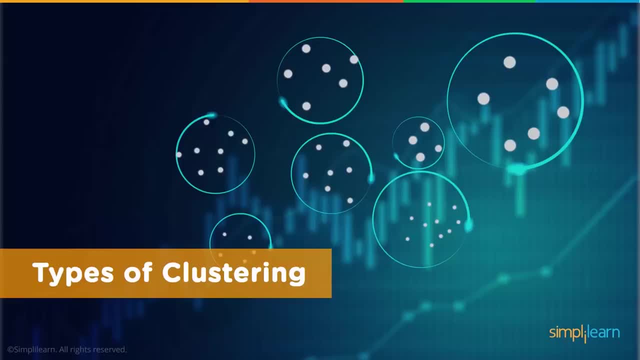 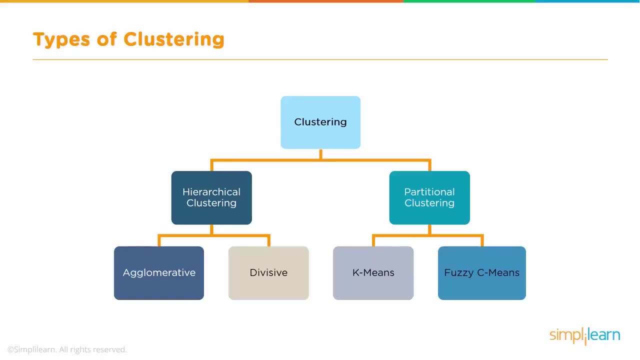 k-means clustering. So let's begin. First of all, what are the types of clustering? There are primarily two categories of clustering: Hierarchical clustering and then partitional clustering- And each of these categories are further subdivided into agglomerative and divisive clustering, and 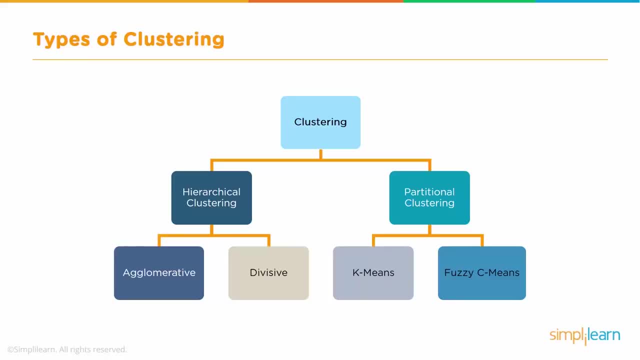 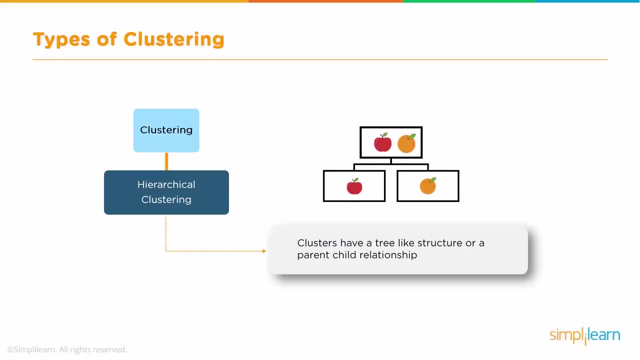 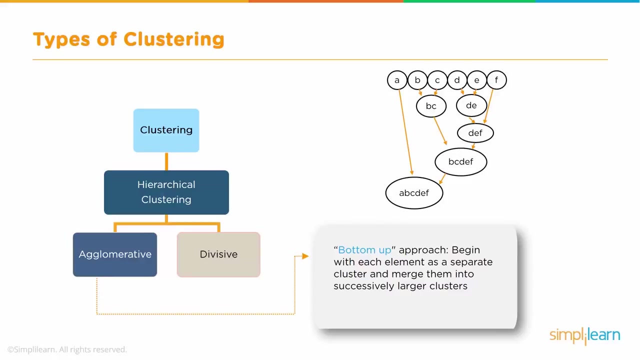 k-means and fuzzy c-means clustering. Let's take a quick look at what each of these types of clustering are. In hierarchical clustering, the clusters have a tree-like structure, and hierarchical clustering is further divided into agglomerative and divisive Agglomerative. 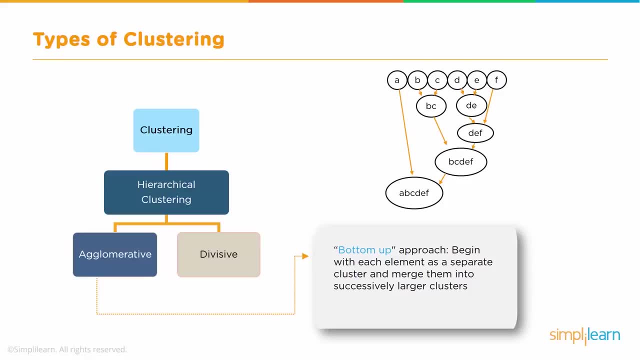 clustering is a bottom-up approach. We begin with each element as a separate cluster and merge them into successively larger clusters. So, for example, we have a, b, c, d, e, f. We start by combining b and c form one cluster, d and e form one more. Then we combine d, e and f, one more bigger. 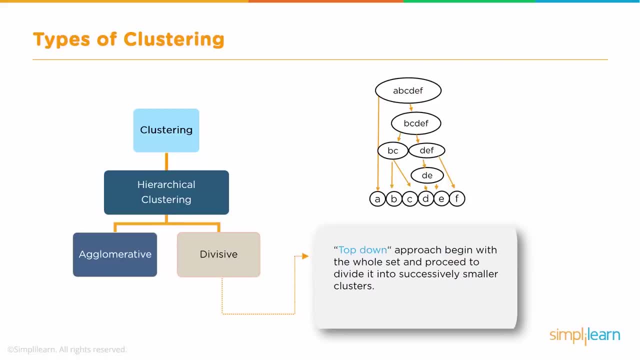 cluster and then add b, c to that and then finally a to it. Compared to that, we have a divisive clustering, or divisive clustering is a top-down approach. We begin with the whole set and proceed to divide it into successively smaller clusters. So we have a, b, c, d, e, f. We first 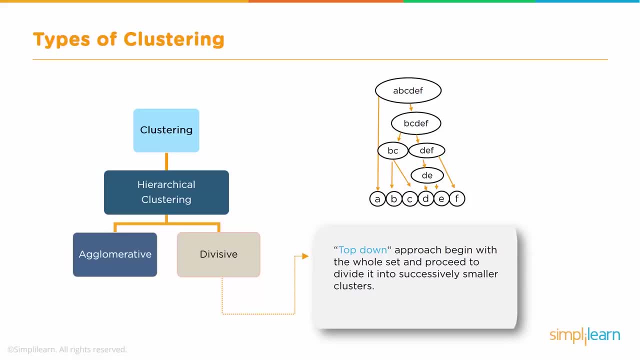 take that as a single cluster and then break it down into a, b, c, d, e and f. Then we have partitional clustering, split into two subtypes: k-means clustering and fuzzy c-means. In k-means. 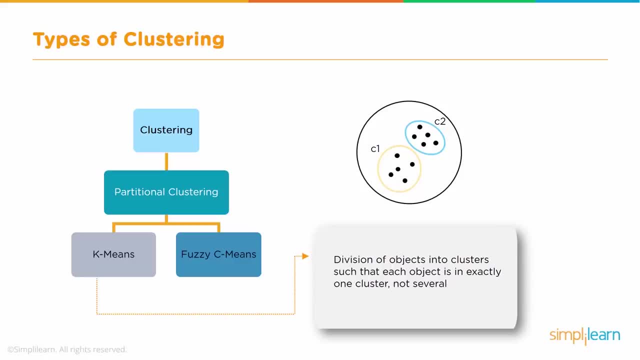 clustering. we divide it into the number of clusters mentioned by the number k. That's where the k comes from. So if we say k is equal to two, the objects are divided into two clusters: c1 and c2.. And the way it is done is the features or characteristics are compared and all objects 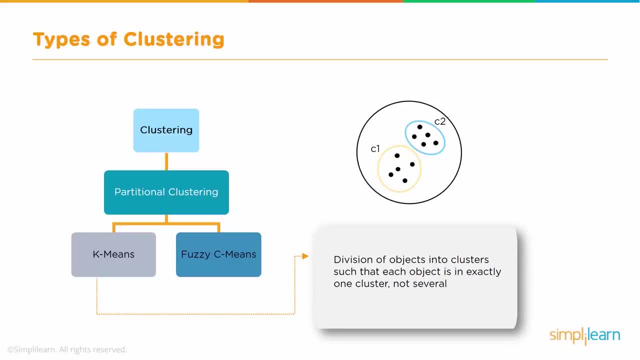 having similar characteristics are clubbed together. So that's how k-means clustering is done. We will see it in more detail as we move forward. And fuzzy c-means is very similar to k-means in the sense that it clubs objects that have similar characteristics together. But while in 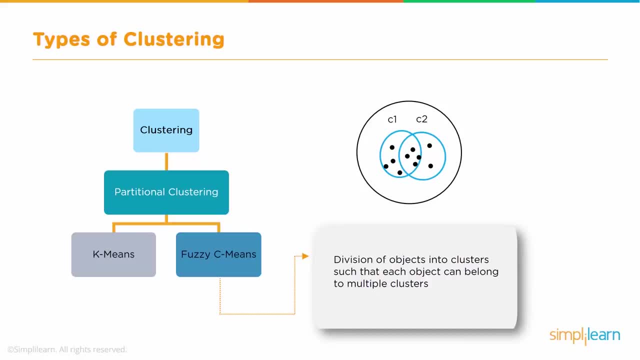 k-means clustering two objects cannot belong to or any object. a single object cannot belong to two different clusters. in c-means, objects can belong to more than one cluster. So that is the primary difference between k-means and fuzzy c-means. So what are some of the applications? 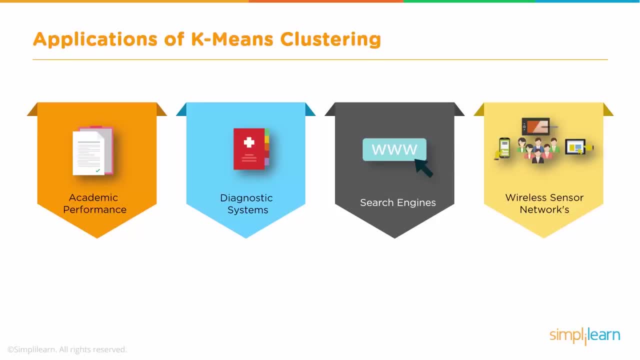 of k-means clustering. k-means clustering is used in a variety of examples or variety of business cases in real life, starting from academic performance diagnostic systems, search engines and wireless sensor networks and many more. So let us take a little deeper look at. 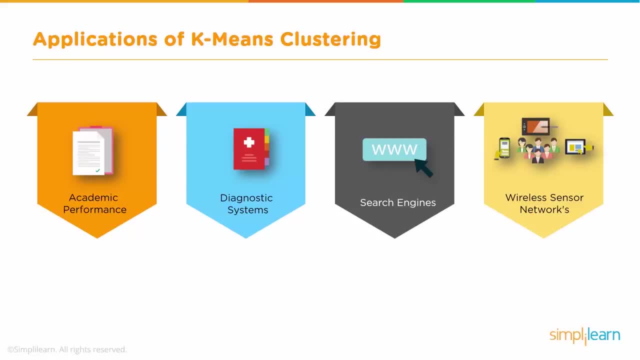 each of these examples Academic performance. So, based on the scores of the students, students are categorized into A, B, C and so on. Clustering forms the backbone of search engines. When a search is performed, the search results need to be grouped together. The search engines very often. 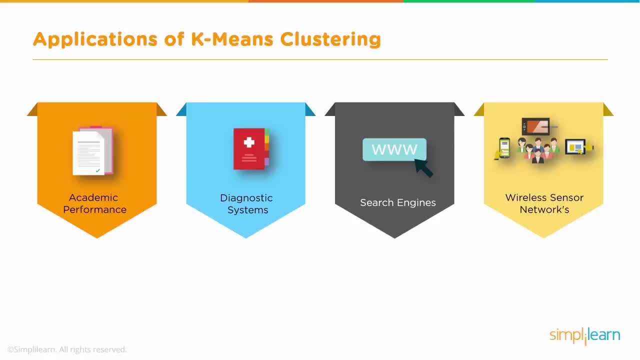 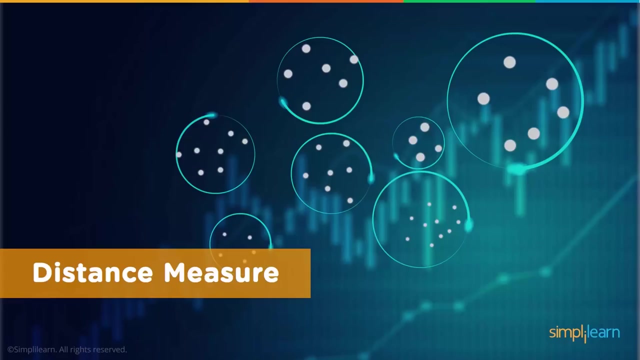 use clustering to do this, And similarly, in case of wireless sensor networks, the clustering algorithm plays the role of finding the cluster heads, which collects all the data in its respective cluster. So clustering, especially k-means clustering, uses distance measure. So 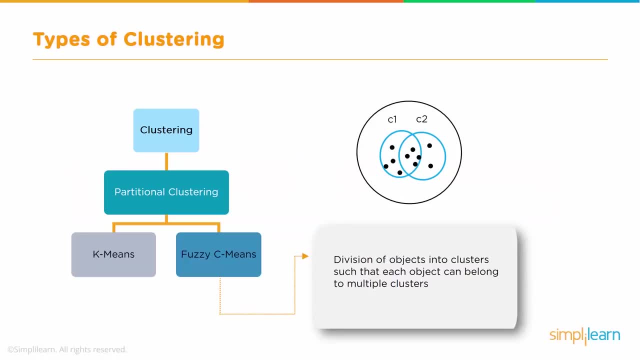 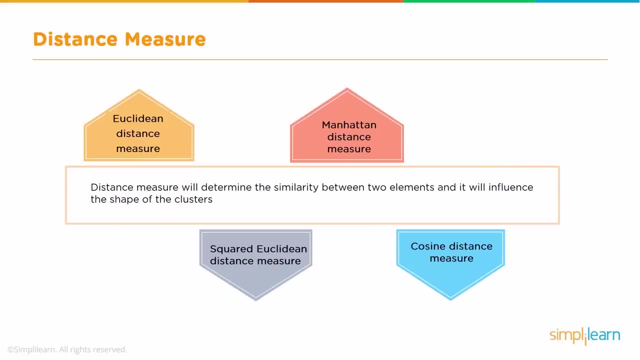 let us take a look at what is distance measure. So, while these are the different types of clustering, in this video we will focus on k-means clustering. So distance measure tells how similar some objects are. So the similarity is measured using what is known as. 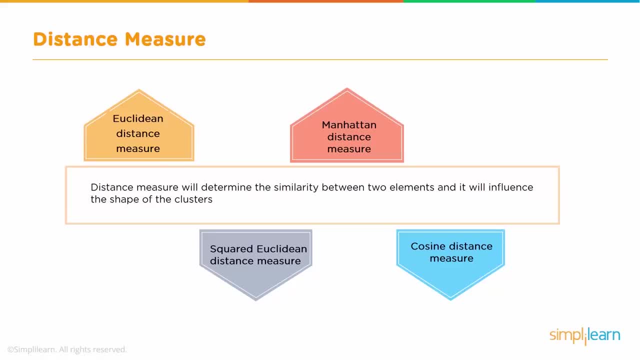 distance measure And what are the various types of distance measures? There is Euclidean distance, there is Manhattan distance, then we have squared Euclidean distance measure and cosine distance measure. These are some of the distance measures supported by k-means clustering. Let us take a look. 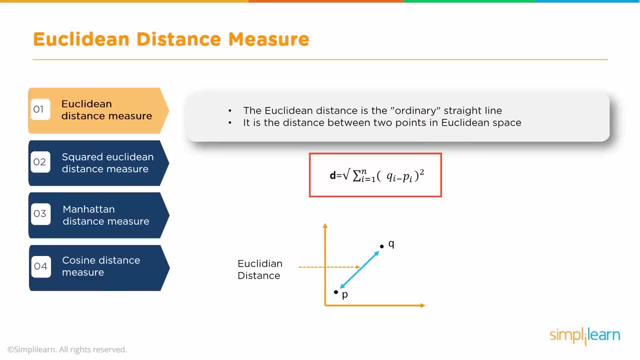 at each of these. What is Euclidean distance measure? Well, Euclidean distance measure is a distance measure. This is nothing but the distance between two points. So we have learned in high school how to find the distance between two points. This is a little sophisticated formula for that. 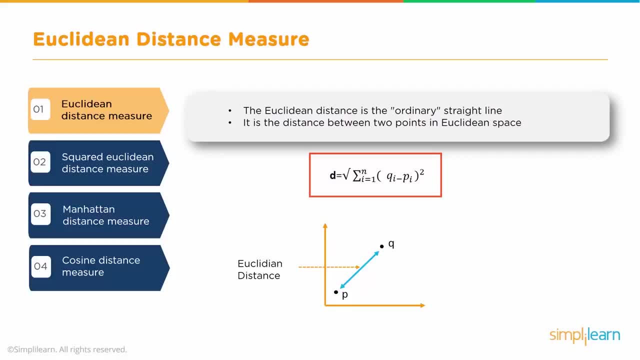 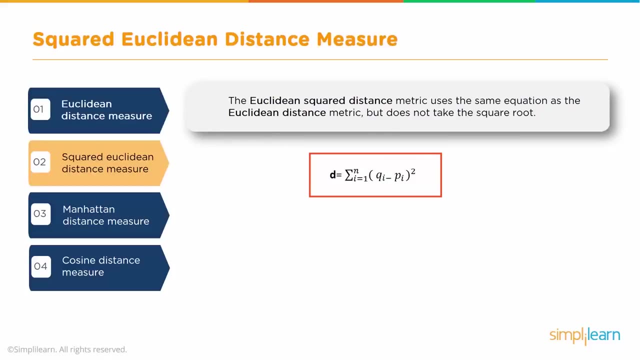 but we know a simpler one: is square root of y2 minus y1 whole square, plus x2 minus x1 whole square. So this is an extension of that formula. So that is the Euclidean distance between two points. What is the squared Euclidean distance measure? It's nothing but. 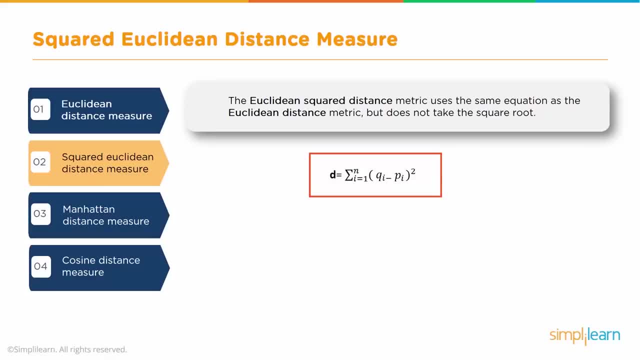 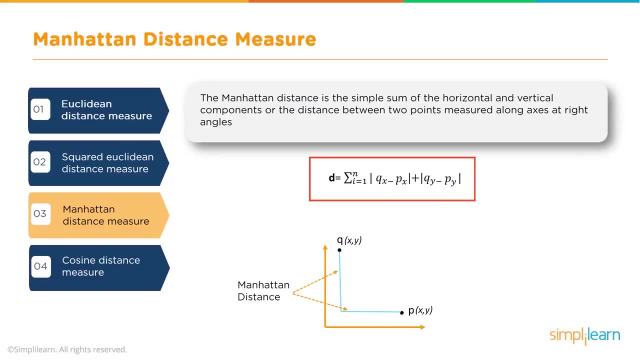 the square of the Euclidean distance, as the name suggests. So instead of taking the square root, we leave the square as it is And then we have Manhattan distance measure. In case of Manhattan distance, it is the sum of the distances across the x-axis and the y-axis, And note that we are 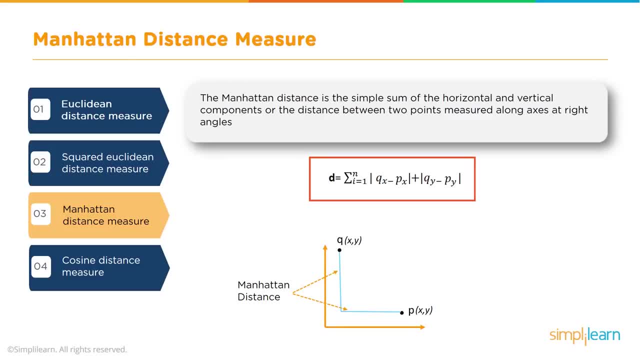 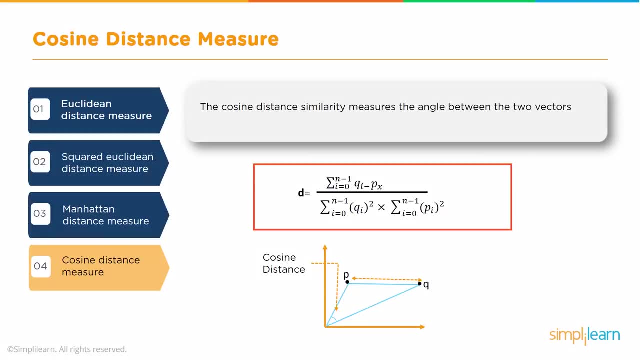 taking the absolute value so that the negative values don't come into play. So that is the Manhattan distance measure. Then we have cosine distance measure. In this case we take the angle between the two vectors formed by joining the points from the origin. So that is the cosine distance measure. Okay, so that was a quick overview about the 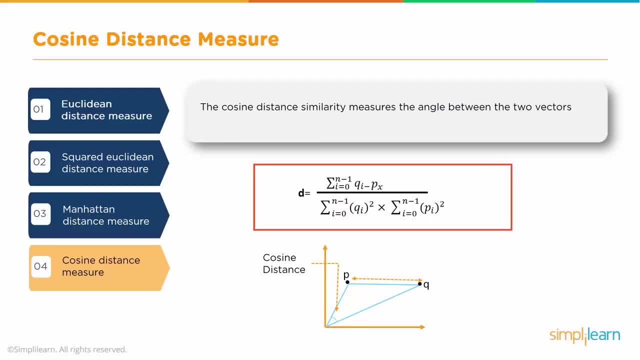 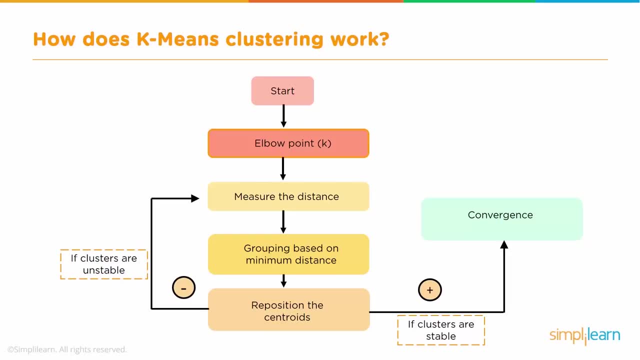 various distance measures that are supported by k-means. Now let's go and check how exactly k-means clustering works. Okay, so this is how k-means clustering works. This is like a flow chart of the whole process. There is a 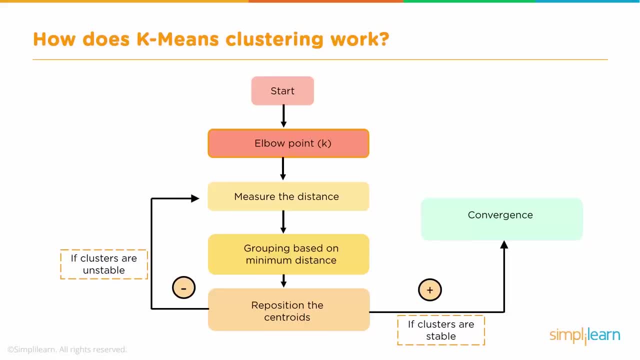 starting point and then we specify the number of clusters that we want. Now there are a couple of ways of doing this. We can do by trial and error. So we specify a certain number- maybe k is equal to 3 or 4 or 5- to start with, And then, as we progress, we keep changing until we get the 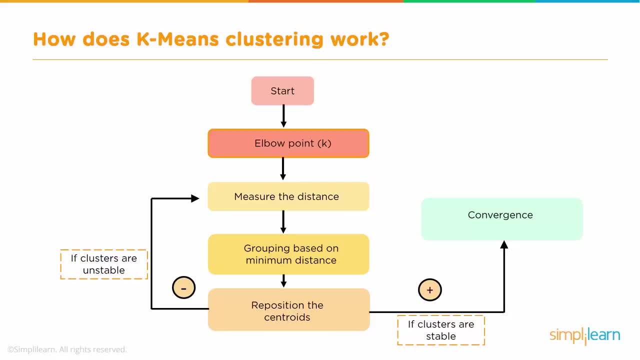 best clusters? Or there is a technique called Elbow technique, whereby we can determine the value of k. What should be the best value of k? How many clusters should be formed? So once we have the value of k, we specify that and then the system will assign that many. 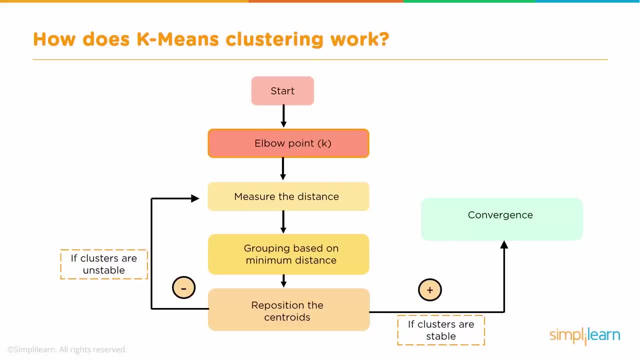 centroids. So it picks randomly that, to start with, randomly that many points that are considered to be the centroids of these clusters, And then it measures the distance of each of the data points from these centroids and assigns those points to the corresponding centroid, from which the distance 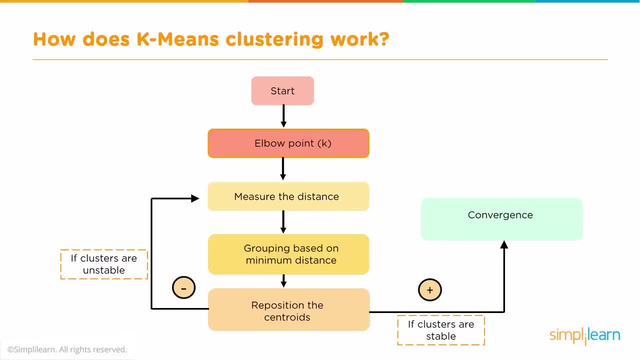 is minimum, So each data point will be assigned to the centroid which is closest to it, And thereby we have k number of initial clusters. However, this is not the final clusters. The next step it does is for the new groups, for the clusters that have been formed. it calculates the mean. 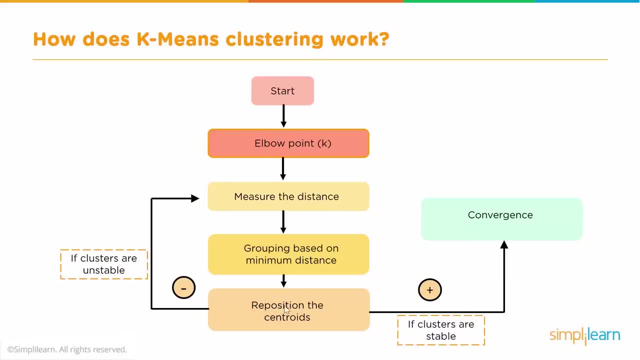 position thereby calculates the new centroid position. the position of the centroid moves compared to the randomly allocated one, So it's an iterative process. Once again, the distance of each point is measured from this new centroid point And, if required, the data points are reallocated to the 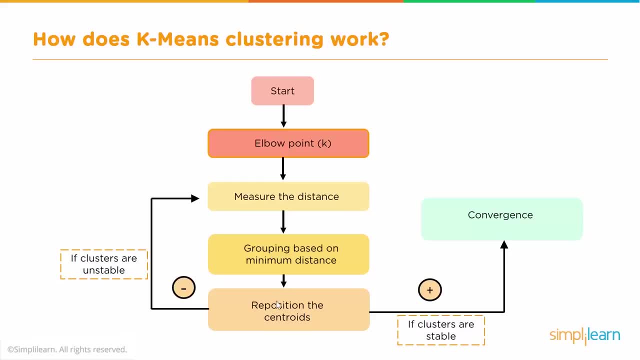 new centroids and the mean position or the new centroid is calculated once again. If the centroid moves, then the iteration continues, which means the convergence has not happened, The clustering has not converged. So as long as there is a movement of the centroid, 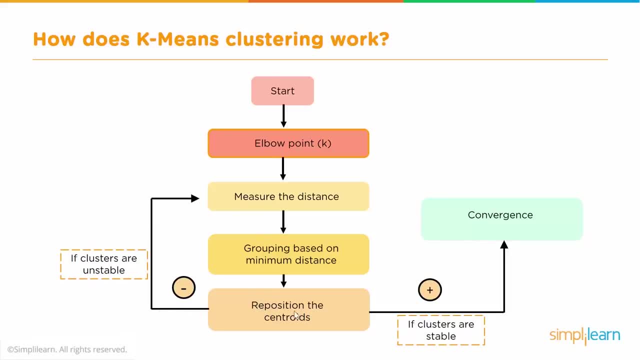 this iteration keeps happening, But once the centroid stops moving- which means that the cluster has converged or the clustering process has converged- that will be the end result. So now we have the final position of the centroid and the data points are allocated accordingly to the closest centroid. I know it's a little difficult to understand from this. 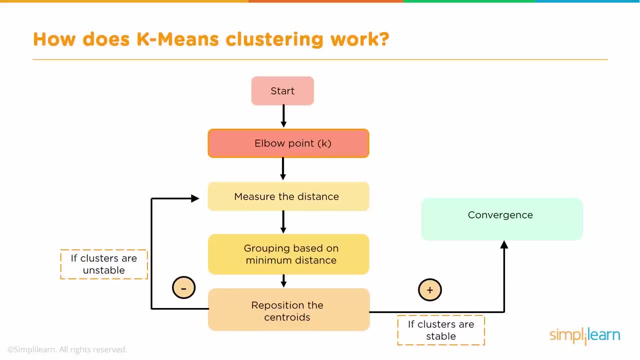 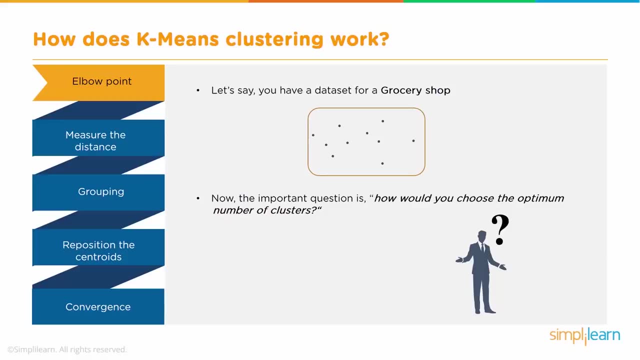 simple flowchart. So let's do a little bit of visualization and see can explain it better. let's take an example: if we have a data set for a grocery shop. so let's say we have a data set for a grocery shop and now we want to find out how many clusters this has to be. 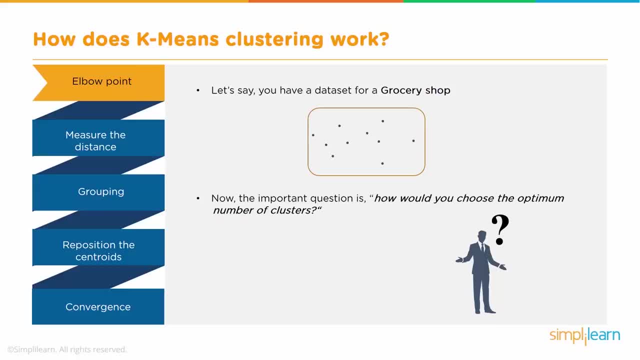 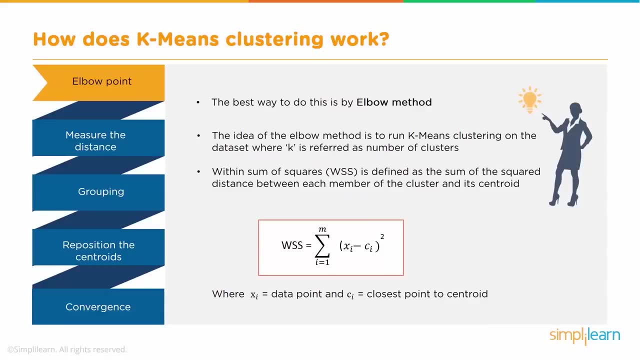 spread across. so how do we find the optimum number of clusters? there is a technique called the elbow method. so when these clusters are formed, there is a parameter called within sum of squares, and the lower this value is, the better the cluster is. that means all these points are very close to each. 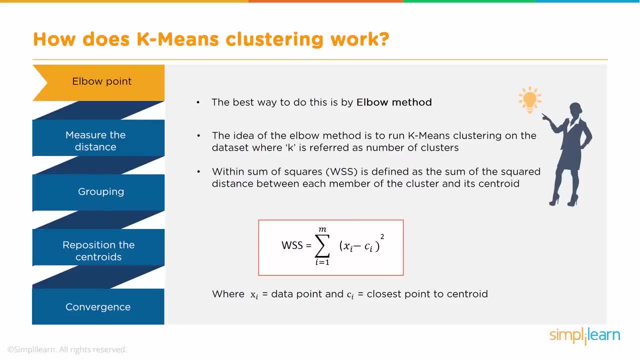 other. so we use this within sum of squares as a measure to find the optimum number of clusters that can be formed for a given data set. so we create clusters or we let the system create clusters of a variety of numbers, maybe of 10, 10 clusters and for. 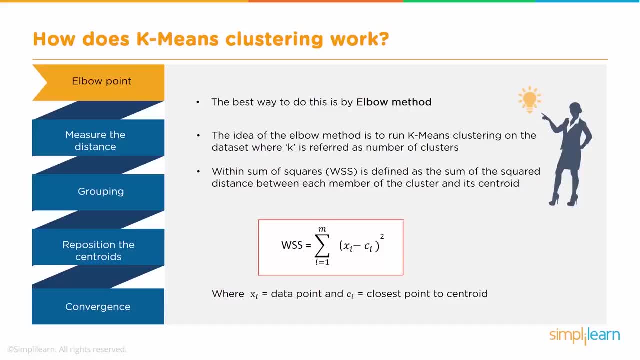 each of these clusters. there is a number of clusters and we create all these clusters here, and for each of these clusters we create a minimum number of clusters and for each of these clusters, value of K, the within SS is measured, and the value of K, which has the least. 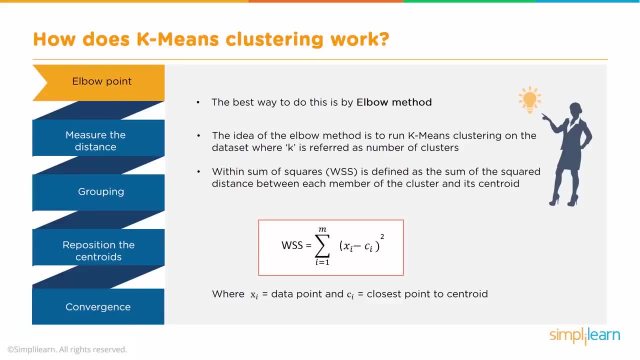 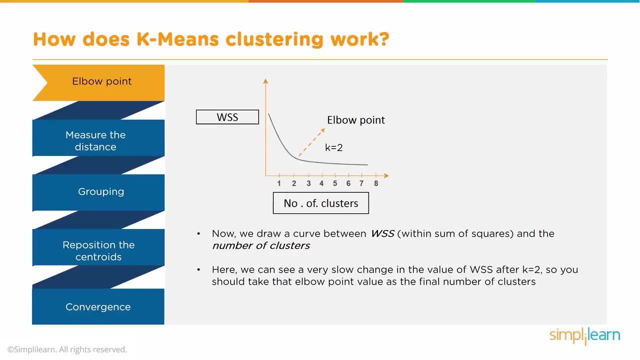 amount of within SS or WSS. that is taken as the optimum value of K. so this is the diagrammatic representation. so we have on the y-axis the within sum of squares or WSS, and on the x-axis we have the number of clusters. so, as you can imagine, 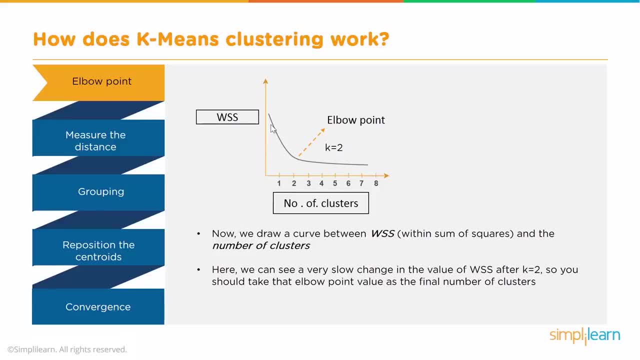 if you have K is equal to 1, which means all the data points are in a single cluster, the within SS value will be very high because they are probably scattered all over the moment. you split it into two, there will be a drastic fall in the within SS value. that's what is represented here, but then, as the value 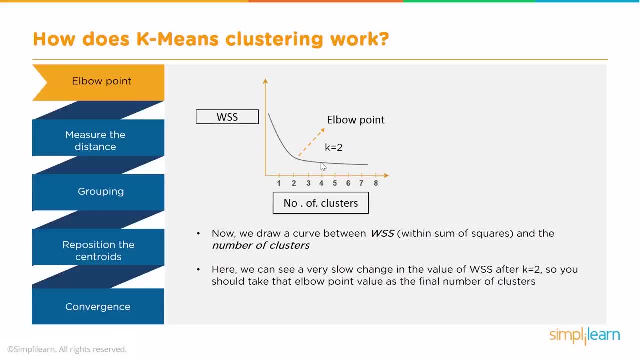 of K increases the decrease. the rate of decrease will not be so high. it will continue to decrease, but probably the rate of decrease will not be high. so that gives us an idea. so from here we get an idea. for example, the optimum value of K should be either two or three or, at the most, four. 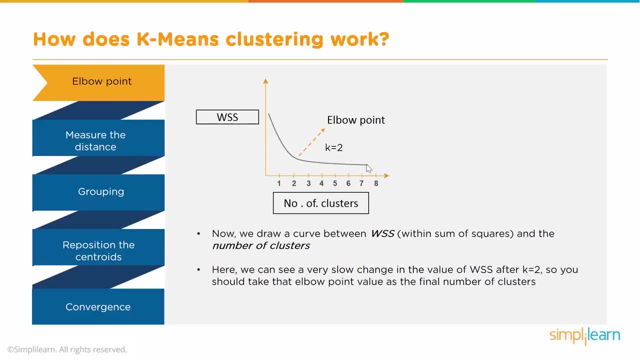 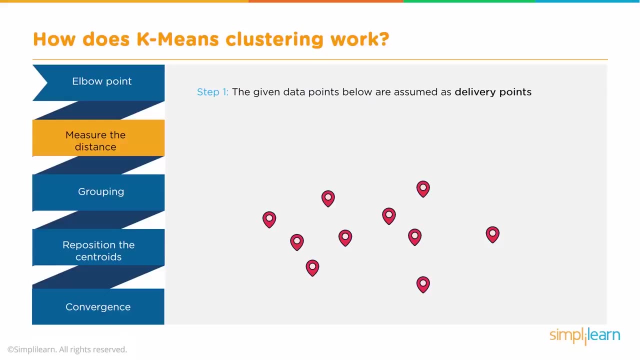 but beyond that, increasing the number of clusters is not dramatically changing the value in WSS because that pretty much gets stabilized. okay, now that we have got the value of K- and let's assume that these are our delivery points- the K value at K and let us assume that these are our delivery points. I have 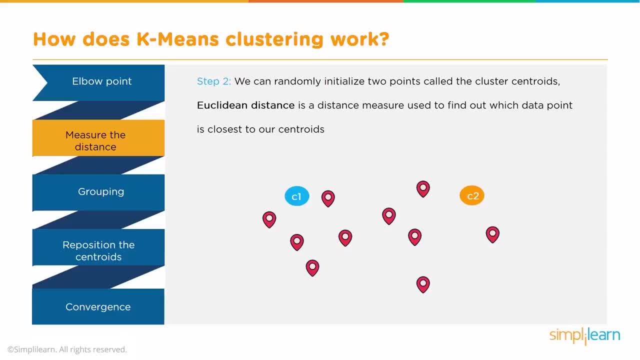 already mentioned that. what are L and L and the L and LZ values? that between L and LZ are basically the Q and the LN and these value points multiplied by K. so let's first try to say that LZ is equal to 1. that means that LZ has 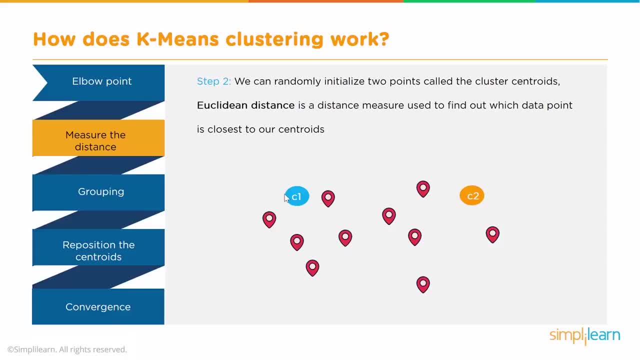 two delivery points. of course it's not a constant quantity, but the relation between both of these delivery points is basically one: Booker's will be assigned, which are close to C1 will be assigned to C1, and these points or locations which are close to C2 will be assigned to C2 and then. so this is. 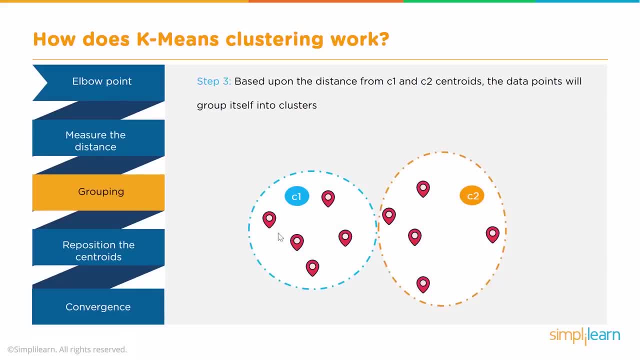 the how the initial grouping is done: this is part of C1 and this is part of C2. then the next step is to calculate the actual centroid of this data because, remember, C1 and C2 are not the centroids. they've been randomly assigned points and only thing that has been done was the data points which are closest to 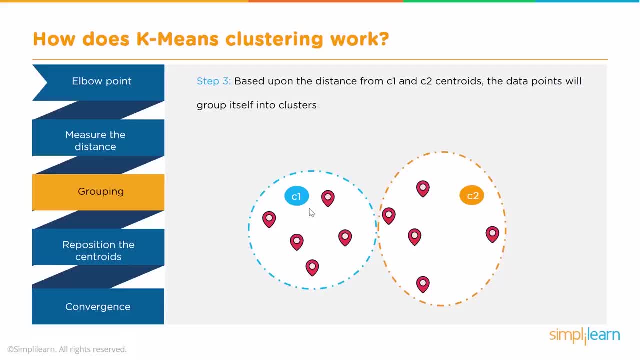 them have been assigned. but now, in this step, the actual centroid will be calculated, which may be for each of these data sets somewhere in the middle. so that's like the mean point that will be calculated and the centroid will actually be positioned or repositioned there. same with C2, so the new centroid. 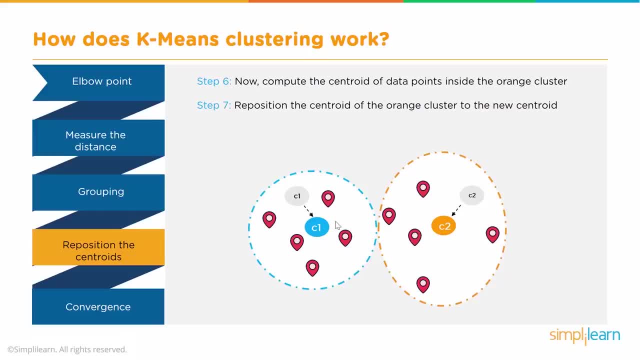 for this group is C2 in this new position and C1 is in this new position. once again, the distance of each of the data points is calculated from these centroids. now, remember, it's not necessary that the distance still remains the or each of these data points still remain in the same group by 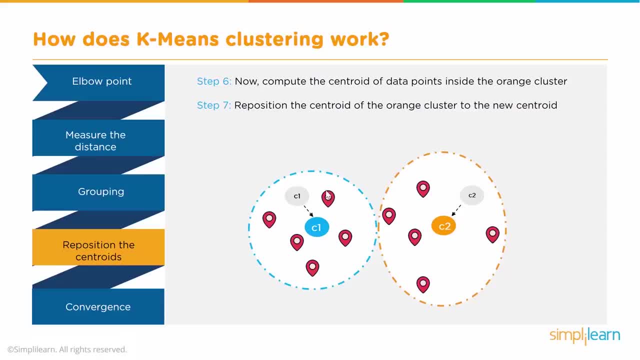 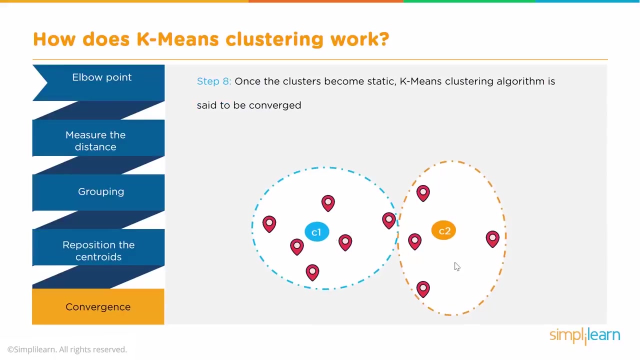 recalculating the distance it may be possible that some points get reallocated like: so you see this. so this point earlier was closer to C2 because C2 was here, but after recalculating repositioning it is closer to C1 than C2. so this is the new grouping, so some points will be. 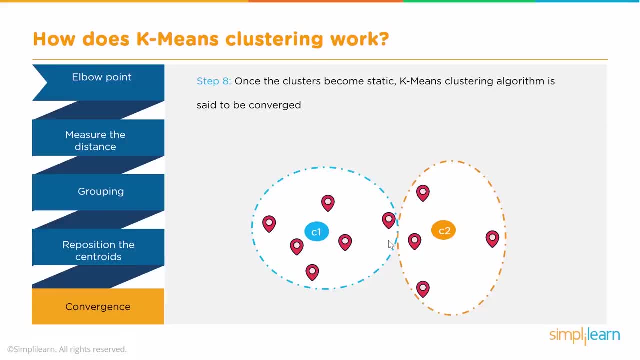 reassigned and again the centroid will be calculated. and if the centroid doesn't change, so that is a repetitive process, iterative process- and if the centroid doesn't change, once the centroid stops changing, that means the algorithm has converged. and this is our final cluster, with this as the centroid, C1 and C2 as 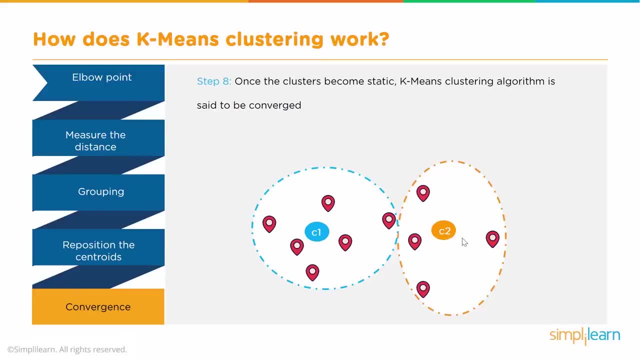 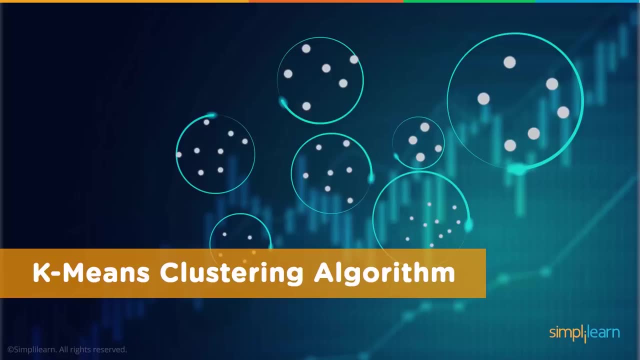 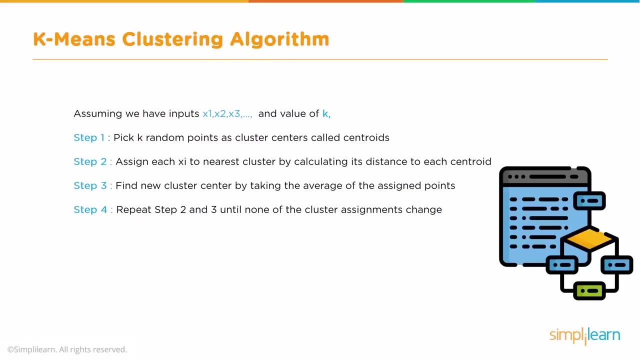 the centroids points as a part of each cluster. so I hope this helps in understanding the whole process. iterative process of k-means clustering. so let's take a look at the k-means clustering algorithm. let's say we have x1, x2, x3, n- number of 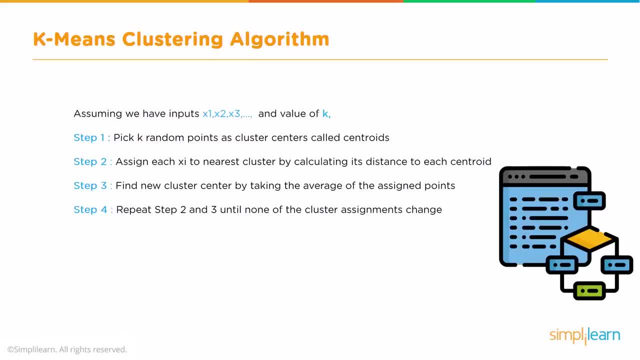 points as our inputs and we want to split this into k clusters or we want to create k clusters. so the first step is to randomly pick k points and call them centroids. they are not real centroids, because centroid is supposed to be a center point, but they are just called centroids and we calculate the distance. 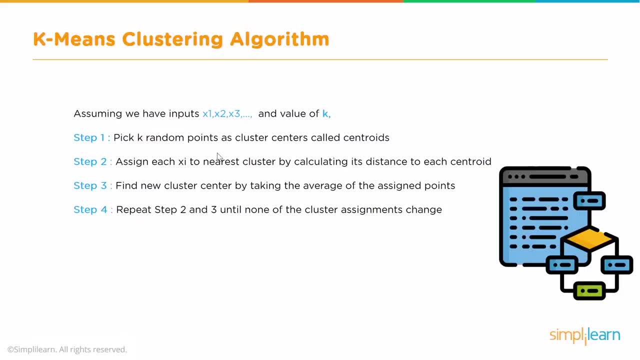 of each and every input point from each of the centroids. so the distance of x 1 from c 1 from c 2, c 3, each of the distances we and then find out which distance is the lowest and assign x1 to that. 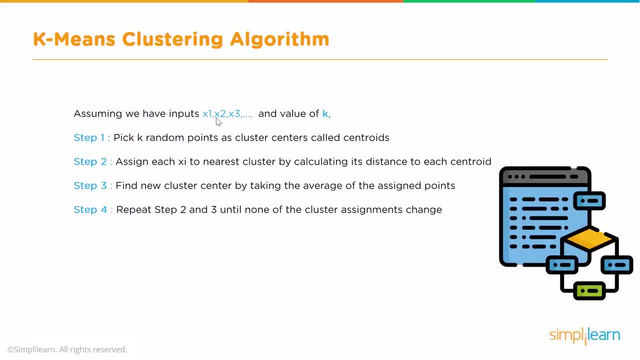 that particular random centroid. Repeat that process for x2.. Calculate its distance from each of the centroids c1,, c2, c3 up to ck and find which is the lowest distance and assign x2 to that particular centroid, Same with x3 and so on. So that is the first round of assignment, that is. 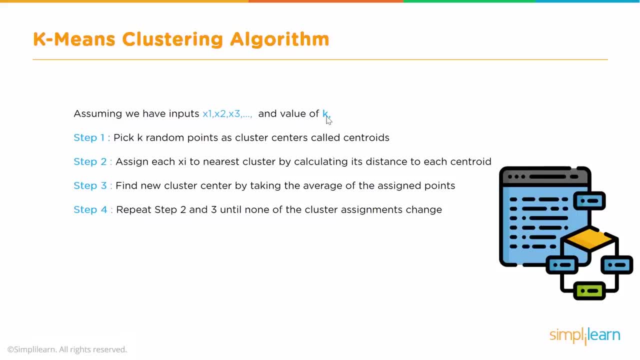 done. Now we have k groups, because there are. we have assigned the value of k, So there are k centroids and so there are k groups. All these inputs have been split into k groups. However, remember, we picked the centroids randomly, so they are not real centroids. So now what we have to do: 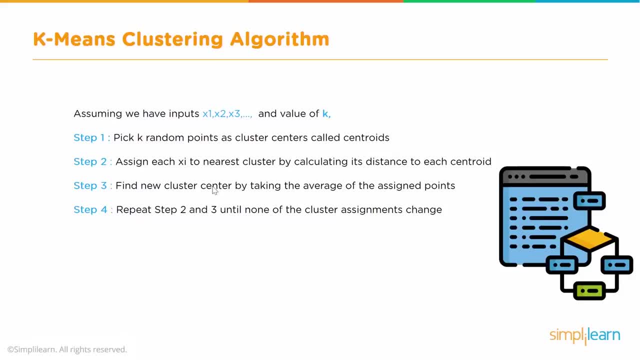 we have to calculate the actual centroids for each of these groups, which is like the mean position, which means that the position of the randomly selected centroids will now change and they will be the mean position of these newly formed k groups. and once that is done, we once again repeat this process of 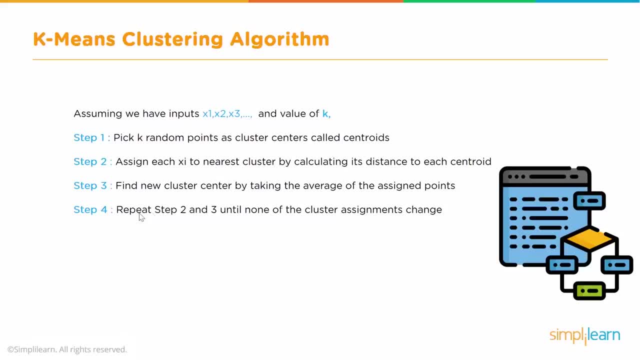 calculating the distance, right. So this is what we are doing as a part of step four. We repeat step two and three. So we again calculate the distance of x1 from the centroid c1,, c2,, c3 and then c, which is the lowest value, and assign x1 to that, Calculate the distance of x2 from the centroid c1. 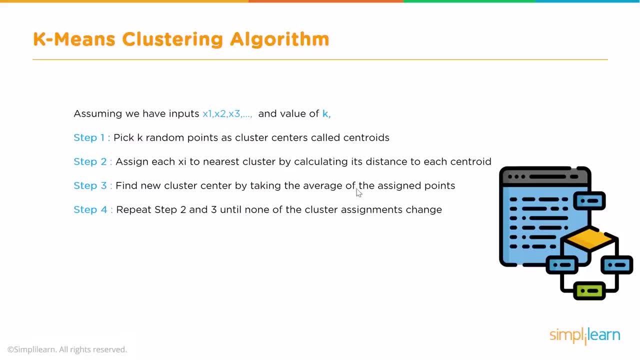 from c1, c2, c3 or whatever up to ck and find whichever is the lowest distance and assign x2 to that centroid and so on. In this process there may be some reassignment: x1 was probably assigned to cluster c2 and after doing this calculation maybe now x1 is assigned to c1. So that kind of 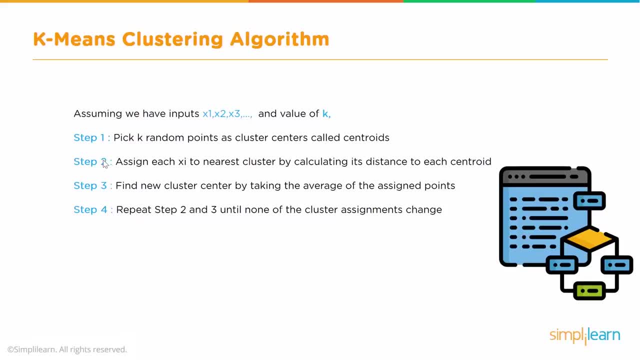 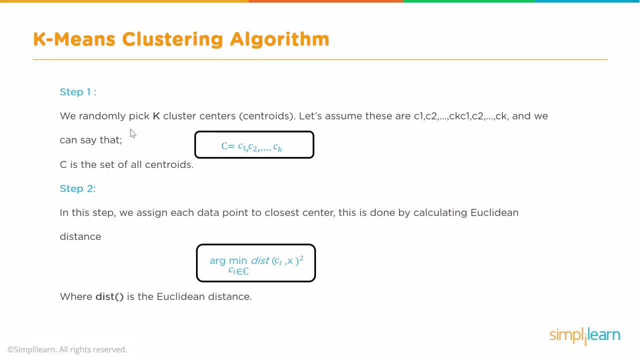 reallocation may happen. So we repeat the steps two and three till the position of the centroids don't change or stop, And that's when we have convergence. So let's take a detailed look at each of these steps. So we randomly pick k cluster centers. We call them centroids because they are not initially they are 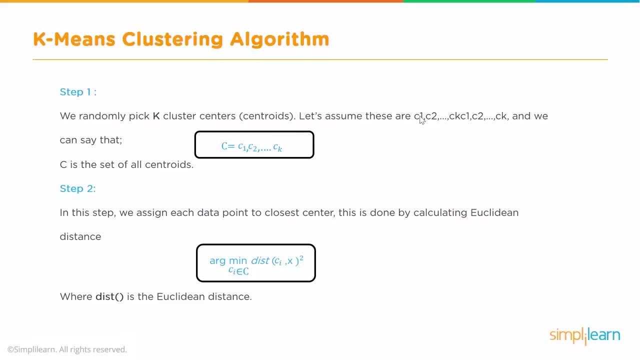 not really the centroids. So we let us name them c1, c2, up to ck. and then, step two, we assign each data point to the closest center. So what we do? we calculate the distance of each x value from each c value. So the distance between x1, c1.. Distance between x1, c2, x1, c3.. And then we find which is. 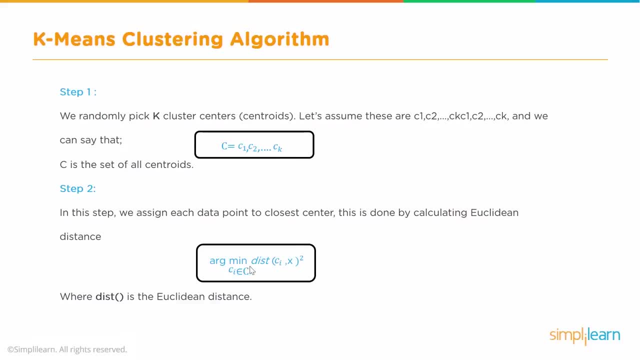 the lowest value, That's the minimum value we find, and assign x1 to that particular centroid. Then we go next to x2.. Find the distance of x2 from c1, x2 from c2, x2 from c3, and so on up to ck. 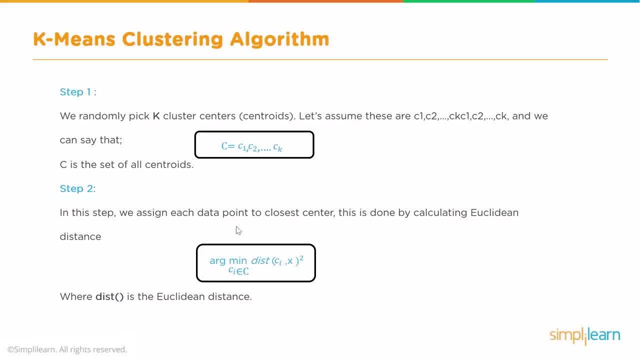 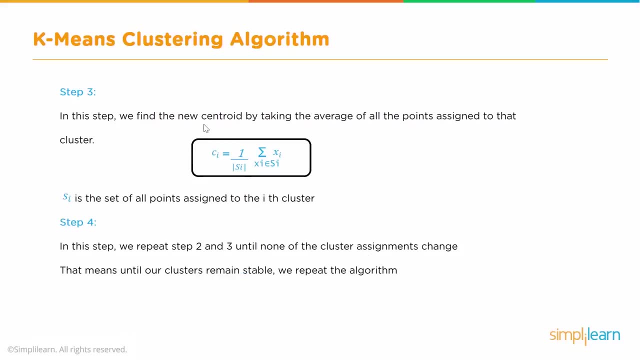 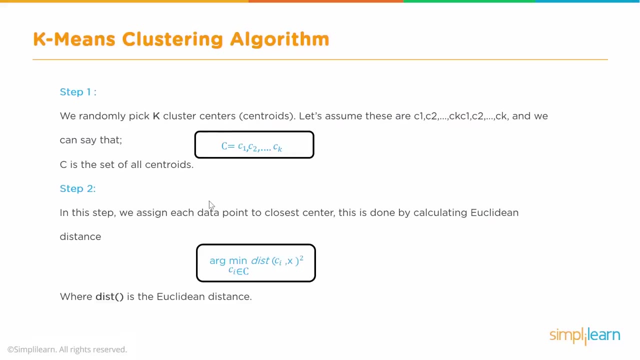 and then assign it to the point or to the centroid Which has the lowest value, and so on. So that is step number two. In step number three, we now find the actual centroid for each group. So what has happened? as a part of step number two, we now have: 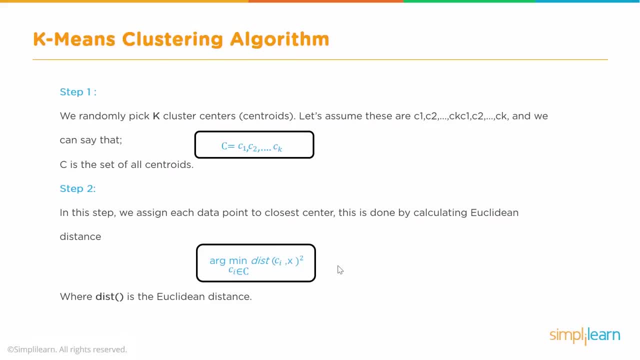 all the points, all the data points, grouped into k groups because we wanted to create k clusters, right? So we have k groups, Each one may be having a certain number of input values. They need not be equally distributed. by the way, Based on the distance, we will have k groups, But remember the initial values of the 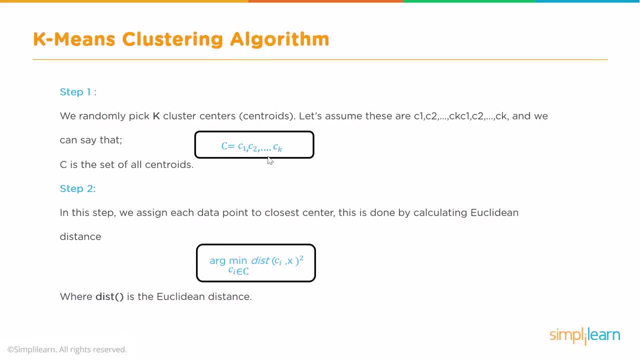 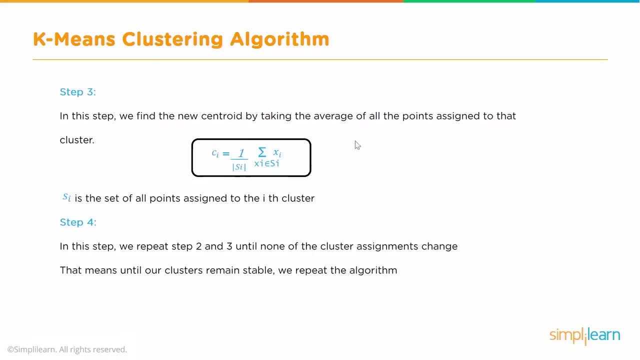 c1, c2 were not really the centroids of these groups, right, We assigned them randomly. So now in step 3, we actually calculate the centroid of each group, which means the original point, which we thought was the centroid, will shift to the new position, which is the actual centroid for each of. 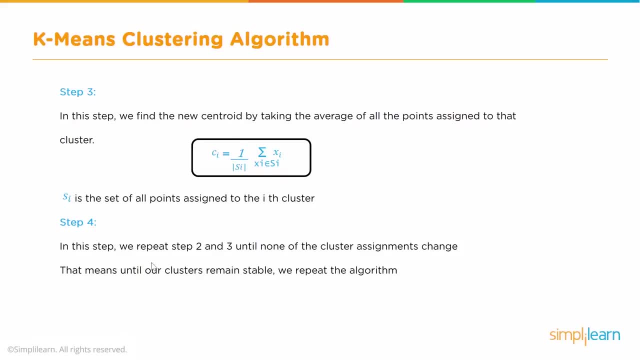 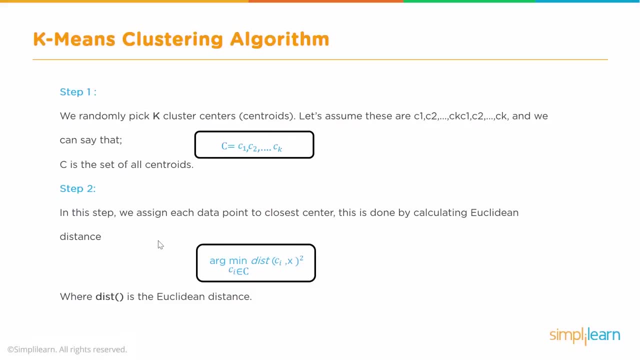 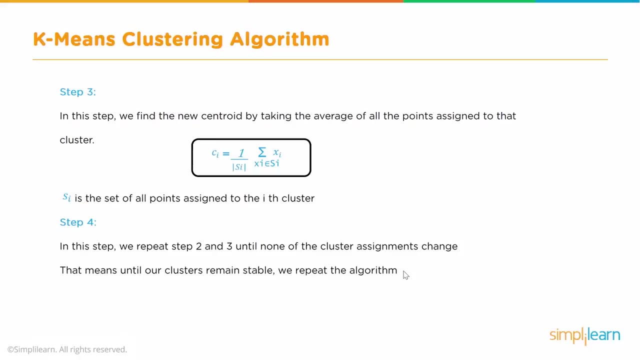 these groups, okay, And we again calculate the distance. So we go back to step 2, which is what We calculate again: the distance of each of these points from the newly positioned centroids And, if required, we reassign these points to the new centroids. So, as I said earlier, there may be a 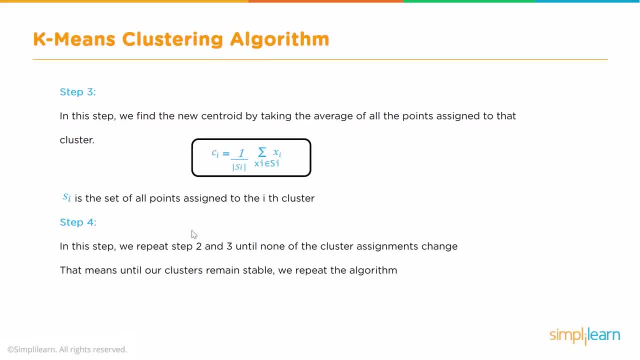 reallocation. So we now have a new set or a new group. We still have k groups, But the number of items and the actual assignment may be different from what was in step 2 here. okay, So that might change. Then we perform step 3 once again to find the new centroid of this new 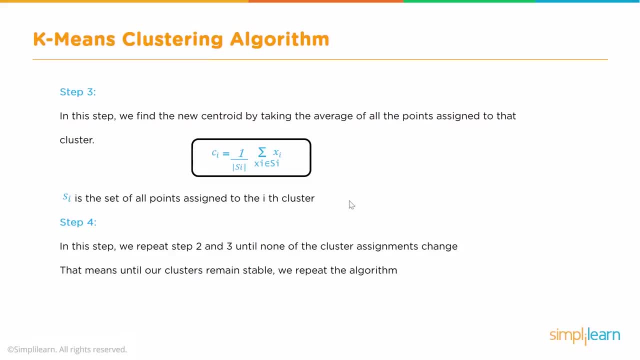 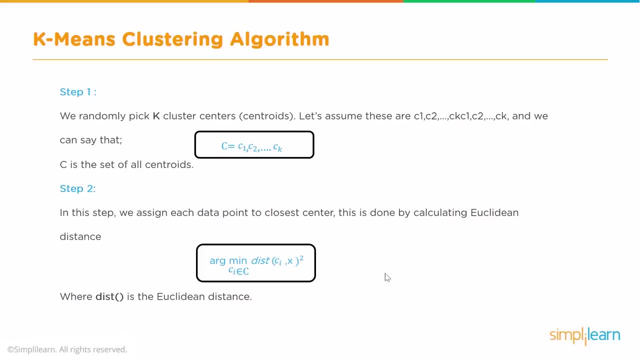 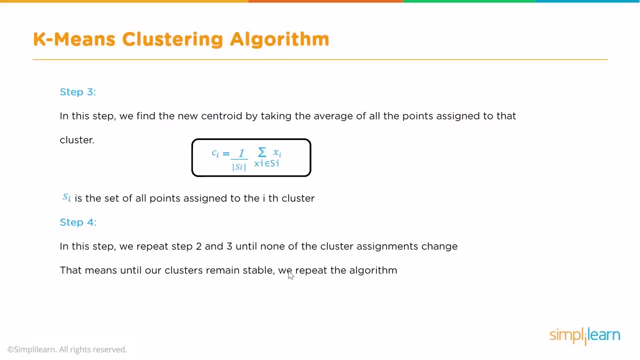 group. So we have again a new set of clusters, new centroids and new assignments. We repeat this step 2 again. Once again we find: And then it is possible that after relating through three or four or five times, the centroid will stop moving, in the sense that when 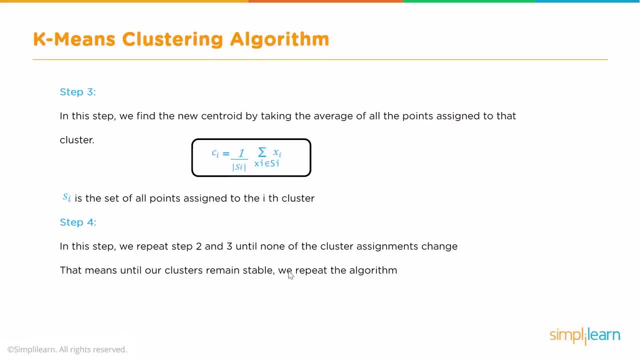 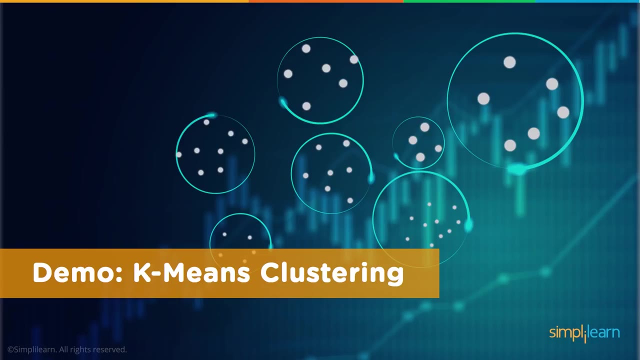 you calculate the new value of the centroid, that will be same as the original value or there will be very marginal change. So that is when we say convergence has occurred And that is our final cluster. That's the formation of the final cluster. All right, so let's see a couple of demos of k-means. 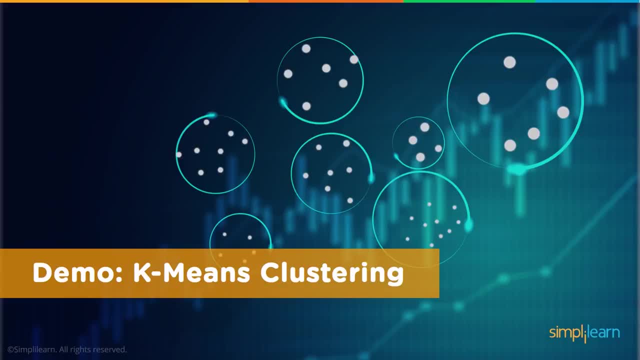 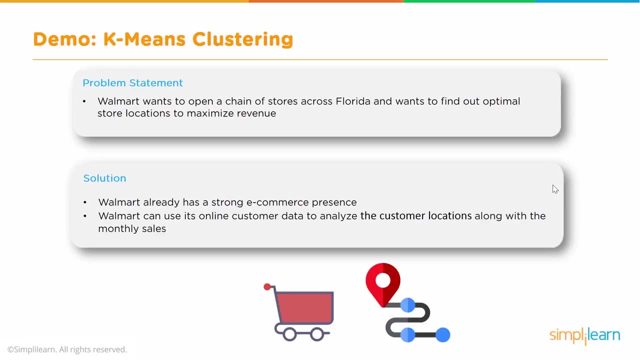 string. We will actually see some live demos in Python Notebook using Python Notebook, But before that, let's find out what's the problem that we are trying to solve. The problem statement is: let's say Walmart wants to open a chain of stores across the state of Florida and it wants to find 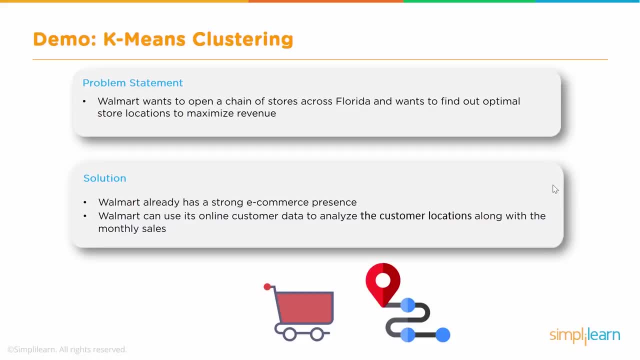 the optimal store locations. Now the issue here is: if they open too many stores close to each other, obviously they will not make profit, But if they, if the stores are too far apart, then they will not have enough sales. So how do they? 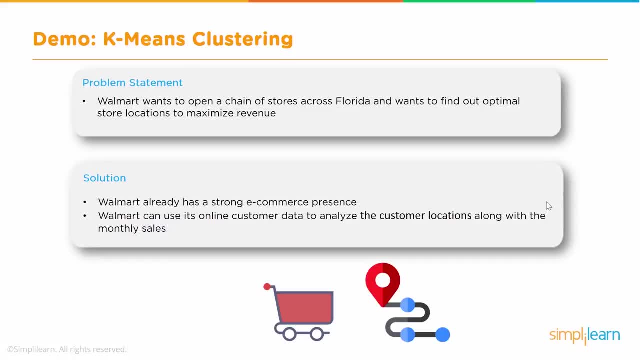 optimize this Now for an organization like Walmart, which is an e commerce giant. they already have the addresses of their customers in their database, So they can actually use this information or this data and use k-means clustering to find the optimal location. 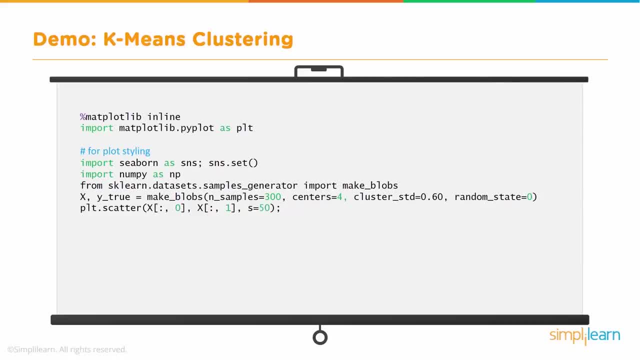 Now, before we go into the Python Notebook and show you the live code, I wanted to take you through very quickly a summary of the code in the slides and then we will go into the Python Notebook. So in this block we are basically importing all the required libraries like NumPy, matplotlib and so on. 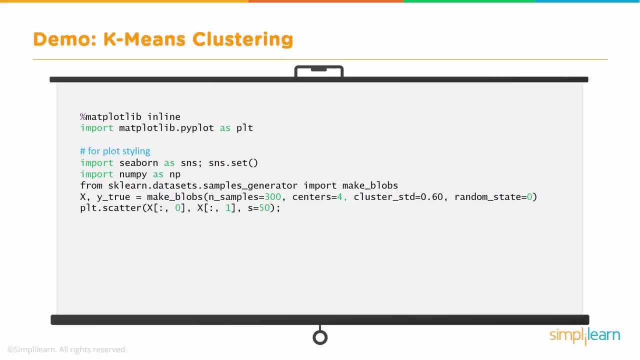 And we are loading the data that is available in the form of, let's say, the addresses. for simplicity, we will just take them as some data points. then the next thing we do is quickly do a scatterplot to see how they are related to each other with respect to each other. So in the scatterplot, 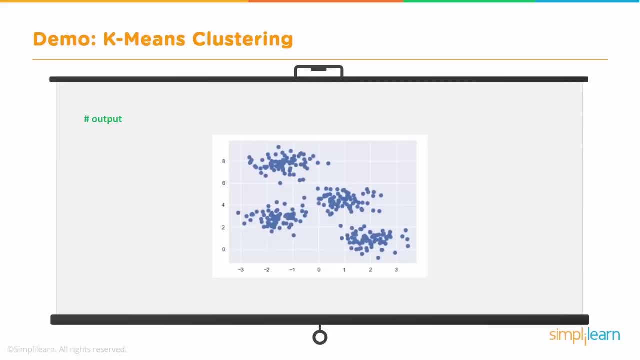 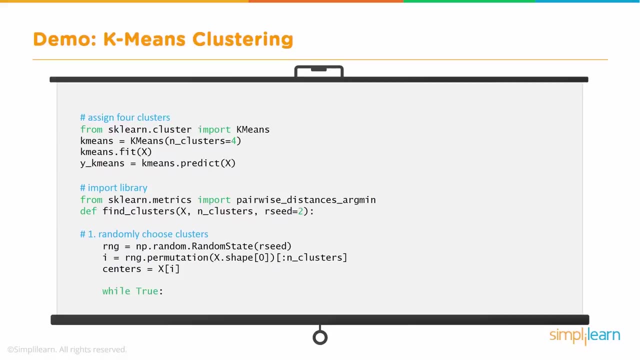 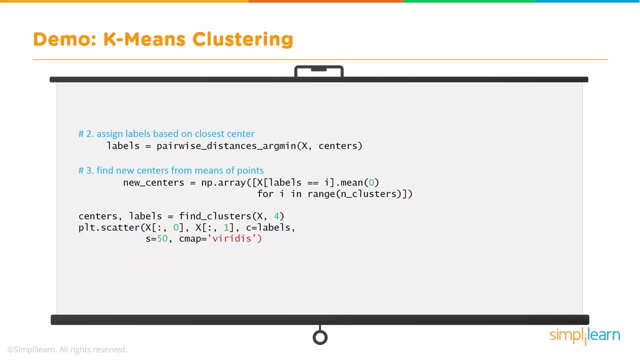 we see that there are a few distinct groups already being formed, So you can actually get an idea about how the cluster would look and how many clusters, what is the optimal number of clusters? and then starts the actual k-means clustering process. So we will assign each of these points to the centroids and then check whether they are the 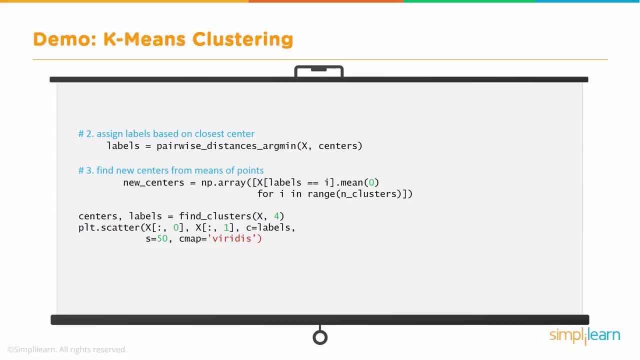 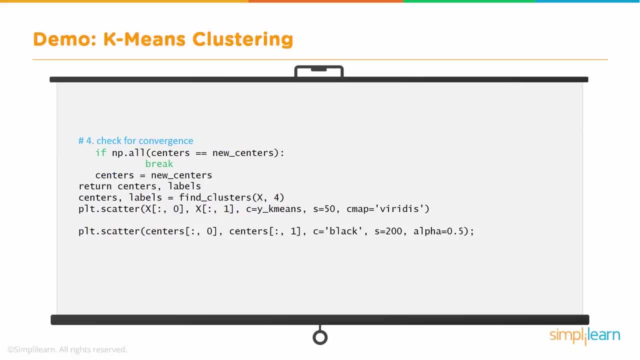 optimal distance, which is the shortest distance, and assign each of the points- data points- to the centroids and then go through this iterative process till the whole process converges And finally we get an output like this: So we have four distinct clusters, and which is, if we 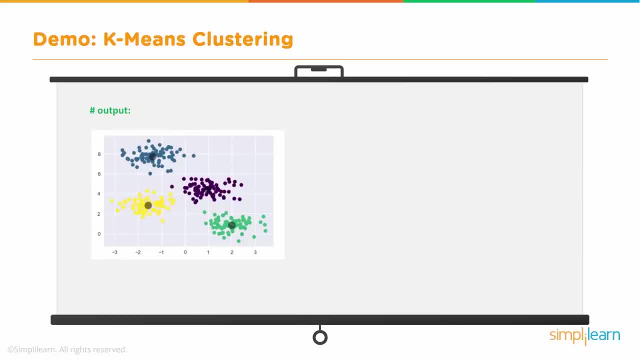 can say that how the population is probably distributed across Florida state and these centroids are like the location where the store should be, the optimum location where the store should be. So that's the way we determine the best locations for the store and that's how we can help Walmart find the best. 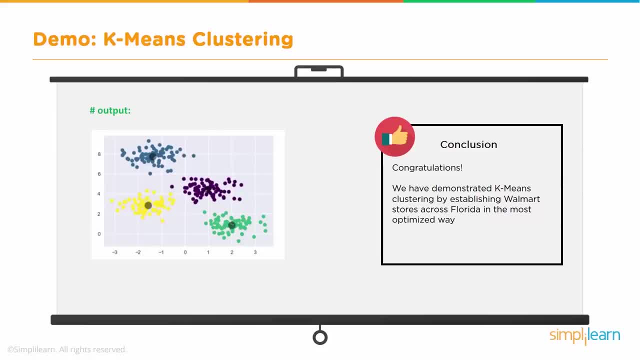 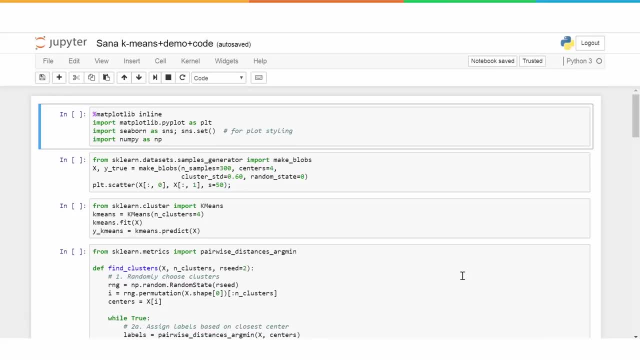 locations for their stores in Florida. So now let's take this into Python notebook. Let's see how this works when we are running the code live. All right, so this is the code for k-means clustering in Jupyter notebook. We have a few examples here which we will demonstrate how k-means clustering. 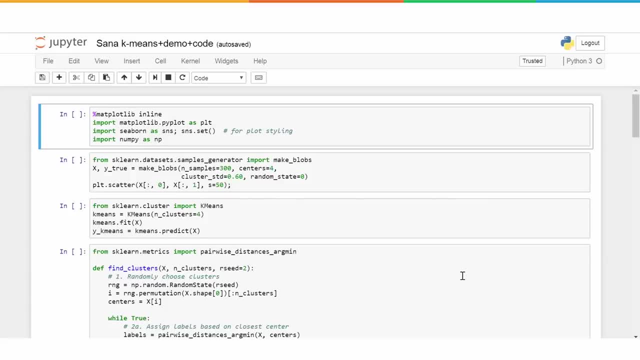 is used, and even there is a small implementation of k-means clustering as well. Okay so, let's get started. Okay so, this block is basically importing the various libraries that are required, like matplotlib and numpy and so on and so forth, which would be used as a part of the code. Then we are going. 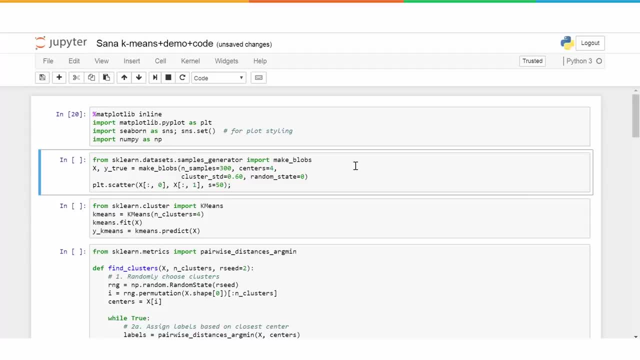 and creating blobs which are similar to clusters. Now this is a very neat feature which is available in scikit-learn. Make blobs is a nice feature which creates clusters of data sets. So that's a wonderful functionality that is readily available for us to create some test data kind of thing. 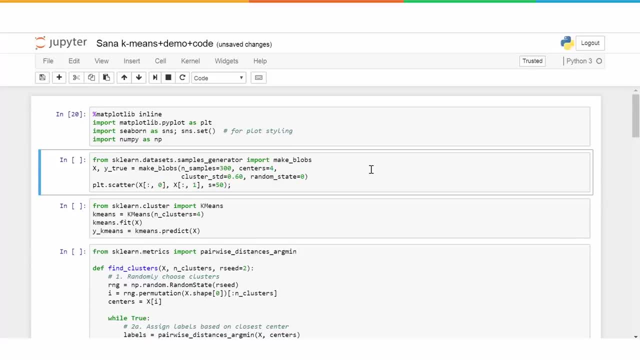 Okay, so that's exactly what we are doing here. We are using make blobs and we can specify how many clusters we want. So centers we are mentioning here, so it will go ahead, and so we just mentioned four, so it will go ahead and create some test data for. 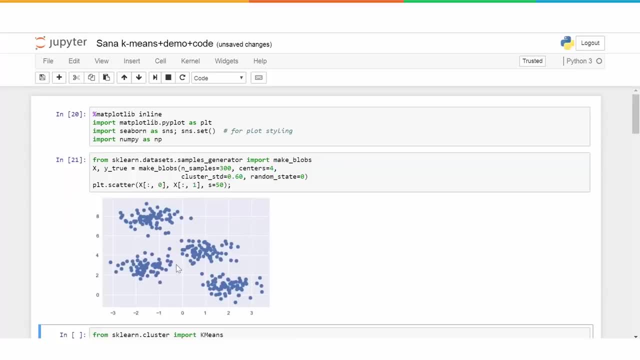 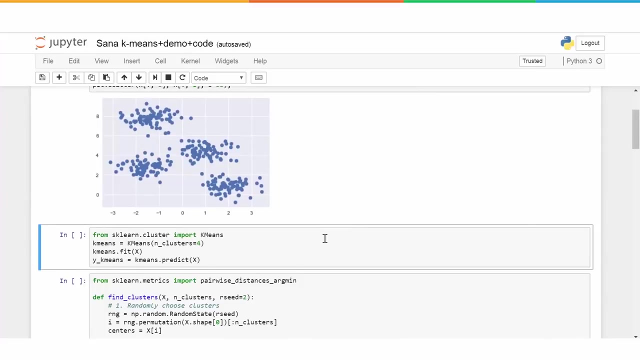 us, And this is how it looks. as you can see visually also, we can figure out that there are four distinct classes or clusters in this data set, And that is what make blobs actually provides. Now, from here onwards, we will basically run the standard k-means functionality that is readily available. 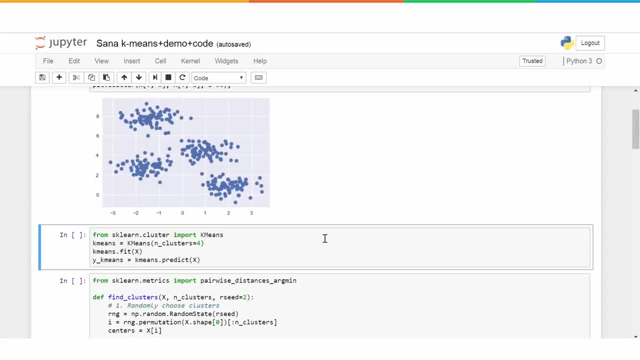 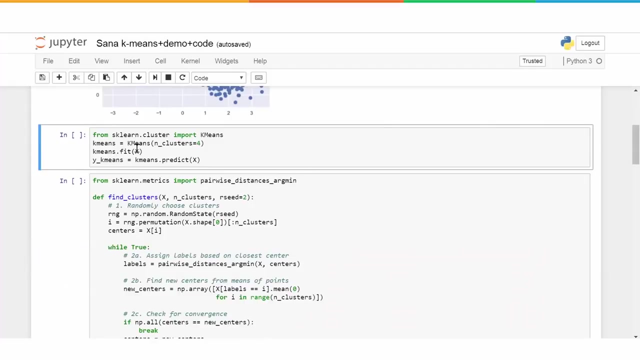 So we really don't have to implement k-means itself. the k-means functionality or the function is readily available. you just need to feed the data and we'll create the clusters. So this is the code for that: We import k-means and then we create an instance of k-means And we specify. 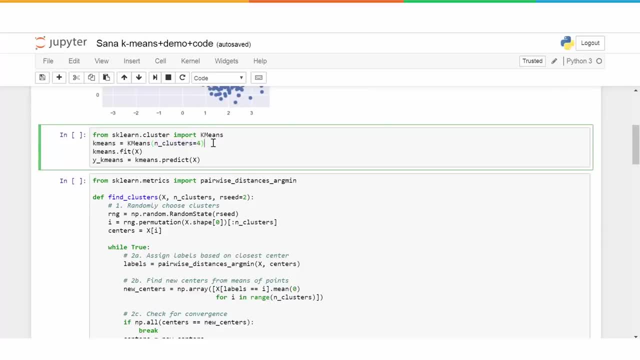 the value of k. this n underscore clusters. value of k. Remember, k means in, k means k is basically the number of clusters that you want to create and it is a integer value. So this is where we are specifying that. So we have k is. 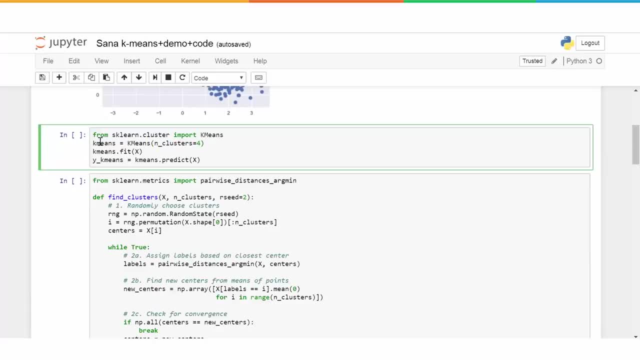 equal to 4, and so that instance is created. We take that instance and, as with any other machine learning functionality, fit is what we use, the function or with the method, rather, fit is what we use to train the model. Here there is no real training kind of thing, but that is the. 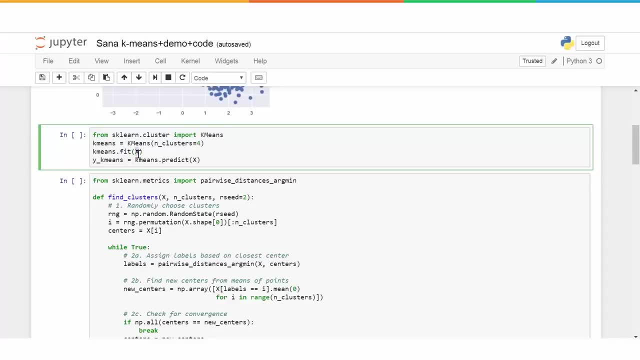 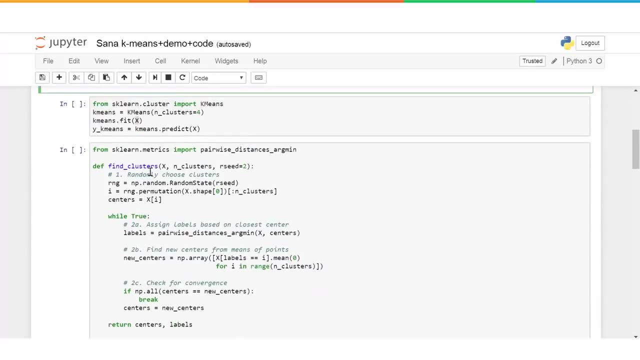 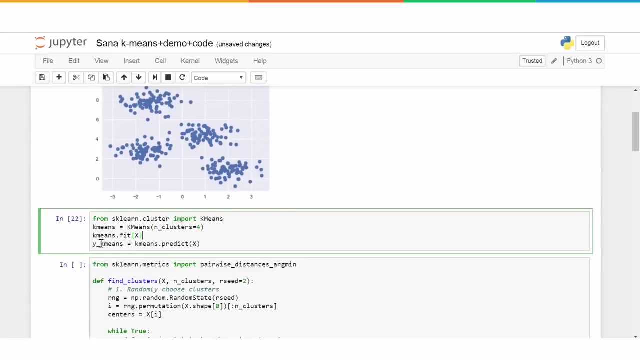 call. So we are calling fit and what we are doing here we are just passing the data, So x has these values, the data that has been created. So that is what we are passing here and this will go ahead and create the clusters, and then we are using. 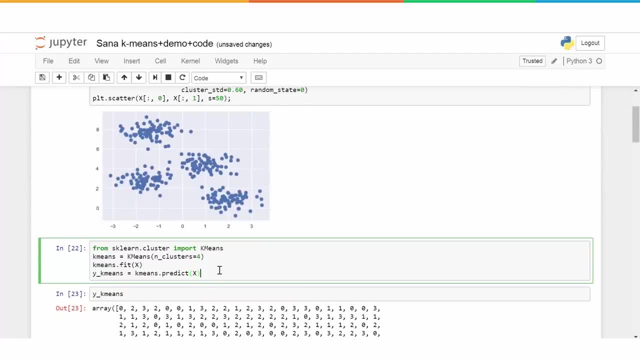 after doing fit, we run the predict, which basically assigns for each of these observations which cluster it belongs to. So it will name the clusters. maybe this is cluster 1, this is 2, 3 and so on. or I will actually start from 0, cluster 0,, 1, 2 and 3 maybe, and then for each of the observations, 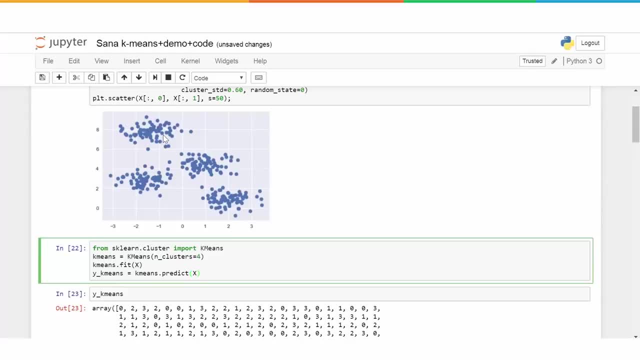 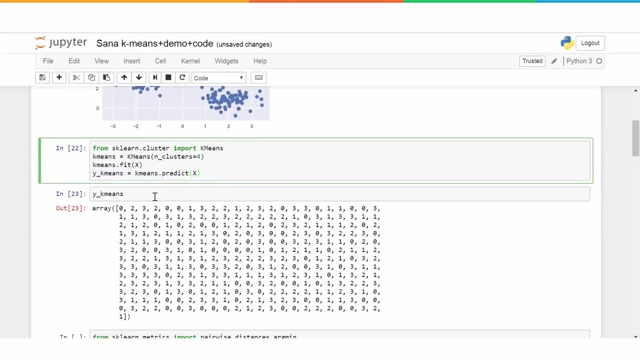 it will assign based on which cluster it belongs to. it will assign a value. So that is stored in y underscore k. So that is what it means when we call predict. that is what it does and we can take a quick look. 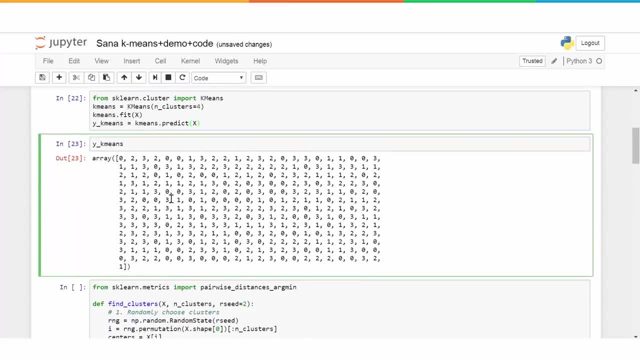 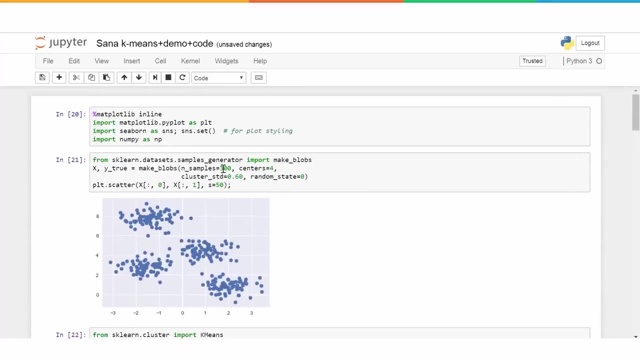 at these y underscore, k means or the cluster numbers that have been assigned for each observation. So this is the cluster number assigned for observation 1, maybe this is for observation 2, observation 3 and so on. So we have how many about? I think, 300 samples right. 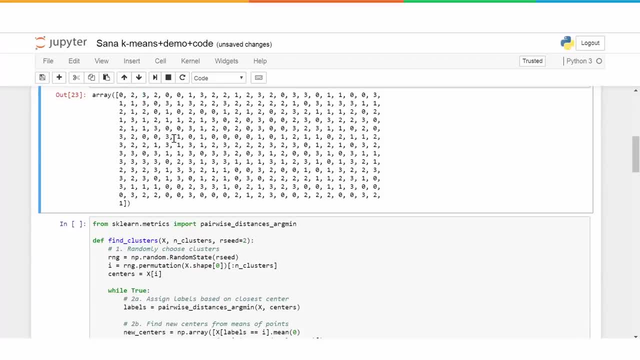 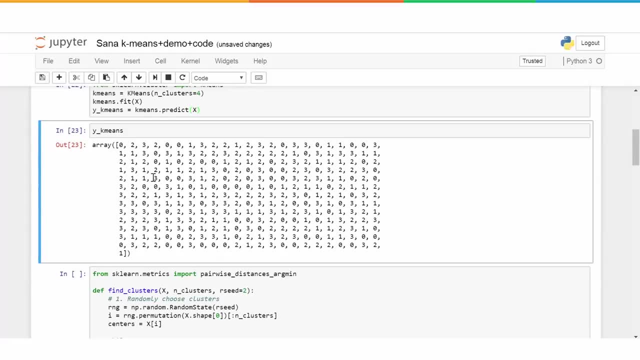 So all the 300 samples. there are 300 values here. each of them the cluster number is given and the cluster number goes from 0 to 3.. So there are 4 clusters. So the numbers go from 0,, 1,, 2,, 3.. 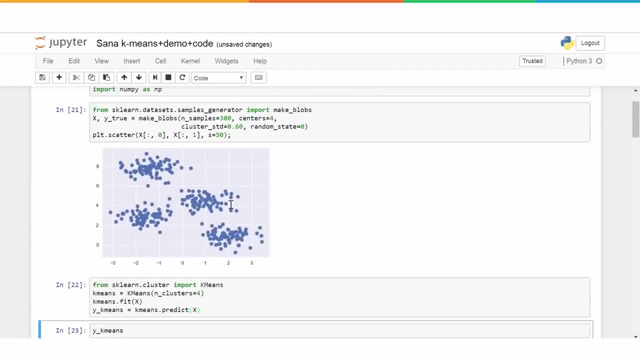 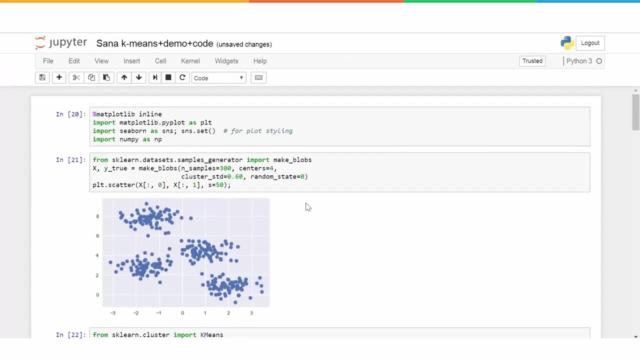 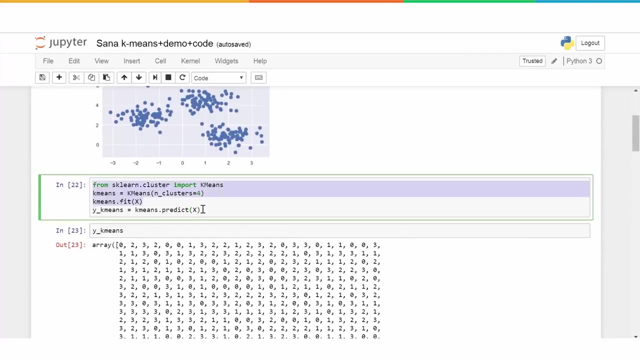 So that is what is seen here. Okay now. so this was a quick example of generating some dummy data and then clustering that. okay, and this can be applied. if you have proper data, you can just load it up into x, for example here, and then run the k. So this is the central part of the k means. 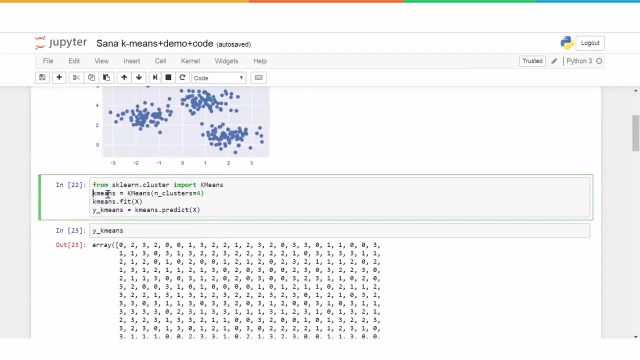 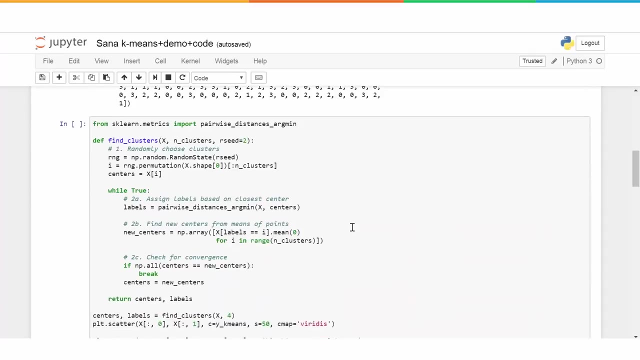 clustering program example. Create an instance and you mention how many clusters you want by specifying this parameter: n underscore clusters, and that is also the value of k, and then pass the data to get the values. Now the next section of this code is the implementation of a k means. Now this is: 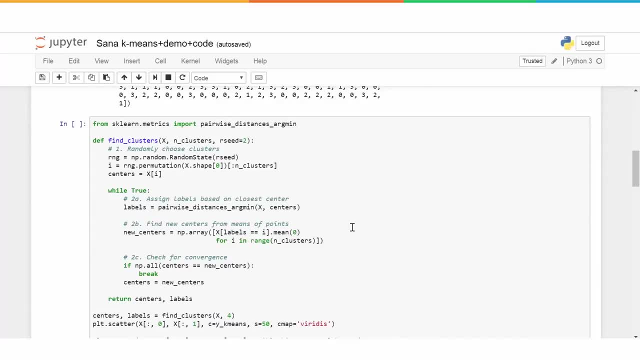 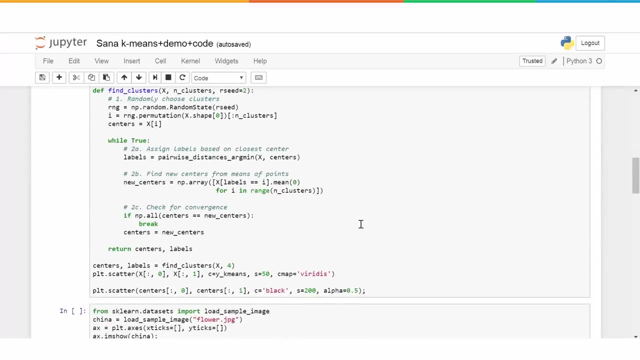 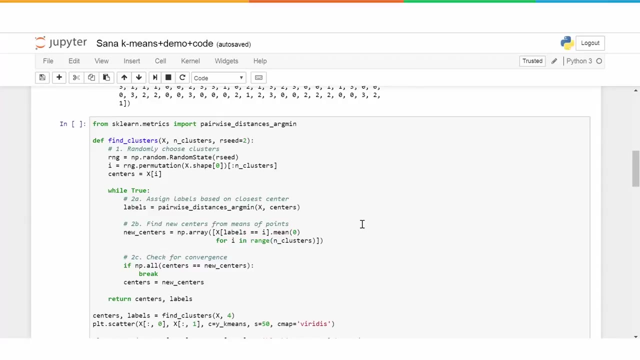 kind of a rough implementation of the k means algorithm. So we will just walk you through- I will walk you through the code at each step, what it is doing, and then we will see a couple of more examples Of how k means clustering can be used in maybe some real life examples, real life use cases. 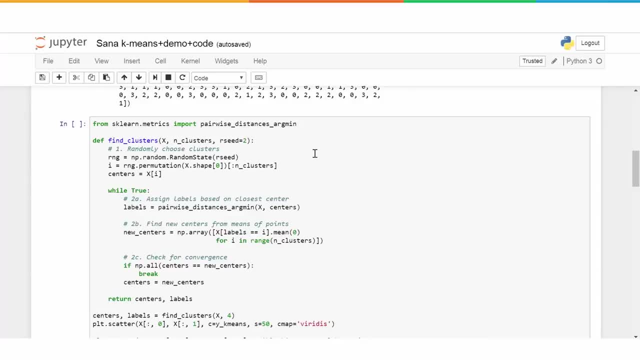 all right. So in this case, here, what we are doing is basically implementing. k means clustering, and there is a function for a library calculates for a given two pairs of points. It will calculate the distance between them and see which one is the closest, and so on. So this is like this is. 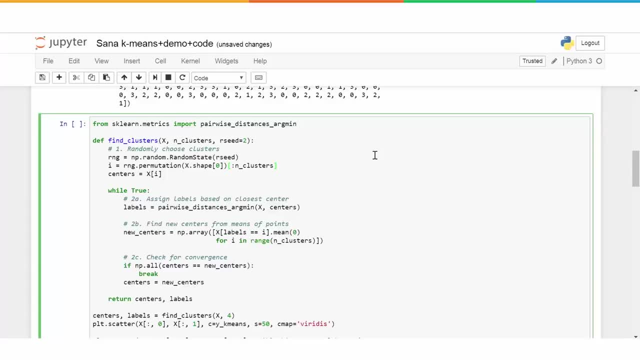 pretty much like what k means does, right? So it calculates the distance of each point or each data set from predefined centroid and then, based on whichever is the lowest, this particular data point is assigned to that centroid. So that is basically available as a standard function and we will be using that here. So 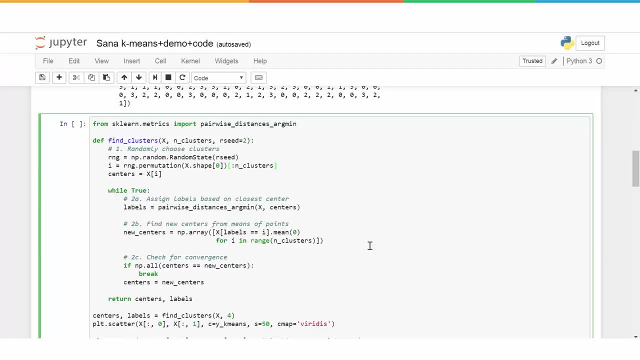 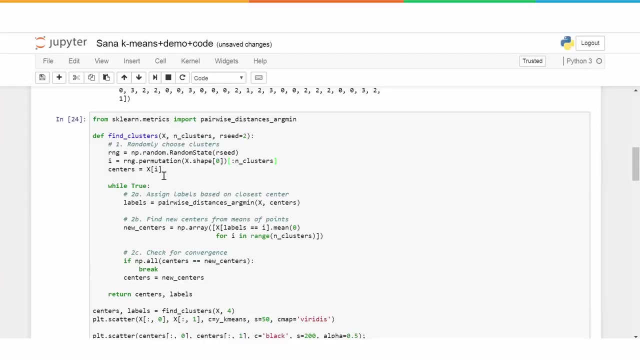 as explained in the slides, the first step that is done- in case of k means clustering- is to randomly assign some centroids. So, as a first step, we randomly allocate a couple of centroids which we call here we are calling as centers, and then 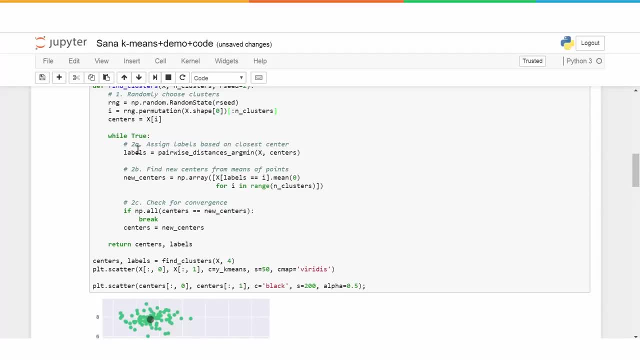 we put this in a loop and we take it through an iterative process. For each of the data points, we first find out using this function, pairwise distance argument. For each of the points, we find out which one- which center or which randomly selected centroid- is the closest and accordingly, 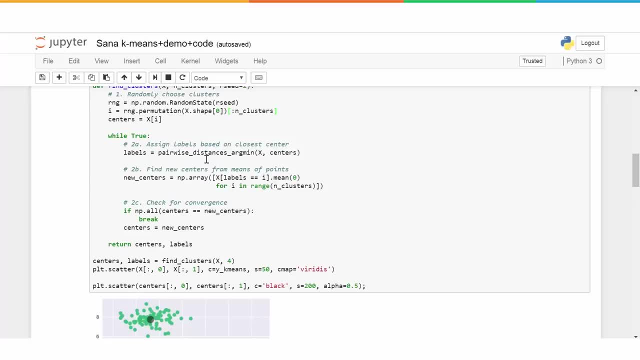 we assign that data, Okay, The data point, to that particular centroid or cluster. And once that is done for all the data points, we calculate the new centroid by finding out the mean position, with the center position right. So we calculate the new centroid and then we check if the new centroid is the coordinates or 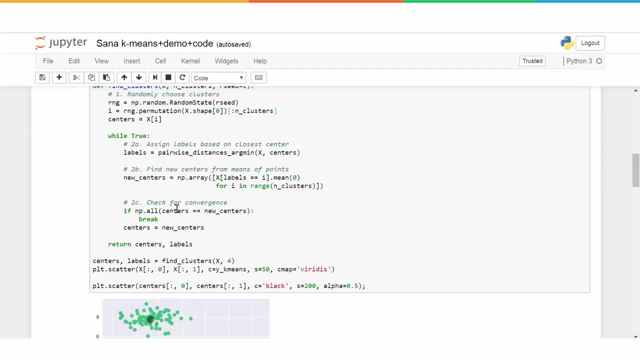 the position is the same as the previous centroid, the positions we will compare And if it is the same, that means the process has converged. So remember, we do this process till these centroid or that centroid doesn't move anymore, right? So the centroid gets relocated each time. this 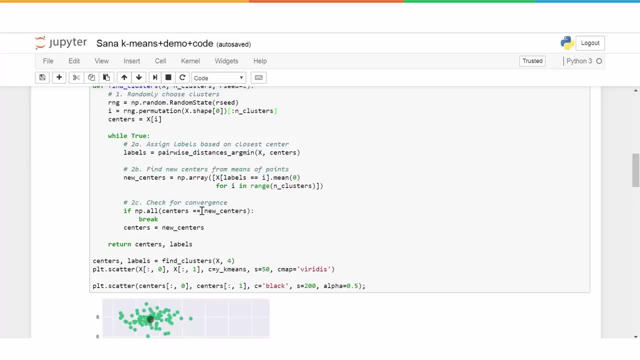 reallocation is done, So the moment it doesn't change anymore. the position of the centroid doesn't change anymore. we know that convergence has occurred, So till that. So you see, here this is like an infinite loop. while true is an infinite loop, It only breaks when the centers or the centers are the same. 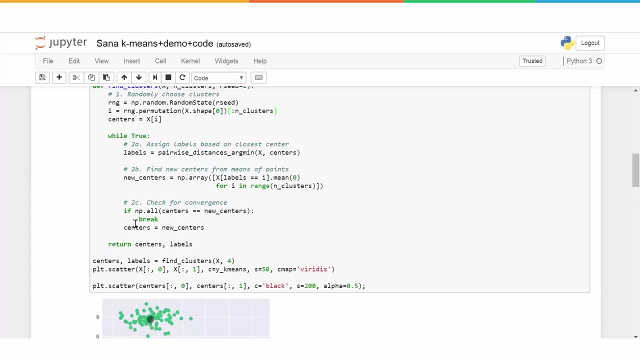 same, the new center and the old center positions are the same, and once that is done, we return the centers and the labels. now, of course, as explained, this is not a very sophisticated and advanced implementation, very basic implementation, because one of the flaws in this is that sometimes, what 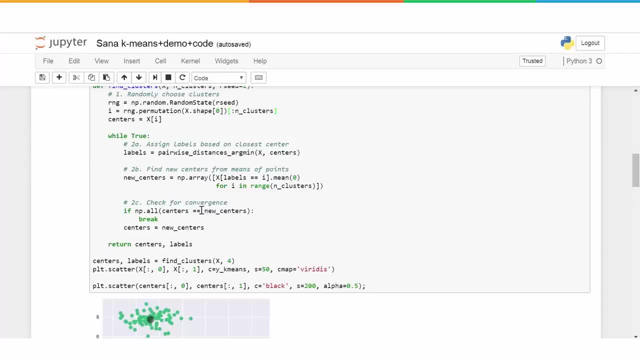 happens is the centroid, the position will keep moving, but in the change will be very minor. so in that case, also with that is actually convergence right. so for example, the change is 0.0001, we can consider that as convergence. otherwise what will happen is this will either take forever or it will. 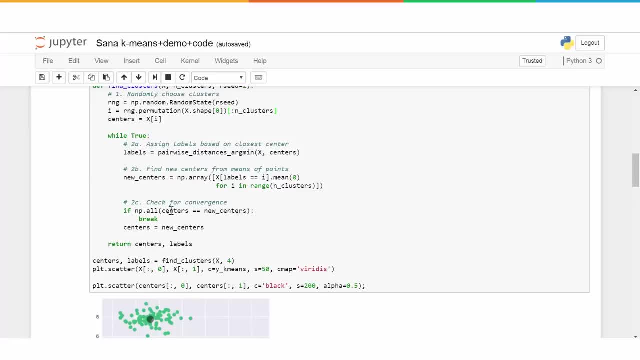 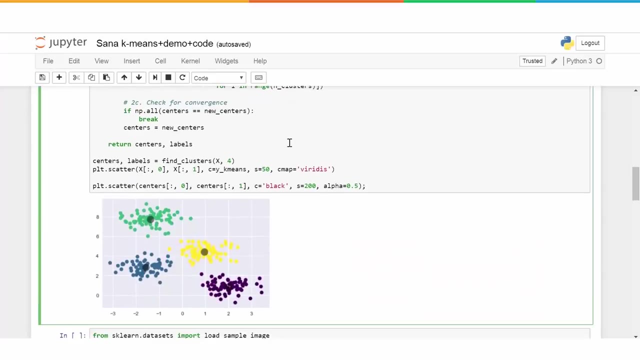 be never ending. so that's a small flaw here. so that is something. additional checks may have to be added here, but again, as mentioned, this is not the most sophisticated implementation. this is like a kind of a rough implementation of the k-means clustering. okay. so if we execute this, 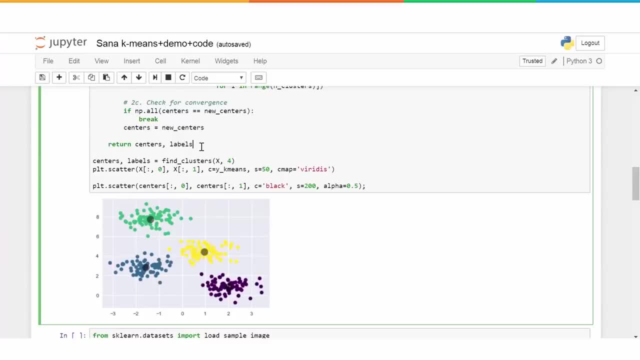 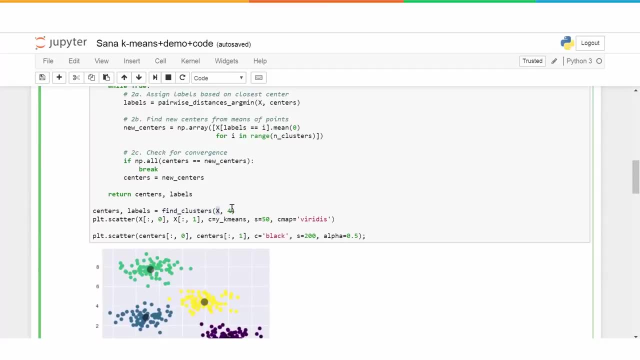 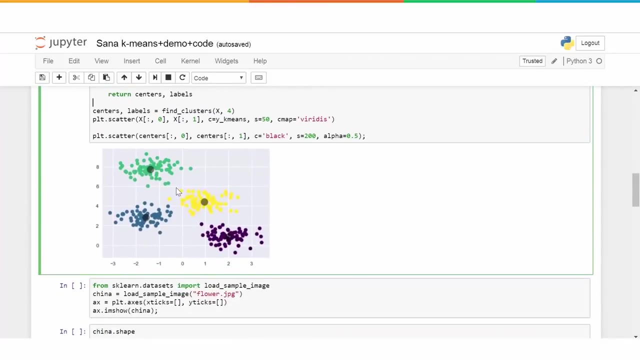 code. this is what we get as the output. so this is the definition of this particular function, and then we call that find underscore clusters and we pass our data, X, and the number of clusters, which is 4, and if we run that and plot it, this is the output that we get. so this is, of course, each 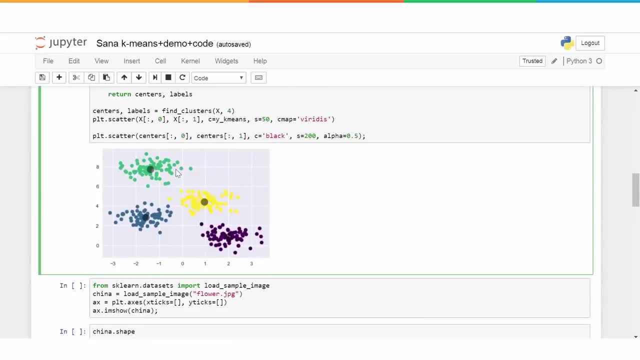 cluster is represented by a different color. so we have a cluster in green color, yellow color and so on and so forth, and these big points here, these are the centroids- is the final position on the center right and, as you can see, visually also, this appears like a kind of a center of all these. 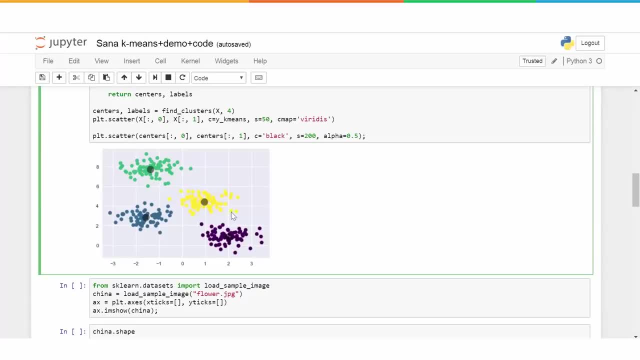 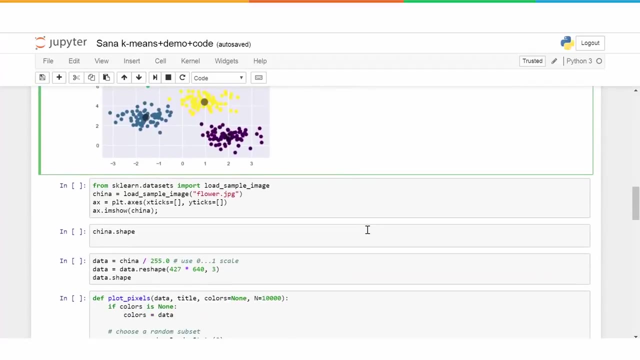 points here, right? similarly, this is like the center of all these points here, and so on. so this is the example, or this is an example of a implementation of k-means clustering, and next we will move on to see a couple of examples of how k-means clustering is used in maybe some real life. 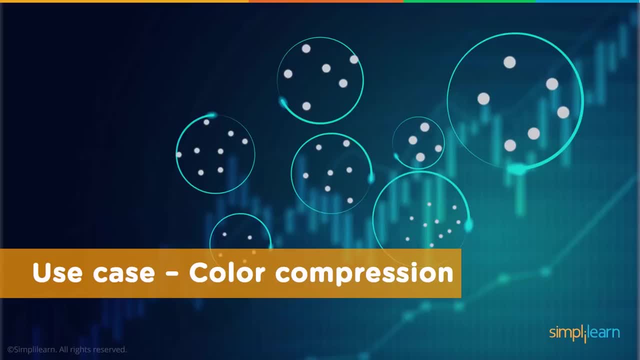 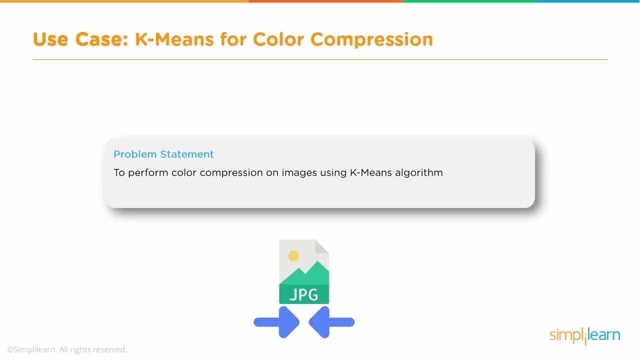 scenarios or use cases. in the next example or demo, we are going to see how we can use k-means clustering to perform color compression. we will take a couple of images, so there will be two examples and we will try to use k-means clustering to compress the colors. this is a common situation in image processing when 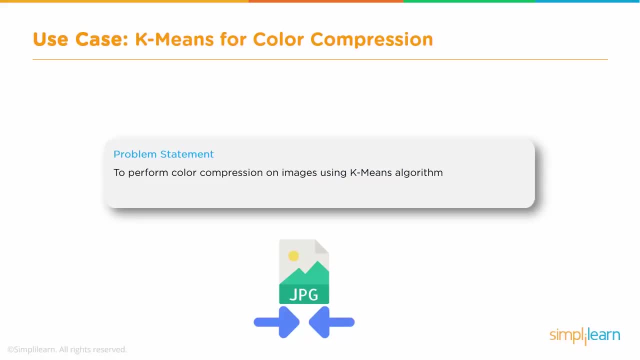 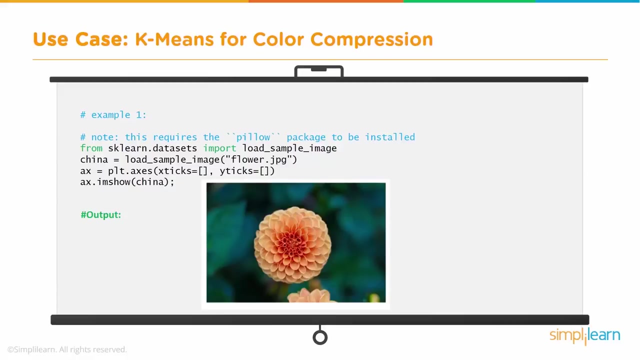 you have an image with millions of colors, but then you cannot render it on some devices which may not be useful in the primary. so that is the scenario where where something like this can be used. so before again we go into the python notebook, let's take a look at quickly the the code. as usual, we 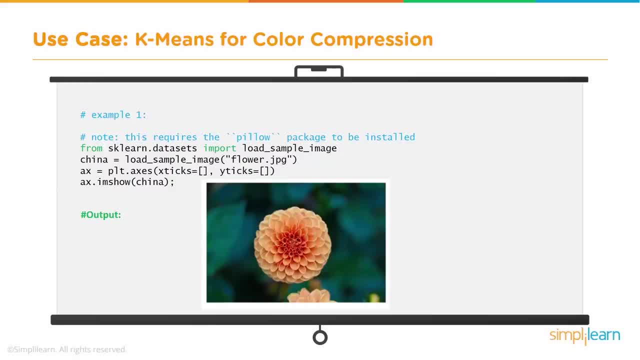 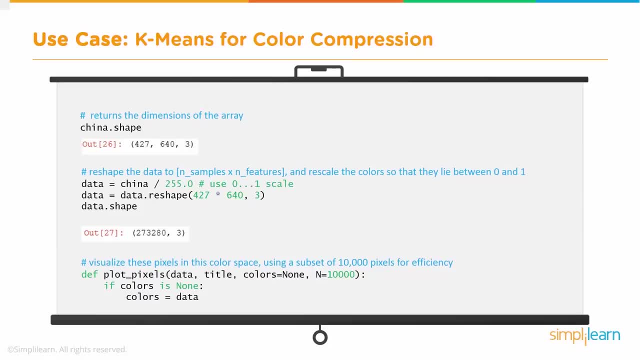 import the libraries and then we import the image and then we will flatten it. so reshaping is basically: we have the image, information is stored in the form of pixels and images like, for example, 427 by 640, and it has three colors. so that's the overall dimension. 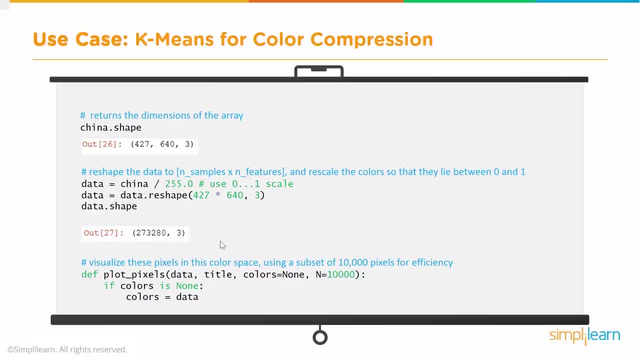 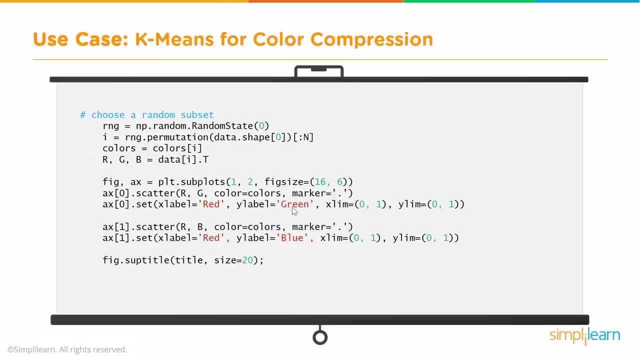 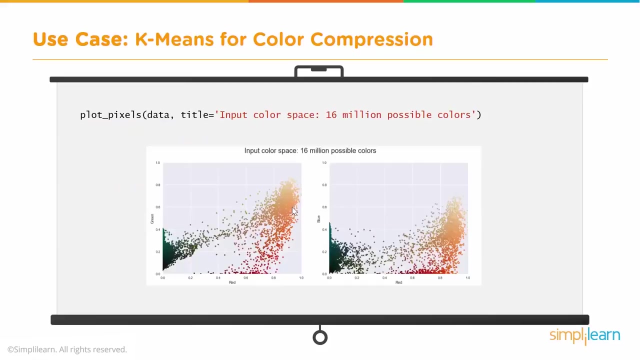 of the of the initial image. we just reshape it and then feed this to our algorithm, and this will then create clusters of only 16 clusters. so this, this colors. there are millions of colors and now we need to bring it down to 16 colors. so we use: k is equal to 16, and this is how, when we visualize, 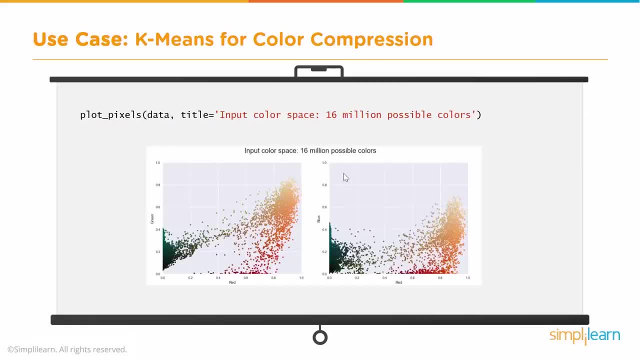 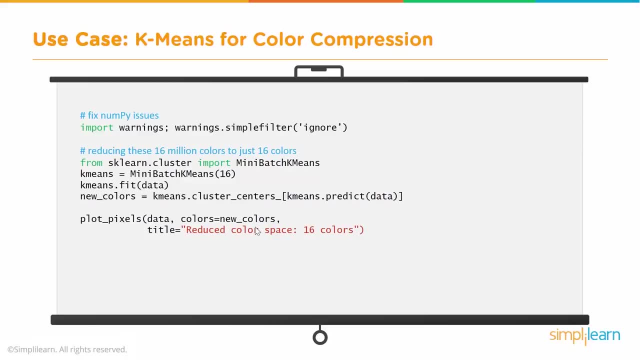 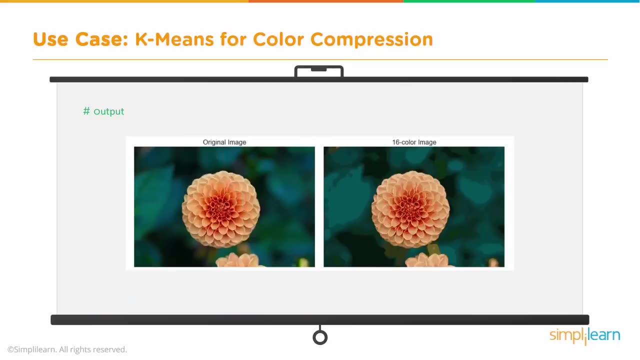 this is how it looks. there are- these are all about 16 million possible colors. the input color space has 16 million possible colors and we just sub compress it to 16 colors. so this is how it would look when we compress it to 16 colors. and this is how the original image looks and after compression. 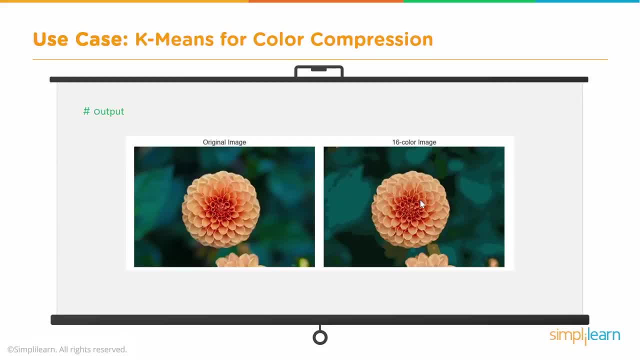 to 16 colors. this is how the new image looks. as you can see, there is not a lot of information that has been lost, though the image quality is definitely reduced a little bit. so this is an example which we are going to now see in python notebook. let's go into the python. 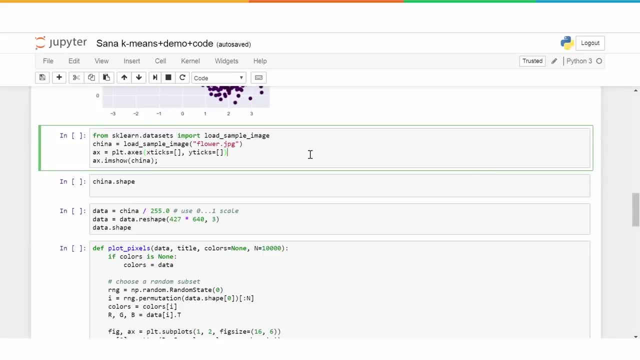 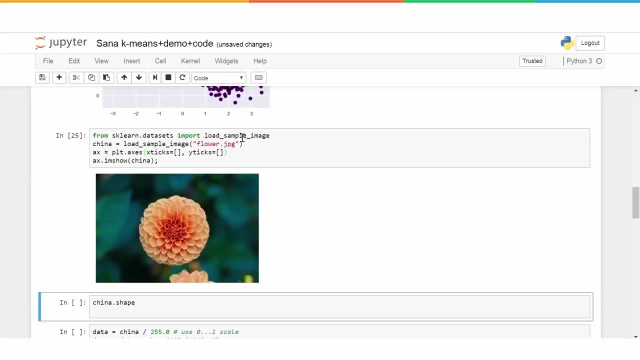 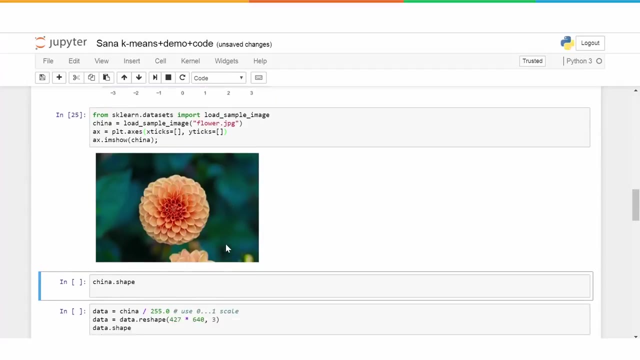 and once again, as always, we will import some libraries and load this image called flowerjpg. okay, so let me load that and this is how it looks. this is the original image, which has, i think, 16 million colors, and this is the shape of this image, which is basically what is. the shape is nothing. 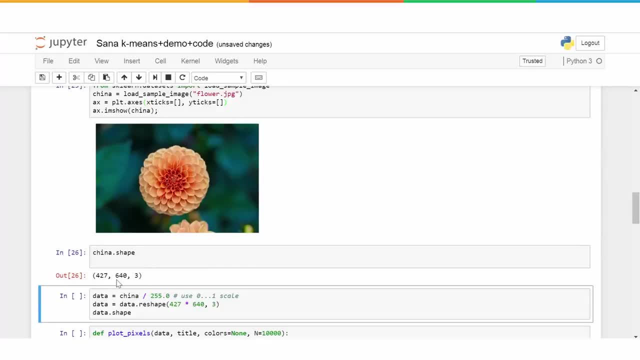 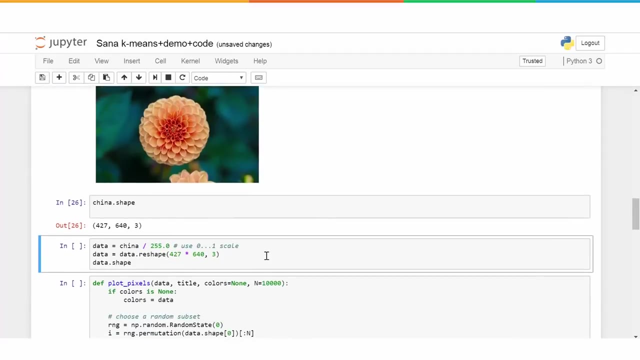 but the overall size right. so this is 427 pixel by 640 pixel and then there are three layers, which is this. three basically is for rgb, which is red, green, blue. so color image will have that right. so that is the shape of this in terms of shape of the image. now what we need to do is data. let's take a look at how data is. 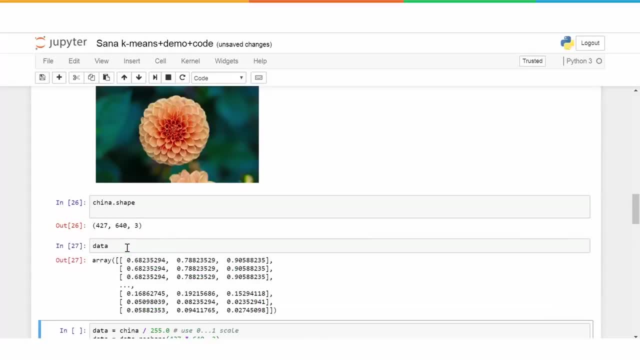 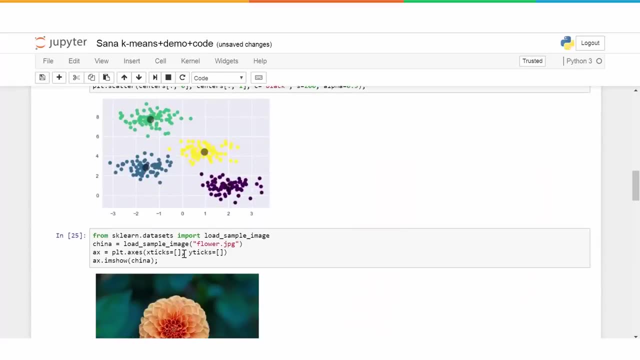 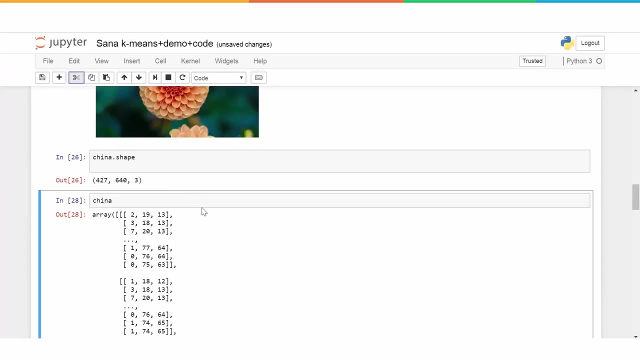 looking. so let me just create a new cell and show you what is in data. basically, we have captured this information, so data is what? let me just show you here. all right, so let's take a look at china. what are the values in china? and if we see here, this is how. 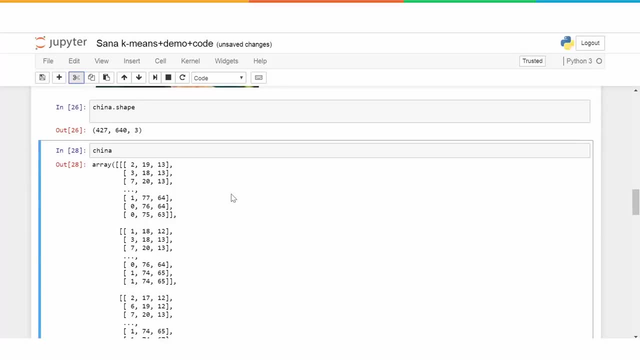 is nothing but the pixel values. okay, so this is like a matrix, and each one has about for for this, 427 by 640 pixels. all right, so this is how it looks. now, the issue here is: these values are large, the numbers are large, so we need to normalize them to between 0 and 1, right so? 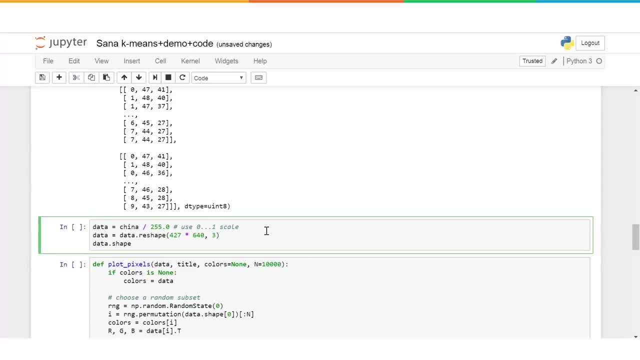 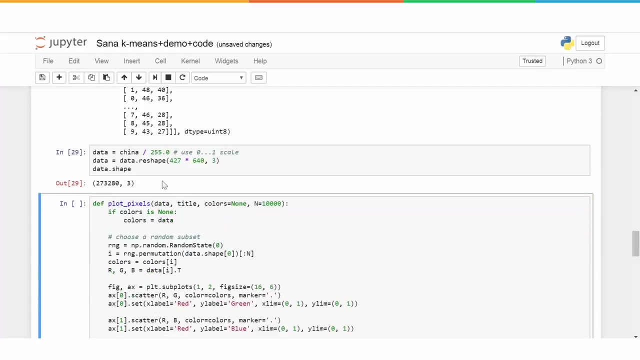 that's why we will basically create one more variable, which is data, which will contain the values between 0 and 1, and the way to do that is divide by 255, so we divide china by 255 and we get the new values in data. so let's just run this piece of code and this is the shape, so we 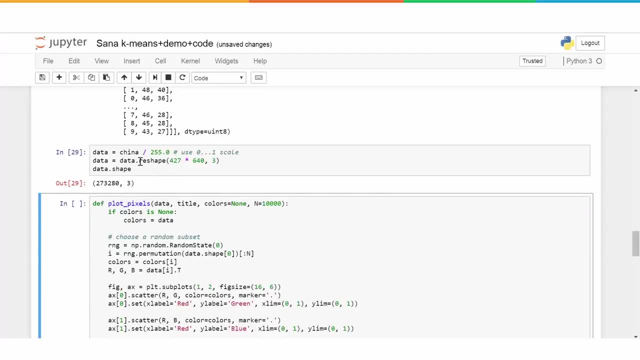 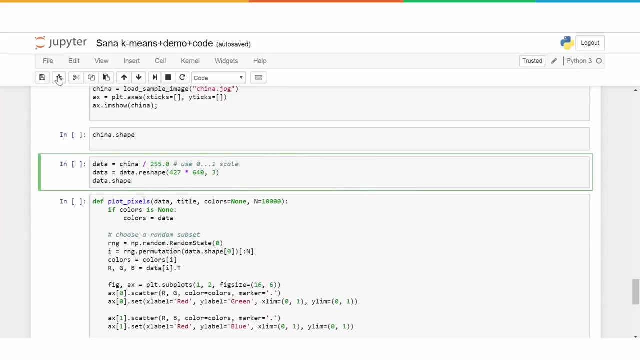 now have also. yeah, what we have done is we changed using reshape, we converted into the three dimensional, into a two-dimensional data set, and let us also take a look at how. let me just insert a, probably a cell here and take a look at how data is looking all right. so this is how data 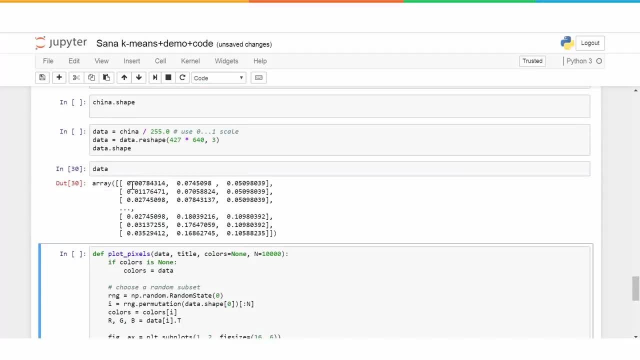 is looking and now you see, this is: the values are between zero and one, right? so if you earlier noticed, in case of china, the values were large numbers. now everything is between zero and one. this is one of the things we need to do, all right? so after that, the next thing that we 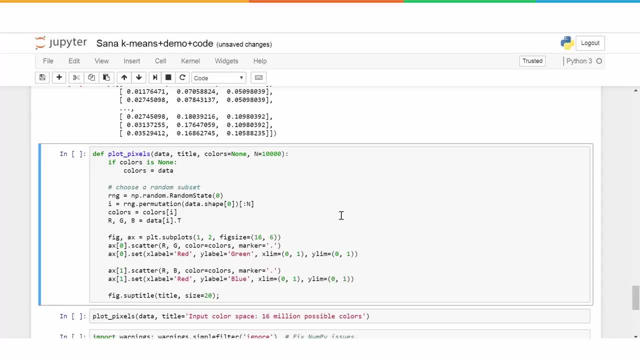 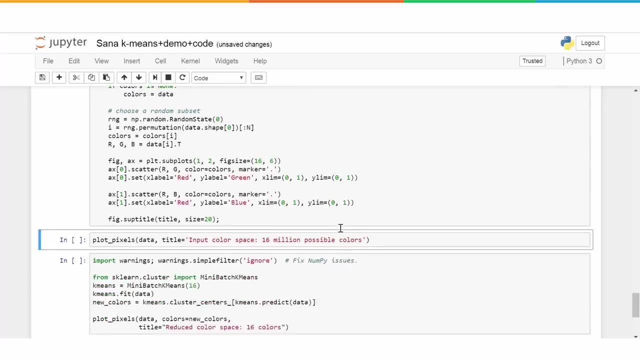 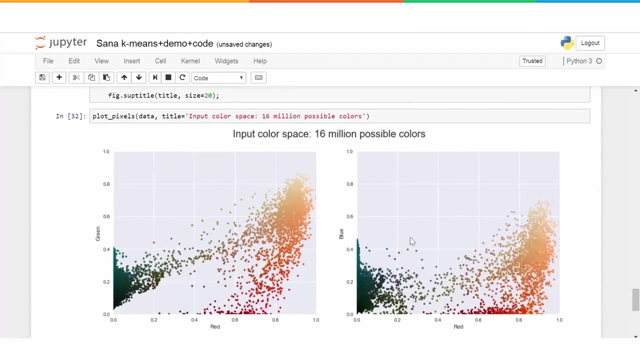 need to do is to visualize this and, uh, we can take random set of maybe 10 000 points and plot it and check and see how this looks. so let us just plot this. and so this is how the original, the color, the pixel distribution is. these are two plots. one is red against green and 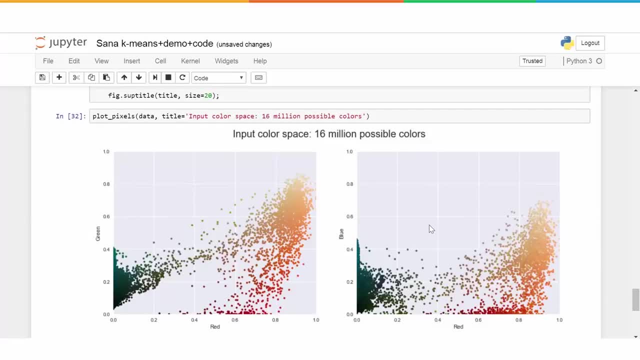 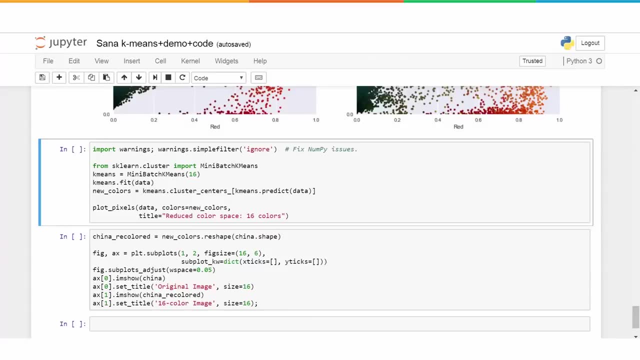 another is red against blue, and this is the original distribution of the color. so, then, what we will do is we will use k-means clustering to create just 16 clusters for the various colors, and then apply that to the image. now what will happen is, since the data is going to be: 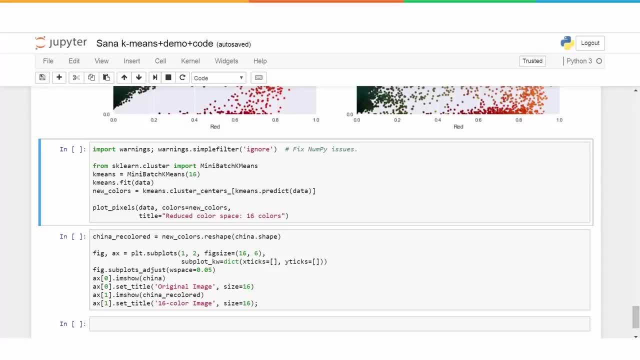 large because there are millions of colors. using regular k-means may be a little time consuming, so there is another version of k-means which is called mini batch k-means, so we will use that, which is which processes in. the overall concept remains the same, but this basically processes it. 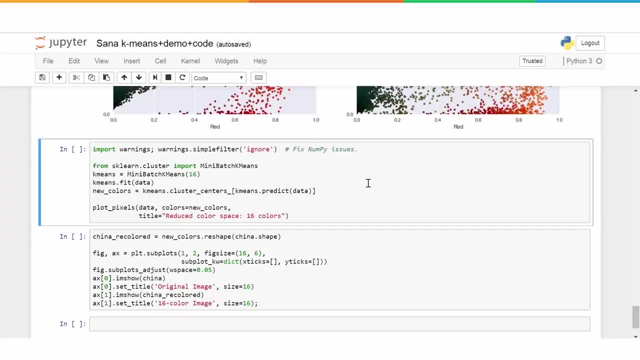 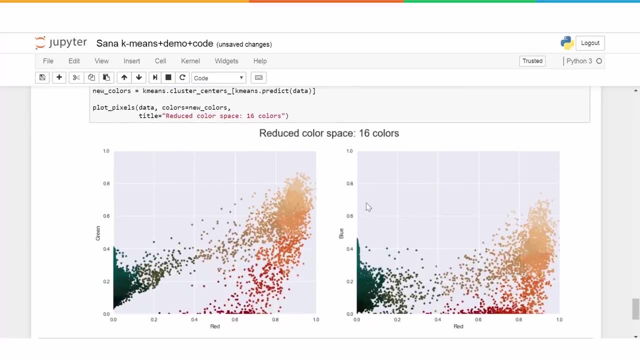 in smaller batches. that's the only thing, okay, so the results will pretty much be the same. so let's go ahead and execute this piece of code and also visualize this so that we can see: are these? this is how the 16 colors, uh, would look. so this is red against green and this is 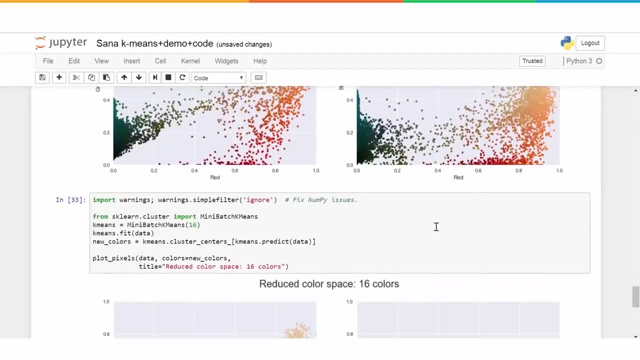 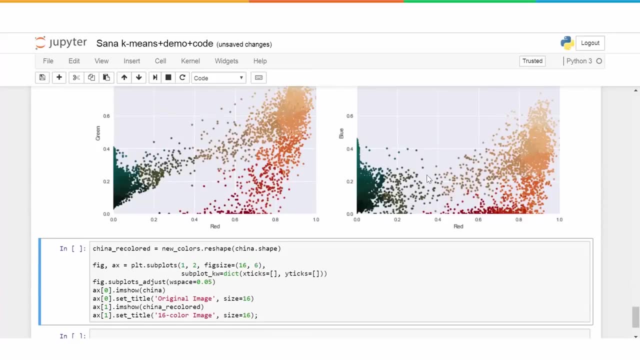 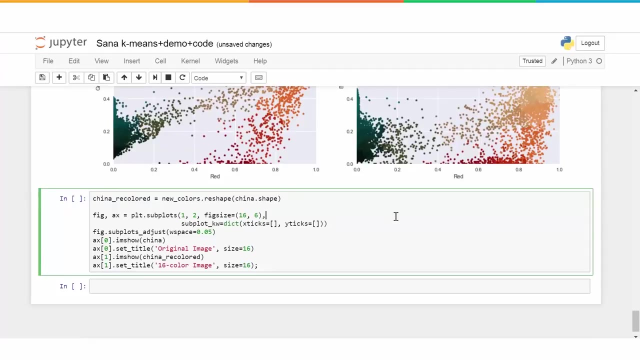 red against blue. there is a quite a bit of similarity between this original color schema and the new one, right, so it doesn't look very, very completely different or anything like that. now we apply this- the newly created colors- to the image, and we can take a look. 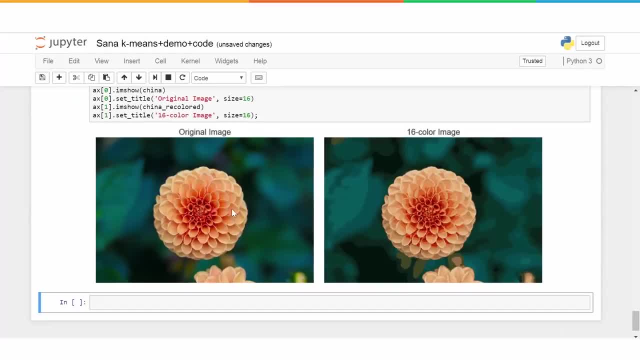 how this is looking. now we can compare both the images. so this is our original image and this is our new image. so, as you can see, there is not a lot of information that has been lost. it pretty much looks like the original image. yes, we can see that. for example, here there is a little. 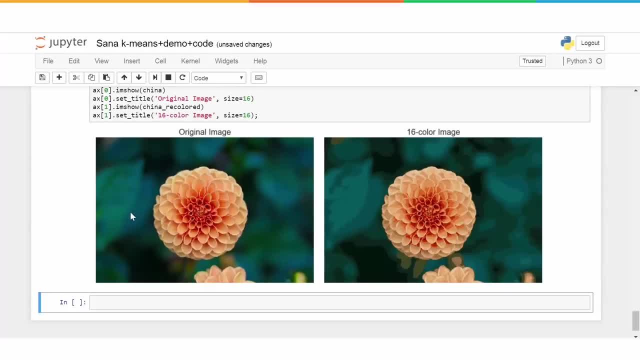 bit. it appears a little dullish compared to this one right because we kind of took off some of the finer details of the color, but overall the high level information has been maintained. at the same time, the main advantage is that now this is a little bit duller than the original color. 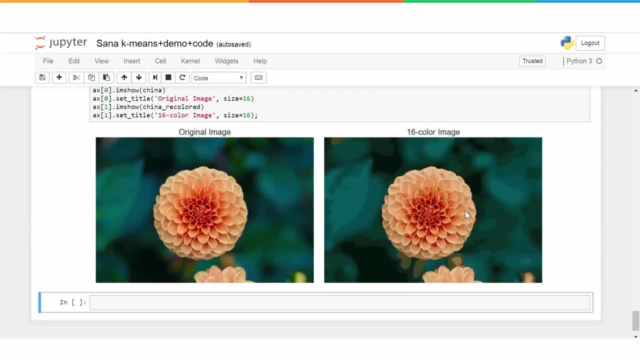 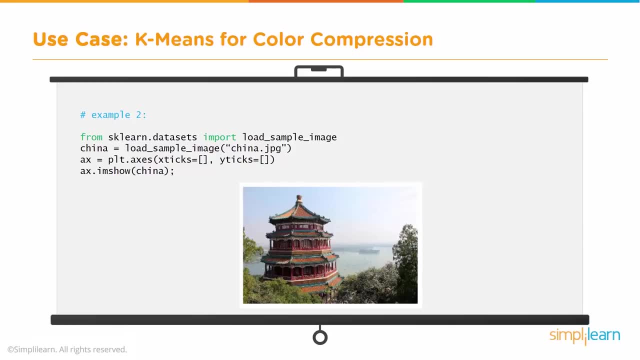 so this can be. this is an image which can be rendered on a device which may not be that very sophisticated. now let's take one more example with a different image. in the second example, we will take an image of the summer palace in china and we repeat the same process. this is a high definition. 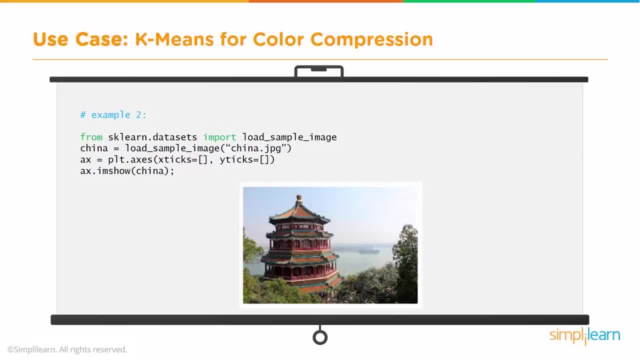 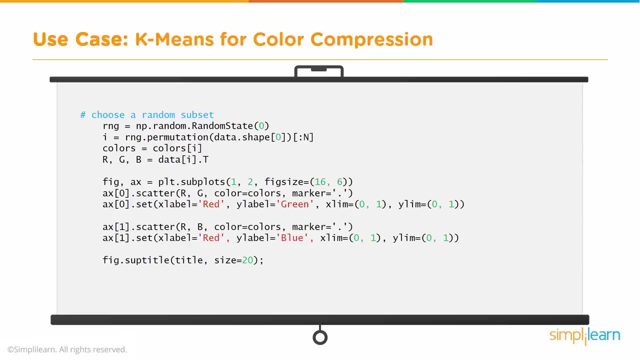 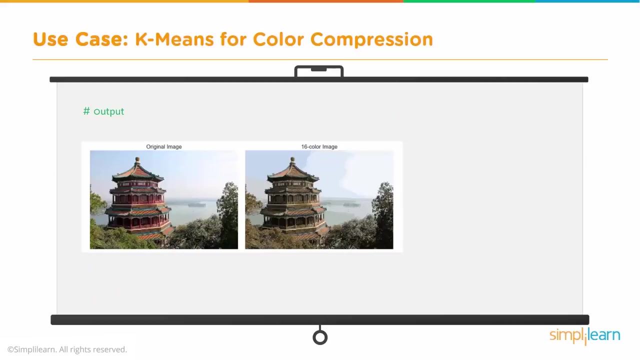 color image with millions of colors and also three-dimensional. now we will reduce that to 16 colors using k-means, clusters, and we do the same process like before. we reshape it and then we cluster the colors to 16 and then we render the image once again and we will see that the color, the quality of the image slightly. 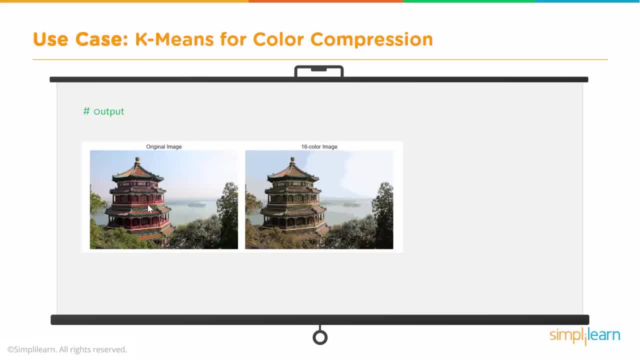 deteriorates, as you can see here. this has much finer details in this which are probably missing here, but then that's the compromise, because there are some devices which may not be able to handle this kind of high density images. so let's run this call in python notebook. 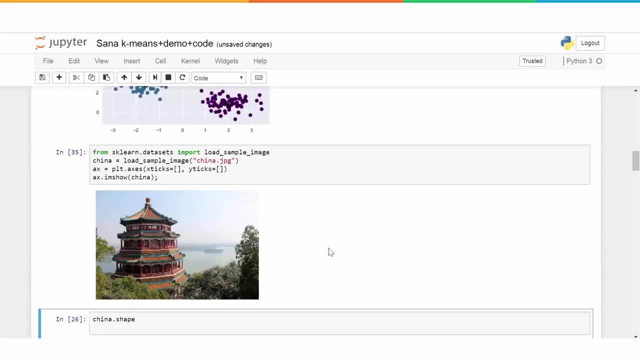 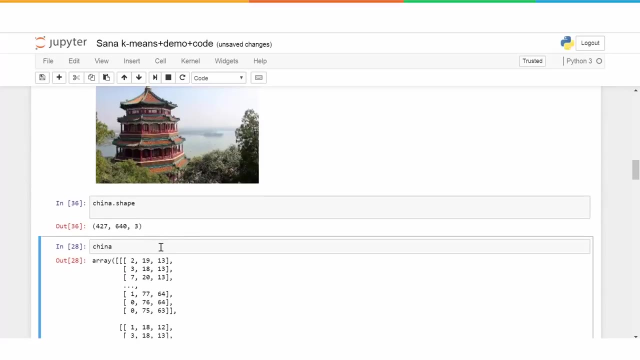 all right. so let's apply the same technique for another picture which is even more intricate and has probably much complicated color schema. so this is the image now once again. uh, we can take a look at the shape, which is 427 by 640 by 3, and this is the new data. would look somewhat like this: compared to the picture, you can see that the colors are much, much better. seçing to collection more, so we can make some children with beaten to white, to purple assistant and lose the traditional coloramızi. let's see now how comes to it. let's take a unlike of a higher degree, so let's apply this one for theization of color, that is. 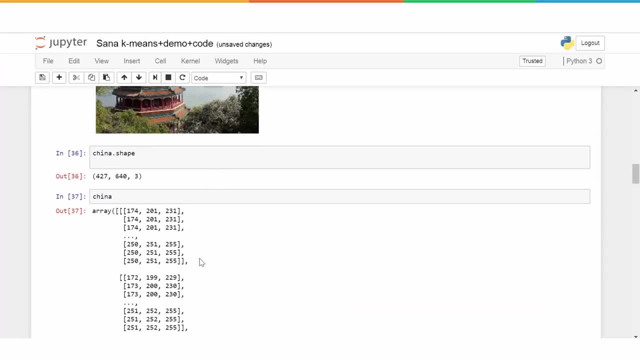 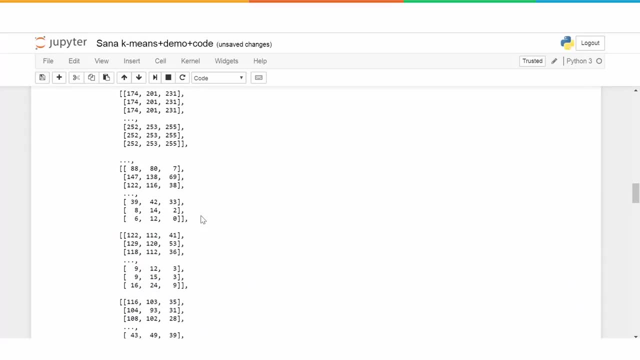 somewhat like this compared to the flower image. So we have some new values here and we will also bring this. as you can see, the numbers are much big, so we will much bigger, So we will now have to scale them down to values between zero and one. 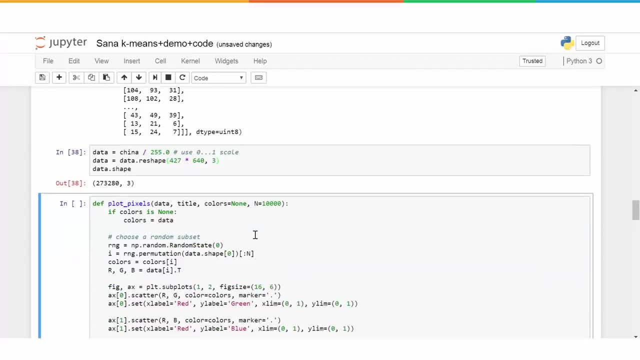 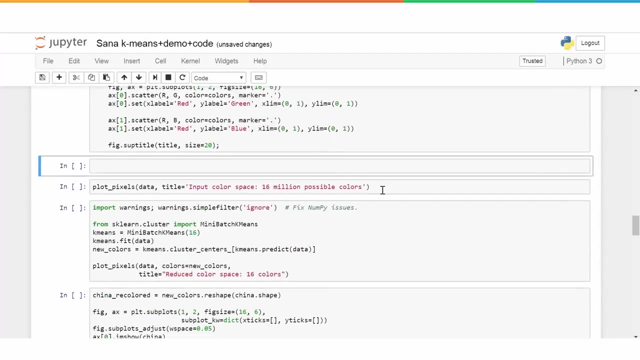 and that is done by dividing by 255.. Let's go ahead and do that and reshape it, okay? So we get a two dimensional matrix and we will then, as a next step, we will go ahead and visualize this how it looks. 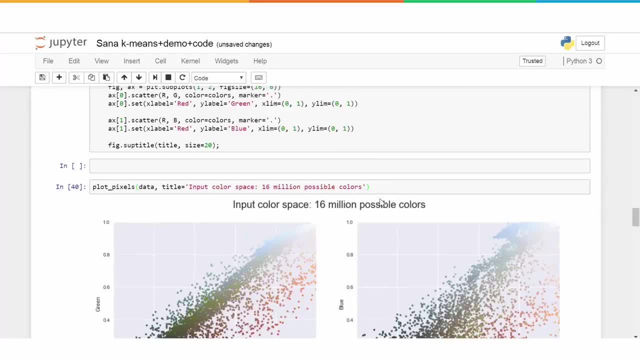 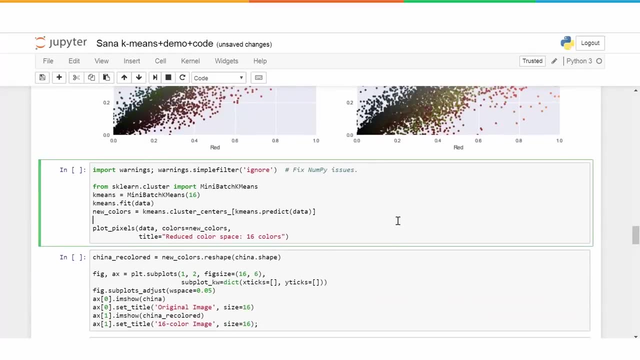 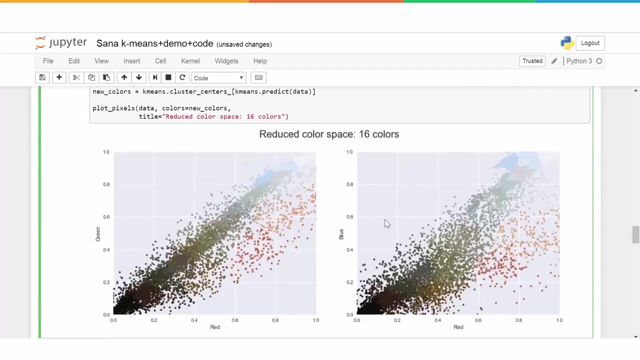 the 16 colors and this is basically how it would look: 16 million colors. And now we can create the clusters out of this, the 16 k-means clusters we will create. So this is how the distribution of the pixels would look. 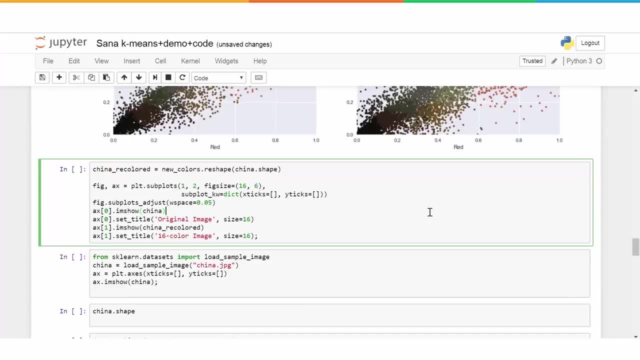 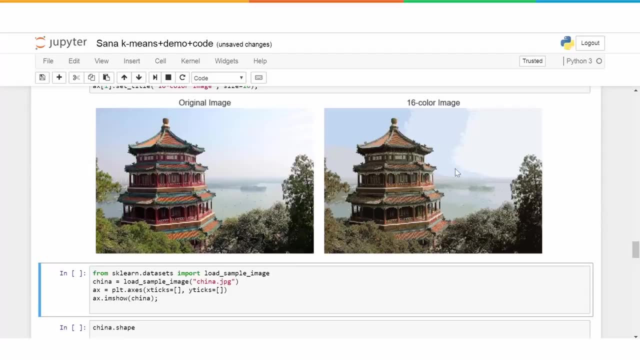 with 16 colors, And then we go ahead and apply this and visualize how it is looking for with the new, just the 16 color. So once again, as you can see, this looks much richer in color but at the same time, 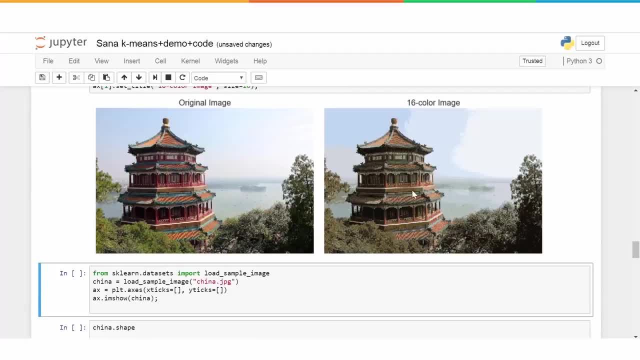 and this probably doesn't have. as we can see, it doesn't look as rich as this one, but nevertheless the information is not lost, the shape and all that stuff, And this can be also rendered on a slightly a device, which is probably not that. 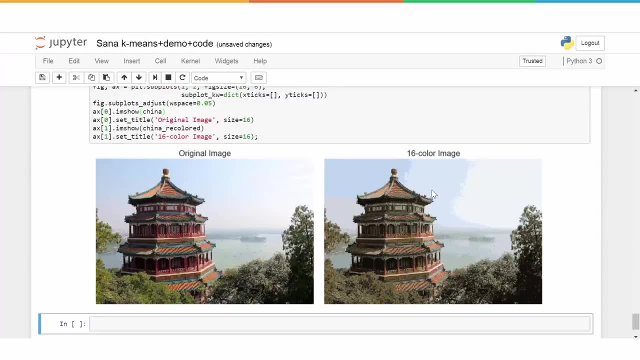 sophisticated. Okay, so that's pretty much it. So we have seen two examples of how color compression can be done using k-means clustering, And we have also seen, in the previous examples of how to implement k-means, the code to roughly how to implement k-means clustering. 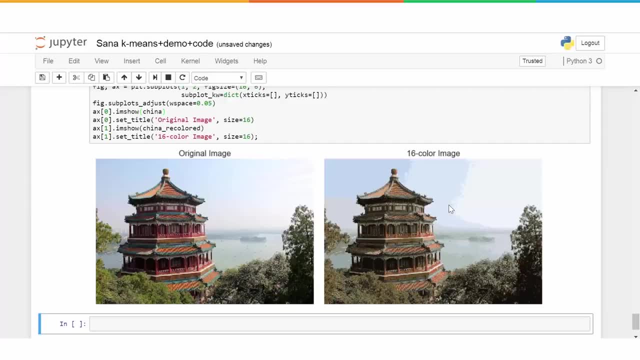 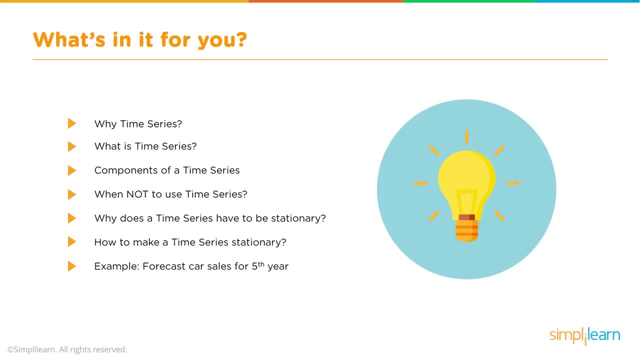 And we use some sample data using blob to just execute the k-means clustering. In this video we are going to talk about what time series forecasting is, and this is a two-part series, And in this first video we will explain what is time series analysis. 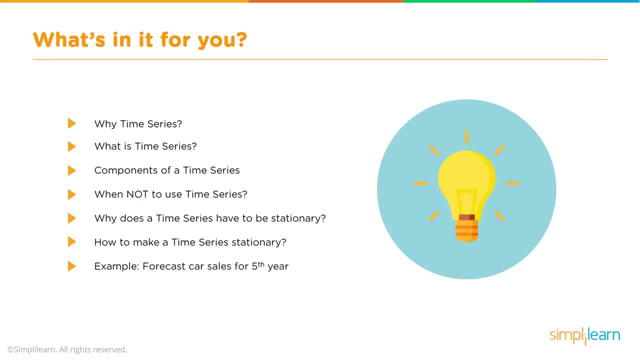 And in the second part we will actually demonstrate it in our studio. So this is what we are going to cover in this video. First of all, why time series? And then we'll talk about what exactly is time series data, And then what are the components of a time series data. 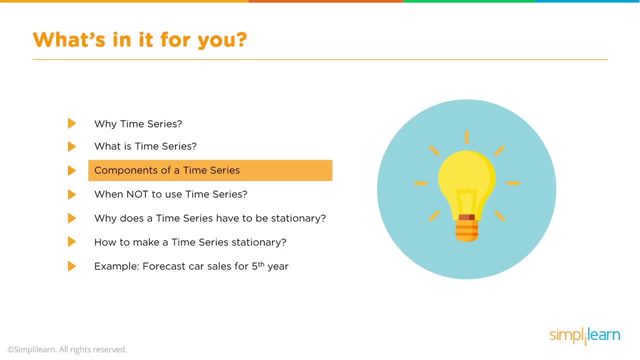 Like, for example, the trends, seasonality and so on, And then we will explain what each of these components are. We'll also talk about when we should not use time series analysis, And we will then explain what is stationary data in terms of time series. 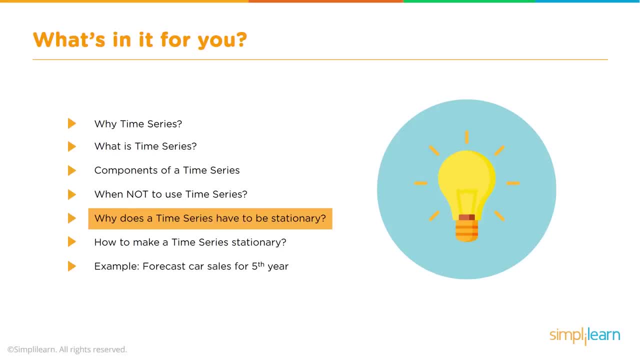 What is the significance of stationary data? And typically time series data is not stationary. So how to make time series data stationary? And then we will take you through an example of a car sales data And we will show you how to solve the time series. 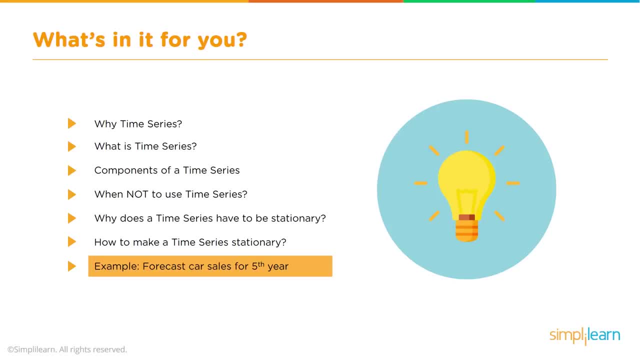 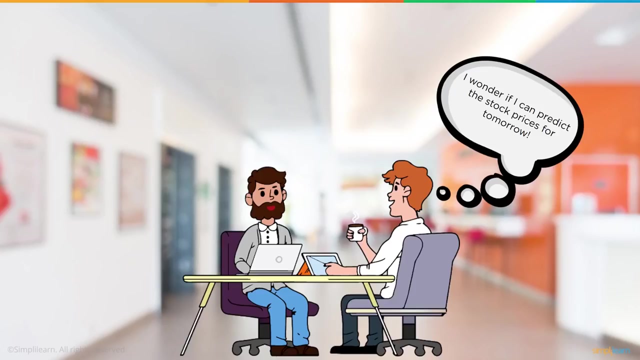 or how to perform the time series analysis manually without using the tool, And then we will do in the second part, we will actually use R and we will do the same thing once again in R. Okay, so without any further delay, let's get started. 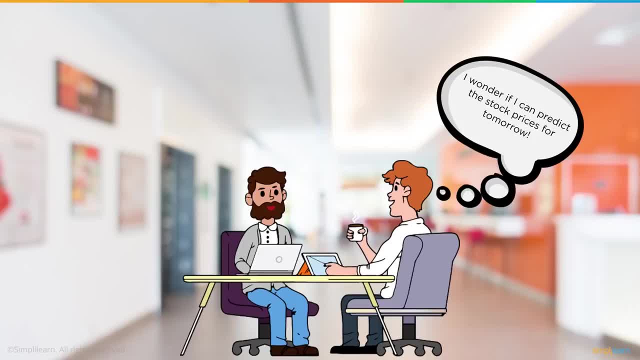 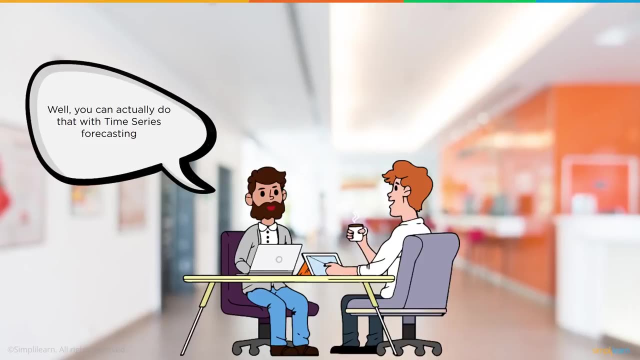 And so why exactly do we need to do time series analysis? Typically, we would like to predict something in the future, And it could be stock prices, it could be the sales or anything that needs to be predicted into the future. That is when we use time series analysis. 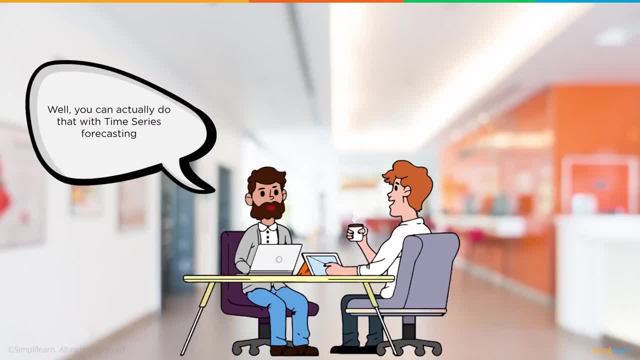 So it is as the name suggests. it is forecasting And typically when we say predicted need not be to the future, in machine learning and data analysis, when we talk about predicting we are not necessarily talking about the future, But in time series analysis we typically predict the future. 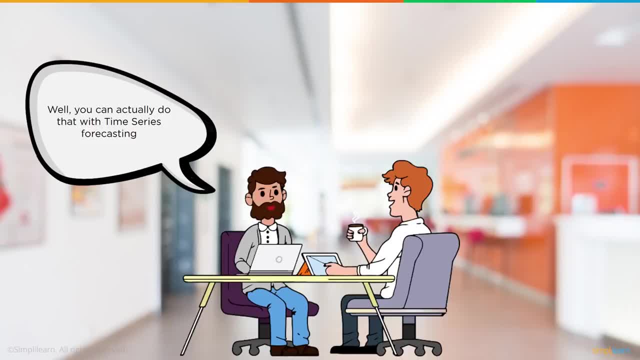 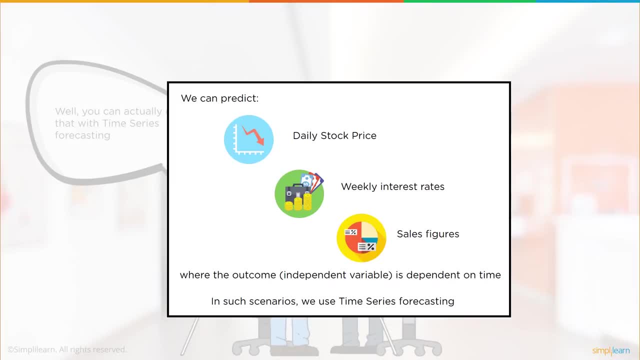 So we have some past data and we want to predict the future. That is when we perform time series analysis. So what are some of the examples? It could be daily stock price, the shares as we talk about, or it could be the interest rates- weekly interest rates. 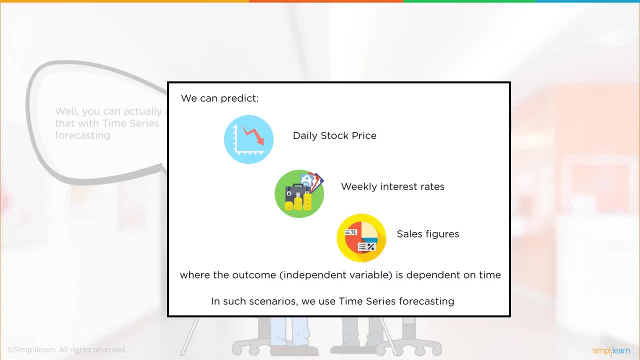 or sales figures of a company. So these are some of the examples where we use time series data. We have historical data which is dependent on time And then, based on that, we create a model to predict the future. So what exactly is a type series? 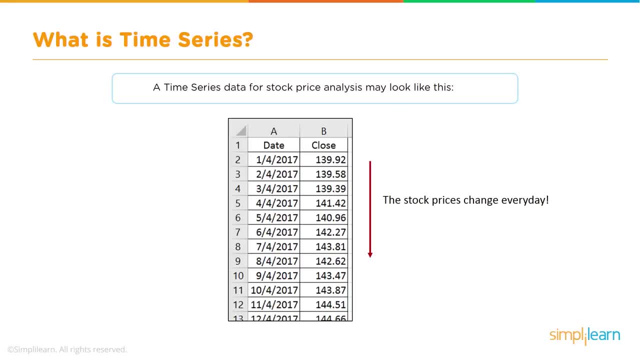 So time series data has time as one of the components, as the name suggests. So in this example, let's say this is the stock price data and one of the components. so there are two columns here. column B is price and column A is basically. 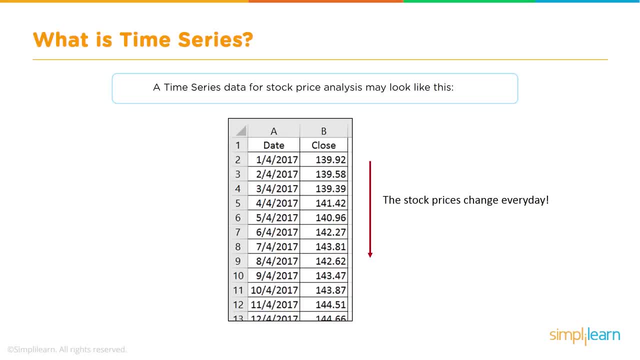 the time information, In this case the time day, so that primarily the closing price of a particular stock has been recorded on a daily basis. so this is a time series data and the time interval is obviously a day. time series or time intervals can be daily, weekly, hourly or 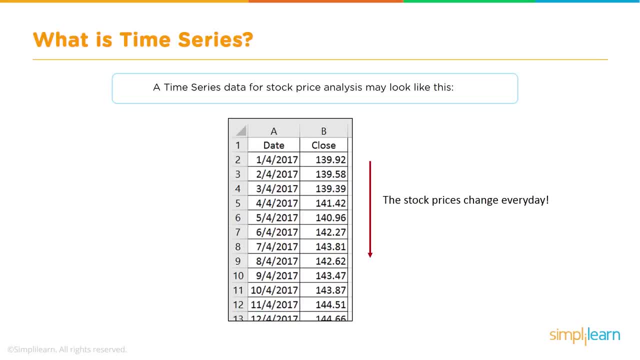 even sometimes there is something like a sensor data. it could be every few milliseconds or microseconds as well, so the size of the time intervals can vary, but they are fixed. so if I am saying that it is daily data, then the interval is fixed as daily. if I'm saying this data is an hourly data, then it is the. 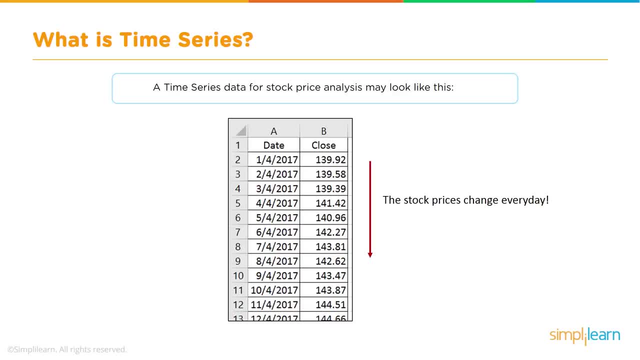 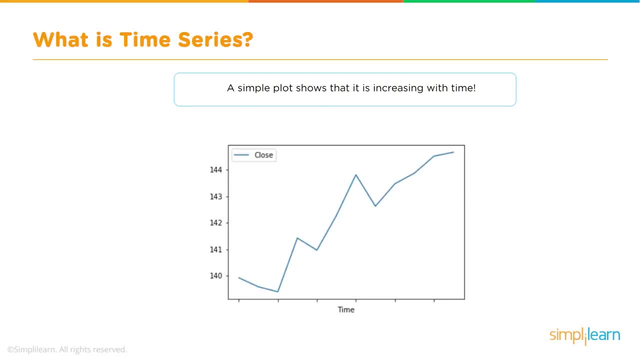 data is captured every hour and so on. so the time intervals are fixed. the interval itself you can decide based on what kind of data we are capturing. so this is a graphical representation- the previous one, here we saw the table representation- and this is how the plot, the data. so on the y-axis is, let's say, 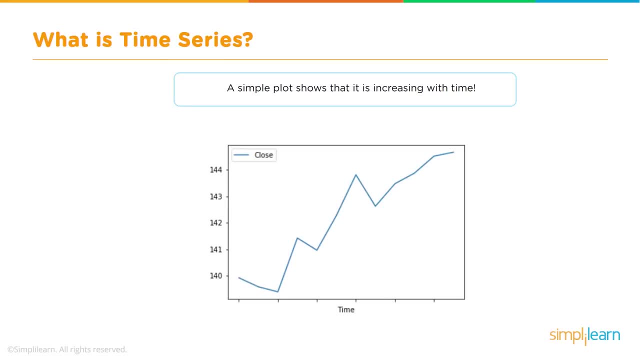 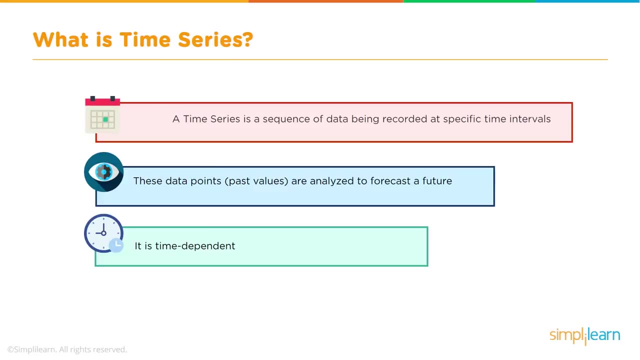 the price or the the stock price, and x-axis is the time. so against time. if you plot it, this is how time series graph would look. so, as the name suggests, what is time series data? time series data is basically a sequence of data that is recorded over a 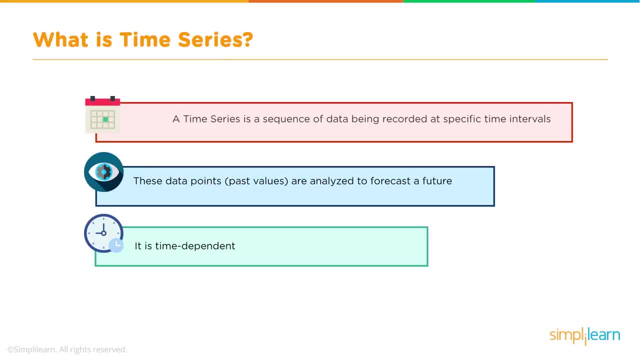 specific intervals of time and based on the past values. so if we want to do an analysis of time series- past data- we try to forecast a future and again, as the name suggests, it is time series data, which means that it is time dependent, so time is one of the components of this data. time series data consists of: 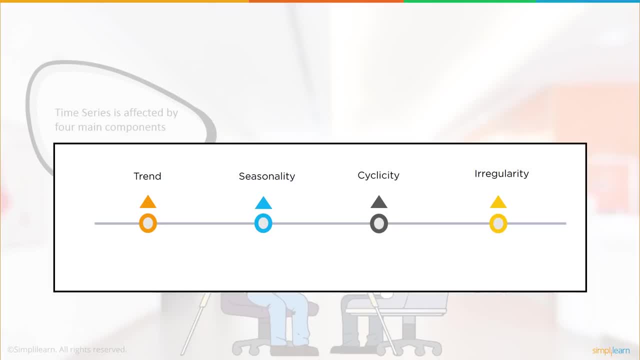 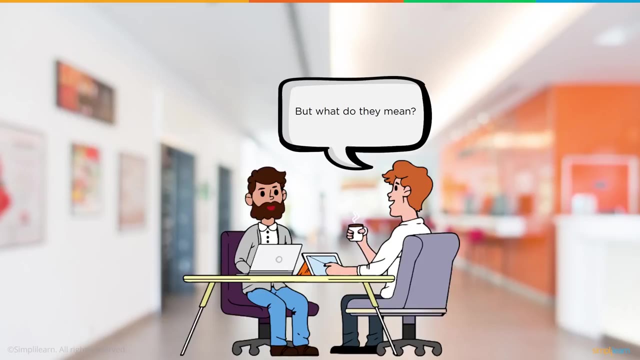 primarily four components. one is the trend, then we have the seasonality, then cyclicity and then, last but not least, irregularity, or the random component. sometimes is also referred to as a random component. so let's see what each of these components are. so what is trend? trend is overall change or the pattern. 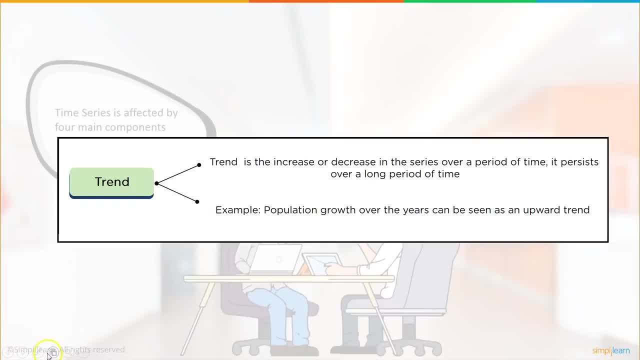 of the data, which means that the data may be. let me just pull up the pen and show you. so let's say, you have a data set somewhat like this, a time series data set somewhat like this. all right, so what is the overall trend? there is an overall trend which is upward trend, as 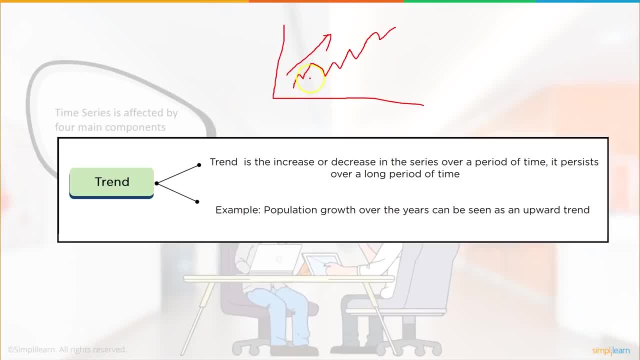 we call it here right, so it is not like it is continuously increasing. there are times when it is dipping, then there are times when it is increasing, then it is decreasing and so on, but overall, over a period of time, from the time we start recording to the time we end, there is a 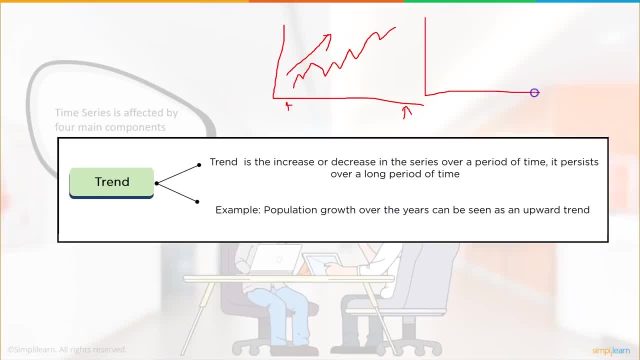 trend. right, there is an upward trend in this case, so the trend need not always be upwards. there could be a downward trend as well. so, for example, here there is a downward trend, right. so this is basically what is a trend overall, whether the data is increasing or decreasing. all right, then we have the 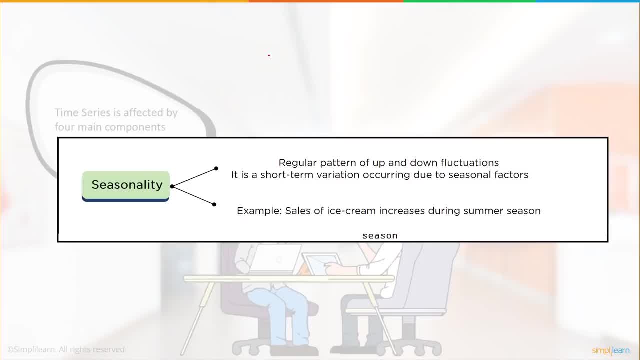 next component, which is seasonality. what is seasonality? seasonality, as the name suggests, once again changes over a period of time and periodic changes, right. so there is a certain pattern. let's take the sales of warm clothes, for example. so if we plot it along the months, so let's say January, February, 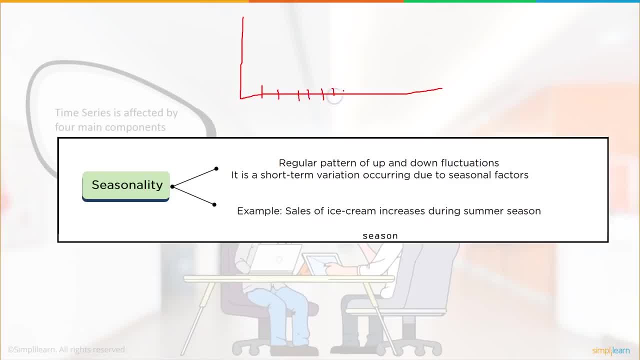 March, April, May, June, July, and then, let's say, it goes up to December. okay, so this is our December. you Thank You, Bob. if you liked this video, please subscribe to the channel and hit the like button. please share it with your friends and family. and so let's say they come down. 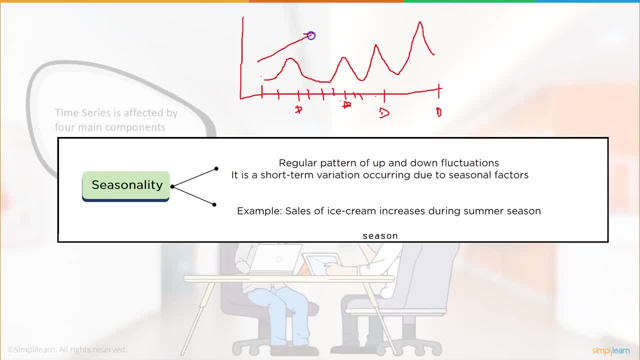 and then there will be again an increase, and then they will come down, and then again an increase, and then they will come down. let's say this is the sales pattern. so you see, here there is a trend as well. there is an upward trend. right, the sales are increasing over. let's say these are multiple years, this. 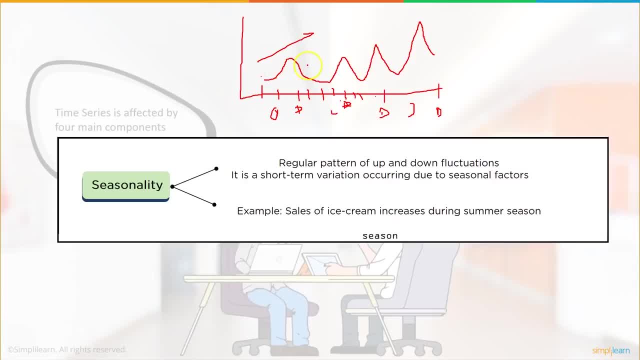 is for year 1, this is for year 2, this is for year 3 and so on. so for multiple years, overall, the trend there is an upward trend, the sales are increasing, but every december the sales are increasing or they are peaking for that particular year. right then, 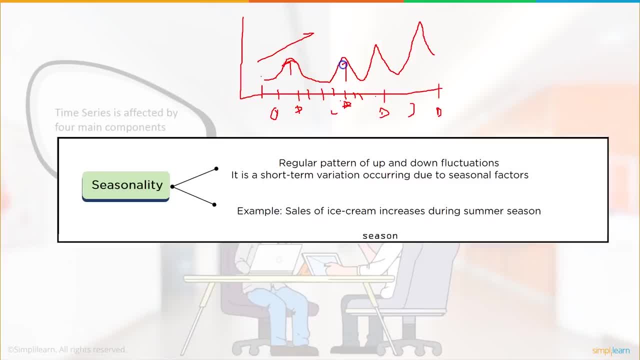 there is a new year again. when december approaches, the sales are increasing again. when december approaches, the sales are increasing, and so on and so forth. so this is known as seasonality. so there is a certain fluctuation, which is which is periodic in nature. so this is known as seasonality. 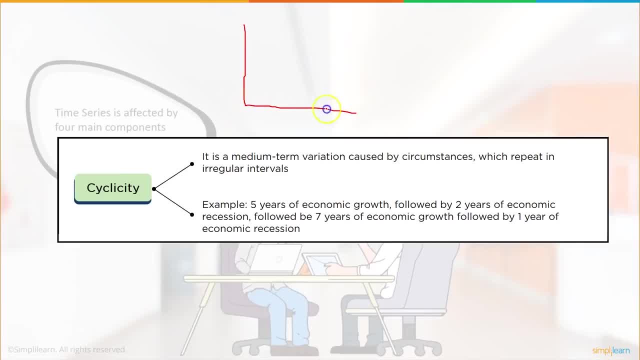 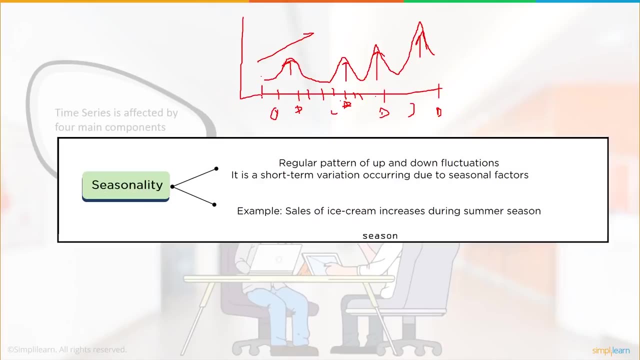 then cyclicity. what is cyclicity now? cyclicity is somewhat similar to seasonality, but here the duration between two cycles is much longer, so seasonality typically is referred to as an annual kind of a sequence, like for example we saw here. so it is pretty much like every year. 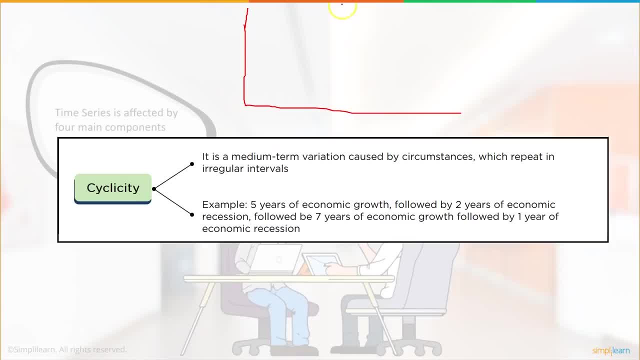 in the month of december, the sales are increasing. however, cyclicity. what happens is, first of all, the duration is pretty much not fixed and the duration or the cycle chakra veut to halt or to discuss multiple cycles of each year. therefore, it's an annual cycle. around the month of december, the sales are increasing. However, the duration is not fixed and the duration 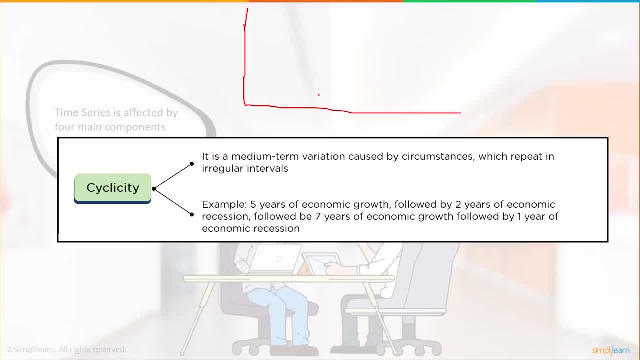 gap length of time between two cycles can be much longer. so recession is an example. so we had, let's say, recession in 2001 or 2002 perhaps, and then we had one in 2008, and then we had probably in 2000, 2012, and so on and so forth. so it is not. 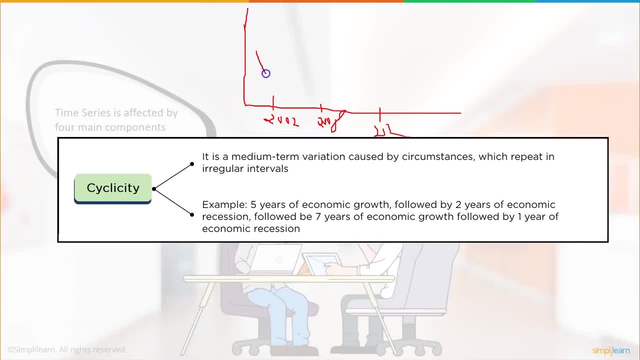 like every year, this happens, probably, so there is usually when we say recession, there is a slump and then it recovers, and then there is a slump and then it recovers, and probably there is another bigger slump, and so on. right, so you see, here this is similar to seasonality, but first of all, this length is much more. 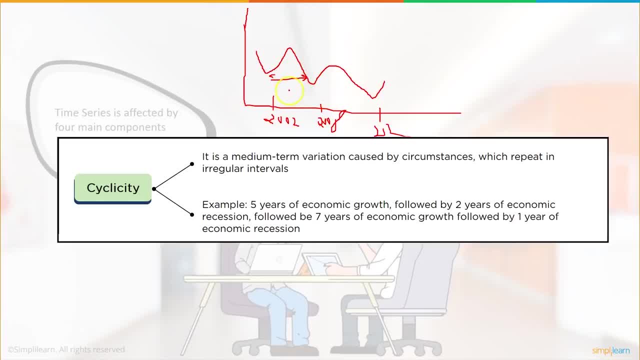 than a year. right, that is number one. and it is not fixed as well. it is not like every four years or every six years. that duration is not fixed, so the duration can vary. at the same time, the gap between two cycles is much longer compared to seasonality. 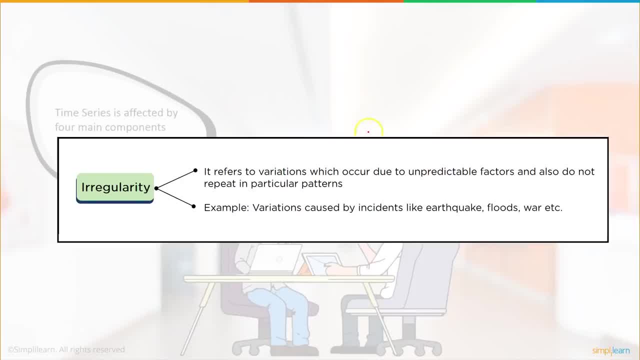 all right. so then, what is irregularity? irregularity is like the random component of the time series data. so there is like you have part which is the trend, which tells whether the overall it is increasing or decreasing. then you have cyclicity and seasonality, which is like kind of a specific 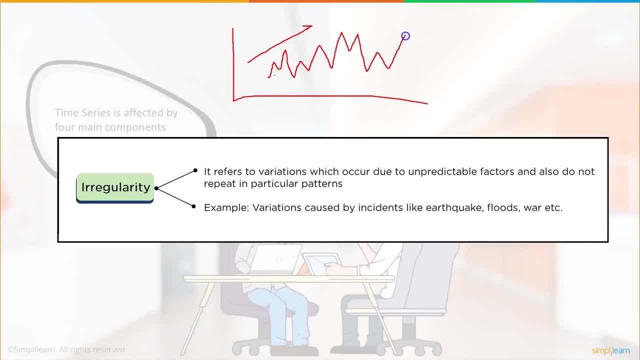 pattern, right. then there is a cyclicity, which is again a pattern, but at much longer intervals. plus, there is a random component, so which is not really which cannot be accounted for very easily, right? so there will be a random component, which can be really random, as the name suggests, right? 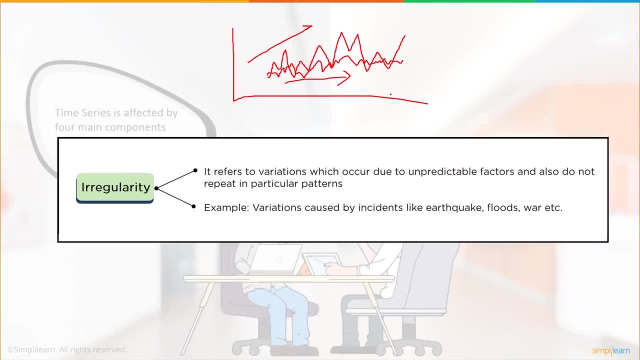 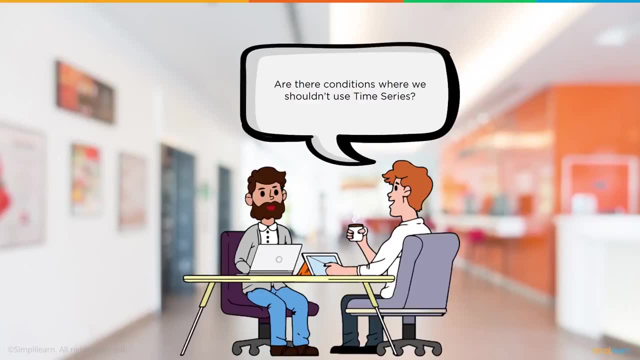 so that is the irregularity component. so these are the various components of time series data. yes, there are conditions where we cannot use time series analysis. right, so is it. can we do time series analysis with any kind of data? no, not really. so what are the situations where we are? 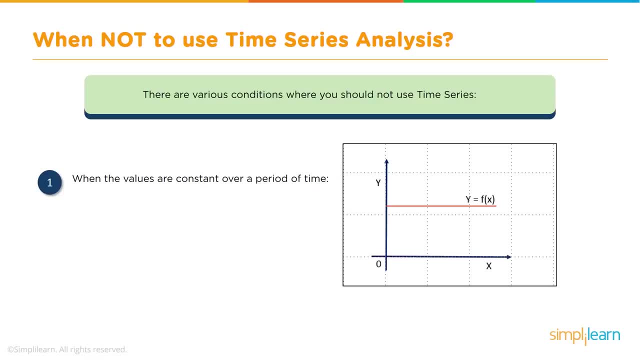 talking about time series analysis, right? so what are the situations where we are talking about? we cannot do time series analysis. so there will be some data which is collected over a period of time, but it's really not changing, so it will not really not make sense to perform any time series. 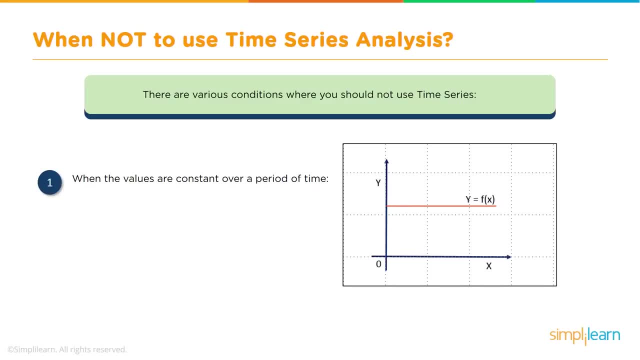 analysis over it, right? for example, like this one: so if we take x as the time and y as the value of whatever the output we are talking about, and if the y value is constant, there is really no analysis that you can do. leave alone time series analysis. right, so that? 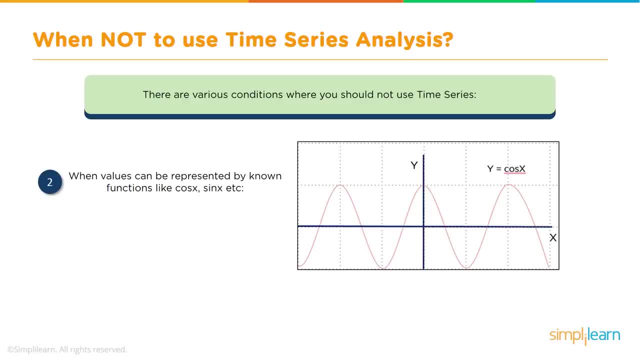 is the reason why we are talking about time series analysis. right, so that is the reason why we are talking about time series analysis. right, so that is the reason why we are talking about time series. another possibility is: yes, there is a change, but it is changing as per a very fixed function, like a. 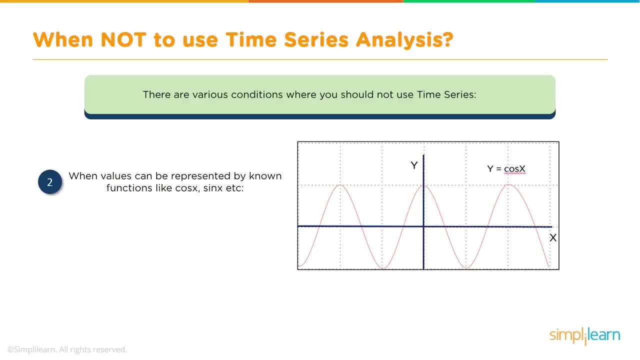 sine wave or a cos wave. again, time series analysis will not make sense in this kind of a situation because there is a definite pattern here, there is a definite function that the data is following. so it will not make sense to do a time series analysis now, before performing any time series. 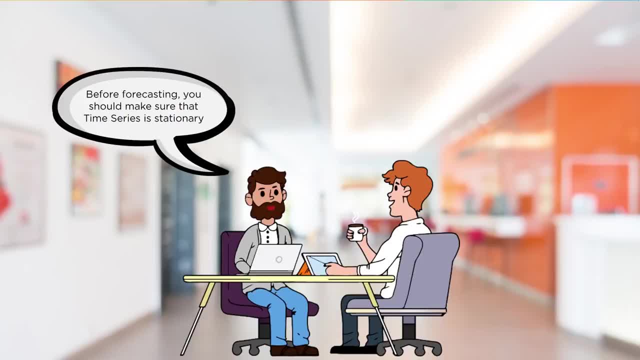 analysis. uh, the data has to be stationary and typically time series data is not stationary, so in which case you need to make the data stationary before we apply any models like arima model or any of these, right? so what exactly is stationary data and what is meant by stationary? 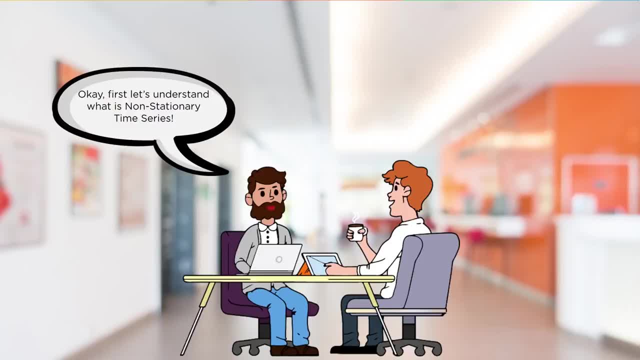 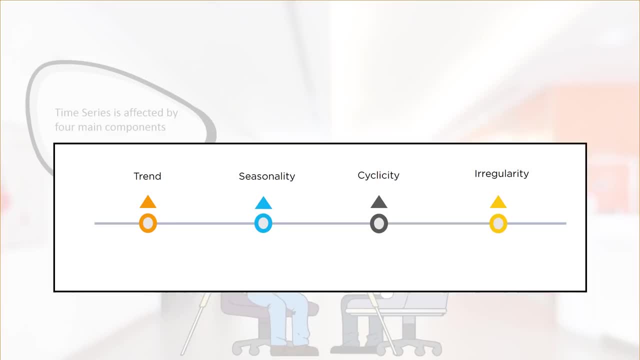 data. let us take a look. first of all, what is non-stationary data? time series data. if you recall from one of my earlier slides, we said that time series data has the following four components: the trend, seasonality, cyclicity and random. random component or irregularity. right so? 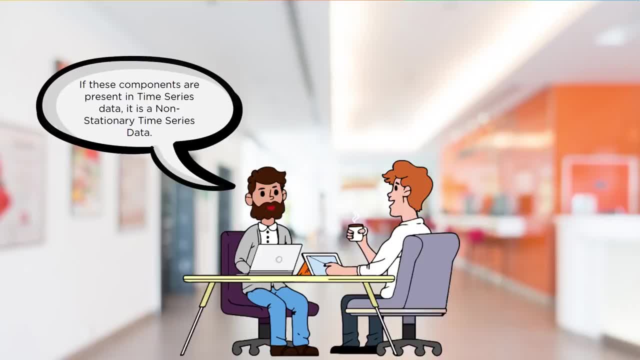 if these components are present in time series data, it is non-stationary, which means that typically, these components will be present. therefore, most of the time a time series data that is collected raw data is non-stationary data, so it has to be changed to stationary data. 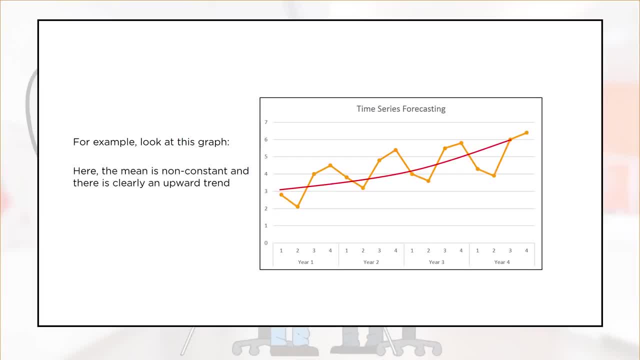 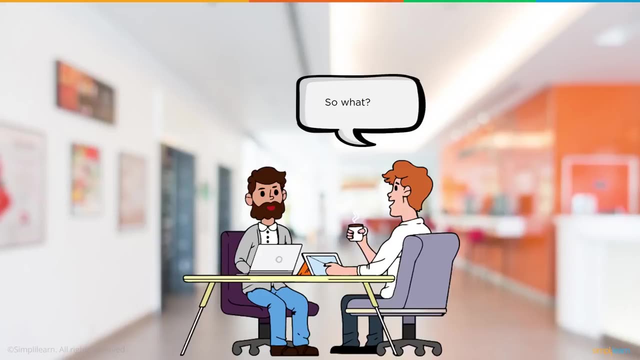 before we apply any of these algorithms. all right, so a non-stationary time series data would look like this, which means like, for example, here there is an upward trend, the seasonality component is there and also the random component, and so on. so if the data is not stationary, then the time series 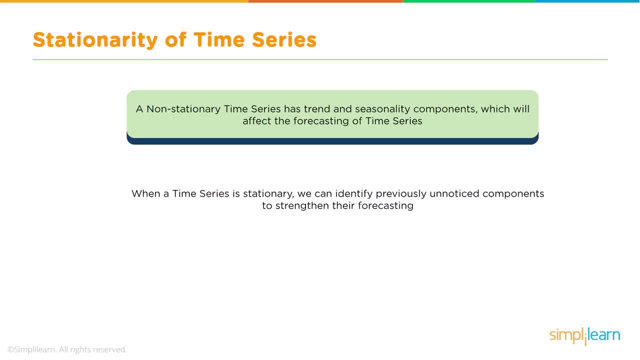 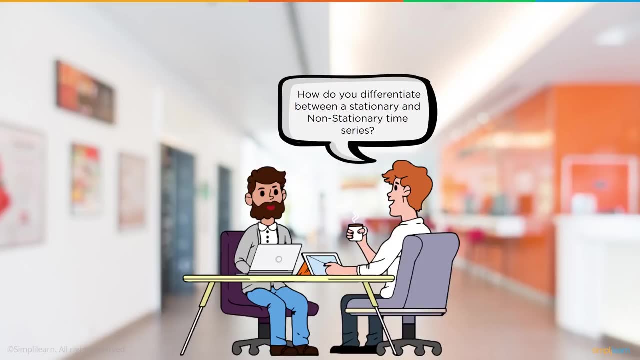 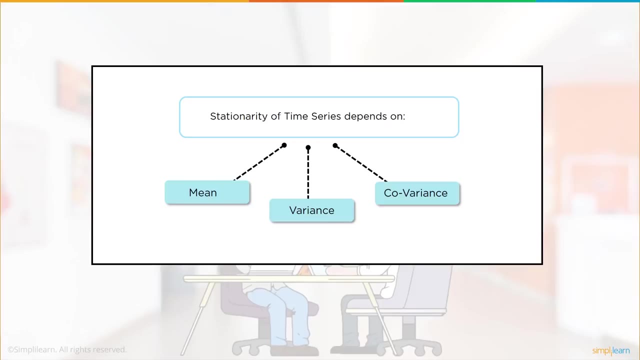 forecasting will be affected, so you cannot really perform a time series forecasting on a non-stationary data. so how do we differentiate between a stationary and a non-stationary time series data? typically, or technically, one is, of course you can do it visually. in non-stationary data, the the data will be more flattish. seasonality will of course, be there, but 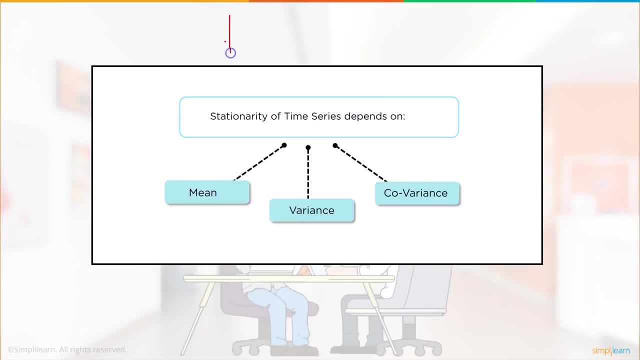 the trend will not be there, so the data may. if we plot that, it may appear somewhat like this right. it's a horizontal line. along the horizontal line, you will see, compared to the original data which was there was an upward trend, so it was changing somewhat like this right. so this is. 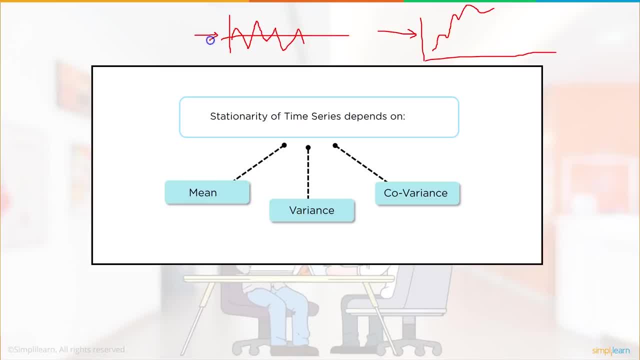 non-stationary data, and this is how a stationary data would look visually. what does this mean? technically, this means that the stationarity of the data depends on a few things but the mean, the variance and the covariance. so these are the three components on which the stationarity of the 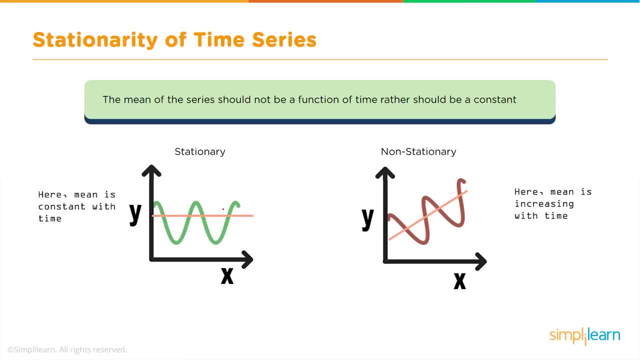 data depends, so let's take a look at what each of these are. for stationary data, the mean should not be a function of time, which means that the mean should pretty much remain constant over a period of time. right, so there is. there shouldn't be any change. so this is how the stationary data would. 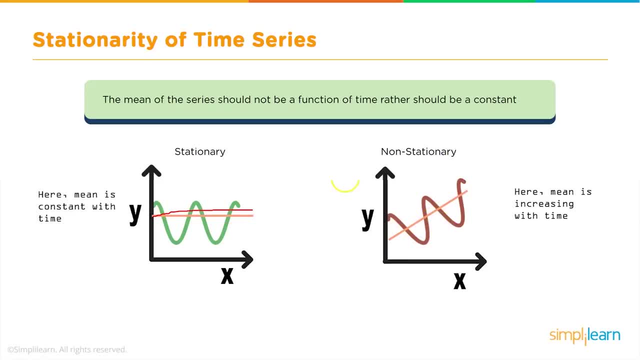 look. and this is how a non-stationary data would look. i've shown in the previous slide as well. so here the mean is increasing. that means there is an upward trend. okay, so that is one part of it. and then the variance of the series should not be also a function of time, so the variance also. 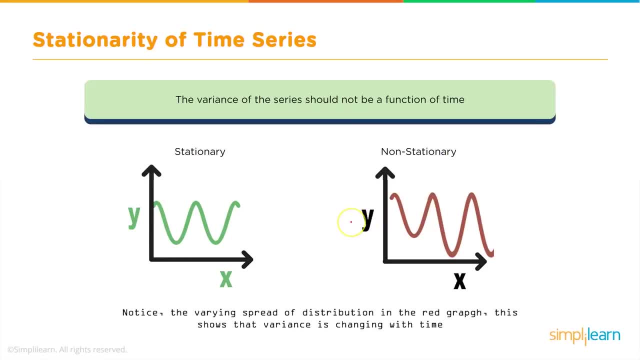 should be pretty much common or should be constant, rather so. this is a if we visually, we take a look, this is how time series stationaries, data would look where the variance is not changing. here the variance is changing. therefore, this is non-stationary and we cannot apply time series. 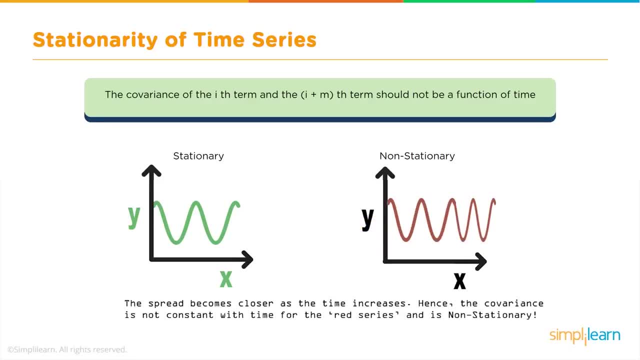 forecasting on this kind of data. similarly, the covariance which is basically of the ith term and the i plus mth term should not be a function of time as well. so covariance is nothing, but not only the variance at the ith term but the relation between the variance at the ith term. 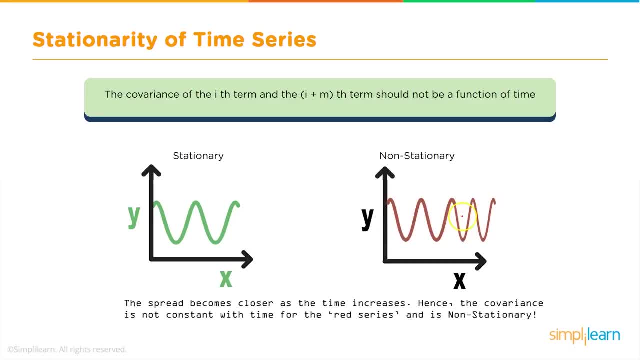 and the i plus mth or the i plus nth term. so as again, once again visually, this is how it would look if the covariance is also changing with respect to time. so these are the three. all three components should be pretty much constant, and that is when you have stationary data. 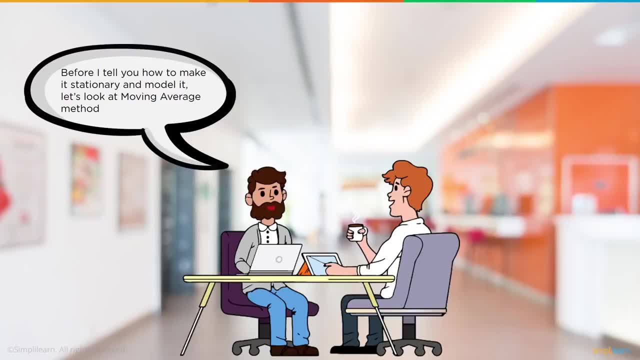 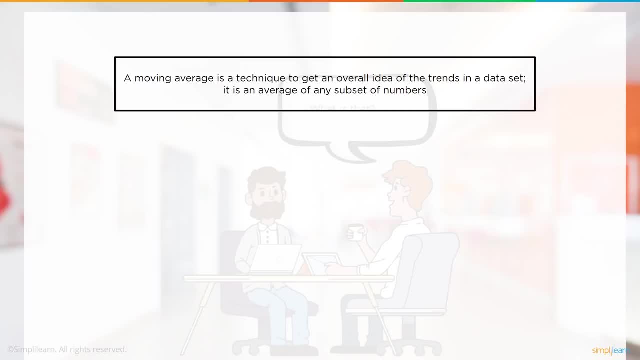 and in order to perform time series analysis, the data should be stationary. okay, so let's take a look at the concept of moving average, or the method of moving average, and let's see how it works. we'll do simple calculations. so let's say: this is our sample data. we have the data for three. 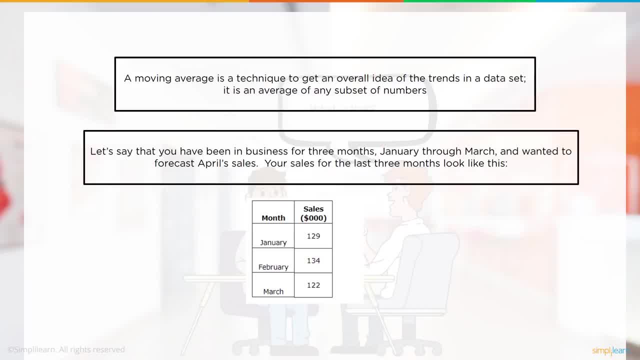 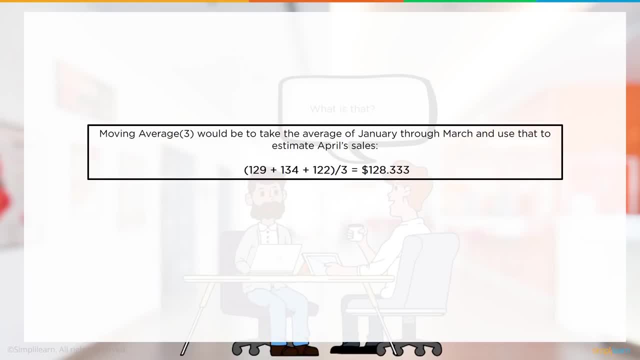 two different values continuously. so 10 to 11 days. we know what the average is is two days. in many cases it is one day. so on the matched bad and so on. so each time we find the average. okay, now here, it is as simple as that. so each time we find it, we ask 3. this is the average. 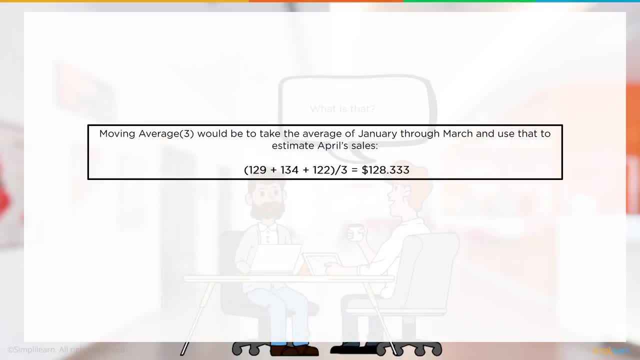 of what we just found, or we break the average by taking the average. so, for instance, let'sít generate the matter of two significant values, but we drop the numbers down, the range of three, six, eight, and then put them together. letís try the контр Est utilizing 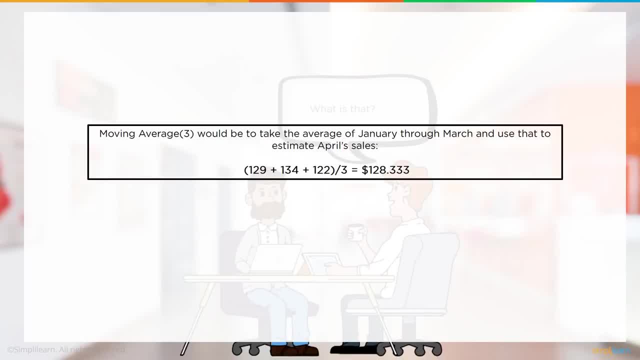 project order for theología versus. place visually for first, the average of the average. so with respect to that, it should not be that we will say that the average is equal to v averages. if you now have a series of data, you keep taking the three values, the next three values and 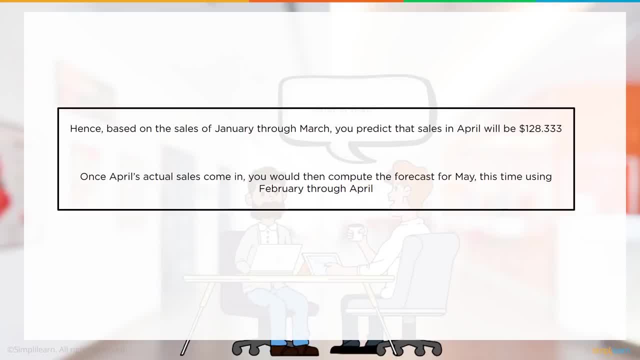 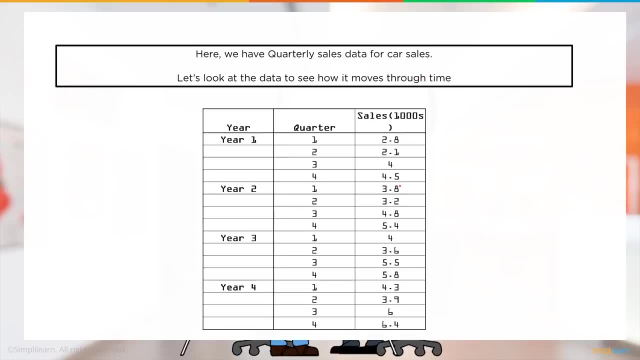 then you take the average of that and then the next three values, and so on and so forth. so that is how you take the moving average. so let's take a little more detailed example of car sales. so this is how we have the car sales data for the entire year. let's say so rather for four years. 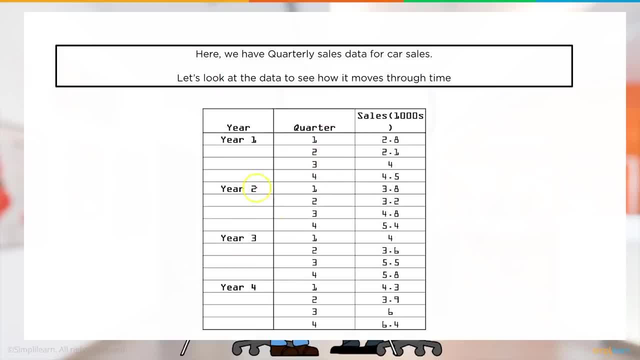 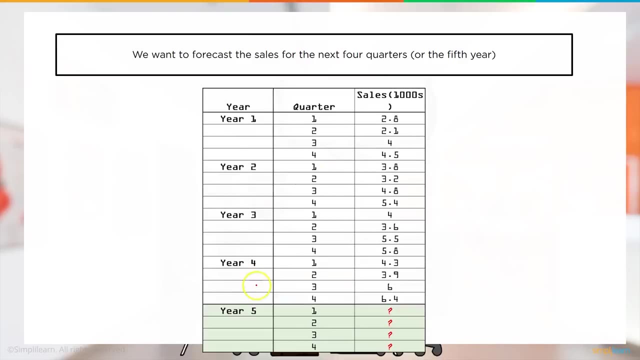 so year one: we have for each quarter, quarter one, two, three, four, and then year two, quarter one, two, three, four, and so on and so forth. so this is how we have sales data of a particular car, let's say, or a showroom, and we want to forecast for year five. so we have the data for four years. we now 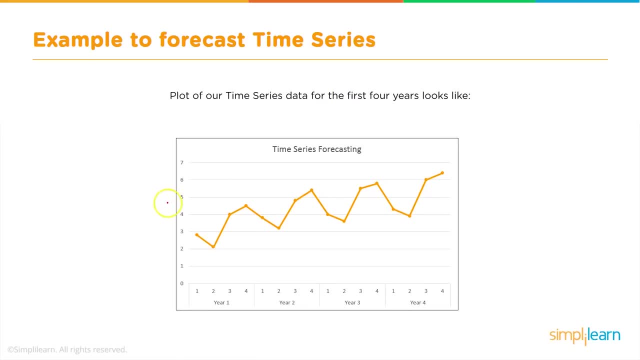 want to forecast for the fifth year. let's see how it works. first of all, if we plot the data as it is taken, the raw data, this is how it would look and what do you think it is. is it stationary? no, right, because there is a trend, upward trend- so this is not a stationary data. so we 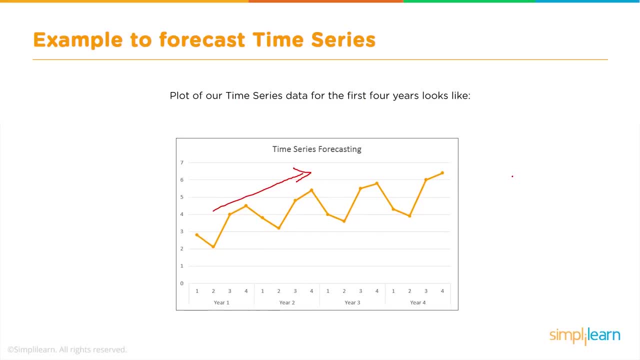 we need to. later we will see how to make it stationary, but to start with, just an example, we will not worry about it for now. we will just go ahead and manually do the forecasting using what is known as moving average method. okay, so we are not applying any algorithm or anything. 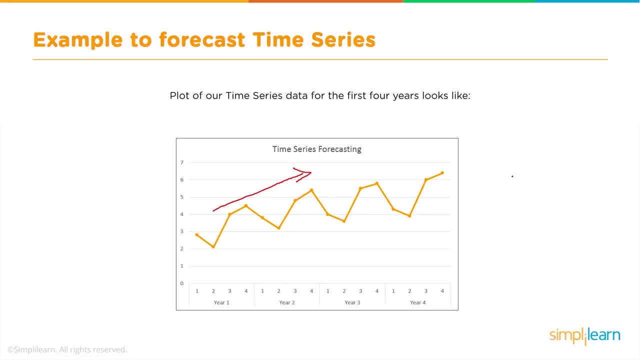 like that. in the next video, we will see how to apply an algorithm, how to make it stationary, and so on. alright, so here we see that all the three or four components that we talked about are there. There is a trend, there is a seasonality and then, of course, there is some random component. 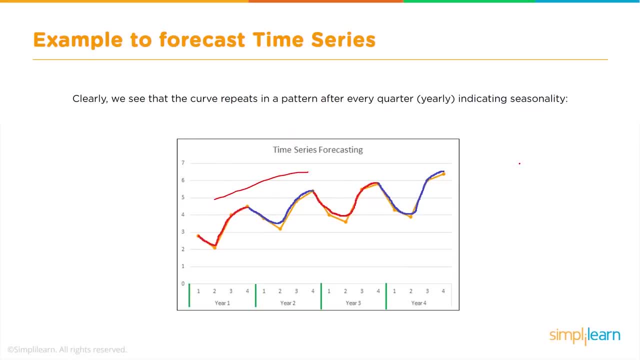 as well. Cyclicity may not be. it is possible that cyclicity is not applicable in all the situations. For sales especially, there may not be unless you are taking sales for maybe 20-30 years. cyclicity may not come into play. 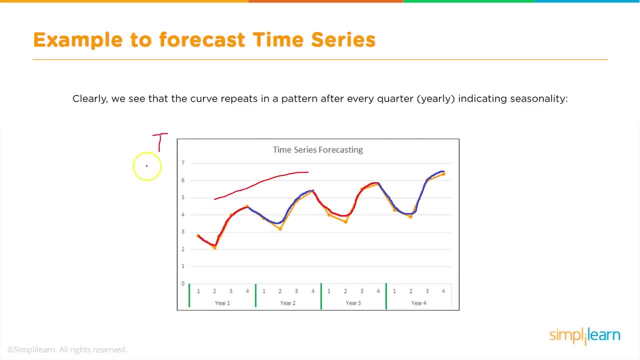 So we will just consider primarily the trend, seasonality and irregularity right. So random, it is also known as random irregularity right, So we were calling the random or irregularity component. So these are the three main components typically in this case we will talk about 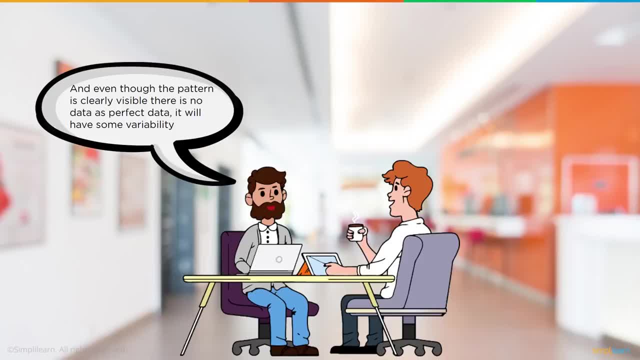 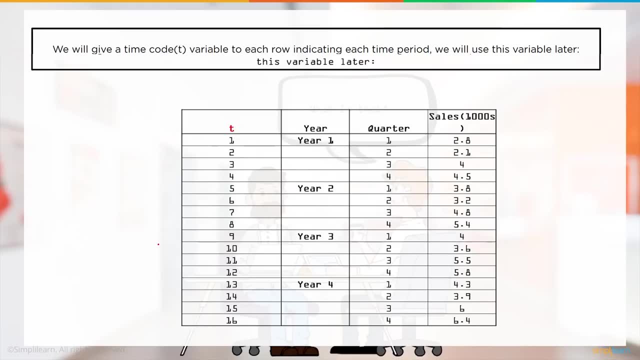 So this is the trend component and we will see how to do these calculations. So let's take a look. redraw the table including the time code. we will add another column, which is the time code, and this is the column, and we just number it like 1,, 2,, 3,, 4, up. 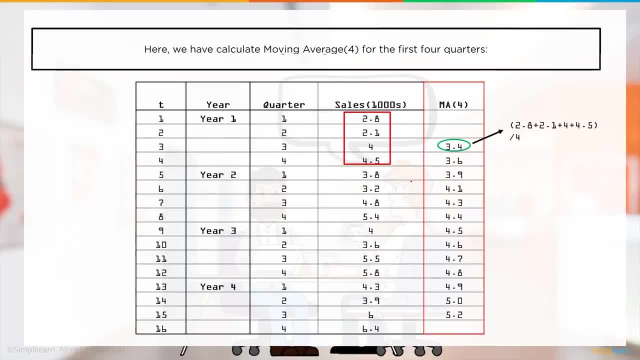 to 16.. The rest of the data remains the same. okay, So we will do the calculations now. Now let us do the moving average calculations, or MA4 as we call it, for each year. So we take all the four quarters and we take an average of that. 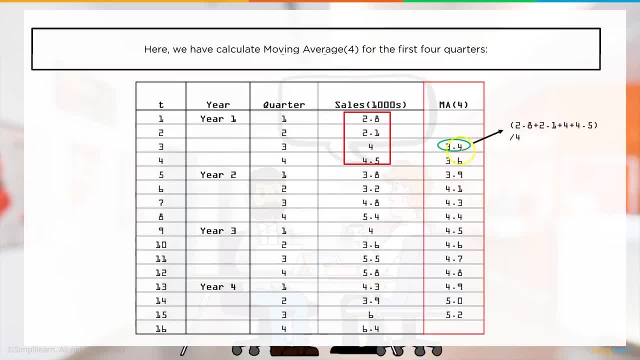 So if we add up these four values and divide by 4, you get the moving average of 3.4. So we start by putting the value here. So that will be for the third quarter. let's say 1,, 2,, 3,, 4.. 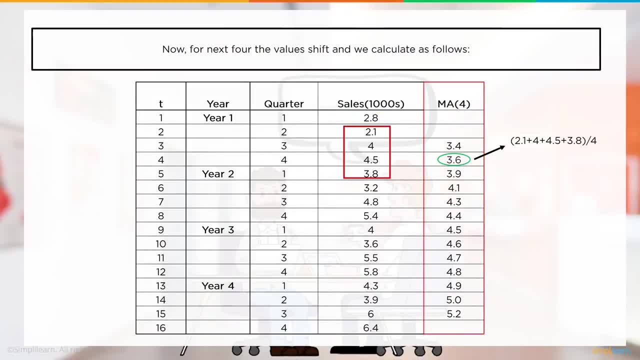 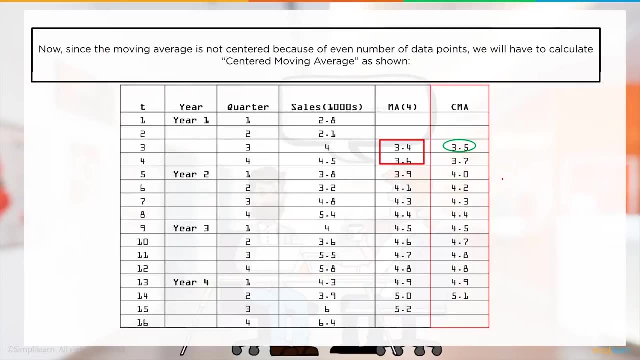 The third quarter, Then we will go on to the next one. So we take the next four values, as you see here, and take the average of that, which is the moving average for the next quarter, and so on and so forth. Now, if we just do the moving average, it is not centered. 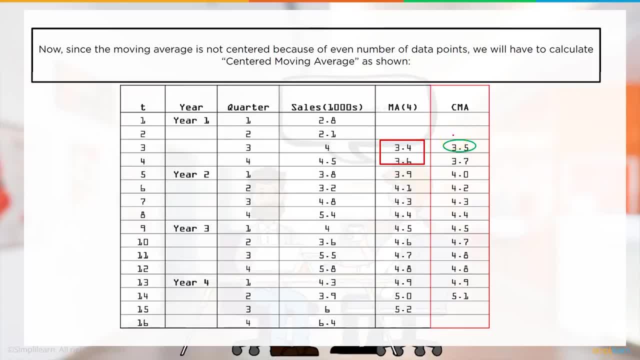 So what we do is we basically add one more column and we calculate the centered moving average as shown here. So here what we do is we take the average of two values And then just adding these values here. So, for example, the first value for the third quarter is actually the average of the third. 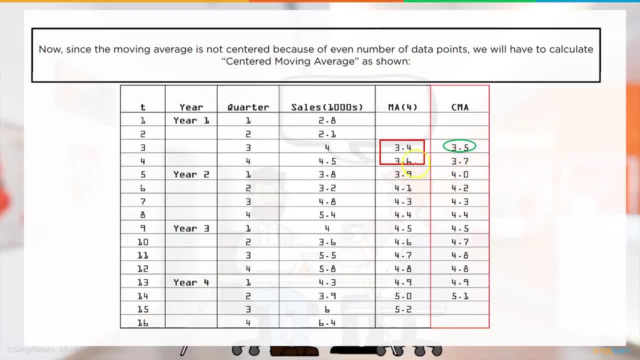 and the fourth quarter. So we have 3.5.. Now it gets centered. So, similarly, the next value would be 3.6 plus 3.9, divided by 2, which is 3.7, and so on and so forth. 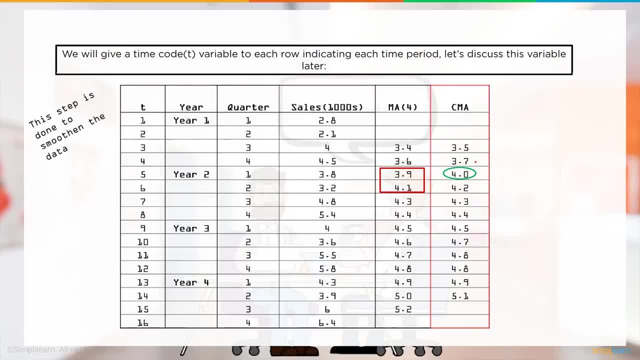 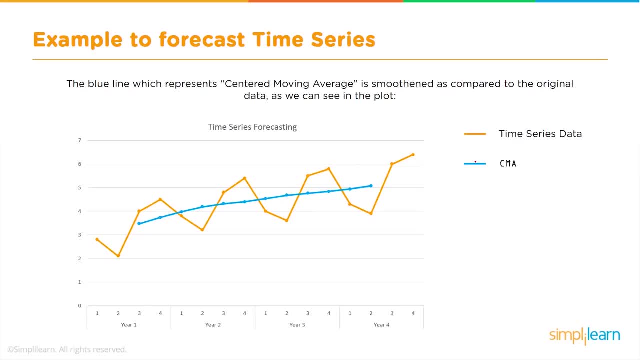 So that is the centered moving average. This is done primarily to smoothen the data so that there are not too many rough edges. So that is what we do here. So if we visualize this data now, this is how it looks right. 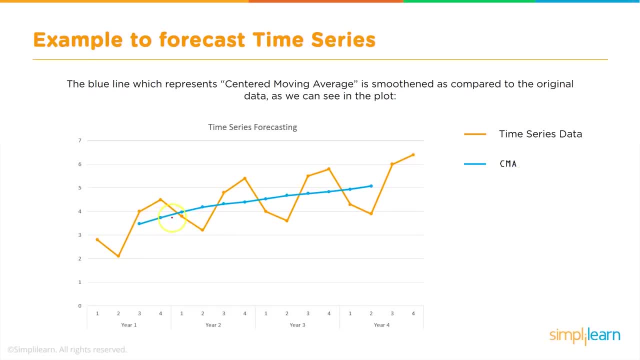 So if we take the centered moving average, as you can see, there is a gradual increase. If this was not the case, if we had not centered it, the changes would have been much sharper. So that is basically the smoothening that we are talking about. 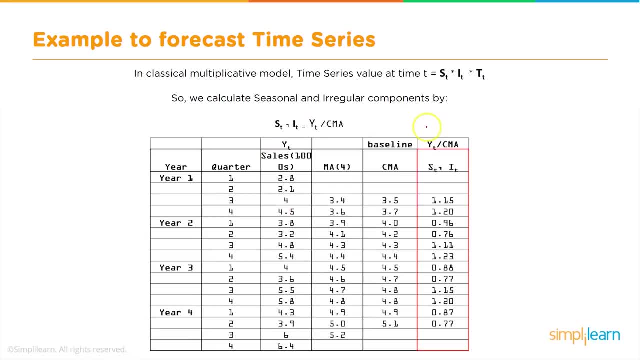 Now let's go and do the forecast for the fifth year. So, in order to do the forecast, what we will do is we will take the centered moving average and we will take the average for the fifth year. We will take the average as our baseline and then start doing a few more calculations. 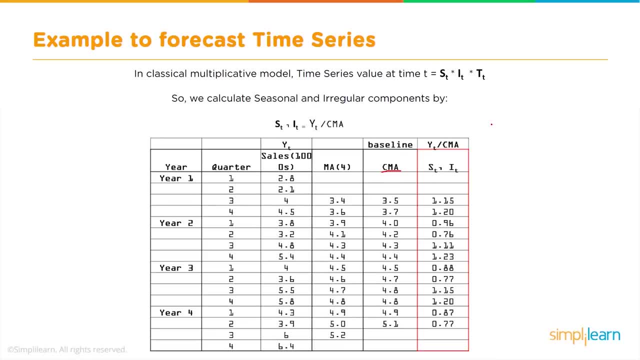 that are required in order to come up with the prediction. So what we are going to do is we are going to use this multiplicity or multiplicative model in this case, and this is how it looks. So we take the product of seasonality and the trend and the irregularity components. 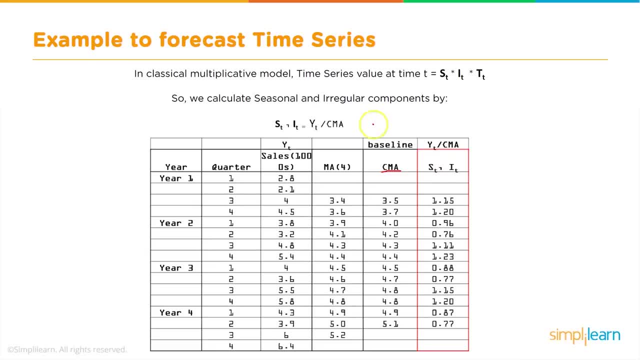 and we just multiply that And in order to get that, this product of these two, We have basically the actual value divided by CMA. YT value divided by CMA will give you the predicted value of YT is equal to the product of all three components. 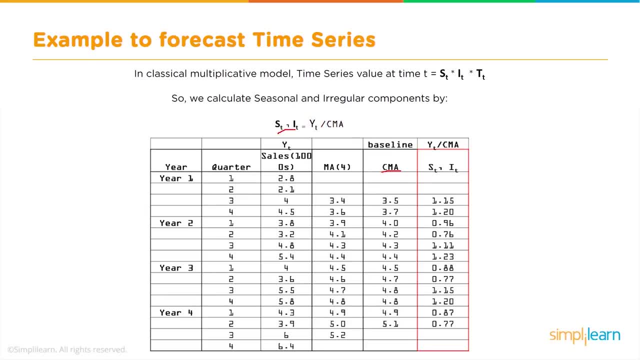 Therefore, ST into IT is equal to YT by CMA. So this is like: this is equal to YT, right? So therefore, if we want ST into IT, the product of seasonality and the regularity is equal to YT by CMA. 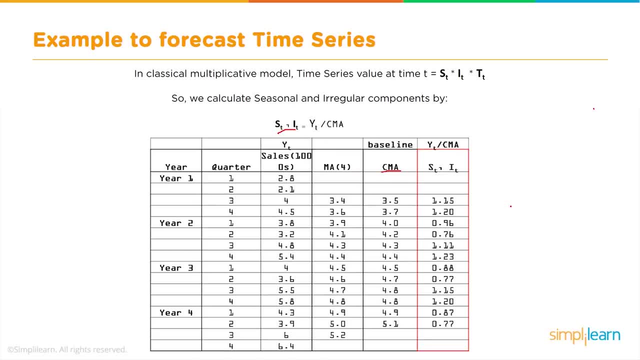 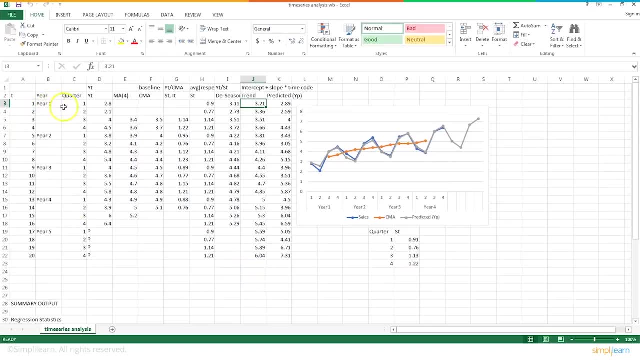 So that is how we will work it out. I also have an Excel sheet of the actual data, So let me just pull that up. All right, So this is how the data looks in Excel, As you can see here: year one: quarter one, two, three, four. year two- quarter one: two. 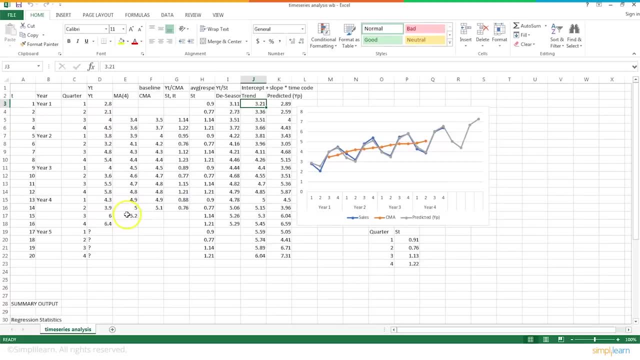 three, four and so on, And this is the sales data. And then this is the moving average. As I mentioned, this is how we calculate and this is the centered moving average. So this is the primary component that we will start working with. 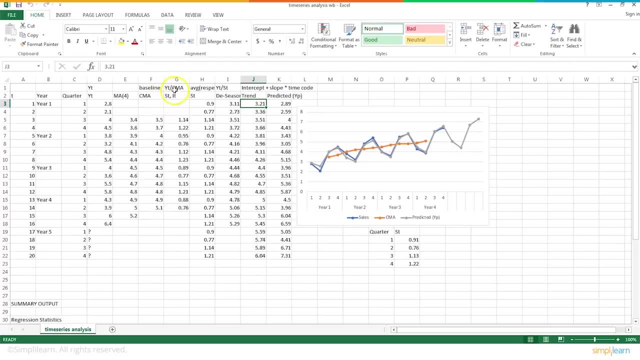 And then we will calculate. since we want the product of ST into YT, that is equal to YT by CMA. So these values are nothing but the YT value divided by CMA. So in this case it is four by 3.5, which is 1.14,. similarly, 4.5 by 3.7, 1.22, and so 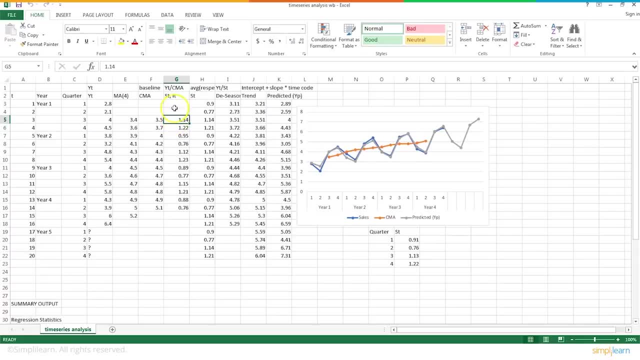 on and so forth. So we take we have the product ST into IT And then the next step is to calculate the average of respective quarters. So that is what we are doing here: average of respective quarters, And then we need to calculate the average of respective quarters. 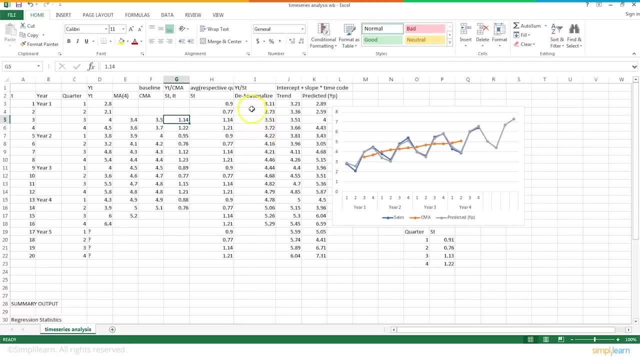 And then we need to calculate the average of respective quarters. Now here we have the non-branded products related to cortar делage, to Mandata, And then, of course, these are measuring the ROI, The cost, and the COD is also the cost, but this is theяжuality of the product meaning. 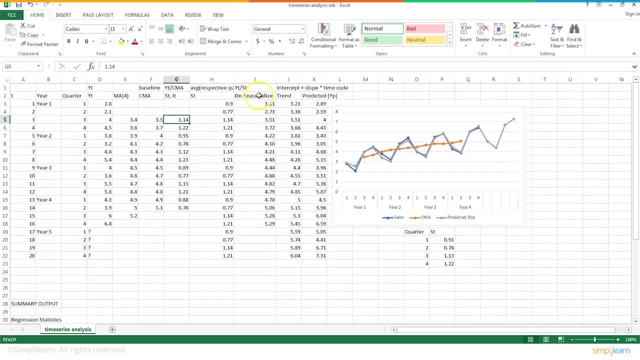 not the released profit. The cost is not the net profit, responsiveness, but the vezuality of the product and the value of the outcome. So now we are going into the next step, The very next step, which is the biggest: the business order, which is our gross profit. 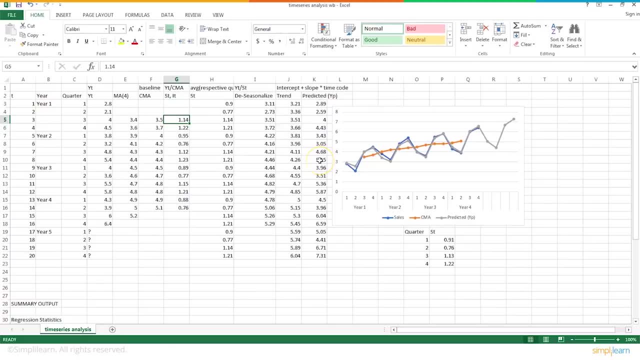 Lets see it know the value. but now that we have our model, we predict ourselves and see how close it is. so we predict it as 2.89, whereas the actual value is 2.8. then we have 2.59, the actual value is 2.1, and so 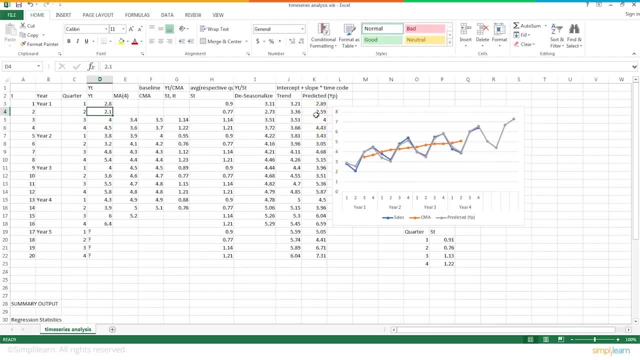 on just to see how our model works and then continue that into the fifth year- because in for fifth year we don't have a reference value- okay, and if we plot this, we will come to know how well our calculations are, how well our manual model- in this case we did not really use a model- 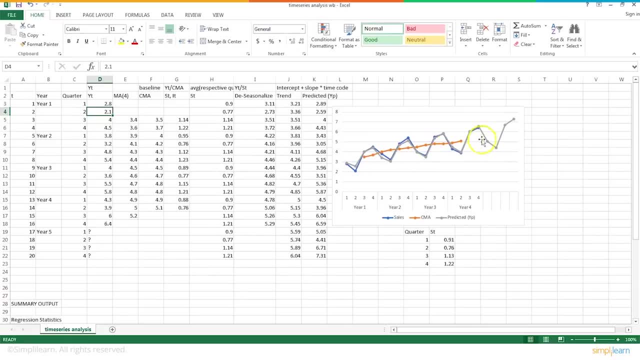 but we did on our own manually, so it will tell us the trend. so, for example, the predicted value is this gray color here and you can see that it is actually pretty much following the actual value, which is the blue color right and the gray color is the predicted value. so the wherever we know. 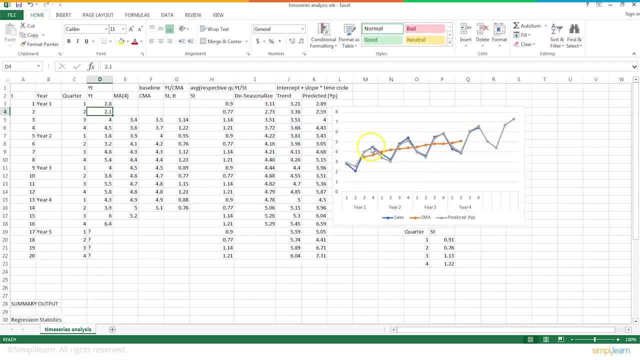 the values up to year four, we can see that our predicted values are following, or pretty much very close to, the actual value. so we can see that our predicted values are following, or pretty much, the actual values and then from here onwards, when the year five starts, the blue color line is not. 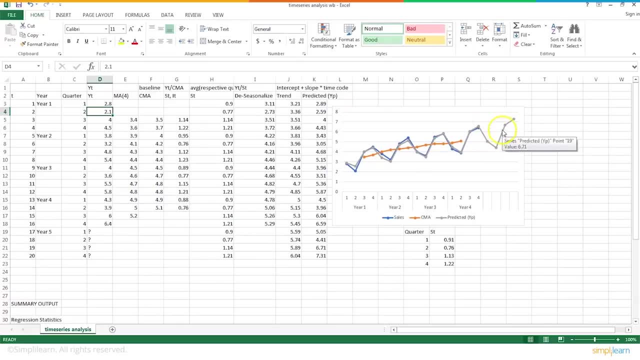 there because we don't have the actual values, only the predicted value. so we can see that, since it was following the trend pretty much for the last four years, we can safely assume that it has understood the pattern and it is predicting correctly for the next one year, the next four. 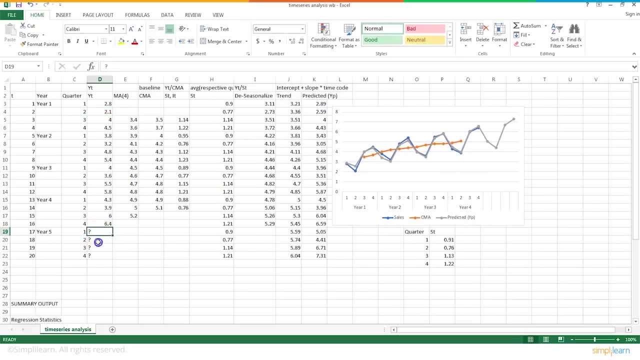 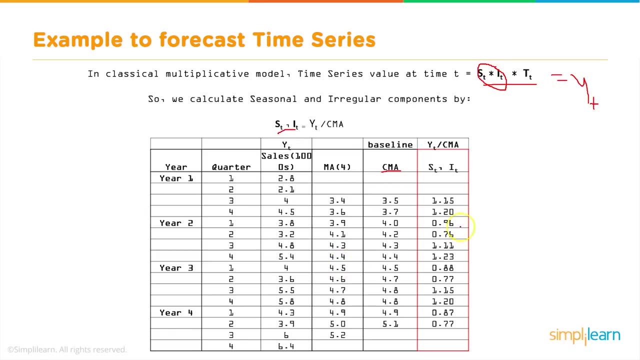 quarters, right, so that is what we are doing here. so these four quarters we did not have actual data, but we have the predicted values. so let's go back and see how this is working in this using the slides. so this is. we already saw this part and i think it was. 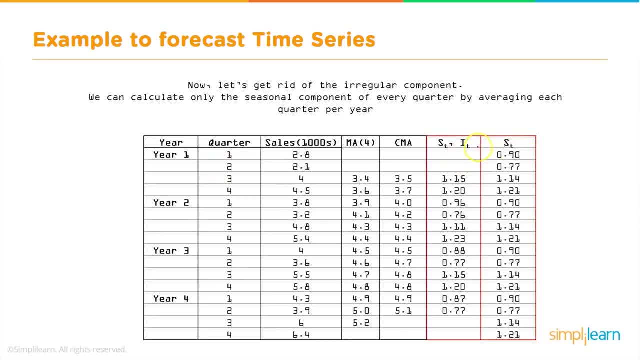 easier to see in the excel sheet. so we calculated the st, it, the product of st, and it using the formula like here: y by yt, by cma. we got that and then we got st, which is basically yt. so this is the average of the first quarters for all the four years and similarly this is the average of the. 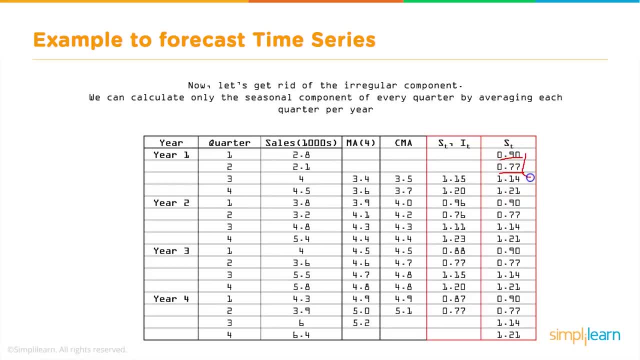 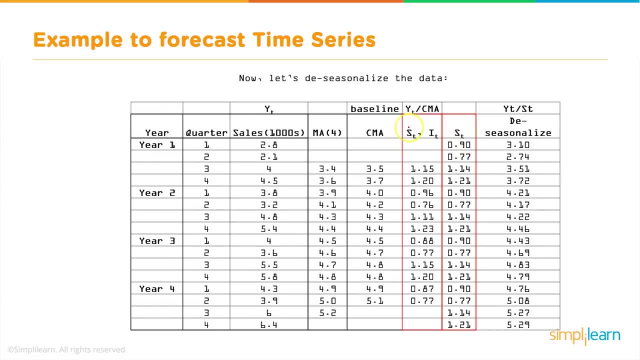 second quarter for all the four years and so on. so these values are repeating, these are. they are calculated only once. they get repeated, as you can see here. and then we get the de-seasonalized data and that is basically yt by st. so we calculated st here and we have yt. so yt by st will give you. 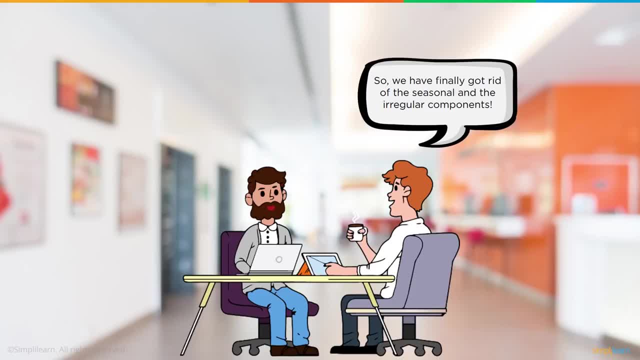 the de-seasonalized data and we have got rid of the seasonal and the irregular components so far. now what we are left with is the trend, and before we start the time series forecasting or time series analysis, as i mentioned earlier, we need to completely get rid of the non-stationary components. so 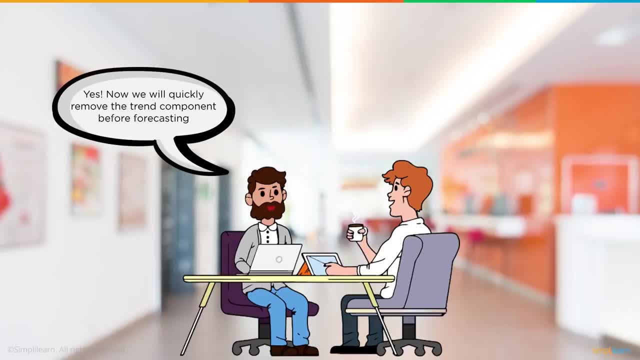 we are still left with the trend component. so now let us also remove the trend component. in order to do that, we have to find the, or we have to calculate the intercept and slope of the data, because that is required to calculate the trend. and how are we going to do that? 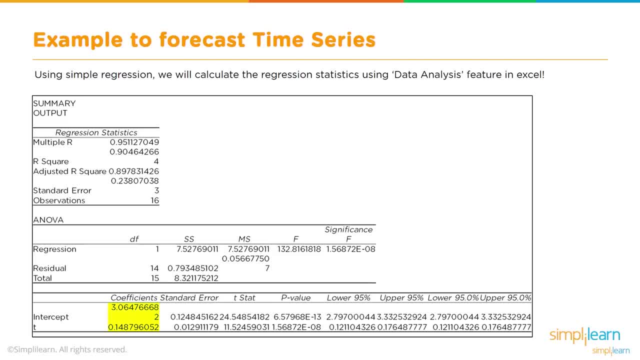 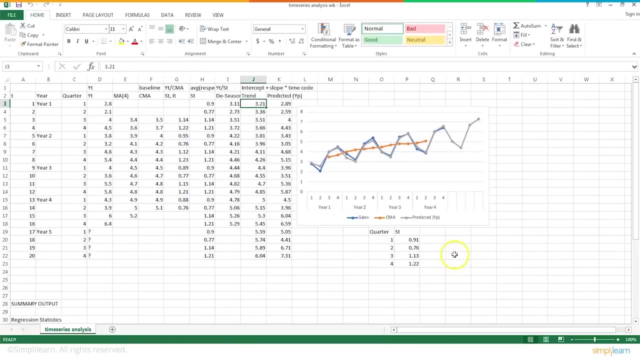 we will actually use what is known as a regression tool or analytics tool. that is available in excel. so you remember, we have our data in excel. so let me take you to the excel, and here we need to calculate the intercept and the slope. in order to do that, we have 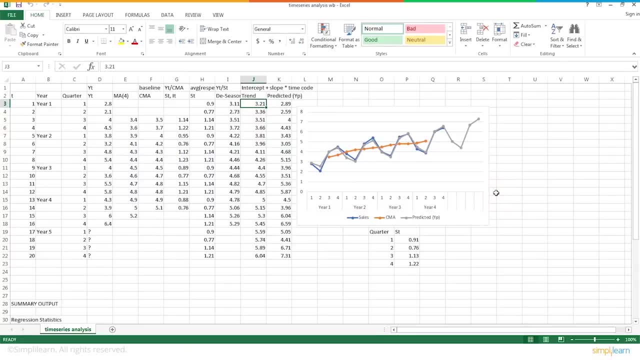 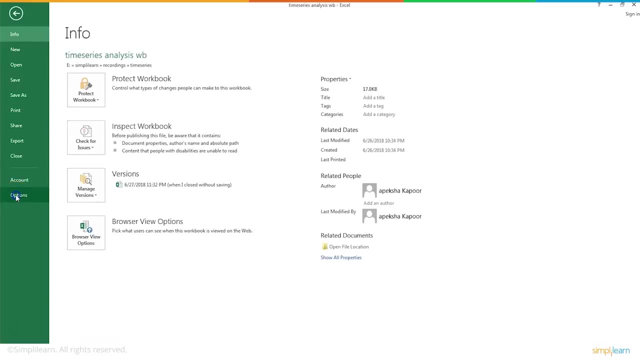 to use the regression mechanism, and in order to use the regression mechanism, we have to use the analytics tool that comes with excel. so how do you activate this tool? so this is how you would need to activate the tool from excel: you need to go to options and in options there will be add-ins. 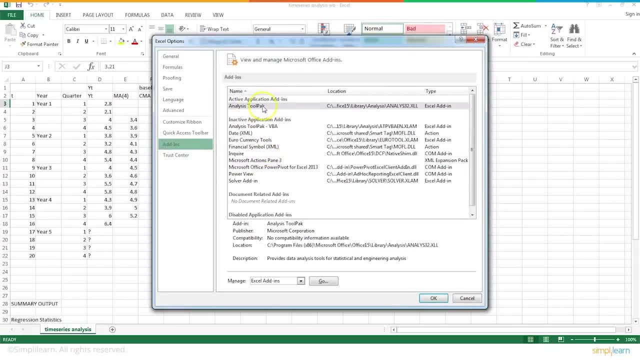 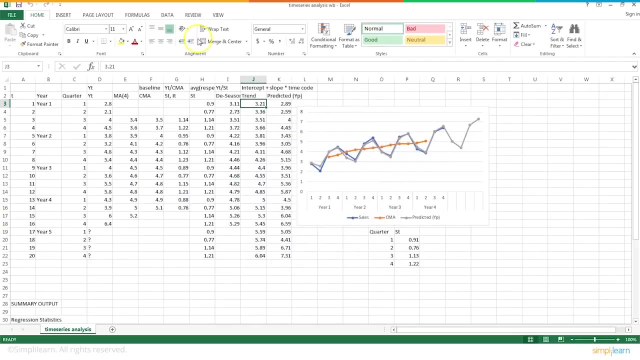 and in add-ins you will have analysis tool back and you select this and you just say go. it will open up a box like this. you say analysis tool pack and you say okay. and now when you come back in to the regular view of excel, in the data tab you will see data analysis activated. so you need to go to. 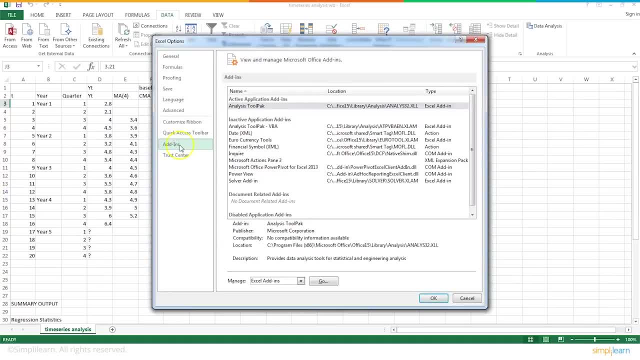 file options and add-ins, then analysis tool pack. typically, since i've already added it, it is coming at the top, but it would come under inactive application add-ins. so when you're doing it for the first time, so don't use vba, you just say analysis tool pack. there are two options: one with vba, like this one, and 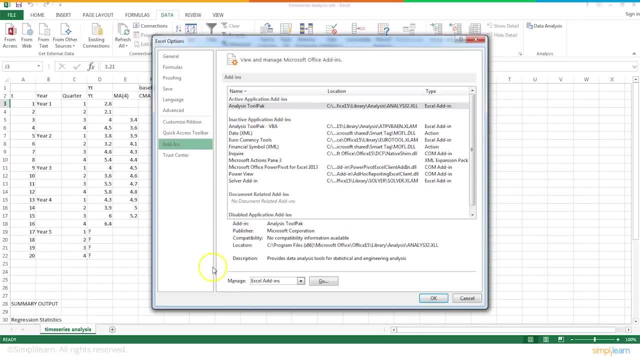 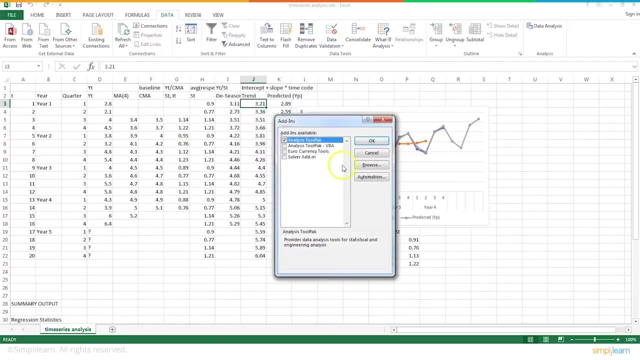 one without vba, so just use the one without vba. and then, instead of just saying: okay, just take care that you click on this go, and not just okay. so you say go, then it will give you these options. only then you select just the analysis tool pack and then you say: okay, all right, so, and then when? 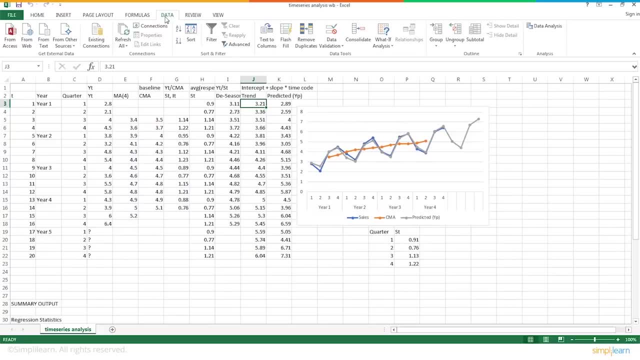 you come back to the main view, you click on data. okay, so this is your normal home view perhaps. so you need to come to data and here is where you will see data analysis available to you and then, if you click on that, there are a bunch of possibilities. what kind of data analysis you? 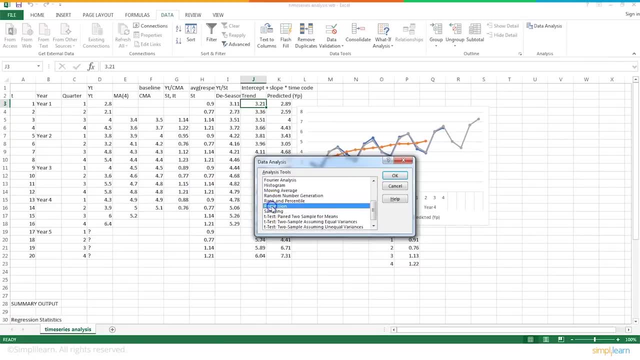 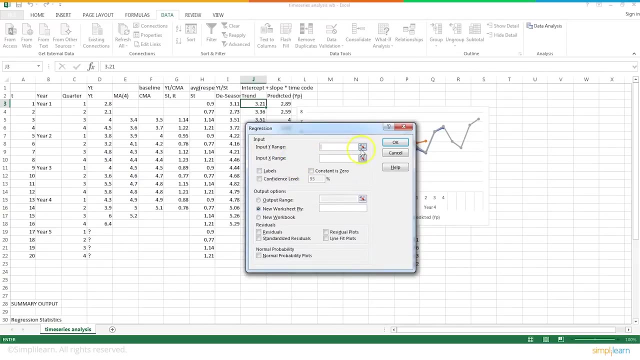 want to do. if there are options are given, write down what kind of data analysis you want to do. now we just want to do regression because we want to find the slope and the intercept. so select regression and you say ok and you will get these options for input y range and input x range. input: 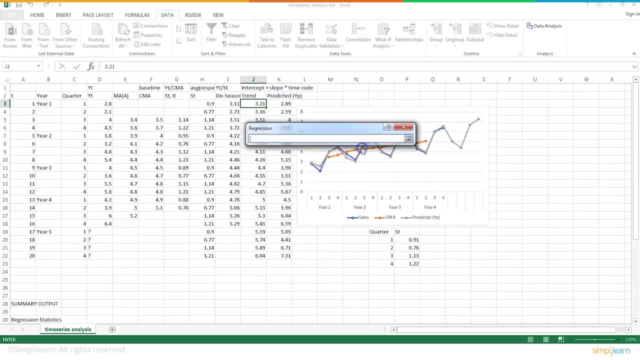 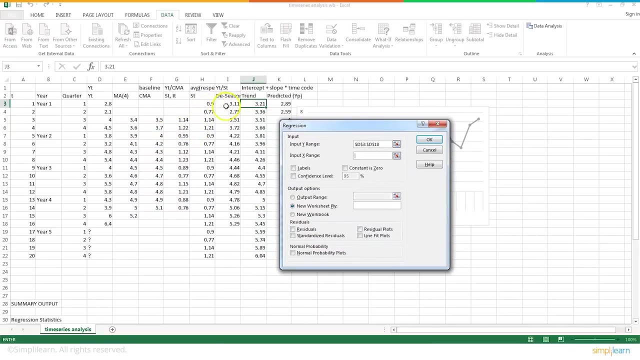 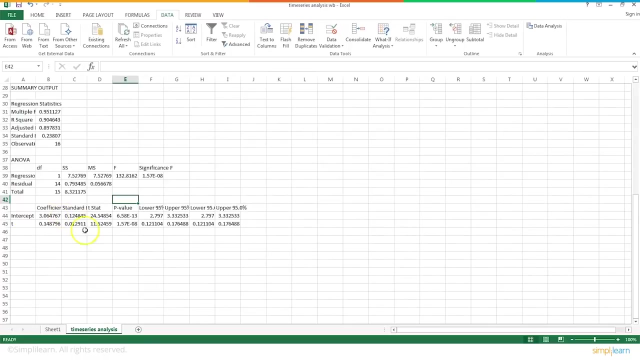 y range is the value yt, so you just select this and you can select up to here and press enter and input x range. you can. but now you start with uh, the baseline, or you can also start with the d season values, so you can just click on these and say: okay, i have already calculated it. so these 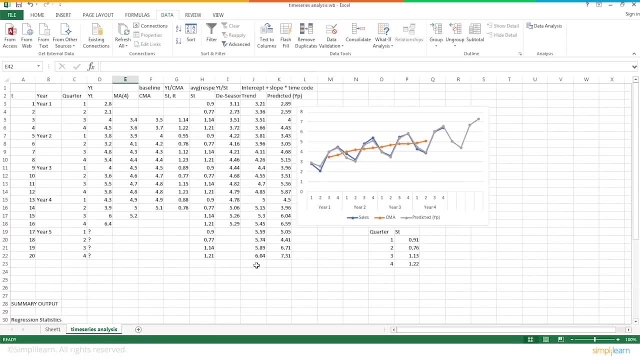 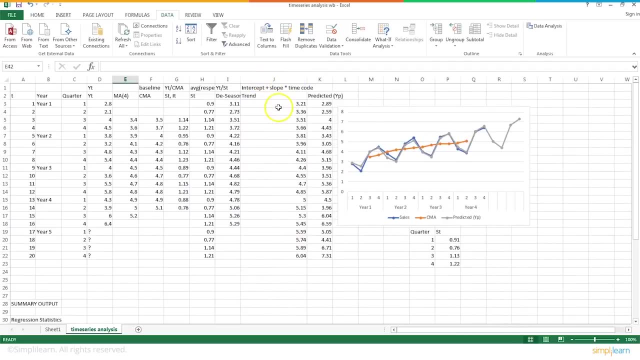 are the intercept and the coefficients that we are getting for these values, and we will actually use that to calculate our trend here, right so? which is in the j column. so our trend is equal to intercept plus slope into the timecode. so the intercept is out here, as we can see in our slide as well. so 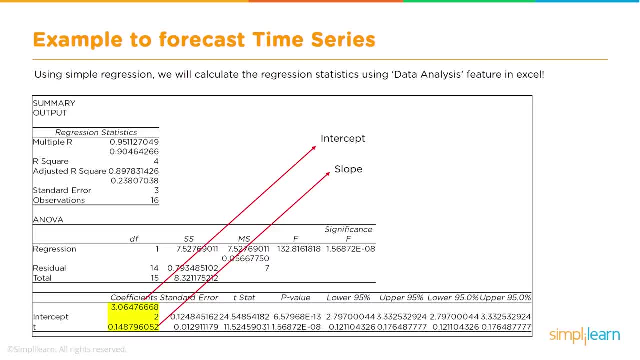 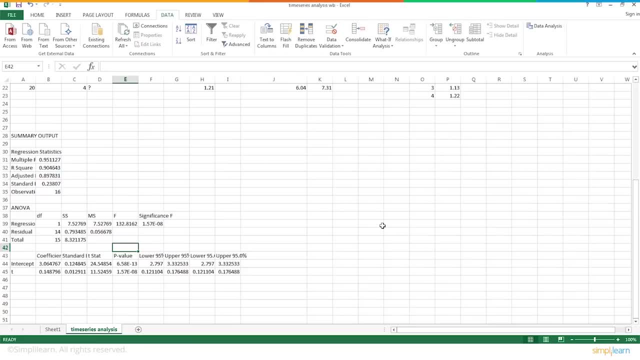 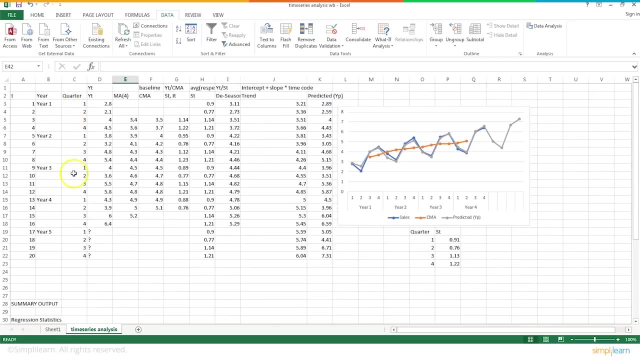 if you see here, this is our intercept and the lower value is the slope. so we have calculated here and it's shown in the slides as well. so intercept, so the formula is shown here. so our trend is equal to intercept plus slope into timecode. timecode is nothing but this one. t. 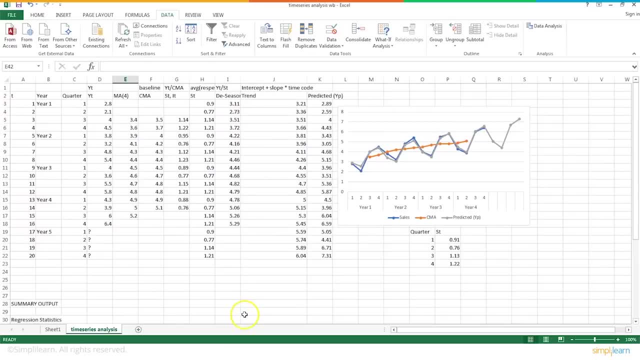 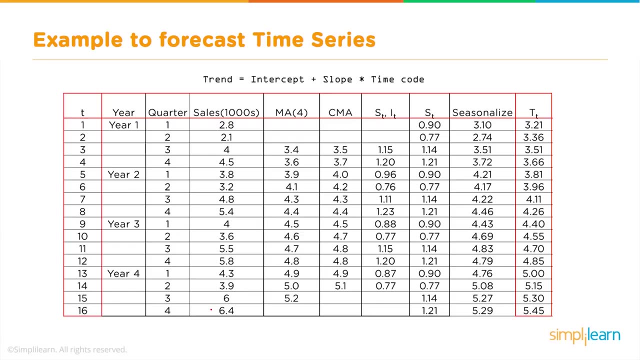 column a: one, two, three, four. okay, so that's how you calculate the trend and that's how you use the data analysis tool from excel. using these two, we calculate the predicted values and using this formula, which is basically, trend is equal to intercept plus slope into timecode, and then we 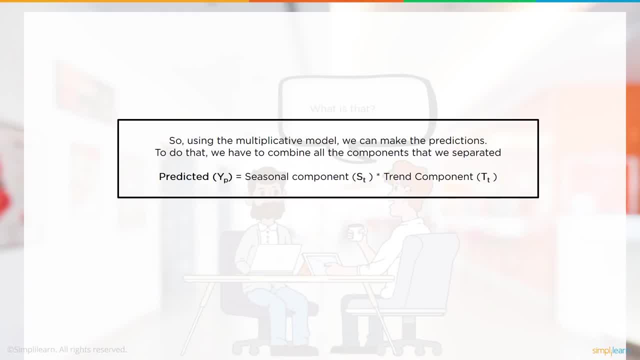 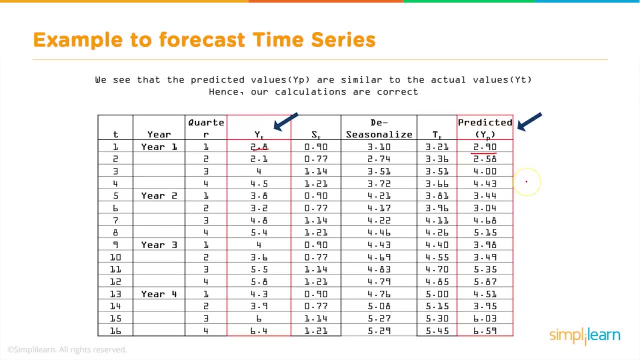 can go and plot it, see how it is looking and therefore. so we see here that the predicted values are pretty close to the actual values and and therefore we can safely assume that our calculations, which are like our manual model, is working, and hence we go ahead and predict for the fifth year, so till four years. we know the. 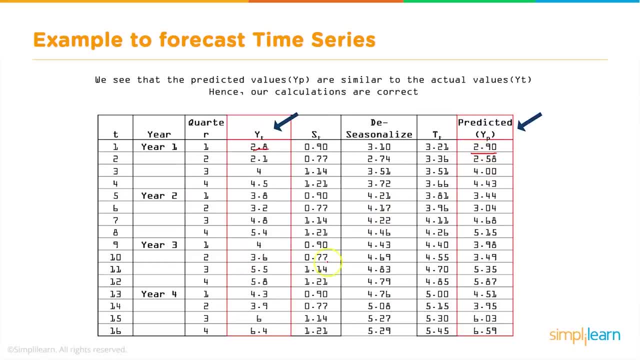 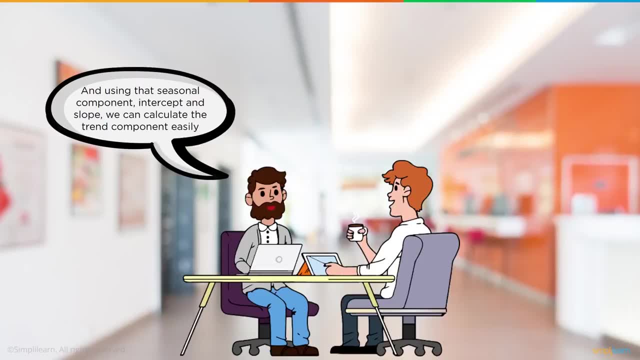 actual value as well, so we can compare how our model is performing. and for the fifth year we don't have reference values. so we can use our equations to calculate the values or predict the values for the fifth year and we can go ahead and safely calculate those values and when we 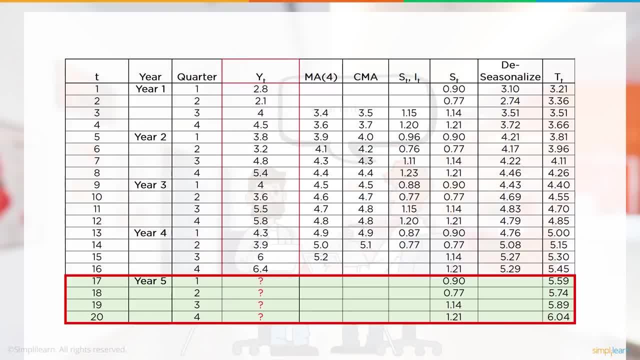 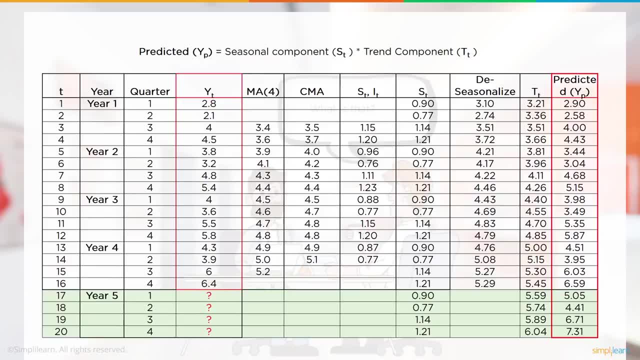 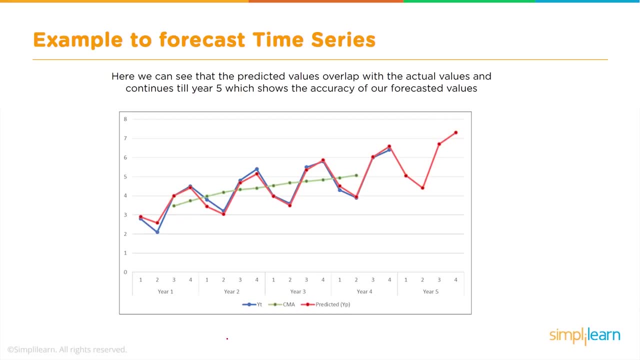 plot, for the fifth year as well, the predicted values. we see that they are pretty much. they captured the pattern and we can safely assume that the predictions are fairly accurate, as we can also see from the graph in the excel sheet that we have already seen. okay, so let's go and plot it so this: 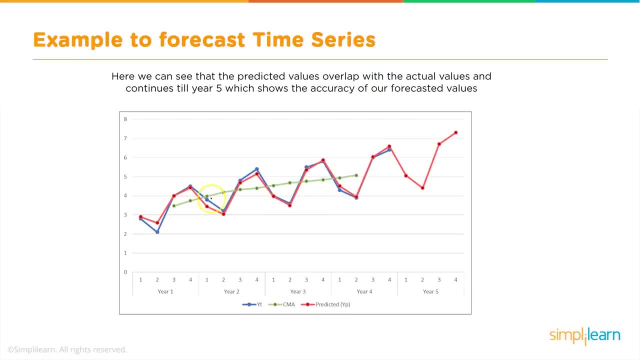 is how the plot looks. this is the cma, or the centered moving average. the green color and then the blue color is the actual data. red color is the predicted value predicted by our handcrafted model. okay, so remember, we did not use any regular forecasting model or any tool we have. 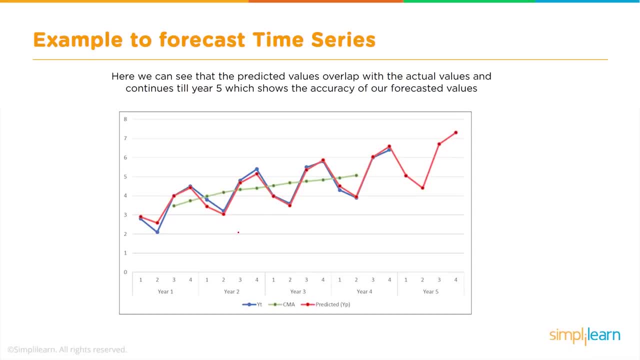 done this manually, and the actual tool will be used in the next video. this is just to give you an idea about how, behind the scenes, or under the hood, how forecasting works. a time series analysis, how it is performed. okay, so it looks like it has captured the trend properly. so up to here is the 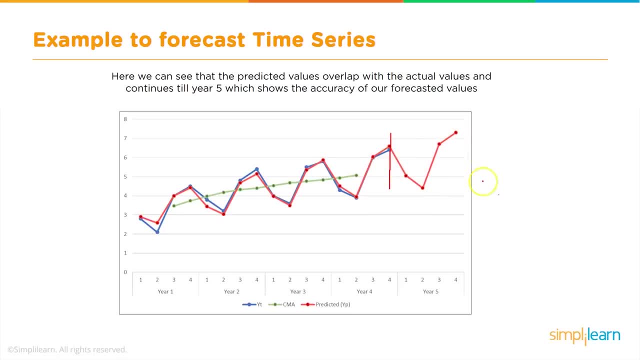 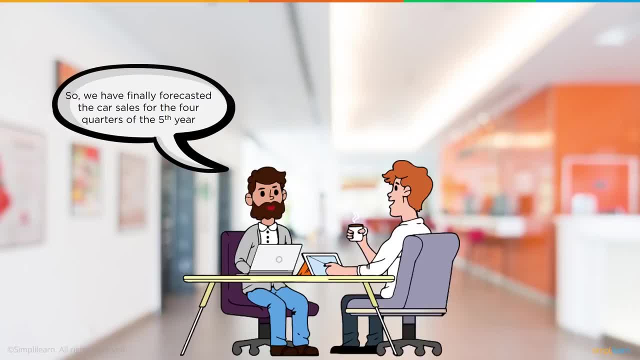 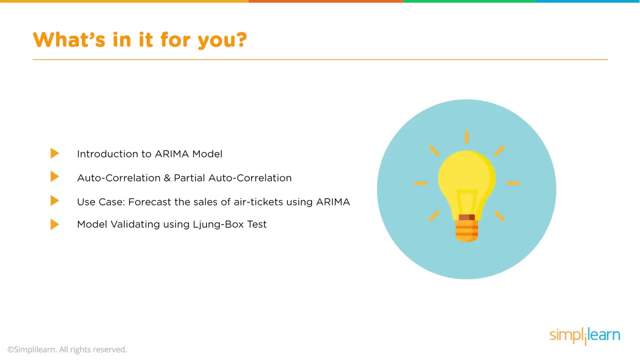 mentioned earlier, we can safely assume that the values are accurate and predicted properly for the fifth year. let's go ahead and implement a time series forecast in our so in this section. what are we going to do? we are going to use arima model. there are different models and 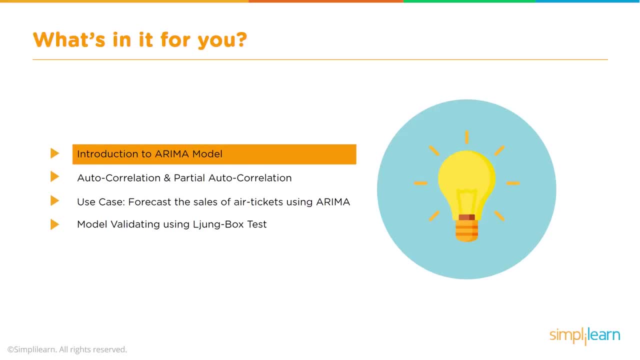 algorithms for performing time series forecast. so we will use arima where is the most common one, and we will also talk about what is autocorrelation and partial autocorrelation, and we will see that in our studio as well, and then we will take you through a use case where 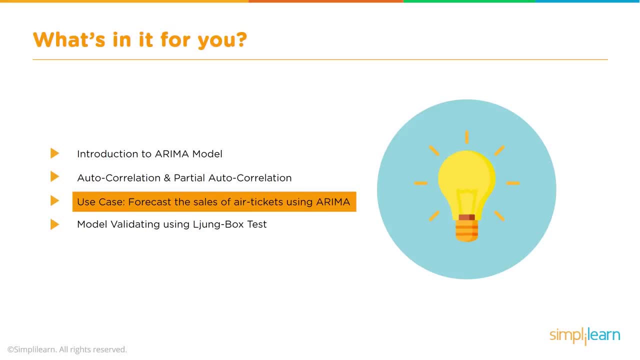 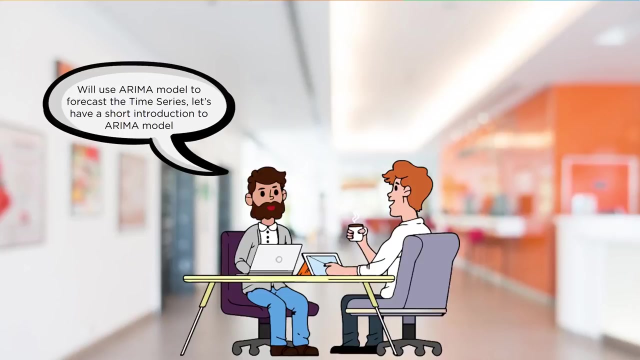 we will focus the air ticket sales for the future and then we will end with the model validation using the junk box text. okay, so with that, let's get started. first of all, as i mentioned, we will be using the arima model to do the forecast of this time series data, so let us try to understand. 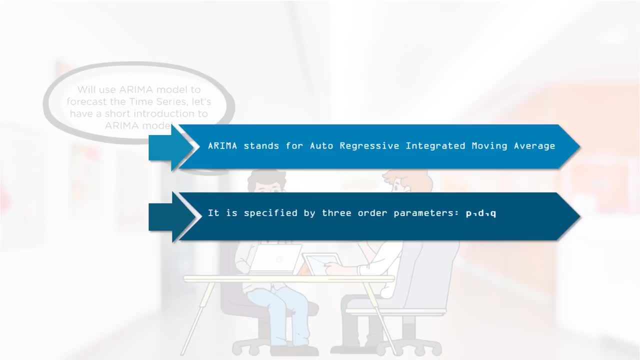 what is arima? so arima is actually an acronym. it stands for autoregressive, integrated moving average. so that is what is arima model, and it is specified by three parameters, which is p, d and q. p stands for autoregressive, so let me just mark this. so there are 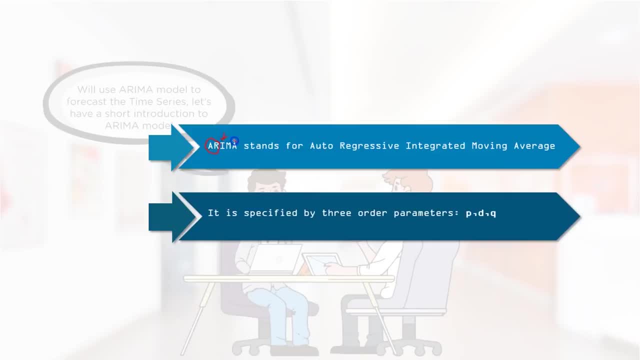 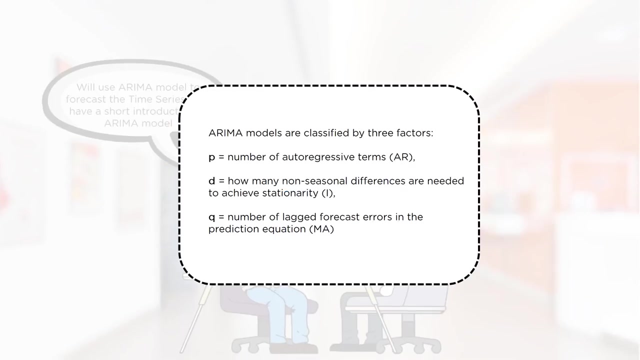 three components here: autoregressive, integrated, moving average. okay, so these three parameters correspond to those three components. so the p stands for autoregressive, d for integrated and q for moving average. so let us see what exactly this is. so these three factors are: p is the number. 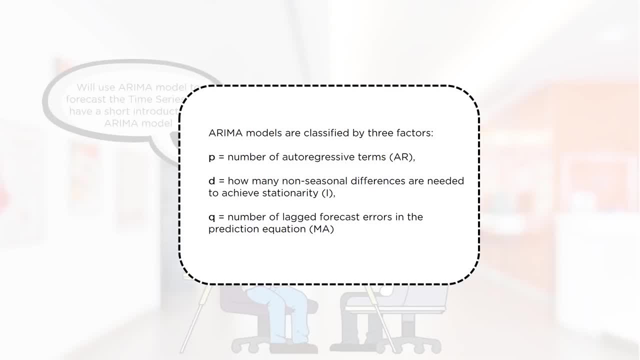 of autoregressive terms, or ar- we will see that in a little bit- and d is how many levels of differences that we need to take care of in order to be able to solve this. so let's look at the next two parameters to do, or differentiation we need to do, and q is the number of lag forecast errors. so we'll see. 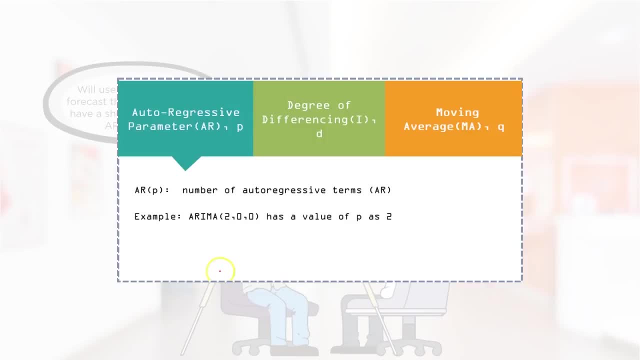 what exactly each of these are. so ar is the number of autoregressive terms, and which is basically denoted by the p, and then we have d, which is for the number of times it has to be differentiated, and then we have q, which is for the moving average. so what exactly ar terms? so, in terms, 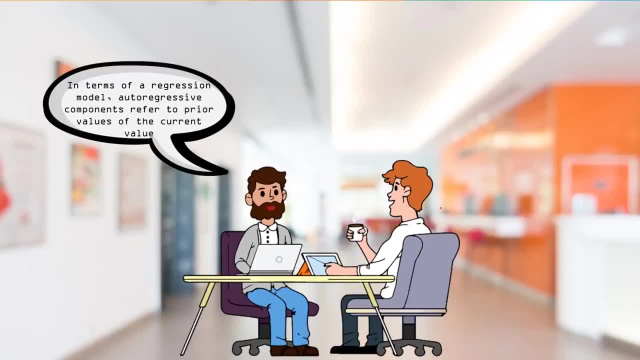 of the regression model. autoregressive components refer to the prior values of the current value. what we mean by that is here: when we talk about time series, data focus on the fact that there is regression. so what exactly happens in regression? we try to do something like, if it is simple, linear. 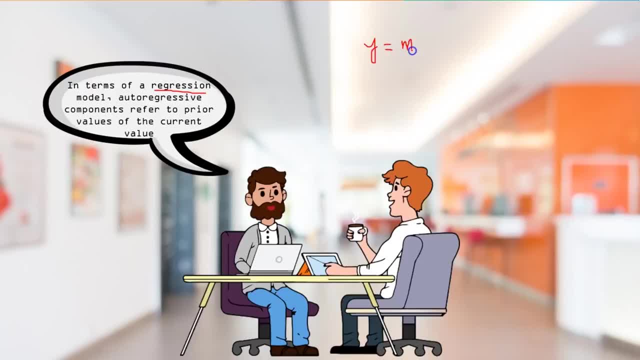 regression, we do some equation like: y is equal to mx plus c, where there are actually there are two variables: one is the dependent variable and then there is an independent variable variable. let me just complete this equation as well: mx plus c, right, so this is a normal. 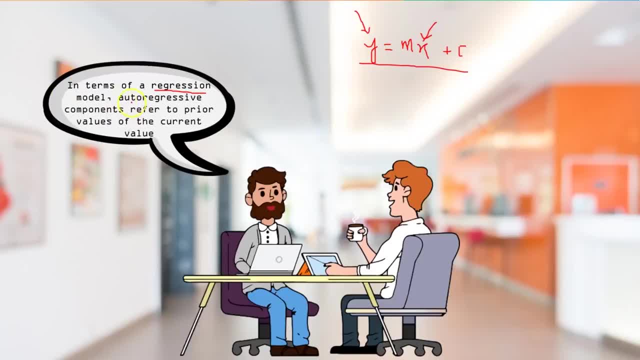 regression curve or a simple regression curve. now, here we are talking about auto regression or autoregressive. so autoregressive, as the name suggests, is regression of itself, so which means that here you have only one variable, which is your maybe the cost of the flights, or whatever it is. 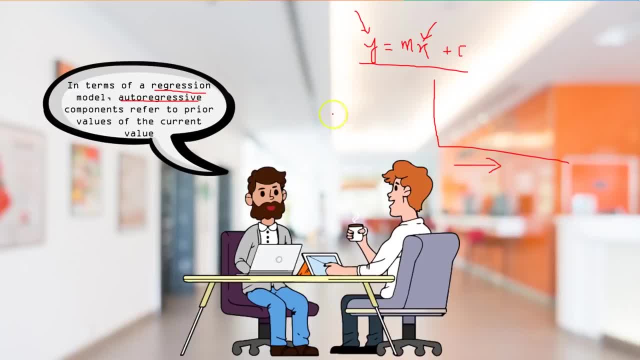 right. and the other variable is basically time dependent and therefore the value at any given time and that we will denote as yt, for example. so there is no x here, there is only one variable, and which is y, and we say yt, which is basically the predicted value at a time interval, t for 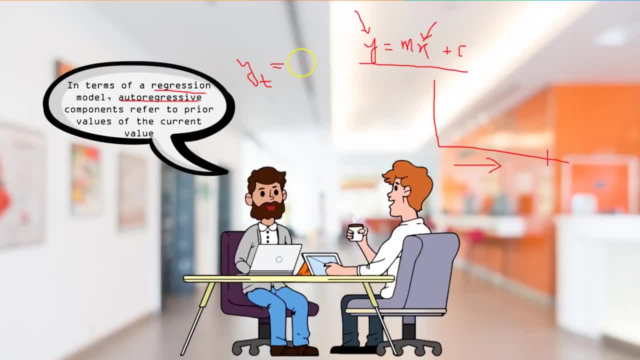 example, is dependent on the previous value. so, for example, there may be a 1 and then yt minus 1, and then there will be like plus a 2 and right, plus a 2 and y t minus 2 and all right, and then plus a 3 into y t minus 3, correct? so basically here what we are. 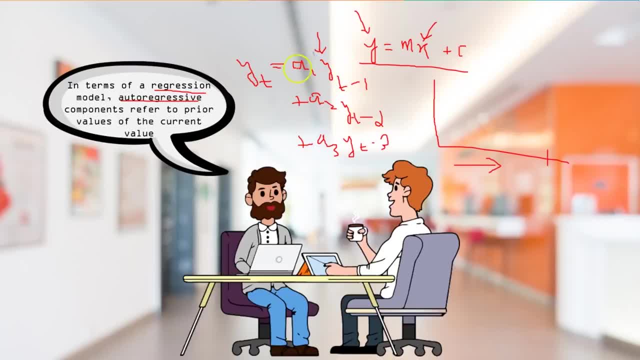 saying is there is only one variable here, but there is a regression component, so we are doing a regression on itself. so that's how the term auto regression comes into play. so only thing is that it is dependent on the previous time values, so there is a lag. let's say this is the 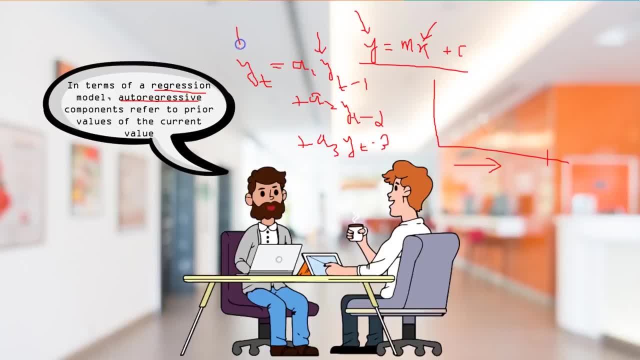 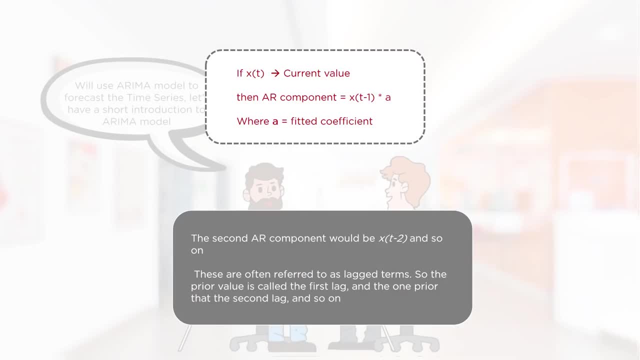 first lag, second lag, third lag and so on. so the current value, which is by t, is dependent on the previous time lag values. so that is what is order regression component. so this is what is shown here. for example, in this case, instead of y we are calling it as x. so that's the same and this. 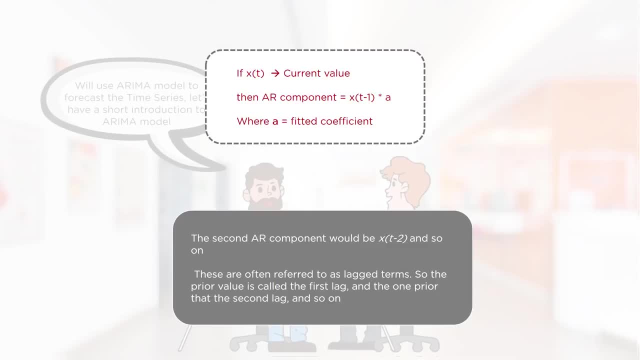 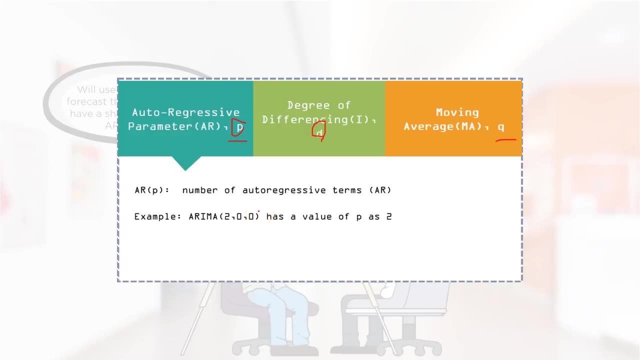 is represented by some equation of that sort: depending on how many lags we take. so that is the ar component, and the term p is basically determines how many lags we are considering. so that's the term before now. what is d? d is the degree of differencing. so here, 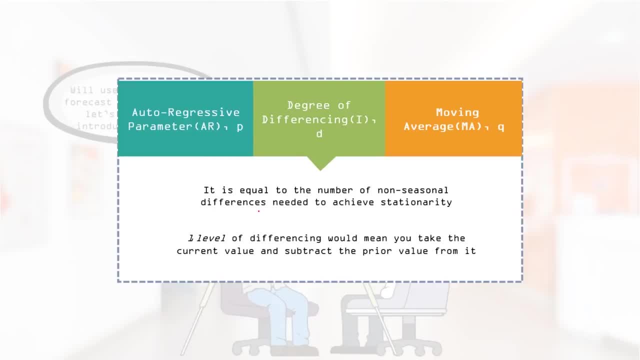 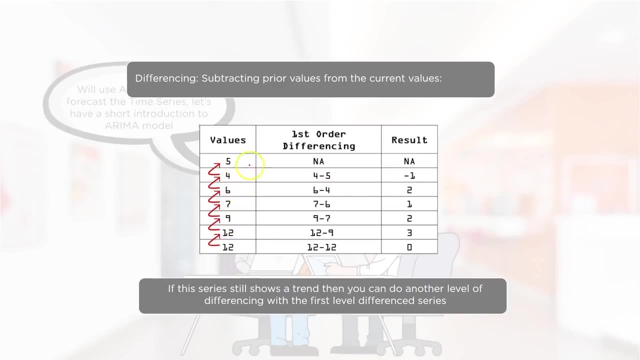 differencing is like to for the non-seasonal differences, right. so, for example, if you take the values like this which are given for 5, 4, 6 and so on and so forth, if you take the differencing of one after another, like, for example, 5 minus 4 or 4 minus 5, the next value with the 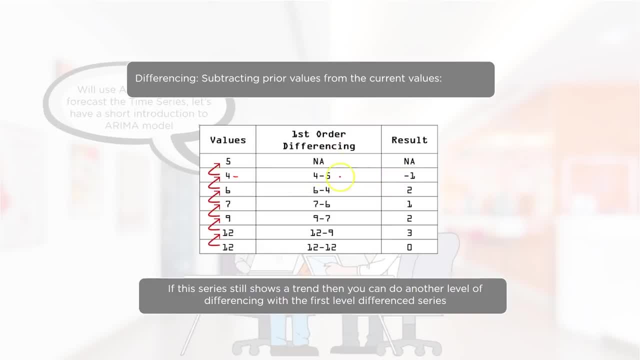 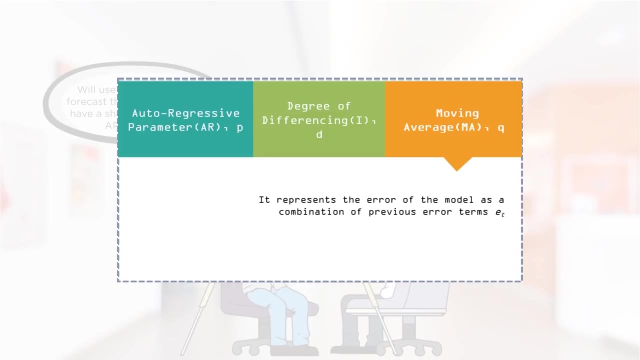 previous value, so 4 minus 5.. so this is known as the first order differencing. so the result is minus 1.. similarly, 6 minus 4 is 2.. 7 minus 6 is 1.. so this is first order differencing, and here we call it as: d is equal to 1. okay, and same way we. 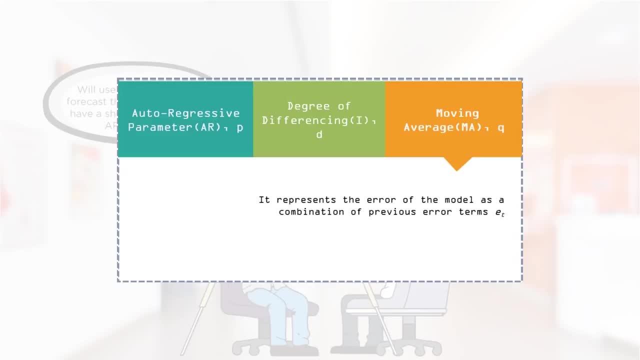 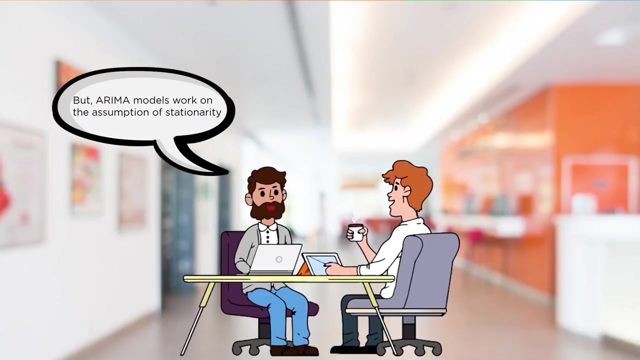 can have second order, third order and so on. then the last one is q. q is the actually why we call it moving average, but in reality it is actually the error of the model. so we also sometimes represent as et all right. so now, arima model works on the assumption that the data is stationary. 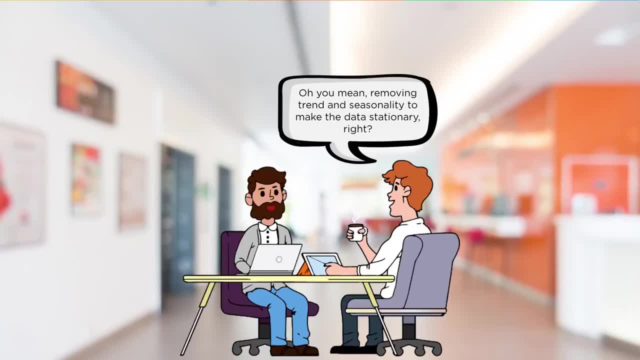 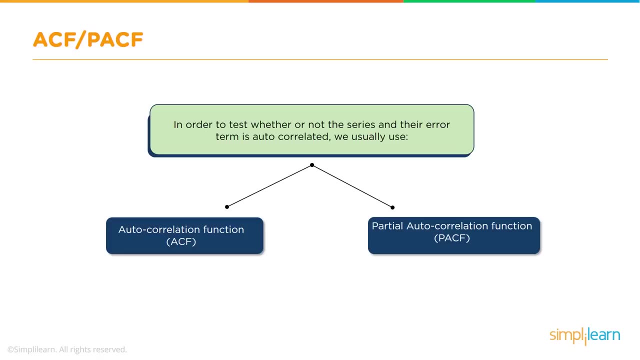 which means that the trend and seasonality of the data has been removed. that is correct. okay, so this we have discussed in the first part: how, what exactly is stationary data and how do we remove the non-stationary part of it? now in order to test whether the data is stationary or not, there are two important 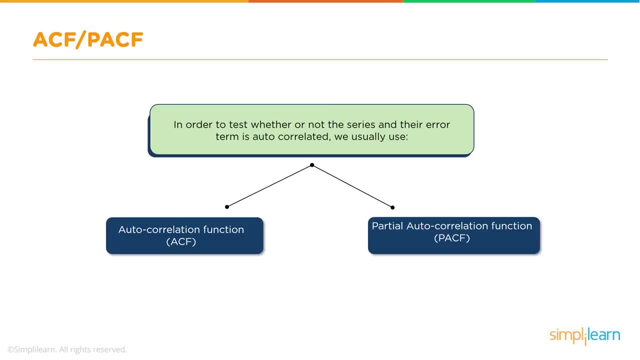 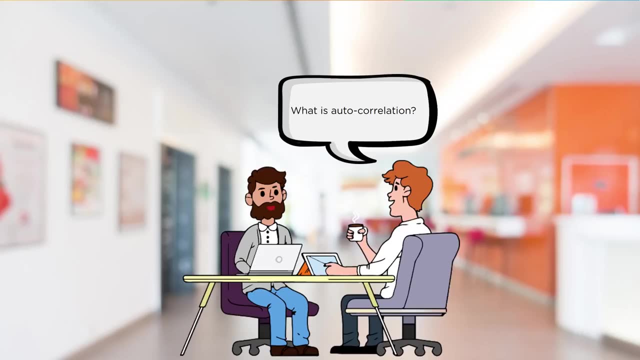 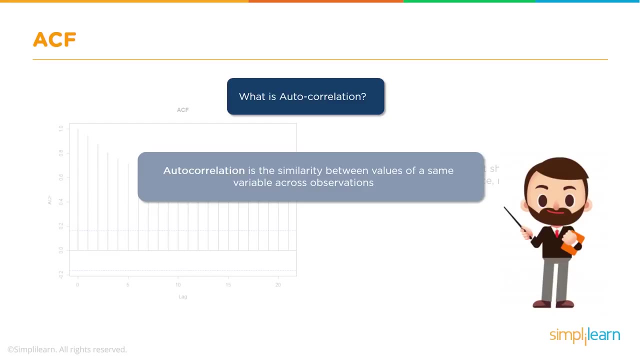 components that are considered. one is the autocorrelation function and the other is the partial autocorrelation function, so this is referred to as acf and pscf. all right, so what is autocorrelation and what is the error of the? is the definition or correlation is basically the similarity between values of a same variable. 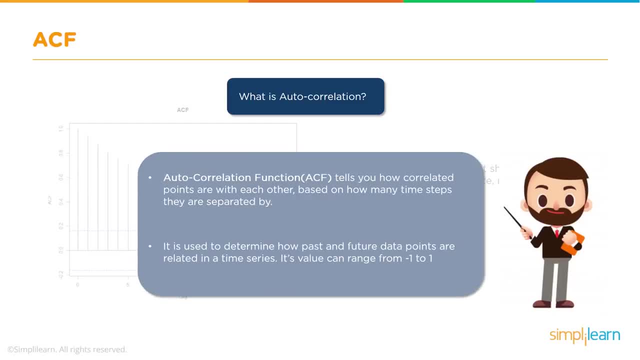 across observations, as the name suggests. now, how do we actually find the autocorrelation function, the value, right? so this is basically done by plotting, and autocorrelation function also tells you how correlated points are with each other based on how many time steps they are separated. 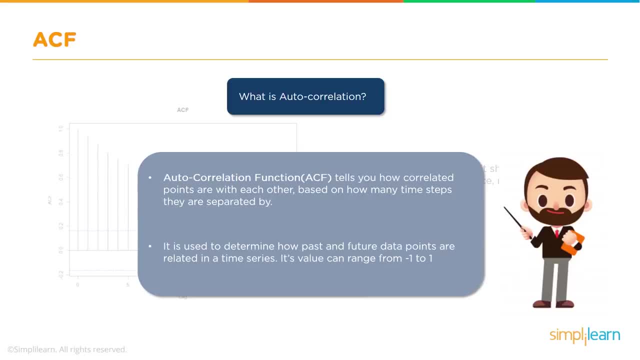 by and so on. that is basically the time lag that we were talking about, and it is also used to determine how past and future data points are related, and the value of the autocorrelation function can vary from minus one to one. so if we plot, this is how it would look: autocorrelation. 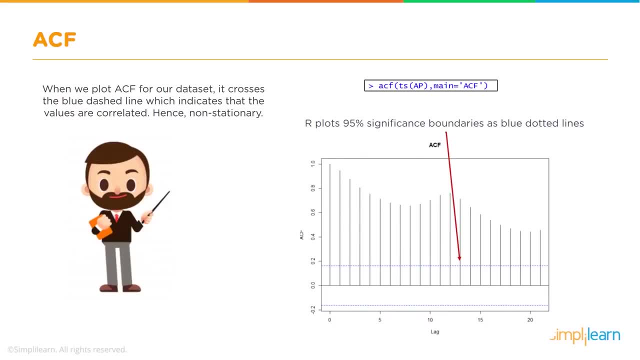 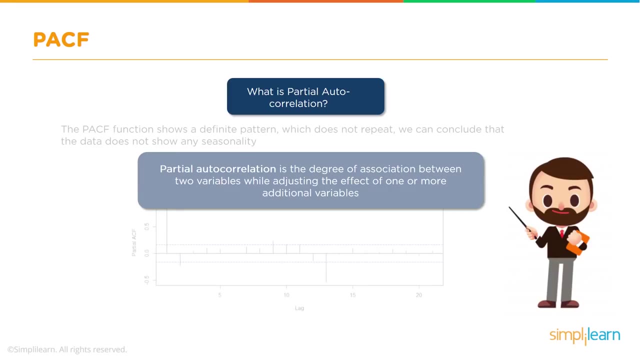 function would look somewhat like this, and there is actually a readily available function in r, so we will see that and you can use that to plot your autocorrelation function. okay, so that is acf and we will see that in our r studio in a little bit. and similarly, you have partial 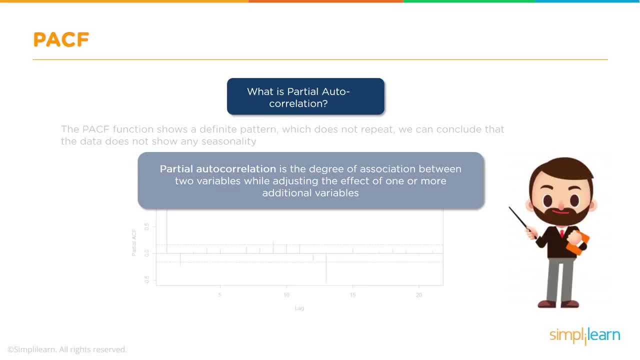 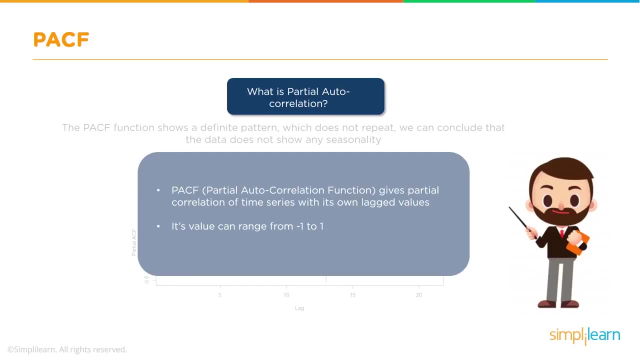 autocorrelation function. so partial autocorrelation function is the degree of association between two variables while adjusting the effect of one or more additional variables. so this again can be measured and it can also be plotted and its value once again can go from minus one to one and it gives the partial correlation of time series with its. 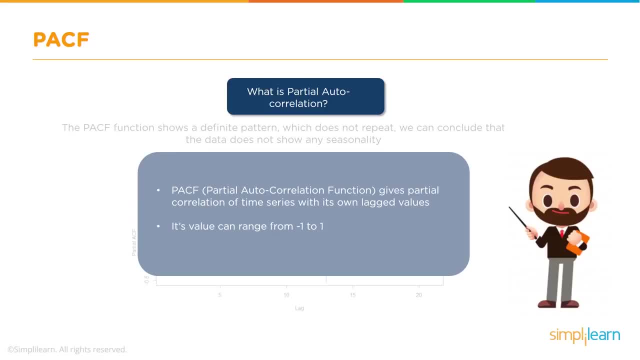 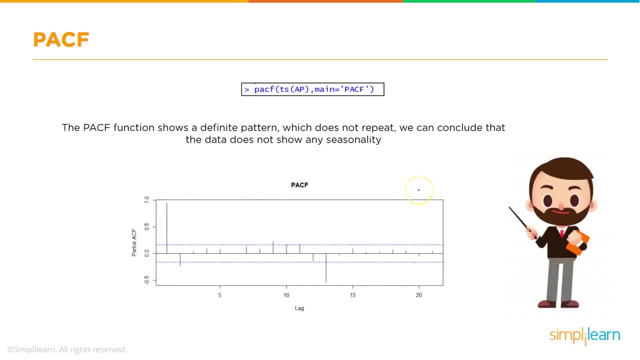 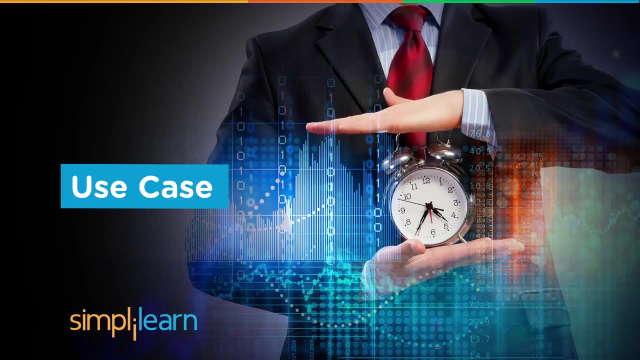 own lagged values, so lag again. we have discussed in the previous uh couple of slides this is how a psef plot would look in our studio. we will see that as well, and once we get into the r studio- and with that, let's get into our studio and take a look at our use case before we go into- 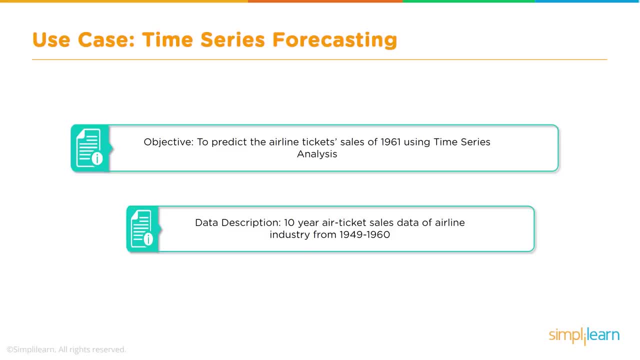 the code. let's just quickly understand what exactly is the objective of this use case. so we are going to predict some values or forecast some values, and we have the data of the airline ticket sales of the previous years and now we will try to find or predict or forecast the values. 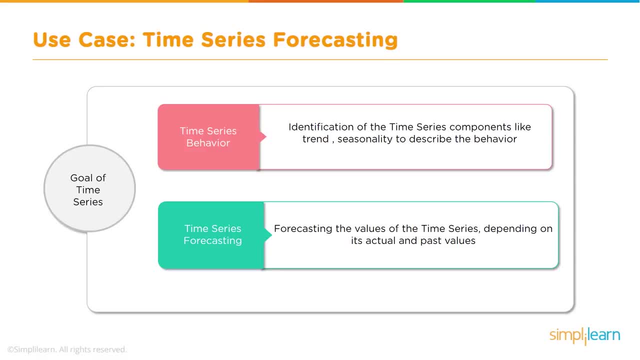 for the future years. all right, so we will basically identify the time series components like trend, seasonality and random behavior. we will actually visualize this in our studio and then we will actually forecast the values based on the past values or history data, historical data. so these are the steps that we follow. we will see in our 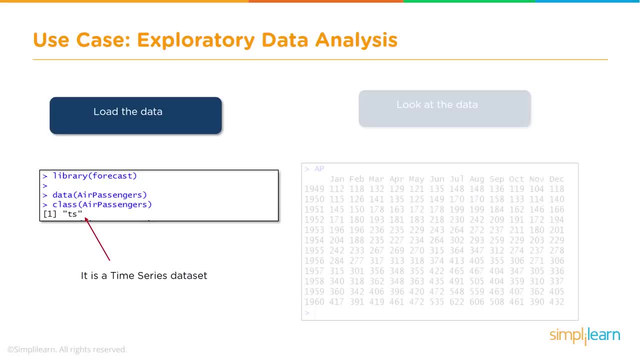 studio in a little bit, just quickly. let's go through what are the steps. we load the data and it is a time series data. we try to find out what class it belongs to. the data is actually air passengers data. they're having a lot of data in r studio. let's go through the data in r studio. 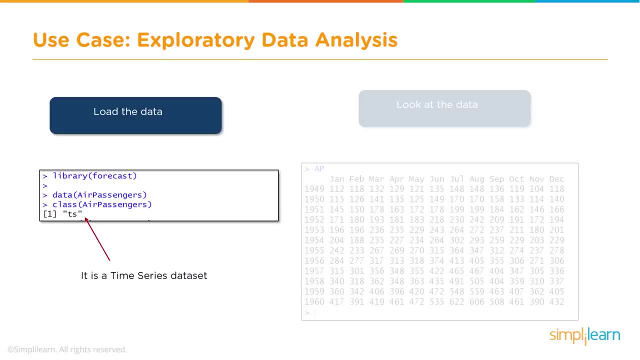 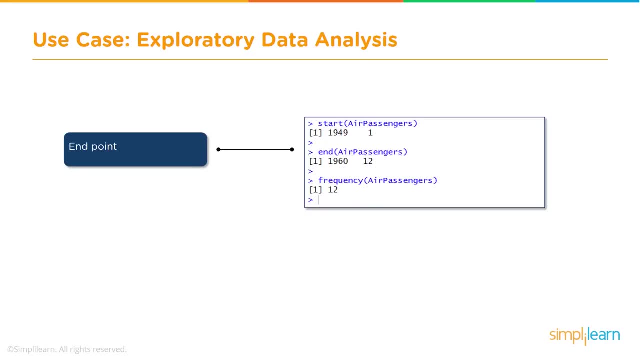 is already comes pre-loaded with r studio, so we will be using that and we can take a look at the data. and then, what is the starting point? what is the end point? so these are all functions that are readily available we'll be using. and then, what is the frequency? it's basically frequency is 12, which 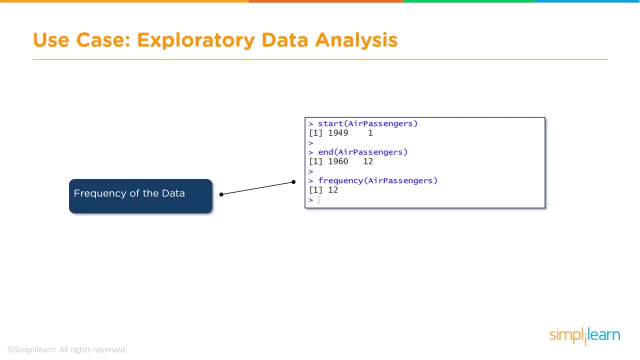 is like yearly data, right, so every month the data has been collected, so for each year it is 12, and then we can check for many missing values, if there are any, and then we can take a look at summary of the data- this is what we do in exploratory data analysis- and then we can plot the data visualize. 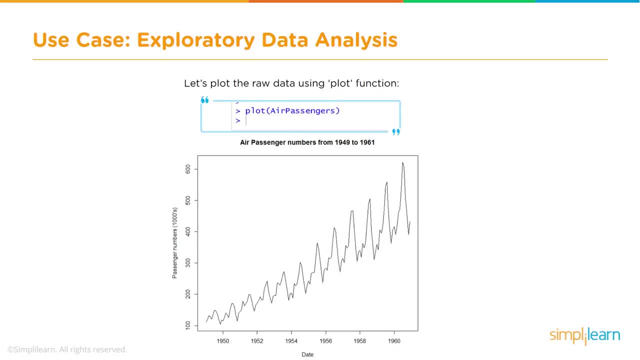 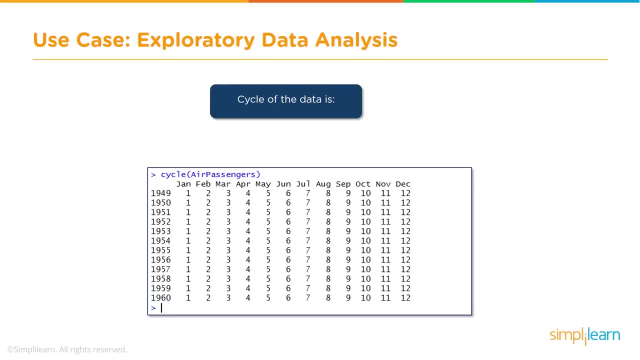 the data, how it is looking, and we will see how the data has some trend, seasonality and so on and so forth. all right, then we can take a look at the cycle of the data using the cycle function and we can see that it is every month, that's the cycle end of every 12 months, a new cycle begins. so 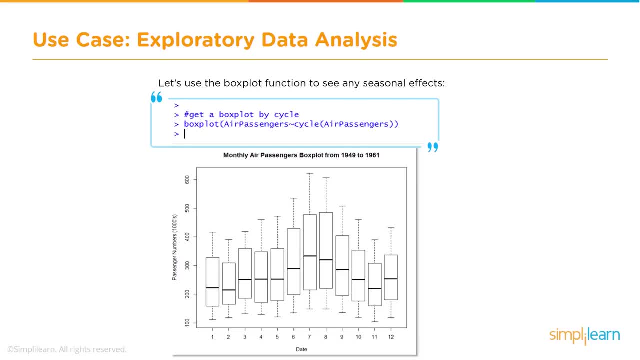 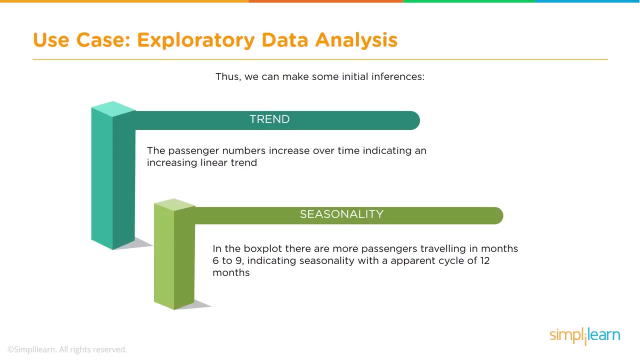 each month of the year is the data is available, then we can do box plots to see for each month how the data is varying over the various 10 or 12 years that we will be looking at this data and from exploratory data analysis we can identify that there is a trend, there is a seasonality. 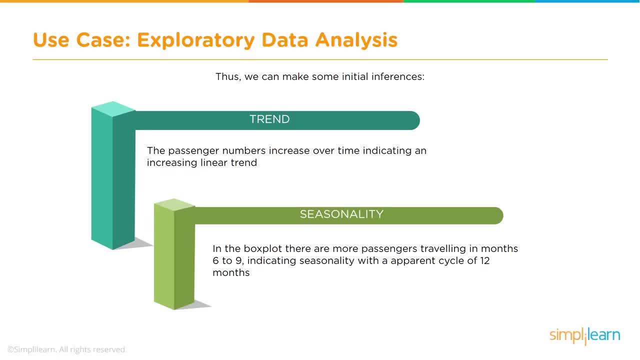 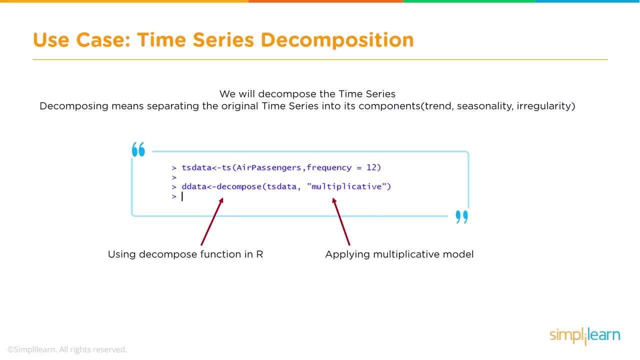 component and how the seasonality component varies. also, we can see from the box plots and we can decompose the data. we can use the decompose function rather to see the various components, like the seasonality trend and the irregularity part. okay, so we will see all of this. 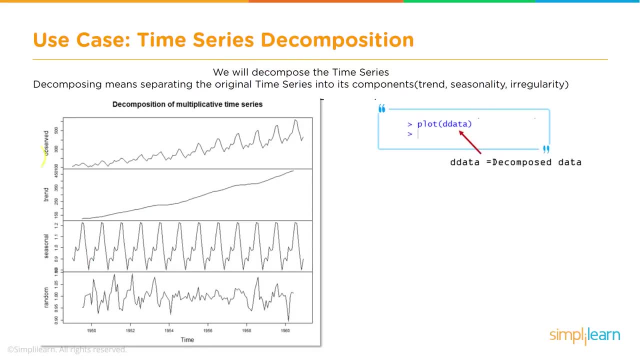 in our studio. this is how they will look. this is the once you decompose and this is how you will. actually you can visualize the data. this is the actual data and this is the trend. as you can see, it's going upwards. this is the seasonal component and this is your random or irregularity right. so 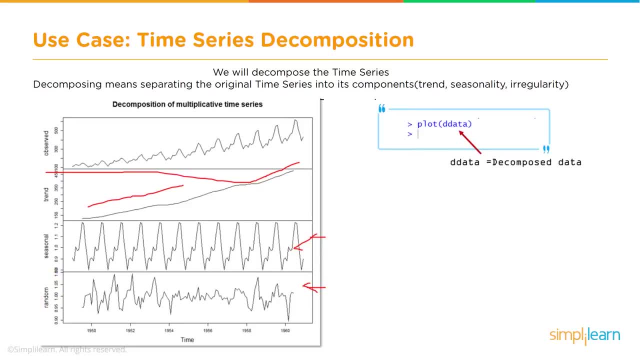 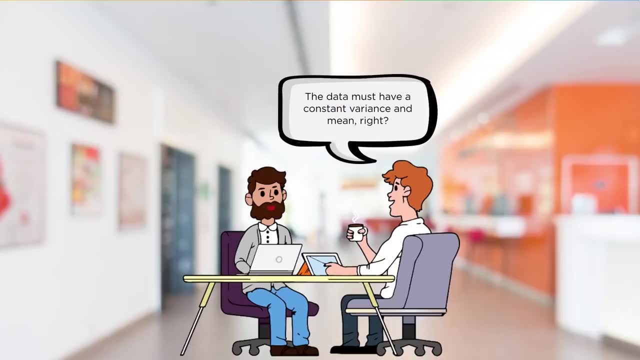 we call it irregularity, or we can also call it random, as you can see here. yes, so the data must have a constant variance and mean, which means that it is stationary before we start any analysis, time series analysis and without. so, basically, if it is stationary, only then it is easy to model. 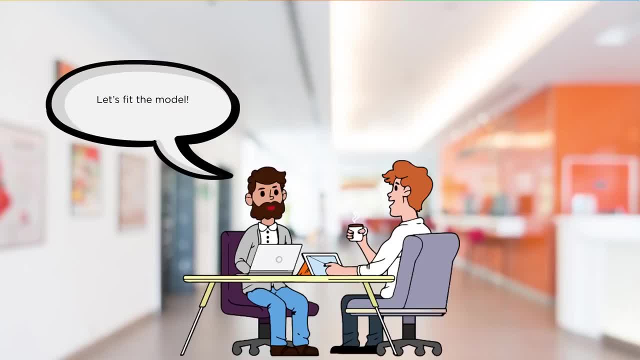 the data perform time series analysis, so we can then go ahead and fit the model. as we discussed earlier, we'll be using a remote model. there are some techniques to find out what should be the parameter, so we will see that when we go into our studio. so the 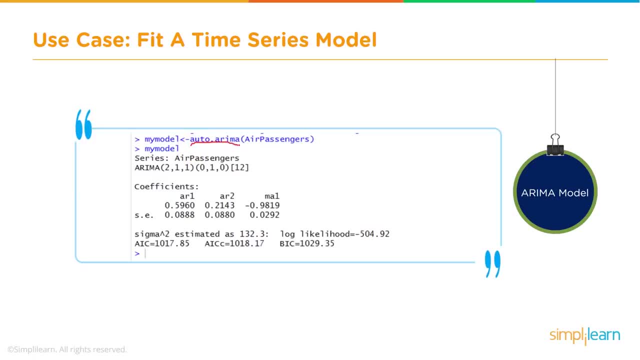 auto arima function basically tells us what should be the parameters, right? so these parameters are the p, d and q that we talked about. that's what is being shown here. so if we use auto or uma, it will basically take all possible values of this pdq, these parameters, and it will find out what is. 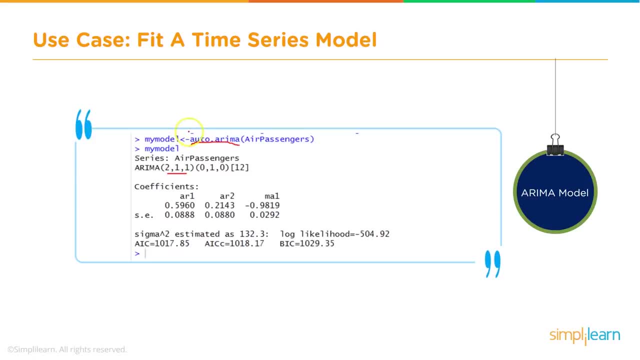 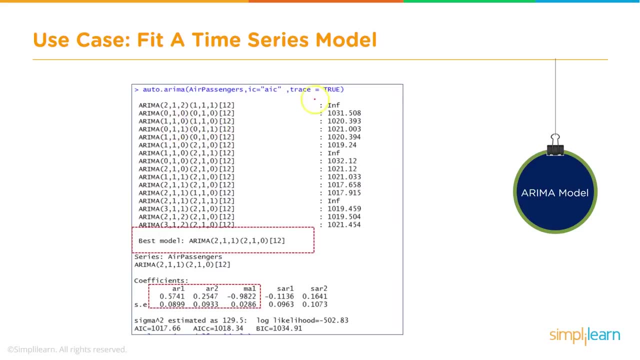 the best value and then it will recommend. so that is the advantage of using auto arena. all right, so, like in this case, it will tell us, or at least parallel, what it is, so that we can see if the available values. but if we use this parameter trace, we set the parameter trace is equal to true, then it will. 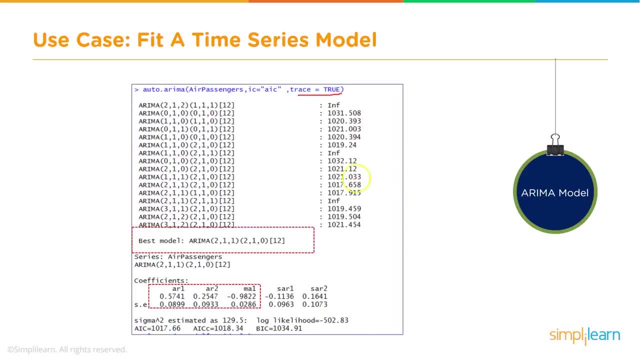 basically tell us what is the value of this aic, which has to be minimum. so the lower the value, the better. so, for each of these combinations of pd and q, it will give us the values here and then it will recommend to us which is the best model. okay, because whichever has the lowest value of this aic. 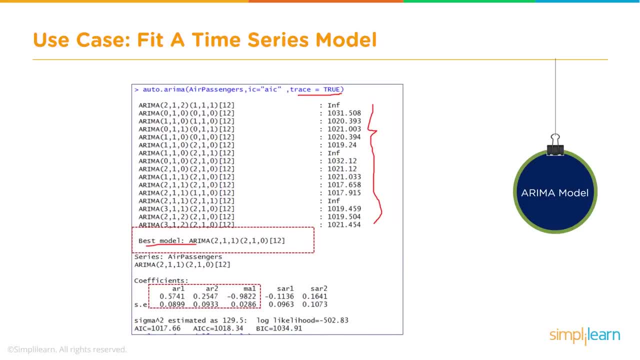 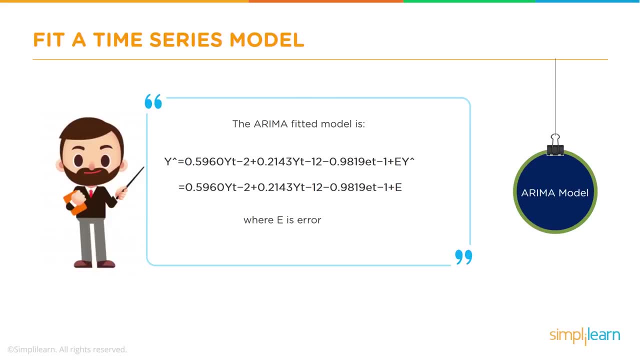 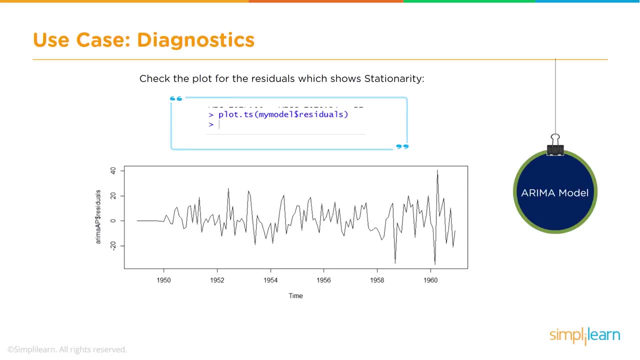 it will recommend that as your best pdq values. so once we have that, we can see that we will. basically, we can potentially get a model or the equation. model is nothing with the equation and based on the parameters that we get and we can do some diagnostics, we can do some plotting. 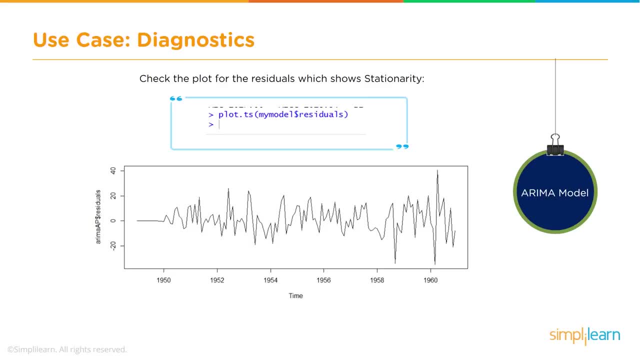 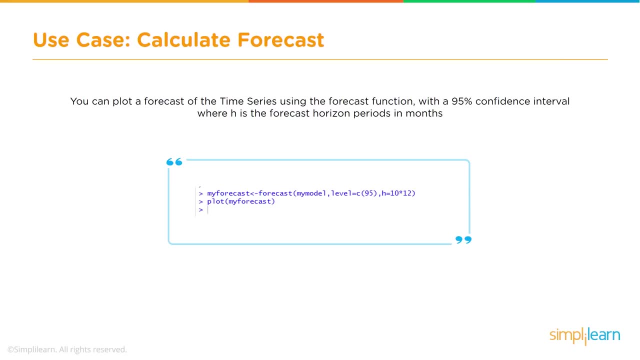 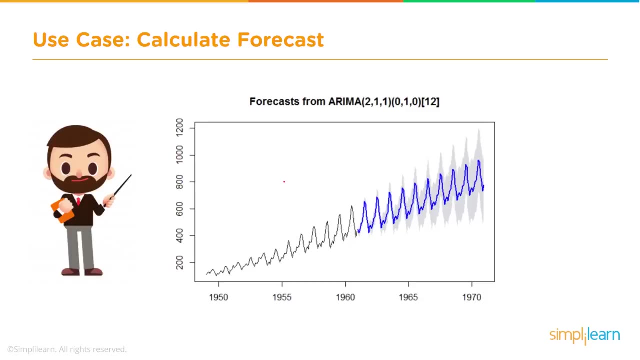 to see how, whether there is a plot for the residuals, so which shows the stationarity, and then we can also take a look at the acf and pscf. we can plot the cf and pscf and then we can do some forecasting for the future here. so in this case we have up to 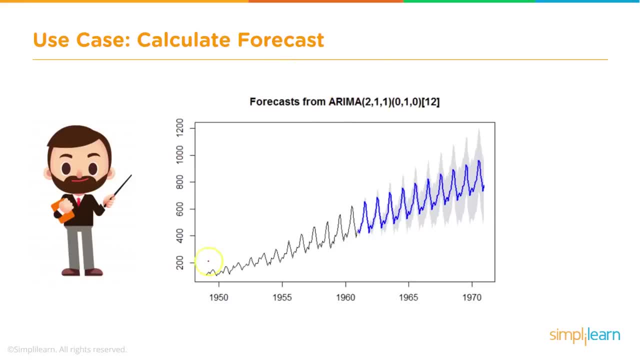 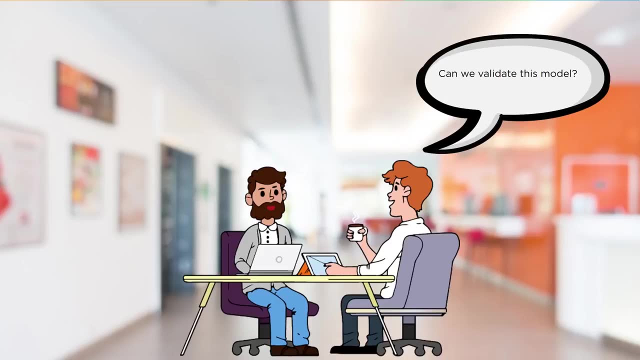 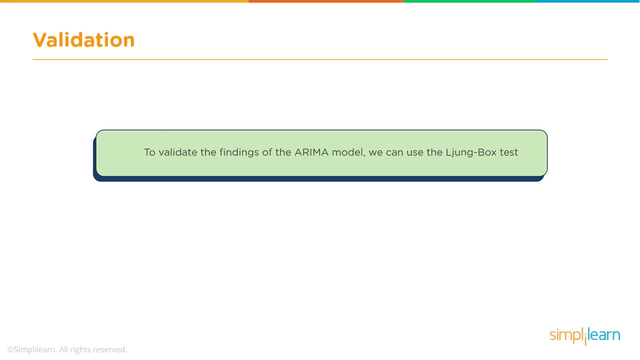 1960, and then we can see how we can forecast for the next 10 years, which is 1970 up to 1970.. and once we have done this, can we validate this model? yes, definitely, we can validate this model. and to validate the findings we use a junk box test, and this is how you just call boxtest, and then you 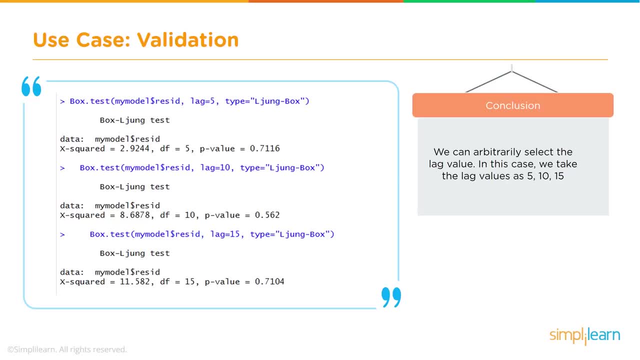 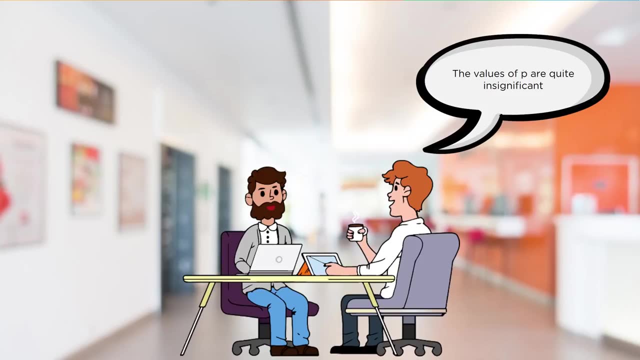 pass these uh parameters and you will get the values that will be returned, which will tell us whether this how accurate this model is, how accurate the predictions are. so the values of p are quite insignificant in this case. we will see that, and that also indicates that our model is. 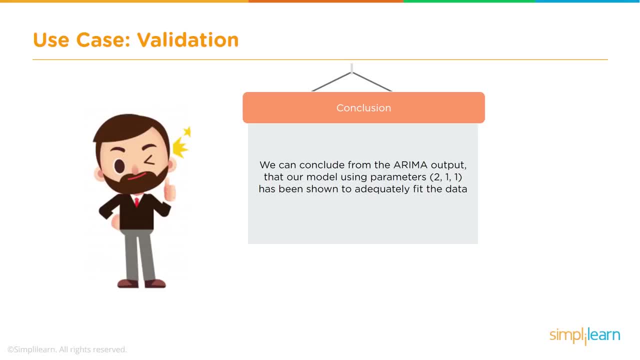 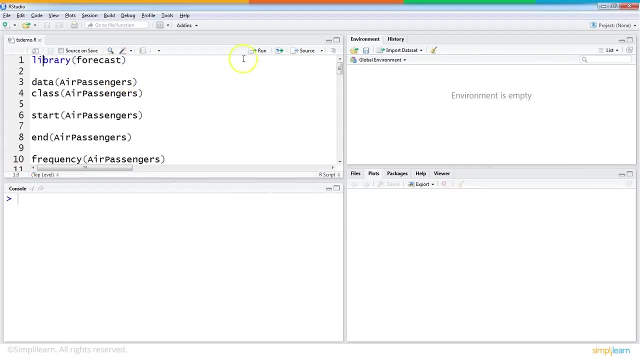 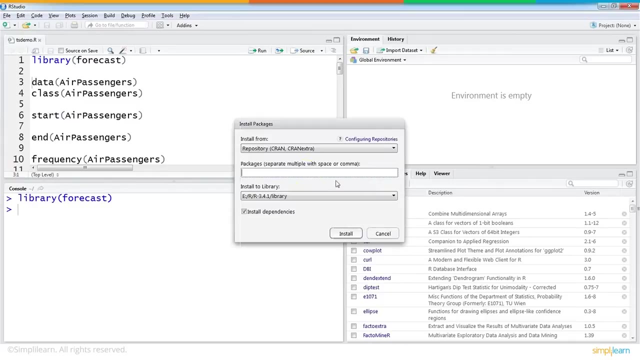 free of autocorrelation, and that will basically be it. so let's go back and into our r studio and go through these steps in real time. so we have to import this library. forecast packages not installed: you have to go here and install the forecast package. okay, so that's the easy way. 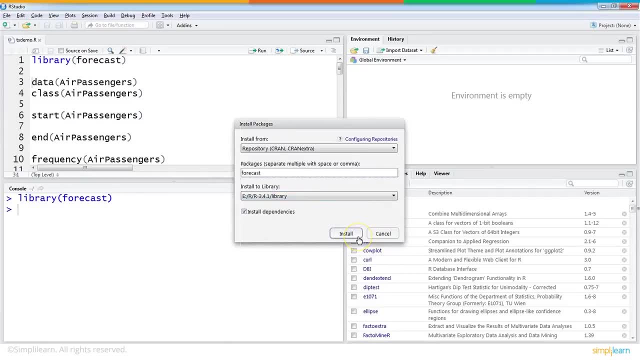 to install rather than to click on this install. i will not do it now because i've already installed, so the first time that's only one time. then after that you just have to load it into memory and then keep going. so we will load this data called air passengers. so by calling this data method and 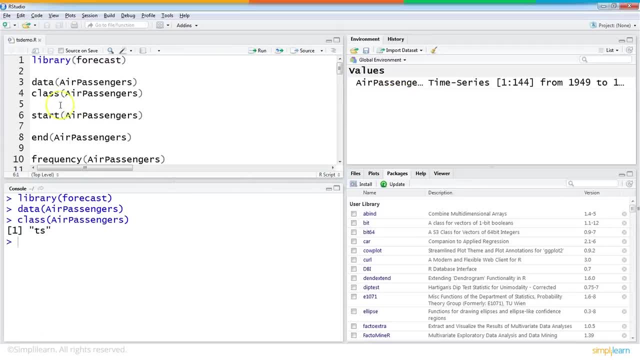 if you see the the data passengers is loaded here and if we check for the class, it is a time series data, ts data, so we can check for the dates. we can also view the data in a little bit and the start date is 1949 and january and our end date is 1960, december, and the frequency is 12, which is 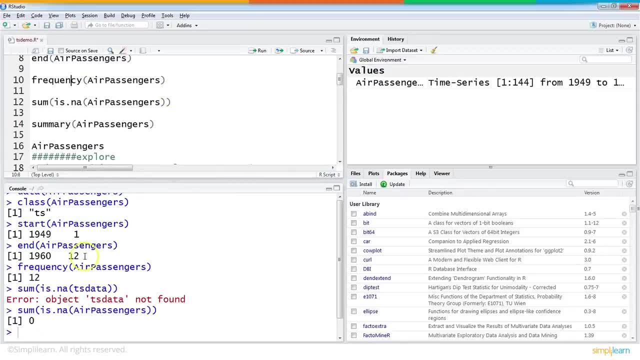 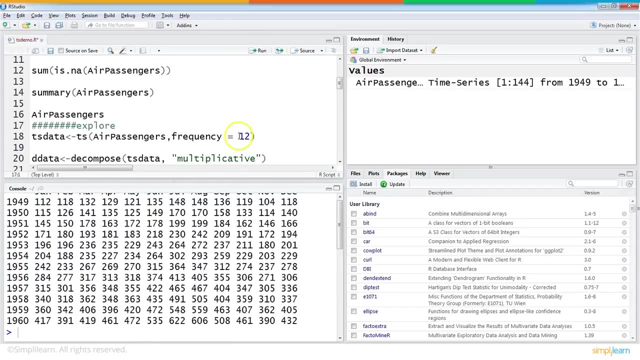 like collected monthly. so that is the frequency, which is 12 here, and then we check if there are any um missing values. there are no missing values. and then we take a look at the summary of the data. this is all exploratory data analysis and then, if you just display the data, this is how it looks. 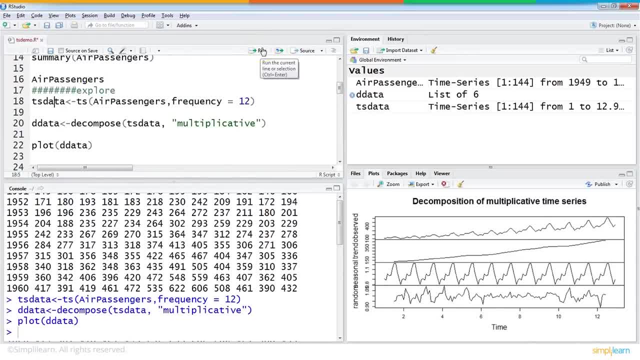 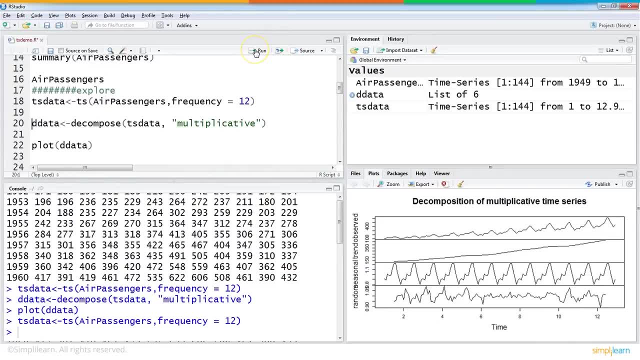 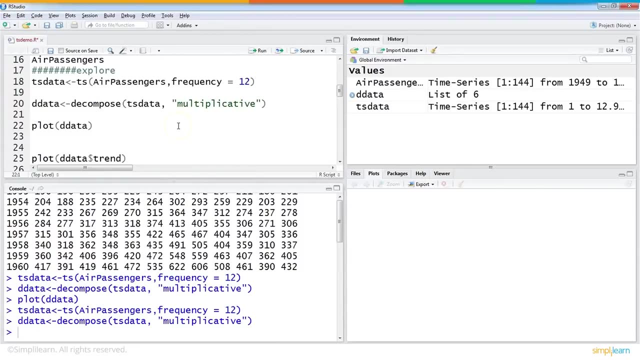 and then we need to decompose this data. so we will kind of store this in an object ts data and then use that to decompose and store the new values. let me just clear this for now: and if we decompose, basically as we have seen in the slides, decomposing is breaking it into the trend, seasonality and the 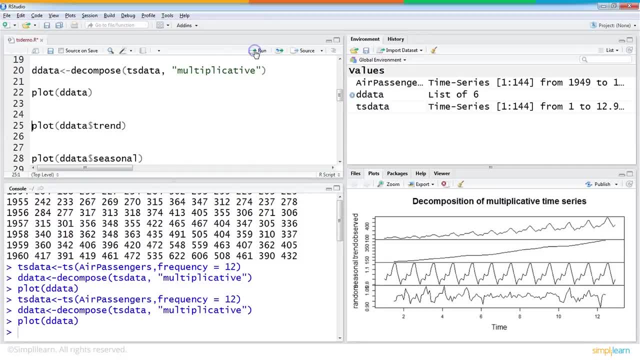 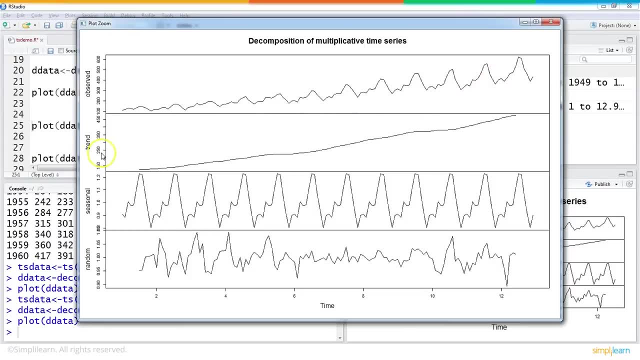 irregular or random components, then you can go ahead and plot it. so when you plot it, you can see here- let me zoom this- this is our original plot, or observed value as it is known, as then we have decomposed the three parts, which is basically the trend. as you can see, there is a 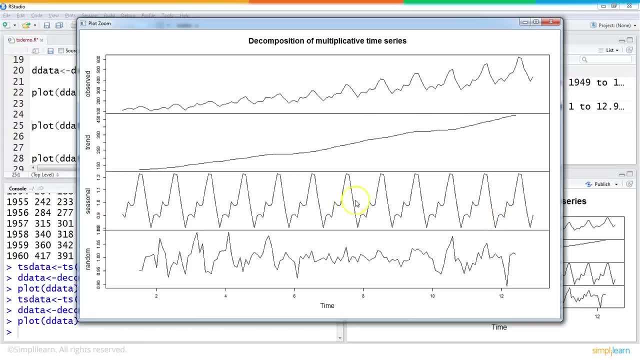 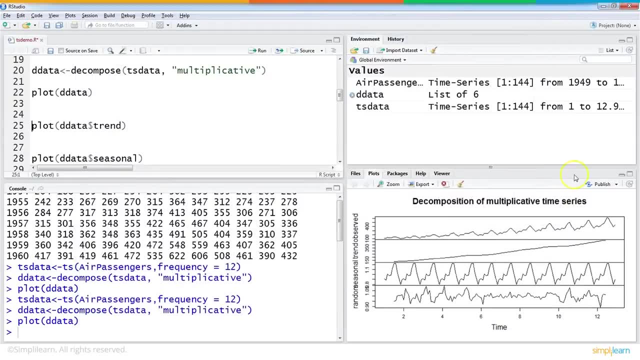 upvote trend, then the seasonal component, so this is some regularly occurring pattern, and then there is a random value which is basically- you cannot really give any equation or function or anything like that- so that's what this plotting has done. then we have the normal rate, which is the random. 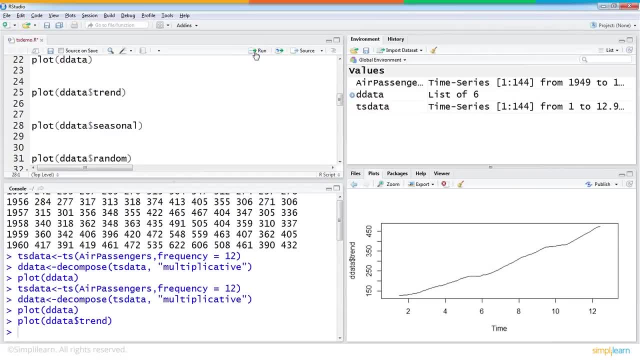 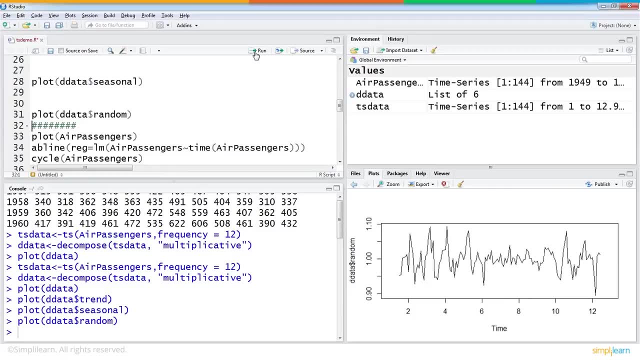 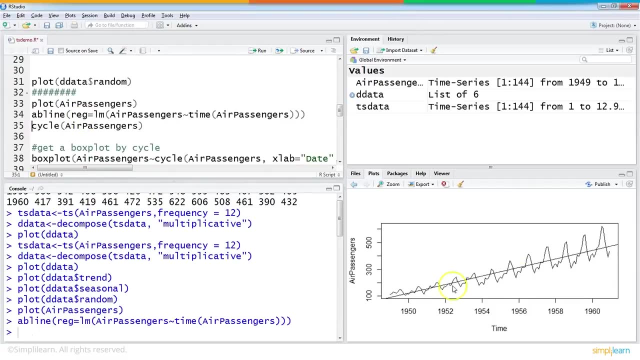 then you can actually plot them individually as well. so these are the individual plots for the trend, for the seasonal component and the random component. all right, so now let's take a look at the original data and see how the trend is in a way. so if we do this linear regression line, it 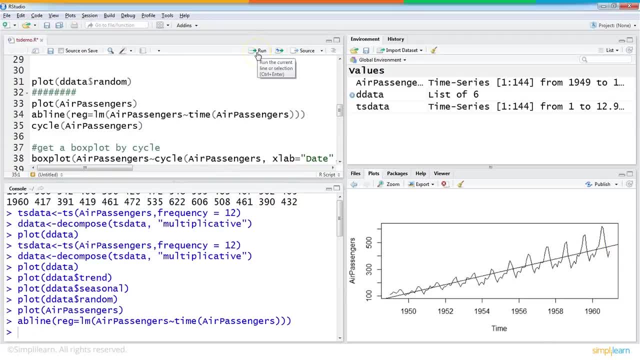 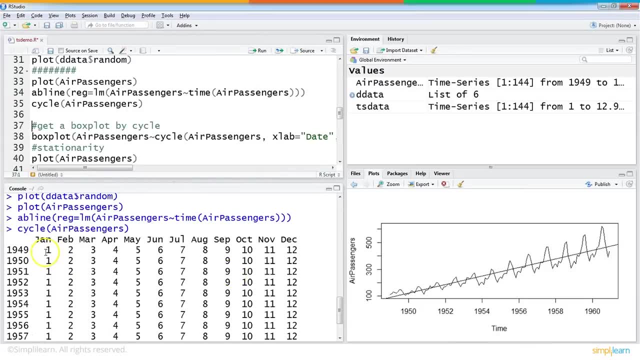 will show that the rate is going upwards and we can also take a look at the cycle that are there, which is nothing, but we have a frequency of 12, right? so the cycles will display that it is january, february to december and then back to january, february, and so on and so forth. 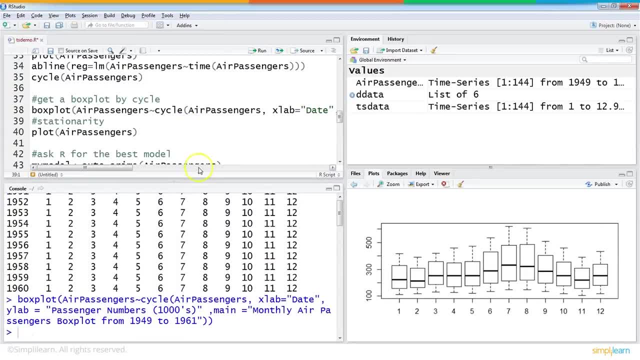 and if we do box plots for the monthly data, you will see that for each of the months right and over the 10 years that the data that we have, we will see that there is a certain pattern right. this is also in a way to find the seasonality component. so while january, february sales are relatively low. around july- august the sales pick up, so especially in july, i think, the sales are the highest, and this seems to be happening pretty much every year, right? so this is every year in july there seems to be a peak in the sales and then it goes down and slightly higher in december. 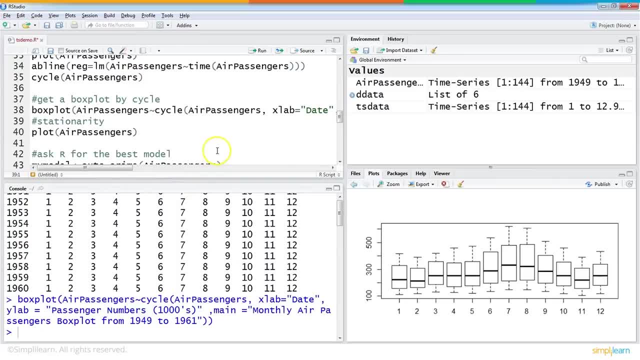 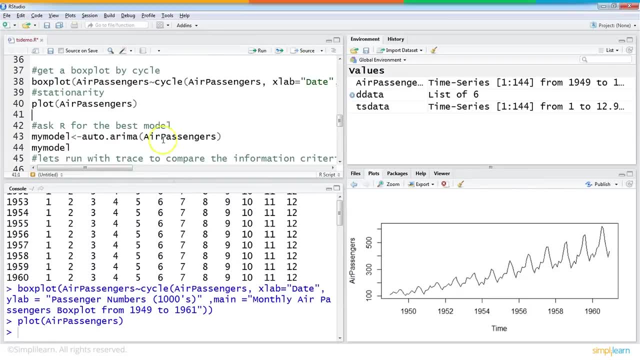 and so on. so that is again part of our exploratory data analysis and once again, let's just plot the data. now, as i said, in order to fit into an arima model, we need the value of the data, that we have, values of pd and q. now one way of doing it is- there are multiple ways actually of doing it- 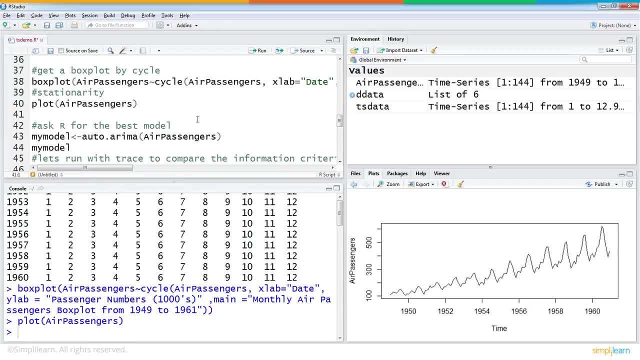 the earlier method of doing it was you draw the autocorrelation function plot and then partial autocorrelation function plot and then observe that and where does this change, and then identify what should be the values of p and q and so on. now r really has a very beautiful 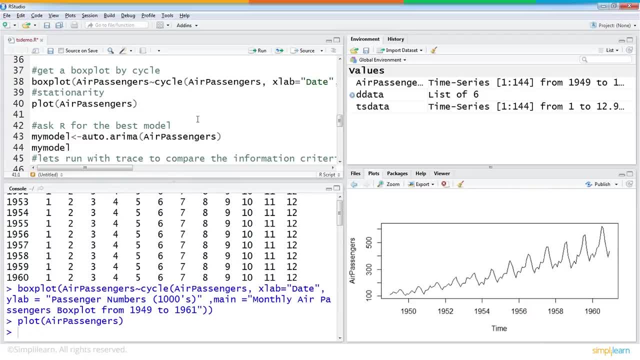 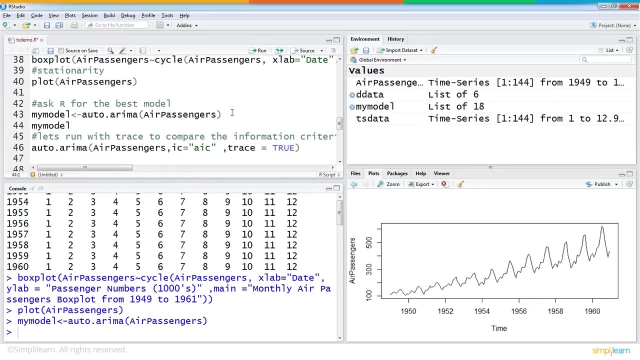 method which we can use to avoid all that manual process that we used to do earlier. so what r will do is there is a method called auto arima and if we just call this auto arima method and it will basically go and test the arima model for all possible values of this parameters, 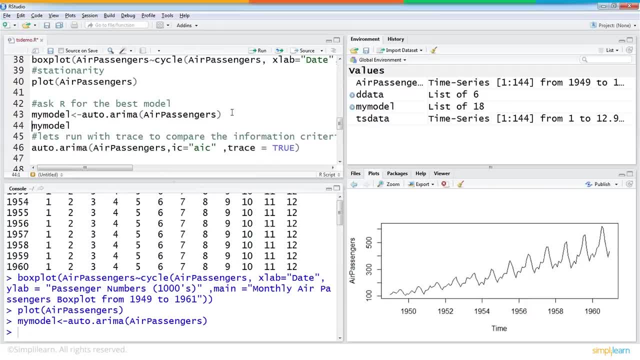 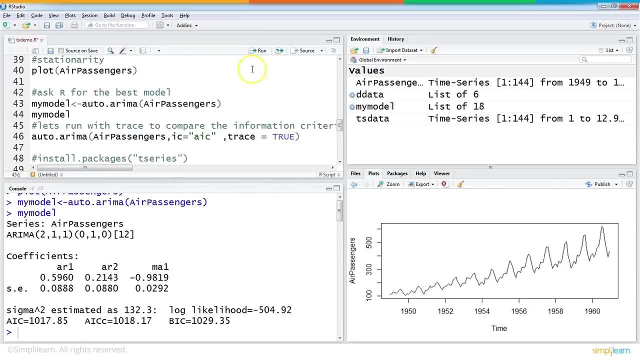 pdq and then it will suggest to you what should be the best model and it will return that best model with the right values of pd and q. so you, we, as data scientists, don't have to do any manual. you know trial and error kind of stuff. okay, so we got the model now and this is the model it it has. pdq values are 2, 1, 1. 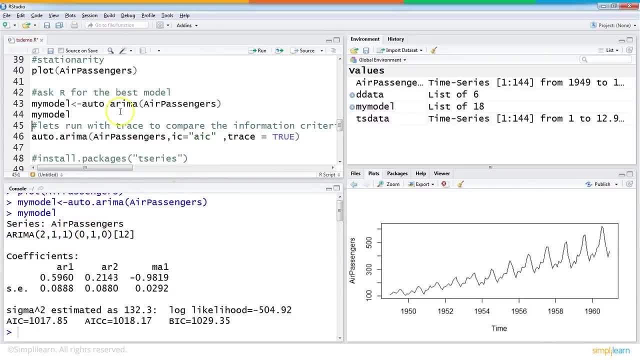 pdq, and this is the seasonal part of it, so we can ignore it for now. and so if we want to actually understand how that has returned these values- 2, 1, 1- as the best one, there is another functionality or feature where we can use this trace function or trace parameter. so if you pass to auto arima, 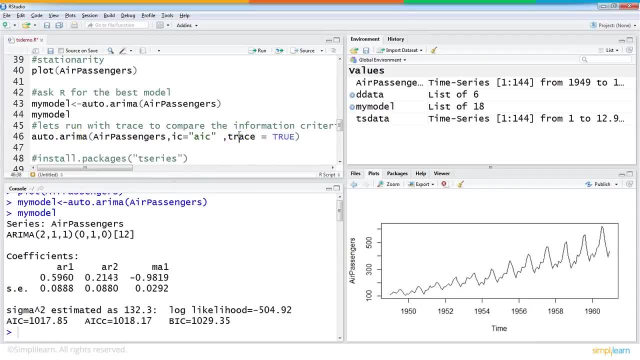 the trace parameter parameter. what it will do is it will show you how it is doing this calculation. what is the value of the aic? basically, aic is what you know- defines the accuracy of the model. the lower the better. okay, so for each combination of pdq, it will show us the value of aic. so let's run it before instead of me. 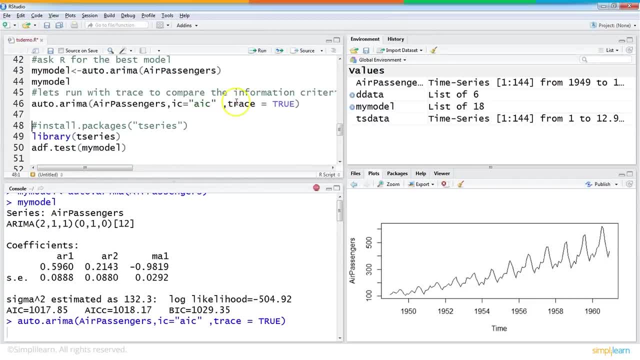 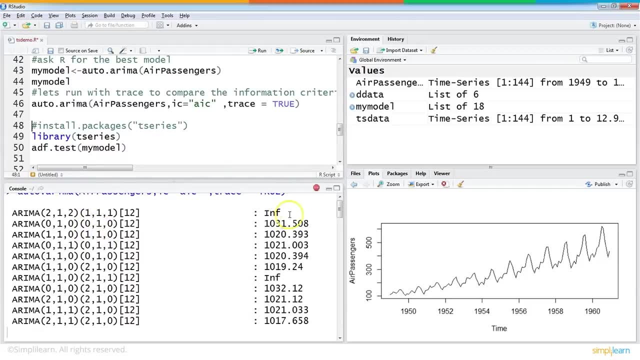 talking so much. let's run this. if we run auto arima with trace, you see here there is a red mark here that means it is performing, it's executing this and here we see the display right. so it starts with certain values of pdq and then it finds that value is too high. 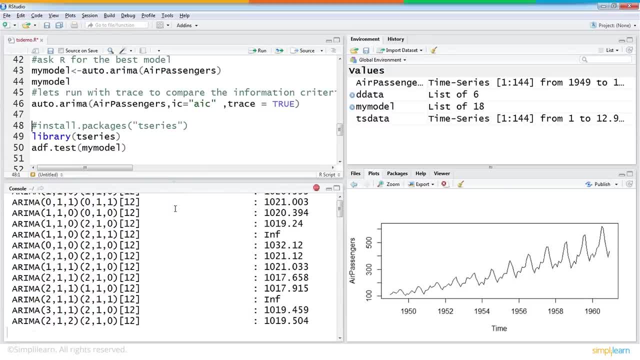 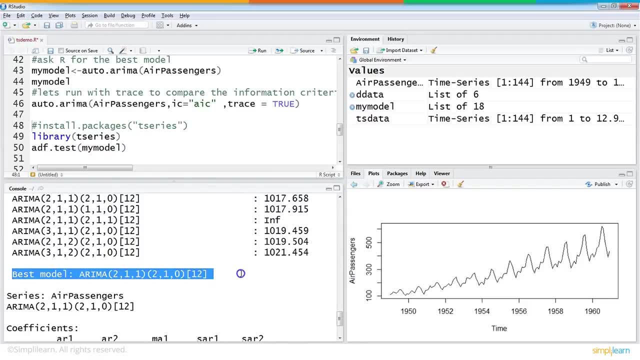 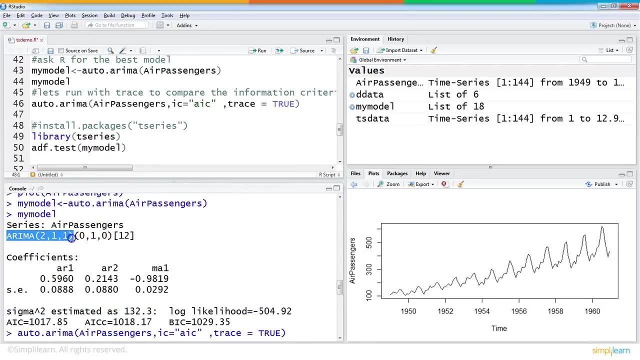 so it starts with again with some 010 and so on and so forth, and ultimately it tells us: okay, this is our best model. you see, here it says: this is our best model. 211. let's go back and see, did we get the same one? yes, we got the same one when we ran without trace as well. right now, why is 211? let us see where is 211. here is our 211, back here, and so on. well, we run our trace as well, and when? yes, we got the same one when we ran without trace as well. right now, why is 2, 1, 1? let us see where is 211. here is our 211. 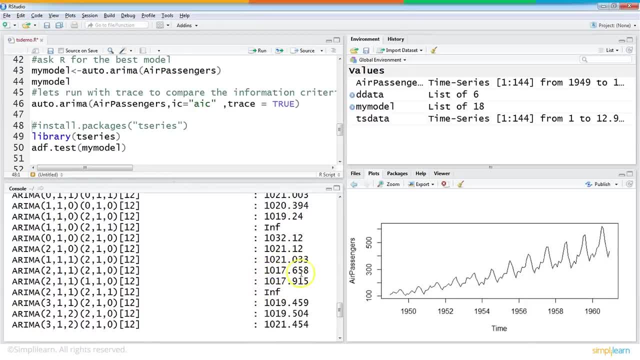 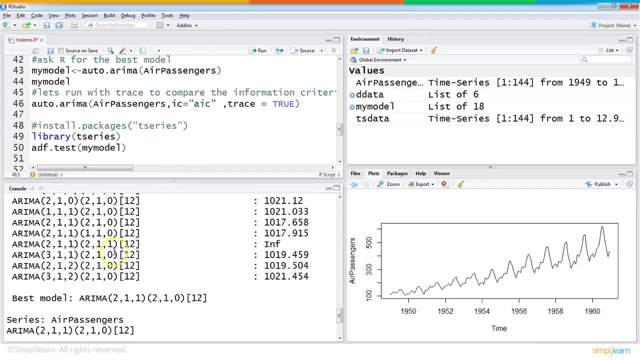 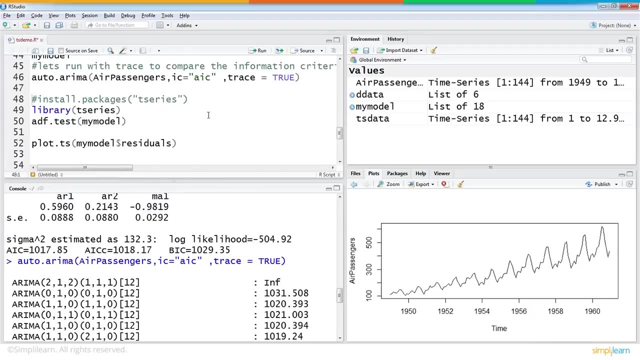 and if you compare the values, you see that 1017 is pretty much the lowest value and therefore it is saying: this is our best model. all other values are higher. so that's how you kind of get your model. and now that you have your model, what you have to do? you need to predict the values, right? 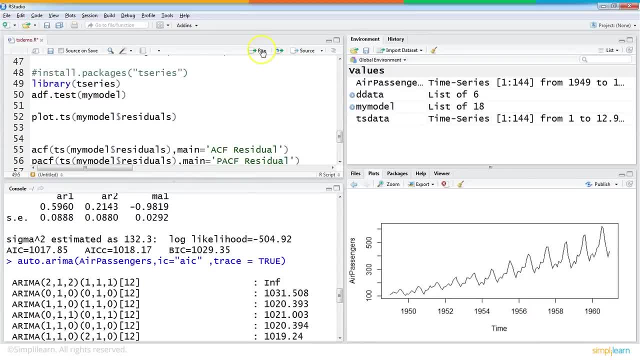 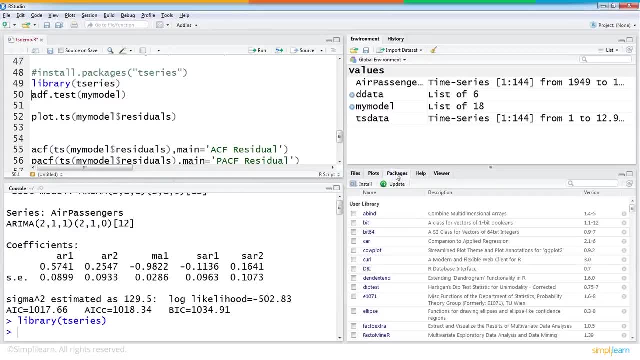 so before that, let us just do some test of these values. so for that you install t-series again. if you are doing it for the first time, you would rather use this package and install and say t-series and install it, and then you just use this library function to load it into your memory. 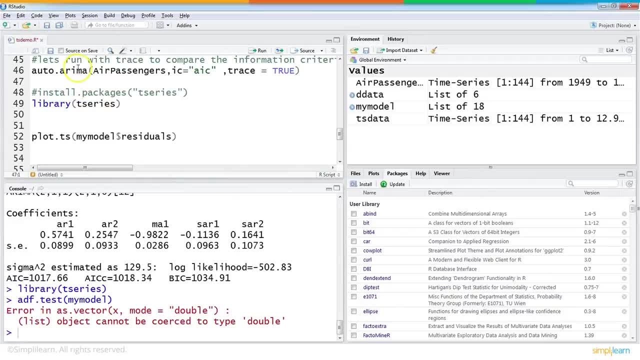 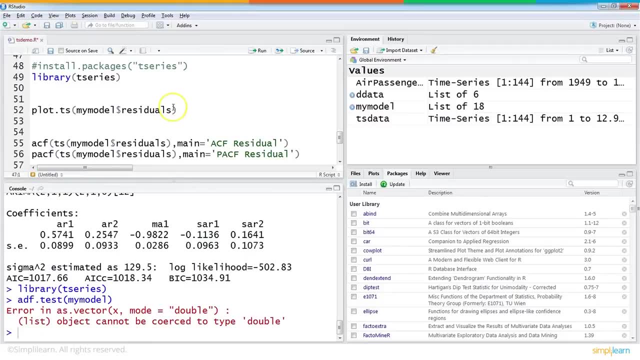 all right. so now that we got our model using auto-arima, let us go ahead and forecast and also test the model and also plot the acf and psef. remember we talked about this, but we did not really use it. we don't have to use that, but at least we will visualize it and 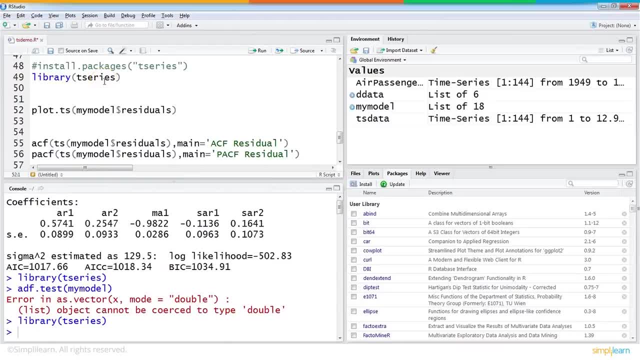 first of all, we're going to do a test of this model and we're going to do a breath test of this model. stick and plot the cf and pscf. remember we talked about this but we did not really use it. we don't some of the stuff we may need, this t-series library. so if you are doing this for the first, 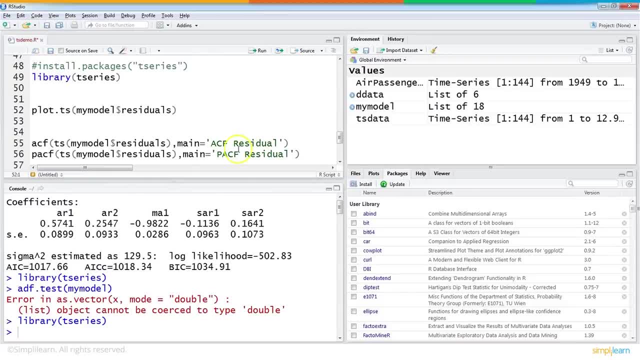 time you may have to install it, and my recommendation is: don't use it in the code. you go here and install t-series- and i will not do it now because i have already installed it. but this is a preferred method and once you install it, you just load it using this library. 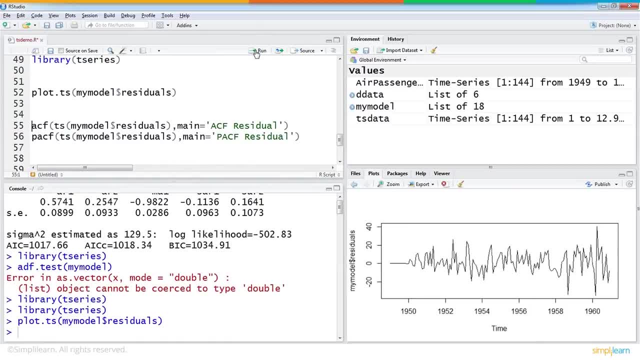 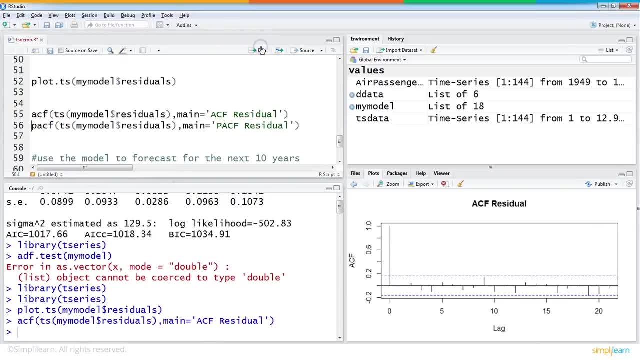 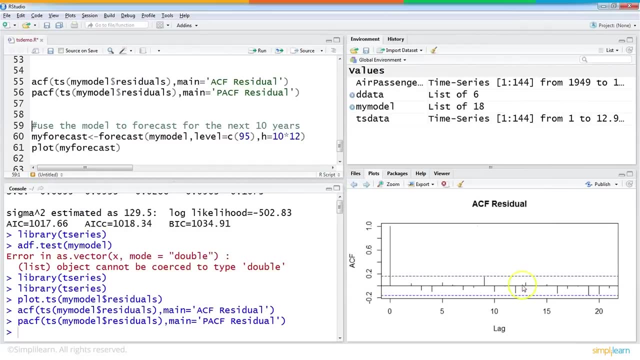 cell function, and then you can plot your residuals. and this is how the residuals look, and you can plot your acf and pscf. okay, so this is how your pscf looks and this is how your acf looks. for now there is really nothing else. we need to do with acf and pscf. this is just to visualize. 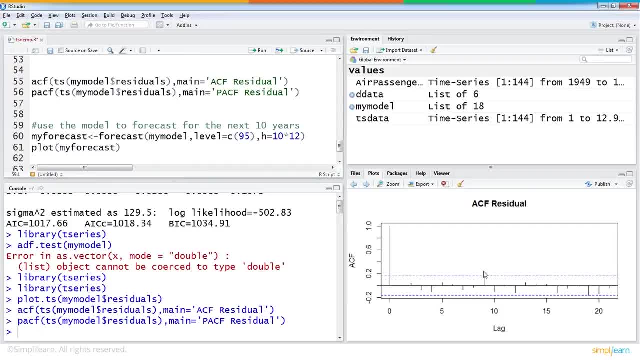 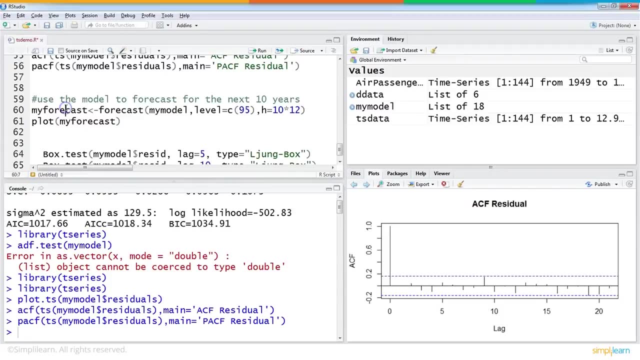 how that, how it looks, but, as i mentioned earlier, we were actually using these visualizations, or these graphs to identify the values of p, d and q, and how that was done. it's uh, out of scope, obviously, this video, so we will leave it at that, and then we will forecast for the next 10 years. how do we? 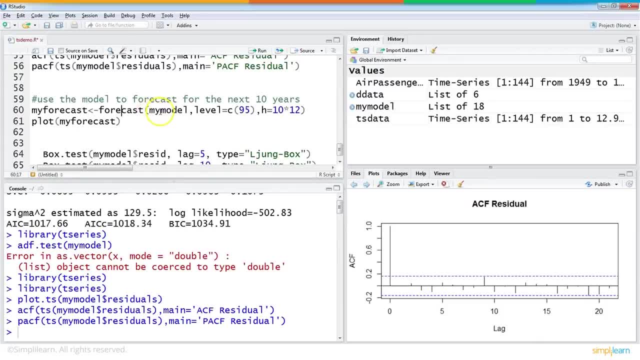 focus that. so we call forecast and we pass the model and we pass what is the level of accuracy that you need, which is 95, and for how many periods? right? so basically, we want for 10 years, which is like 10 into 12 time periods. so that's what we are doing here and now we can plot the forecast value. 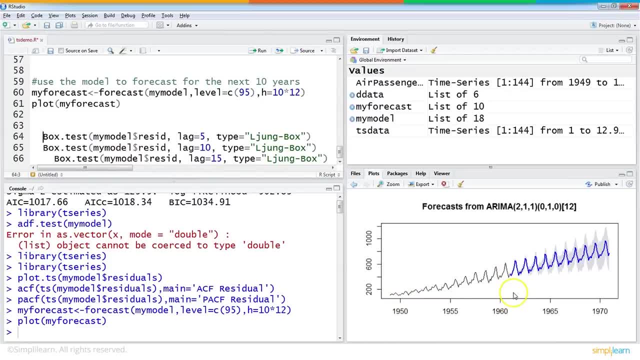 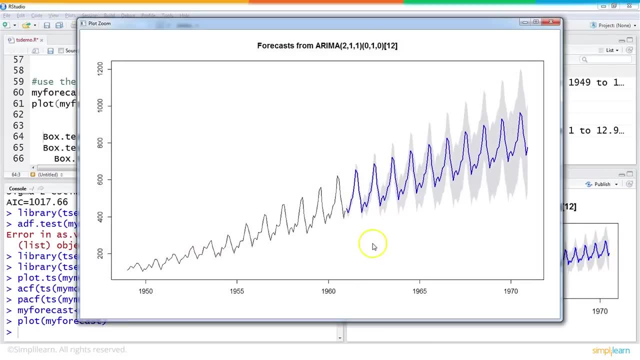 so you can see this is the original value up to, i think, 62 or whatever, and then it goes up to 72.. this blue color is the predicted value. let's go and zoom it up so that we can see it better. so up from here onwards, you're forecasting and you can see that it looks like our model has kind of learned. 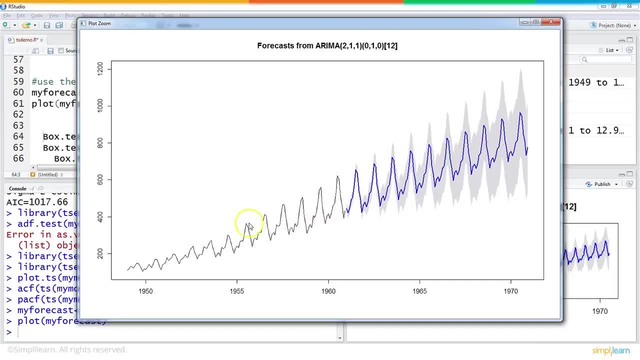 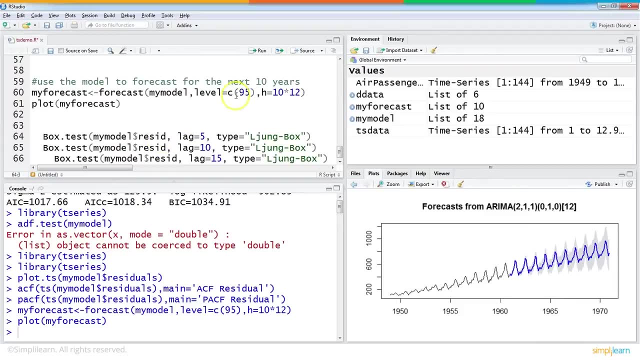 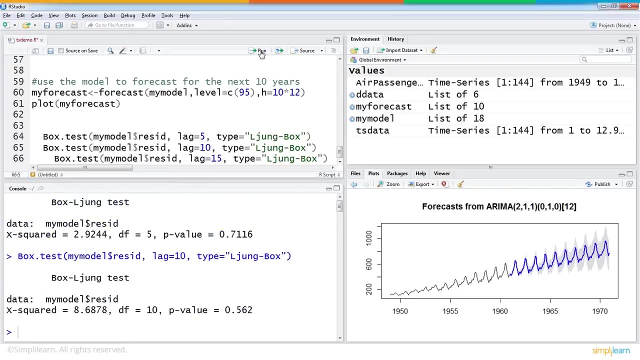 the pattern and this pattern looks very similar to what we see in the actual data. now, how do we test model? so we can do what is known as a box test and we pass our model here, residuals, basically with different lags, and from those values, here the p-values. 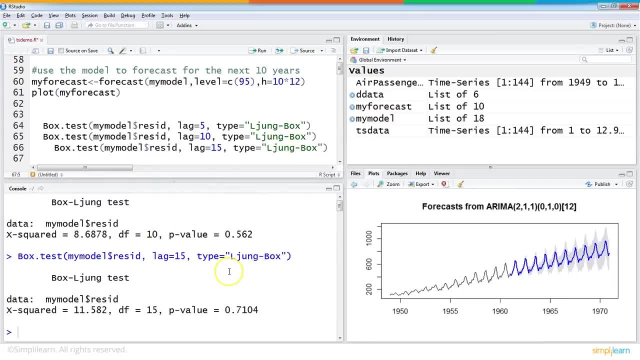 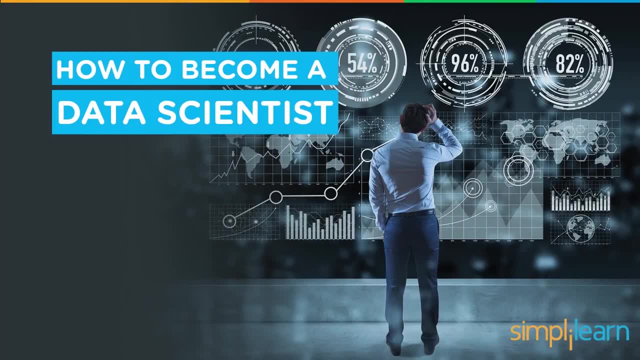 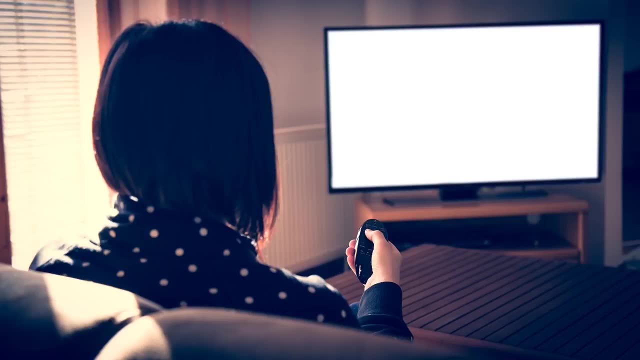 here we find that they are reasonably low p-values, which means our model is fairly accurate. hi guys, I'm Rahul from simply learn, and today I'm going to tell you how you can become a successful data scientist. now, before I begin, let me give you an example. share at home and you board and you feel like watching a TV. 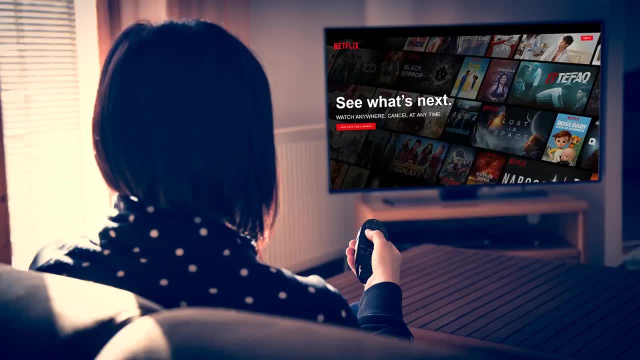 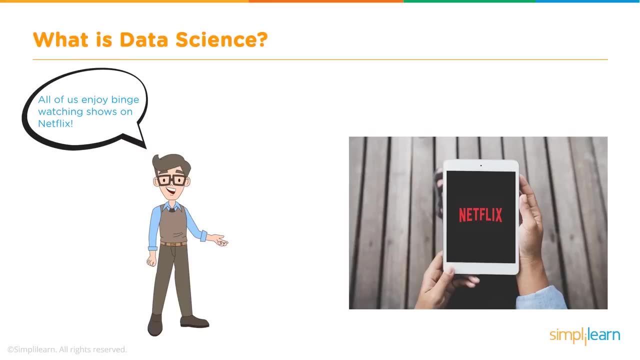 show or a movie. then you get on Netflix. you scroll through all the TV shows and movies that they offer. then you're recommended the latest season of Deadpool because you've seen shows similar. we all enjoy building shows on Netflix, but do you actually know how much of data science is used along with Netflix? 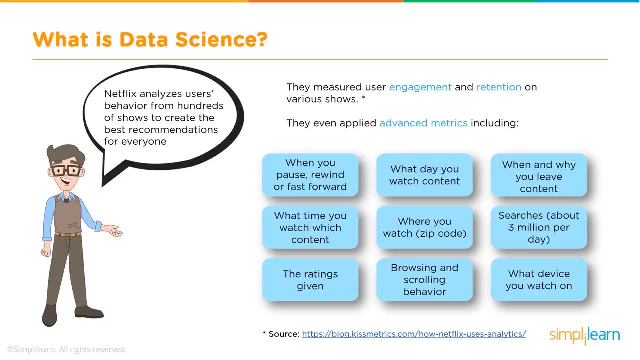 Netflix analyzes the users behavior from hundreds of different TV shows and movies to create the best recommendations for everyone. they measure user engagement and retention on various shows. now currently, they're even applying advanced metrics that include when you pause, rewind or fast-forward- that's when you see something really cool and 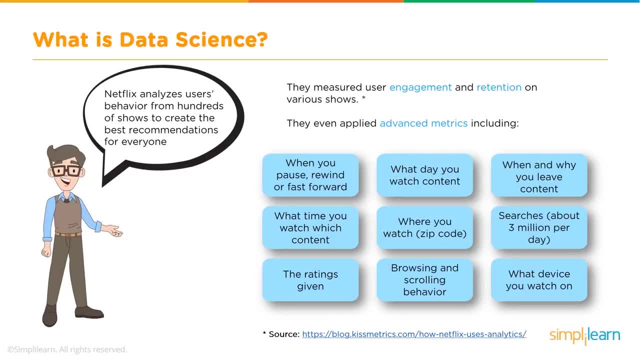 you want to watch it again. what do you watch? the content. for example, some days you feel like watching a comedy show, or sometimes drama and so on. when and why you leave the content when you stop watching a show? why did you start? what time you watch? which content children tend to watch in the morning and adults 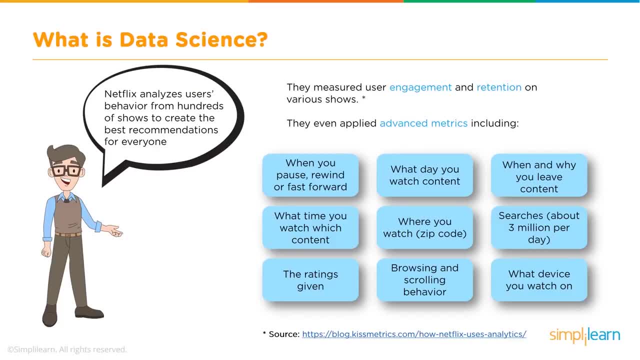 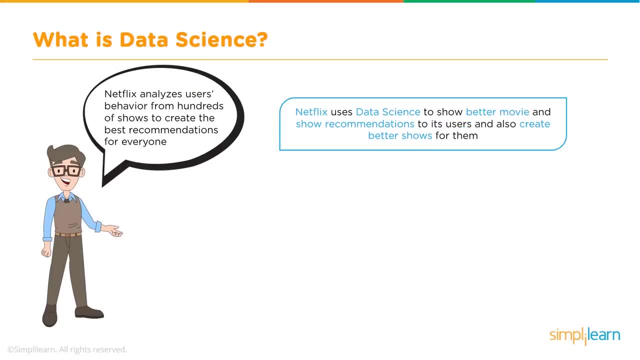 when they return from work, from where you watch in the world, searches for the show, the ratings given, browsing and scrolling behavior, and what device you watch. the program on Netflix uses data science to show better movie and show recommendations. They say they are creating better shows for the users. 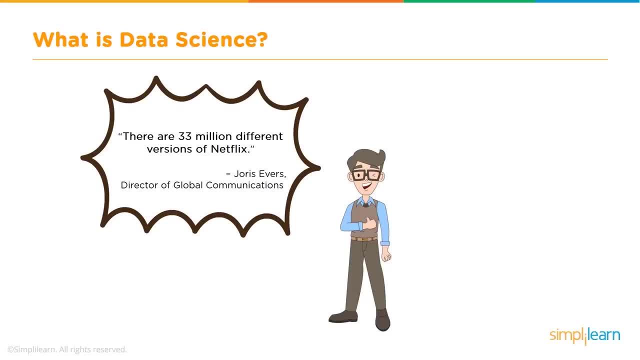 There are 33 million different versions of Netflix, says Joris Evers, who is the director of Global Communications. Netflix at the moment has more than 125 million users worldwide, which means, on an average, only 4 people get the same iteration of Netflix. This is because of all the personalization that is done to suit the user's needs. 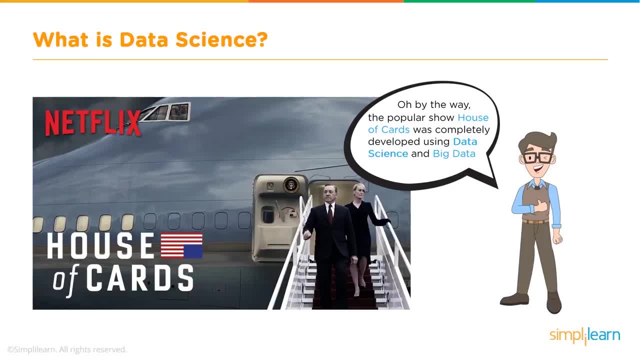 Oh, did you also know that the popular show House of Cards was created completely using data science and big data? This was using the advanced metrics that I mentioned earlier. Netflix collected user data from another show called the West Wing. From this, they took into consideration where people rewound a particular scene when they 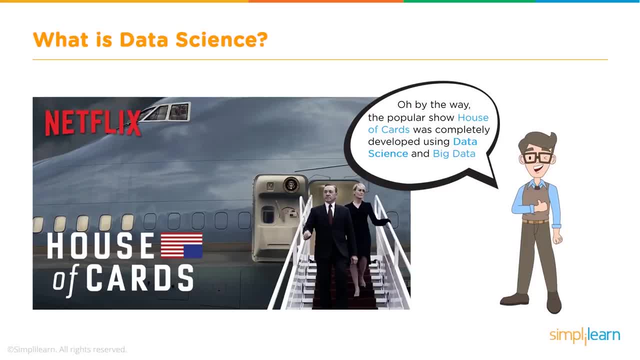 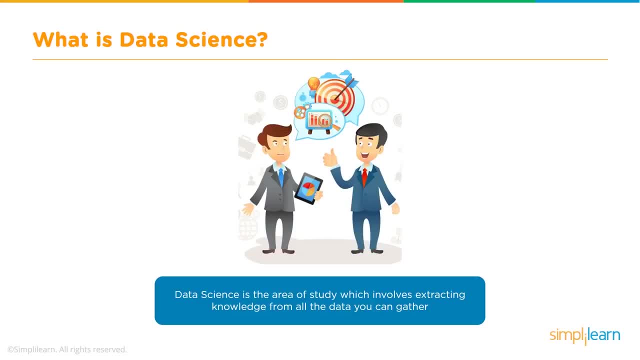 fast forwarded and when they stopped watching the show. With this, they were able to create what they believed was a perfectly engrossing show. Data science is the area of study which involves extracting knowledge from all the data that you can gather. Now that you understood what data science is, let's talk about what a data scientist 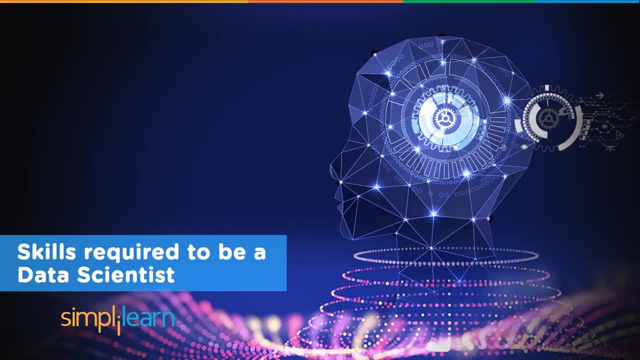 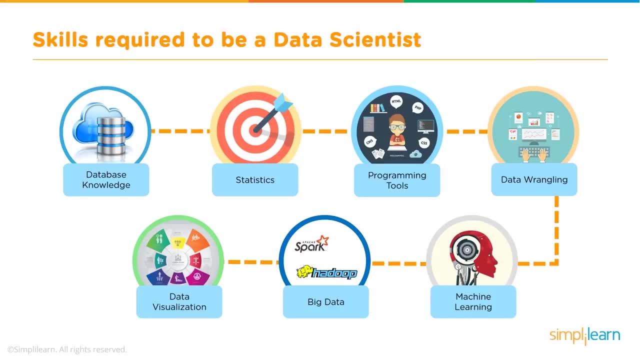 does. We'll go through all the skills that are required by a data scientist. A data scientist needs to have the following 7 skills: Database Knowledge, Statistics, Programming Tools, Data Wrangling, Machine Learning, Big Data and Data Visualization. Let's go one by one. 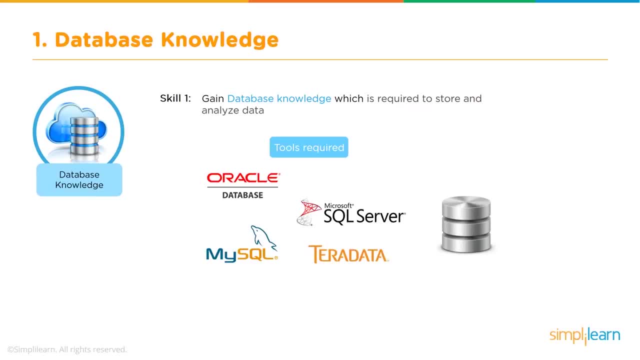 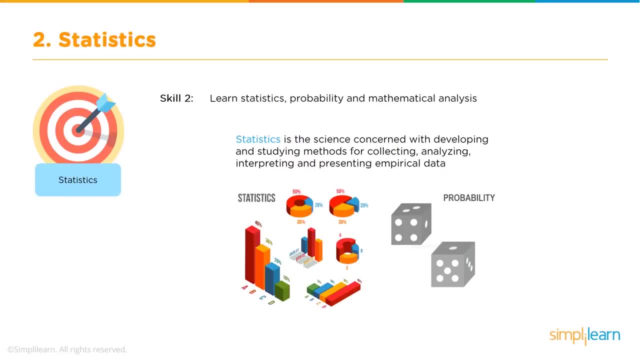 Skill 1. Database Knowledge: Gaining database knowledge is required to store and analyze data. Oracle Database, SQL Server, MySQL and Teradata are some of the tools that are required for this Skill 2. Statistics: Learning, Statistics, Probability and Mathematical Analysis. 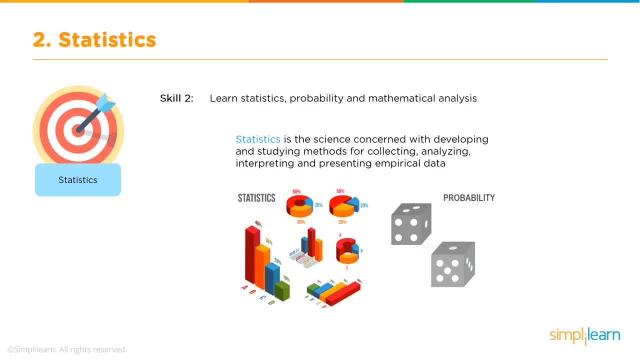 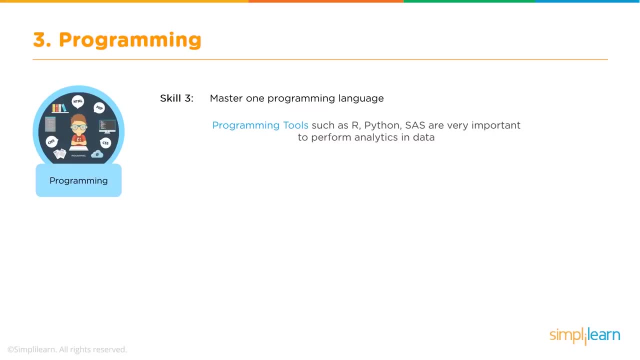 Statistics is the science concerned with developing and studying methods for collecting, analyzing, interpreting and presenting empirical data. Skill 3. Programming: Mastering one programming language. Programming tools such as R, Python and SAS are very important to perform analytics in data. 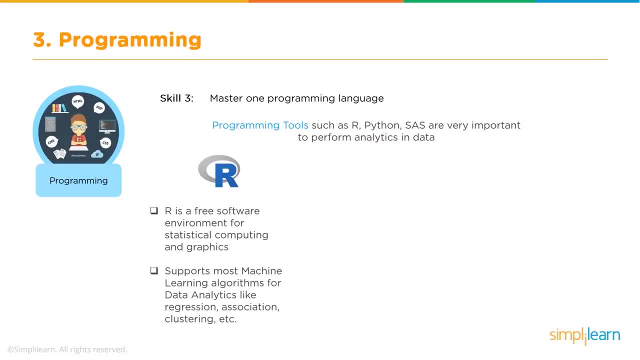 R is a free software environment for statistical computing and graphics. It supports most machine learning algorithms for data analytics like regression, association, clustering and so on. Python is an open source general purpose programming language, and libraries such as NumPy and SciPy are used in data science. 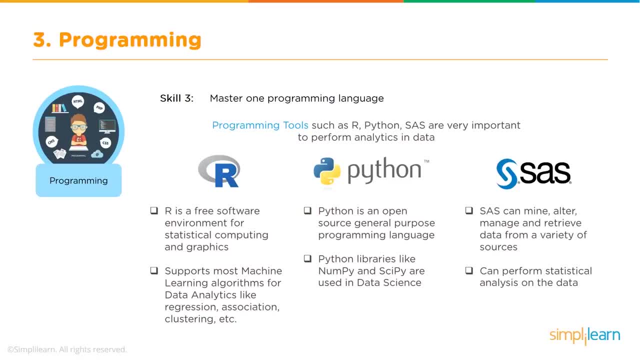 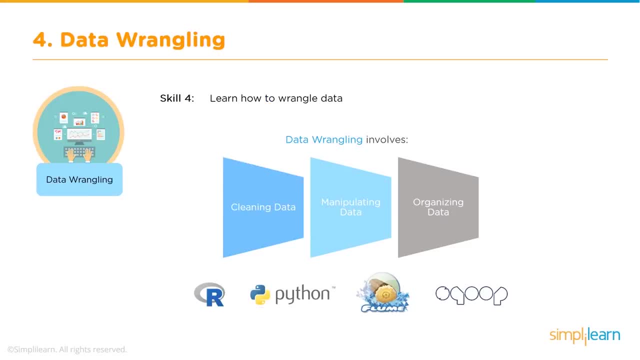 SAS can mine, alter, manage and retrieve data from a variety of sources. It can also perform statistical analysis on the data. Skill 3.: Data Wrangling- Learning how to wrangle data. Data wrangling involves cleaning data, manipulating data and organizing the data. 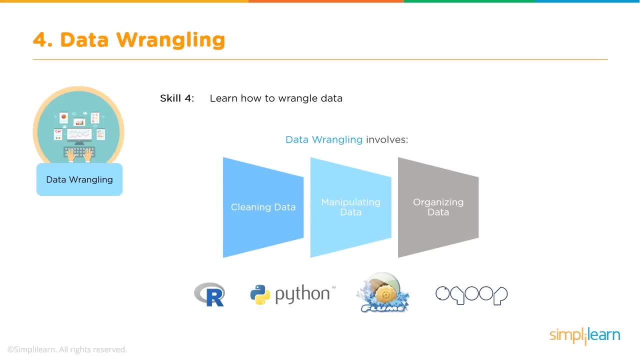 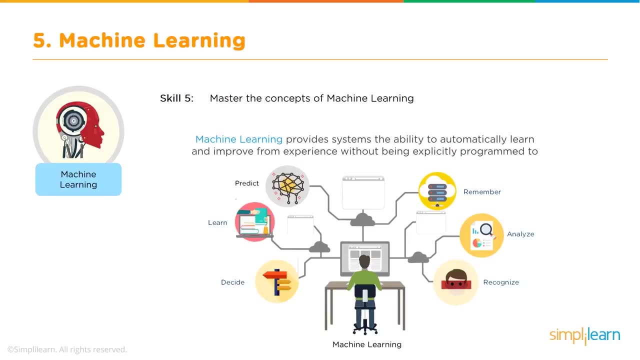 Some of the tools that are used are R, Python, Flume and Scoop Skill 5. Machine Learning: To master the concepts of machine learning, Machine learning provides systems the ability to automatically learn and improve with experience, without being actually programmed to do that. 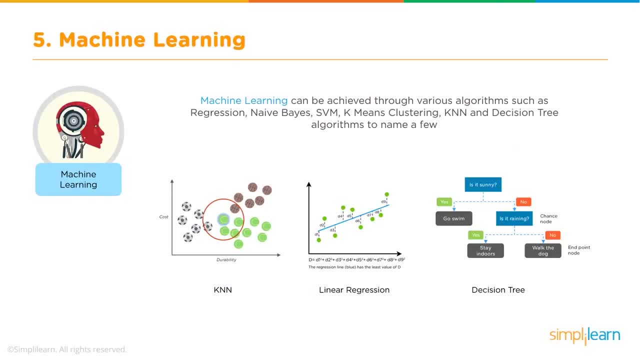 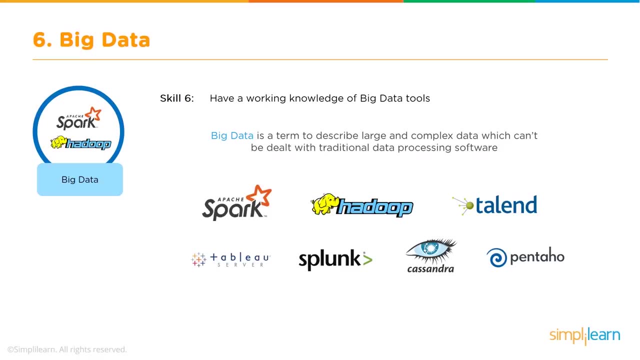 Machine learning can be achieved through a number of different algorithms like Regression, NaiveBase, SVM, K-Means, Clustering, KNN, Decision Tree, just to name a few. Skill 6. Big Data: Having working knowledge of big data tools. 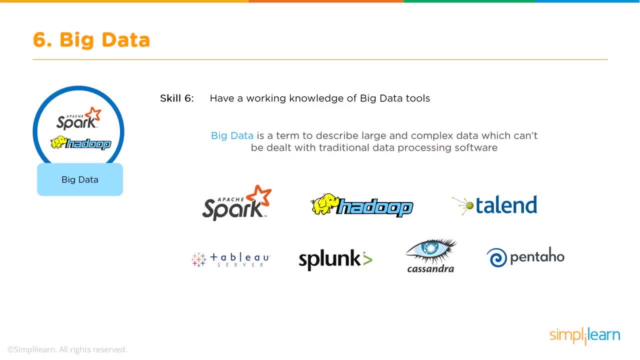 Big data is a term that is used to describe large and complex data that cannot be dealt with with traditional data processing software. Some of the tools that are used, or softwares that are used, are Apache, Spark, Hadoop, Talent Tableau, Splunk, and so on. 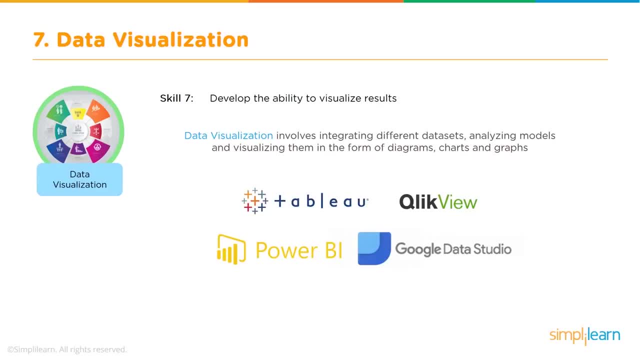 Number 7. Data Visualization: To develop the ability to visualize results, Data visualization involves integrating different data sets, analyzing models and visualizing them in the form of diagrams, charts and graphs. Some of the tools or softwares that are used are Tableau, K-Means and Scope. 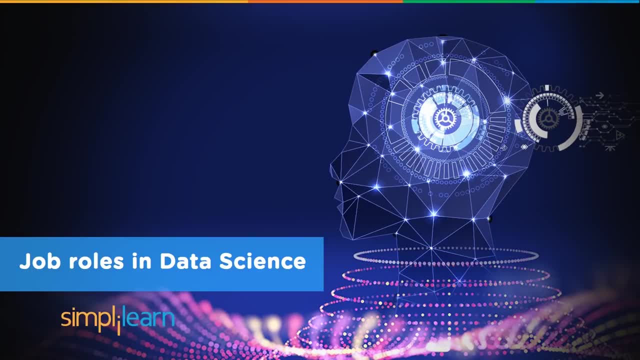 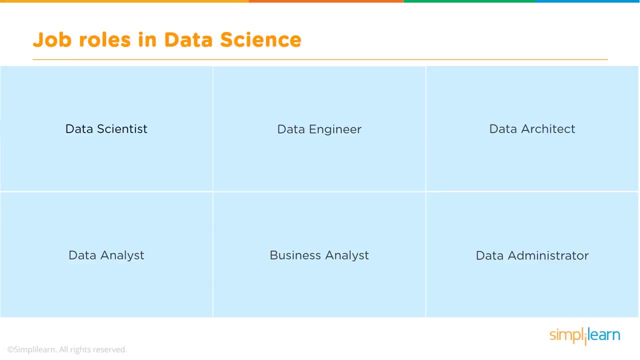 Most are Tableau, Clickview, Power BI and Google Data Studio. Let's talk about some of the job roles in data science. We have Data Scientist, Data Engineer, Data Architect, Data Analyst, Business Analyst and Data Administrator. Let's go one by one. 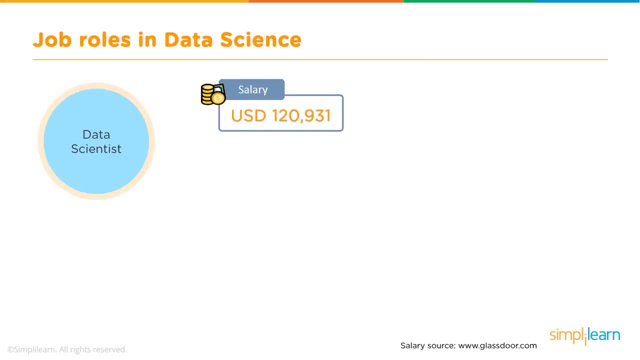 Data Scientist. A data scientist earns around $120,000 per year and these are their responsibilities: To create data-driven business solutions and analytics, drive optimization and improvement of product development. To use predictive modeling to increase and optimize customer experience- revenue generation. 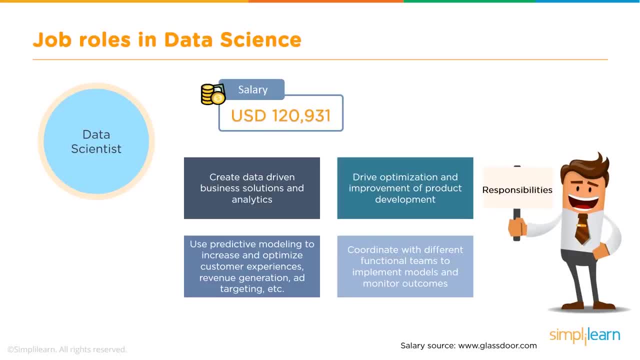 targeting and so on. A data scientist is responsible for coordinating with different functional teams to implement models and monitor their outcomes. Data Engineer- A data engineer earns around $130,000 per year. Some of the responsibilities are assembling large, complex data sets to identify design. 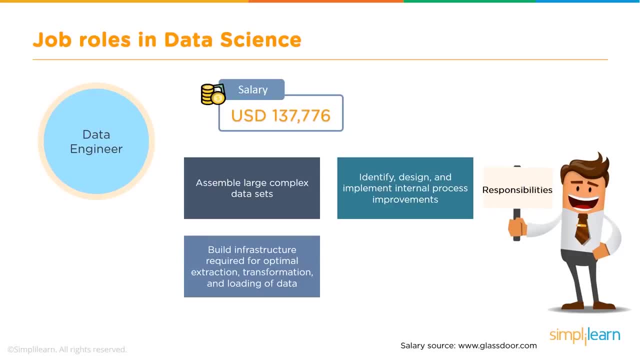 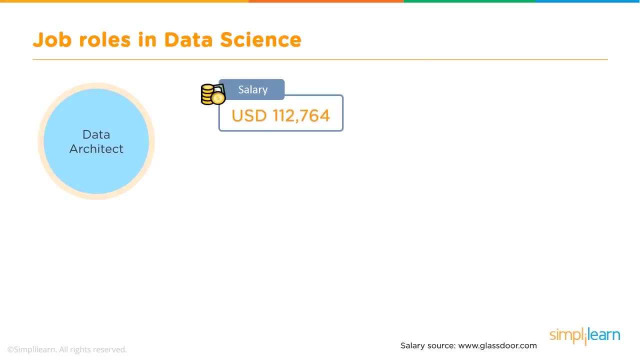 and implement internal process improvements. to build infrastructure required for optimal extraction, transformation and loading of data. to build analytics tools that utilize the data pipeline. Data Architect- A data architect earns around $112,000 per year and these are their responsibilities: To develop database solutions. 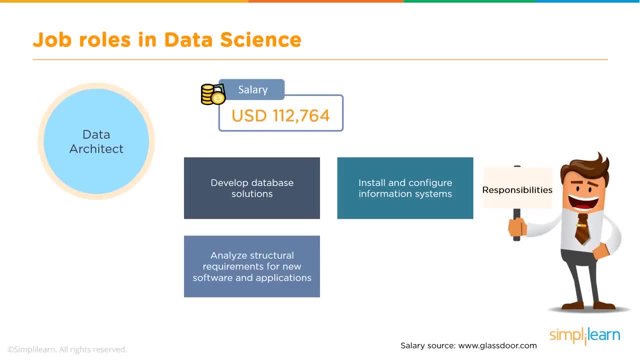 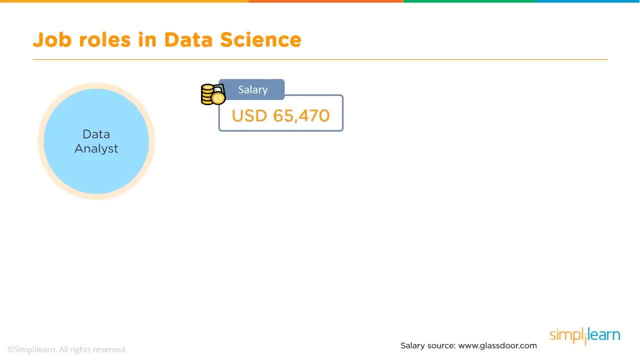 To install and configure data. To create and manage data. To configure information systems. To analyze structural requirements for new software and applications. To migrate data from legacy systems to new solutions. Data Analyst- A data analyst earns around $65,000 per year and these are their responsibilities. 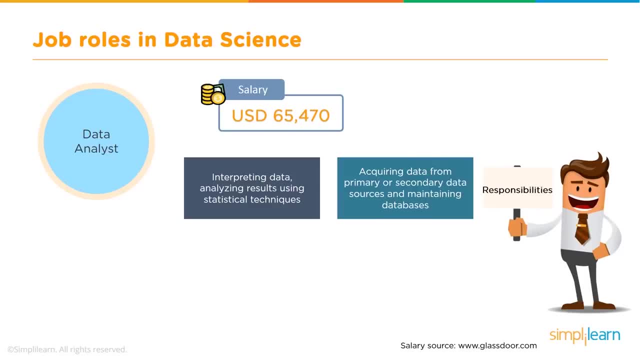 To interpret data and analyze results, using statistical techniques. To acquire data from primary or secondary data sources. and maintaining databases. To develop and maintain data analyses, data collection systems and other strategies. working with management to prioritize business and information needs. Business Analyst. A business analyst earns around $70,000 per year and these are their responsibilities. 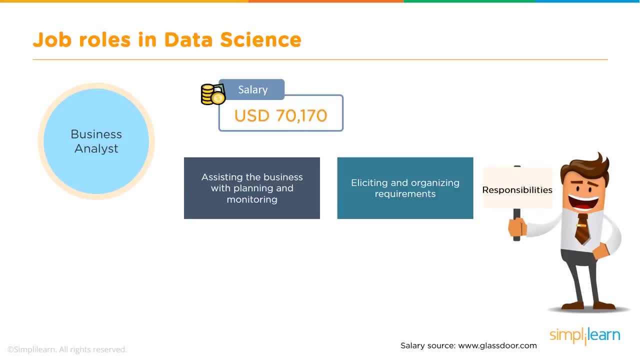 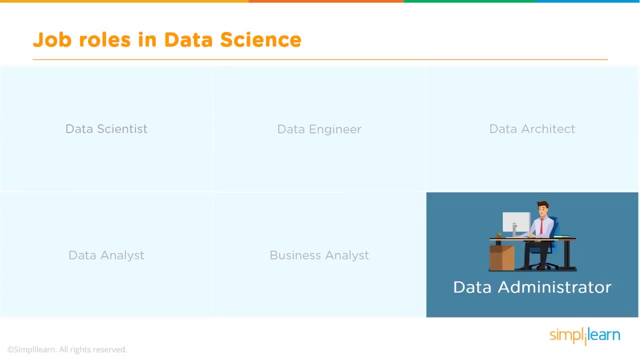 To assist the business with planning and monitoring, eliciting and organizing requirements, validating the resource requirements and developing cost estimate models. creating informative, actionable and repeatable reporting. Data Administrator. A data administrator earns around $54,000 per year, and these are their responsibilities. 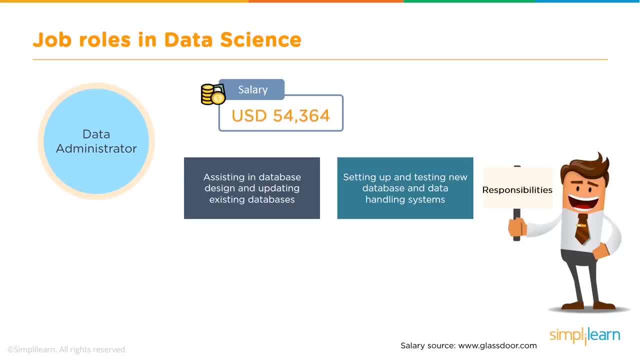 Assisting in database design and updating existing databases, setting up and testing new database and data handling systems, sustaining the security and integrity of data and creating complex security systems. A data analyst must be good at data engineering and software design and software infrastructure, as well as runningands. in addition to the Virtual reality, milligram systems and the 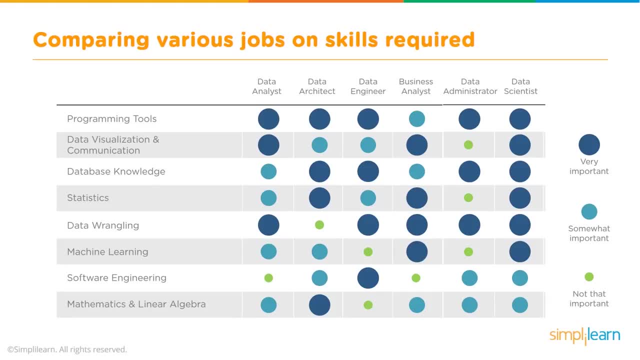 security of the database and each one of its own data. To be a data analyst, you need to be very understanding of databases and its code of Play, as these are the very parameters that allow data to be extracted. Let's talk about skills required for the job. 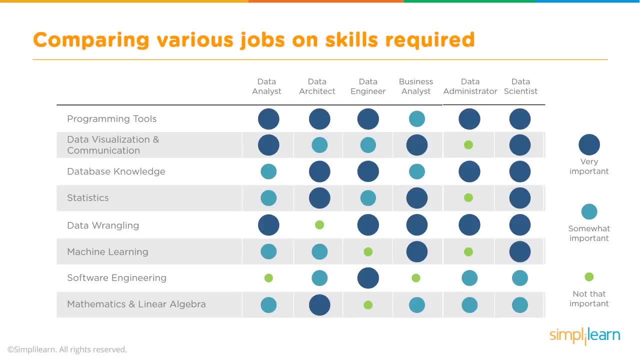 It is very important that a data analyst has a sound knowledge in programming tools, data visualization and communication and data wrangling. A data architect needs to know a lot about programming tools, database knowledge, statistics, mathematics and linear algebra. A data engineer must be good with programming tools, database knowledge, data wrangling. 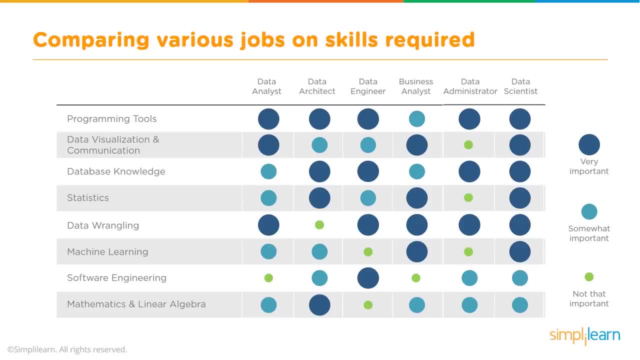 and software engineering. A business analyst needs to be good at data visualization and communication, statistics, data wrangling and machine learning. data needs to be good with programming tools, database knowledge and data wrangling. now, however, data scientist needs to be good at programming tools, data visualization, database knowledge. 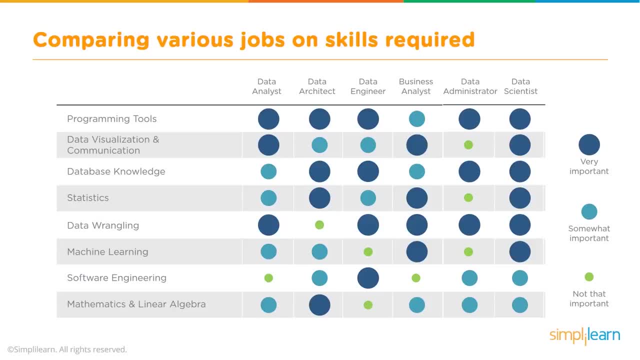 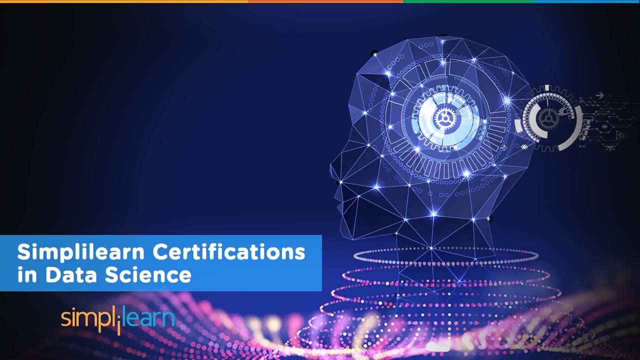 statistics, data wrangling and machine learning. they also need to know a good amount of knowledge on software engineering, mathematics and linear algebra, which means you basically need to know everything about the data. this goes to show that being a data scientist isn't easy, but it also cements why it is one of the most lucrative jobs in data science now. simply learn also provides. 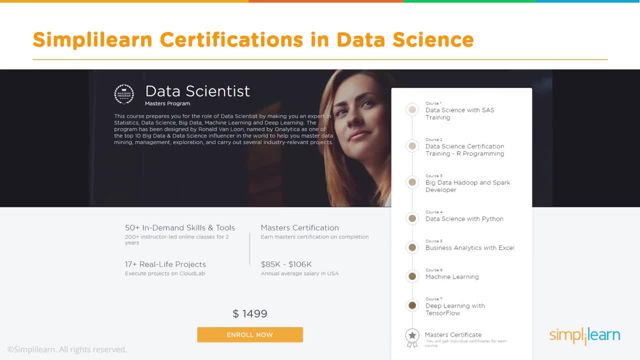 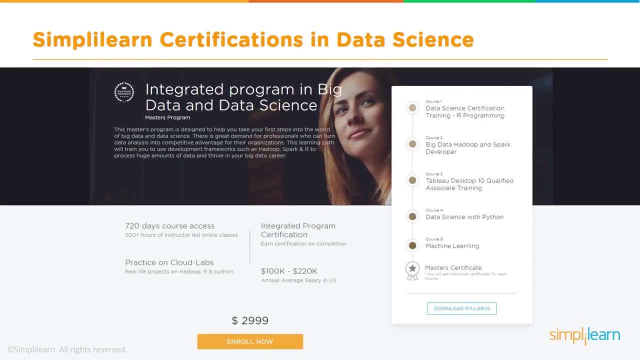 certifications in data science. it provides a data science certification which is a master's program. under this program we have courses in data science with sas training. data science certification training with our programming, big data, hadoop and spark. developer data science with python. business analytics with excel. machine learning, deep learning with tensorflow. we also have an integrated program. 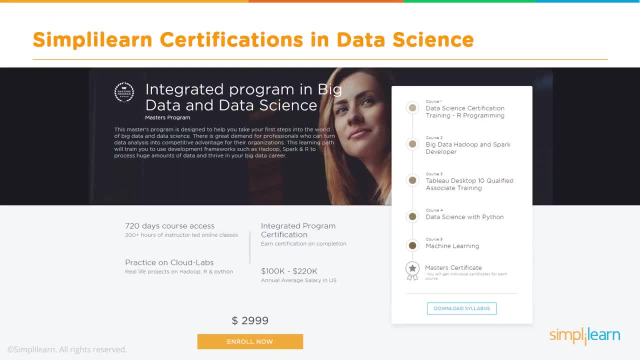 in big data and data science. this is also a master's program. the courses that are covered are: data science certification training with our programming- big data, hadoop and spark. developer tableau desktop 10 qualified associate training, data science with python and machine learning. we also have data science certification courses. 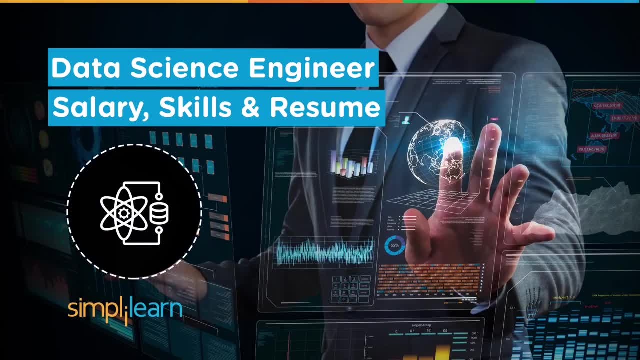 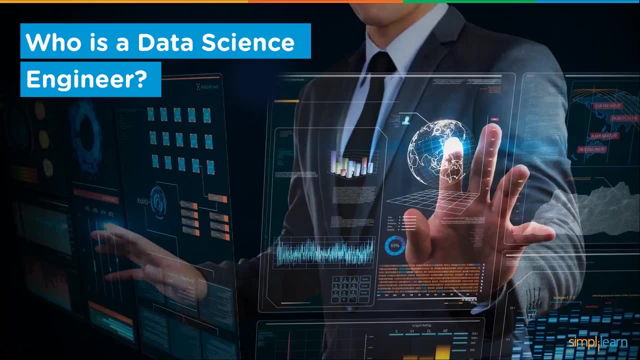 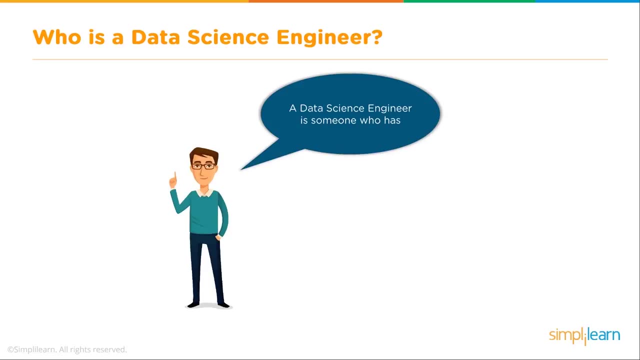 separately in python, r and sas. welcome to data science engineer salary, skills and resume. who is a data science engineer? are you a data science engineer or are you going to be looking for a different field? what exactly is a data science engineer? well, a data science engineer. 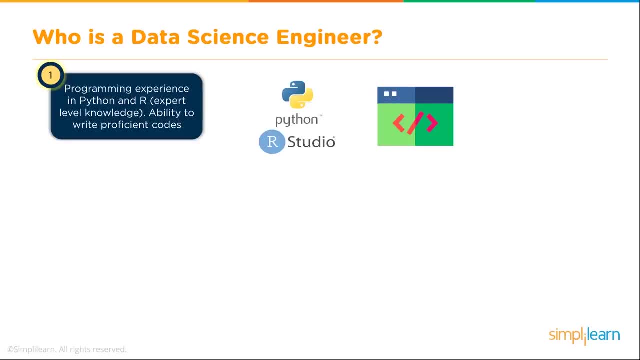 is someone who has programming experience in python and r, expert level knowledge, ability to write proficient code codes, and they we have python and r. i'm going to say python or r. once you become really proficient at one language, transferring those skills into another one is usually fairly easy. now, r is a. 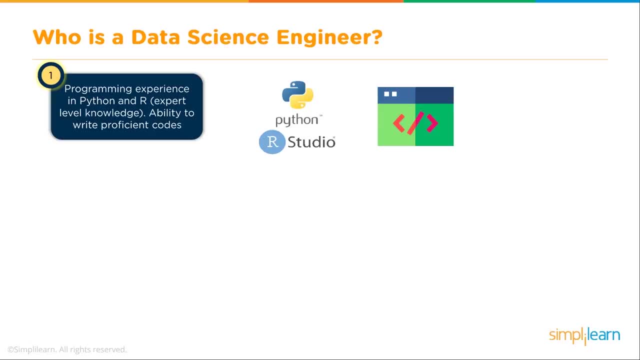 little different because it is an analytics platform. so going from python to r- if you already know the data analytics in python, moving to r is pretty easy. now r doesn't have all the other code that you can access with python. there's so many things you can do with python that that are: 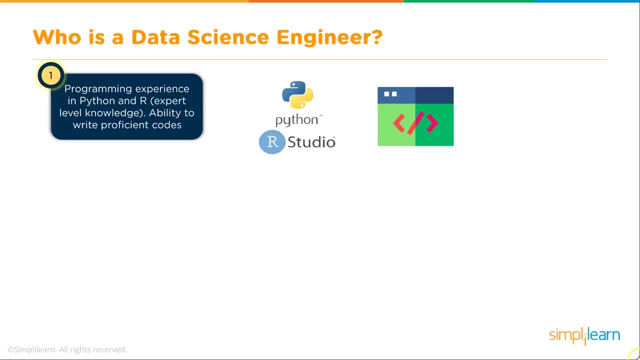 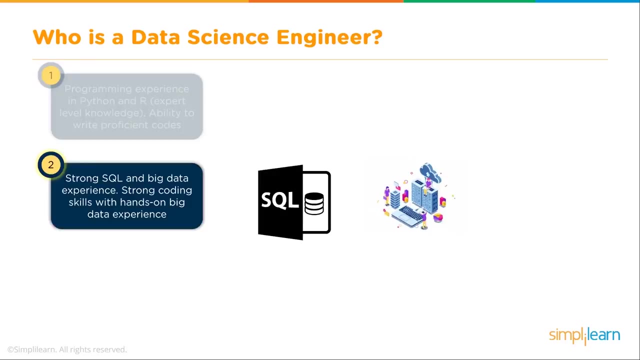 not data analytics. so it's important to keep in mind that you should probably be pretty well rounded in python and really have a solid foundation in r, or have a solid foundation in r and be well rounded in another programming language where you really get the programming side of it, strong sql and big data experience. so you have to have a strong coding skill with hands. 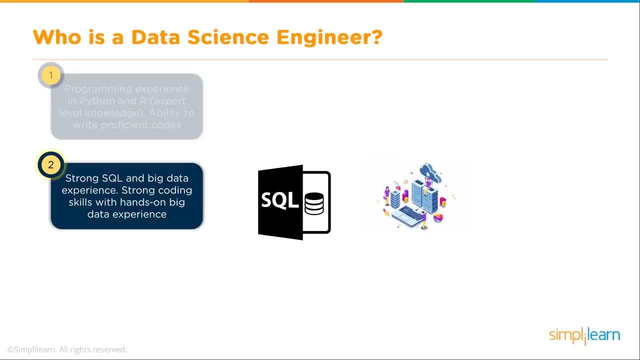 on big data experience and of course, we're showing sql here, most commonly used. whether you're using a microsoft sql server or mysql server, you're going to want to make sure that you know what you're using and you're going to have a strong coding skill with your sql server so you can also start. 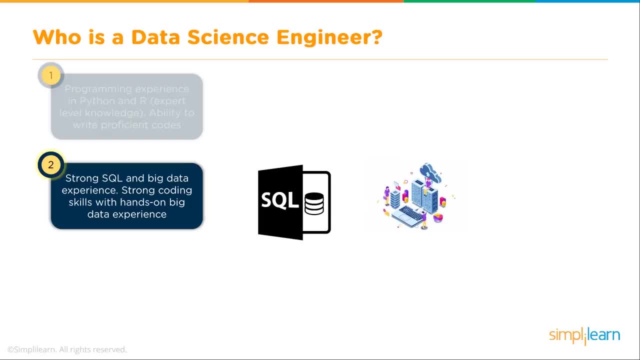 thinking. hadoop and spark and big data access. hadoop file system is not a huge jump if you've already learned your sql and you've already learned your basics and coding. hadoop sits on top of all that and does a wonderful job creating huge clusters of data, but you really need to know. 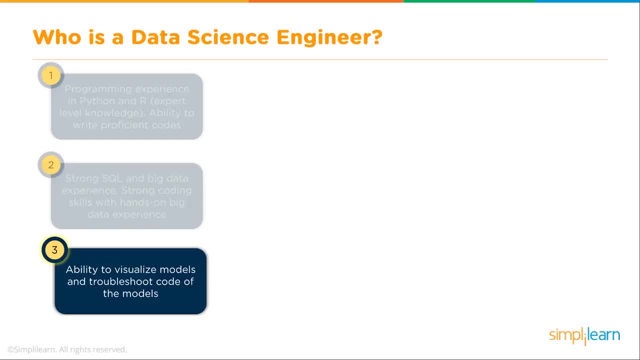 your sql, because that is so common in most of the large companies now accessing their data, and an ability to visualize models and troubleshoot code of the models. this is a kind of an interesting one. these models are can get very complicated, so you get to be able to break them down. 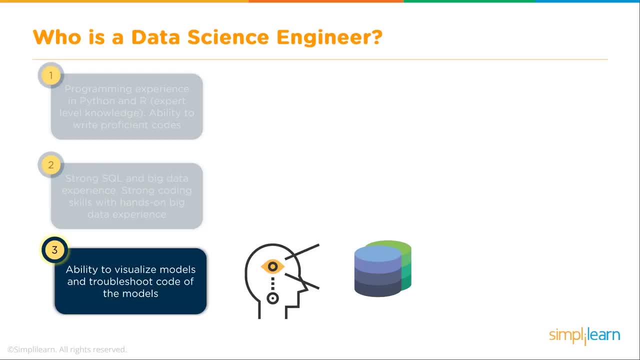 into something that you can put the pieces together and digest each of the pieces. so being able to visualize these models is very important and then being able to drill down and troubleshoot the different models or the pieces in those models. you need to be a versatile problem solver equipped. 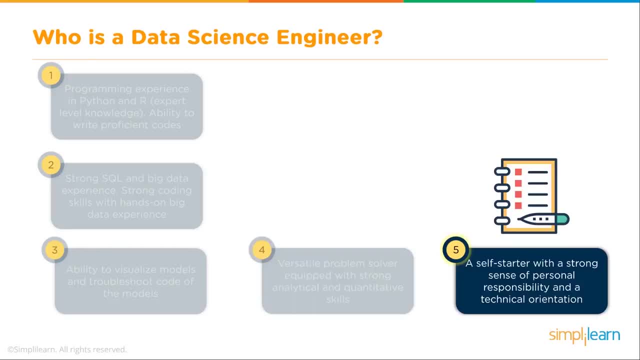 with strong analytical and quantitative skills, a self-starter with a strong sense of personal responsibility and technical orientation. this is an interesting one, because when you talk about data science engineer, it's such a new field that most companies don't have it well defined. they don't know what they're looking for. you might not even know what you're looking for. you might have an. 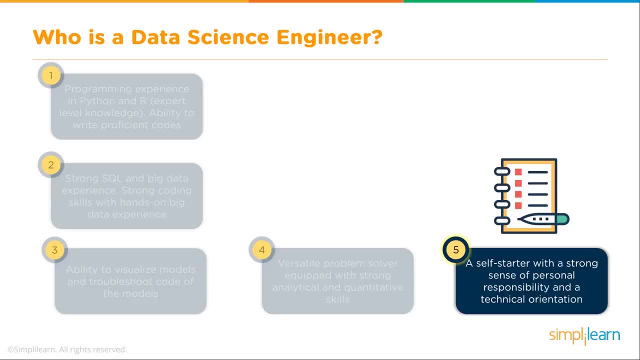 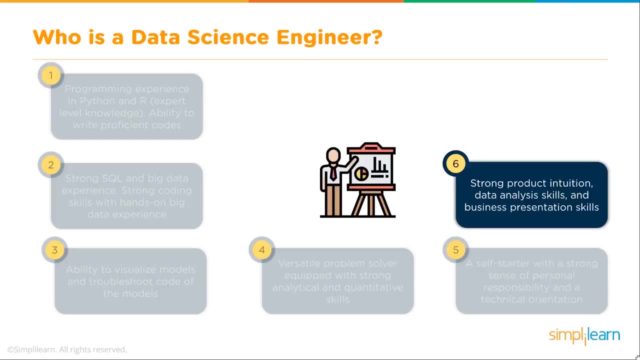 idea and you're looking for patterns, but where do those patterns lead you? so you really need that self-starter side to jump in there and figure out where to go and be able to communicate that back to the team. and there we go. we have a strong product, intuition, data analysis skills and business. 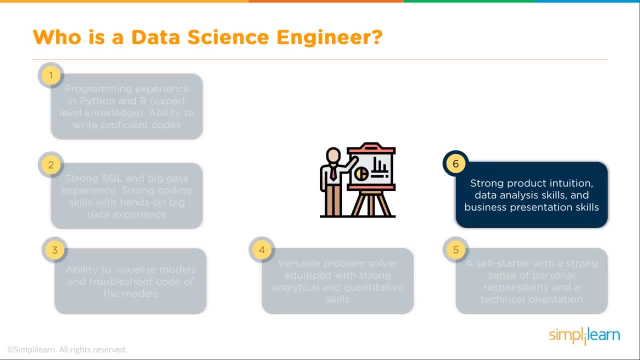 presentation skills, and this is what i was talking about- is you got to bring that back to the team. so if you don't have a strong product intuition, if you don't know what's going on with the company, what they need and where you're going with your analysis, it's going to be a dead end and you got. 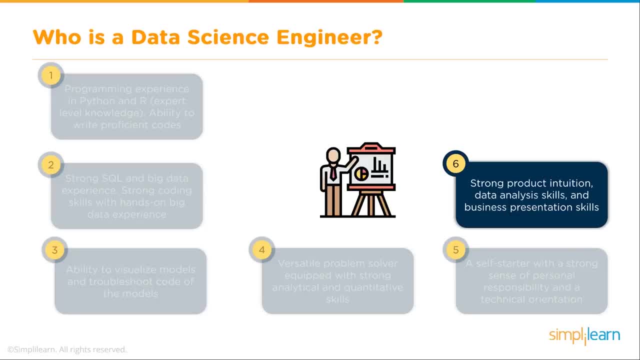 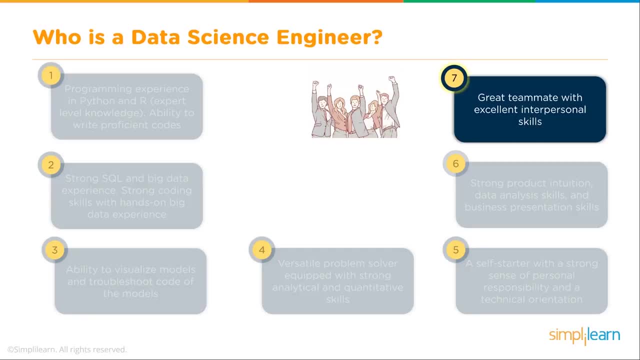 to be able to present that to the shareholders, to your co-workers, which leads us to great teammate with excellent interpersonal skills. and this is kind of a strange one, because you spend so much time behind your desk so you have to be able to kind of float between. you're studying all the data. 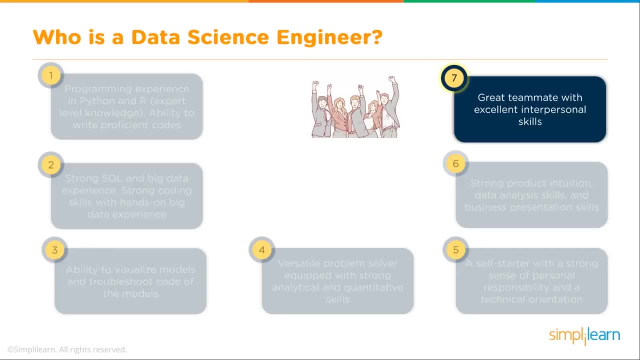 and being able to explain this to people in simple terms that they can understand. no one wants somebody to come up and say, yeah, the peace corps and the f score is this, that and the other thing, and you might have two people in the room. understand you. you have to be able to sit down and explain what that means and why. so let's take a look at. 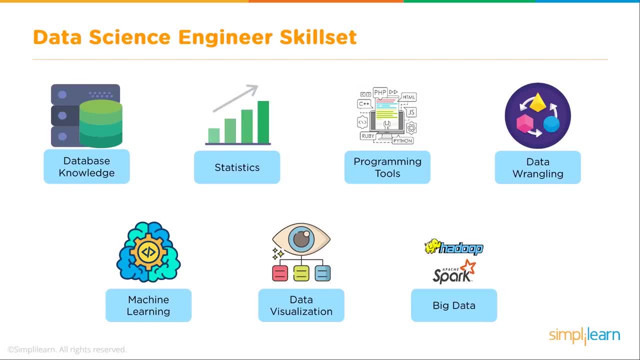 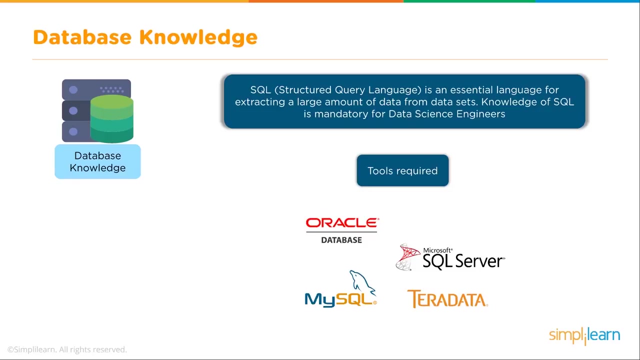 the data science skill set. we talk about data science engineer skill set. we're talking about database knowledge, statistics programming tools, data wrangling- probably the least favorite and most used- machine learning, data visualization and then the touch on big data. and so we'll start with, of course, your sql structured query language, think rows and columns. it's an essential language for 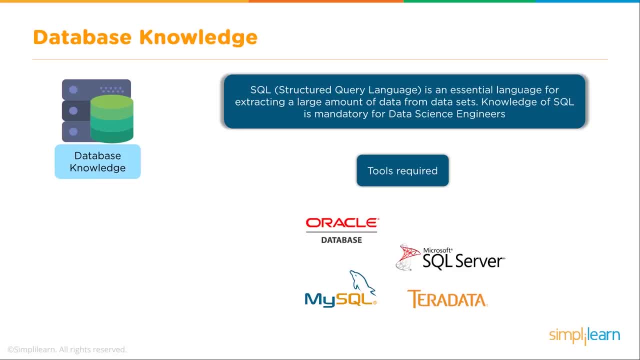 extracting a large amount of data from data sets. so knowledge of the sql is mandatory for data science engineers and you can see there's tools required. there's the oracle database. i mentioned my sql server, microsoft sql server, teradata. there are so many different forms of sql and it'll just 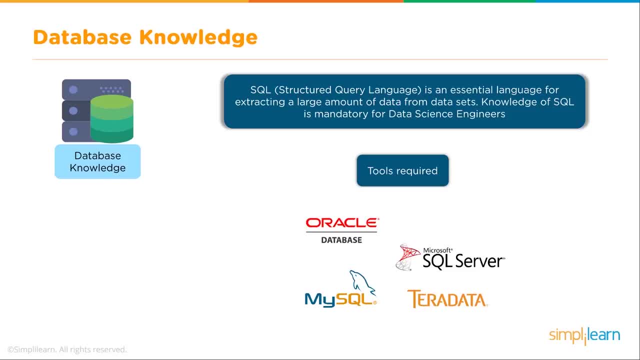 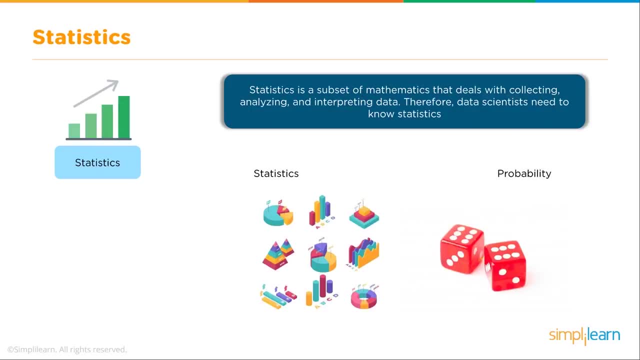 keep coming back and coming back. so if you don't have a solid basic understanding of sql, go get it important because it will come up, you know it's. if you don't know it, it's going to bite you- and statistics of course we are, you know. that's what this is all about is figuring out and predicting. 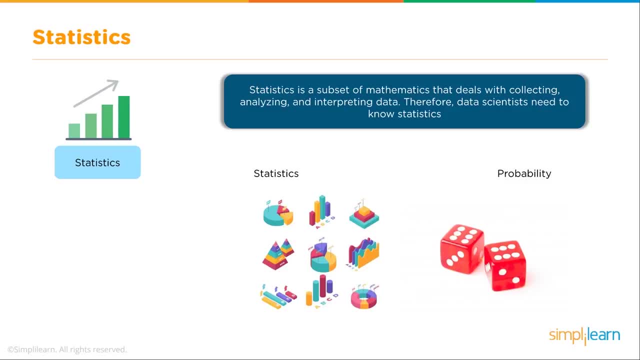 things. so you need to know your statistics. statistics is a subset of mathematics that deals with collecting, analyzing and interpreting data. therefore, data scientists needs to know statistics, so you need to understand your probabilities and what that means and what the p score means in the f score and means and mode and median. all that information, standard deviation, all of those you 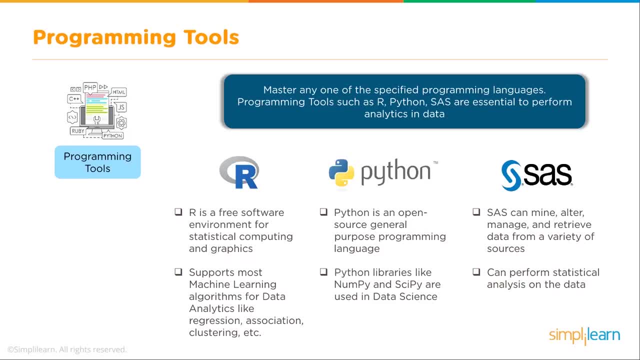 need to be aware of. and then we get into the programming tools, and i mentioned this earlier a little bit, but you need to master any one of these specific programming languages. programming tools such as r, python, sas are essential to perform analytics in data and again, you know you can move in there and you can. 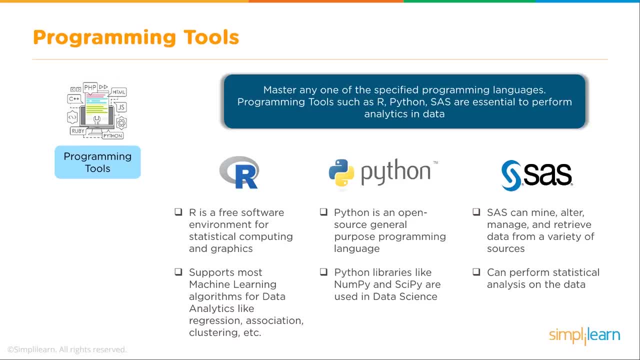 be an expert in gist r, you can be an expert in just sas. in a little bit you can be an expert in python, because most of these, when we're talking about data science and data wrangling, you really kind of get down to the point where you really get to the point where you really get to the point where 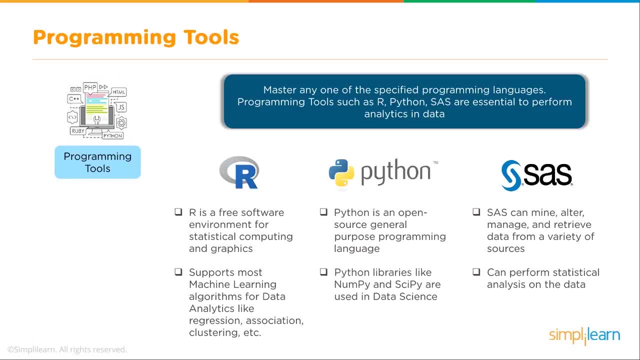 you really need to have a full programming language, at least the basics, and if you're going to be working in data science, python right now is the main one, but you know there's also java, c, plus, plus, so you need to know a solid language, at least the basics of it, so you can understand how to do. 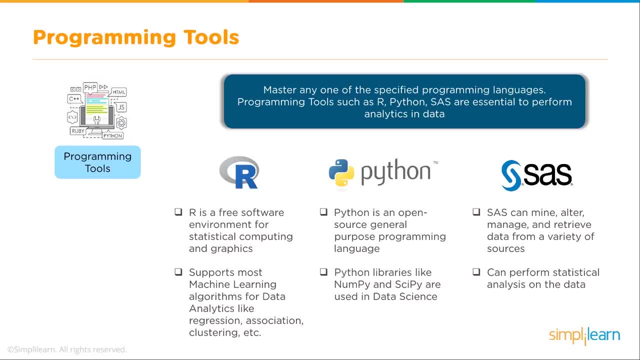 basic iterations and things like that. i always found that interesting that my sister who runs a university data analytics center- that's the first question she asked her people candidate to come and work for her- is: how do you iterate through data? you'd be amazed at how many people 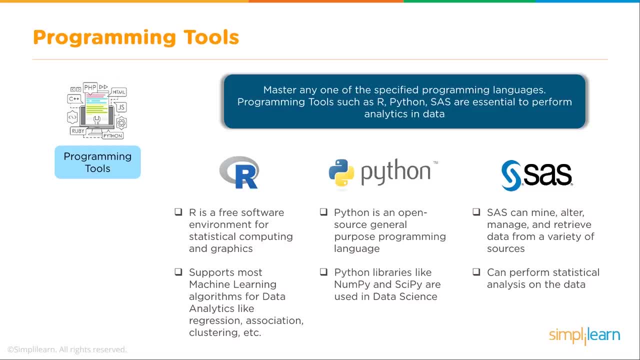 understand that very basic concept in programming. so when we look at r, r is a free software environment for statistical computing and graphs supports most machine learning algorithms for data analytics like regression, association, clustering and etc. python. python is an open source general purpose programming language and there's our general purpose. i was just talking about you. 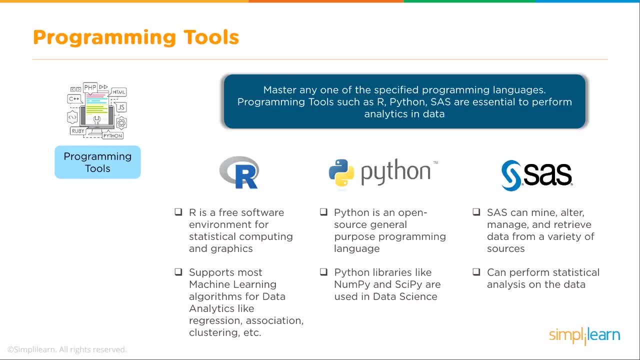 need to know a little bit about python. libraries like numpy and scipy are used in data science. scipy, yeah, numpy and scipy are very central to python and i'd throw pandas in there also that module. those are very central to working with python and data analytics. and then sas, sas. 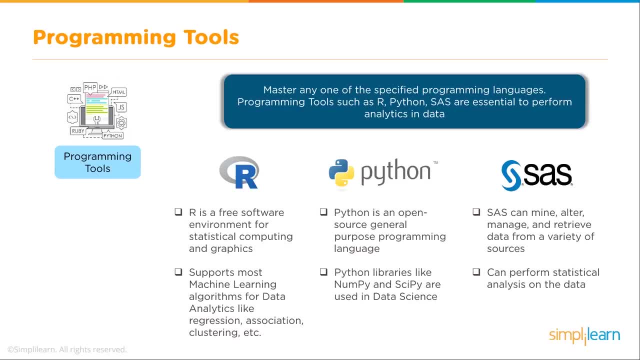 can mine, alter, manage and retrieve data from a variety of sources. it can perform statistical analysis on the data. so where r is the open source platform? sas is more like the paid for platform and so it has some things more automated because people are paying for it, developing it, but it's. 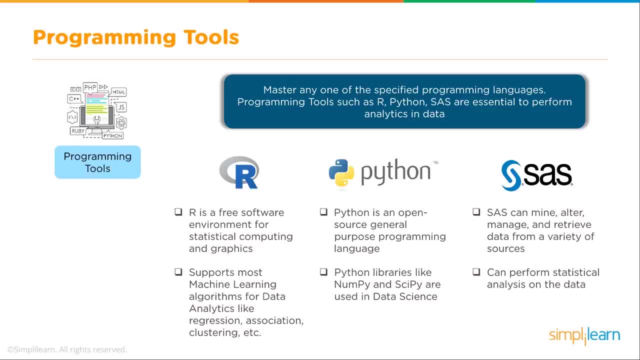 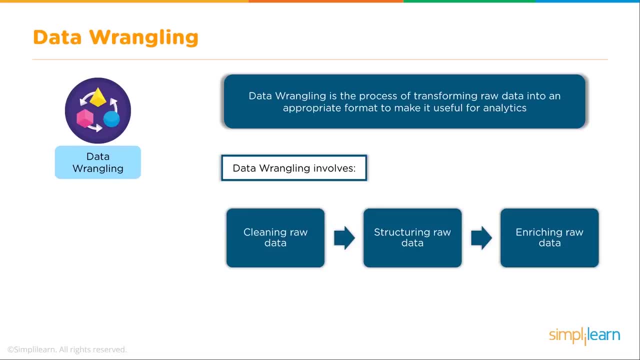 also, if you really start using it as a company, you're gonna have to pay for it. where r is free is uh free software. python's also open source and free to use. so we're going to talk a little bit about data wrangling, and i mentioned earlier. 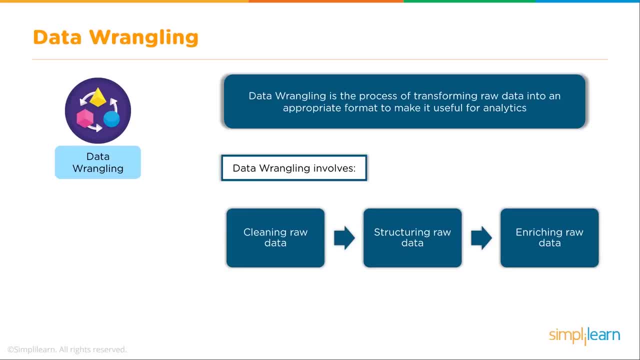 that is, uh, both the probably people's least favorite aspects of data science and also probably one of the places you spend the most time. so when we talk about data wrangling, it is a process of transforming raw data into an appropriate format to make it useful for analytics. 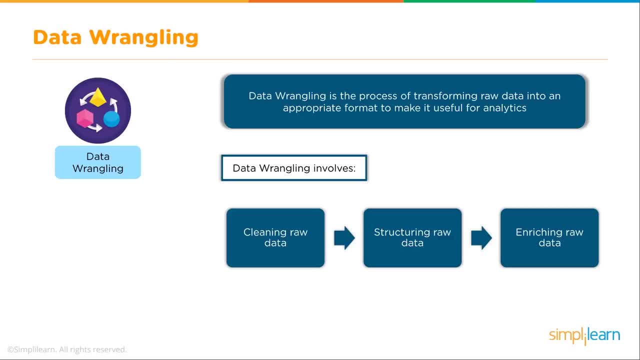 and it involves cleaning raw data, structuring raw data and enriching raw data. and this gets interesting because you'll get stuff like this in the next few weeks or so, and then you'll get stuff like this in the next few weeks or so, and then you'll get stuff. 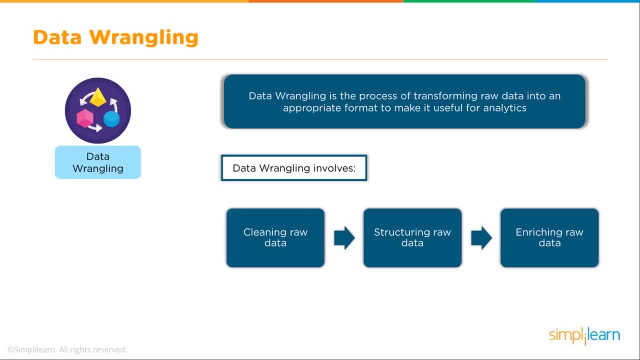 on something like in python. you might get stuck on something that is a date time based on an integer 64 numpy set. you might not know what all those terms mean, because you work in r or something like that, but you get the point that it's all one particular format, and then you have to figure out. 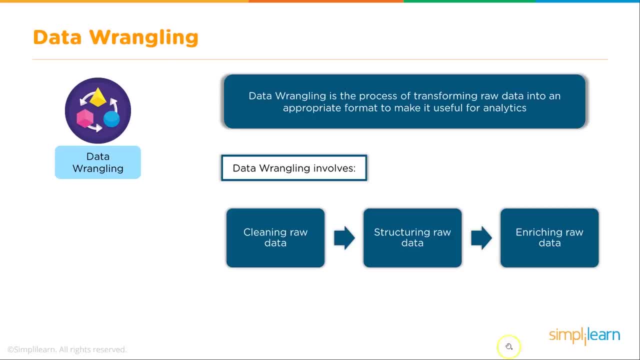 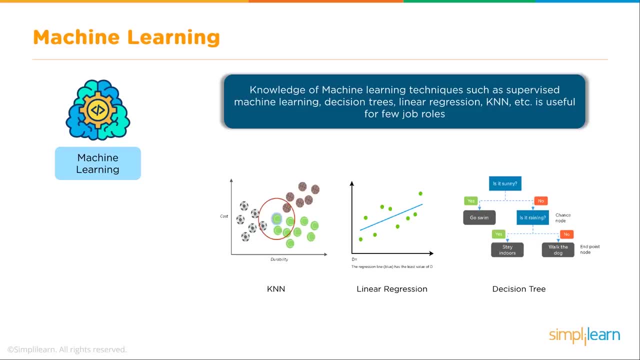 how to switch it so that the computer can see it correctly in whatever format you're using or whatever analytics platform you're using. knowledge of machine learning techniques such as supervised machine learning, decision trees, linear regression, knn, etc. is useful for a few job roles. so this is kind of interesting, because sometimes that's the center of the job role of a. 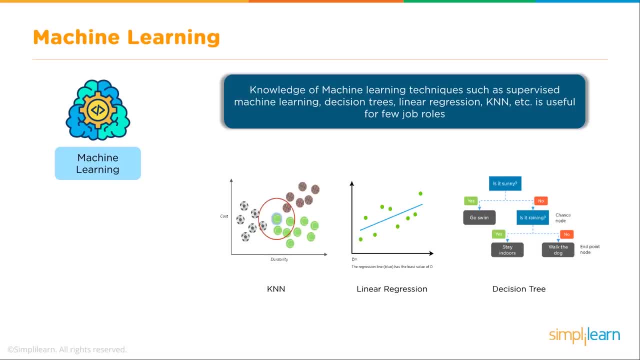 data scientist and sometimes you just have to be able to apply the programming skills to it so you can get the answer and let somebody else fine-tune your machine learning techniques. so it really depends on what it is you're working with and you can see, here we have our nearest neighbor. 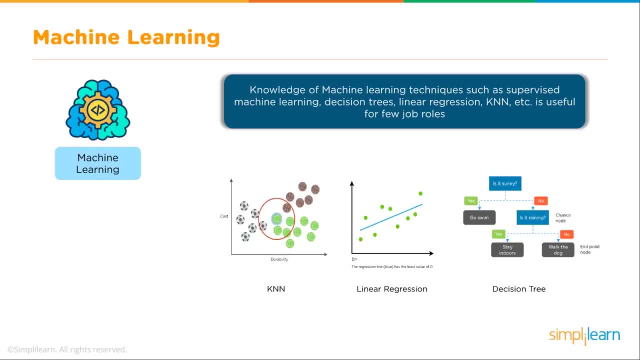 set up where it groups things together that look alike linear regression- you're drawing a line through the data or curve, so you can predict what the next value is going to be. and then our nice decision tree which starts splitting things up and says: you know, it's sunny out, yes, let's go swimming. no, it's raining, we're. 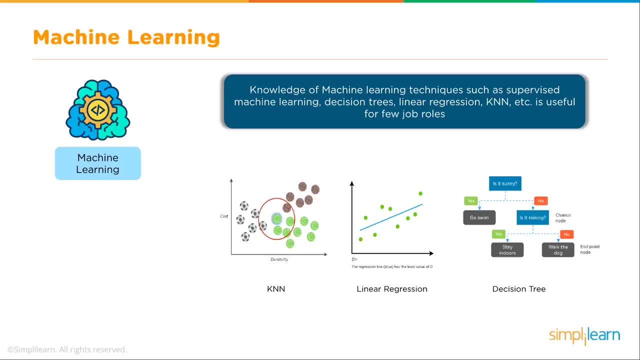 not going to go swimming? yes, it's sunny out, we might go swim. it's raining, we'll stay indoors. yes, we'll walk the dog, no. so you have a decision tree that helps figure out how you get to the end result. so decision trees can be pretty powerful. and data visualization. data visualization is the 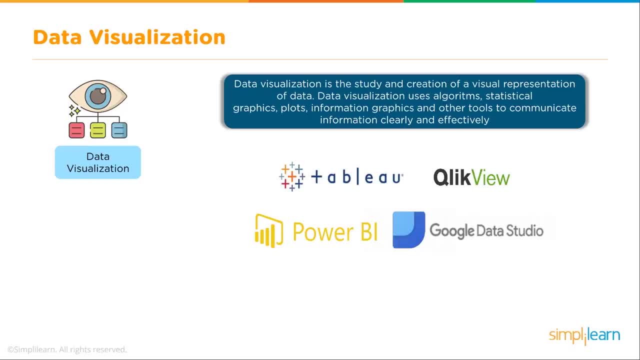 study and creation of visual representation of data. data visualization uses algorithms, statistical graphs, plots, information graphics and other tools to communicate information clearly and effectively. this one you really have to master as a data science. this one you really have to master as a data scientist. and there certainly 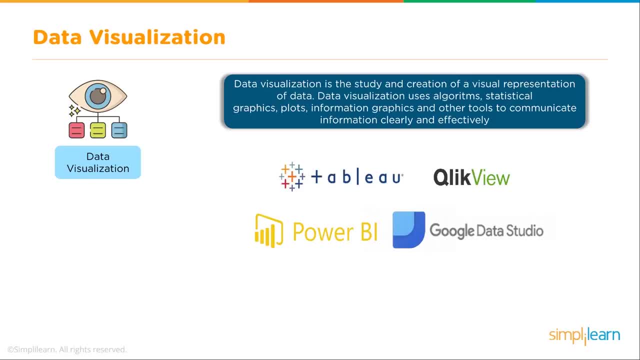 are so many different tools to use to visualize it. but when you're communicating, a picture is worth a thousand words. when you can put a picture up and people can look at and go, oh, i see what's going on and say, yeah, yeah, this is good, people hear that and they just kind of go: okay, it's good, but why? 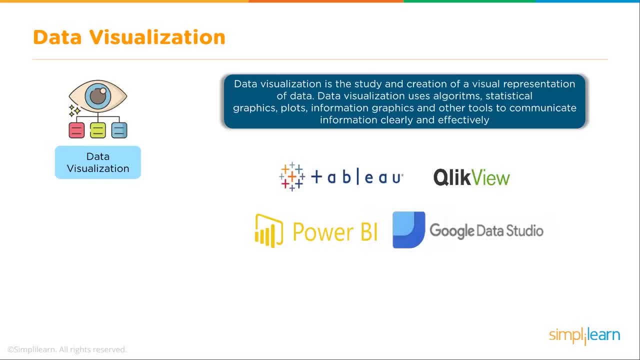 and you might say: you know, okay, these numbers make it look good. no, people want something they can see, and there certainly is. uh, tableau is probably um, one of the most popular ones out there. calic view, power, bi, google data studio. in python there's the pi kit and seaborn, there's all. 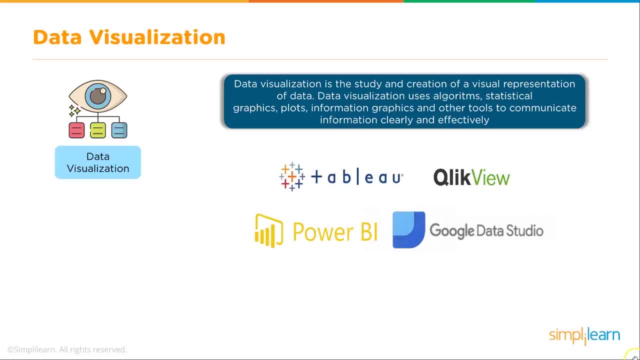 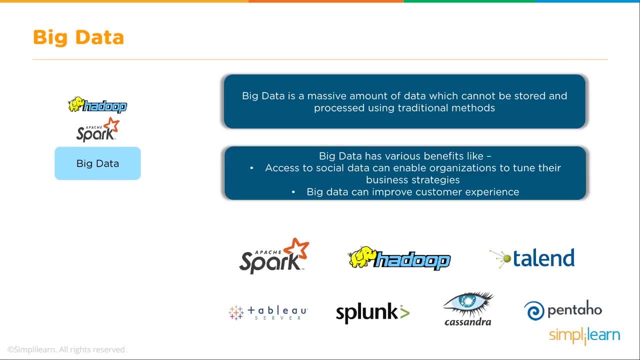 kinds of different options for visualization. you need to master probably at least one or two of them so you understand how they work and how they're different. and then big data. big data is a massive amount of data which cannot be stored and processed using traditional methods. big data- 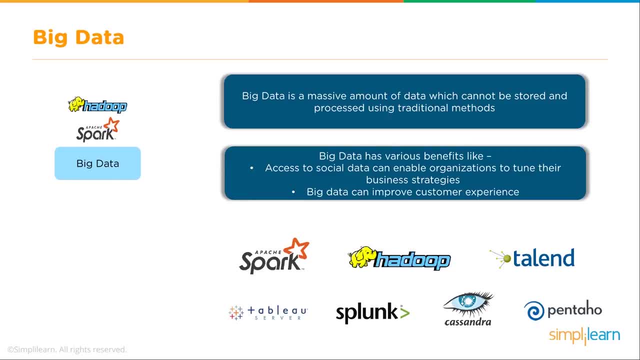 has various benefits, like access to social data can enable organizations to tune their business strategies. big data can improve customer experience. uh, and so we're. usually, when you say big data, we're almost always talking about hadoop and apache spark. it used to be hadoop as your file. 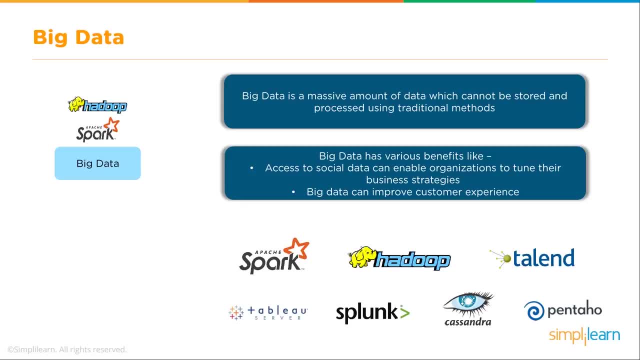 so that's how you store all your data going across the nodes, and there certainly are other ways to store it. when we talk about hadoop, we're usually talking about at least 10 terabytes of data when you're dealing with a hadoop file structure, and then you can use spark where hadoop process is. 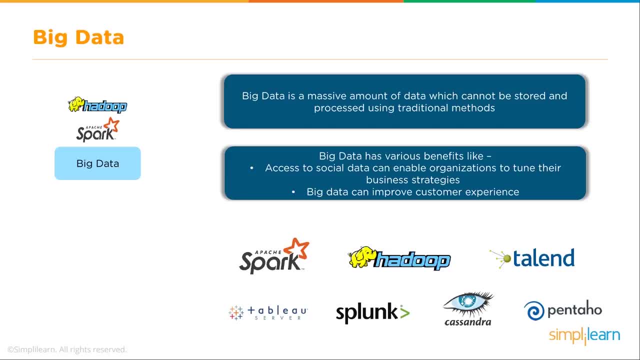 on and off the hard drive so it's continually reading and writing to the hard drive. spark is running in your ram and so when you're doing a very intensive data process, you'll run a spark setup which will spread those processes over multiple computers. and, of course, 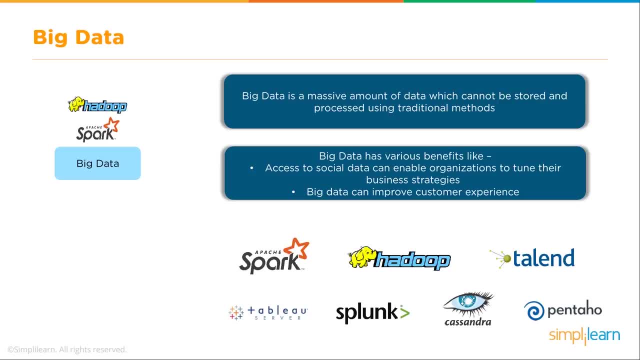 now the two combine and spark sits on top of hadoop and you get your big data. there's also a talent. tablo has its own server setup. there's splunk cassandra- you'll hear the cassandra database pinto- i'm not even sure how to pronounce that one. it's not one i've worked with. 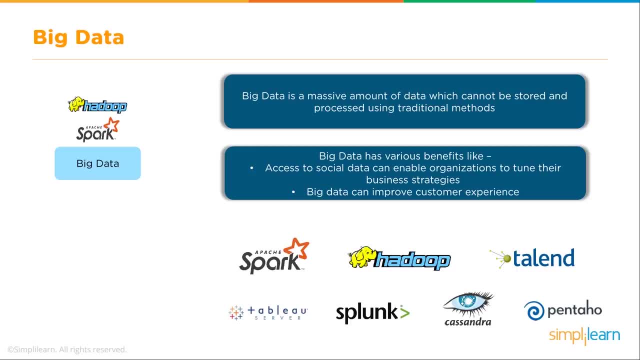 certainly there's a lot of options for big data. the two big players are, of course, hadoop and spark, and even your sql servers and my sql servers will spread across five different servers and you can be talking about big data across five servers with those pulling them into, say, apache, spark, to do your high-end processing and then 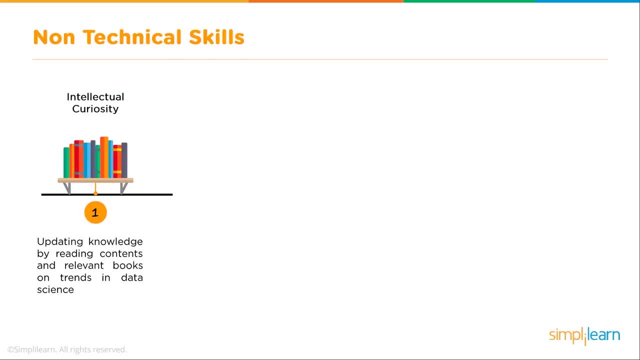 there's non-technical skills. probably the most important one in data science and any of our data analytics is intellectual curiosity, updating knowledge by reading contents and relevant books on trends in data science. this is such there's so much going on in this field and it's exploding now. 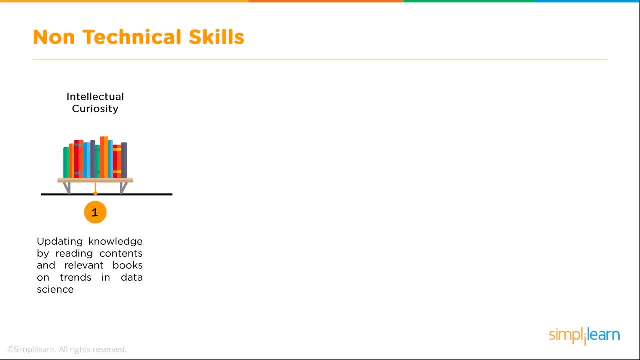 that it's hard to keep track of it all. so you really need to have that curiosity in the data science process to be able to do your high-end processing. and then there's non-technical skills, probably even more so than a lot of other fields, but i would say in just today's world you need 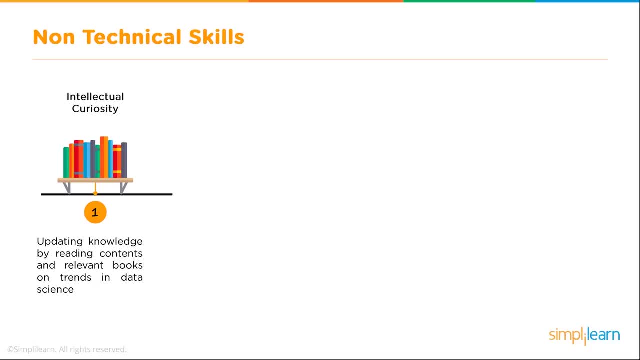 intellectual curiosity, because things are changing so rapidly in today's world, the way that's going with our technology. understanding how the problem solved can impact the business. business acumen- this is the one where a lot of people kind of skip over. you have to have a little business sense. 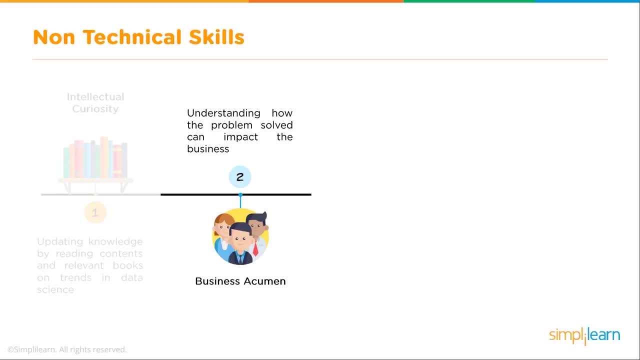 if you don't know how it's going to impact the business, you're going to be in trouble. why do they want to even pay you to be there unless they know what's going on and they're getting something in return? so this is your bottom line for your paycheck is what's going on with the business. 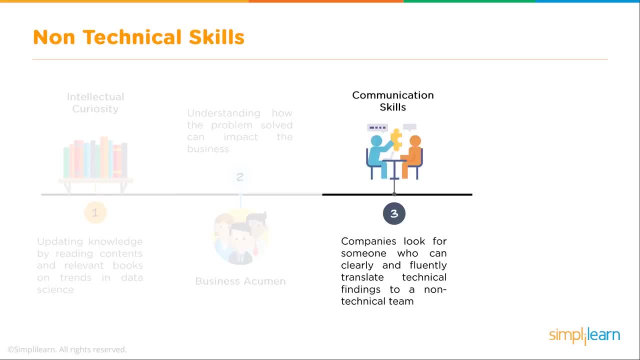 how is this going to impact the business? what are you doing for them? in communication skills companies look for someone who can clearly and fluently translate technical findings to a non-technical team, and i've talked about this a bunch and i can't even iterate this enough if you. 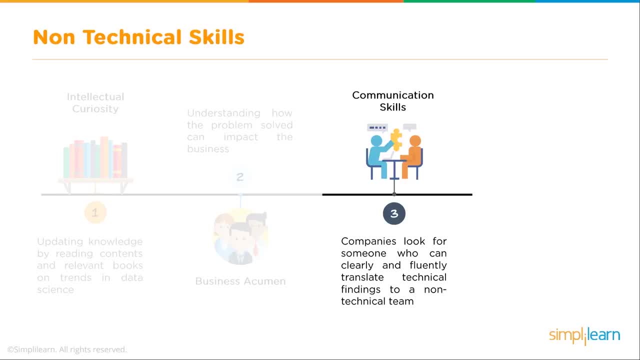 are struggling with your communication skills, work on building them. they don't have to be. you know, this isn't rocket science, where you have to know all these complicated terms. which you need to do is take the complicated terms you know from data science and reduce that down to something. 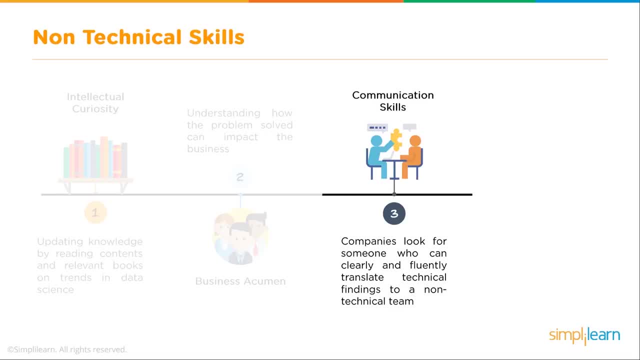 that anybody can understand. so when you come up and you have, uh, you know, knn, no one knows what knn is, you know, unless they're in data science nearest neighbor looking for things that match together. you got to explain that to people who do not have the technical skill in the data science arena and 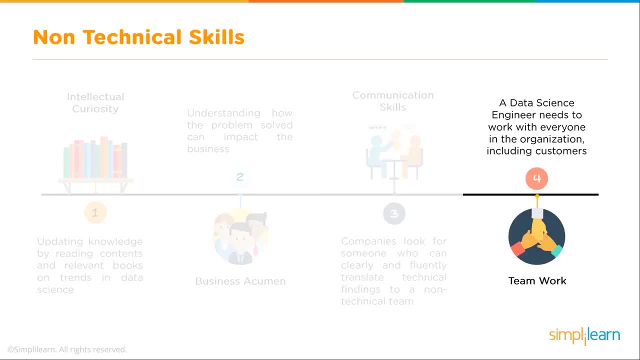 a data science engineer needs to work with everyone in the organization, including customers, so it's teamwork, and that's always one that throws people for a loop. but ultimately, you are analyzing your customers information and so sometimes getting in there and rolling up your sleeves if you're- let's say, you're- doing data. 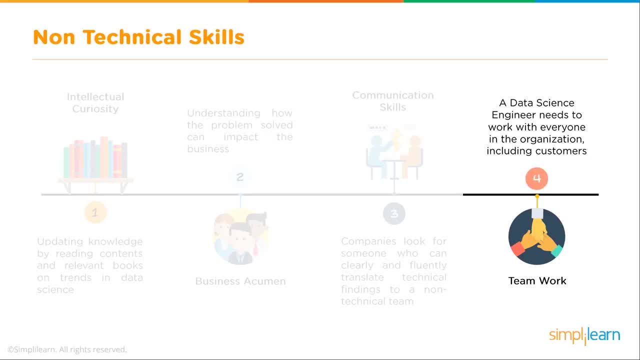 analysis for a sales team and you're backing a sales team, you might have to get in there and go start making some sales and making some phone calls and see what it's like. what is that team doing when they call 15 people in cold calls and then they do a follow-up two weeks later? 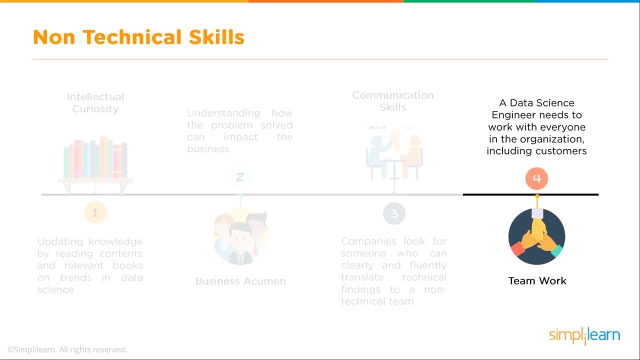 or three weeks later. which one works better- two or three? does it work better to call and send a fax? call and send an email? you know when you should you show up in person if it's that kind of business. so working with everybody, including the customer, is very important. with the 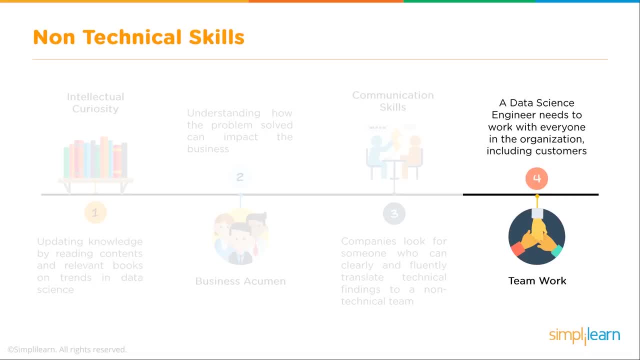 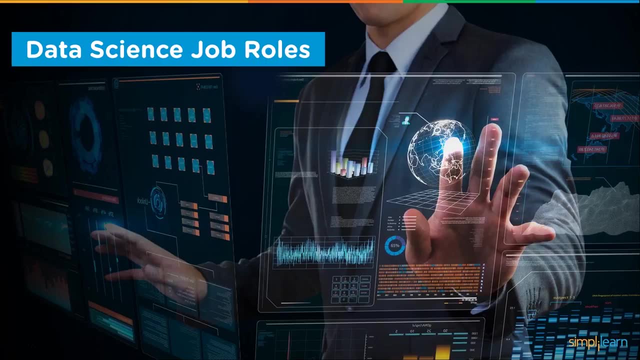 data and with this kind of setup and non-technical skills for a data scientist. so let's take a look at some of the roles a data science plays in the job market. let's drill in there just a little bit here. so when you have a data scientist, they're going to perform predictive analysis. 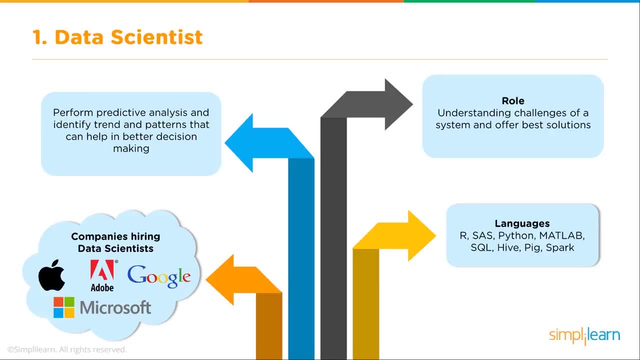 and identify trend and patterns that can help in better decision making. companies hiring data- Apple, Adobe, Google, Microsoft- I would say that's even expanding down to smaller companies. you know where you're talking about. only a hundred employees or something like that. they're starting to look at data scientists because they 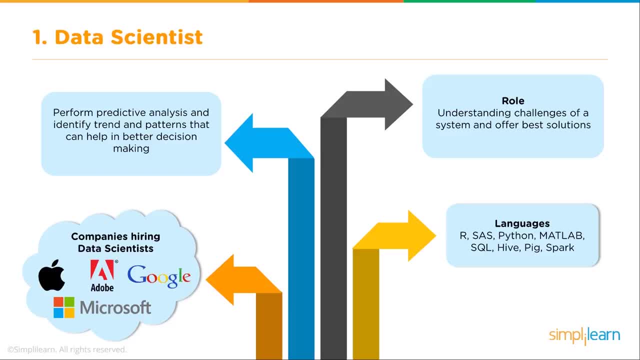 need them to come in and be a part of that team, and the rule is understanding challenges of a system and offer best solutions. this should always be. the goal of a data scientist is to be looking at the whole system and then trying to find those patterns that are gonna best enhance the company or the business or 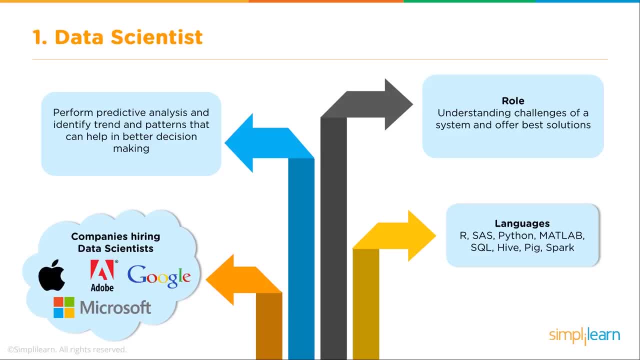 the whatever group may be working with the sales team or the marketing team, and you can see languages pretty important to have a. these are a number of different languages and again it depends on your own specialty. there's all kinds of different variations, but we have our SAS, Python, MATLAB, SQL, hive pig, spark you. 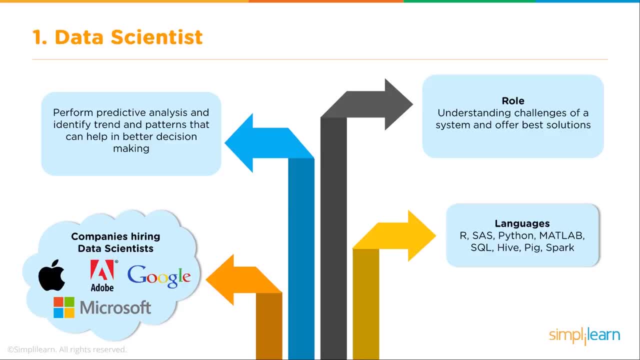 should have at least a knowledge of all of these. maybe a Python programmer never used our download. it go through the basics, so at least you know what's going on in our versus Python, because our is pretty powerful for doing a very quick display and then, of course, a lot of things you can do in Python. you have to 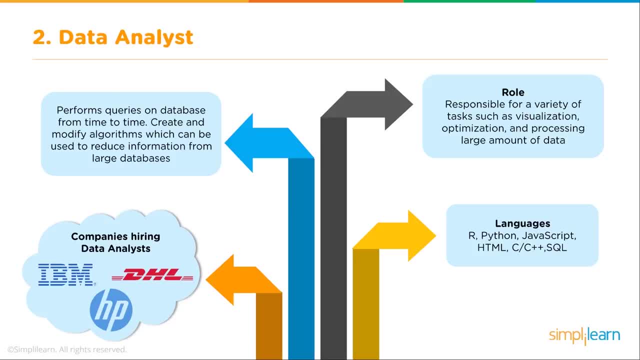 be able to do queries on database from time to time, create and modify algorithms which can be used to reduce information from large databases. I mean, usually this is one of those things you do at the beginning: you set it up and then you kind of let it go until it breaks and you have to go back and fix. 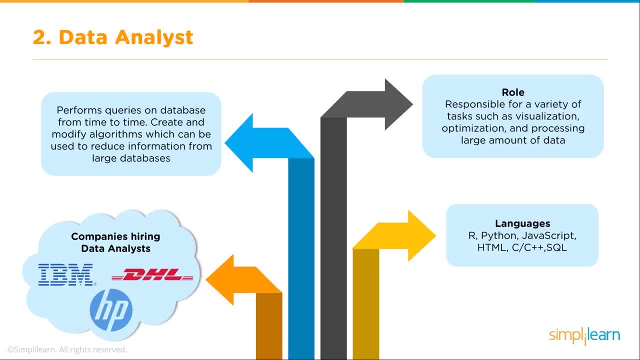 it because your query isn't working. that certainly is a very common thing to have happen, especially if you're pulling data off the web and the internet. and then we have some more companies that are hiring data analysis, like IBM, DHL, HP, and so we're talking about data analyst. the role is responsible for a 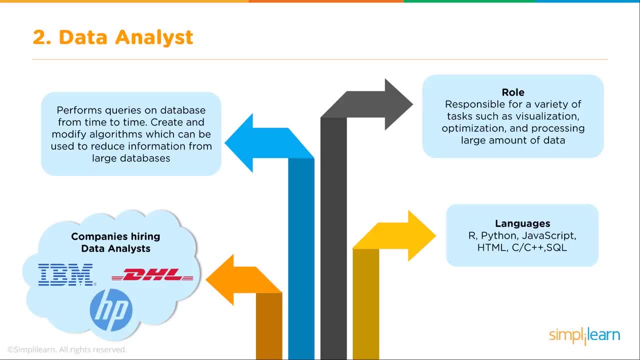 variety of tasks such as visualization, optimization and processing large amount of data, and so we're talking about a data analyst. we're also- we're still talking a lot of the same stuff, which you'll see. we now thrown in JavaScript and HTML in here, because that's pretty common with the data analyst versus a. 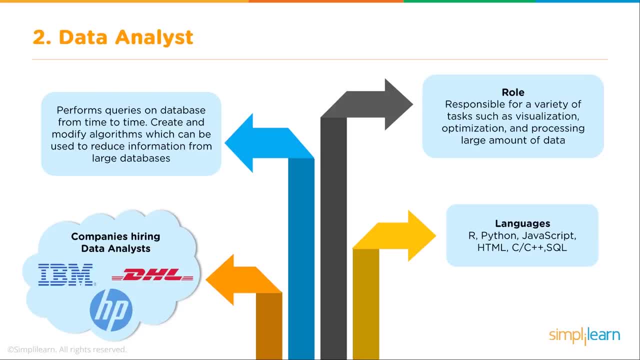 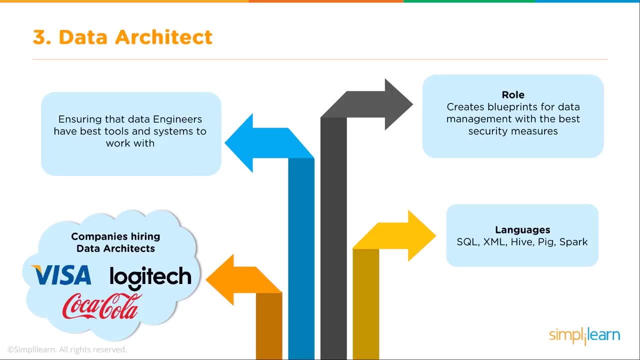 data scientist and you can see that SQL is still pretty solid and also cc++ is pretty big, so some companies also use Java. I'd put Java in the languages also on that- for a data analyst. and then you have a data architect ensuring that data engineers have best tools and systems to 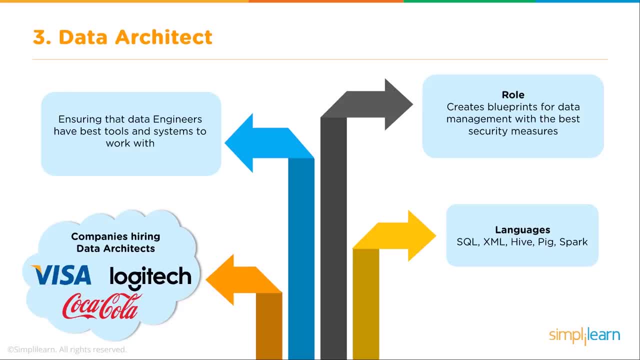 work with, and so companies hiring a data architect are like visa, Logitech, coca-cola: they create blueprints for data management with the best security measures. I cannot highlight that a data architect really spends a lot of time with security measures. that's big. how many hacks have we seen in the last year? 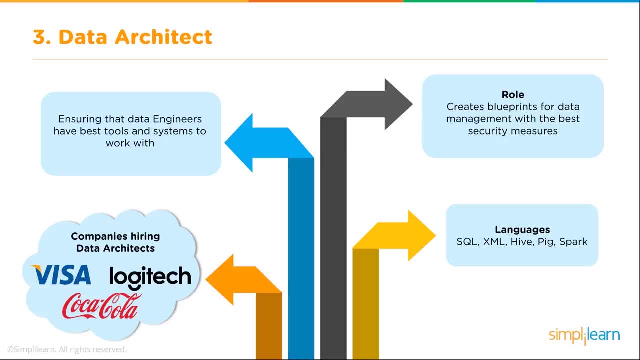 on. large companies have lost a lot of money and they've lost a lot of money. they've lost data for millions of their customers and how badly that affects some. and we're looking at languages, as you see that SQL is pretty solid across all of these under a data architect XML, that's one that a lot of the data 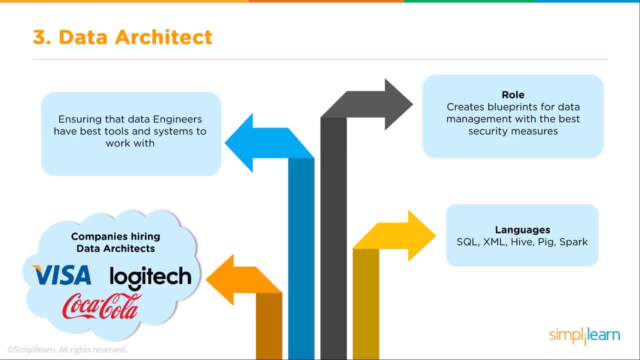 science jobs don't really. you don't see as much, but you're gonna see more XML with a data architect, because there's a lot of XML files that are that have your security measures embedded in them and, of course, your hive pig. those are Hadoop systems for doing some basic queries. so instead of doing the high-end queries, 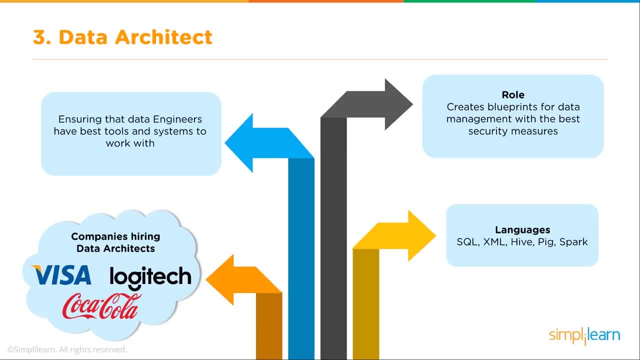 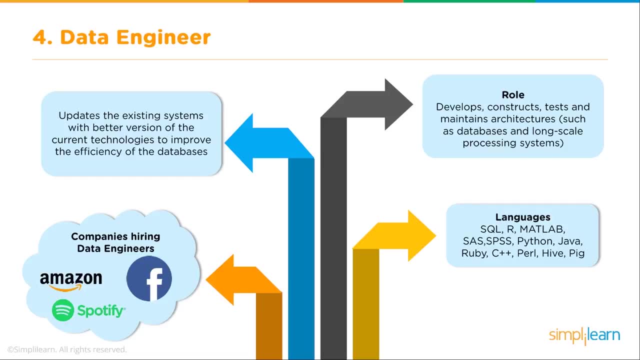 you know how these simplified query systems built into Hadoop and spark. so if you're using big data, you're gonna want to know your spark also. and then we have our data engineer. the data engineer updates the existing systems with better version of the current technologies to 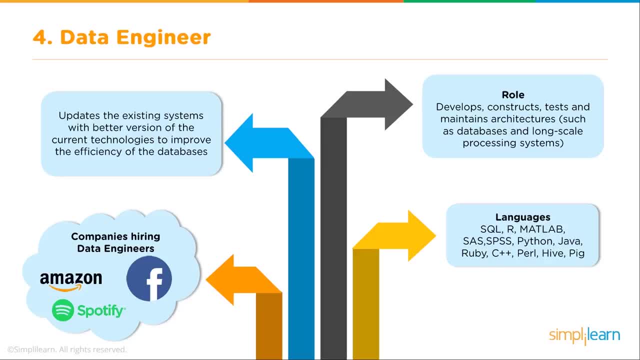 improve the efficiency of the databases. think admin here a lot of work tracking down what version you're in of the different programs. what version of Python are you using? what version of are using what version of C++? so companies hiring data engineers are like Amazon, Spotify, Facebook. 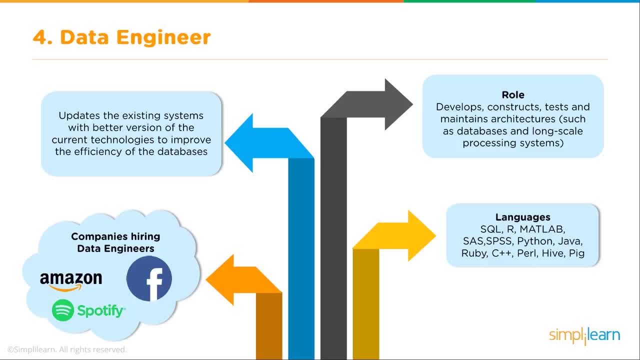 and they develop, construct, test and maintain architectures such as databases and long-scale processing systems. and here we have our languages, or SQL, our MATLAB, SAS, SPSS, Python, Java, Ruby, C++, pearl, hive pig you pretty much as a data engineer at this level when you talk about admin and updating all. 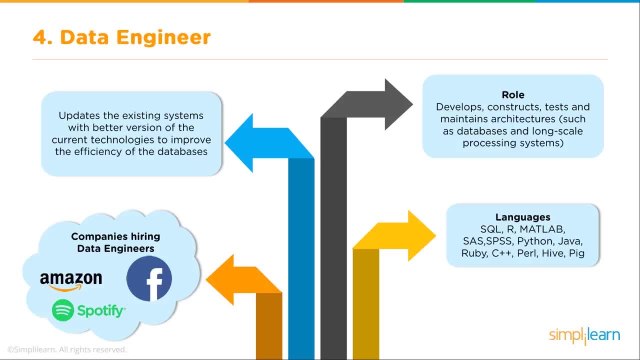 these databases need to know all the different stuff that's being used in the company, and you're testing out these structures to make sure they work, and so you really are talking admin level kind of setups, if you like, spinning up an admin on to Google Cloud Service or 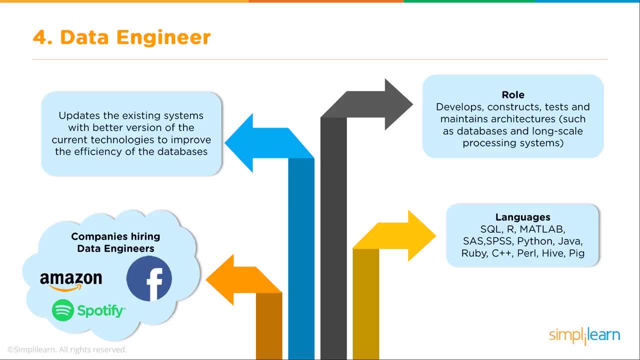 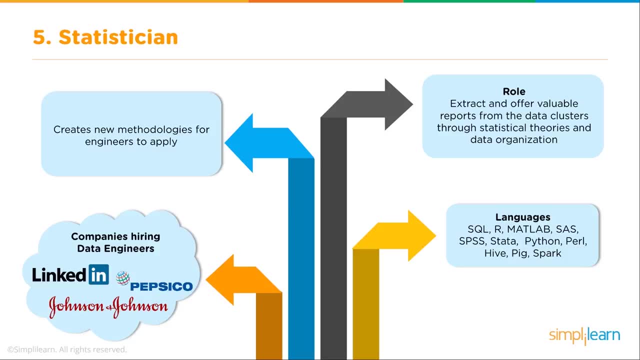 Amazon Cloud Service. now you start to get an idea what we're talking about, because then you can test it out up there and then you can bring it back and update it to the company. statistician creates new methodologies for engineers to apply, and so, when we look at this, this is where we're digging into the 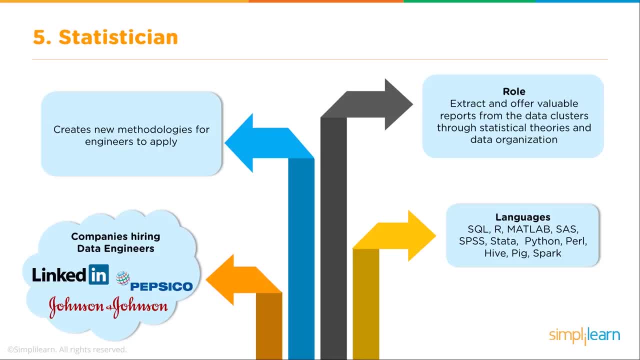 math of which models to use, what setups going to work? what kind of activation do we have on our neural network? these little tweaks are going to make a big difference and we look for methodologies at a large level. what kind of data we're going to be looking at? how we're going to pull together companies? 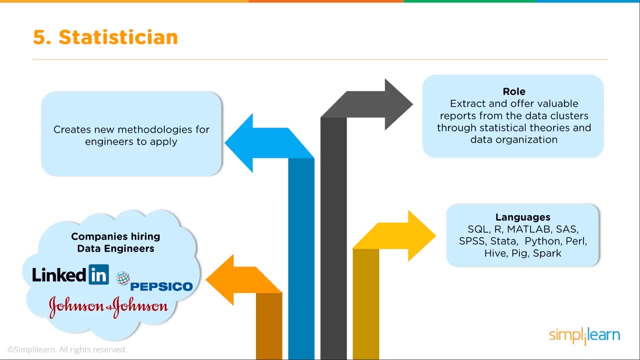 hiring a data engineer or talking about statisticians were talking about linkedin pepsico, Johnson and Johnson, and of course, these companies probably hire a little bit of everything, but they have a lot of statisticians working for them. as we look at the role, extract an offer valuable reports from the data clusters. 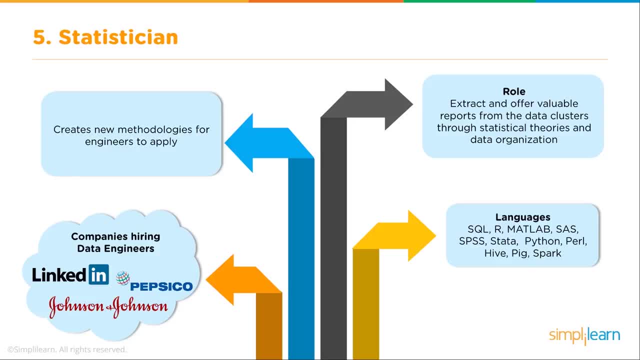 through statistical theories and data organization and the languages across the board. we're still seeing SQL R, MATLAB, SAS, SPSS data. that's a new one. they went up the scene in some of the other roles- Python, Pearl, an older version, and that shouldn't be a surprise. 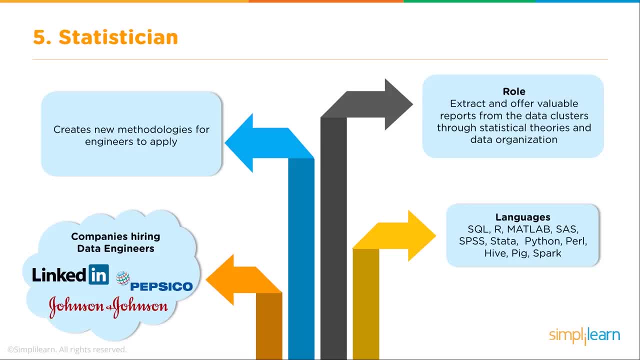 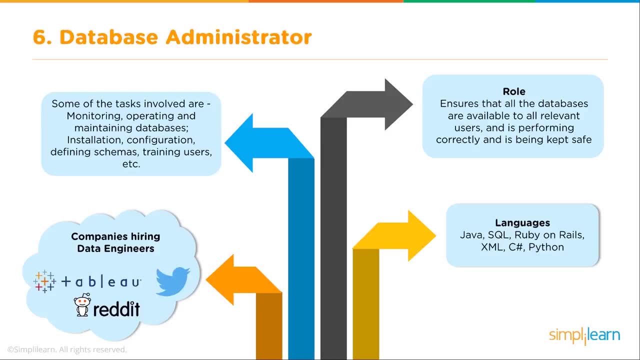 because a lot of these companies probably built a lot of the original packages on Pearl, if you look at Johnson and Johnson and of course your big data, high pig and spark, and then our database administrator I mentioned. the other one is an admin. they're more an admin level for the software itself. administrator is 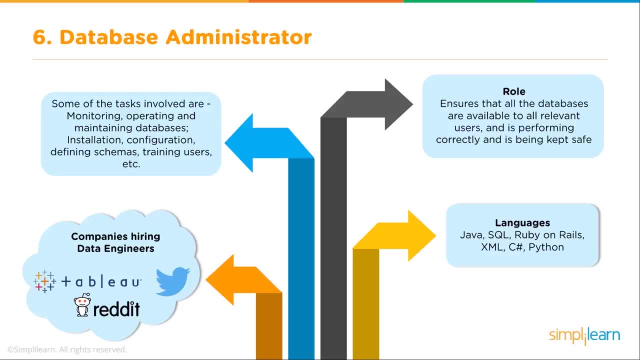 another level. some of the tasks involved are monitoring, operating and maintaining databases, installation configuration, defining schemas, training users, etc. and this is interesting: training users because when you build a database and you define all the different tables that are embedded in that database and how they're all connected, the end users got to have that information, otherwise you're in trouble. 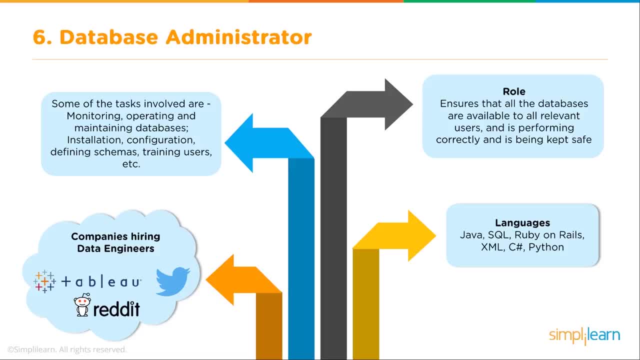 when we have companies hiring data engineers. course, tableau, Twitter read it. the role ensures that all the databases are available to all relevant users. getting a little security in there. what role do they have? is allowed in and not, and is performing correctly, is being kept safe, and you better be ready to. 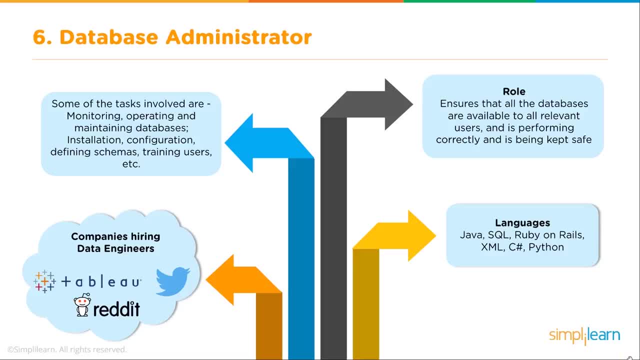 spend some time in security because, again, that's a very big thing nowadays with the number of people who hack into these databases in the languages are gonna be covered. you have your C, Sharp, your Java, sql, Ruby on rels, XML. again there's that XML because a lot of your security is embedded in XML files: Python. 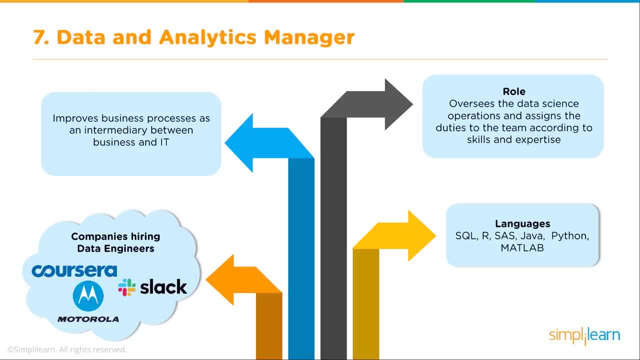 all the main players, depending on what the company's using: data and analytics manager. So when you see manager, that means that somebody is going to sit on top and organize the people underneath, So they're going to improve the business process as an intermediary between business and IT. 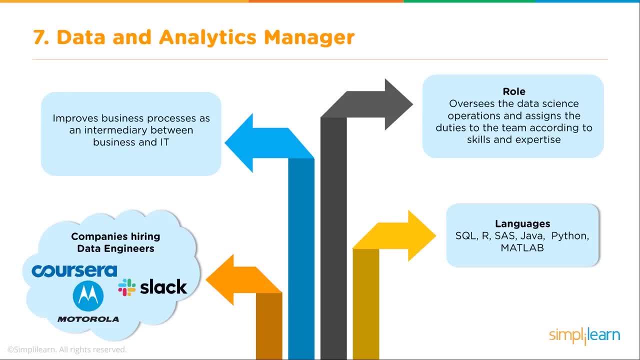 Oh, you better have some really good communication skills for this one. Some of the companies hiring data engineers are Coursera, Motorola, Slack. Of course, these companies are hiring data scientists in almost all of these fields. So the role oversees the data science operations and assigns the duties to the team according to skills and expertise. 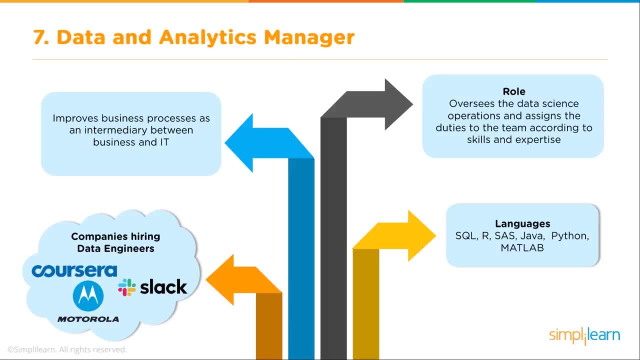 So that's a big one. You better be able to communicate what's going on, help your team members come out and be able to communicate with other people. So sometimes your job is just being able to get people to talk to each other. 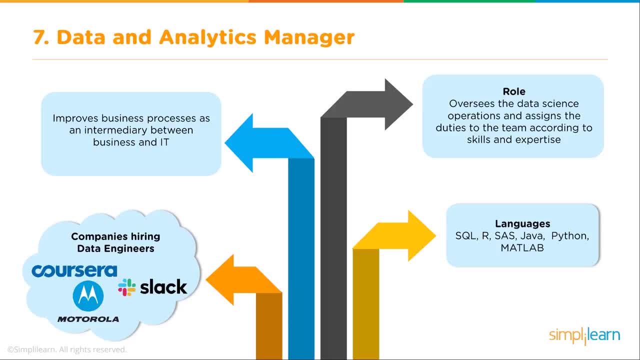 The big thing on that is the whole communication line going from one end to the other Because you can't communicate all the information that everybody's working on. You have to pretty much come in there And help people communicate what there's going on. 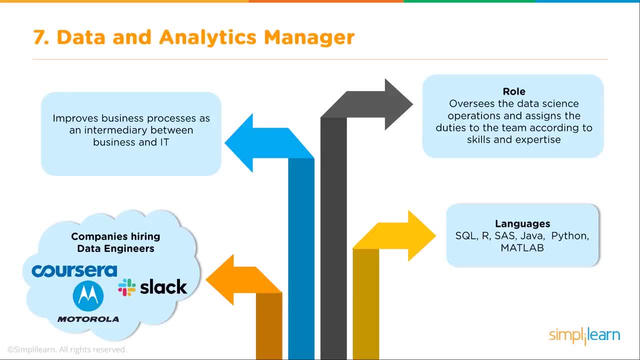 And also know what they're up to, without being micromanagement, Because that will crash a company. if you micromanage everybody But if you just let them do whatever they want and they never talk to each other, that will also destroy the company. 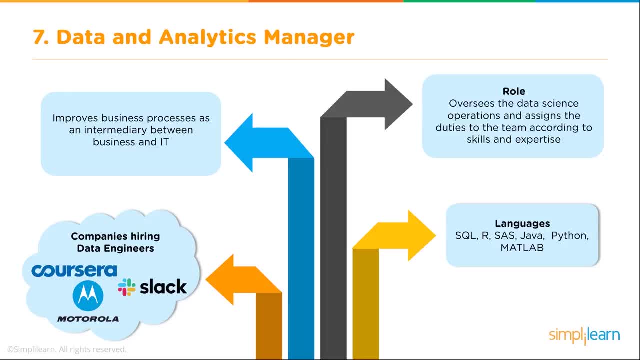 You've got to find that nice middle ground And you really have to have an overview of everything. as a data and analytics manager- One of the things I mean- you know it's good to have at least one or two solid bases of programming under your belt for a data analytics manager. 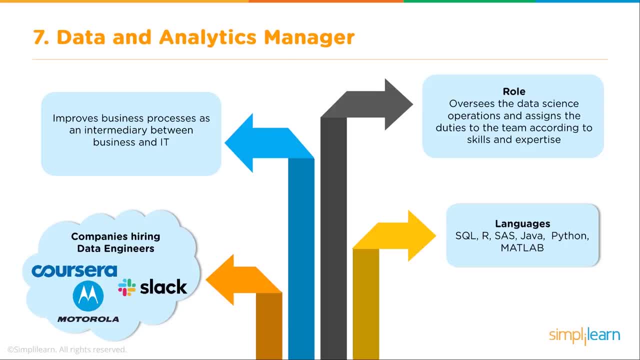 But you do need to have a very general, A general understanding of all the different tools being used so that you know what's going on with your different team members. Of course, SQL R, SAS, Java, Python, MATLAB- all of those are big. 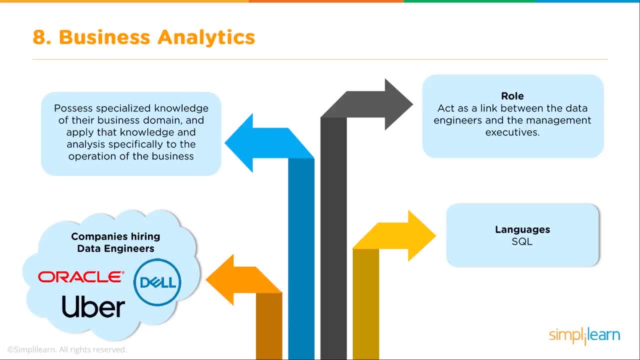 Business analytics. So this is, when you're talking about your BI or your business intelligence and your business analytics, Very important to know. this is kind of a subdivision of a lot of the other stuff. we've talked about A lot of the other roles we've looked at. 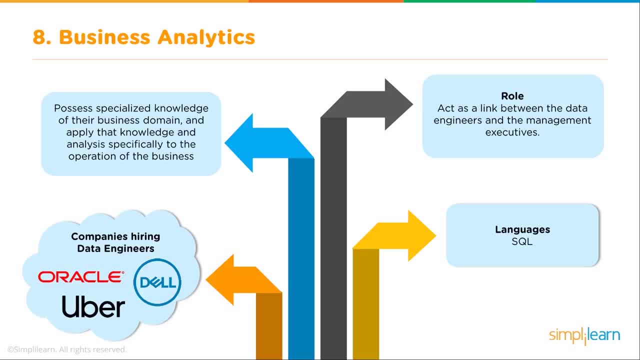 So you possess specialized knowledge of their business domain And apply that knowledge To analysis, specifically to the operation of the business. So you might be a specialist in banking. You might be a genetics engineer, So you know about genetics. You might just be general business, helping the marketing. 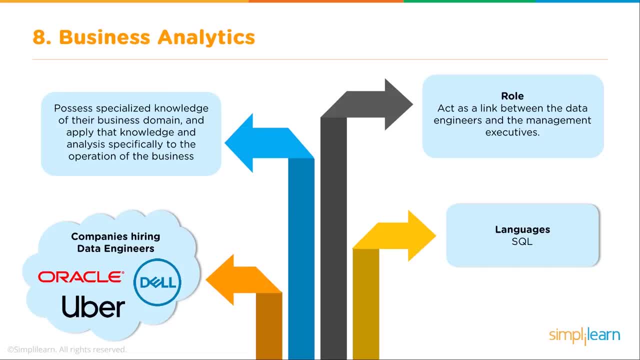 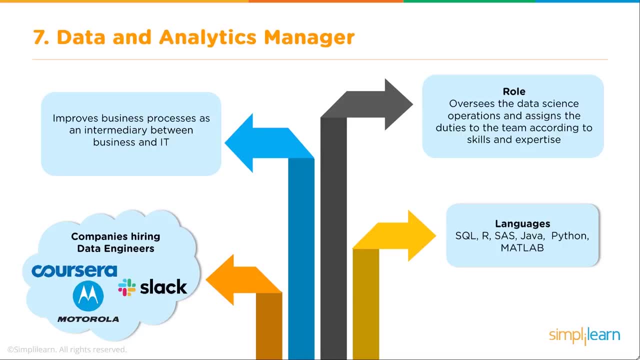 So a lot of companies hiring data engineer are Oracle, Uber, Dell, And the role acts as a link between the data engineers and the management executives. So it's very similar to when you go back up here and we look at data analytics manager. 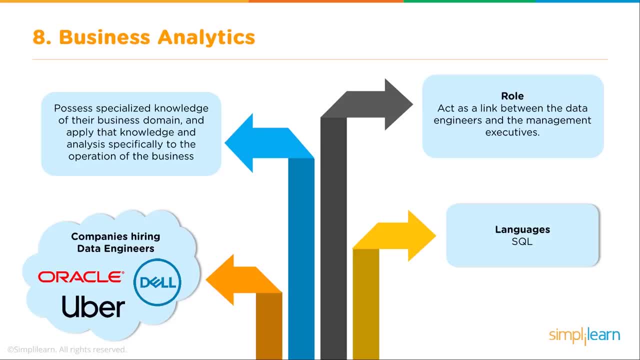 A business analytics is going to also kind of fill that role. There's a lot of people in between, but they're more specialized in business And you better know SQL because we're talking about business specifically. Most of the large companies are storing their data that's up and running right now. 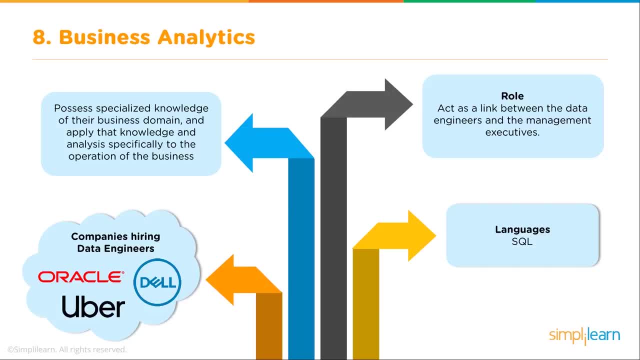 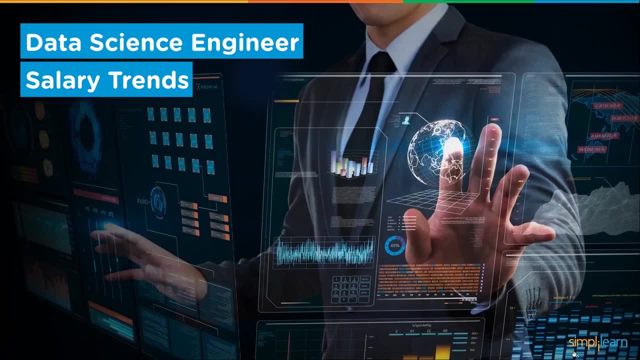 That people are accessing to purchase something on the Home Depot website or the Uber They're logging in. You better know your SQL. It's very central to business analytics, So let's go ahead and take a look at the data science engineer salary trends. 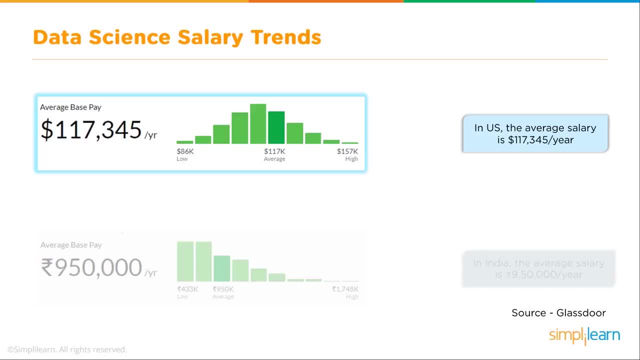 And you'll see that our source is Glassdoor. That's where we're pulling a lot of our data from. The base pay is around $117,000 in the US- the average salary- And when we look at India, we're talking about $950,000 a year. 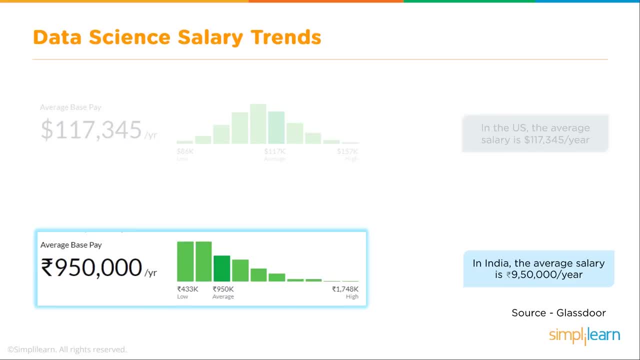 And those are based on some of them. you need to go ahead and dig deeper to find out what education level versus entry level, But those are pretty solid base once you're in the industry and once you created your career in there. When we look at the job titles, the most common job title is data scientist. 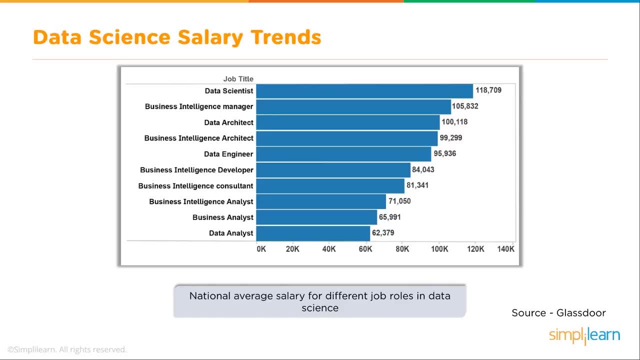 Business intelligence manager is the second greatest one. That's kind of good to note. That's why they put that up there as being its own little subcategory of data science managers- a business intelligence manager, because it's such a high level of jobs. 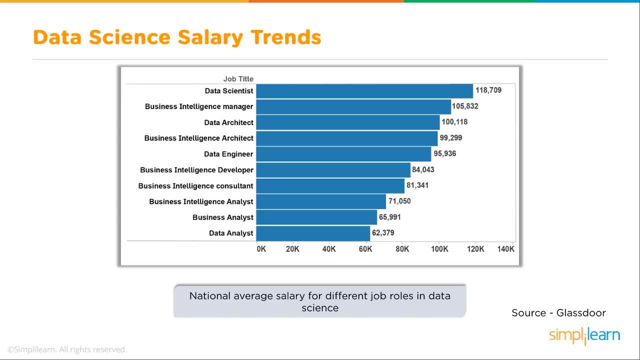 And then we looked at some of the other ones: data architect, business intelligence architect. Again, your BI, your business intelligence, gets its own ranking because it's such a high level. you know it's a business. People want their businesses to make money. 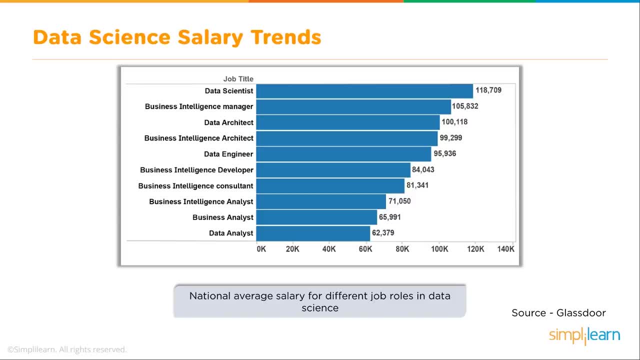 So that's who's hiring, Of course, data engineer, business intelligence developer, business intelligence consultant, business intelligence analyst, business analyst and data analyst. So you can look at the data analyst as being the general one that doesn't go specific to business. 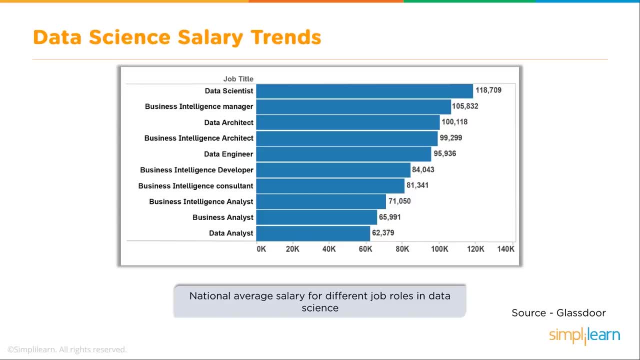 So if you're looking just for your career, as far as getting a job probably should have some kind of business understanding in the background. And again, you know your companies want to make money, So they're going to hire someone who knows business. 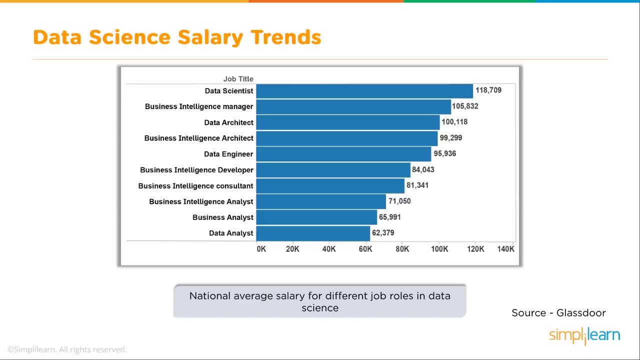 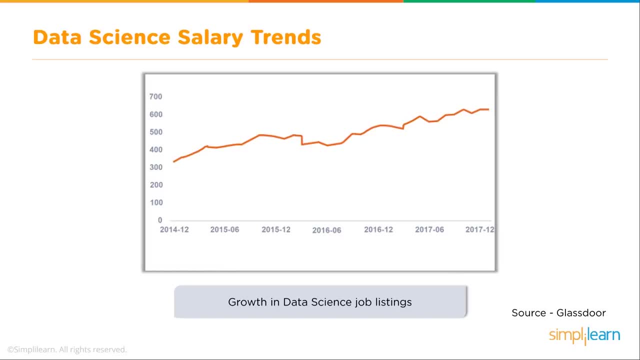 If banking business, if you specialize in banking or retail, specialize in retail and marketing, And you can see here on the data science salary trends And the growth in data science job listings. It's continually going up. It's since 2014 to 2012.. 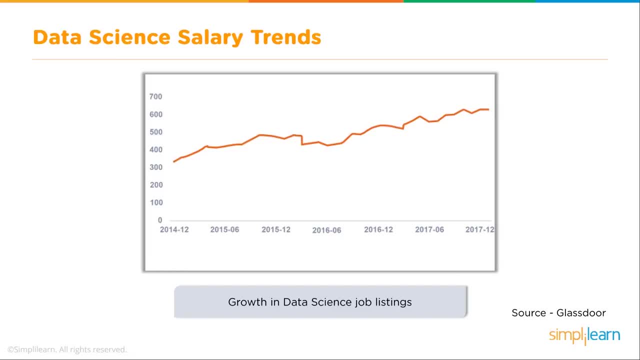 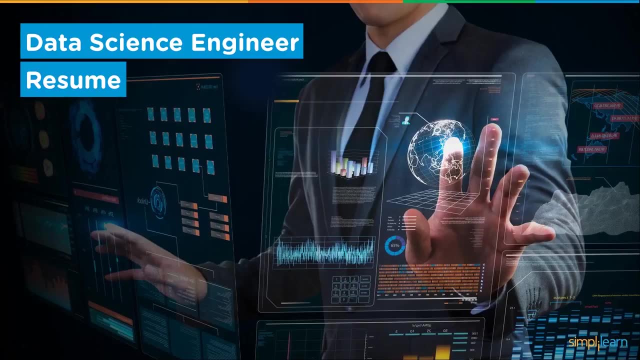 We've gone from 400 to 600. That's a pretty big increase. So you know, a huge growth in this market is one of the biggest growing markets right now for jobs and careers. So let's go ahead and take a look at building a resume. 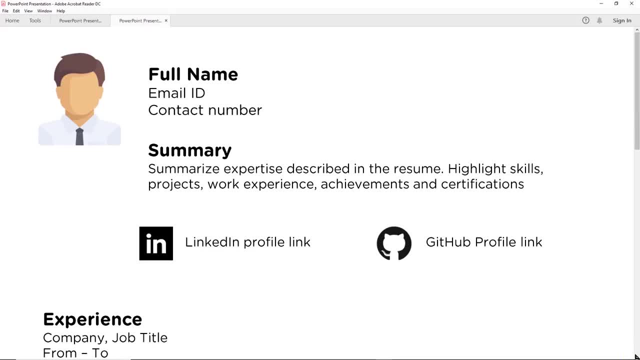 Always exciting putting ourselves out, selling ourselves, And if you looked at some of our other videos dealing with resumes, you'll see a trend Here. the top part is so different than what resumes were in the 90s, In the 2000 to 2010,. they've evolved. 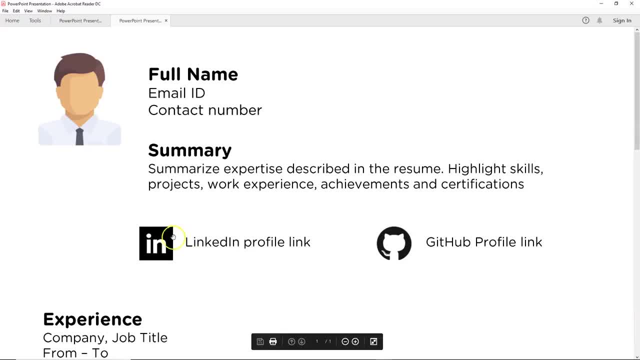 They've really evolved. It used to be 2000,, 2010,. maybe LinkedIn, maybe one other reference. Now you're going to see that we want those references. This is a sales tactic which now has come into resumes. Used to be that, if you are a real estate agent, every real estate agent I knew I used to deal with real estate software. 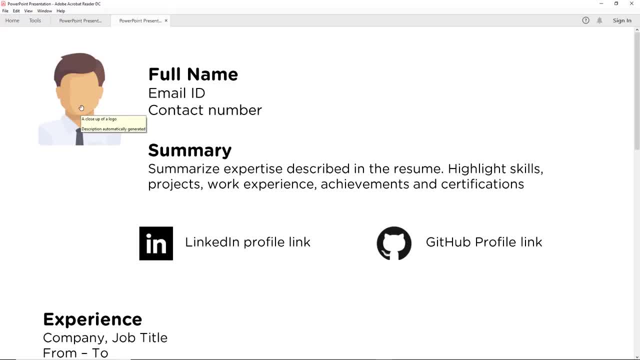 For the real estate industry. back in the 90s, every real estate agent wanted their picture on their business card. They wanted their picture if they could put on their contracts. They wanted people to see the face. So that's really a big change is to make sure that it stands out. 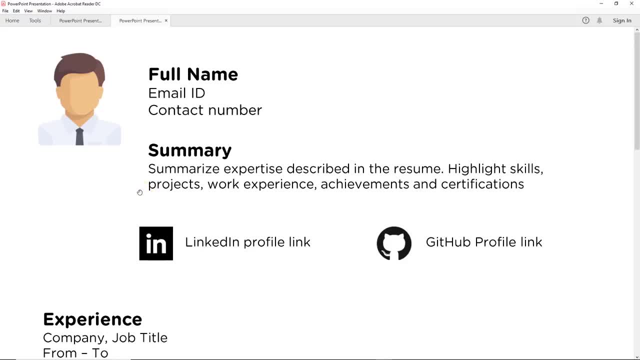 You stand out. Here's a picture of somebody, So you're more than just a couple of letters and a name And of course, you need your contact. information should always be at the top. You have your summary. What are you focusing on? 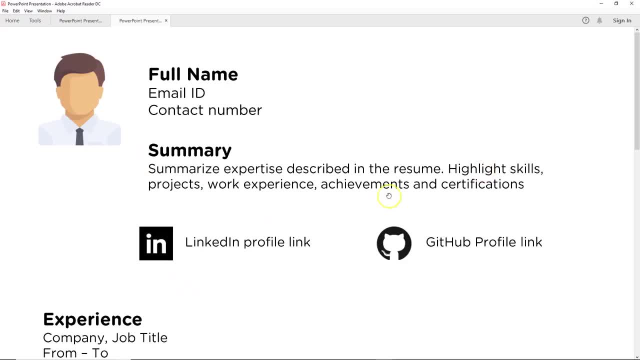 Be a little careful with your summary, because if you have everything in your summary and then they scroll down to experience and education and skills, they're going to stop. The second you repeat yourself in your resume. that usually means to the reader: Hey, this person doesn't have anything more to offer me. 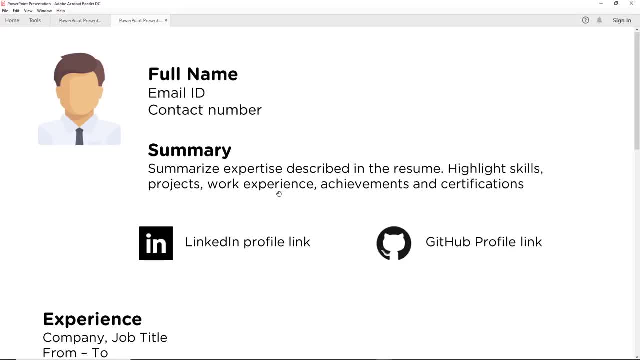 I'm done. So be a little careful how you word your summary. Most companies appreciate when you come in here and you've adjusted this summary to be both about you and how you're going to serve that company. So it's worth researching that company to find out how those connect and put that in the summary. 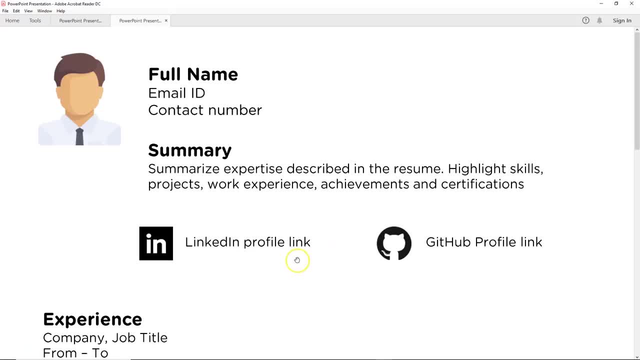 Take some time to do that. That's actually a pretty big deal And the references are huge also, especially in data science, When you're talking about any of the programming or data science, data analytics having a place to go where they can look it up and scroll down and see different things you're doing. 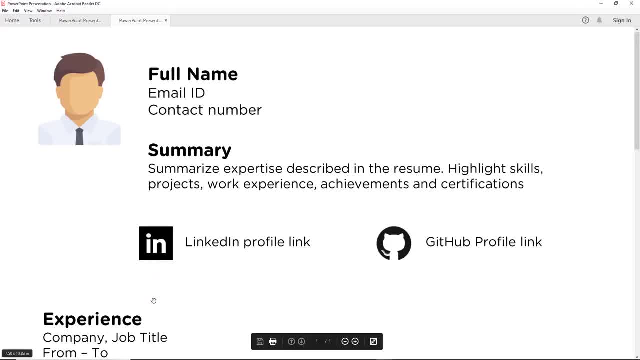 whether it's LinkedIn in this case, which is the business profile most commonly used, GitHub, where you have stuff published, Facebook. I'm always hesitant because that tends to push more towards social media type jobs and other jobs, But certainly there's people who have 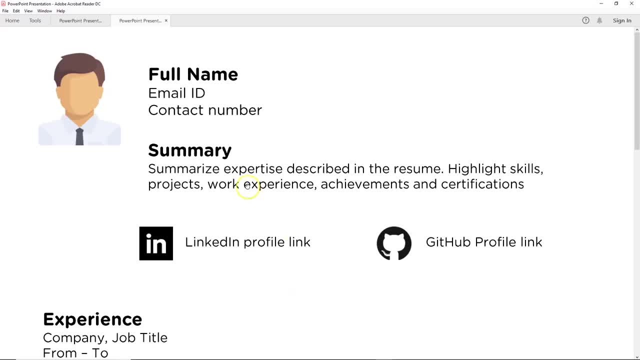 Facebook who do marketing and stuff like that. But these links, having these basic links here, is important. People are starting to look for that for some other setup. Maybe you have a personal website. This is a good place to put that so that they now have a multitude of links that go back to you and highlight who you are. 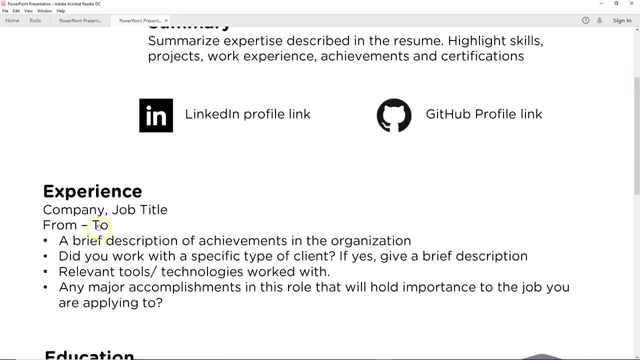 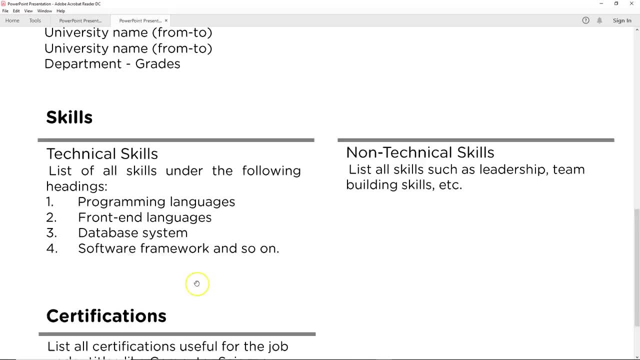 And then the next part or next four parts. So for the next four parts we have a combination of experience, education, skills, certifications, And you can see they're organized If you have. you know, a lot of people like to see what kind of degree you have. 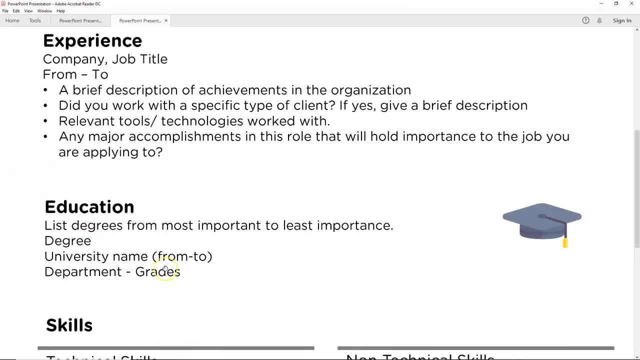 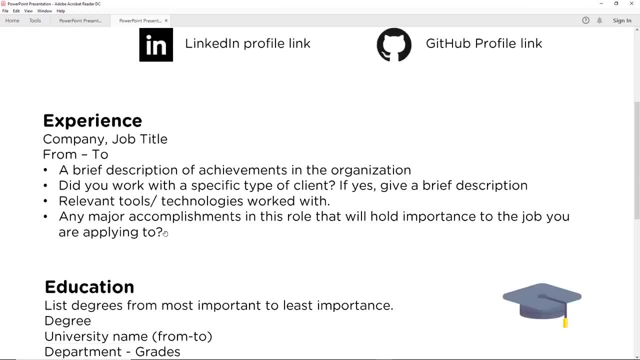 They want to know where it came from. And if you just got out of college, you're going to put education at the top And then maybe you'll put skills after that And then your experience at the bottom. If you've been in the field for years, you know my degree. just to give you my age: 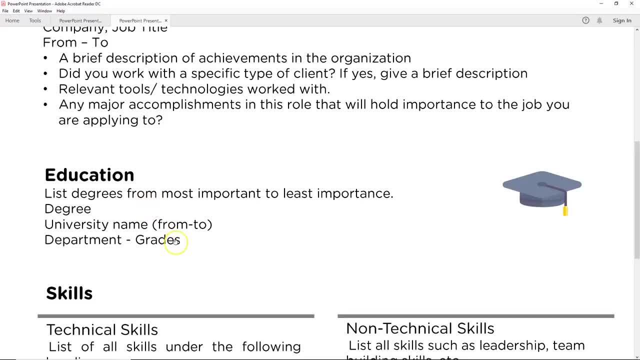 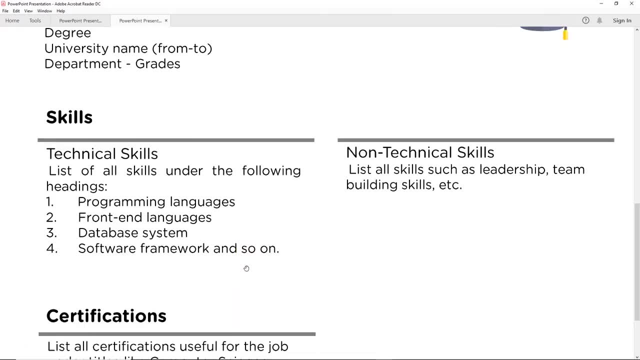 goes back to the early 90s. So I usually put education at the very bottom And then, because a lot of the stuff I'm trying to sell myself on right now is my skills, I actually put that at the top and I'll put my education. 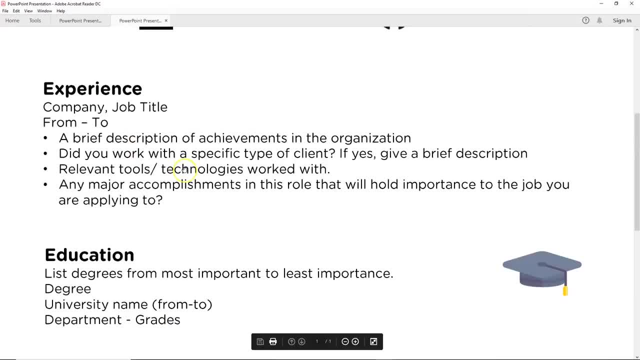 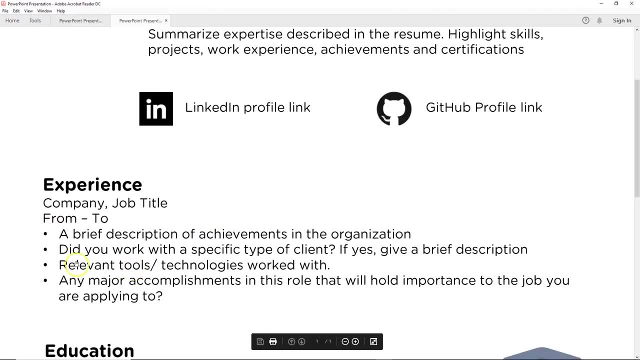 my certifications at the bottom, my skills And then my experience is, since it's a huge part of my resume. goes next: You can organize these in whatever order you want. That's going to work best for you and sell you. Remember you're selling yourself. 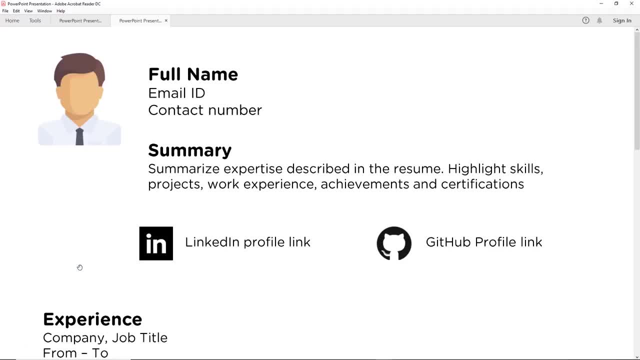 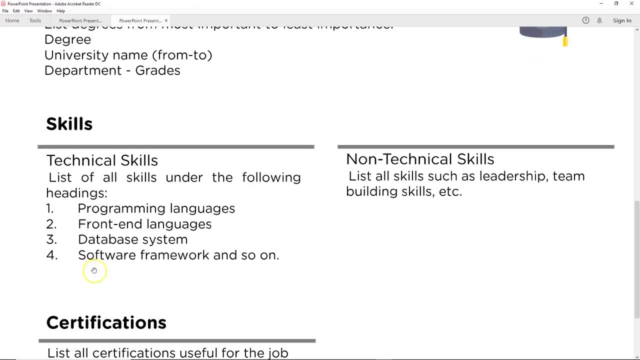 This is your image. Probably don't wear an old tie dye T-shirt with holes in it. You know something nice because it is professional. And of course, your summary, your. and then what do you have to offer the company? Again, when I put out resumes- and I haven't done a resume in a while- 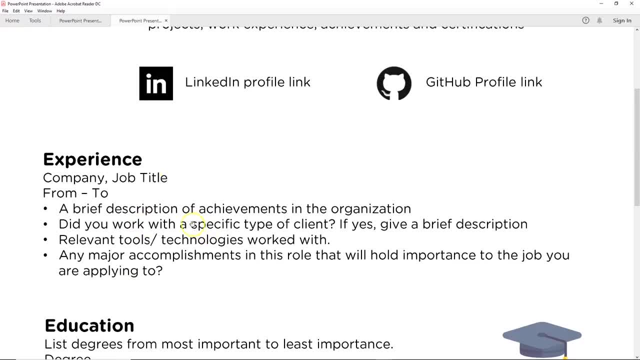 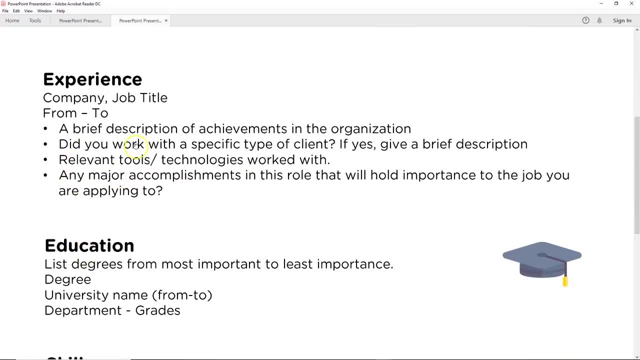 you go in there and you can take this and reorganize this. So if the company is looking for something specific, you might put the experiences specific to that company. You might even take experience if you have like a long job history, like I do. 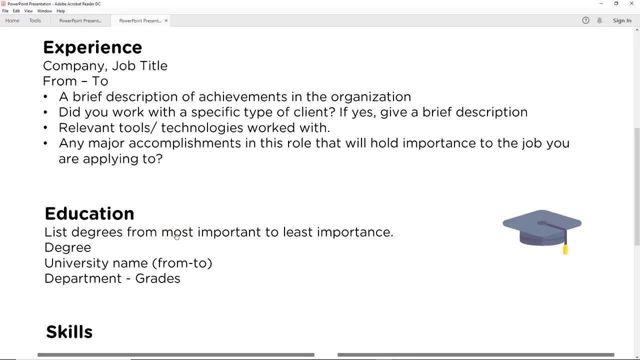 I've gone into a lot of different things. You might leave out those companies or those experiences that had nothing to do with data science, because it just becomes overwhelming. Resume should only take about 30 seconds to glance over, maybe a minute, Maybe a few drops, because after that point you've lost the person's interest. 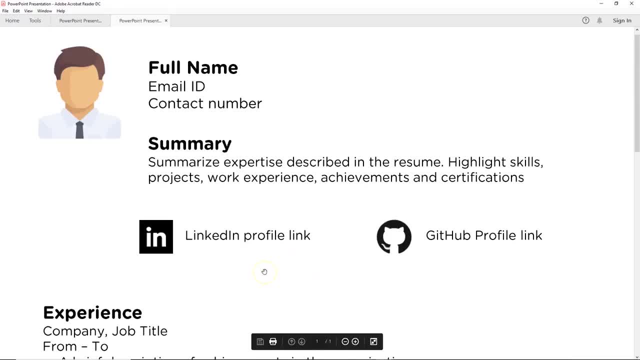 And if they want to dig deeper, they now have links, They have your website, they have LinkedIn and they can now take this and they come back to it and they go: OK, let's look at this person a little closer. So quick overview. 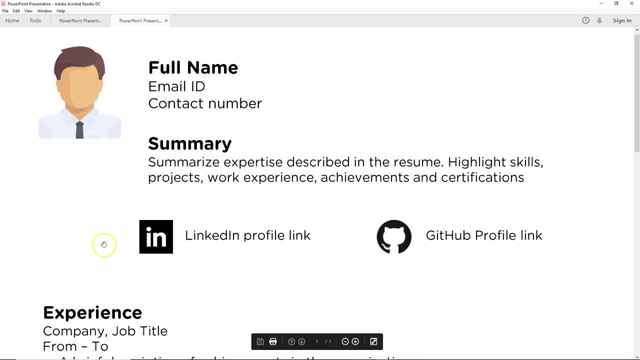 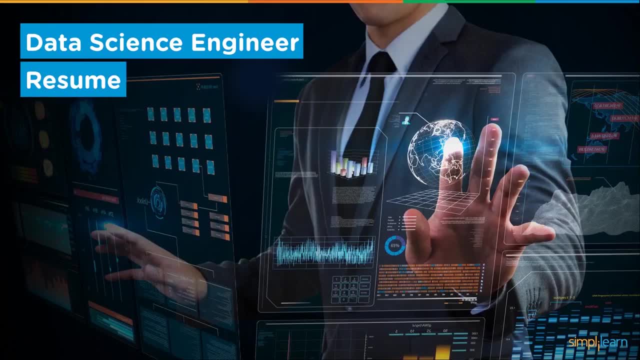 This is your sell sheet selling you to the company. So always tie it to the company so that you have that. What am I going to give this company? What are they going to get from me? We've covered a lot on data science engineer in general. 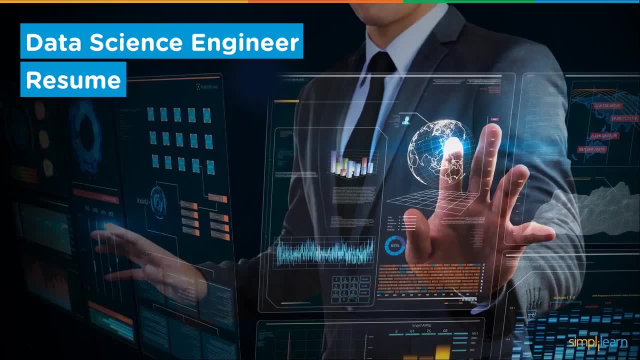 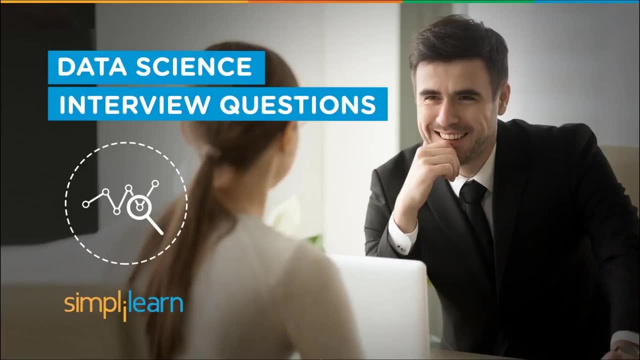 and we've gone over a basic resume. Remember, keep it simple, indirect. That is so important with that resume. Welcome to data science interview questions. My name is Richard Kirshner with the Simply Learn team. That's wwwsimplylearncom. 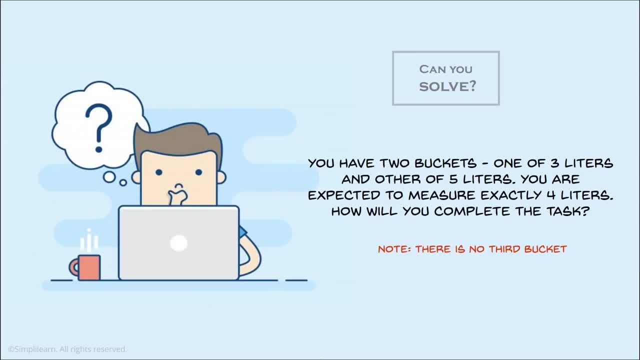 Get certified. get ahead. Before we dive in and start going through the questions, one at a time, we're going to start with some of the logical kind of concept that enters in a lot of interviews. In this one you have two buckets. 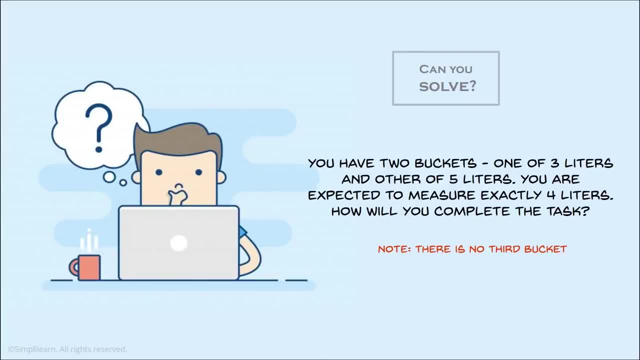 one of three liters and the other five liters. You're expected to measure exactly four liters. How will you complete the task And note you only have the two buckets. You don't have a third bucket or anything like that, Just the two buckets. 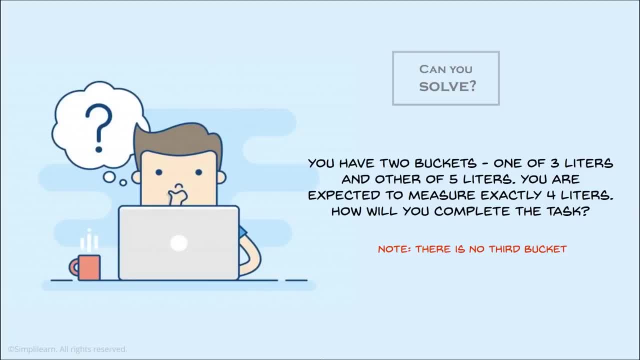 And the object of the question like this is to see how well you are thinking outside the box. In this case, you're in a larger box, You have two buckets and also the pattern which you go on, And what that means is, if you look at the two buckets, 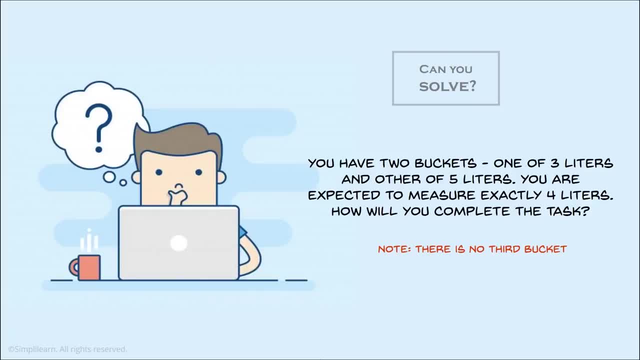 we'll show you their answer in just a second. You have a bucket with three liters and a bucket with five liters, And the first thought is: what happens if you go from left to right- So we have a direction- And what happens if you pour the three liters into the five liter bucket? 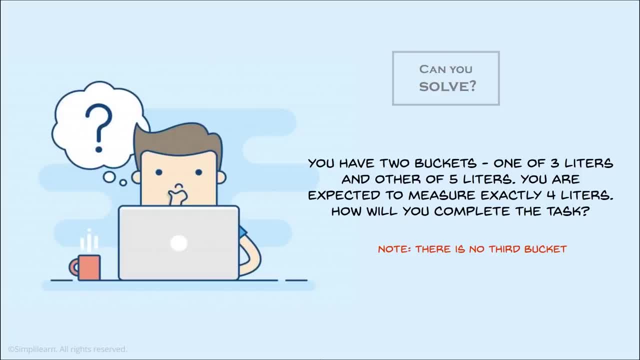 You have an empty bucket of three liters, And what's really important here is thinking outside the box. you realize that you have a five liter bucket that has three liters in it and two empty liters, So you have two additional liters you can fill up. 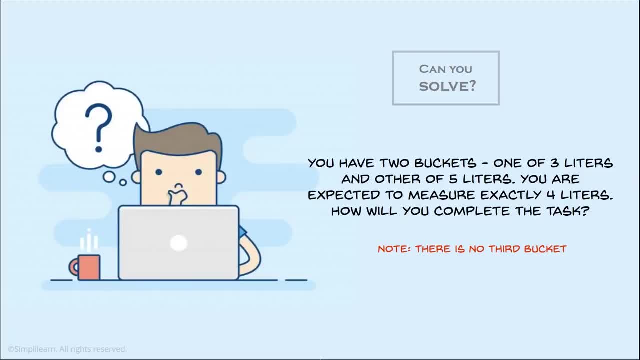 If we continue that process, we can pour from the left to right, from the small bucket to the large bucket. You can now measure in two additional liters into the five liter bucket, And three minus two is one, And you can keep doing that. 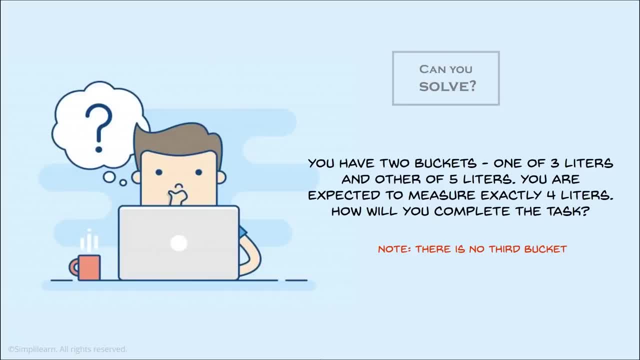 You can empty the five liter bucket in pour those three liters in. That's what you're going to do. You can get one liter in and then you can pour three liters in. What's cool about these questions as you explore them is you realize. 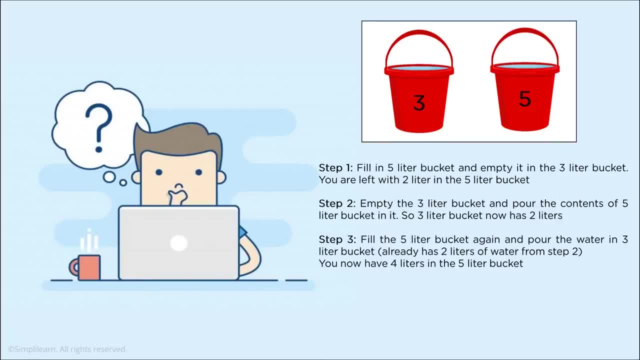 there's multiple ways usually to solve. I went from small bucket to big bucket- The Simply Learn team. their solution that they pulled out was: you fill the five liter bucket and empty it into the three liter bucket. Now you're left with two liters in the five liter bucket. 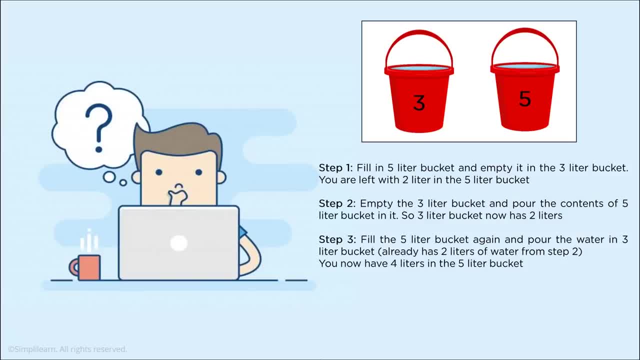 So that's great, We can empty the three liter bucket. So now we're going from large to small. Remember, we went from small to large, So you can go both either way, But you have to go one way or the other, it turns out. 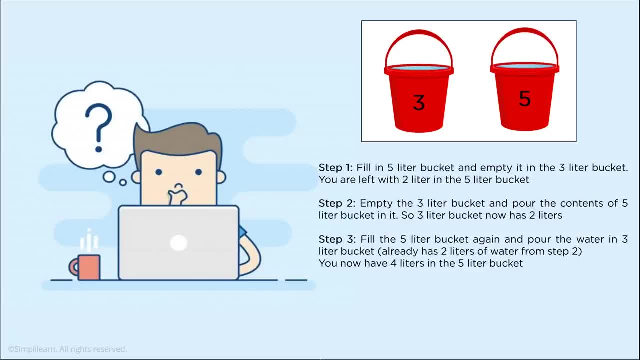 And you can empty the three liter bucket and pour the contents of the five liter bucket in it. So the three liter bucket now has two liters, And if it has two liters that means it has an empty one liter. And by now you probably have guessed that if you have an empty space, 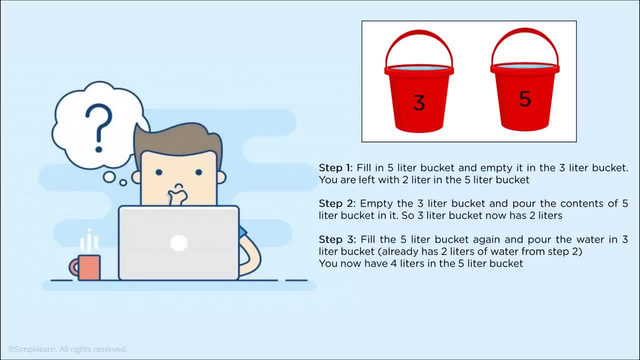 you can start using that empty space of one liter as a measuring. So we fill the five liter bucket again and we pour the water in the three liter bucket that already has the two liters, And so we're only pouring one liter in there, And five minus one is four. 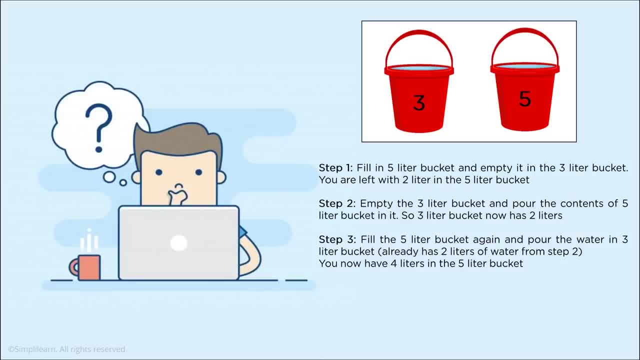 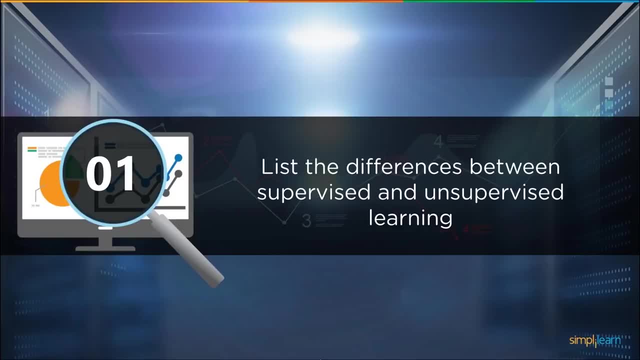 So interview questions. they break up into all kinds of different patterns. We have logic like this one, which is a lot of fun. We have questions that come up that are more about our vocabulary list: the difference between supervised and unsupervised learning- probably one of the fundamental breakdowns in data science. 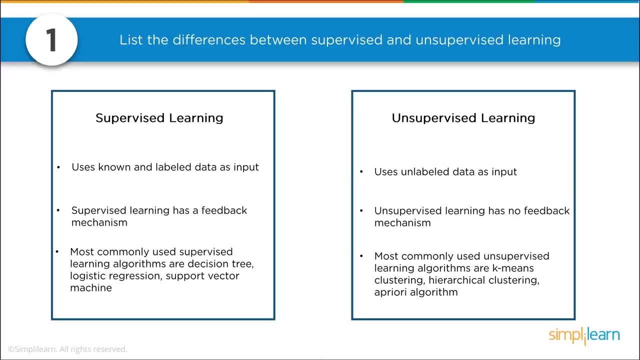 And supervised learning uses known and labeled data as input. Supervised learning has a feedback mechanism. Most commonly used supervised learning algorithms are decision tree, logistic regression support vector machine, And you should know that those are probably the most common use right now. 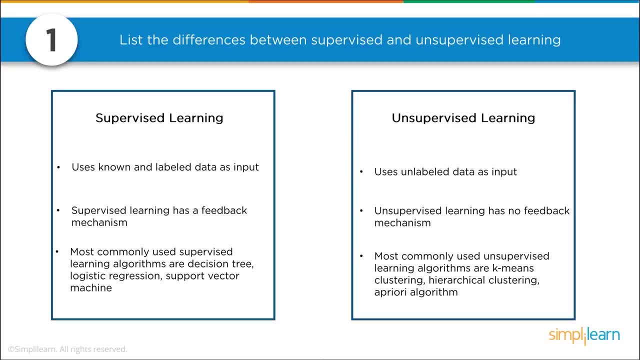 And there certainly are so many coming out. So that's a very evolving thing, And be aware of a lot of the different algorithms that are out there outside of the deep learning, because a lot of these work faster on raw data and numbers than they do than a deep neural network would. 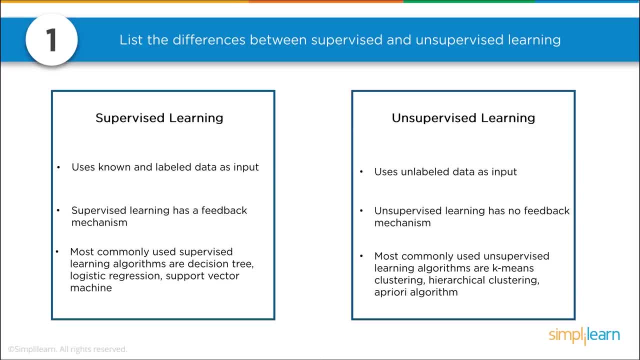 Unsupervised learning uses unlabeled data as input. Unsupervised learning has no feedback mechanism. Most commonly used unsupervised learning algorithms are k-means clustering, hierarchical clustering, the aporial algorithm, And there certainly are more. I'm going to say k-means definitely is at the top of the list. 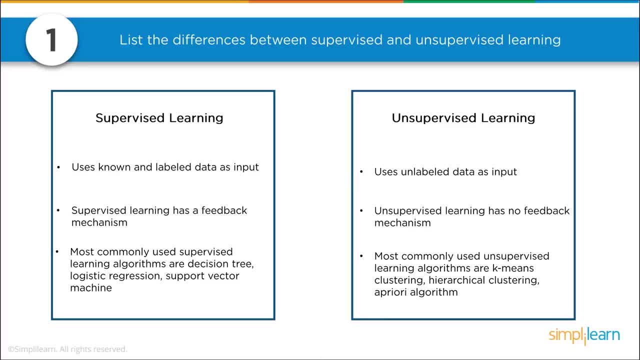 And the hierarchical clustering. those two are used so many times, So really important to understand what those are and how they're used. And most important is understand that supervised learning is. you have your data set where you have training data and you have all those different pieces. 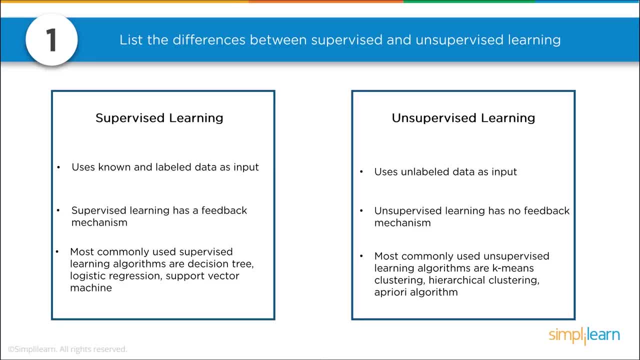 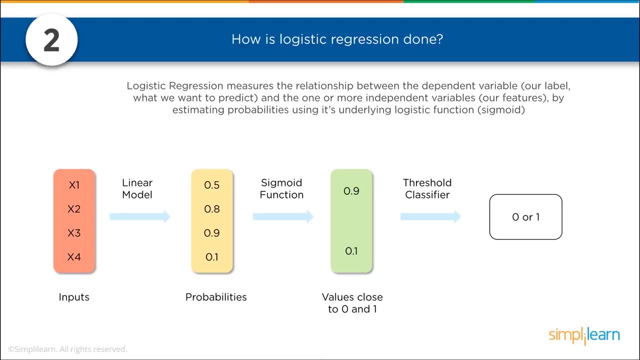 moving around, but you're able to train it, You know the answers And, unsupervised, we're just grouping things together that look like they go together. How is logistic regression done? Logistic regression measures the relationship between the dependent variable, our label- what we want to predict- and the one or more independent variables. 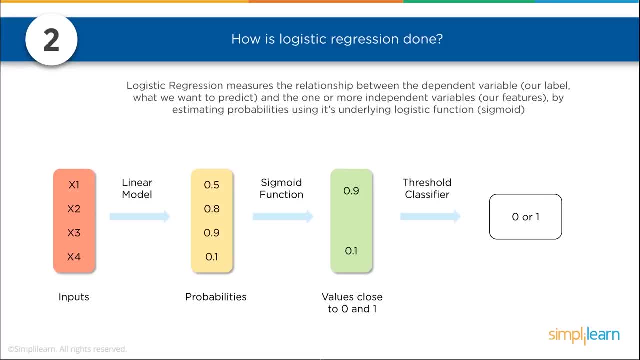 our features by estimating probability using its underlying logistic function, sigmoid. And whenever I draw these charts, I always end up drawing them the right-hand side first, because you want to know what your output is. what is it you want out of here? 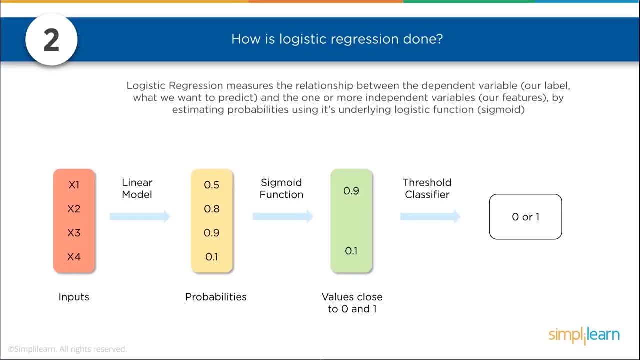 And the left-hand side. what do you have going in? So you have your in and out. You can see we have a nice labeled image here. to help you remember this: We have our inputs, We have our linear model, We have our probabilities. 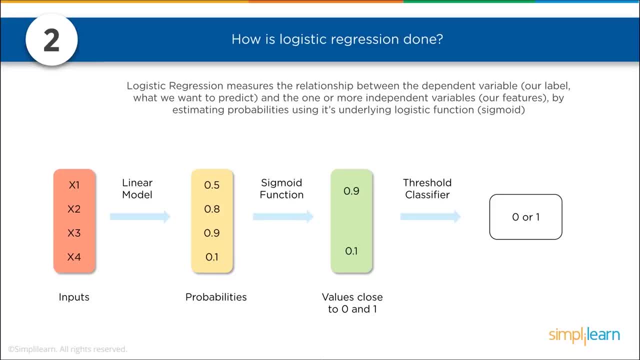 What are the probabilities of it being a certain way based on these features coming in The sigmoid function- And it's important to note that the sigmoid function is maybe the most commonly used, but it's only one of a number of functions that are out there. 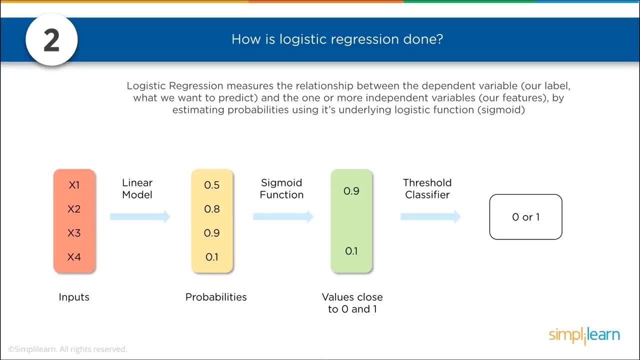 And the sigmoid function turns our probabilities into a value between 0 and 1, or very close to 0 or very close to 1, between 0.1 and 0.009.. And based on that we generate an answer, in this case, of 0 or 1.. 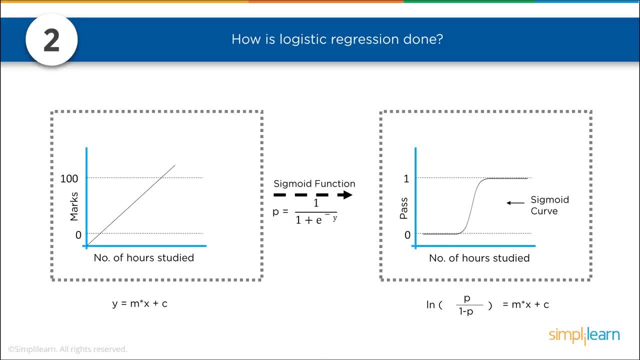 How is logistic regression done? So last time we talked about the sigmoid function. Generally, depending on what's your interview and level of math and what expertise you're going in for the market, you'll have to understand that formula of the probability equals 1. 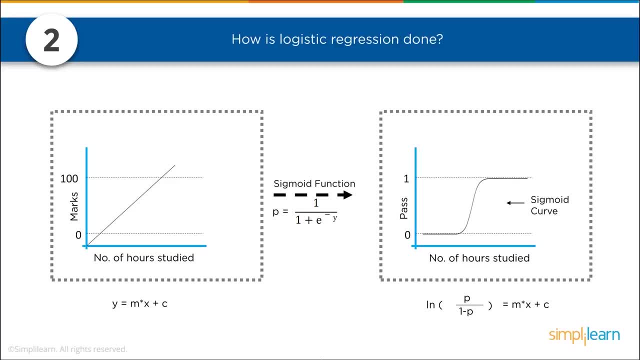 over 1, plus e to the negative y, And that's e to the base 2.. So you have your probability function or your sigmoid function, which pushes it. As you can see, we have a nice visual of that And that helps a lot to have that visual on the sigmoid function. 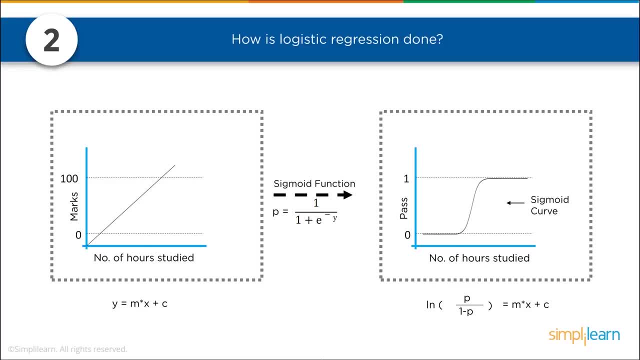 You definitely should know. your y equals m times x plus c, your basic Euclidean geometry of forming a line in the slope, plus the intercept, the y-intercept, And then you have your natural log, And the natural log is to the e, as opposed to base 2 or base 10.. 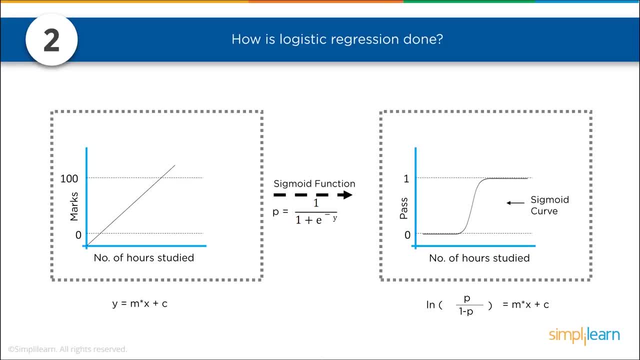 So your natural log to the e of the probability over 1 minus a probability equals your m times x plus c or your Euclidean line. That helps a lot as far as the graphing and understanding the sigmoid function. So we'll just keep pushing on. to question number three: 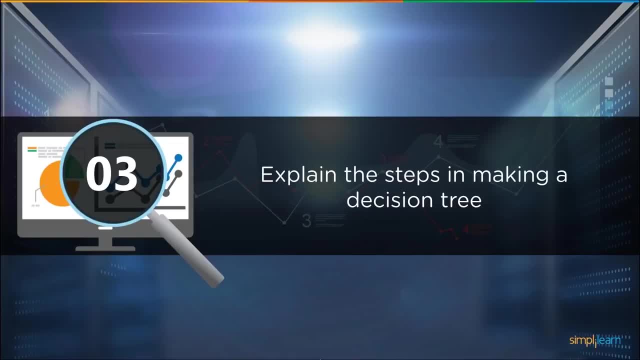 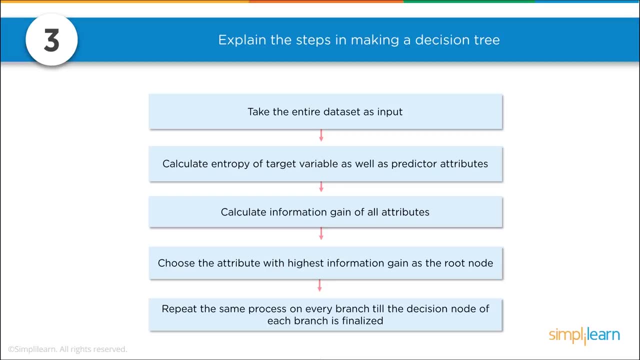 Explain the steps in making a decision tree, And I noticed last time we brought up the decision tree in the forest a lot of questions came up. What is the difference? So let's go through that: When you make a decision tree, you're going to take the entire data set as input. 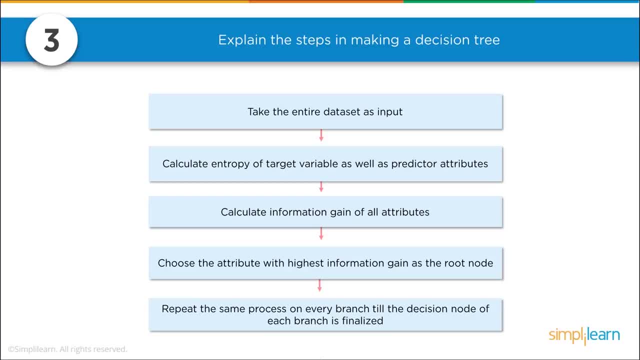 You're going to calculate entropy of the target variable as well as the predictor attributes. I remember entropy is just how chaotic is it? So if you have, like you know, banana and grapes and oranges, if you're mixing in fruit, and that's your data coming in? 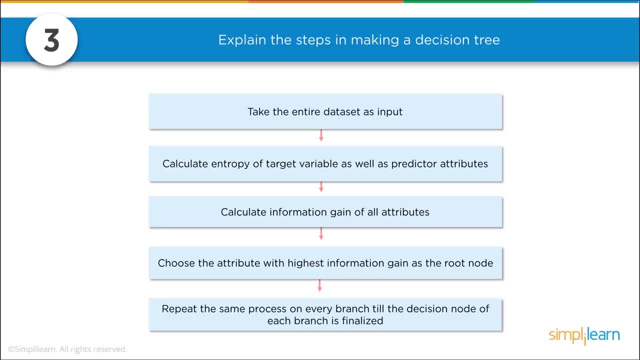 you have all these different objects that are so separate from each other, And the more they become uniform, the lower the entropy, And we call that information gain. So we gain information on sorting different objects from each other. So you have your entropy. 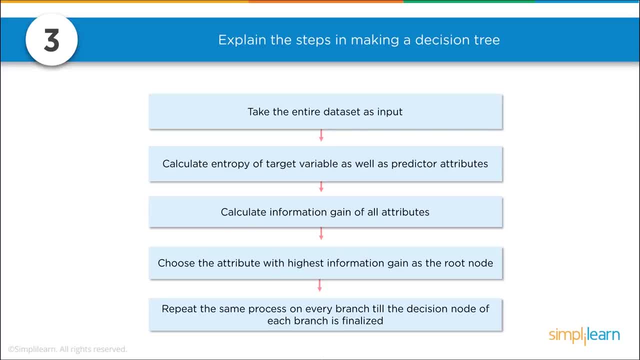 You have to calculate your information gain of all attributes And then you choose the attribute with the highest information gain as the root node. So if you can separate your group and each group, chaos in each group is lowered. whichever split lowers the chaos the most. 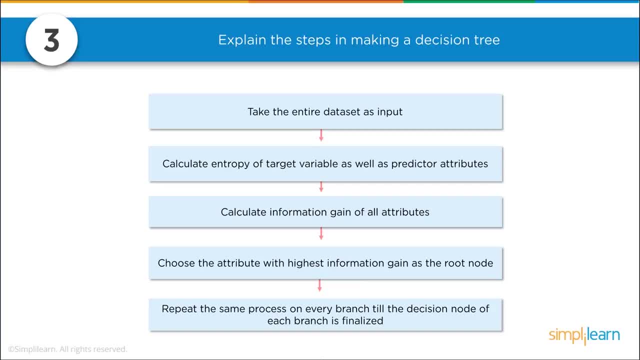 that's where you split it And that's your root node. At that point you repeat the same procedure on every branch till the decision node of each branch finalized. So understanding that setup is pretty important as far as decision trees- And you can see here we have a nice visual of a decision tree- 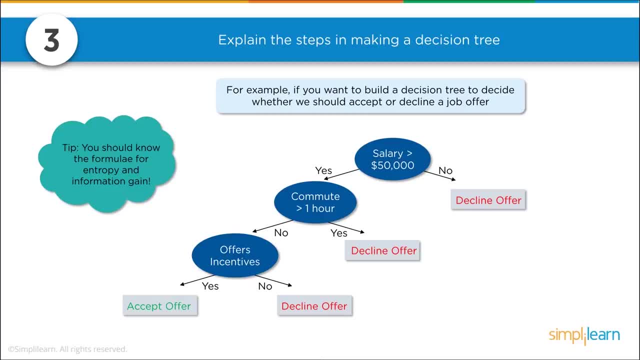 For example, if you want to build a decision tree to decide whether we should accept or decline a job offer. since these are interview questions, that's a good one to ask And, just as a tip, you should be pretty aware of the formula for entropy and information gain. 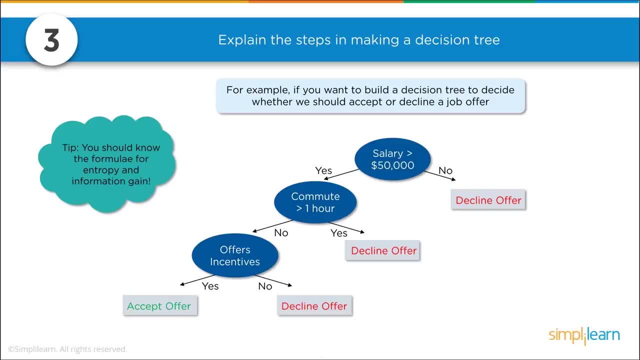 So you need to look those up if you don't remember those. And the salary: if it's greater than $50,000, no decline the offer. Yes, it's got a good salary. The commute is greater than an hour. 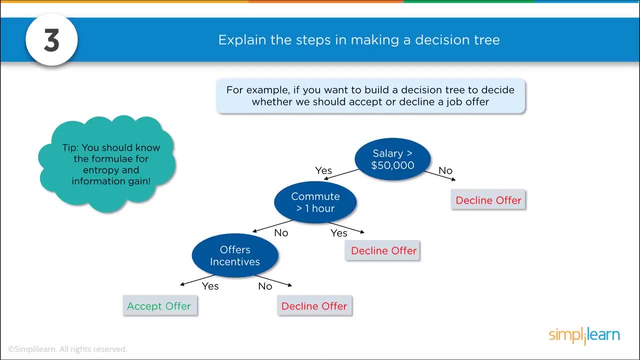 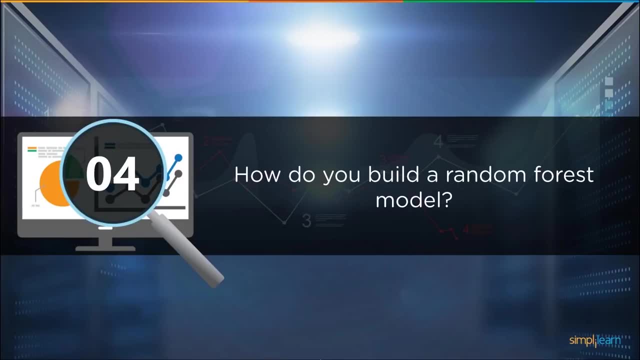 Yes, decline the offer. No offers incentives. Yes, accept the offer, No incentives, decline the offer. So we use decision tree pretty much for everything. if you want And if you have a decision tree, then you also should understand how do you build a random forest model. 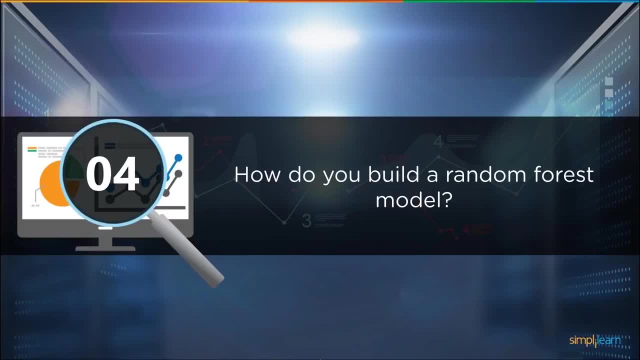 And remember that a random forest is build up of a number of decision trees. So if you split your data up into a lot of different packages and you do a decision tree in each of those different groups of data, the random forest is bringing all those trees together. 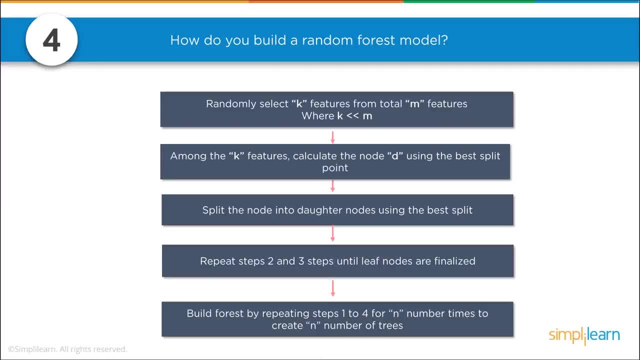 So how do you build a random forest model? Randomly select K features from a total of M features. where K is less than M Among the K features, calculate the node D using the best split point. Split the node into daughter nodes using the best split. 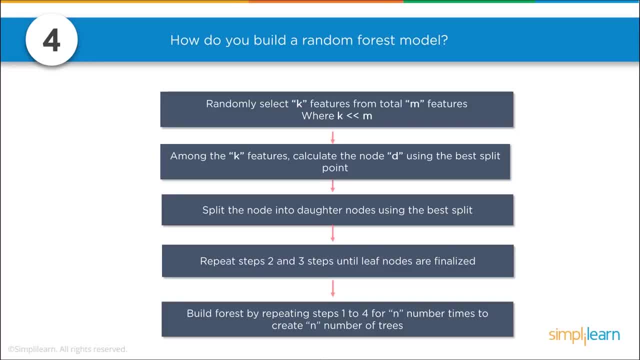 Repeat steps two and three steps until leaf nodes are finalized. Build forest by repeating steps one to four for N number times to create N number of trees. So you can see it's got the same build pattern as the tree, but instead you're building a number of different trees. 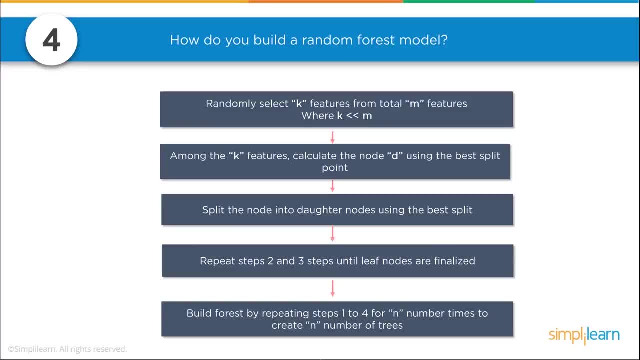 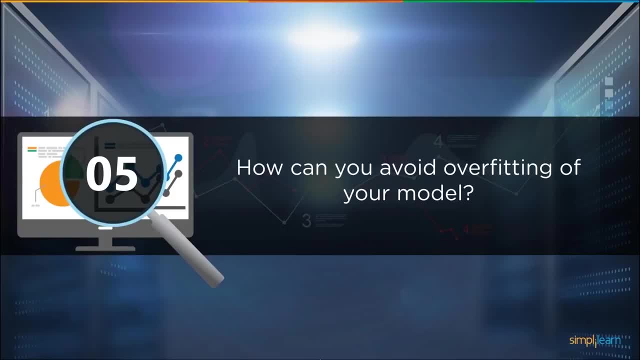 little small trees, so it all have an N leaf node. Random forest has a vote at the end and whoever gets the most votes wins. That's the answer. How can you avoid overfitting of your model? Very important question in any kind of mathematical. 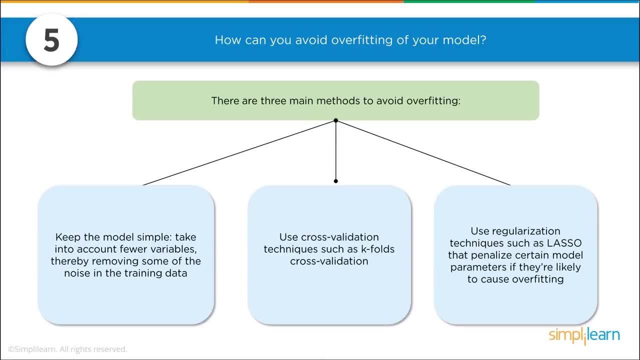 scientific data science setup in any of them. There are three main methods to avoid overfitting And you should really understand overfitting. Overfitting means that your model is only set for a very small amount of data and ignores the bigger picture. 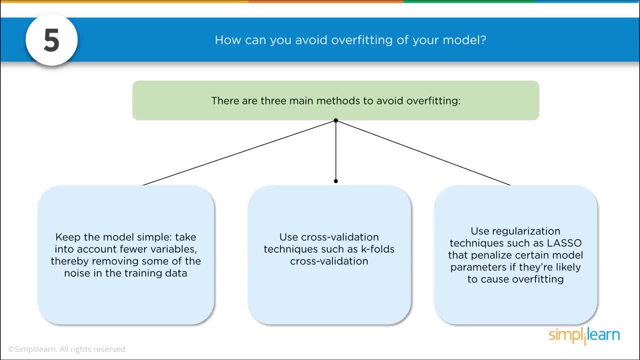 Keep the model simple. Take into account fewer variables, thereby removing some of the noise in the training data. Good advice for any programming at all: Use cross-validation techniques such as K-folds cross-validation. Use regularization techniques such as LASSO that penalize certain model parameters if they're likely to cause overfitting. 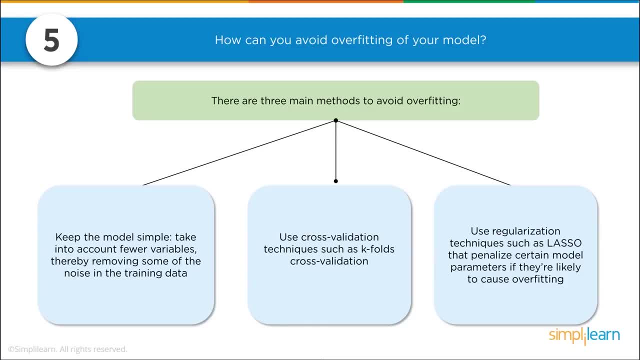 And you should also be well aware that your cross-validation techniques- that's like a pre-data or your LASSO and your regularization techniques are usually during the process. So when you're prepping your data, that's when you're going to do a cross-validation. 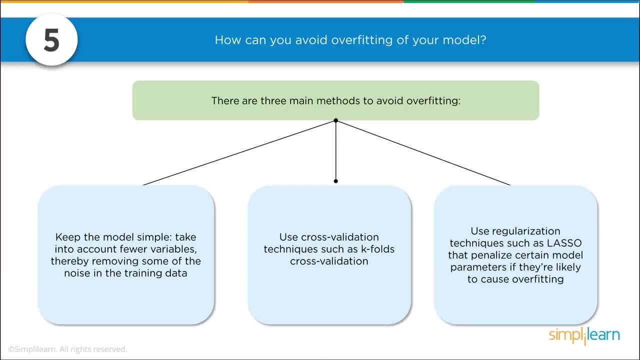 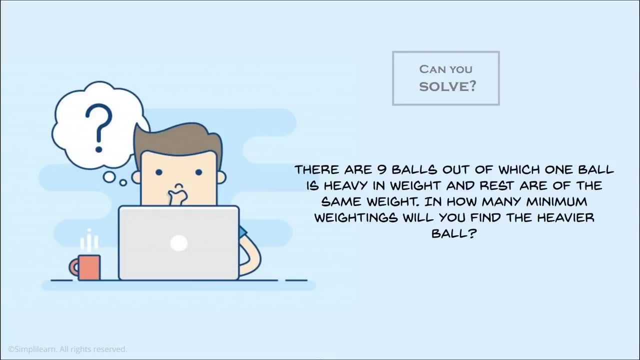 such as like splitting your data into three groups and you train it on two groups and test it on one and then switch which two groups. you tested on that kind of thing, So can you solve another one of these? I love these things. There are nine balls, out of which one ball is heavy in weight. 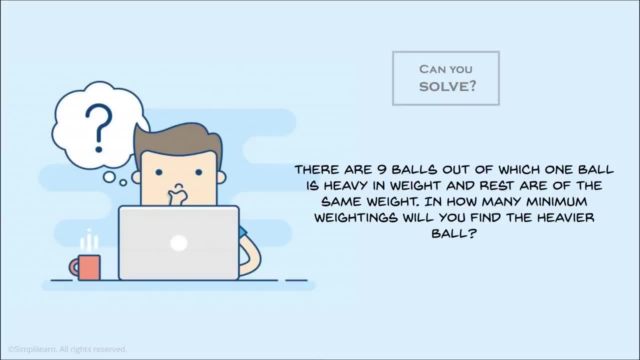 and the rest are of the same weight And how many minimum weighings will you find the heavier ball? When we say weighing, think of a scale where you can put objects on one side and the other and you can see which side is heavier. 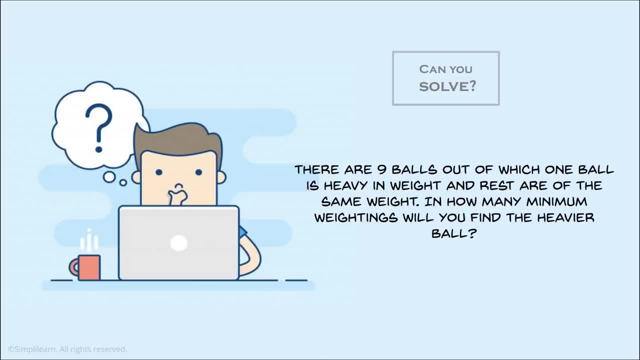 And you want to minimize that. You want to split the balls up in such a way that you're going to do as few measurements as you can. You will need to perform two weighings, So you can get it down to just two weighings. 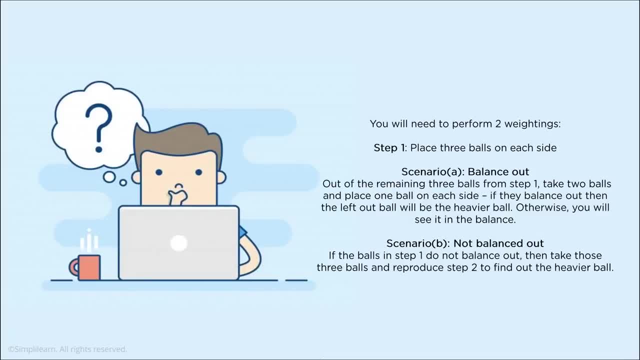 And I always think if there's nine balls, I'm going to divide them into three groups of three, Place three balls on each side So you can just randomly pick six of the balls, and three on one side, three on the other, And if they balance out, both sides are equal. 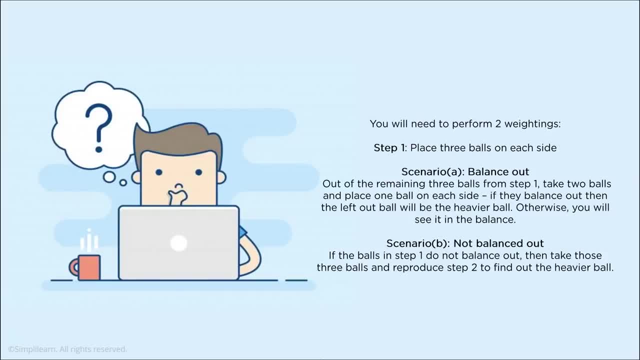 then you know the heavy weight isn't in any of those. So out of the remaining three balls from step one, take two balls and place one ball on each side. A little tricky there, because I always want to put all three. I want to put two on one side and one on the other. 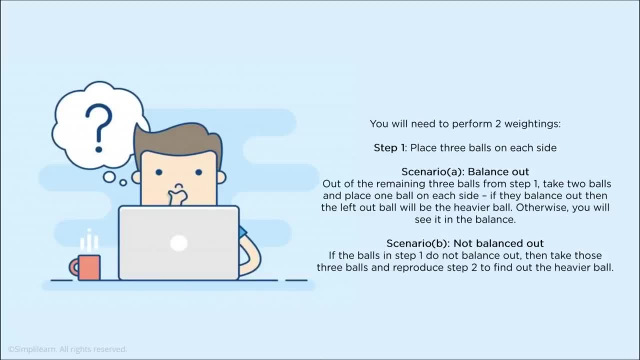 But no, just randomly pick two of those, put one on each side. If they balance out, then the left out ball- the one you didn't measure- will be the heavier one. Otherwise you'll see it in the balance. You'll see which one's heavier because it'll take one of the balls down. 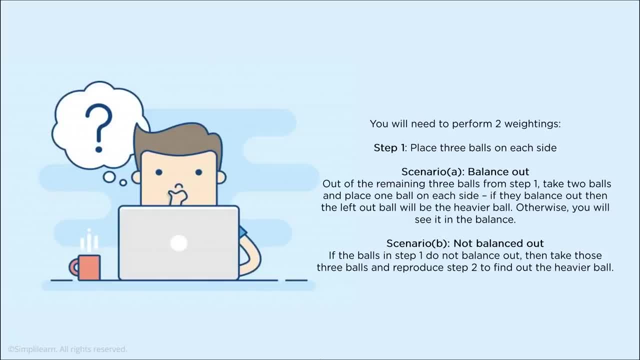 Now we go to scenario B, where they did not balance out. So now we know which side has a heavier ball in it, And it's just very similar to what we did before. If the balls in step one do not balance out, then take those three balls that had the heavier side on them. 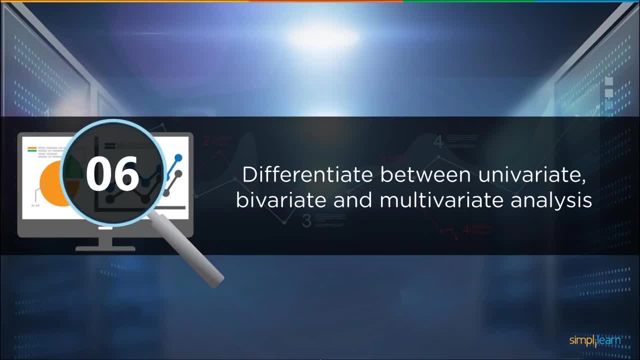 and reproduce. step two, to find out the heavier ball Difference between univariate, bivariate and multivariate analysis. And hopefully, if you know a little Latin, you'll kick in there that you have uni and you have bi and you have multi. 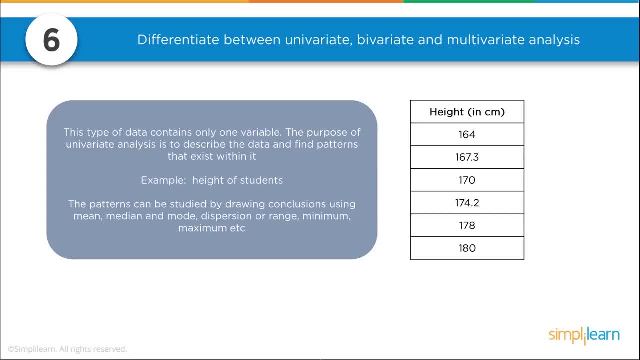 because the answer is in the words themselves. So the first one: this type of data contains only one variable, So that's the univariate. The purpose of the univariate analysis is to describe the data and find patterns that exist within it. So when you only see one variable coming in, 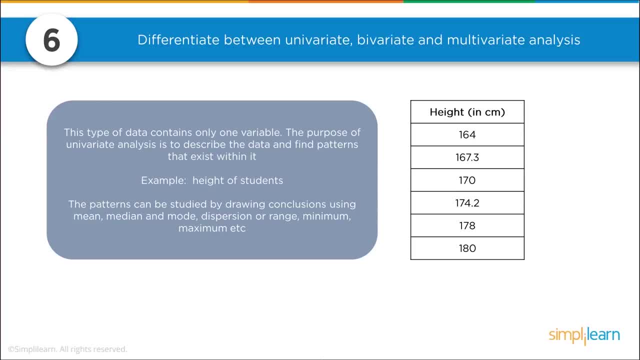 in this case we're using height of students. you're limited as far as what you can do with that data, So you can come up and draw different patterns and conclusions from those patterns using the means, the median, the mode, dispersion range: minimum, maximum. 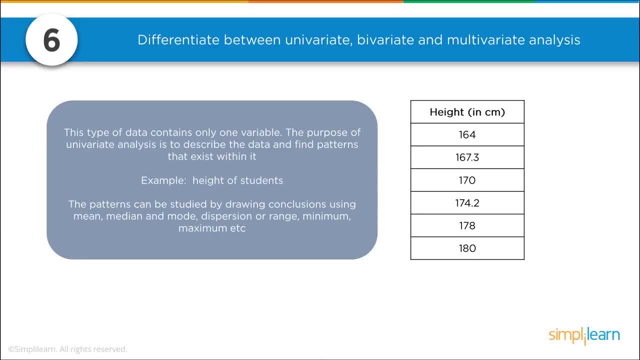 So we're describing the data. So all those words would describe the data And that's about all you can do. with data like that. There's no correlation, There's nothing to go beyond that as far as guessing or predicting anything, So we move into bivariate. 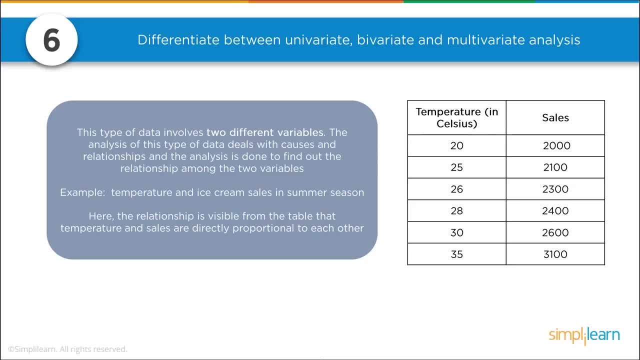 You know, uni means one, bi means two: Bivariate. this type of data involves two different variables. The analysis of this type of data deals with causes and relationships And the analysis is done to find out the relationship among the two variables. 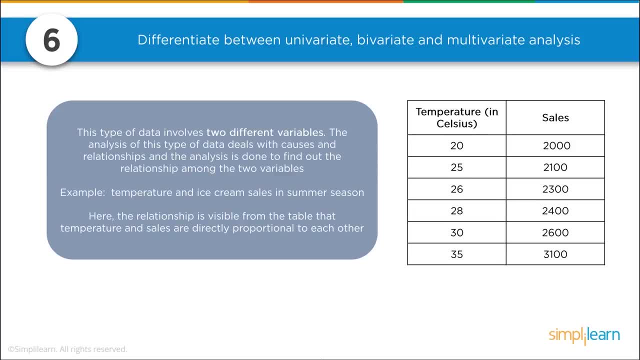 And this is always a favorite one, because everybody loves ice cream in the summer, when it's hot, and very few people go for ice cream in the winter, when it's really cold. So it's easy to see the correlation in the data: the temperature and ice cream cells. 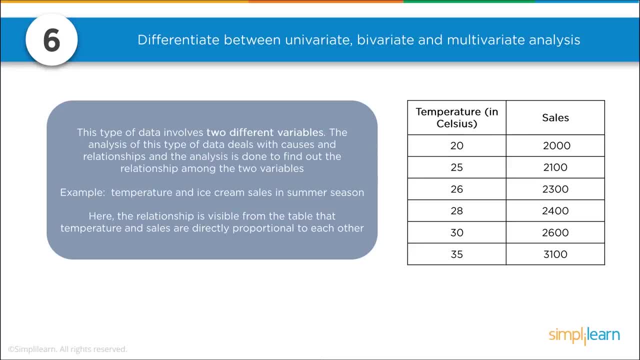 in summer season, And you can see here where the temperature goes from 28 to 35. And as the temperature goes up, so does the sales of ice cream. It goes from 2,000, I'm not sure 2,000 to what. 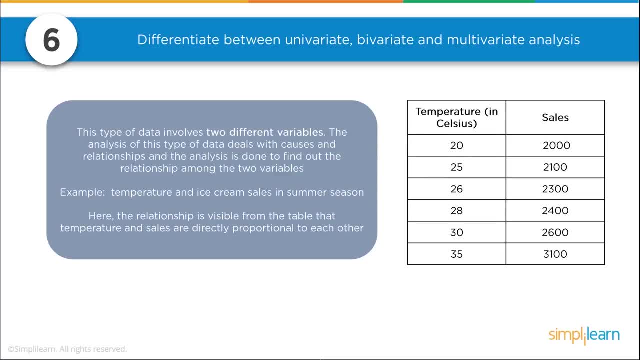 So I'm guessing it's a very large chain, because if they're selling 2,000 ice cream cones and they have a lot of business, good for them. A little vendor on the corner selling 2,000 ice cream cones a day and 3,100 the next day. 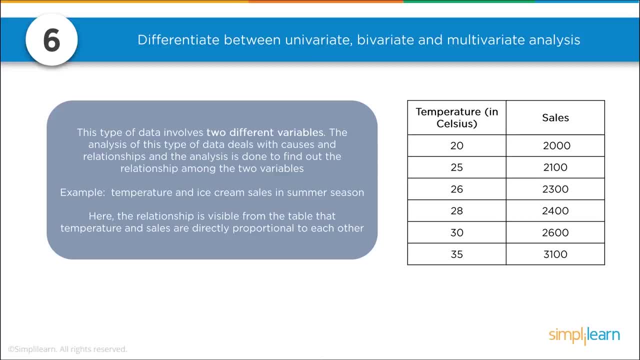 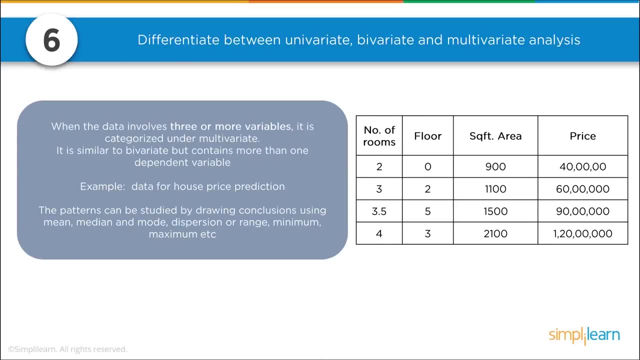 Here the relationship is visible from the table that temperature and cells are directly proportional to each other. So the hotter the temperature, we can predict an increase in sales. So the word prediction should come up. So we have description and prediction. When the data involves three or more variables, it is categorized under multivariate. 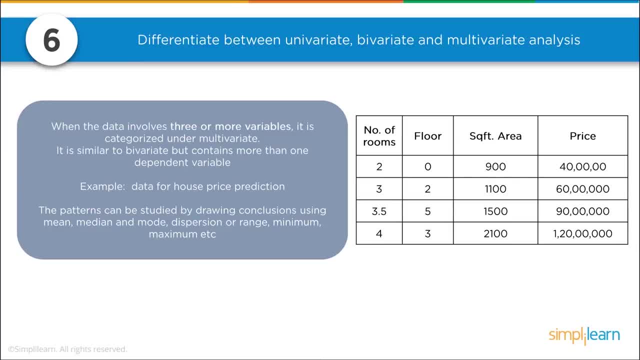 It is similar to bivariate but contains more than one dependent variable. In this example, another really common one: the data for house price prediction. the patterns can be studied by drawing conclusions using mean, median and mode dispersion or range minimum, maximum, et cetera. 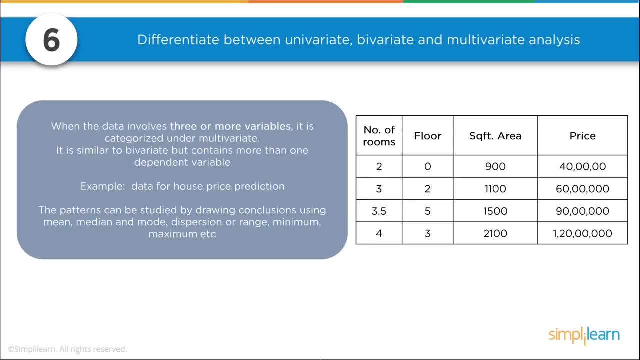 And so you can start describing the data- that's what all that was- and then using that description to guess what the price is going to be. So this is very good if you're in the market and you have already looked at the area and 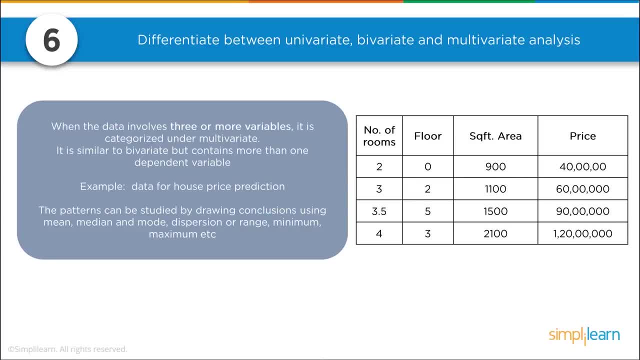 you already know that a two bedroom, zero floor, 900 square foot house usually runs about 40,000,. you can guess what the next one that looks similar to it is. And I'll just throw in another word in there. I don't see very often, unless you're really a hardcore data science. we talked about 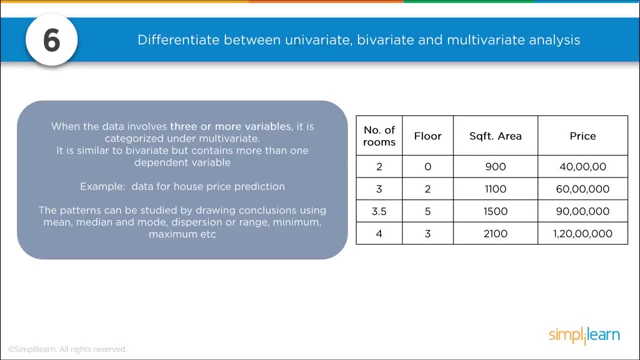 describing the data descriptive. we talked about predictive, and there's also postscriptive. Postscriptive means we're going to change the variables to try to guess what the outcome is if we change what's going on. So that would be the next step. 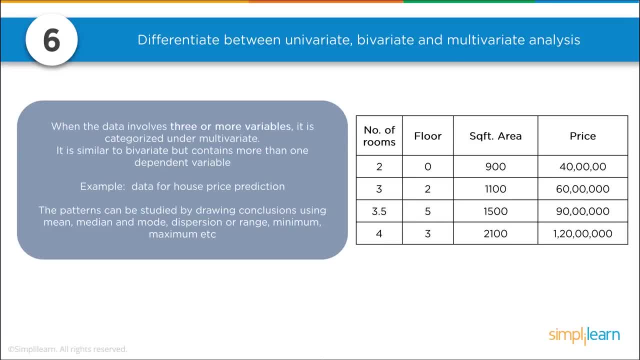 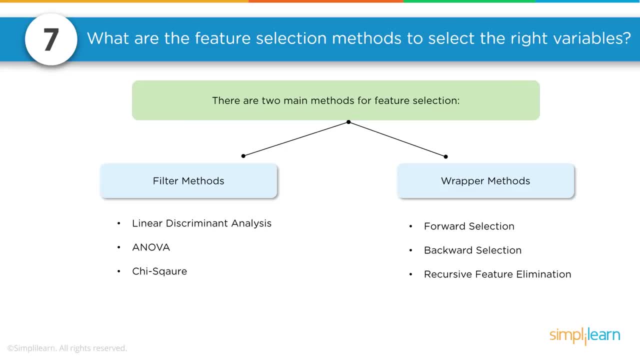 That usually doesn't show up, unless you're dealing with some really hardcore data science groups. What are the feature selection methods to select the right variables? There are two main methods for feature selection. There's filter methods and wrapper methods, And when you're filtering your before. we discuss the two methods real quick. 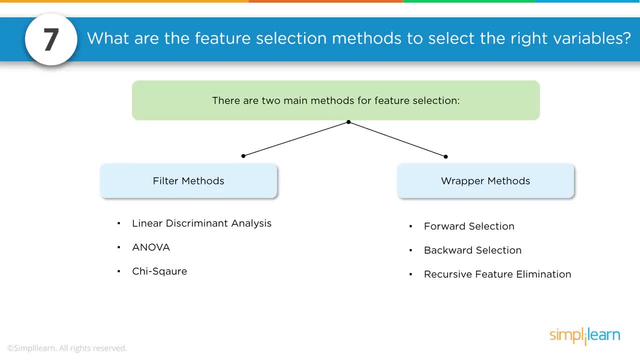 the best analogy for selecting features is: bad data in, bad answer out. So when we're limiting or selecting our features, it's all about cleaning up the data coming in so it's cleaner and is more representative of what we're trying to predict. 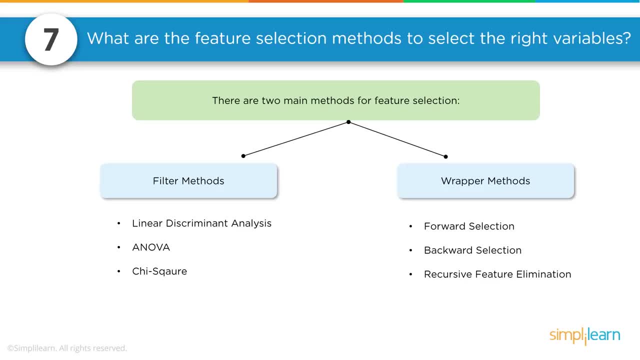 Filter method: Filter methods as they come in. we have linear discrimination analysis, ANOVA, chi-squared- chi-squared is probably the most common one- And these are all part of pre-processing. We're taking out all the outliers, all the things that have a difference, that is. 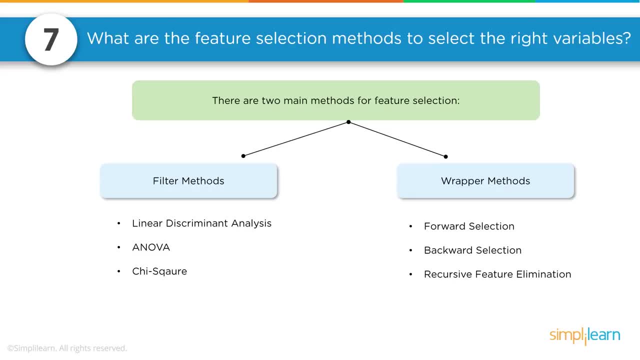 very different from the data. we're looking at the odd ones And sometimes you take the odd ones out and then you analyze them separately to see why they're odd. But remember your filter methods. You don't have to pull all that weird stuff out. 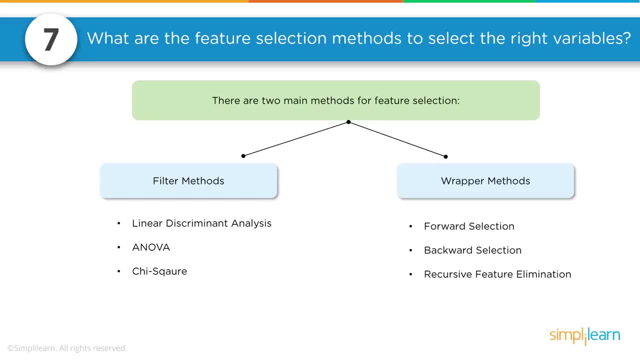 Wrapper methods, on the other hand, are forward selection, backward selection, recursive feature elimination, And one of the most important things to remember about wrapper methods is they're very labor-intensive. You have to have some pretty high-end computers if you're doing a lot of data analysis with the wrapper method. 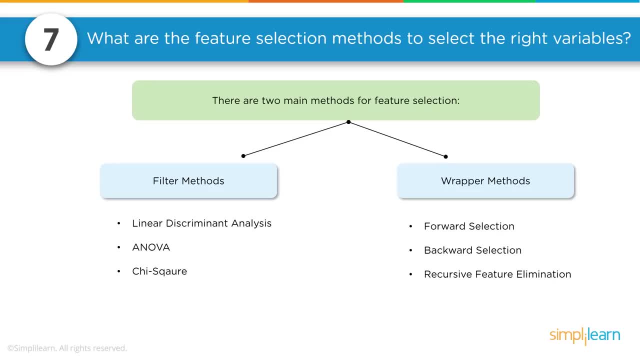 And just quickly forward. selection means you have all your different features. They're off to the side and we test just one feature at a time. We keep adding them in until we get a good fit Backward And then we start removing features and we run a test on that to see how well it does. 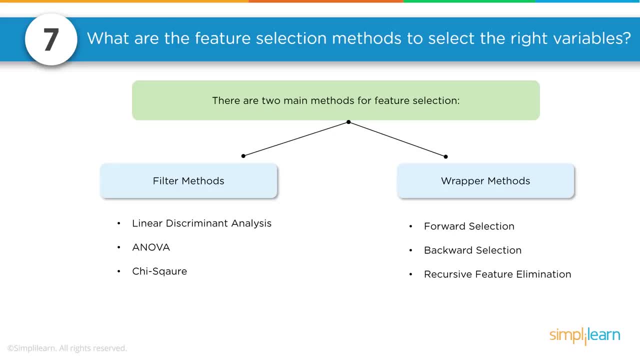 And then we start removing features to see what works, And recursive, which is the most processing-hungry algorithm out there, goes through and just recursively looks through all the different features and how they pair together. But again we have filter method and wrapper method. 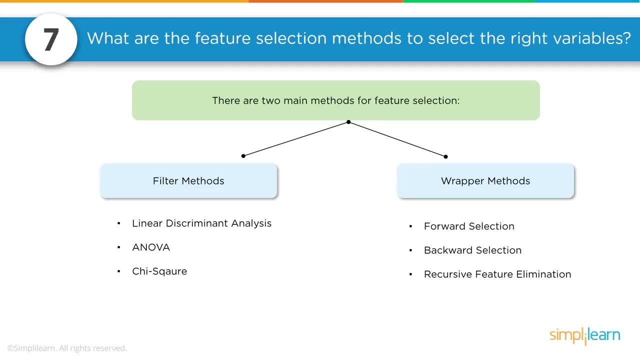 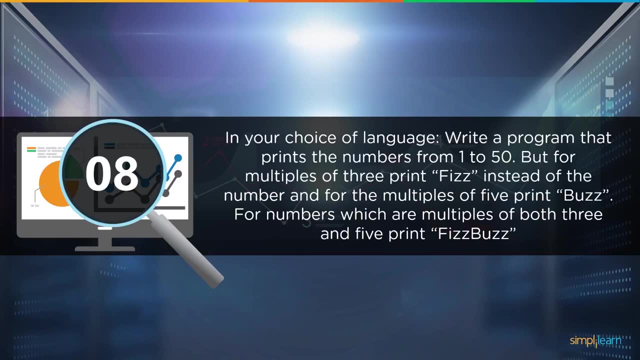 And it's important to understand that we're sorting the data out and finding out which features are going to represent the data the best and which ones are not going to really add any value to our models. Let's jump to number eight In your choice of language. 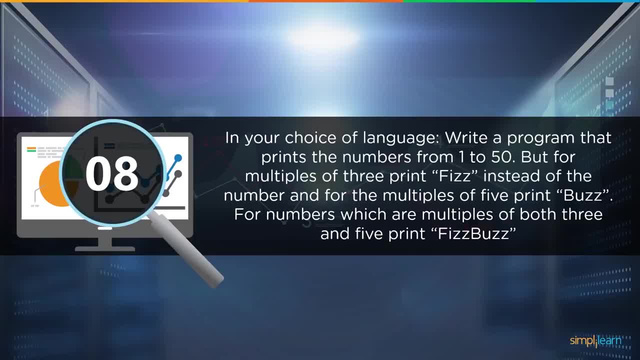 write a program that prints the numbers from 1 to 50. But for multiples of 3, print fizz instead of the number. And for the multiples of 5, print buzz. For numbers which are multiples of both 3 and 5, print fizz-buzz. 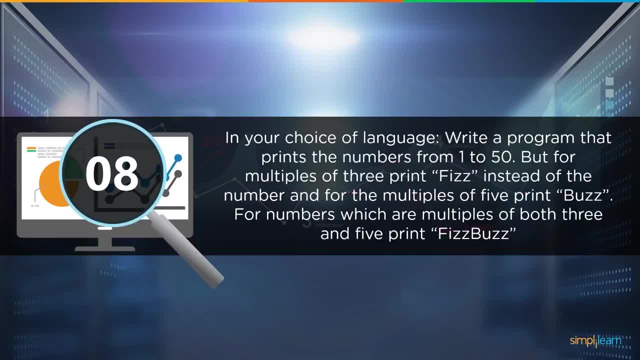 And this really is testing your knowledge in iterating over data Very important. My sister, who runs the university the data science team, is in charge of their department. The first question she asks in her interview of anybody who comes in is: how do they iterate through data? 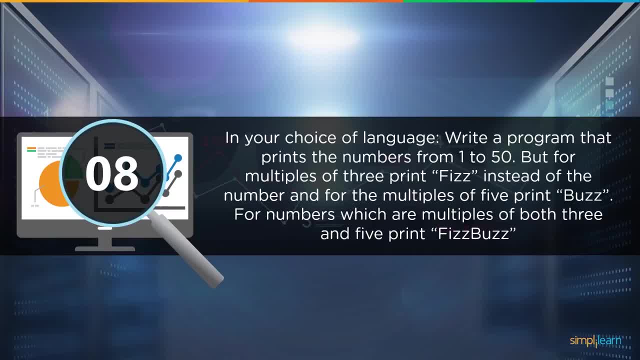 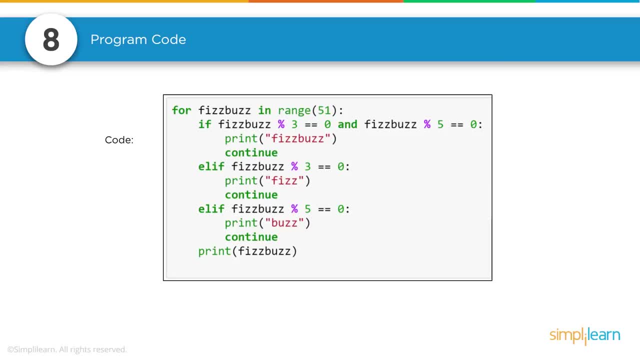 So this question comes up a lot and it's very important you have an understanding. And there's actually a slight error on this code which I'll point out in just a second. The concept is we have fizz-buzz in range. You have range 51, which in this case goes from 0 to 51.. 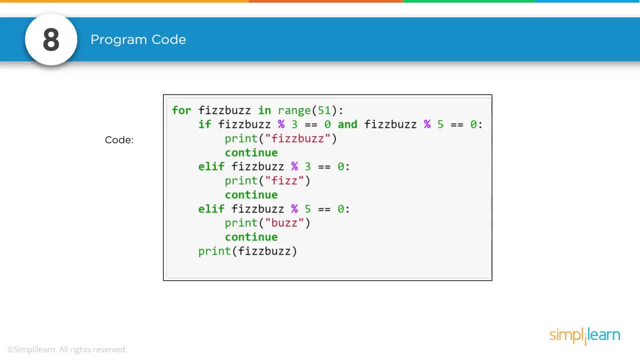 And I'm going to challenge you to see if you can catch the error, And I'll tell you at the end of the code where the error is. What that means is that we're going to go through all the numbers 0,, 1,, 2,, 3,, 4.. 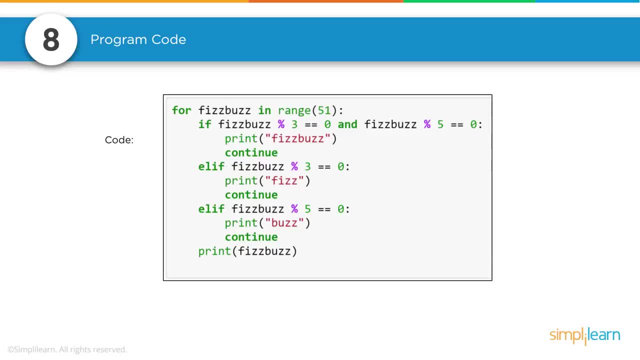 And we're going to process through this loop. Fizz-buzz divided by 3 equals 0.. And fizz-buzz divided by 5 also equals 0. Then print fizz-buzz, Continue, And else, if fizz-buzz divided by 3 equals 0.. 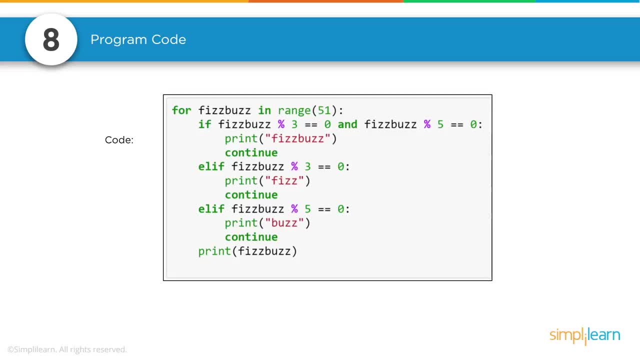 Then print fizz. Print fizz, Continue, Else if fizz-buzz divided by 5 equals 0.. Print fizz-buzz, Continue. And print fizz-buzz. You print the answer. In this case, fizz-buzz is either going to be the number we generated, which is 0.. 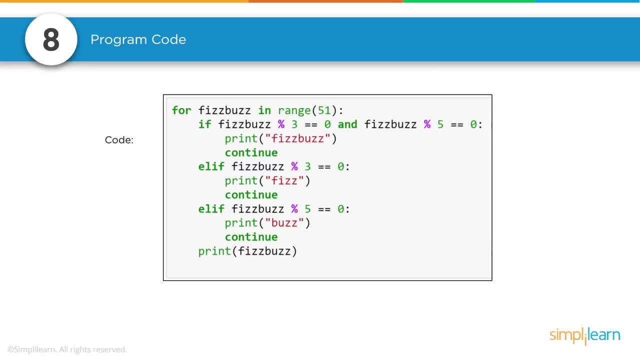 Or it will be the fizz-buzz: fizz or buzz. Whew, that's a mouthful. Now, if you didn't catch the error in the code- which is always a fun game- find the error. It has to do with the range. 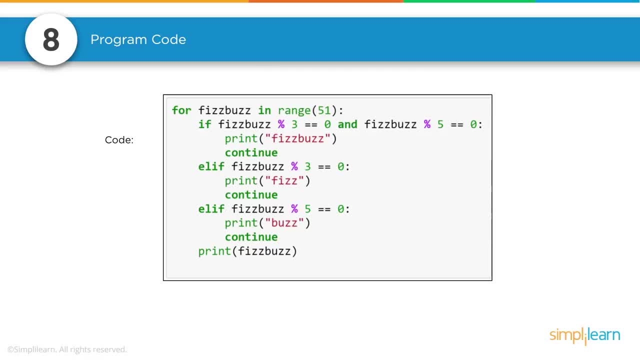 And it's important to remember. the range here says range to 51. That's 0 to 51, which is correct. We want to go to 51 because it stops. It gets to 50 and it stops, So that's 0 to 50.. 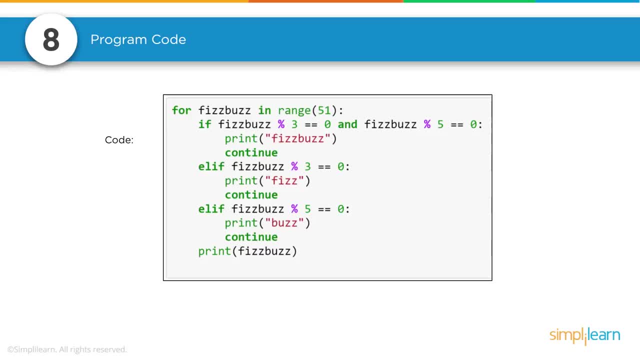 But if you remember, the question asks from 1 to 50. So the range should be 1 comma 51,, not just 51,, which does 0 to 51. In this particular script in Python you could leave out continue. 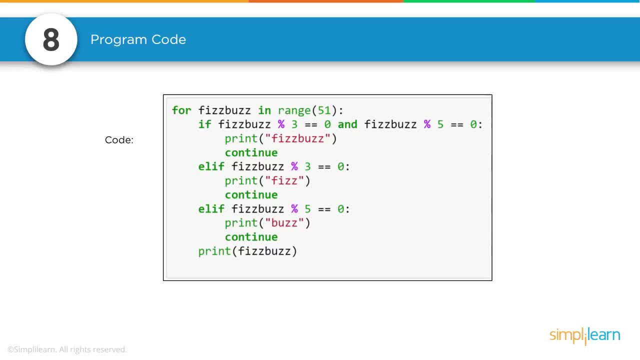 But the continue in this script skips the next elsef So it doesn't keep processing it going down. And in programming mode a lot of scripts you don't need the continue answer, So it would depend on what script you chose And there's probably some other ways to do this. 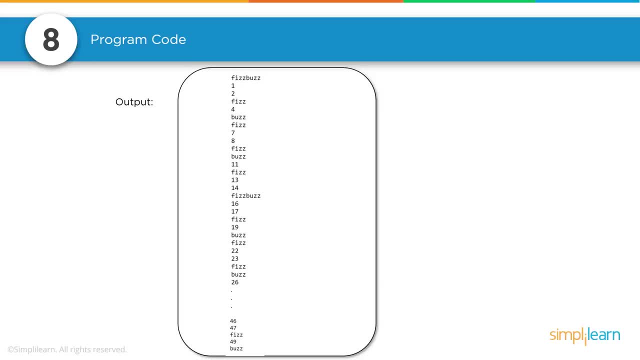 It's a lot of fun And you can see here from the output, we end up with fizz-buzz for 0, which shouldn't be there- 1,, 2, fizz, 4, buzz, fizz, 7,, 8, fizz, buzz, 11, fizz, and so on. 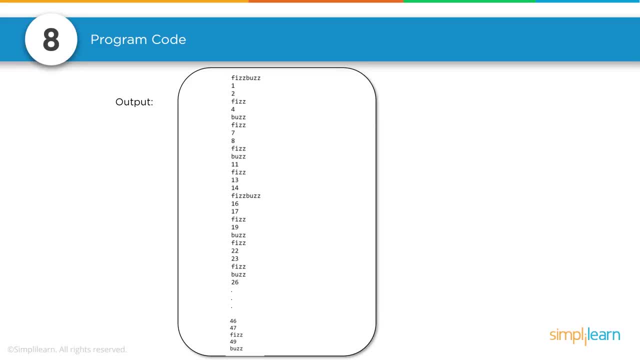 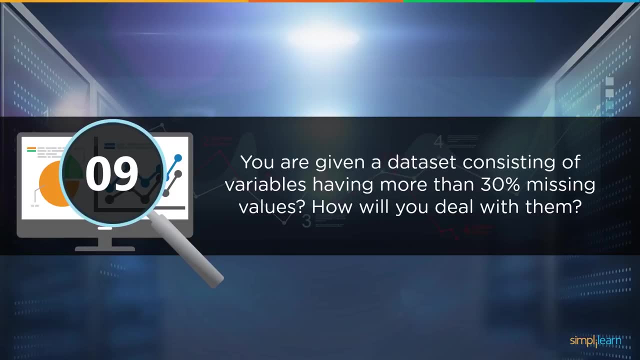 Sounds like a drinking game from my college days, so long ago, many decades ago. You are given a data set consisting of variables having more than 30% missing values. How will you deal with them? Oh, the joy of messy data coming in. 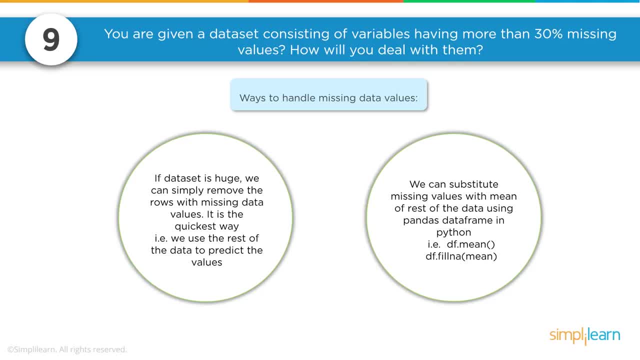 Ways to handle missing data values. Data set is huge. We can just simply remove the rows with missing data values. It is the quickest way, ie we use the rest of the data to predict the values. You just go in there and say: any row of our data that has a NA in it, get rid of it. 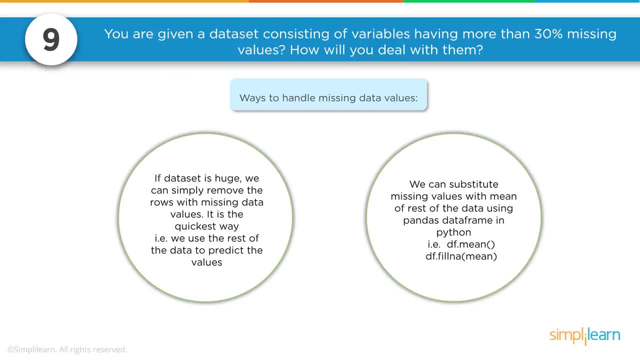 That doesn't work with smaller data. So with smaller data you start running into problems because you lose a lot of data, And so we can substitute missing values with the mean or average of the rest of the data using Panda's data frame in Python. 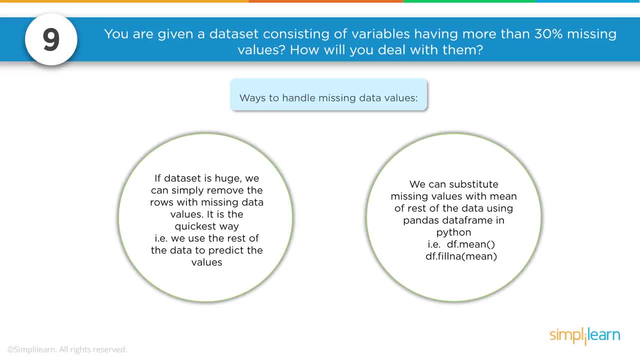 There's different ways to do this, obviously in different languages, And even in Python there's different ways to do this. But in Python it's real easy. You can do the dfmean so you get the mean value. So if you set mean equal to that, then you can do a dffillna with the mean value. 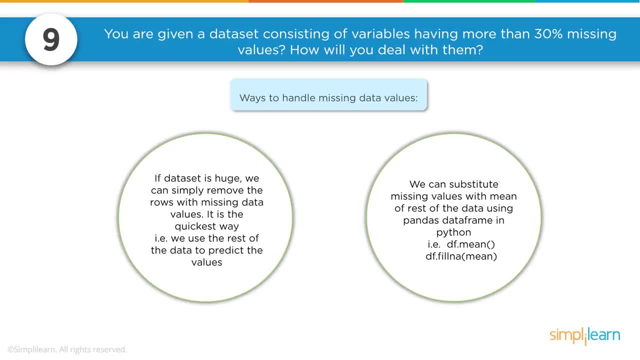 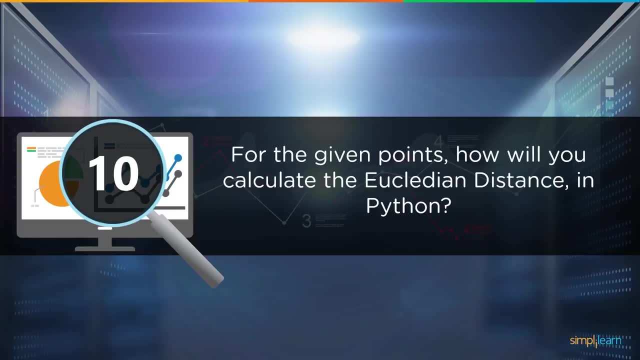 Very easy to do in a Python Panda script And if you're using Python you should really know Pandas and NumPy number Python and Pandas data frames For the given points. how will you calculate the Euclidean distance in Python? 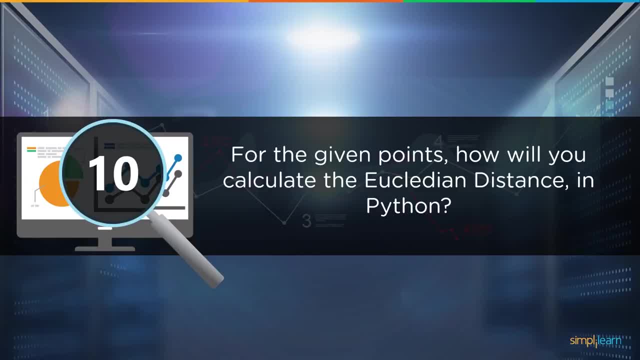 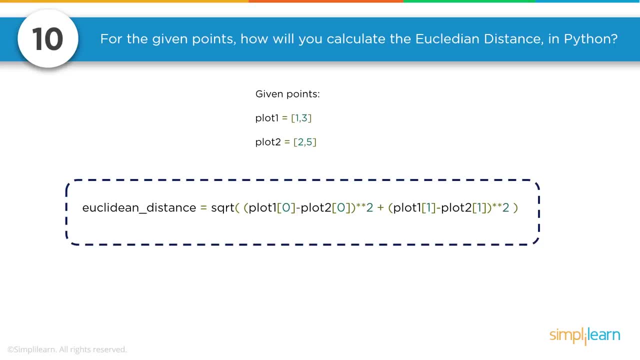 So back to our basic algebra from high school. Euclidean distance is the line on the triangle, And so if we're given the points, plot one equals one comma three, plot two equals two comma five- we know that from this we can take the difference of each one of those points. 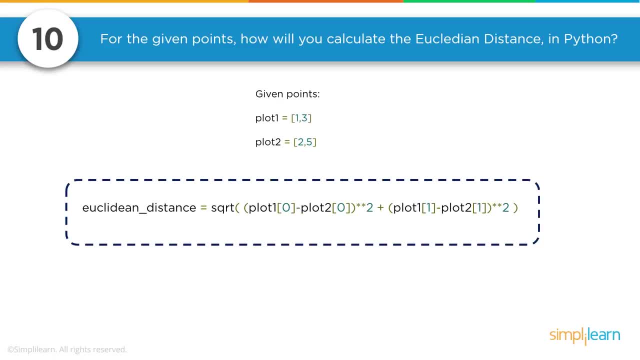 square them and then take the square root of everything. So the Euclidean distance equals the square root of plot one. zero minus plot two is zero squared plus plot one of one minus plot two of one, squared mouthful there. And you can remember if you have multiple dimensions that go past two dimensions. 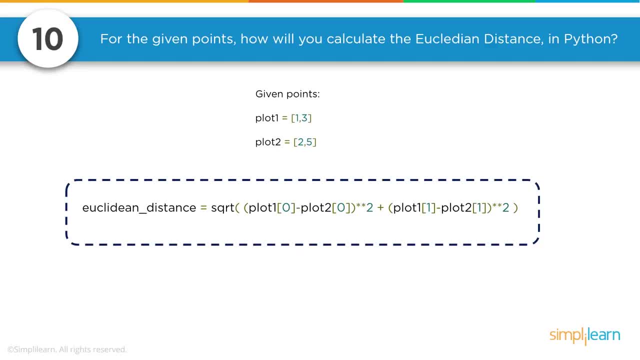 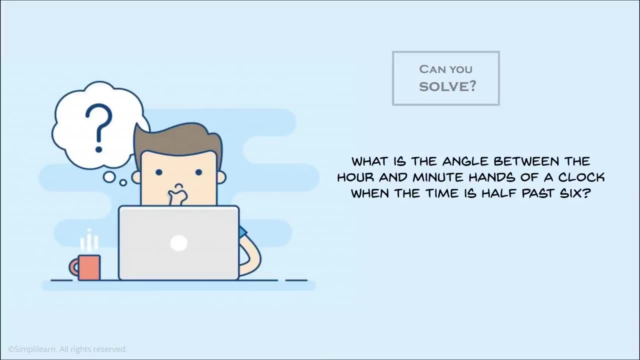 you could have. plot three can simply be the distance from plot one. You only need to do one side of that, or plot two. You can do either way and square that and take the square root of that. Another mind bender: how to calculate something. 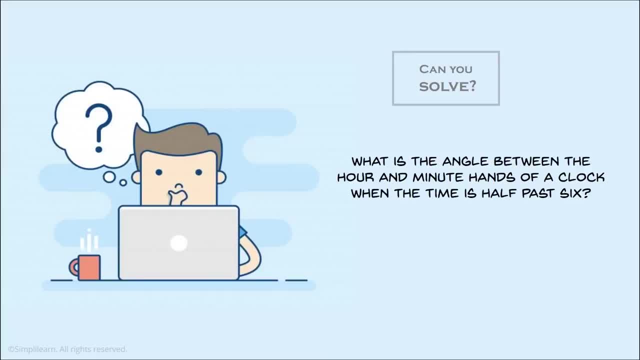 how to figure out the solution to something. What is the angle between the hour and minute hands of a clock when the time is half past six? So you want to kind of imagine that clock: the large hand is pointed down to the thirty and the other hand is going to be right between the six and the seven. 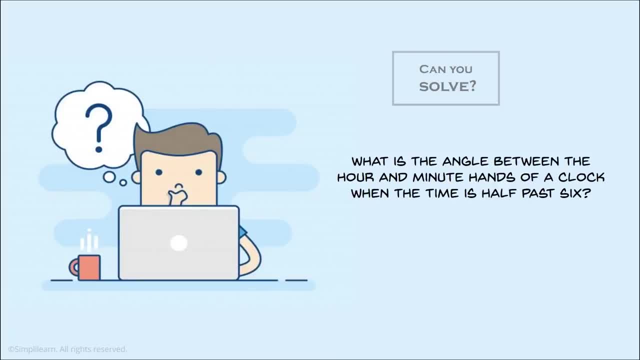 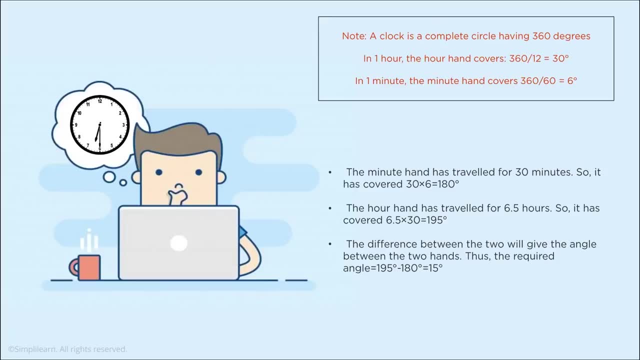 because it's half past six. There's actually a couple of ways to solve this, but let's take a look and see how they did it. Note: a clock is a complete circle having 360 degrees In one hour. the hour hand covers 360 over 12.. 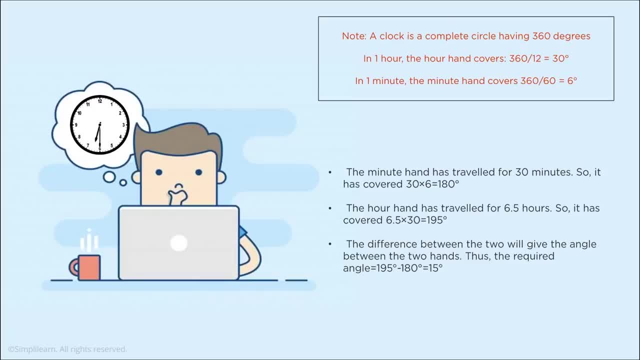 So it equals 30 degrees for each hour In one minute. the minute hand covers 360 degrees over 60 minutes, or six degrees per minute. The minute hand has traveled for 30 minutes, so it has covered 30 times six, which equals 180 degrees. 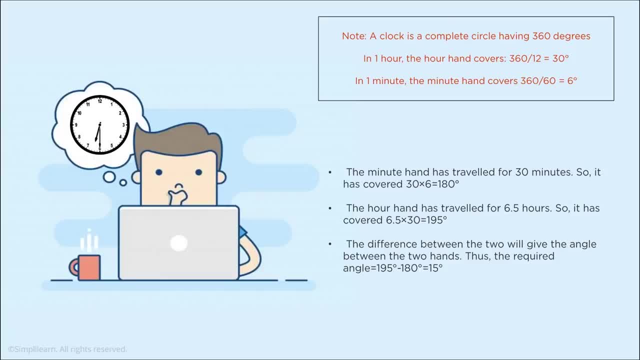 So we know that's 180 degrees from the 12. The hour hand has traveled for 6.5 hours, six and a half 6.5, so it's covered 6.5 times 30, which equals 195 degrees. 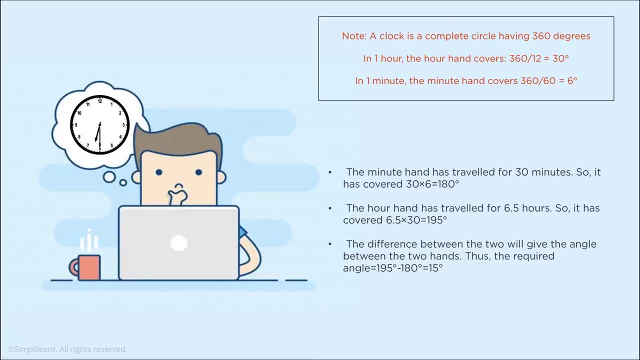 The difference between the two will give the angle between the two hands. Thus the required angle equals 195. minus 180 equals 15 degrees. And this is nice the way they solved it, because you can now punch in any kind of time within reason. 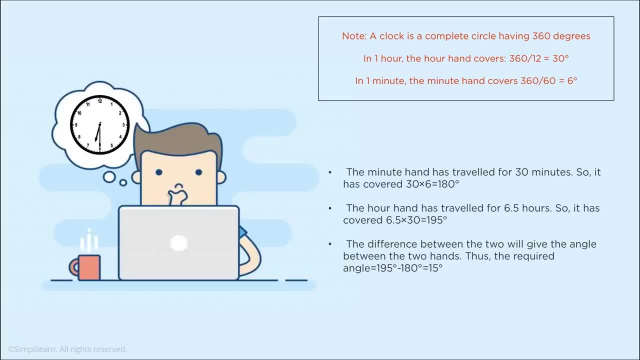 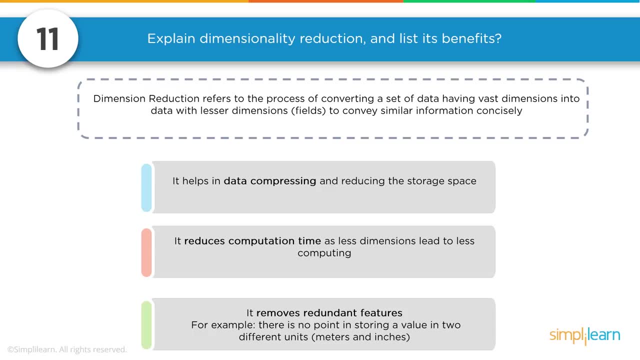 The other part is on the hours is you have to be able to convert the hours into decimals? Explain dimensionality reduction and list its benefits. Dimension reduction refers to the process of converting a set of data having vast dimensions into data with lesser dimensions. 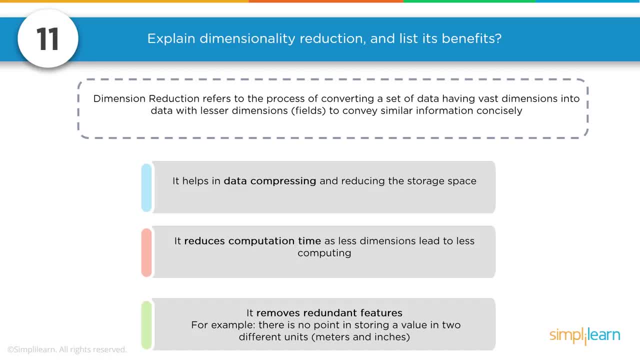 fills to convey similar information concisely. It helps in data compressing and reducing the storage space. It reduces computation time, as less dimensions lead to less computing. It removes redundant features. For example, there is no point in storing a value in two different units: meters and inches. 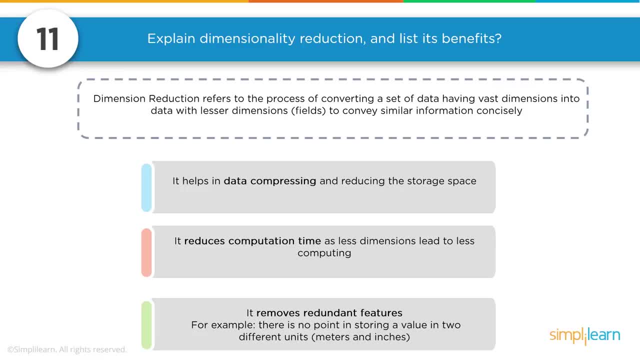 And I certainly run into a lot with this, with text analysis. I've been known to run a text analysis over a series of documents ends up with over 1.4 million different features. That's a lot of different words being used And if you do what they call by connect them, 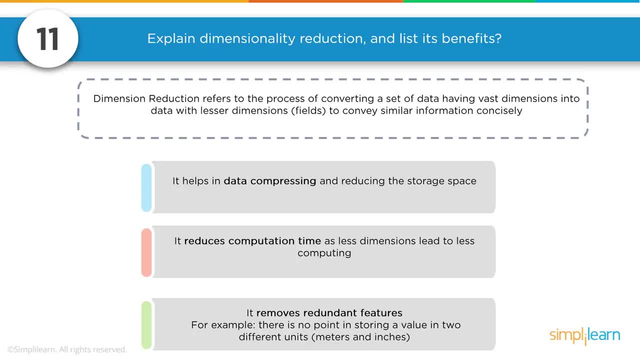 you connect two words together. now you're up to 4.8 million different features and you start having to figure ways to bring that down. What can we get rid of That kind of thing? So you can see where that can get really high in on processing. 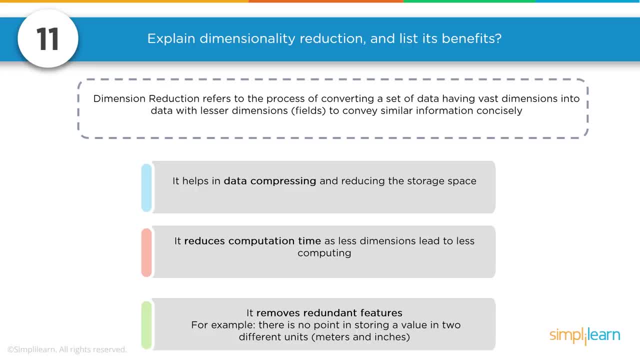 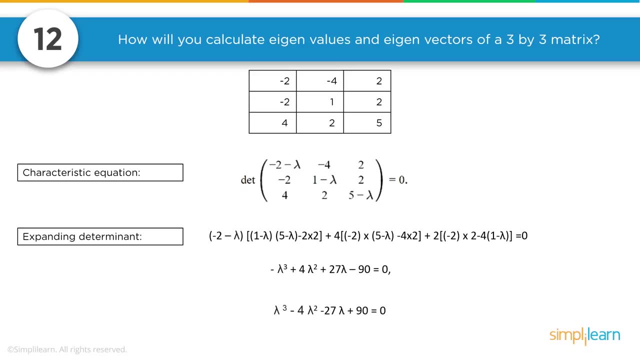 and learning how to reduce the list dimensions is very important. How will you calculate eigenvalues and eigenvectors of a 3x3 matrix, And what they're really looking for here is when you write it out, for the eigen is that you know that you're going to use the lambda. 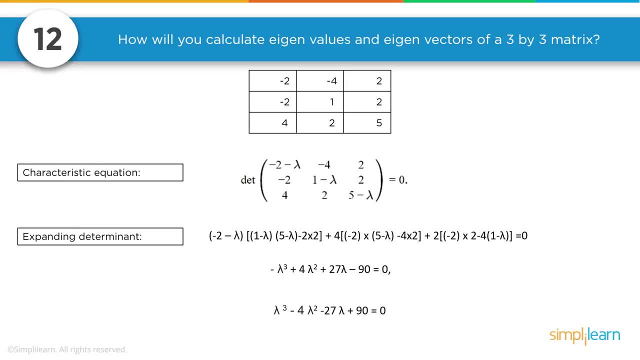 That's the most common one. Obviously, you can use any symbol you want, but lambda is usually what they use And that you do it down the middle diagonal. And so when you take that matrix and you take the characteristic equation, you end up with the determinant and that's the minus 2 minus lambda. 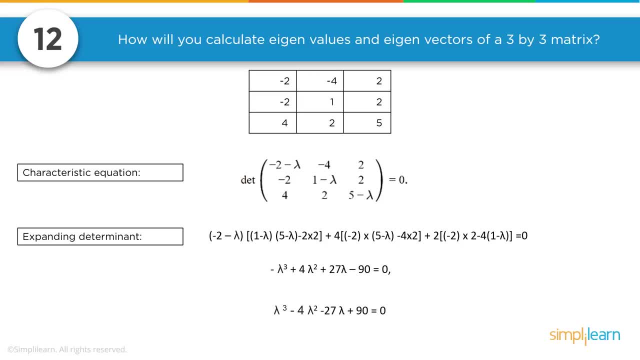 minus 4, 2, minus 2, 1 minus lambda, 2, 4, 2, 5 minus lambda, And that's what they're looking for and you know that's equal to 0.. So when you're doing a matrix in the eigen setup with the eigenvectors, 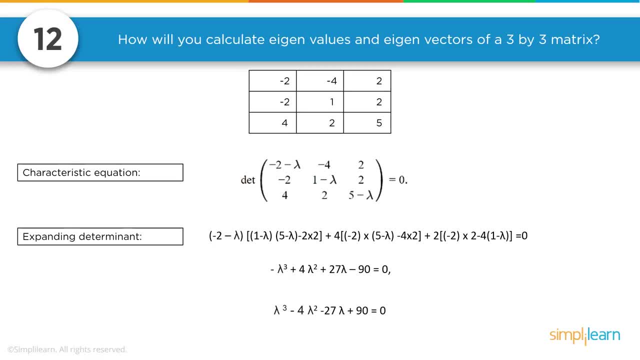 that's all going to come out equal to 0.. And then you can go ahead and write the whole equation out So we can expand the determinant. As you can see right here, the minus 2 minus lambda times, it's a mouthful. 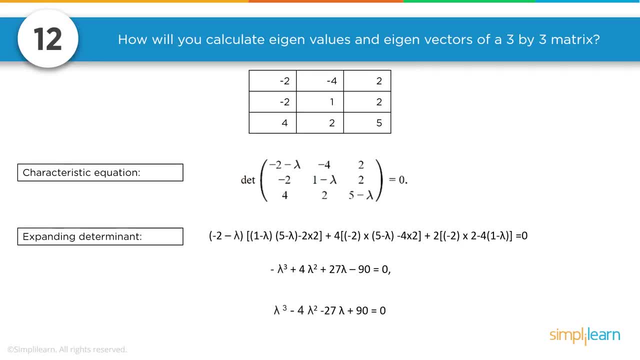 I'll leave it up here for a second so you can look at it when you break it down. And if you look into the algebraic functions, you end up with minus lambda cubed plus 4 lambda squared plus 27 lambda minus 90 equals 0.. 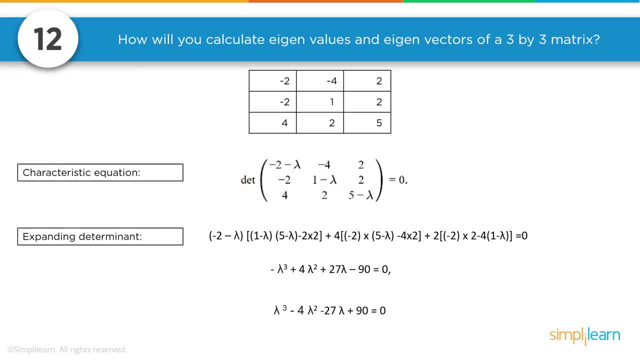 So now we have a nice algebraic equation built from the eigenvectors And always remember you can hit the pause button and you can also send a note. Send a note to SimplyLearn. if you have more questions on vectors or on this, Definitely have that resource available to you. 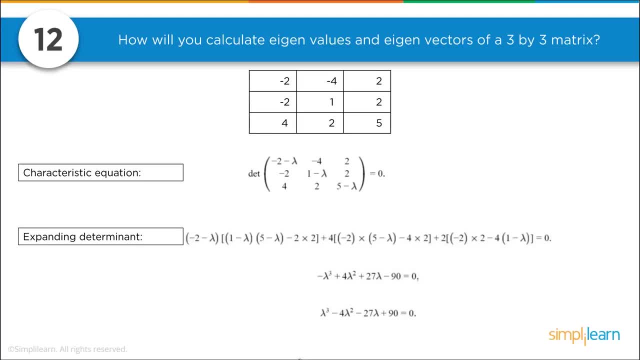 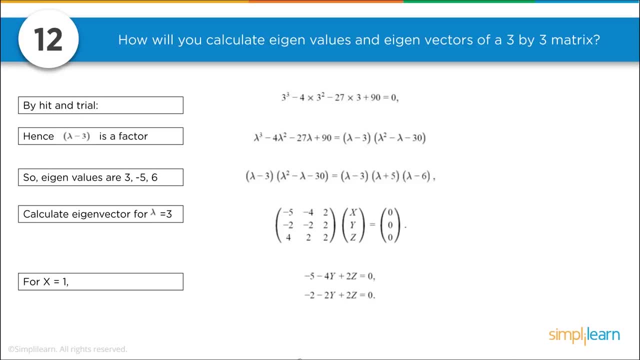 or post down in below on the YouTube video comments. And so when we calculate the eigenvalues and eigenvectors of a 3x3 matrix, as we continue on down the math of this- and to be honest, I really don't like working with matrices like this- 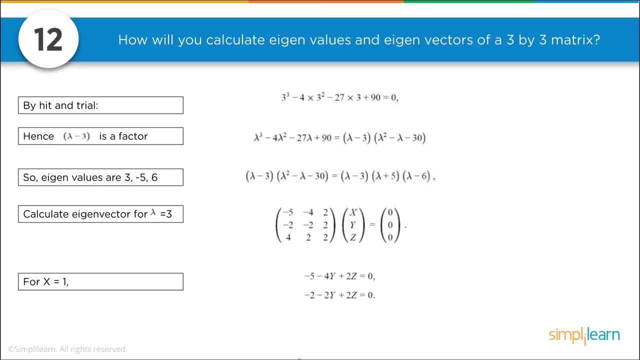 It's important to understand the math behind it and it's important to know the code just enough so that you're not lost when someone's explaining it or it comes up when I'm working on different data science models. Of course, if you're dealing with the high-end math side of it, 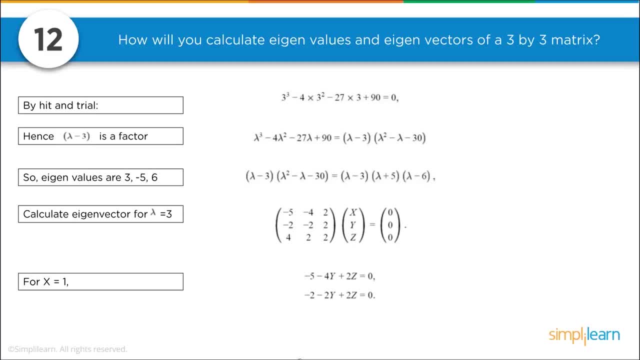 then you better know this First is by hit and trial. So you try in different variables to solve for 0. And you can come in here and you'll find that if we put in the 3 in there we end up with a 0 at the end and substitute the 3.. 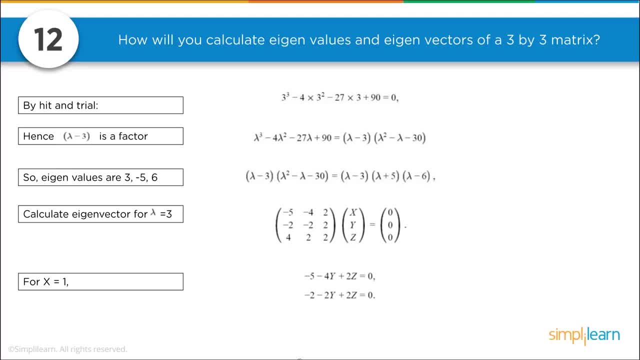 Hence we end up with lambda minus 3 as one of the factors, And you can do the math going out on that where we have lambda cubed minus 4, lambda squared minus 27. lambda plus 90 equals lambda minus 3 times lambda squared minus lambda minus 30.. 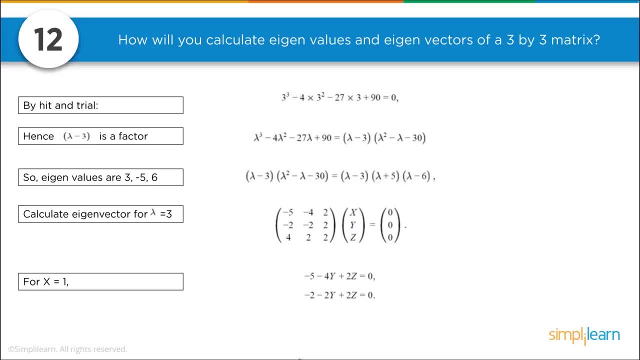 So eigenvalues, based on that one, are 3 minus 5 and 6.. And then from there we can calculate the eigenvector for lambda equals 3.. And you can see here where the matrix, as we write it out, is the minus 5 minus 4, 2, minus 2, minus 2, minus 2, 4, 2, 2.. 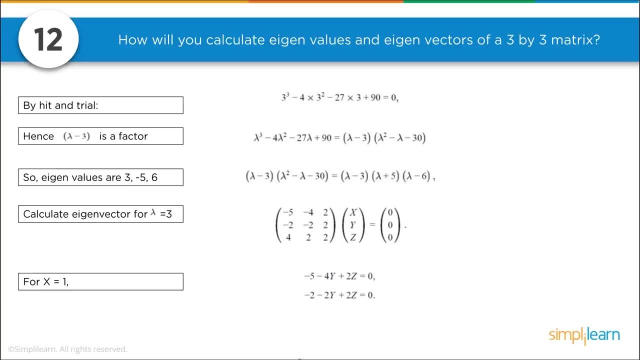 That was from the beginning. Put in the x, y and z equals 0, 0, 0. And so when we put in those numbers and we calculate them out, we have for x equals 1,. we have the minus 5, minus 4y, plus 2z equals 0,. 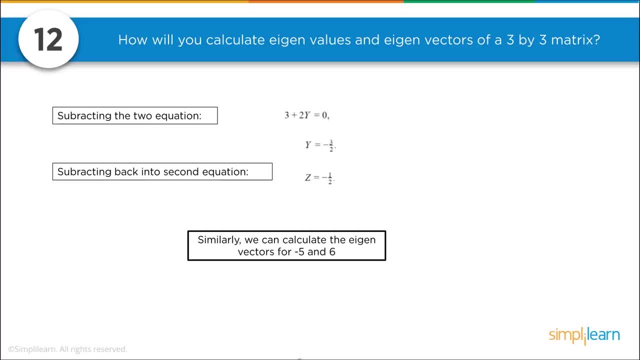 minus 2, minus 2y plus 2z equals 0.. And subtracting the two equations we just had, we get 3 plus 2y equals 0, y equals minus 3 over 2, and z equals 0. 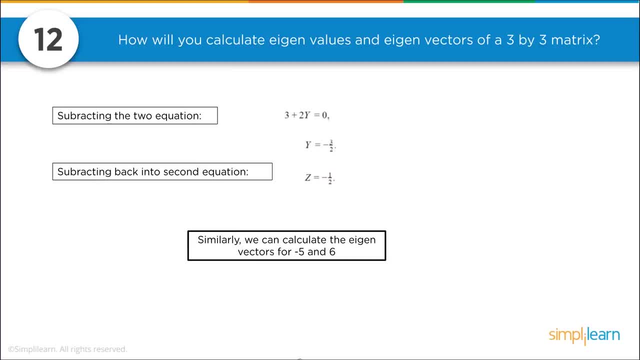 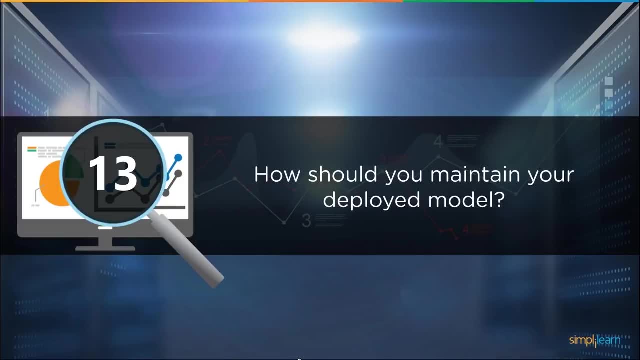 So that's minus 1 over 2.. That's going back to the first equation, And similarly we can calculate the eigenvectors for minus 5 and 6.. How should you maintain your deployed model? Ooh, distribution time, my favorite. 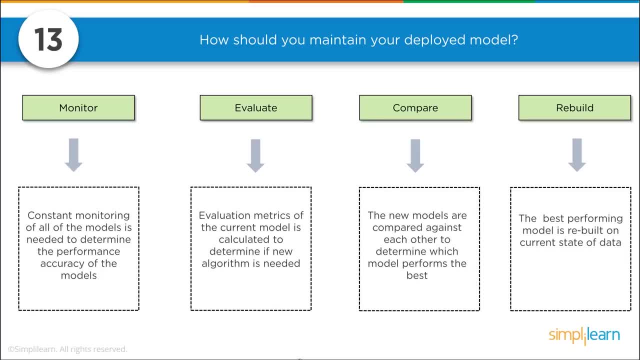 I spent 10 years in software distribution. So first thing- and this is true not just of your data science model, but of any computer code going out there- This basic setup can work, although usually there's a little added steps in there. 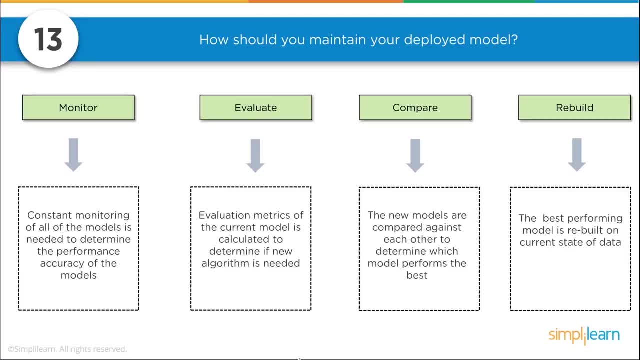 First we're going to monitor it So we have a constant monitoring of all the model is needed to determine the performance accuracy of the models. So, yeah, we want to just keep an eye on it. We want to make sure they're accurate. 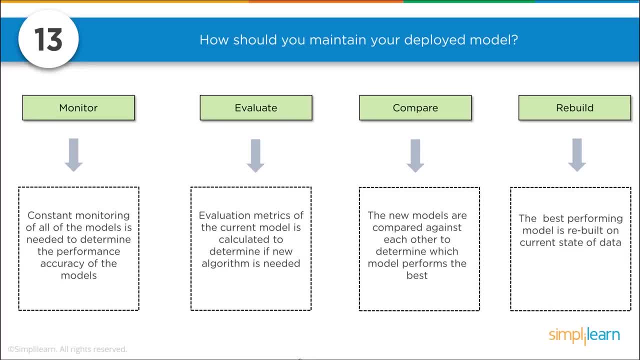 We want to make sure that, whatever they're supposed to predict- or I threw in that bonus word- post script, where you change something and you want to figure out how your changes are going to affect things- We need to monitor it and make sure it's doing what it's supposed to do. 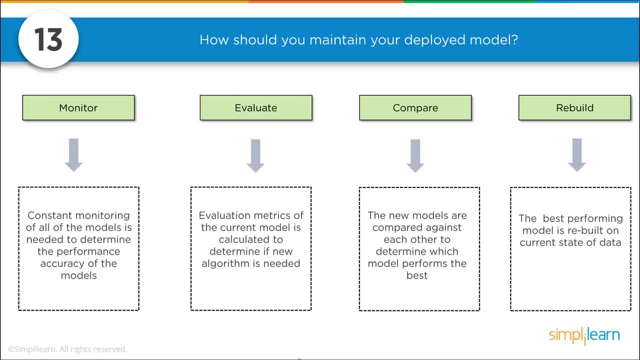 Evaluation metrics of the current model is calculated to determine if new algorithm is needed, And then we compare it. The new models are compared against each other to determine which model performs the best, And then we do a rebuild. The best performing model is rebuilt on the current state of data. 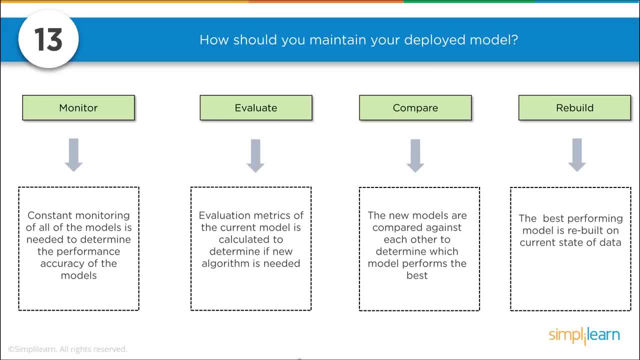 This is interesting. I found this out just recently. If you're in weather prediction, the really big weather areas have about seven or eight different models, depending on what's going on, And so you actually have almost a little forest going on there where they're like. 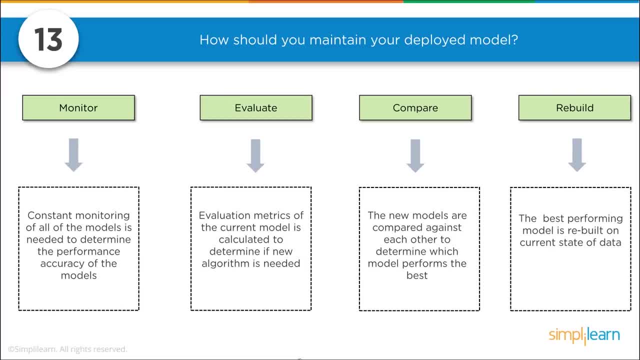 which model is going to fit best, And this is what we're going to use to predict the weather with. So not only do you don't necessarily get rid of the models, but you figure out which models fit, data of what's going on or the current state of data. 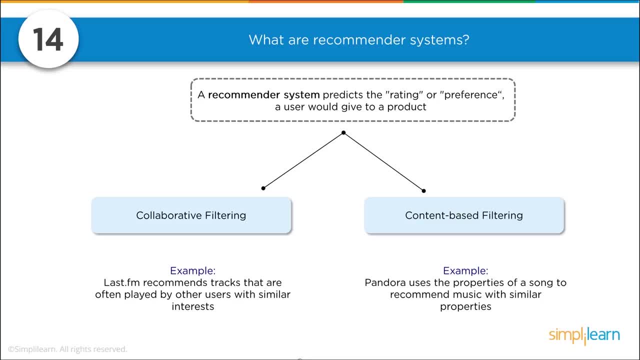 What are recommender systems? Most commonly they're used nowadays in marketing, So very big industry understanding. recommender systems predicts the rating or preference a user would give to a product, And they're split into two different areas. One is collaborative filtering. 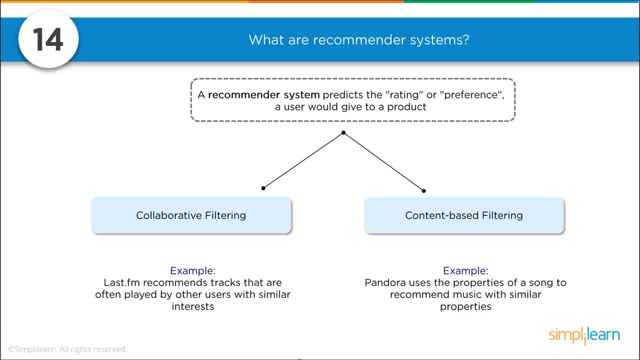 And a good example of that is the lastfm recommends tracks that are often played by other users with similar interests. So people who, if you're on Amazon, people who bought this, also bought that. It's got me a few times. And then there's content based filtering. 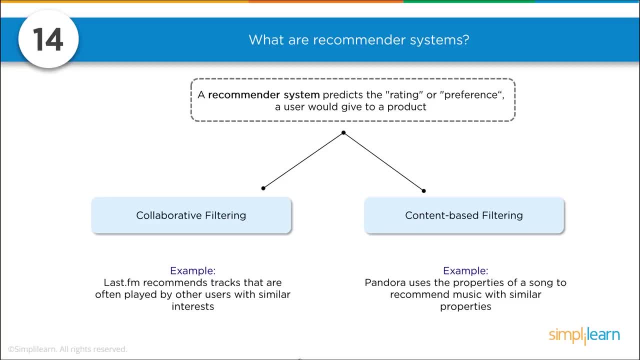 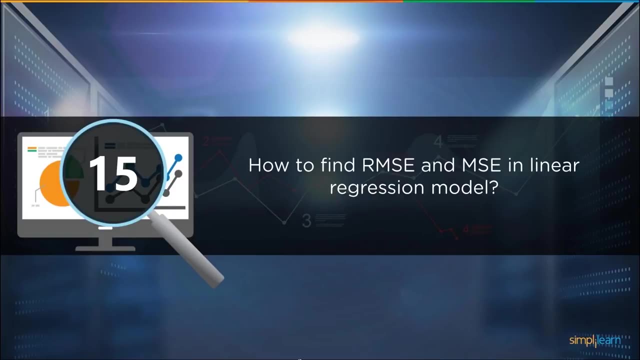 And we're looking at content. We're looking at who else is listening to the music. These example Pandora, which uses the properties of a song to recommend music with similar properties. So you have collaborative filtering and content based filtering. How to find RMSE and MSE in linear regression model. 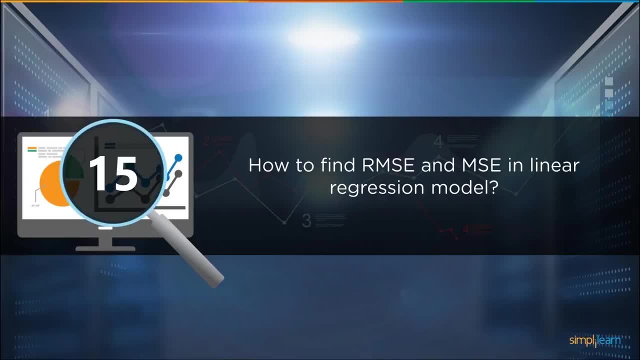 Hopefully you remember what the two acronyms mean, because that is like half the answer. We have the root mean square error and the mean square error in linear regression model. So we're looking for error in the RMSE and the MSE. These are the two of the most common measures of accuracy for a linear regression model. 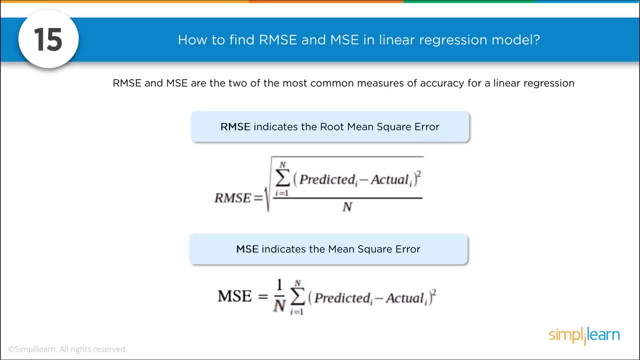 And you can see, here we have the root mean square error. RMSE equals- And this is the square root- of the sum of the predicted minus the actual squared over the total number. So we're just looking for the average mean, So we're looking for the average over the end. 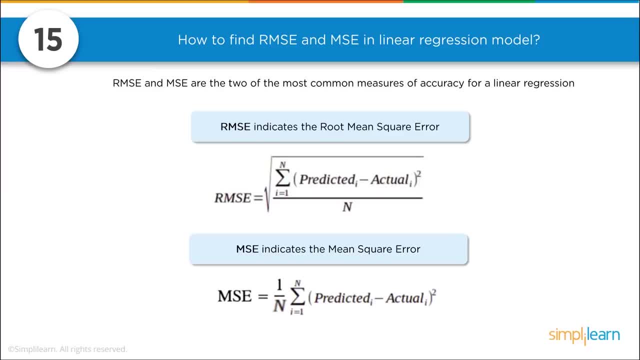 And the reason you need to know about the difference between RMSE versus MSE is when you're doing a lot of these models and you're building your own model, why do you need to take the square root of it? It doesn't change the value as far as the way you're using it. 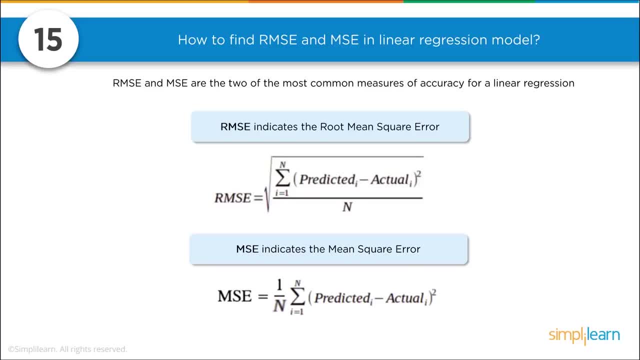 because you're looking to see whether the error is greater or less than So why add that extra computation in? So a lot of models use the MSE, which indicates the mean square error or the average error, And it's the same formula minus the square root at the end or across the whole thing. 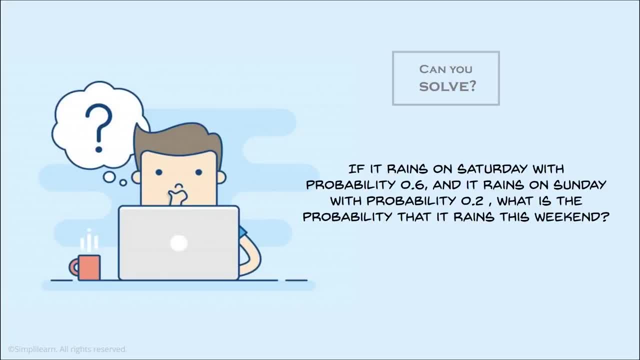 Another riddle to solve. If it rains on Saturday with a probability of 0.6 and it rains on Sunday with a probability 0.2,, what is the probability that it rains this weekend? And the trick in probabilities on this case is we need to know what is the probability of it not raining. 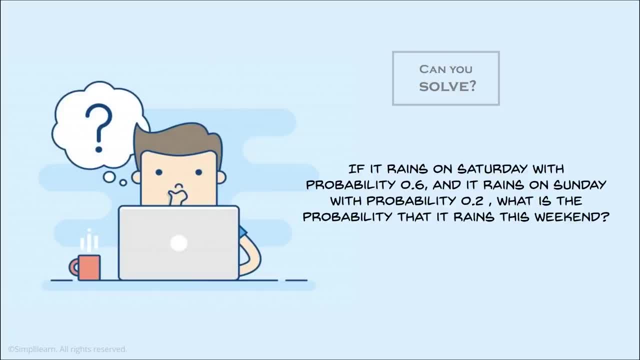 What's the chance of it not raining on Saturday? And if it doesn't rain on Saturday, we want to take that and combine that with the chance of it not raining on Sunday. The total probability which, in this case, we're just going to use 1,. 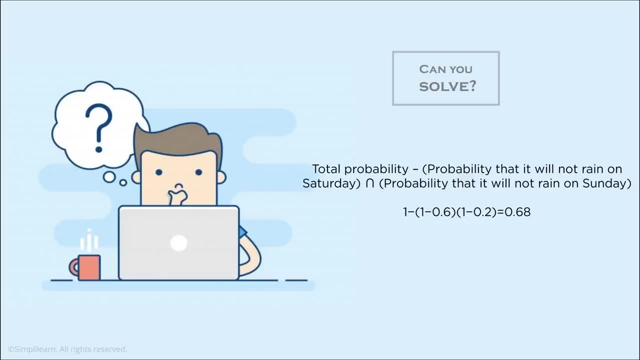 minus the probability that it will not rain on Saturday. so that's 1 minus 0.6.. We're going to take that as a union, which we simply just multiply them together- of the probability that it will not rain on Sunday. 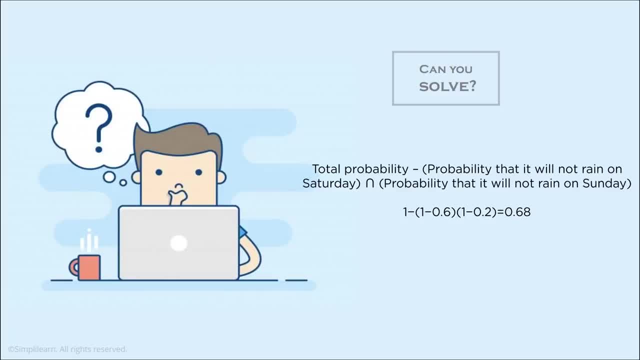 It's important to recognize the union here, or the, and you can see by the formula down here. we end up with 0.68 or 68% chance that it will rain on the weekend, And there are a couple other ways to solve this. 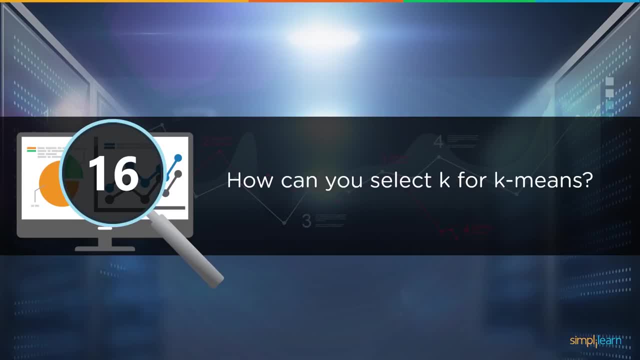 but this is probably the most traditional way of doing that. How can you select K for K-means? So first you better understand that what K-means is and that K is the number of different groupings. And most commonly we use is the ELBO method to select K for K-means. 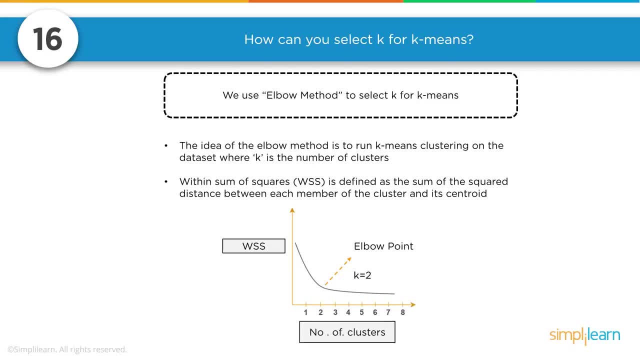 The idea of the ELBO method is to run K-means clustering on the data set, where K is the number of clusters Within the sum of squares. WSS is defined as the sum of the squared distance between each member of the cluster and its centroid. 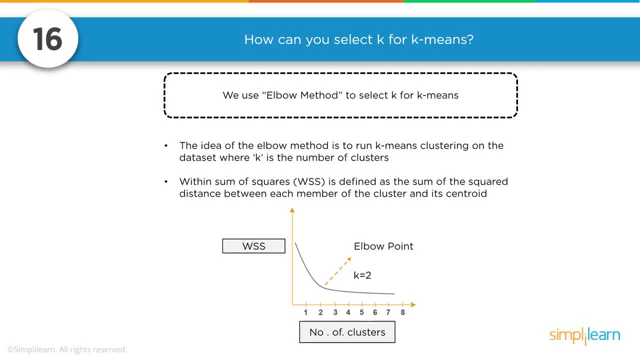 And you should know all the terms for your K-means on there And with the ELBO point. and again, here's our iteration. in our code- we talked about that earlier- You iterate starting with. usually you don't start right at 1,, but you might start with 2,, 3, or 4.. 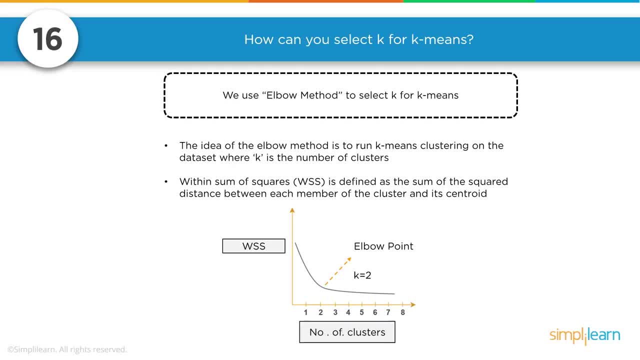 And you just see where it comes out and you can see the nice ELBO there, which is easy to see graphically, Where the number of K clusters and the WSS value drops, And then it just kind of flattens out and there's no reason to take the K-means any further. 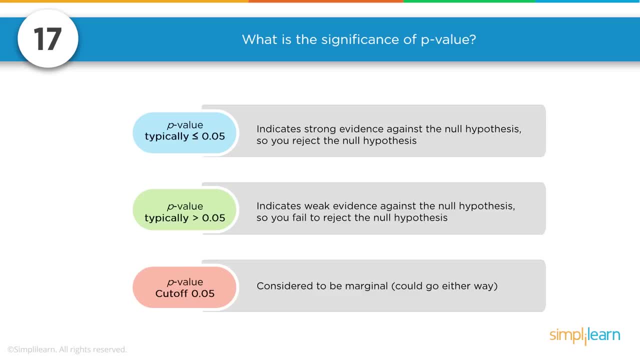 What is the significance of P-value? Oh, good one, Especially if you're dealing with R, because that's the first thing that pops up. P-value, typically less than or equal to 0.05, indicates a strong evidence against the null hypothesis. 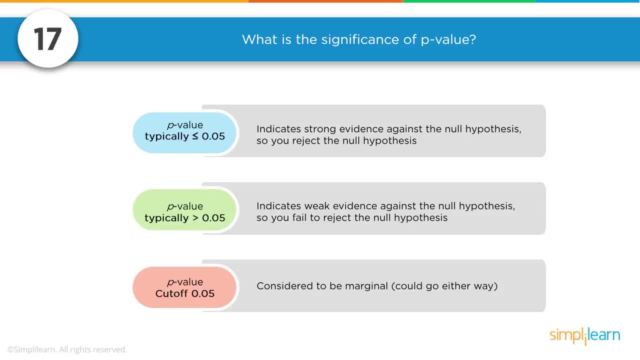 And you should know why we use null hypothesis instead of the hypothesis. So you reject the null hypothesis. It's very important that term null hypothesis in any scientific setup and also in data science. It doesn't mean that it's true. It means that there's a high correlation. that it's true. 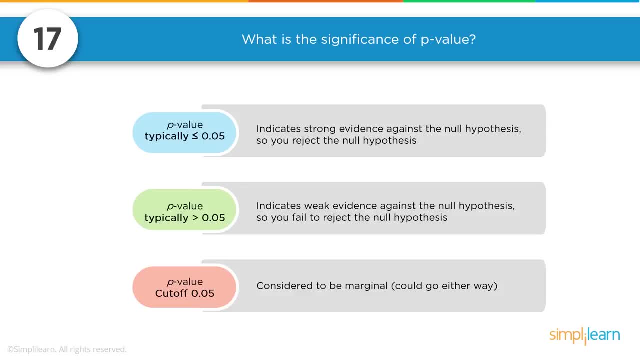 So if your null hypothesis means it's not true, your hypothesis has a high correlation, that it's probably true. And if the P-value is typically greater than 0.05, it indicates a weak evidence against the null hypothesis. So you fail to reject the whole null hypothesis. 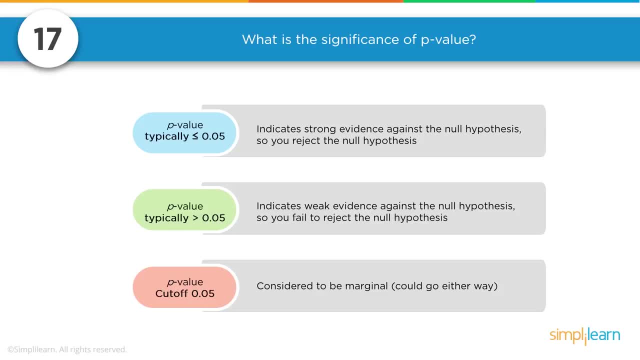 And if you reject that, then your actual hypothesis is probably not true. The correlation of your data with what you think it's saying is probably incorrect, And if you're right at the cutoff of 0.05, it's considered to be marginal. 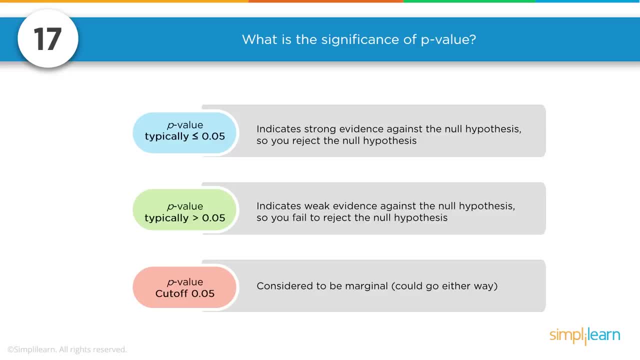 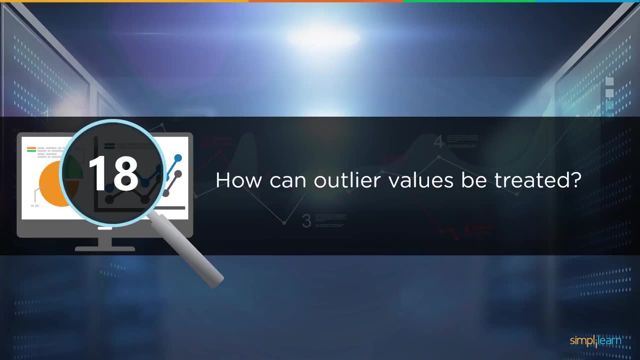 Could go either way, And again you can use that P-value on different features to decide whether you're going to include your features as far as something worth exploring in your data science model. How can outlier values be treated? Oh, good one. 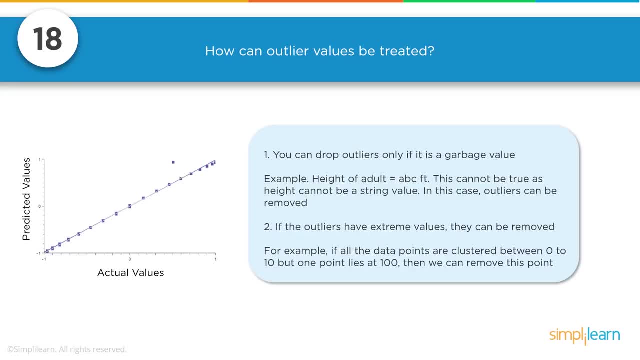 You can drop outliers only if it is a garbage value. So sometimes you end up with like one outlier that just is probably someone's measurements way off. Height of an adult equals ABC feet. This cannot be true, as height cannot be a string value. 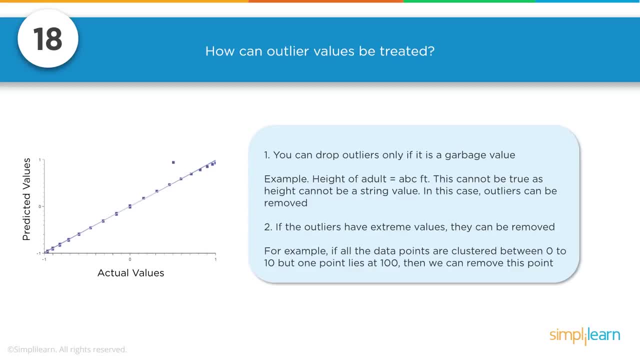 In this case, outliers can be removed. If the outliers have extreme values, they can be removed. For example, if all the data points are clustered between 0 to 10, but one point lies at 100,, then we can remove this point. 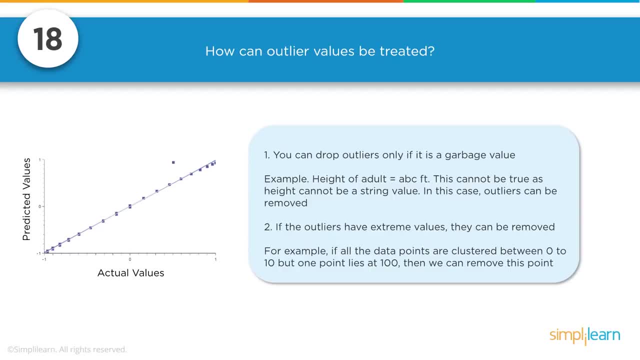 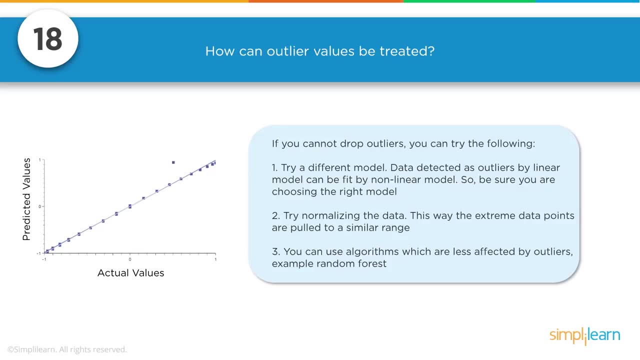 And again, sometimes you just look for the outliers so you can see what's going on, if there's something unusual there, So maybe the equipment's not calibrated correctly. If you cannot drop outliers, you can try the following: Try a different model. 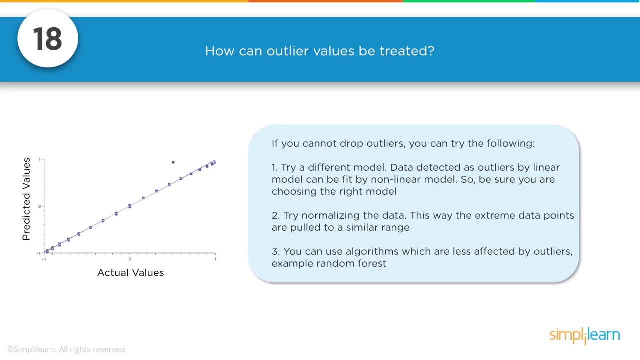 Data detected as outliers by linear model can be fit by nonlinear model, So be sure you are choosing the right model. So if it has like more of a curved look to it instead of a straight line, you might need to use something other than just a straight line linear model. 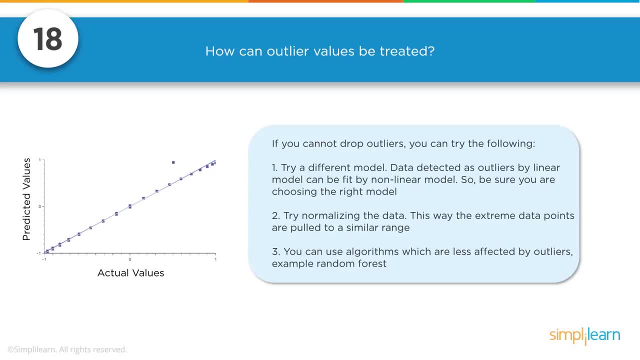 Try normalizing the data. This way, the extreme data points are pulled to a similar range. If you can use algorithms which are less affected by outliers- example: random forest- So there is another solution is you can come up with the random forest. 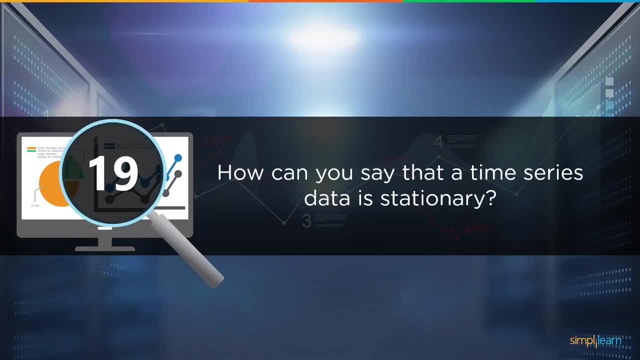 which a lot of times it completely bypasses your outliers. How can you say that a time series data is stationary? Oh, that's an interesting term. Stationary meaning it's not moving, but it's a time series. We can say that a time series is stationary when the variance and mean 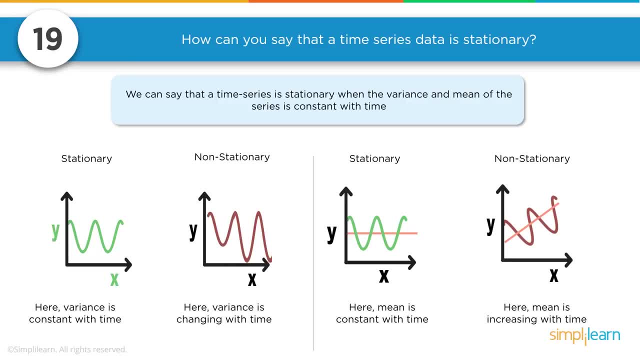 of the series is constant with time, And this graphic example is very easy to see. We have our: the variance is constant with time. So we have our first variable, y and x, and x being the time factor and y being the variable. 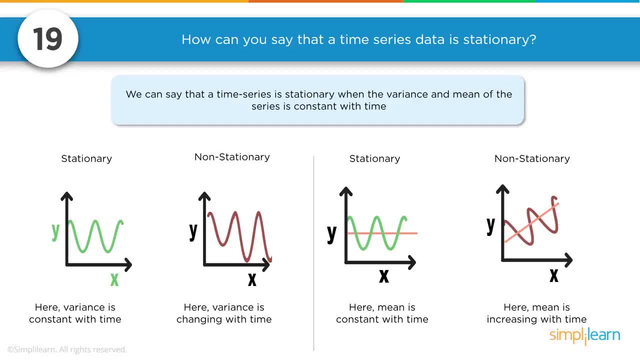 As you can see, goes through the same values all the time. It's not changing in the long period of time, So that's stationary. And then you can see in the second example, the waves get bigger and bigger, So that's non-stationary. 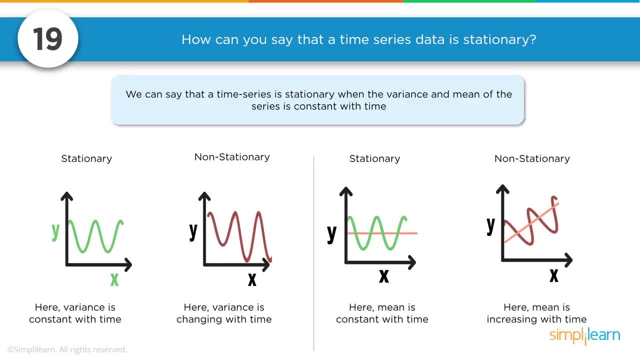 Here the variance is changing with time. Again we have y, which stays constant, So that if you look at the bigger picture, it's the same wave over and over again. And then of course we have, where the wave is growing in size, going up. 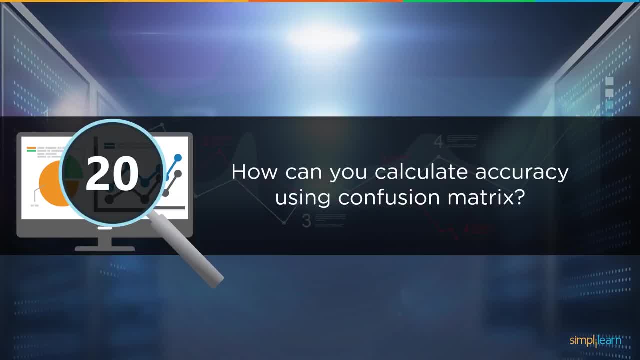 It can also go down, So it also be non-stationary. How can you calculate accuracy using confusion matrix? Oh, great one, Confusion. Confusion matrixes are so useful when you're taking that first look at data and also when you're showing the shareholders and you want to ask them for money. 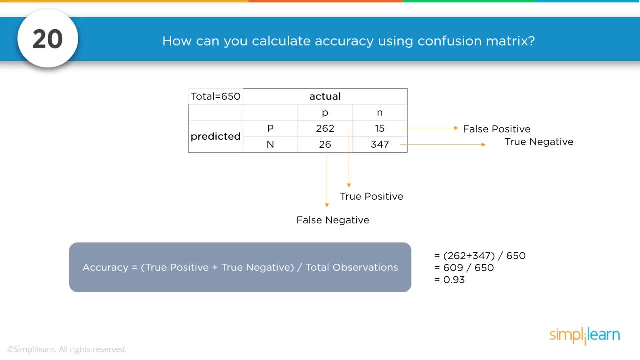 How can you calculate accuracy using confusion matrix? So you have your total data- that we're looking at is 650, and you have your predicted values and your actual values, and you have your predicted p and your actual p. And so when we look at this, 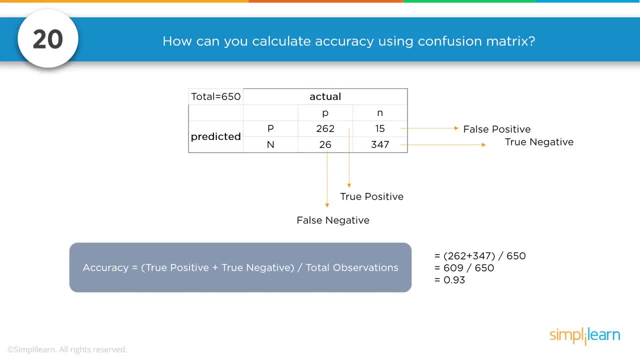 you'll note that if the predicted p and the actual p are 262, but our predicted p also had 15, that weren't correct. So you can see there's a false positive there of 15.. And the same thing with the n. 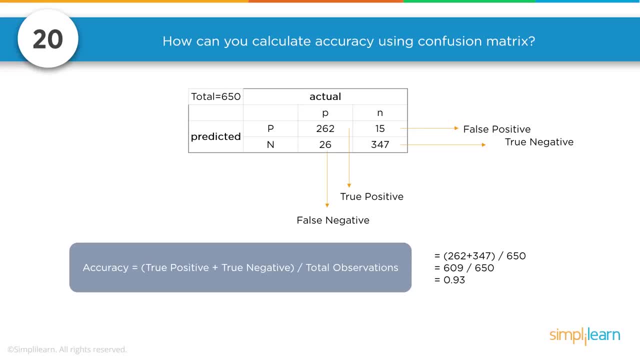 You can see where n predicts n and it has a false negative of 26 out of the total number of n values in there, And so we can do an accuracy on there. The true positive plus the true negative is our total observations, So you have a total of 0.93 accuracy, or 93%. 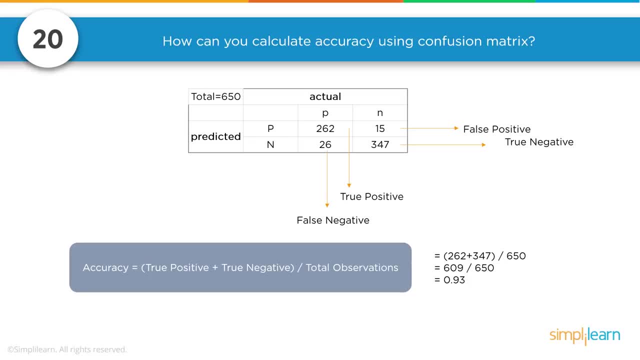 And just a quick note on this. This is so important because it's one thing: if someone is being diagnosed with, say, cancer, you know this is life death. or is my nuclear reactor going to blow up Suddenly? if the p is the probability of it blowing up? 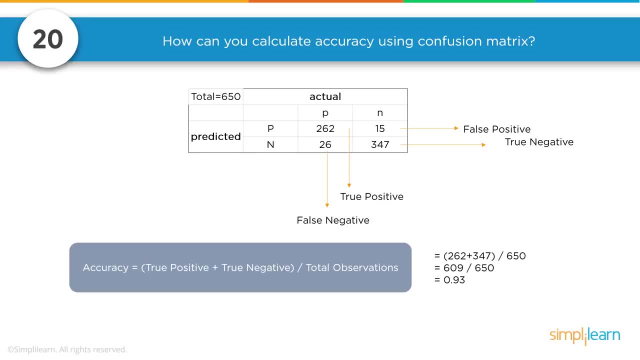 and let's say you have 15, that's a lot less than, say, the 26 chances of it blowing up, you know. So the actual domain of your data is very important. So if you're non-positive, you don't really care about the predicted value, having non-positive as positive. 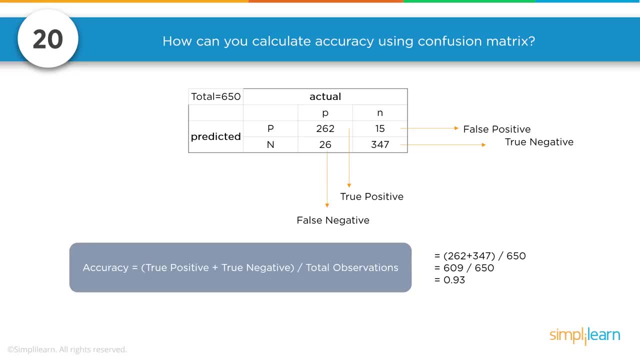 because they're going to go do a biopsy on the cancer or whatever anyway. But you're very interested if you have a positive, an actual positive value which is looked at as negative, a false negative. That's really important in that domain, depending on what domain you're in. 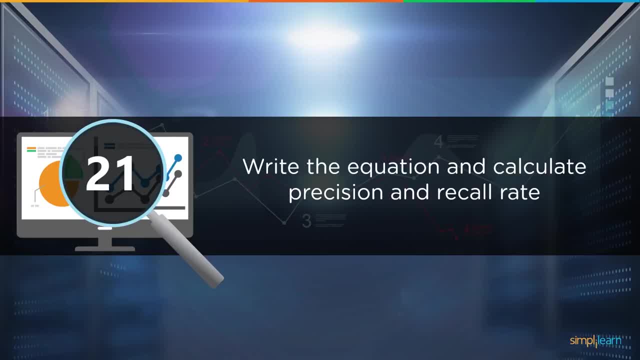 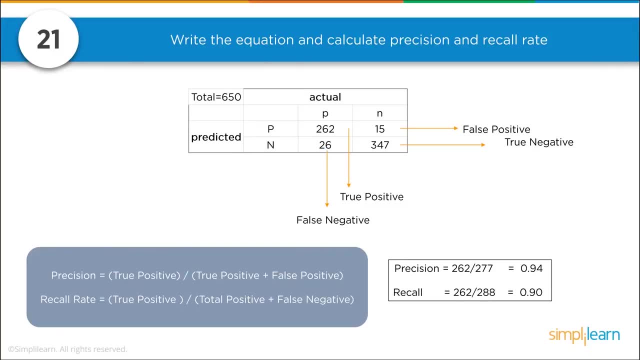 Write the equation and calculate precision and recall rate And so continuing with our confusion. matrix- I was just talking about the different domains. We have. the precision equals 262 over 277.. So your precision is the true positive over the true positive, plus false positive. 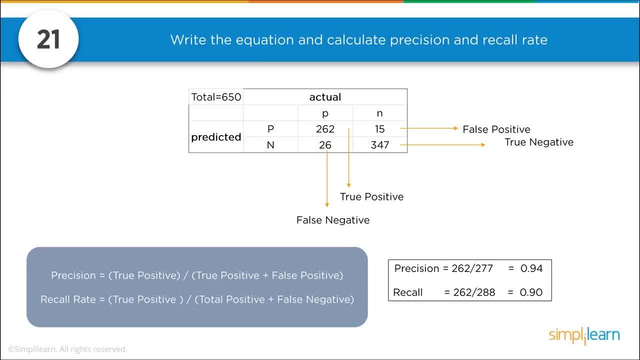 And the recall rate is your true positive over the total positive plus false negative, And you can see here we have the 262 over 277, equals a 94.. And the recall over here is the 262 over 280, which equals 0.9 or 90%. 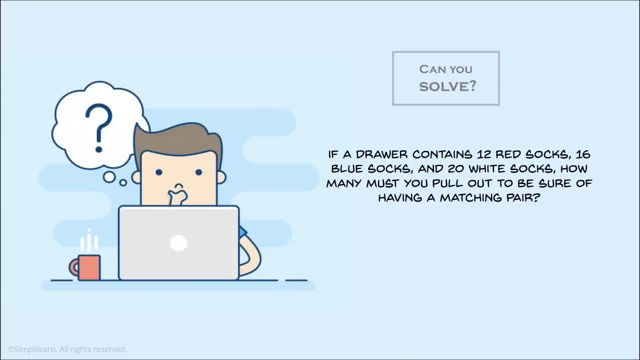 And, oh good, we're going to take a pause for another brain teaser. If a drawer contains 12 red socks, 16 blue socks and 20 white socks, how many must pull out to be sure of having a matching pair? The last time I went through these kind of brain teaser, things was like 20 years ago. 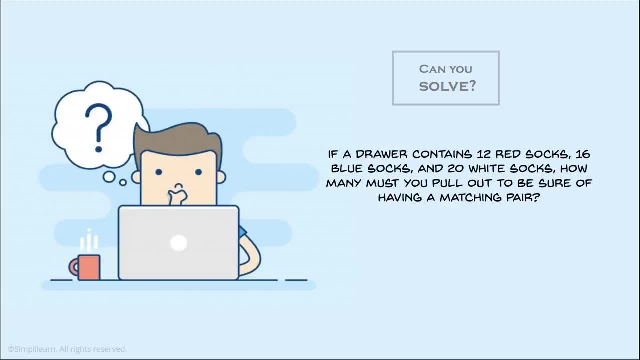 And I had six people sitting across the table waiting for my answer. That's kind of mind-numbing when you're in an interview like that. Hopefully you're not stuck in an interview like that, But on this you need to ask yourself how many different colors of socks are there? 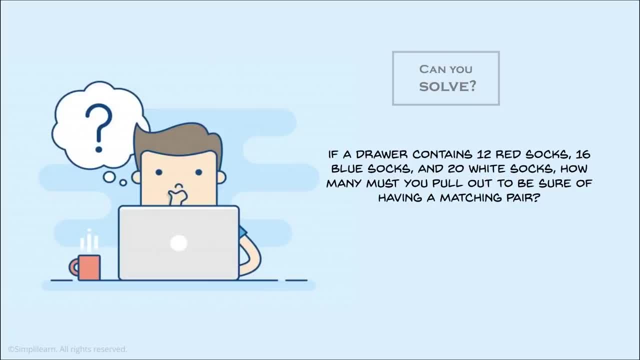 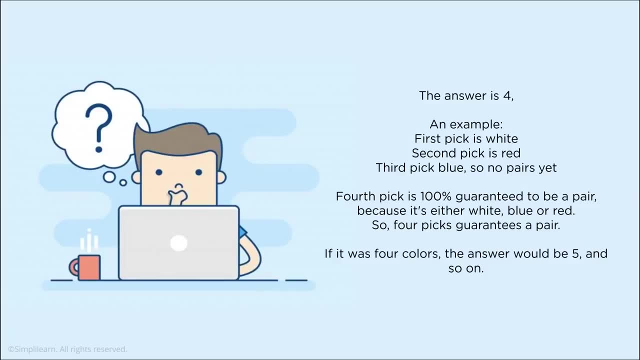 So they've thrown a lot of extra data in here that you don't need to solve the answer. The answer is four. An example: your first pick is white, your second pick is red. third pick is blue. so no pairs yet. 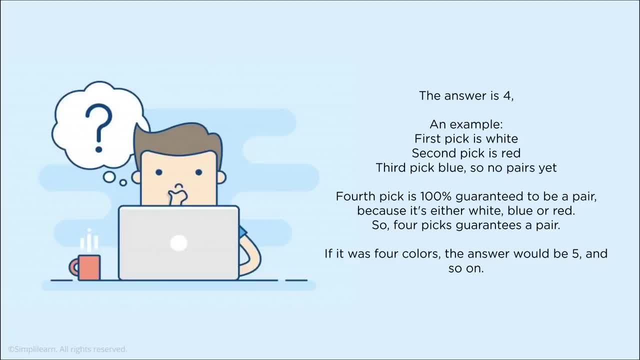 And that means when you get to the fourth pick, there's 100% chance you're going to have a match. So the most is going to be four that you ever have to pull out of your drawer. If it was four colors, the answer would be five, and so on. 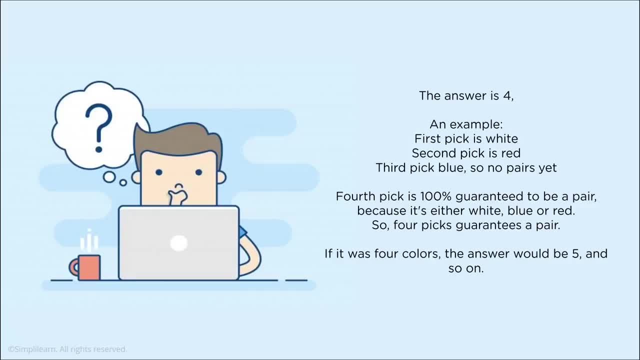 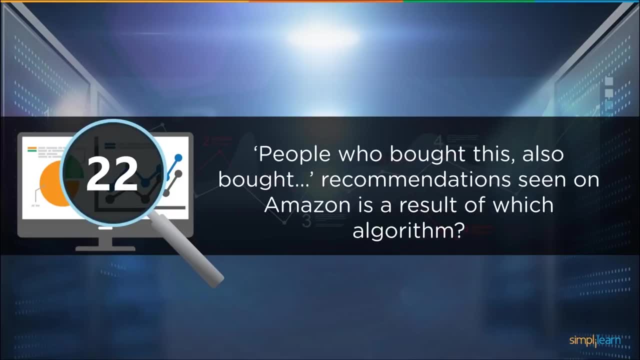 It doesn't matter how many white socks you have or how many red socks or blue socks- different pairs you have- It's the different colors, the number of different colors. People who bought this also bought recommendations seen on Amazon, as a result of which algorithm. 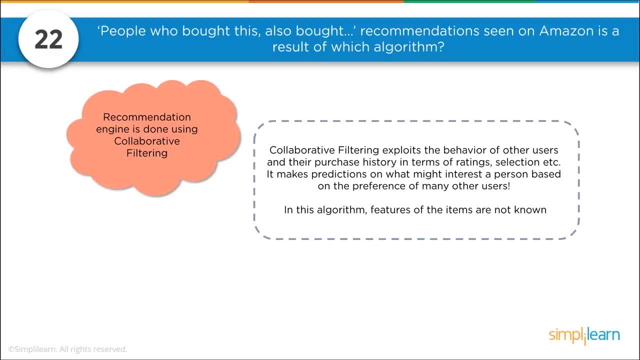 Ooh, we covered this earlier. Recommendation engine is done with collaborative filtering. Collaborative filtering exploits the behavior of other users and their purchase history in terms of ratings, Selection, et cetera. It makes predictions on what you might interest a person based. 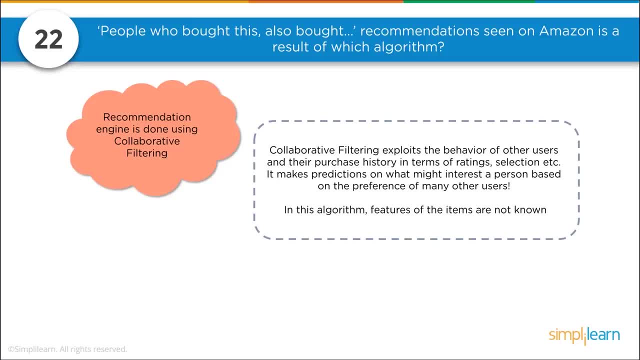 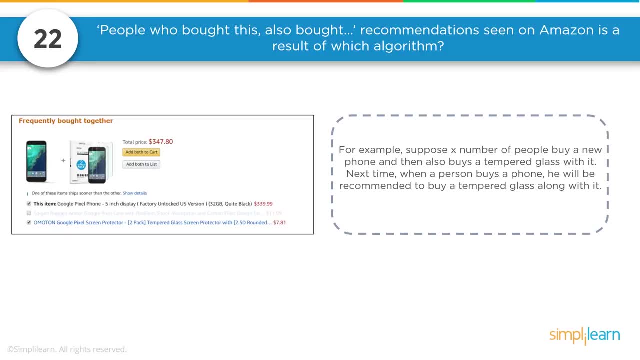 on the preference of many other users And this algorithm. features of the items are not known And we have a nice example here where they took a snapshot of a sales page. It says, for example: suppose X number of people buy a new phone. 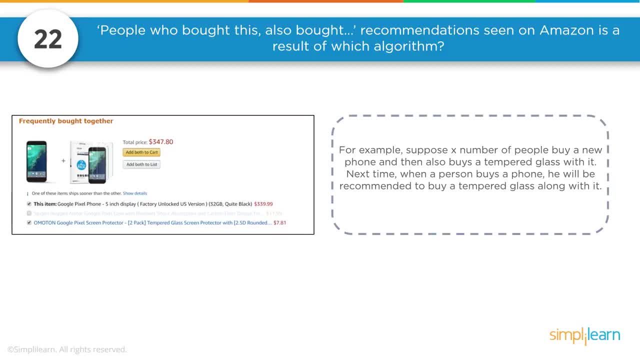 and then also buy tempered glass with it. Next time when a person buys a phone, he'll be recommended to buy tempered glass along with it, And if you remember the vocabulary words we covered earlier, this is the recommendation. This is collaborative. The other word was content based. 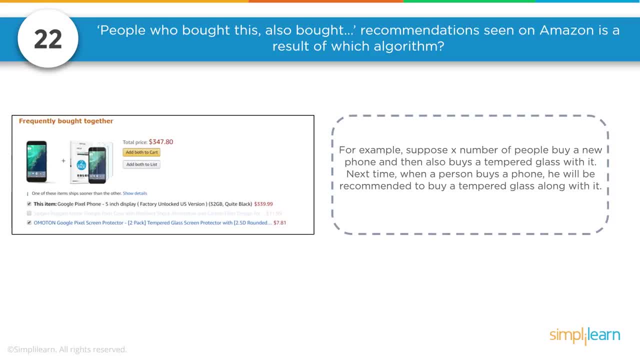 So, looking at things with similar content versus collaborative, which is similar people Remember. you know you're not going to know every vocabulary word, but it also doesn't hurt to get your three by five cards out and make yourself a vocabulary stack of cards. 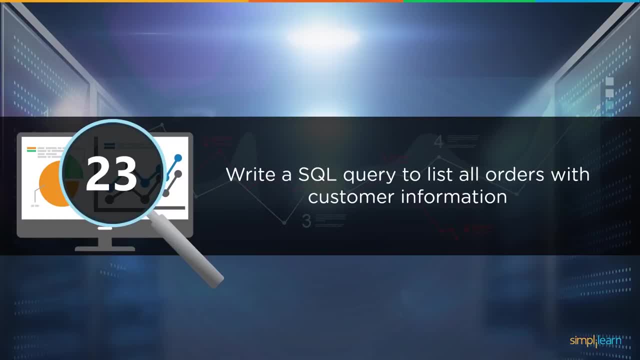 Buy an app on your phone for it SQL query. I remember back in the 90s it was so important to know SQL query and only a few people got it. Nowadays it's just part of your kit. You have to know some basic SQL. 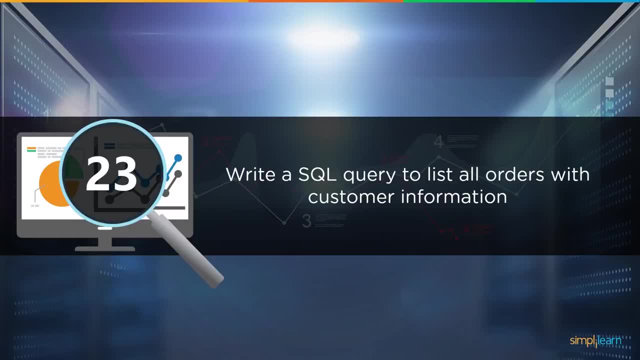 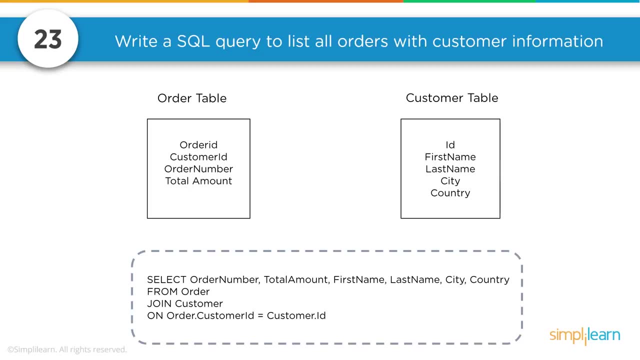 So write a basic SQL query to list all orders with customer information And you can kind of make up your own name for the database And you can pause it here if you want to write that down on a paper And let's go ahead and look at this. 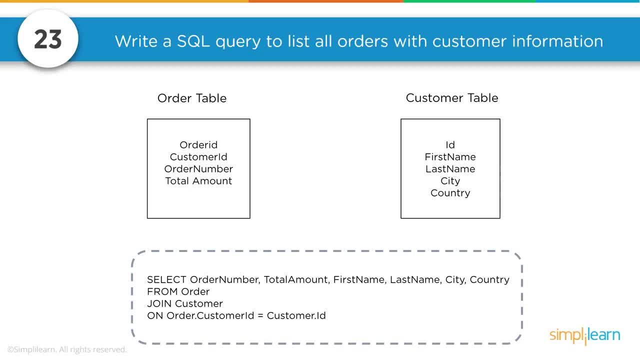 We have to list all orders with customer information, And so usually you have an order table and a customer table and you have an order ID, a customer ID, order number, total amount And then from your customer table you have ID. first name, last name, city, county. 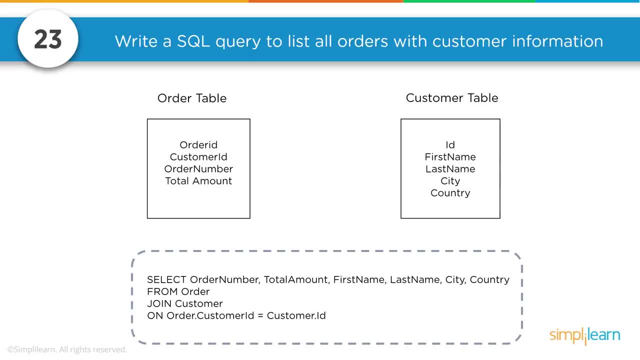 And so if we're going to write in SQL with this, we're going to select keyword there for SQL, selecting order: number, total amount, first name, last name, city, country. So that's the columns we're going to look at. 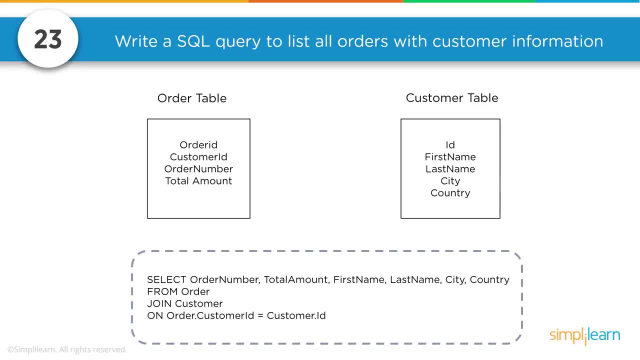 We're going to do that from our order, where we're going to join it with our customer, And we're going to join it on the order. customer ID equals the customer ID. So very basic SQL query that's going to return a table of data for us. 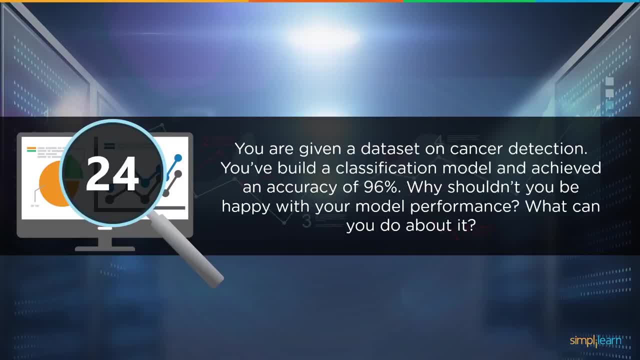 You are given a data set on cancer detection. You've built a classification model and achieved an accuracy of 96 percent- Whoo 96 percent. Why shouldn't you be happy with your model performance? What can you do about it? That's an interesting one, because this comes up. 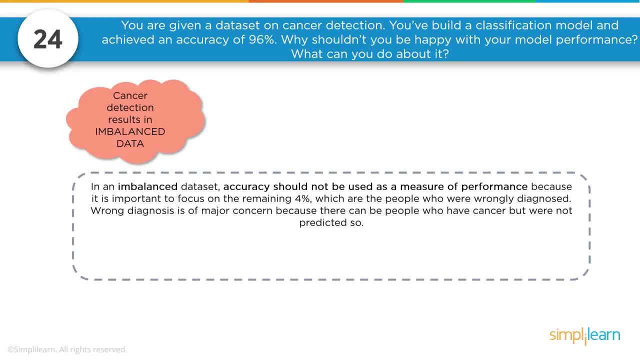 That's one of the standard data sets on there is for cancer detection. Cancer detection results in imbalanced data, In an imbalanced data set. accuracy should not be based as a measure of performance, because it is important to focus on the remaining 4 percent. 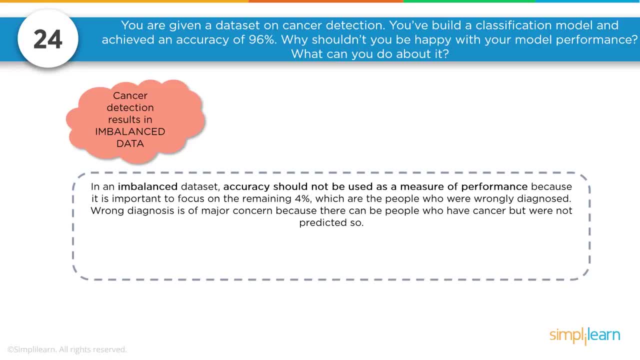 which are the people who were wrongly diagnosed? We talked a little bit about this earlier. You have to know your domain. You know this is the medical cancer domain versus weather domain. You know weather channel. they can get by with 50 percent wrong. 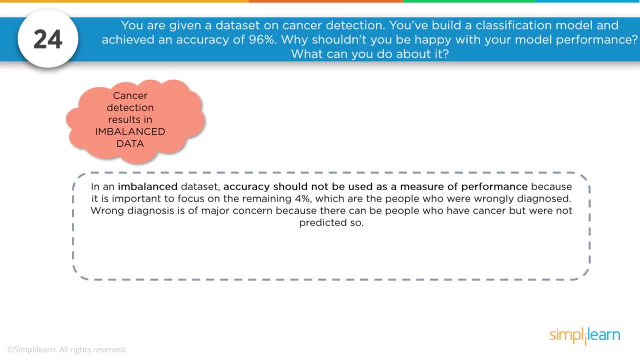 In cancer. you don't want 4 percent of the people being wrongly diagnosed. Wrong diagnosis is of a major concern because there can be people who have cancer but were not predicted. so In an imbalanced data set, accuracy should not be used as a measurement performance. 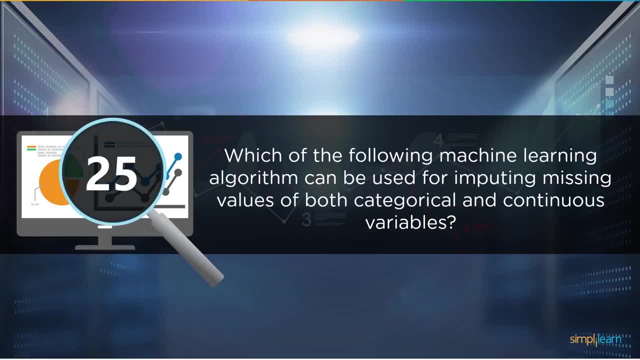 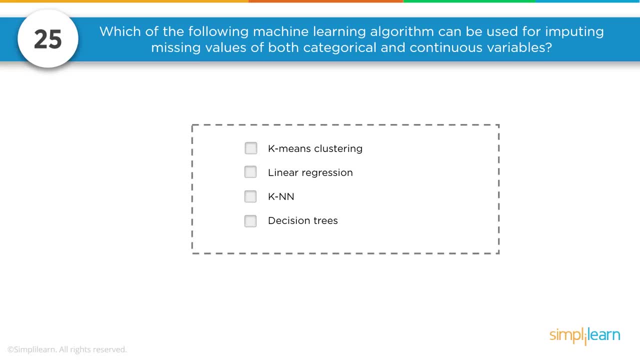 Which of the following machine learning algorithm can be used for inputting missing values of both categorical and continuous variables. And so we have a couple choices here. We have k-means clustering. We have linear regression. We have the k-NN- nearest neighbor. 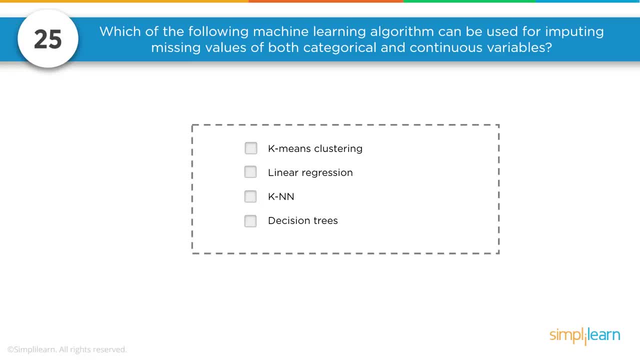 And decision tree, And which of the following machine learning algorithms can be used for inputting missing values of both categorical and continuous variables? Now, certainly you can use some preprocessing to do some of that, but you should have gone with the k-nearest neighbor. 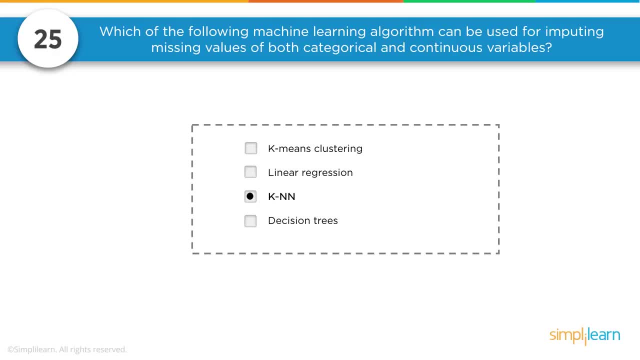 because it can compute the nearest neighbor and if it doesn't have the value, it just computes the nearest neighbor based on all the other features, where, when you're dealing with k-means, clustering or linear regression, you need to do that in your preprocessing. 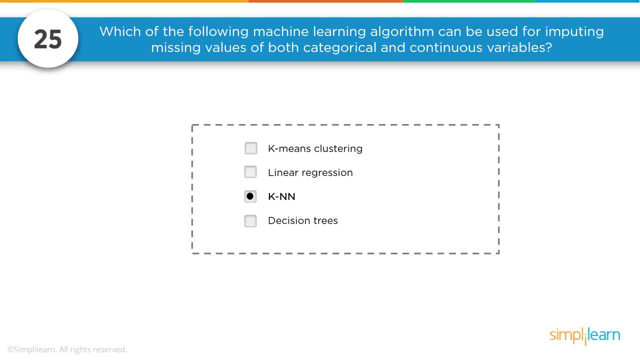 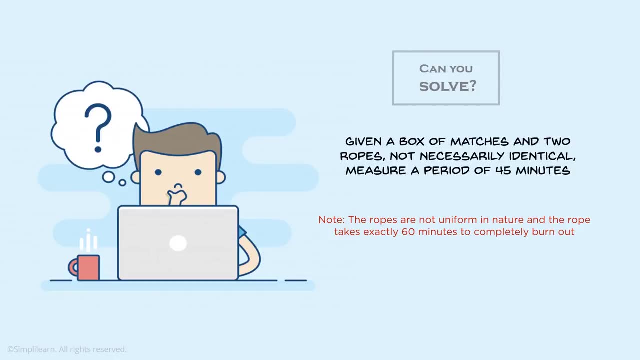 Otherwise it'll crash Decision trees also, although there's some variance on that too. Can you solve Another riddle- always fun ones- Given a box of matches and two ropes- not necessarily identical measure, a period of 45 minutes. 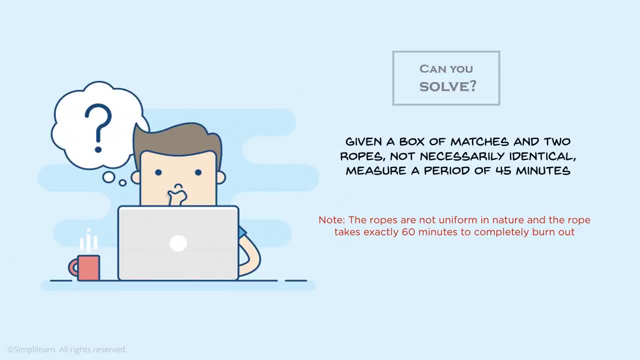 And in this particular setup the ropes are not uniform in nature and the rope takes exactly 60 minutes to completely burn out. So each rope takes up to 60 minutes to burn out, And there's actually a couple of different solutions to this. 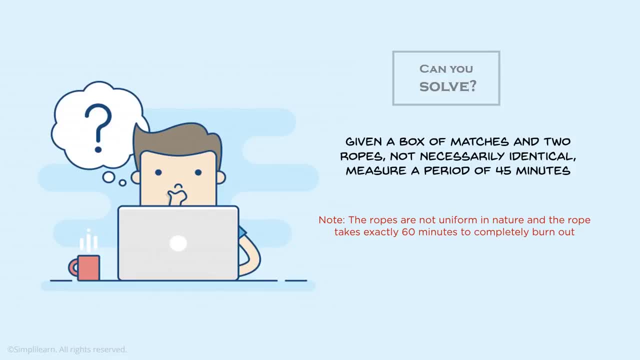 But let me go ahead, And one of the things is they're not uniform in nature, So even though they take 60 minutes anyways, let's go ahead and see what they did to solve it, And then we can also look at different options. 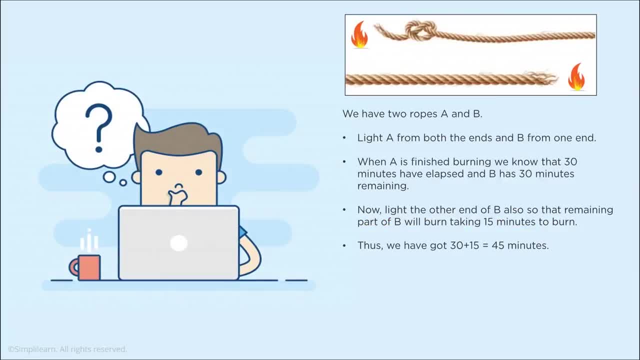 We have two ropes, A and B. Light A from both ends and B from one end. Okay, When A is finished burning, we know that 30 minutes have elapsed and B has 30 minutes remaining. Now light the other end of B also, so that the remaining part of B will burn. 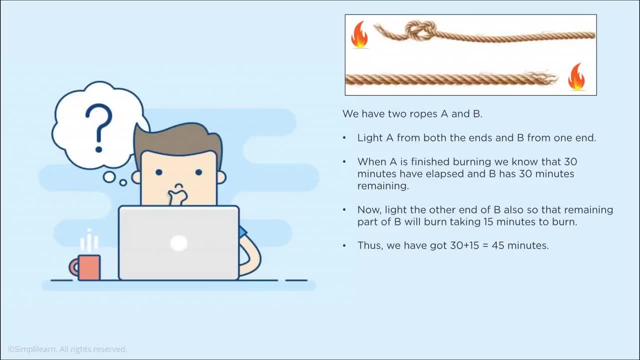 taking 15 minutes to burn This, we have gotten 30 plus 15 equals 45 minutes. Excellent solution. Mine, which I like, was to take one rope, fold it in two, So we know it's a half hour. Take the other rope, fold it in four places. 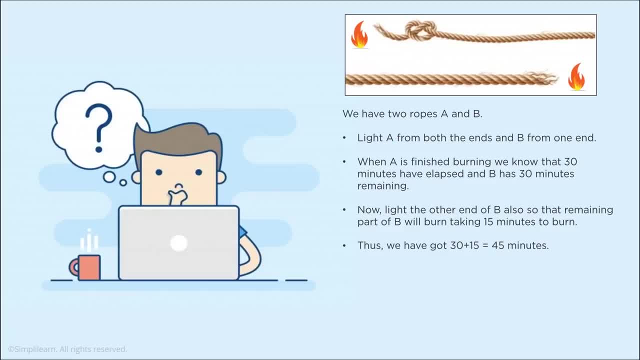 So we know that that one's 15 minutes And then you can just connect the two and burn it straight across. I think they're trying to cover that by saying they're not regular. The ropes have some irregularities. Maybe that's what they meant by that. 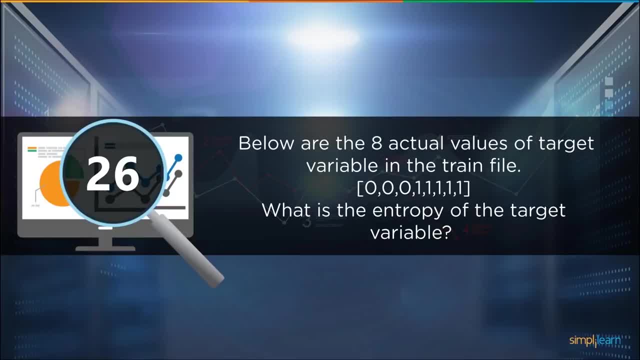 You couldn't do something like that. That's my solution. Below are the eight actual values of target variable in the train file. So we have a training file. Not to be confused with the train on the tracks We have 0, 0, 0, 1, 1, 1, 1, 1.. 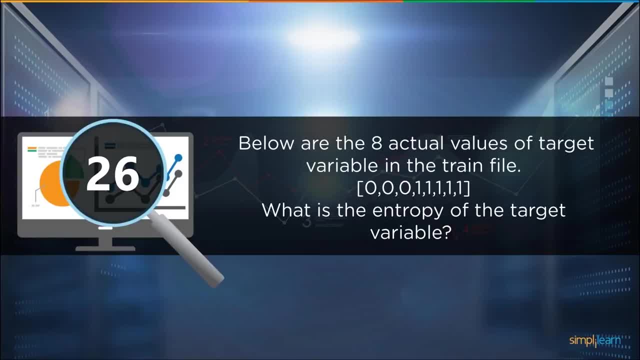 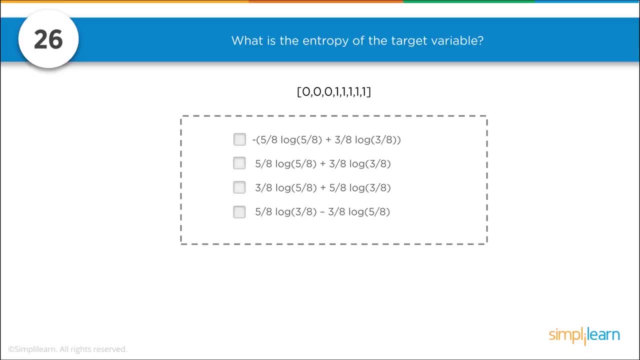 What is the entropy of the target variable? We mentioned earlier that you should know your entropy and how to calculate the entropy. What is the entropy of the target variable? So we have a couple of options here. We have minus 5 over 8. logarithm of 5 over 8. plus 3 over 8- logarithm of 3 over 8.. 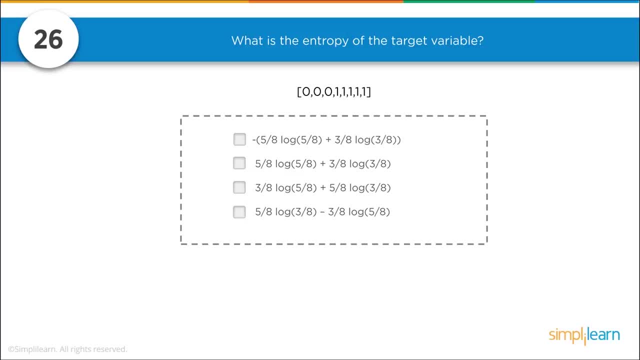 OK, let's just see where they got those numbers from. We have 1,, which is going to be 5 1s and 3 0s, And then we have a total of 8.. OK, and then we have the option of 5,, which is the number of 1s. 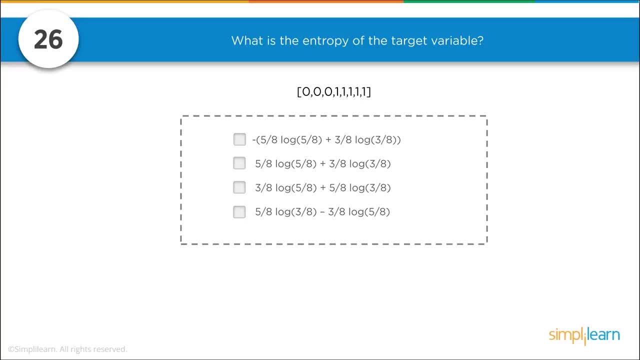 5: 8 logarithm of 5: 8s plus 3: 8s. logarithm of 3: 8s. And we also have 3: 8s logarithm of 5: 8s plus 5: 8s. logarithm of 3: 8s. 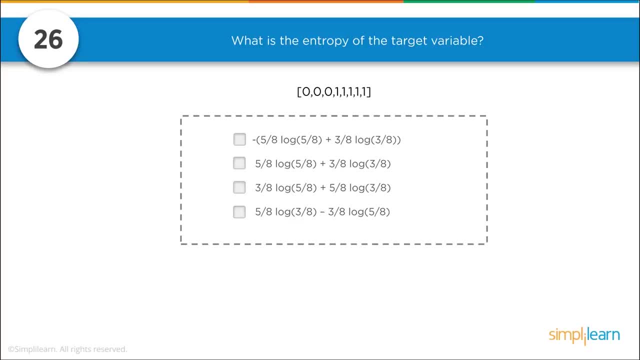 And then we kind of reverse those numbers around And let's see what you're going to get here. Which one did you think it was? You should check the first one. So what is the entropy of the target variable? The key there is a target variable. 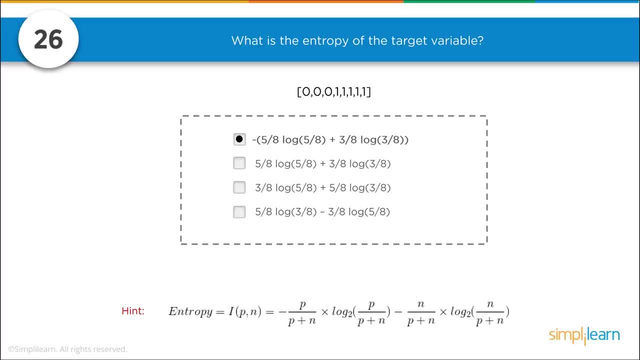 So we're looking at, the target in this case is going to be 1.. Usually that's what you're looking for, And so the entropy of that one we want to subtract out the entropy of the non-target variable. Whoops, I had that backwards. 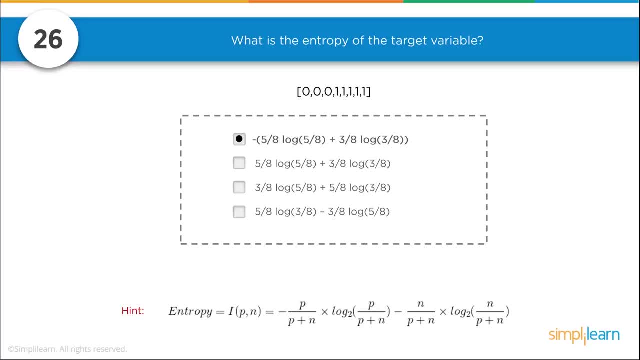 We're looking at 0, so we want to subtract out the 5- 8s from there. So 5- 8s logarithm 5 8s or negative 5 8s- logarithm 5 8s plus 3: 8s: logarithm 3 8s. 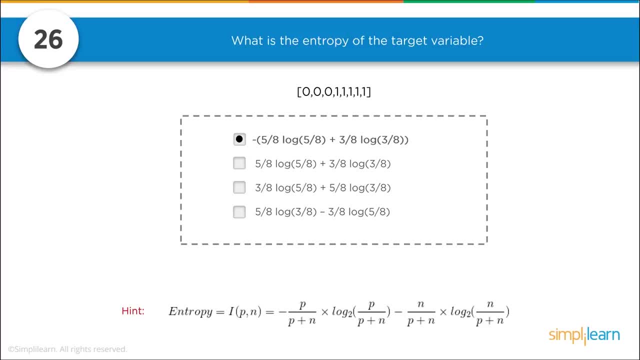 And they have a hint on the bottom. Entropy equals i of p of n. So we have a negative p plus p and n times the logarithm base 2 of p over p plus n, minus the n over p plus n times the logarithm 2 of n over p plus n. 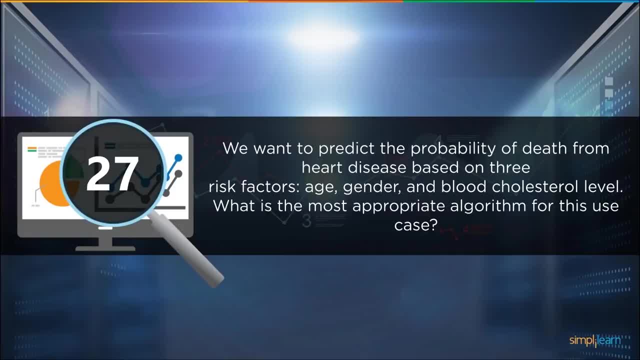 We want to predict the probability of death from heart disease based on three risk factors: Age, gender and blood cholesterol level. What is the most appropriate algorithm for this case? So we have three features and we want to know the predictability of death. 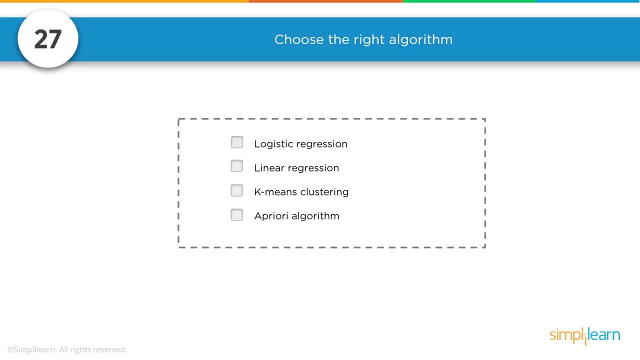 OK, a little morbid there. Choose the right algorithm. Do we want to use logistic regression for this? Linear regression, k-means clustering or the aproria algorithm, And if you selected logistic regression, then you probably got the right answer. 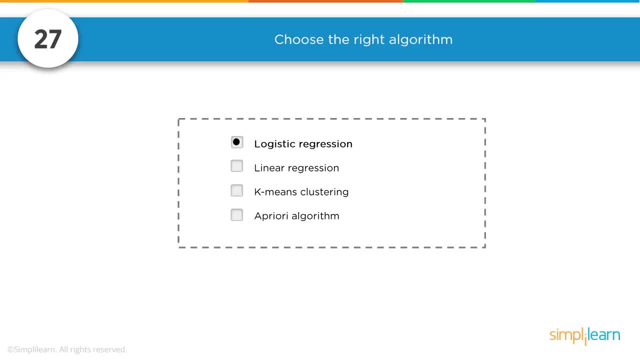 Linear regression, remember- deals with like you take your line and draw a line through the data, and of course you don't necessarily have to use a straight line. There's other means for that, but you're dealing with a lot of numbers And k-means means we're just going to cluster objects together. 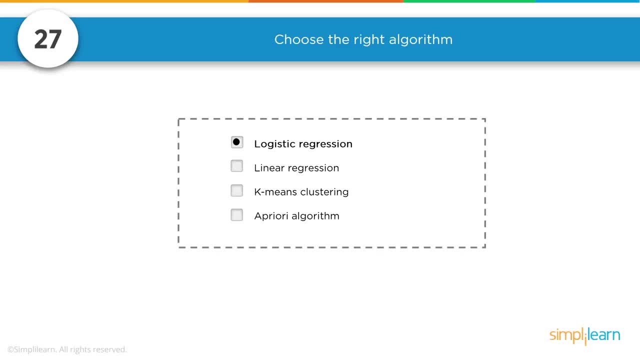 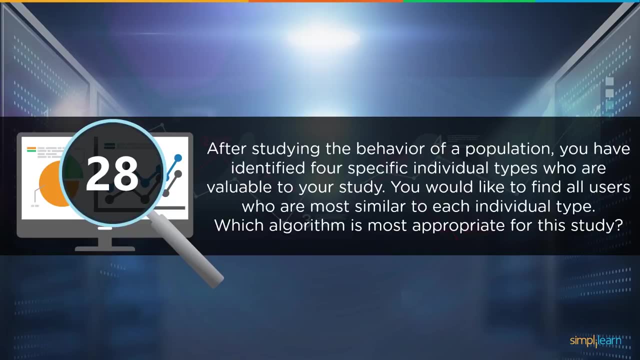 With the logistic regression, though you can mix those things together in buckets, So really the logistic regression is what you want to use in that model would be the most apt fit. After studying the behavior of a population, you have identified four specific individual types who are valuable to your 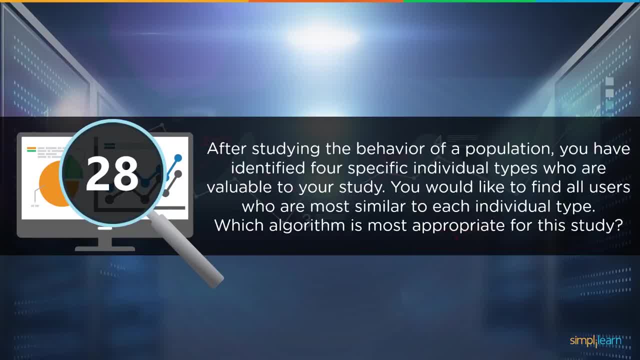 study You would like to find all users who are most similar to each individual type. Which algorithm is most appropriate for this study? Certainly, identifying census in just about a lot of different markets is common, So maybe they have a census or whatever it means. 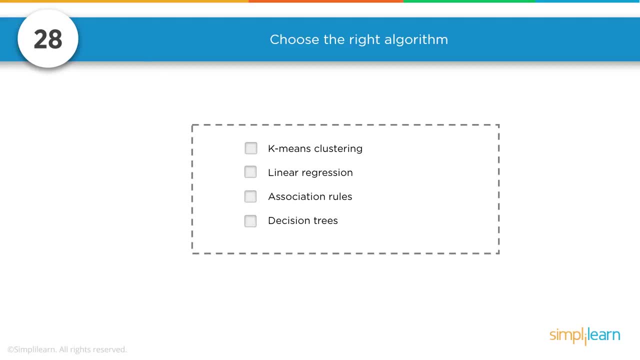 But let's take a look at some of the different algorithms we might use on this. We have k-means, clustering, linear regression, association rules and decision trees, And I'll give you a hint: We're looking for grouping people together by similarities. 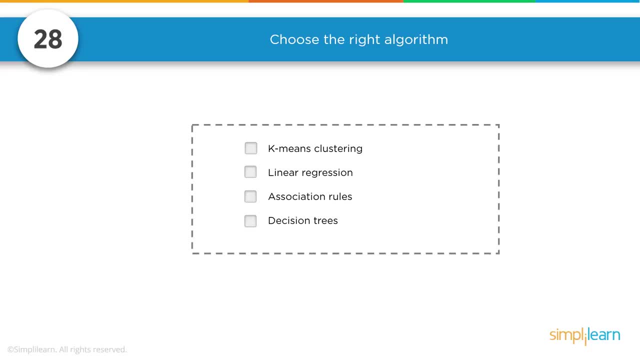 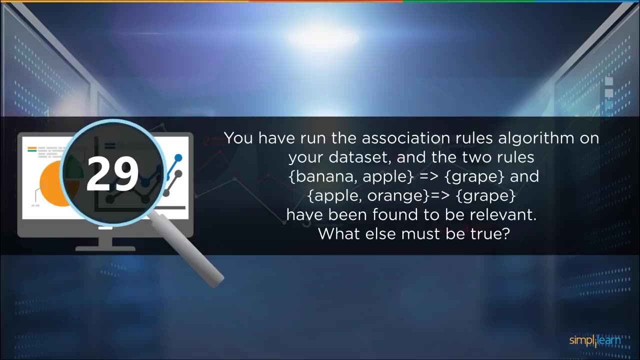 And by four different similarities, so very specific. They gave you one of the values, specifically the k value, So k-means clustering would be great for this particular problem. You have run the association rules algorithm on your data set and the two rules- banana apple is associated with grape and apple orange is associated. 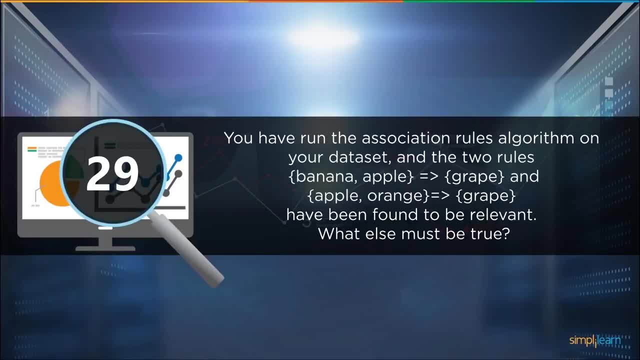 with grape have been found to be relevant. What else must be true? So this would challenge you to understand association rules. You could picture in this particular one. you're going shopping and you almost always see somebody who has bananas. They usually have grapes in their bag also. 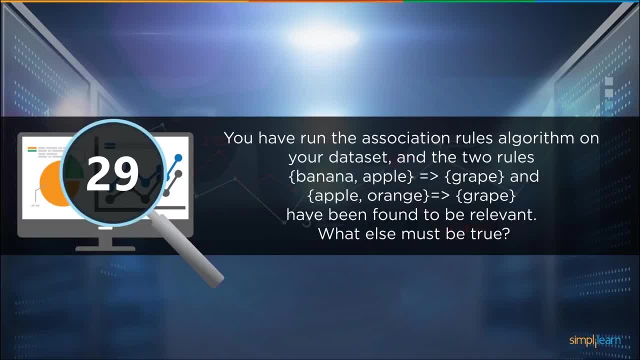 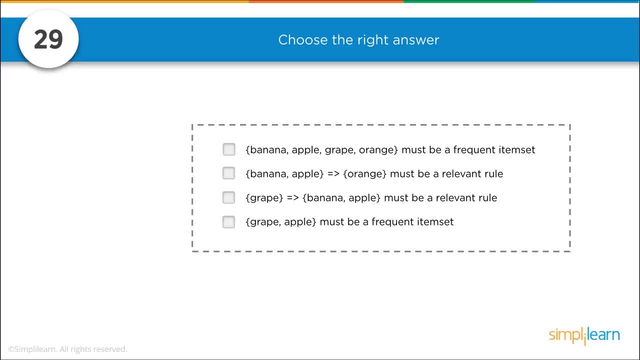 And somebody who has apples usually has grapes in their bags, and then apples and oranges is also associated with grapes, And let's go and take a look at that. And we have a couple of different options here. First one is banana, apple and grape. 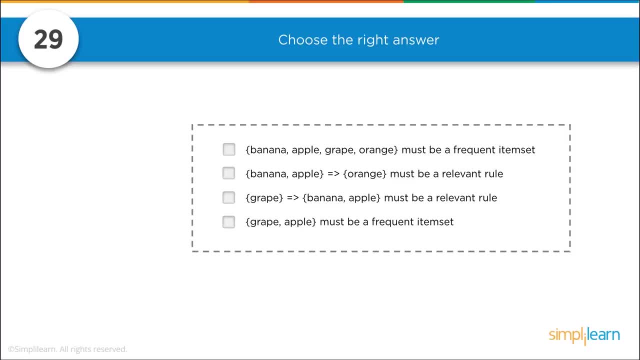 Orange must be a frequent item set, Not so much Banana apples. Oranges must be relevant rule. Grape is common with banana. Apple must be a relevant rule. And how about grape Apple must be a frequent item set. Let's go back and take a look at that. 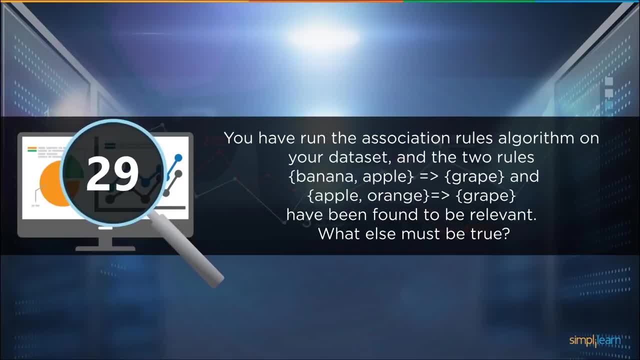 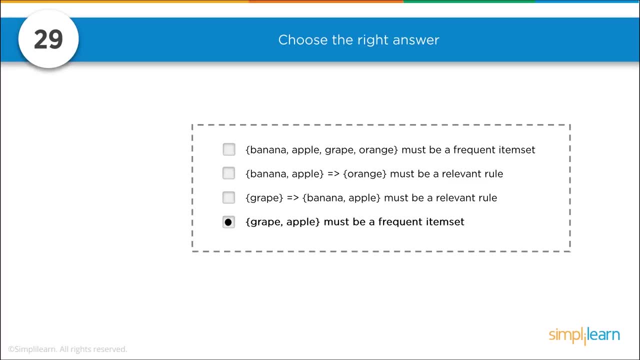 And we notice that we have bananas, apples to grapes, We have apple orange to grape Boy. there's a lot of grapes and a lot of apples in there, And so, if you said the last one, grape and apple must be a frequent item set. 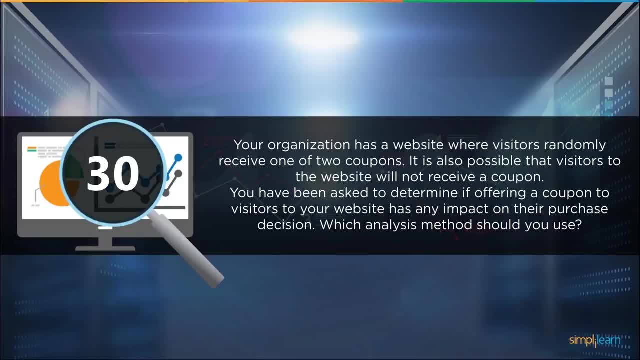 Then you got it correct. Your organization has a website where visitors randomly receive one of two coupons. It is also possible that visitors to the website will not receive a coupon. You have been asked to determine if offering a coupon to visitors to your website has any impact on their. 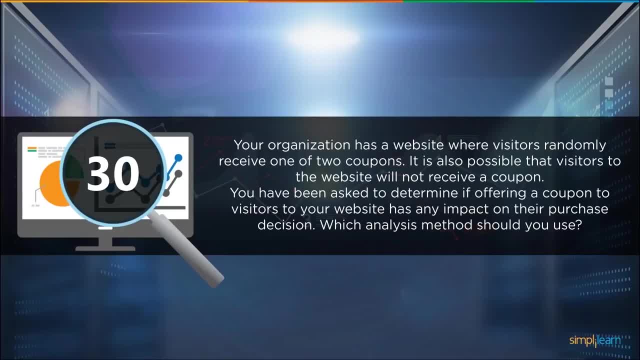 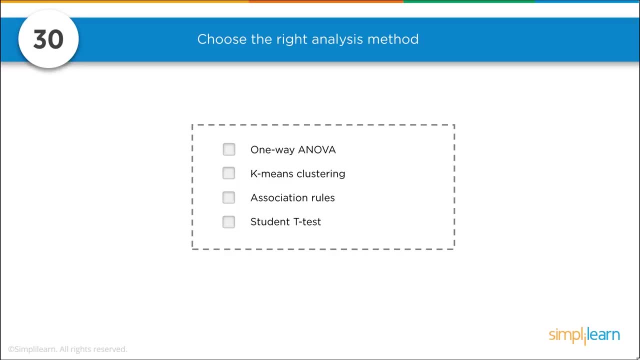 purchase decision. Which analysis method should you use? And so let's go ahead and start by giving you another hint and give you some limiting your selection. We have a one way ANOVA, K-means, clustering, association rules and student T-test. 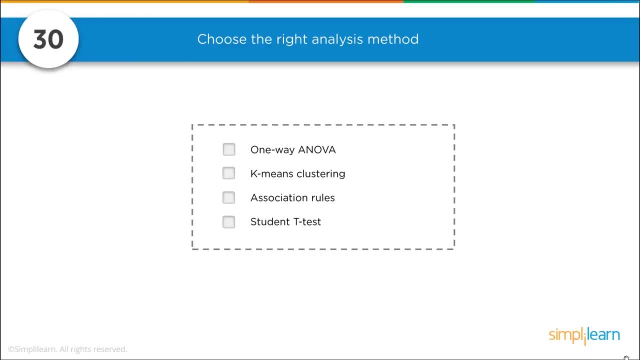 So obviously you should know what each one of these means. But let's take a look at the question again. So you want to know which method should you use to see if the coupon's valid for their purchase? Well, we're not clustering and we're not associating things together.